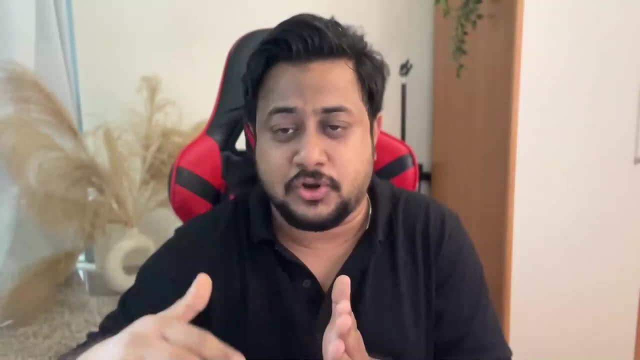 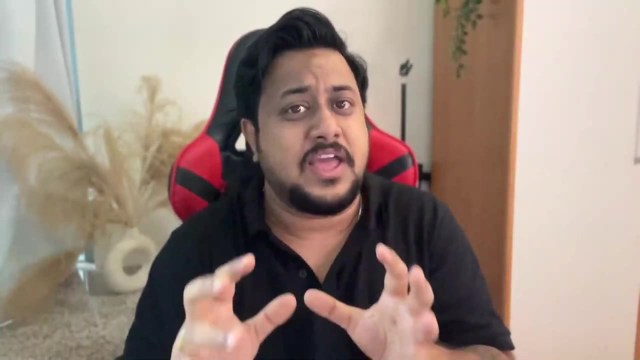 is one of the stepping stones towards your next targets or your next goals. Without EDA, you cannot really go ahead with your next steps. So understanding EDA is very, very important. and EDA is not just about performing univariate, bivariate or multivariate analysis. EDA is way. 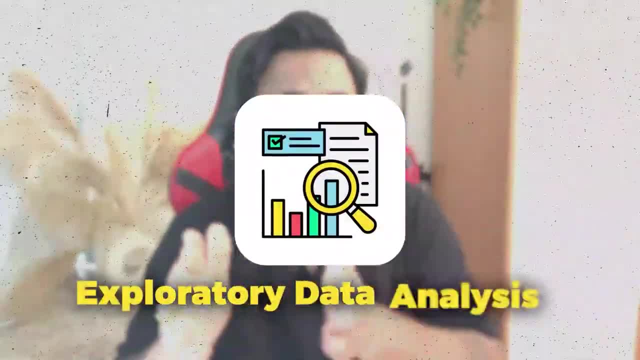 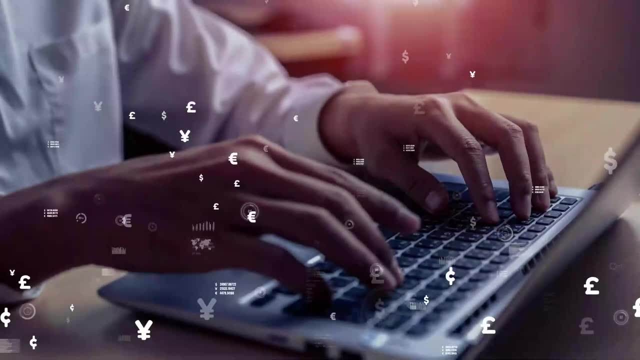 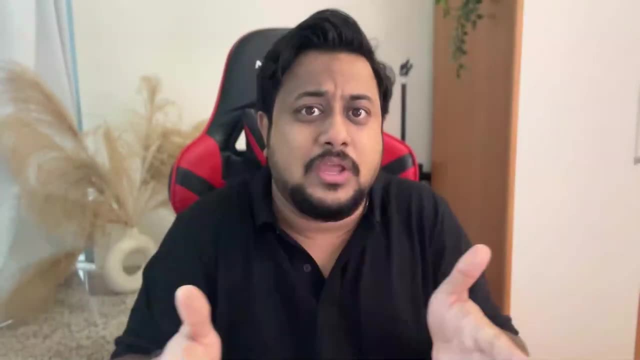 beyond that, As the name suggests, exploratory data analysis is one of the most important skills, where we actually indulge with the business stakeholders or even the clients, to get the data, understand the data, what the data is telling us, and then inside gathering While doing all these. 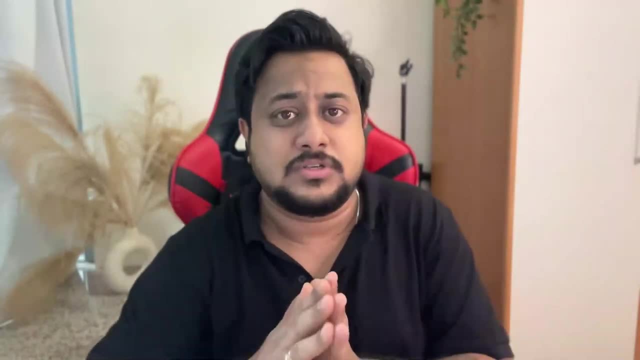 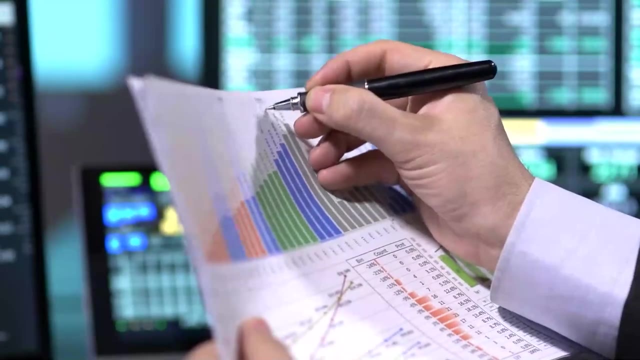 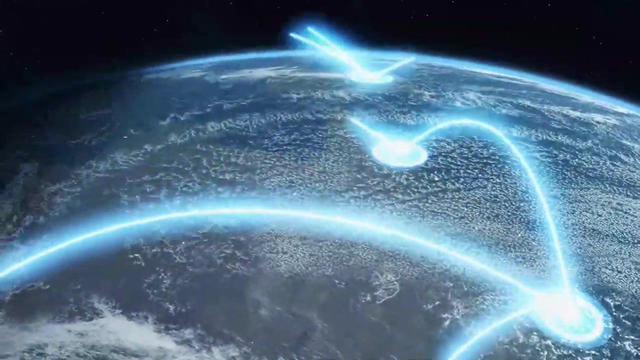 steps. there are multiple things that we perform. that includes data cleaning, data transformations, data preparation, outlet treatments, understanding whether data is following a normal distribution or not, and, way beyond that, feature encoding, feature scaling. lot more things comes into ada, so it is just not doing univariate, bivariate or multivariate analysis. now talking about where 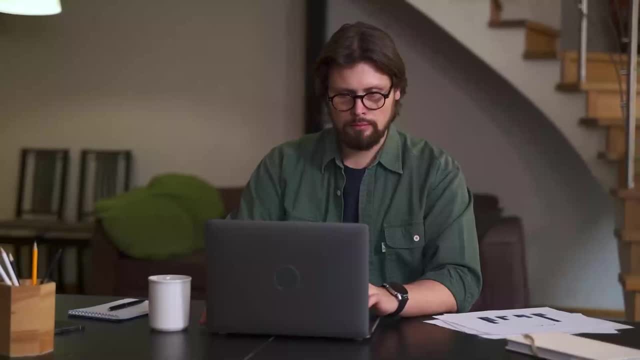 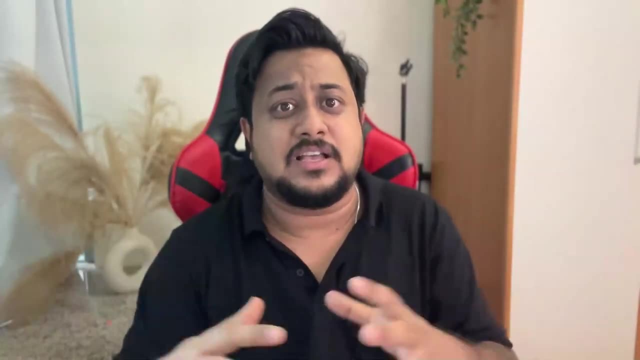 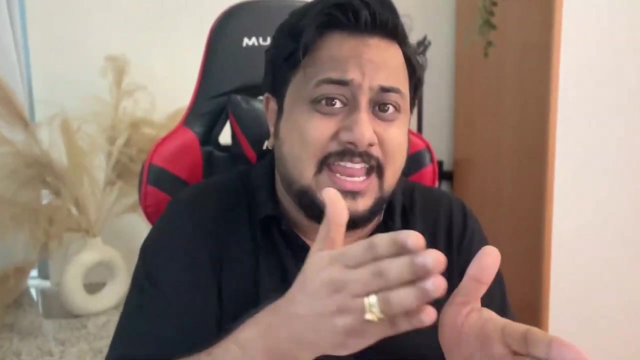 do we learn ada? there are multiple videos, multiple blogs where you can go through and understand ada, but what you will not find on the internet freely is a structured program. now, in this video, we are going to talk about ada, and we are also going to talk about each and everything about ada. this: 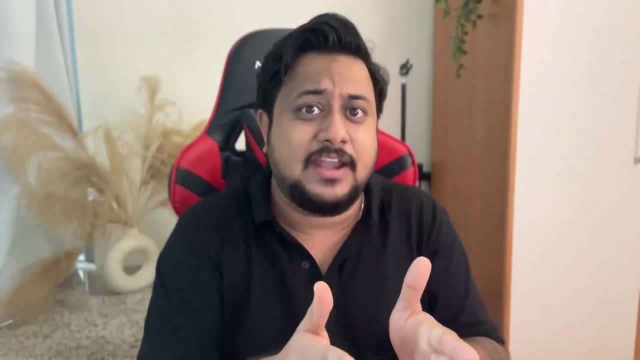 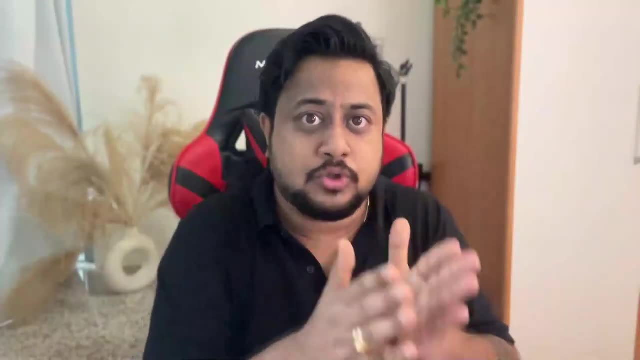 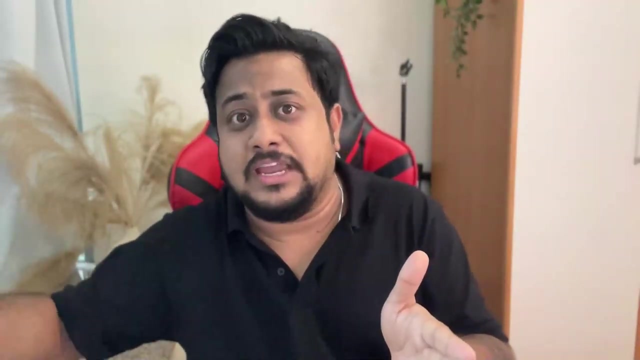 video is going to be a long video because we have divided the entire scope of ada in multiple short videos. so go through this particular course, go through this particular video and i'm pretty much sure you will be able to understand each and everything of the data. so let's get started now. what's next after going through this video is you have to. 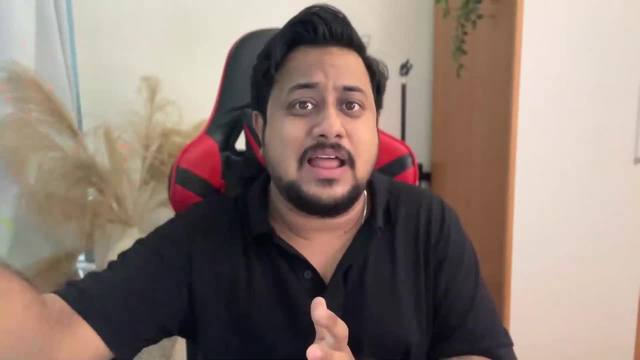 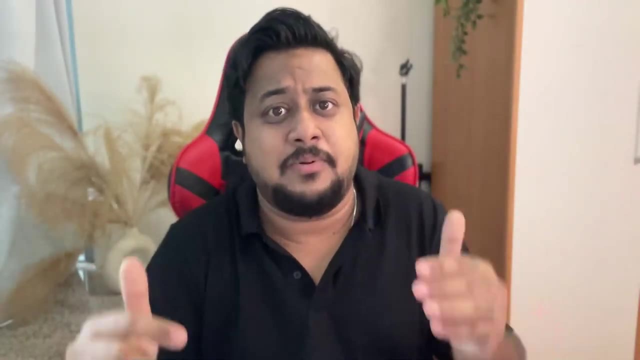 pick a use case and start performing ed now to get an idea on your portfolio projects around ada. there are many videos on my channel. in case you still need any help, let me know in the comment section below on which area you want to perform ad and i can guide you accordingly. so let's get. 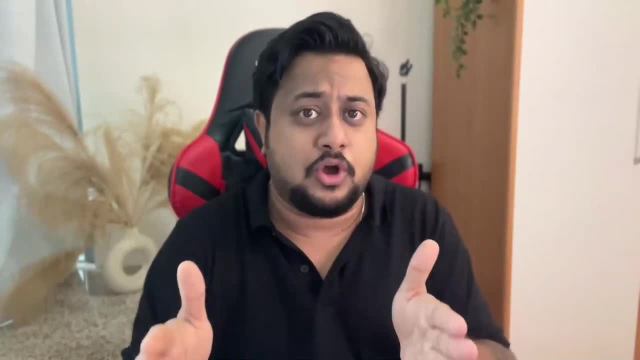 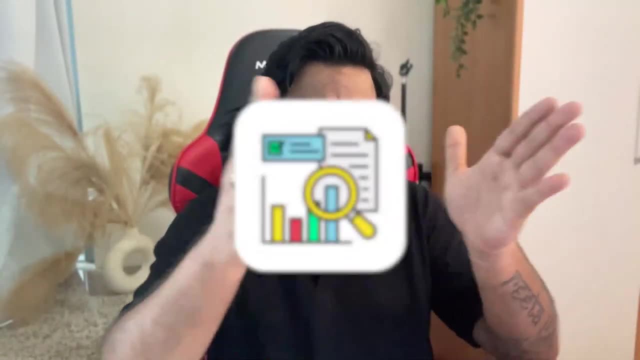 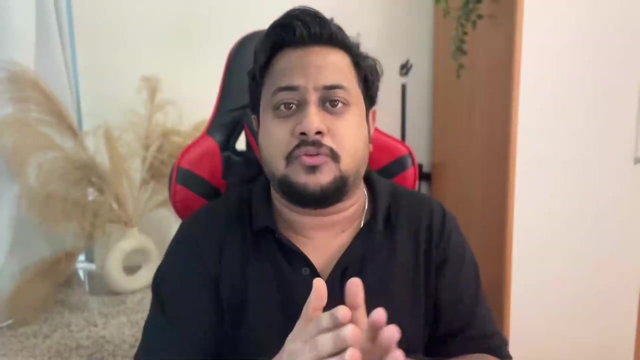 we are going to talk about EDA and we are also going to talk about each and everything about EDA. This video is going to be a long video because we have divided the entire scope of EDA in multiple short videos. So go through this particular course, go through this particular video and 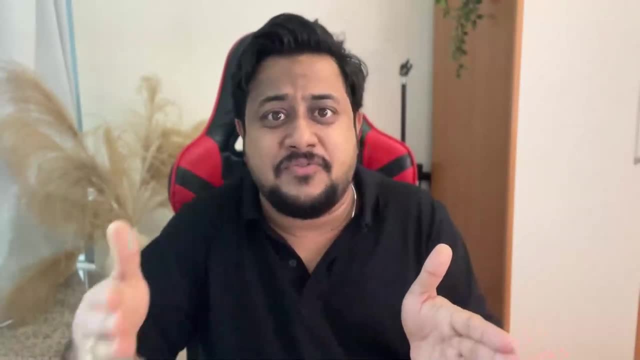 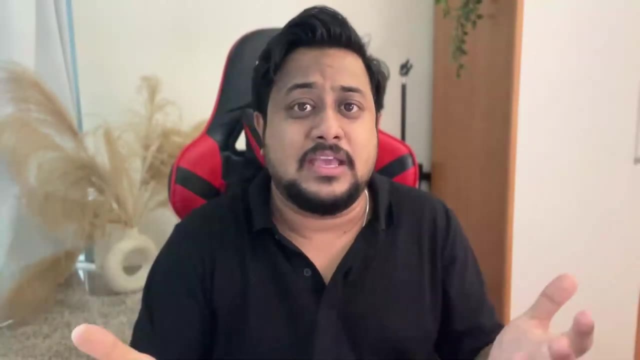 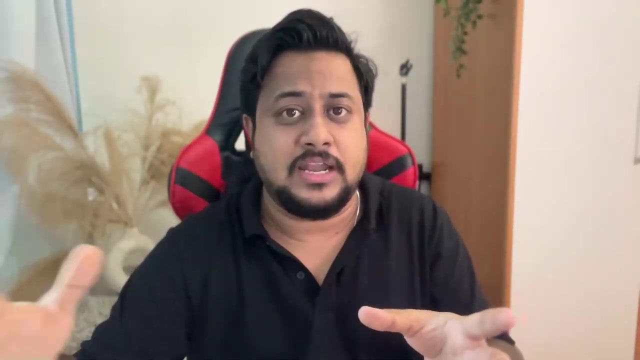 I'm pretty much sure you will be able to understand each and everything while we do the EDA process. Of course, what's next after going through this video is you have to pick a use case and start performing EDA Now to get an idea on your portfolio projects around EDA. there are many. 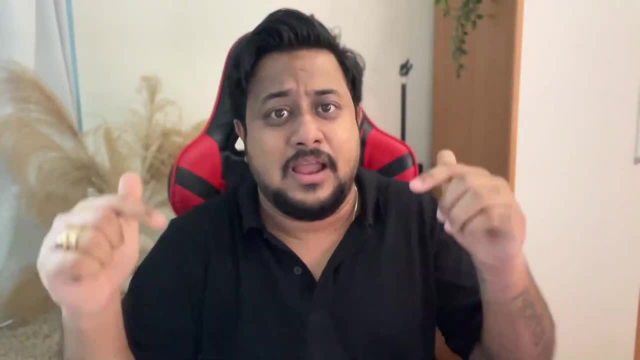 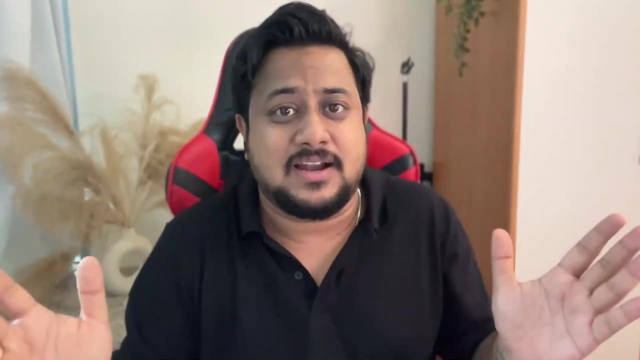 videos on my channel. In case you still need any help, let me know in the comment section below on which area you want to perform EDA and I can guide you accordingly. So let's get started. I wish you all the best. if you are in your data analytics journey, This video is definitely going. 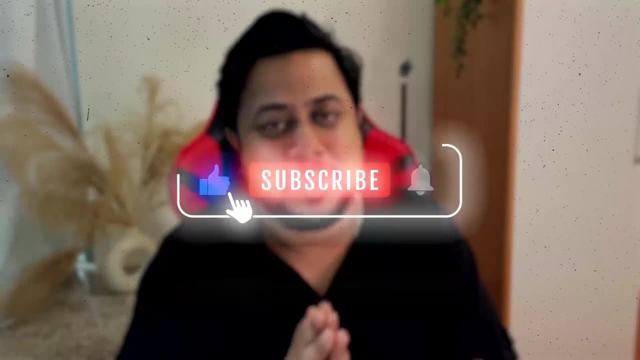 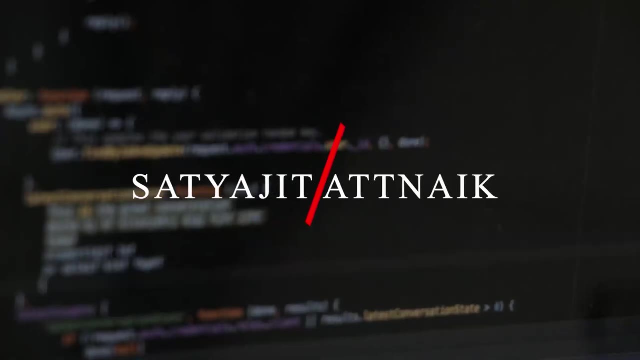 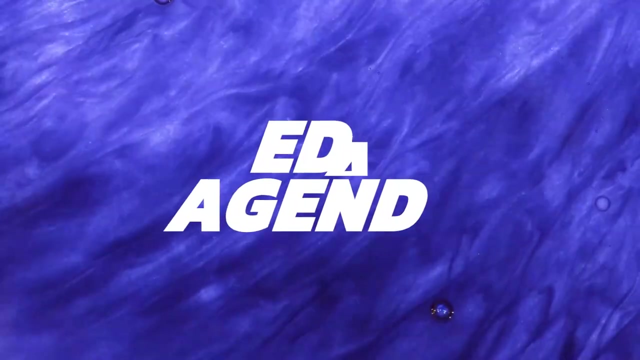 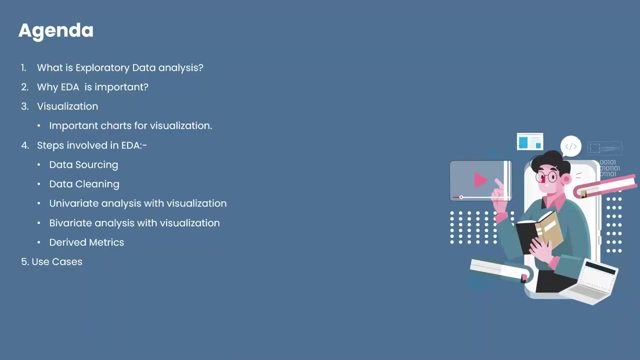 to be very much helpful for you. I will see you in the next video. Bye, bye, Hi. welcome to this module on exploratory data analysis. We all know when it comes to solving a data analytics or a data science problem, it all starts with the business. 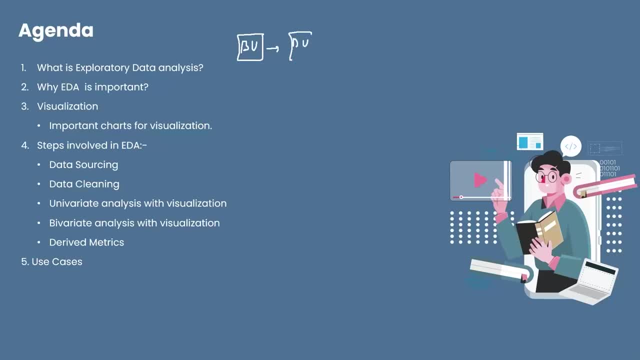 So let's first understand the business understanding part, Then comes our data understanding, Then comes our data collection, data preparation. These are one of the most important steps that we all know in the field of data analytics Before getting into the actual analysis process. first of all, we need to understand the business problem, Then the 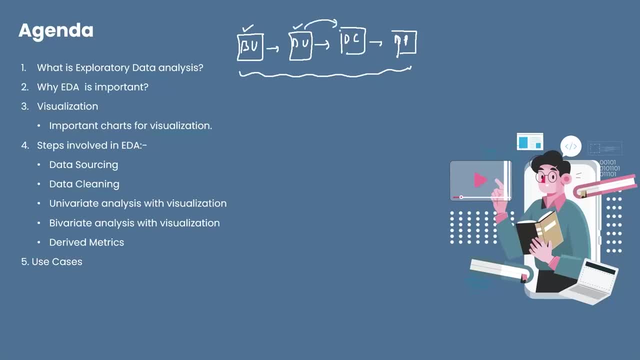 data understanding is must and then only we get started with our data collection part. Data preparation is again one of the steps where we prepare the data, We take unclean data and finally clean the data. The output of the data cleaning and the data preparation part is the clean data, And that's where EDA comes into picture. 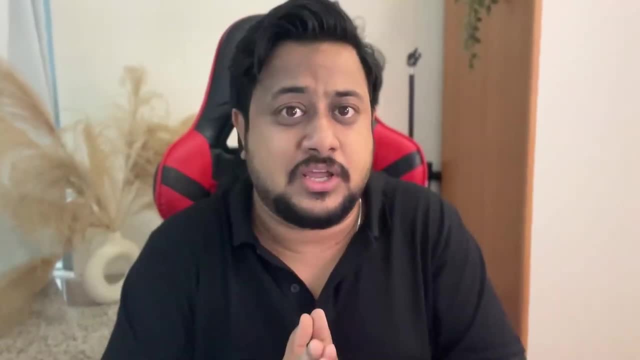 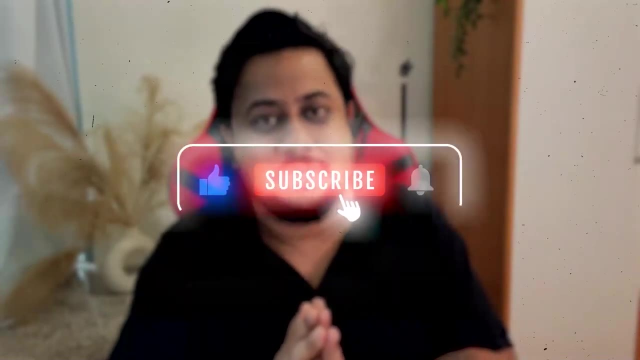 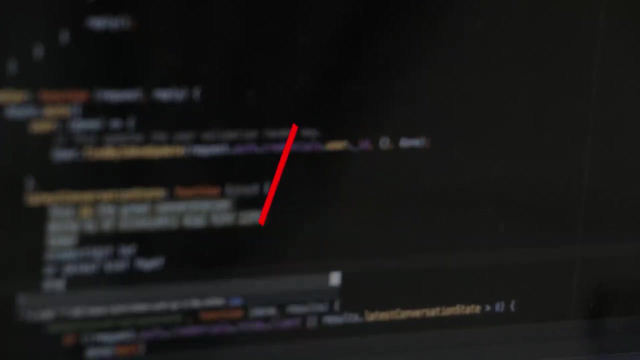 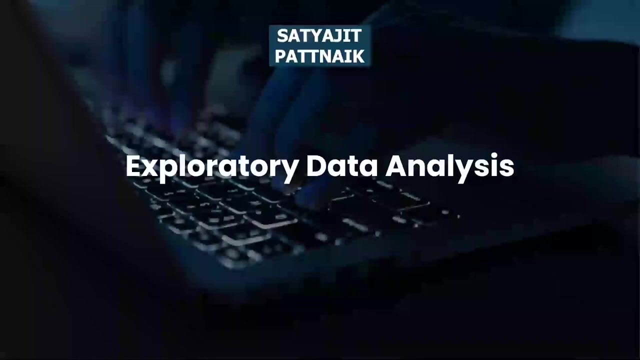 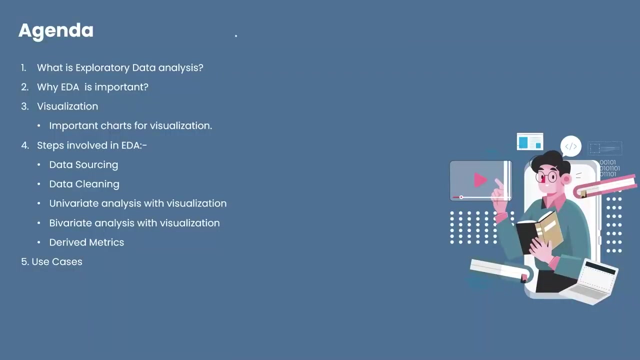 started. i wish you all the best. if you are in your data analytics journey, this video is definitely very much helpful. don't forget to like, share and subscribe the channel. see you in the video. hi, welcome to this module on exploratory data analysis. we all know when it comes to solving a data analytics or a data science problem, 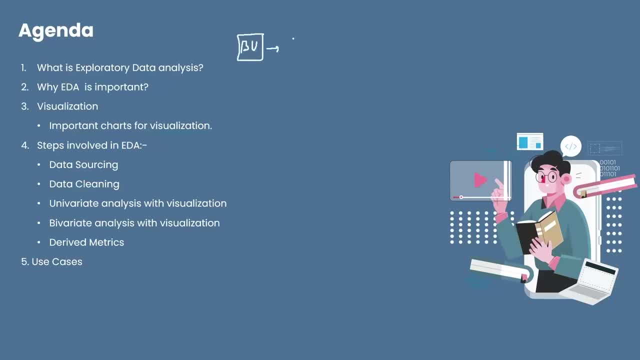 it all starts with the business understanding part, then comes our data understanding, then comes our data collection, data preparation. these are one of the most important steps that we all know in the field of data analytics. before getting into the actual analysis process, first of all we need to understand the business problem, then the data understanding is must and 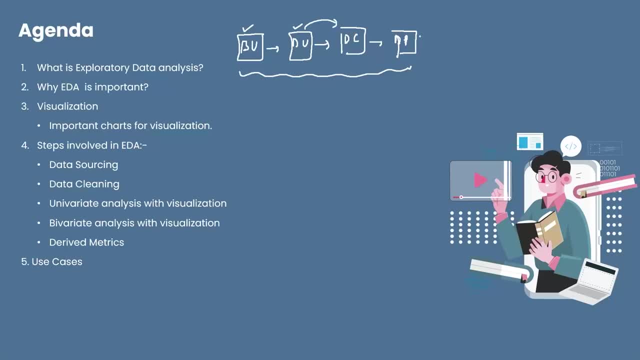 then only we get started with our data collection part. data preparation is again one of the steps where we prepare the data, we take unclean data and finally clean the data. the output of the data cleaning and the data preparation part is the clean data, and that's where eda comes into picture. 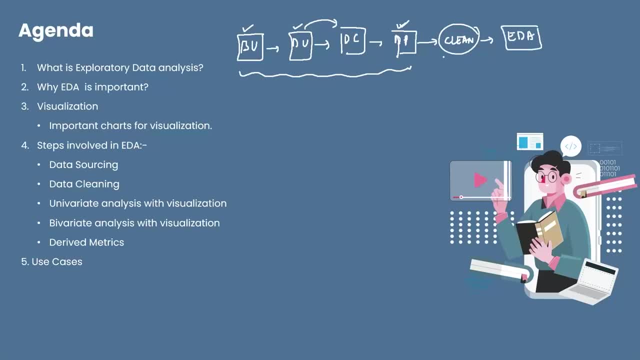 so eda expects that the data is cleaned so that it helps us in analyzing the data, and the output of eda are all insights. whatever the data is trying to tell us, eda is by far one of the most important fields, one of the most important areas, one of the most important. 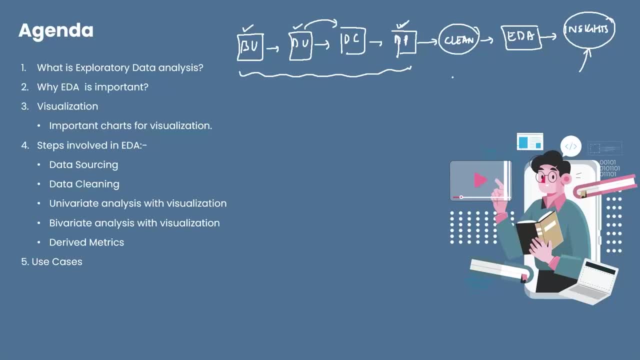 modules. when it comes to the data analysis part, talking about eda- in this particular module, we will be learning what is exploratory data analysis, why eda is important to us, what is the power of visual analytics or, in simple terms, visualization. we will also be talking about some of the important charts for visualization. 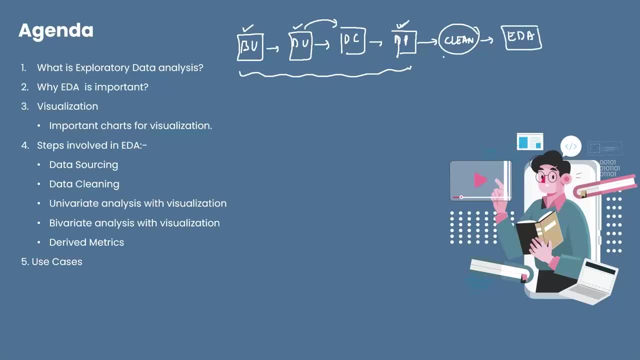 So EDA expects that the data is cleaned so that it helps us in analyzing the data, And the output of are all insights. whatever the data is trying to tell us, eda is by far one of the most important fields, one of the most important areas, one of the most important modules when it comes. 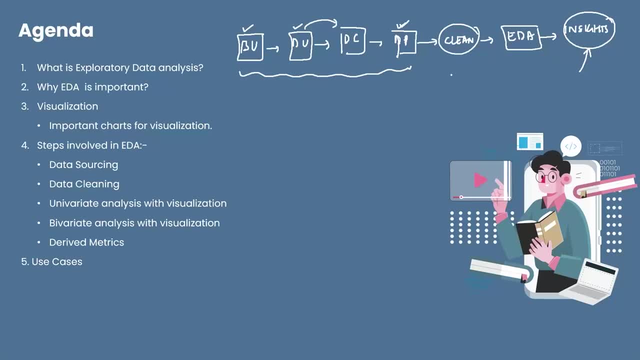 to the data analysis part, talking about eda. in this particular module, we will be learning what is exploratory data analysis, why eda is important to us, what is the power of visual analytics or, in simple terms, visualization. we will also be talking about some of the 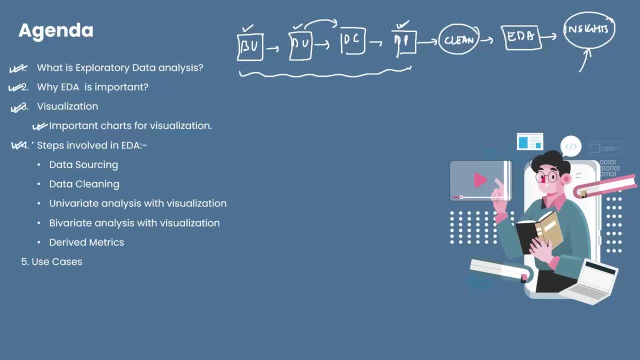 important charts for visualization. what are the different steps involved in eda, starting with data sourcing, cleaning some univariate, bivariate analysis, which is basically your categorical data analysis, and we will also talk about some numerical data analysis, and then we will talk about derived metrics after we go through each and every topic. finally, we will be talking about some of the use cases. 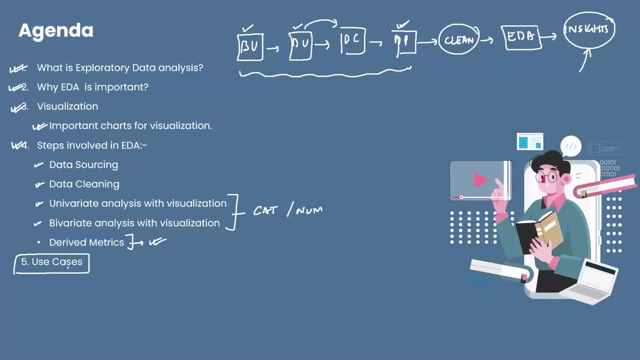 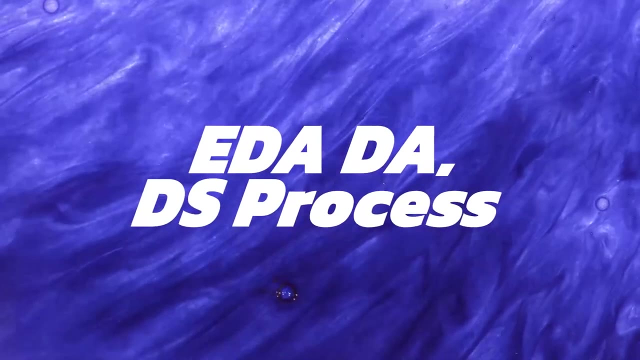 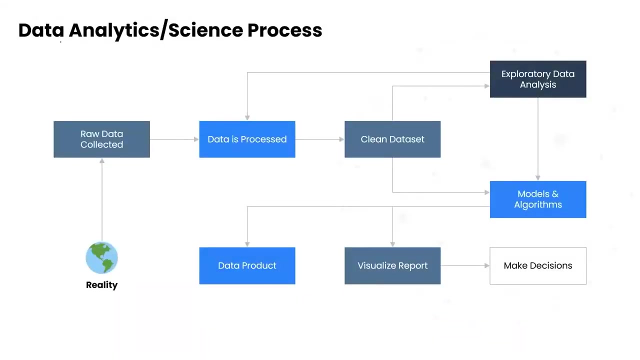 that are applicable for eda. and, lastly, we will be going through one of the use cases and we will be explaining you how to perform eda for that particular use case using python. how do you deal with data analytics? hi, in this video we shall be talking about the data analytics or science process. now this: 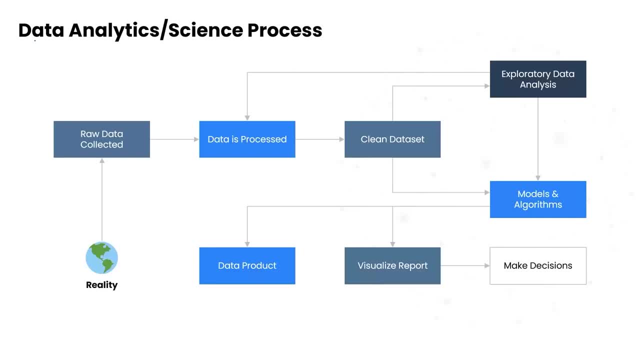 this particular flow chart will give you a better understanding on how exactly things works. generally speaking, we already know it's all about business understanding, then data understanding, then data collection, preparation, ed and model building, but in some the cases that does not give you the right picture. this particular flowchart is more close to how to 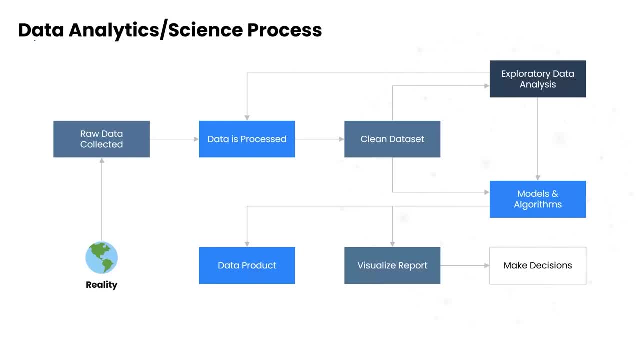 solve an actual problem statement: how to solve an actual problem in a real world scenario. now there are multiple things we need to discuss in this particular flowchart. i am pretty much sure that by the end of this video, you will have a better understanding on what exactly is eda. 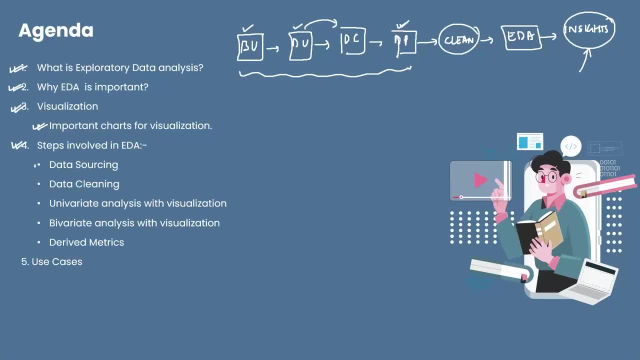 what are the different steps involved in eda, starting with data sourcing, cleaning, some univariate, bivariate analysis, which is basically your categorical data analysis, and we will also talk about some numerical data analysis, and then we will talk about derived metrics after we go through each and every topic. finally, we will be talking about some of the use. 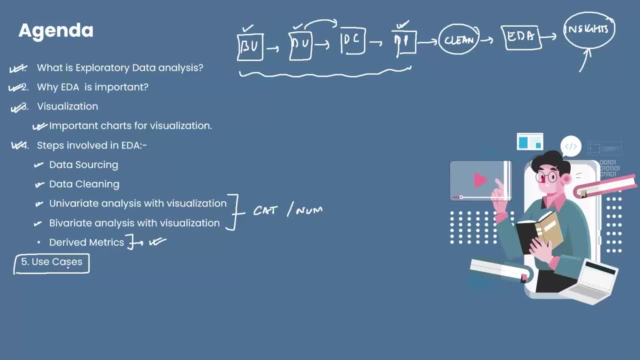 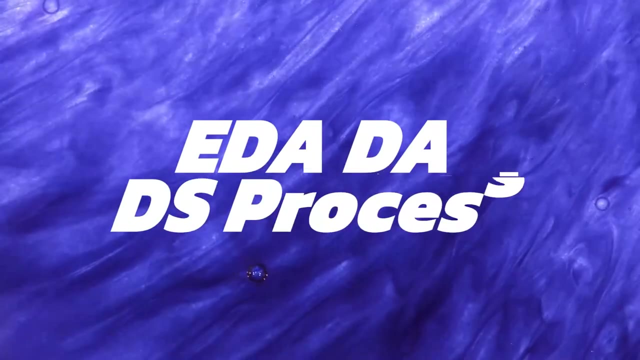 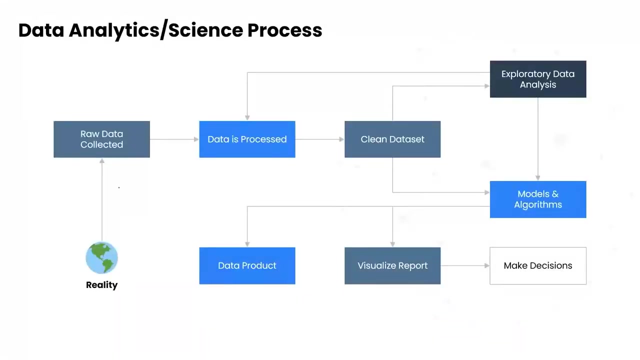 cases that are applicable for eda. and, lastly, we will be going through one of the use cases and we will be explaining you how to perform eda for that particular use case using python. so let's get started. hi, in this video we shall be talking about the data analytics, or science. 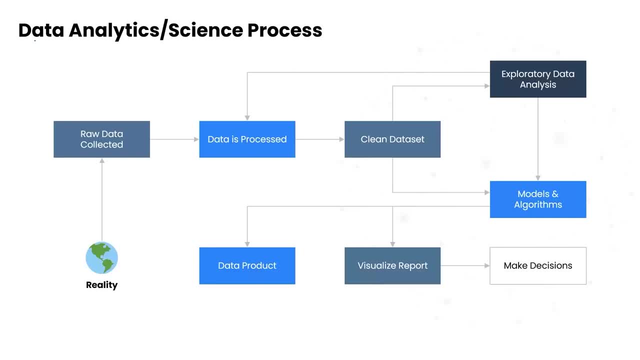 process. now this, this particular flow chart, will give you a better understanding on how exactly things works. speaking we already know, it's all about business understanding, then data understanding, then data collection, preparation, eta and module building, but in some of the cases that does not give you the right picture. 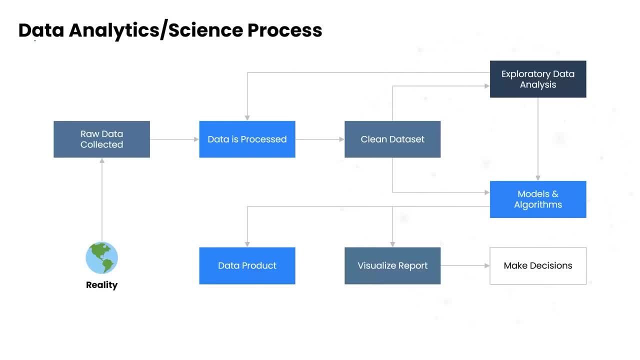 this particular flow chart is more close to how to solve an actual problem statement: how to solve an actual problem in a real world scenario. now there are multiple things we need to discuss in this particular flowchart. i am pretty much sure that by the end of this video you will have a better 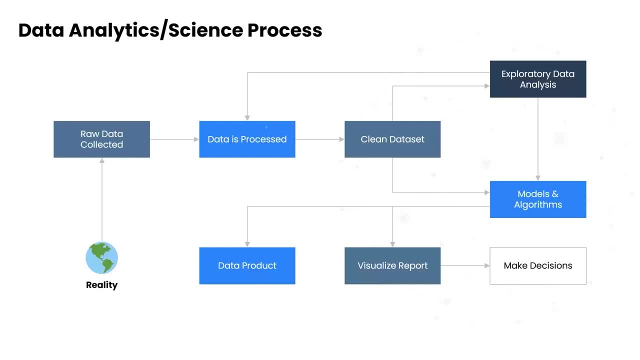 understanding on what exactly is eda, what exactly are model building processes and how this entire data analytics or data science process works. it all starts with data. data is most important to perform any kind of analysis or to create a dashboard or to create a model. without data, nothing is possible, so it all starts with the reality. 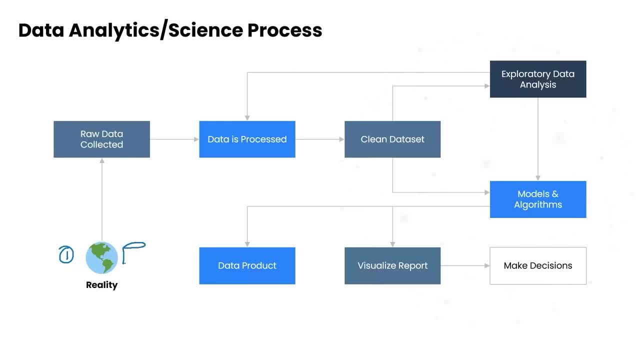 reality basically means: what type of data do we have? do we have a database? if we don't have a database, from where can we get the data? is it through web scraping? is it directly through some clients? so whatever medium or whatever source the data comes from, that depends and changes from scenario to scenario. 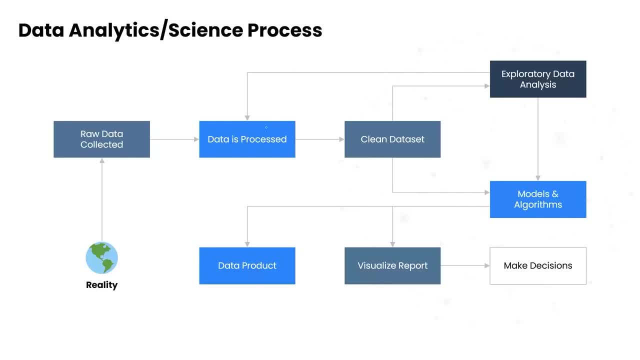 what exactly are model building processes and how this entire data analytics or data science process works. it all starts with data. data is most important to perform any kind of analysis or to create a dashboard or to create a model. without data, nothing is possible. so it all starts with the reality. reality basically means: what type of data do we have? 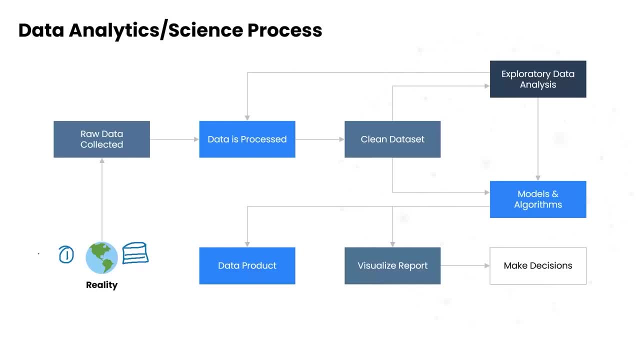 do we have a database? if we don't have a database, from where can we get the data? is it through web scraping? is it directly through some clients? so, whatever medium or whatever source the data comes from, that depends and changes from scenario to scenario. at some scenarios you might have to 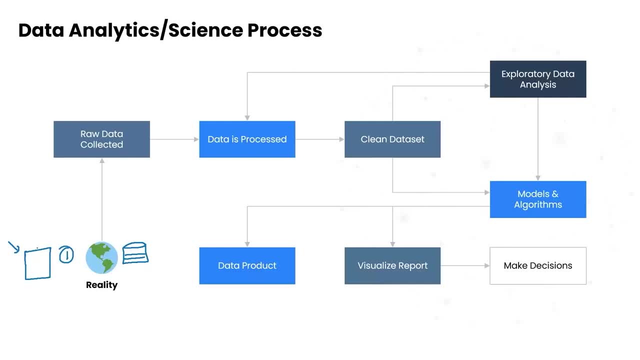 extract the data from your own company's database. in some scenarios you have to do web scraping. in some scenarios, your client will be providing you the data. so the first step is always the data collection part. the data that is collected initially is all your raw data. now from the raw. 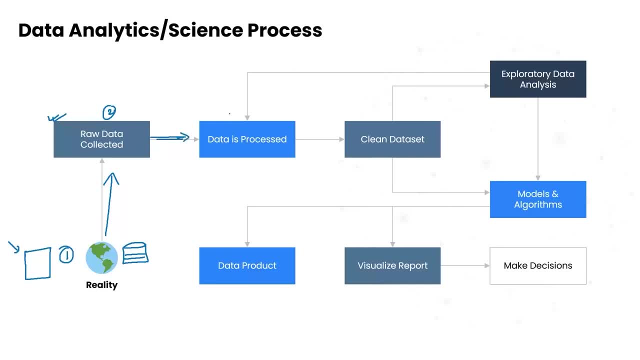 data. the next step is always data processing. data is being processed, data is being processed and prepared. now, in this preparation step, the output is always a clean data. what do we perform here? there are multiple things that are performed. for example, the data that you have captured is having 200 columns or 100 columns. 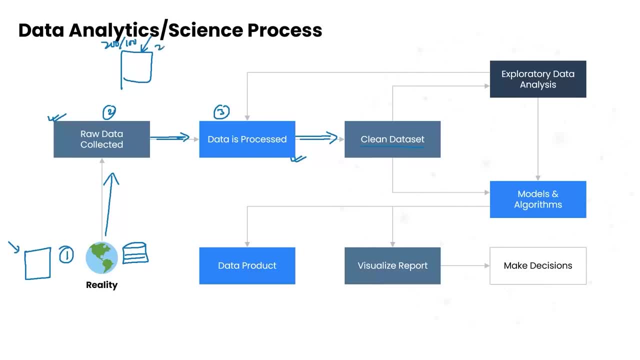 now you know, using your domain knowledge, that you don't need 20 of these columns. they are not relevant for the problem statement, so you get rid of them. there are some missing values. you want to get rid of them. there are some invalid data types. there are some. 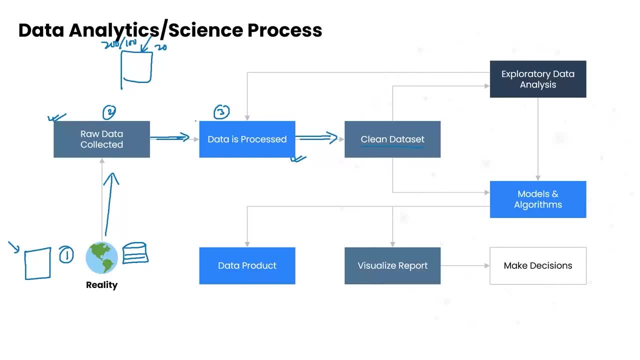 special characters which you want to get rid of. so there are some techniques that we follow here to clean the data. the output of the data processing part is a clean data. clean data goes as an input for your eda process. in the eda process, also using some sort of analysis, let's say outlier detection or probably. 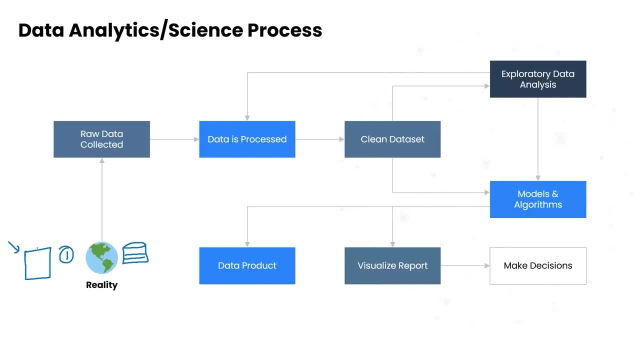 at some scenarios, you might have to extract the data from your own company's database. in some scenarios, you have to do web scraping. in some scenarios, your client will be providing you the data. so that's why we have a database where we can get the data from. where can we get the data, is it? 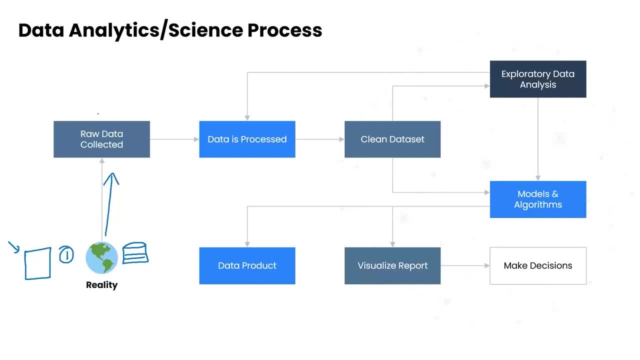 so the first step is always the data collection part. the data that is collected initially is all your raw data. now, from the raw data, the next step is always data processing. data is being processed, data is being processed and prepared now, in this preparation step, the output is always a clean data. what do we perform? 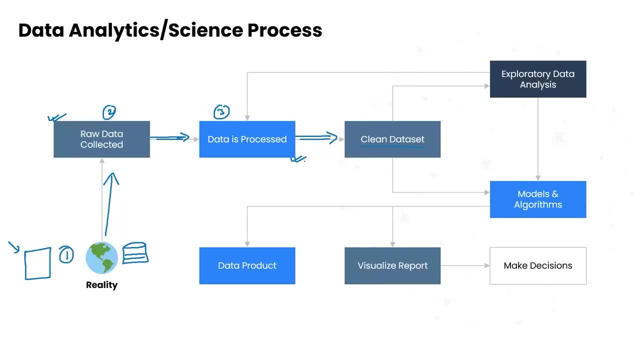 there are multiple things that are performed. for example, the data that you have captured is having 200 columns or 100 columns. now you know, using your domain knowledge, that you don't need 20 of these columns. they are not relevant for the problem statement, so you get rid of them. 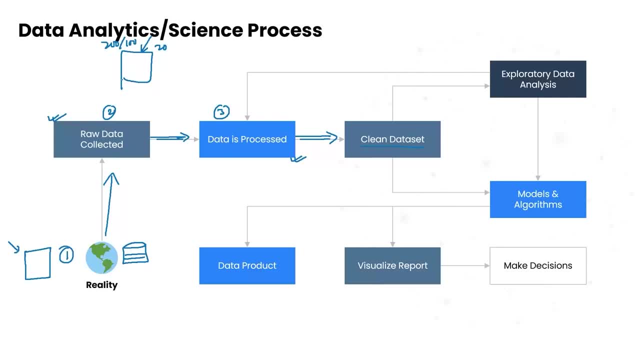 there are some missing values. you want to get rid of them. there are some invalid data types. there are some special characters which you want to get rid of. so there are some techniques that we follow here to clean the data. the output of the data processing part is a clean data. 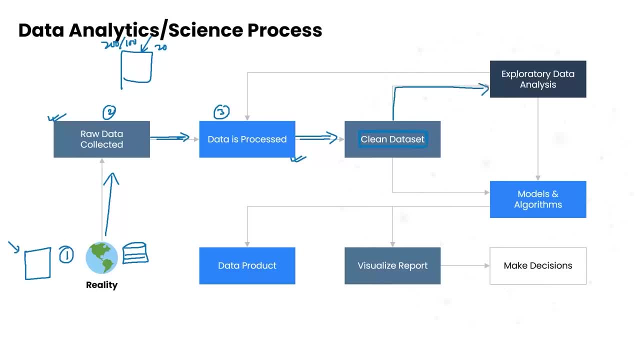 clean data goes as an input for your eda process. in the eda process, also using some sort of analysis, let's say outlier detection or probably any other analysis we come across, and we find that you know what, out of the 80 columns that are present, 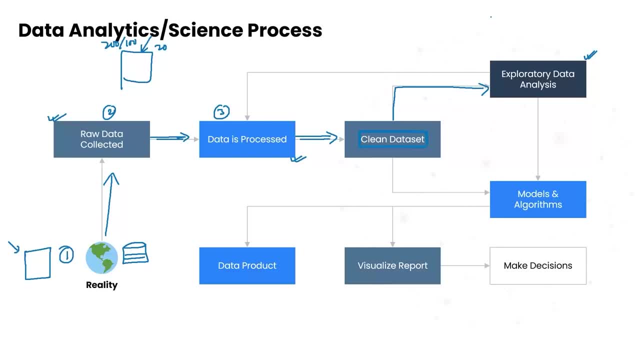 probably 10 or 15 are not relevant and that you finalize based on your analysis. so again, you have to go through this data processing step. so, in short, this data processing, data cleaning part and the eda part is kind of an iterative process. you process the data. 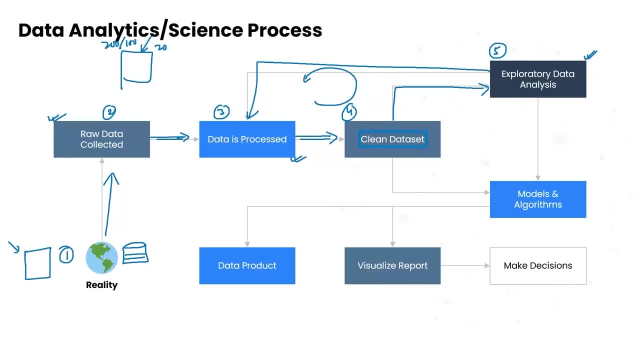 then get the clean data set. then do eda. while doing eda also, you realize that there are some of the data sets or some of the columns that are not relevant, some of the rows that are not relevant, some of the records that are outliers. i need to get rid of them. you again come back again do the. 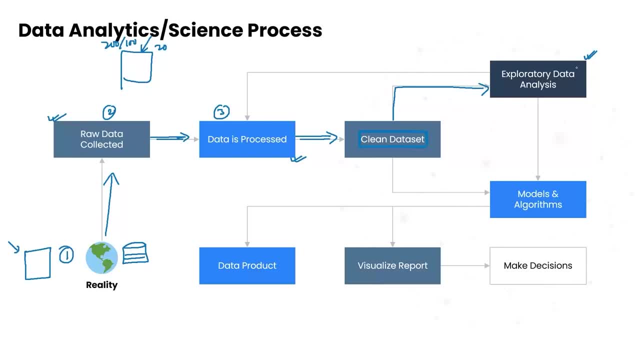 any other analysis we come across and we find that you know what, out of the 80 columns that are present, probably 10 or 15 are not relevant and that you finalize based on your analysis. so again, you have to go through this data processing step. so, in short, this data processing. 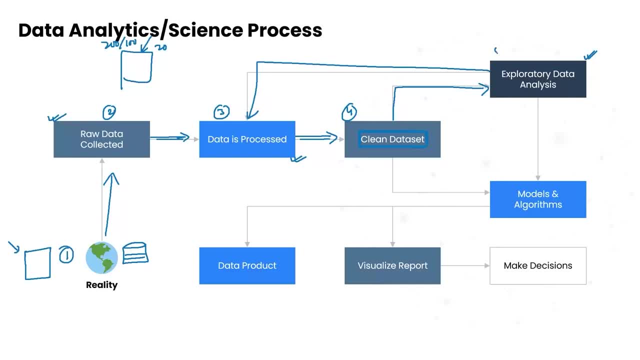 data cleaning part and the eda part is kind of an iterative process. you process the data, then get the clean data set, then do eda. while doing eda also, you realize that there are some of the data sets or some of the columns that are not relevant, some of the rows that are not relevant. 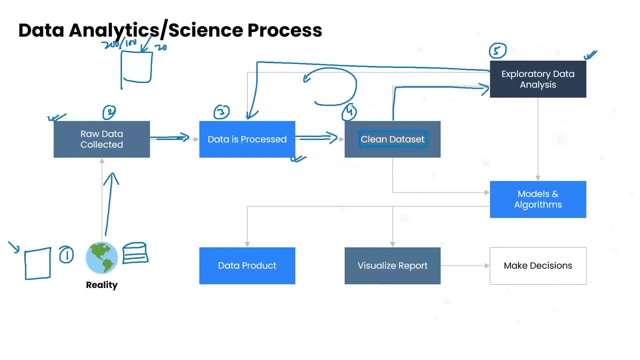 some of the records that are outliers. i need to get rid of them. you again come back again, do the data processing part. so i'll just pause and show you how you can do that Ultimately after doing this iterative process. after doing this iterative process, let's say, finally you have done your EDA, Finally you have done your exploration of data. So your insights are with you. You know the problem statement and you know what are the possibilities why this problem has occurred. 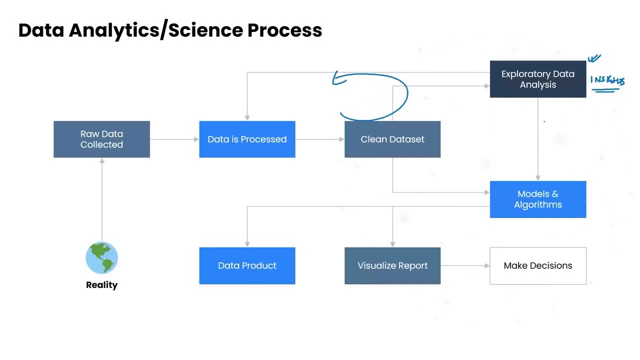 So after EDA generally comes your model building part. In some cases, in some companies, in some scenarios, you do not have to do the EDA. Directly from the clean data you can take and start with the model building part. EDA is not important in some of the scenarios But if you do EDA that is a better scenario. That is better thing to do. 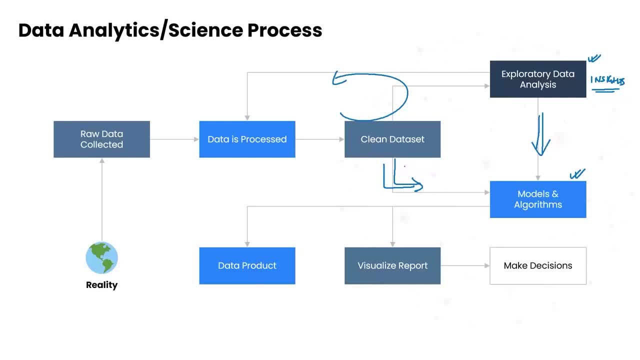 So, after EDA or without EDA, finally you take and start with the model building part, And this is where your machine learning engineers or data scientists come into picture. After your model is prepared, after your algorithms are set, then you prepare your final data product. Then you finally visualize the report. 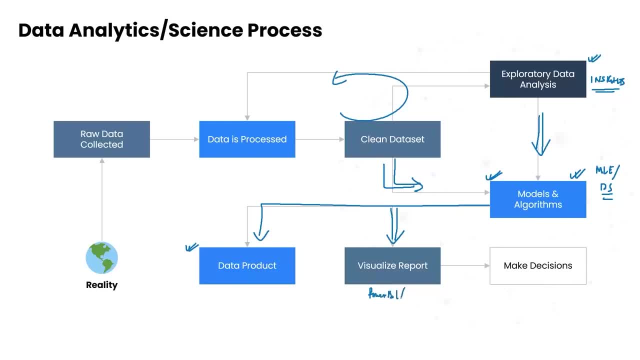 Using some Power BI or Tableau or probably Python, you kind of create some visualizations that you showcase to your customers- your end customers or to your higher management- and based on that you finally take some decisions. so that is how the entire data analytics and data science process happens. 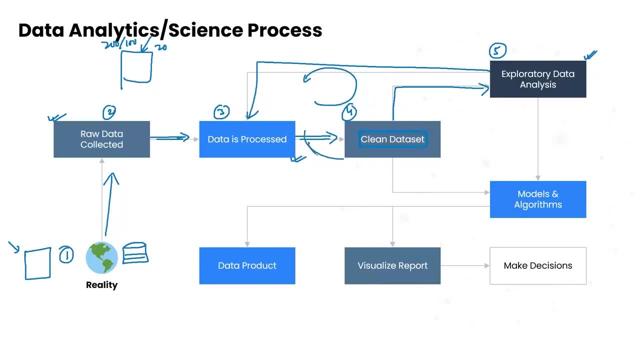 data processing part. so, ultimately, after doing this iterative process, after doing this iterative process, let's say, finally you have done your ed, finally you have done your exploration of data. so your insights are with you, you know the problem statement and you know what are the possibilities why this problem has occurred. after eda generally comes your model building part. 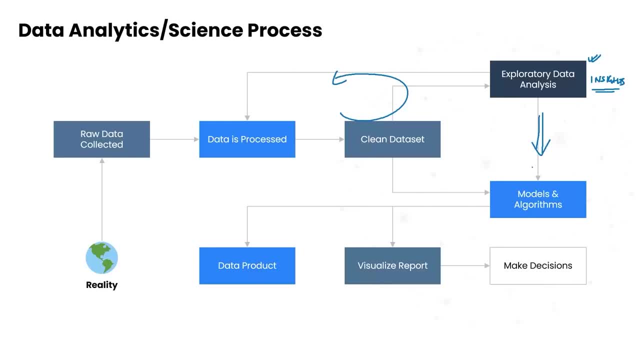 in some cases, in some companies, in some scenarios you do not have to do the ed directly from the clean data. you can do the clean data from the clean data. you can do the clean data from the clean data. you can take and start with the model building part. eda is not important in some of the 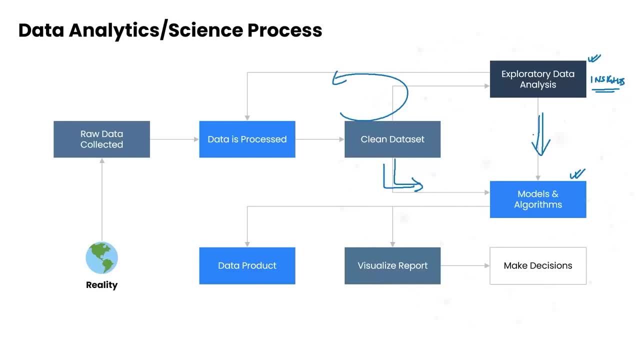 scenarios. but if you do eda, that is a better scenario. that is better thing to do so after eda or without eda. finally, you take the clean data and try to do the model building part, and this is where your machine learning engineers or data scientists come into picture. 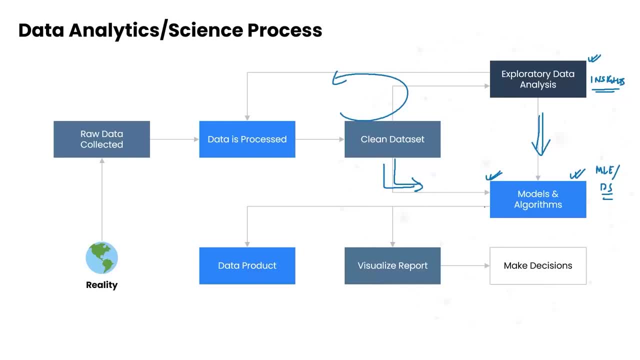 after your model is prepared, after your algorithms are set, then you prepare your final data product. then you finally visualize the report using some power bi or tableau or probably python. you kind of create some visualizations that you showcase to your end customers or to your higher management and based on that you finally take 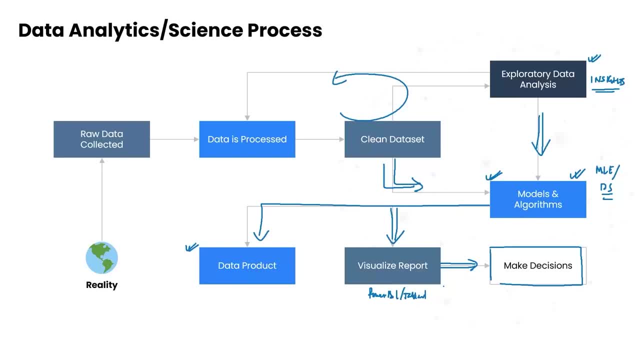 some decisions. so that is how the entire data analytics and data science process happens. so in this particular module definitely, collection of data is little bit difficult to cover because there are so many scenarios, so many, uh, you know, things that can be done in the collection part we will mostly 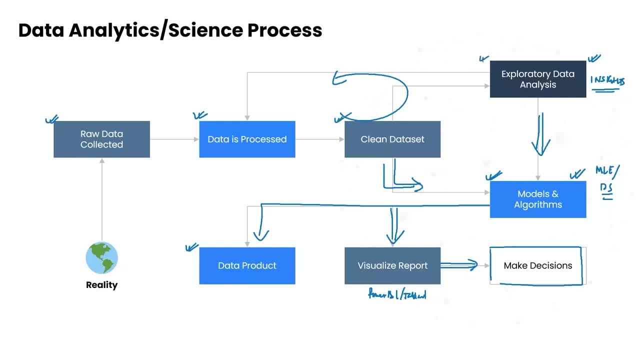 be focusing on the data processing, data cleaning and the eda part. so by the end of this particular module you will have a clear picture on how data is processed, cleaned and how the data analysis is done, eda is done, and how do we get the insights from the data. 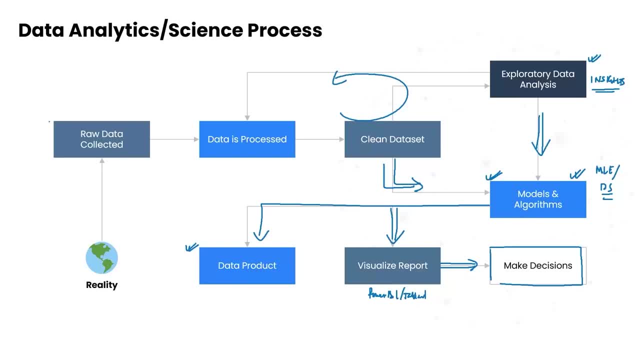 so in this particular module definitely, collection of data is little bit difficult to cover because there are so many scenarios, so many- you know- things that can be done in the collection part. we will mostly be focusing on the data processing, data cleaning and the eda part. so by the end of 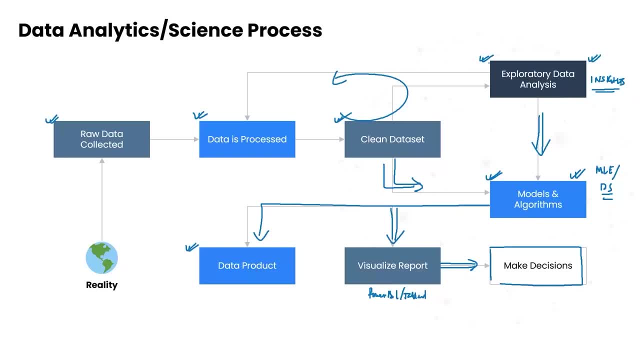 this particular module, you will have a clear picture on how data is processed, cleaned and how the data analysis is done, eda is done, and how do we get the insights from the data. what data is trying to tell us? so that's all about this particular end-to-end process in. 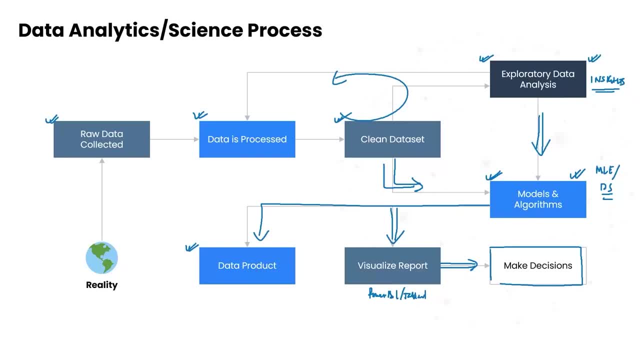 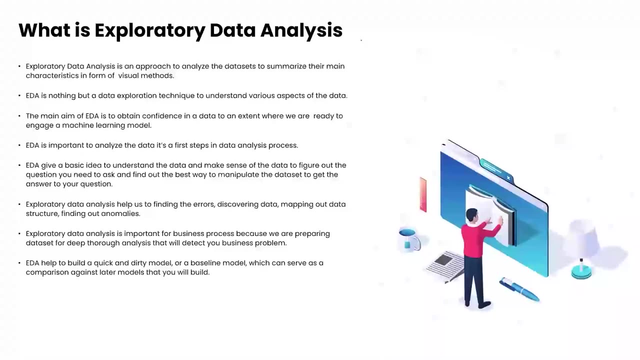 the next video, we shall be talking about few other topics related to eda. what is eda, what is visualization, steps involved in eda and so on. what is exploratory data analysis? in simple terms, we call it as eda. exploratory data analysis is an approach to analyze the data. 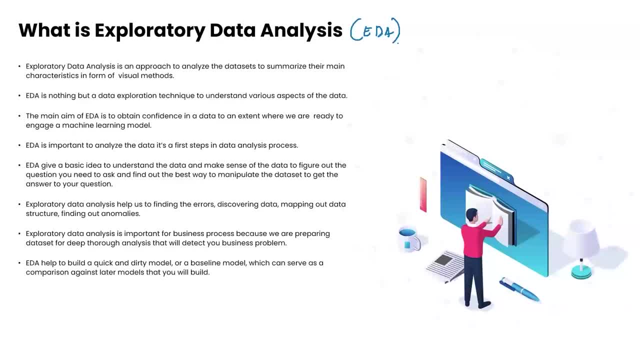 sets to summarize their main characteristics in the form of visual methods. eda is nothing but a data exploration technique to understand various aspects of the data. the main aim of eda is to obtain confidence in a data to an extent where we are ready to engage a. 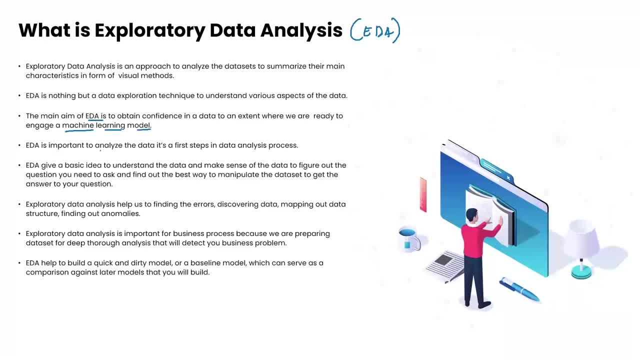 machine learning model. eda is important to analyze the data as it is a first step in the data analysis process. eda gives a basic idea to understand the data and make sense of the data. to figure out the question you need to ask and find out the best way to manipulate the data set to get the answer to your question. 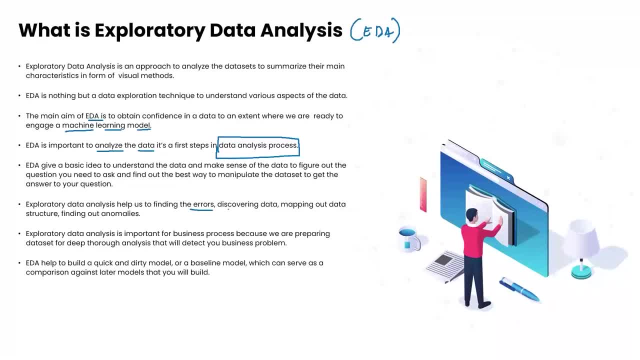 exploratory data analysis helps us in finding errors, discovering data and mapping out data structure, finding out anomalies. anomalies are nothing but outliers. exploratory data analysis is important for business process because we are preparing data set for deep, thorough analysis that will detect your business problem. eda help to build a quick and dirty model or a baseline model. 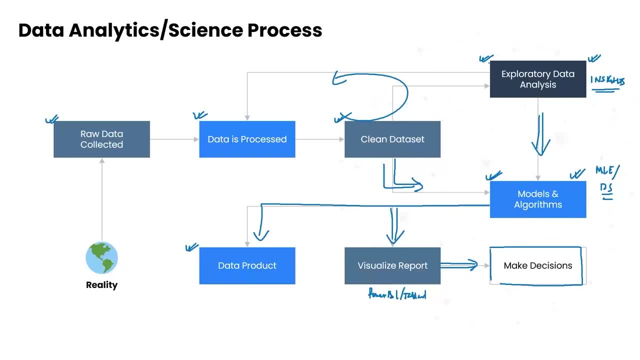 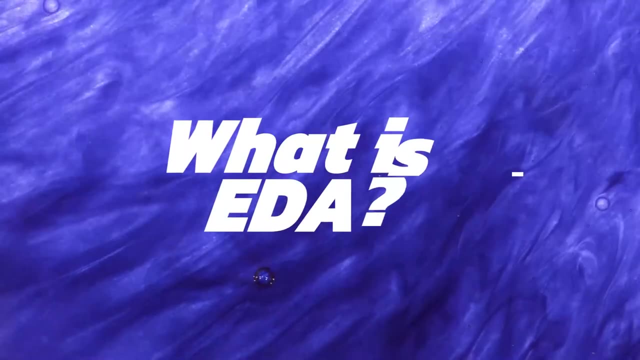 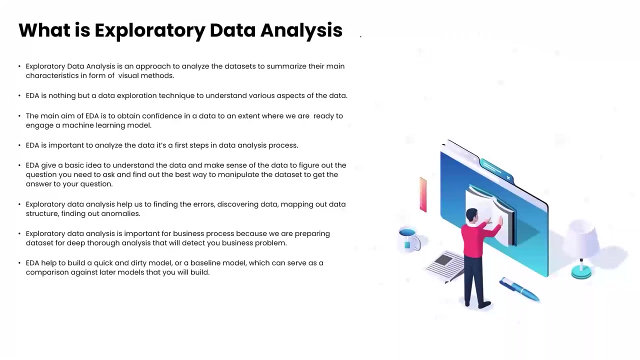 what data is trying to tell us. so that's all about this particular end-to-end process. in the next video, we shall be talking about few other topics related to eda. what is eda, what is visualization, steps involved in eda and so on. what is exploratory data analysis? 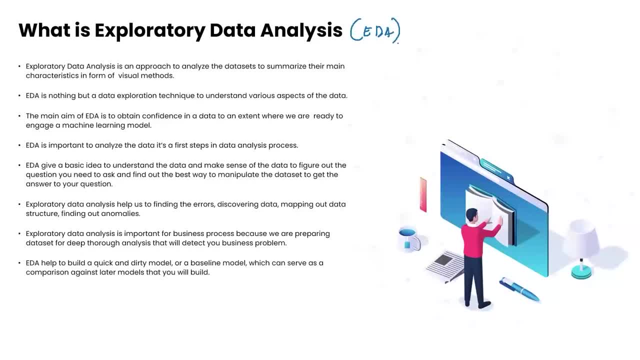 in simple terms, we call it as eda. exploratory data analysis is an approach to analyze the data sets, to summarize their main characteristics in the form of visual methods. eda is nothing but a data exploration technique to understand various aspects of the data. the main aim of eda is to obtain confidence in a data. 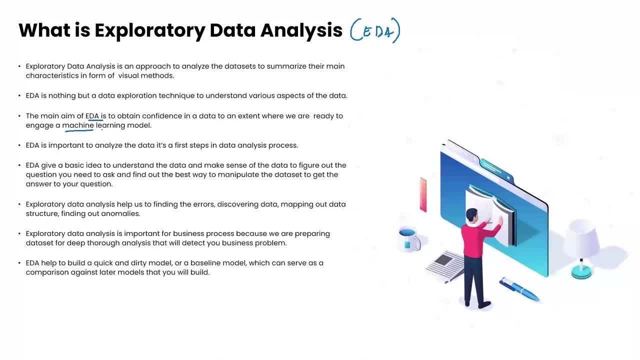 to an extent where we are ready to engage a machine learning model. it is important to analyze the data, as it is a first step in the data analysis process. eda gives a basic idea to understand the data and make sense of the data, to figure out the question you need to ask and find out the best way to manipulate the data set. 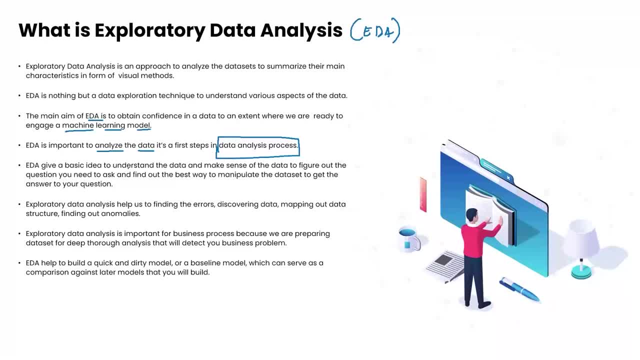 to get the answer to your question. exploratory data analysis helps us in finding errors, discovering data and mapping out data structure, finding out anomalies. anomalies are nothing but outliers. exploratory data analysis is important for business process because we are preparing data set for deep, thorough analysis that will detect your business problem. 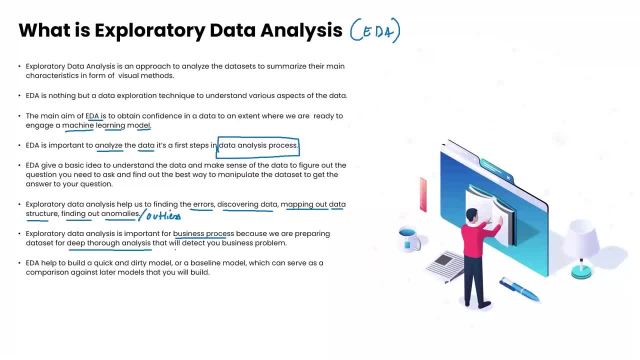 eda helped to build a quick and dirty model, or a baseline model, which can serve as a comparison against later models and many otherthree majorסiveるreliance that you will build. what do we understand with this? in simple layman's term, edia is one form of a step or an approach which is used to analyze data sets. 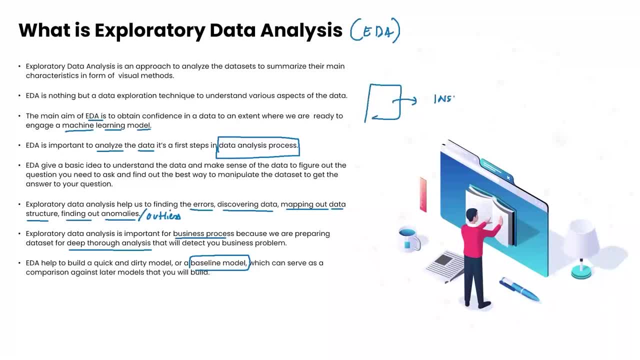 so that we can analyze data sets and get some insights out of it. and the insights has to be in the form of visual, because the edaincites, the output of eda, has to be presented to a higher management or to a client who might not be able to. 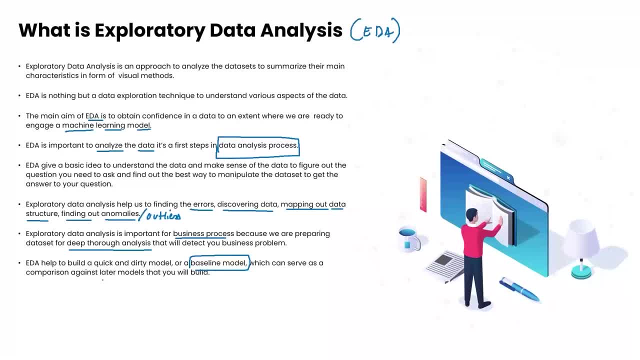 which can serve as a comparison against later models that you will build. what do we understand with this? in simple layman's term, eda is one form of a step or an approach which is used to analyze data sets, so that we can analyze data sets and get some insights out of it, and the insights has to be in the form of visual. 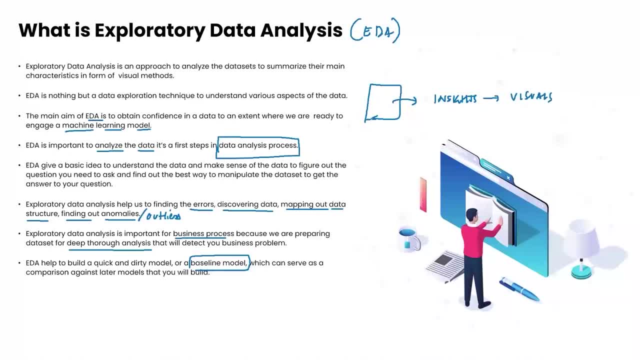 because the eda insights, the output of eda, has to be presented to a higher management or to a client who might not be able to understand or interpret well from a python code. so it has to be visually appealing so that a non-technical person who has no idea about 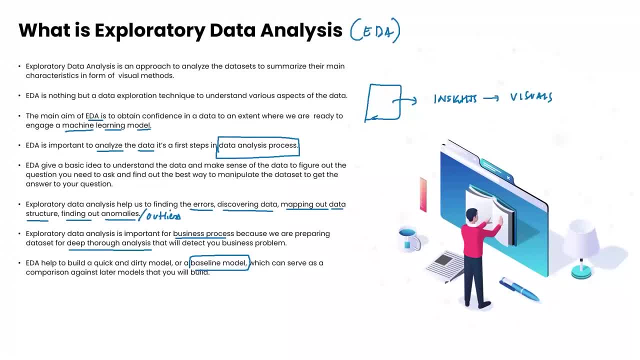 data analytics or data science, will be able to understand what the data is telling us: whether a person staying in japan is more likely to churn or a person staying in indonesia. whether males are more likely to churn than females. if yes, why? whether somebody who has been doing a payment through credit cards are more likely to churn. 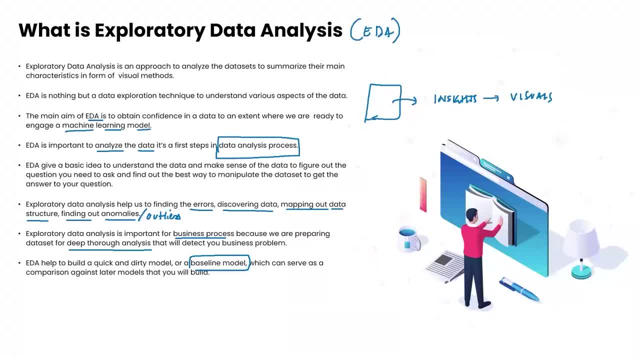 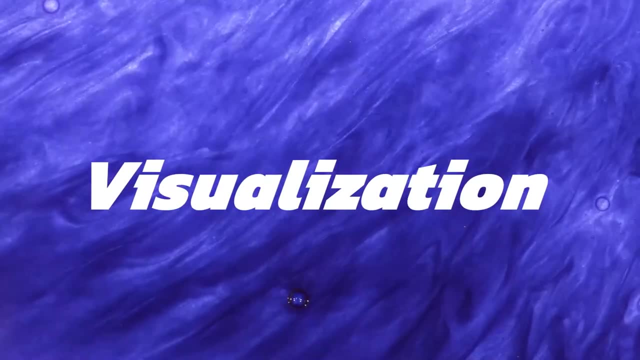 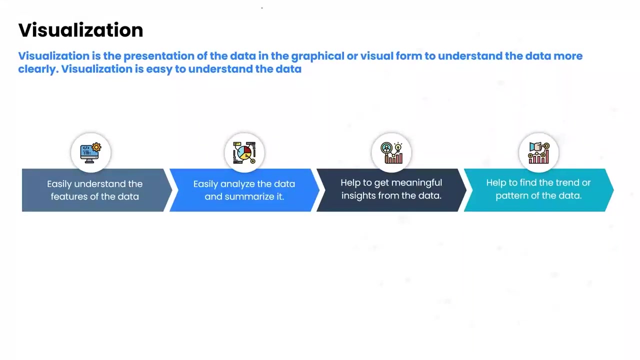 what is the reason behind it? so, ultimately, eda is simply nothing but an approach to analyze your data, to summarize their main characteristics in the form of visual methods. what is visualization? we all know visualization and what is the power of visualization. because, ultimately, in the field of data analytics, visualization is very important. because, 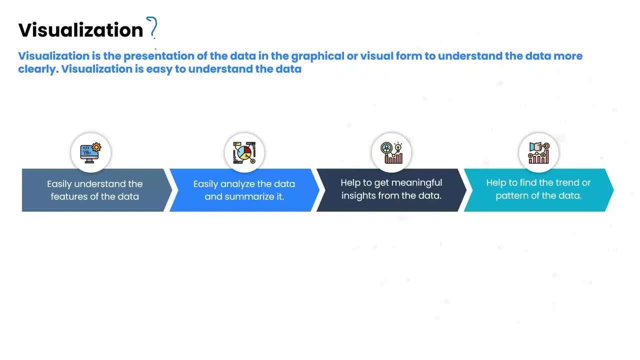 that is one of the ways how we showcase our insights to the end customer or to a higher management who might not have that much of knowledge into python. visualization is simply the presentation of the data in the graphical or visual form to understand the data more clearly. if you discuss our vidéo of the data analytics algorism, 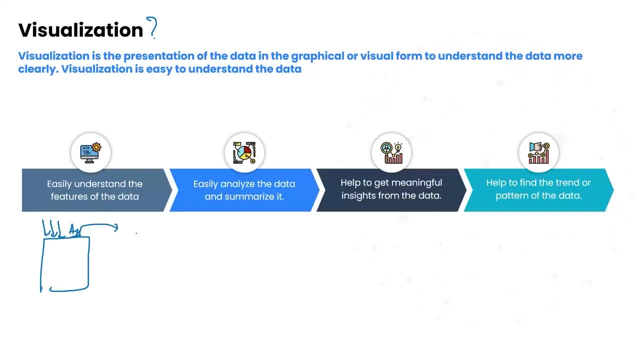 gonna give you an jan Tutorial and I hope you'll like it. now, if you talk about, let's say, i have data and there are multiple columns. one of the columns is age. if somebody asks you what is the characteristics or what are the summary statistics that you are, 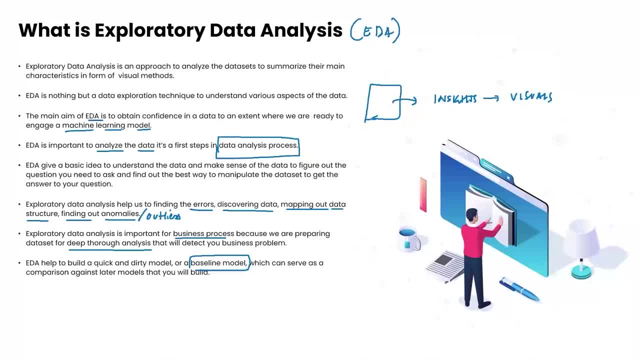 understand or interpret well from a python code. so it has to be visually appealing, so that a non-technical person who has no idea about data analytics or data science will be able to understand what the data is telling us: whether a person staying in japan is more likely to churn. 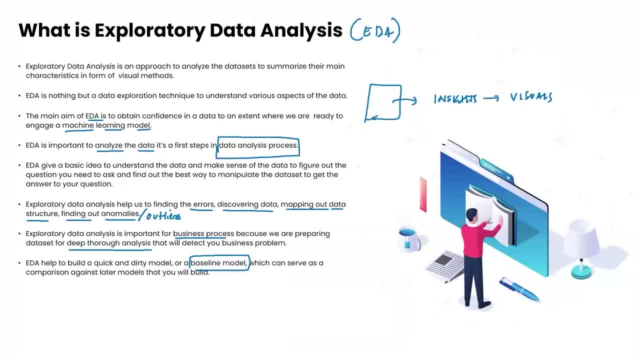 or a person staying in indonesia, whether males are more likely to churn than females. if yes, why? whether somebody who has been doing a payment through credit cards are more likely to churn. what is the reason behind it? so, ultimately, eda is simply nothing but an approach to analyze. 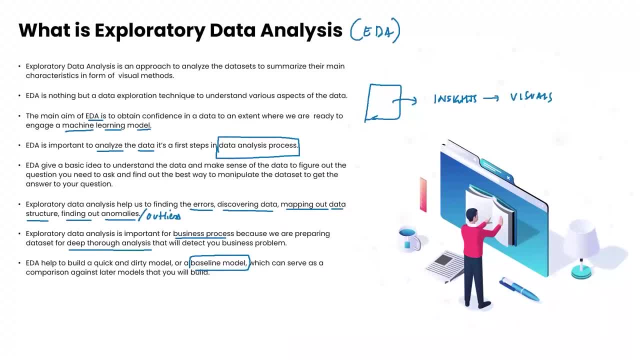 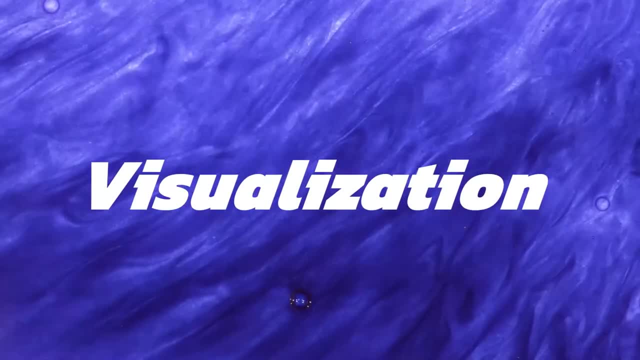 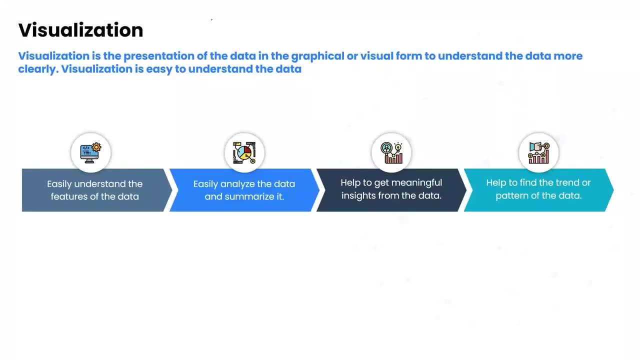 your data to summarize their main characteristics in the form of visual methods. what is visualization? we all know visualization and what is the power of visualization? because, ultimately, in the field of data analytics, visualization is very important because that is one of the ways how we showcase our insights to the end customer or to a higher management. 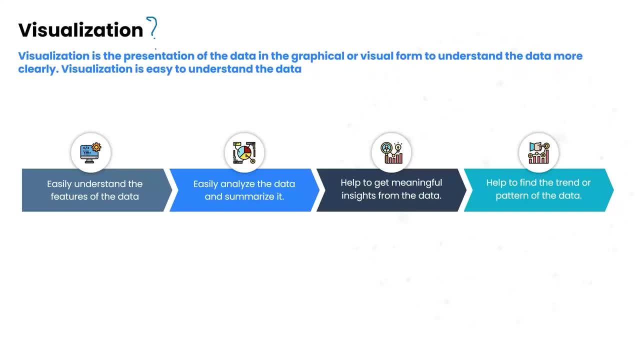 so if you can visualize the data in one way or another, then you might not have that much of knowledge into python. visualization is simply the presentation of the data in the graphical or visual form to understand the data more clearly. now, if you talk about, let's say, i have data and there. 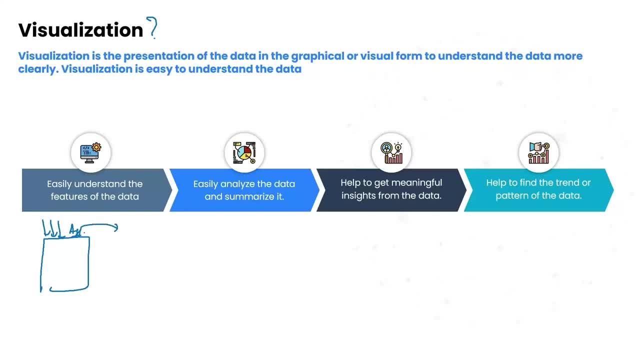 are multiple columns. one of the columns is age. if somebody asks you what is the characteristics or what are the summary statistics that you are getting from age, that age, the mean age, is basically 25. the 25th percentile is, uh, your, let's say, 32. the 75th 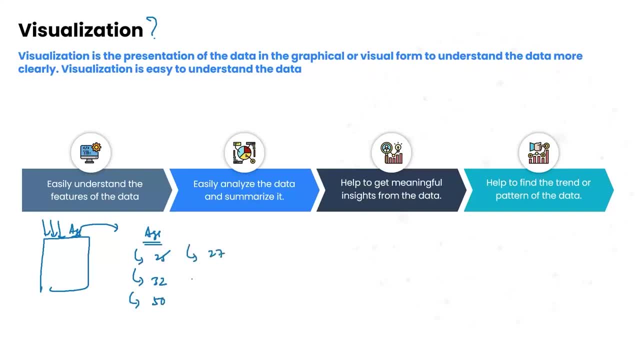 percentile is 50, the median value is 27 and the maximum value is 92, or else, if somebody asks you, can you give me details about the gender? you probably tell that male are 1400 and female are like 2000, whether this is a better way of showcasing or this definitely a visual technique. 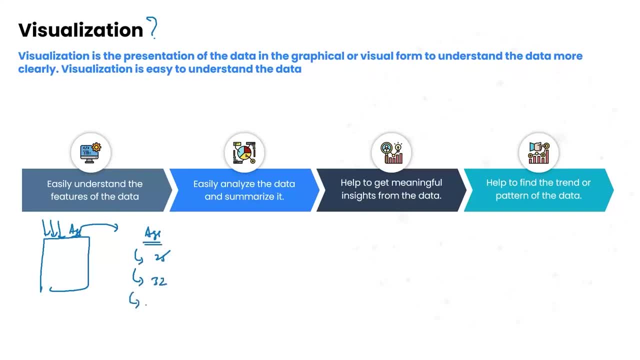 getting from age. then you tell that age, the mean age is basically 25.. that 25th percentile is um, median value is 27 and the maximum value is 92. or else, if somebody asks you, can you give me details about the gender? you probably tell that male are 1400 and female are like 2000. 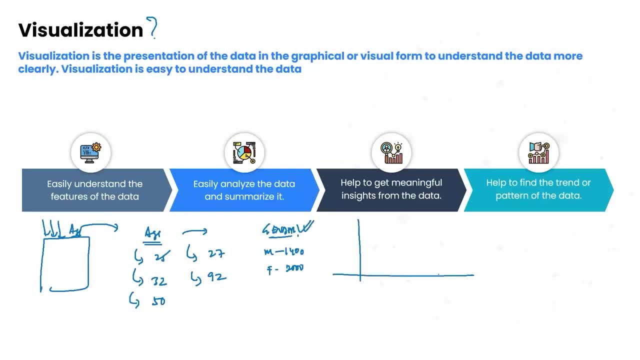 whether this is a better way of showcasing or this definitely a visual technique or a visual way is more intuitive and more attractive for an end customer to understand. about the data, anybody can clearly understand that. you know females are larger in number. probably females are way more than the number of males. or else, if you want to visualize in: 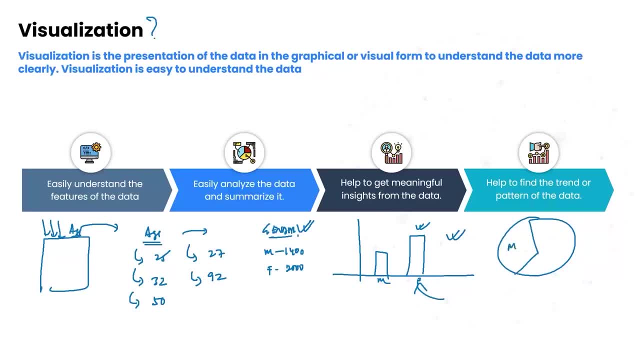 another way, using a pie chart. then also you will be able to understand that female are more in numbers than male using numbers. words also we can interpret, but visually. visual form is always a better form to showcase the data. so visualization is nothing but the presentation of the data in graphical or visual form to 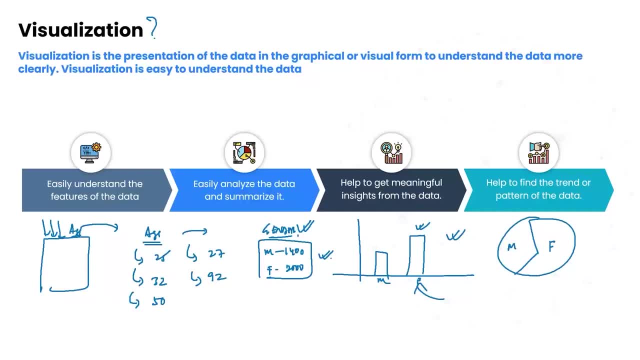 understand the data more clearly. what are the advantages of visualization? easily understand the features of the data. easily analyze the data and summarize it. help to get meaningful insights from the data and help to find the trend or pattern of the data. what are the different types of visualization that we use? there are different types of visualizations. 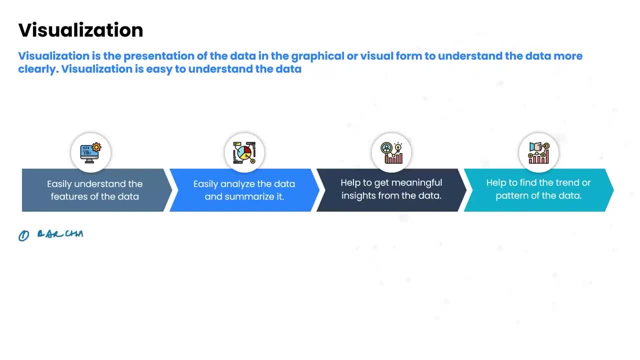 for example, we'll talk about a bar chart. let's say you have a column like gender. you can easily plot a bar chart to showcase the distribution of male and female. the same can also be done using a pie chart- male and female. imagine you are analyzing a numerical column. what 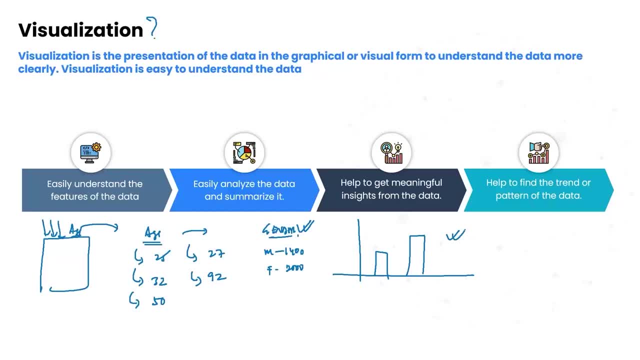 or a visual way is more intuitive and more attractive for an end customer to understand about the data. anybody can clearly understand that. you know females are larger in number. probably females are way more than the number of males. or else, if you want to visualize in another way, using a pie chart, then also you will be able to. 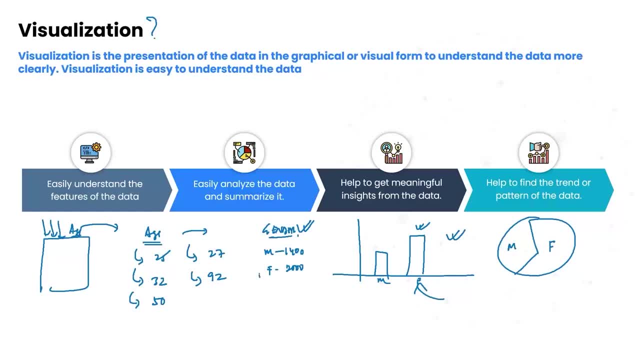 understand that female are more in numbers than male. using numbers also, we can interpret, but visually. visual form is always a better form to showcase the data. so visualization is nothing but the presentation of the data in graphical or visual form to understand the data more clearly. so the different types of visualization easily understand the features of the data easily analyze. 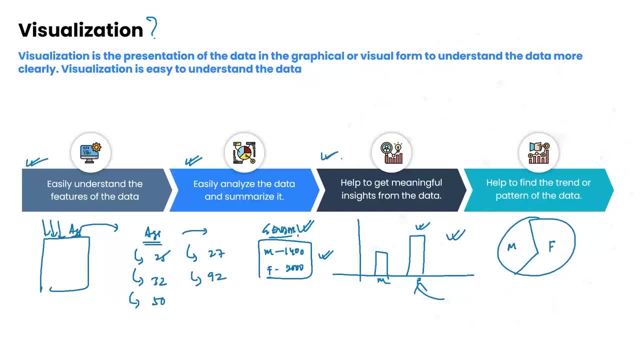 the data and summarize it, help to get meaningful insights from the data and help to find the trend or pattern of the data. what are the different types of visualization that we use? there are different types of visualizations. for example, we'll talk about a bar chart. you have a column like gender. you can easily plot a bar chart to showcase the distribution of male and 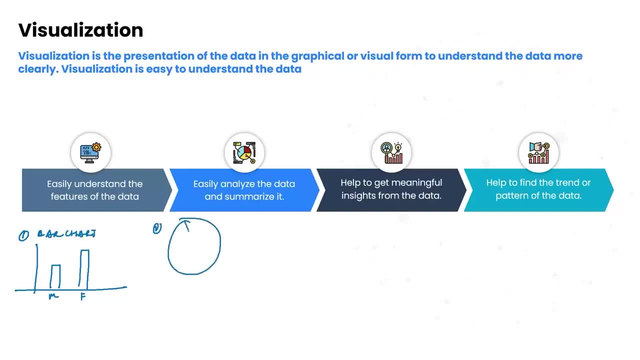 female. the same can also be done using a pie chart, male and female. imagine your analyzing a numerical column. what is the distribution of age? can I use a bar chart? probably? the age could vary from 18 to 90. in that case, you will end up having 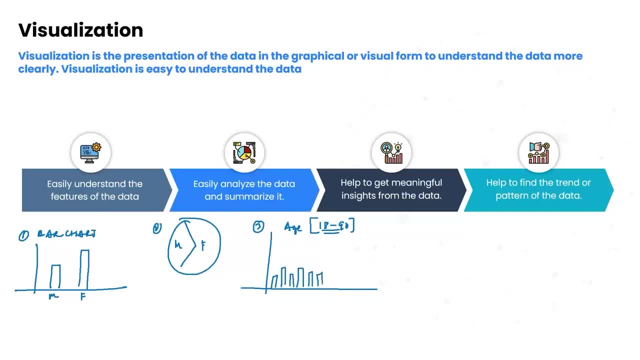 70 to bars, which is little bit difficult to interpret. so a better technique is to use a line chart which will be able to tell that there is a spike between 22 and 25, which means most of the people are within the range of 22 to 25. let's say you are analyzing height versus weight. two: numerical features. definitely you can take the ratio of height and width and take the ratio of height and width according to your nicht. essentially, if you take the ratio of height and width, you can say the number of cells that you canidirate. if you take the ratio of height and width, you can have in your chart. that is extremely important. 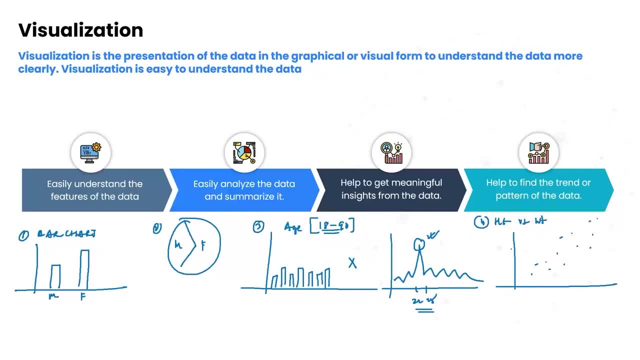 to make sure that you have a accurate representation of the physical environment. you can also have a size that you can calculate: a good representation of the gender and the age of the person. you can also help of a scatter plot to understand the distribution of the data and what is the. 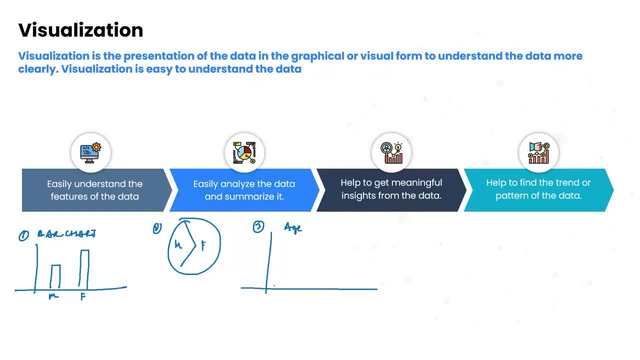 is the distribution of age. can i use a bar chart? probably the age could vary from 18 to 90. in that case, you will end up having 72 bars, which is little bit more than 72 bars those who are in front of you. there is a little bit difficult to interpret, so a better technique. 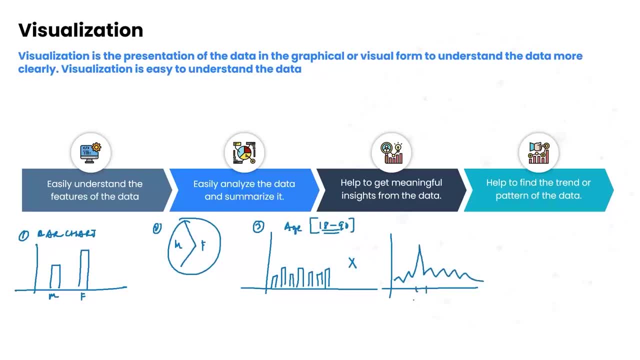 is to use a line chart which will be able to tell that there is a spike between 22 and 25, which means most of the people are within the range of 22 to 25. let's say you are analyzing height versus weight, two numerical features. definitely, you can take help of a scatter. plot to understand how this can be done and comment if the description is correct or not. let's say you have an associate of each and every one of the students or students. you can comment by the name or name and visit the section. you have the option of providing. 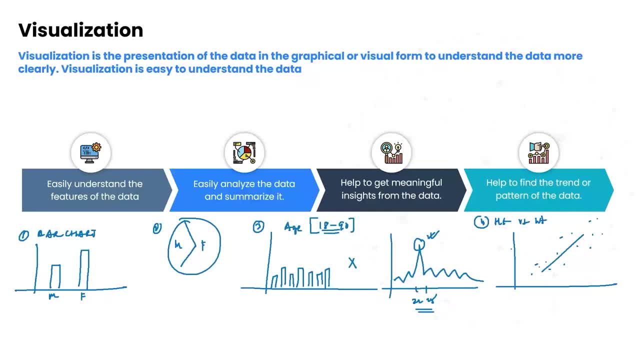 a bar chart. so what I'll do here is: let you evaluate this, and either you have to evaluate the distribution of the data and what is the relationship between height and weight? in this graph, it is quite evident that the when the weight is increasing, the height is also. 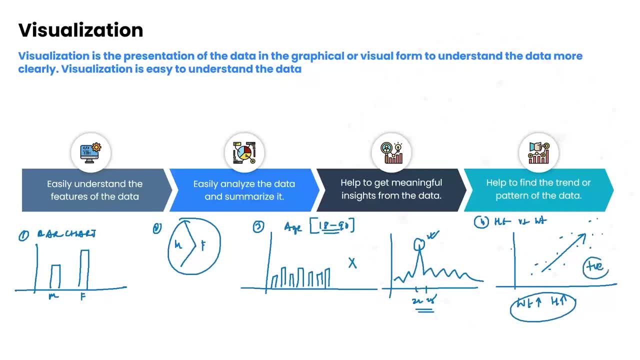 increasing, which means there is a positive correlation. so there are different types of charts, including bar charts, pie charts, line charts, area charts, box and whisker plots, violin plots, scatter plots, pair plots and a whole bunch of different other plots and diagrams and visualizations that we can use to summarize the data or to showcase what the data is telling us. 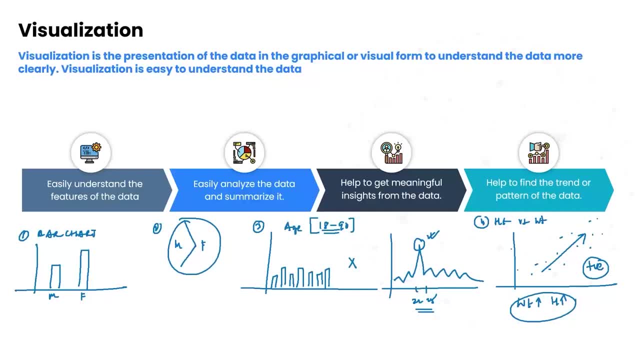 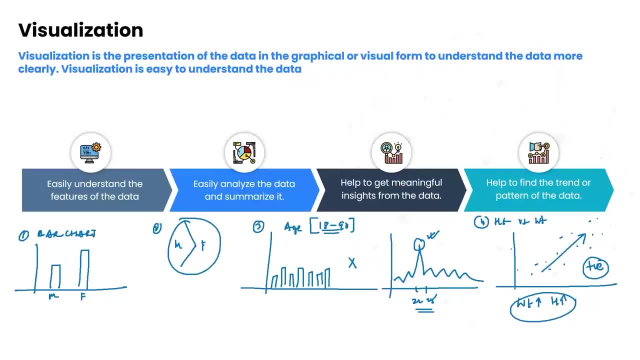 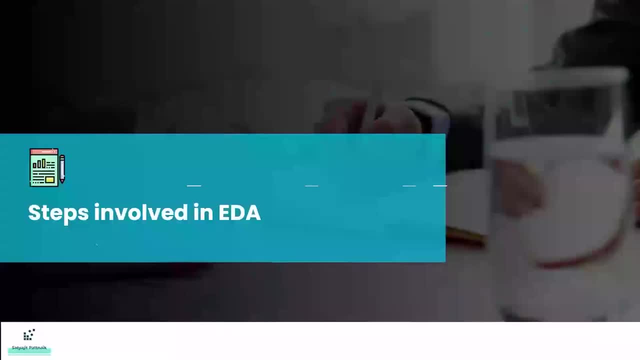 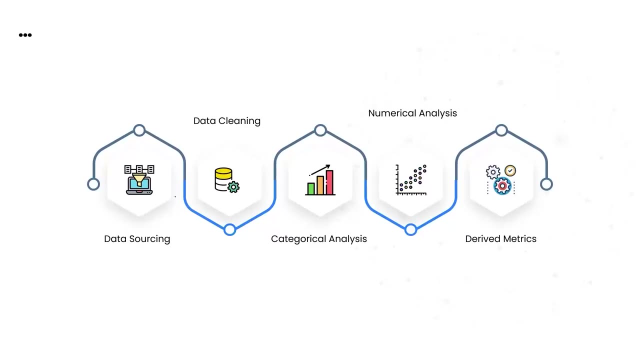 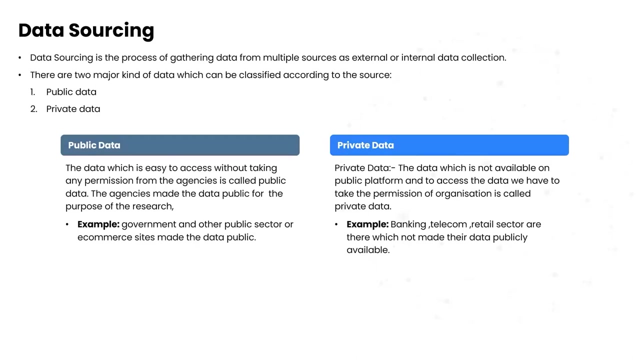 and to the end customer or to our managers. hi, in this video we shall be focused on the steps involved in the eta process. the first step is all about data sourcing. what do you mean by data sourcing? data sourcing is the process of gathering data from multiple sources. 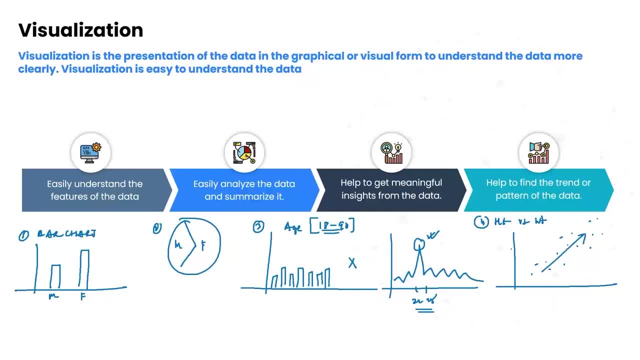 relationship between height and weight. in this graph it is quite evident that the when the weight is increasing, the height is also increasing, which means there is a positive correlation. so there are different types of charts, including bar charts, pie charts, line charts, area charts, box and whisker plots, violin plots, scatter plots, pair plots and a whole bunch of different other. 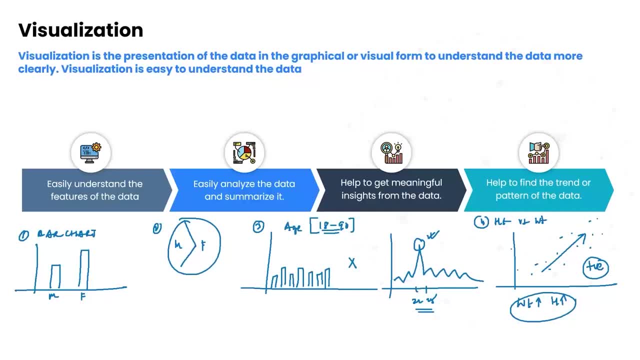 plots and diagrams and visualizations that we can use to summarize the data or to showcase what the data is telling us. so visual analytics is one of the most powerful analytics in the field of data analytics and we usually go for this technique, go for the visualization technique to showcase. 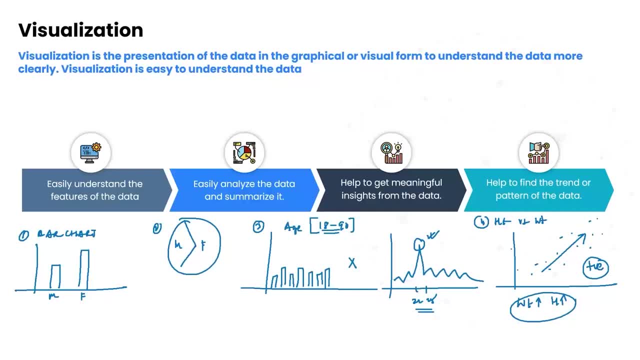 our table of contents for the data analysis, and that's what we are gonna talk about today. we are going to use the table of contents and let's now see how to do that with the data analysis, so our insights to an end customer or to our managers. 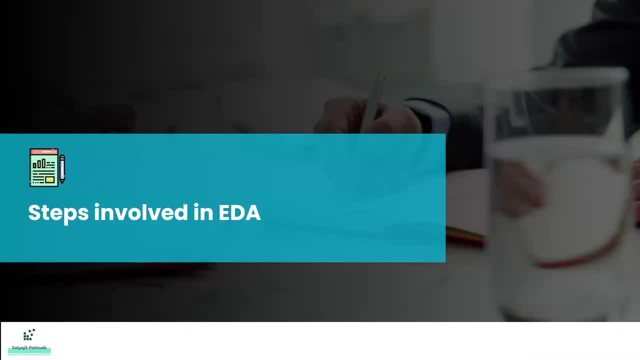 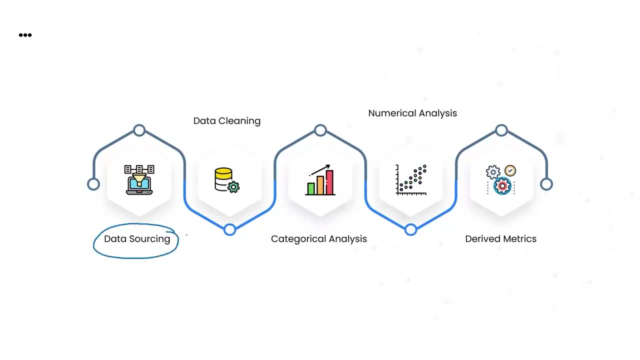 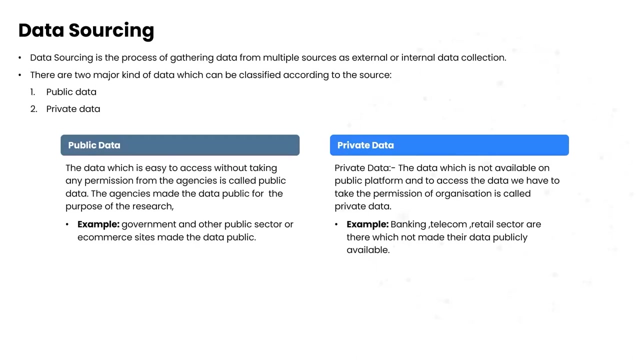 hi, in this video we shall be focused on the steps involved in the ETA process. the first step is all about data sourcing. what do you mean by data sourcing? data sourcing is the process of gathering data from multiple sources as external or internal data collection. there are two major kind of data which 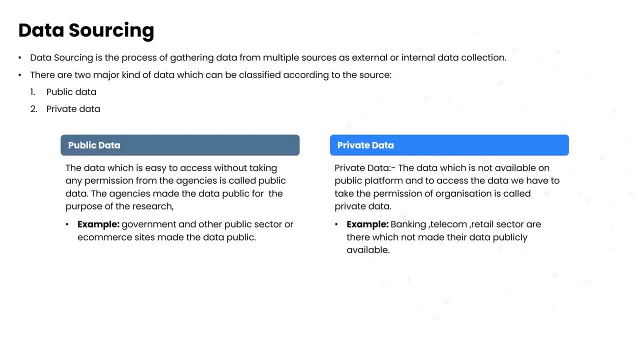 can be classified according to the source. one is public data and one is private data. what do you mean by public data and private data? public data is the data which is easy to access without taking any permission from the agencies. the agencies made the data public for the. 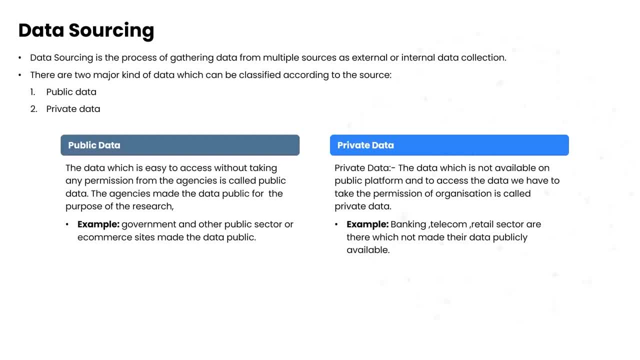 purpose of research, for example, multiple government websites and other public sector on e-commerce websites that make the data publicly available. you can easily extract the data, download the data or use some web scraping techniques to get public data for your analysis. the second type of data is private data, The data which is not available on the public platform, and to get 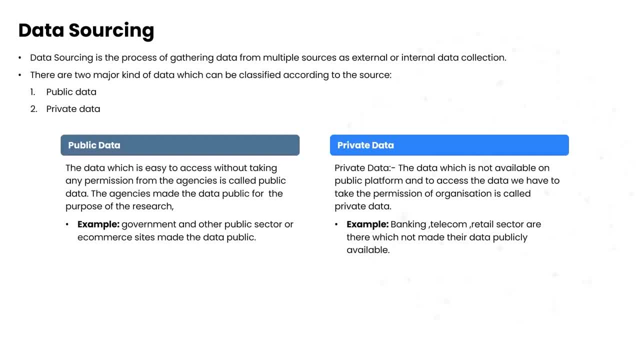 access to the data, we have to take permission of the organization. Now, for example, you are currently working with a telecom company or a banking company. You have to work on multiple banking use cases. In order to work on such use cases, you have to reach to your own organization's. 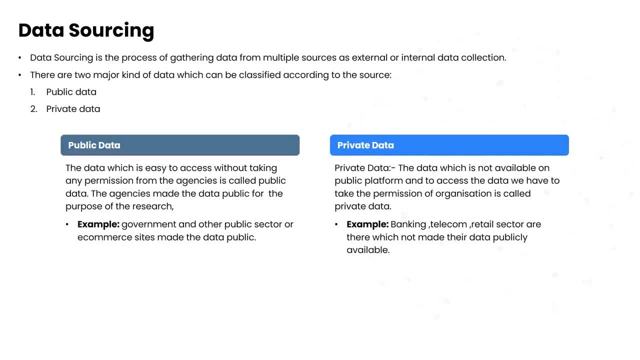 as external data sources, and this process is used to gather data from multiple sources as external or internal data collection. there are two major kind of data which can be classified according to the source: one is public data and one is private data. what do you mean by public data? 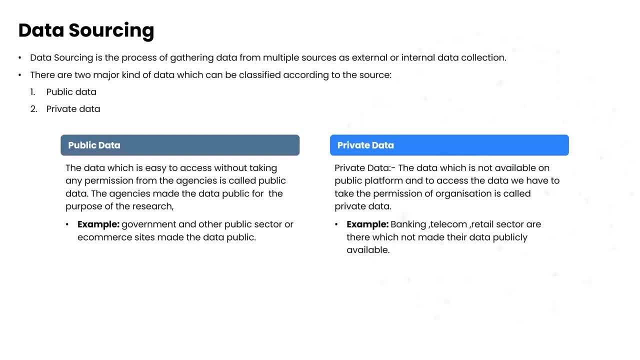 and private data. public data is the data which is easy to access without taking any permission from the agencies. the agencies made the data public for the purpose of research, for example, multiple government websites and other public sector or e-commerce websites that make the data publicly available. you can easily extract the data, download the data or use some. 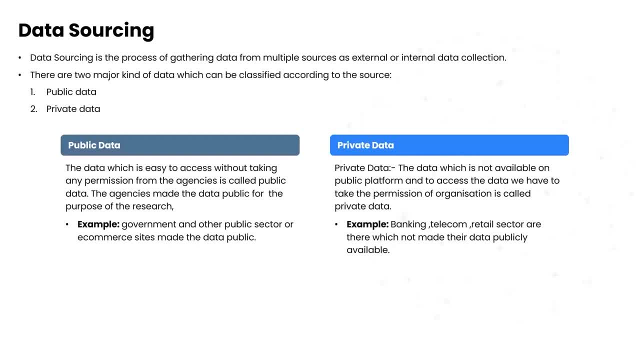 web scraping techniques to get public data for your analysis. the second type of data is private data, the data which is not available on the public platform, and to get access to the data, we have to take permission of the organization. now, for example, you are currently working with a. 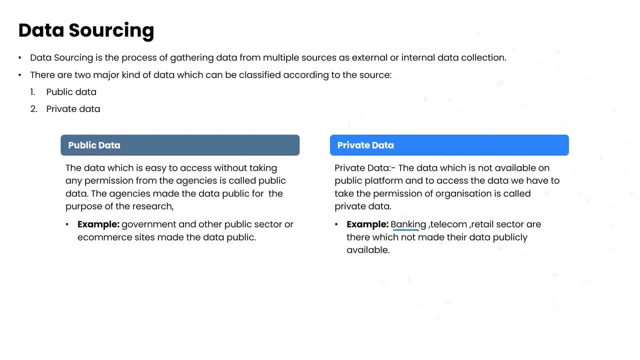 telecom company or a banking company, you have to work on multiple banking use cases. in order to work on such use cases, you have to reach to your own organization's dba team, which is your database administration team, to help them give you access for the data. once they give you the access to the data, you can either download it. 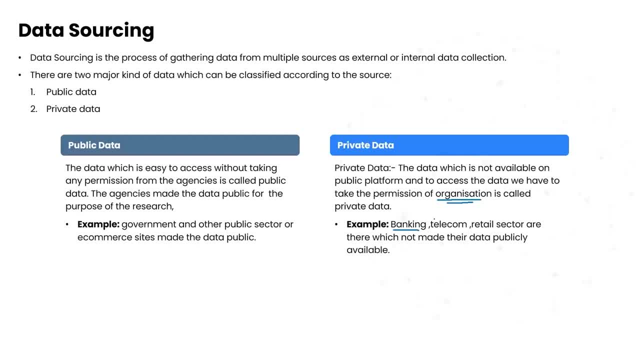 or create a connector to use the data for your analysis process, but depending on the use case that you are trying to solve, you have to choose your data source wisely. if i also talk about one of the scenarios talking about different companies, there are different types of companies, one of them: 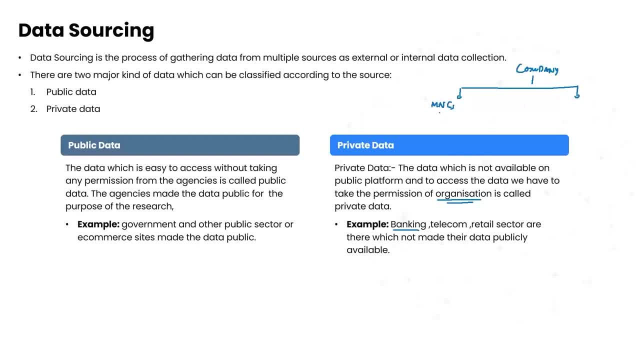 being mncs, which are your multinational companies most likely, when you are working as a data analyst or as a data scientist in an mnc. in an mnc, there could be multiple databases that the company must be handling, based on the type of data you need. you need to go and talk to 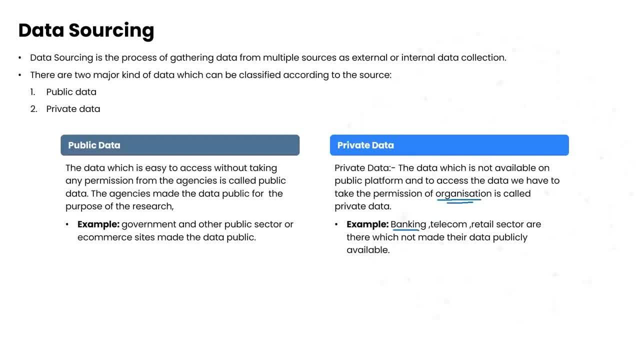 DBA team, which is your database administration team, to help them give you access for the data. Once they give you the access to the data, you can either download it or create a connector to use the data for your analysis process, But depending on the use case that you are trying to solve. 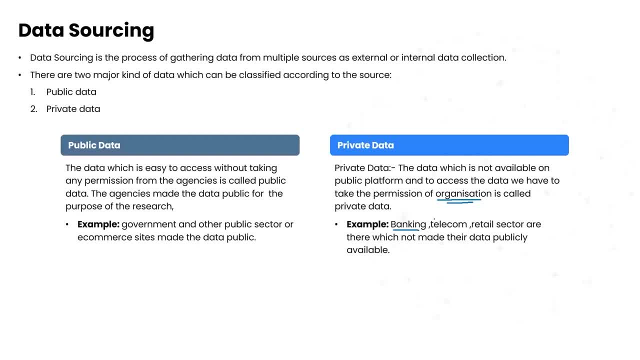 you have to choose your data source wisely. If I also talk about one of the scenarios talking about different companies, There are different types of companies, One of them being MNCs, which are your multinational companies Most likely when you are working as a data analyst or as a data scientist in. 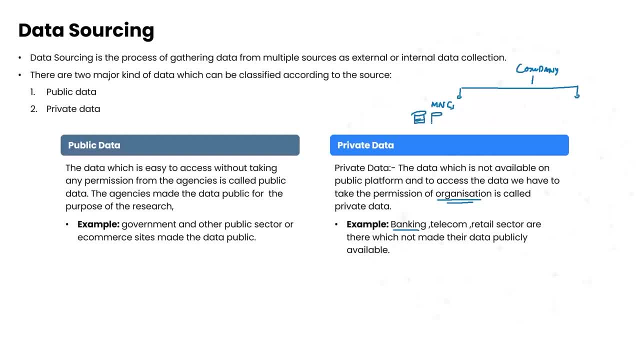 an MNC. In an MNC, there could be multiple databases that the company must be handling. Based on the type of data you need, you need to go and talk to each of these database administrators. They can give you access to the data. Once you get access to the data, then you can start. 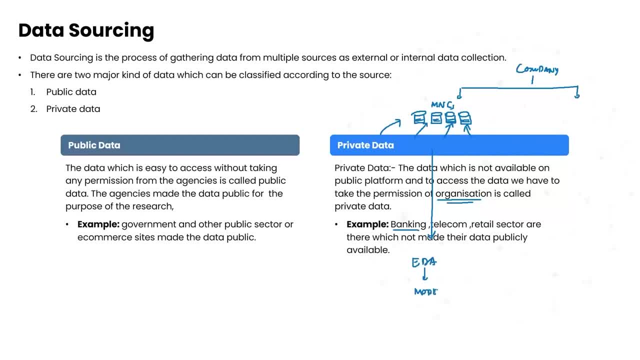 working on your EDA and then work on the model building part. If you are working for a mid-level company, again, mid-level companies might not have huge databases like MNCs, but still they would be having some databases. Again, the process is same: You go ahead, take access. 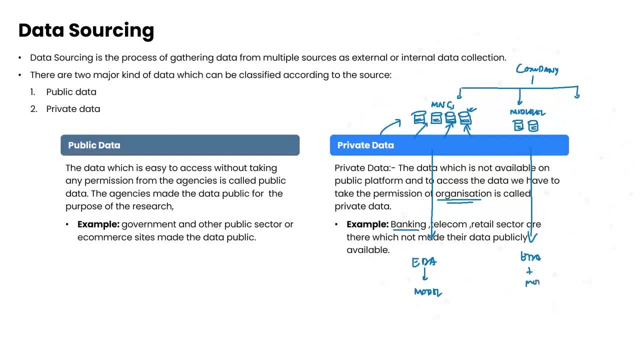 and then start working on EDA or model building. How to start working on EDA In small level companies or in startups? there are again further two steps. One is a startup is a mid-level startup. Then again you have to follow the same technique like this: If 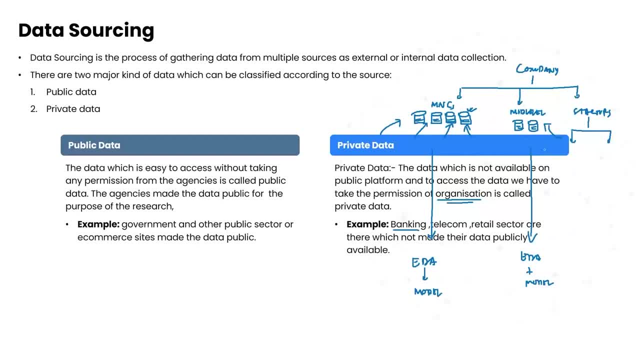 the startup has a database, go ahead and get access to the database and start working If the startup is completely new. in that case, there are two further scenarios. One is the startup has a client and one the startup has no client. How to start working on EDA. 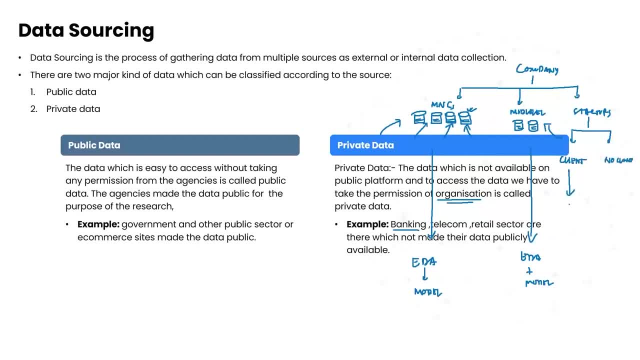 If the startup has a client, there is a possibility that the data must be taken from the client itself and then you can perform your EDA and model building part. And if you don't have a client, then you have to get help of the public data to either do some web scraping. 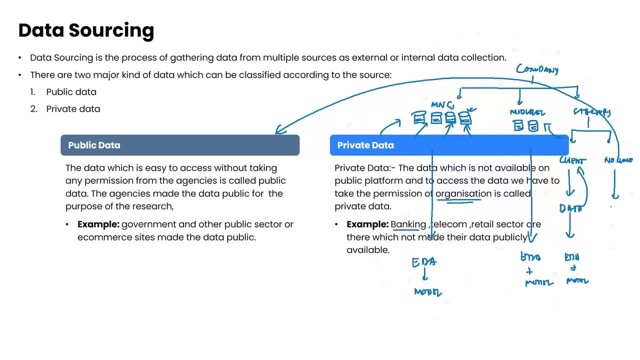 technique, or get some data from some government or some open public sector websites and then start working on your model building or model building How to start working on EDA. You have to get the data for the EDA process. So, depending on the type of company you are, 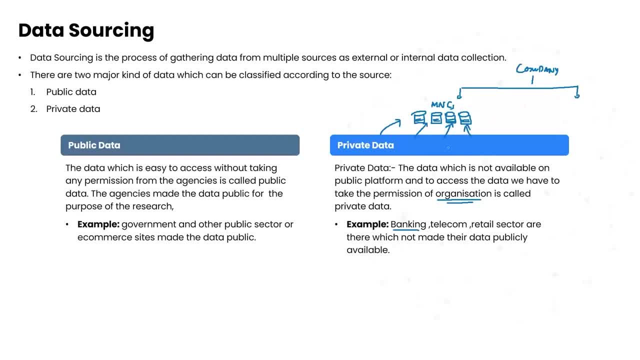 each of these database administrators so that they can give you access to the data. once you get access to the data, then you can start working on your eda and then work on the model building part. if you are working for a mid-level company- again, mid-level companies might not have huge databases like mncs, but still they would be. 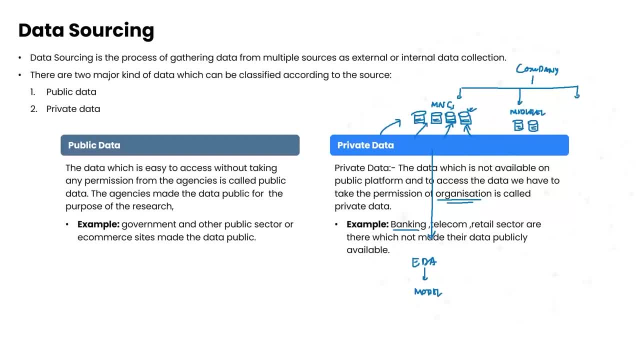 having some databases. again, the process is same. you go ahead, take access and then start working on ed or model building in small level companies or in startups. there are again further two steps. one is a startup, is a mid-level startup. then again you have to follow the same technique, like this: 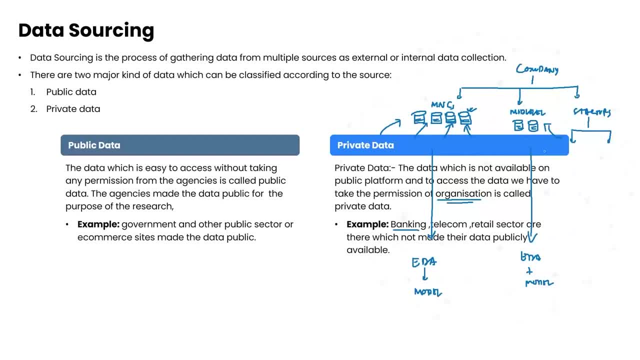 if the startup has a database, go ahead and get access to the database and start working if the startup is completely new. in that case there are two further scenarios. one is the startup has a client and one, the startup has no client. if the startup has a client, there is a possibility. 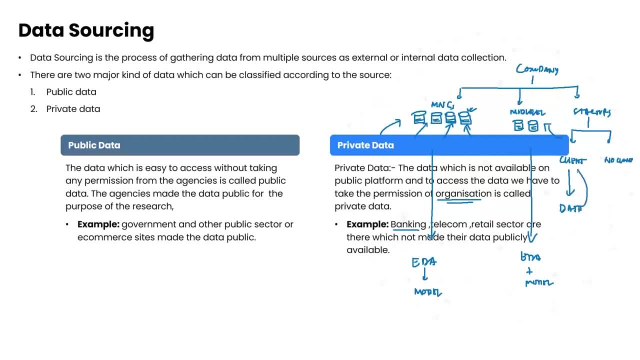 that the data must be taken from the client itself and then you can perform your eda and model building part. and if you don't have a client, then you have to get help of the public data to either do some web scraping technique or get some data from some government or some open public sector websites. 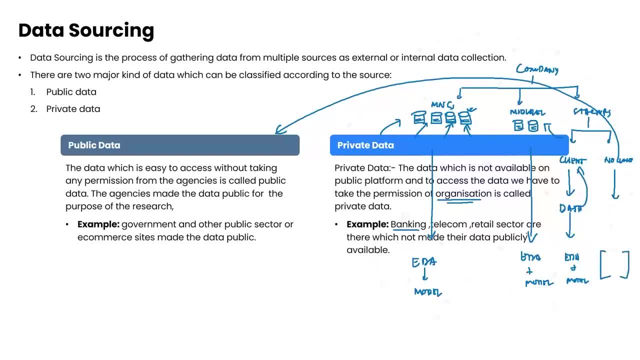 and then start working on your model building or the ada process. so, depending on the type of company you are using you are working, depending on the type of use case that you are handling, you need to understand what should be your data source and, based on that, you should get the data for the 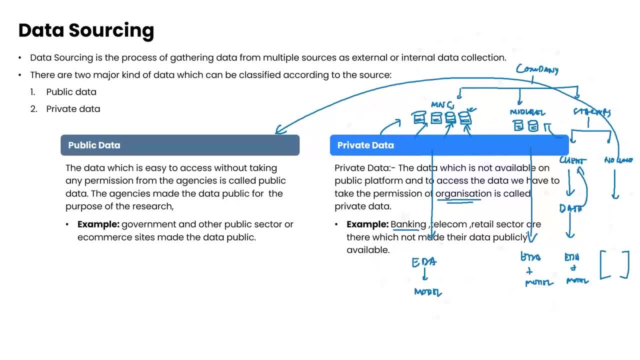 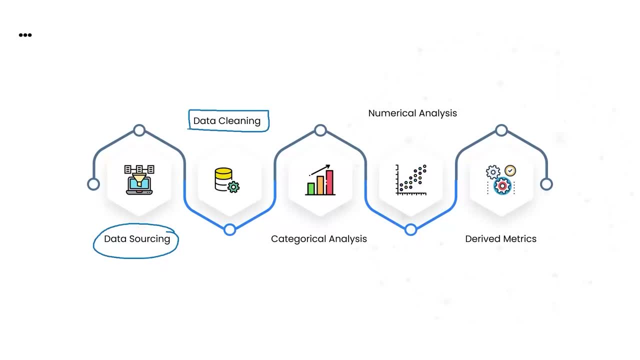 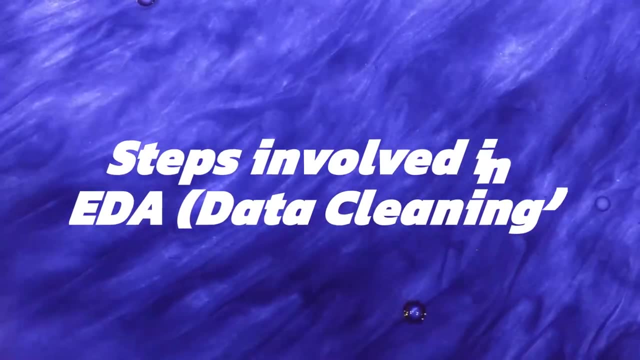 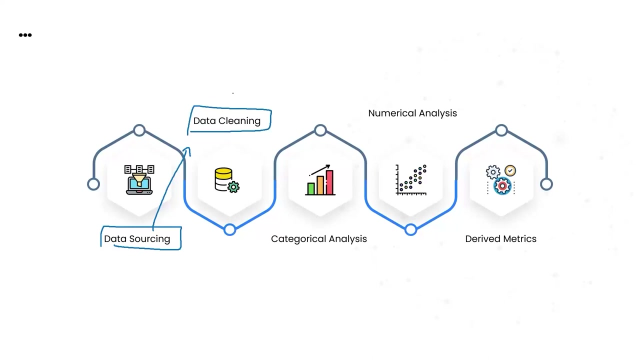 next processes. after data sourcing comes the next process, which is basically your data cleaning process, which will be explained in the next video. after data sourcing comes your data cleaning. once you get the data, then comes your data cleaning process, which basically takes the unclean data and gives you a clean data. what do you mean by data cleaning? after collecting the 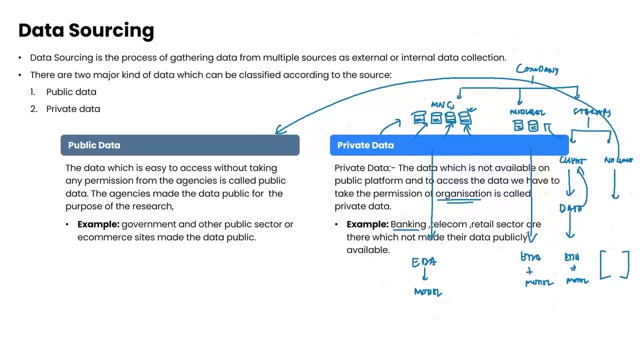 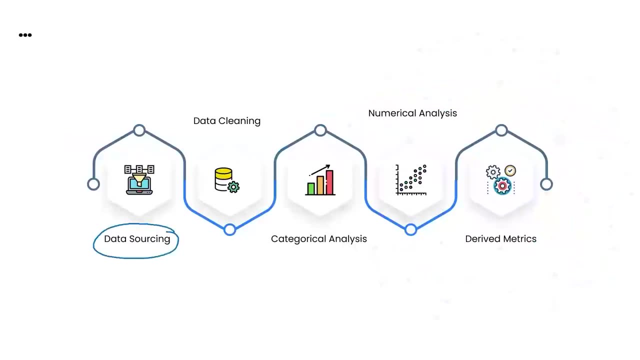 using you are working, depending on the type of use case that you are handling, you need to understand what should be your data source And, based on that, you should get the data for the next processes. After data sourcing comes the next process, which is basically your data cleaning process. 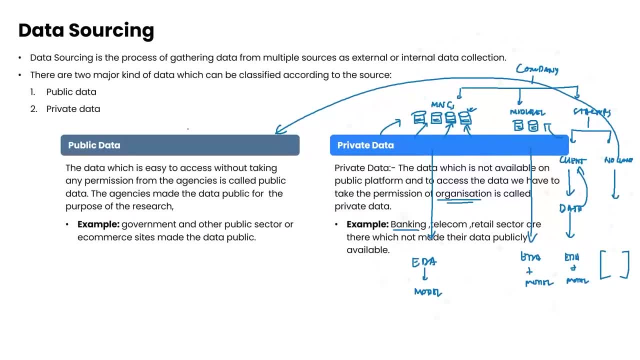 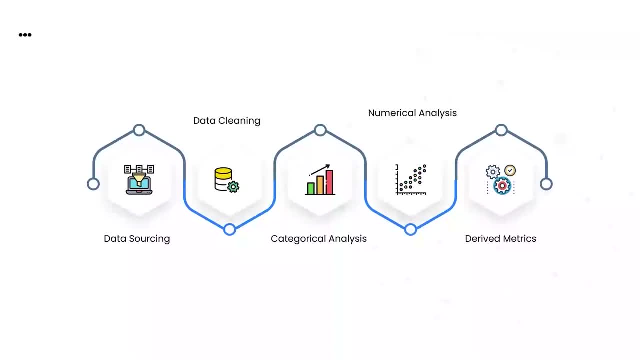 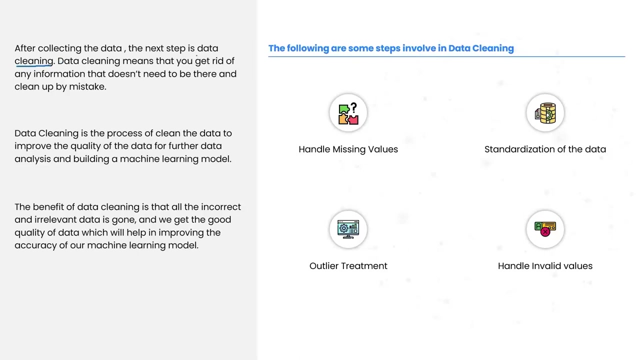 which will be explained in the next video. after data sourcing comes your data cleaning. once you get the data, then comes your data cleaning process, which basically takes the unclean data and gives you a clean data. what do you mean by data cleaning? after collecting the data, the next step is data cleaning. data cleaning means that. 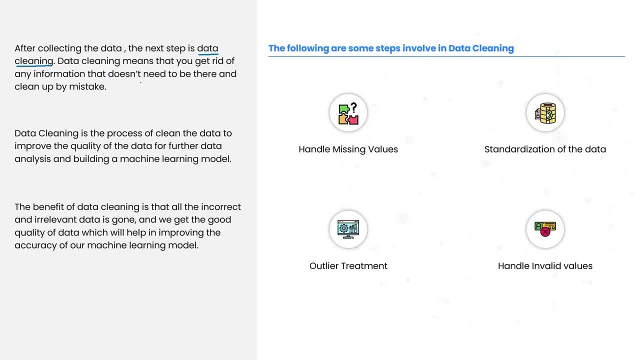 you get rid of any information that does not need to be there and clean up data cleaning is the process of cleaning the data to improve the quality of the data, for further data analysis and building a machine learning model. initially you get the data, then you clean the data. 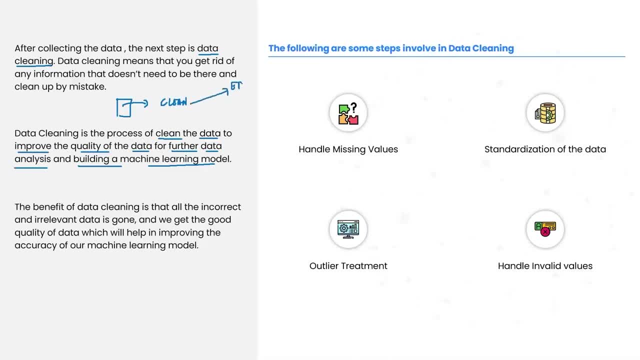 and once the data is clean, either you go for eda or you go for the machine learning model building part. sometimes you go through eda and then go to the machine learning, and sometimes you directly go to the machine learning. but whatever you do- either eda or this- this is a prerequisite and one of the important steps. 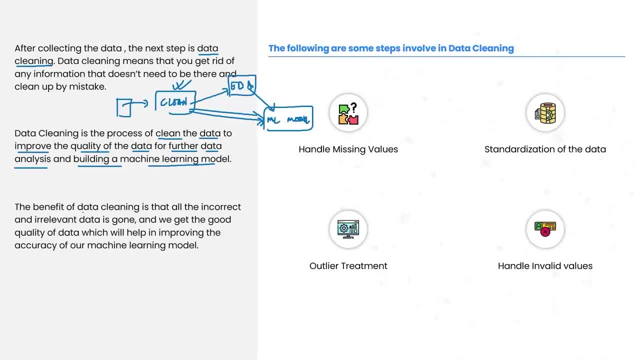 data cleaning is very important. the benefit of data cleaning is that all the incorrect and irrelevant data is gone and we get the good quality of data, which will help in improving the accuracy of our predictive models or machine learning models. what are the major steps that we involve in the data cleaning process? the major steps are handling missing values, standardization. 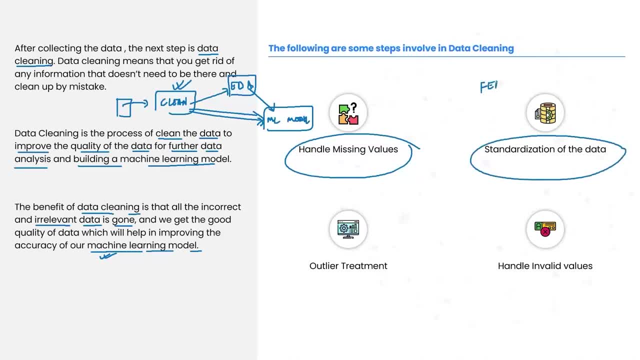 of the data, which, in simple terms, we call it as feature scaling technique. we also have outlier treatment and handling values: handling invalid data types or handling invalid values. most time, once we have the data, we usually have missing values. missing values could be because of multiple reasons. it could 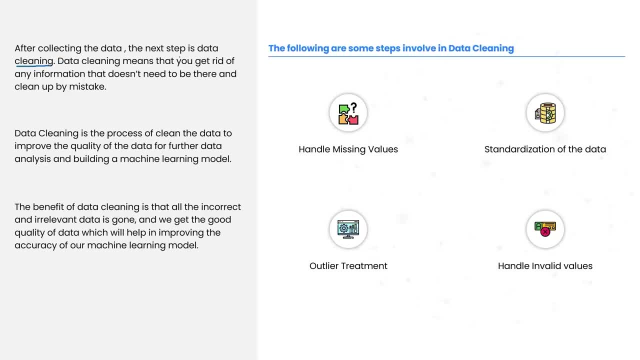 data. the next step is data cleaning. data cleaning means that you get rid of any information that does not need to be there and clean up. data cleaning is the process of cleaning the data to improve the quality of the data for further data analysis and building a machine learning model. initially, you get the 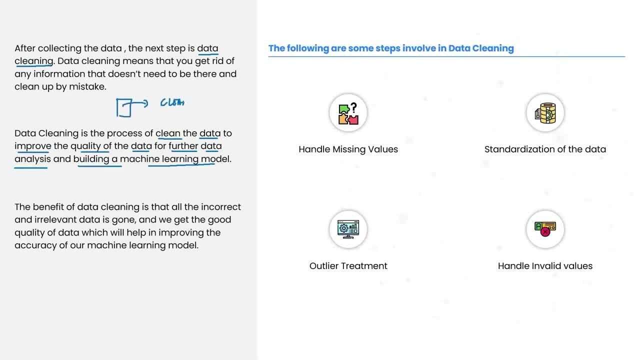 data, then you clean the data. and once the data is clean, either you go for eda or you go for the machine learning model building part. sometimes you go through eda and then go to the machine learning and sometimes you directly go to the machine learning. but whatever you do, either eda, 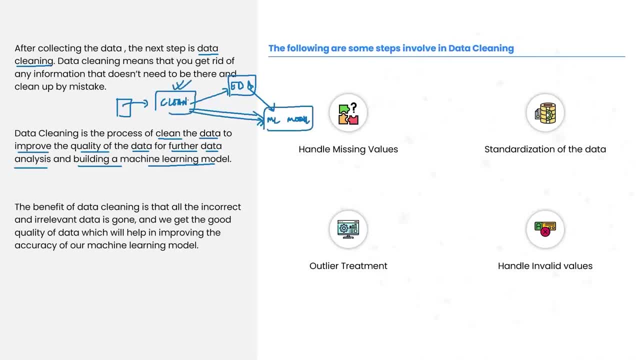 or this. this is a prerequisite and one of the important steps. data cleaning is very important. the benefit of data cleaning is that all the incorrect and irrelevant data is gone and we get the good quality of data which will help in improving the accuracy of our predictive models. 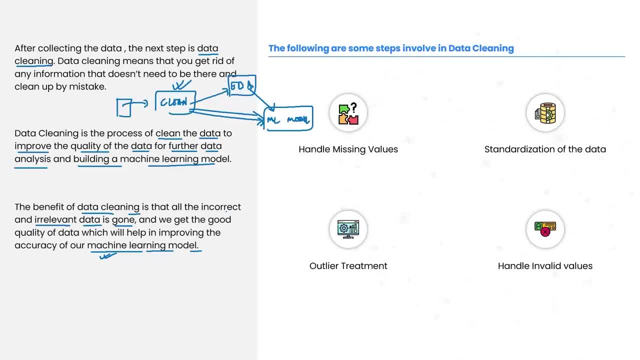 or machine learning models. what are the major steps that we involve in the data cleaning process? you? the major steps are: handling missing values, standardization of the data, which, in simple terms, we call it as feature scaling technique. we also have outlier treatment and handling invalid data types or handling invalid values. 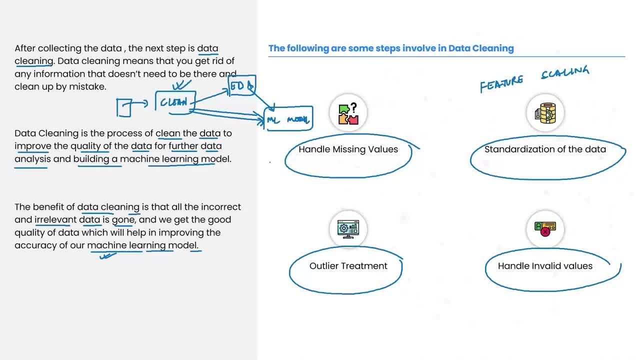 most time, once we have the data, we usually have missing values. missing values could be because of multiple reasons. it could be actually be missing in the database or the data source, or it could be a missing value because of the scripts. maybe you have written down a script to get data from the database and while that process happens, due to 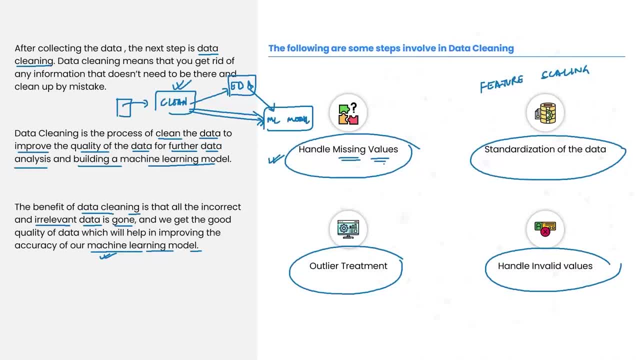 some reasons, you have some missing values. the reasons of having missing values are multiple, but in order to analyze it, in order to do some further activities, we always have to impute these missing values. either we delete those records or we impute them. we will be learning through each. 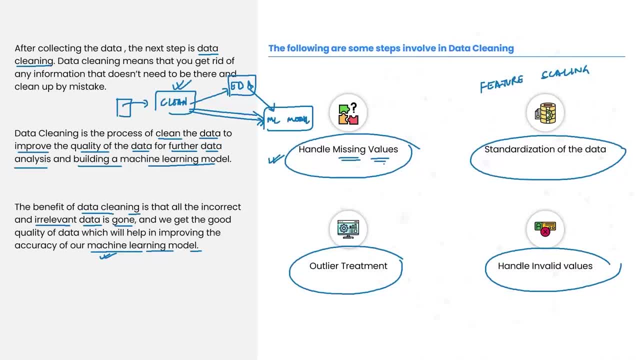 be actually be missing in the database or the data source, or it could be a missing value because of the scripts. maybe you have written down a script to get data from the database and while that process happens, due to some reason, you have some missing values. the reasons of having missing values are multiple, but in order to analyze 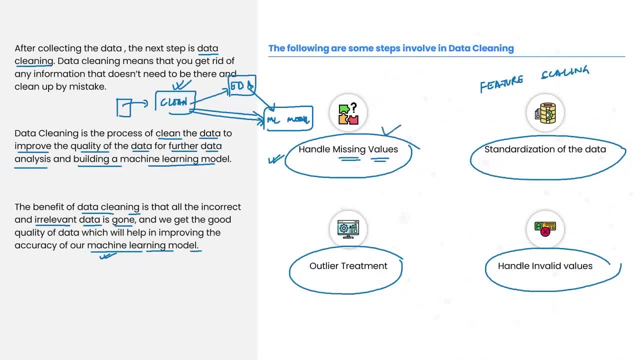 it in order to do some further activities. we always have to impute these missing values. either we delete those records or we impute them. we will be learning through each of these processes as part of separate videos. after missing values, we also have a technique called as feature scaling. 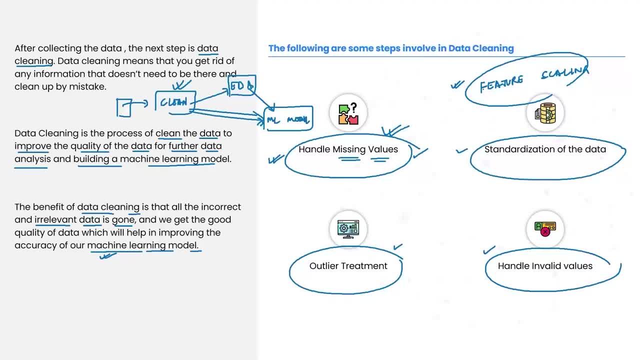 again, feature scaling is an important technique. we will be studying about feature scaling, which basically has standardization and normalization- two different techniques- and most of the data that we deal with definitely have outliers in it. what do you mean by outliers? in simple terms, if most of your data points are within this range, 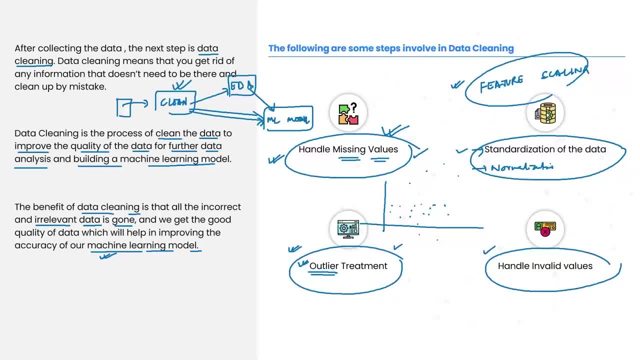 and some of the data points are scattered way above or way below then the rest of the data points. these data points are called as outliers. sometimes we have to treat outliers- either we get rid of them or we deal with it- and sometimes we also have invalid values. invalid values like, let's say, you are dealing with h. 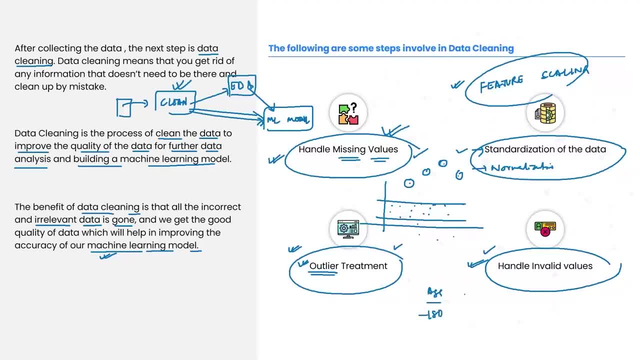 there is an age like 180 minus 180, or there is some columns where you have some special characters. you have to deal with these situations. sometimes you'll read: at least: you have to deal with these situations. think what's happening in this case to connect that value to the public business kind of way. now, 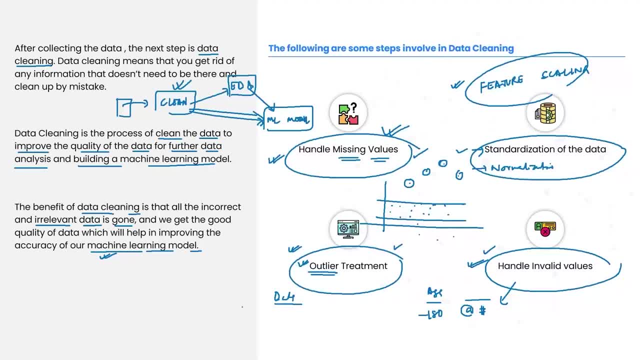 have a date column, but the date you have is not in a date format. so there are multiple scenarios that could occur here and we have to deal with it as part of the data cleaning process. in the next video we shall be talking about each one of these steps in detailed manner. see in the 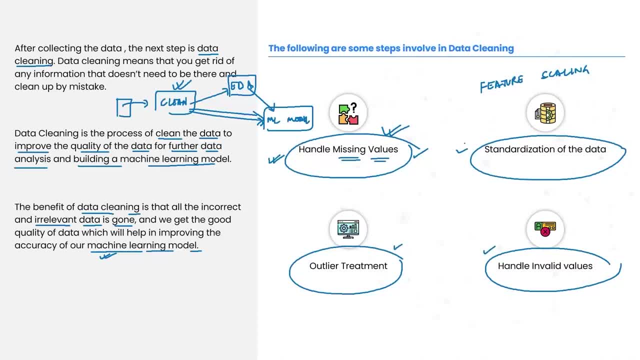 of these processes as part of separate videos. after missing values, we also have a technique called as feature scaling. again, feature scaling is an important technique. we will be studying about feature scaling, which basically has standardization and normalization- two different techniques- and most of the data that we deal with definitely have outliers in it. what do you mean by? 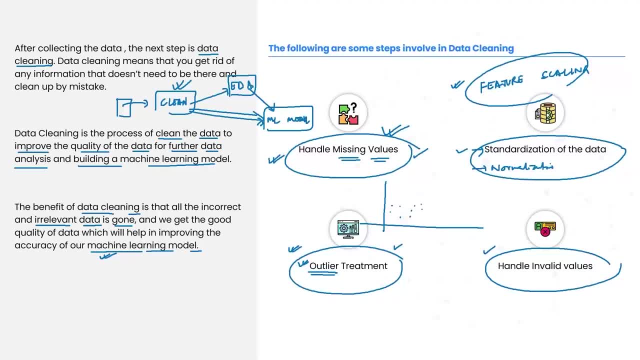 outliers. in simple terms, if most of your data points are within this range and some of the data points are scattered way above or way below, then the rest of the data points. these data points are called as outliers. sometimes we have to treat outliers: either we get rid of them or we deal with it, and sometimes we 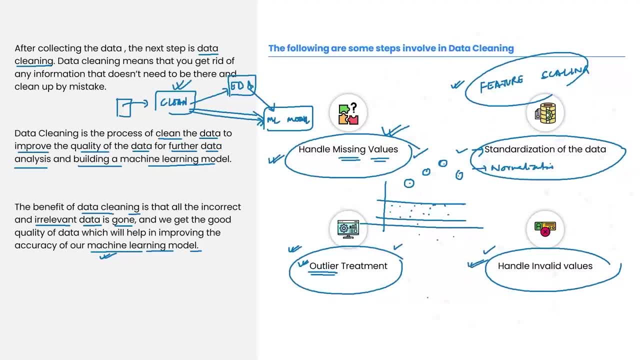 also have invalid values. invalid values like, let's say, you are dealing with age. there is a age like one eight minus 180, or there is some columns where you have some special characters. you have to deal with these situations. sometimes you have a date column, but the date you have is: 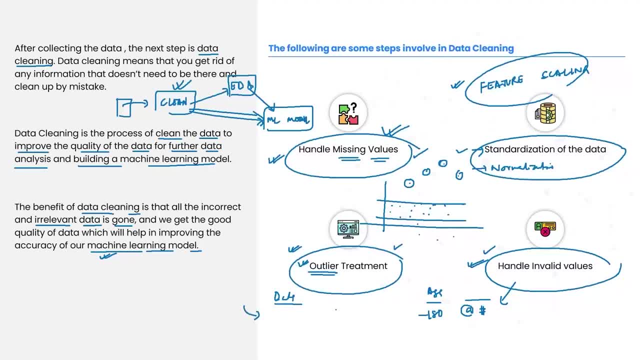 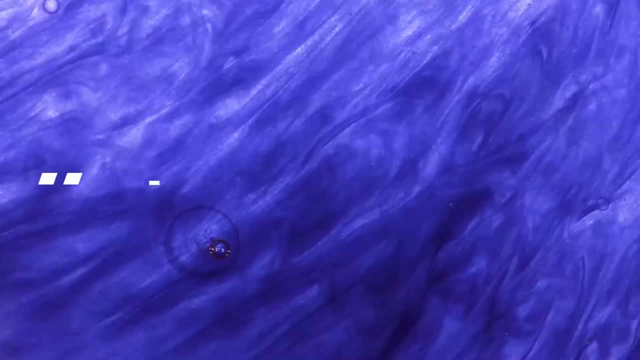 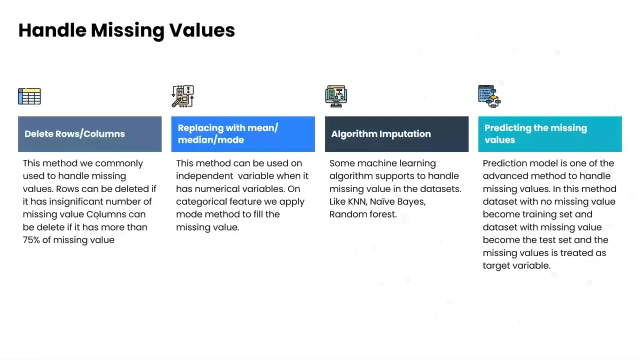 not in a date format. so there are multiple scenarios that could occur here and we have to deal with it as part of the data cleaning process. in the next video, we shall be talking about each one of these steps in detailed manner. see you in the next video. in this video, we shall be talking 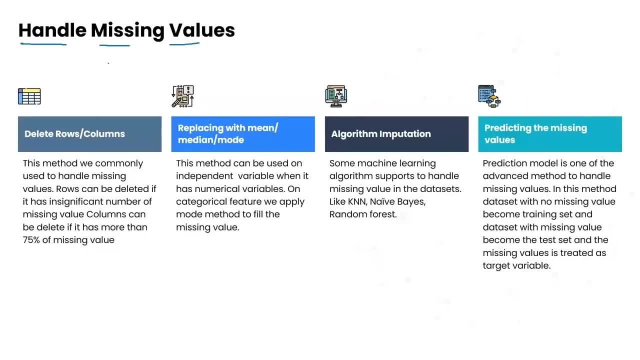 about how to handle missing value issue when it comes to the data analysis part. in the data cleaning part, missing values are one of the most important common issues. how do we get rid of them? let's try to understand theoretically and going forward. we will also show you how to deal with missing value problem in python. there are multiple 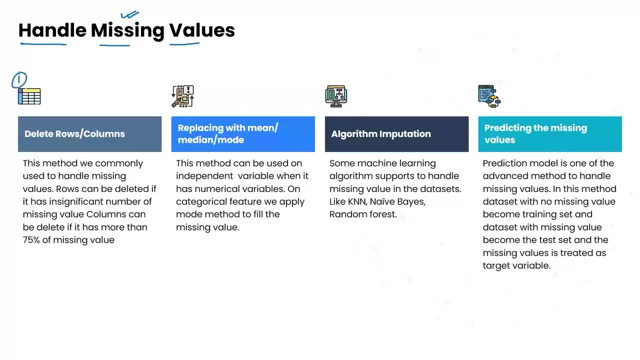 techniques to handle missing values. the first technique is: either you delete the rows or columns. this method is commonly used to handle missing values. rows can be deleted if it has insignificant number of missing value. column can be deleted if it has more than 75 percent of missing values. now there is no thumb. 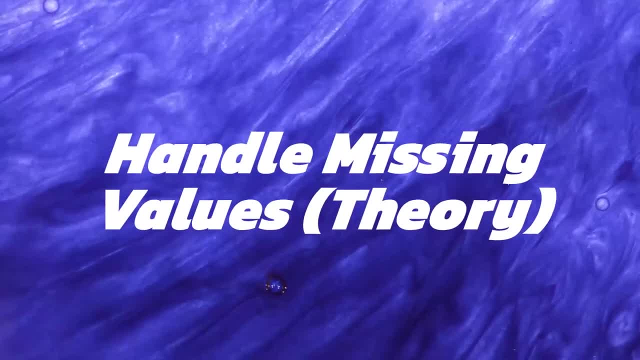 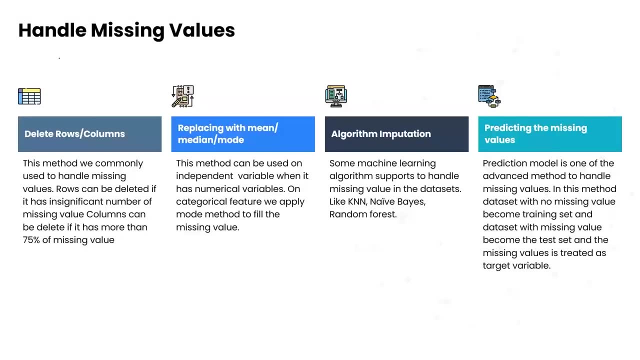 next video. in this video we shall be talking about how to handle missing value issue. when it comes to the data analysis part. in the data cleaning part, missing values are one of the most important common issues. how do we get rid of them? let's try to understand theoretically and going forward. we 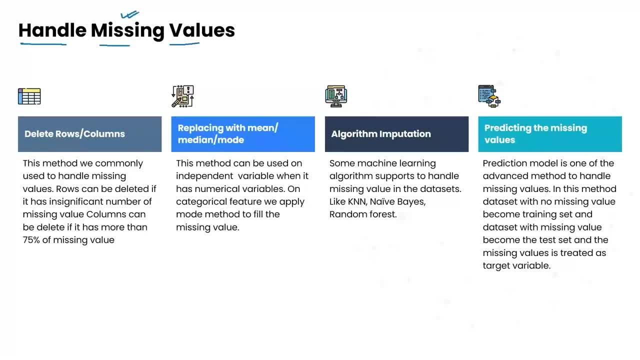 will also show you how to handle missing value issues and how to handle missing value issues, how to deal with missing value problem in python. there are multiple techniques to handle missing values. the first technique is either you delete the rows or columns. this method we commonly use to handle missing values. rows can be deleted if it has insignificant number of missing value. 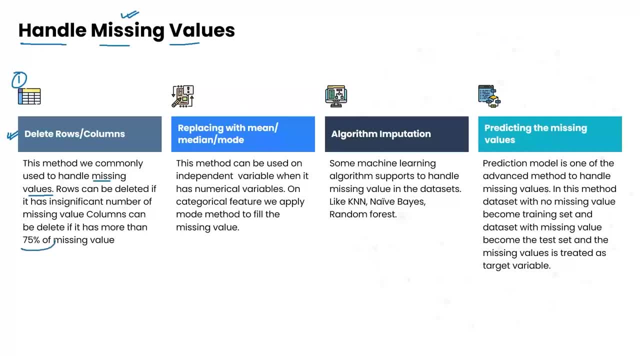 column can be deleted if it has more than 75 percent of missing values. now there is no thumb rule on whether you should delete rows or columns, but there are some techniques. let's say you have data now imagine one of the columns is there which has no dependency on any other column. 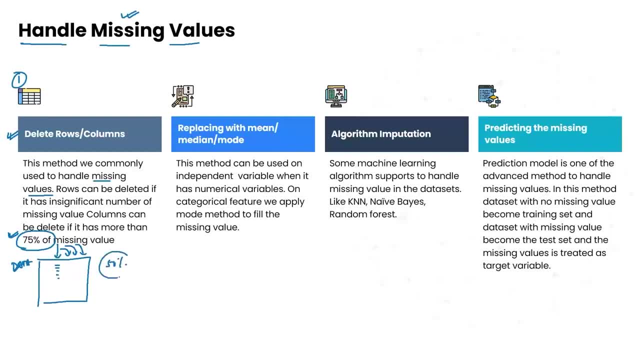 and this column has already like 50 percent of missing values. there is no need of impugning this column. it's better to delete that column or else, if you are dealing with data and some of these records are having missing values, some of the rows are missing, maybe just two percent or 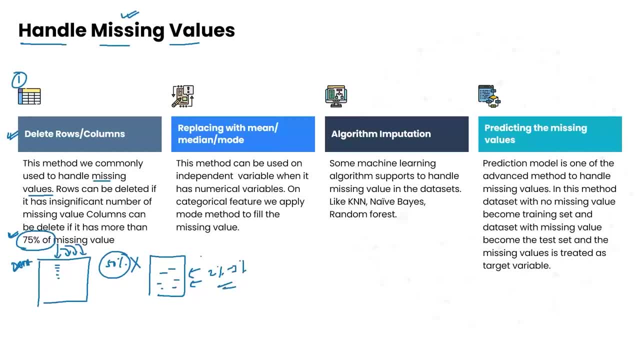 three percent of the data are missing. now, in this case, either you impute them or you delete them because it's too less. comparing to a 10 000 records data set, two percent is nothing, one percent is almost uh, one percent is almost hundred and two percent is almost 200 records. right so 200 records, even if you delete them. 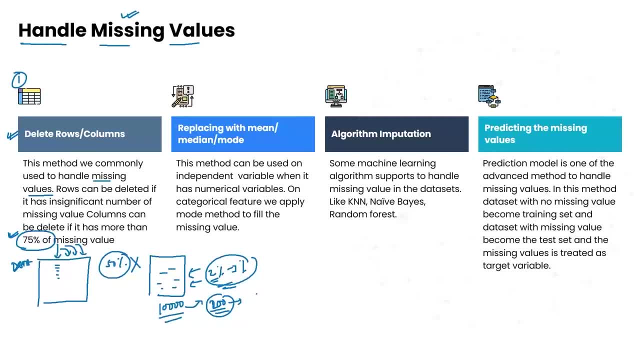 of course, you are missing out on information. ultimately, you will be having 9 800 records, but it all depends whether you are imputing it or deleting it. in certain scenarios we delete it. in certain scenarios we impute it. if it comes to imputing, that means replacing the null values. 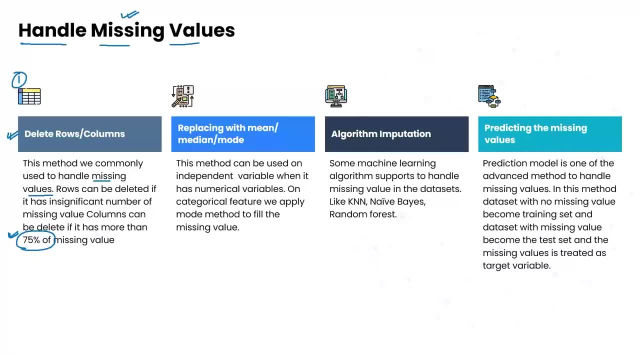 rule on whether you should delete rows or columns, but there are some techniques. let's say you have data. now imagine one of the columns is there which has no dependency on any other column. it is like 50 percent of missing values. there is no need for imput. this column is better. 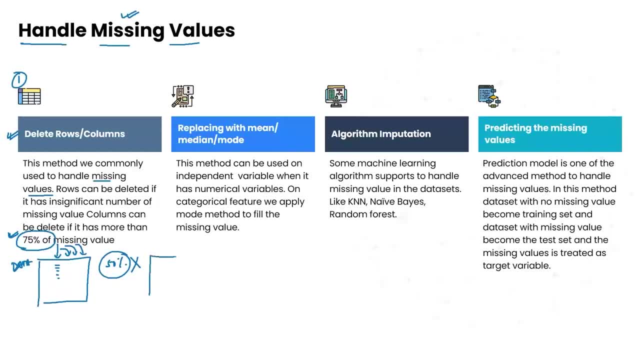 to delete that column if you are dealing with data, that's, the rolls are missing etwas ele. In this case it'll be deleted because it's Copenhere comparing to later this records data set. two percent is nothing, one percent is almost uh. one percent is almost 100. 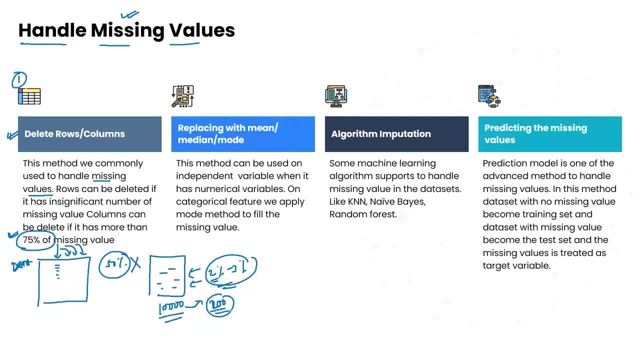 and two percent is almost 200 records. right, so 200 records. even if you delete them, of course, you are missing out on information. ultimately, you will be having 9800 records, but it all depends whether you are imputing it or deleting it. in certain scenarios we delete it in certain. 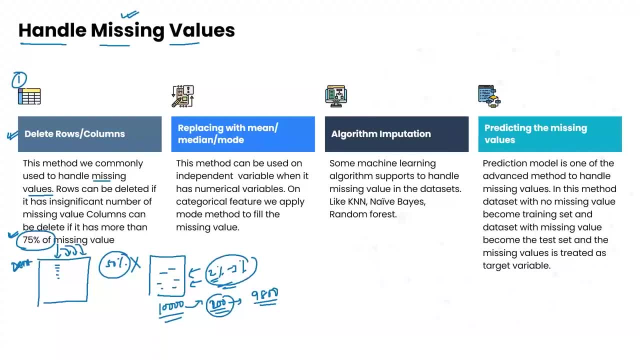 scenarios, we impute it. if it comes to imputing, that means replacing the null values. what is the right way to replace? sometimes we go with some arbitrary numbers. now, for example, we are dealing with a column called as h. sometimes we randomly fill a random value. let's say 25, let's try to. 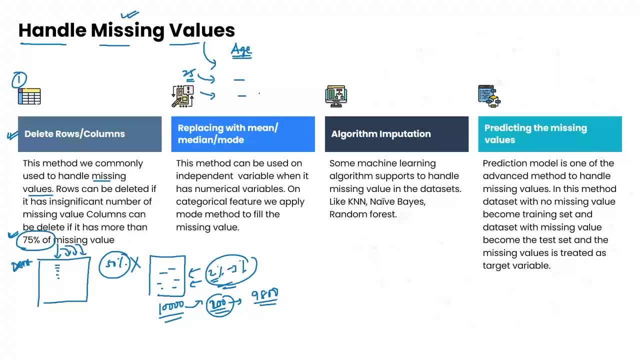 fill 25 in all the missing values that we have. that technique also works, but is this the right technique? no, i would say it is one of the idiotic techniques to fill a random number into age. a better technique is to use the mean or median value, for example. age has a certain mean. 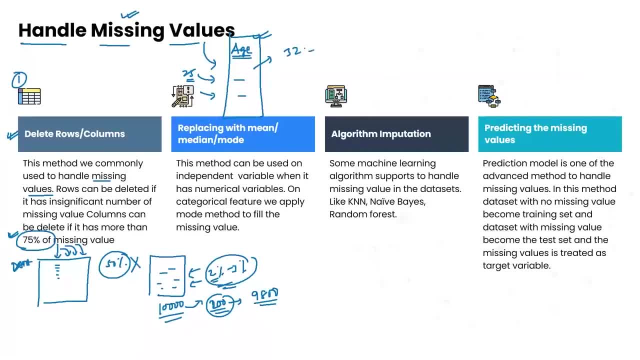 for all the values that it has. let's say, the mean is 32 point something. so if you impute the records with the mean value, that is 32 makes more sense than imputing a random number. similarly, in certain scenarios we also impute the median value. 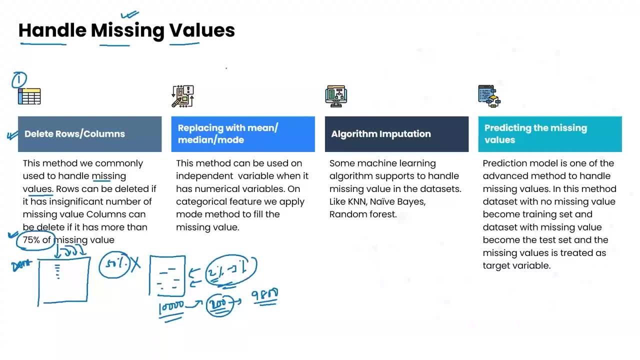 what is the right way to replace? sometimes we go with some arbitrary numbers. now, for example, we are dealing with a column called as age. sometimes we randomly fill a random value. let's say 25. let's try to fill 25 in all the missing values that we have. that technique also works, but is this the right technique? 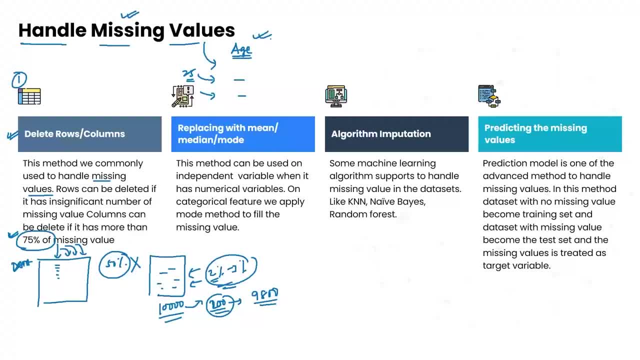 no, i would say it is one of the idiotic techniques to fill a random number into age. a better technique is to use the mean or median value, for example. age has a certain mean for all the values that it has. let's say the mean is 32 point something. so if you impute the records with the mean value, 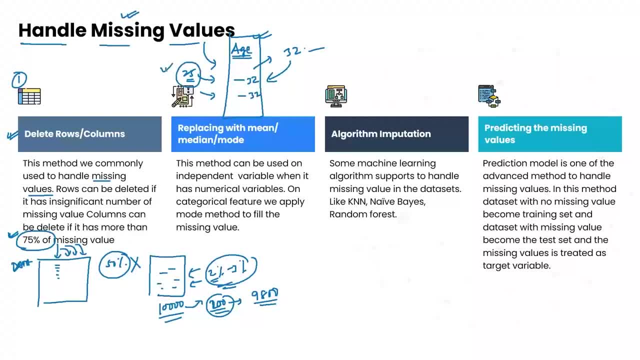 that is 32, makes more sense than imputing a random number. similarly, in certain scenarios we also impute the median value. let's say the median value is 31. you impute them. mode is mostly used for categorical data. which of these techniques is good? mean or median or mode. 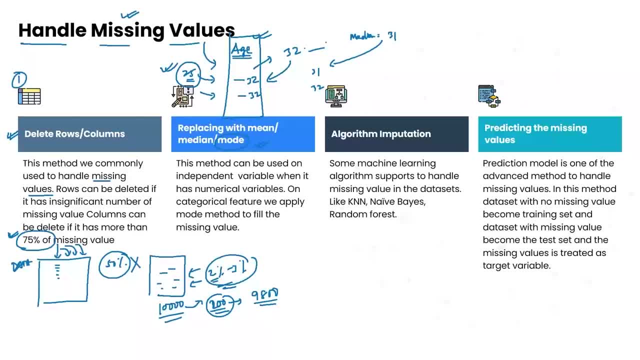 it all depends, at least for the process of ada. you can impute any of these numbers. if you are building a machine learning model or a predictive model, in that case you are dealing with this missing value problem. in that case there is no right or wrong. you should always do a hit and 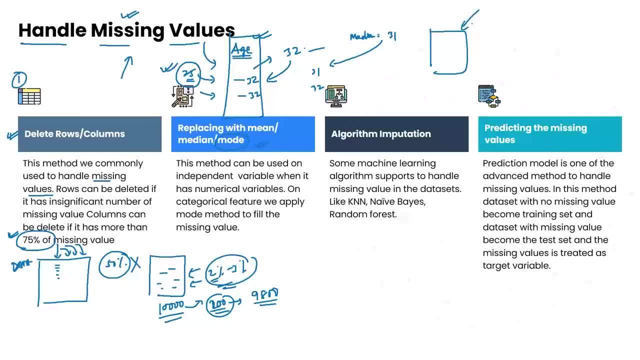 run. that means you have data. let's say the age column you are imputing with mean. go ahead and build the model and check the model's accuracy. let's say the model's accuracy is 80 percent. again come back, impute it using median. again build the model and check if you see an increase. 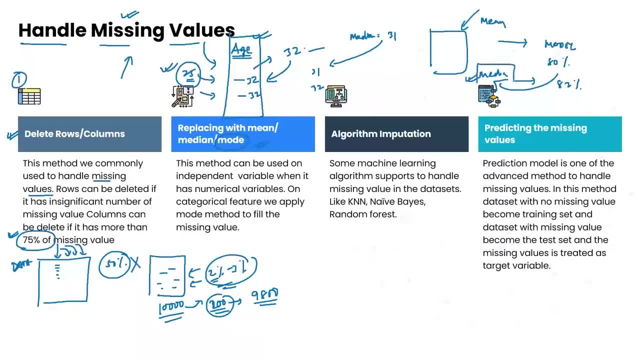 in accuracy. probably you can finalize that median is a better technique in certain scenarios. we also go for algorithmic imputation. that means when your ultimate goal is to build a predictive model or a machine learning model, some machine learning models or some machine learning algorithms, supports to handle missing values. that means they do not care about the missing values. 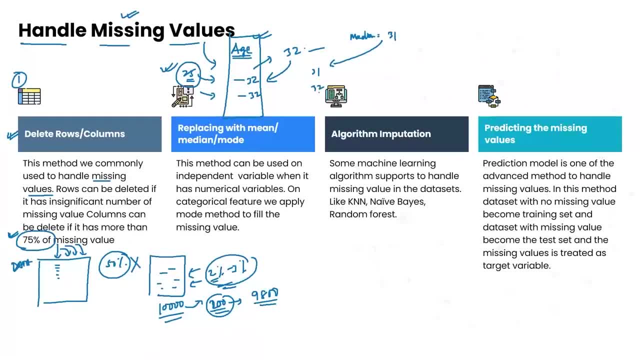 let's say the median value is 31. you impute them. mode is mostly used for categorical data. which of these techniques is good? mean or median or mode? it all depends, at least for the process of ada. you can impute any of these numbers if you are building a machine learning model or a. 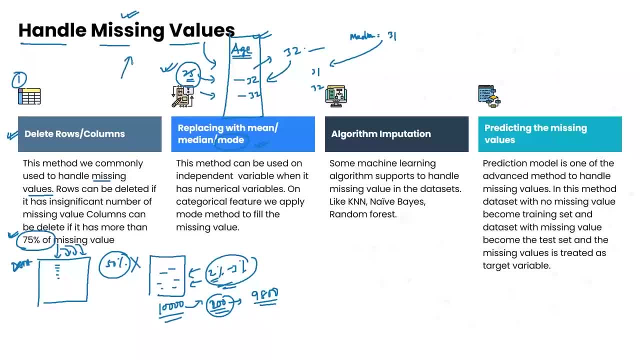 model. in that case, you are dealing with this missing value problem. in that case there is no right or wrong. you should always do a hit and try. that means you have data, let's say the age column you are imputing with. mean, go ahead and build the model and check the model's accuracy. 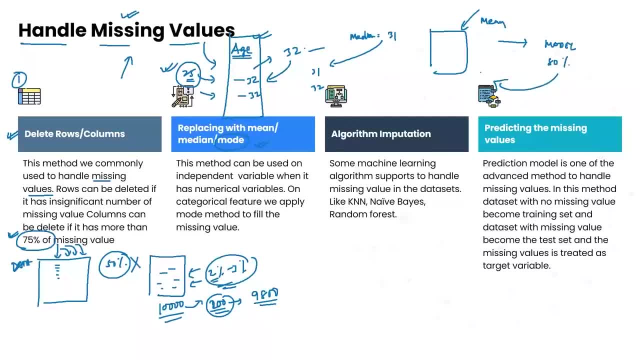 let's say the model's accuracy is 80 percent. again come back, impute it using median. again build the model and check. if you see an increase in accuracy. probably you can finalize that median is a better technique. in certain scenarios we also go for algorithmic imputation. that means when your 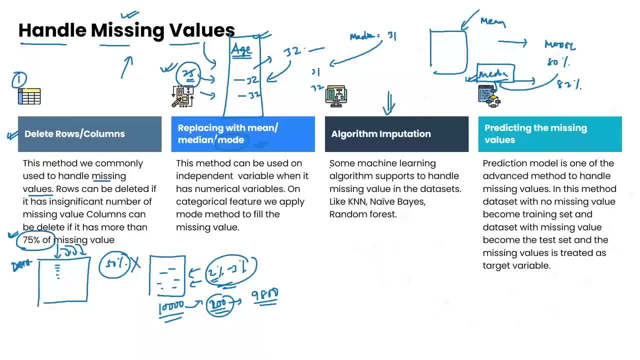 ultimate goal is to build a predictive model or a machine learning model, some machine learning models or some machine learning algorithms supports to handle missing values. that means they do not care about the missing values. even if you have missing values, you just call these algorithms and they will be able to handle that internally. so if your final goal is to create a model, create a. 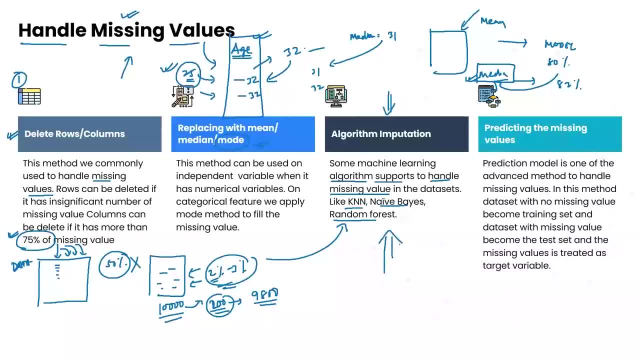 predictive model. in that case you can also go for this algorithmic imputation, but, as in this case, we are only focused on the eda part, on the analysis part, we will not be considering this particular technique. we will also be only be considering these techniques like mean, median and mode. there are also some advanced techniques to 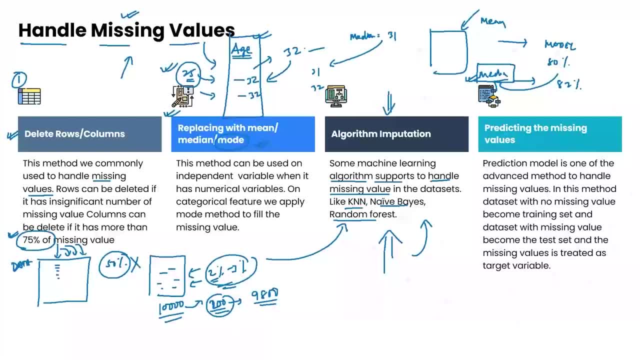 handle missing values. some of the advanced techniques are predicting the missing values using some time series forecasting. problem prediction model is one of the advanced method to handle missing values. in this method, data set with no missing value becomes training data set and data set with missing values becomes the test data set and the missing 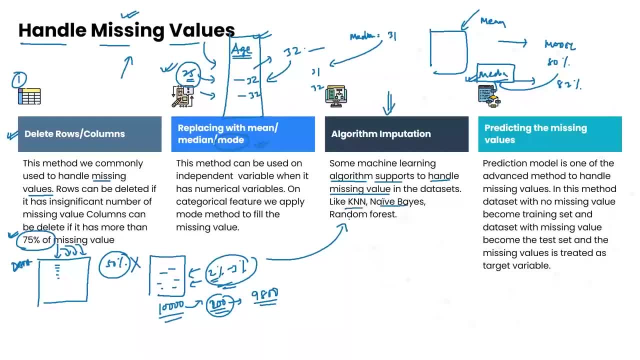 even if you have missing values, you just call these algorithms and they will be able to handle that internally. so if your final goal is to create a model, create a predictive model, in that case you can also go for this algorithmic imputation. but, as in this case, we are only focused on the eda part, on the analysis part we will not. 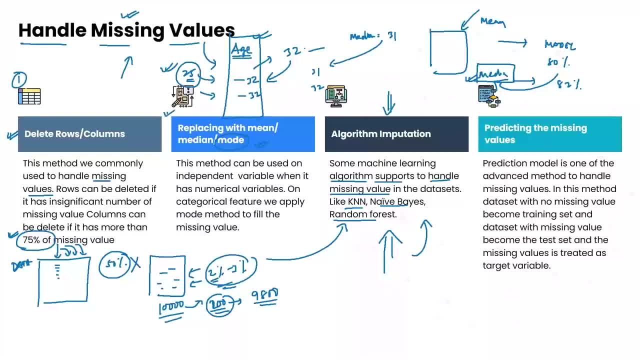 be considering this particular technique. we will also be only be considering these techniques like mean, median and mode. there are also some advanced techniques to handle missing values. some of the advanced techniques are predicting the missing values using some time series. forecasting. problem prediction model is one of the advanced method. 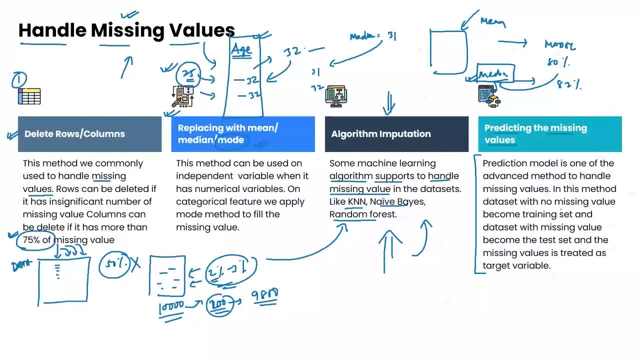 to handle missing values. in this method, data set with no missing value becomes training data set and data set with missing values becomes the test data set and the missing values are treated as target variable. which basically means just imagine you have data and let's say, out of 10 000 records. 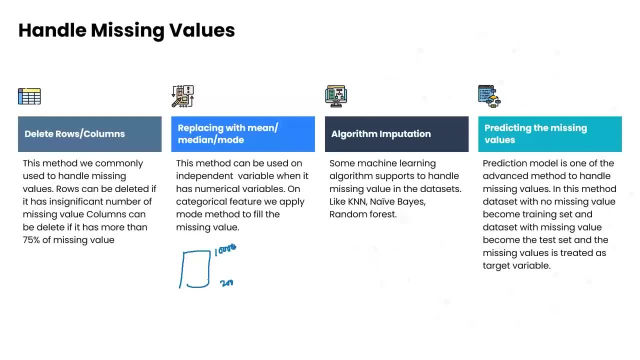 2 000 records or out of 1000 records, 200 are null records for age. then what we do is we usually take those 800 records and try to do prediction for these 200, and once the predict predictions are done, these predicted values are taken into consideration and then you perform your eda. 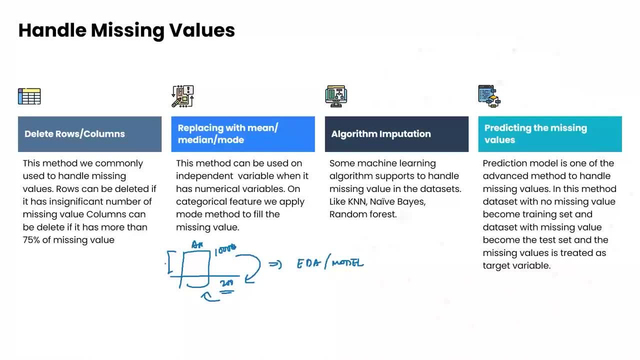 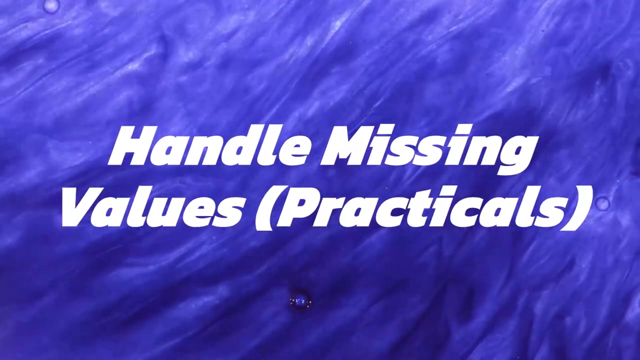 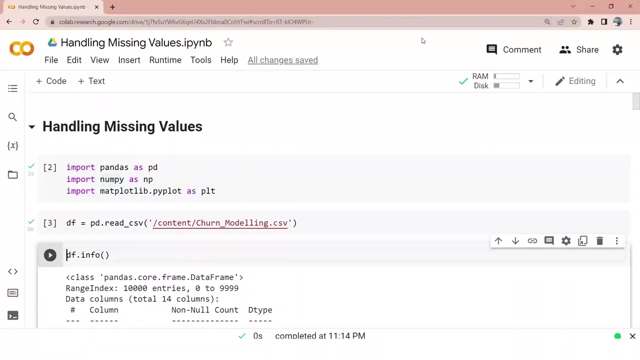 or model build. now, this technique is an advanced technique. you can or you cannot use. it's up to you. particular session on handling missing values. let's go ahead and see the pythonic part and on how to handle missing values using various techniques. jumping on to the python part, jumping on to the practicals part on how do we actually 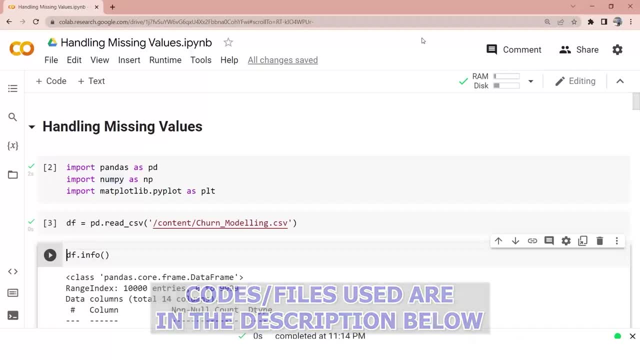 handle missing values in real-time scenario. for this particular exercise, we have a data set called as churn modeling data set. we'll try to quickly see what the data set is all about. we have manually created some of the null values in that particular data set so that we can handle. 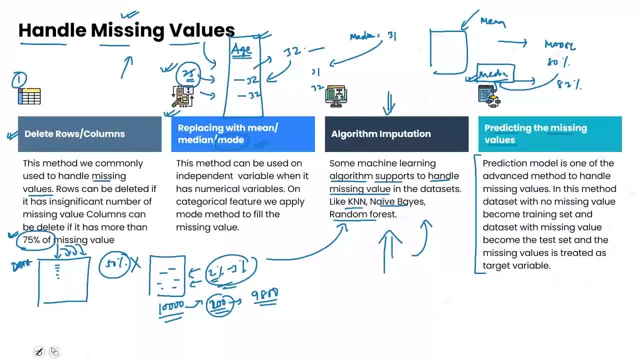 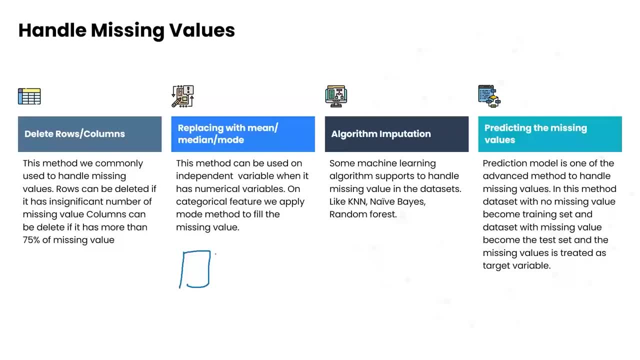 values are treated as target variable. which basically means: just imagine you have data and let's say, out of 10 000 records or out of thousand records, 200 are null records for age. then what we do is we usually take those 800 records and try to do prediction for these 200. 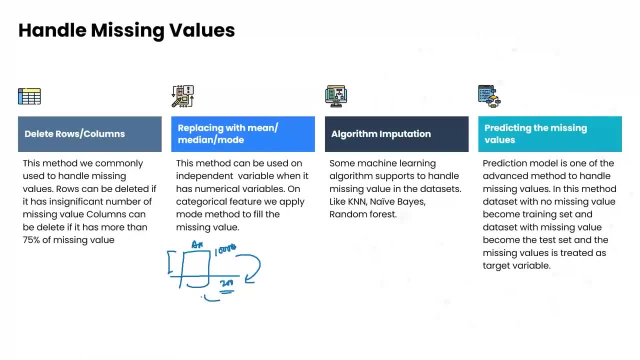 and once the predict predictions are done, these predicted values are taken into consideration and you perform your eda or model build. now this technique is an advanced technique. you can or you cannot use, it's up to you. that's all about this particular session on handling missing values. 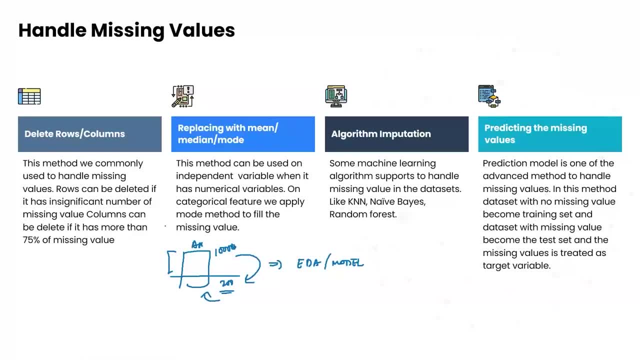 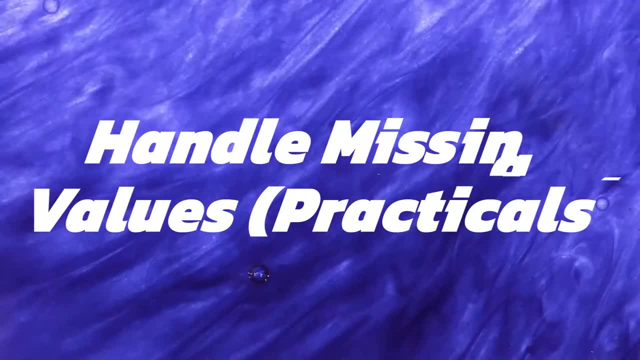 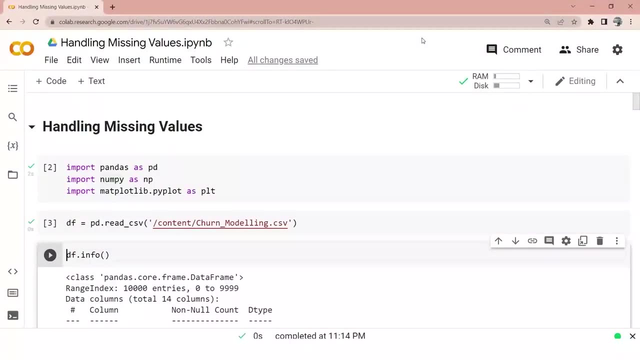 let's go ahead and see the pythonic part and on how to handle missing values using various techniques. so, jumping on to the python part, jumping on to the practical part, on how do we actually handle missing values in real time scenario. for this particular exercise, we have a data set called 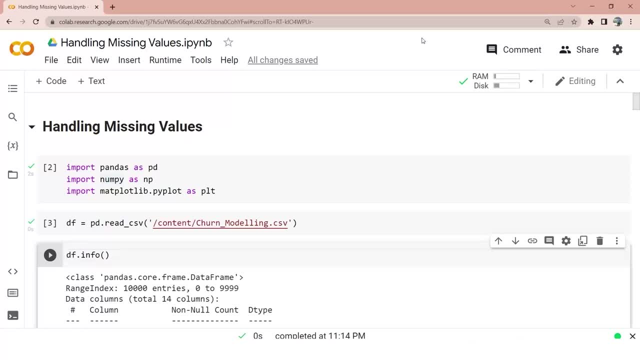 as churn modeling data set. we'll try to quickly see what the data set is all about. we have manually created some of the null values in that particular data set so that we can handle that missing value, and probably i will tell you techniques on what we should do and what we usually do while in this journey of 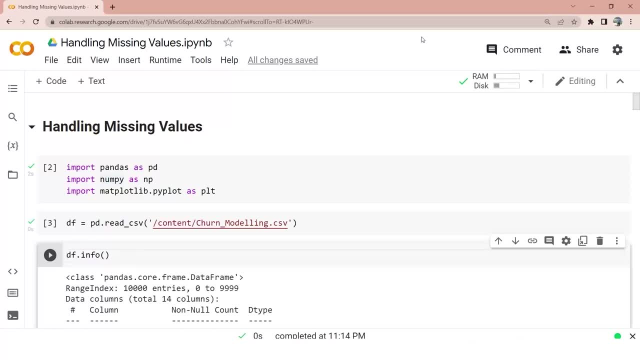 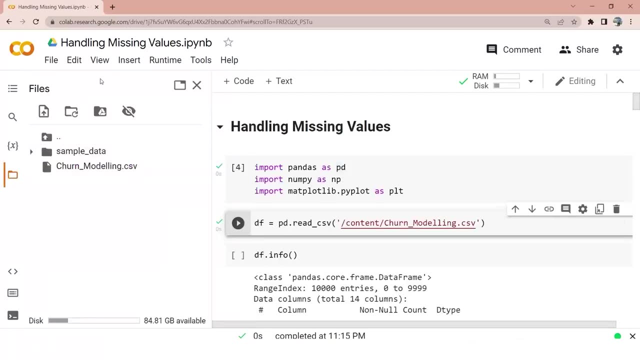 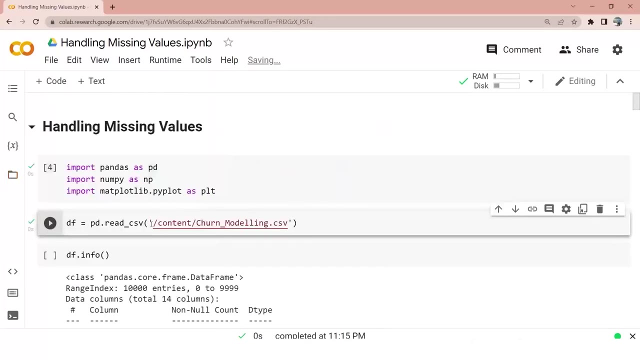 the data cleaning process. so we'll get started by importing all these libraries: pandas, numpy and matplotlib. as you can see, I am using Google collab, so I have just right clicked and uploaded the churn modeling file here, and here I am reading it using slash content: slash the churn modeling file the moment I run my 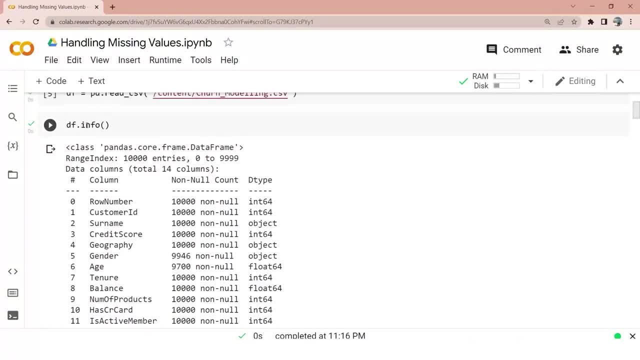 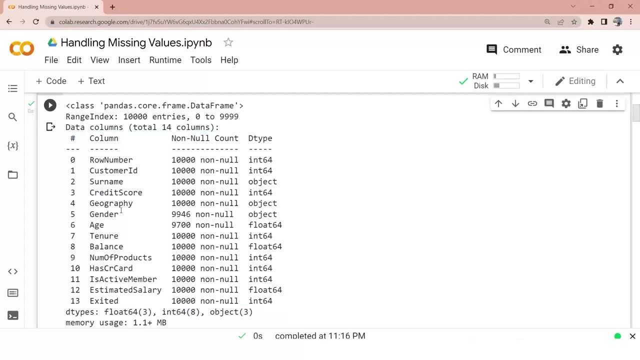 data frame is ready. the first thing that I can do is dot info, which will clearly give me a quick information about the entire data set. we have manually created some null values for these two columns, but you can see it's quite visible. gender: we have fifty four null values and for age: we have almost three hundred. 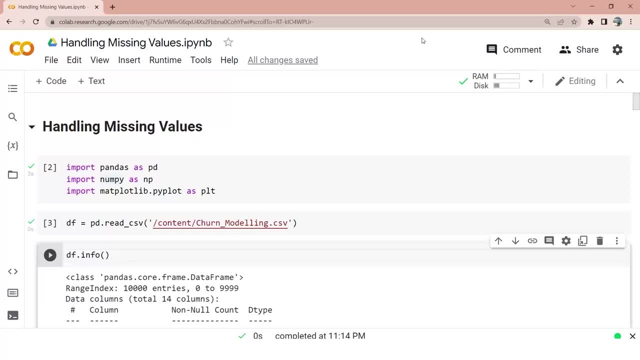 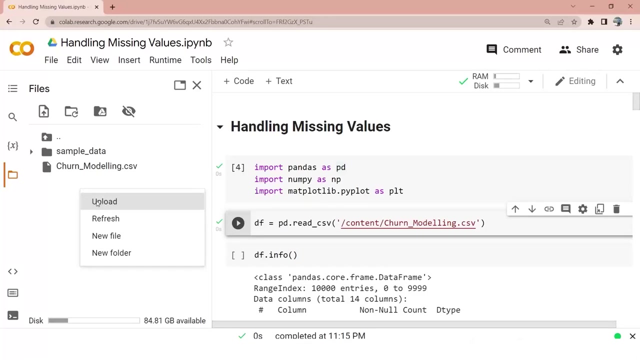 that missing value and probably i will tell you different techniques on what we should do and what we usually do while in this journey of the data training process. so we'll get started by importing all these libraries: pandas, numpy and matplotlib. as you can see, i'm using google collab, so i have just right clicked and uploaded the churn modeling. 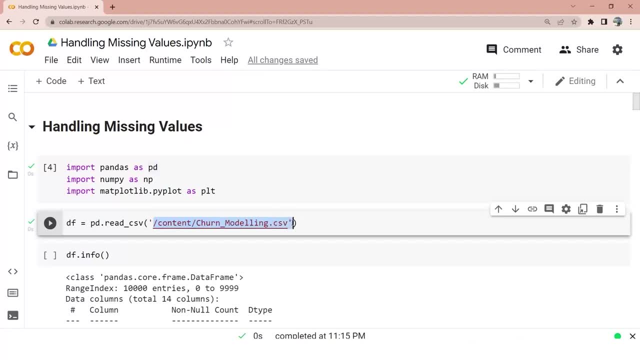 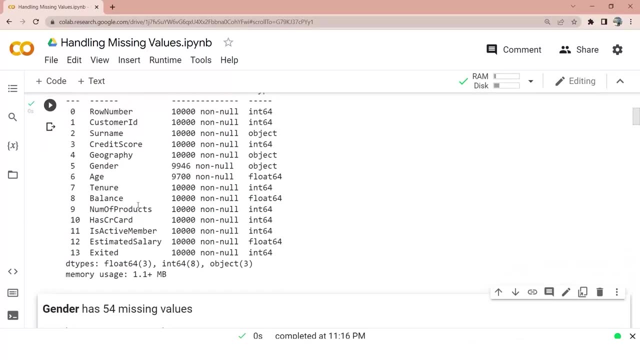 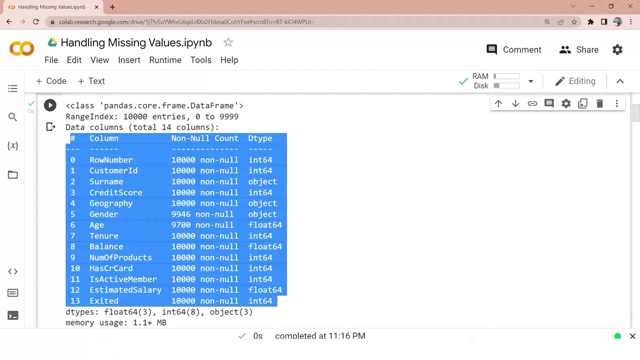 file here and here i'm reading it using slash content. slash the churn modeling file. the moment i run, my data frame is ready. the first thing that i can do is dot info, which will clearly give me a quick information about the entire data set. we have manually created some null values for these. 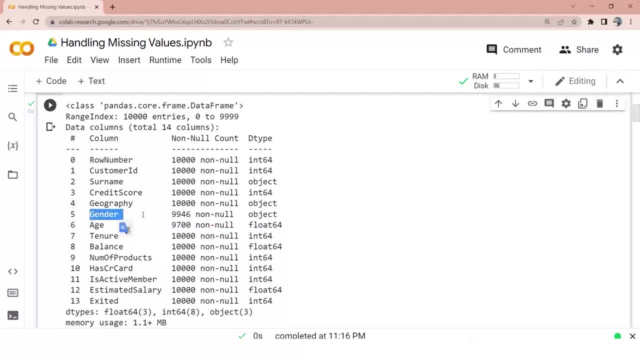 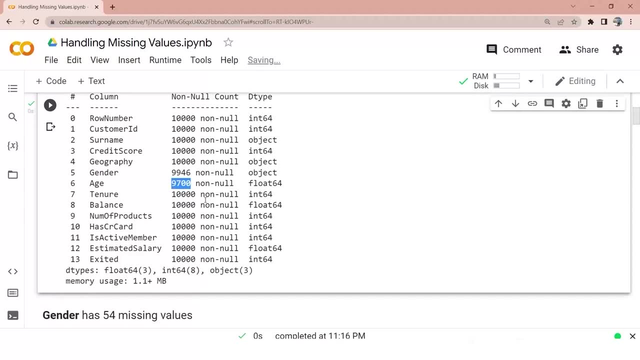 two columns, but you can see it's quite visible. gender: we have 54 null values and for age we have almost 300 null values. how much percentage is 300 out of 10 000? if you start calculating, 300 divided by 10 000 is almost three percent. 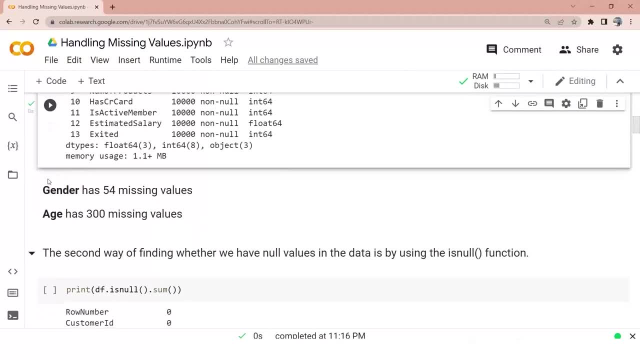 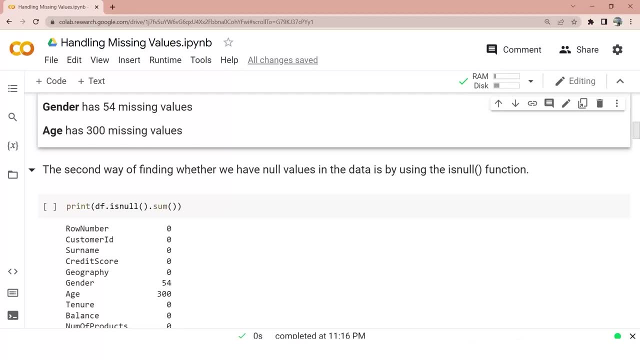 percent of null values. so these are the insights that are written here. the second way of finding whether we have null values in the data is by using the is null function. simply, you can print data frame: dot is null dot sum. the moment you print in, you will be. 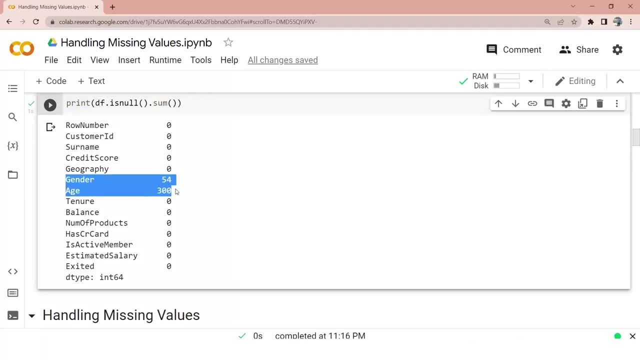 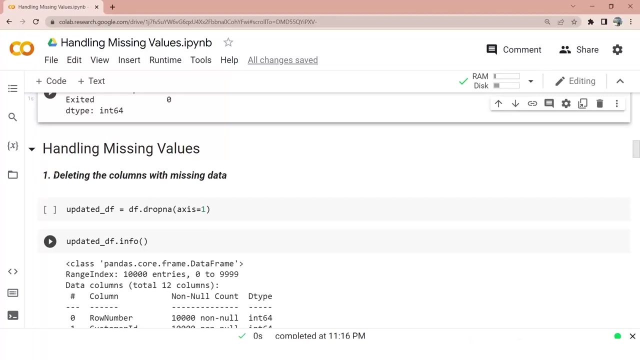 able to get something like this, which clearly states that gender has 54 null values and age has 300 null values. now we know that our data set has null values. what's next is how to handle them, so there are different techniques that are mentioned here. the first technique is deleting the columns with missing data. 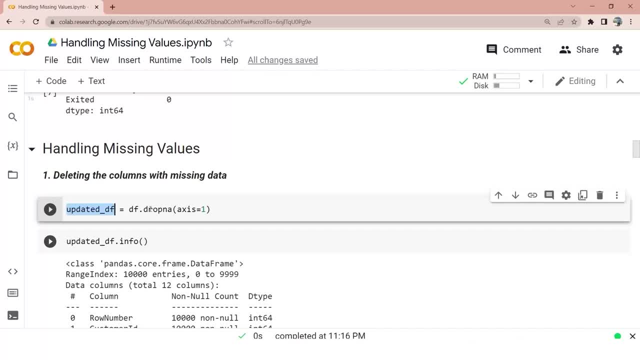 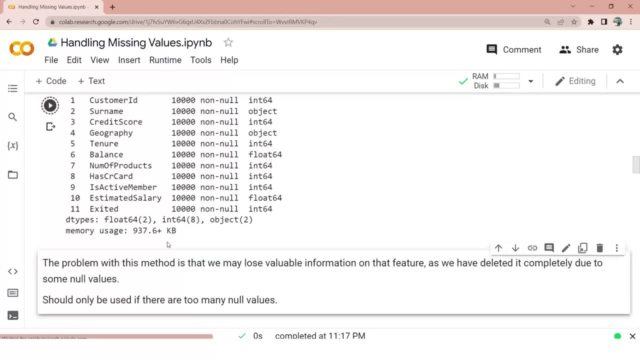 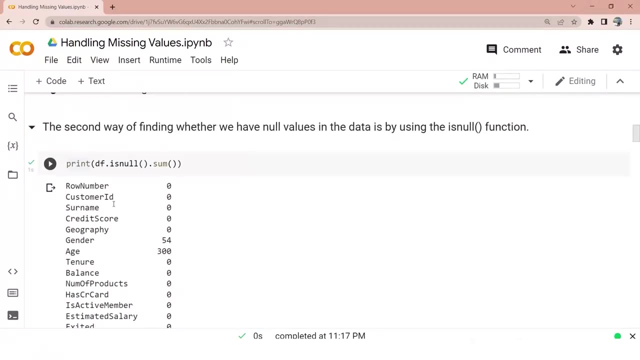 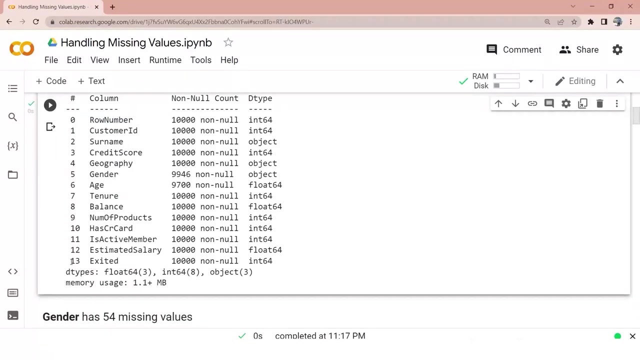 first of all, i have created a new data frame and i am doing df dot drop na axes equals to 1. the moment i run this and then i do updated dfinfo, you can see that my two columns are gone. i don't see gender and age anymore here. initially there were columns ranging from 0 to 13, so almost 14 columns. 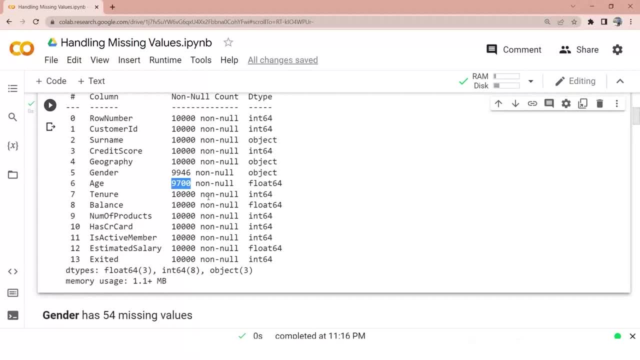 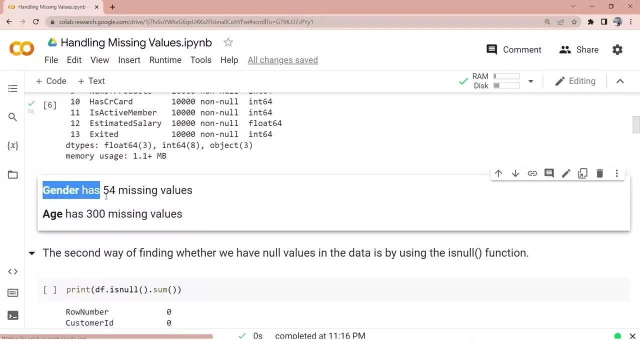 null values. how much percentage is 300 out of 10,000? if you start calculating, 300 divided by 10,000 is almost three percent. three percent of non values. so these are the insights that are written here. the second way of finding whether we have 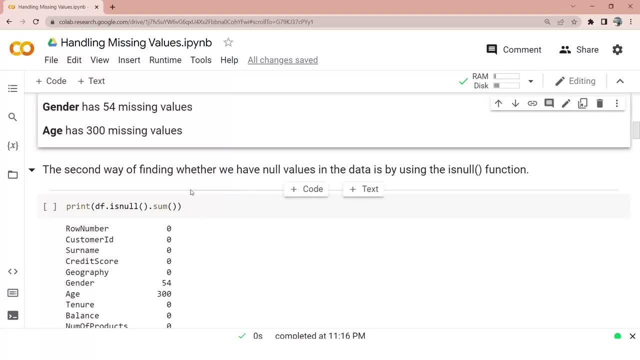 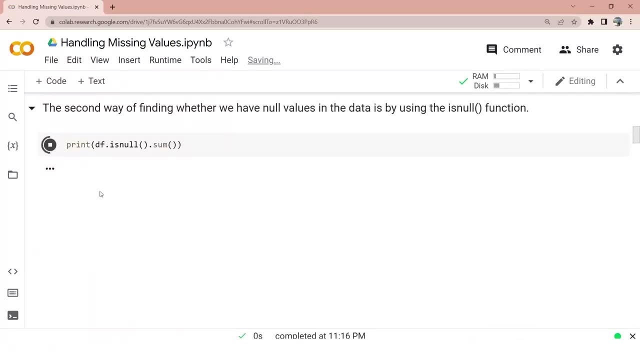 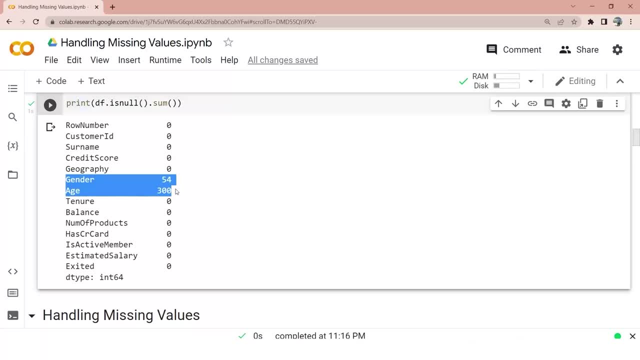 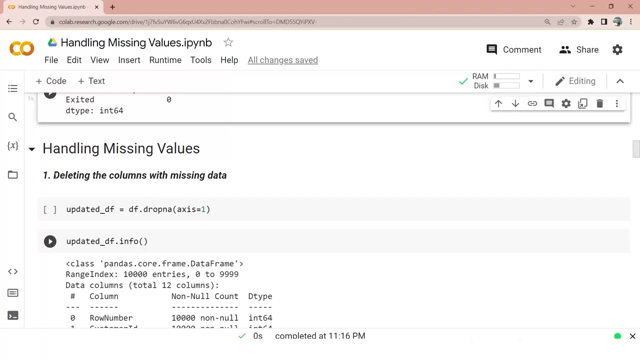 age has three hundred null values. now we know that our data set has null values. what's next is how to handle them. so there are different techniques that are mentioned here. the first technique is deleting the columns with missing data. first of all, I have created a new data frame and I am doing df, dot, drop na. 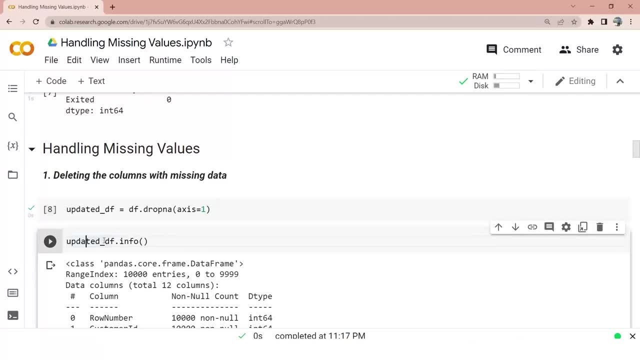 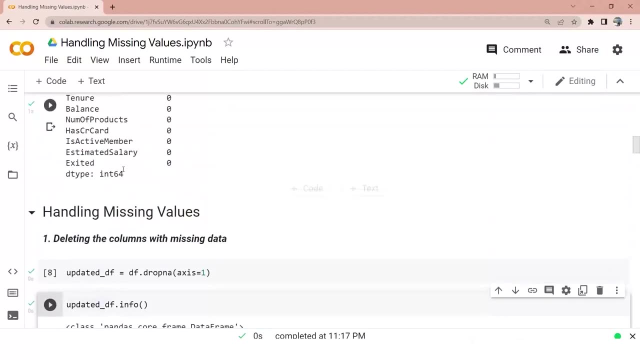 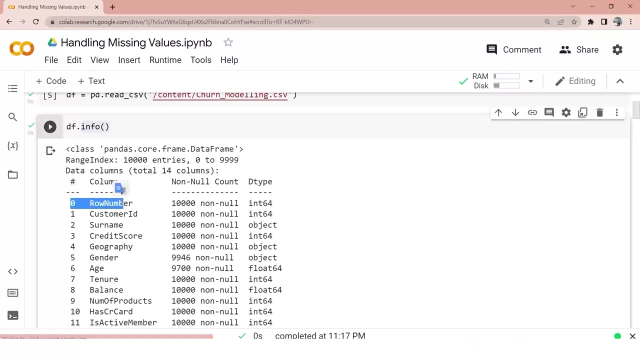 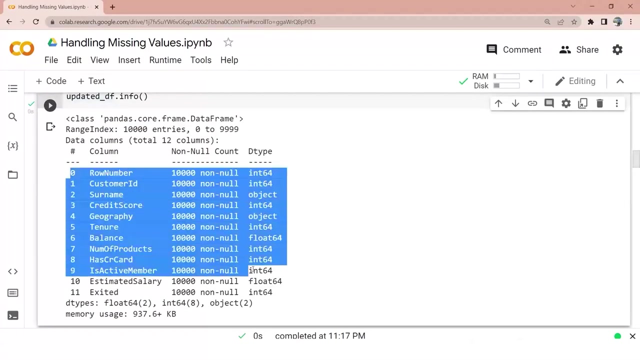 axis equals to one. the moment I run this and then I do, updated df dot info, you can see that my two columns are gone. I don't see gender and age anymore here. initially there were columns ranging from 0 to 13, so almost 14 columns, and now we have 0 to 11, that is, 12 columns. so age and gender has been dropped. 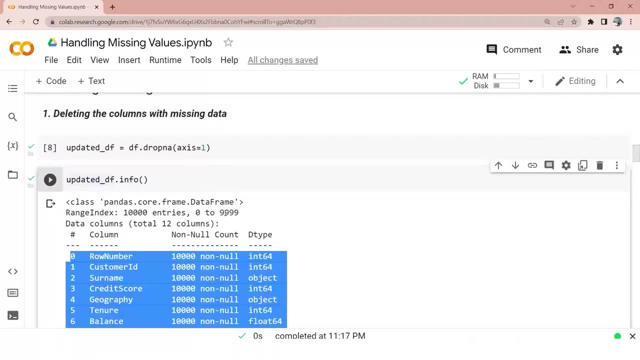 is this a wise decision to do? in this particular scenario, where age has three percent null rates and gender has less than one percent of null values? it is not a wise decision to drop these columns, because they could be carrying a lot of information. the problem with this method is that 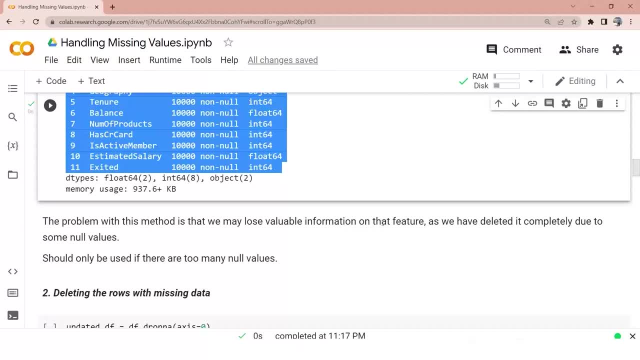 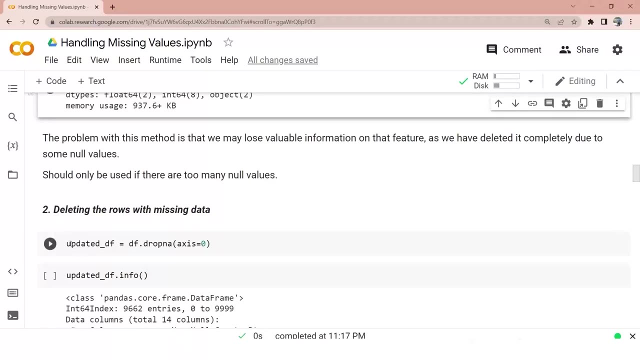 we may lose valuable information on that feature, as we have deleted it completely due to some. null values should only be used if there are too many null value. second technique is deleting the rows with missing data, so i'm again creating another data frame. dfdropna axis equals to zero. 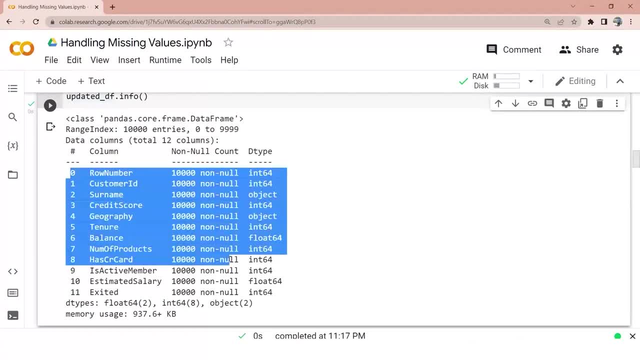 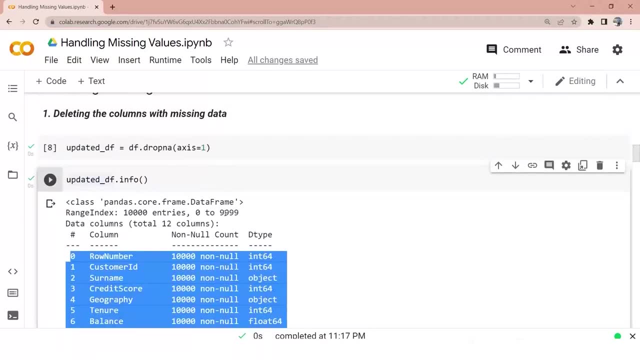 and now we have 0 to 11, that is, 12 columns. so age and gender has been dropped. is this a wise decision to do? in this particular scenario, where age has three percent null rates and gender has less than one percent of null values, it is not a wise decision to drop these columns because 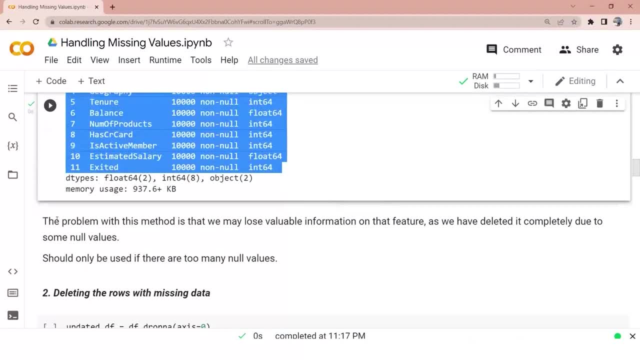 they could be carrying a lot of information. the problem with this method is that we may lose valuable information on that feature as we have deleted it completely due to some null values should only be used you. there are too many null value. second technique is deleting the rows with missing data. so i'm 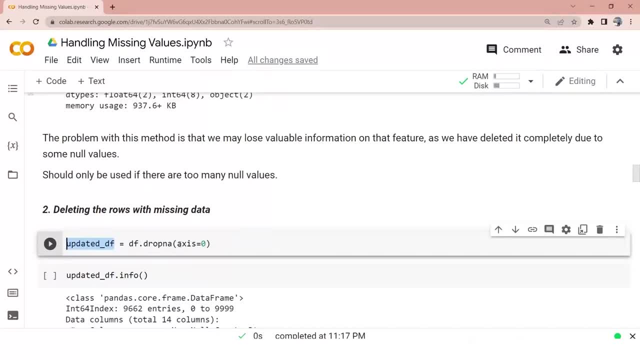 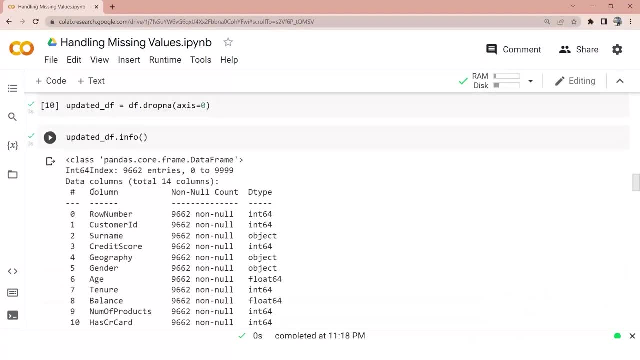 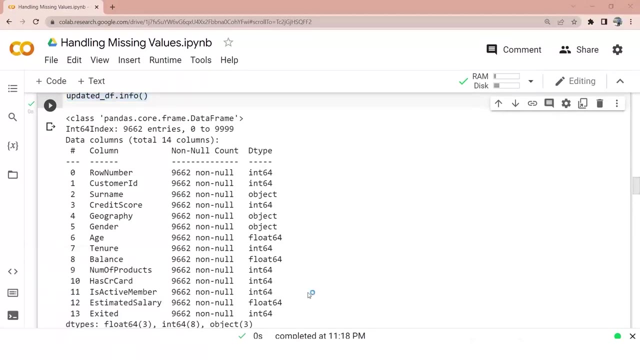 again creating another data frame, dfdropna. axis equals to 0, axis equals to 0 means it will only be deleting the rows. now you can see when i'm doing dot info, whichever rows let's say. let's say i have a data, i have multiple columns, we'll talk about four columns. this particular record is null value. 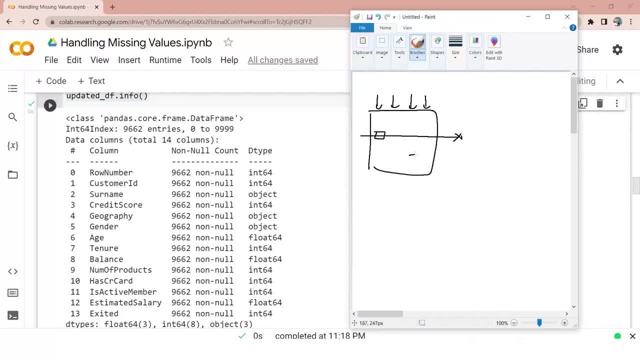 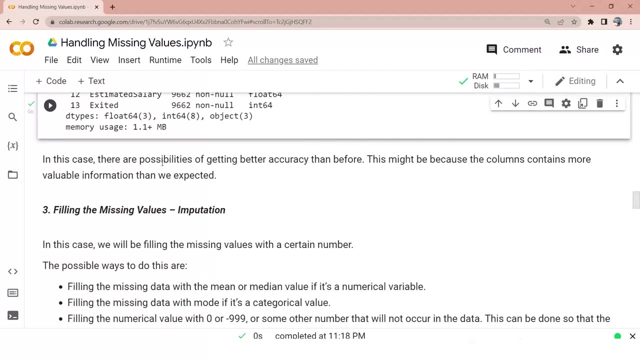 that means this entire row is deleted. this particular value is null value. that means this entire row is deleted. this is what is done here, so we are left out with 9662 records. in this case, there are possibilities of getting better accuracy than before. this might be because 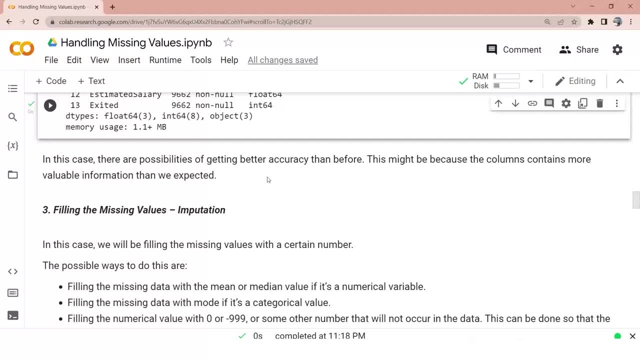 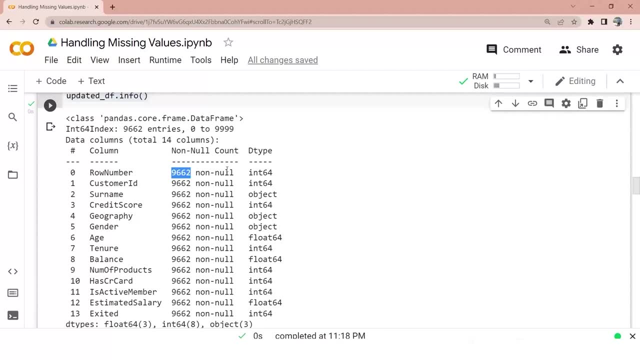 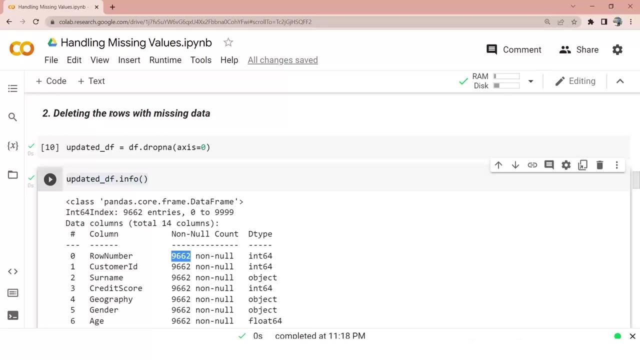 the columns contains more valuable information than we expected. so usually when we go ahead with the machine learning model building or the predictive model building, this can be an accepted way. you can delete these rows. that is fine, because some of the columns in these rows are non. but 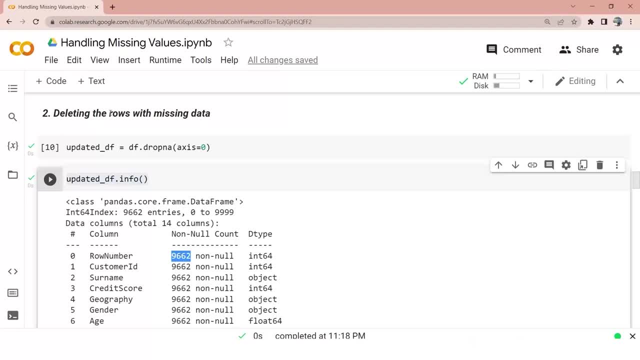 again, there are some better techniques as well, which is imputation and, as we told, when it comes to predictive analytics or machine learning model buildings, it's going to 보여 suscented. but again, there are some better techniques as well, which is imputation and, as we told, when it comes to predictive analytics or machine vidare, that is acceptable, and so on. but then a high competitive model building is nicely noticeable. well, this can be accepted and either that's acceptable. 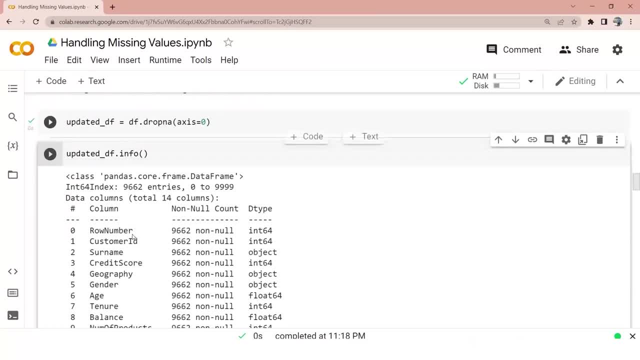 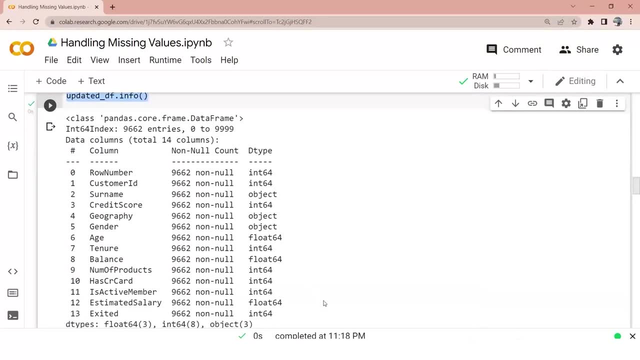 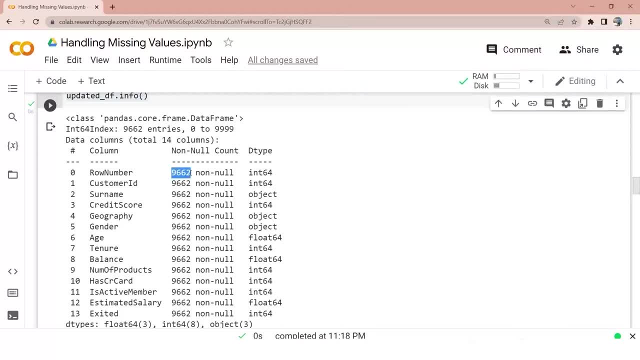 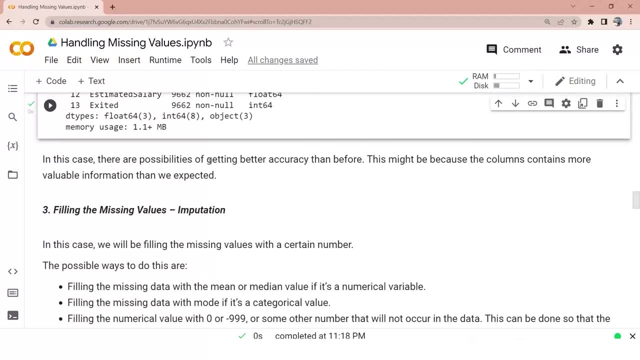 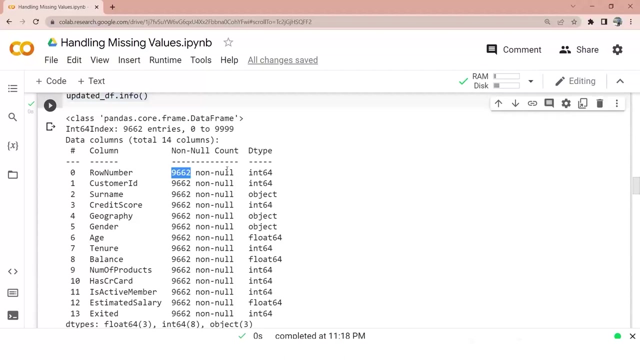 so done here, so we are left out with 9662 records. in this case there are possibilities of getting better accuracy than before. this might be because the columns contains more valuable information than we expected. so usually when we go ahead with the machine learning model building or the predictive model building, this can be an accepted way. you can delete these rows, that is. 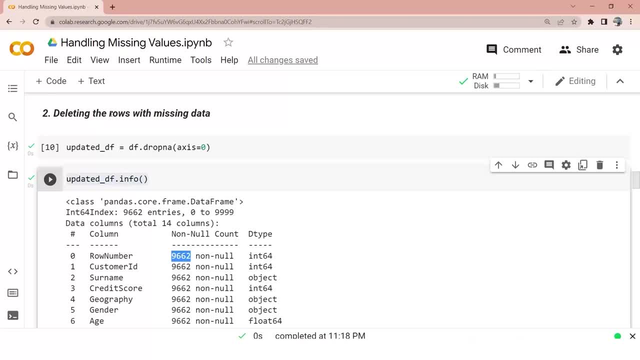 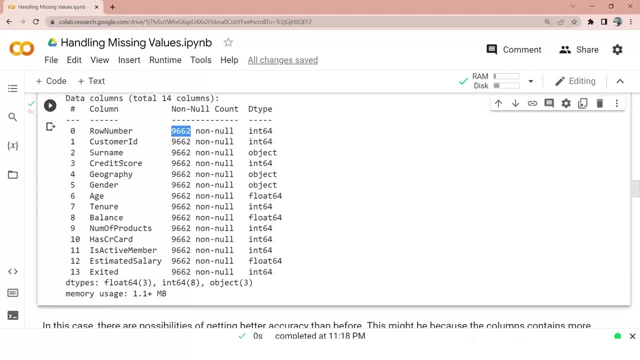 fine, because some of the columns in these rows are null. but again, there are some better techniques as well, which is imputation, and, as we told, when it comes to predictive analytics or machine learning part, nobody can really tell you which technique is the best, whether the deleting rows is best. 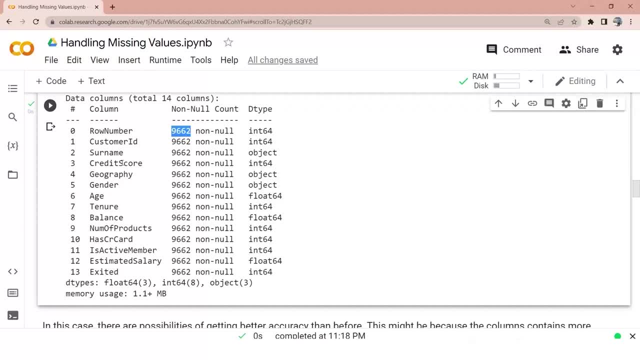 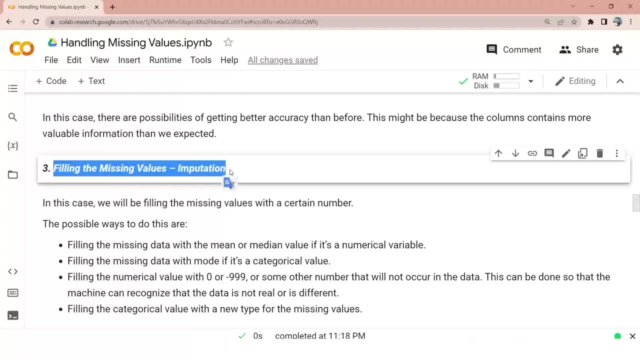 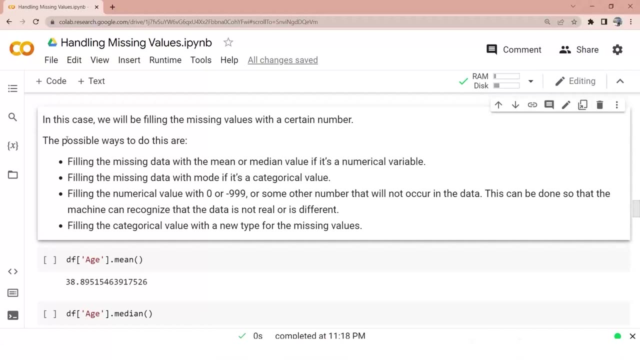 or deleting columns are best or imputation is best. it's all about hit and trial. moving on to the next technique, which is filling the missing values. imputation: in this case, we will be filling the missing values with a certain number. the possible ways to do this are filling the missing value with the mean or median value, if it is a numerical. 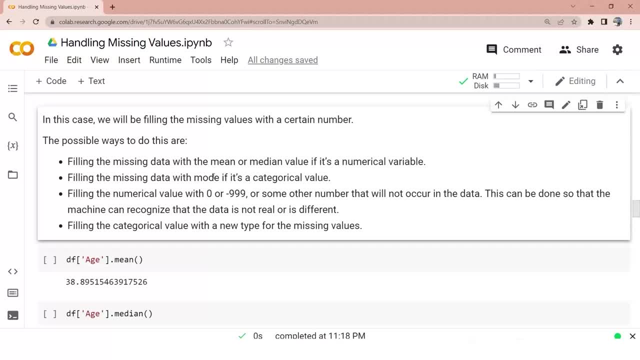 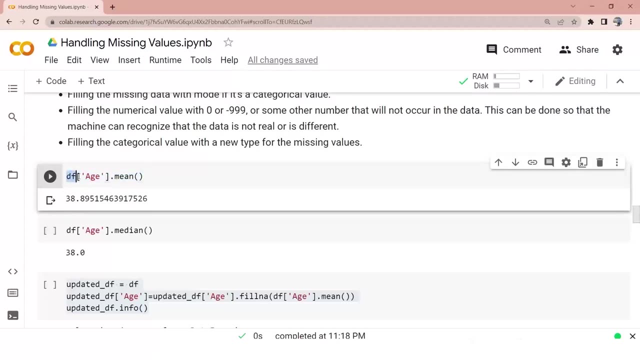 variable. if it is a categorical, we will use mode, or else some idiotic approaches are to randomly fill it with some random data. now, how to calculate the mean of the edge column? you can see, i'm just calling the df of age dot mean, which is 38.89. what is the median? the median is 37.. 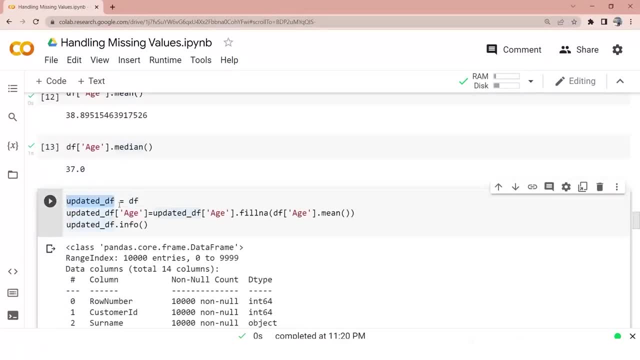 so here, what i'm doing is i'm creating a data frame called as updated df, taking the help of df in the updated df for the age column. i am doing a data frame called as updated df, taking the help of df in the updated df for the age column. 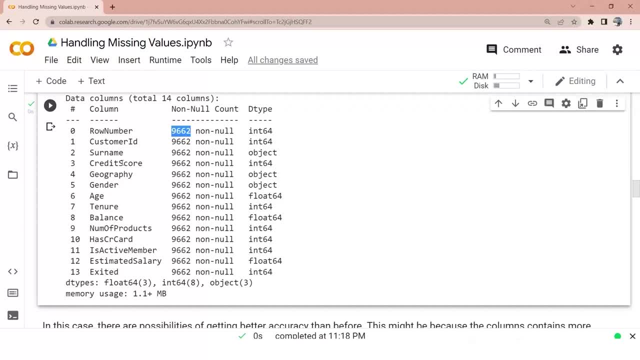 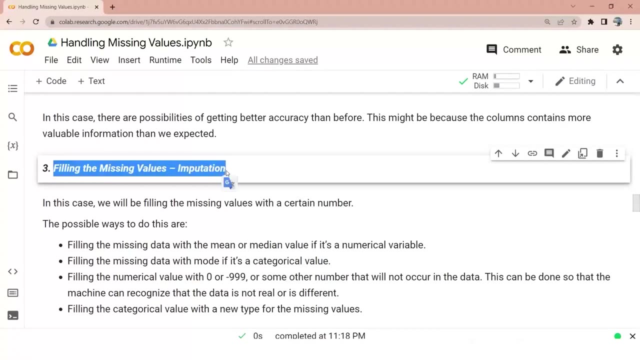 learning part. nobody can really tell you which technique is the best, whether the deleting rows is best, or deleting columns are best or imputation is best. it's all about hit and trial. moving on to the next technique, which is filling the missing values: imputation, in this case, we will be filling 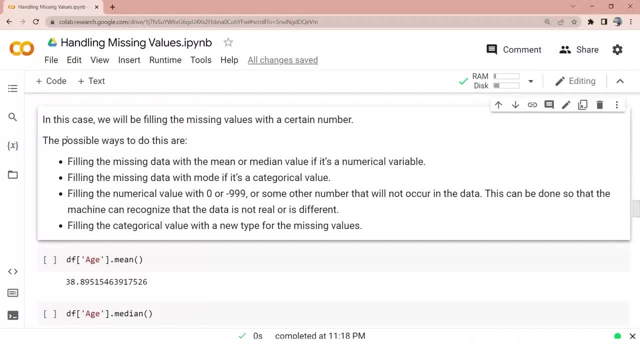 the missing values with a certain number. the possible ways to do this are filling the missing value with the mean or median value, if it is a numerical variable. if it is a categorical, we will use mode, or else some idiotic approaches are to randomly fill it with some random data. 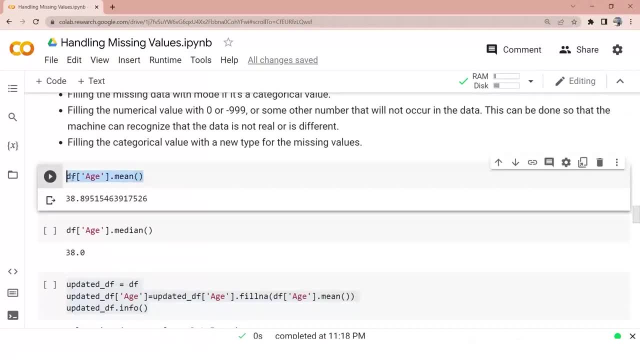 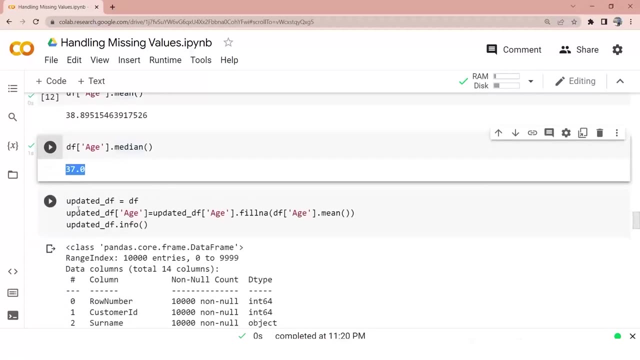 now how to calculate the mean of the age column. you can see, i'm just calling the df of age dot mean, which is 38.89. what is the median? the median is 37.. so here what i am doing is i'm creating a data frame called as updated df, taking the help of 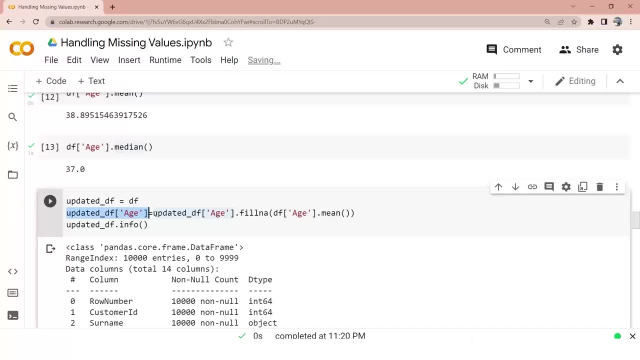 df in the updated df for the age column i am doing updated df of age. dot fill na what i am filling. i am filling the mean value. try to remember this. fill na. fill na basically fills the null records. we also have drop n a. drop na basically means drops the null records. in this case we are filling the null values with. 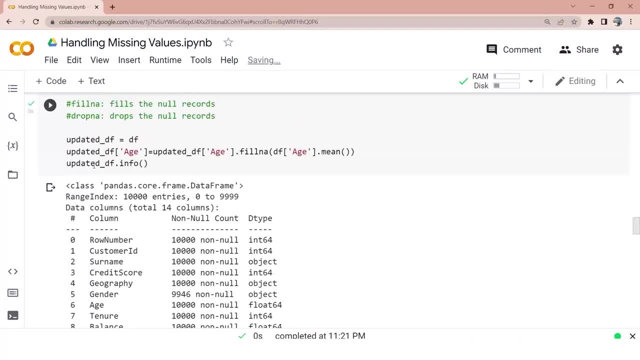 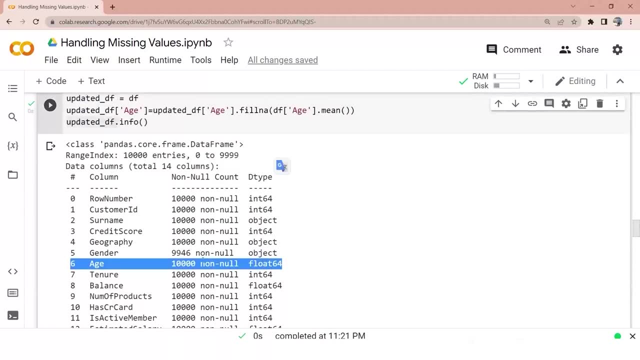 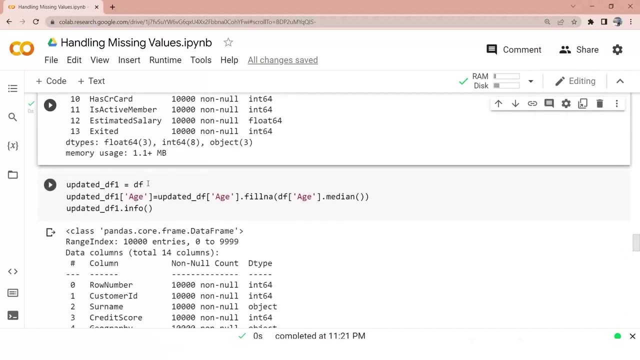 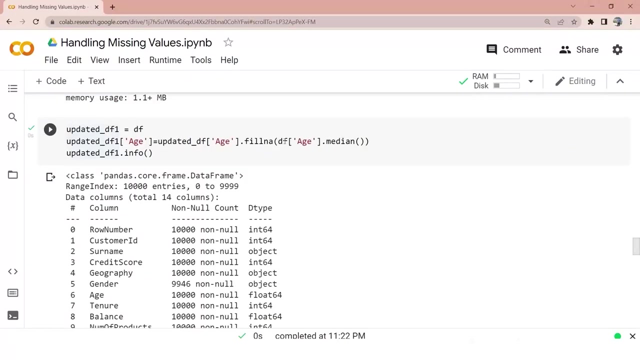 the mean value. now, if you do this and then you do the updated dfinfo, you can see the age records are treated. now age does not have any null values. because you have already treated it similarly, i will now treat it with median and you can see, upon treating it with median again, the age null values are gone. which of them is good. 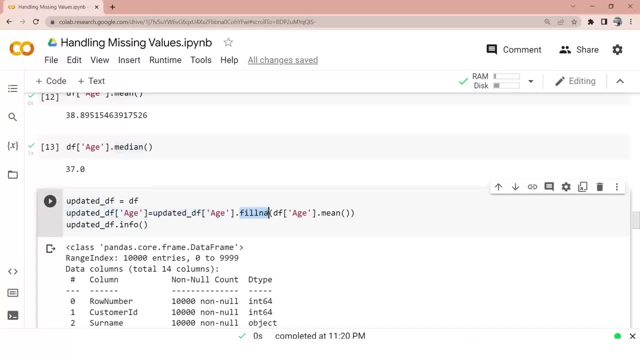 i am doing updated df of age. dot fill na what i am filling. i am filling the mean value. try to remember this. fill na. fill na basically fills the null records. we also have drop na. drop na basically means drops the null records. in this case, we are filling the null values with the mean value. now, if you do this, 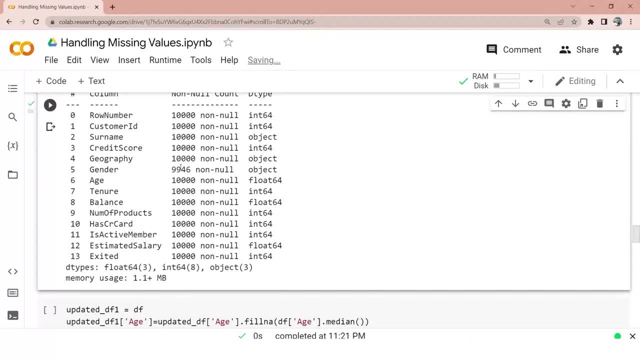 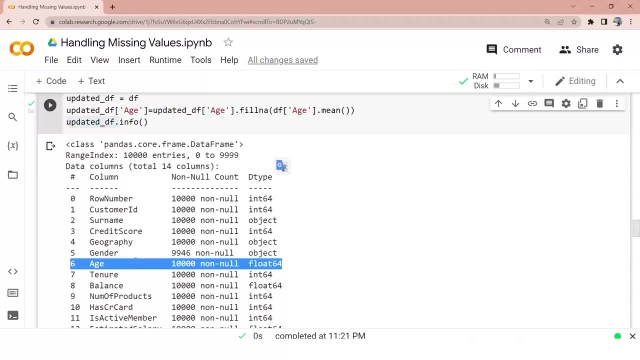 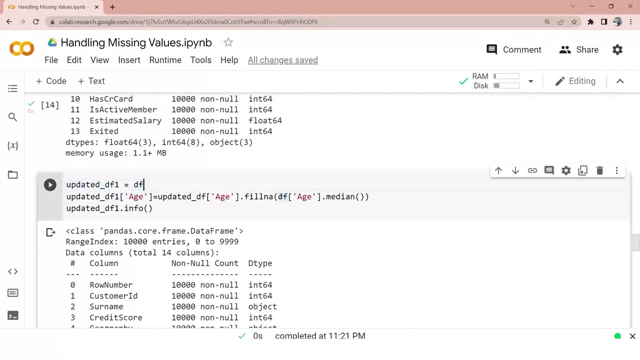 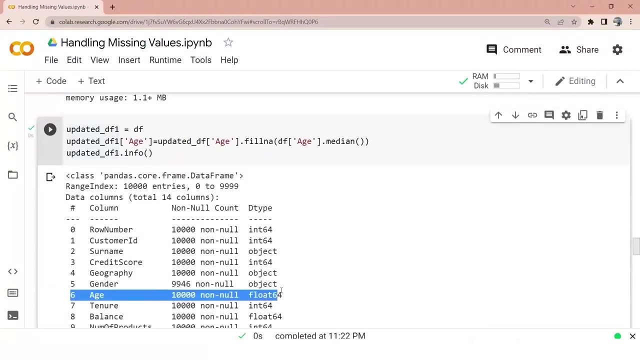 and then you do the updated df dot info. you can see the age records are treated. now age does not have any null values. because you have already treated it similarly, i will now treat it with median and you can see, upon treating with with median, again the age null values are gone. which of them is good, mean or median. 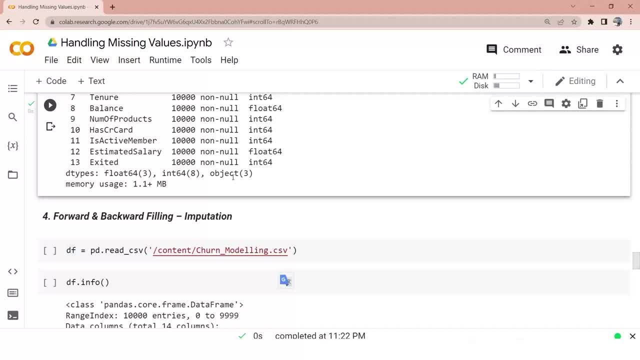 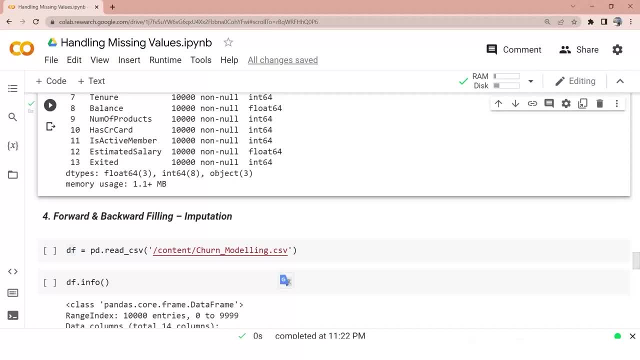 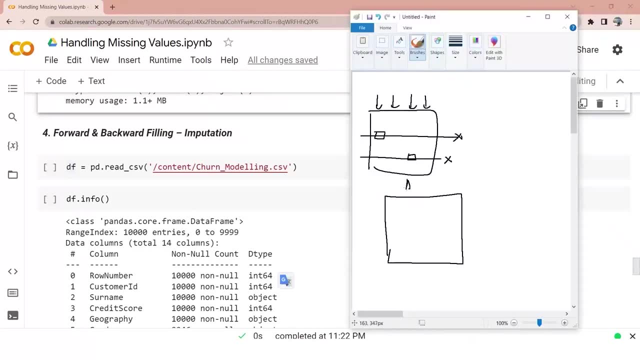 it is better to use mean some other techniques are forward and backward filling, which basically means this: you have a data set and i'm talking about age. so age, let's say 25 null 29, 30 null, 35- forward filling and backward filling means this value gets updated here, so it becomes 25. this 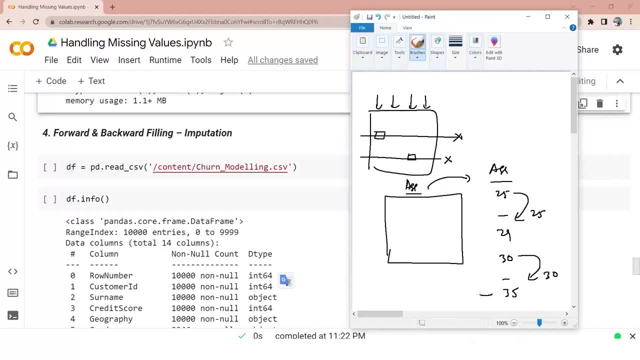 value gets updated here, this becomes 30, or else other way around: this value gets updated here- 35, and this value gets updated here, which is 29. so there are different techniques using which we can impute which of them is the best technique. it's all about hit and trial. 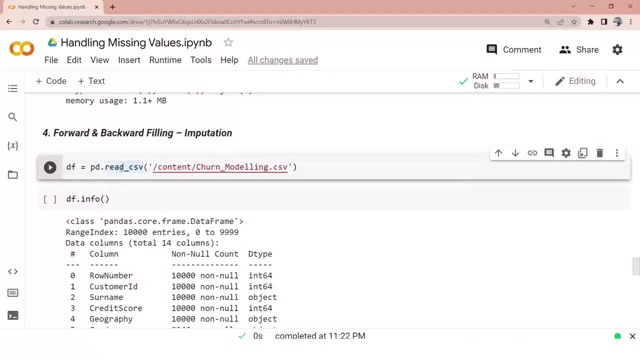 the more hit and trial we do and then build our models, we'll probably be getting more understanding that this is a better technique. but as we are into the ada process we just have to learn what are the different techniques to handle missing values, because in analysis we 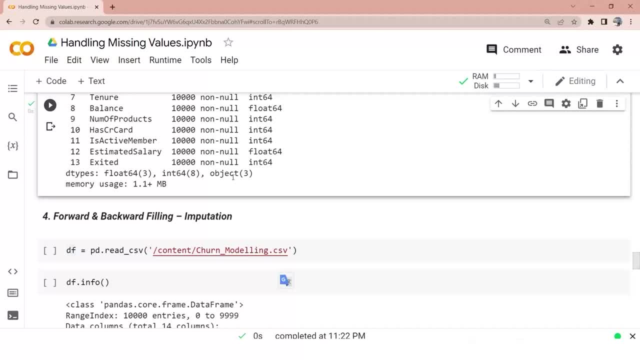 mean or median. the concept remains the same. there is no thumb rule that mean is better than median or vice versa. sometimes, when you have too many outliers, it is better to use median. when you have less outliers, it is better to use mean. some other techniques are for selecting results. you have 그럼. 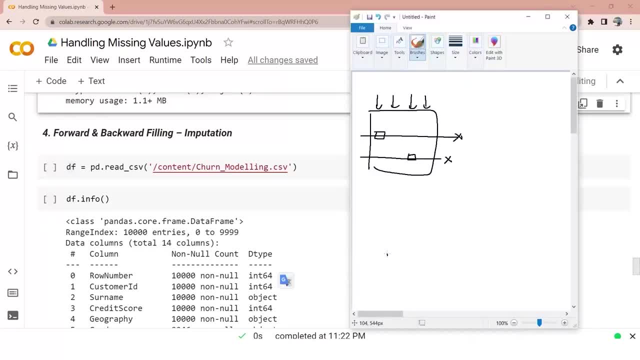 forward and backward filling, which basically means this: you have a data set and i am talking about age. so age, let's say 25 null 29, 30 null 35- forward filling and backward filling means this value gets updated here, so it becomes 25. this value gets updated here, this becomes 30. 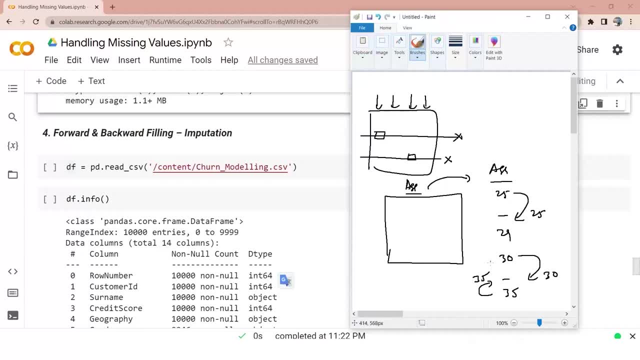 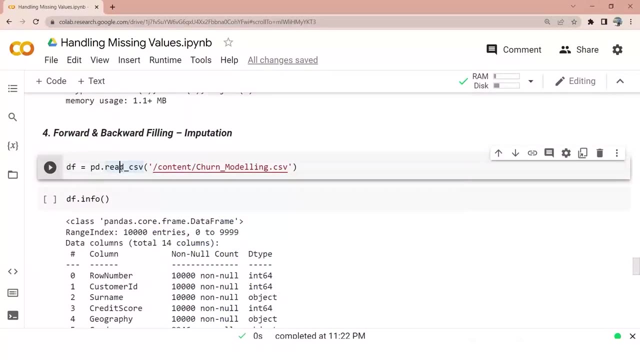 or else other way around: this value gets updated here- 35, and this value gets updated here, which is 29. so there are different techniques using which we can impute which of them is the best technique. it's all about hit and drag: the more hit and trial we do and then build our models. 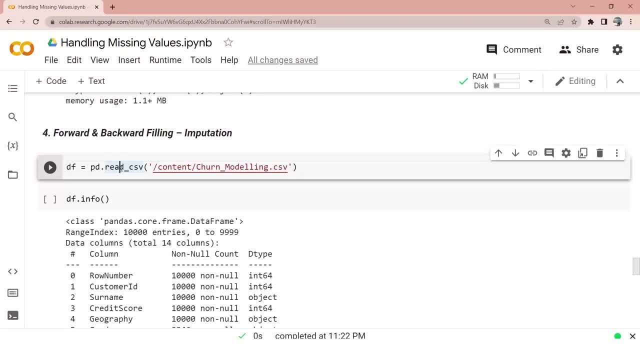 we'll probably be getting more understanding that this is a better technique. but as we are into the ada process, we just have to learn what are the different techniques to handle missing values, because in analysis we don't have to understand which is best, which is not best. 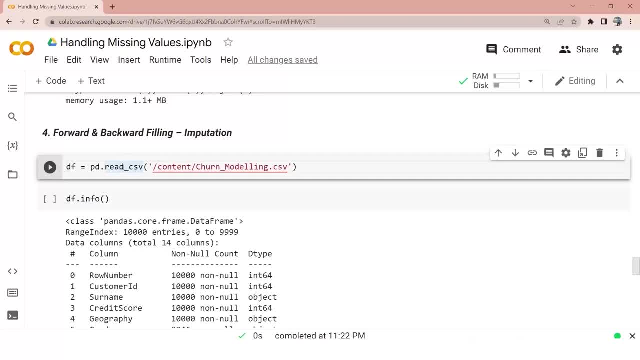 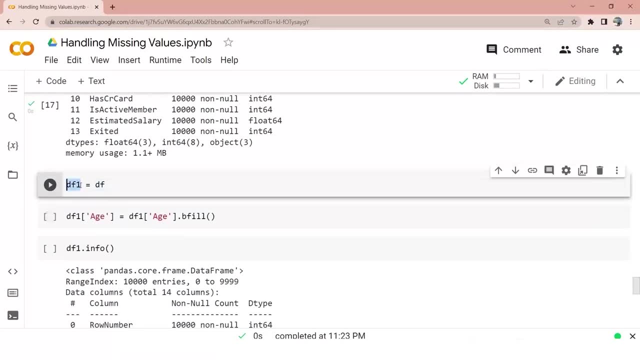 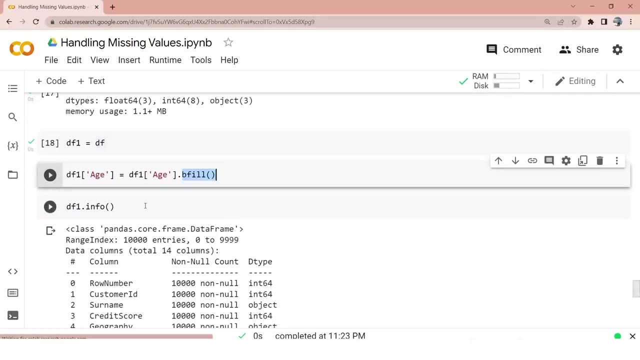 which technique is good, which is not good. so i'll be reading this data frame, dfinfo, again. you can see null values. i'm creating another data frame and in this new data frame i'm using the b fill. okay, backward fill and you can see, once i'm doing backward fill, my values are. 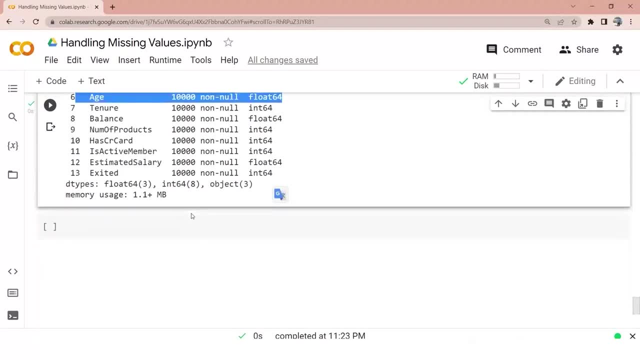 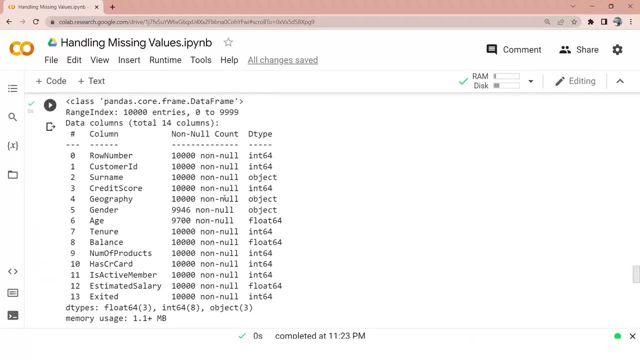 being updated. my age values are being updated and, similarly, if you want to do forward fill, just simply change it to f fill. that's it. apart from that, as we already discussed theoretically that there are some time series forecasting algorithms as well, which are very, very advanced techniques. we usually understand it theoretically. in practical applications, the amount of efforts, 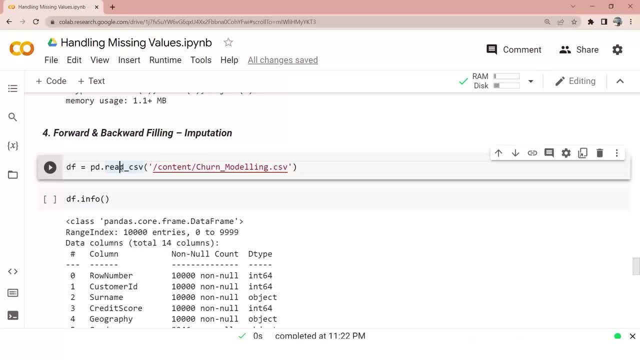 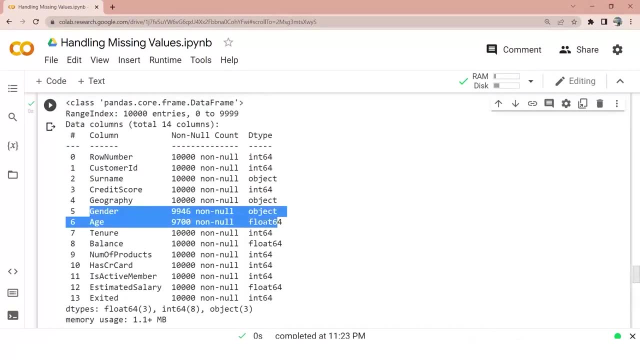 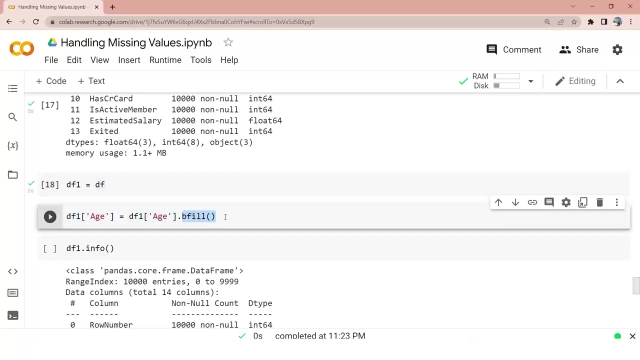 don't have to understand which is best, which is not best, which technique is good, which is not good. so i will be reading this data frame dfinfo again. you can see null values. i'm creating another data frame and in this new data frame i'm using the b fill. 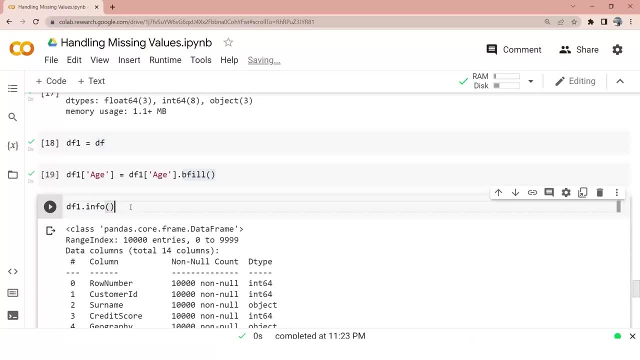 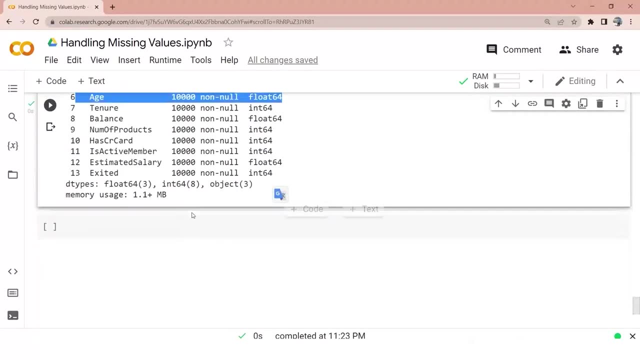 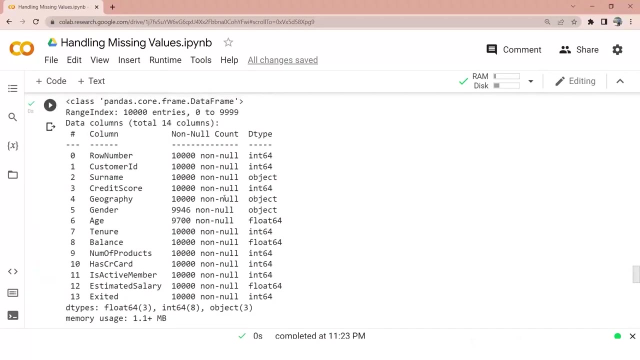 okay, backward fill and you can see, once i'm doing backward fill, my values are being updated, my age values are being updated and, similarly, if you want to do forward fill, just simply change it to f fill. that's it. apart from that, i'm going to use the backward fill and i'm going to use the. 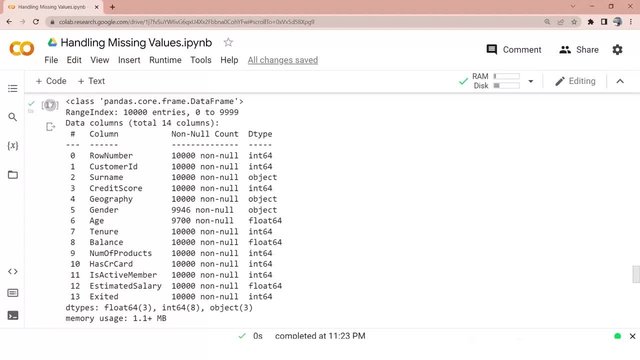 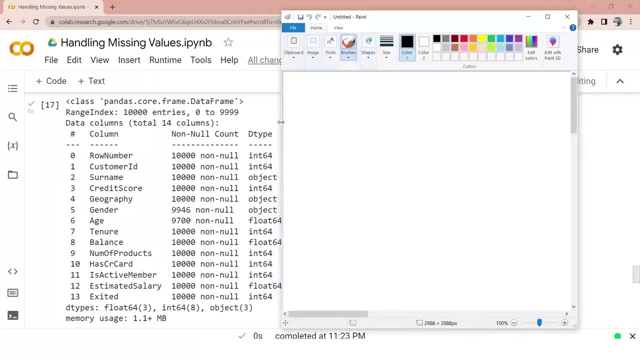 acho in the now. if you want to do it backward fill. so if you want to do it backward fill, just repeat after me. so that's it. apart from that, as we already discussed theoretically that there are some time series forecasting algorithms as well, which are very, very advanced techniques. 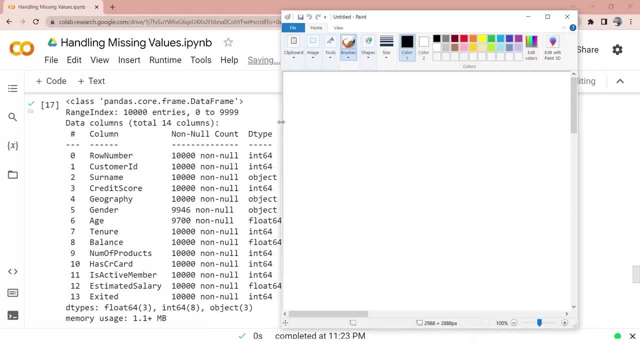 we usually understand it theoretically in practical applications, the amount of efforts we spend in doing that technique, we can actually ignore that and focus more on the model building part. try to explain what do you mean by that time series forecasting technique of handling missing values. imagine you have a column date and let's say you have salary or sales. sales is a better 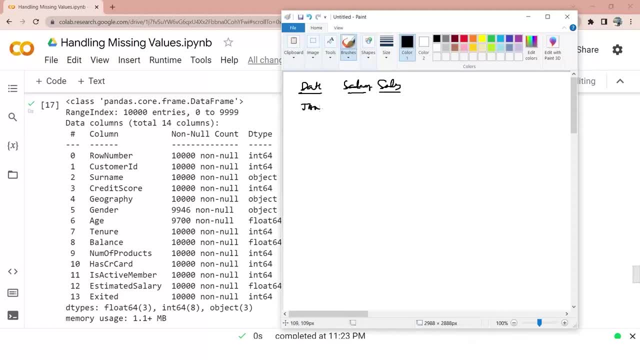 column. you have jan 1, jan 2, and you have different sales value: 120 dollar, 150 dollar, 110 dollar, 80 dollar- and all these are in millions. okay, 70 dollar- null value. 80 dollar- null value. 120 dollar, 130 dollar- null value, something like that. now, this technique can be very tedious. that's why we don't 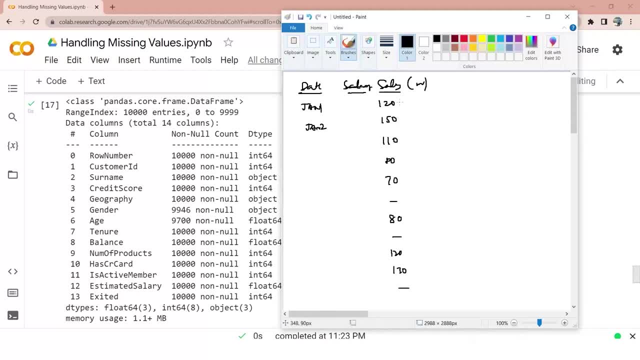 use it practically but theoretically. try to understand this. what happens here is to impute this null value. we can take this five records, insert it into a time series algorithm and then do a one-step prediction. let's say the predicted value is 90.. this prediction goes here: 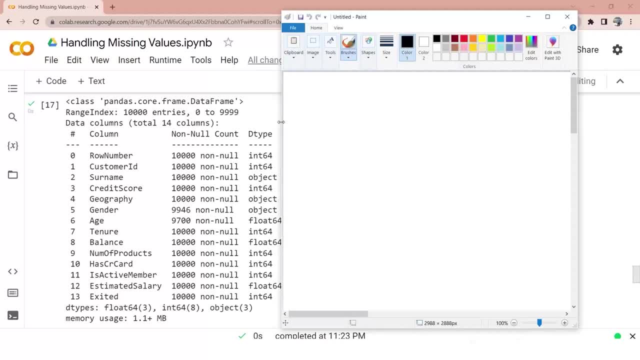 we spend in doing that technique, we can actually ignore that and focus more on the model building part. so we usually don't you do that technique, we don't apply that technique. but theoretically i will try to explain what do you mean by that time series forecasting technique of handling missing values. imagine you. 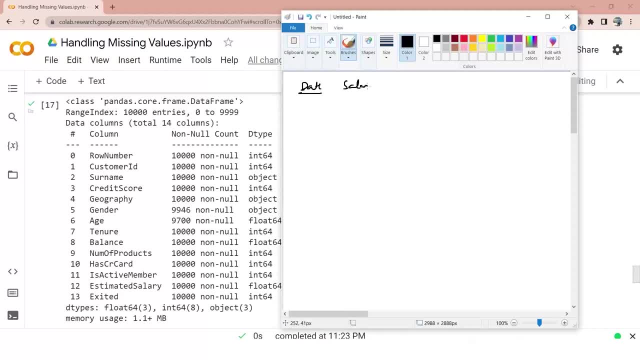 have a column date and let's say you have salary or sales- sales is a better column- you have jan 1, jan 2 and you have different sales value: 120 dollar, 150 dollar, 110 dollar, 18 dollar, and all these are in millions. okay, 70 dollar, null value, 80 dollar, null value, 120 dollar, 130. 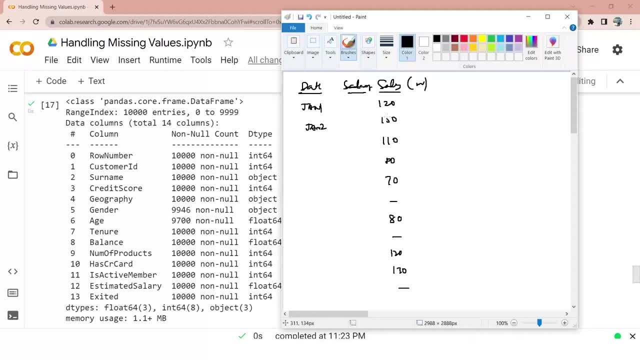 dollar null value, something like that. now, this technique can be very tedious. that's why we don't use it practically but theoretically. try to understand this. what happens here is to impute this null value. we can take this five records, insert it into a time series algorithm and then. 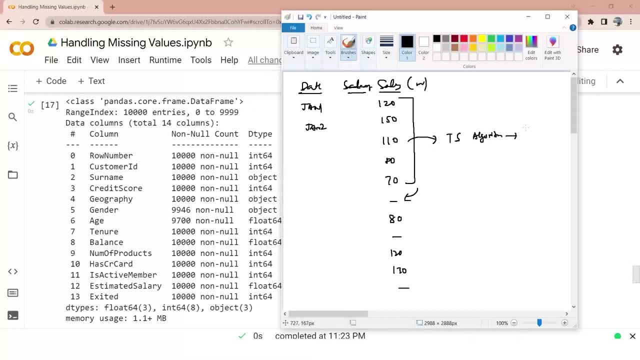 we can take a number of times in this algorithm and then do a one-step prediction. let's say the predicted value is 90.. this prediction goes here. now, next step, what happens is we take all these values- 120, 150, 110, 80, 70, the predicted value 90, 80. using them again, i call another time. 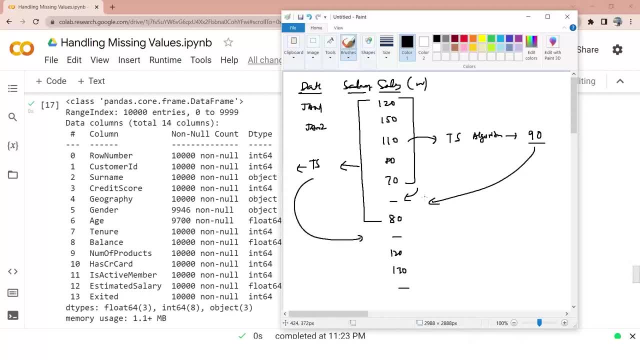 series algorithm. again, i do a one step prediction. whatever the value i impute here, same goes, same goes with here, and this process goes on. imagine you have at least 100 null values. you will be creating 100 algorithms, and creating an algorithm could be tedious in terms of. 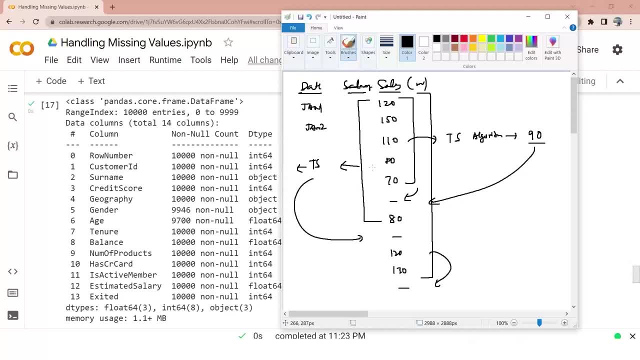 time consumption. it could be tedious in terms of memory consumption as well, so we usually don't put more efforts in these kind of techniques rather than we go for mean, median or mode techniques. so that's all about this particular video on handling missing values. i hope you 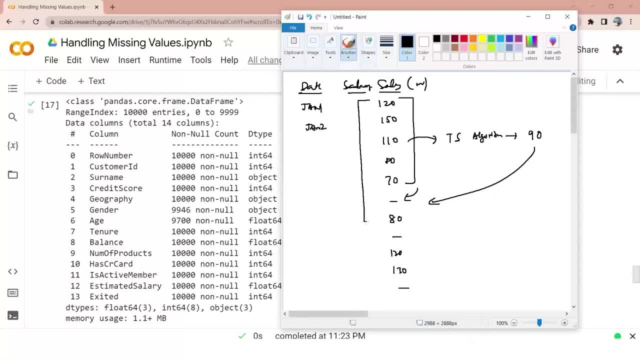 now next step. what happens is we take all these values- 120, 150, 110, 80, 70, the predicted value 90, 80, using them again, i call another time series algorithm. again, i do a one-step prediction. whatever the value i impute here. same goes with. 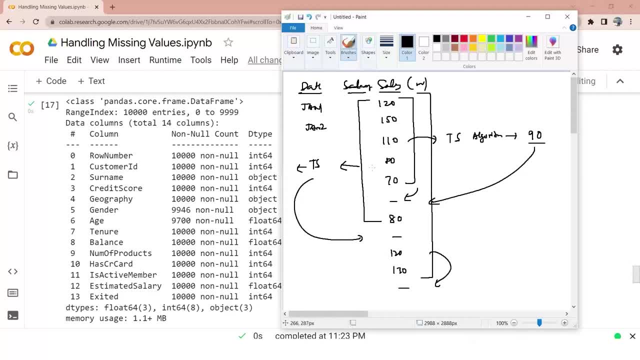 here and this process goes on. imagine you have at least 100 null values. you will be creating 100 algorithms, and creating an algorithm could be tedious in terms of time consumption. it could be tedious in terms of memory consumption as well, so we usually don't put more. 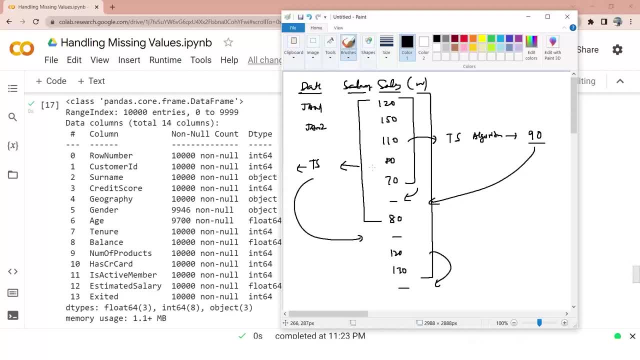 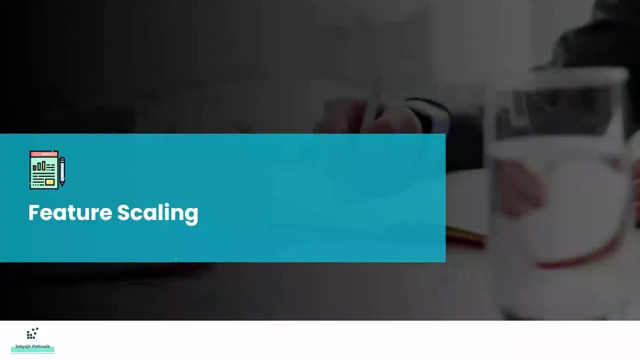 efforts in these kind of techniques rather than we go for mean, median or more techniques. so that's all about this particular video on handling missing values. I hope you understood this. in the next videos we shall be talking about few other techniques that we follow in the data cleaning process, the next technique that we are going to understand. 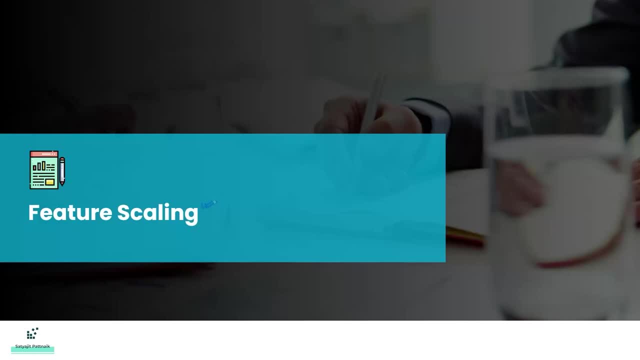 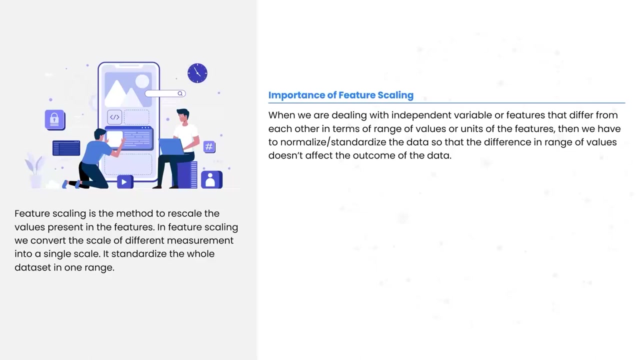 is feature scaling, and this technique is also used as part of the data cleaning process. however, feature scaling is more important when it comes to predictive model building, but sometimes we also use it in the eda process. let's try to understand what exactly is feature scaling and why feature scaling is important. feature scaling is the method to rescale the 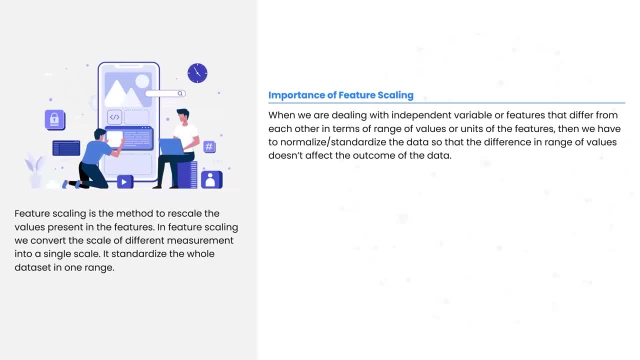 values present in the features. in feature scaling we convert the scale of different measurements into a single scale. it standardized the whole data set in one range. importance of feature scaling: when we are dealing with independent variable or features that differ from each other in terms of range of values or units of the features, then we 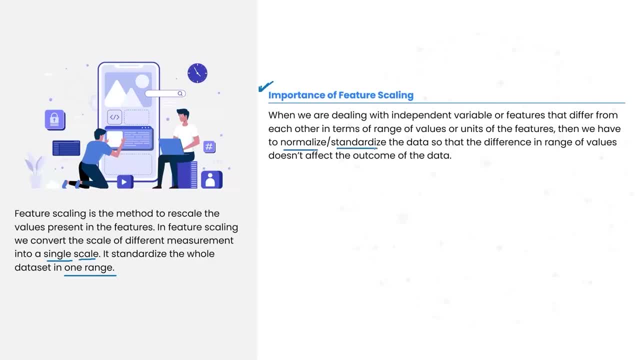 have to normalize or standardize the data so that the difference in range of values doesn't affect the outcome of the data. as we have talked about in the last video that we are using the dataanson inницate, i told you feature scaling is very important when it comes to predictive modeling or predictive 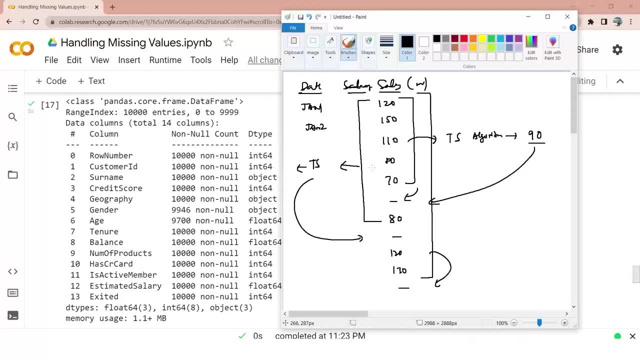 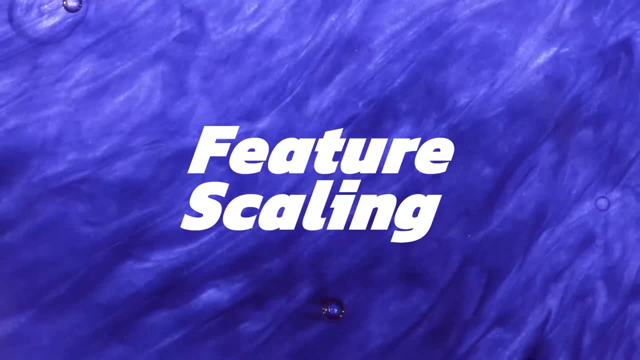 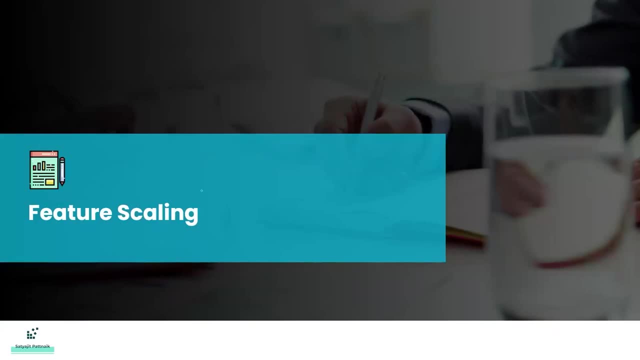 understood this. in the next videos, we shall be talking about few other techniques that we follow in the data cleaning process. the next technique that we are going to understand is feature scaling, and this technique is also used as part of the data cleaning process. however, feature scaling is more important when it comes to predictive model building, but 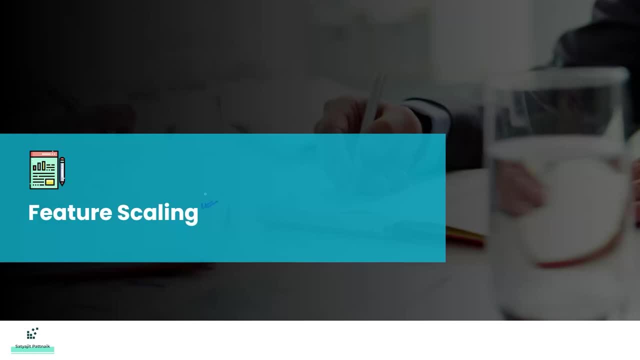 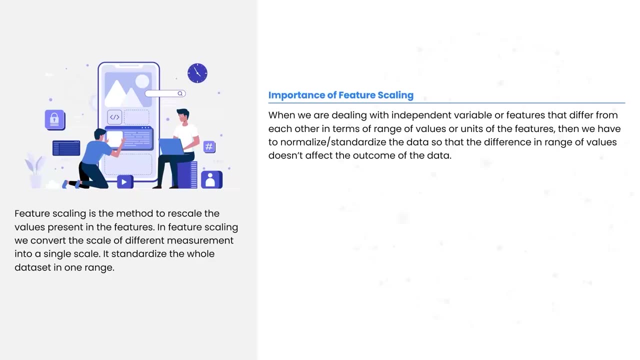 sometimes we also use it in the eda process. let's try to understand what exactly is feature scaling and why feature scaling is important. feature scaling is the method to rescale the values present in the features. in feature scaling we convert the scale of different measurements into. 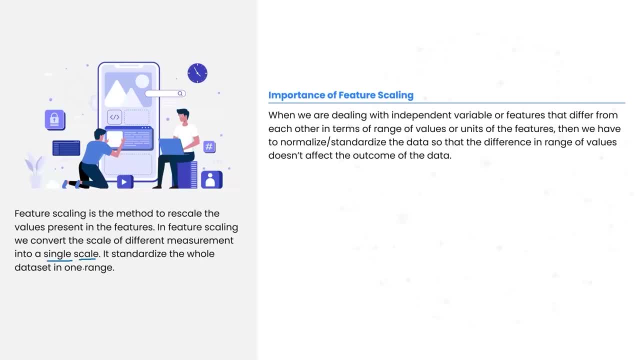 a single scale. it standardize the whole data set in one range. importance of feature scaling. when we are dealing with independent variable or features that differ from each other in terms of range of values or units of the features, then we have to normalize or standardize the data so that the difference in range of values doesn't affect the outcome of the 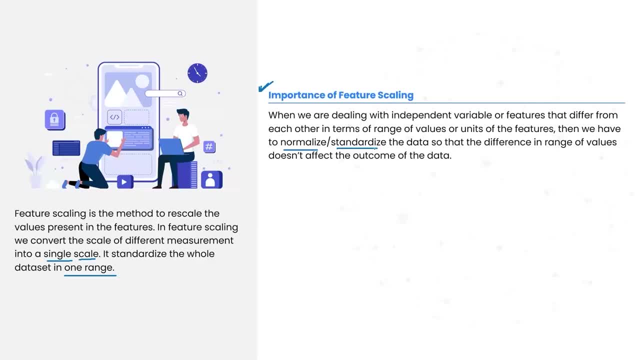 data. as i told you, feature scaling is very important when it comes to predictive modeling or predictive analytics. when it comes to the eda part or the descriptive analytics part, well, it depends on how important this technique is, but let's try to understand. why do we need now? why do we need? 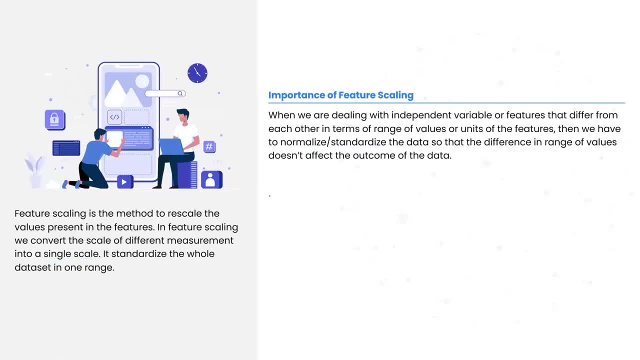 feature scaling. so imagine you are analyzing some data. you are analyzing some data and i'm going to show you how to do that, and that ultimately you have to feed this data to your machine learning model or to your predictive model so that the model can understand the data and be capable enough to 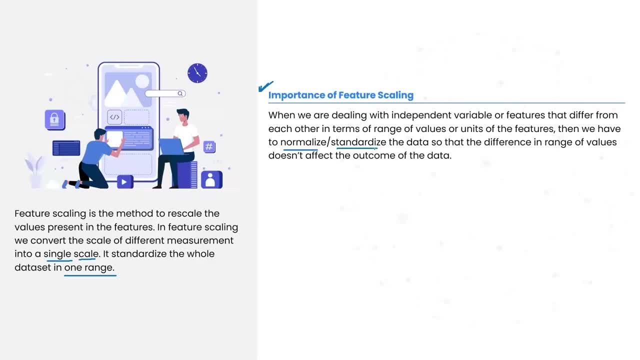 analytics. when it comes to the eda part or the descriptive analytics part, well, it depends on how important this technique is, but let's try to understand. why do we need now, why do we need, feature scaling? so imagine you are analyzing some data. you are analyzing some data and that 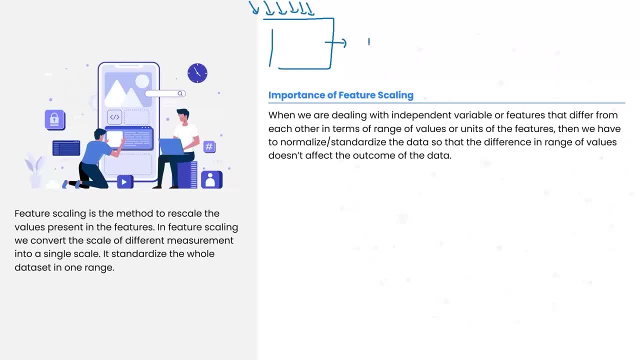 ultimately, you have to feed this data to your machine learning model or to your predictive model so that the model can understand the data and be capable enough to predict something. now your machine learning models or algorithms are nothing but run on computer. and what is the most accepted format of computers? the most accepted format is bytes. 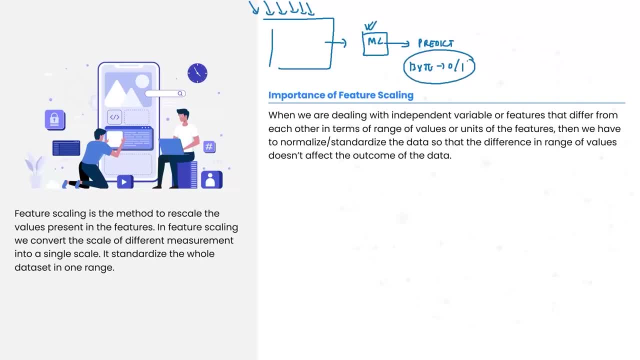 which is in the form of zeros and ones. computers don't understand categorical data, they don't understand any characters, they only understand numerical values. so imagine i talk about a feature called as height. i say i have five customers or five people, and the heights are something like this: 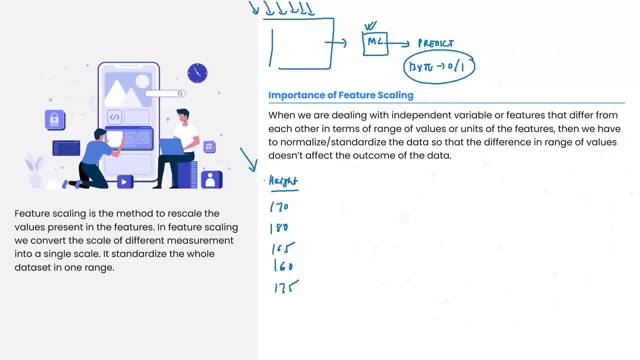 now, if i ask you what is the units of height? and i give you an idea that these are human, relate human beings. i'm analyzing people, i'm analyzing customers data. when i see this column, it is quite obvious that i know that these are in centimeters. why? because we have been trained with so many data till now. we know that. 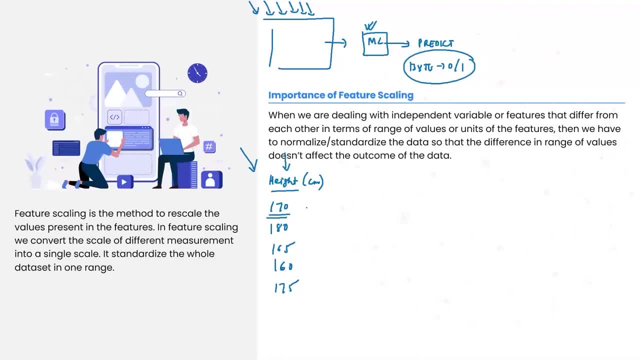 if it is in hundreds places, it is in centimeters. if it is something like this, we know that it will be in meters. if it isn't like this, we know it isn't feet and inches. right, let's say i'll talk about weight. we are analyzing customers data. let's say somebody's weight is 85, we know that. 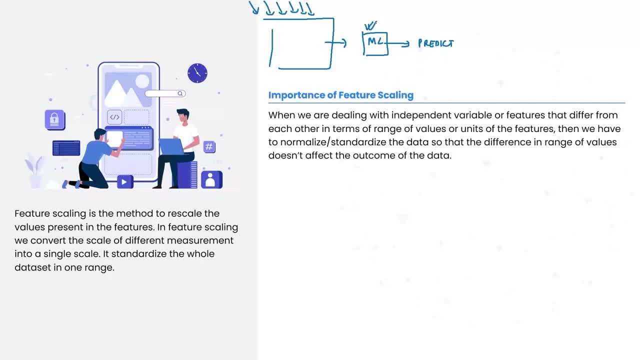 predict something. now your machine learning models or algorithms are nothing but run on computers. and what is the most accepted format of computers? the most accepted format is bytes, which is in the form of zeros and ones. computers don't understand categorical data, they don't understand any characters, they only understand numerical values. so imagine i talk about a feature. 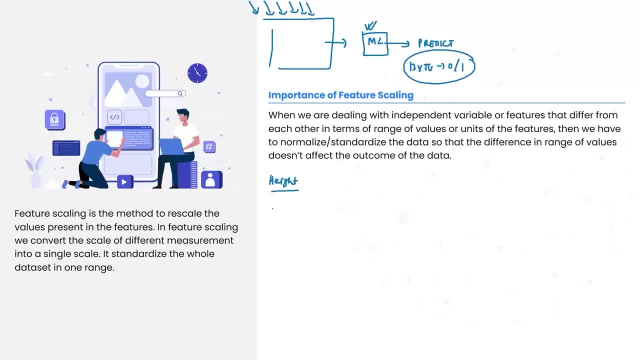 called as height. let's say i have five customers or five people, and the heights are something like this. now, if i ask you what is the units of height and i give you an idea that these are human related, human beings and analyzing people- i'm analyzing customers data. when i see this column, it is quite obvious. 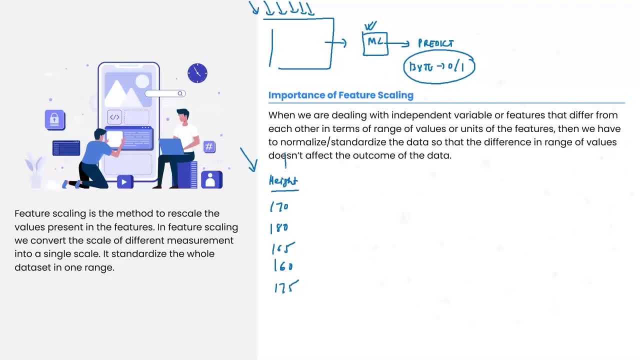 that i know that these are in centimeters. why? because we have been trained with so many data till now. we know that it is real and that it is the data that we use in our lab. and how do we can take that at all? it is in hundreds places. it is in centimeters. if it is something like this, we know that it will be. 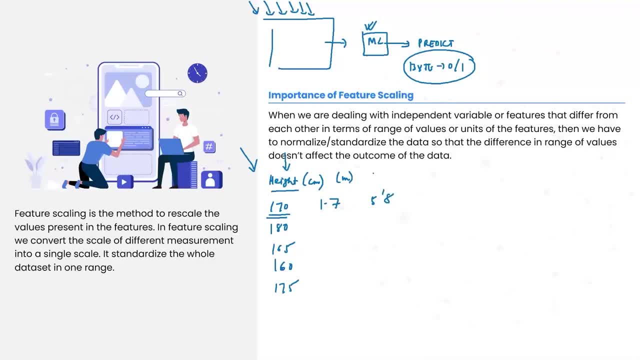 in meters. if it isn't like this, we know it isn't feet and inches. right, let's say i'll talk about weight. we are analyzing customers data. let's say somebody's weight is 85, we know that it has to be kg. very, very rare scenarios it will be lb, but it has to be kg. it cannot be grams, it cannot be. 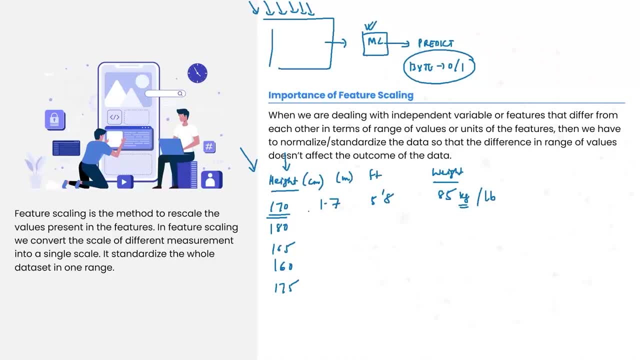 any other units. so ultimately these numbers matter. if you have two columns- height and weight, imagine you have this column and this column. somebody is having 80, 90 kgs, 65, 60 and 75.. if you feed this data to your machine learning models, there are high chances that your model will. 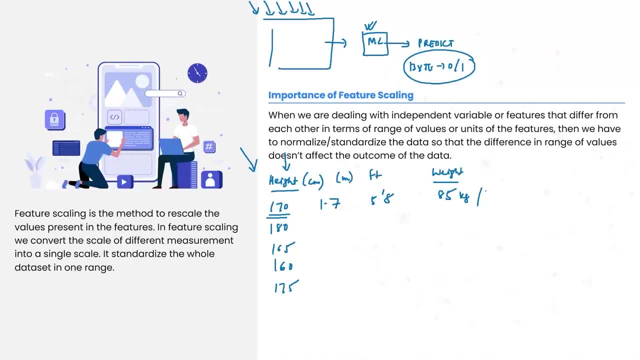 it has to be kg. very rare scenarios it will be lb, but it has to be kg. it cannot be grams, it cannot be any other units. so ultimately these numbers matter. if you have two columns- height and weight, imagine you have this column and this column, you somebody is having 80, 90 kgs, 65, 60 and 75. if you feed this data to your machine learning models, 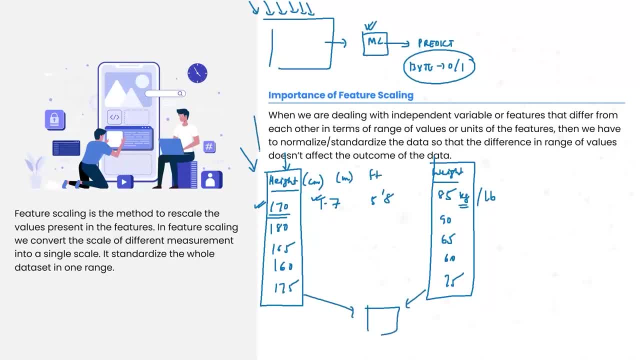 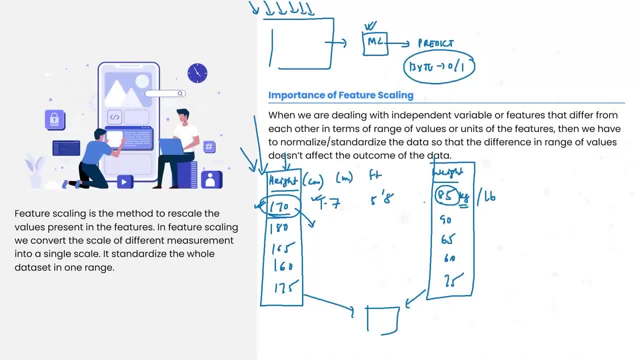 that concept in order to neutralize that concept. in order to neutralize that concept, in order to de-prioritize that, so that machine learning algorithms or your predictive models do not prioritize any column given their data, we should always go for the feature scaling part. if you scale down all the columns, all the numerical columns, to the scaled values, then we 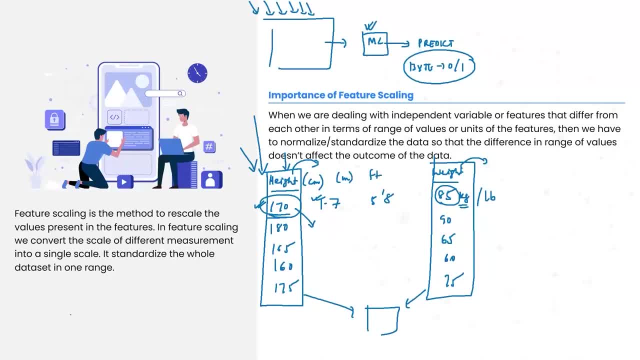 know that they are right now in a proper scale. we'll take a small example to let you understand more about this concept. let's say i have weight 85, 80, 75, 70. i'll give some space so that i can have the feature scaled value. 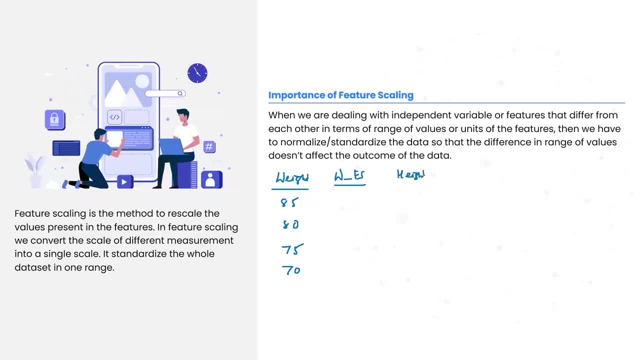 and next i have height and i will have the scaled height value. let's say, height is 170, 165, 168, 170. and i will have the scaled height value. let's say height is 170, 165, 168, 170. these are four people. 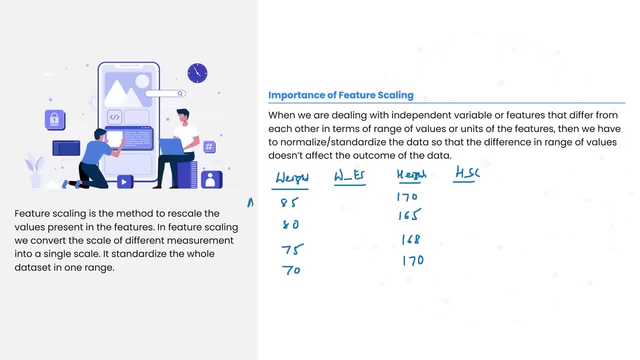 these are four people. these are four people right now. what is the let's say: this is person right now. what is the let's say: this is person right now. what is the let's say: this is person: a person b, person c and person d. a person b, person c and person d. 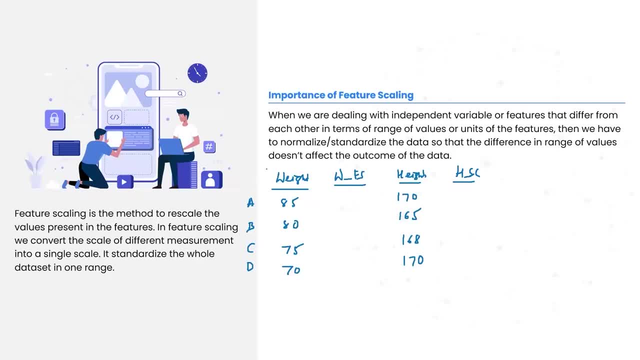 a, person b, person c and person d. now my question here is: which person has? now my question here is: which person has? now my question here is: which person has the highest weight, the highest weight, the highest weight? a has the highest weight. which person has the lowest weight? d has. 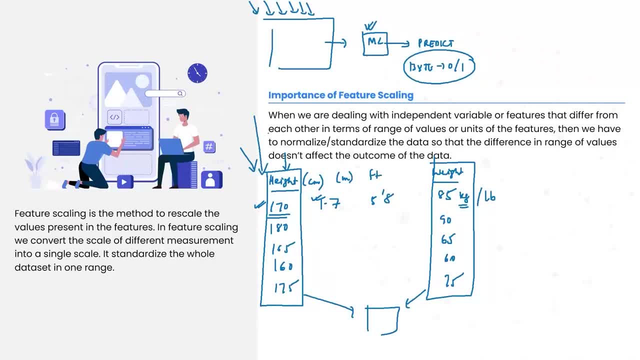 try to give priority to height, because height is larger in number. it is in 100 places. these are intense places. so in order to neutralize that concept, in order to de-prioritize that, so that machine learning algorithms or your predictive models do not prioritize any, 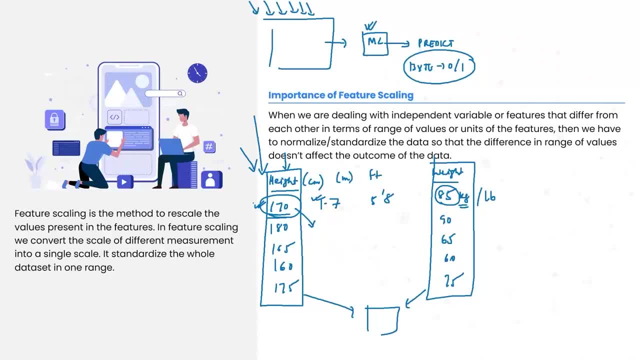 call. given their data, we should always go for the feature scaling part. if you scale down all the columns, all the numerical columns, to the scaled values, then we know that they are right now in a proper scale. we'll take a small example to let you understand more about this concept. let's say i have weight 85, 80, 75. 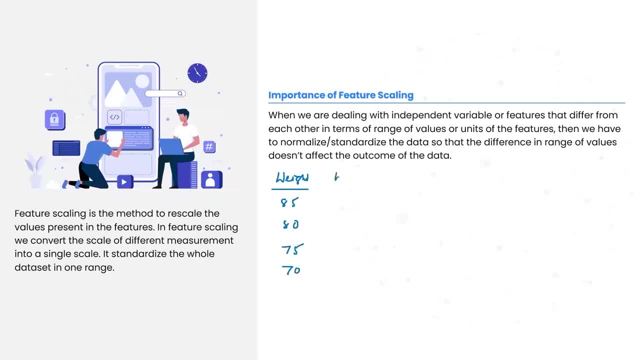 and maybe the window value is 170, 170, 165, 170. i'll give some space so that i can have the feature scaled value brightness to equal 1.ティ to true height and i will have the scaled height value. let's say height is 170, 165, 168, 170. these are people right now. what is the? let's say this person a, person b- human are oldu far right now. what is the veure roster? let's say this is person a, person b- human. the total distance between gender entity whom h orders for diabetes asset can be considered, or persons who are an individual. c sometimes role. 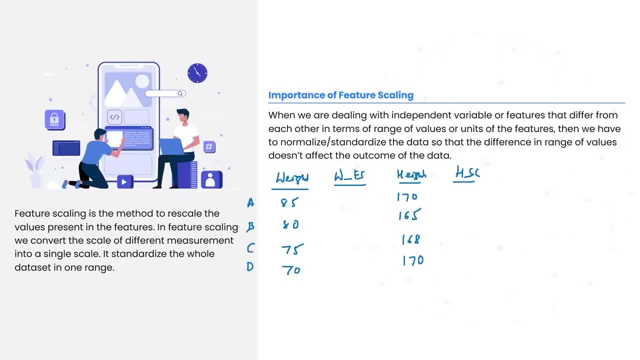 person C and person D. now my question here is: which person has the highest weight? a has the highest weight. which person has the lowest weight? D has the lowest weight, lowest highest height? a and D both have highest height and lowest height is B understood? so these are the feature features that we are. 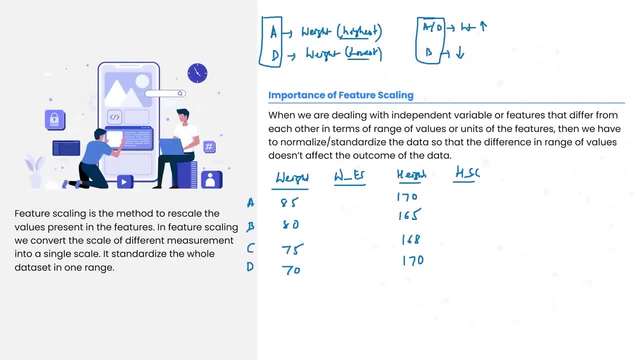 analyzing right. a and D are having highest and lowest weight and a and D combined have highest height and B has the lowest weight. now let's try to analyze this question now. let's try to analyze this question now. let's try to scale it down now. I want to scale it down in a range of 0 to 1. so what? I will. 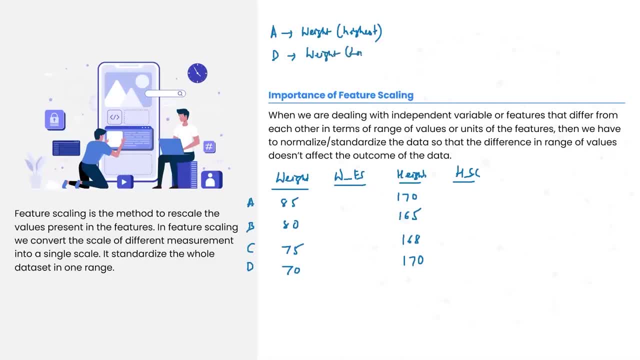 which person has the lowest weight. d has which person has the lowest weight. d has the lowest weight, the lowest weight, lowest highest height. a and d both have highest height and lowest height is b understood. so these are the feature features that we are analyzing. right, a and d are having highest 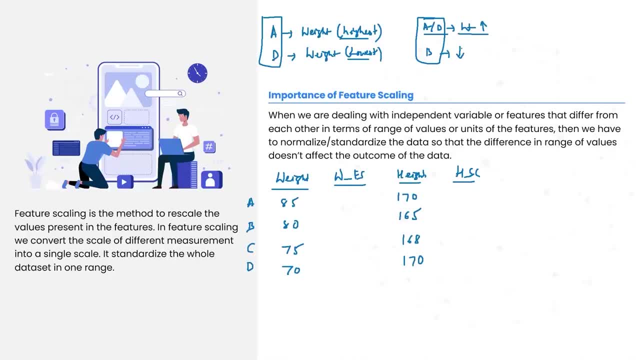 and lowest weight, and a and d combined have highest height and b has the lowest weight. now let's try to scale it down now. i want to scale it down in a range of 0 to 1.. so what i will do is i will divide each number by the highest number, so the scale value will be 85 by 85, which is 1. 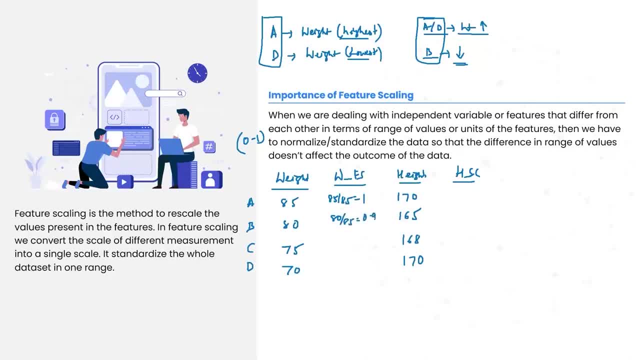 80 by 85, which is, let's say, 0.95. we'll try to take help of calculator: 80 by 85 is 0.95, 75 by 85, 75 by 85 is 0.88 and 70 by 85 is 0.82. 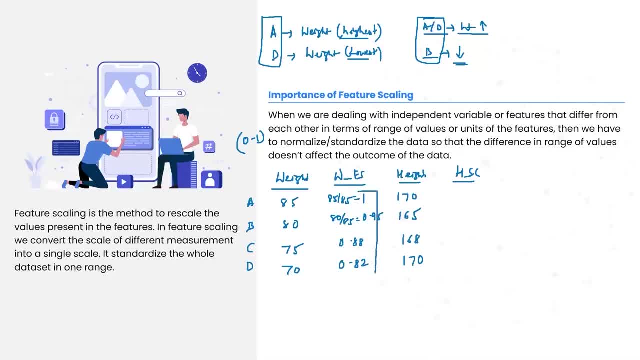 now, these are all my scaled values. what is highest here? person a, still the same with the original value. lowest value is person d- same. so you can see the features, but the importance is not changing. the importance of each feature is same. a used to be the highest weight. d used to be the lowest weight in the scaled down values also. 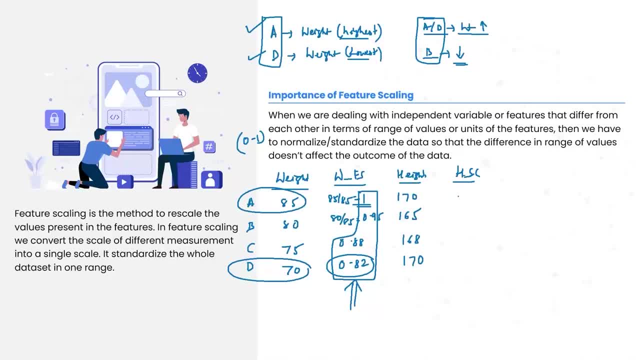 a is highest and d is lowest, same with the height. one 170 by 170 is one, one 165 by 170. 165 by 170 is 0.97. by 170 is 0.98. you can see this is still the highest 170, 170 person a and D still. 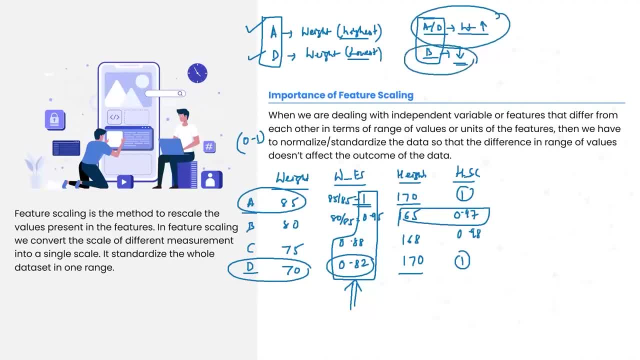 the highest and person B still the lowest. so you can see that the feature importance is not decreasing. however, we are coming up with new features which are nothing but the scaled-down values. now you can see weight is in tense value and height is in hundreds places, but the scaled-down values both are within the 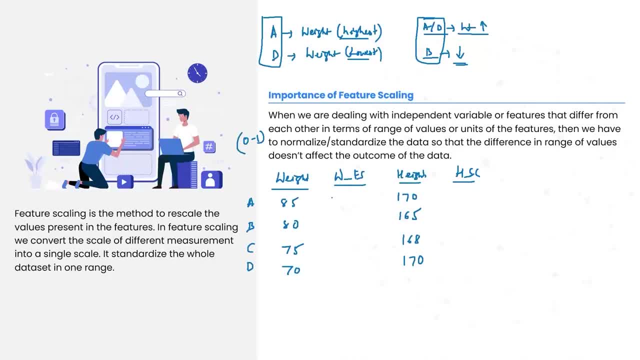 do is I will divide each number by the highest number. so the scale value will be 85 by 85, which is 180 by 85, which is, let's say, point nine five. we'll try to take help of calculator: 80 by 85 is point nine five. seventy five by eighty. 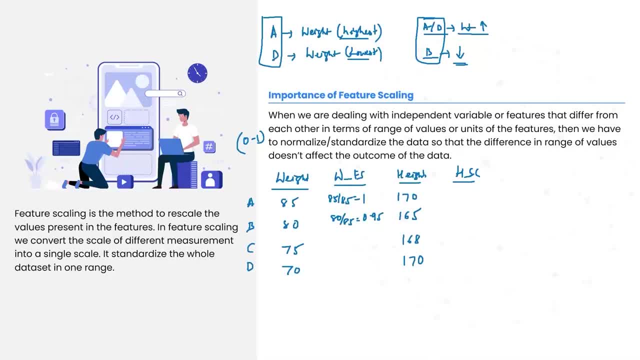 five: 75 by 85 is 0.88 and 70 by 85 is 0.82. now these are all my scaled values. what is highest here? person? a still the same with the original value. lowest value is person d same. so you can see the features. importance is not changing. the importance of each feature is same. a used. 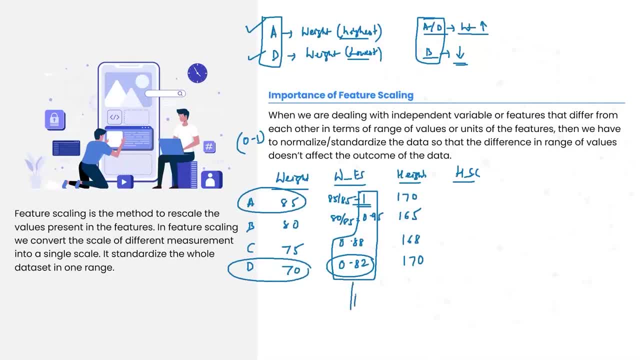 to be the highest weight. d used to be the lowest weight in the scaled down values also, a is highest and d is lowest, same with the height one. 170 by 170 is 1. 1. 165 by 170- 165 by 170 is 0.97. 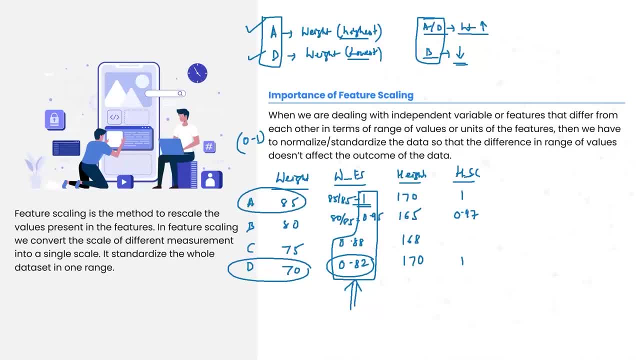 so and 168 by 170 is 0.98. you can see this is still the highest, 170, 170, person a and d still the highest and person b still the lowest. so you can see that the feature importance is not decreasing. however, we are coming up with new features which are nothing but the. 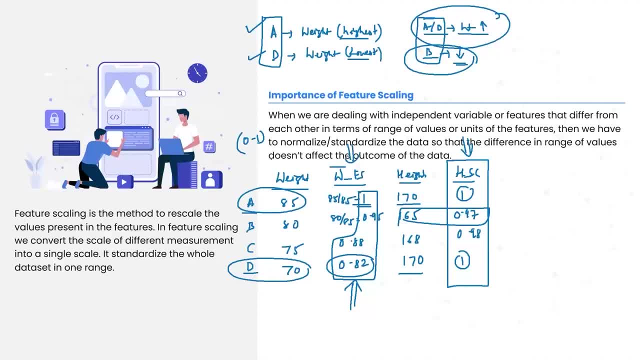 scaled down values- now you can see way- is intense value and height is in hundreds places, but the scale down values both are within the range of 0 to 1 and 0 to 1, so these are most accepted. when it comes to the model building part, feature scaling is blindly one of the most important techniques. when e t. 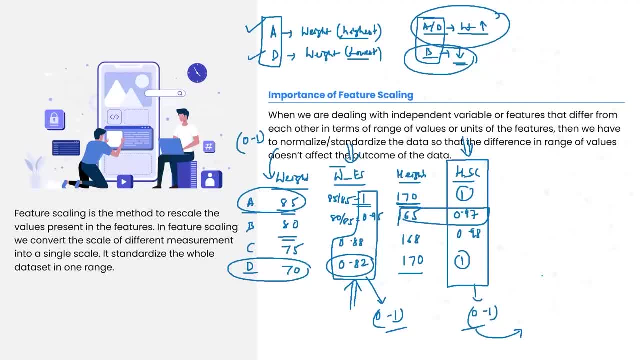 comes to the model building part in the predictive modeling part. however, in the field of e, d, a, as sometimes we perform feature scaling and sometimes we đó operate that feature scaling is going times, we do not perform feature scaling, but understanding feature scaling is very important. majorly one of these techniques i already told you that divide every value with the maximum value. 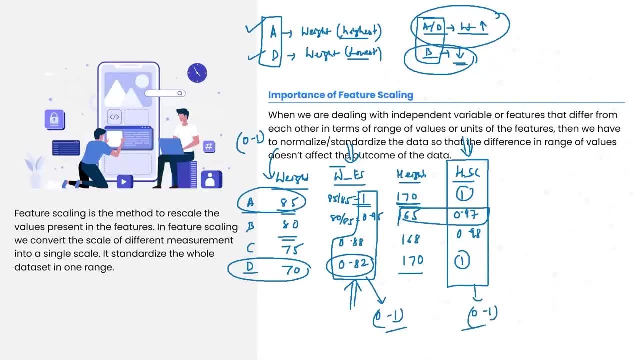 range of 0 to 1 and 0 to 1, so these are most accepted. when it comes to the model building part, feature scaling is blindly one of the most important techniques when it comes to the model building part. in the predictive modeling part, however, in the field of EDA at, sometimes we perform feature scaling and sometimes we 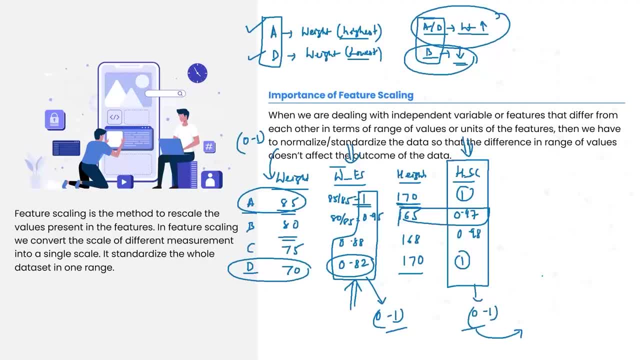 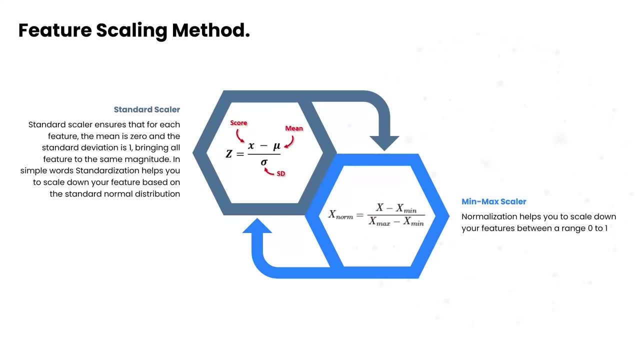 do not perform feature scaling, but understanding feature scaling is very important, majorly one of these techniques. I already told you that divide every value with the maximum value. that can also be a feature scaling technique, but the two most accepted techniques to most accepted feature techniques: feature scaling techniques. 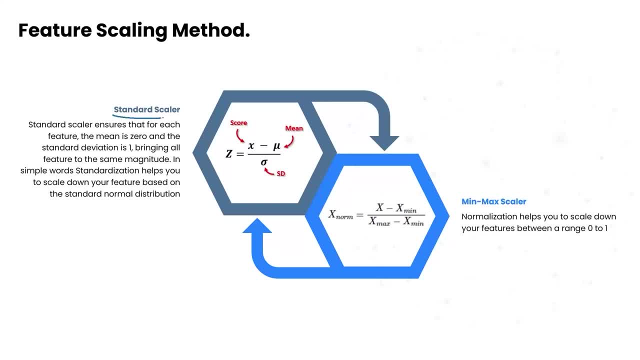 when it comes to statistics is: one of them is standardization and one of them is normalization. standardization and normally addition. the formula of standardization and normalization is very simple. standardization follows the same technique. you have- you must have remember this- normal distribution and the standardized normal distribution. 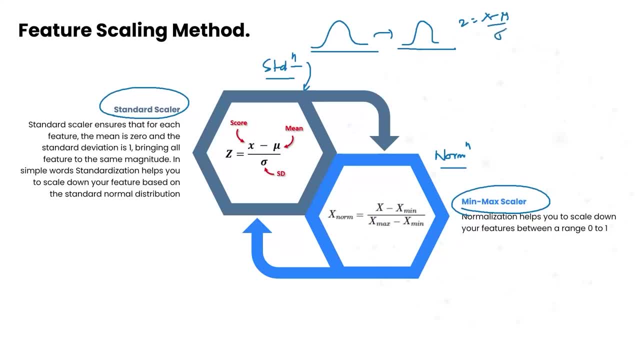 right Z score used to be x minus mu by Sigma. now that's what your standardization is all about. normalization is: the normalized value is x minus x minimum, divided by x maximum minus x minimum. so talking about the theoretical concepts, standard scalar ensures that for each feature, the mean is 0 and the standard deviation is 1.. 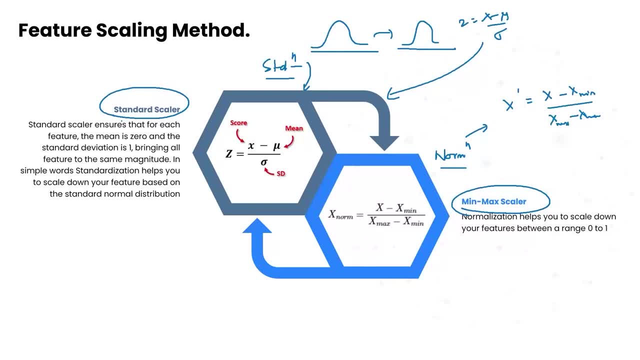 bringing all feature to the same magnitude. in simple words, standardization helps you to scale down your feature based on the standard normal distribution, and normalization helps you to scale down your features between a range of zero to one. which of these techniques are more powerful if you know that your data is somehow following the 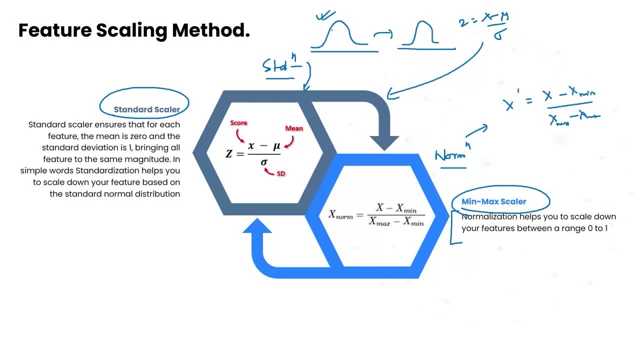 standardization technique, the normal normal distribution technique. you should always go for standardization. if your data is not normally distributed, you should go for normalization. that's all about this particular topic. on feature scaling, in the next video we shall be jumping into the standardization and normalization part separately and then we will talk about the 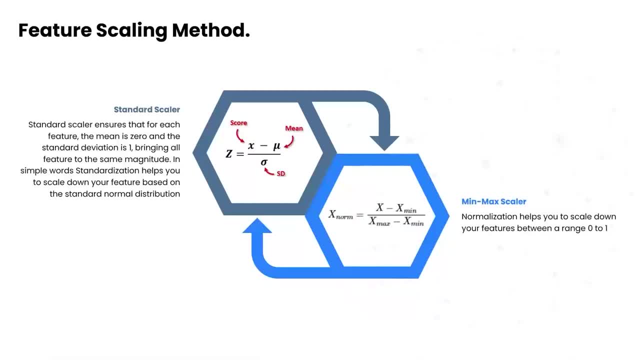 that can also be a feature scaling technique, but the two most accepted techniques, two most accepted feature techniques, feature scaling techniques when it comes to statistics is: one of them is standardization and one of them is normalization, standard digestion and normalization. the formula of standardization and normalization is very simple: standardization follows the same. 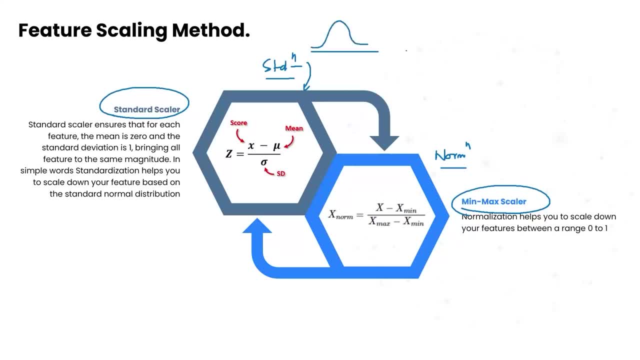 technique you have. you must have remembered this normal distribution and the standardized normal distribution right z score used to be x minus mu y sigma. now, that's what your standardization is all about and normalization is: the normalized value is x minus x minimum, divided by x maximum. 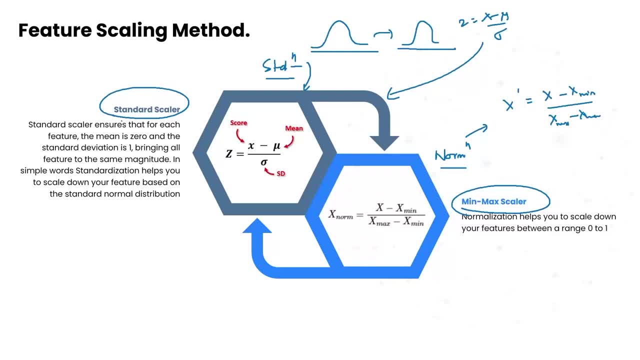 minus x minimum. so talking about the theoretical concepts, standard scalar ensures that, for each feature, the mean is zero and the standard deviation is one, bringing all feature to the same magnitude. in simple words, standardization helps you to scale down the standardization and normalization helps you to scale down your feature based on the standard normal distribution. 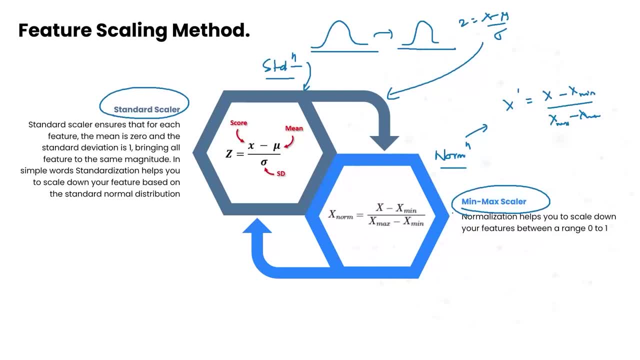 and normalization helps you to scale down your features between a range of zero to one. which of these techniques are more powerful? if you know that your data is somehow following the standardization technique, the normal normal distribution technique, you should always go for standardization. if your data is not normally distributed, you should go for normalization. 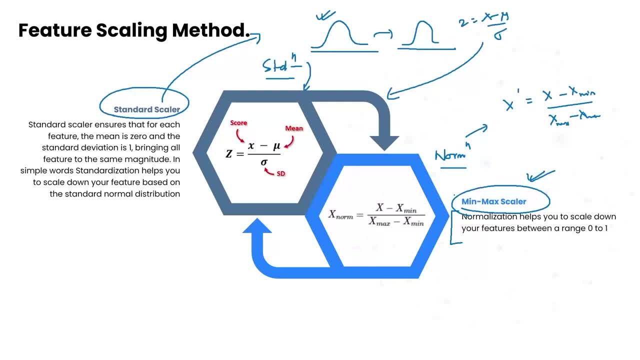 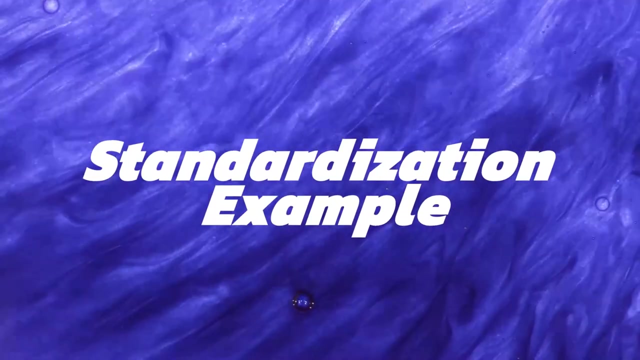 that's all about this particular topic. on feature scaling, in the next video we shall be jumping into the standardization and normalization part separately and then we will talk about the python part. how do we implement feature scaling using a sample data and how do we perform the standardization and normalization? see you in the next video. let's talk about our first. 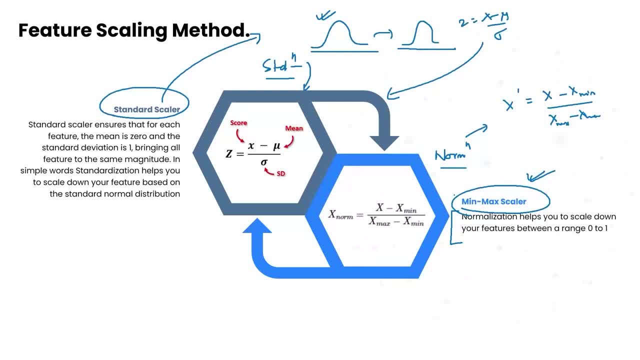 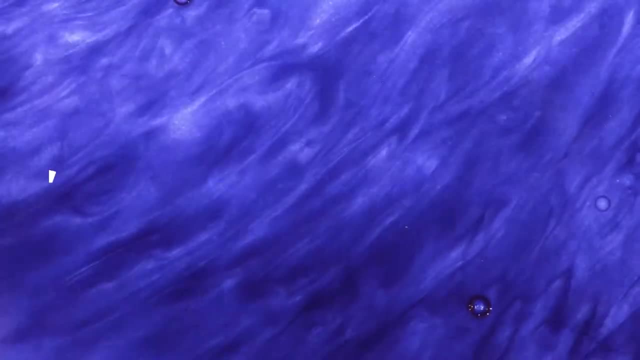 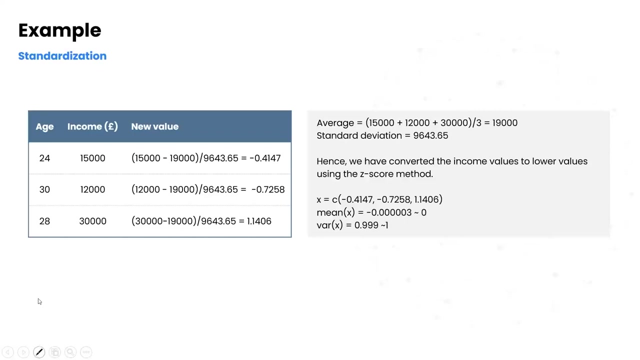 python part. how do we implement feature scaling using a sample data and how do we perform the standardization and normalization? see in the next video. let's talk about our first feature scaling technique. in this video we shall be focusing on the standardization part. we'll try to take an example and show you how standardization can be performed and going. 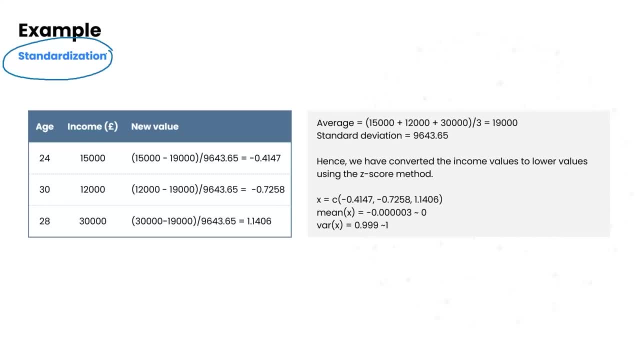 forward. we'll also have a session on how to apply standardization and normalization, both using a python code, using a sample data set. just to repeat once again, standardization in statistics is a process of converting data to z score values based on the mean and standard deviation of the data. the standardized data will have mean equals to 0 and the values will 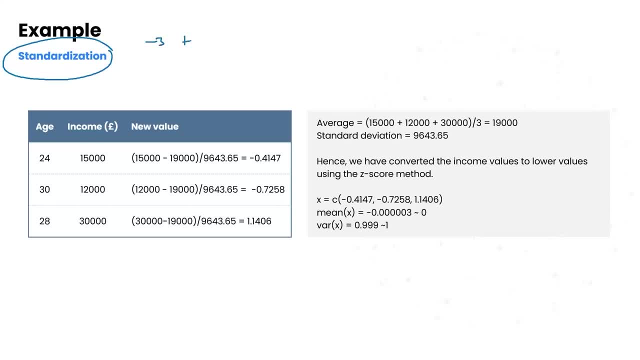 generally range between minus 3 and plus 3.. almost 99.7 percent data will fall. we all know about normal distribution, which basically lies between mu mu plus one standard deviation, plus two standard deviation, plus three standard deviation and going on the left hand side also. 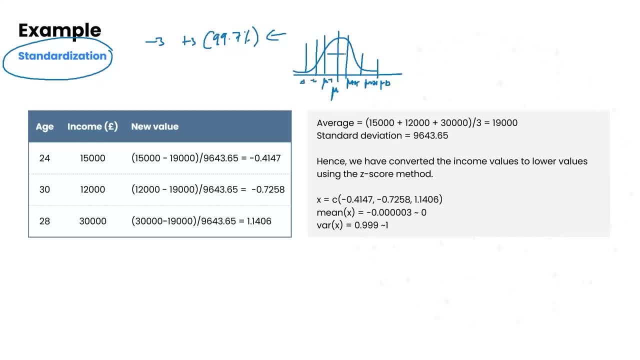 minus one standard deviation, minus two, minus three, 68 percent lies here, 95.4 lies here and 99.7 percent lies here. now, this graph on the scale of z score is nothing but 0, 1, 2, 3 minus 1 minus 2. 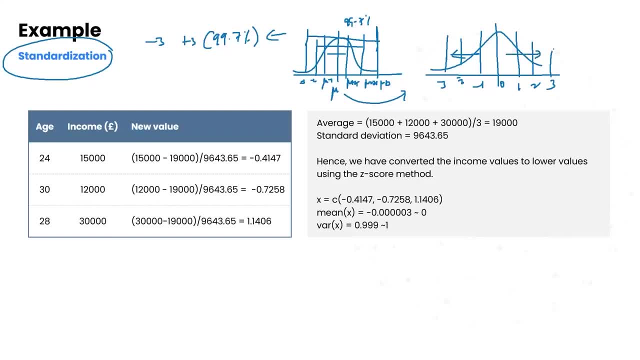 and minus 3.. that means between the range of plus minus 3 z value- 99.7 percent data lies. the formula of z score is very simple. z score is nothing but x minus mu divided by sigma, where mu is the mean value and sigma is 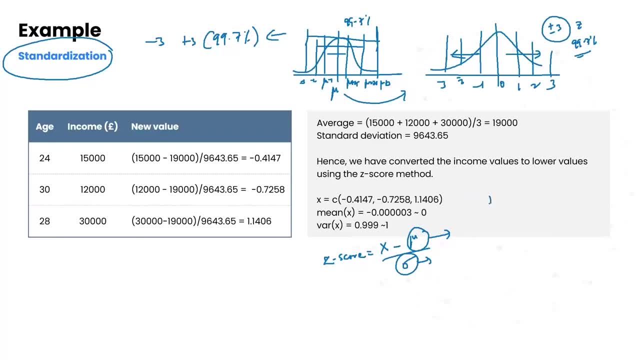 the standard deviation sigma. we all know sigma formula is summation of xi minus mu, square divided by n in the case of population and n minus 1 in the case of sample. so, taking this example on the screen, we have age, we have income, so let's say we are going to standardize the income part. 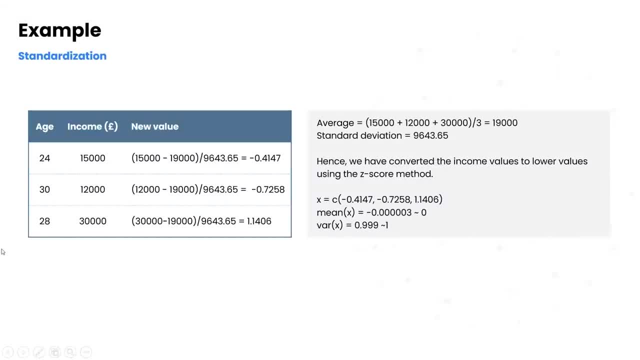 feature scaling technique. in this video we shall be focusing on the standardization part. we'll try to take an example and show you how standardization can be performed and going forward. we'll also have a session on how to apply standardization and normalization, both using a python code, using a sample data set. just to repeat once again, standardization in statistics. 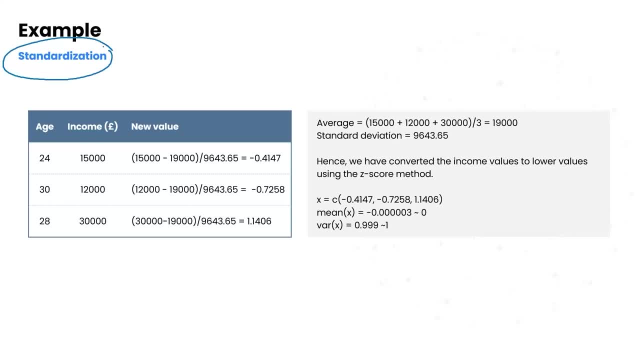 is a process of converting data to z score values based on the standardization and normalization of the data. the standardized data will have mean equals to 0 and the values will generally range between minus 3 and plus 3.. almost 99.7 percent data will fall. we all know about normal distribution. 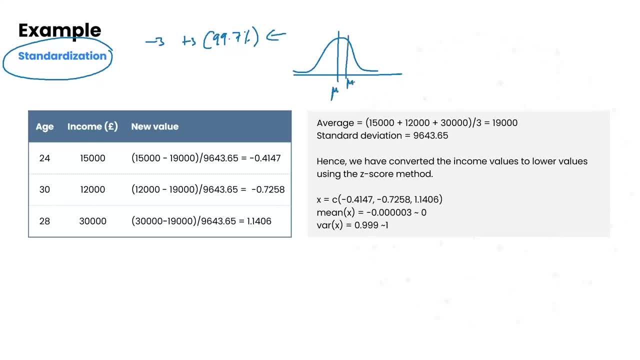 which basically lies between mu, mu plus 1 standard deviation, plus 2 standard deviation, plus 3 standard deviation and going on the left-hand side of the table, we'll talk about standardization and normalization of the data. we have a certain graph from the standardization show here where we have critical. 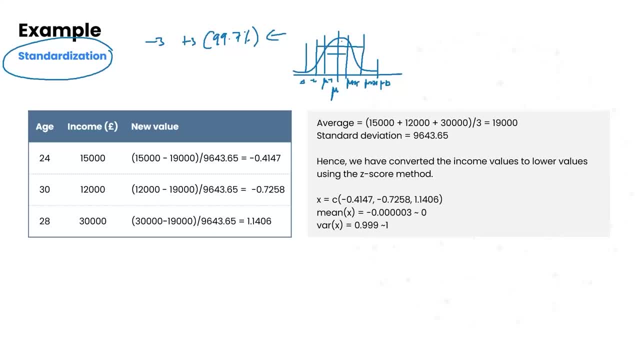 stuff. we call this diagram on our left-hand side also: minus 1 standard deviation, minus 2, minus 3, 68 percent lies here, 95.4 lies here and 99.7 percent lies here. now, this graph on the scale of z-score is nothing but 0, 5, 10, 9. 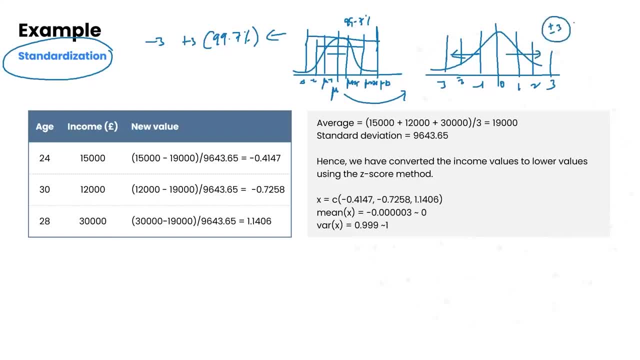 1, 2, 3, аша, 1 2 minus 4- 99.7 percent data lies. the formula of z score is very simple: z score is nothing but x minus mu divided by sigma, where mu is the mean value and sigma is the standard deviation. 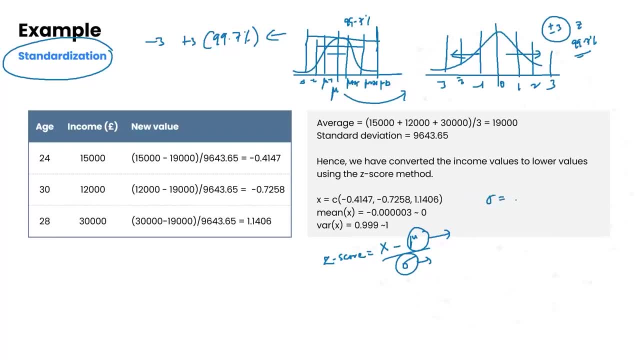 sigma. we all know sigma formula is summation of xi minus mu square, divided by n in the case of population and n minus one in the case of sample. so, taking this example on the screen, we have age, we have income. so let's say we are going to standardize the income part. so let's say i have 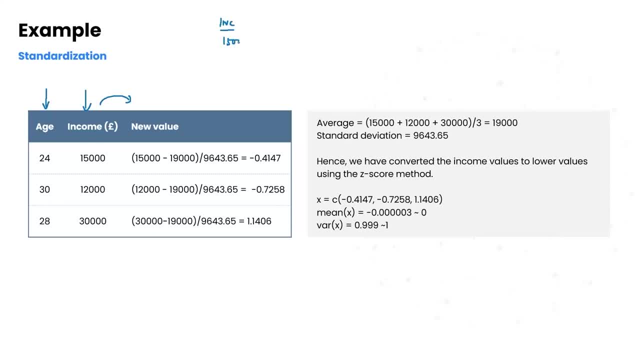 so let's say i have income as fifteen thousand, twelve thousand and thirty thousand thousand. what will be my mean value? my mean value will be sum of fifteen thousand plus twelve thousand plus thirty thousand divided by three, which is twenty seven, plus fifty seven by three, which is almost nineteen thousand. so if i talk about x minus mu by sigma before that, we also 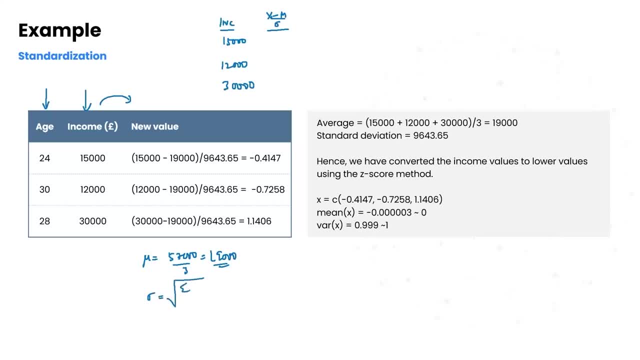 should calculate the sigma using the sigma formula: summation of x, i minus mu, square divided by n. you can also calculate the sigma value. in this case, the sigma value is 9643.65. so if you do this, which is 15, 000 minus the mean value divided by the sigma, same with here, same. 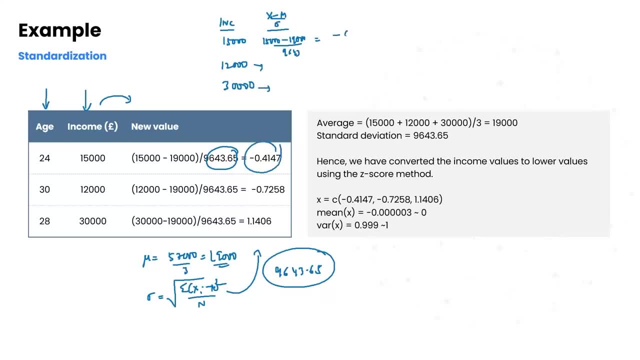 with here and finally, you will be getting the standardized value, which is minus 0.4, minus 0.72 and one point. these are all the standardized values and they are within a scale of something. that's how standardization looks like, so we have to calculate the mean value. 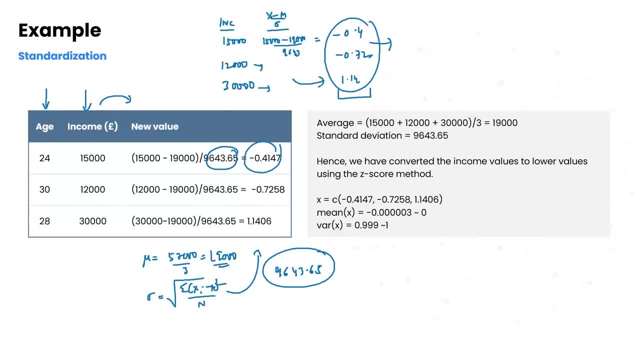 and then we have to calculate the standard deviation and then calculate the standardized value. when it comes to python, we will be introducing one of the libraries, which is called as sk learn library- sk learn- inside that has multiple methods, which starts with standard scale, min max scalar and so many other scalars which we will be using, which performs these activities. 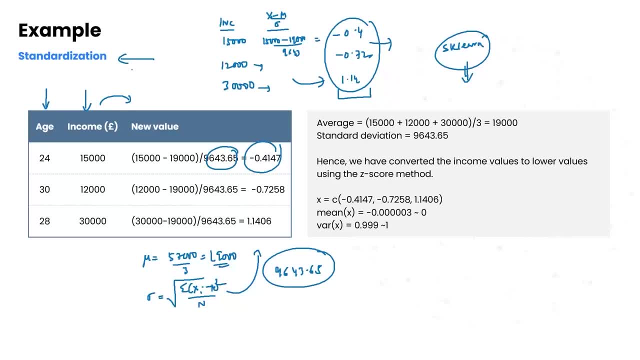 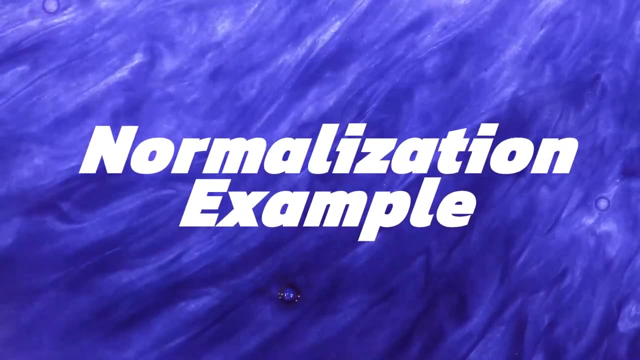 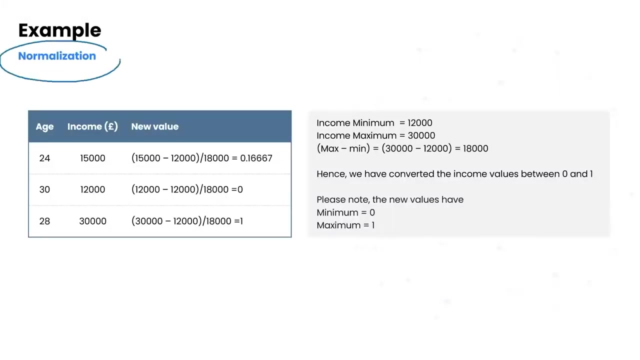 so that's all about this particular example on standardization. in the next video we shall be talking, we'll be taking a similar example and show you how normalization works and going forward, we'll have a separate session on the python part. let's take an example related to normalization. we all know what is normalization: the formula, 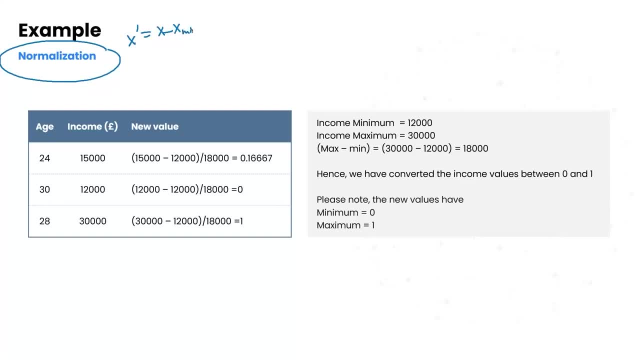 of normalization is x minus x minimum, divided by x maximum minus x minimum. it's another way of scaling down the values to a particular scale. right? if you have multiple features with different values, you can scale down the values to a particular scale, right? if you have multiple. 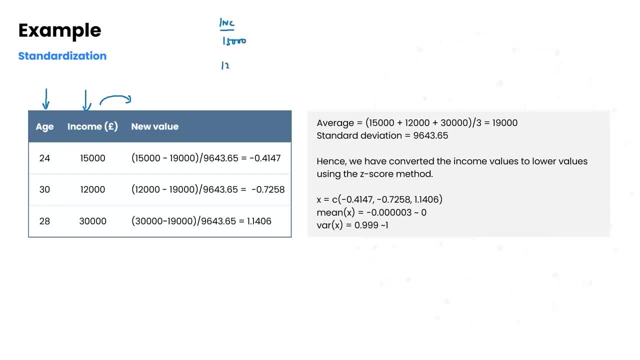 income as fifteen thousand, twelve thousand and thirty thousand. what will be my mean value? my mean value will be sum of fifteen thousand plus twelve thousand plus thirty thousand divided by three, which is twenty seven plus fifty seven by three, which is almost nineteen thousand. so if i talk about x minus mu by sigma, before that we also should calculate: 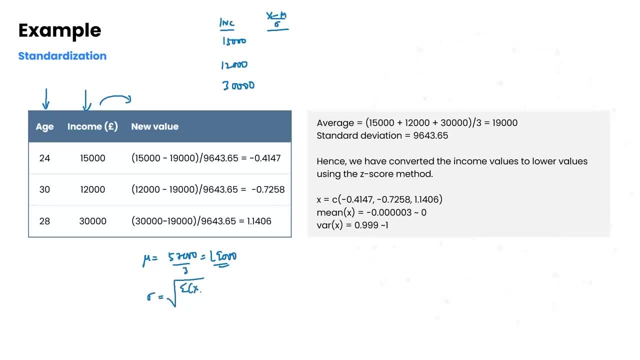 the sigma. using the sigma formula: summation of xi minus mu square divided by n, you can also calculate the sigma value. in this case, the sigma value is nine, six, four, three point six, five. so if you do this, which is fifteen thousand minus the mean value divided by the sigma, same with here, same with here and finally, you will be getting 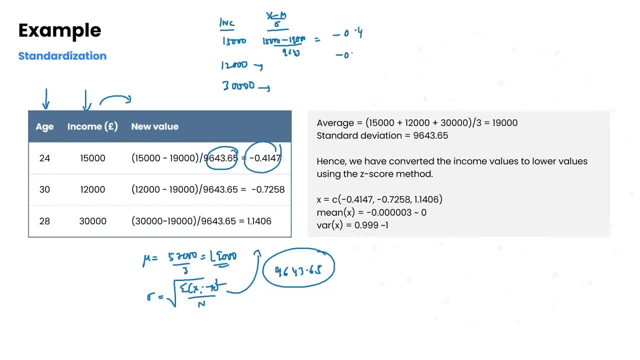 the standardized value, which is minus point four, minus point seven, two and one point one four, and these are all the standardized values and they are within a scale of something. that's how standardization looks like. so we have to calculate the mean value and then we have to calculate the standard deviation and then calculate the standardized. 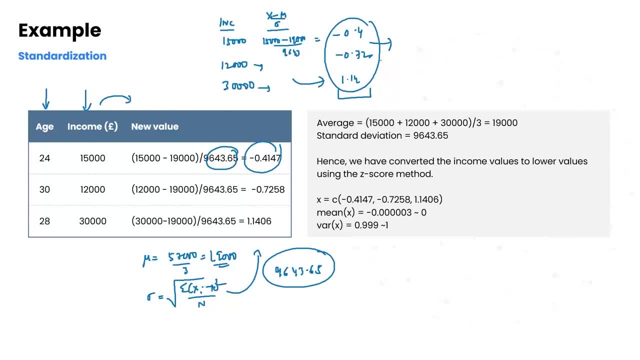 value. when it comes to python, we will be introducing one of the libraries, which is called as sk learn library- sk learn- inside that has multiple methods, which starts with standard scalar, mean, max scalar and so many other scalars which we will be using- which performs these activities. so that's all about this particular example on standardization. in the next video we 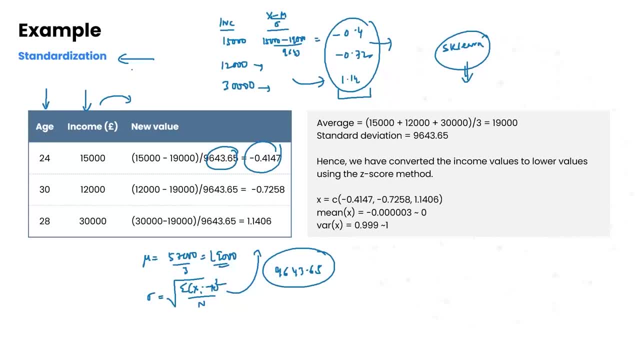 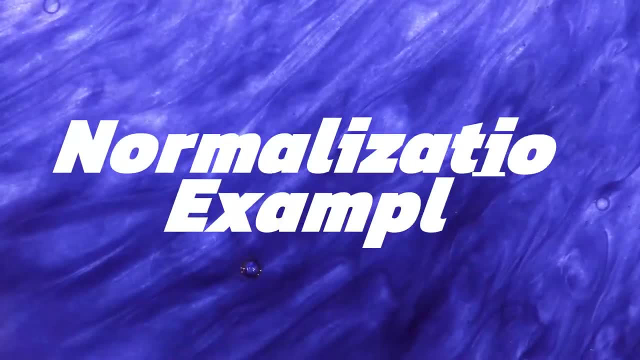 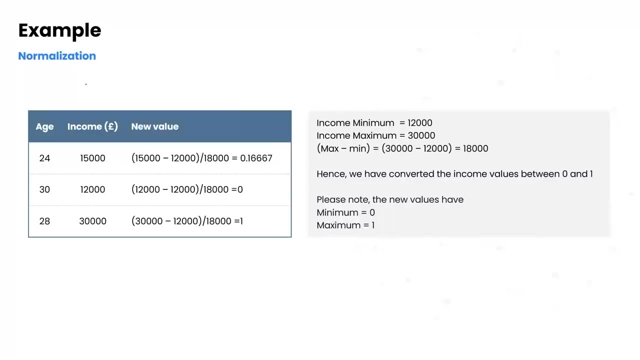 shall be talking. uh, we'll be taking a similar example and show you how normalization works and, going forward, we'll have a separate session on the python part. let's take an example related to normalization. we all know what is normalization. the formula of normalization is x minus x minimum, divided by x maximum minus x minimum. it's another way of scaling down the 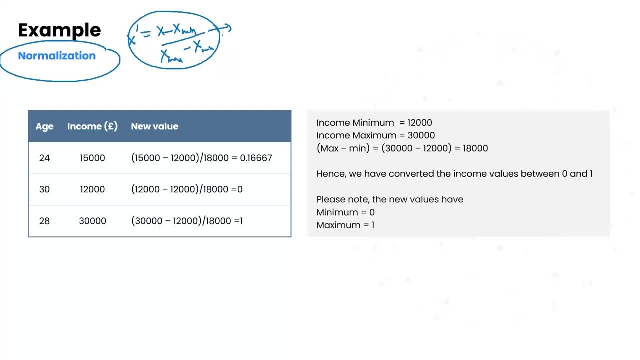 values to a particular scale. right, if you have multiple features with different numbers. one of the features is in tens format, one of the features is in thousands format. so when you pass these raw values to your machine learning or to your predictive model, they will be biased, they will. 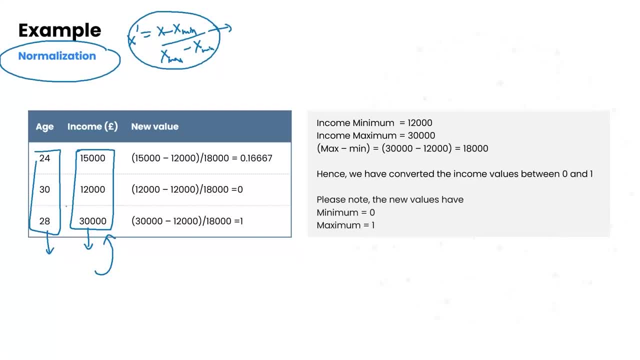 be biased towards income with an income. also, they will be biased towards these larger numbers. so, in order to have an unbiased model, we perform feature scaling. let's try to take the same example and see how do we perform normalization in this particular example. so we have income fifteen. 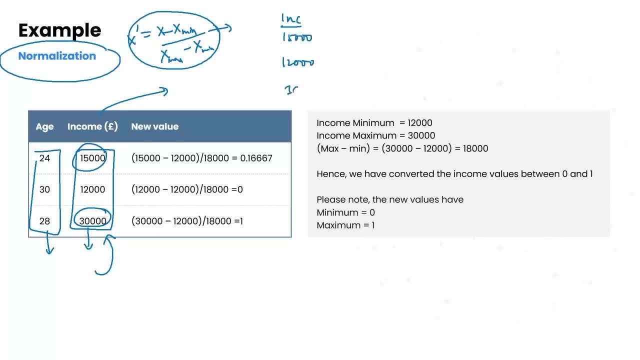 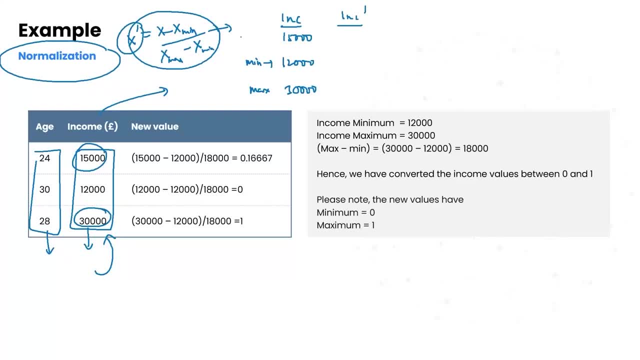 dash, which is the normalized value. x minus x mean fifteen thousand minus twelve thousand, which is three thousand, divided by thirty thousand minus twelve thousand eighteen thousand, which is three by eighteen, which is one, by six, which is zero, point one, six, dot, dot dot. similarly for the second one. 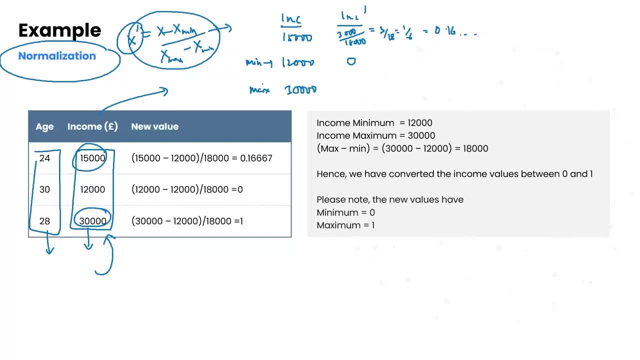 the numerator will be zero. so it will be zero. for the third one, the numerator will be thirty minus twelve, which is eighteen by eighteen, which will be one. so the normalized values are point one, six, zero and one, and, as we all know, that normalization always lies within the range of zero to one. the 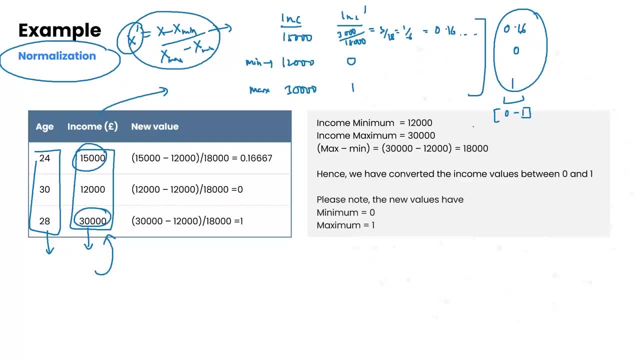 maximum value could be one and the minimum value could be zero. so that's all about normalization. in the next video. we shall be doing that in the next video. we shall be doing that. in the next video we jumping into the python part and we will be introducing you some of the python libraries. 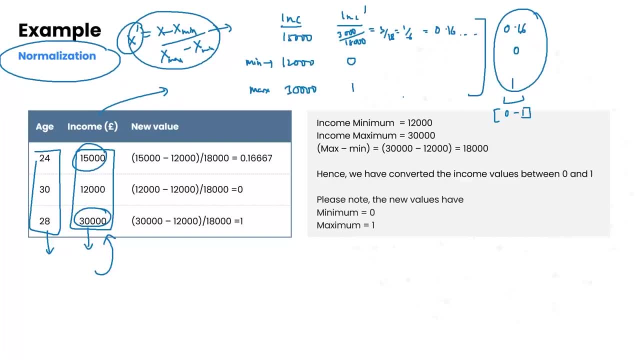 that you might not know till now. we will be introducing them, installing them and using those libraries. we will be performing the same standardization and normalization so that you can have some practical knowledge on these topics. that's all about this particular video on the normalization example. see you in the next video. 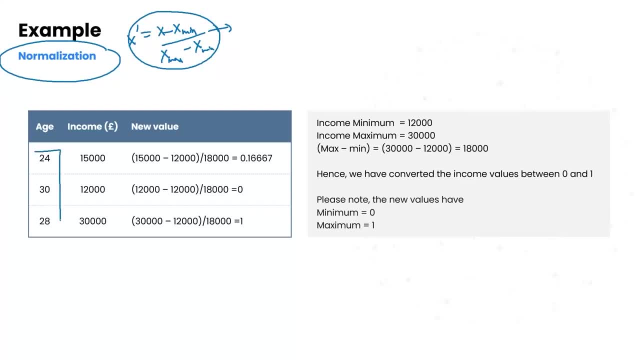 different numbers. one of the features is in tens format. one of the features is in thousands format. so when you pass these raw values to your machine learning or to your predictive model, they will be biased. they will be biased towards income with an income also, they will be biased. 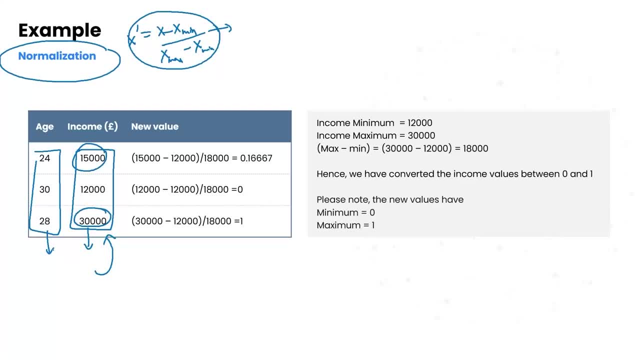 towards these larger numbers. so, in order to have an unbiased model, we perform feature scaling. let's try to take the same example and see how do we perform normalization in this particular example. so we have income fifteen thousand, twelve thousand and thirty thousand. in this case, we'll 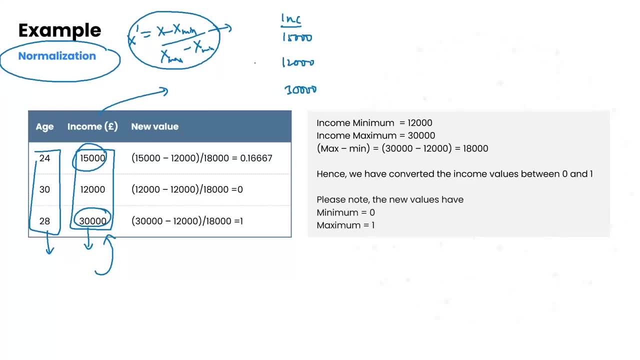 have to figure out what is the minimum value. the minimum value is this. the maximum value is this. so what is the income dash, which is the normalized value? x minus x mean 15 000 minus 12 000, which is by 30 000 minus 12 000, 18 000, which is 3 by 18, which is 1 by 6, which is 0.16. dot, dot, dot. 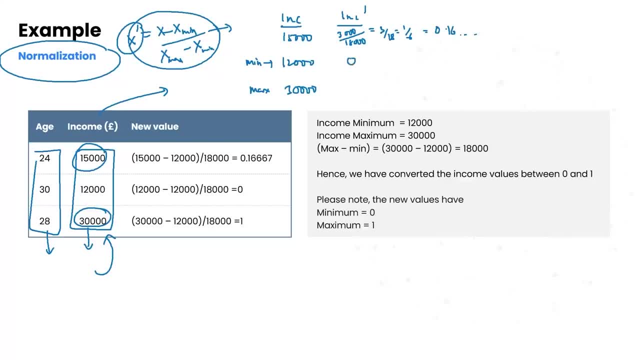 similarly, for the second one, the numerator will be 0, so it will be 0.. for the third one, the numerator will be 30 minus 12, which is 18 by 18, which will be 1.. so the normalized values are 0.16, 0 and 1 and, as we all know that normalization always lies within the range of 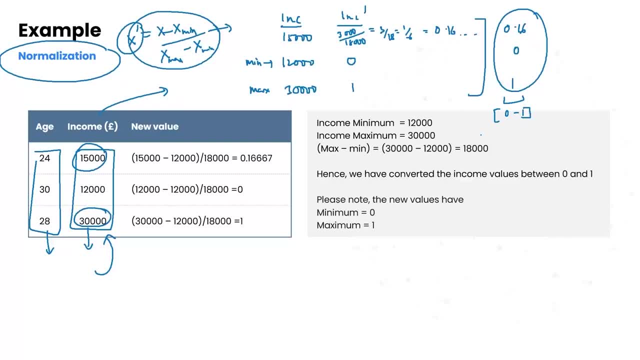 0 to 1, the maximum value could be 1 and the minimum value could be 0. so that's all about normalization. in the next video we shall be jumping into the python part and we will be introducing you some of the python libraries that you might not know till now. we will be 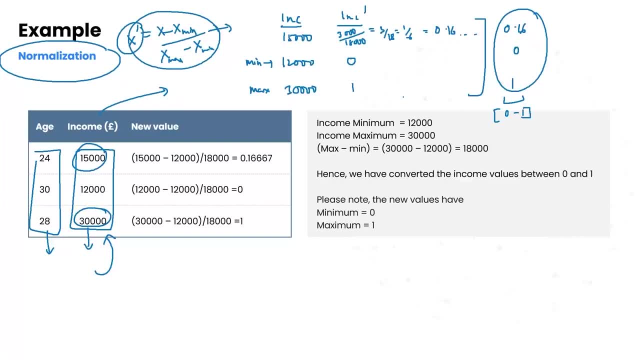 introducing them, installing them and using those libraries. we will be performing the same process for the power of the terminal system. we will be introducing them for the standardization and normalization so that you can have some practical knowledge on these topics. that's all about this particular video. on the normalization example, see in the next video. 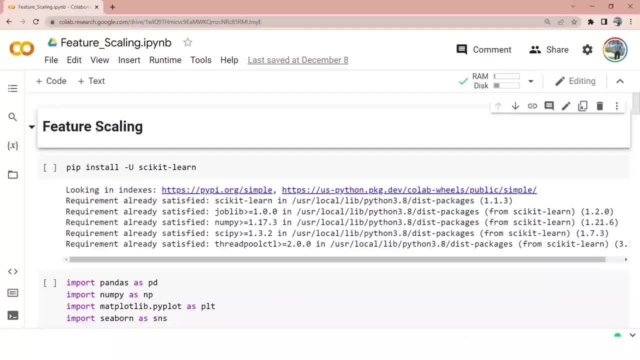 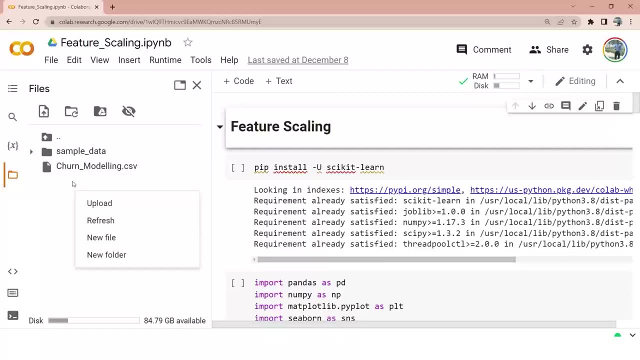 let's get started with the python part. so, as usual, i'm using google collab and i have just right clicked and uploaded my csv file. in case you are using jupyter notebook, you can use your local directory, fetch the data set and get started with this exercise, or else there are other ways. 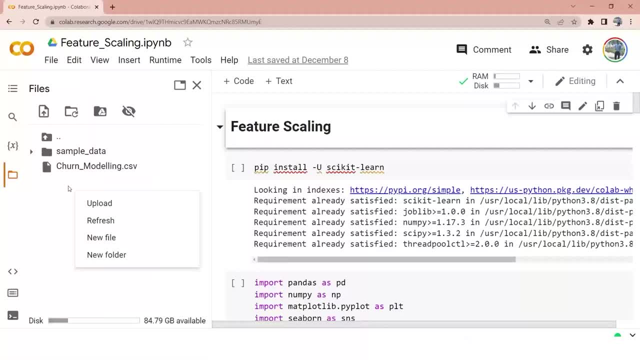 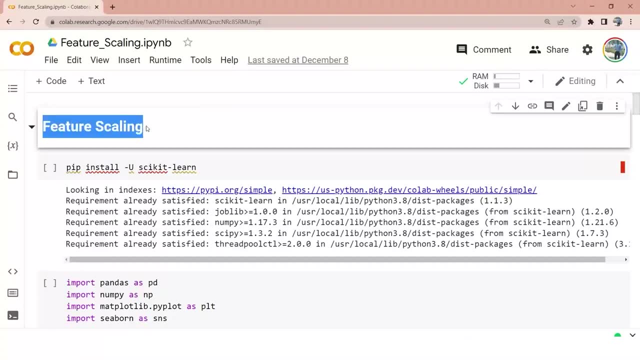 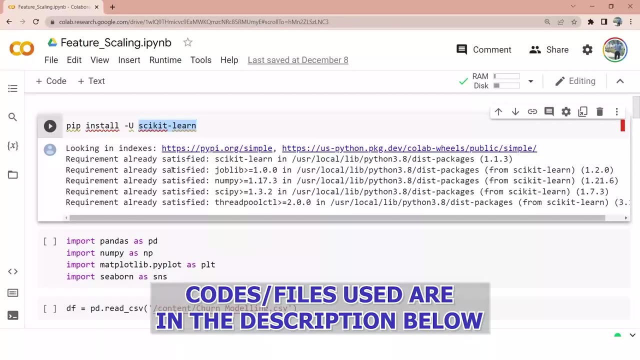 to import from a google drive as well. i'm pretty much sure you must be aware of those things. so, getting into the topic of feature scaling, the first thing that we need to do for feature scaling is to install a library called saikhityal, which is also called as skler. in my case, i have already installed this library. 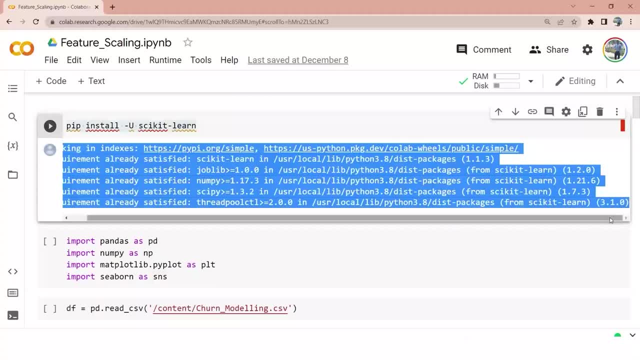 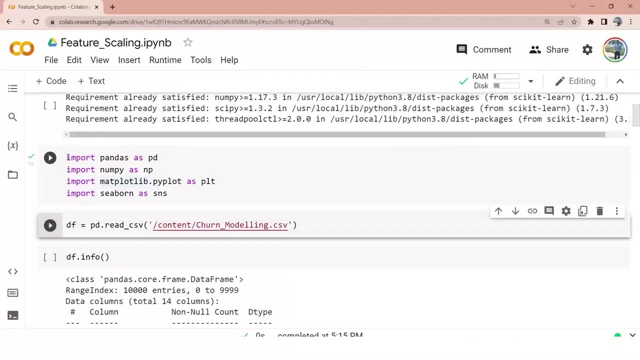 so for me it is giving me a warning. that requirement already satisfied, right? so i'll quickly get started with my exercise. i have imported all the libraries which is nambai pandas matplotlib, seaborn, etc. and i have started all the libraries which is nambai pandas, matplotlib. bottlenecks, simplest utility, environmental management and how to do that work which is just hung as well- that is in the chat- all these easy tools which you don't even need to find that from等等 pir differential. we have, you know it, and we have also foundMEDIT because you 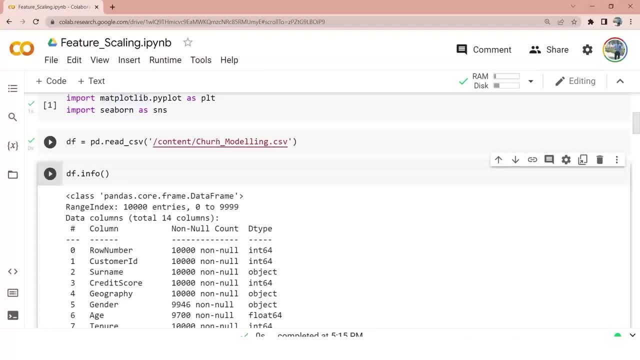 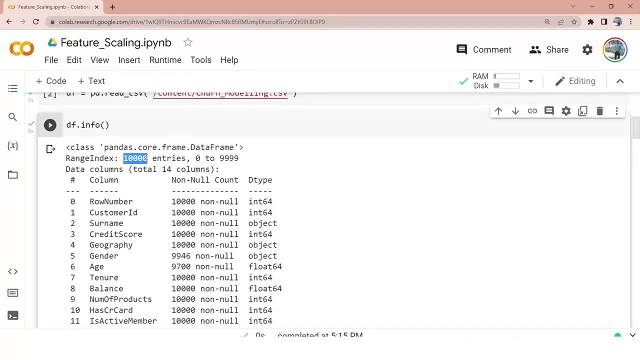 have very few questions, so please feel free to ask something which might not even provide an answer to them. in the comments, any additional questions or recommendations which you will get. started reading the file churn modelingcsv. and upon doing dot info, this is what i'm getting: that it is having 10 000 records and these are the different columns. some of them have null values. 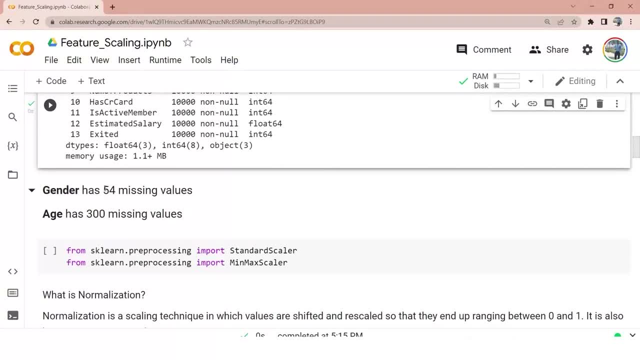 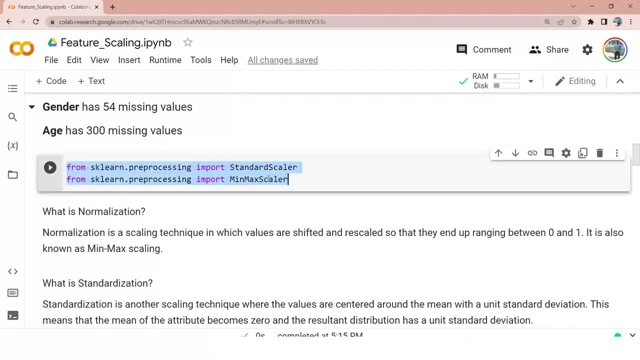 and then we'll get started. gender has 54 missing values. age has 300 missing values. here i'm importing the standard scalar and min max scalar. these are the two things that's important for sklearn and using these two functions, these two you know methods inside the sklearn library. 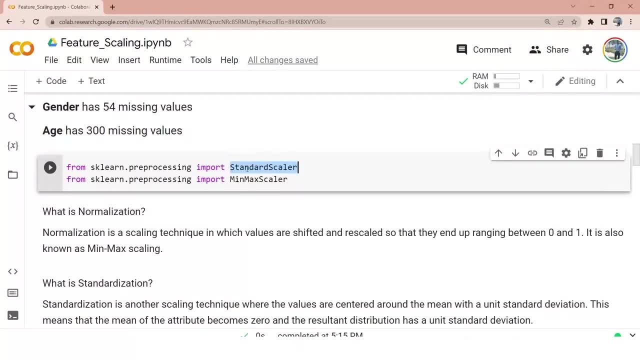 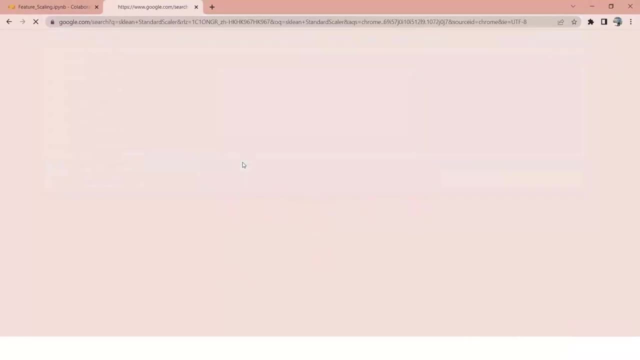 you will be performing standardization and normalization. so this standard scalar is basically the standardization technique and this min max scalar is basically for the normalization part. if you want to know more about this, probably go ahead and just search sklearn standard scalar. you will be getting the 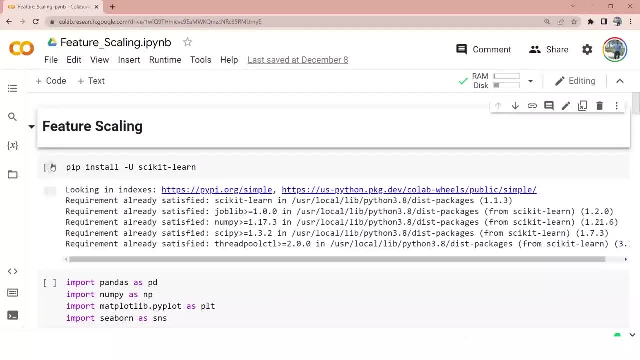 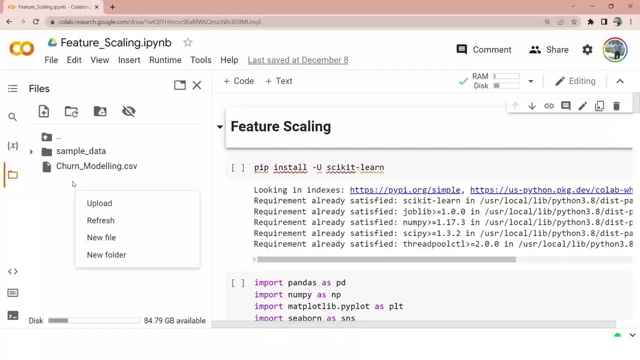 let's get started with the python part. so, as usual, i'm using google collab and i have just right clicked and uploaded my csv file. in case you are using jupyter notebook, you can use your local directory, fetch the data set and get started with this exercise, or else there are other ways to. 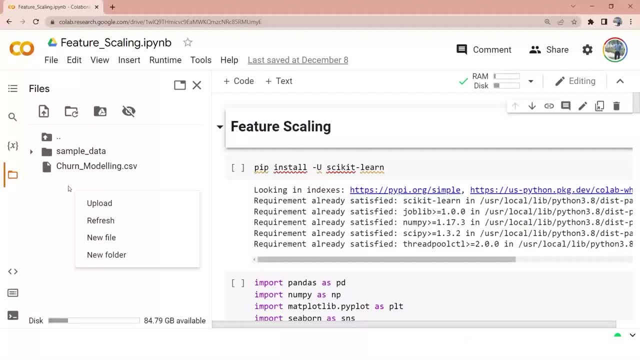 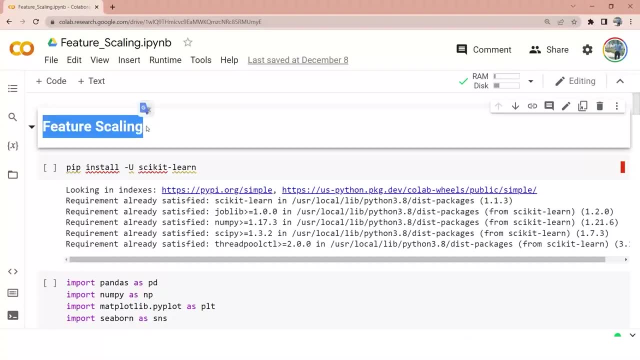 import from a google drive as well. i'm pretty much sure you must be aware of those things. so, getting into the topic of feature scaling, the first thing that we need to do for feature scaling is to install a library called a psykit learn, which is also called 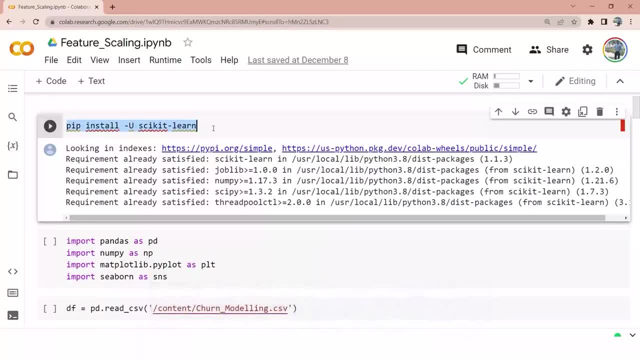 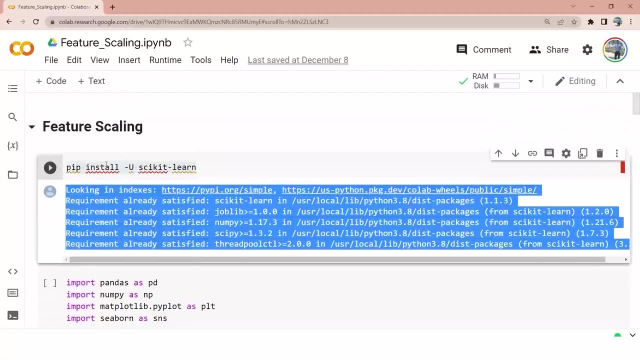 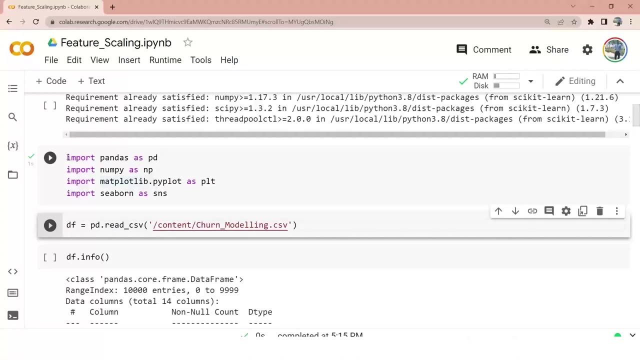 as sklearn. in my case, i have already installed this library, so for me it is giving me an warning. that requirement already satisfied, right? so i'll quickly get started with my exercise. i have imported all the libraries, which is numby, pandas, matplotlib, seaborn, etc. and i have started. 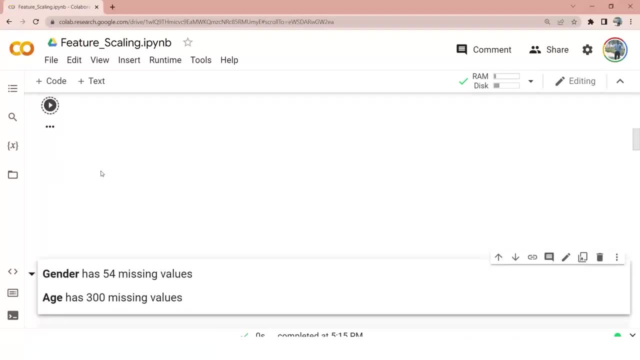 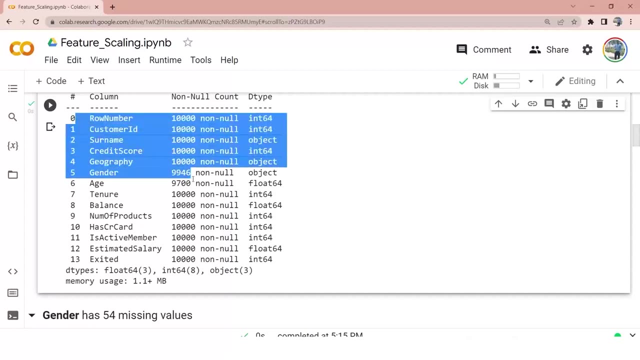 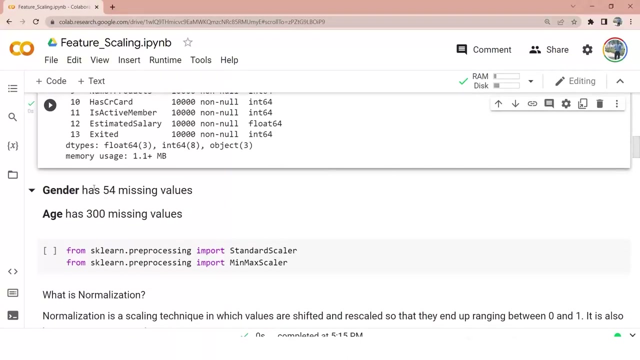 reading the file churn modelingcsv and upon doing dot info, this is what i'm getting: that it is having 10 000 records and these are the different columns. some of them have null values, and then we'll get started. gender has 54 missing values. age has 300 missing values. here i'm importing the 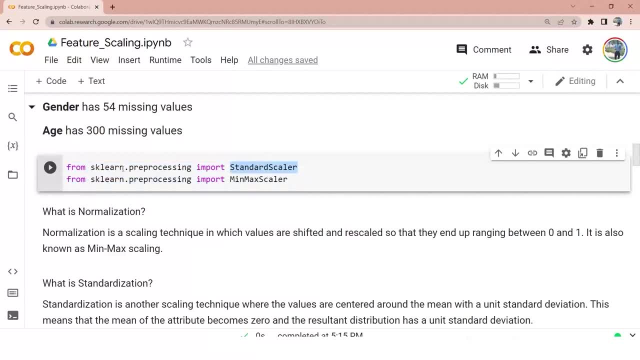 standard scalar and minmax scalar. these are the two things that's important for sklearn and using these two functions- these two you know methods- inside the sklearn library you will be performing standardization and normalization. so this standard scalar is basically the standardization technique and this minmax scalar is basically for the normalization part. if you want to know. 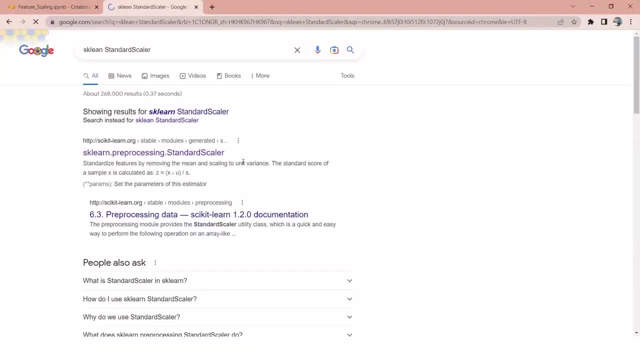 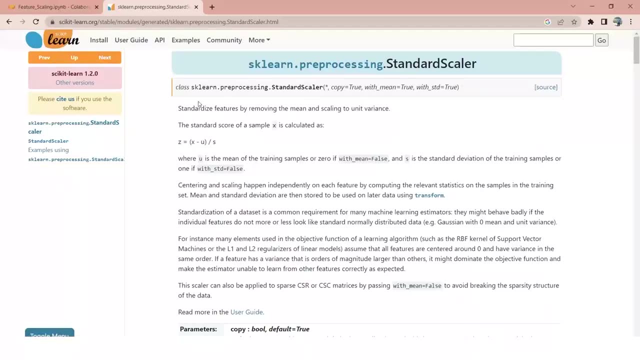 more about this. probably go ahead and just search sklearn- standard scalar. you will be getting the documents, official documentations of psykit learning and you can go through this particular page to understand more about the standard scalar. standardized features by removing the mean and scaling to unit variance, the standard. 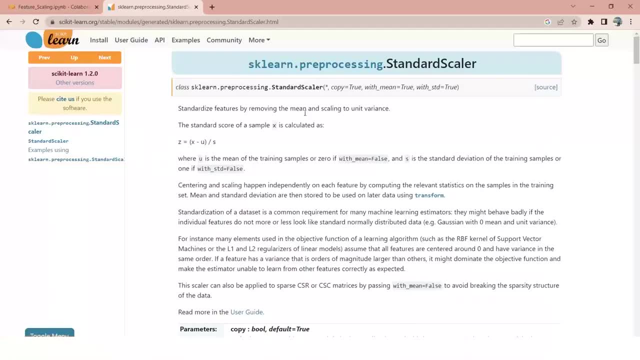 the documents, official documentations of scikit learning, and you can go through this particular page to understand more about standard scaling, standardized features. by removing the mean and scaling to unit variance, the standard score of a sample x is calculated as z equals to x minus mean divided by sigma, which we already know right, and the same goes with: 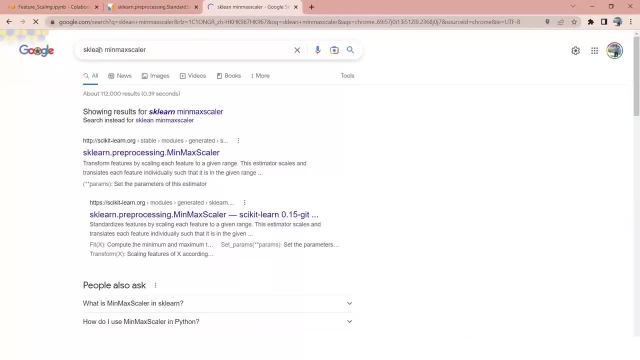 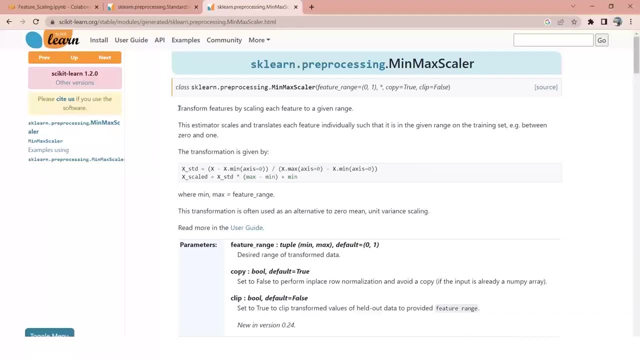 normalization. also, if you just search sklearn min max scalar, you will be getting their official documentation. go ahead and you will be able to understand about this particular thing. transform features by scaling each feature to a given range. now, going ahead. we all know what is normalization and what is. 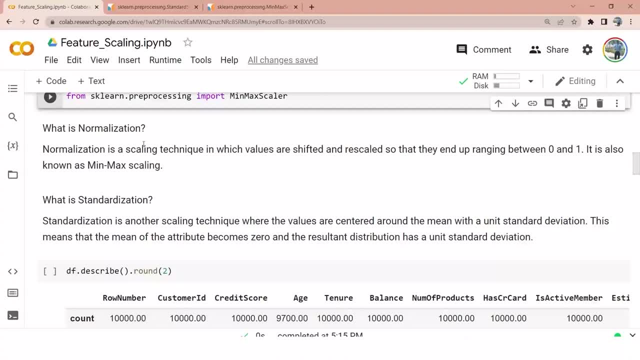 standardization. normalization is a scaling technique in which values are shifted and rescaled so that they end up ranging between 0 and 1.. it is also known as mean max scaling. what is standardization? it's another scaling technique where the values are centered around the 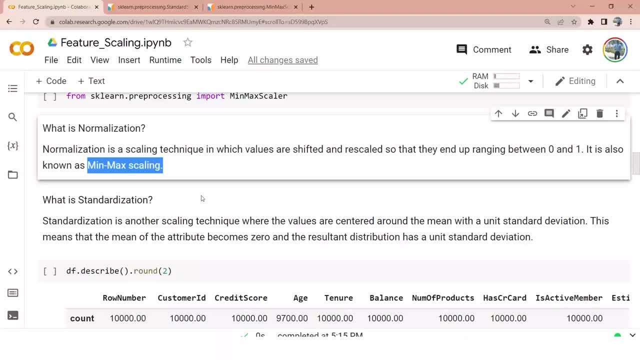 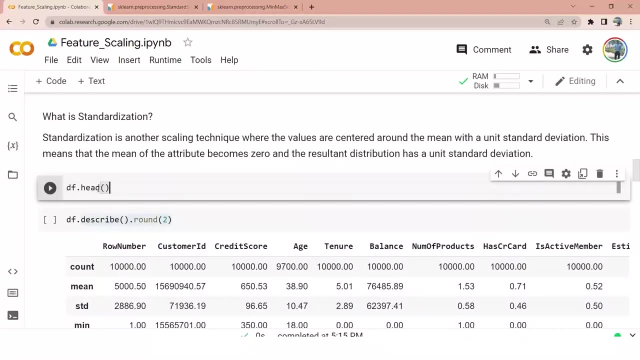 mean with a unit standard deviation. this means that the mean of the attribute becomes 0 and the resultant distribution has a unit standard deviation. first of all, i want to let you know how our data frame looks like. in order to show the data frame, i will just print dot head and you can. 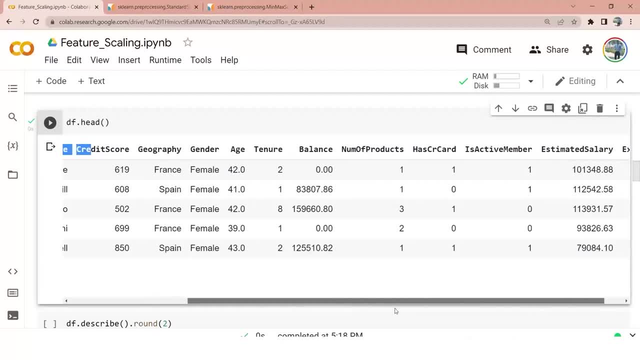 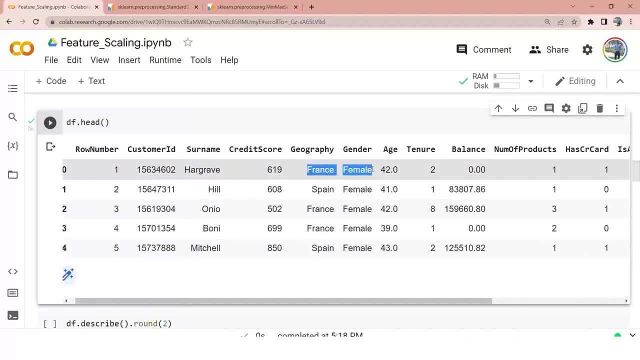 see i have row number, customer id, surname, bla bla bla. so many columns. one thing you must notice is some of these columns are having categorical values and some of these columns are, you know, not important for our analysis. now, just in case your columns are not important for your analysis, 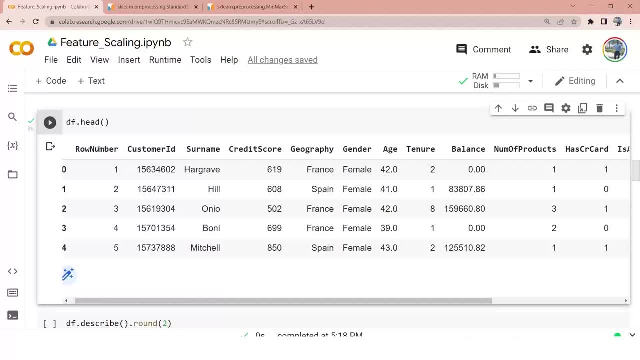 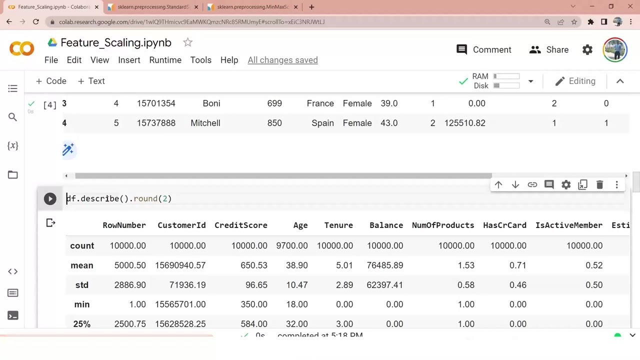 simply remove them. in this exercise we are not focusing on that part. we are focusing majorly on how to perform standardization and normalization. that's why i will not be showing you all those things. so what i will do is i'll quickly do the dot describe method. 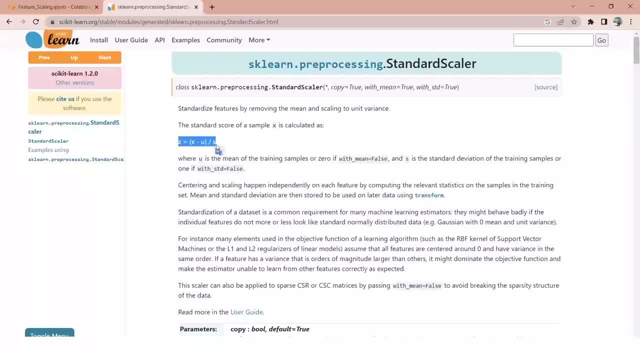 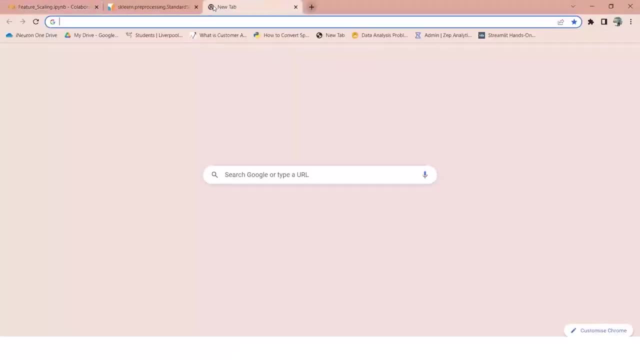 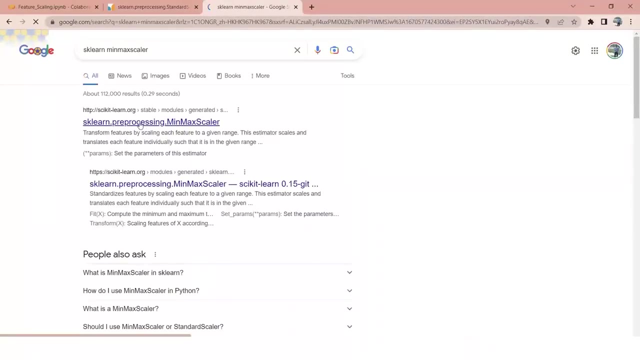 score of a sample x is calculated as z equals to x minus mean divided by sigma, which we already know right, and the same goes with normalization. also, if you just search sklearn minmax scalar, you will be getting their official documentation. go ahead and you will be able to understand. 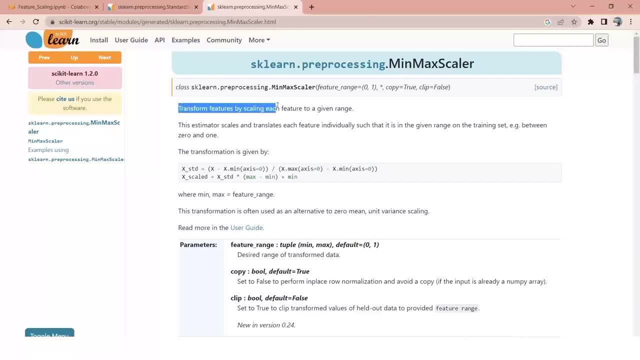 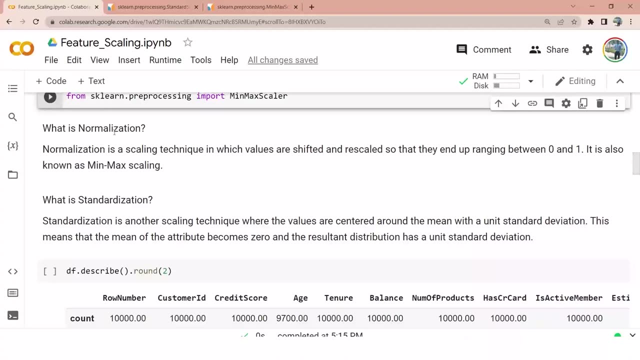 about this particular thing: transform features by scaling each feature to a given range. now going ahead, we all know what is normalization and what is standardization. normalization is a scaling technique in which values are shifted and rescaled so that they end up ranging between zero and one. 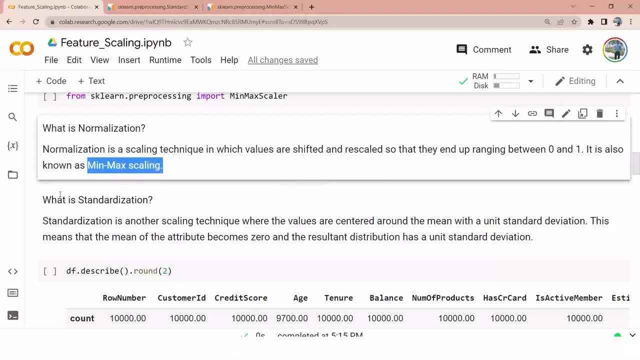 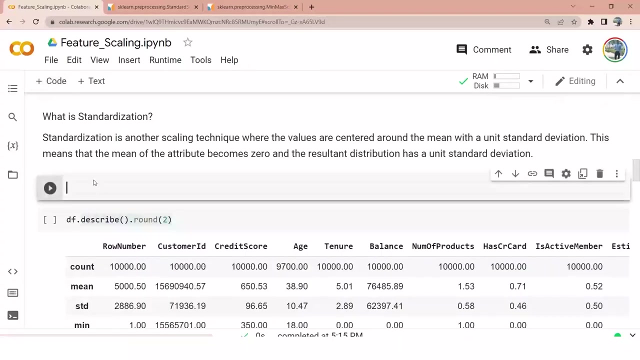 it is also known as mean max scaling. what is standardization? it's another scaling technique where values are centered around the mean with a unit standard deviation. this means that the mean of the attribute becomes zero and the resultant distribution has a unit standard deviation. first of all, i want to let you know how our data frame looks like. in order to show the data frame, 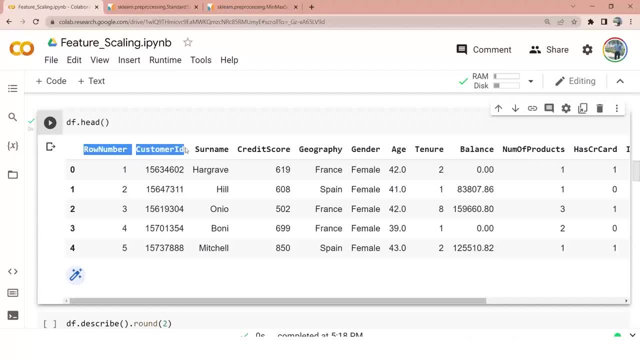 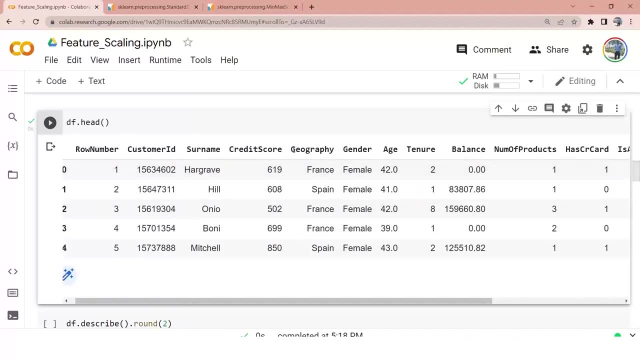 i will just print dot head and you can see i have row number, customer id, surname, blah, blah, blah. so many columns. one thing you must notice is some of these columns are having categorical values and some of these columns are, you know, not important for our analysis. now, just in case, 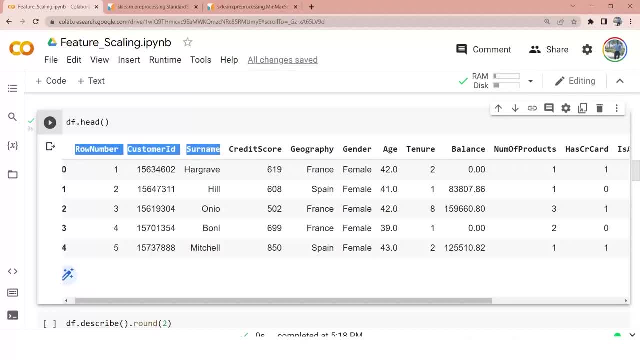 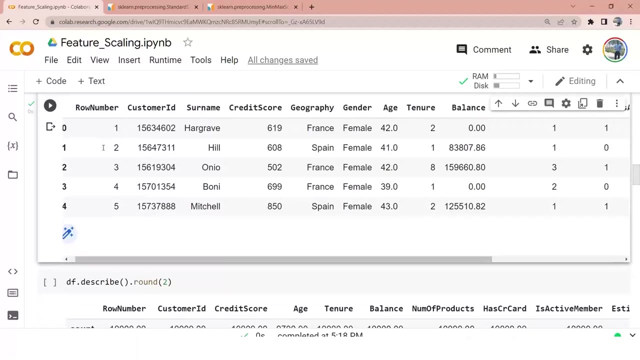 your columns are not important for your analysis, simply remove them. in this exercise we are not focusing on that part. we are focusing majorly on how to perform standardization and normalization. that's why i will not be showing you all those things. so what i will do is i'll quickly do the dot describe method, which basically shows the 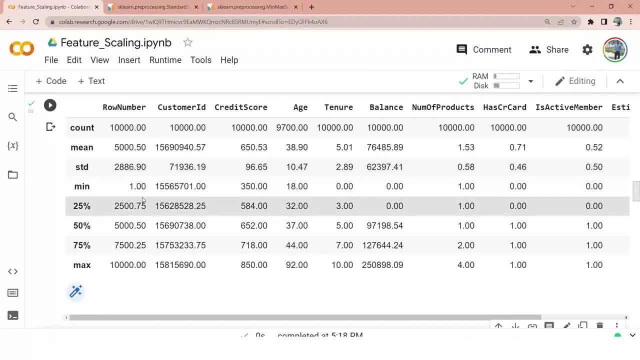 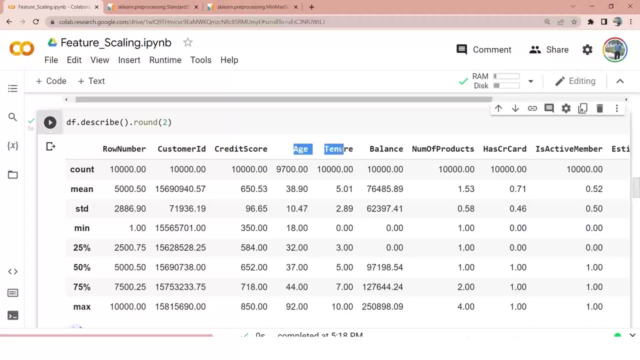 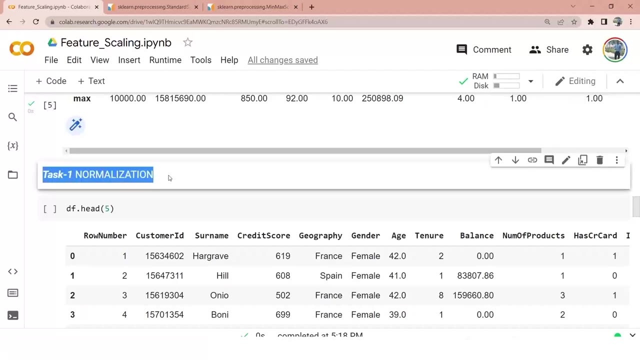 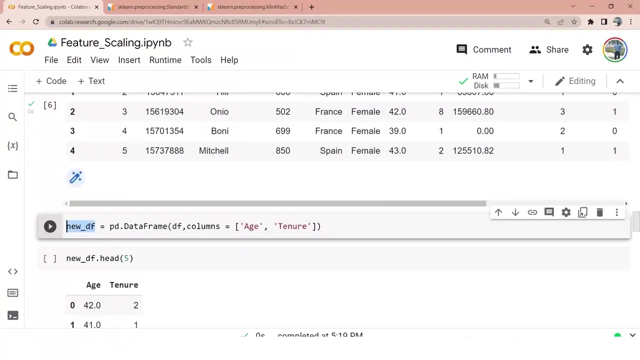 which basically shows the statistical information of all the numerical columns. i will choose some of these numerical columns may be age and tenure- and using them i will be doing the normalization. so task one, we will be talking about normalization. that's how my df looks like. i am creating a new data frame, only with age and tenure. that's it, only age and tenure. 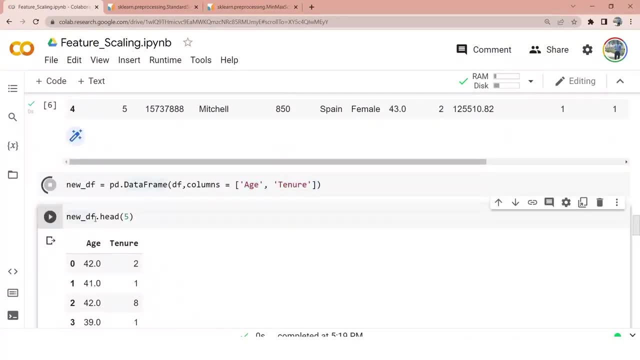 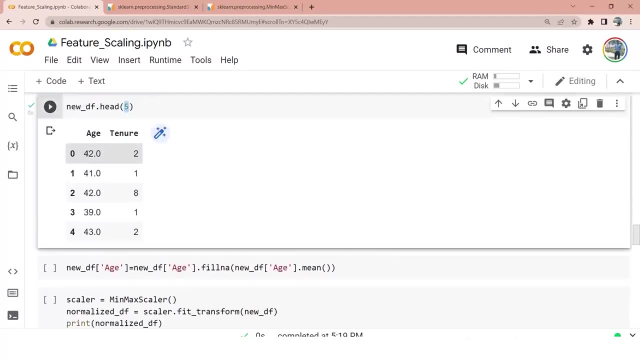 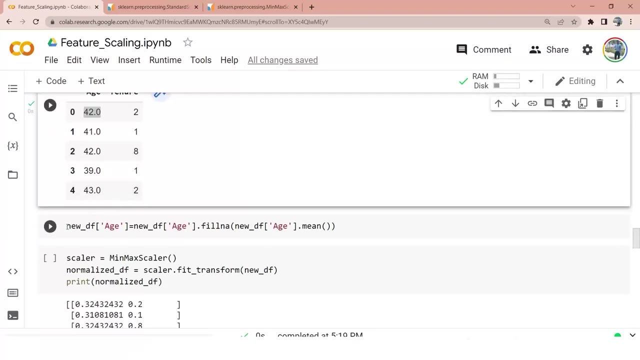 i don't want any other things. so how does my new df looks like? my new df looks like this: obviously, these are only five records, but you know that this is in one's place and this is in tens places. right as we have some null values, we are imputing the null values here. 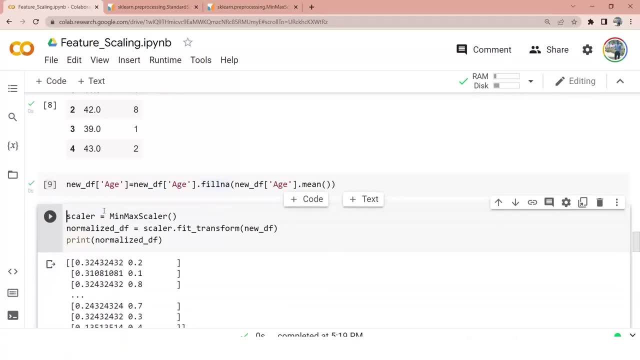 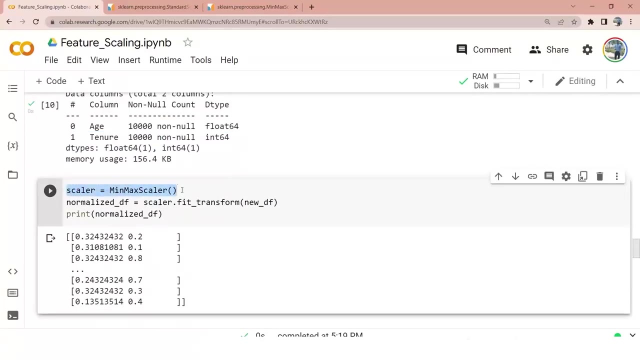 with the mean value. so once i run this, my null values are gone. if you just want to cross check after this, just do info and you will see that there are no null values anymore. done now. this is where i want to call my min max scalar. so scalar equals to min max scalar. now this: 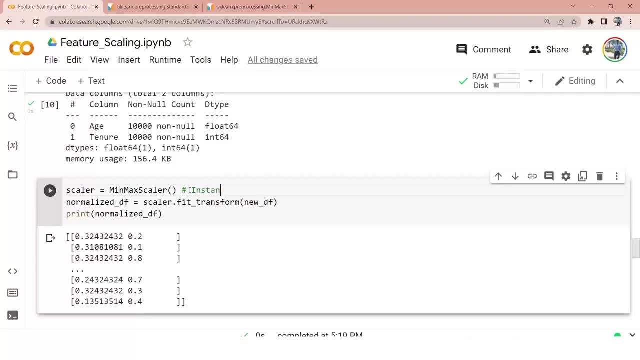 line is basically: i am instantiating the min max scalar function. i'm initiating that function. now i have a variable named normalized df equals to scalar dot, quit, transform new df. so i'm calling the scalar function and if i want to call this df, i'm just going to. 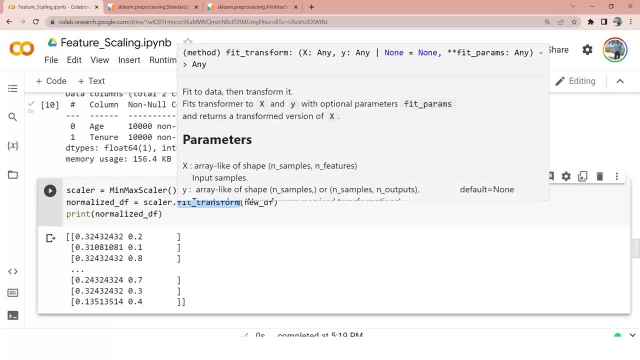 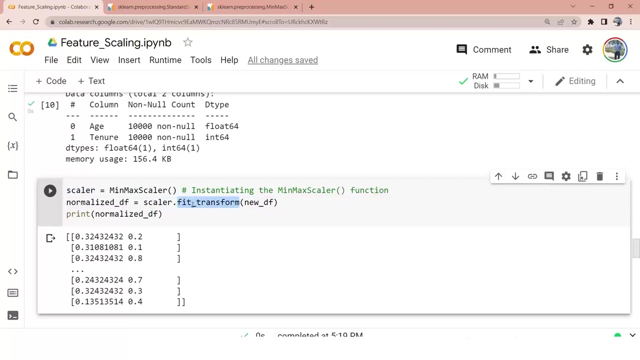 dot fit, transform, fit, transform basically fits and transforms the data. it basically does the conversion part. x, z equals to x minus mu by sigma, and then it fits the data. you will understand more about fitting data probably when we jump into the predictive analytics part, but for now just imagine that this is fit and transform. we basically convert the data. 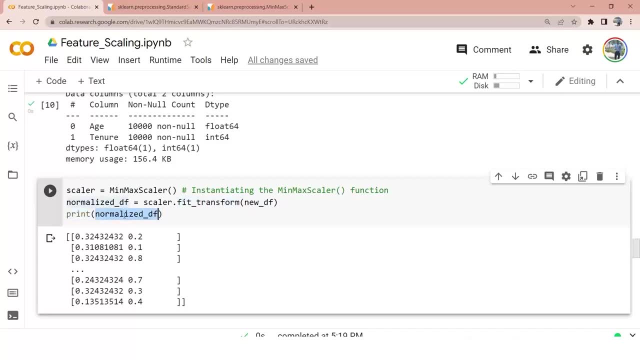 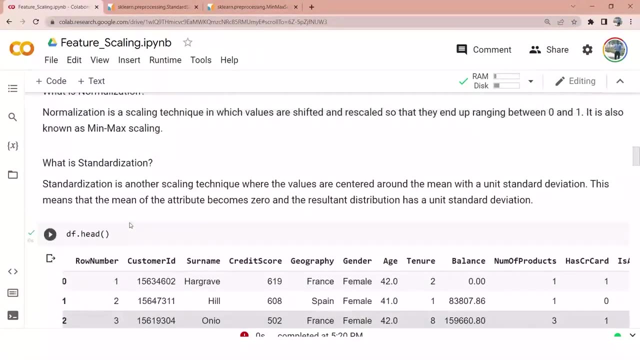 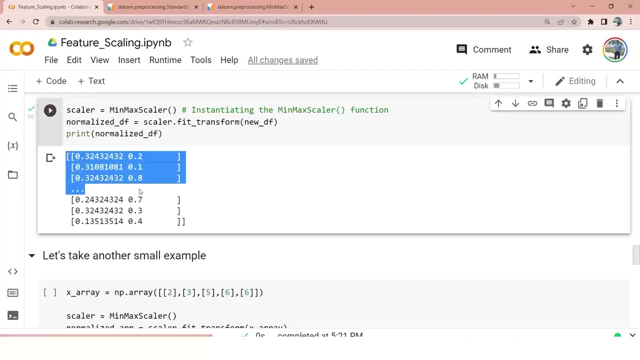 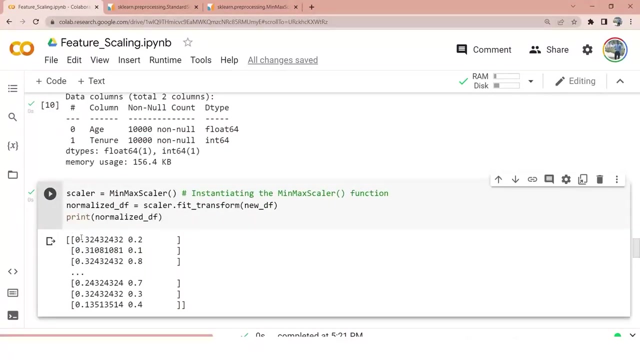 and fit it and you can see the normalized df looks like this. okay, min max scalar is not defined. we'll have to define it again and then we will run this and you can see that's how my normalized data looks like, and obviously they does not look like this, right they? they are. both of them are in. 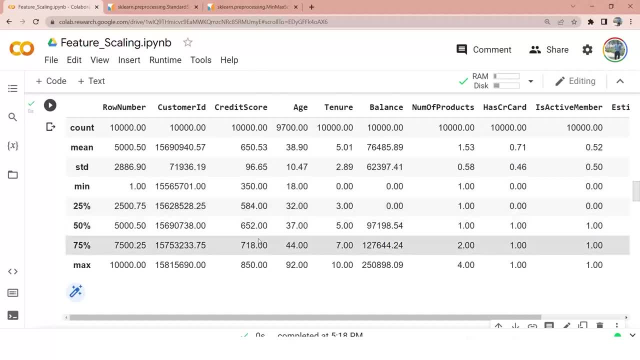 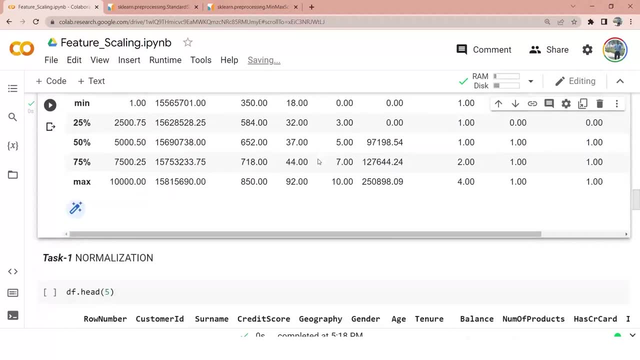 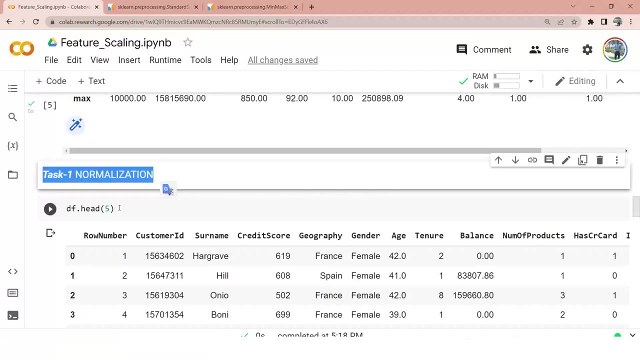 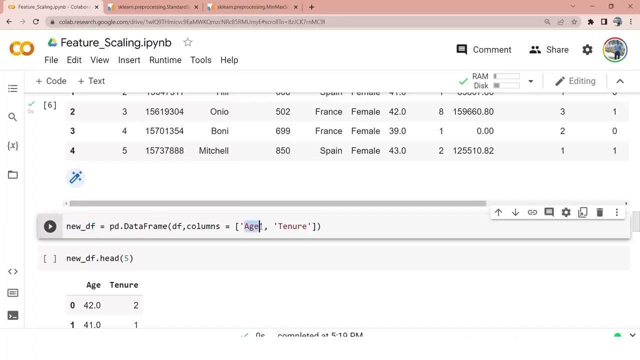 statistical information of all the numerical columns. i will choose some of these numerical columns may be age and tenure, and using them i will be doing the normalization. so task one, we will be talking about normalization. that's how my df looks like. i am creating a new data frame, only with age and tenure. that's it, only agent tenure. i don't want any other things. 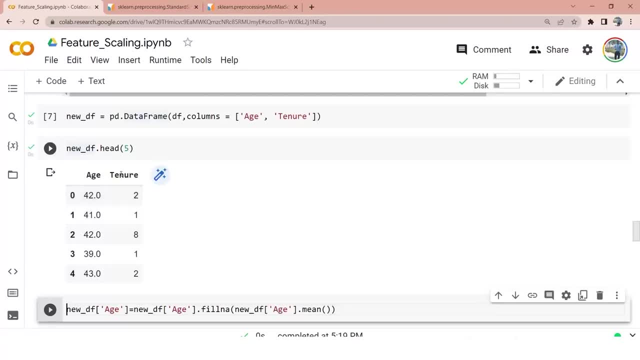 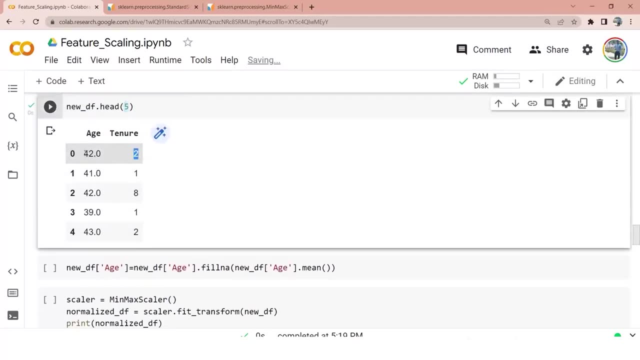 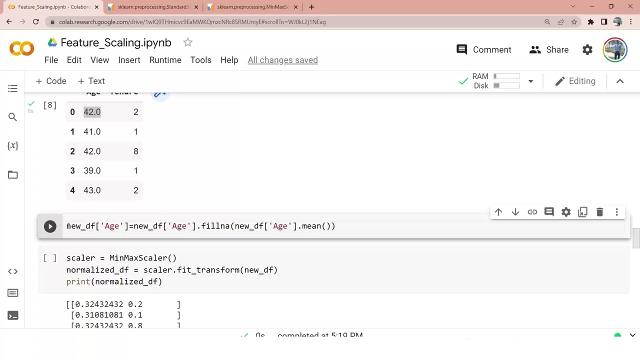 so how does my new df looks like? my new df looks like this. obviously, these are only five records, but you know that this is in one's place and this is in tens places. right, as we have some null values, we are imputing the null values here with the mean value. 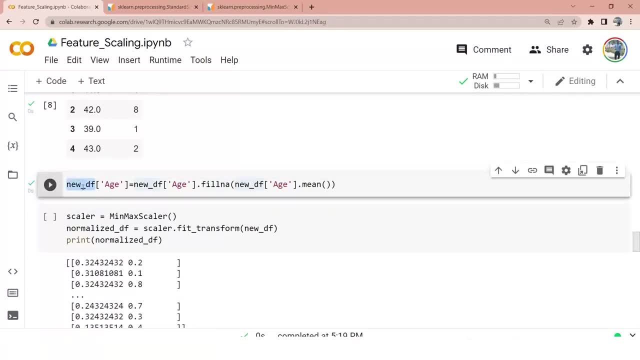 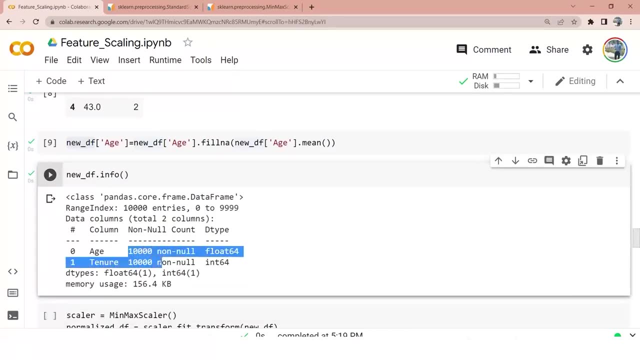 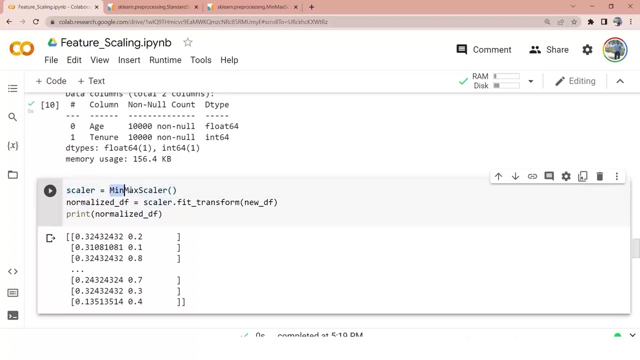 so once i run this, my null values are gone. if you just want to cross check after this, just do info and you will see that there are no null values anymore. done now. this is where i want to call my min max scalar. so scalar equals to min max scalar now. 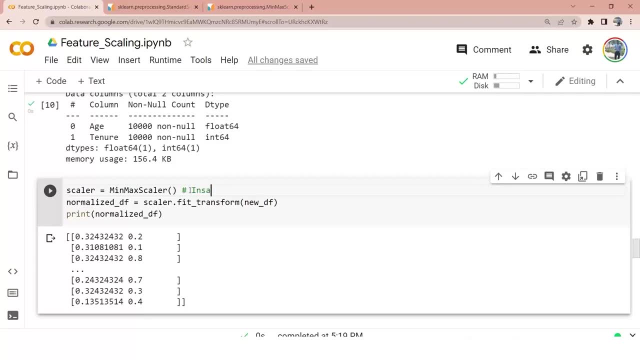 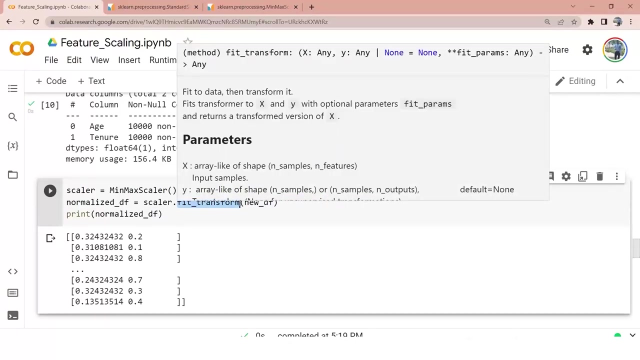 this line is basically: i'm instantiating the min max scalar function. i'm initiating that function. now i have a variable name: normalized df equals to scalar dot fit, transform, newdf. so i'm calling the scalar dot fit, transform. fit. transform basically fits and transforms the data. it basically does the conversion part x z equals to x minus mu by sigma. 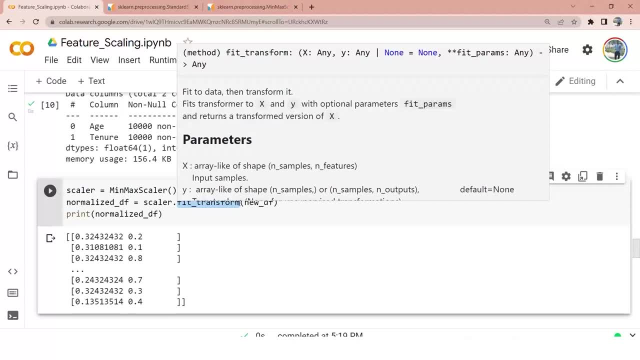 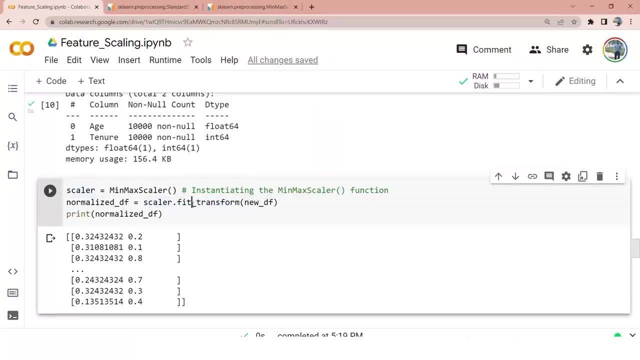 and then it fits the data. you will understand more about the conversion part of the conversion part based on the data, about fitting data, probably when we jump into the predictive analytics part, but for now, just imagine that this is fit and transform. we basically convert the data and fit it and you can see the 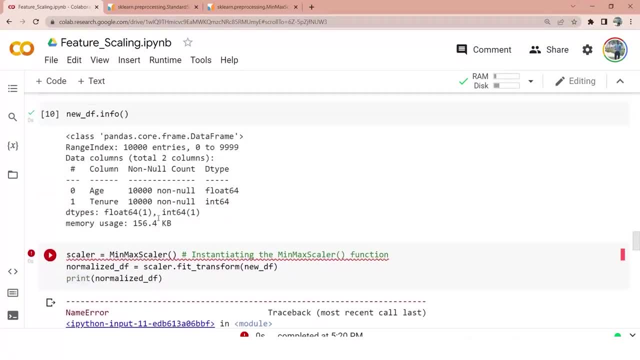 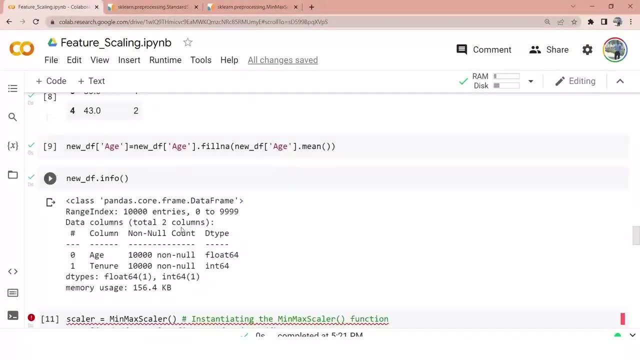 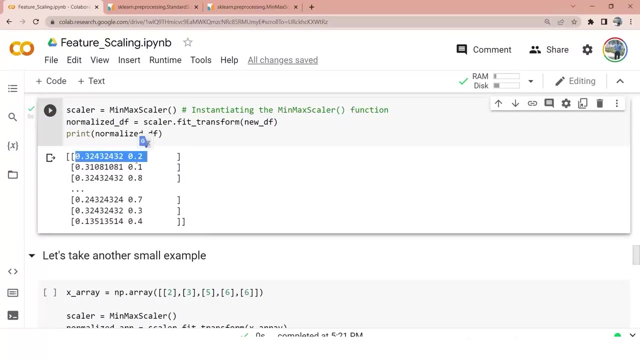 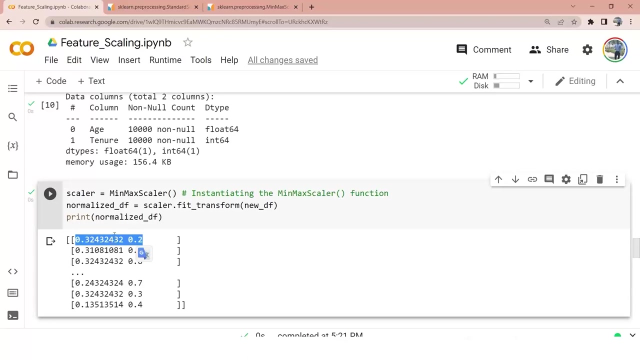 normalized df looks like this: okay, minmax scalar is not defined. we'll have to define it again and then we will run this and you can see that's how my normalized data looks like. and obviously they does not look like this, right? they they are. both of them are in a same similar scale. right now you might not be. 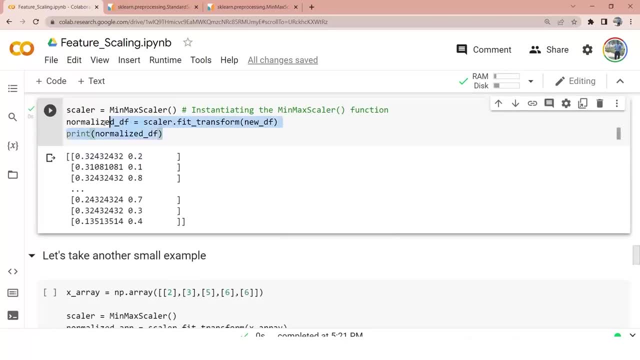 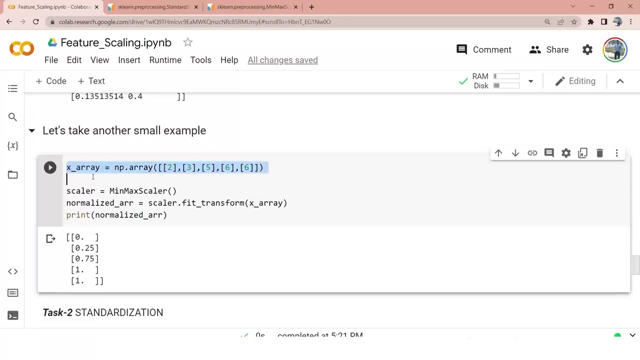 similar scale. right now you might not be able to understand what's happening inside. right, there are so many values. we have ten thousand records, so we'll try to take a small example. mathematically i will show you how things are happening and i will also show you the output here. you can see i have taken an 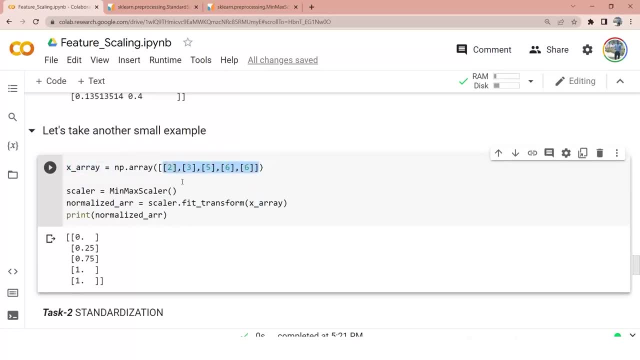 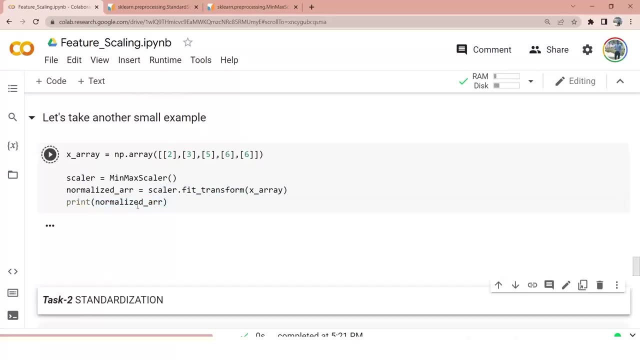 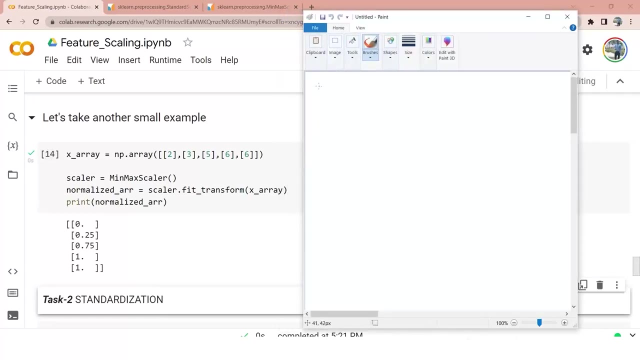 array of five objects: two, three, five, six, six, and i'm calling the min max scalar and i'm calling the fit transform and i'm printing the normalized array. that's how my output looks like. so let's try to do it using notepad, using paintbrush, so we have data, so i will. 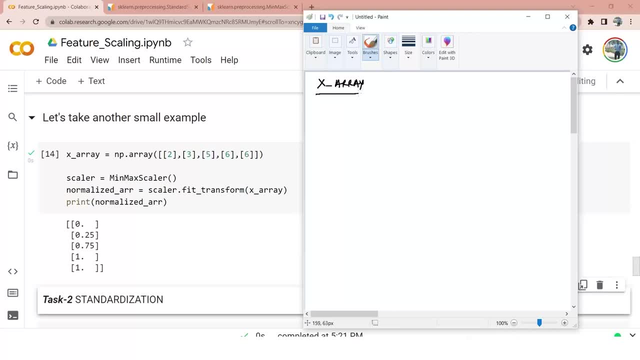 write it down as x array: two, three, five, six, six. what is normalization? x dash equals to x minus x minimum divided by x maximum minus x minimum. two, three, five, six, six. and we have normalization x dash equals to x minus x minimum divided by x maximum minus x minimum equal to x. or we can see that it is an operation. in this case, we have one state, we have a given. 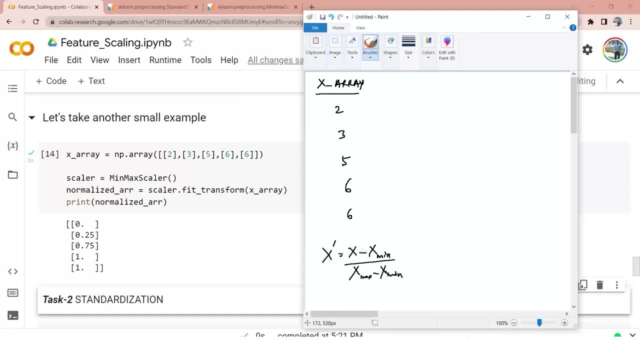 minimum, simple. so what is the numerator part x minus x mean. sorry, we'll talk about the entire thing. okay, what is the minimum value? this is the minimum value. the maximum value is this: so for this, the x dash will be x minus x. minimum: 2 minus 2: 0 divided by anything will be 0. 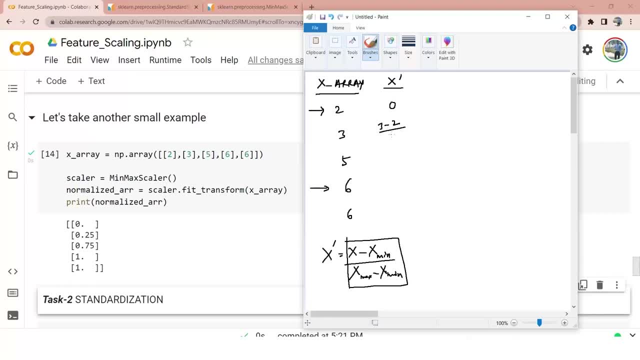 this will be 3 minus 2, divided by 6 minus 2, which will be 1 by 4, which will be 0.25, this will be 5 minus 2 divided by 6 minus 2, which is 3 by 4, which is 0.75, this will be 6 minus 2. 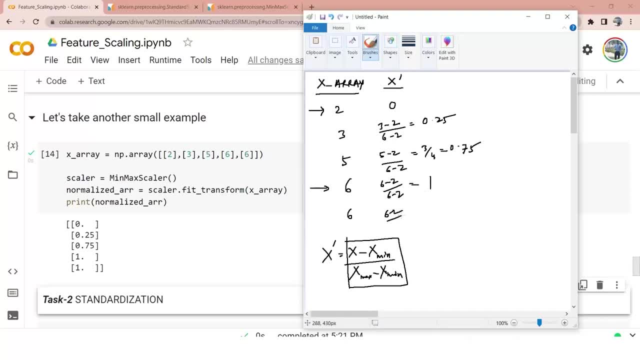 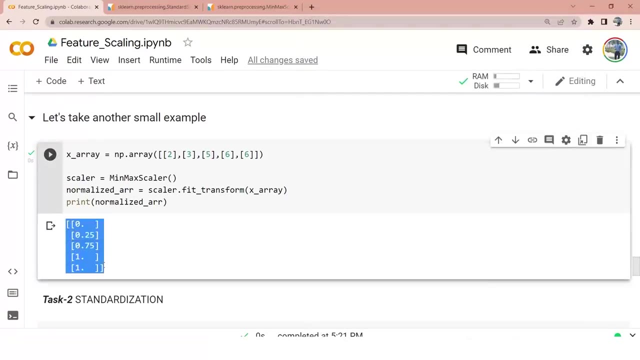 divided by 6 minus 2, which will be 1, 6 minus 2. divided by 6 minus 2, which will be 1, so the final values are 0, 0.25, 0.75, 1 and 1, and that is what it is: 0, 0.25, 0.75 and 1, and that is what is. 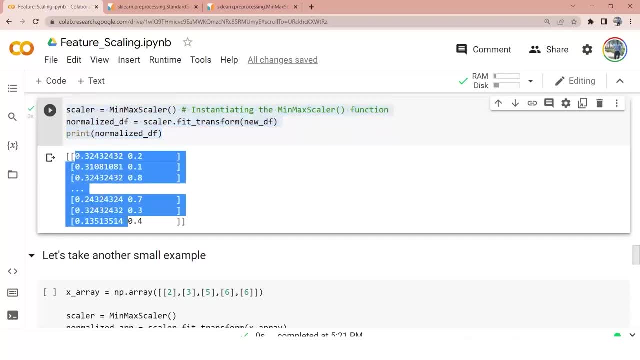 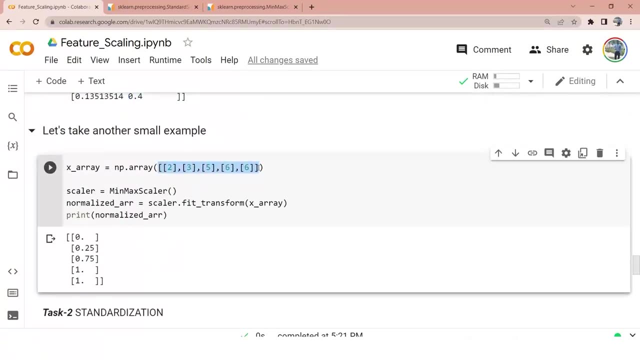 able to understand what's happening inside. right, there are so many values. we have 10 000 records, so we'll try to take a small example: minmax, scalar mathematically. i will show you how things are happening and i will also show you the output here. 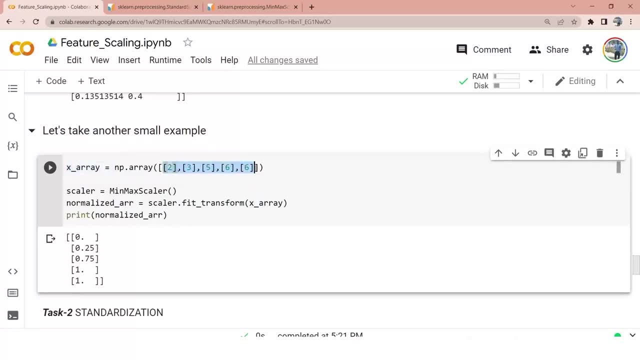 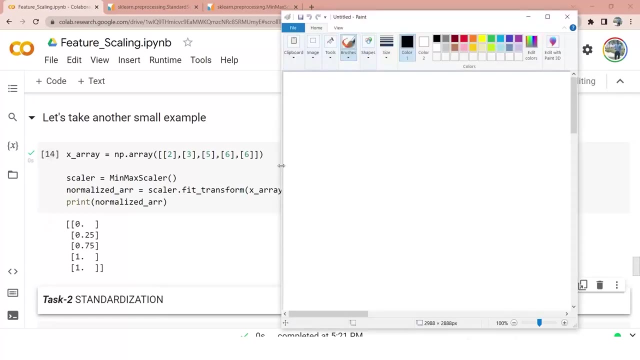 you can see, i have taken an array of five objects- two, three, five, six, six- and i'm calling the min max scalar and i'm calling the fit transform and i'm printing the normalized array. that's how my output looks like. so let's try to do it using notepad, using paintbrush, so we have data. so i 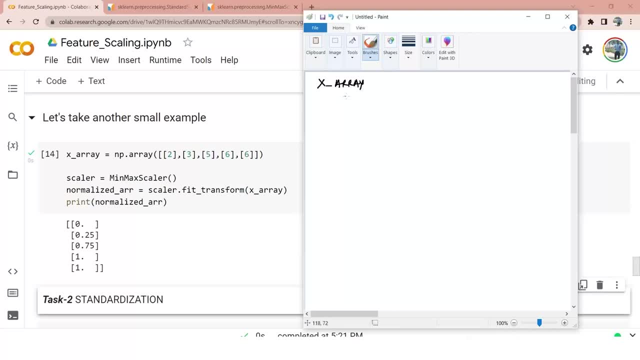 will write it down as: x array two, three, five, six, six. what is normalization? x dash equals to x minus x minimum, divided by x maximum minus x minimum, simple. so what is the numerator part x minus x mean. sorry, we'll talk about the entire thing, okay. what is the minimum? 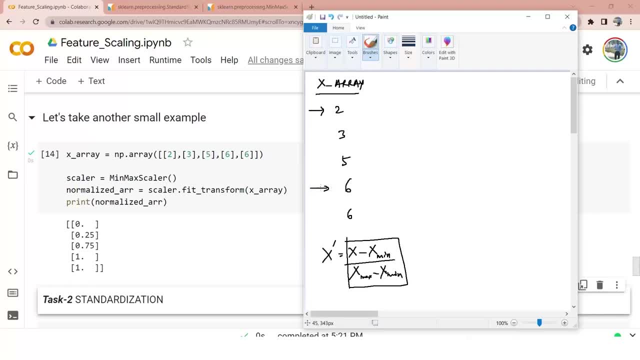 value. this is the minimum value. the maximum value is this, so for this, the x dash will be x minus x. minimum: 2 minus 2: 0 divided by anything will be 0, this will be 3 minus 2, divided by 6 minus 2, which will be 1 by 4, which will be 0.25, this will be 5 minus 2 divided by 6 minus 2. 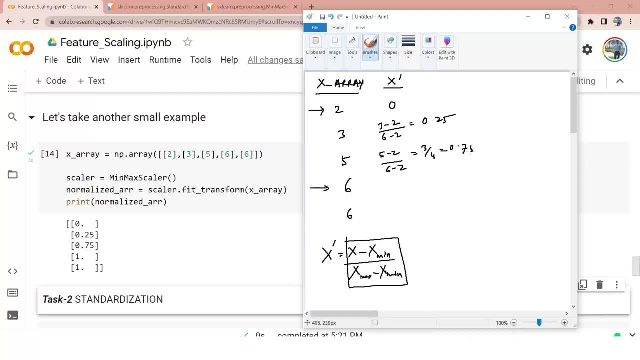 which is 3 by 4, which is 0.75. this will be 6 minus 2, divided by 6 minus 2, which will be 1, 6 minus 2 divided by 6 minus 2, which will be 1.. so the final values are 0, 0.25, 0.75, 1 and 1, and that is what it is. 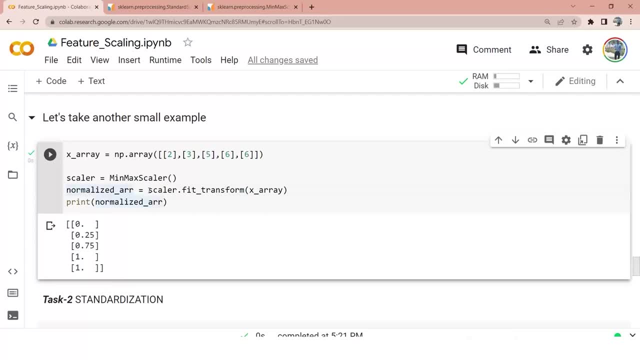 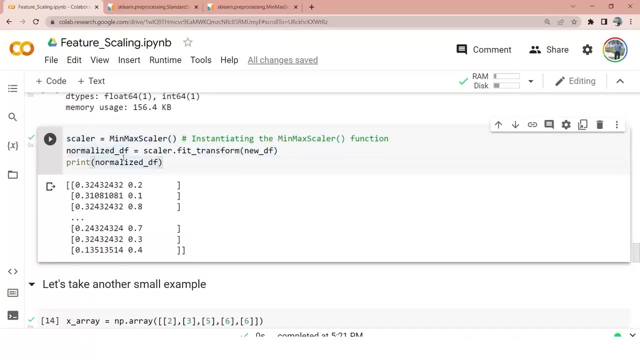 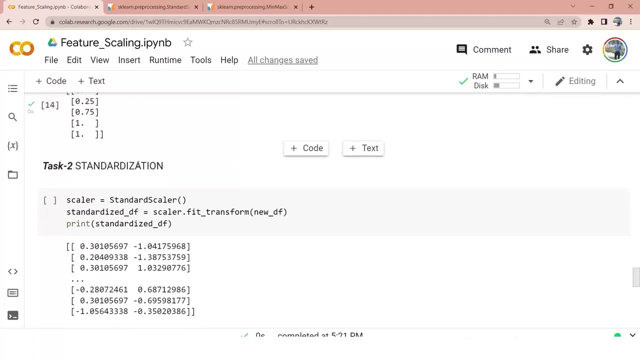 0, 0.25, 0.75 and 1, and that is what is happening inside, right? so if you want to cross check on a big data set, probably you can cross check that. so that's all about normalization. coming back to standardization, very similar technique. instead of min max scalar here i'm calling my standard scalar. 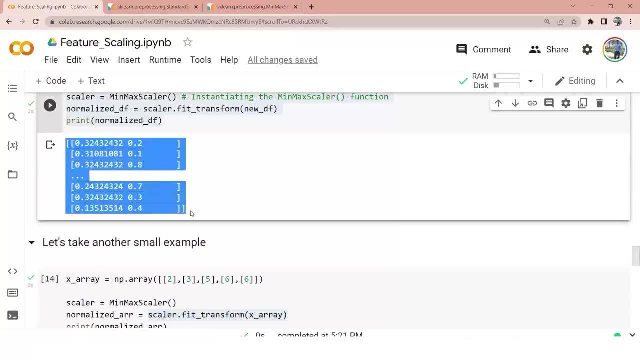 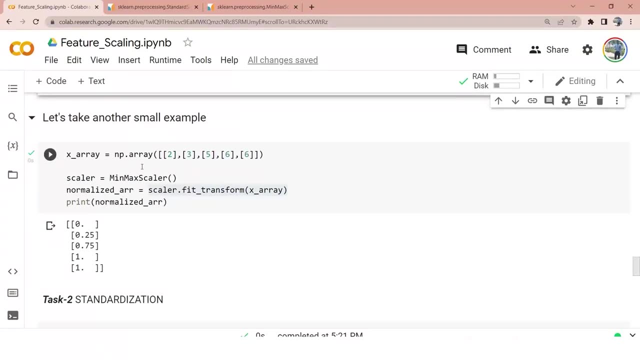 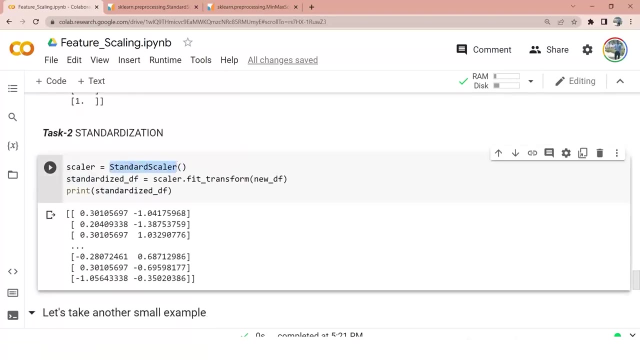 happening inside right. so if you want to cross check on a big data set, probably you can cross check that. so that's all about normalization. coming back to standardization, very similar technique. instead of min max scalar, here i'm calling my standard scalar and i'm doing the same operations, exact same piece. 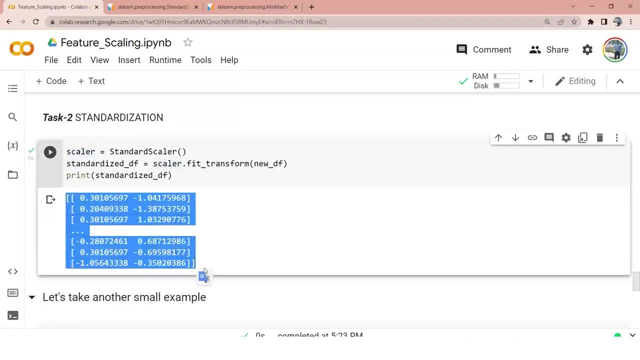 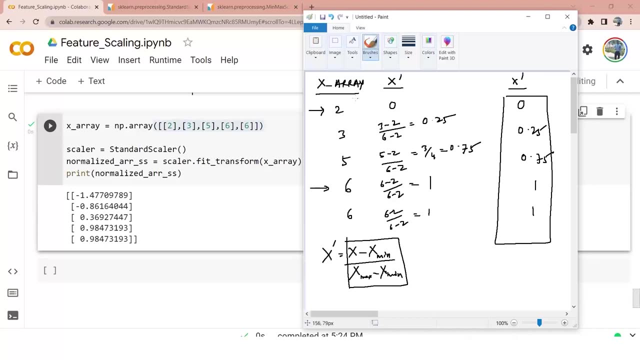 of code. if i run this, you can see my standardized values. are this again? taking this example, same example. i will be using the standardization technique, so i will rub this off. i will again take my x value, which is 2, 3, 5, 6 and 6. what will be the mean value? 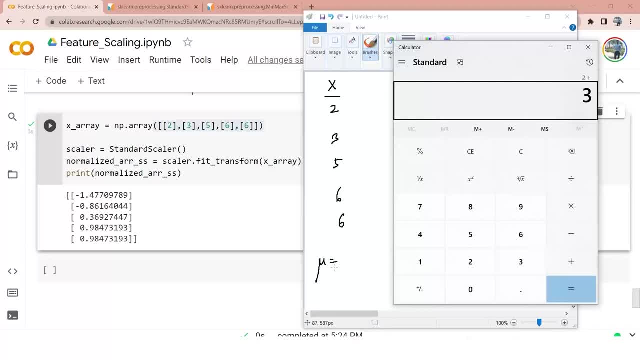 mean value. The mean value will be 2 plus 3 plus 5 plus 12 divided by 5, which is 4.4.. What is the standard deviation? Standard deviation is root over of xi minus mu, square divided by n. So let us try to calculate. 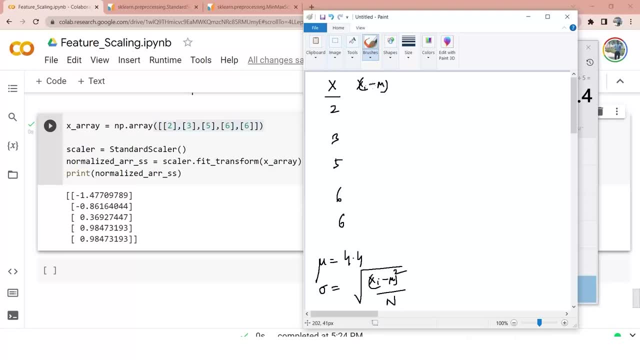 What is xi minus mu square? It is 2 minus 4.4, 2.4 square. It is 1.4 square. It is 0.6 square. It is 1.6 square. It is 1.6 square. 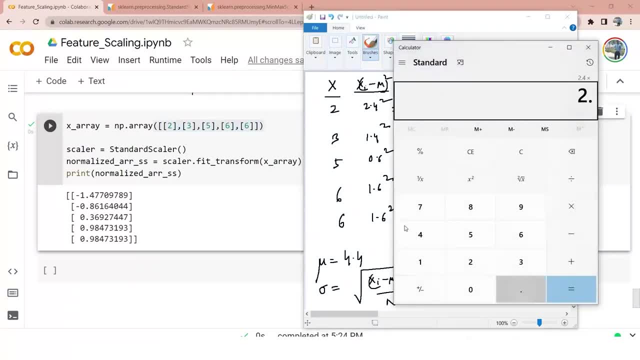 So what will be the actual values? 2.4 into 2.4 is 5.76.. 1.4 into 1.4 is 1.96.. 0.36.. 1.6 into 1.6 is 2.56.. 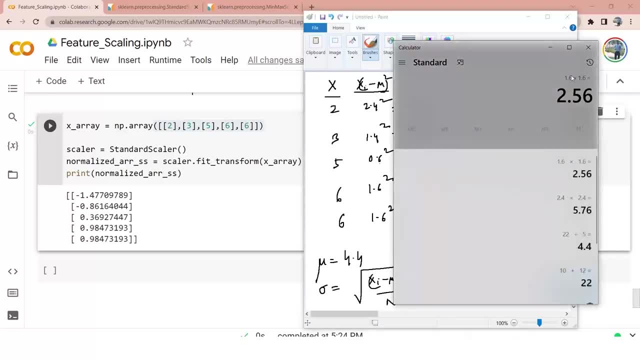 And this is 2.56.. We will just cross check for 1.4 into 1.4.. 1.4 square is 1.96.. My bad, 1.4 square is 1.96.. Done. 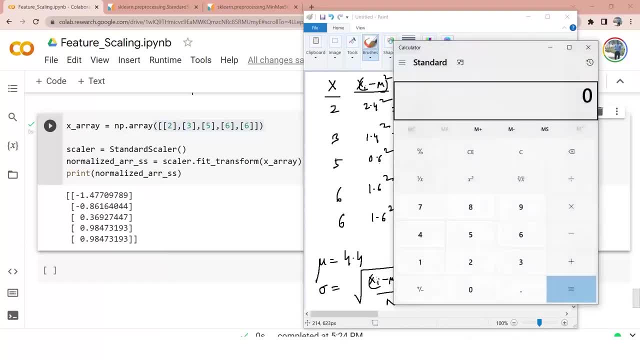 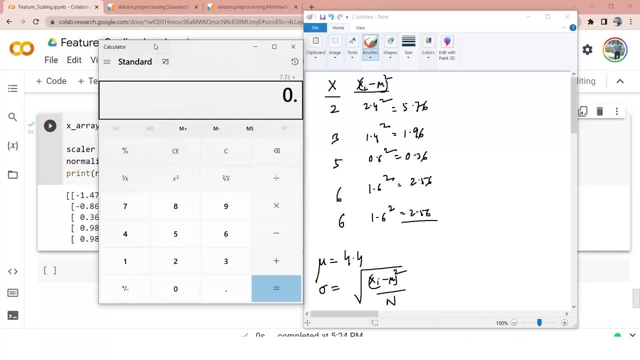 Now we will try to add this up. How to add it? 5.7.. 7.6 plus 1.96 plus 0.36 plus 2.56 plus 2.56, which is 13.2.. 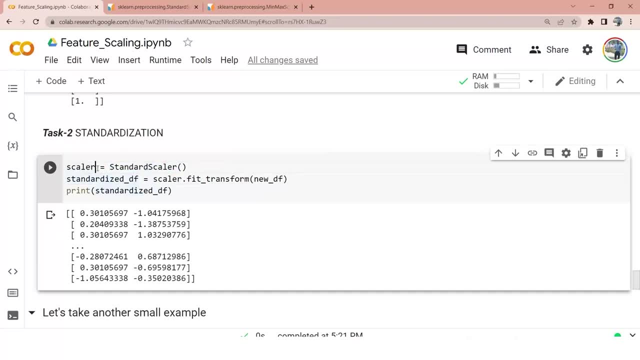 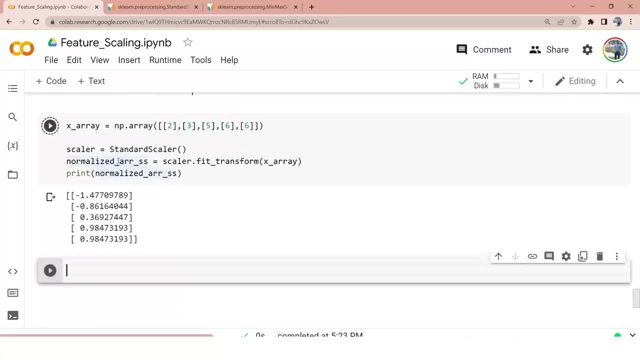 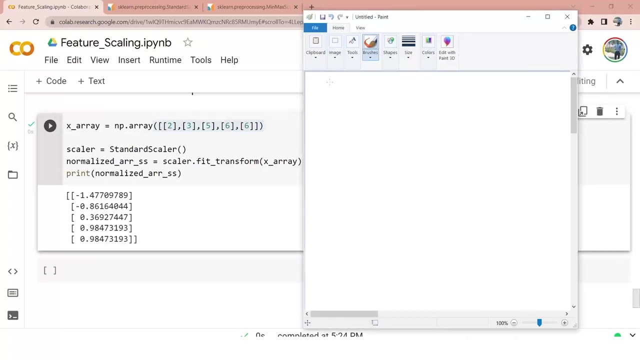 and i'm doing the same operations, exact same piece of code. if i run this, you can see my standardized values. are this again? taking this example, same example. i will be using the standardization technique, so i will rub this off. i will again take my x value, which is 2. 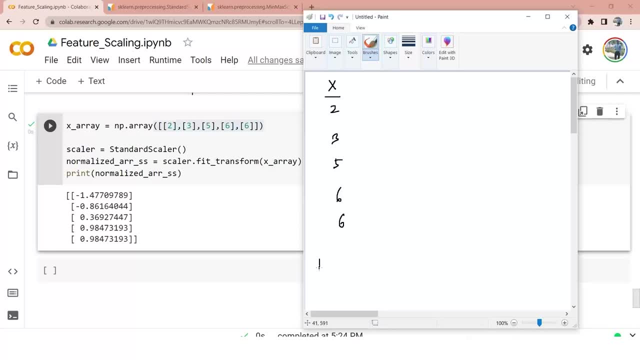 3, 5, 6 and 6.. what will be the mean value? the mean value will be 2 plus 3 plus 5 plus 12, divided by 5, which is 4.4. what is the standard deviation? standard deviation is root over of x, i minus mu, square. 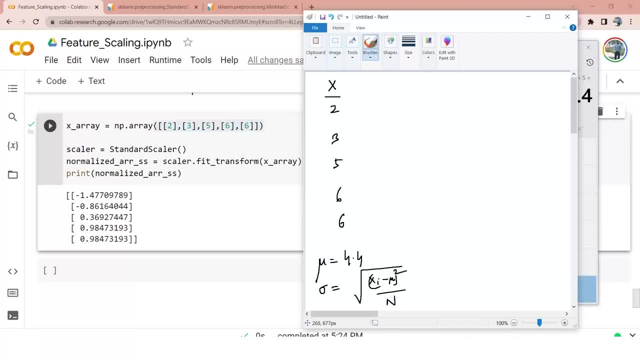 here divided by n. so let's try to calculate what is xi minus mu square. it is 2 minus 4.4. 2.4 square. it is 1.4 square. it is 0.6 square. it is 1.6 square. it is 1.6 square. 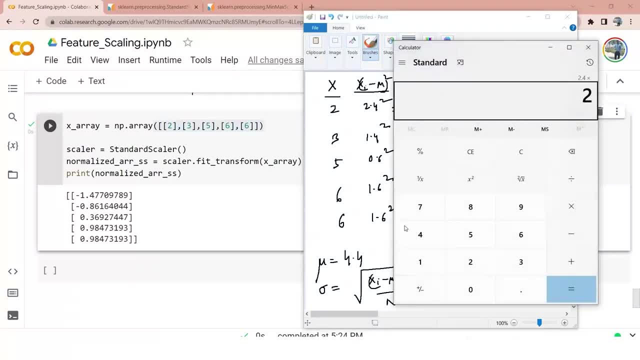 so what will be the actual values? 2emos point four into two. point four is five. point seven: six. one point four into one. point four is 1.96, 0.36. 1.6 into 1.6 is 2.56. 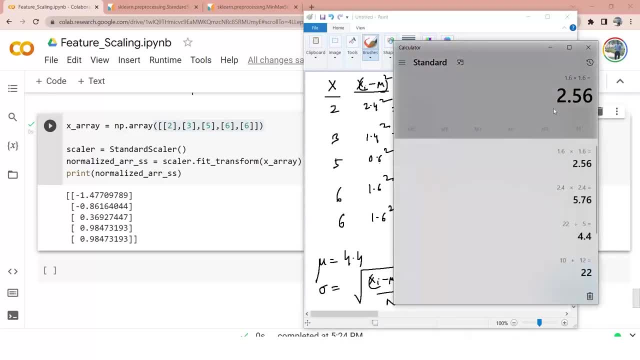 and this is 2.56. we'll just cross check for 1.4 into 1.4. 1.4 square is 1.96. my bad, 1.4 square is 1.96. done now we'll try to add this up. how to add it? 5.76. 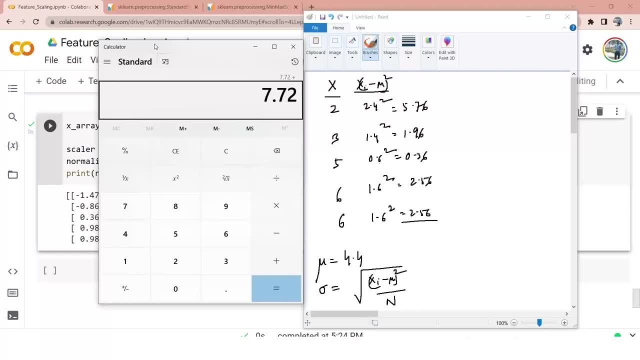 plus 1.96 plus 0.36, plus 2.56 plus 2.56, which is 13.2- 13.2. so my standard deviation will be 13.2 divided by as this is, uh, we'll try to consider. 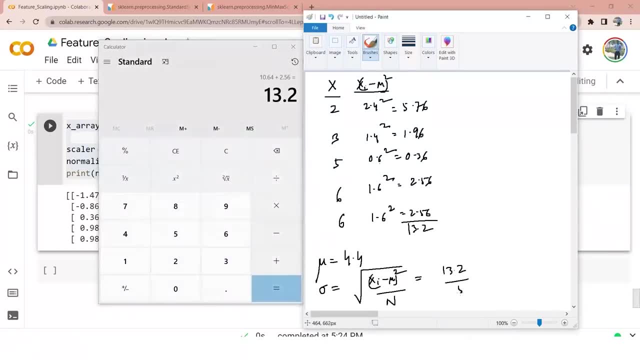 this as a population data divided by 5. divided by 5 is 2.64, is 2.64, and then, by the time from here, if we start to knocking out, these values are, then this d has to go on to the vec. what is this? c, f, j and d will depends on what it has. 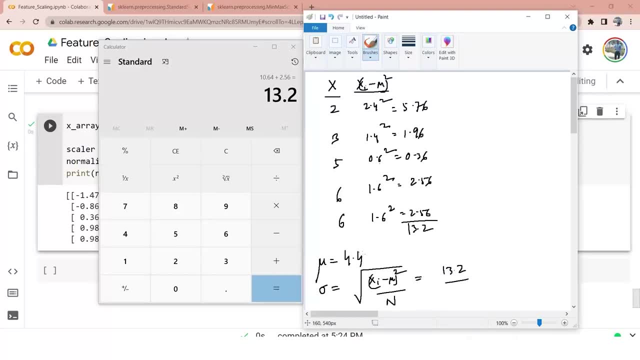 So my standard deviation will be 13.2 divided by as this is, we will try to consider this as a population data divided by 5, divided by 5 is 2.64.. 2.64. And then its root over is 1.62.. 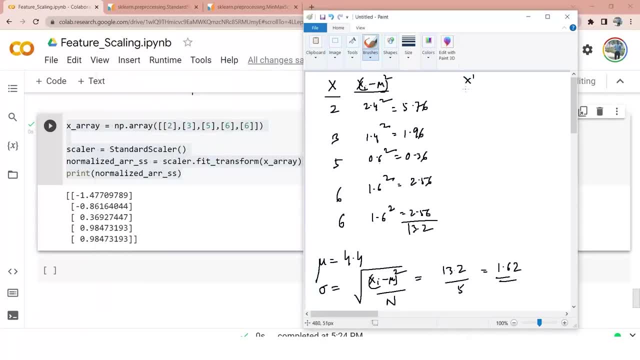 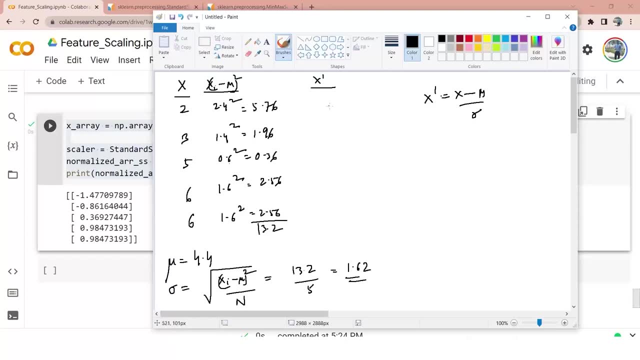 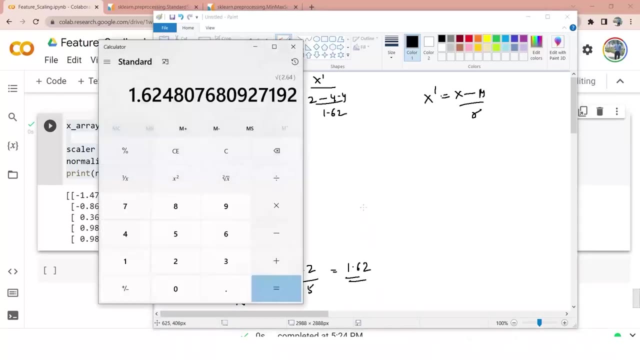 That's my sigma Right. So what is my x dash? My x dash formula is x minus mu by sigma. So this will be 2 minus 4.4 divided by 1.62.. So let's try to cross check. 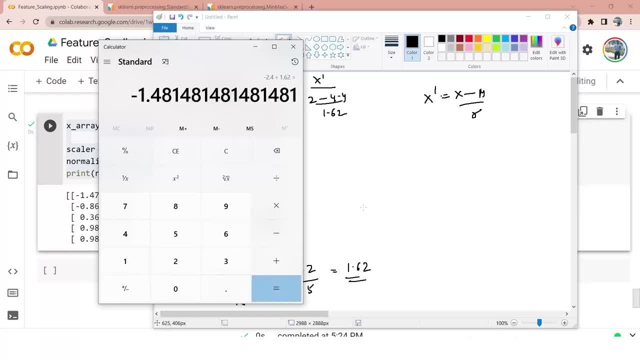 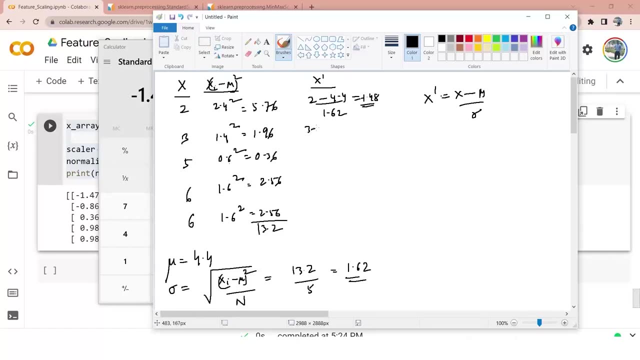 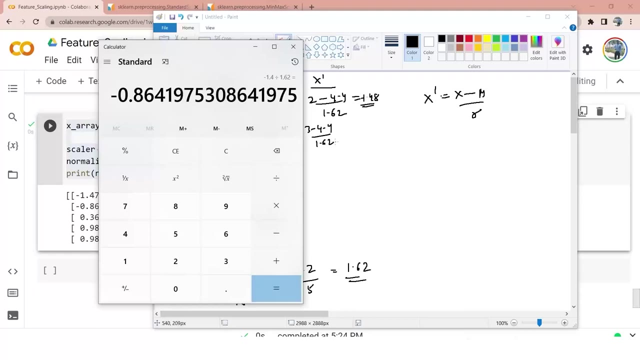 2 minus 4.4 divided by 1.62, which is minus 1.4.. Minus 1.62.. Minus 1.48.. For the second one, 3 minus 4.4 by 1.62,. 3 minus 4.4 divided by 1.62,, it is minus 0.86, minus 0.86.. 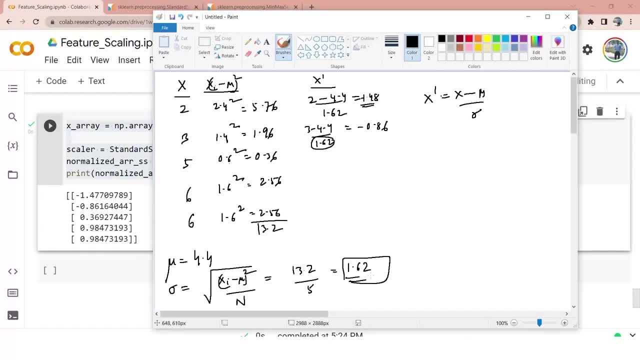 See, I'm only taking two decimals. The actual value is more than two decimals, right? So these values and these values will not be exact replica, but you can see it's almost close. Here it is minus 1.47.. 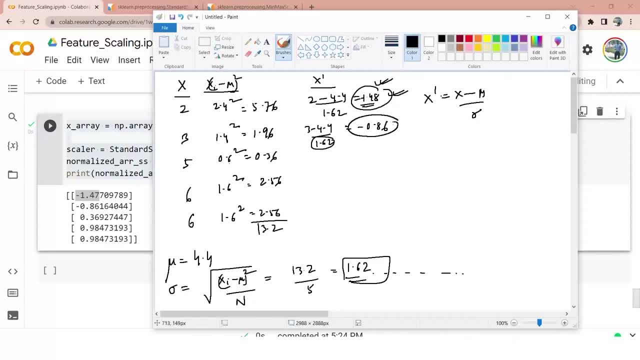 Here it is minus 1.48.. Minus 0.86, minus 0.86.. We'll try to calculate for this one, which is 6 minus 4.4, divided by 1.62, which is 0.98.. 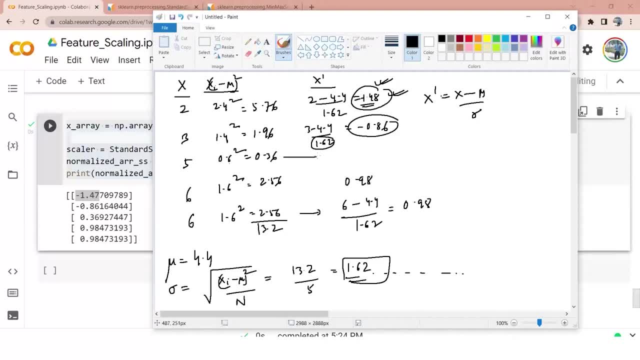 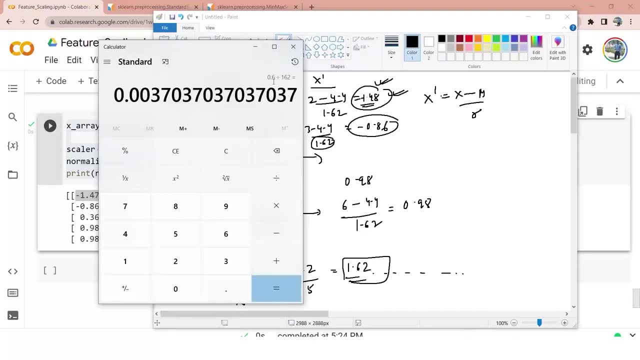 Obviously, for this is also 0.98.. So we'll calculate for the last number, also divided by 1.62, which is Sorry, Sorry, N200, which is 0.37.. 0.37. 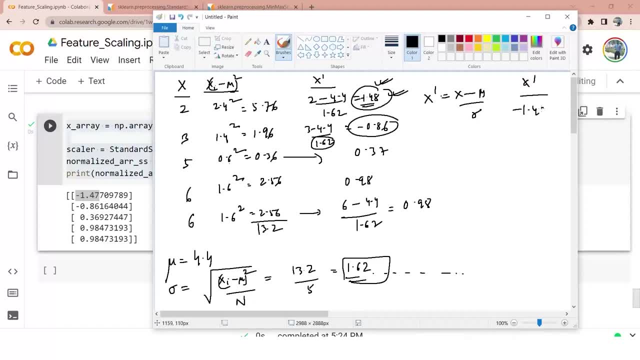 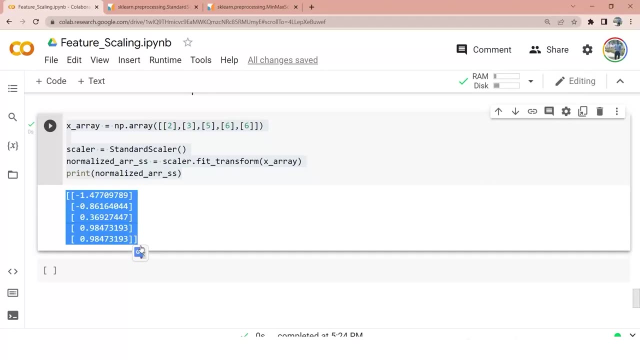 So you can see the x dash values are 1.48, minus 0.86,, 0.37,, 0.98, and 0.98. And you can see these numbers are matching. So that's all about standardization and normalization. 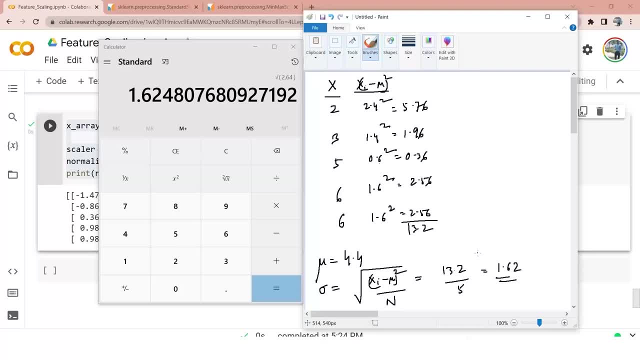 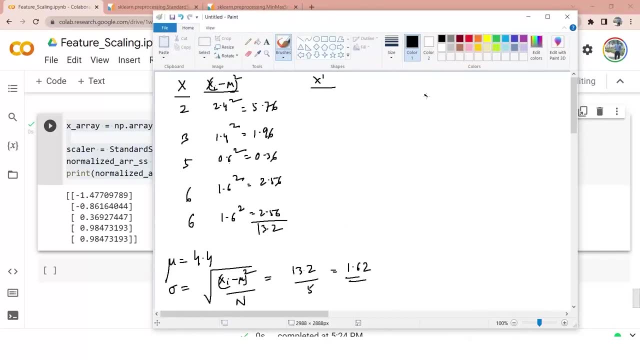 to c, f, v. we'll discuss this. we have to remember that these values are mostly papers''. then its root over is 1.62. that's my sigma, right. so what is my x dash? my x dash formula is x minus mu by sigma. so this will be 2 minus 4.4 divided by 1.62. so let's try to cross check. 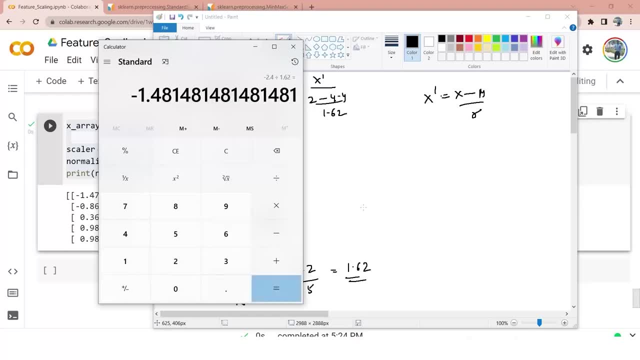 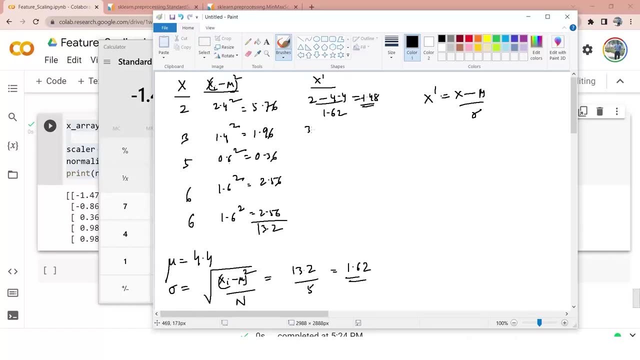 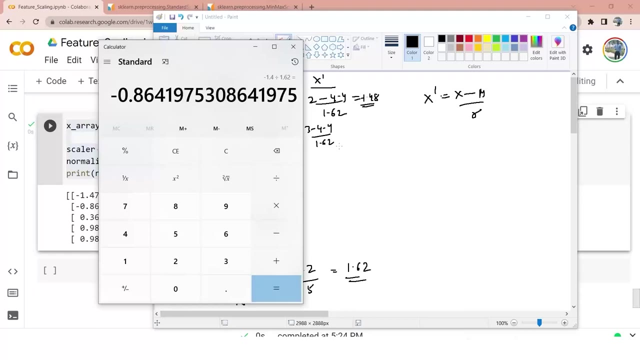 2 minus 4.4 divided by 1.62, which is minus 1.4 minus 1.48. for the second one, 3 minus 4.4 by 1.62. 3 minus 4.4 divided by 1.62, it is minus 0.86 minus 0.86. 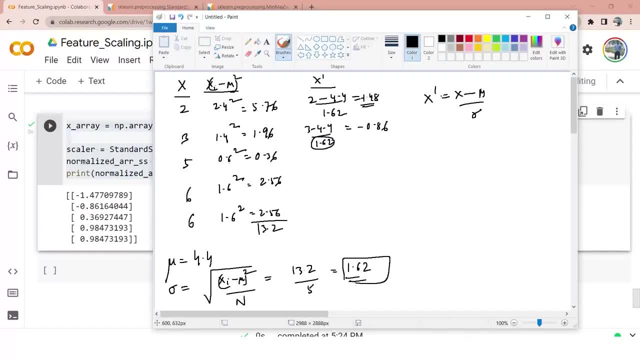 see, i am only taking two decimals. the actual value is more than two decimals, right. so these values and values will not be exact replica, but you can see it's almost close. here it is minus 1.47. here it is minus 1.48, minus 0.86, minus 0.86. we'll try to calculate for this one, which is 6. 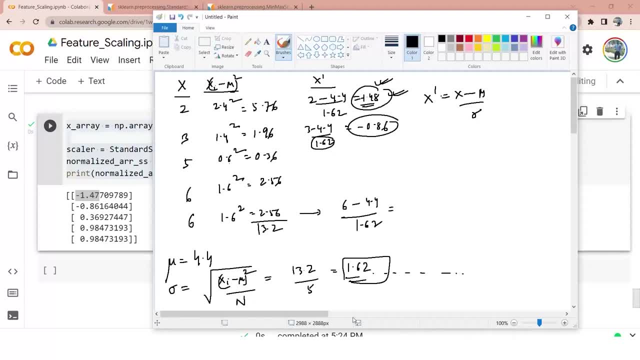 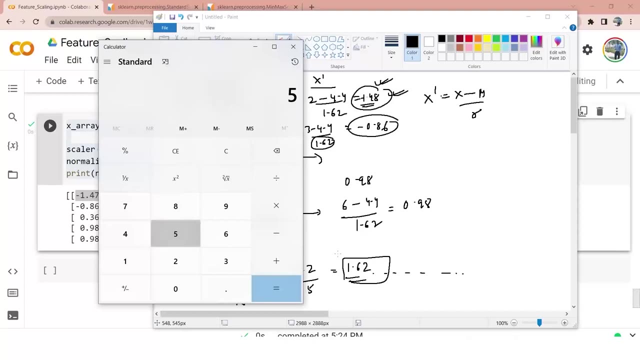 minus 4.4 divided by 1.62, which is 6 minus 4.4 divided by 1.62, which is 0.98. obviously, for this is also 0.98, so we'll calculate for the last number, also divided by. 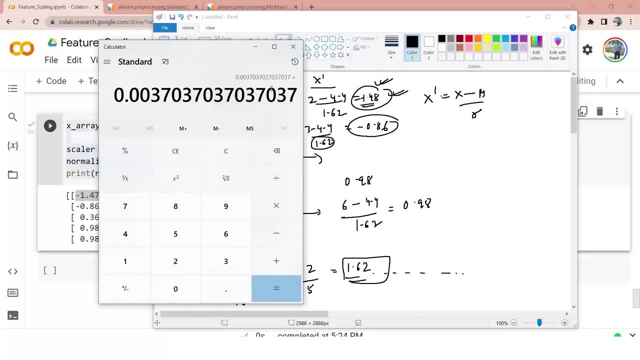 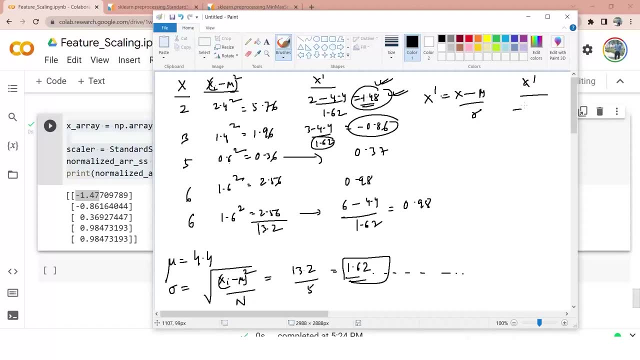 1.62, which is sorry, uh, in 200, which is 0.37, 0.37. so you can see, the x dash values are 1.48 minus 0.86, 0.37, 0.98 and 0.98 and you can see. the x dash values are 1.48 minus 0.86, 0.37, 0.98 and 0.98, and you can see. the x dash values are 1.48 minus 0.86, 0.97, 0.98 and 0.98, and you can see. 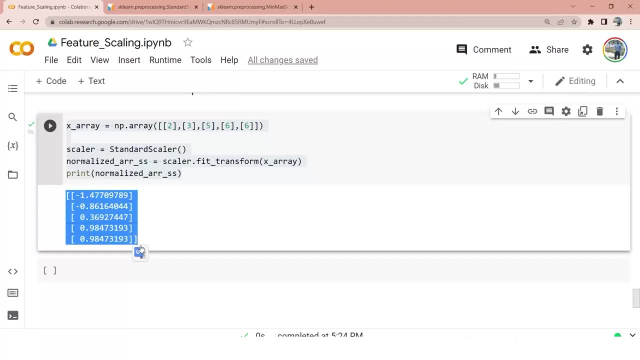 these numbers are matching. so that's all about standardization and normalization. as i told you- repeating once again, standardization or normalization in one is one of those mandatory steps before getting into the predictive analytics part. talking about the ada part, it might not be necessary, but it's important to know all these techniques. so that's all about feature scaling. 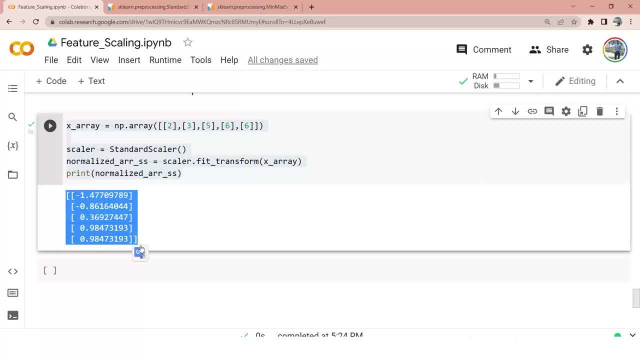 As I told you, repeating once again, standardization or normalization is one of those mandatory steps. Before getting into the predictive analytics part, Talking about the ADA part, it might not be necessary, but it's important to know all these techniques. So that's all about feature scaling. 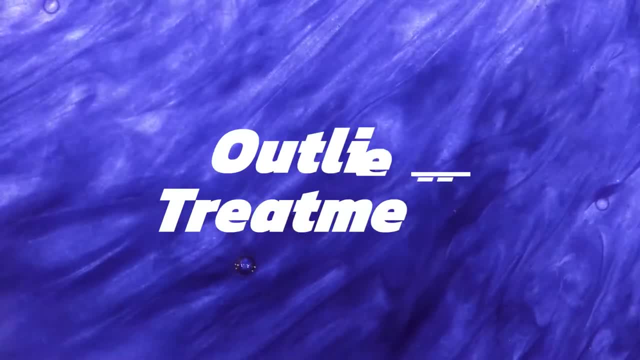 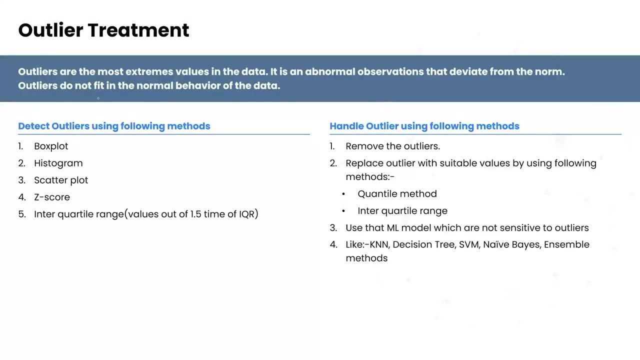 We'll see you in the next video. Let's talk about the next type of data cleaning activity that we do, which is outlier treatment. Outlier treatment- In simple terms, outliers- are the most extreme values in the data. it is an abnormal observation that deviates from. 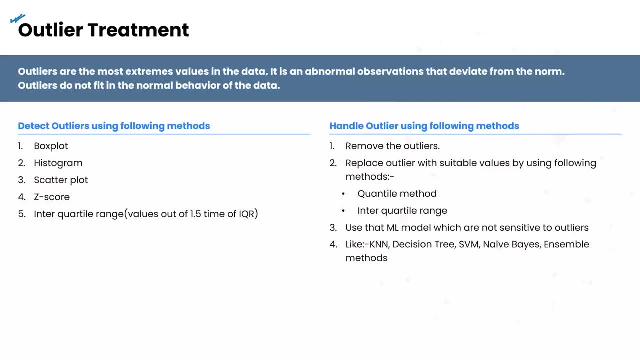 the normal data outliers do not fit in the normal behavior of the data. outliers are also called as anomalies. now how do we spot outliers? there are different techniques to spot outliers, but before getting into the detection part, let's try to understand what outlier is. now imagine there are different people with different age: 28, 29, 31, 92, 28. now if i simply plot them, 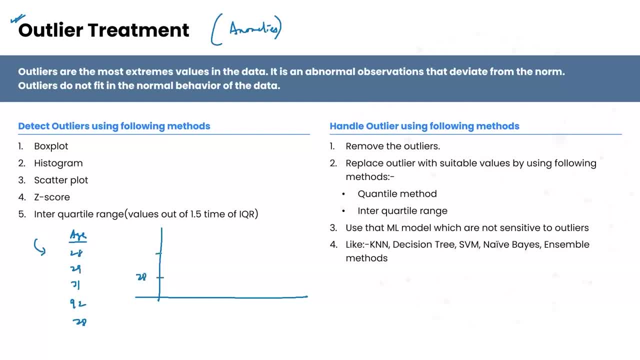 most of them are in the range of 28 to 31, but one of them is far away from that particular distribution. this basically means that this data point is not a part of the regular distribution of the data, which makes it as an outlier, as a potential outlier. similarly, let's say you: 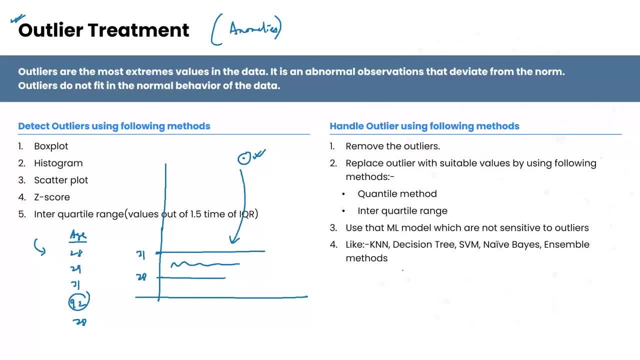 are analyzing sales data in. in the month of january we did a 120 million sales, then 150 million, then 130 million and then suddenly one month there was a 10 million sales and again we are back to track. so you can see, in the month of april there is a downfall. most of the data points are here. 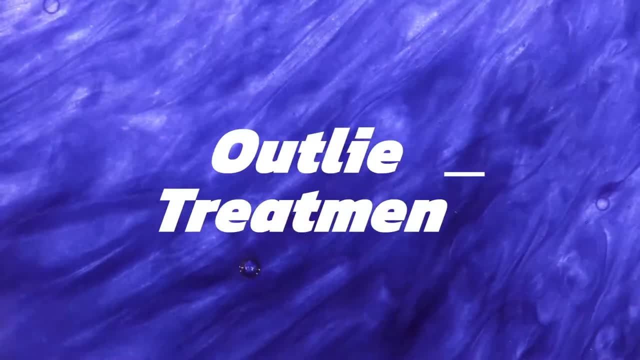 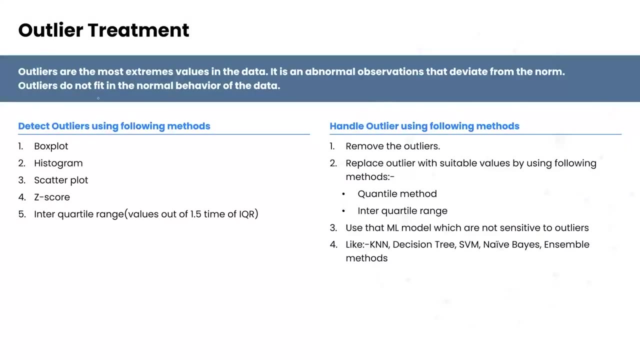 we'll see you in the next video. let's talk about the next type of data cleaning activity that we do, which is outlier treatment. in simple terms, outliers are the most extreme values in the data. it is an abnormal observation that deviates from the normal data. outliers do not fit in the normal behavior of the data. 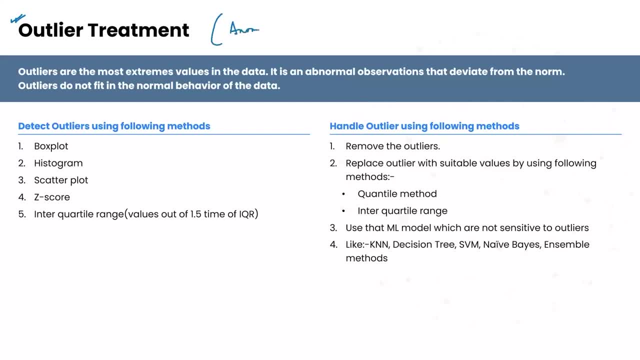 outliers are also called as anomalies. now how do we spot outliers? there are different techniques to spot outliers, but before getting into the detection part, let's try to understand what outlier is. now imagine there are different people with different age: 28, 29, 31, 92, 28.. now if i simply plot them, 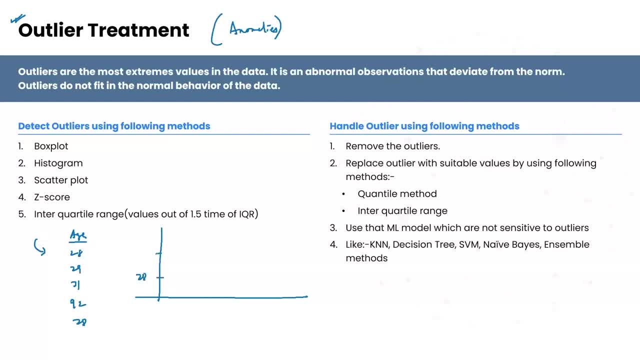 most of them are in the range of 1.98 and 0.98. these values are actually slightly different and of 28 to 31, but one of them is far away from that particular distribution. this basically means that this data point is not a part of the regular distribution. 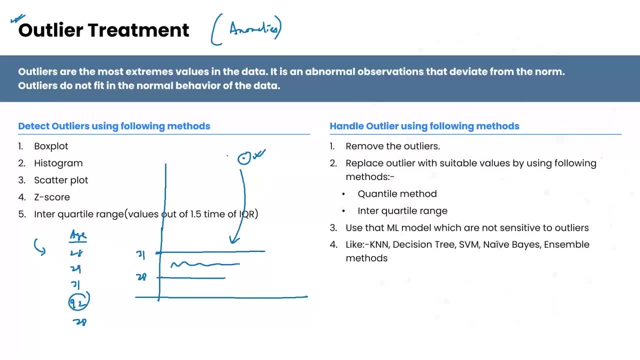 of the data which makes it as an outlier, as a potential outlier. similarly, let's say you are analyzing sales data in in the month of January we did a hundred twenty million sales, then a hundred fifty million, then a hundred thirty million and then, suddenly, one month, there was a ten million sales and again. 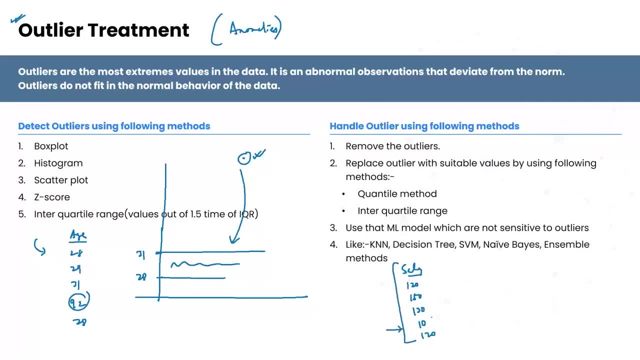 we are back to track so you can see in the month of April there is a downfall. most of the data points are here, but in this April month you see a very high demand downfall. now this could also be a outlier, so outliers are pretty much common in any kind of data. what needs to be done to detect outliers there are. 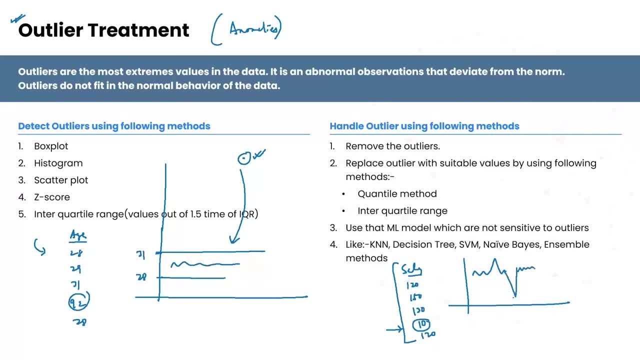 but in this april month you see a very high downfall. now this could also be a outlier, so outliers are pretty much common in any kind of data. what needs to be done to detect outliers? there are different techniques to detect outliers. now we shall be talking about each of these techniques. the first technique: to detect an. 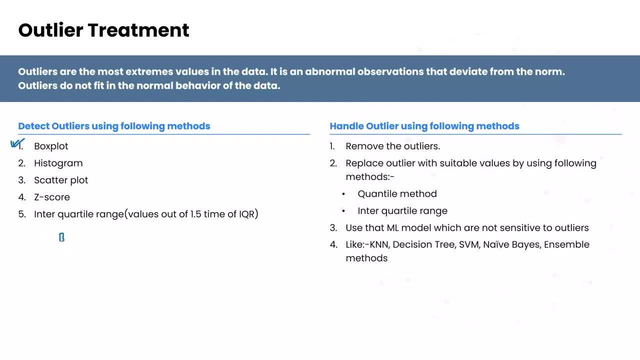 outlier is a box plot. box plot is simply one of the plots which looks like this, where it focuses on five important factors or five important measures, one of them being minimum value, which is this question, one of the one of them being maximum value, which is this, one of them being the median value, which is this. 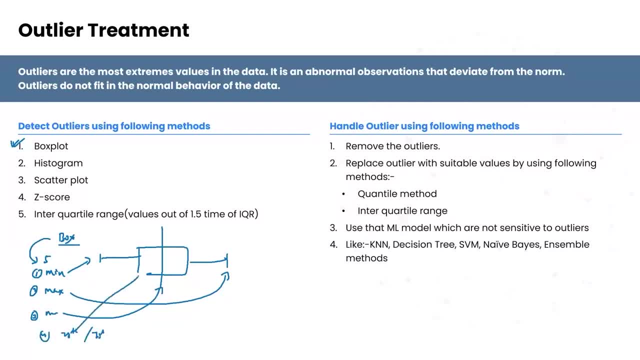 25th percentile and 75th percentile, which is this and this it is also called as q1 and q3. using box plots also, you will be able to identify the outliers. let's say, in this particular portion, fifty percent, of your data lies. the part of theımant to be 1 is 5. 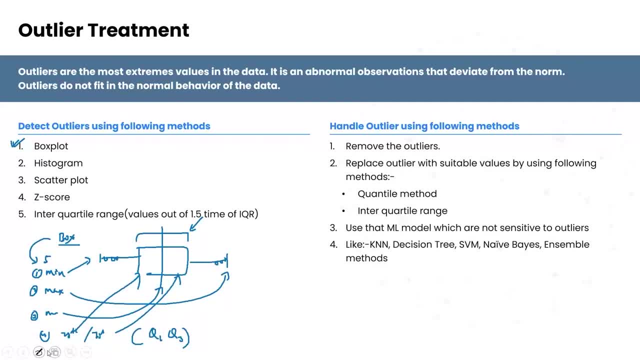 here could be your potential out layers: using histograms also, you can spot out layers. for example, you have h and you have different distribution: 28, 29 dot dot dot, and one of them is 92 dot dot dot, something like that. what if you spot- let's say you draw the graph, it looks: 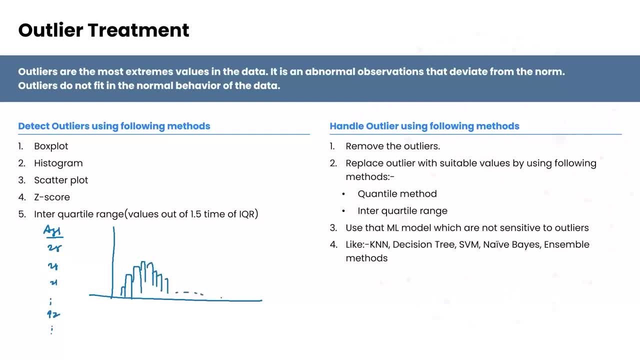 like somewhere like this and then somewhere you have a data point here. or else if you convert this into a age bin- 25 to 31 age bin, 15 to 21 age bin and based on age bins, when you are plotting the histogram, you potentially spot an out layer somewhere here. using scatter plots also, you can 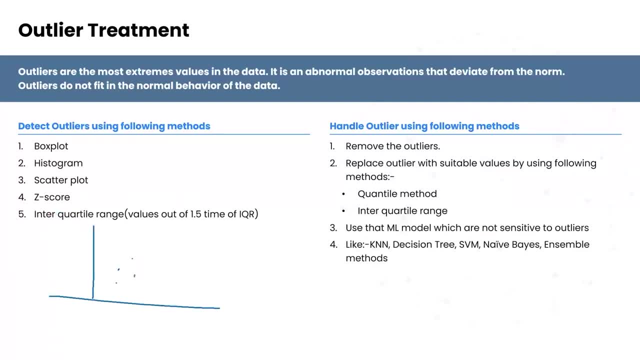 identify out layers. let's say, most of your data points are around this area, so it is quite evident that most of the data points are in this range and the data points falling out of that range are the potential out layers. another way of identifying out layers is the most classical way, which is the normal distribution curve. we 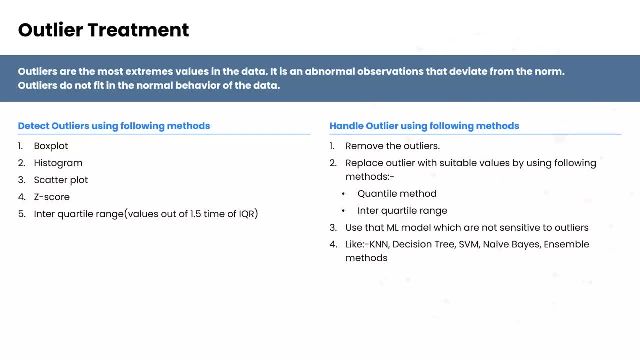 different techniques to detect outliers. now we shall be talking about each of these techniques. the first technique to detect an outlier is a box plot. box plot is simply one of the plots which looks like this, where it focuses on five important factors or five important measures. one of 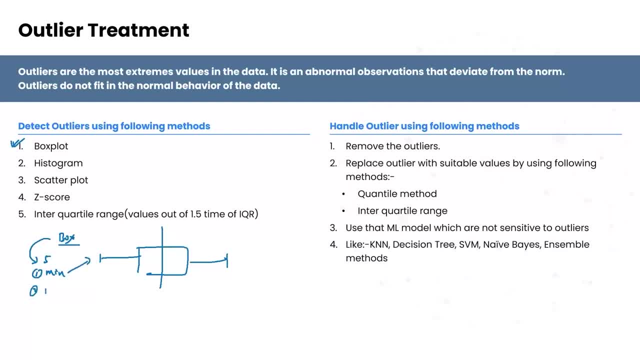 them being minimum value, which is this, one of the one of them being maximum value, which is this, one of them being a median value, which is this: 25th percentile and 75th percentile, which is this and this it is also called as Q 1. 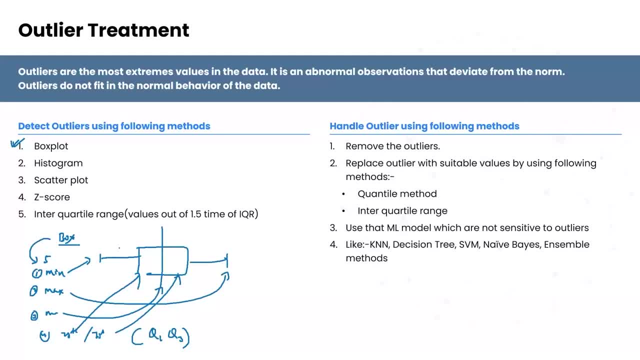 and q3. using box plots also, you will be able to identify the outliers. let's say, in this particular portion 50 percent of your data lies. the data points which are lying around here could be your potential outliers. using histograms also, you can spot out layers. for example, you have age. 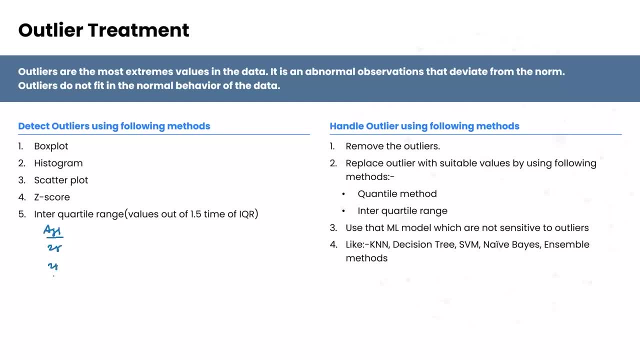 and you have different distribution: 28, 29 dot dot, and one of them is 92 dot dot dot, something like dot dot, and one of them is 92 dot dot dot, something like out. what if you spot, let's say you draw the graph, it looks like somewhat like this, and then somewhere you have a data point here, or else if you convert, 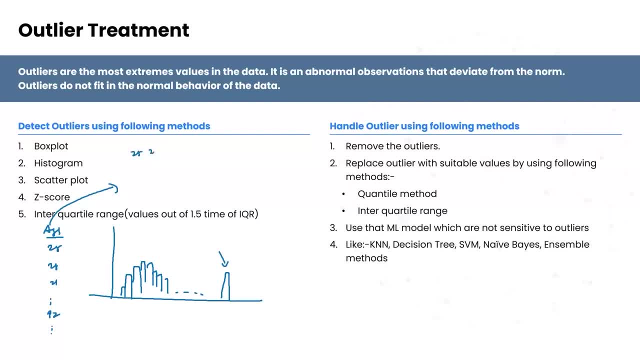 this into a age bin 25 to 30, one one age bin, 15 to 21 age bin and based on age bin, that means generic age. consider that this is theAsked class of the data in the table, but you also age bins. when you are plotting the histogram, you potentially spot an outlier somewhere here. 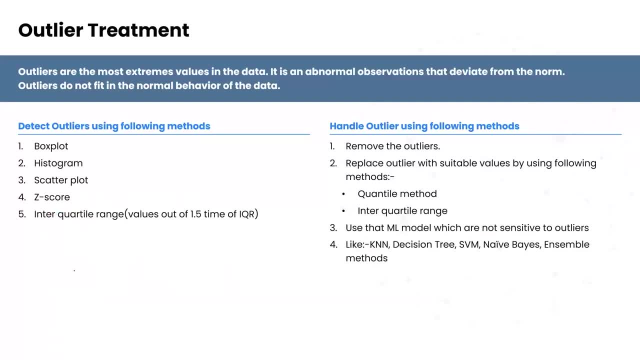 using scatter plots also, you can identify outliers. let's say, most of your data points are around this area, so it is quite evident that most of the data points are in this range and the data points falling out of that range are the potential outliers. another way of identifying outliers: 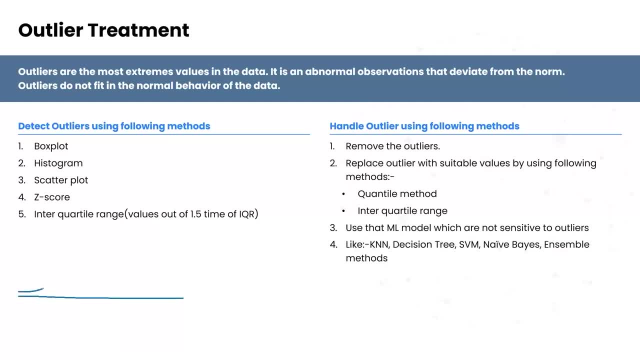 is the most classical way, which is the normal distribution curve. we all know that in a normal distribution curve, almost 99.7 percent of the data lies between plus minus three. standard deviation: one, two, three, one, two, three. we all know that this is basically 99.7 percentage data. right, this is plus three sigma. 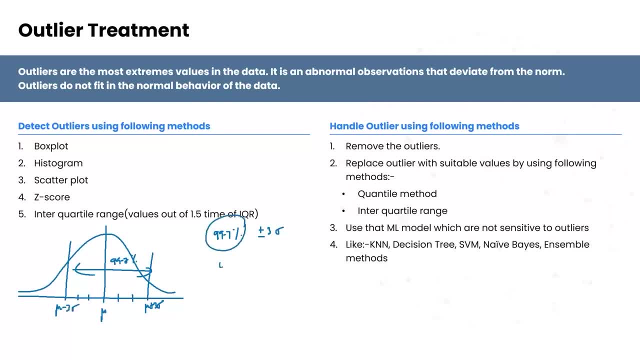 and this is minus three sigma. what happens to the point three percent, which lies beyond this, are nothing but your outliers. so there are different techniques using which we identify outliers. what needs to be done with those outliers? so, by격's, this is the way you should be working with these outliers. 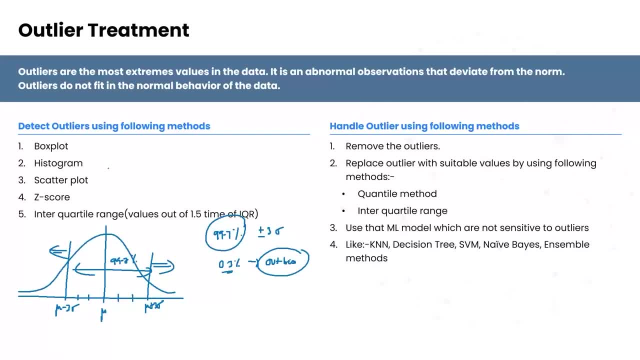 you should be working with the outliers. so if you try to use outliers to your outlier, you are not going to be able to outlier because you are not going to be able to outlier, and so there is no rule for that. that in this particular scenario, we should get rid of this. in this particular scenario, we should not get rid of this. 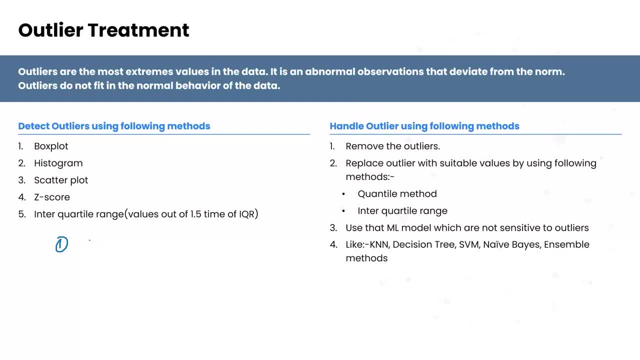 data to predict something. just a simple example is: imagine you have been noting down the temperature of your country. let's say you, you stay in malaysia, you have date and you have temperature. every day you are noting the temperature. obviously some of these temperatures could be outliers. suddenly in one of the days there was 41 degrees, suddenly it was 17 degrees. let's say: 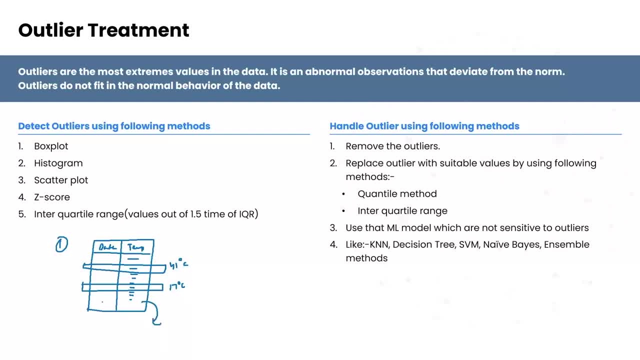 now, if you are forecasting the value, let's say you have data for six months and you want to forecast for the next particular instance, so you should always take care of these outliers. you should not drop these outliers because it's a time series forecasting problem and each data point is important. there could be an internal pattern that you are not able. 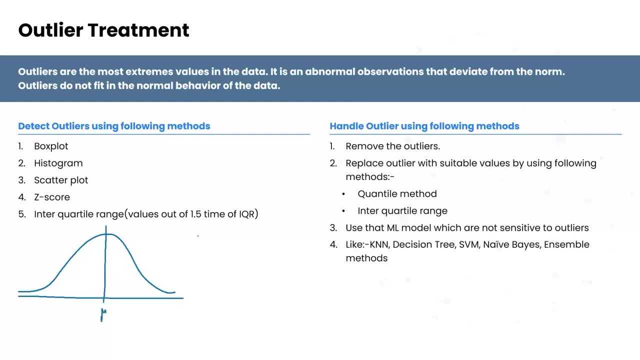 all know that in a normal distribution curve, almost 99.7 percent of the data lies between plus minus 3 standard deviation: one two, three. one two three. we all know that this is basically 99.7 percentage data. right, this is plus three sigma and this is minus three sigma. what happens to the 0.3 percent? 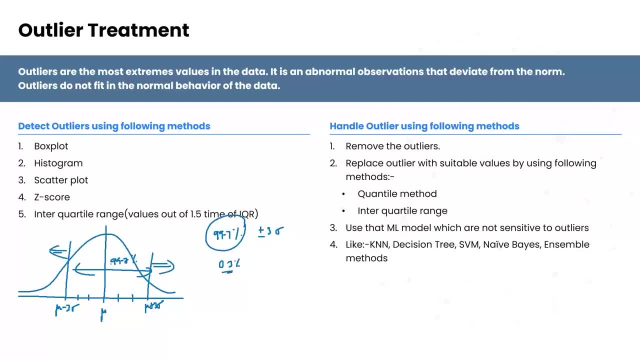 which lies beyond this are nothing but the percent of the data that isbiggest your outliers. so there are different techniques using which we identify outliers. what needs to be done with those outliers is- there is no thumb rule for that- that in this particular scenario, we 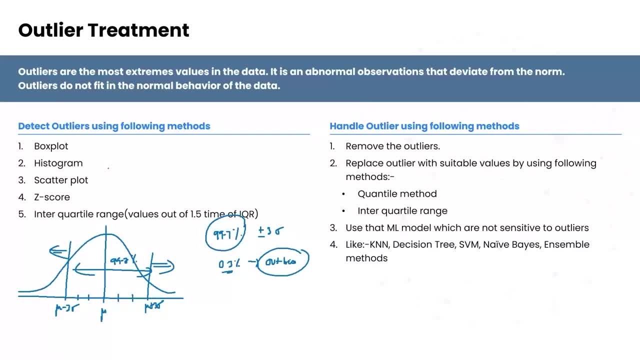 should get rid of this in this particular scenario. we should not get rid of this now. i can give you some of the examples where you need or need not have to treat. doubtless the first use case is time series forecasting. time series forecasting is one of those areas and our predictive analytics where 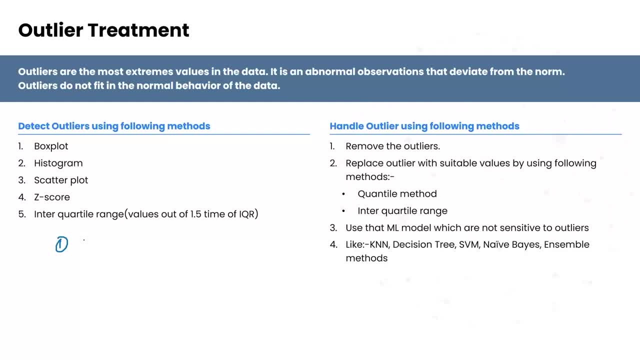 we use time series data to predict something. just a simple example is: imagine you have been noting down the temperature of your country. let's say you, you stay in Malaysia, you have date and you have temperature. every day you are noting the temperature. obviously some of these temperatures could be outliers. suddenly, in one of the days there was 41 degrees suddenly. 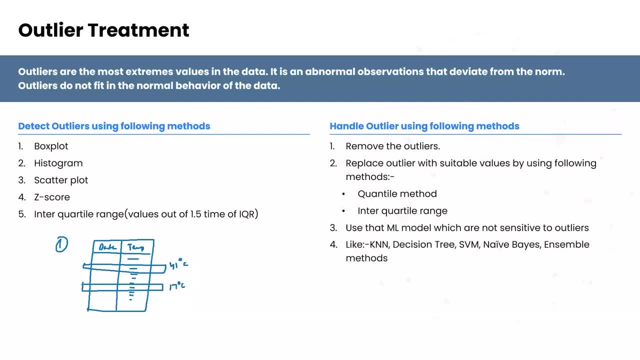 it was 17 degrees, let's say. now, if you are forecasting the value, let's say you have data for six months and you want to forecast for the next particular instance- so you should always take care of the data and you should always take care of the data and you should always take care. 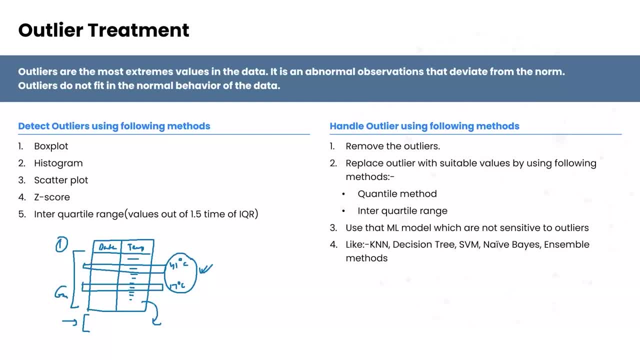 of these outliers. you should not drop these outliers because it's a time series forecasting problem and each data point is important. there could be an internal pattern that you are not able to understand where your models could be able to understand. so never get rid of your outliers. 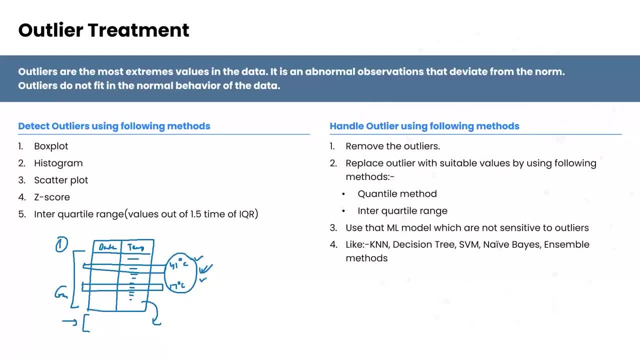 to understand where your models could be able to understand. so never get rid of your outliers, especially in a time series problem. there are multiple other scenarios. maybe one of the scenarios could be if you are dealing with a data set and one or two people are basically falling in this category, where their age is very high. 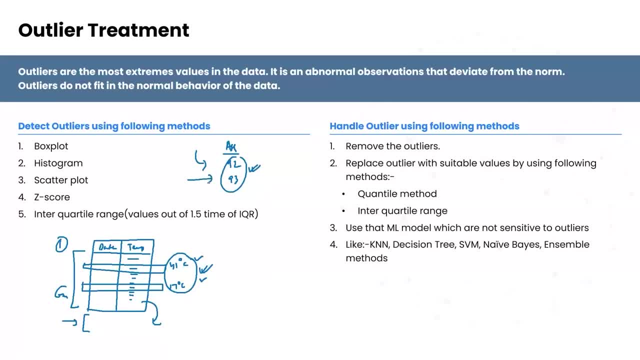 now, in this case, if you want to remove, you can remove. if you want to keep it, you can remove it. there is no right or wrong. the process is very simple, exactly like the way we discussed earlier when it comes to predictive analytics. it is a iterative process. it is 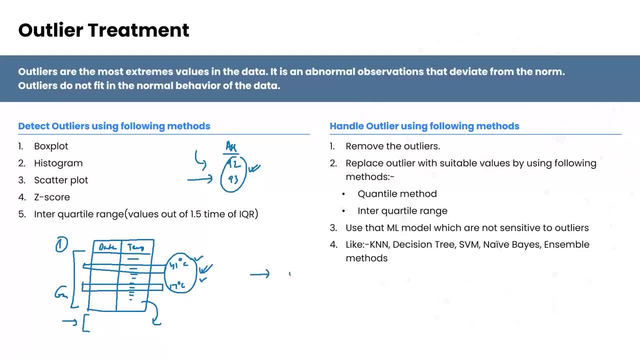 a hit and trial process. first of all, you remove them, check the model's behavior, how the model is performing, again, go back and then again add those outliers and see how the model is behaving. that is how we finalize our predictive analytics model, whether it is behaving well with the outliers or not, because going forward in the 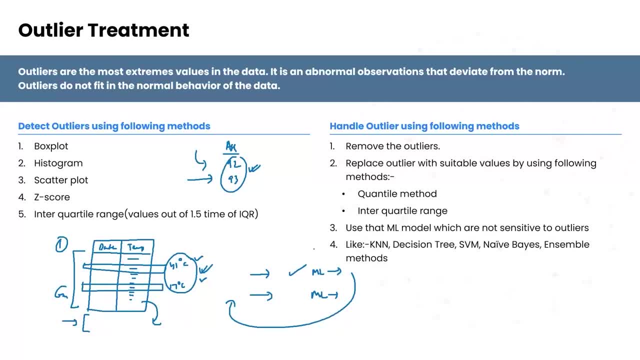 predictive analytics, you will learn a lot of algorithms which are not prone to outliers. that means they do not care about outliers. you can see the point number four, where we have multiple algorithms like k, nearest neighbors, decision trees, support vector machines, knife base and some ansible methods which do not worry about outliers. 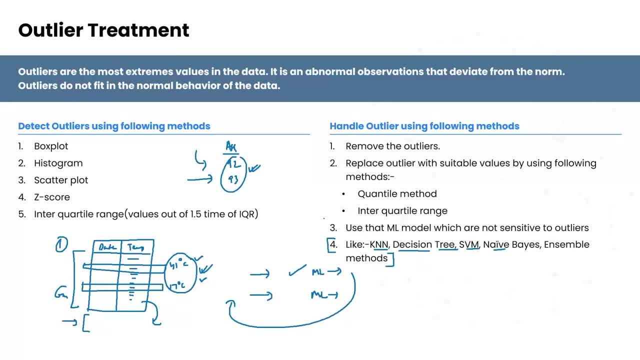 they are okay if the data is having outliers. so how do we handle outliers? using following methods: remove the outliers- yeah, could be one of the techniques. replace outliers with suitable values by using following methods: quantile method or interquartile range, use that ml model- which are not sensitive to outliers. okay, so with due course of time, once we jump. 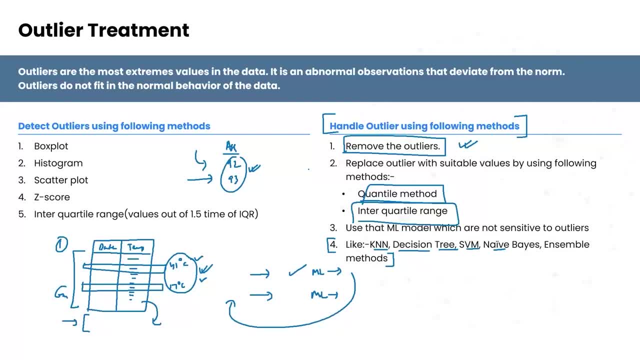 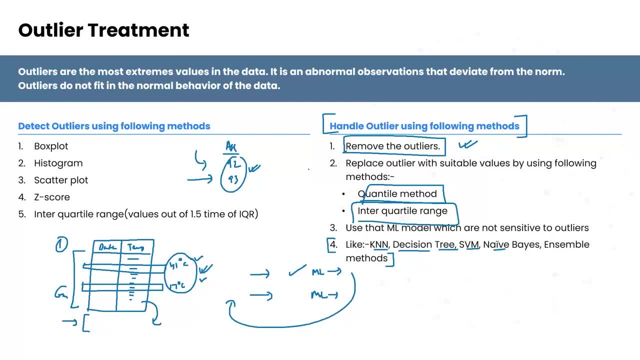 predictive analytics. we should always do a hit and trial. there is no right or wrong when it comes to the descriptive part or the ada part, where we are just analyzing the data. in that case it is completely fine whether to keep the outlier or not keep. that is completely. 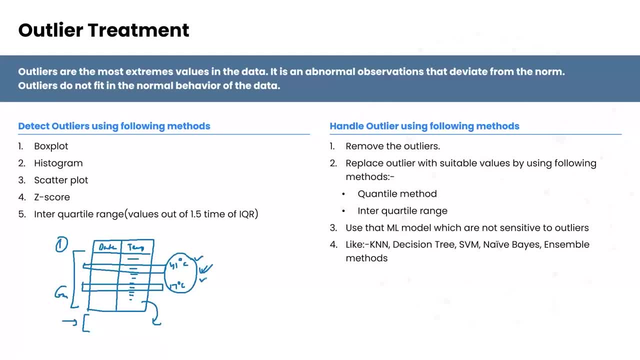 especially in a time series problem. there are multiple other scenarios. maybe one of the scenarios could be: if you are not able to understand your models, you should never get rid of your outliers if you are dealing with a data set and one or two people are basically falling in this category. 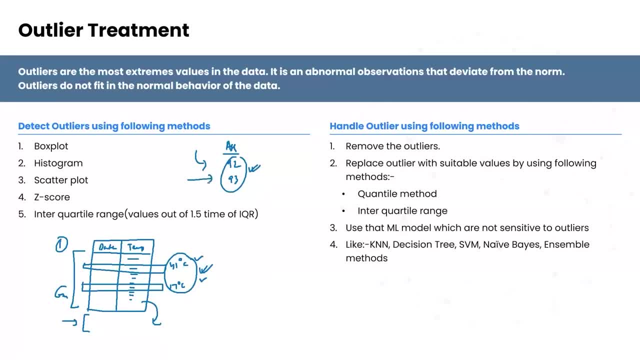 where their age is very high. now, in this case, if you want to remove, you can remove. if you want to keep it, you can keep it. there is no right or wrong. the process is very simple, exactly like the way we discussed earlier when it comes to predictive analytics, it is a iterative process. 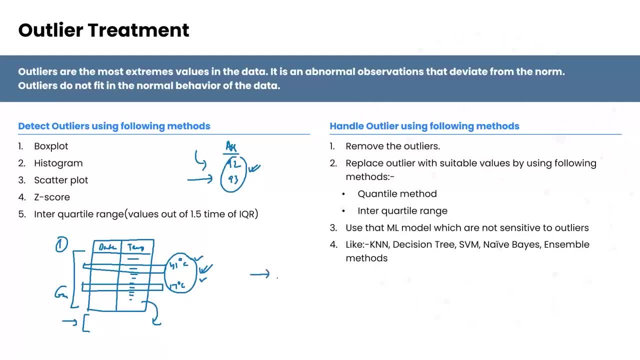 it is a hit-and-trail process. first of all, you remove them, check the model's behavior, how the model is performing, again go back and then again add those outliers and see how the model is behaving. that is how we finalize our predictive model: whether it is behaving well with the outliers. 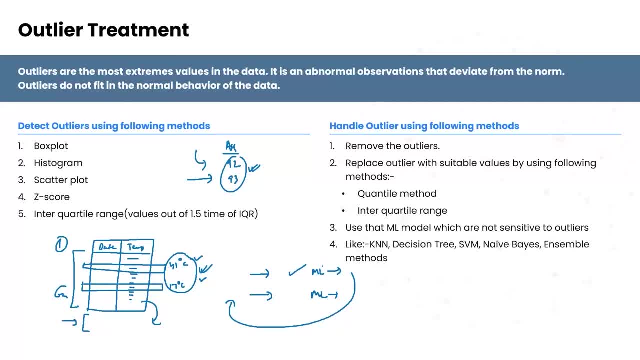 or not, because going forward in the predictive analytics, you will learn a lot of algorithms which are not prone to outliers. that means they do not have a clear outcome. that means they do not care about outliers. you can see the point number four, where we have multiple algorithms like 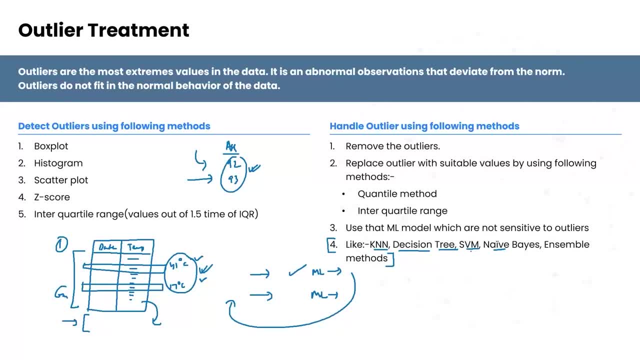 k. nearest neighbors- decision trees, support, vector machines, knife base and some ansible methods which do not worry about outliers. they are okay if the data is having outliers. so how do we handle outliers? using following methods: remove the outliers- yeah, could be one of the techniques. replace outliers with suitable values by using following methods: quantile method. 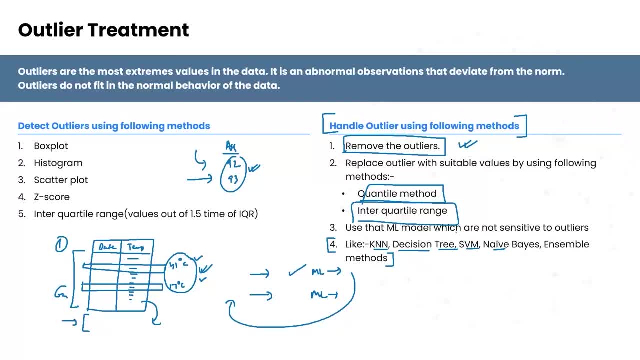 or interquartile range, use that ml model, which are not sensitive to outliers. okay, so with due course of time, once we jump into practicals, probably you will have better understanding on where to keep the outliers and where to ignore the outliers, especially in the field of predictive, predictive analytics. we should always do a. 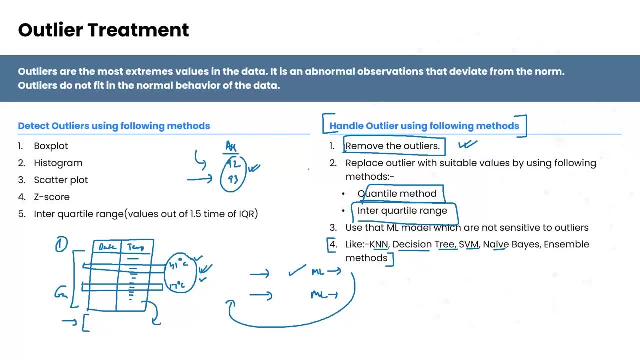 hitting test trial. there is no right or wrong when it comes to the descriptive part or the ada part, where we are just analyzing the data, in that case it is completely fine. whether to keep the outlier or not keep, that is completely fine. so that's all about the theoretical concepts behind outlier. 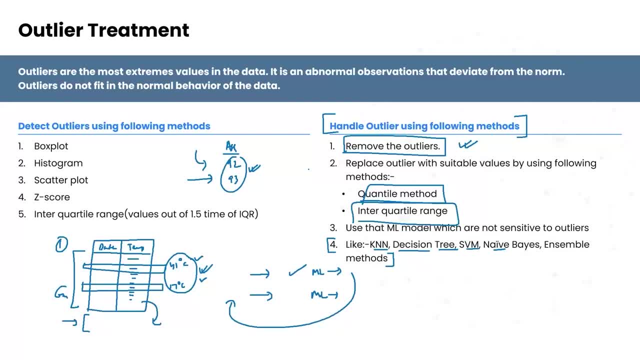 fine. so that's all about the theoretical concepts behind outlier treatment. in the next video we shall be talking about the python part. how do we see an outlier using boxplot histograms and how do we see using the normal distribution and all those things? so that's all about this. 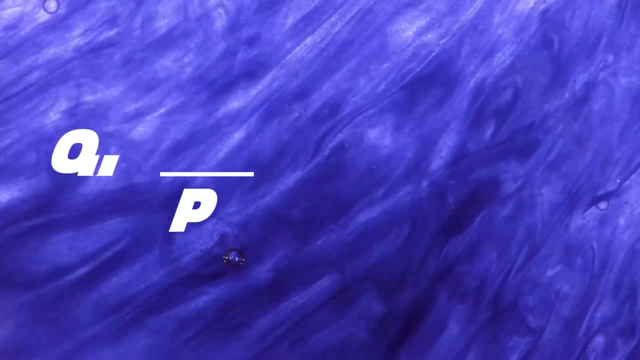 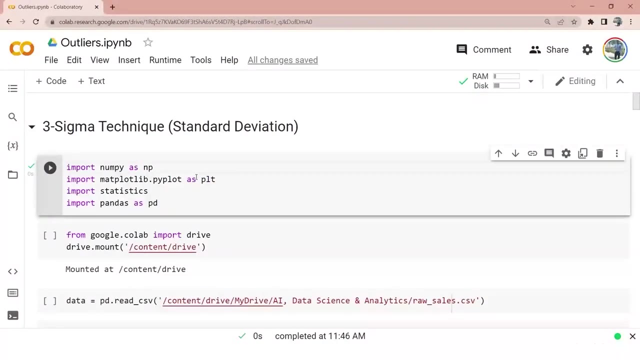 particular video. see you in the next video. bye, bye, hi. welcome to this practical session on outliers. in this video we shall be talking about the different techniques that you want we use to identify outliers in data. so the first technique i am going to talk about is the three. 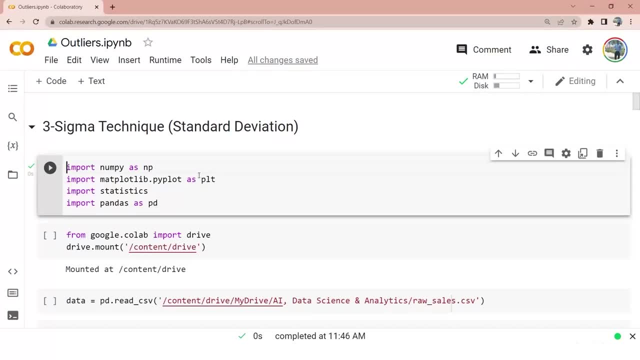 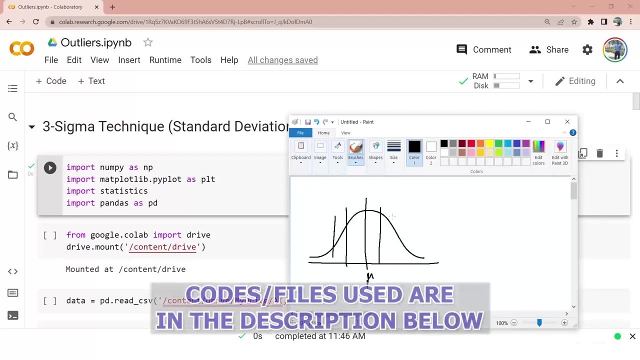 sigma technique, which is based on the principles of normal distribution, which we already know. normal distribution is nothing but something like this: right, where the middle value is your mean value, we have plus minus one, plus minus two, plus minus three standard deviation. anything beyond your plus minus three standard deviation is treated as an outlier if your data is perfectly. 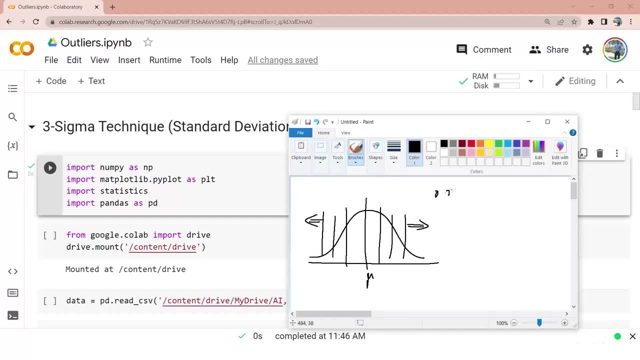 following the normal distribution curve, then 0.3 percentage of your data will be your outliers. but as we know, normal distribution is a hypothetical scenario. not all data can be hundred percent normally distributed. so your anything beyond plus minus three standard deviation could be any value ranging from 0.3 to x percentage. that could be even one percentage, two percentage. 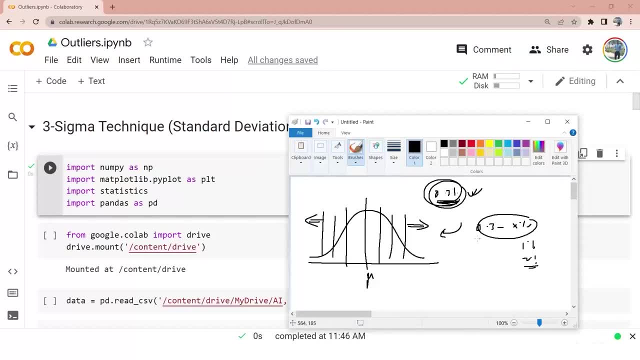 it depends how normally distributed your data is. so in this particular example, when i talk about three sigma technique, that basically means anything that falls beyond your plus minus three standard deviation is treated as an outlier. so we have created a function for this particular technique and we will be passing it on to the next class. 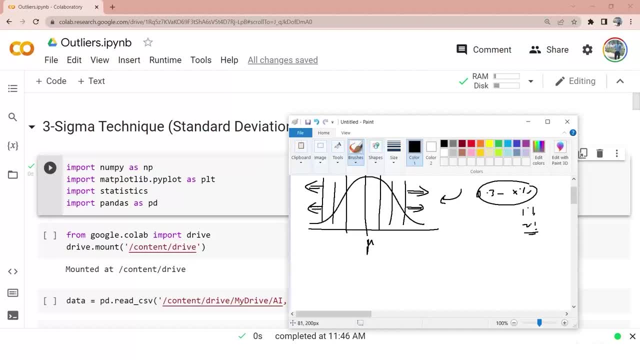 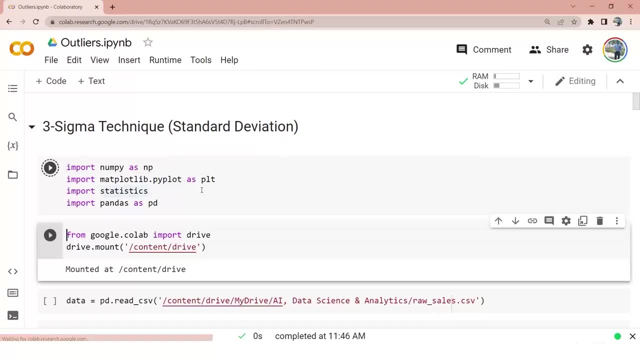 so we have created a function for this particular technique and we will be passing the data and we will be seeing what all data points are falling beyond this particular three sigma rule. so, firstly, i have imported all these libraries: numpy, matplotlib, statistics is one of the libraries that we do statistical related things and we have pandas, as i am using google collapse. 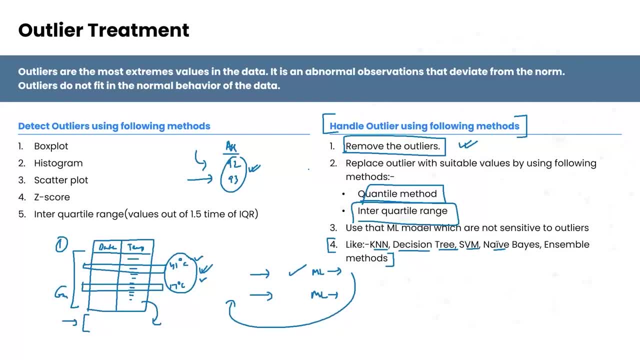 treatment. in the next video we shall be talking about the python part. how do we see an outlier using box plot histograms and how do we see using the normal distribution and all those things? so that's all about this particular video. see you in the next video. bye-bye. 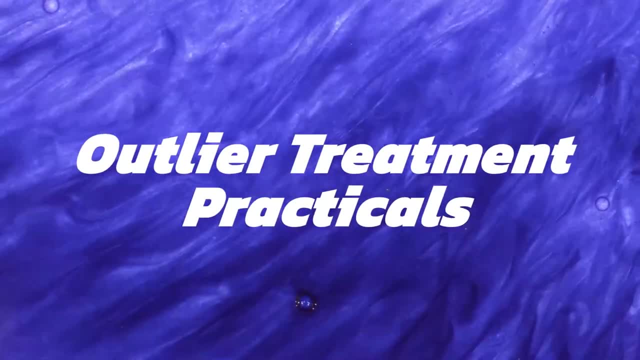 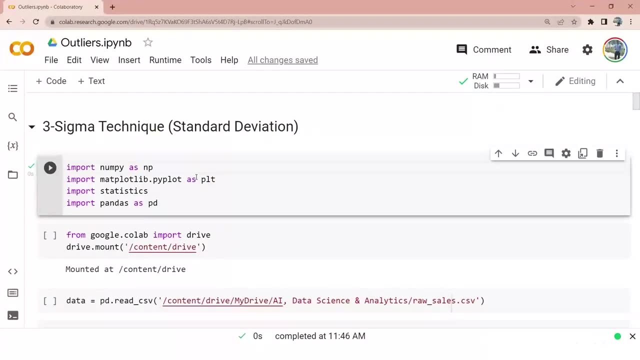 hi, welcome to this practical session on outliers. in this video we shall be talking about the different techniques that we use to identify outliers in data. so the first technique i am going to talk about is the three sigma technique, which is based on the principles of normal distribution, which we already know. normal distribution is nothing but something like this: 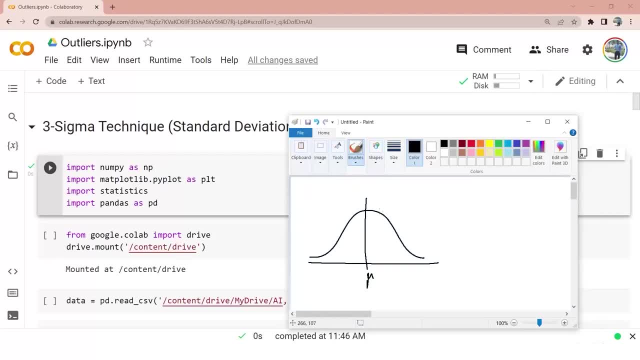 right where the middle value is your mean value, we have plus minus 1, plus minus 2, plus minus 3 standard deviation. anything beyond your plus minus 3 standard deviation is treated as an outlier. if your data is perfectly following the normal distribution curve, then 0.3 percentage of your 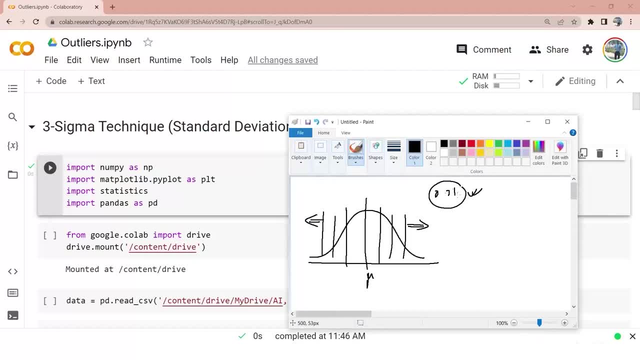 data will be your outliers. but, as we know, normal distribution is a hypothetical scenario. not all data can be 100 normally distributed, so your anything beyond plus minus 3 standard deviation could be any value ranging from 0.3 to x percentage. that could be even one percentage two. 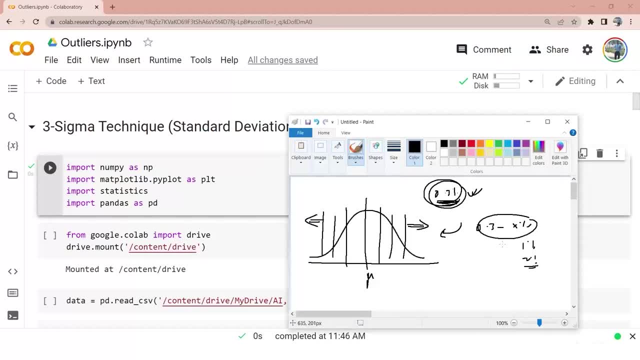 percentage. it depends how normally distributed your data is. so in this particular example, when i talk about three sigma technique, that basically means anything that falls beyond your plus minus three standard deviation is treated as an outlier. so we have created a function for this particular technique and we will be passing the data and we will be seeing what all. 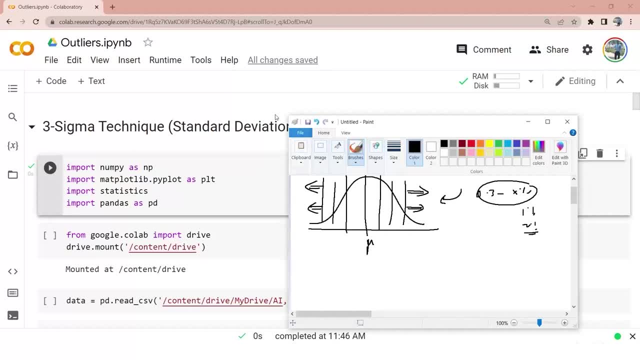 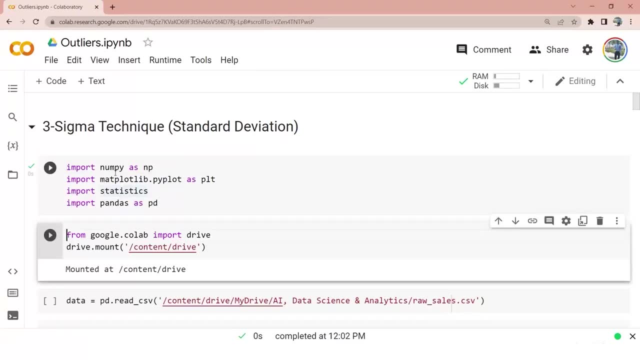 data points are falling beyond this particular three sigma rule. so, firstly, i have imported all this library as numpy and i have imported all these libraries as numpy and i have imported all these libraries as numpy. matplotlib statistics is one of the libraries that we do statistical related things and we have pandas. as i am using google collapse, so i have mounted my google drive. 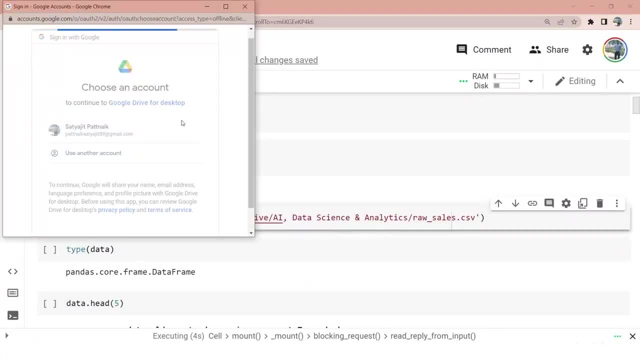 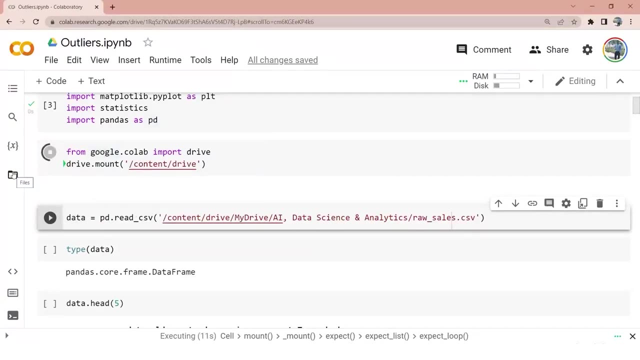 so i have mounted my google drive. so i'm going to give access to my google drive so that i can read this file from my google drive itself. but just in case you don't want to do this, you can just click on files, upload this particular file and you are good to go. so the data, the drive, has been mounted. 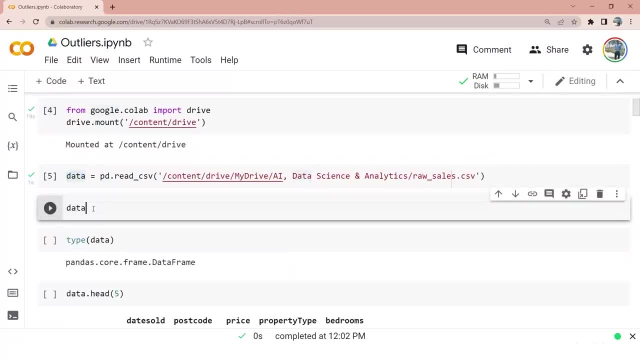 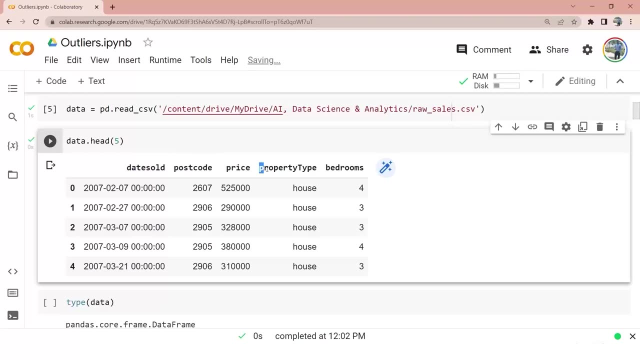 and that's how my data looks like. right? so if i just do data dot head, that's how my data looks like. i have data: sold postcode, price, property type, bedrooms, fahrenstein. here, once again, you need to see some information to be used when you dancesact the king sergeant, so we have been creating a quality page function here, in this case, where the screen is yellow centerですね. that's work on. what does that mean? so that's all you need to do, as i have created these files from one side of an online privacy escrame. here we are adding some design and other available supports. so you need to create a cloud folder to you car dot com to create your own product code page and сделd data streetglare. you can save it demonstrating right click on image. personal blog y. 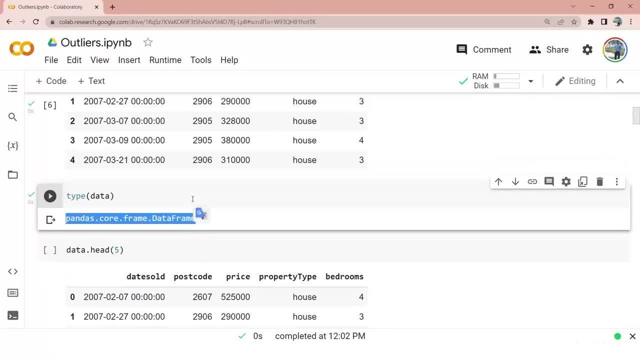 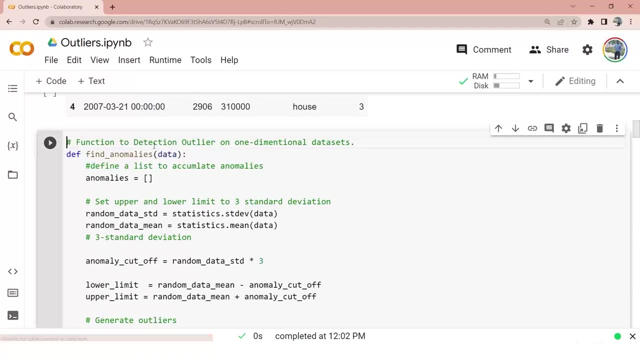 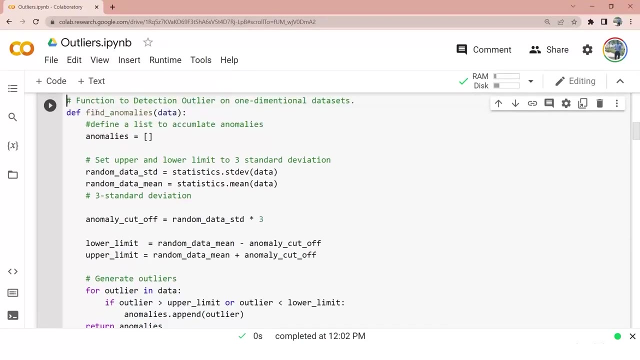 the type of data. it's quite evident it is a data frame because it is used from pd, dot c, read csv. now, this is the function that we have created: function to detect outlier on one dimensional data sets. if you look at this particular function, it's very easy to understand. i have defined the 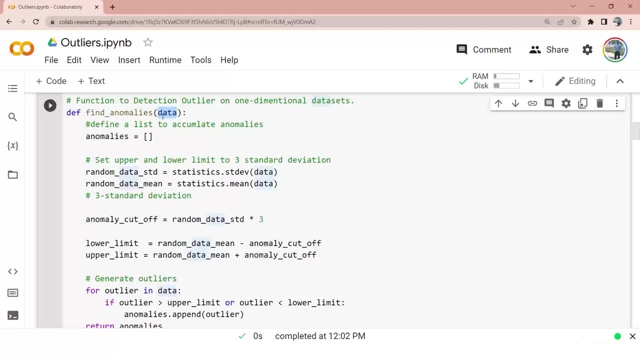 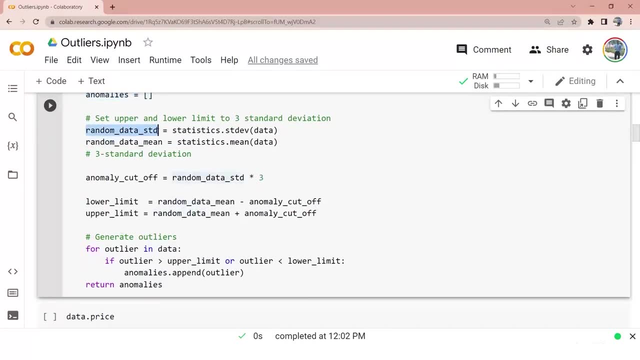 function name as find anomalies. i am expecting some data here. i have created a null list, an empty list. first of all, i'm calculating the standard deviation. second of all, i'm calculated, calculating the mean, using the statistics library and i'm storing the standard deviation and mean. very 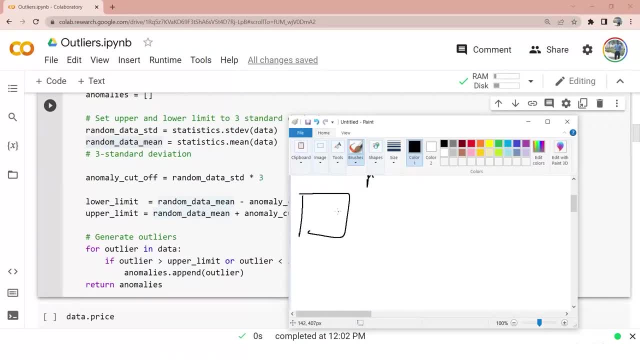 simple. so what's happening here is i have the data and i am calculating the standard deviation, which is my sigma and my mean, which is my mu. next is i have defined anomaly cutoff equal to standard deviation into 3.. so i have defined a variable called as anomaly cutoff, which is standard deviation into 3. 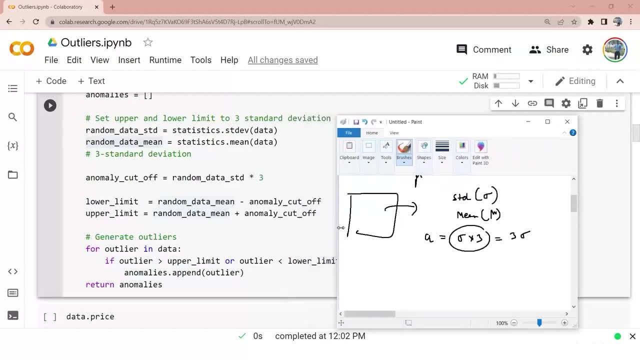 which is simply 3 sigma. you can see i have defined. my lower limit equals to random data mean minus anomaly cutoff. so my lower limit is mean minus 3 sigma. my upper limit cutoff is mu plus 3 sigma. this is pretty clear. this part is basically mu minus 3 sigma and this is your mu plus 3 sigma, right? so the logic that we are going. 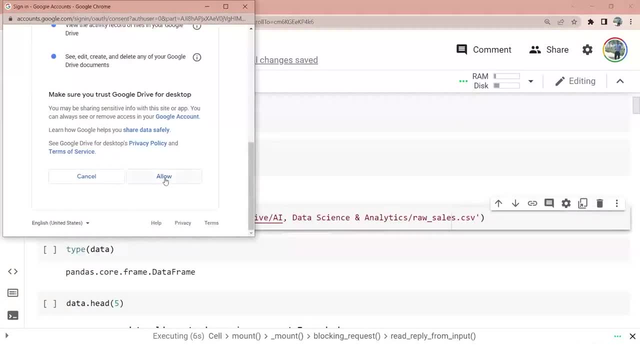 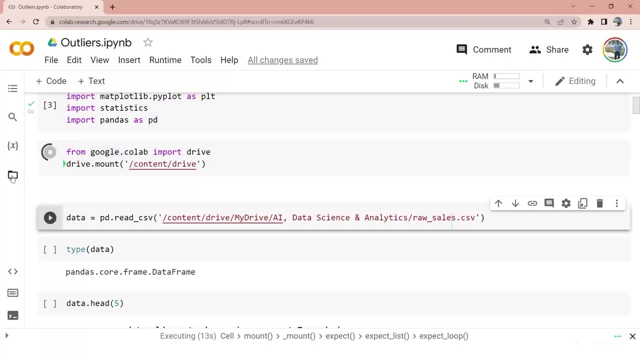 so i'm going to give access to my google drive so that i can read this file from my google drive itself. but just in case you don't want to do this, you can just click on files, upload this particular file and you are good to go. so the data, the drive, has been mounted, and that's how my data looks like. 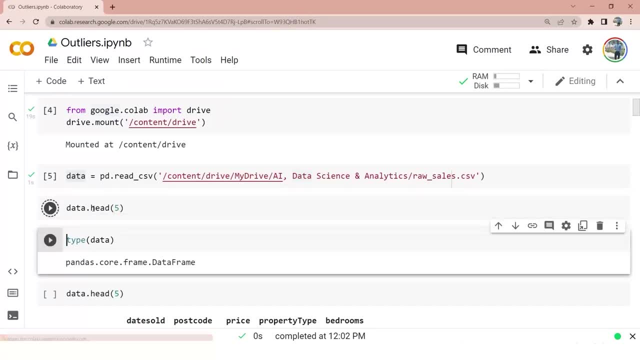 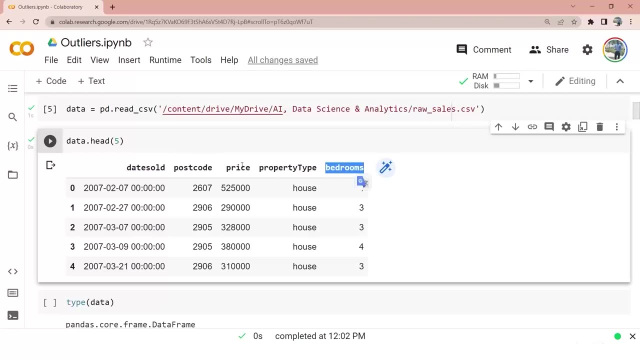 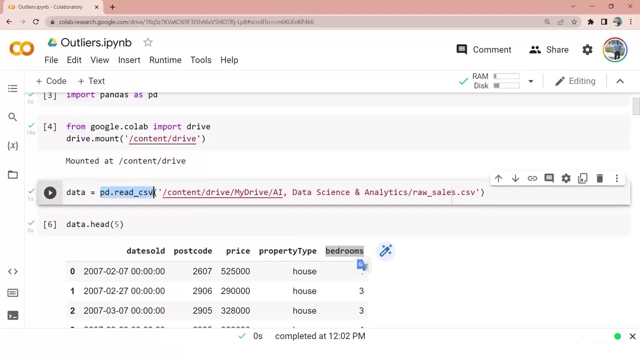 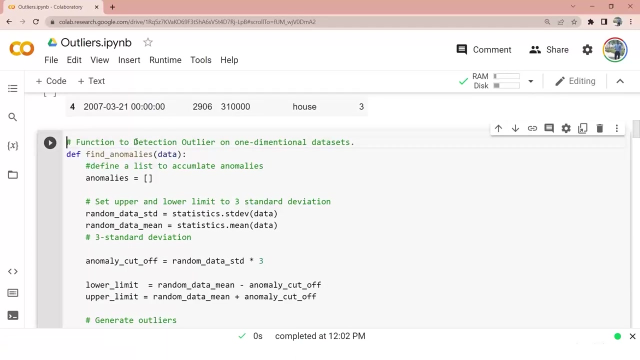 right. so if i just do data dot head, that's how my data looks like. i have data: sold postcode, price, property type: bedrooms. what is the type of data? it's quite evident: it is a data frame, because it is used from pd, dot c, read csv. now, this is the function that we have created. function to: 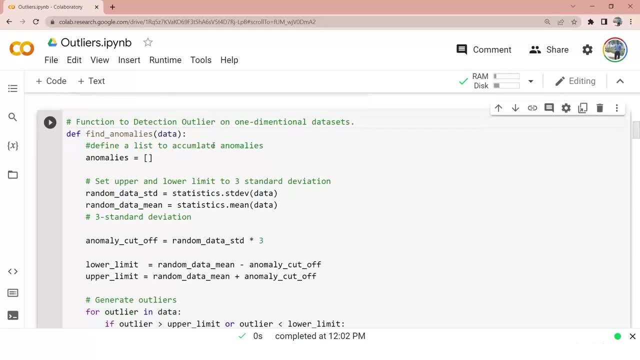 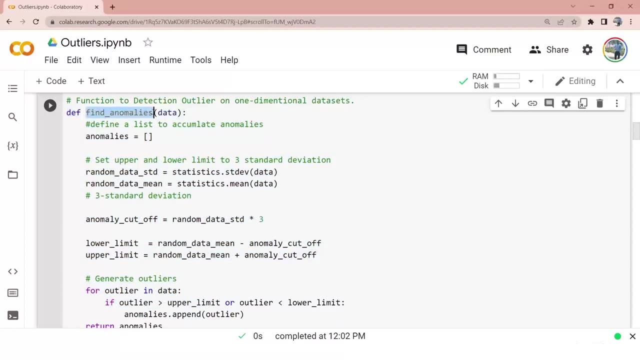 detect outlier on one dimensional data sets. if you look at this particular function, it's very easy to understand. i have defined the function name as find anomalies. i am expecting some data here. i have created a null list, an empty list. first of all, i am calculating the standard deviation. 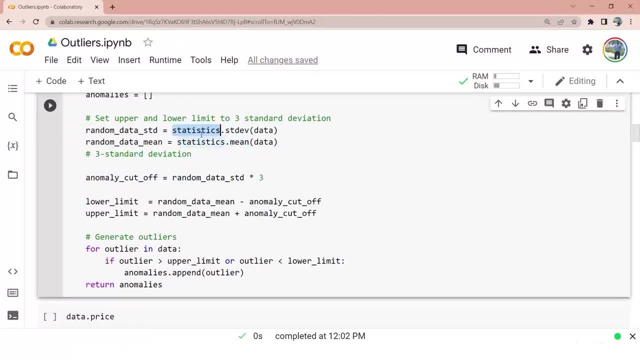 second of all, i am calculated, calculating the mean, using the statistics library, and i'm storing the standard deviation and mean. very simple. so what's happening here is i have the data and i am calculating the standard deviation, which is my sigma, and my mean, which is my. 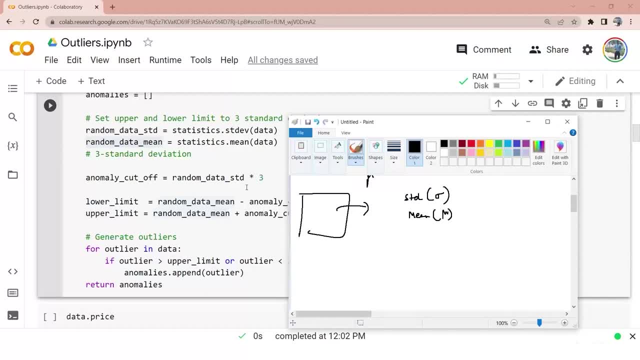 mu next is: i have defined anomaly cutoff equal to standard deviation into 3. so i have defined a variable called as anomaly cutoff, which is standard deviation into 3, which is simply 3 sigma. you can see, i have defined my lower limit. equals to random data mean minus anomaly cutoff. so my 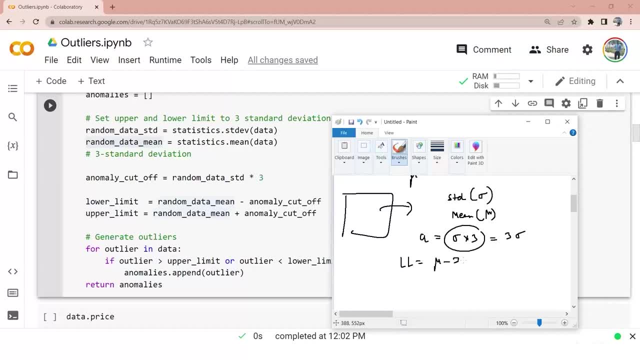 lower limit is mean minus 3 sigma. my upper limit cutoff is mu plus 3 sigma. this is pretty clear. this part is basically mu minus 3 sigma, and this is your mu plus 3 sigma, right? so the logic that we are going to apply here is anything that is greater than mu plus 3 sigma, or anything that 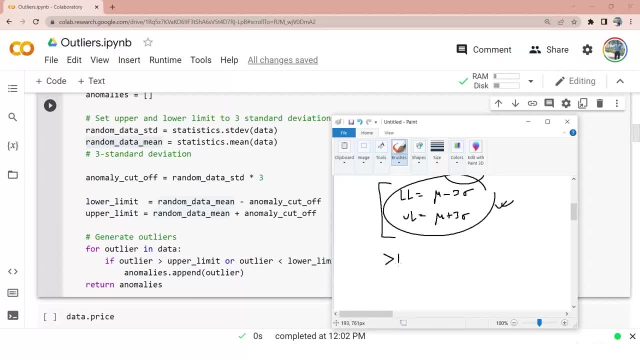 to apply here is anything that is greater than mu plus 3 sigma, or anything that is less than mu minus 3 sigma are basically your outliers. so you can see i'm running a loop over the data for outlier in data. if outlier is greater than upper limit or outlier is lower than, lesser than the lower limit, i'm 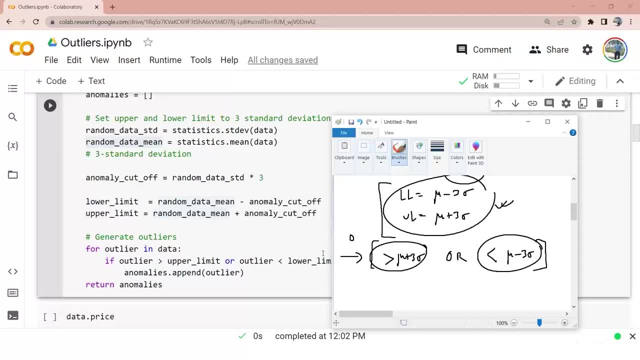 appending this particular data set to anomalies. so let's say i have a data set of 10 records: 10, 20, 50 and 120, let's say, four records. so what's happening here is, for each element, i have calculated the mean, i have calculated the standard deviation, anything that is greater than 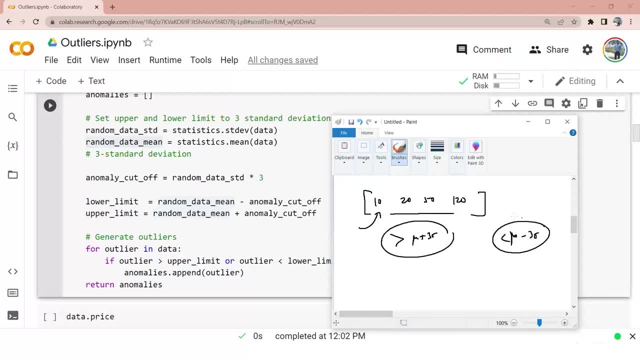 this or anything that is less than this. for example, let's say this one: this value kind of follows this if block it is successful, so in the anomalies this particular data point will be appended, and if you return anomalies you will get something like this: that this is an. 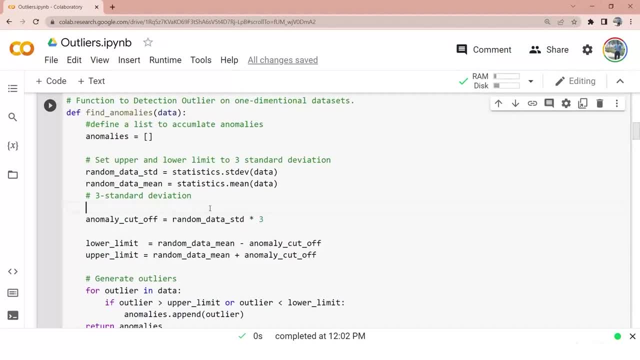 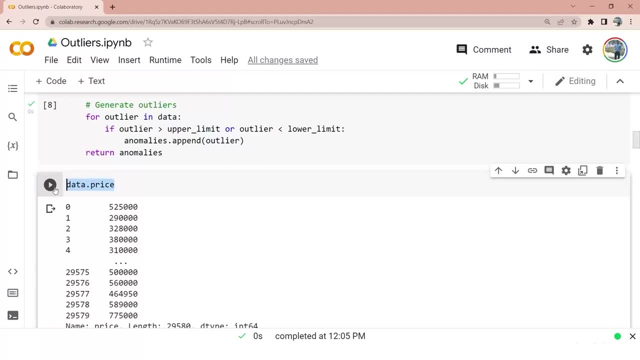 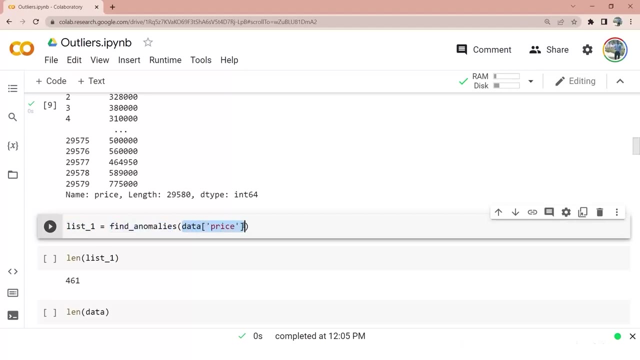 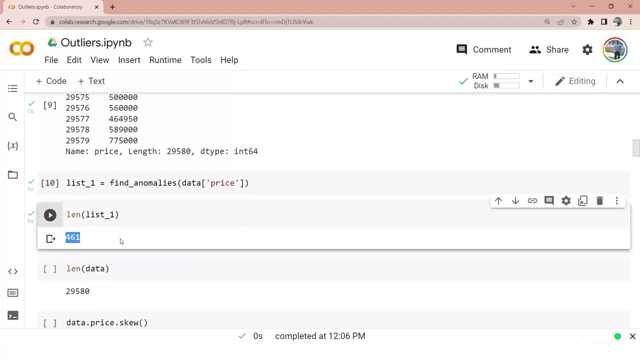 anomaly. okay, so we'll try to quickly run this function and we are going to run this function using the. i'm going to pass this price data, so i'm calling list one equals to find anomalies data of price. if i run this and if i run this, you can see there are 461 outliers. 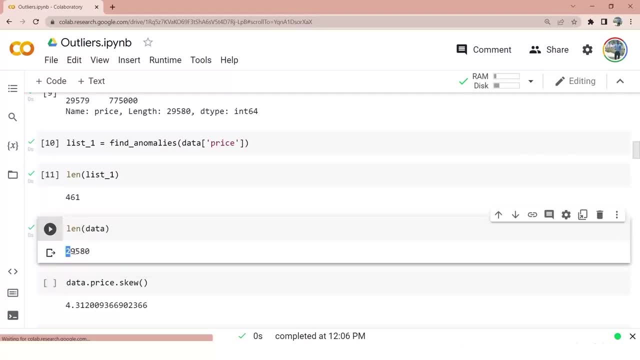 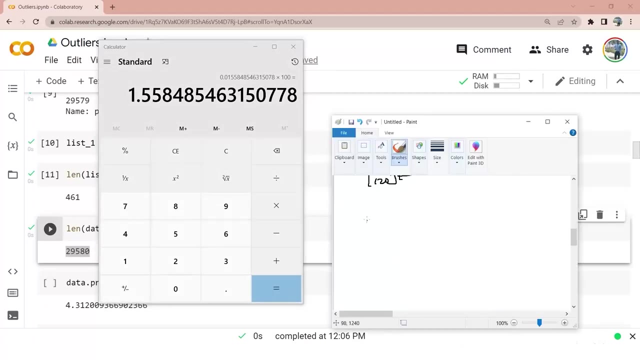 what is the total length of data? it is 29 580. now, if you start calculating 461 divided by 29580 into 100, which is almost 1.55 percent. 1.55 percent of the data are beyond the range of plus minus 3. 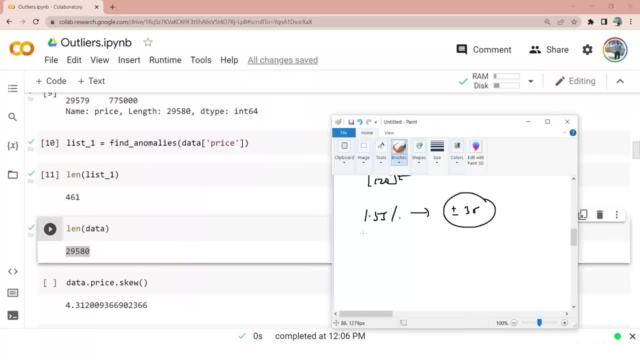 sigma and we know that in in the case, the data is fully available so we can calculate the range of plus minus 3 sigma. and we know that in in the case the data is fully normally distributed. it has to be 0.3 percent data, so this clearly means that the data is not. 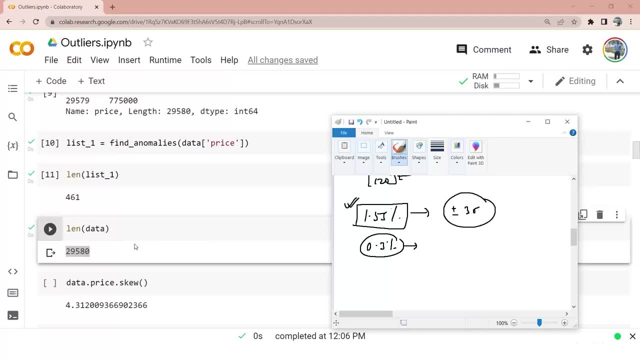 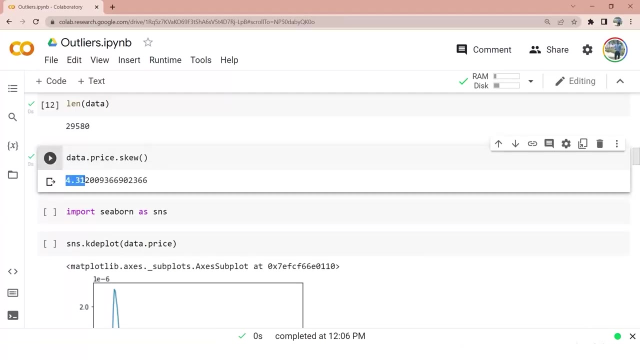 normally distributed. so that's why i'm going to use some skewness function or kurtosis function to see whether the data is skewed or not. so you can see, my skew value is 4.31, which clearly means that the data is rightly the data is. 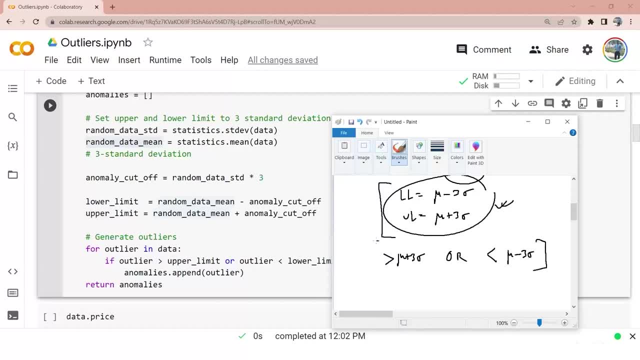 is less than mu minus 3 sigma are basically your outliers. so you can see i am running a loop over the data for outlier. in data, if outlier is greater than upper limit or outlier is lower than lesser than the lower limit, i am appending this particular data set. 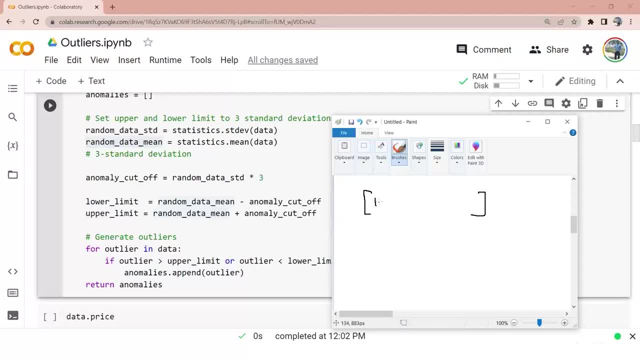 to anomalies. so let's say, i have a data set of 10 records: 10, 20, 50 and 120, let's say, 4 records. so what's happening here is, for each element, i have calculated the mean, i have calculated the standard deviation, anything that is greater than this or anything that is less than this. 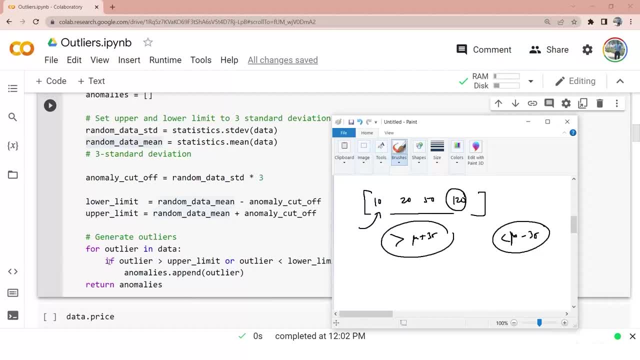 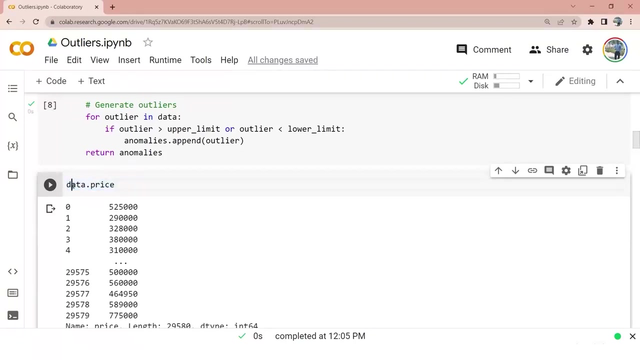 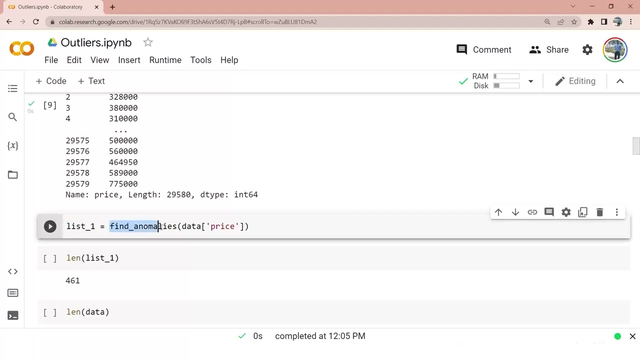 for example, let's say this one, this value kind of follows this, if let's actually r? OWN, sorry. so here in this x5, take me to x 12. okay, nasa stores declare our brief personal data. now i am entering r, our IP, into my private dicesh дом. I N K, that is the name of the data set we are running. here is your standard outcome of a household Todd also dire filming an anomaly which is used in different versions, or anything like that. we will need random data, key variant growth data, taking SPD data, divide it into thousands of them. so if we run an anomaly based into r own data which depends on what vendor. so if you have an looking kind of API, drop into dataб view which would type data. 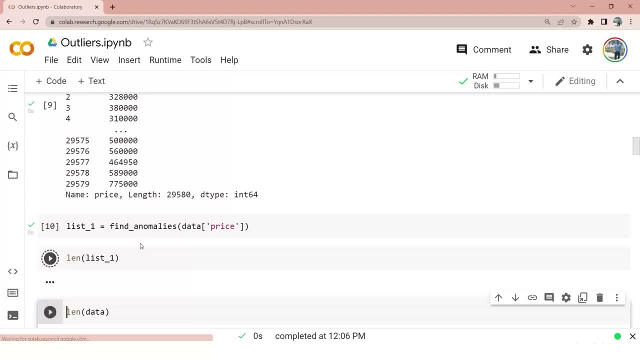 data pepper need to log into data. gss data border on you in this data block. it is successful. so in the anomalies this particular data point will be upended and if i run this, you can see there are 461 outliers. what is the total length of data? 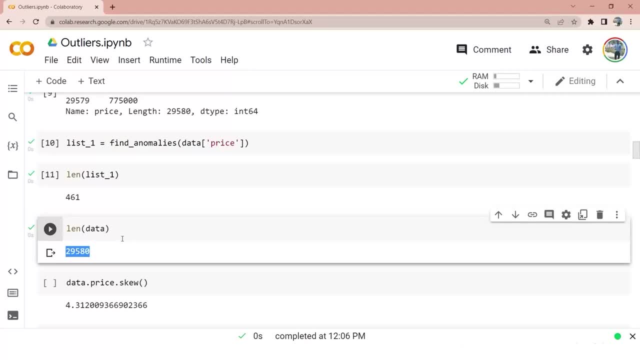 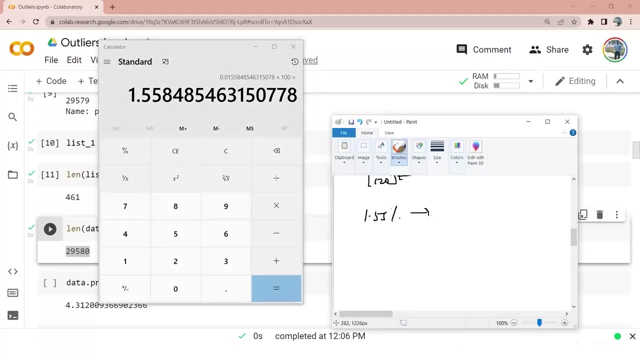 it is 29580. now if you start calculating 461 divided by 29580 into 100, which is almost 1.55 percent. 1.55 percent of the data are beyond the range of plus minus 3 sigma and we know that in in the case the data is fully normally distributed, it has to be 0.3 percent data. 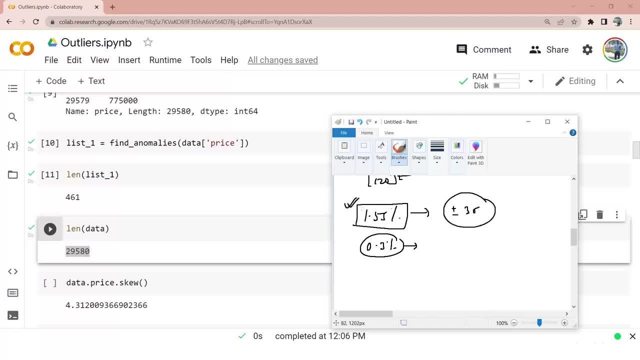 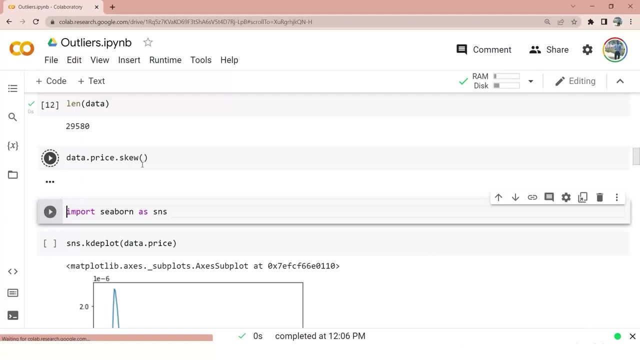 so this clearly means that the data is not normally distributed. so that's why i'm going to use some skewness function or kurtosis function to calculate the length of data, to see whether the data is skewed or not. so you can see, my skew value is 4.31, which clearly means 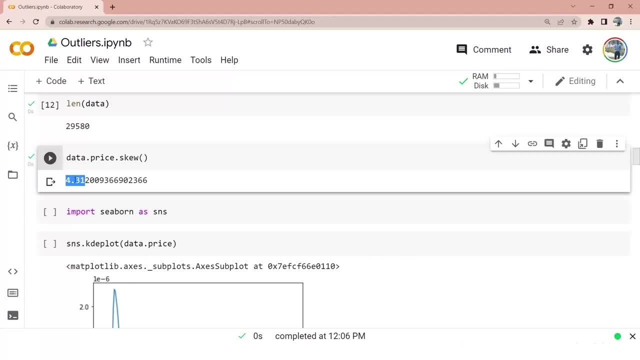 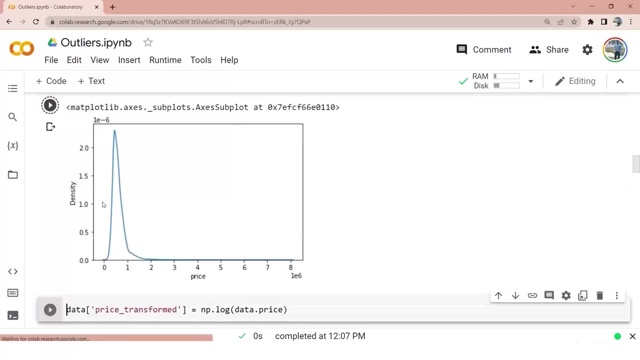 that the data is rightly. the data is positively skewed and if you want to plot your data for that, i have imported the seaborn library. i'm plotting the kde plot and you can see it is quite evident that it is skewed right. your normal distribution is like this: 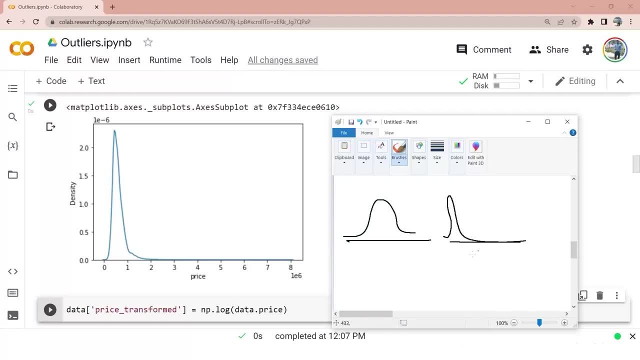 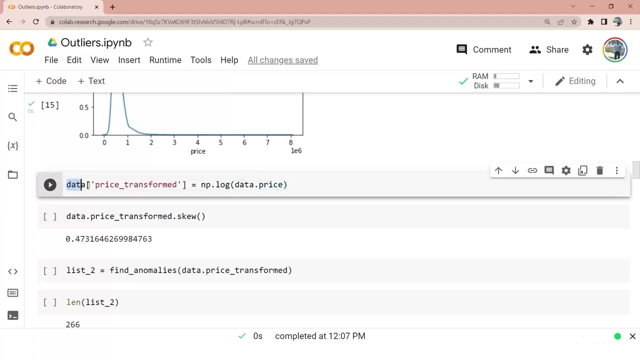 but in this case it is like this. it is something like this which clearly means it is not normally distributed. now let's say i want to do some transformation, so i have converted the data into a logarithmic scale. once i do this, i again run the skewness score. it is somehow closer to zero, not exactly the same. 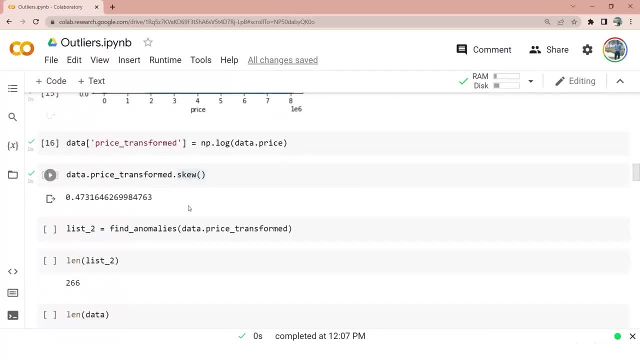 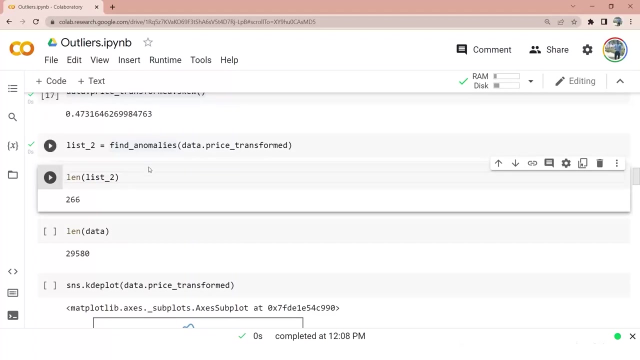 exactly zero, but at least less than the previous skewness value, which means the newly transformed data is somehow in a better shape as compared to the original data. now, if i run again the anomalies for the newly created data, you will see that the total number of failures are, or the outliers are, 266. 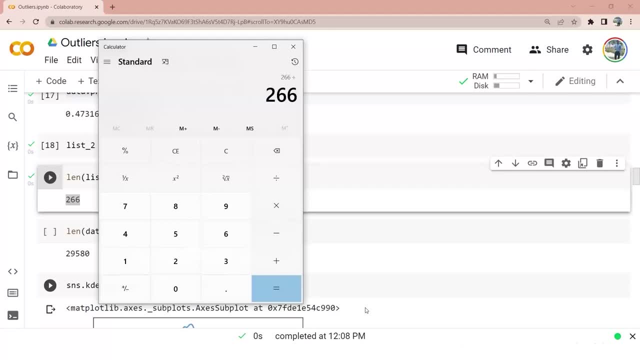 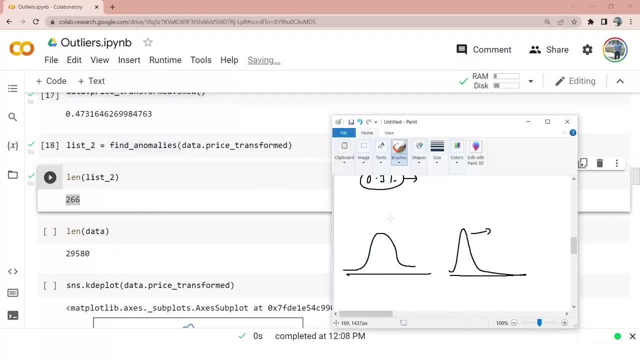 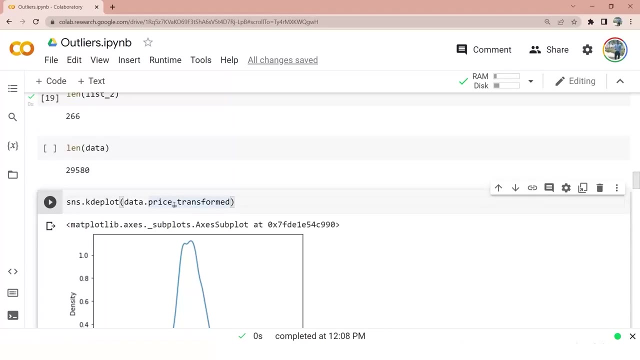 now what is the percentage? 266 divided by 295? 266 divided by 295, 80 into 100 is 0.9 percent. better, 0.9 percent. so coming closer towards the normal distribution graph. and if you plot the transform data and you can see, the transform data looks like this: 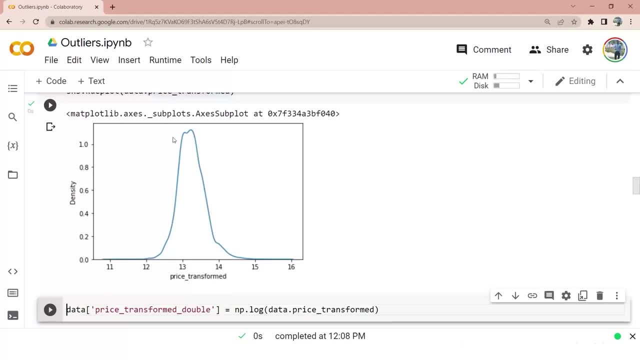 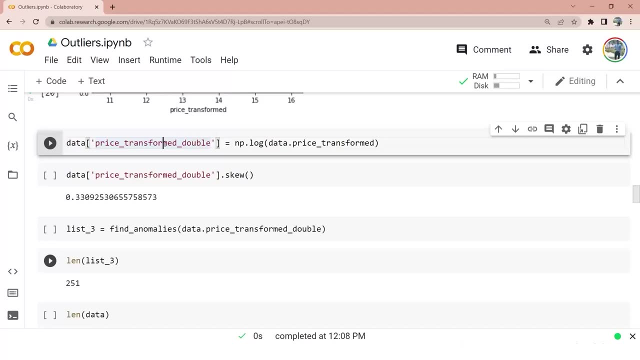 and it pretty much is not normally distributed, but somehow it looks closer to it again. let's say, i want to do a double transformation. i'm going to do a double logarithmic transformation by again converting the transform data into numpylog, and now my skewness score is even less. 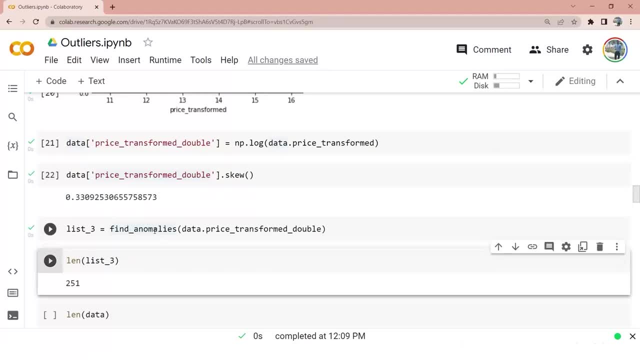 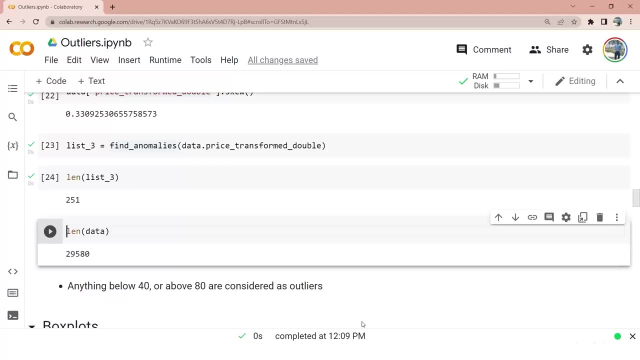 0.33. i will again run anomalies, find anomalies on this newly transformed data and you can see 251 records. now what is the percentage? 251 divided by 295, 80 into 100? almost 0.8 percent. so again, further reduction in the data and it is somewhat closer to normal distribution. 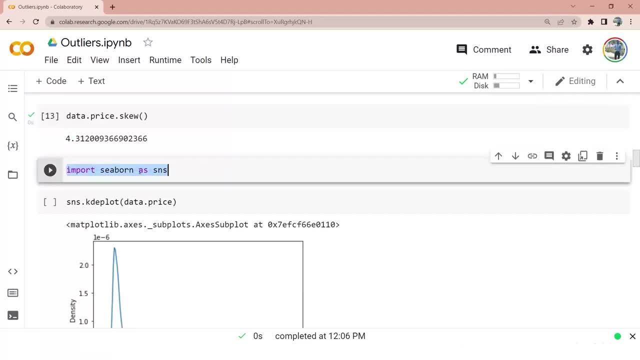 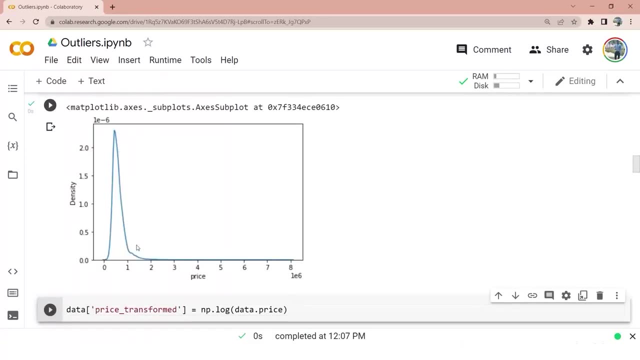 positively skewed and if you want to plot your data for that i have imported the seaborn library. i'm plotting the kd plot and you can see it is quite evident that it is skewed right. your normal distribution is like this, but in this case it is like this. it is something like this which clearly 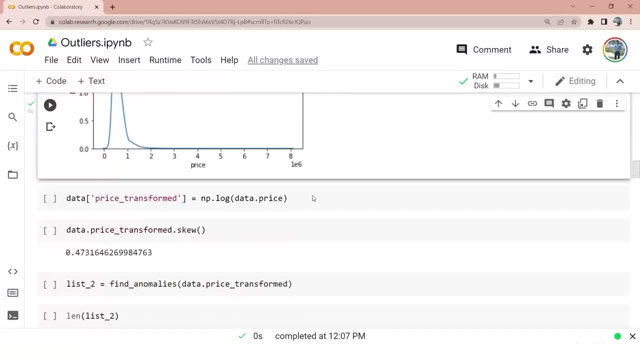 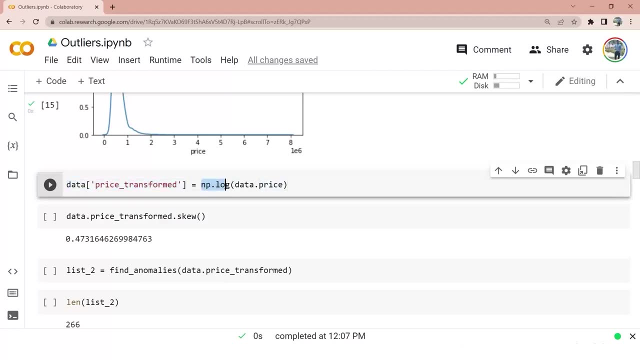 means it is not normally distributed. it is something like this which clearly means it is not normally distributed. now let's say i want to do some transformation, so i have converted the data into a logarithmic scale. once i do this, i again run the skewness score. it is somehow closer to zero. 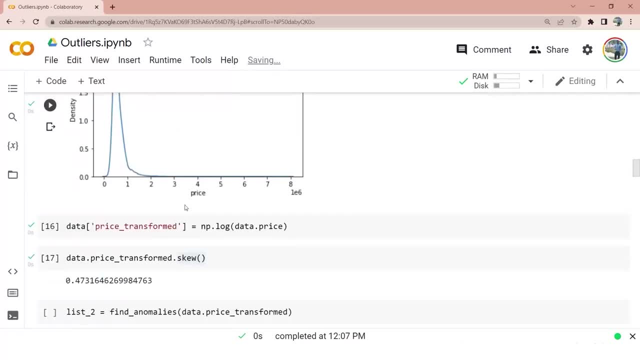 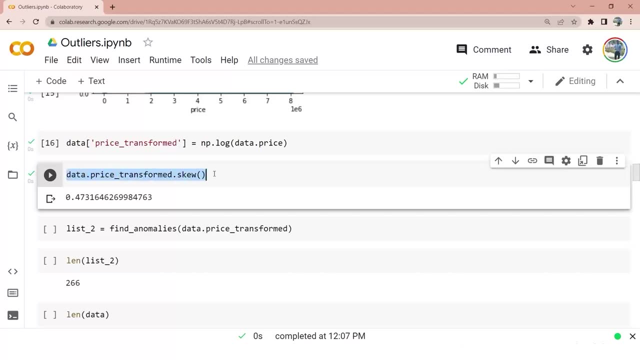 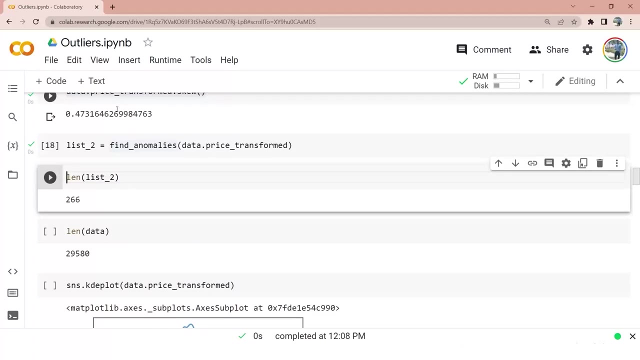 not exactly zero, but at least less than the previous skewness value, which means the newly transformed data is somehow in a better shape as compared to the original data. now, if i run again the anomalies for the newly created data, you will see that the total number of failures are, or the outliers are, 266. now what is the percentage? 266 divided by 29580 into 100. 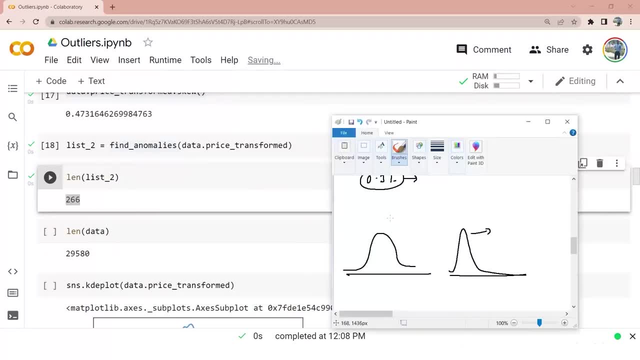 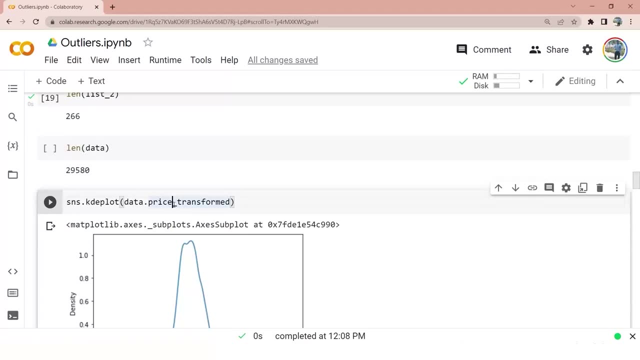 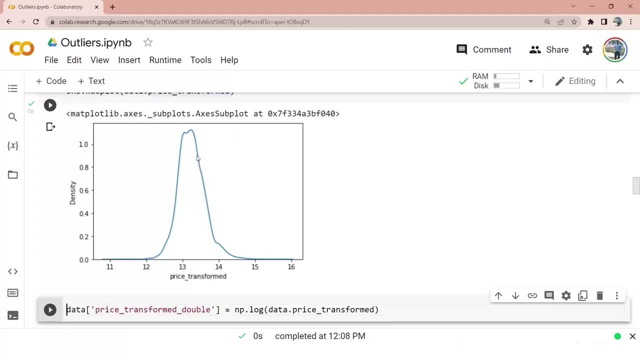 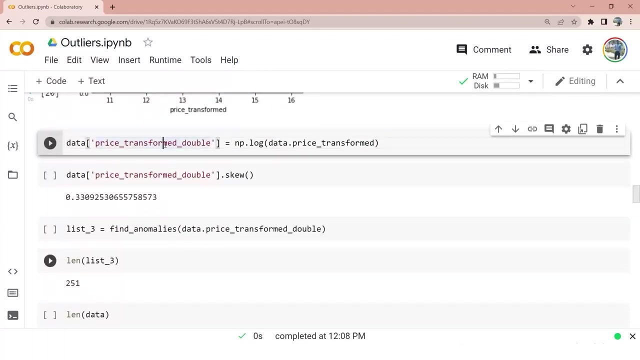 is 0.9 percent better, 0.9. so coming closer towards the normal distribution graph. and if you plot the transform data, you can see the transform data looks like this and it pretty much is not normally distributed, but somehow it looks closer to it again. let's say i want to do a double transformation, i'm 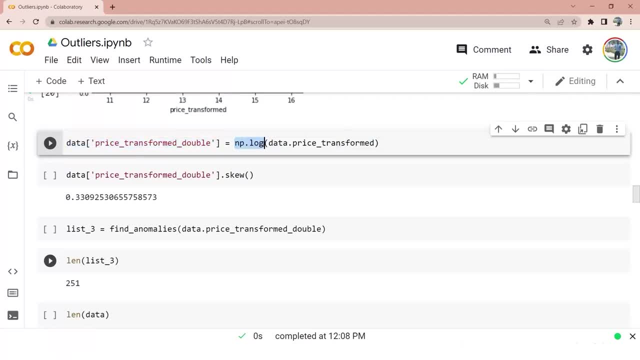 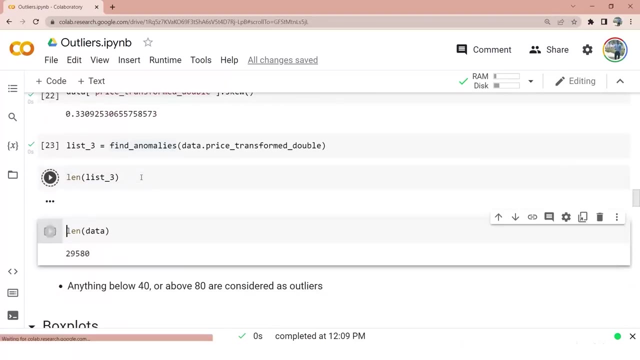 going to do a double logarithmic transformation by again converting the transformed data into numpylog, and now my skewness score is even less 0.33. i will again run anomalies, find anomalies on newly transformed data and you can see 251 records. now what is the percentage? 251 divided by 295? 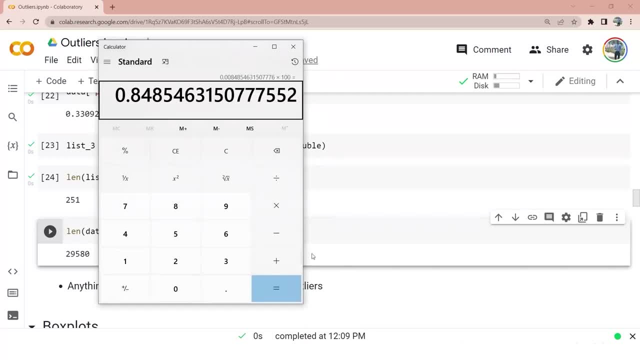 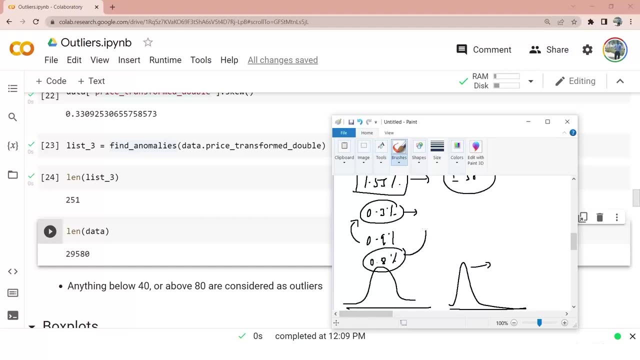 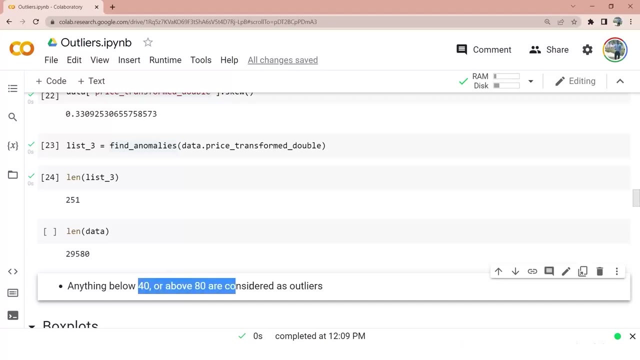 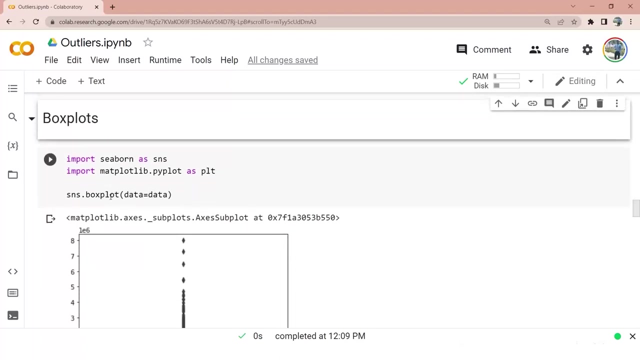 80 and 200, almost 0.8 percent. so again, further reduction in the data, and it is somewhat closer to normal distribution. so anything below 40 or above 80 are considered as outliers somehow. the second technique is going to be box plots. now, box plot is a visual way of understanding the data. 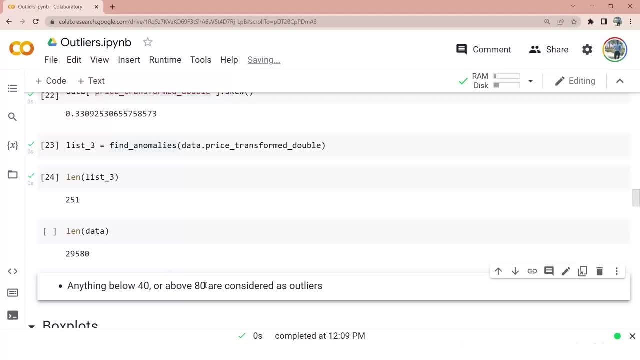 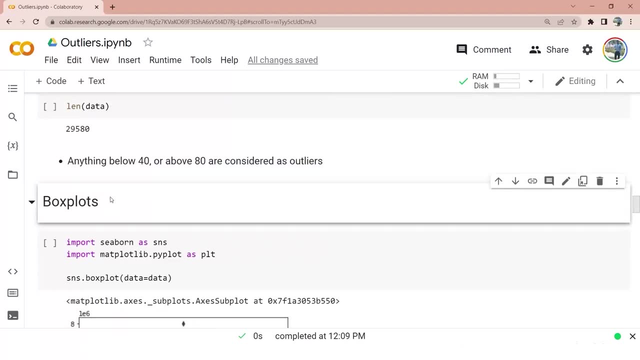 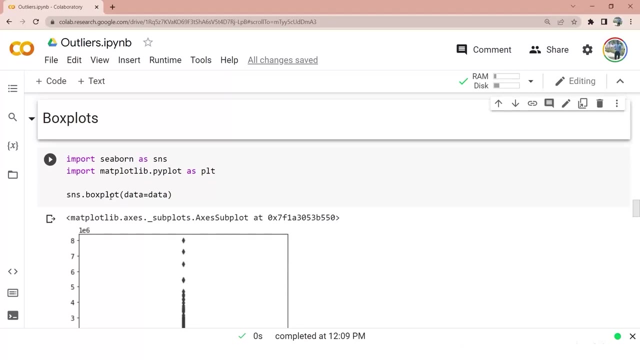 so anything below 40 or above 80 are considered as outliers somehow. the second technique is going to be box plots. now, box plot is a visual way of understanding the data. it's a visual way of identifying the outliers, similar to box plot. you can also use uh scatter plots, you can also do histograms, but again, box plots are better as. 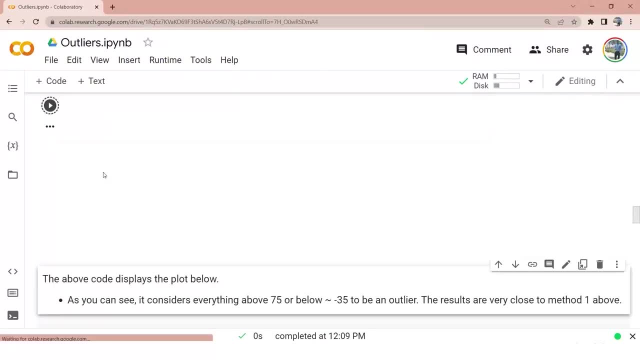 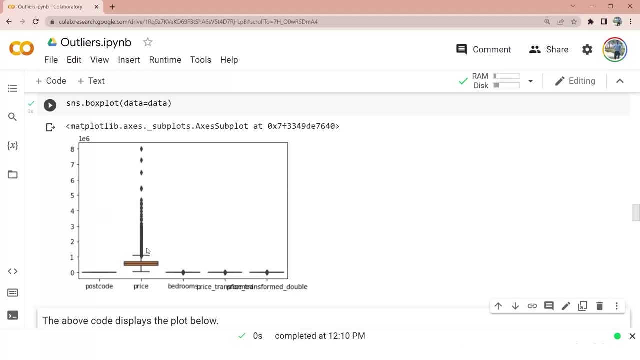 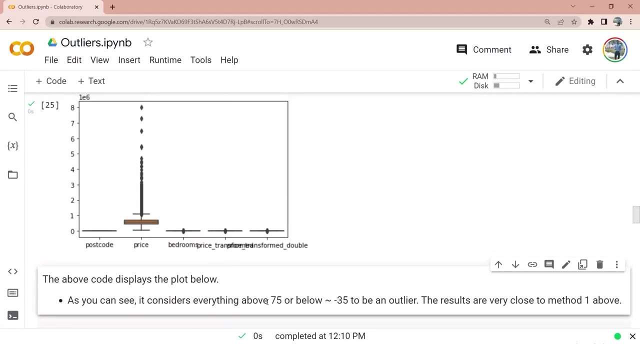 compared to other type of visual analytics. so here i'm importing the seaborn library and my matplotlib library. i'm just plotting the data for all the columns and you can see for price. i can see a lot of outliers. as you can see, it considers everything above 75. 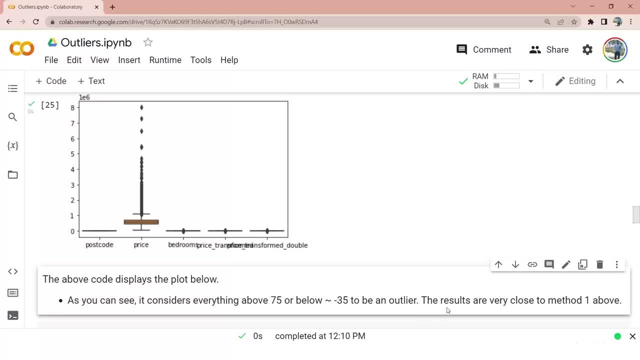 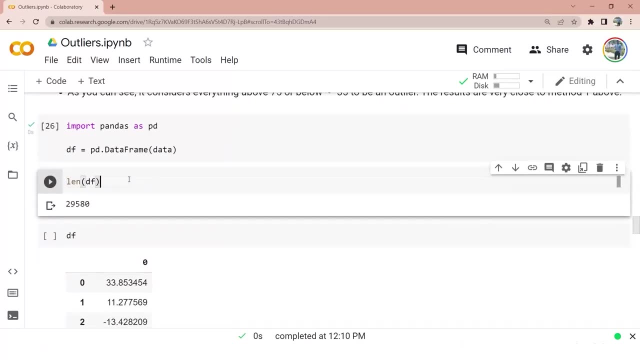 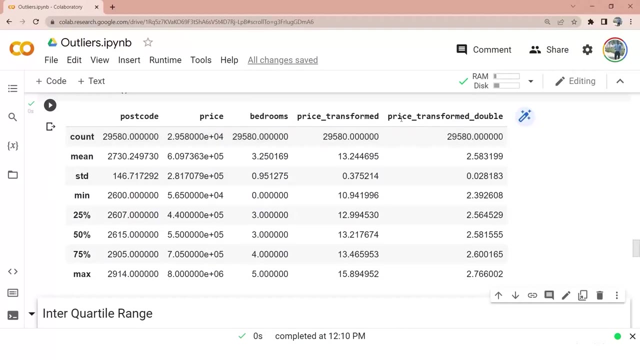 and below 35 to be an outlier. the results are very close to method one above. so that's how my data frame looks like and i am just going to do the describe method. for the price transformed and the double transformed. you can see that the third quartile is almost 2.6. 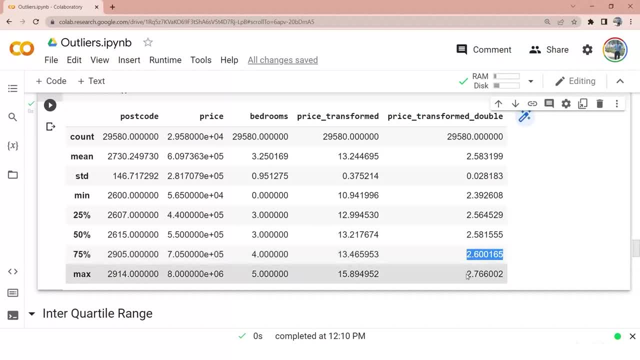 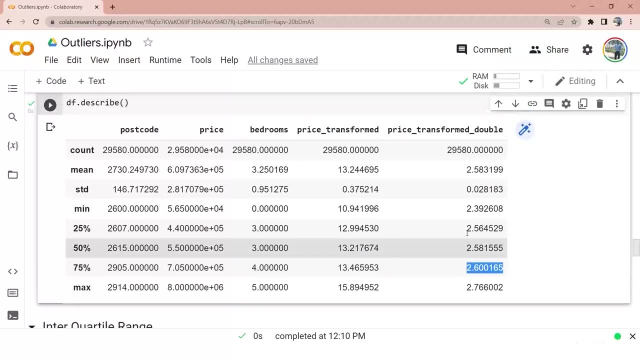 the next term is separate. Москвan mówi. the maximum is almost 2.75. so there are pretty much good amount of outliers here. but you know, i'm just visualizing it and i'm able to spot that there are some outliers in the 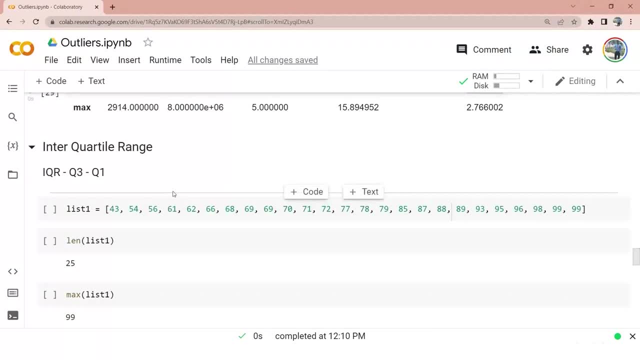 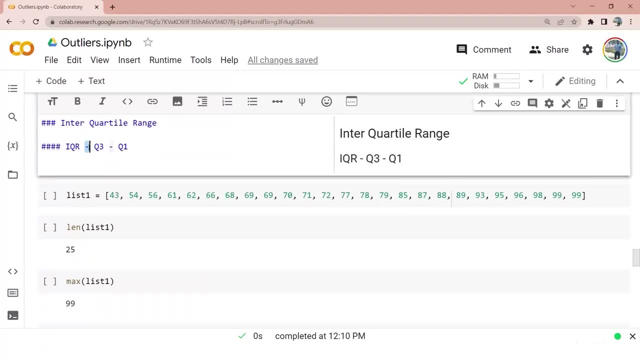 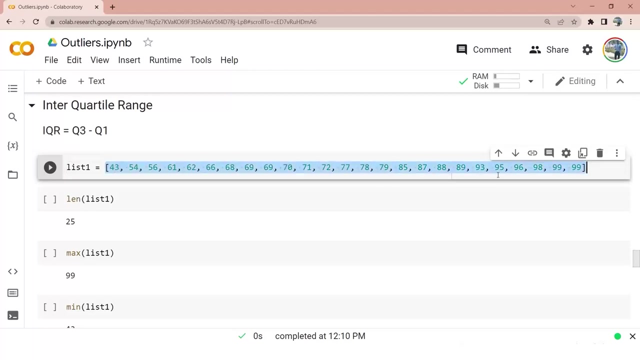 box plots interquartile range. interquartile range, basically, is nothing but q3 minus q1. so q3 is your third quartile and q1 is your first quartile. in this example you can see it's a list of multiple numbers. the length of this list is 25. the maximum of this list is 99. okay, which is. 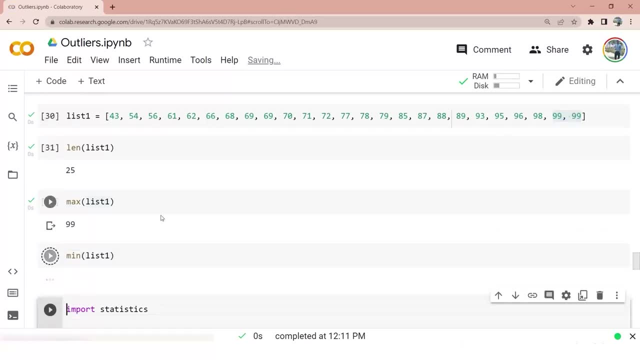 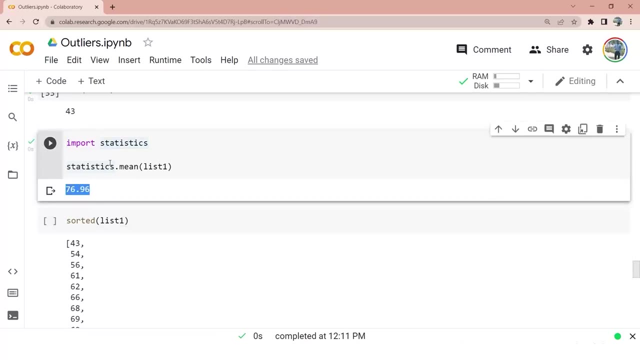 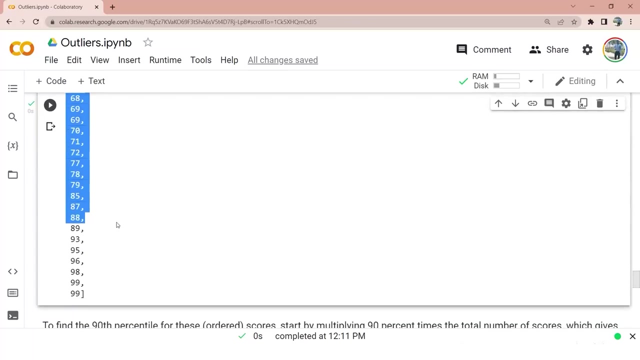 two values. i think yeah, there are two values and the minimum is 43. so using the statistics mean i am getting. the mean value is 76.96. okay, if you sort the list- that's how my list looks like in a sorted manner to find the 90th- 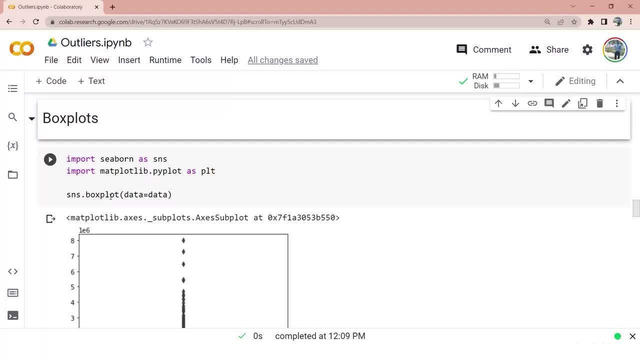 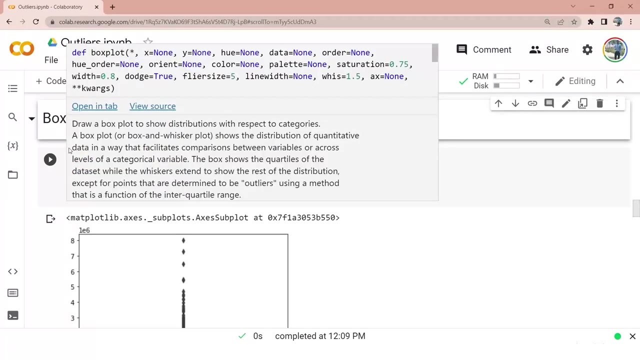 it's a visual way of identifying the outliers, similar to box plots. you can also use scatter plots, you can also do histograms, but again, box plots are better as compared to other type of visual analytics. so here i'm importing the seaborn like data and i'm going to use the seaborn like data, and i'm going to use the seaborn like data. 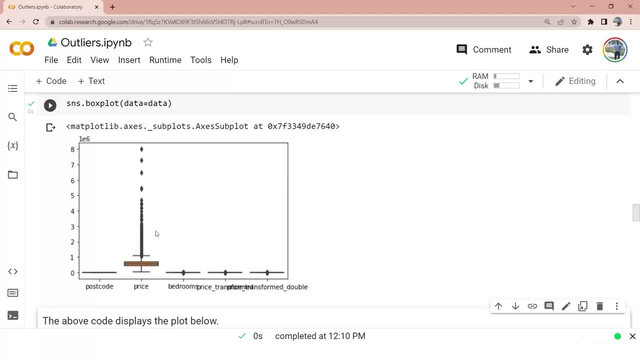 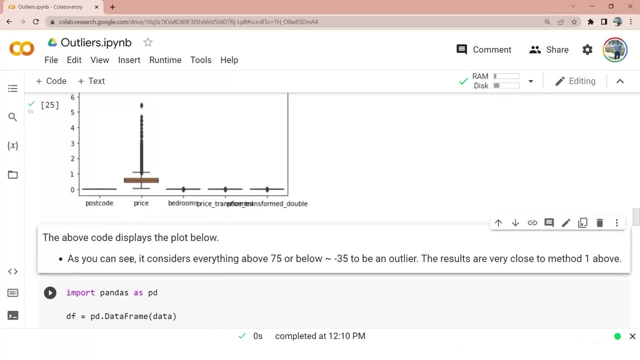 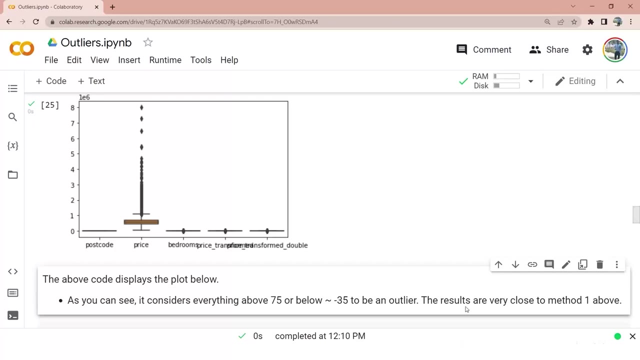 library and my matplotlib library. i'm just plotting the data for all the columns and you can see for price i can see a lot of outliers. as you can see, it considers everything above 75 or below 35 to be an outlier. the results are very close to method one above. 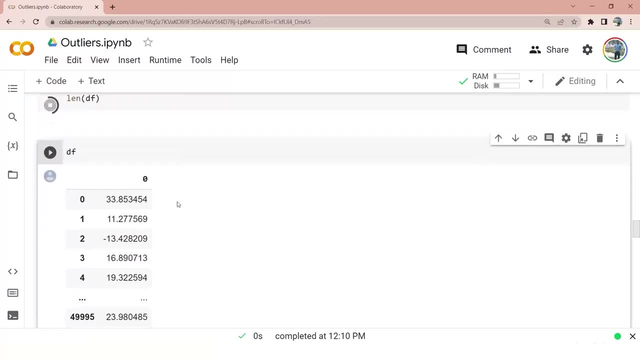 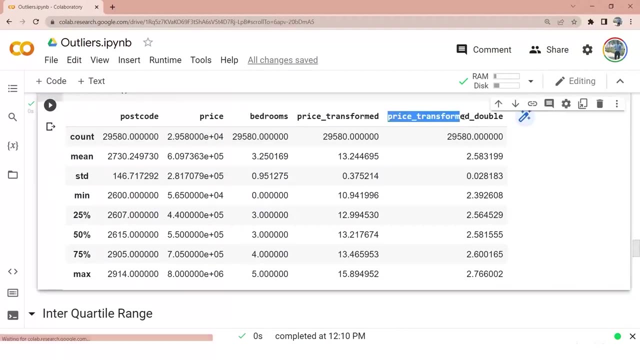 so that's how my data frame looks like and i'm just going to do the describe method. for the price transformed and the double transformed, you can see that the third quartile is almost 2.6. the maximum is almost 2.75. so there are pretty much good. 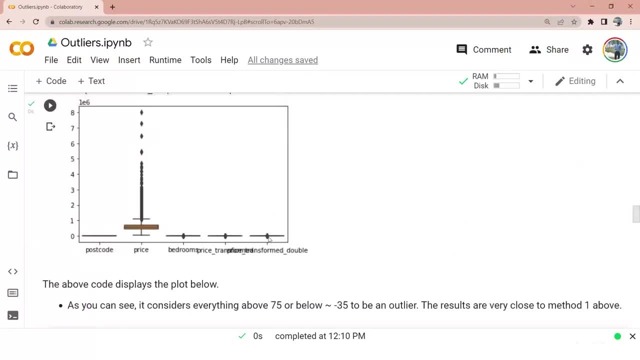 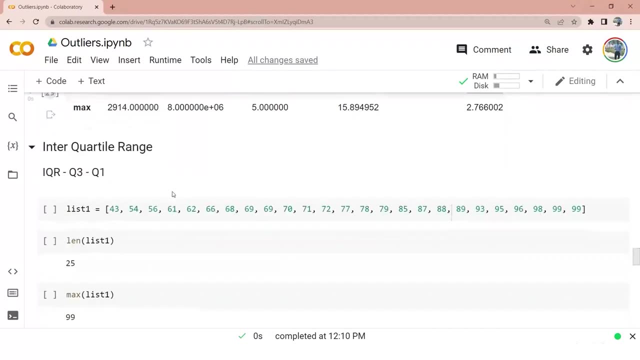 amount of outliers here. but you know, i'm just visualizing it and i'm able to spot that there are some outliers in the box plots. so let's get started. we're going to use the same equation for the first quartile. we're going to be using the paper wise. 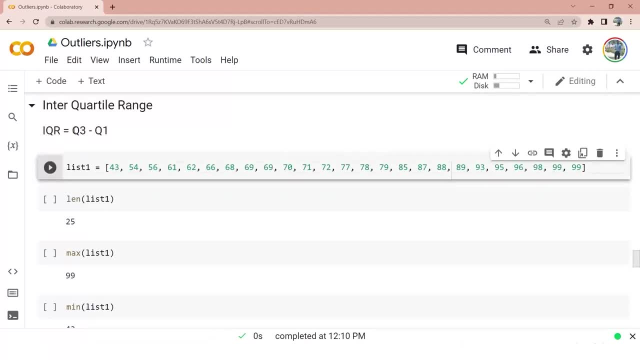 which is nothing but the bar's range, which is nothing but the bar's range, u3 minus q1. so q3 is your third quartile and q1 is your first quartile. in this example you can see it's a list of multiple numbers. the length of this list is 25. 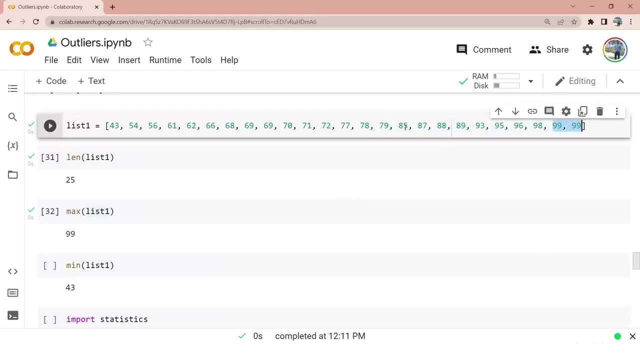 the maximum of this list is 99, okay, which is two values. i think, yeah, there are two values and the minimum is 21.13. so once we have a number in order to use it, then we just do a whole array of the numbers in the chart to come up with a total of 99 values. 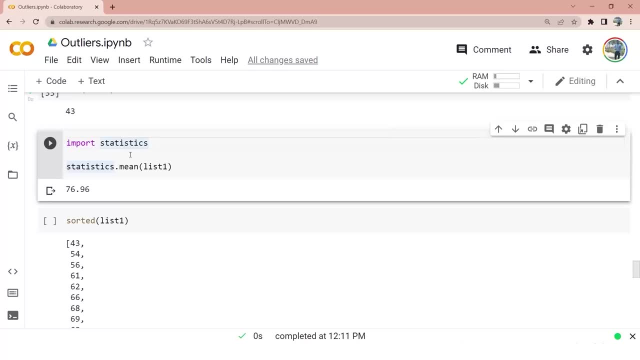 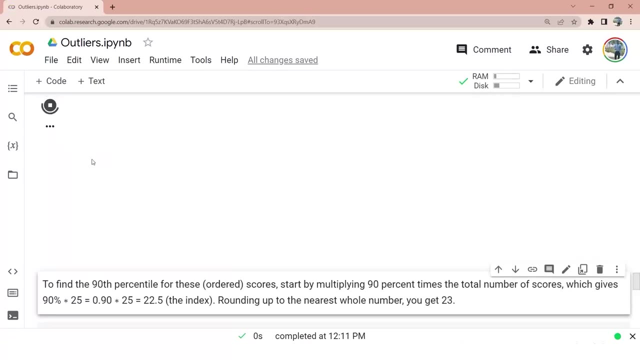 is 43, so using the statistics mean i am getting. the mean value is 76.96. okay, if you sort the list, that's how my list looks like in a sorted manner. to find the 90th percentile for these data, the ordered scores start by multiplying 90 percent times the total number of scores, which gives 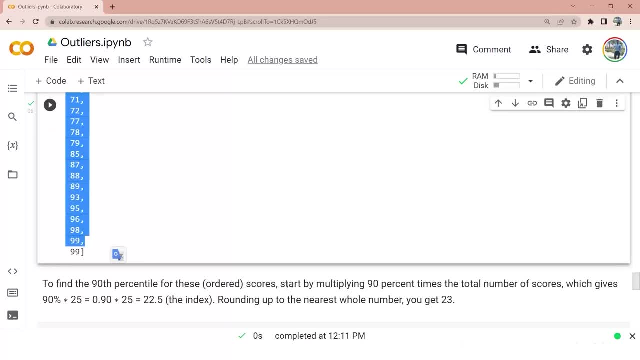 percentile for these data, the ordered scores start by multiplying 90 times the total number of scores, which gives 90 percent into. multiplied with 25, which is 0.9, into 25, which is 22.5, the index, if you round up the index. 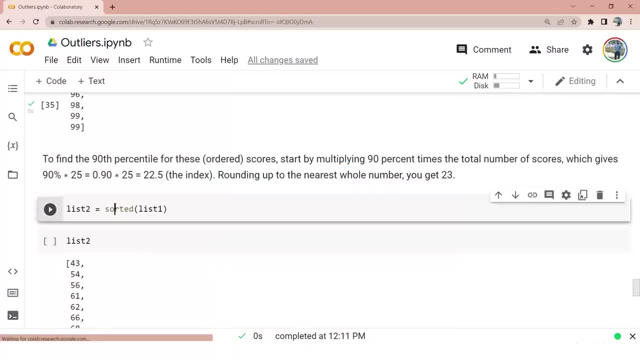 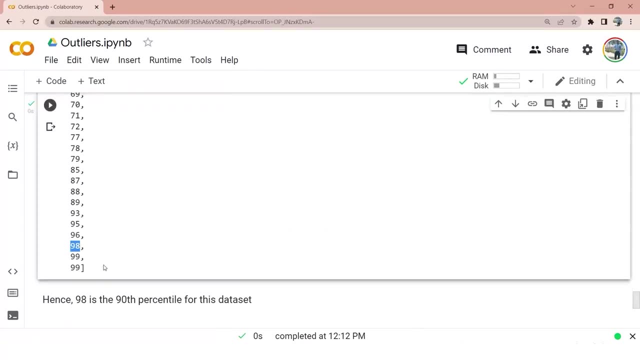 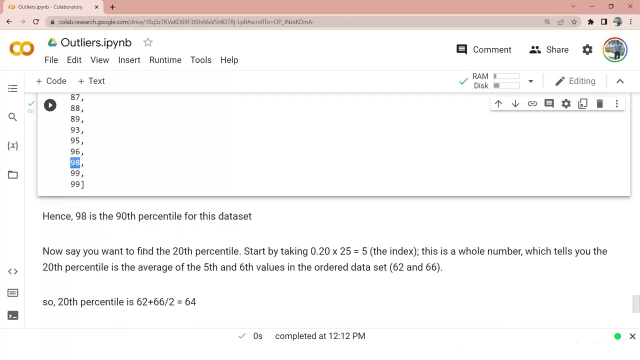 it is 23. so what is my 23rd element, hence 98, which is? this 23rd element is the 90th percentile for this data set. now say you want to find the 20th percentile. start by taking 0.2 into 25. so there are 25 elements. 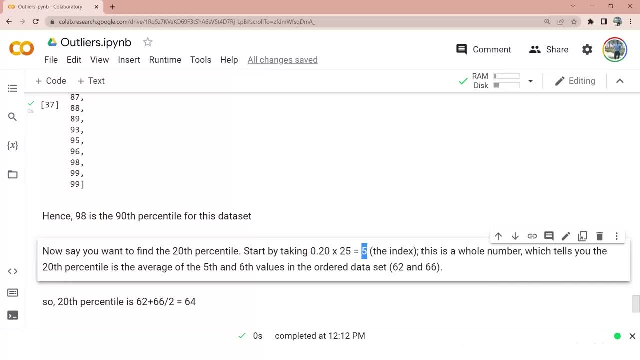 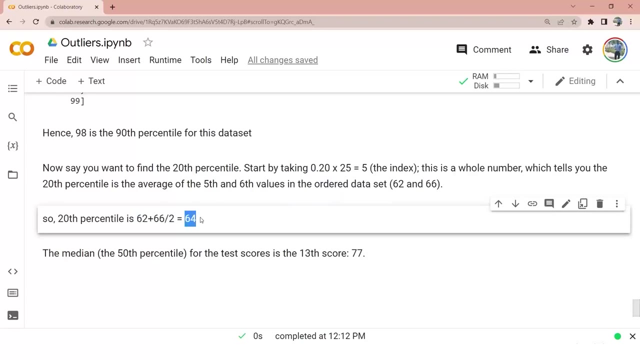 so i will do 0.2 into 25, which is 5. the index. this is a whole number which tells you the 20th percentile is the average of the fifth and sixth values in the other data set. so 20th percentile is 62 plus 66 by 2, which is 64, the median, the 50th percentile. 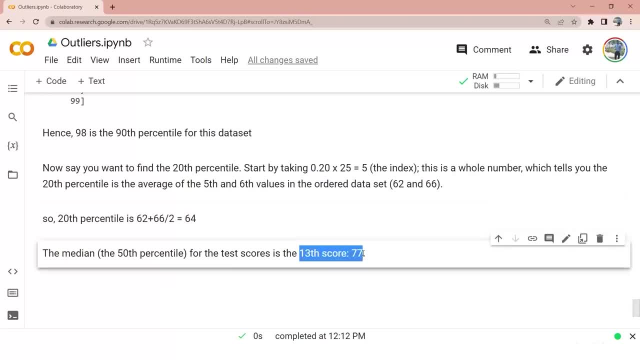 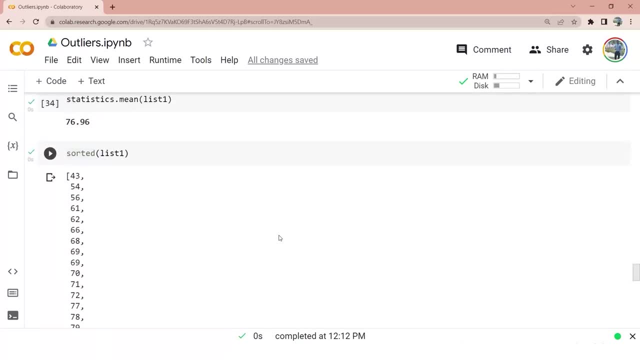 for the test score is the 13th score, which is 77.. so these are some different techniques to identify outliers, starts and organization de and scient Pepper LImp Map and looking for using well doing and모 spending costs fine plants sets. 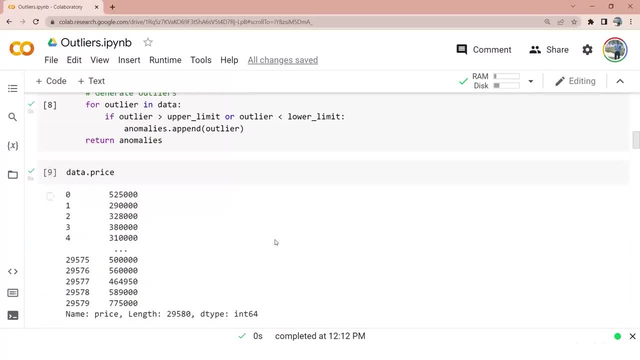 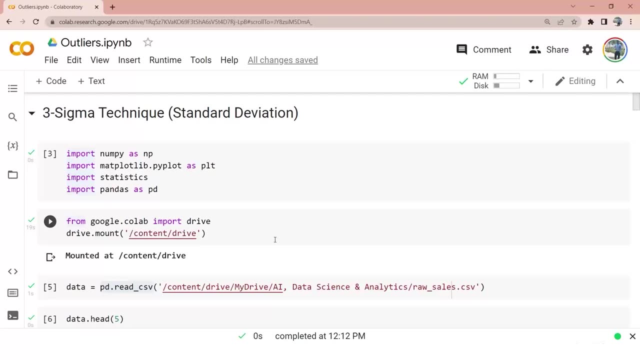 standard deviation technique, which is the most important technique, because that's one of those techniques that is most reliable. we usually go for the six, three sigma technique to identify outliers. apart from these, there are multiple other outlier algorithms, outlier detection algorithms, which we will go through in the predictive analytics part, where we will talk about. 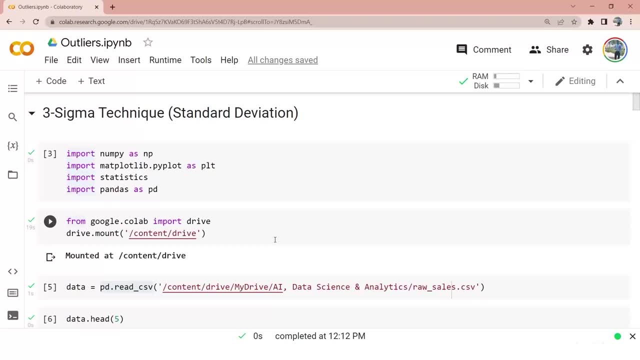 luminol algorithm, which is a outlier algorithm specially created for outliers. we'll try to go through that, but for the time being, i hope you had an understanding on how to identify outliers using the python code. that's all about this particular video. see you in the next video, till. 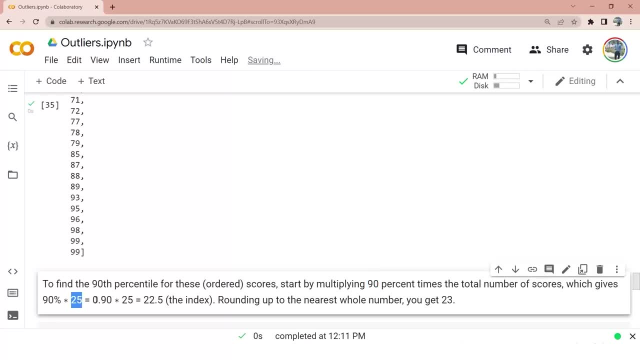 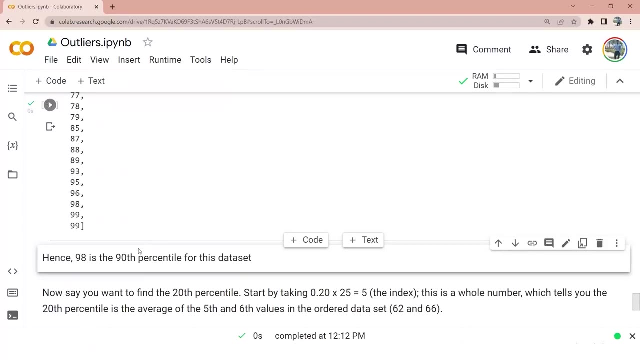 90 percent into, multiplied with 25, which is 0.9, into 25, which is 22.5, the index: if you round up the index, it is 23. so what is my 23rd element, hence 98, which is this 23rd element is the 90th percentile for this data set. 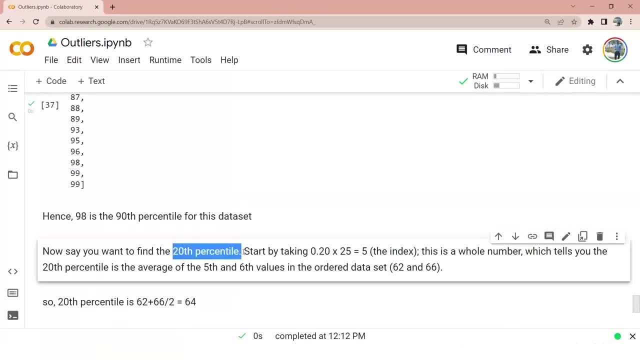 now say you want to find the 20th percentile, start by taking 0.2 into 25. so there are 25 elements. so i will do 0.2 into 25, which is 5, the index. this is a whole number which tells you the 20th percentile. 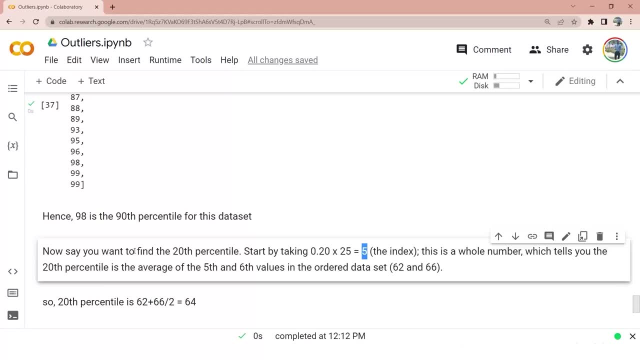 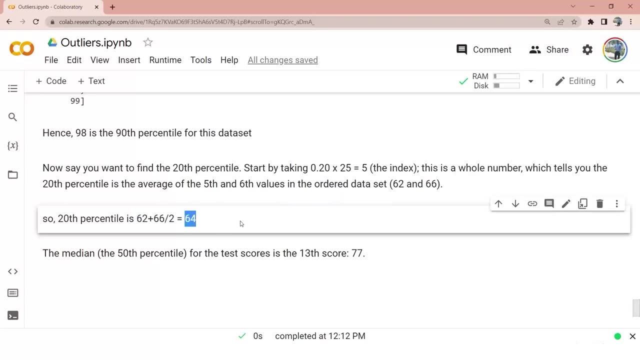 is the average of the fifth and sixth values in the order data set. so 20th percentile is 62 plus 66 by 2, which is 64.. the median, the 50th percentile for the test score, which is 74, and the median the 50th percentile for the test score, which is 77.. 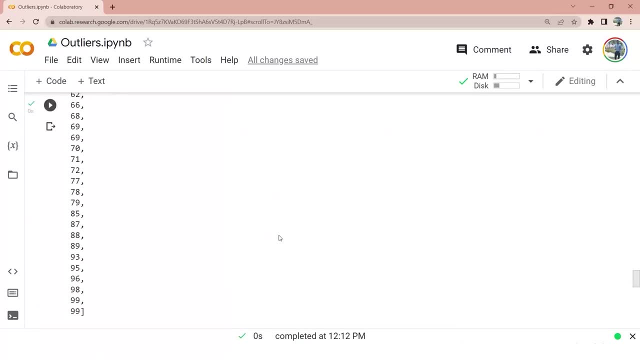 so these are some different techniques to identify outliers, starting with the standard deviation technique, which is the most important technique, because that's one of those techniques that is most reliable. we usually go for the six- 3 sigma technique to identify outliers. apart from these, there are multiple other outlier algorithms, outlier detection algorithms, that are available. 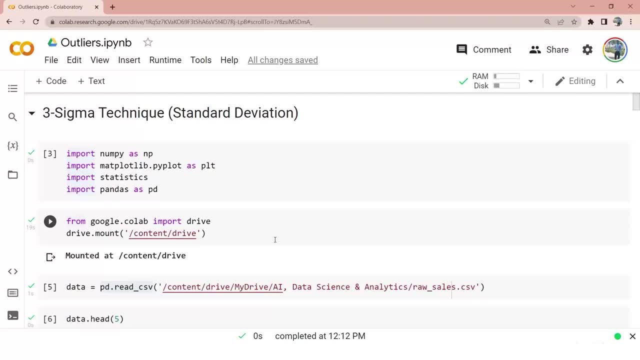 which we will go through in the predictive analytics part, where we will talk about luminal algorithm, which is a outlier algorithm specially created for outliers. we'll try to go through that, but for the time being, i hope you had an understanding on how to identify outliers using the python code. that's all about this particular video. see you in the next video. 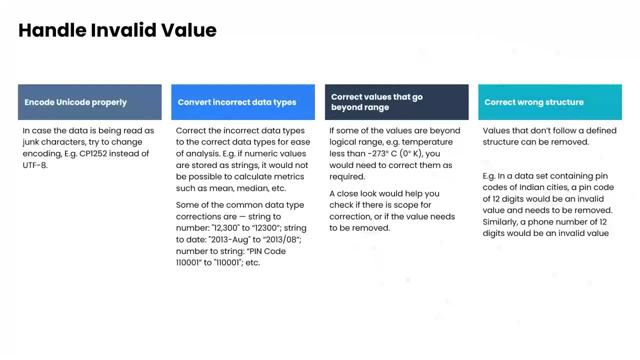 the next type of issue that we are going to talk about when it comes to the data cleaning part is handling invalid values. now, while dealing with data, there could be multiple scenarios where you would get some invalid values. for example, you are dealing with a column, a date column, and you are 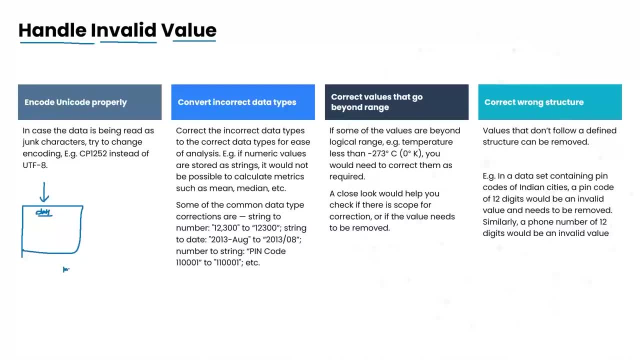 expecting it to be in a certain format, maybe mm yyyy format, and you are expecting it to be in a certain format. and you are expecting it to be in a certain format. and you are expecting it to be in a format, but it is in a different format. or it is in text, or it is in something else, or it is an epoch. 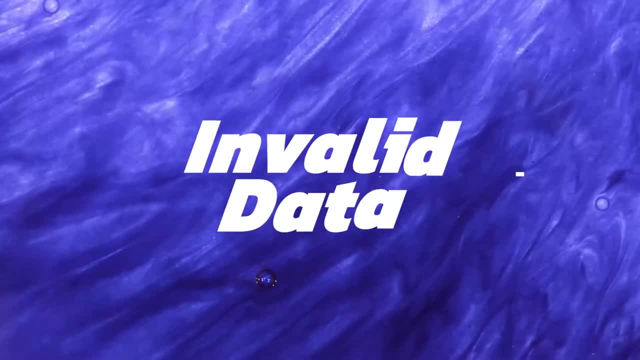 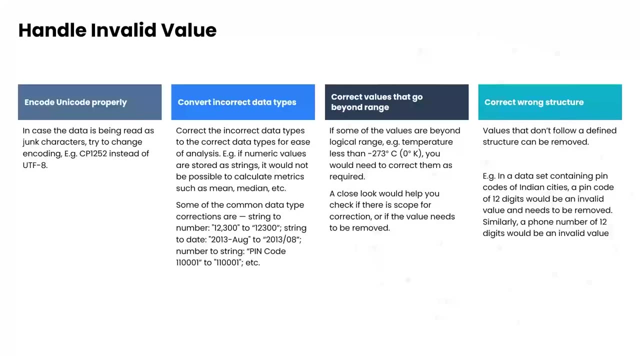 then bye. the next type of issue that we are going to talk about when it comes to the data cleaning part is handling invalid values. now, while dealing with data, there could be multiple scenarios where you would get some invalid values. for example, you are dealing with a column, a date column, and you are expecting it to be in a certain format. maybe mm. 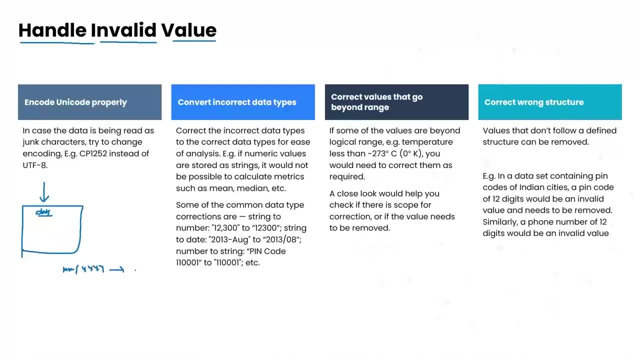 yyy format, but it is in a different format. or it is in text, or it is in some thing else, or it is an epoch, epoch date, something like that, or else you are expecting one of the columns and one of these columns are having a lot of special characters. there could be column where 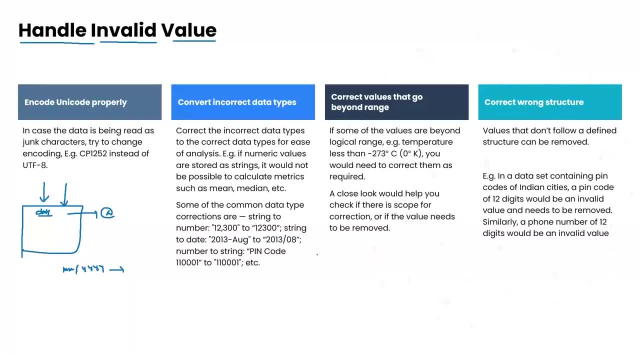 it is not having logical values. for example, a logical value of a person's age could be between 0 to 100. what if somebody has minus 20.. now, that could be an issue, while the data collection part there could be a data collection issue because of which you are having minus 20 or minus 40 if you. 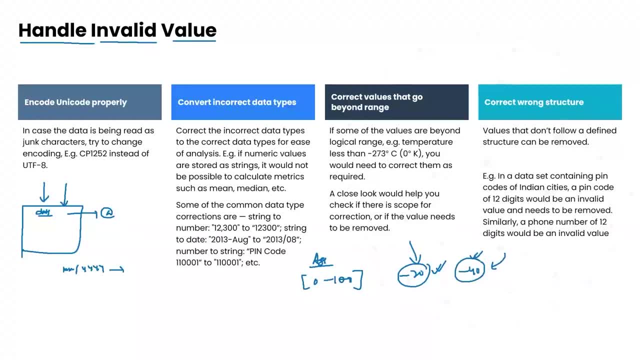 see such scenarios. you have to deal with it. you have to ignore them or treat it as a null value and deal with it. so there are multiple scenarios when it comes to invalid values. encode unicode properly in case the data is being read as junk characters. try to change encoding technique. 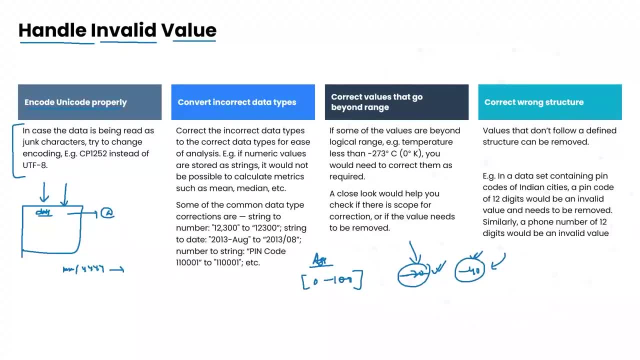 now. this is a common mistake that we usually face when it comes to encoding and decoding. sometimes, when we are reading the data set using pandasread csv, sometimes the data set itself is encoded in a different unicode technique, so you have to change the unicode technique so that 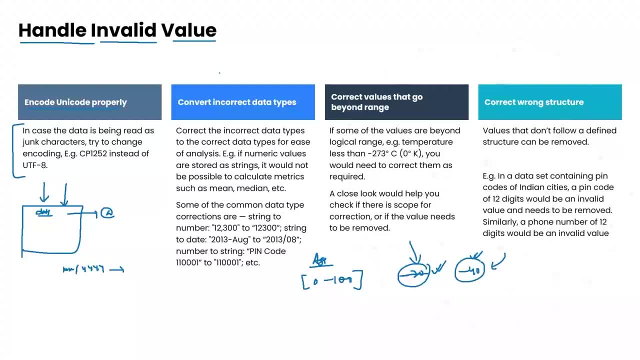 you are able to read the file, else it will throw you error unicode error. convert incorrect data types. correct the incorrect data types to the correct data types for ease of analysis. example: if numerical values are stored as strings, it would not be possible to calculate metrics such as mean. 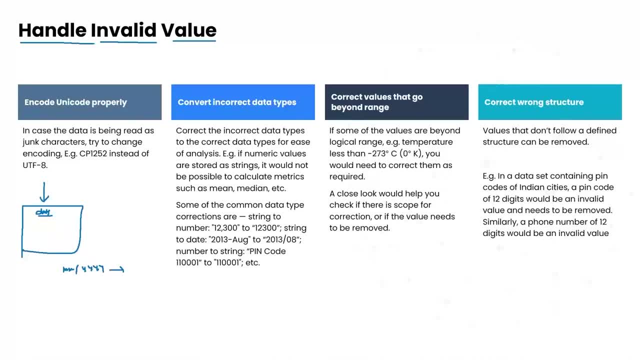 epoch date, something like that, or else you are expecting one of the columns and one of these columns are having a lot of special characters. there could be column where it is not having logical values. for example, a logical value of a person's age could be between 0 to 100. what if? 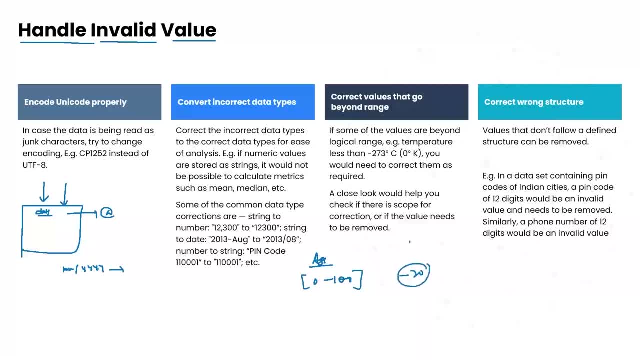 somebody has minus 20. now that could be an issue, while the data collection part- there could be a data collection issue because of which you are having minus 20 or minus 40. if you see such scenarios, you have to deal with it. you have to ignore them or treat it as a null value and deal. 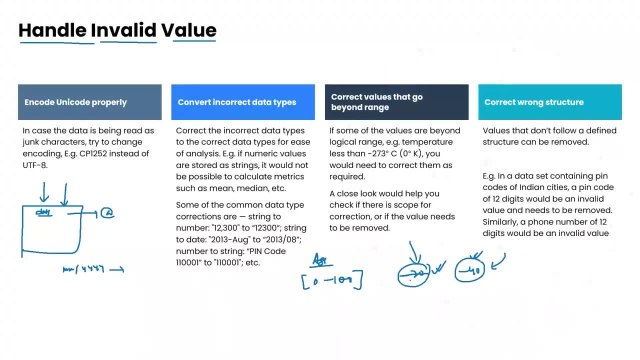 with it. so there are multiple scenarios when it comes to invalid values. encode unicode properly. encode unicode properly. encode unicode properly. in case the data collection is not going to be- the data is being read as junk characters- try to change encoding technique now. this is a common mistake that we usually face when it comes to encoding and decoding. sometimes, when we are 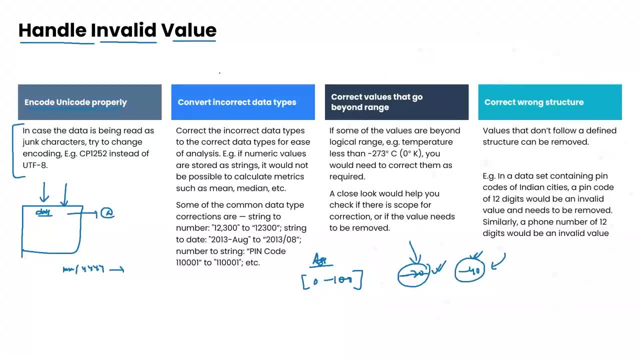 reading the data set using pandas dot read csv. sometimes the data set itself is encoded in a different unicode technique, so you have to change the unicode technique so that you are able to read the data, both the encoded and the unicode, necessary for this kind of data collection. 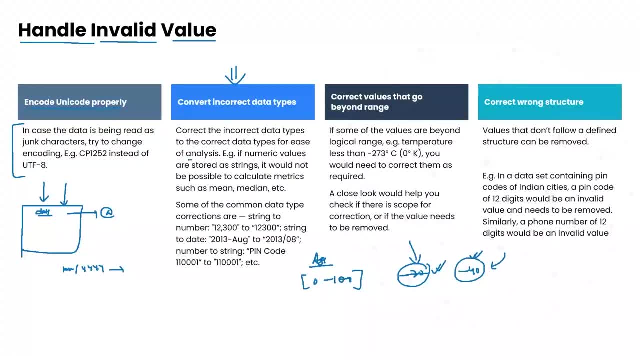 so if you are getting many types of data and sometimes it will throw you error, unicode error. convert incorrect data types. correct the incorrect data types to the correct data types for ease of analysis. example, if numerical values are stored as strings, it would not be possible to calculate. 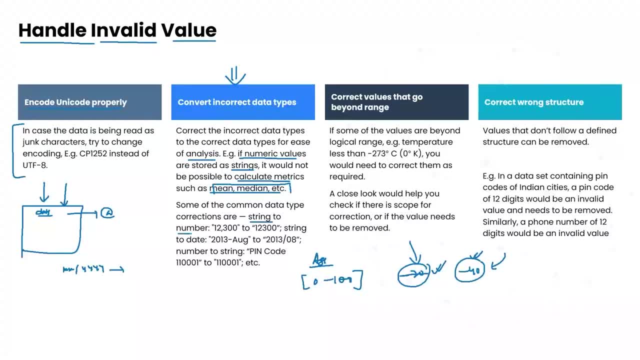 metrics such as mean media right- very common problem. sometimes our numerical values are also stored as strings. some of the common data type corrections are: string traverse in video number this to this: where you have a comma 12, 300, you want to convert it into a number. 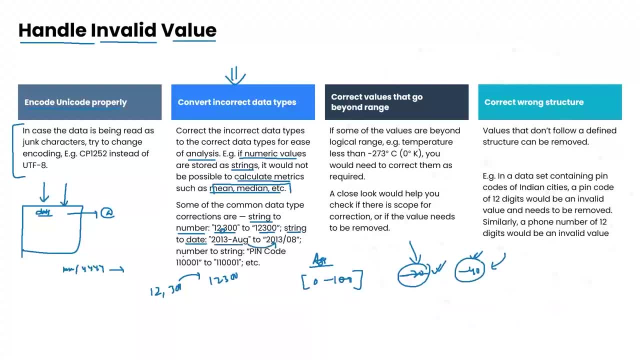 string to date this to this number, to string pin code this to this. so there could be multiple scenarios where your data is not in the expected data type format and you have to change it, correct the values that go beyond range, as i was talking about, in certain scenarios. 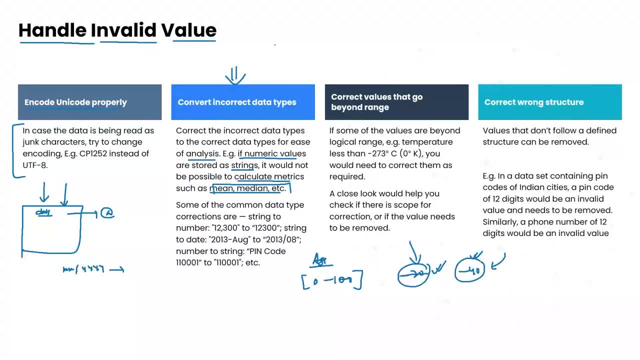 median right- very common problem. sometimes our numerical values are also stored as strings. some of the common data type corrections are: string to number. this to this. where you have a comma 12, 300, you want to convert it into a number. string to date this to this. 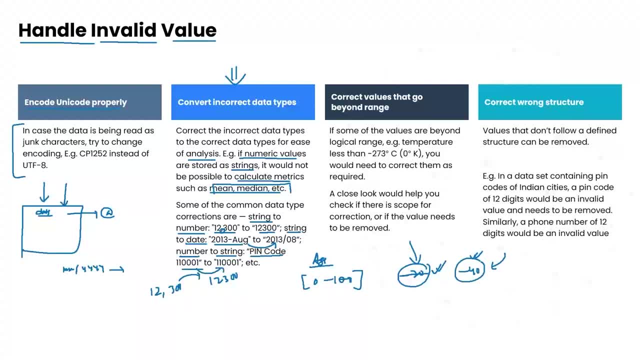 number to string. pin code this to this, so there could be multiple scenarios where your data is not in the expected data type format and you have to change it. correct the values that go beyond range, as i was talking about. in certain scenarios your values in that column could be some values that. 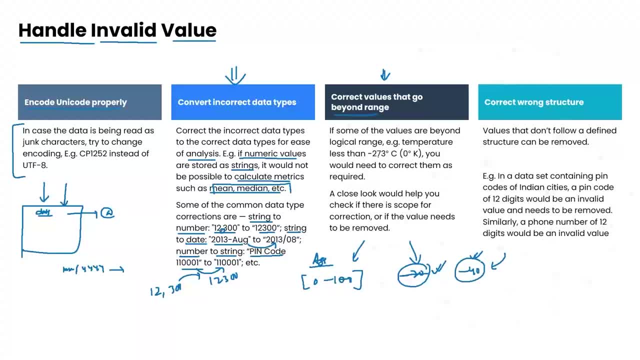 you would vai face to say your data type, and all over of the table will be in that structure. right now. just use a set setting. you can see that i am using code. you only have to apply frangibles to the set in strata list. you can do this till the end. and finally, you have to change theárioserducesseds to the set in strata list. all these, speaking in the particular order, happens only when the string and suby ł Frage- meaning in indian, for example- gives you it takes to get it, which makes no sense. for example, temperature less than. minus 273 degree celsius does not exist. but if you get it, what will you? right, you have to deal with it. correct the wrong structure. values that don't follow a defined structure can be removed. example: in a data set containing pincodes of indian cities, intrigued of twelve digits would be an invalid value, right? 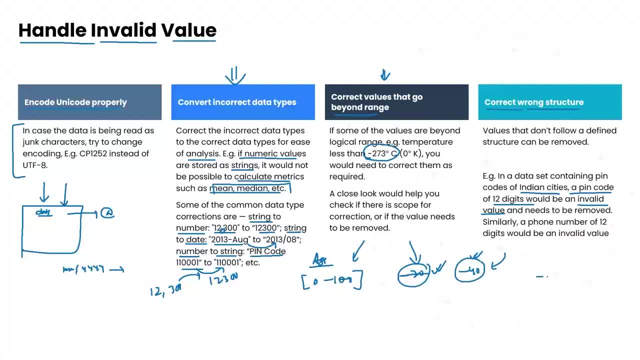 pin codes of Indian cities are always in the format of 6 digits, right? so if you are considering 12 digits, it could be an error. now, talking about Hong Kong, let's say Hong Kong does not have a pin code. what if you have a column called as pin? 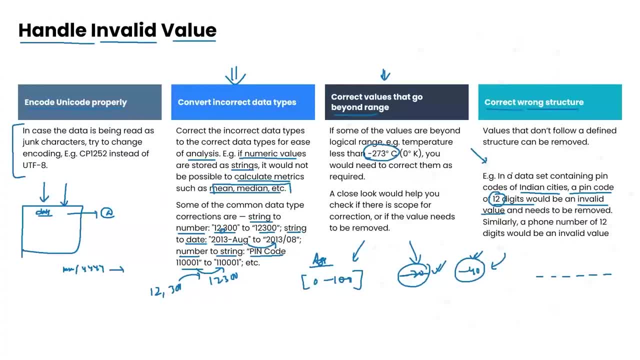 code with some random values, or else in Japan, or else in Malaysia, you have some car, we you have a concept of pin code, right? in that case, if your pin code is completely different, you are expecting 8 digits, but you are getting 12 or 15. 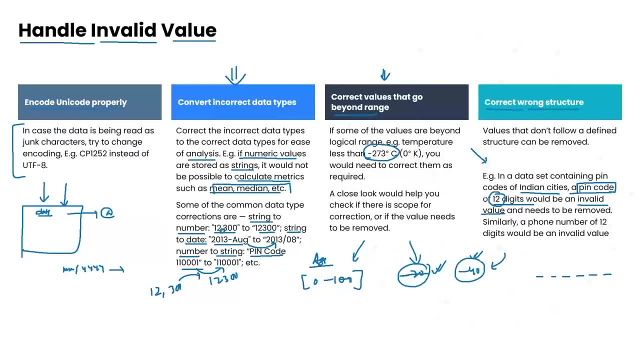 digits, which is completely wrong, right. so there are so many scenarios, so many instances where we have to deal with this. there is no practical applications like practical code for this particular slide so that I can help you out in different scenarios. but this is all about experience once you jump into the 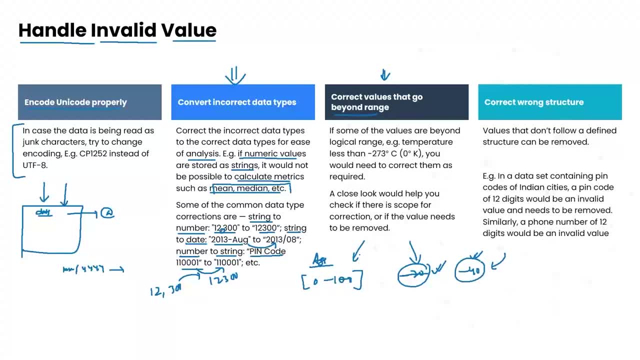 your values in that column could be some values, which makes no sense. for example, temperature less than minus 273 degrees celsius does not exist. but if you get it, what will you do? right, you have to deal with it. correct the wrong structure, values that don't follow a defined structure. 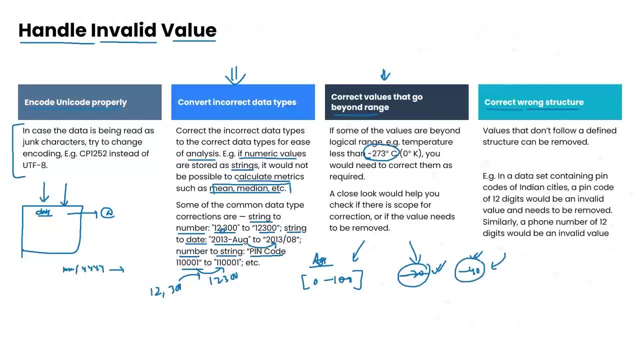 can be removed. example, in a data set containing pin codes of indian cities, a pin code of 12 digits would be an invalid value, right? pin codes of indian cities are always in the format of six digits, right? so if you are considering 12 digits, it could be an error now talking about. 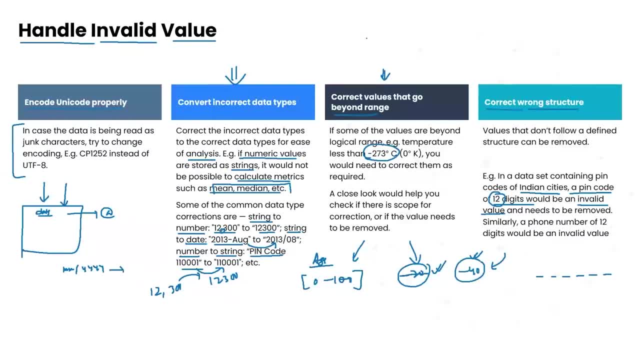 hong kong. let's say hong kong does not have a pin code. what if you have a column called as pin code, with some random number in it, random values, or else in japan, or else in malaysia you have some call, you have a concept of pin code. 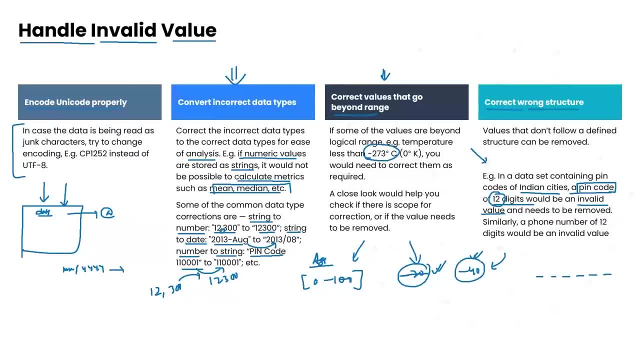 right. in that case, if your pin code is completely different, you are expecting eight digits, but you are getting 12 or 15 digits, which is completely wrong, right? so there are so many scenarios, so many instances where we have to deal with this. there is no practical. 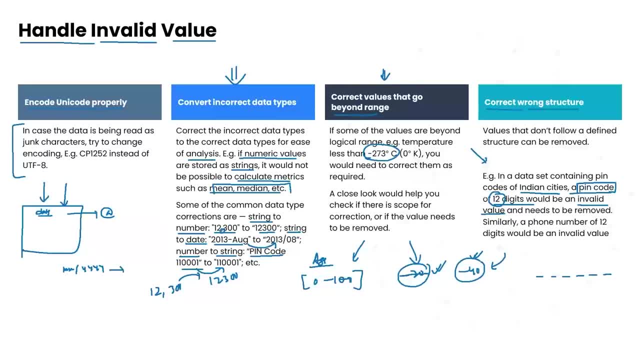 applications like practical code for this particular slide so that i can help you out in different scenarios. but this is all about experience. once you jump into the field of data analysis, once you start doing the ada part, you will come across so many scenarios where you have to deal with it and automatically will learn by experience. that's all about this particular video. 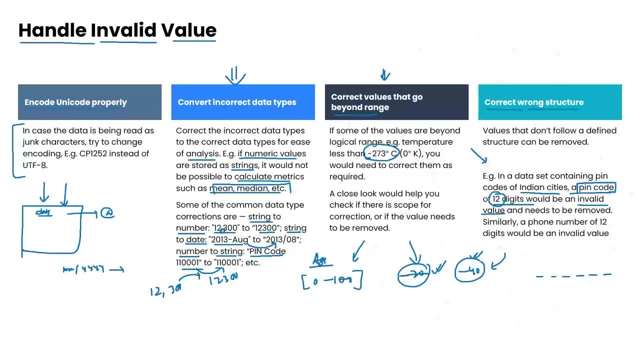 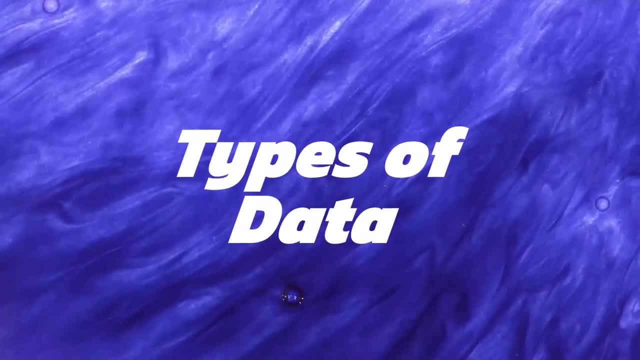 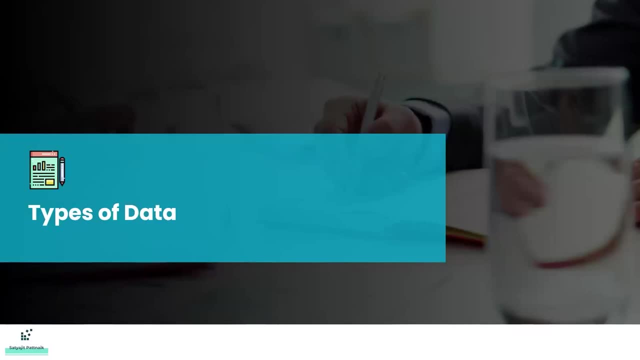 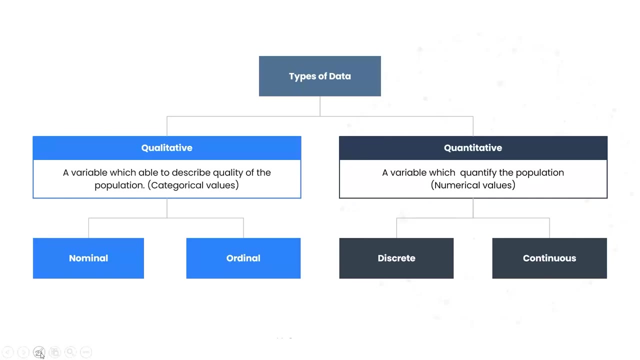 in the next video, we shall be talking about various other topics related to types of data and various other types of analysis. hi, in this video, we shall be talking about the different types of data. now, this is something that we already discussed in the past. majorly, there are two types of data, one of them being qualitative. 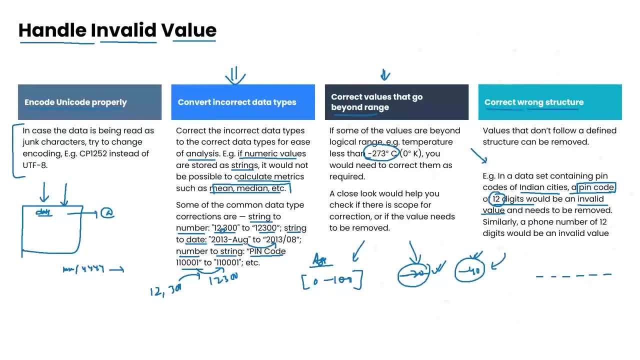 field of data analysis. once you start doing the EDA part, you will come across a so many scenarios where you have to deal with it and automatically will learn by experience. that's all about this particular video. in the next video, we shall be talking about various other topics related to types of data and 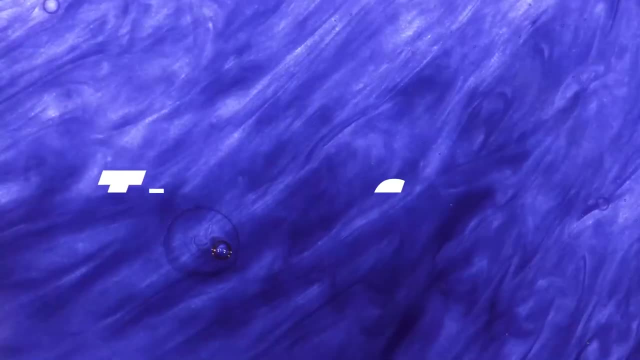 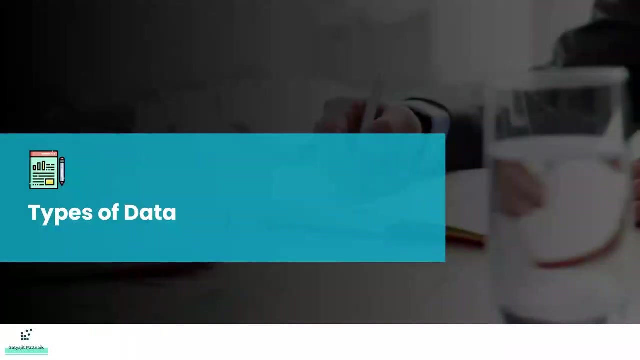 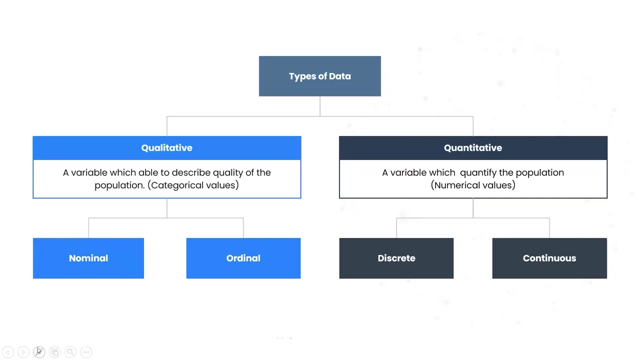 various other types of analysis. hi, in this video, we shall be talking about the different types of data. now, this is something that we already discussed in the past. majorly, there are two types of data, one of them being qualitative data and one of them being quantitative data. qualitative data simply are the 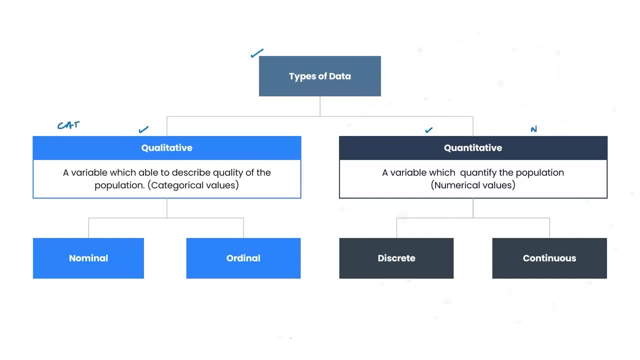 categorical data and quantitative data are your. numerical data, a variable which is able to describe the quality of the population, are called as qualitative, and the variable which quantifies the population are here quantitative data. under categorical data or under qualitative data, there are further two types, one of them being nominal and one of them being ordinal. nominal data simply is the type of data. 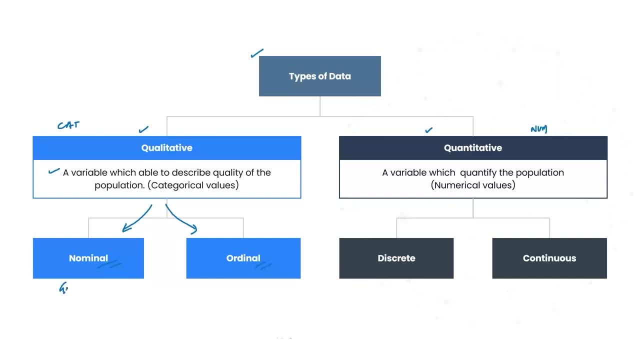 that is not in any order, for example, gender- male or female. location, japan, india, indonesia or korea or any other country. so these are your nominal categorical data. ordinal are those kind of data that is in an order now, for example, economic status, low, medium or high grades, a, b or c and so on. they are in an order. you go from left to right or right. 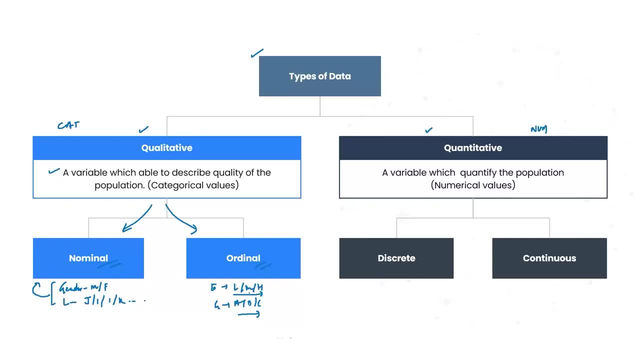 to left. they are in an order, either in ascending order or descending order. coming on to the quantity quantitative part, quantitative is of two types, one of them being discrete and one of them being continuous. discrete numerical data are those kind of data that are discrete in nature. for example, if somebody asks you how many students do we have in a class. 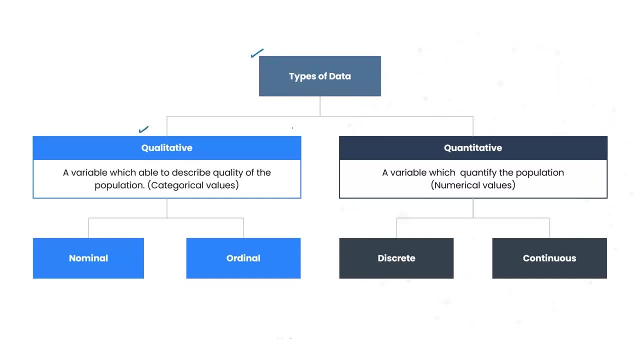 data, and one of them being quantitative data. qualitative data simply are the categorical data, and quantitative data are your numerical data. a variable which is in the category of data is called quantitative data, and quantitative data is the type of data that is able to describe the quality of the population. 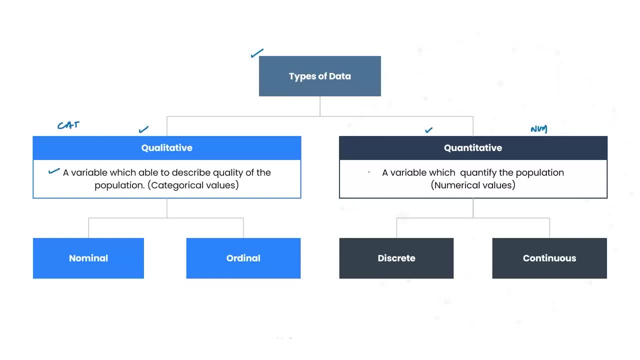 are called as qualitative, and the variable which quantifies the population. are your quantitative data, under categorical data or under qualitative data? there are further two types, one of them being nominal and one of them being ordinal. nominal data simply is the type of data that is not in any order. 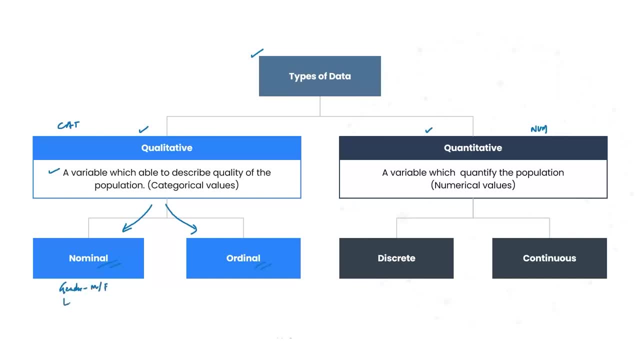 it has nothing to do withchw good food or health already hadchen data regarding two major things this is also where all kinds of relationships are � and two of them beingient to occasions for all kinds of life choices and especially it has to do with age 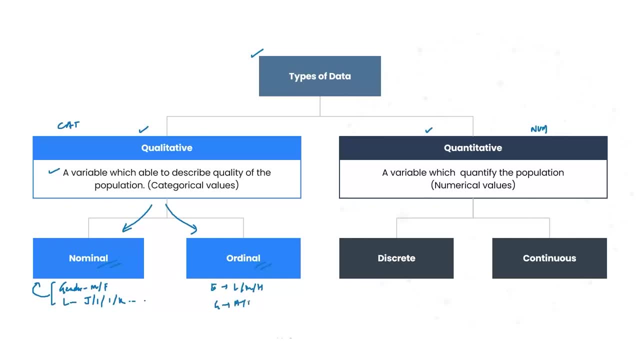 and it also has to deal with the biological class of how babies şimdi, our quiero Evet. so the next forward studied up to the Aido will come forth. so this kind the combination of data will be different for you if you were in a national Ontario area, Будup world, when you fundamentals in India or by any one mind like compare them with job abilities, if your position and political status can also be the same, 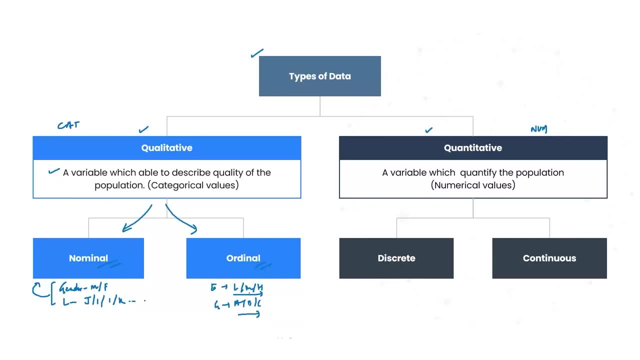 you go from left to right or right to left, they are in an order, either in ascending order or descending order. coming on to the quantitative part, quantitative part quantitative is of two types, one of them being discrete and one of them being continuous. discrete numerical data are those 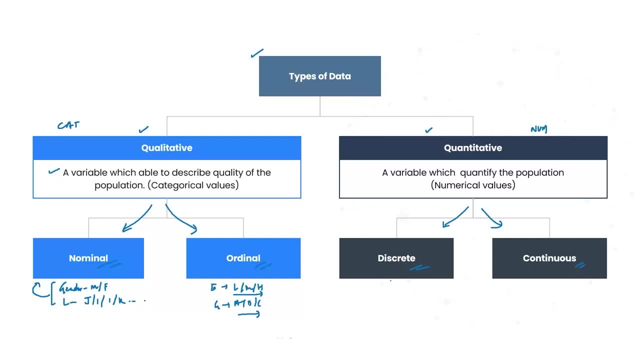 kind of data that are discrete in nature. for example, if somebody asks you how many students do we have in a class, your answer has to be 42 or 45 or 50. it cannot be 42.5. there cannot be 42.5 students in a class or 42.7 students in a class, not possible. so these type of data are discrete. 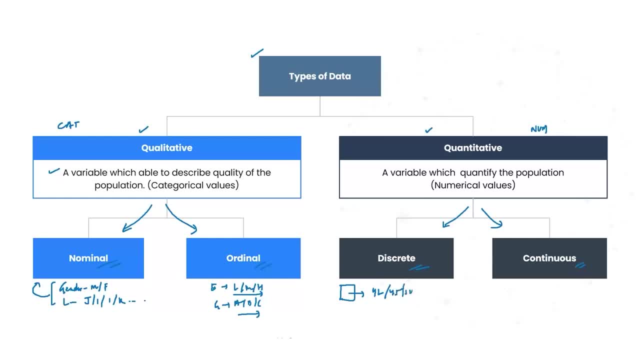 your answer has to be 42 or 45 or 50. it cannot be 42.5. there cannot be 42.5 students in a class or 42.7 students in a class, not possible. so these type of data are discrete data. 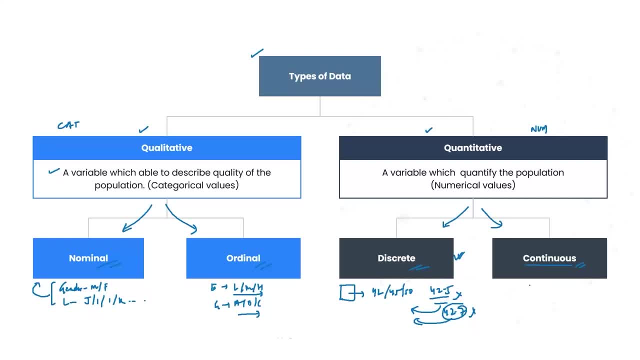 continuous data are continuous in nature, for example, temperature range. what is the temperature in your country right now? or in your place right now? 37.7 degrees or 37.2 degrees? so it could literally be any number within a range of something to something. so these are the different types of 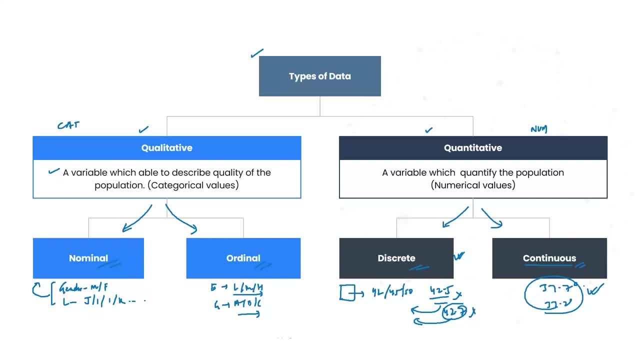 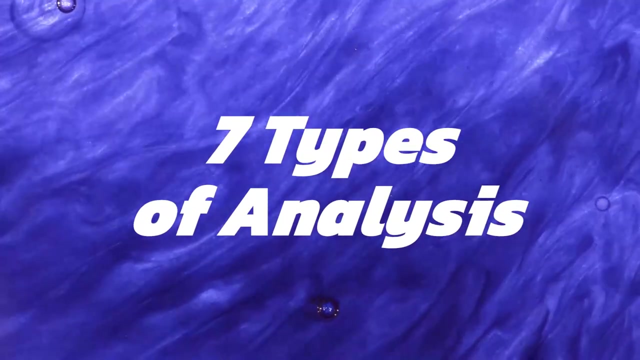 data. the reason why we talked about this topic is that, from the next slide onwards, we will be jumping into each one of these type of data- categorical and numerical- and we will be performing some categorical and numerical analysis. that's all about this particular video. see in the next video. 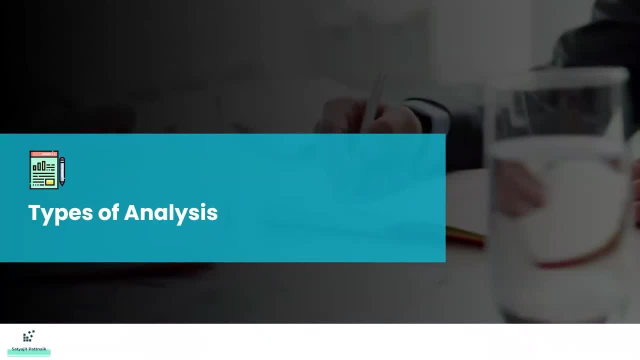 in this video, we shall be talking about the types of data: categorical and numerical analysis, about the different types of analysis that we perform. we all know that data are of two types: categorical, numerical. and based on the type of data, we should decide which type of analysis we need to do, because our ultimate goal is to 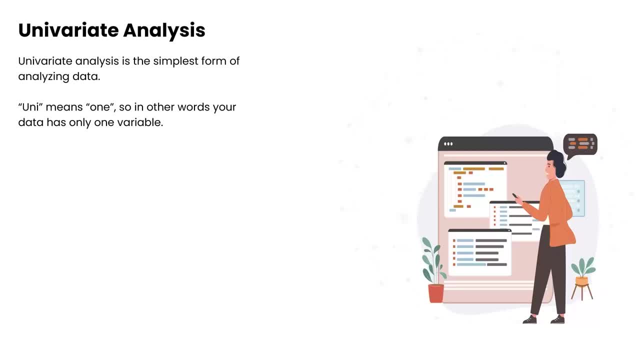 understand the data and understand the various characteristics. now the first topic is going to be univariate analysis. univariate analysis is basically one type of analysis where we only deal with one variable. uni basically means one variable. now, what do you mean by univariate analysis? univariate analysis? 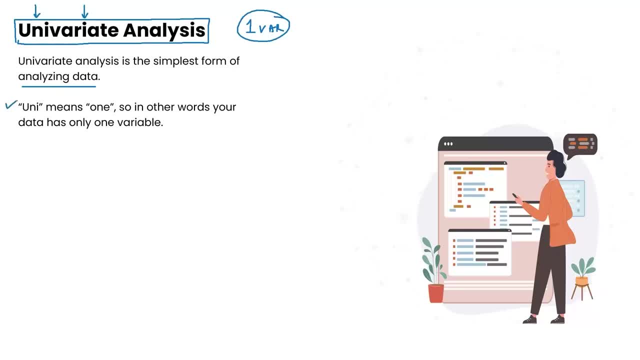 is the simplest form of analyzing data. uni means one, so in other words, your data has only one variable. now, taking an example, I will try to explain this: univariate analysis. univariate analysis can be done for numerical and can be done for categorical data, but we mostly use it for categorical data because it gave us more insights in 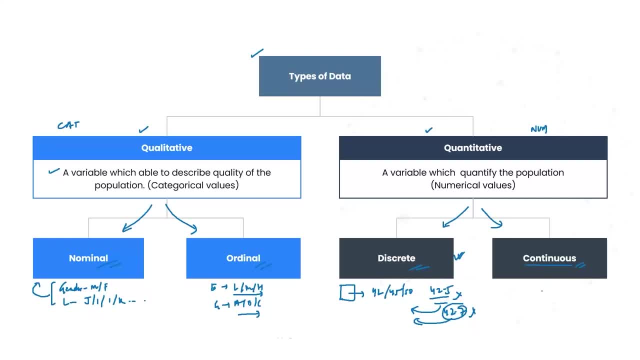 data. continuous data are continuous in nature. for example, temperature range. what is the temperature in your country right now? or in your place right now? 37.7 degrees or 37.2 degrees? so it could literally be any number within a range of something to something. so these are the different types of data, the reason why we talked about this topic. 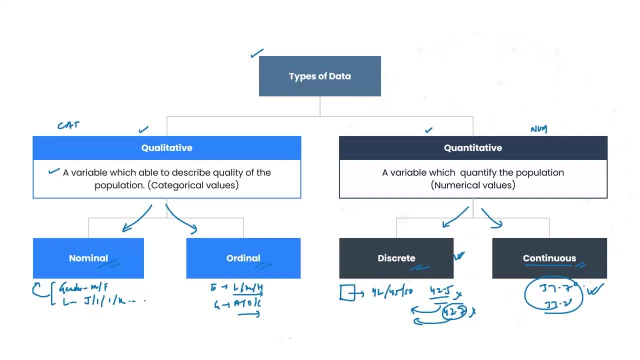 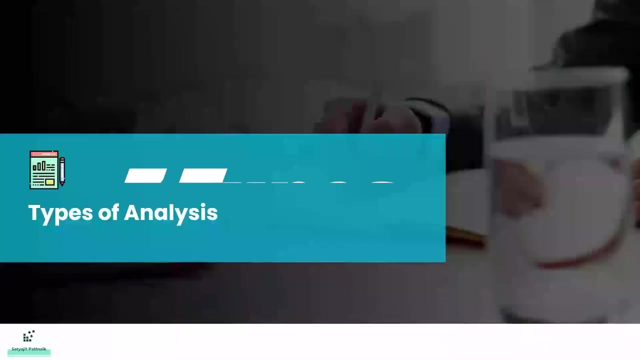 is that, from the next slide onwards, we will be jumping into each one of this type of data, categorical and numerical, and we will be performing some categorical and numerical analysis. that's all about this particular video. see in the next video. in this video we shall be talking about the different types of analysis that we perform. 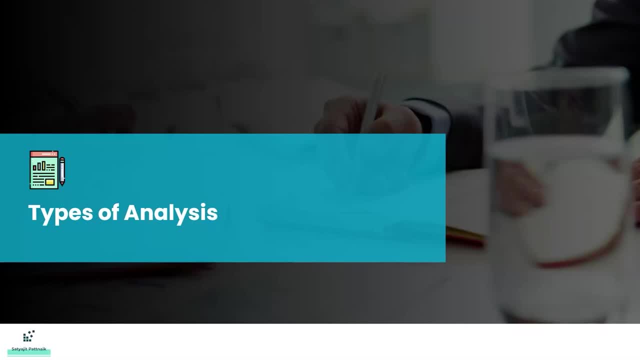 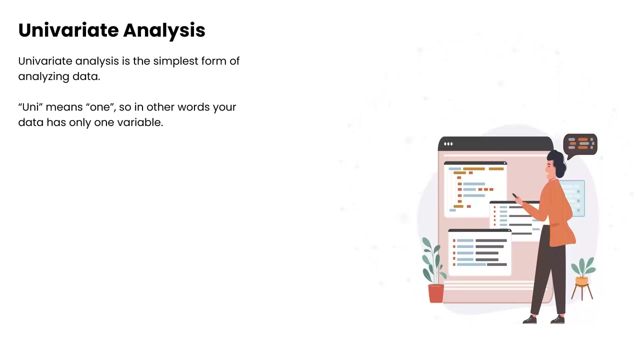 we all know that data are of two types: categorical, numerical and based on the type of data, we should decide which type of analysis we need to do, because our ultimate goal is to understand data and understand the various characteristics. now the first topic is going to be univariate analysis. 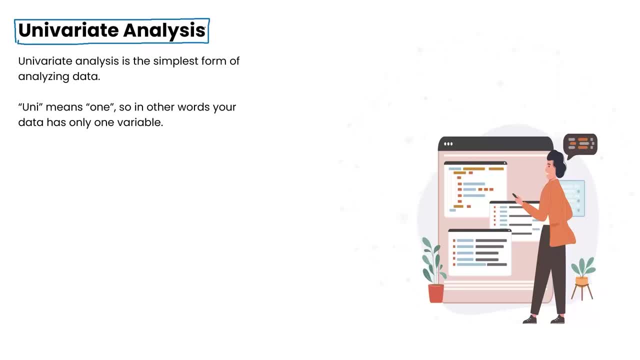 univariate analysis is basically one type of analysis where we only deal with one variable. uni basically means one variable. now, what do you mean by univariate analysis? univariate analysis is form of analyzing data. uni means one, so in other words, your data has only one variable. now, taking an example, I will try to explain this univariate analysis. 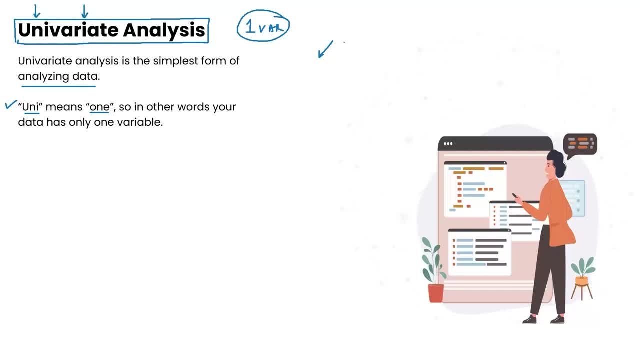 univariate analysis can be done for numerical and can be done for categorical data, but we mostly use it for categorical data because it give us more insights in terms of numerical data. we just get to know what are the summary statistics of this numerical column. now we'll start with categorical data, so we 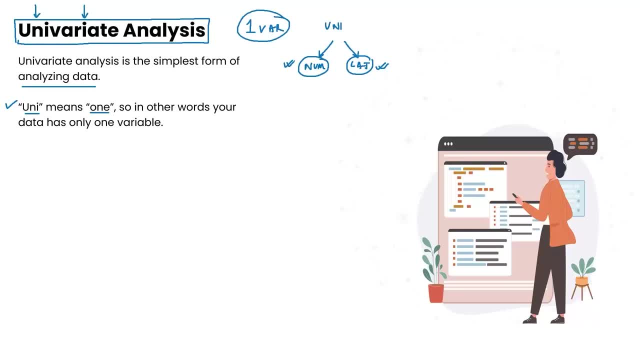 terms of numerical data, we just get to know what are the summary statistics of data and what are the data that we are using. in terms of numerical data, we just get to know what are the summary statistics of this numerical column. now we'll start with categorical data, so we will take an 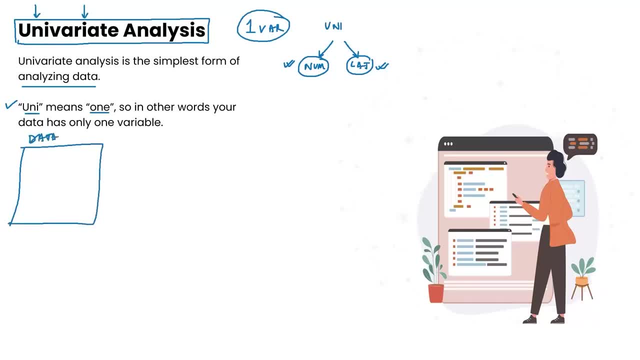 example of one type of data that we have. let's say, you are analyzing customers data. now, this data is a churn records. churn records, which basically means that you, as a data analyst, have joined a company. let's say, the company's name could be anything. I will give a generic name: vodafone is a global telecom provider. well, let's say: 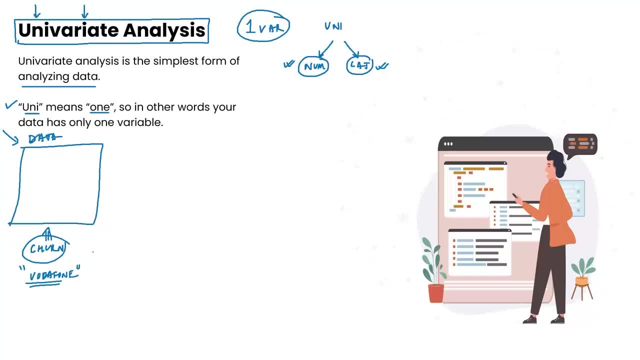 you have started using vodafone. you join this company as a data analyst. your manager gives you a data that hey, you know what? these are all the customer related information. our company's churn rate is almost twenty five percent, which means almost twenty five percent of the people in. 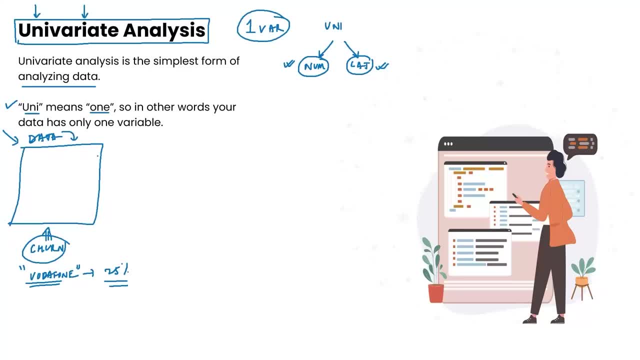 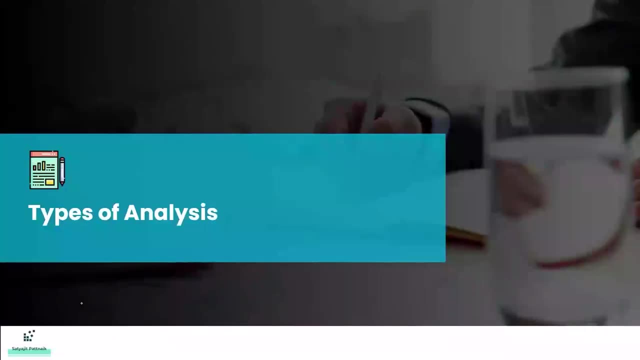 leave our company on a monthly basis. why people leave companies? they leave Vodafone or they leave in this video. we shall be talking about the types of analysis now. before getting into the types of analysis, first of all we need to understand what type of data we are analyzing. we all know data is majorly of two types. one is categorical. 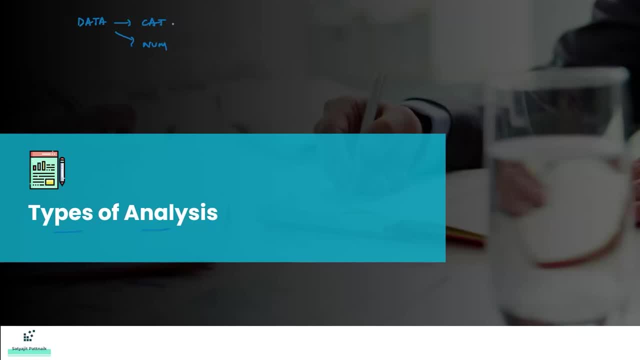 data, and one is numerical data. once we know our data properly- we know what are our categorical data and what are our numerical data- further we can take our next steps in analyzing the data. so the first topic that we are going to discuss is going to be univariate analysis. 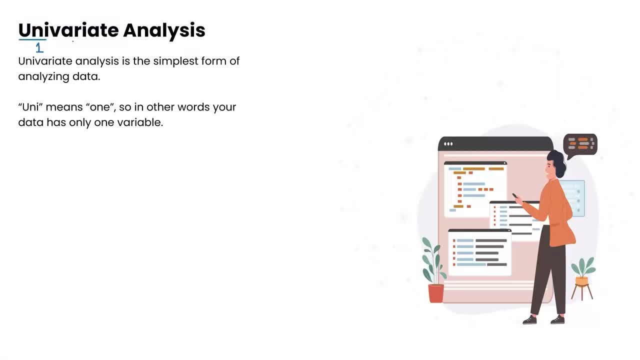 in terms. uni means one. variate means variable, so when you are analyzing just one variable, that is called as a univariate analysis. it is the simplest form of analyzing data. uni means one, so in other words, your data has only one variable. univariate analysis can be applicable for numerical data and can be 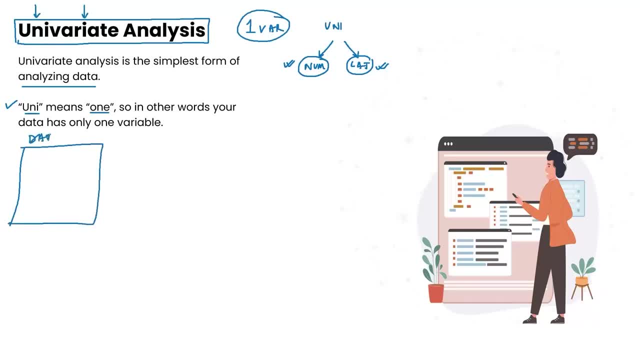 will take an example of one type of data that we have. let's say you are analyzing customers data. now, this data is a churn records. churn records, which basically means that you, as a customer, you are analyzing the customer's data and you, as a data analyst, have joined a company, let's say the company's name could be: 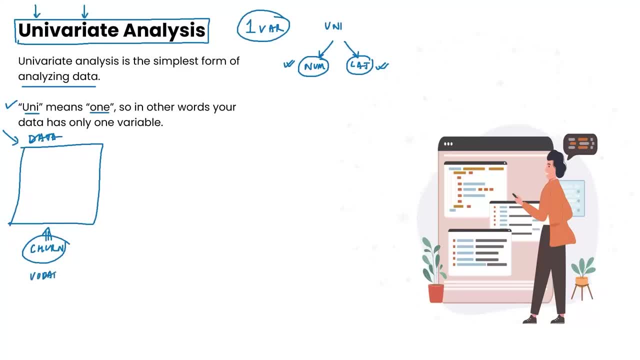 anything, I will give a generic name. Vodafone is a global telecom provider. so let's say, you have started using Vodafone. you join this company as a data analyst. your manager gives you a data that, hey, you know what? these are all the customer related information. our company's churn rate is almost 25% and 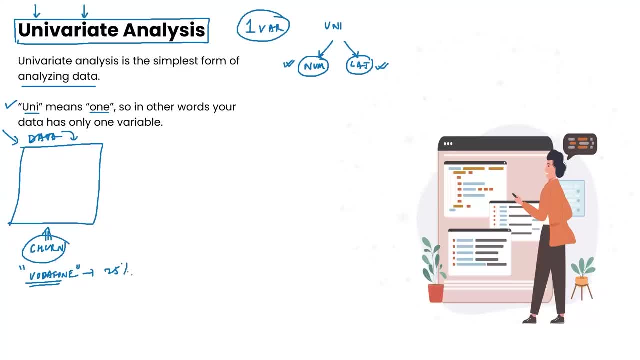 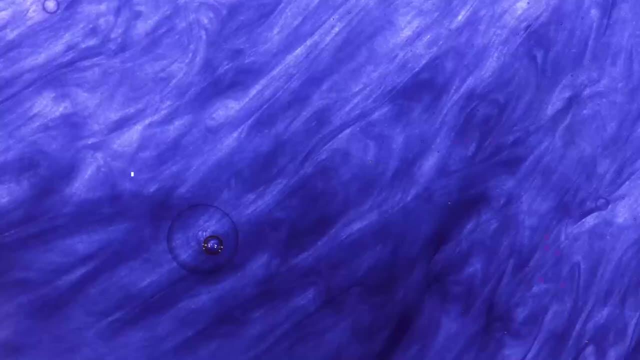 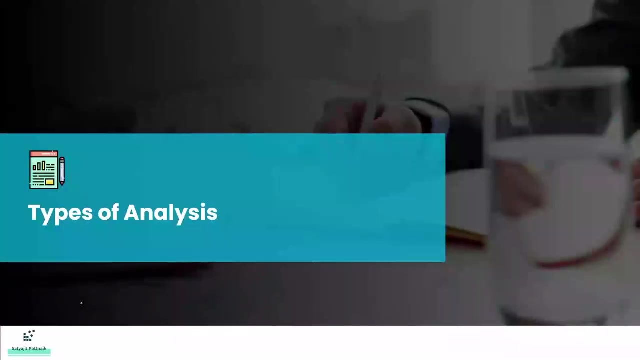 you can use it to get your data. and then you can use it to get your data, which means almost 25% of the people leave our company on a monthly basis. why people leave companies? they leave Vodafone or they leave. in this video, we shall be. 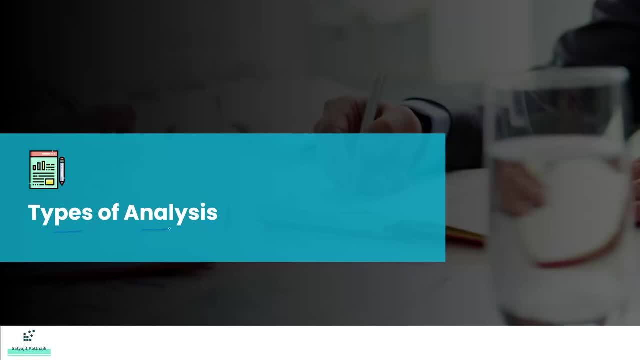 talking about the types of analysis now before getting into the concept. so let's into the types of analysis. first of all, we need to understand what type of data we are analyzing. we all know data is majorly of two types. one is categorical data and one is numerical data. 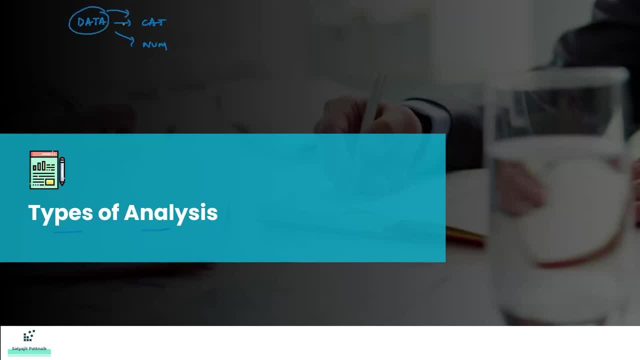 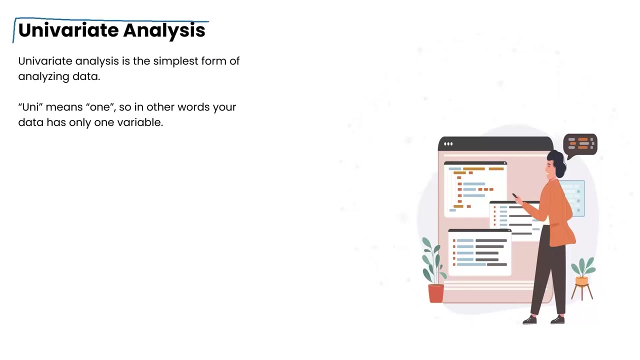 once we know our data properly- we know what are our categorical data and what are our numerical data- further we can take our next steps in analyzing the data. so the first topic that we are going to discuss is going to be univariate analysis. in simple terms, uni means one, variate means variable. so when you are analyzing just one variable, that is. 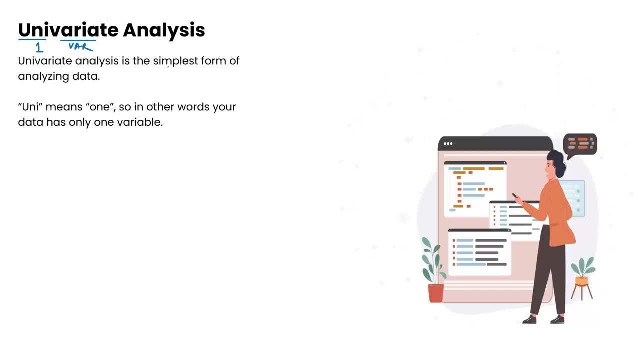 called as a univariate analysis. it is the simplest form of analyzing data. uni means one, so in other words, your data has only one variable. univariate analysis can be applicable for numerical data and can be applicable for categorical data in numerical data. let's say we are analyzing a column h. what are the insights that we could get? 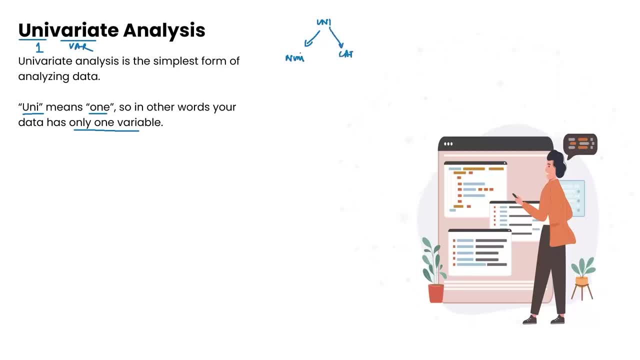 applicable for categorical data in numerical data. let's say we are analyzing a column age. what are the insights that we could get? once we print the summary statistics of this column, or probably plot a box plot, we will have a better understanding about its statistical values. what is the minimum? 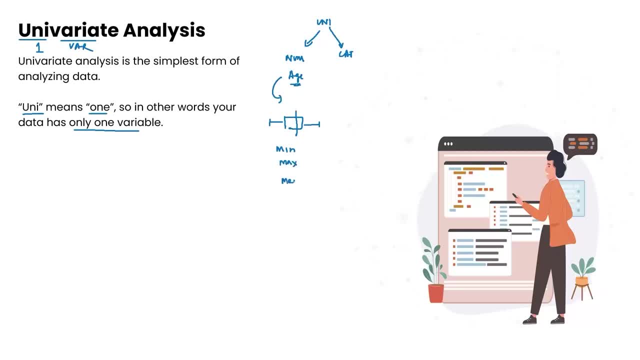 age? what is the maximum age? what is the median age, which is the twenty-fifth percentile, seventy-fifth percentile, and so on. so this will basically tell us how our data spread is for a particular numerical column. similarly, with the categorical column, we also get to know the distribution. for example, I have a 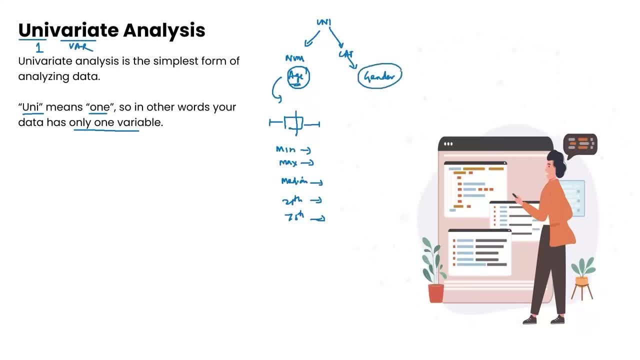 column called as gender, and if somebody asks you, can you do the univariate analysis of gender. it simply means you need to analyze and understand what is the univariate analysis of gender. and what is the univariate analysis of gender? it simply means you need to analyze and understand what is the 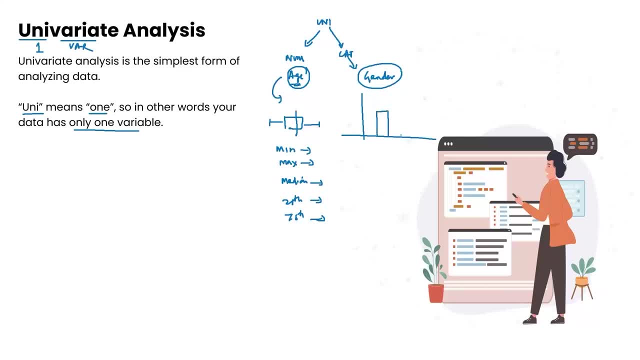 distribution of this particular column. let's say, the distribution is something like this: there are 8,000 male and 2,000 females, which clearly indicates that male are larger in number, and the ratio is almost 4 is to 1. so this is the simplest form of analysis, which is univariate analysis. so if you are 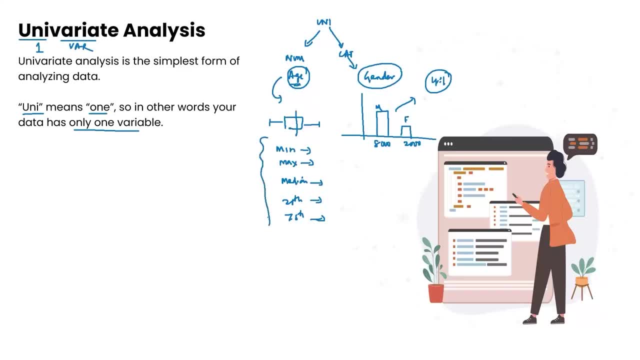 dealing with a numerical column, you get the statistical information and get to know how the spread of the data is, and if it is a categorical column, then you get to know how the distribution of the details. now let's try to take an example and understand more. imagine I will be taking a telecom related use case. 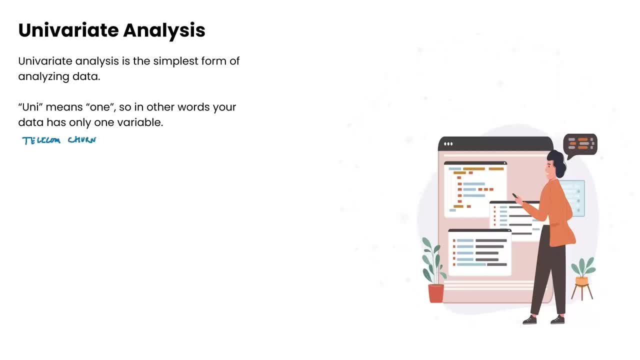 telecom churn analysis. this is my use case. so, for example, I'll consider a company- let's say a company which is a company, which is a company which is a XYZ, or just I will give a name. let's say you join this company called as Vodafone as a data analyst. now your manager tells you that hey, you know what? 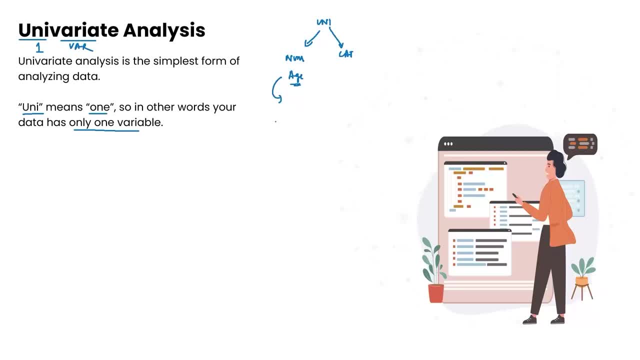 once we print the summary statistics of this column, or probably plot a box plot, we will have a better understanding about its statistical values. what is the minimum age, what is the max minimum age? what is the median age, what is the 25th percentile, 75th percentile and so on? 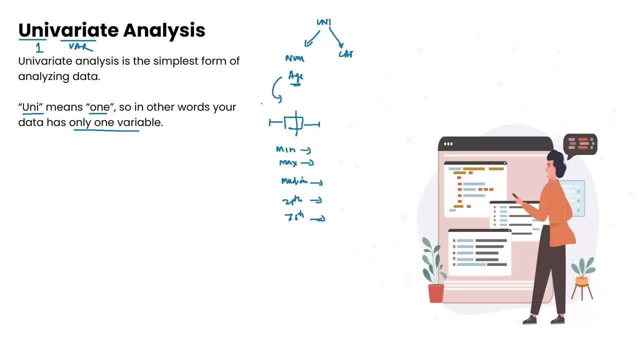 so this will basically tell us how our data spread is for a particular numerical column. similarly, with the categorical column we also get to know the distribution. for example, i have a column called as gender and if somebody asks you, can you do the univariate analysis of gender. 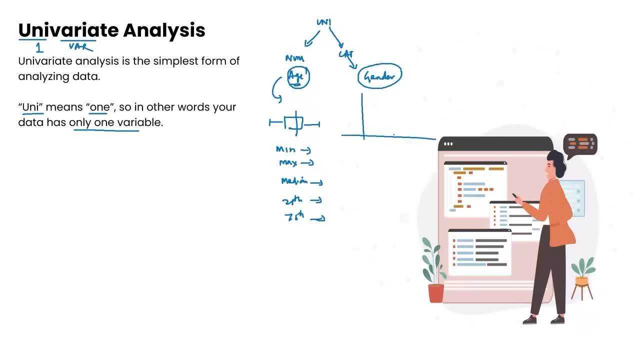 it simply means you need to analyze and understand what is the distribution of this particular column. let's say the distribution is something like this: there are eight thousand male and two thousand females, which clearly indicates that male are larger in number and the ratio is almost four is to one. so this is the simplest form of analysis, which is univariate analysis. so if you are dealing 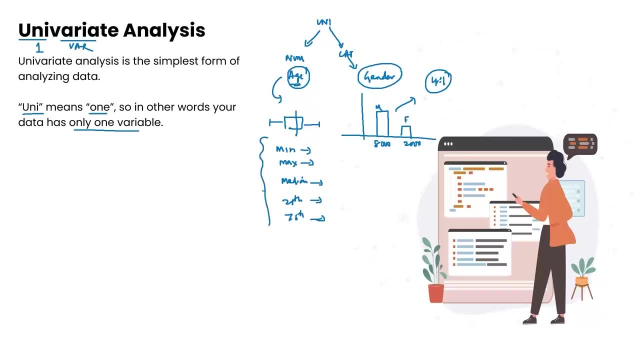 a numerical column, you get the statistical information and get to know how the spread of the data is. and if it is a categorical column, then you get to know how the distribution of the data is. now let's try to take an example and understand more. imagine i will be taking a telecom. 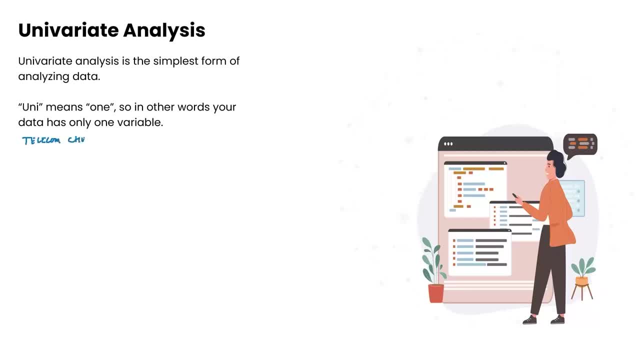 related use case: telecom churn analysis. this is my use case. so, for example, i'll consider a company- let's say xyz, or just i'll give a name- let's say you join this company called as vodafone as a data analyst. now your manager tells you that: hey, you know what? 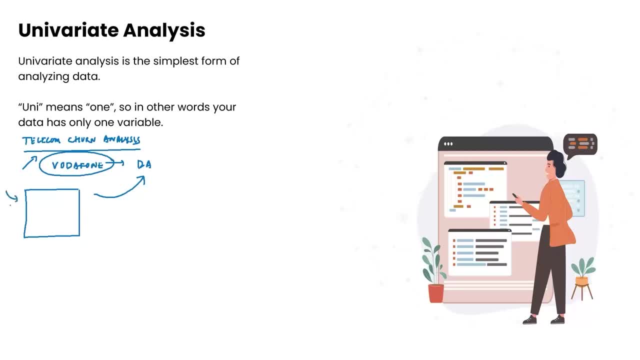 we have a set of data which is having data for the past 24 months, almost two years. my data is telling that almost 25% is my churn rate. what do you mean by churn? churn basically means when somebody leaves a particular company and join other company. with the context of 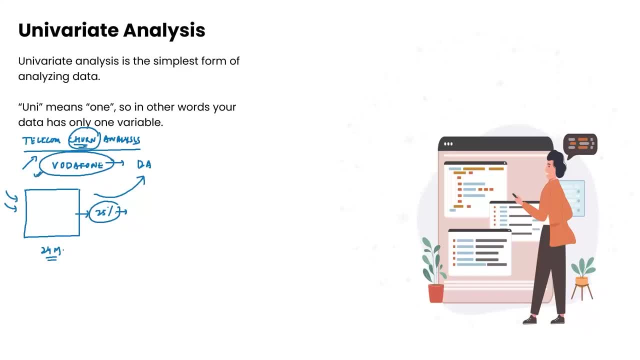 telecom churn basically means if a user who was a Vodafone user has switched to another network and that switch could be because of multiple reasons. if the customer was not happy with the services or Vodafone was charging more, there could be multiple reasons because of which customers churn and join another company. for example, churning with context with 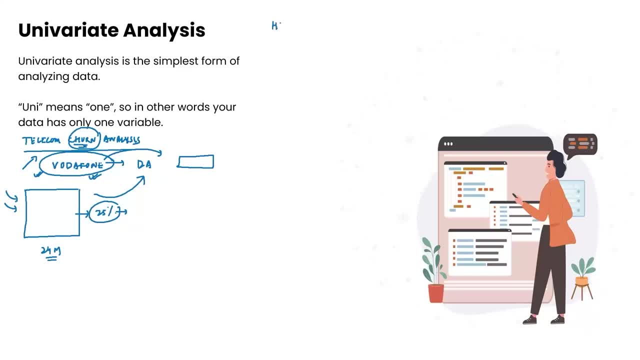 banking. let's say, today you are using one bank, it's a HSBC. tomorrow you get a better deal from standard chartered. so you probably start using incentive standard, standard chattered bank services because they are giving you better returns, better rates, in your own standard chattered bank services. so let's star to chart a value: rich company hedge fund. 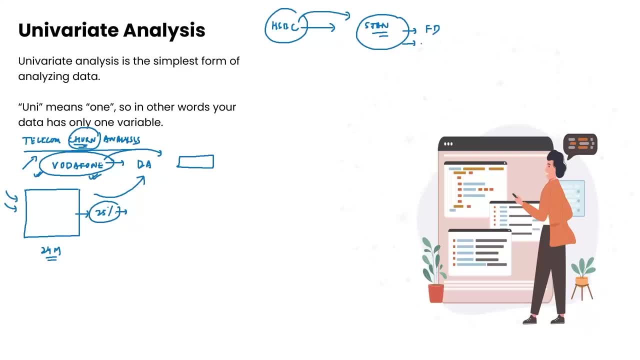 fixed deposits better rates in your normal deposits in the bank. so probably you will leave hsbc and start using standard chapter, which means you are churning out from hsbc. so it is a loss to the hsbc company. so in this particular example, if a user is leaving vodafone, 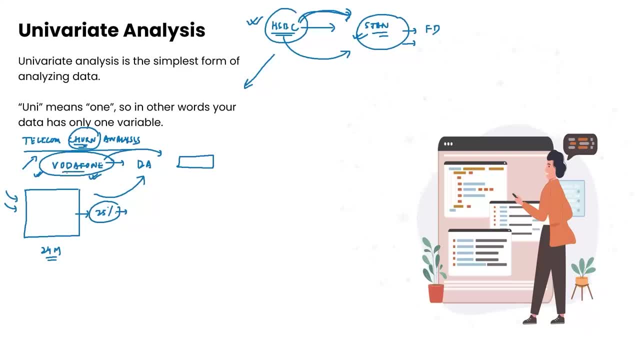 and joining another telecom company, that means it is a loss to the vodafone company. your task as a data analyst is to understand the data and come up with some insights. what could be the potential reasons why people are churning and what are the characteristics of people that are? 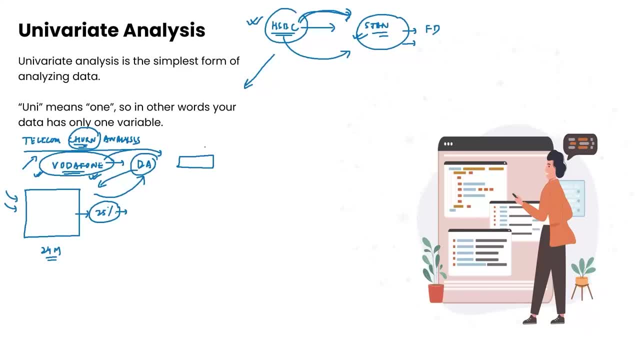 churning right and your ultimate goal is to understand the pattern. so imagine you have a data set of thousand records, simply thousand customers you have and the churn rate is almost 25, which is 750 is to 250. that means 250 churners and 750 active people, and there are multiple. 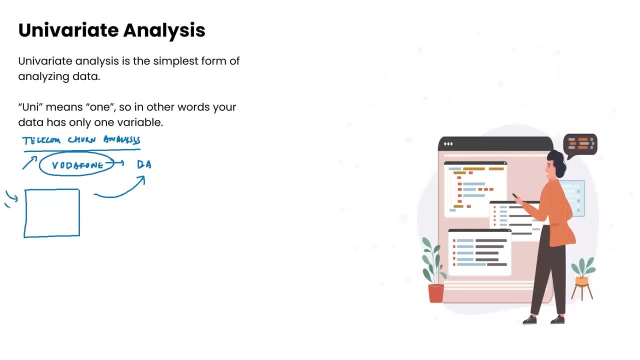 we have a set of data which is having data for the past 24 months, almost two years. my data is telling that almost 25 percent is my churn rate. what do you mean by churn? churn basically means when somebody leaves a particular company and join other company. 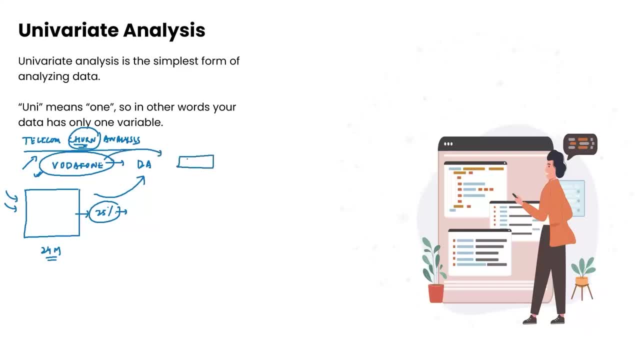 with the context of telecom. churn basically means if a user who was a vodafone user has switched to another network, If the customer was not happy with the services or Vodafone was charging more, there could be multiple reasons because of which customers churn and join another company. 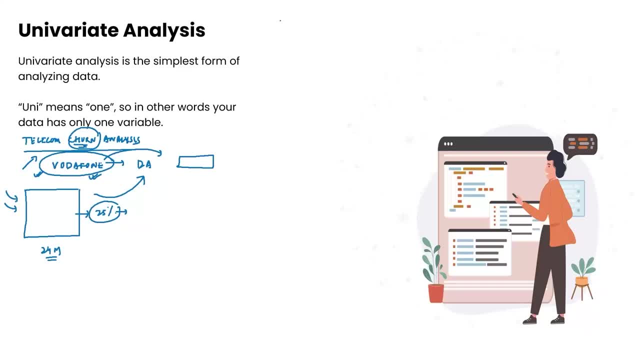 For example, churning with context with banking, Let's say today you are using one bank. let's say HSBC. Tomorrow you get a better deal from Standard Chattered. so you probably start using Standard Chattered bank services Because they are giving you better returns, better rates in your fixed deposits, better rates in your normal deposits in the bank. 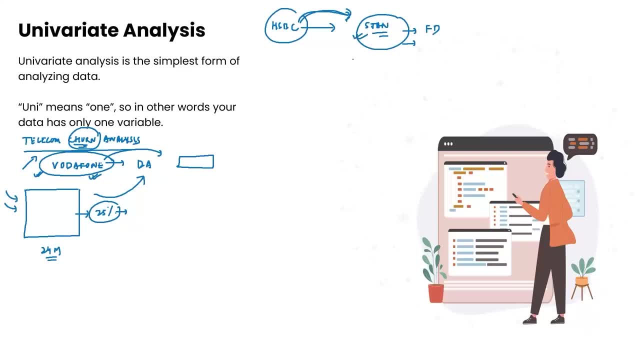 So probably you will leave HSBC and start using Standard Chattered, which means you are churning out from HSBC. So it is a loss to the HSBC company. So in this particular example, if a user is leaving Vodafone and joining another telecom company, 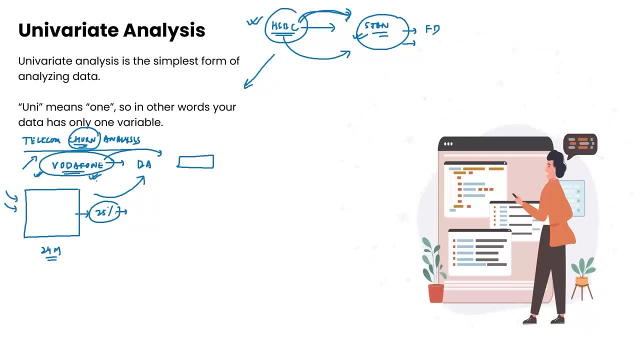 that means it is a loss to the Vodafone company. Your task as a data analyst is to understand the data and come up with some insights. What could be the potential reasons why people are churning and what are the characteristics of people that are churning? 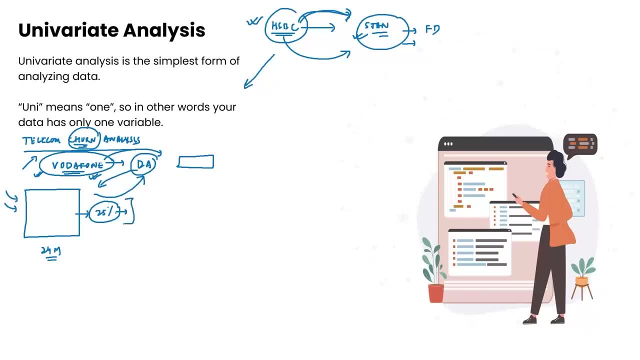 Right, And your ultimate goal is to understand the pattern. So imagine you have a data set of 1000 records, Simply 1000.. 1000 customers you have and the churn rate is almost 25%, Which is 750 is to 250.. 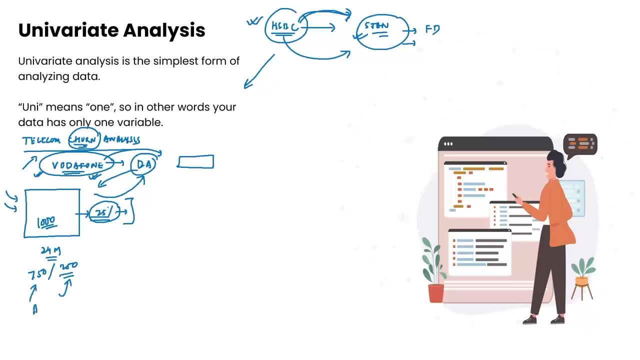 That means 250 churners and 750 active people, And there are multiple columns here: Age, gender, location and so on. As you are dealing with univariate analysis, what you do is you start analyzing columns one by one. So let's say, I start analyzing my gender column. 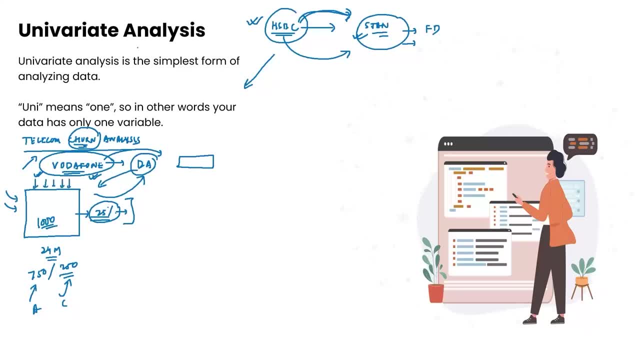 columns here: age, gender, location and so on. as you are dealing with univariate analysis, what you do is you start analyzing columns one by one. so let's say, i start analyzing my gender column. so what will be done? as part of my univariate analysis, i will first try to analyze the overall customers. 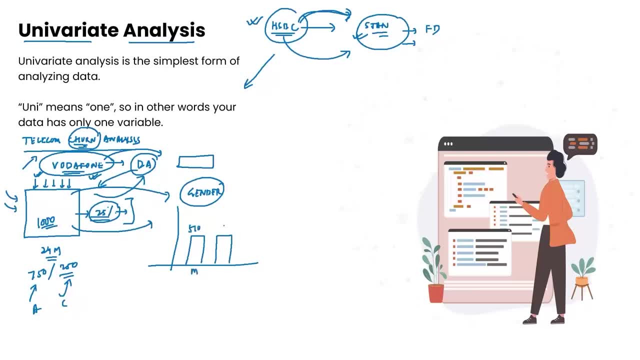 just imagine there are 510 male and 490 female, which clearly means that female and male ratio are almost one is to one. the next step is to analyze the people that have churned. so let's say you see a similar trend: almost 125 male and almost 125 female. so the next step is to analyze the people that have churned. 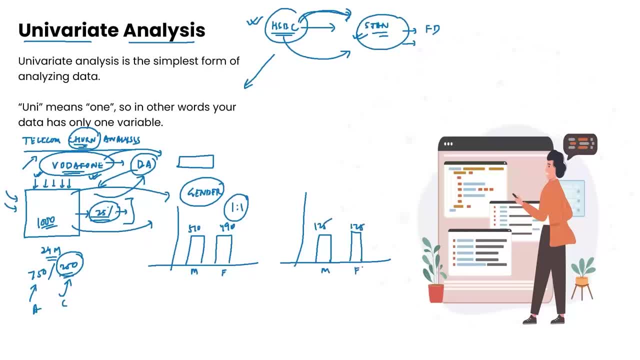 so let's say you see a similar trend: almost 125 male and almost 125 female and almost 125 female, 25 female have churned, which also means a similar ratio of churn with respect to male and female. so the insight here will be: gender has not much of impact on churning. 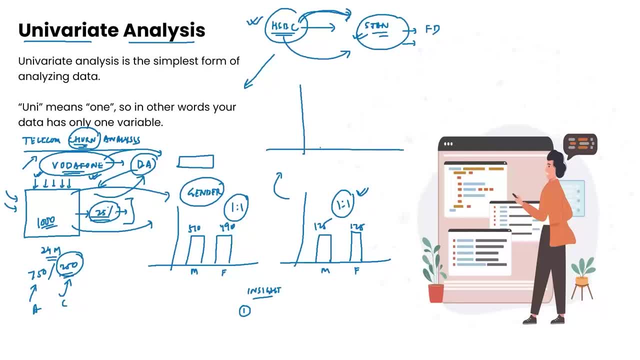 but what if, for the churned customers, you see a trend like this: almost 180 male and almost 70 female, which means more than 2.5 is to 1 ratio. so a lot of people who are male have churned. so that will go as an insight that male customers are more likely to churn. the reasons are: 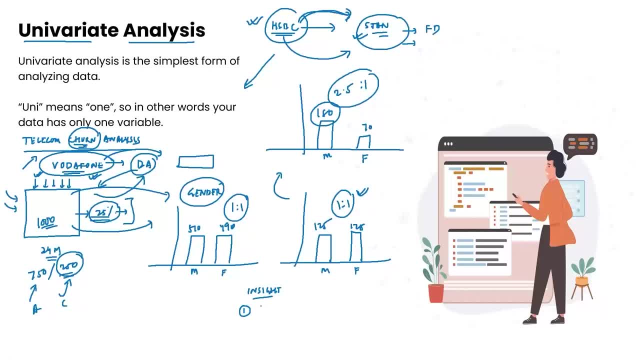 unknown, but this is what the insight that you are getting from univariate analysis. similarly, if you talk about any other categorical analysis, you will see that the churn of male customers is more likely to churn than the churn of female customers. you will do the same thing. you first start analyzing with the 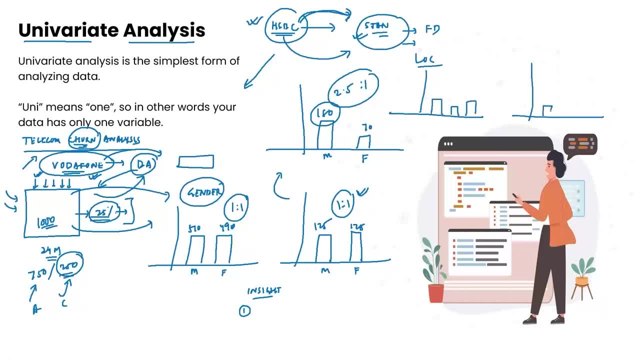 original data and then start analyzing with the churn data and then you compare the percentage of the distribution of the data in the original data and in the churn data and then you will start capturing the insights. in a similar fashion, you also analyze your numerical columns. let's say you talk about age. 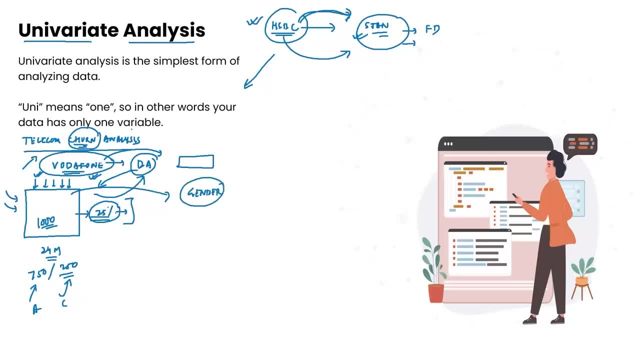 So what will be done? as part of my univariate analysis, I will first try to analyze the overall customers. Just imagine there are 510 male and 490 female, which clearly means that female and male ratio are almost 1 is to 1.. 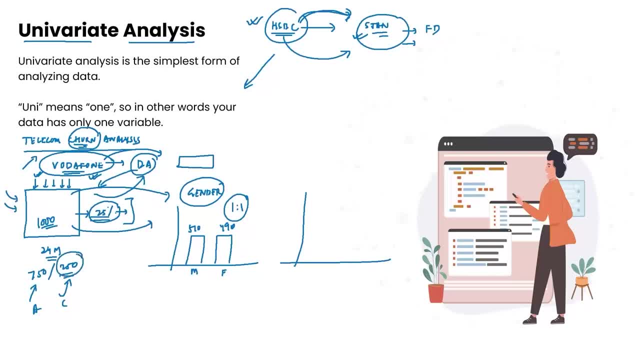 The next step is to analyze the people that have churned. So let's say: you see a similar trend: Almost 125 male and almost 125 female have churned, Which also means a similar ratio of churn with respect to male and female. 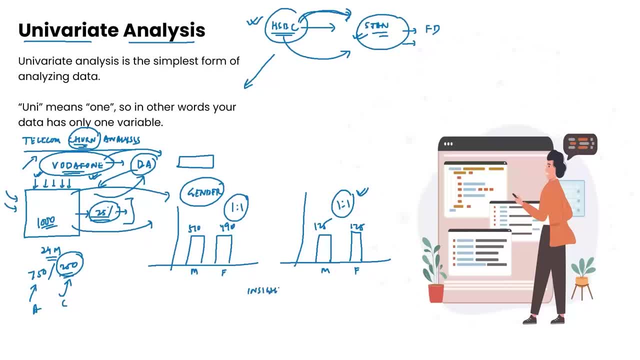 So the insight here will be: gender has not much of impact on churning, But what if, for the churned customers, you see a trend like this: Almost 180 male and almost 70 female, Which means more than 2.5 is to 1 ratio. 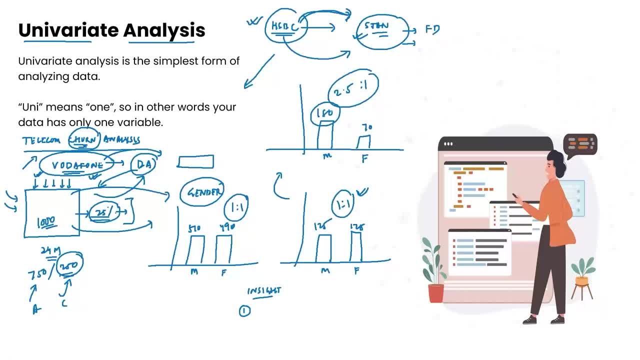 So a lot of people who are male have churned, So that will go as an insight that male customers are more likely to churn. The reasons are unknown, but this is what the insight that you are getting from univariate analysis. Similarly, if you talk about any other categorical column, let's say location, 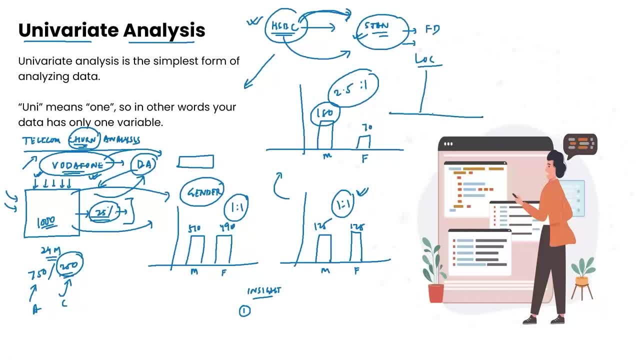 You will do the same thing. You first start analyzing with the original data and then start analyzing with the churned data, And then you compare the percentage of the distribution of the data in the original data and in the churned data And then you will start capturing the insights. 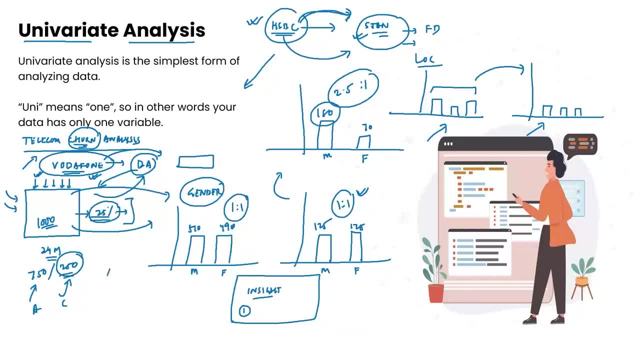 In a similar fashion, you also analyze your numerical columns. Let's say you talk about age. In your original data, your mean age is 25.. Your maximum age is 92.. In the churned data, the mean age is around 35 and the maximum age is 92.. 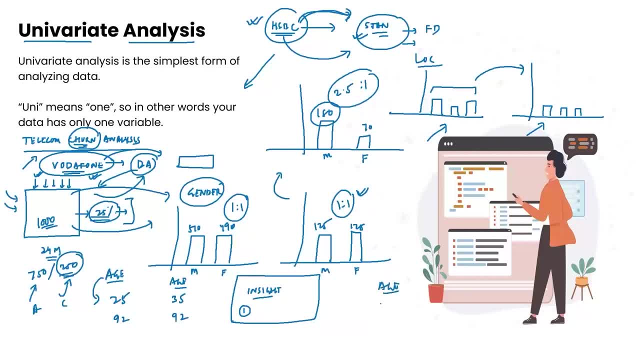 And in the unchurned data that means the active customers. the mean age is 23 and the maximum age is 56. Which clearly means that people who are having more age or who are into the seniority level, they are the high churners. 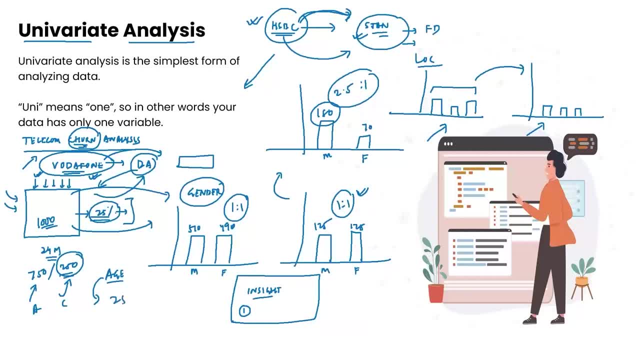 in your original data, your mean age is 25. your maximum age is 92.. in the churn data, the mean age is around 35 and the maximum age is 92, and in the unchurned data that means the active customers- the mean age is 23 and the maximum age is 56, which clearly means that people who are having more age 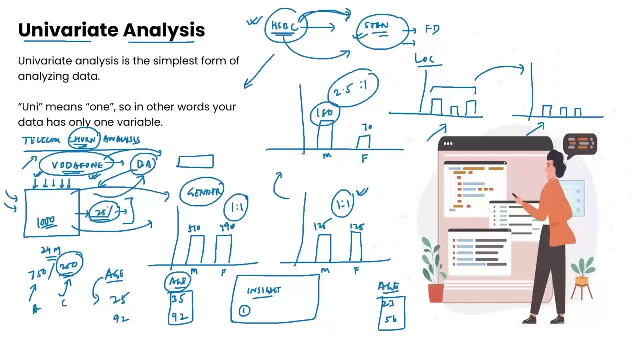 or who are into the seniority level. they are the high churners. now we are not talking about the reasons. we are just talking about the insights that we are getting from each type of analysis. theoretically, that's all about univariate analysis. in the next video we shall be talking about bivariate and numerical analysis, and once we are done with the theoretical, 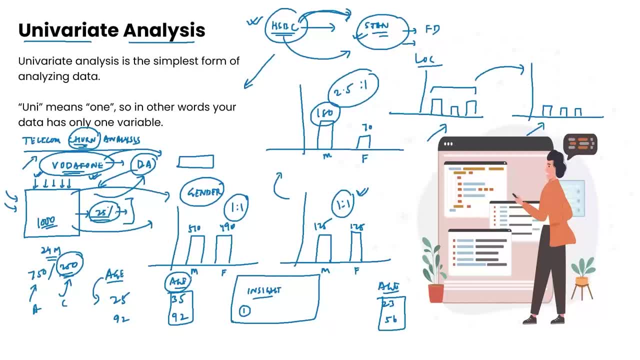 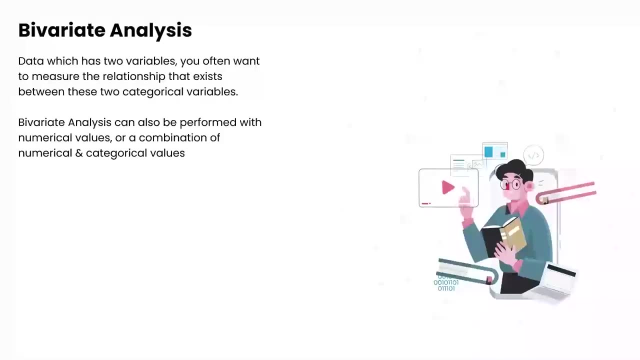 concepts. we will jump into the practicals to show you how each of this analysis is done using a public data set. the next thing that we are going to discuss is bivariate analysis. the concept here remains the same, similar to uni by means two and variate means variables. 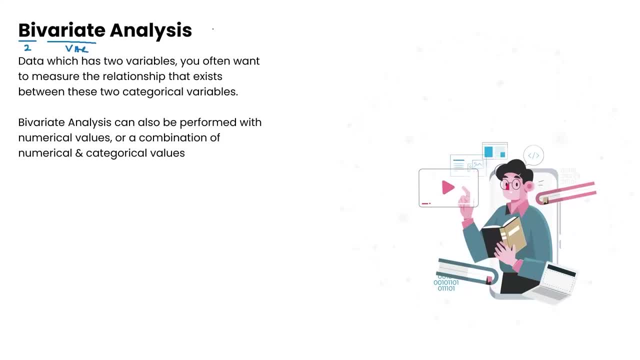 so when we start analyzing two variables, that we call it as a bivariate analysis, so a data which has two variables- you often want to measure the relationship that exists between these two categorical variables. bivariate analysis can also be performed with numerical values or a combination of numerical and categorical. 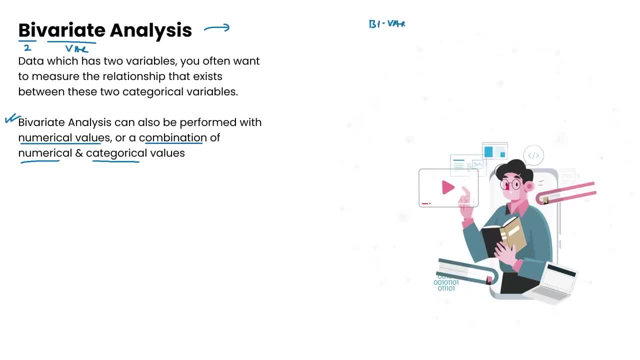 so, in short, bivariate analysis can be done both for numerical and categorical values. we will take the same churn analysis example- telco churn analysis- and we will try to understand now, before getting into the use case. let me just quickly explain you the basics. let's say you are analyzing two numerical attributes. 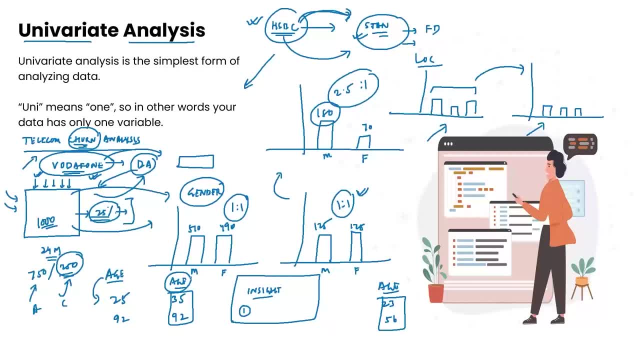 Now we are not talking about the reasons. We are just talking about the insights that we are getting from each type of analysis. Theoretically, that's all about univariate analysis. In the next video, we shall be talking about bivariate and numerical analysis. 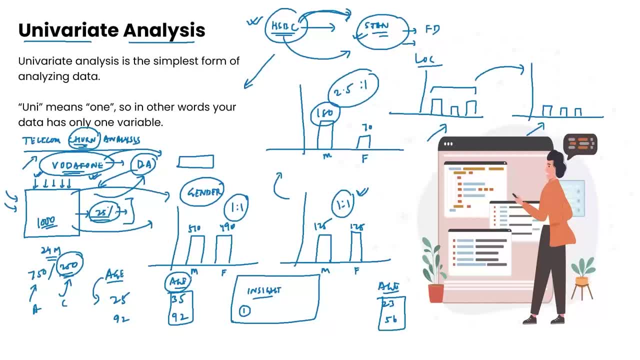 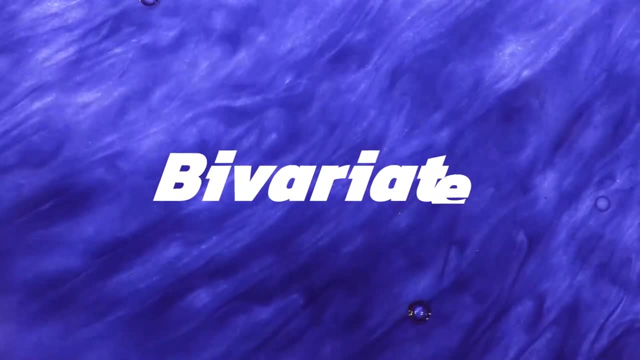 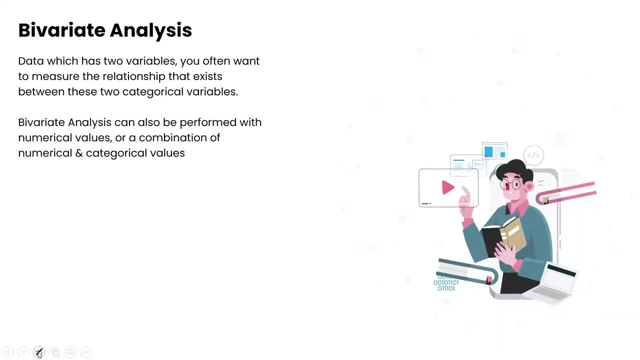 And once we are done with the theoretical concepts, we will jump into the practicals to show you how each of these analysis is done using a bivariate analysis, Public dataset. The next thing that we are going to discuss is bivariate analysis. The concept here remains the same, similar to uni. 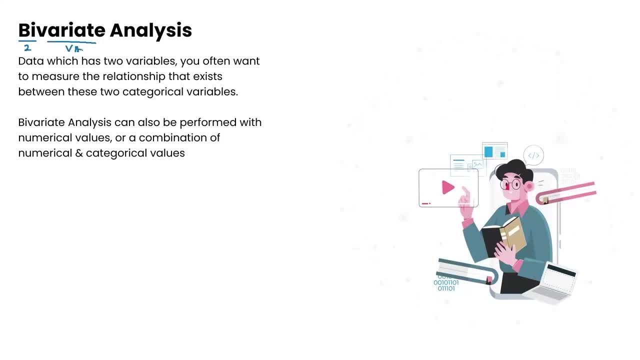 Bi means two and variate means variables. So when we start analyzing two variables, that we call it as a bivariate analysis, so a data which has two variables. you often want to measure the relationship that exists between these two categorical variables. bivariate analysis can also be performed with numerical values. 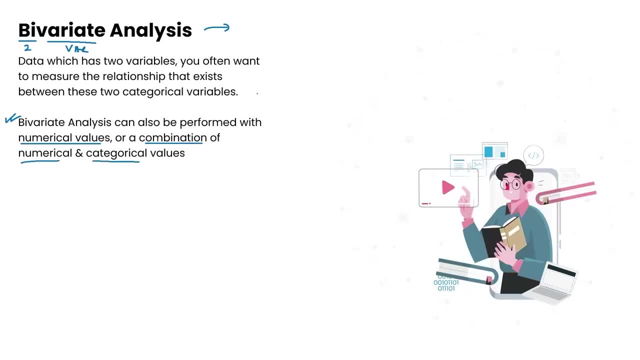 or a combination of numerical and categorical. so, in short, bivariate analysis can be done both for numerical and categorical value. we will take the same churn analysis- example, telco churn analysis- and we will try to understand. now, before getting into the use case, let me just quickly explain you. 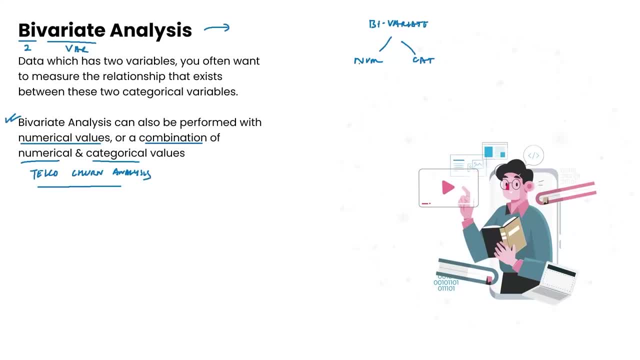 the basics. let's say you are analyzing two numerical attributes or two numerical columns. that means you are analyzing two variables. let us say age and salary. when you are analyzing two numerical attributes, the best way to visualize is using a scatter plot. let's say age in my x-axis. 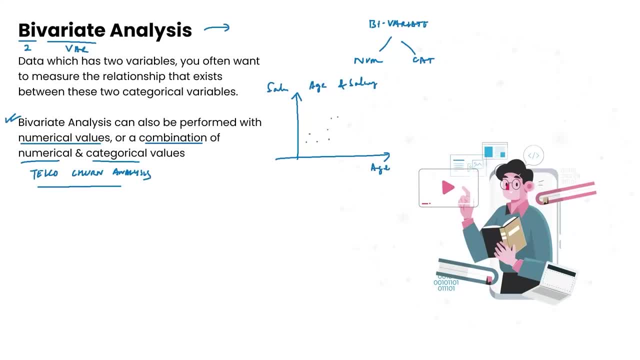 and salary in my y axis and you start plotting the graph and you see a graph like this. using this graph, you can also interpret that there is a covariance and a positive correlation. as you can see, the trend is increasing. that means when the age is increasing, the salary is also increasing and vice versa. 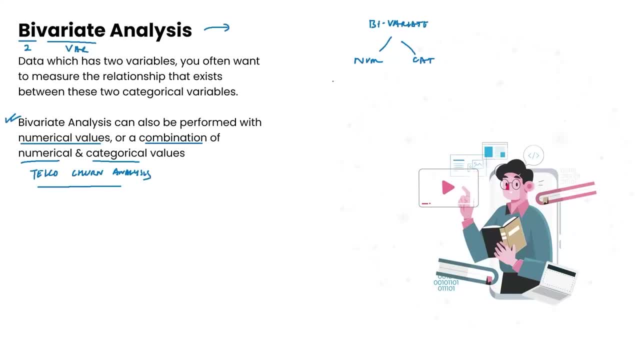 or two numerical columns. that means you are analyzing two variables, let's say age and salary. when you are analyzing two numerical attributes, the best way to visualize is using a scatter plot. let's say age in my x-axis and salary in my y-axis and you start plotting the graph and you see a graph like this: 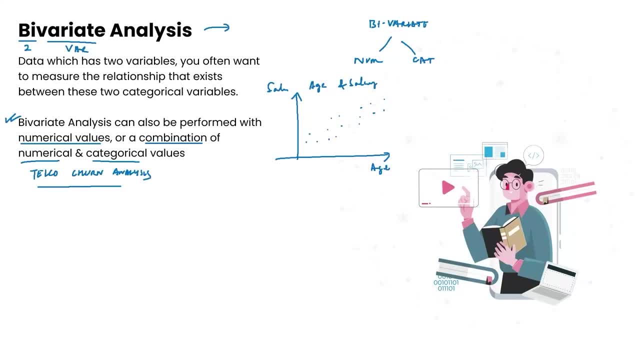 using this graph, you can also interpret that there is a positive covariance and a positive correlation. so, as you can see, the trend is increasing. that means when the age is increasing, the salary is also increasing, and vice versa: when the age is decreasing, the salary is also decreasing. 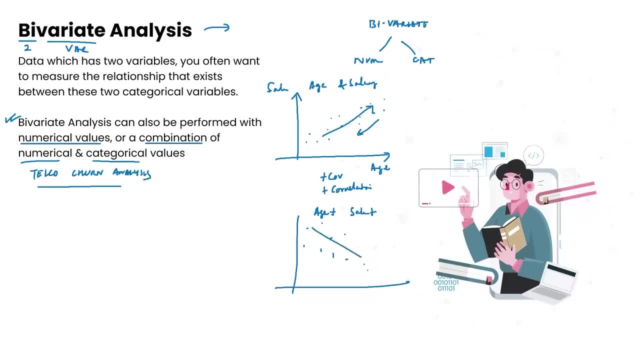 if you see a graph like this, it could potentially say you that when the age is increasing, the salary is decreasing, which means a negative correlation. and when you see a graph like this, where your data are randomly distributed, it is very difficult to understand the numerical relationship between these two numerical variables. so we can assume that there is no correlation, zero correlation. 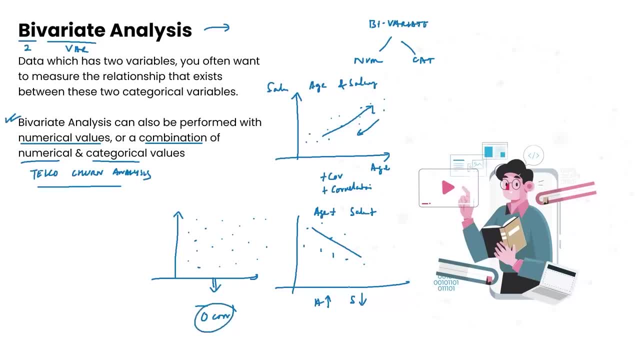 and we all know what is correlation, what is covariance. we usually use correlation to understand the relationship between two numerical attributes. correlation ranges from plus one to minus one, where values closer to minus 1 means negative correlation, which is this scenario. a value closer to 1 is positive correlation, which is this scenario, and a value near to 0 means no correlation, which is: 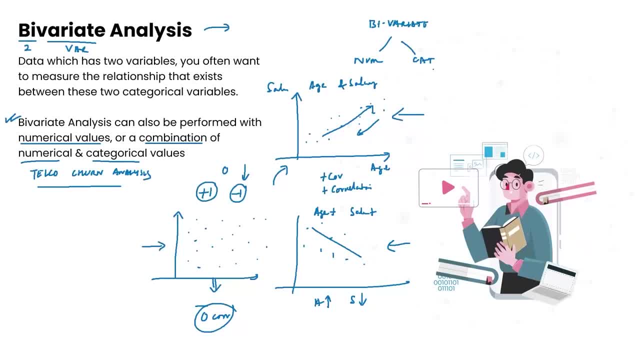 this graph. similarly, if you start analyzing two categorical features, let's say gender and location, and just imagine i have two locations, just for the ease of understanding two location, let's say japan and malaysia. and gender, i have male and female. so i first start analyzing my numerical attributes, sorry, my categorical values for the original data. let's say: 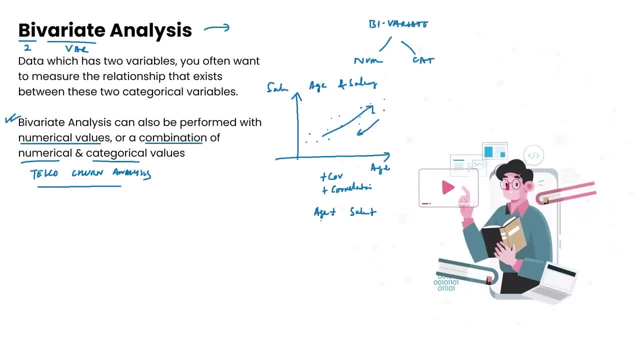 when the age is decreasing, the salary is also decreasing. if you see a graph like this, it could potentially say you that when the age is increasing, the salary is decreasing, which means a negative correlation. and when you see a graph like this, where your data points are randomly distributed, it is very 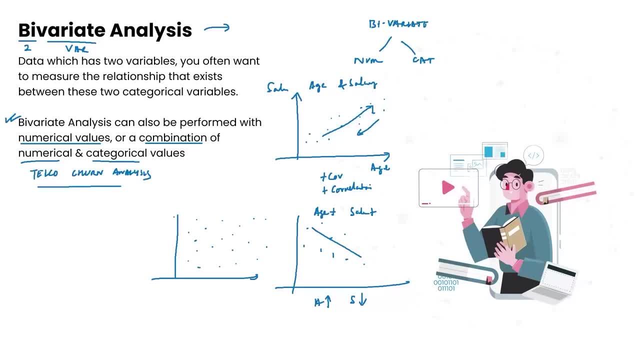 difficult to understand the numerical relationship between these two numerical variables, so we can assume that there is no correlation, zero correlation, and we all know what is correlation, what is covariance? we usually use correlation to understand the relationship between two numerical attributes. correlation ranges from plus one to minus one, where the values closer to minus one means negative correlation. 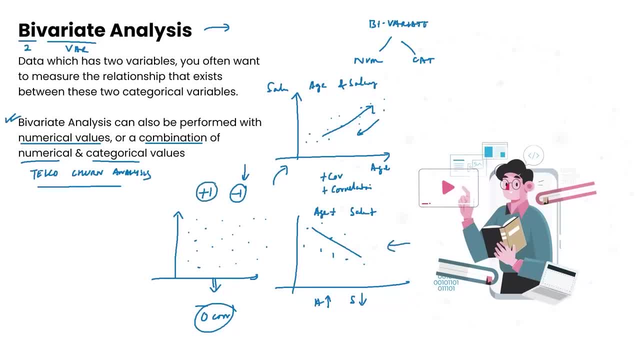 which is this scenario. a value closer to one is positive correlation, which is this scenario, and a value near to zero means no correlation, which is this graph. similarly, if you start analyzing two categorical features, let's say gender and location, and just imagine i have two locations, just for the ease of 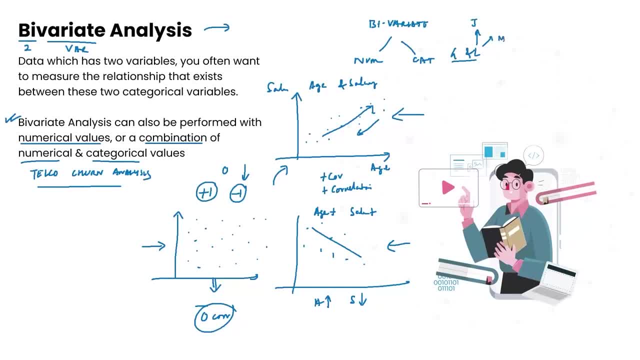 understanding. I have two location, let's say Japan and Malaysia, and gender. I have male and female. so I first start analyzing my numerical attributes- sorry, my categorical values for the original data, let's say for male and female, Japan, Malaysia, Japan and Malaysia. the malaysia: that means most of the people are from japan and less people from malaysia. 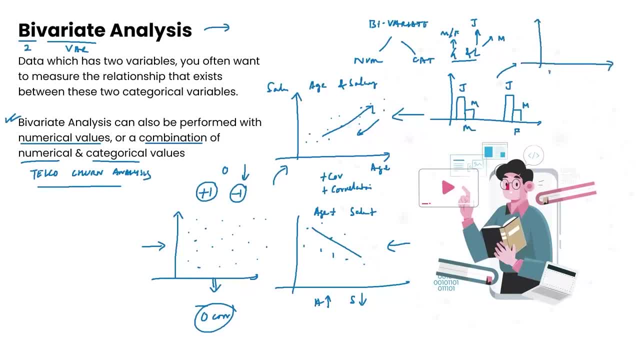 same graph i will do for the churned customers: male, female, japan, malaysia, japan, malaysia. now, if you see a graph like this, it is quite evident that the females who are staying in malaysia are more likely to churn. why we don't know, but this is what my insight is telling me. 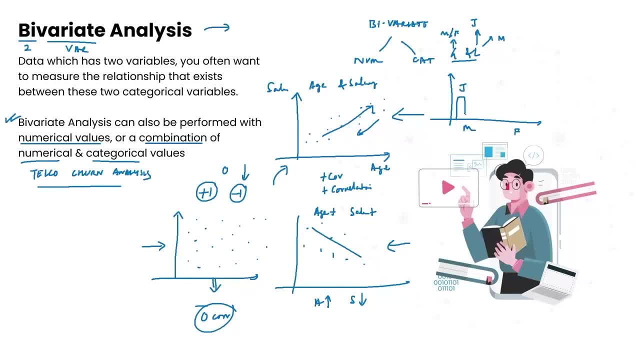 for male and female: japan, malaysia, japan, malaysia. that means most of the people are from japan and less people from malaysia. same graph i will do for the churned customers: male, female, japan, malaysia, japan, malaysia. now, if you see a graph like this, it is quite evident that the females who are staying 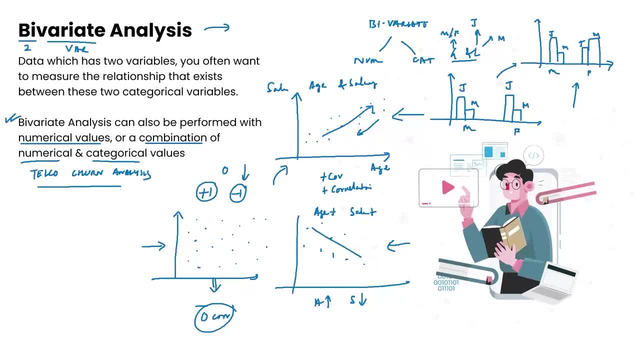 in malaysia are more likely to churn. why we don't know, but this is what my insight is telling me. and a similar technique has to be done for a combination of numerical and categorical. let's say you are analyzing age and gender. you first analyze on the original data. let's say for 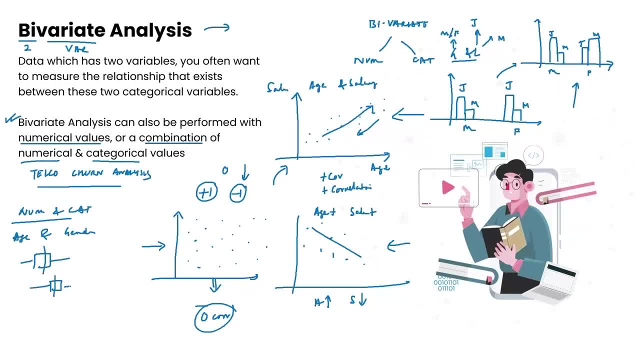 male customers. how does my box plot looks like for female customers? how does my box plot looks like? and same you do for the churn customers and you identify the difference. you can also make use of some different other type of charts to understand, but the concept remains the same: that bivariate analysis is done with two variables. it could be two numerical, two categorical. 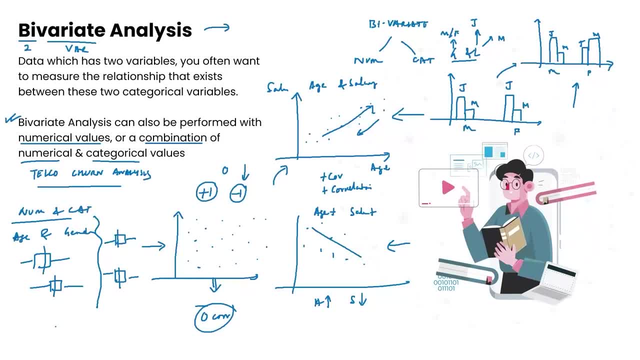 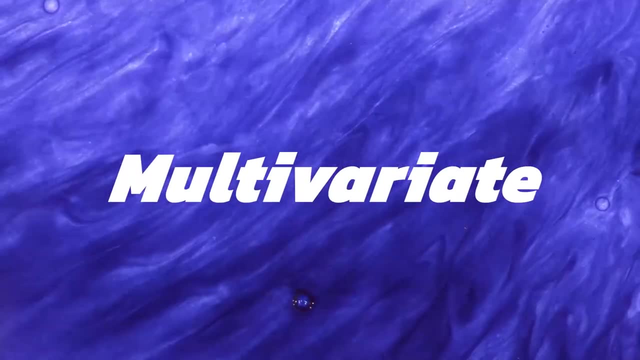 or a combination of numerical and categorical analysis. that's all about bivariate analysis. in the next video we shall be talking more about numerical analysis and what could be done in the numerical analysis part. so once again, the worked out can be used for many different kinds of averaged data. 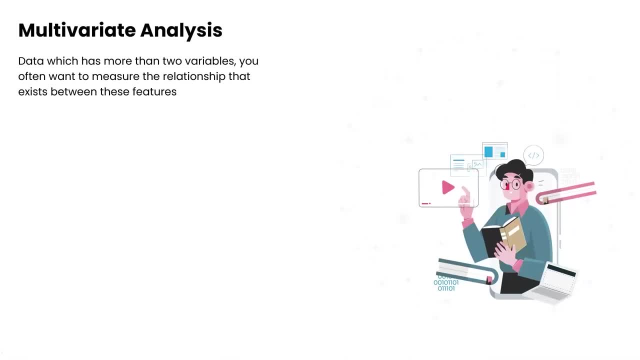 but let's first talk about bivariate and other responses. the next thing that i'm going to discuss is multi-variant analysis. the next thing that i'm going to discuss is multivariate analysis. again, the concept here remains the same: the more deep dive you are trying to do with your data. 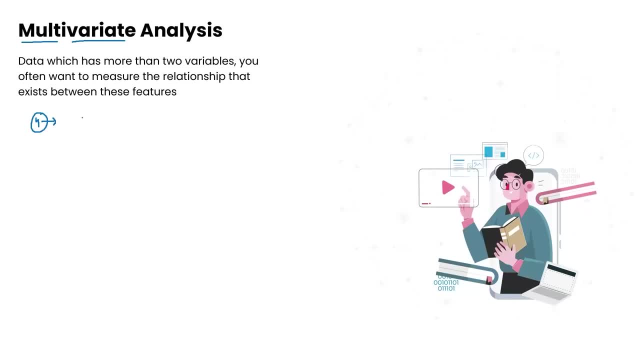 the more features you analyze, the more insights you get. the graph will be very complex to understand. the analysis itself will be very complex, but you could end up getting more insights when you go into the multivariate area. hence, EDA is performed based on your requirements. if you have a specific given time to finish EDA and get insights, you could. 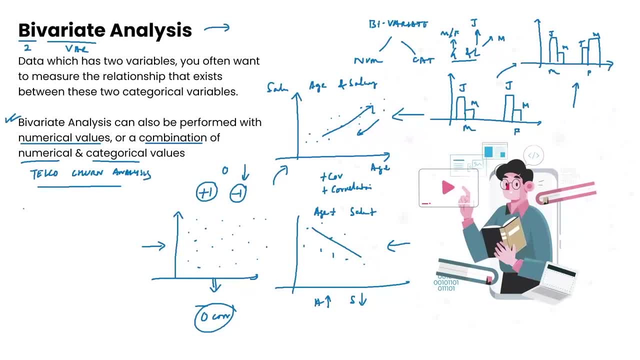 and a similar technique has to be done for a combination of numerical and categorical. let's say you are analyzing age and gender. you first analyze on the original data. let's say: for male customers, how does my box plot looks like? for female customers, how does my box plot looks like? and same you do for the churn customers. 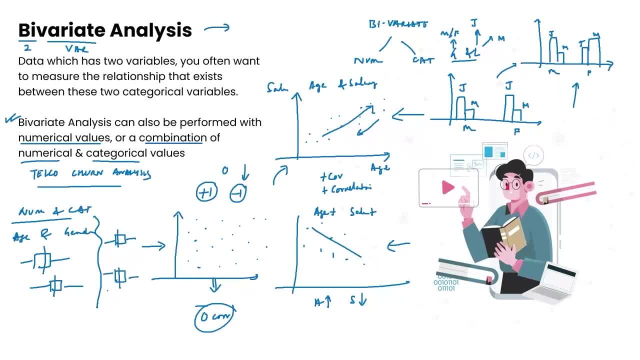 and you identify the difference. you can also make use of some different other type of charts to understand, but the concept remains the same: that bivariate analysis is done with two variables. it could be two numerical, two categorical or a combination of numerical and categorical analysis. that's all about bivariate. 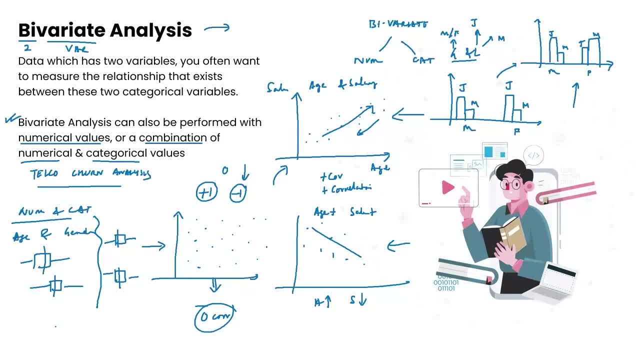 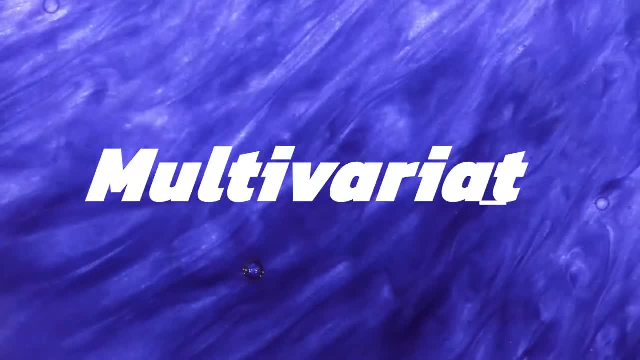 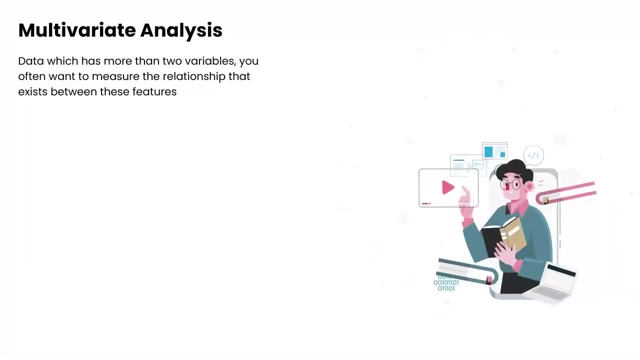 bivariate analysis. in the next video we shall be talking more about numerical analysis and what could be done in the numerical analysis. the next thing that i'm going to discuss is multivariate analysis. again, the concept here remains the same: the more deep dive you are trying to do with your data, the more features you analyze. 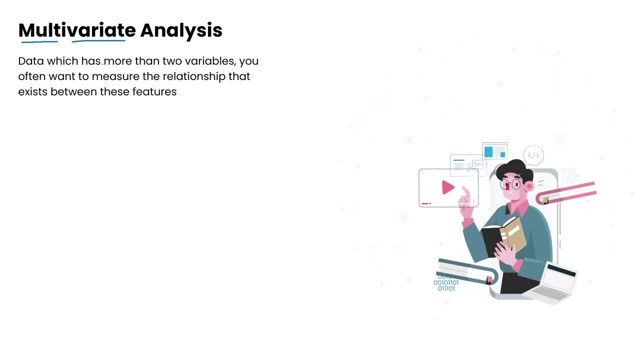 network of interactions. esse admitted to, yourков continue to work with you and the more insights you get. so multi means multiple and variate means variable. let's see you're analyzing four columns, four categorical columns. obviously the graph will be very complex to understand the analysis itself. 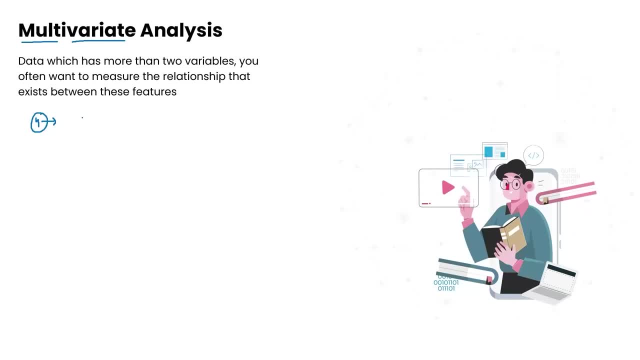 will be very complex, but you could end up getting more insights when you go into the multivariate area. hence eda is performed based on your requirements. if you have a specific given to finish eda and get insights, you could probably skip multivariate analysis. but if you have enough, 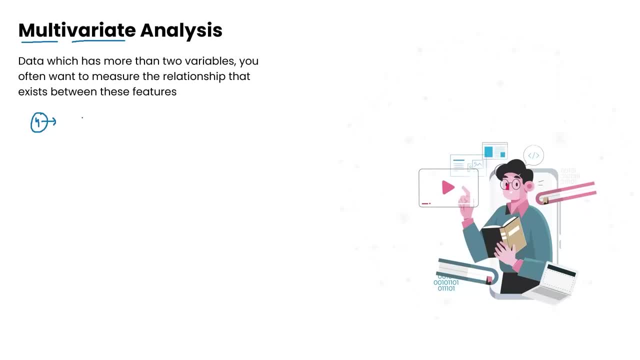 time for your analysis process. you can jump from univariate, bivariate to multivariate, so three variable, four variable, and the more variables you analyze it becomes more and more complex, but it will be fruitful. so, in simple terms, multivariate analysis is kind of analysis where more than two 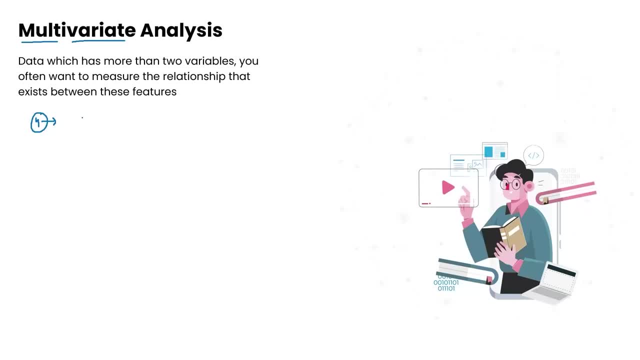 probably skip multivariate analysis. but if you have enough time for your analysis process, you can jump from univariate, bivariate to multivariate. so three variable, four variable, and the more variables you analyze it becomes more and more complex, but it will be fruitful. so in simple terms, 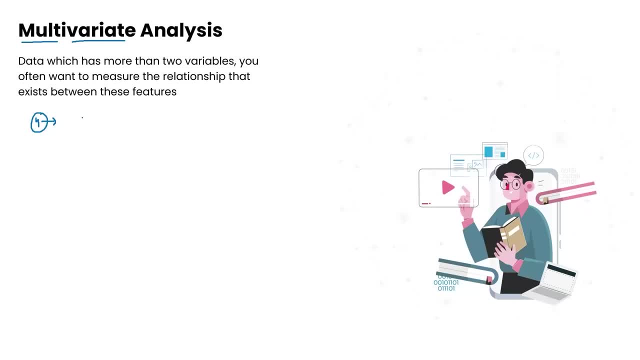 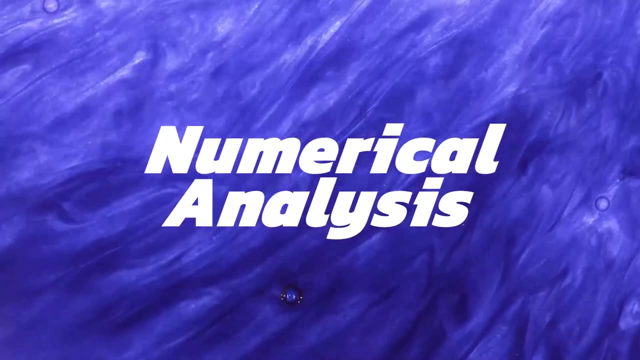 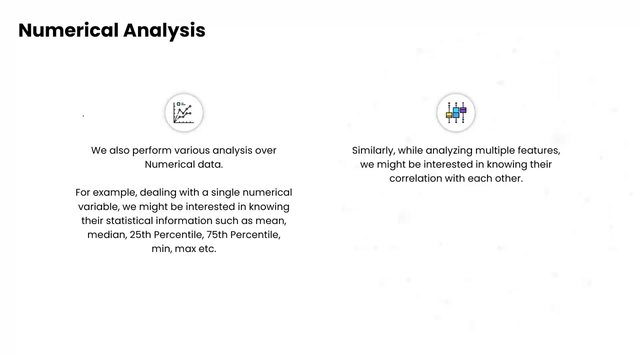 multivariate analysis is kind of analysis where more than two variables are involved. again, this could be a combination of categorical, numerical, only categorical or only numerical attributes. in this video we shall be focusing on the numerical analysis part. we all covered bivariate, univariate and multivariate. somehow numerical analysis was already covered there, but let's try. 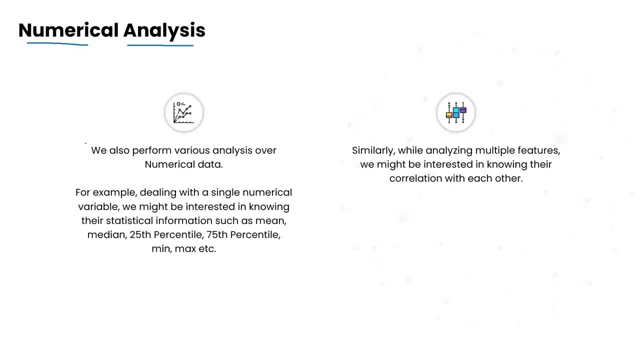 to discuss. what extra do we do when it comes to the numerical data? we also perform various analysis over numerical data. so, for example, dealing with a single numerical variable, we might be interested in knowing the statistical information, such as mean, median, 25th percentile, 75th percentile, minimum, maximum, etc. and 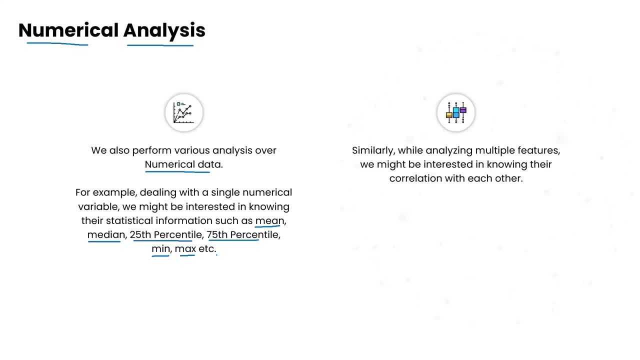 when you are dealing with more variables, you might be interested in knowing how these variables are related to each other, whether they are positively correlated, negatively correlated or they are not correlated. so when it comes to numerical data analysis, we also perform multiple types of analysis. one could be a box plot symbolizing a single variable analysis, where you are analyzing just one single. 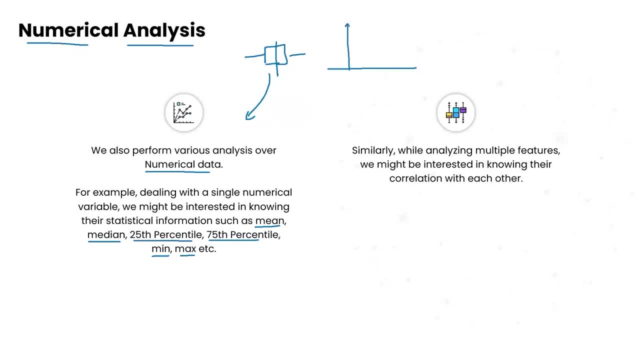 numerical attribute. when you are analyzing multiple numerical attributes, you could use a scatter plot to understand the correlation between these variables. there is another thing that we also do, which is again finding the correlation. but imagine you have a data set where there are hundreds of numerical columns, hundreds of numerical columns. is it feasible to plot scatter plots for each and every combination? 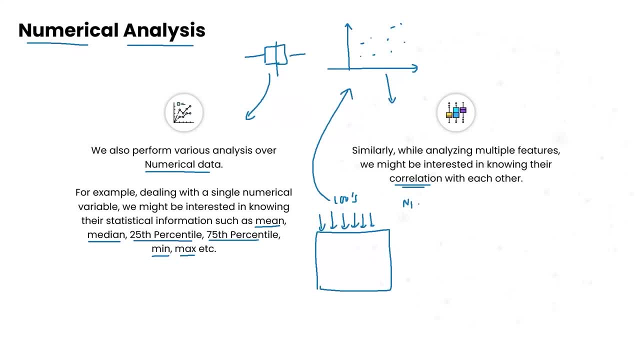 of numerical attributes. let's say numerical attribute one with two, you plot one graph, one with three, one with four, one with five, one with six. imagine how many scatter plots you will end up by analyzing the total number of numerical sigma elements within a Y axis. here for so. 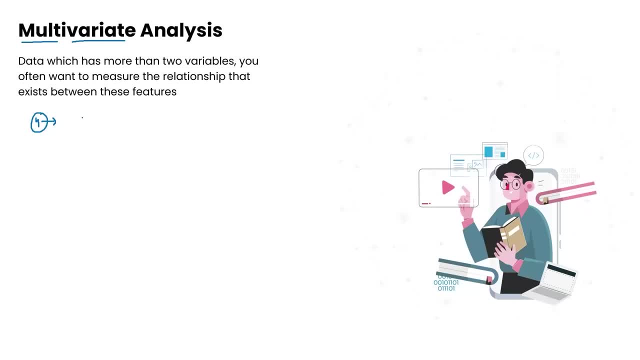 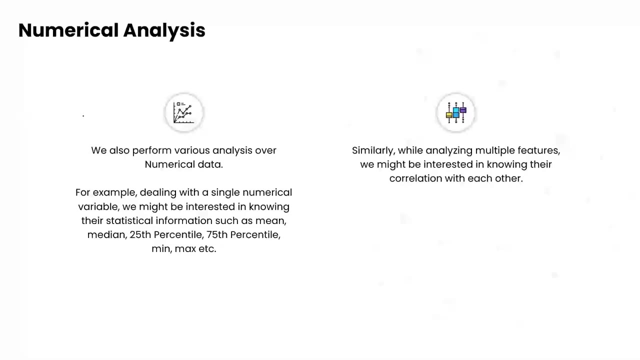 variables are involved again. this could be a combination of categorical, numerical, only categorical or only numerical attributes. in this video we shall be focusing on the numerical analysis part. we all covered bivariate, univariate and multivariate. somehow numerical analysis was already covered in our last part of today's video. now we shall start with the numeric analysis. 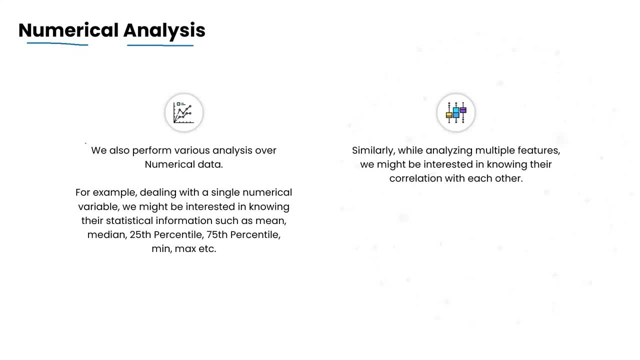 covered there, but let's try to discuss. what extra do we do when it comes to the numerical data? we also perform various analysis over numerical data. for example, dealing with a single numerical variable, we might be interested in knowing the statistical information, such as mean median, 25th percentile, 75th percentile, minimum, maximum, etc. and when you are dealing. 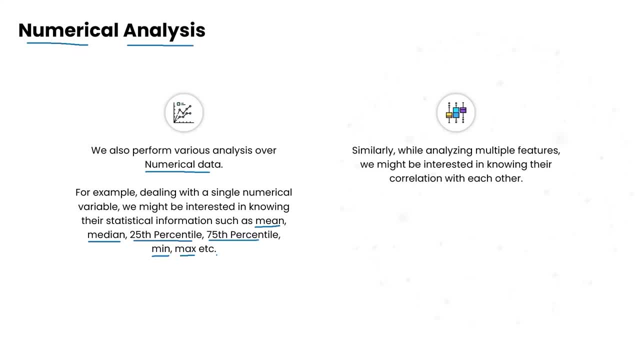 with more variables, you might be interested in knowing how these variables are related to each other, whether they are positively correlated, negatively correlated or they are not correlated. so, when it comes to numerical data analysis, we also perform multiple types of analysis. one could be a box plot symbolizing a single variable analysis where you are analyzing. 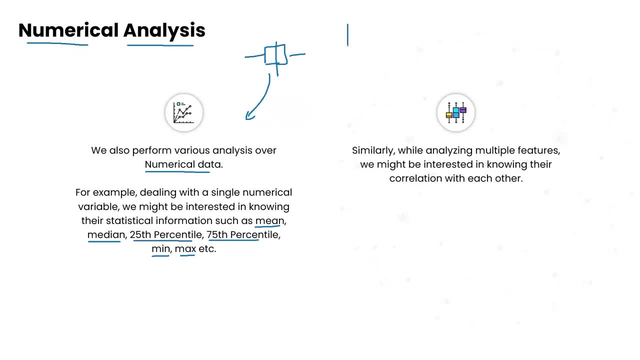 just one single numerical attribute. when you are analyzing multiple numerical attributes, you could use a scatter plot to understand the correlation between these variables. there is another thing that we also do, which is again finding the correlation. but imagine you have a data set where there are hundreds of numerical columns. 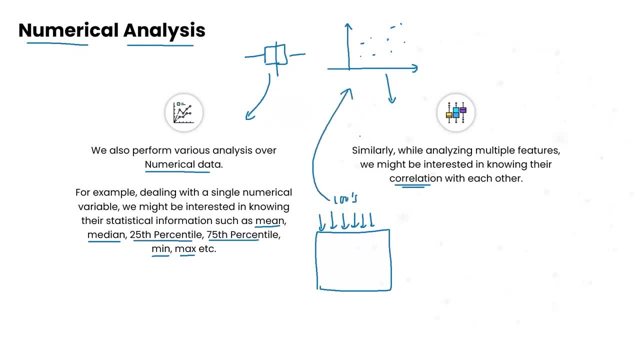 hundreds of numerical columns. is it feasible to plot scatter plots for each and every combination of numerical attributes? let's say, numerical attribute one with two, you plot one graph. one with three, one with four, one with five, one with six. imagine how many scatter plots you will end up. so, instead of doing scatter plots for each and every numerical attribute, 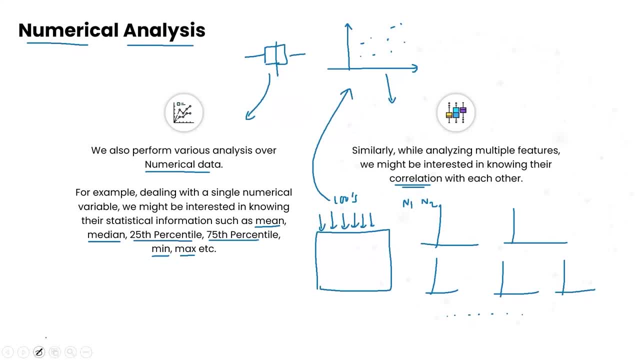 with each other. a better way of handling this kind of data will be using the corr function, which is a part of the data set, so that you can understand the correlation between these data set. so let's say the corp is a part of pandas data frames when you are using the data. 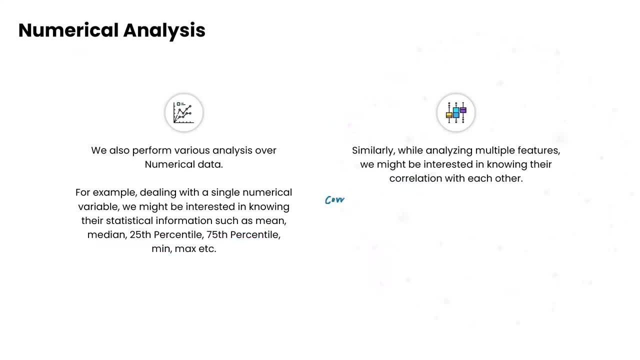 so, instead of doing scatter plots for each and every numerical attribute with each other, a better way of handling this kind of data will be using the sentenced function, which is a part of pandas. when you are using the date, you can simply call the correlation function and you can plot it using a heat plot hitman. 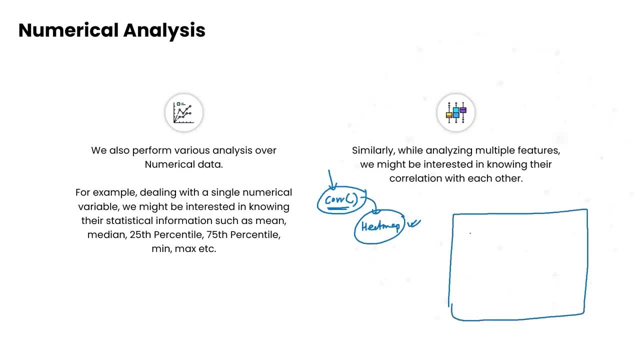 you will end up getting a graph like this, which is your 100 variable cross 100 variable map: variable 1: variable 2 dot dot dot. variable 100. variable 1: variable 2 dot dot dot. variable 100. and this heat map will tell you or will give you an idea of which variables are having positive. 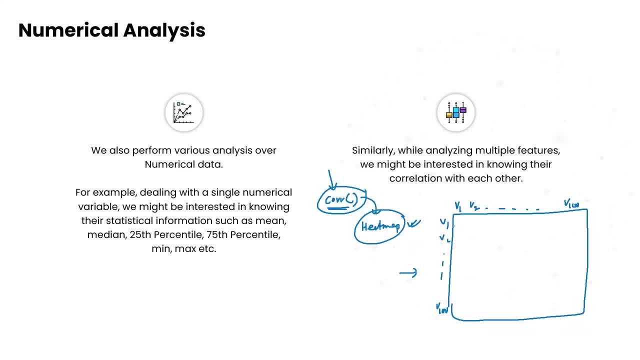 or negative correlation with each other. let's say this is a grid, this is a matrix like this. now imagine this box is having some dark color, which potentially means, from the scale that you identified, that this is having a positive correlation, so you can easily spot that variable. 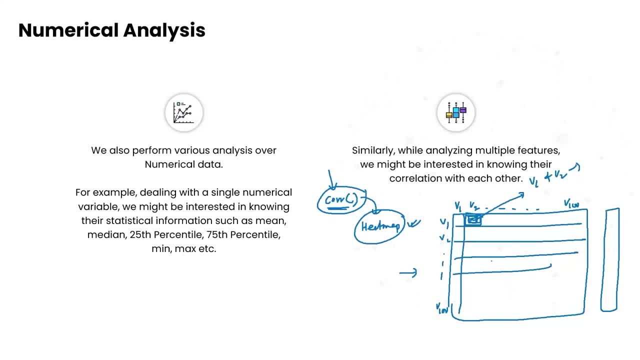 1 and variable 2 are positively correlated. let's say, this particular value is very light shade, somewhere close to minus 1, which clearly means that variable 50 and variable 2 are negatively correlated. so using the grid, using the color grid, you will be able to identify correlation between multiple. 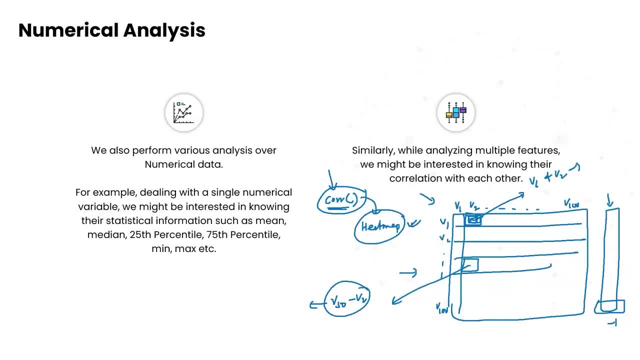 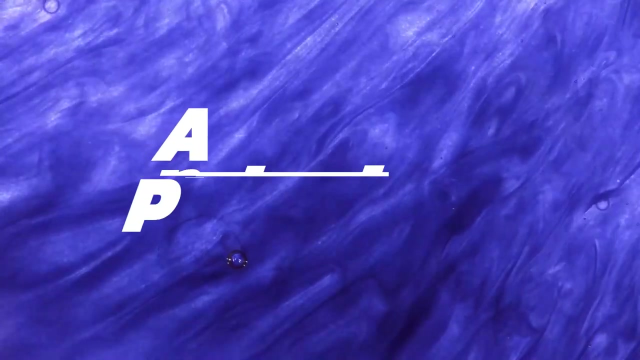 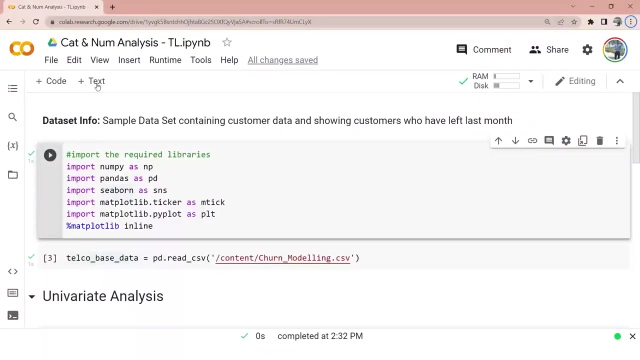 numerical attributes. apart from this, we also perform multiple other types of numerical analysis, which includes kernel density estimation plots, histogram plots and multiple other plots. so once we jump into the practicals, i will show you, using a demo data, on how do we perform different types of analysis. let's jump into the coding part to understand more about how to perform different. 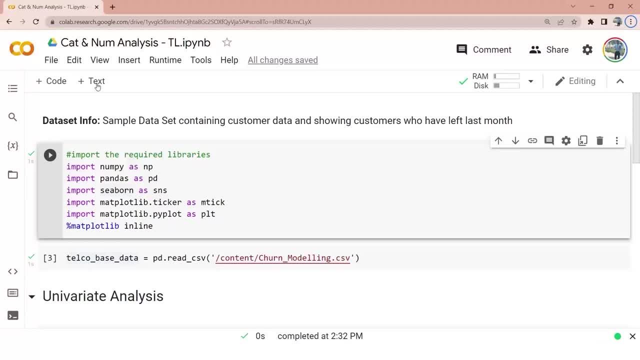 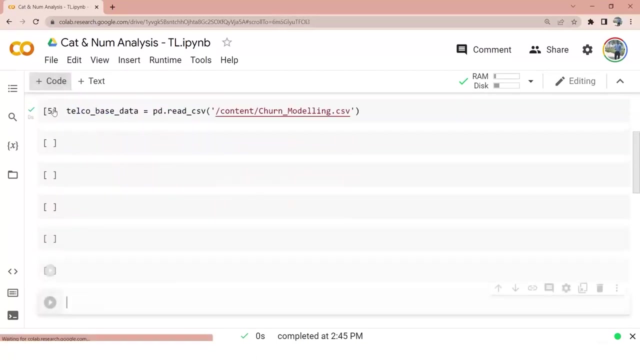 types of analysis, be it univariate, bivariate or numerical analysis. so for this particular exercise, i am going to import all the required libraries and then i have already uploaded the same churn modelingcsv file, so i'm going to fetch that using the pandasread csv. how does my data set looks like? that's how my data set looks like. 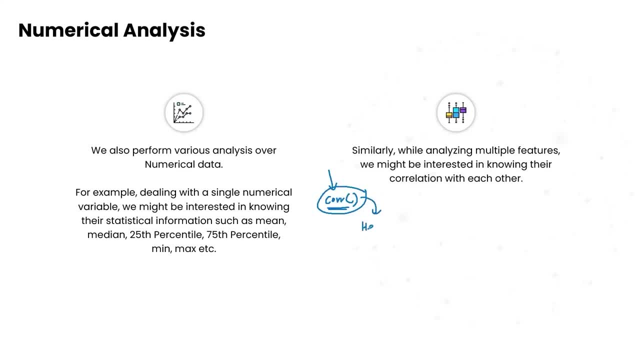 you can simply call the correlation function and you can plot it using a heat plot, heat map. when you plot it using a heat map, you will end up getting a graph like this, which is your hundred variable, cross, hundred variable map variable, one variable, two, dot dot dot variable. 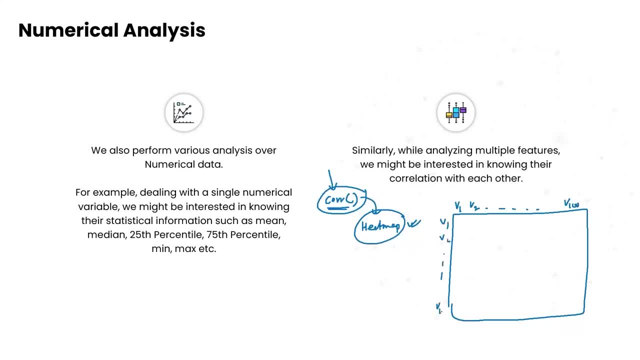 hundred variable one variable two, dot dot variable hundred. and this heat map will tell you, or will give you an idea of which variables are having positive or negative correlation with each other. Let's say: this is a grid, this is a matrix like this: Now imagine: 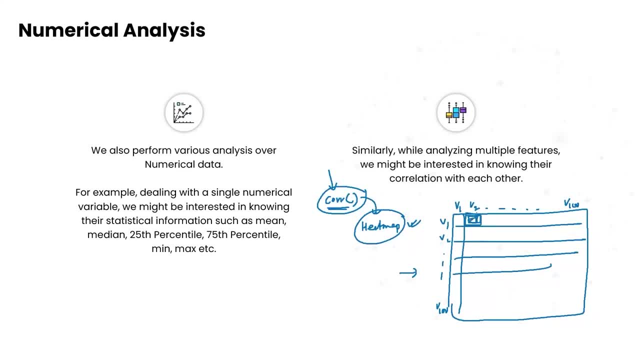 this box is having some dark color, which potentially means, from the scale that you identified, that this is having a positive correlation. So you can easily spot that variable 1 and variable 2 are positively correlated. Let's say this particular value is very light shade, somewhere close to minus 1, which clearly means that variable 50 and variable 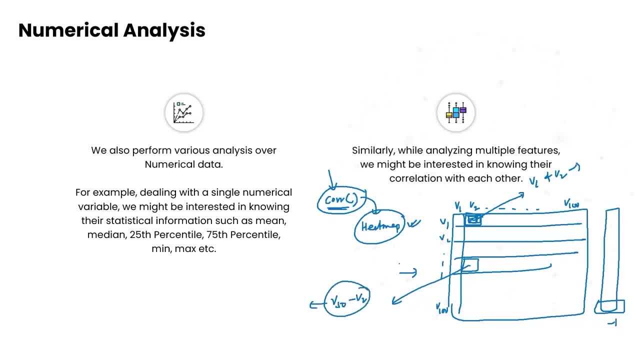 2 are negatively correlated. So using the grid, using the color grid, you will be able to identify correlation between multiple numerical attributes. Apart from this, we also perform multiple other types of numerical analysis, which includes kernel density estimation plots, histogram plots and multiple other plots. So once we jump into the practicals, I will show. 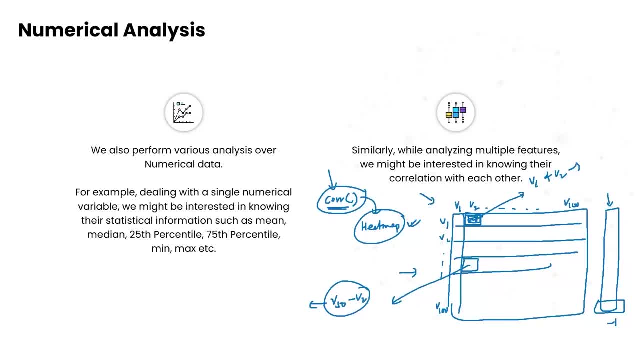 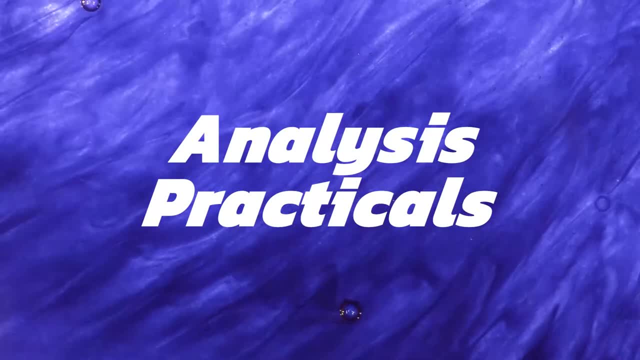 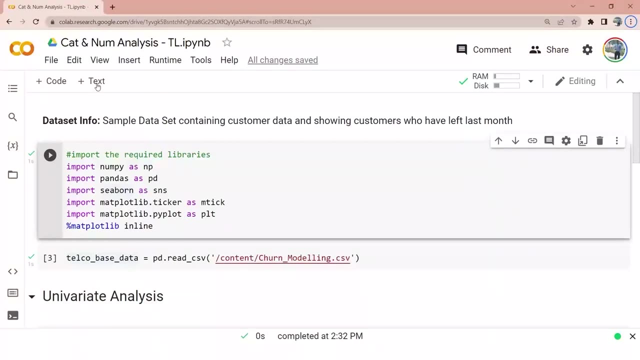 you using a demo data on how do we perform different types of analysis. Let's jump into the coding part to understand the code. So let's first understand more about how to perform different types of analysis, be it univariate, bivariate or numerical analysis. So for this particular exercise, I'm going to import all the 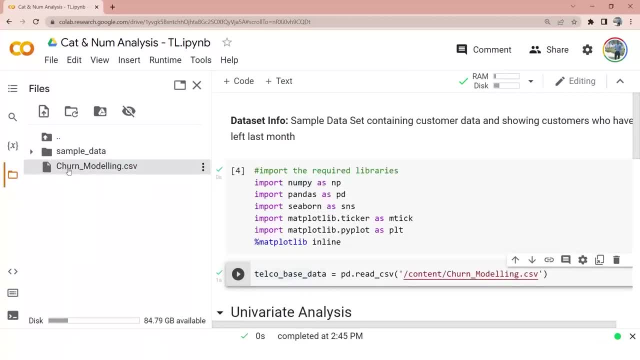 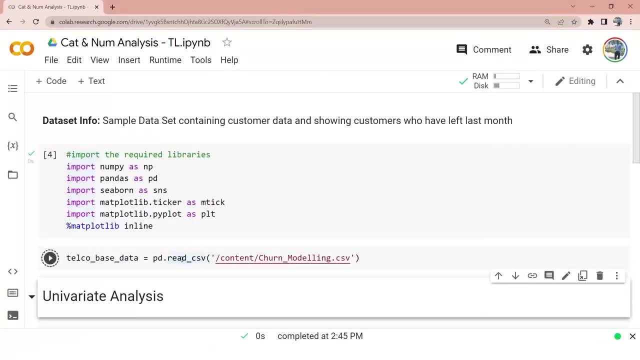 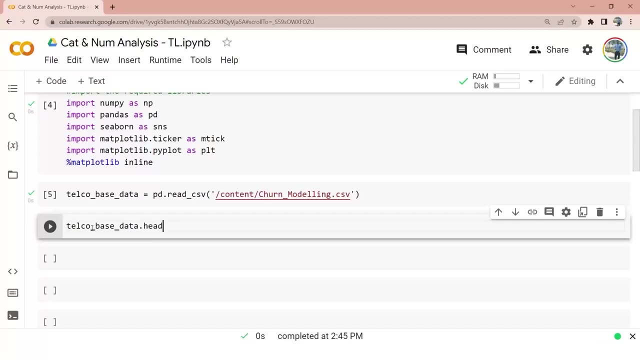 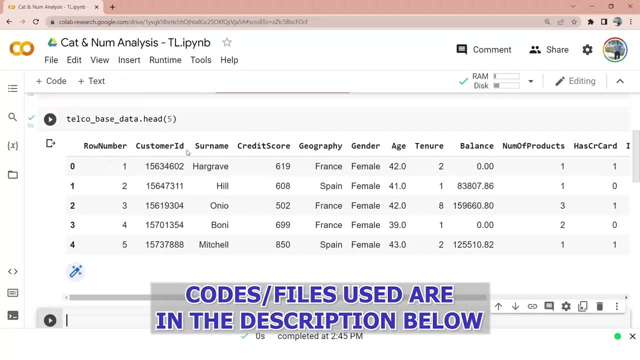 required libraries. And then I have already uploaded the same churn modelingcsv file, So I'm going to fetch that using the pandasreadcsv. How does my data set looks like? I have columns like row number, customer id, surname, credit score, and there is a column called 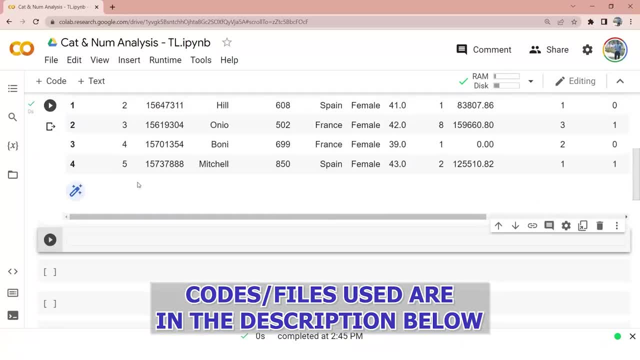 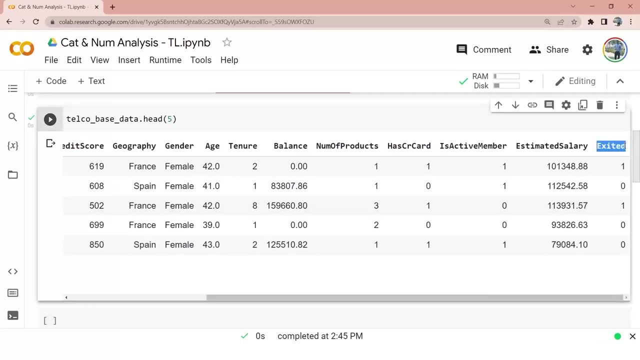 i have columns like row number, customer id, surname, credit score, blah, blah, blah, and there is a column, column, column, a column called as exited, which basically tells whether the customer has left the company or is still in the company. one means this customer has exited, he or she is a churned customer and zero. 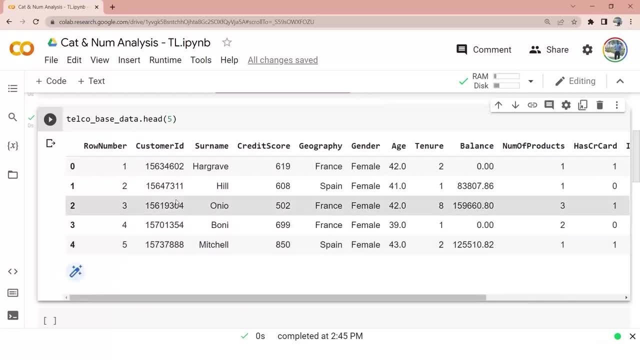 means they are still active. your target as part of eda is to understand what is the characteristics of the people that have churned and probably why, but in this particular exercise we will be talking about these details in detail, which is also covered in the next video, so i hope you guys have enough time to. 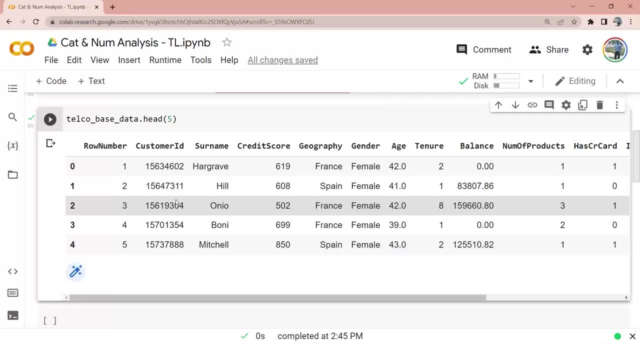 invest in your own data. so in this particular video, we will be majorly focusing on the different types of analysis using python. once we cover this, once we jump into the actual eda case study, where we will be taking the exact same data set, i will be explaining you the entire analysis activities. 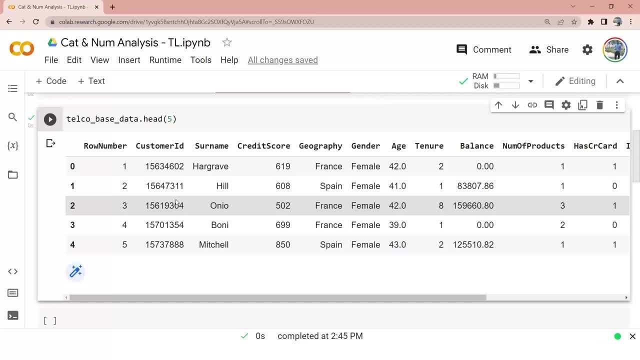 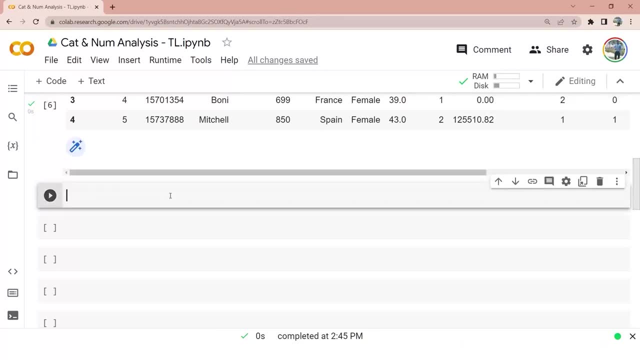 starting from step number one till the end, and i will also show you how insights are fetched. so in this particular video we will just be focusing on the university bivariate and the準 variate and the numerical analysis. so firstly, i will only take some of these new categorical columns. 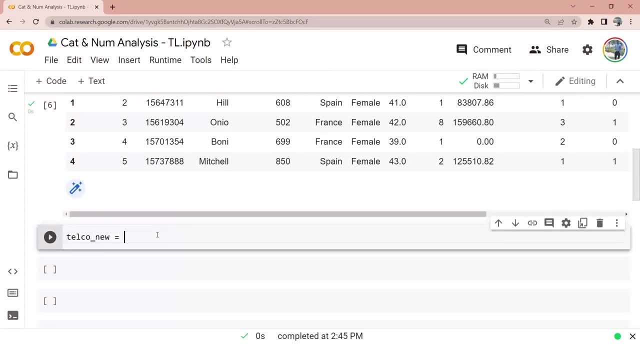 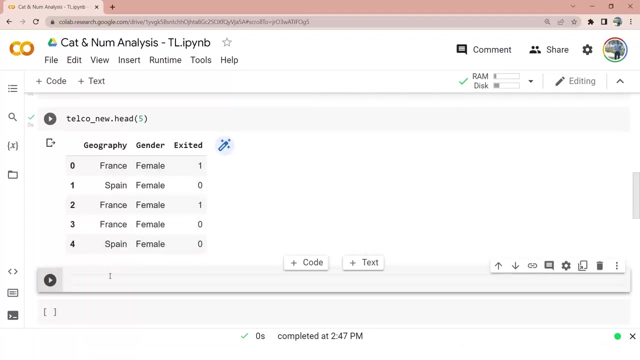 and i will create a new data frame- so telco new equals to telco base data- and then i will just choose geography and gender and exited column done if you want to see how your telco new looks like. it looks like this, okay. so firstly i will be starting with a count plot. i will be using a 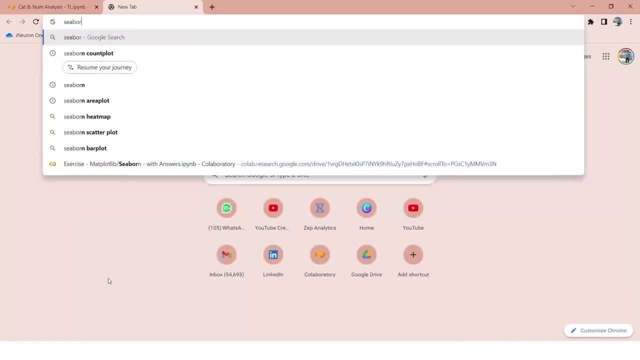 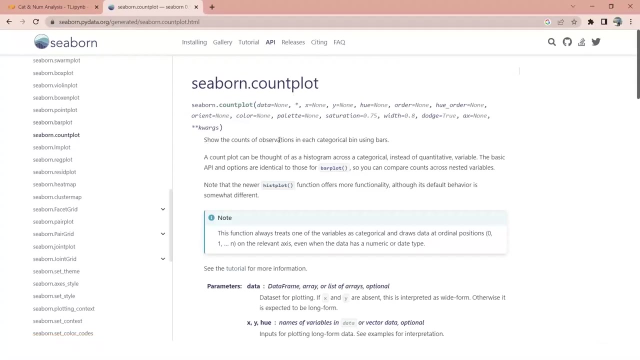 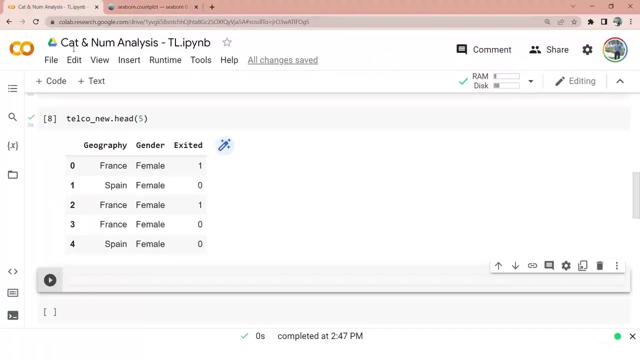 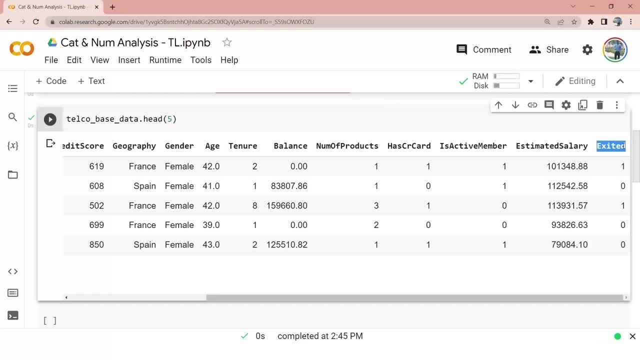 as exited, which tells whether the customer has left the company or is still in the company. One means this customer has exited, HE or SHE is a churned customer, and zero means that you can set to zero. Anyone can set the highest value to 0, even if their company is still active. You can turn off lenses while you are in the company or our tasks by selecting to change individuals as less дан. martyrs include those who have abandoned the company. A colon storied: calculate the total number of customers. our customer that has left term huh. 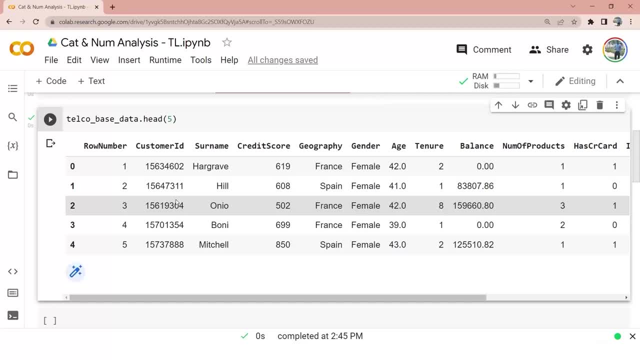 like 15, and then two columns thatcoat out to see whether customers have turned active. if the target as part of eda is to understand what is the characteristics of the people that have churned and probably why, but in this particular exercise we will be majorly focusing on the 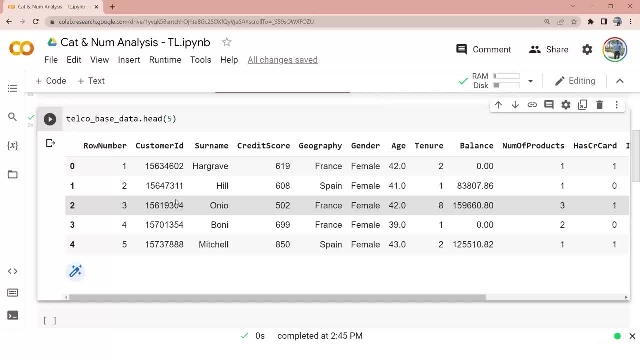 different types of analysis using python. once we cover this, once we jump into the actual eda case study, where we will be taking the exact same data set, i will be explaining you the entire analysis activities, starting from step number one till the end, and i will also show you how insights 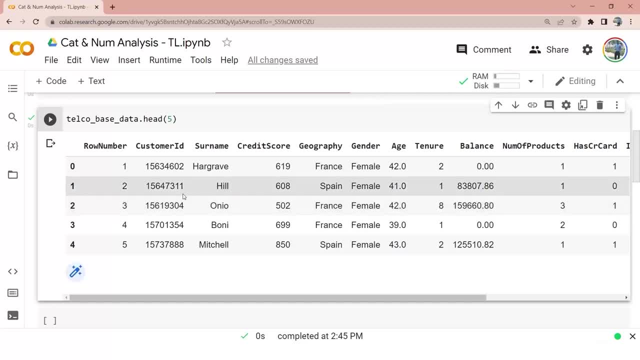 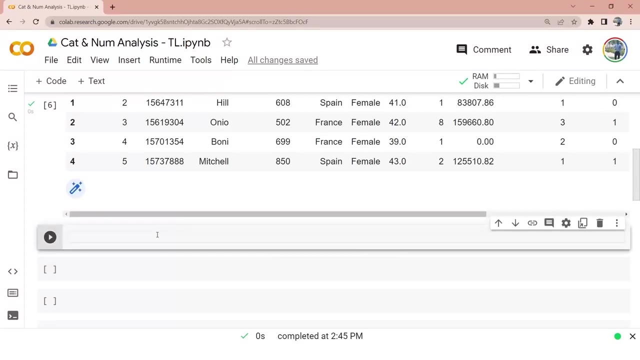 are fetched. so in this particular video we will just be focusing on the univariate bivariate and the numerical analysis. so firstly i will only take some of these new categorical columns and i will create a new data frame. so telco new equals to telco base data. 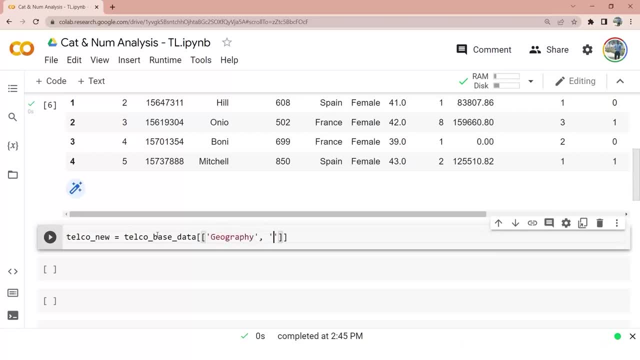 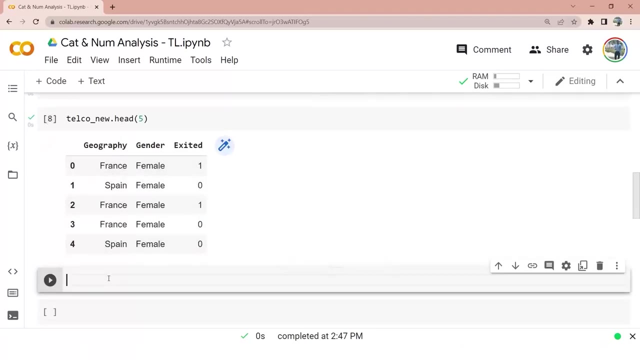 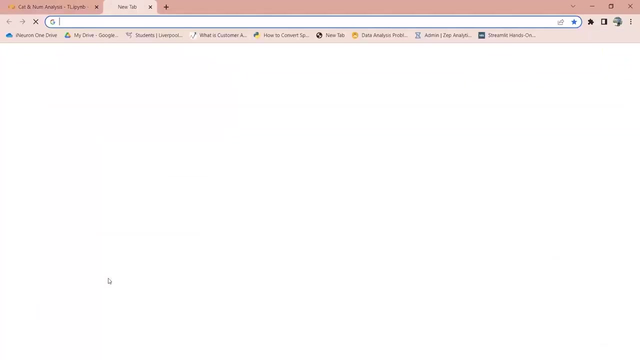 and then i will just choose geography and gender and exited column done. if you want to see how your telco new looks like, it looks like this, okay. so firstly, i will be starting with a count plot. i will be using a count plot which is a seaborn- seaborn count plot. i'll be using this: what is? 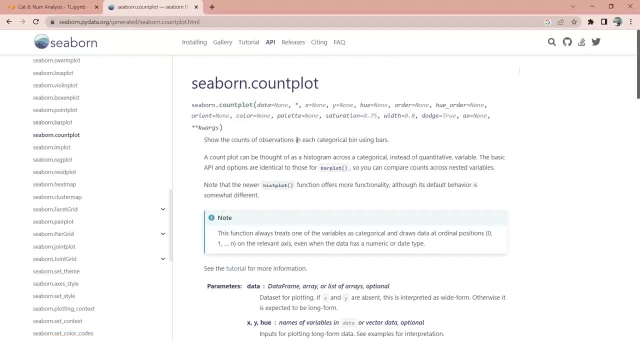 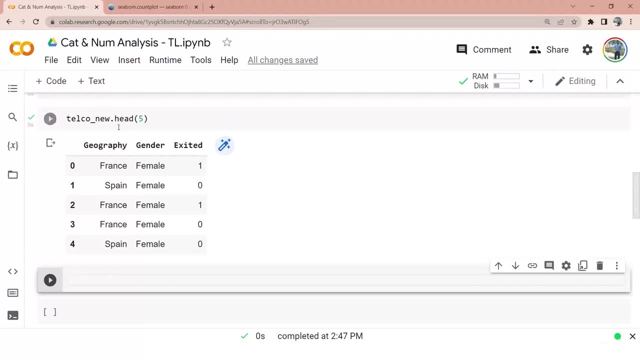 the count plot shows the counts of observation in each categorical bin using bars. it's up to you how you want to visualize it. you can use a simple bar chart. you can use any any libraries bar chart. in my case, i am just using account plot, so what i will do here is 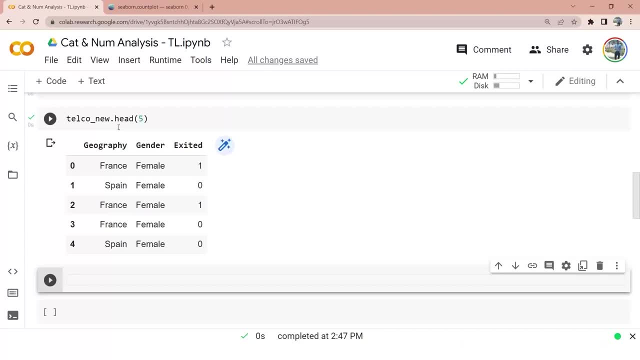 you can use any any libraries bar chart. in my case i'm just using a count plot, so what i will do here is i will write a for loop for i predictor in. i'll probably explain this code after writing it. columns equals to, let's say, i want to just skip my exited column. 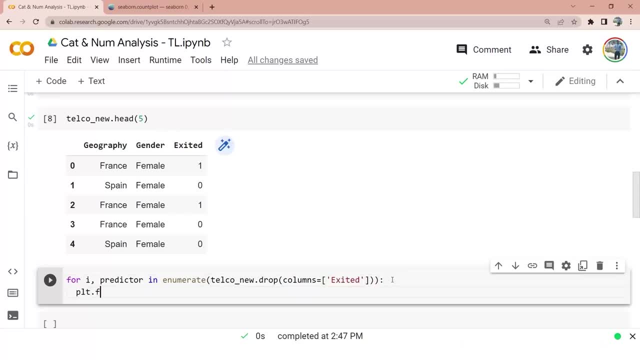 and then plt dot figure and then t-bond dot count plot. here i will pass my data. what is my data? telco new? x equals to predictor, which is what i am passing here and my. there will be a hue of exited. you can see in my data telco new i have three columns. 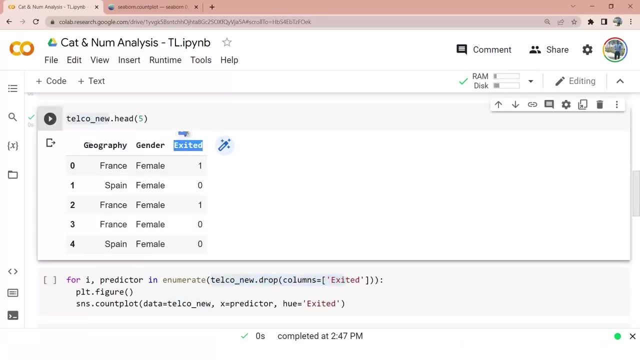 so here i'm dropping exited column and i'm only taking these two columns, so i'll be, i'll be running through a loop over these two columns and i will be plotting the count plot of the telco data, where x is my predictor. let's say, first time the predictor will be geography and the second 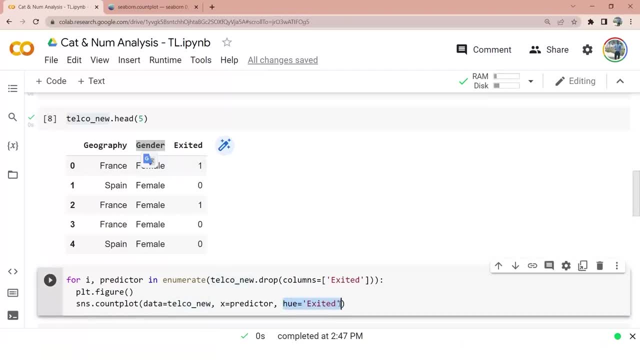 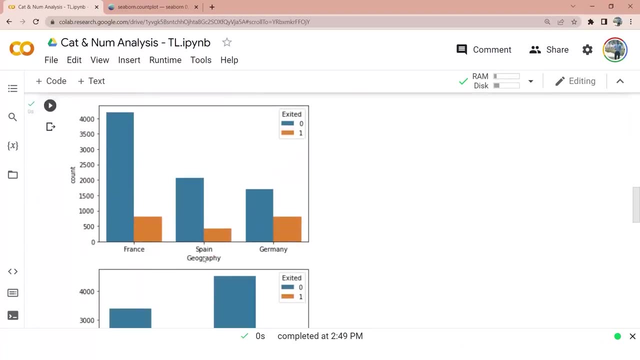 time, my predictor will be gender and i'm using a hue for exited. so if you run this, you will be getting two graphs, because there are two columns: one is geography and one is gender. now what do you interpret from this particular graph? the geography graph you can see for france, people who have left are around 800, see you. 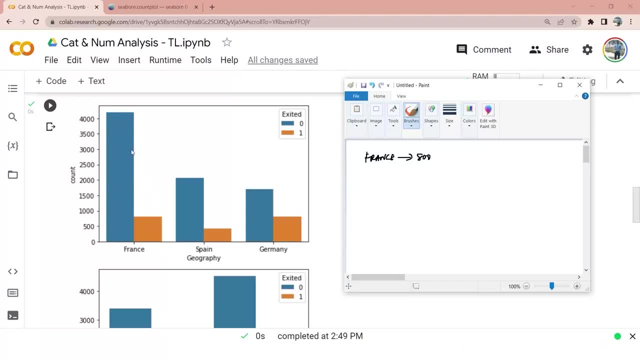 can also plot the labels, in case you want to have a further analysis. i'm just visually taking some inputs. let's say the churned customers are somewhere around 800. so let's say the churned customers are somewhere around 800. so let's say the 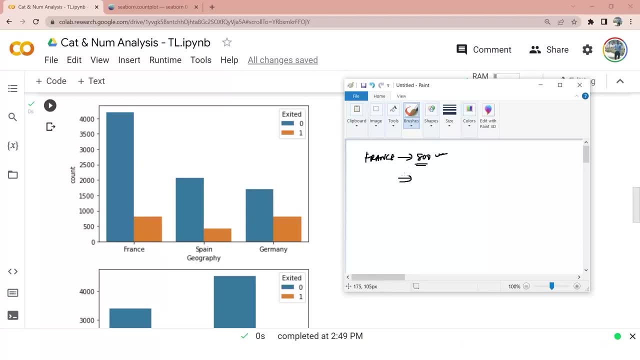 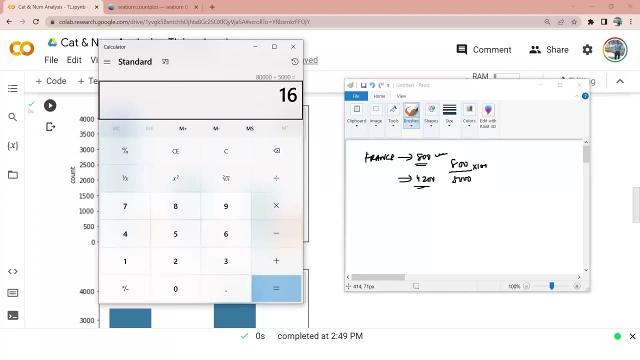 churned customers are somewhere around 800 and the non-churned are somewhere around 4200, right? so what is the ratio of churned 800 by 5000- almost in 200, which is 800, into 100 divided by 5000, which is around 16 percent. 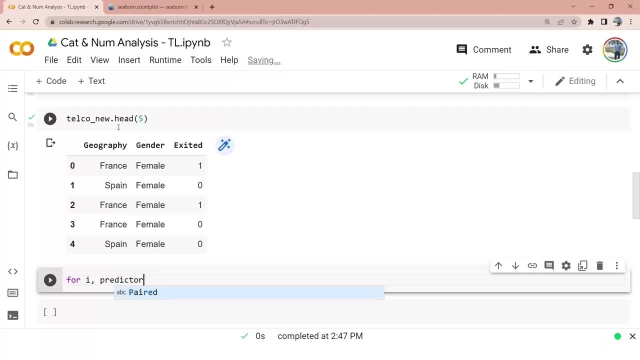 i will write a for loop for i predictor in i'll probably x foi explain this code after writing it. columns equals to: let's say, i want to just skip my exited column and then plt dot figure and then tbon dot count plot. here i will pass. 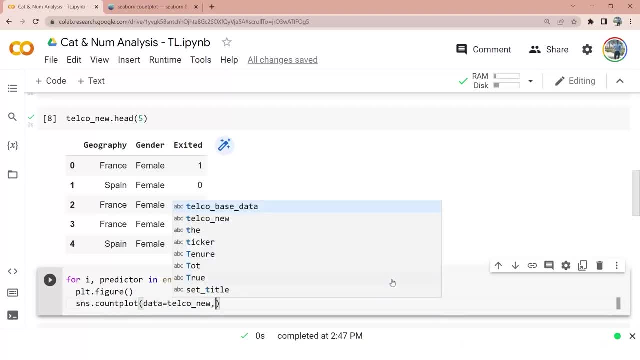 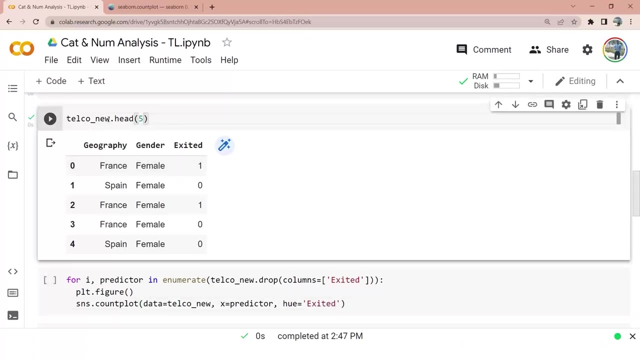 my data. what is my data? telco new: x equals to predictor, which is what i am passing here and my. there will be a hue of exited. you can see in my data telco new, i have three columns. so here i am dropping exited column and i am only taking these two columns, so i will. 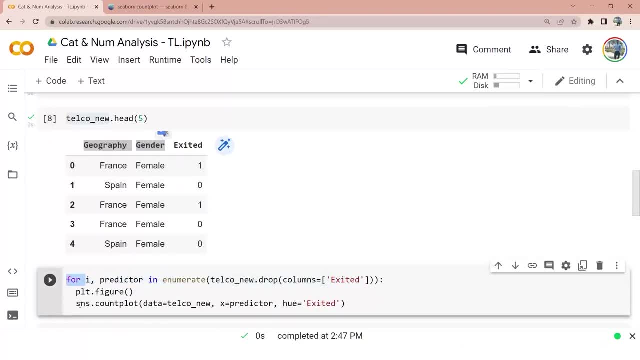 be. i will be running through a loop over these two columns and i will be plotting the count plot of the telco data where x is my predictor. let's say, first time the predictor will be geographic, and then i will be running through a loop over these two columns and i will be 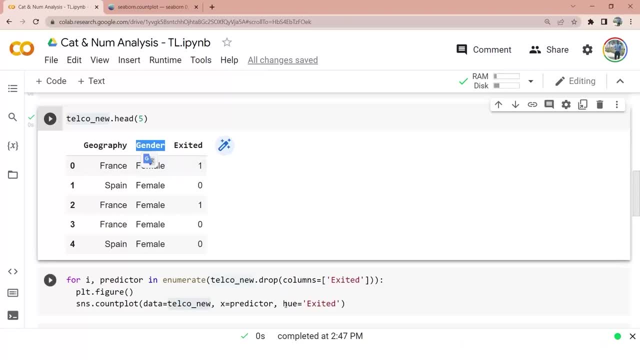 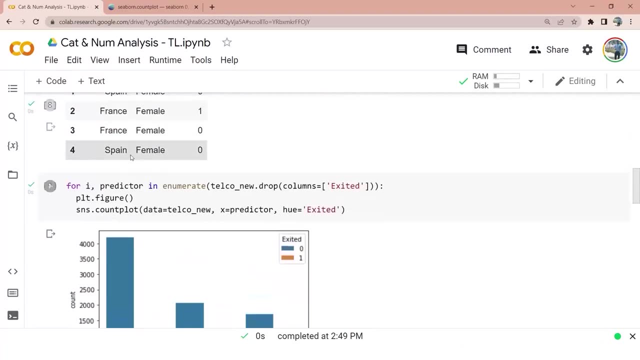 taking the exited column, and then the second time my predictor will be gender, and i am using a hue for exited. so if you run this, you will be getting two graphs, because there are two columns: one is geography and one is gender. now what do you interpret from this? 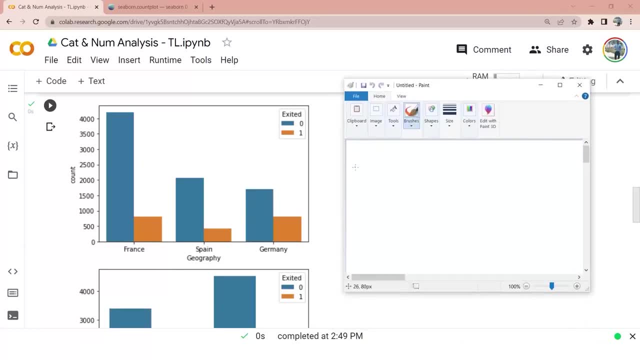 particular graph, the geography graph you can see for france, people who have left are around 800. see, you can also plot the labels in case you want to have a further analysis. i'm just visually taking some inputs. let's say, the churned customers are somewhere around 800. 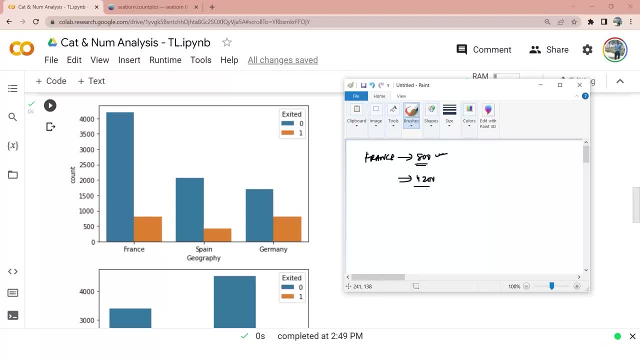 and the nonchurned are somewhere around 4200, right? so what is the ratio of churned? 800 by five thousand, almost in two hundred, which is eight hundred into hundred divided by five thousand, 16%. but in the case of Germany you can see how many churned customers again. 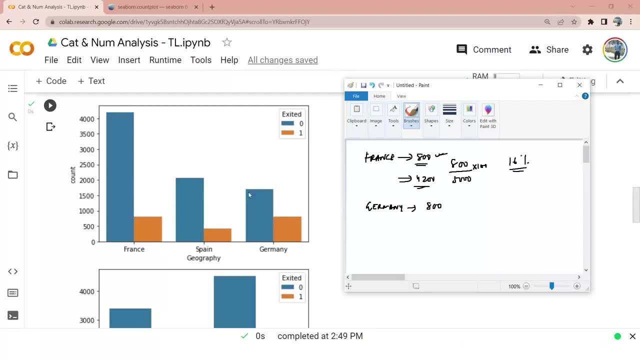 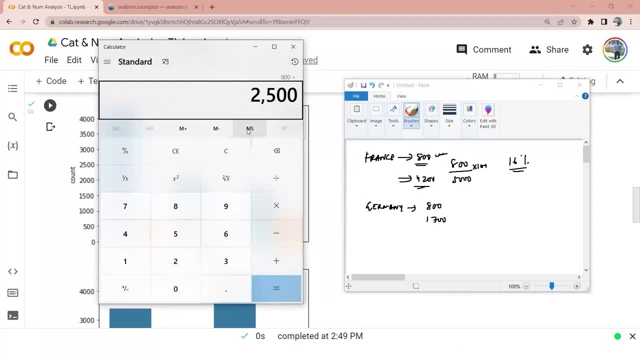 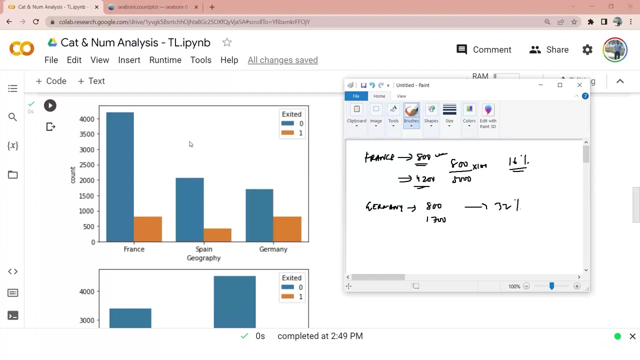 around 800 or 900. how many not churned around 1700 or something. so what is the ratio here? 800 divided by 2500 into 100, my bad 800. 800 divided by 2500 into 100, which is almost 32 percent. what is my original churn ratio? let's try to. 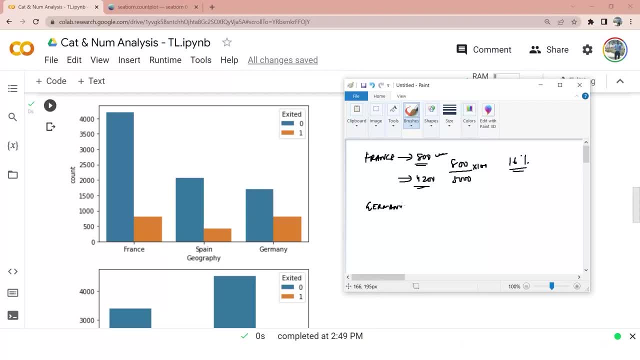 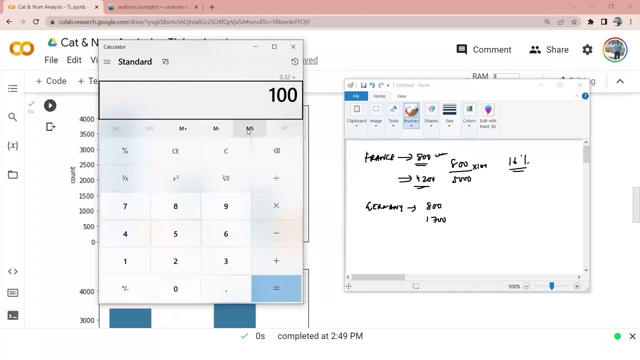 but in the case of germany you can see how many churned customers again around 800 or 900, how many not churned around 1700 or something. so what is the ratio here? 800 divided by 2500 into 100- sorry, my bad 800. 800 divided by 2500 into 100, which is almost 32. 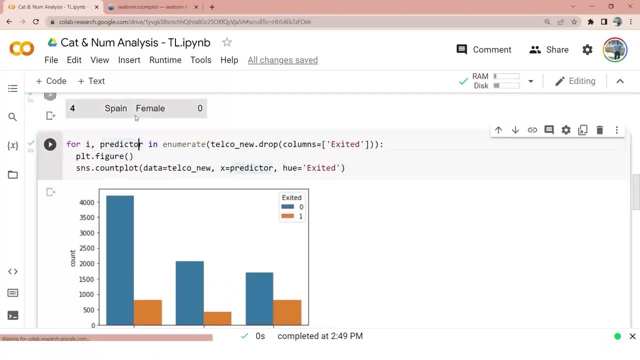 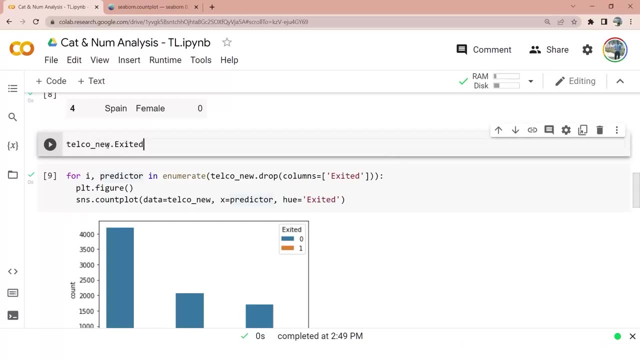 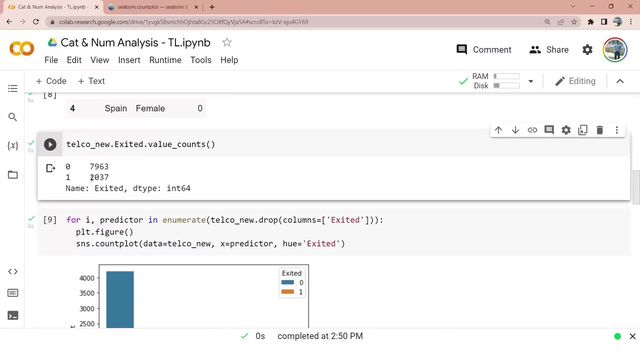 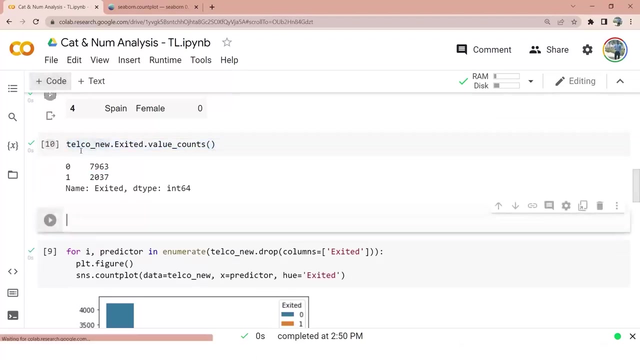 percent. what is my original churn ratio? let's try to check that. so let's say telco new. so let's say telco new dot exited dot value counts. if you do this you will be getting this ratio, which is 8000, is to 2000, so i assume the churn ratio is almost 20. if you want to get the exact ratio, exact percentage, 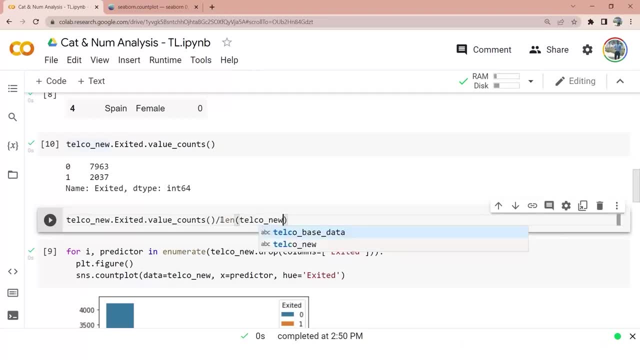 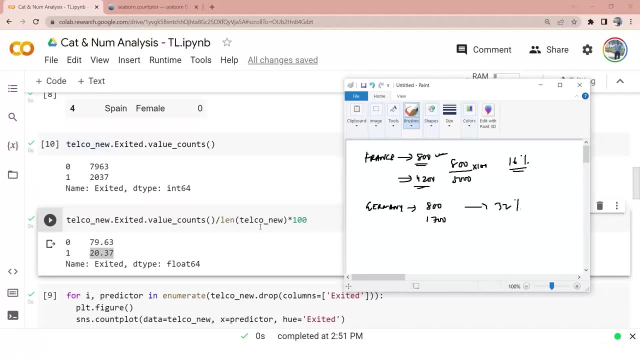 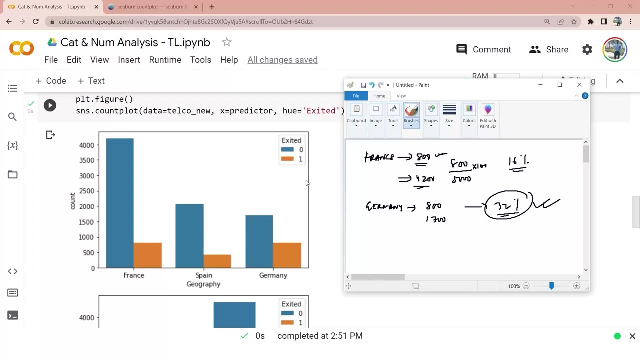 divide it by the total length of telco and then multiply it with 100, you will see that almost 20 percent is your churn rate. but in the case of germany the churn rate is high. so from this univariate analysis i am getting an insight that people staying in germany are. 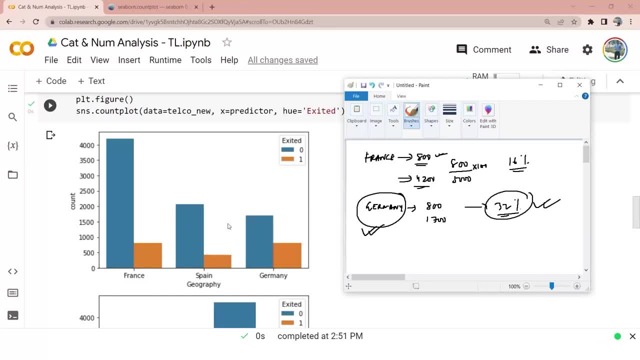 more likely to churn. you can do the same for spain also. univariate analysis, without doing the graphical thing. you can also simply do dot value counts and you can also try to get the insights. but visual analytics is more intuitive, right. it gives you more insights, it helps you understand. 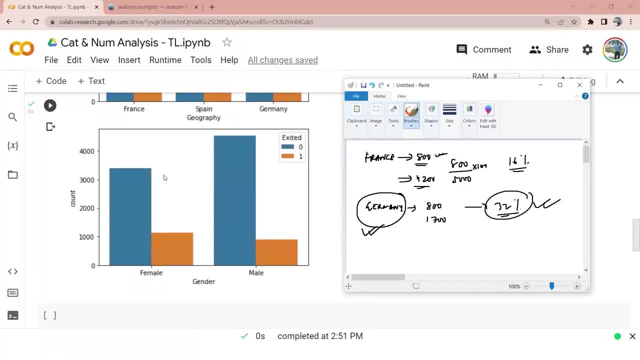 better as compared to just numbers. similarly, from the second graph i would say female are more churners as compared to male. you can see the total number of people in male are high, but the churners are more in female. so one insight here is: female are more. 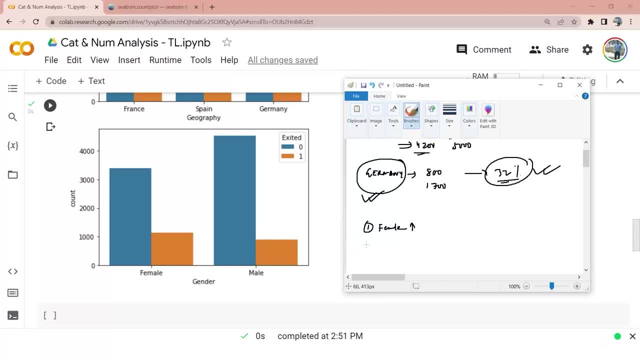 churners. so the second insight that we got is people staying in germany are more churners. these are the two insights that i got from my simple univariate analysis. so in your case you have a data of 100 variables. you have to simply go through each and every graph and you have to 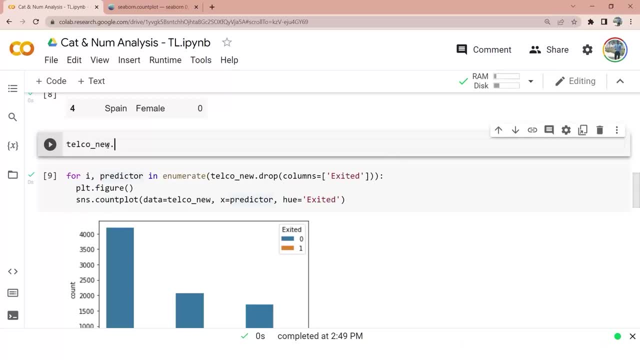 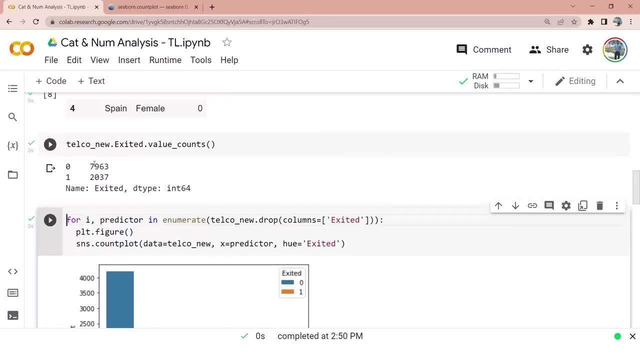 check that. so let's say, telco, new dot, exited dot value counts. if you do this you will be getting this ratio, which is 8000, is to 2000. so I assume the churn ratio is almost 20 percent. if you want to get the exact ratio, exact percentage, 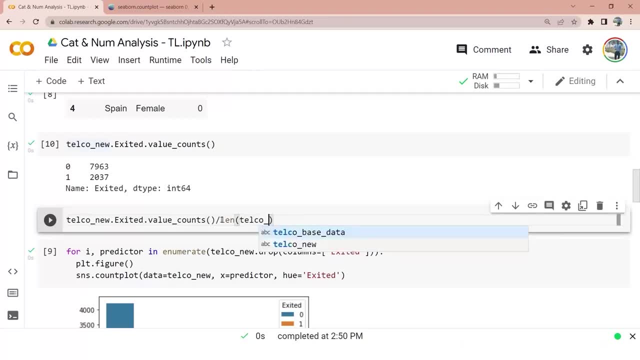 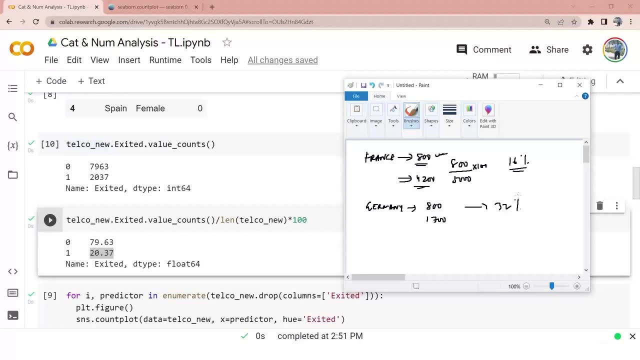 divided by 2000, and then you can see that the churn ratio is almost 20 percent. divide it by the total length of telco and then multiply it with 100, you will see that almost 20 percent is your churn rate. but in the case of Germany, the 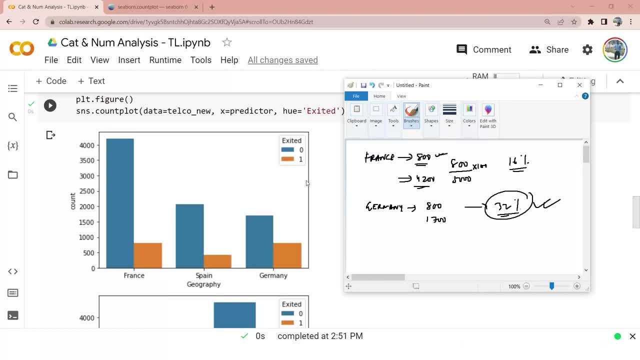 churn rate is high. so from this univariate analysis I am getting an insight that people staying in Germany are more likely to churn. you can do the same for Spain, also. univariate analysis, without the doing the graphical thing. you can also simply do dot value counts and you can also try to. 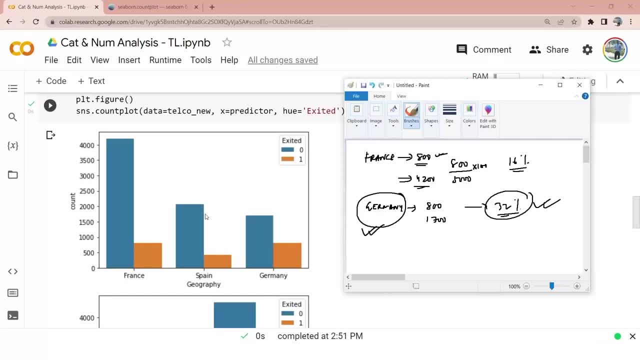 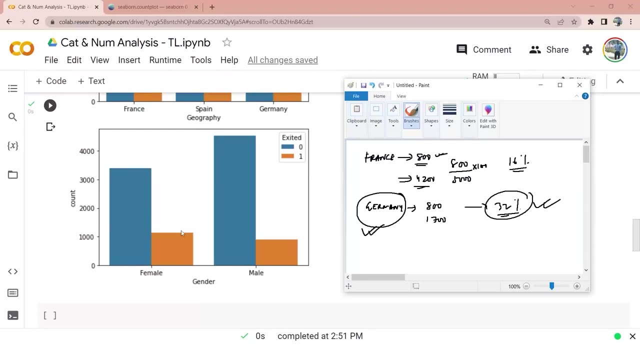 get the insights. but visual analytics is more intuitive, right? it gives you more insights, it helps you understand better, as compared to just numbers. similarly, from the second graph, I would say female are more churners as compared to male. you can see the total number of people in male are high, but the total number of people in male are high. but 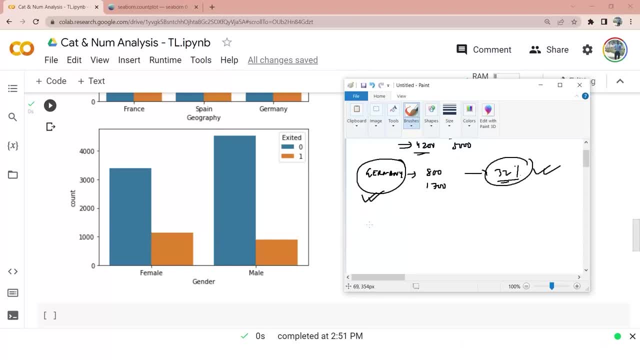 the churners are more in female. so one insight here is: female are more churners. so the second insight that we got is people staying in Germany are more churners. these are the two insights that I got from my simple univariate analysis. so in your case you have a data of hundred. 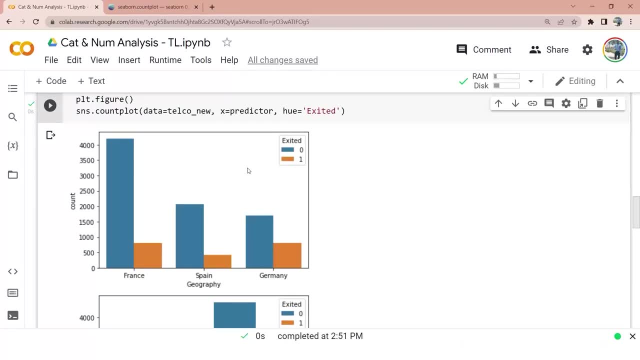 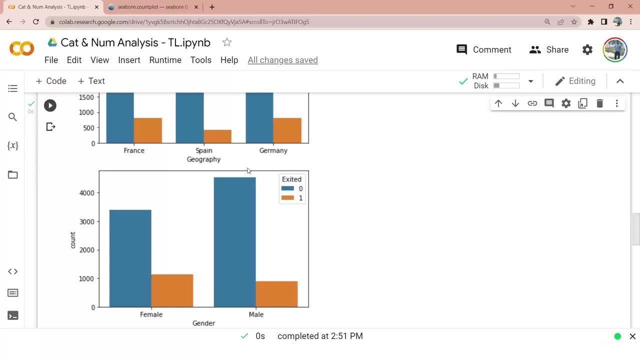 variables. you have to simply go through each and every graph and you have to interpret. sometimes you would get insights. sometimes you won't get insights. but if you don't get insights that does not mean that this particular column is not important. just imagine, for example, you get that for gender the ratio is almost same in the original data. also it is in the. 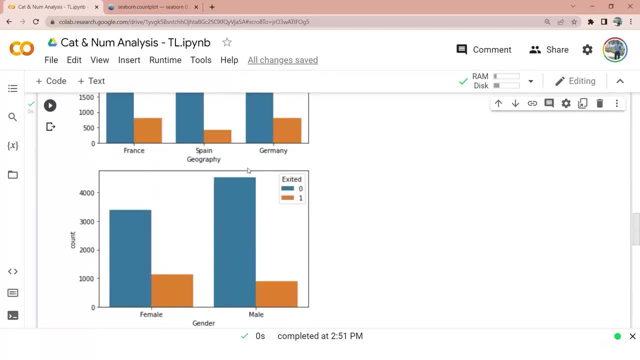 interpret. sometimes you would get insights, sometimes you won't get insights. but if you don't get insights that does not mean that you will get insights. but if you don't get insights, that does not mean that this particular column is not important. just imagine, for example, you get that for gender the ratio is almost same in the original data also. 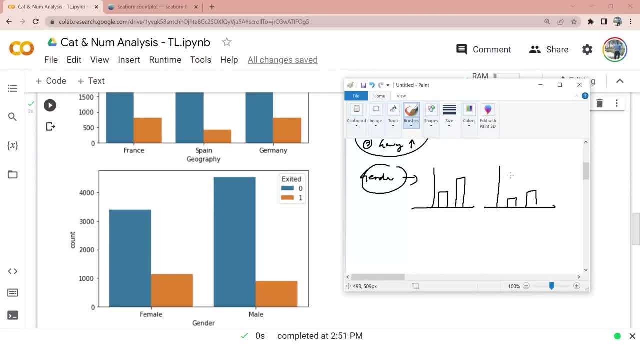 it is in the same ratio and in the churn data also it is in the same ratio. does that mean gender is not important? no, that means gender alone is not important. gender combined with any other feature is not important. no, that means gender alone is not important, gender combined with any other feature. 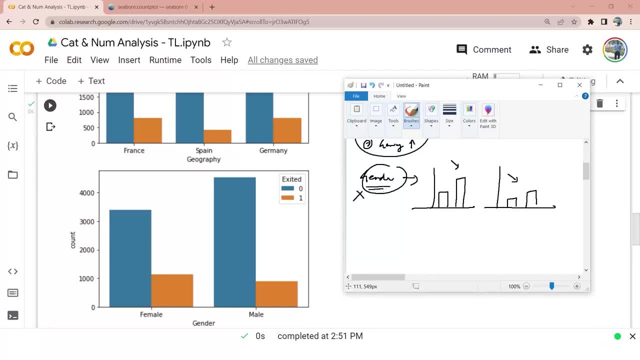 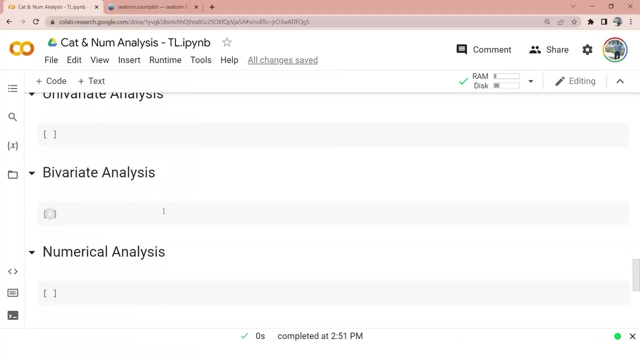 right. so sometimes your univariate analysis might not give you those much of information, so you should always go ahead and do bivariate, trivariate, multivariate and other analysis. jumping on to the, we already performed univariate analysis, which is this piece of code. so i'll just take this code above here: 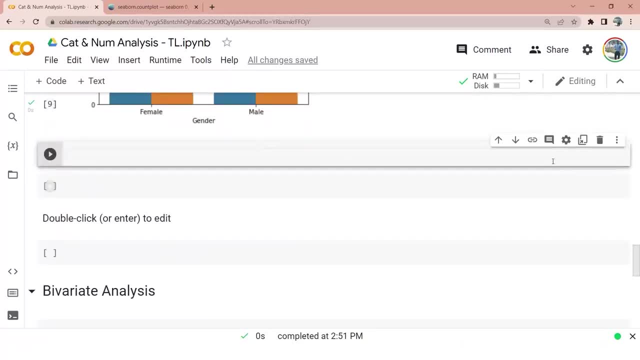 so this is my univariate analysis done. now talking about the bivariate analysis. so in case of bivariate analysis, i'll again use another type of plot. the reason behind using another type of plot is you will be introduced to these kind of plots as well, so which is a win-win. 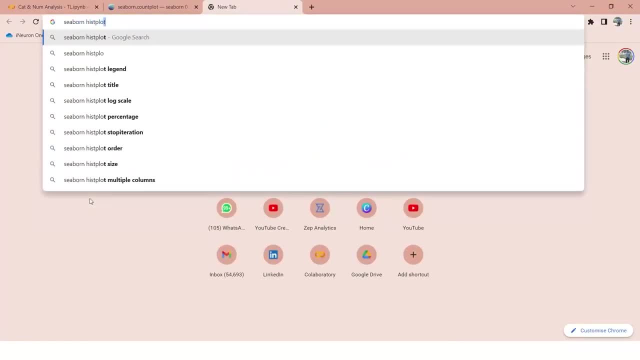 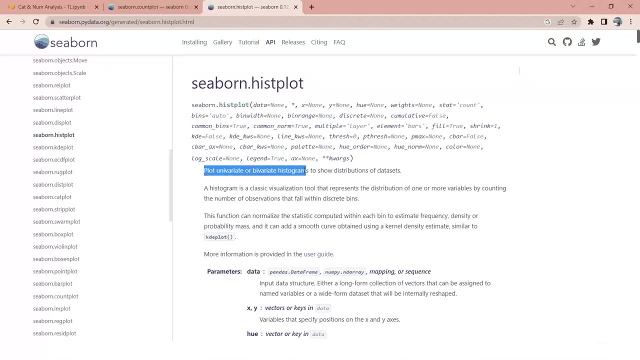 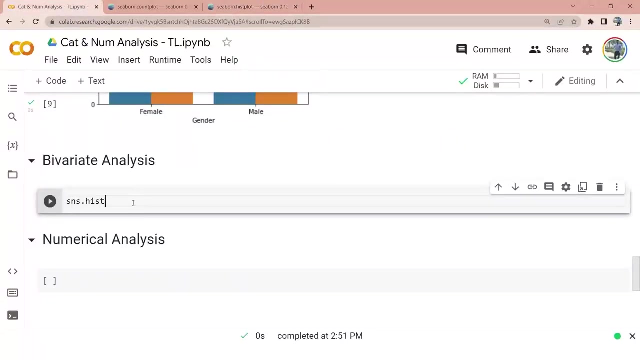 situation. so i'm going to use seaborn hist plot. okay, what do you mean by a hist plot plot? so this case, we are going to use bivariate and bivariate histograms to show distributions of the data. so in this case, let's say i will just simply plot hist plot. 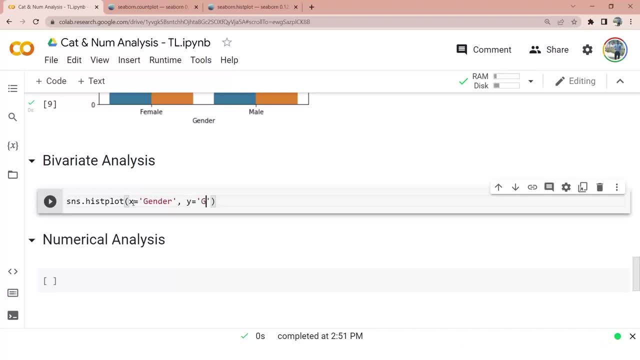 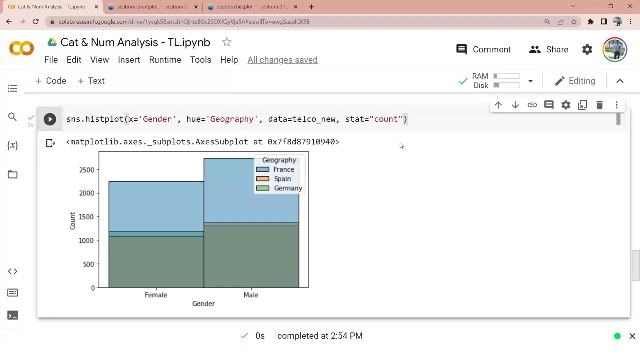 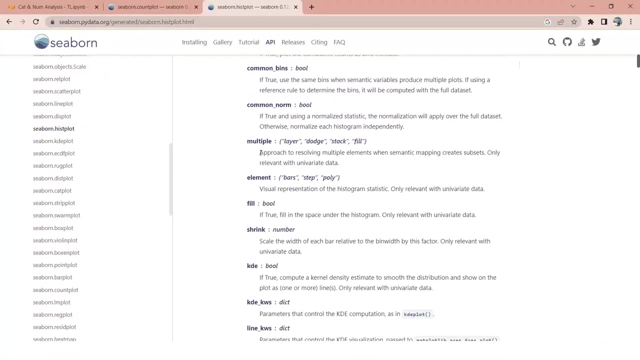 x equals to gender, y equals to geography. no, i don't need y, so i will just use u as geography. and then what is my data? my data is telco. new equals to count. that's it. okay, let's also use the multiple feature approach to solving. 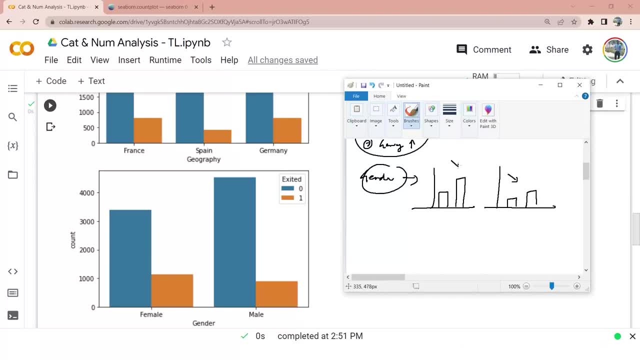 same ratio and in the churn data also it is in the same ratio. does that mean gender is not important? no means gender alone is not important. gender, combined with any other feature, could be an important insight, could be an important feature, right? so sometimes your univariate analysis might not give you those much of information, so you 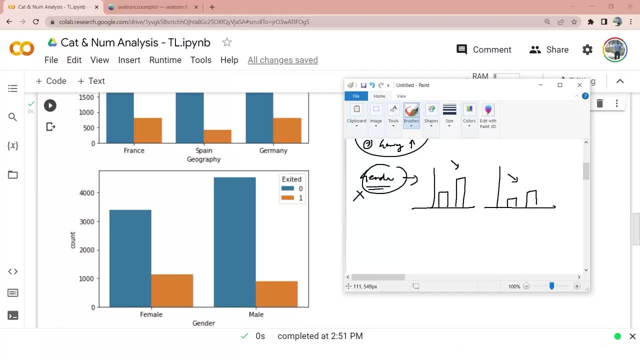 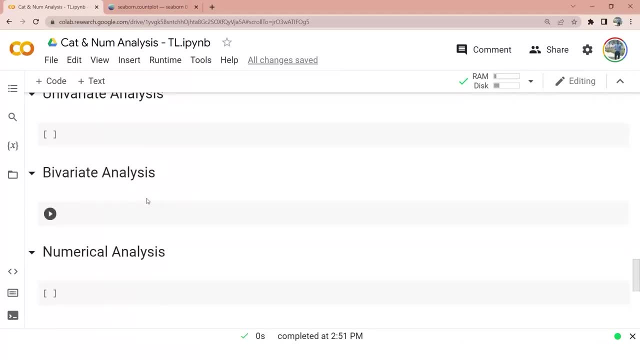 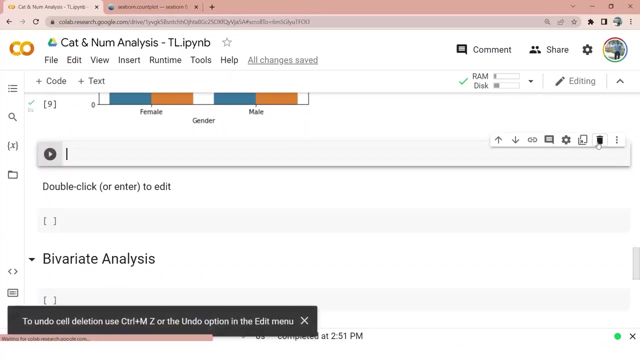 should always go ahead and do bivariate, trivariate, multivariate and other analysis. jumping on to the, we already performed univariate analysis, which is this piece of code, so I'll just take this code above here. so this is my univariate analysis done now talking about the bivariate analysis. so in case, 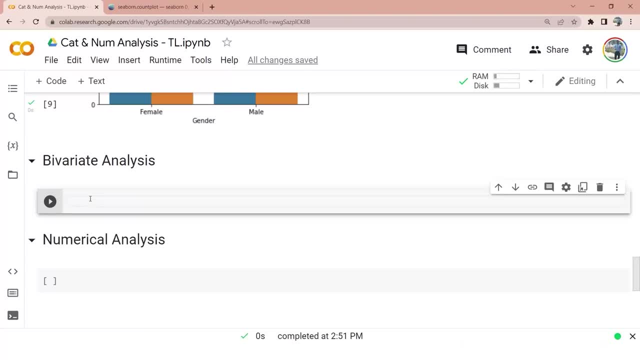 of bivariate analysis, I'll again use another type of plot. the reason behind using bivariate analysis is that the reason behind using bivariate analysis is that another type of plot is you will be introduced to these kind of plots as well, so which is a win-win situation, so I'm going to use seaborne hist plot, okay. 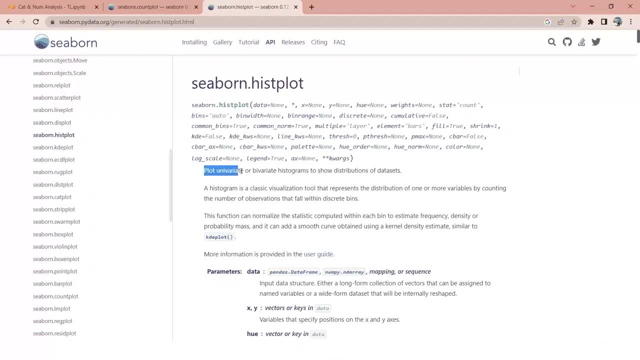 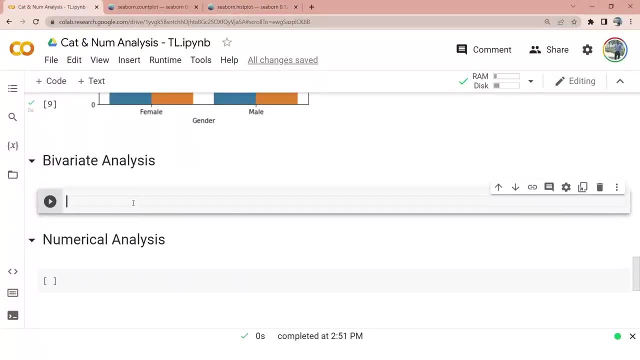 what do you mean by a hist plot plot? univariate or bivariate histograms to show distributions of the data. so in this case, let's say I will just simply plot hist plot: X equals to gender, Y equals to geography. no, I don't need y, so I will just use U as geography. and then what is? 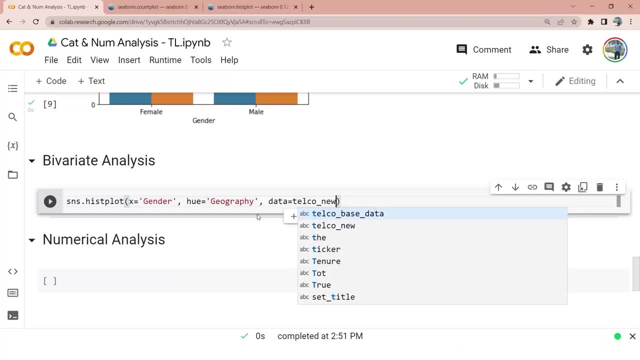 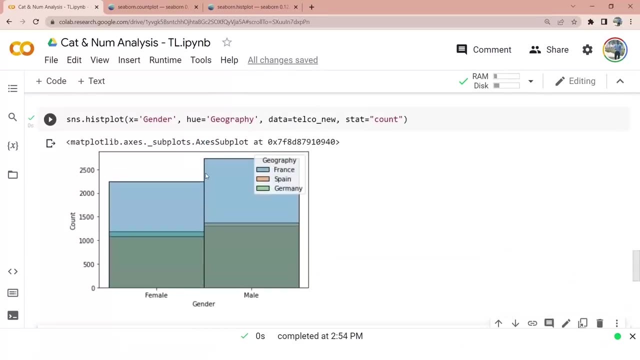 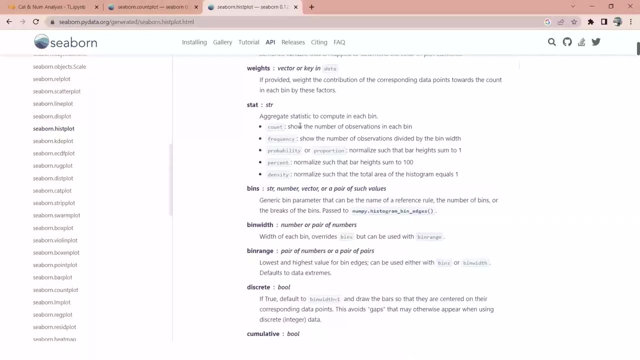 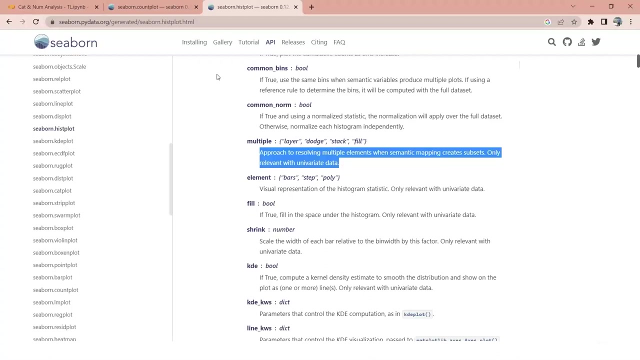 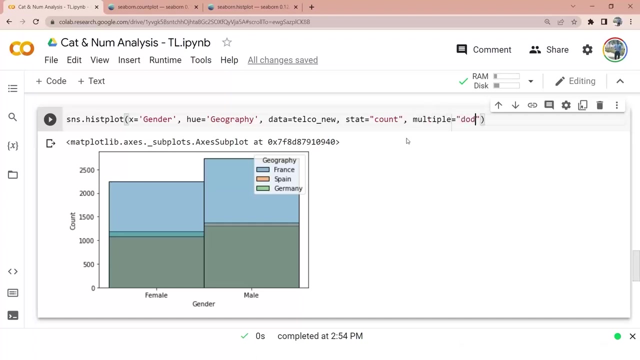 my data. my data is telco new. that equals to count. that's it. okay, let's also use the multiple feature approach to solving multiple element when semantic mapping creates subsets only relevant with univariate data. but yeah, we can use a multiple also. multiple equals to touch. you don't have to memorize all these codes as i 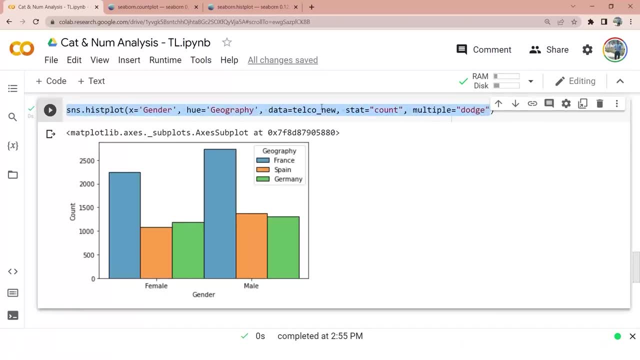 told you before. also, when it comes to python part in the data analysis or data science areas, nobody will ask you about writing codes. can you write down a code for hist plots? no, you can definitely take help of the web to plot down anything. so in this case you can see. 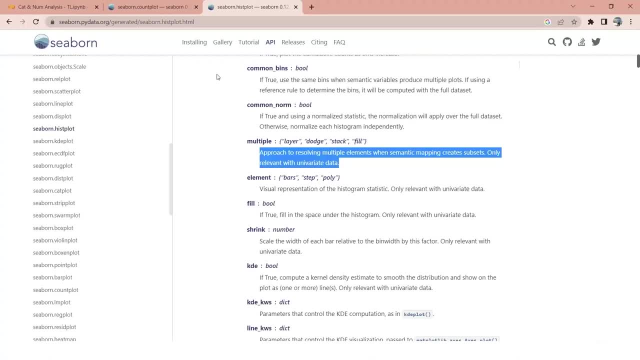 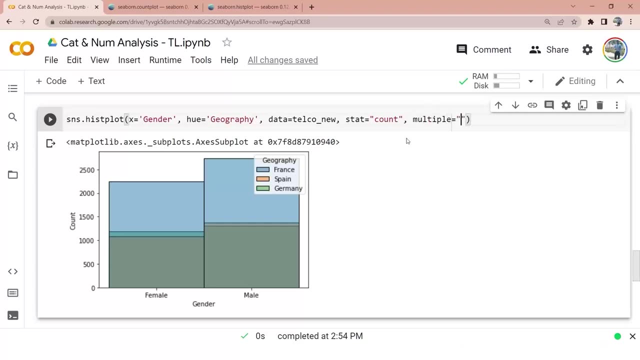 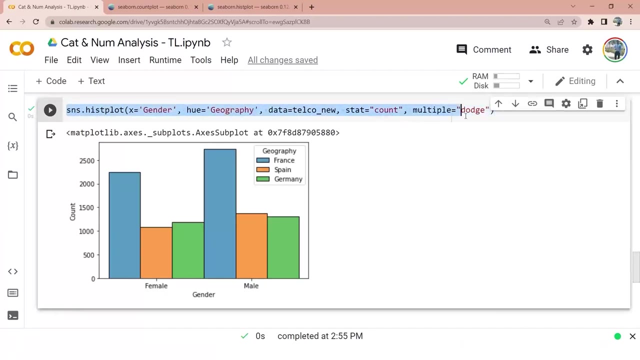 multiple elements when semantic mapping creates subsets only relevant with univariate data. but yeah, we can use a multiple also, multiple equals to touch. you don't have to memorize all these codes, as i told you before. also when it comes to python part in the data analysis or data science areas, nobody will ask you about writing codes. 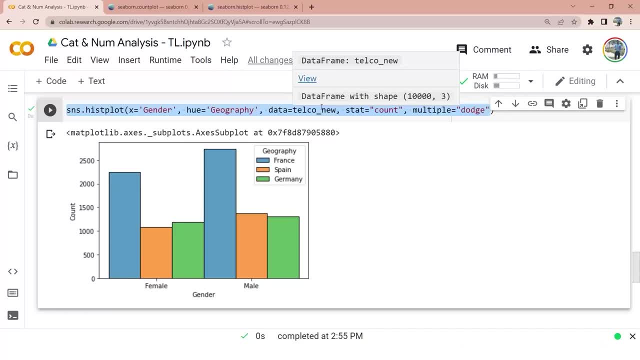 can you write down a code for hist plots? you can definitely take help of the web to plot down anything. so in this case you can see. obviously the graph might not look that good, but it is quite evident that for female customers you can see france, spain and germany. for male customers, france, spain and germany- right. 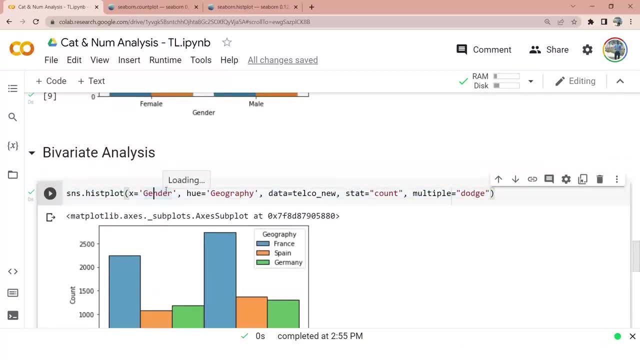 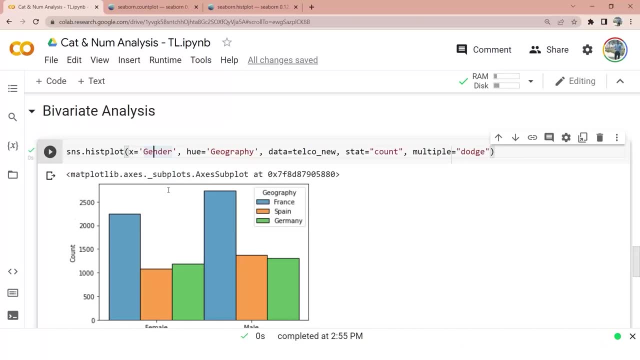 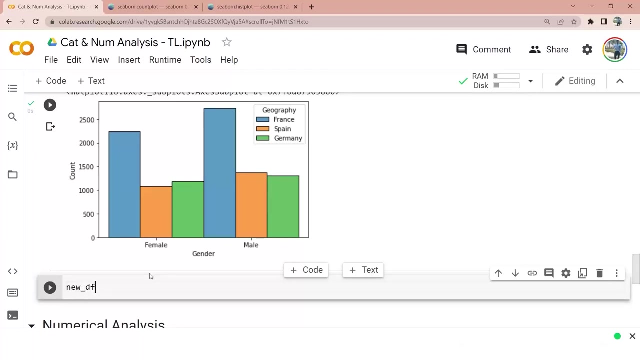 you can also do the same thing for your churned customers and you can also get some insights. let's say: let's say we will create a new data frame only for the churned customers. let's try to do that, so i will create a new df. let's say i will just do telco new of target one, which is telco new dot lock of. 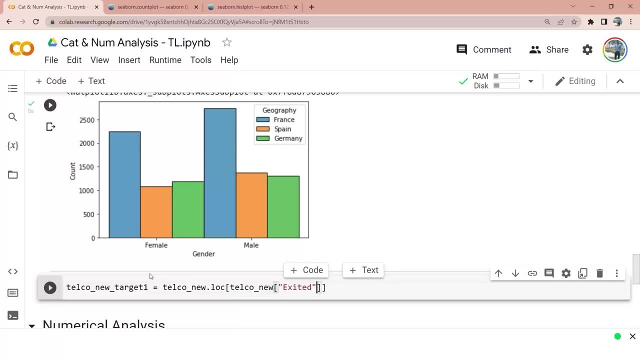 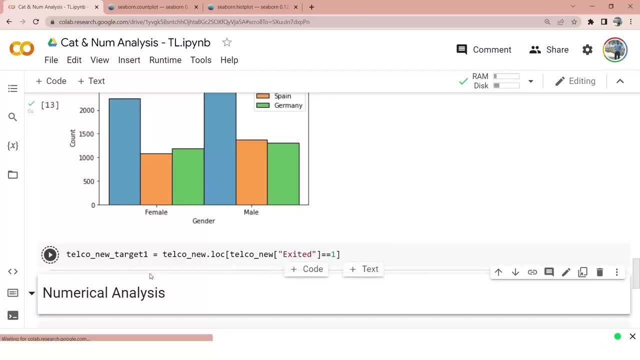 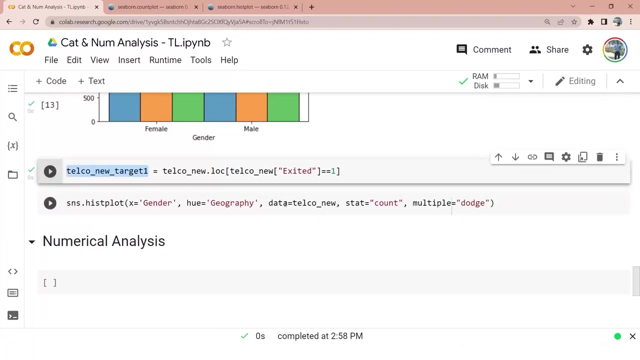 telco new of exited equals to equals to zero. equals to equals to one. so these are all my churned customers, right? so i am only selecting exited equals to one and these are my churned customers. same thing i will just copy paste here. i will change. 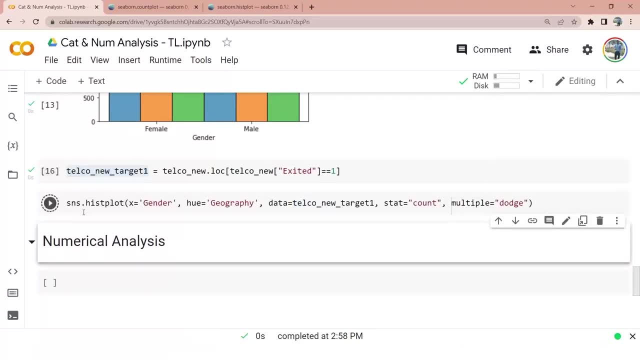 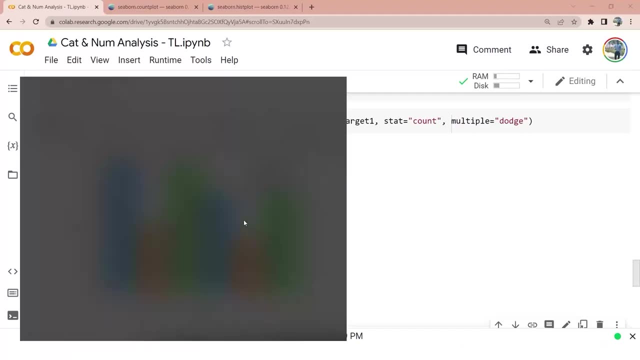 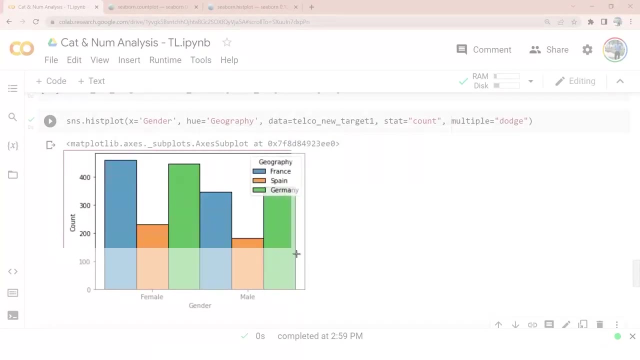 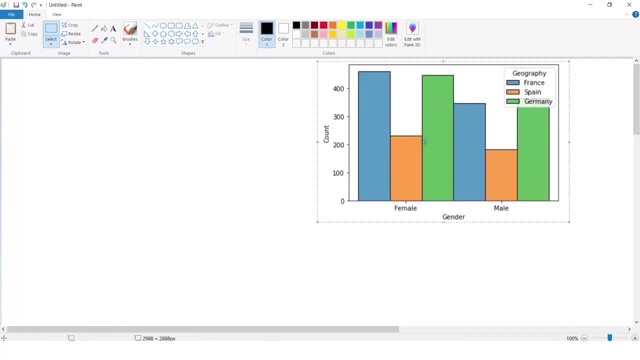 my data frame. that's it. everything remains the same. now you can see that this is the graph for the churned customers, so let's try to snipe it out and then we will analyze this on paintbrush. so that's my churned customers and that's my original data. 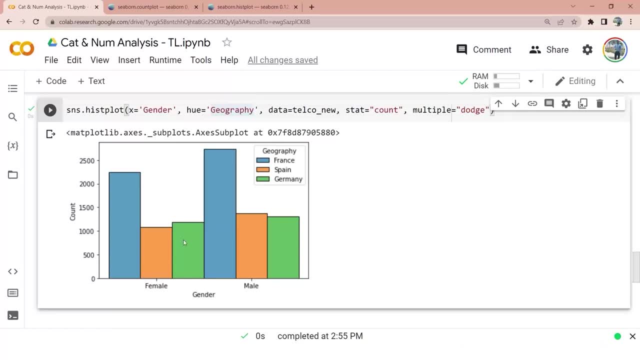 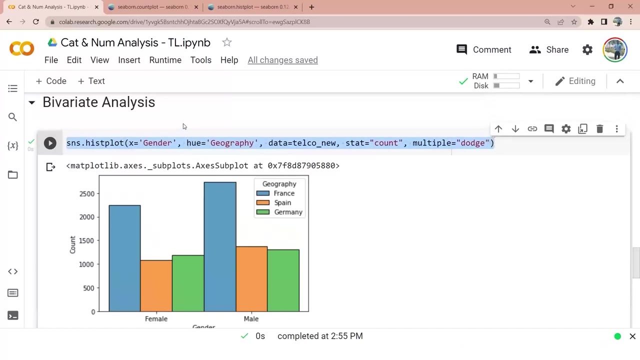 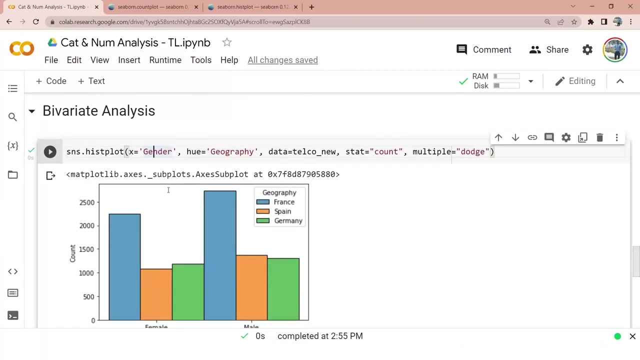 obviously the graph might not look that good, but it is quite evident that for female customers, you can see france, spain and germany. for male customers, france, spain and germany. right, you can also do the same thing for your churned customers and you can also get some insights. 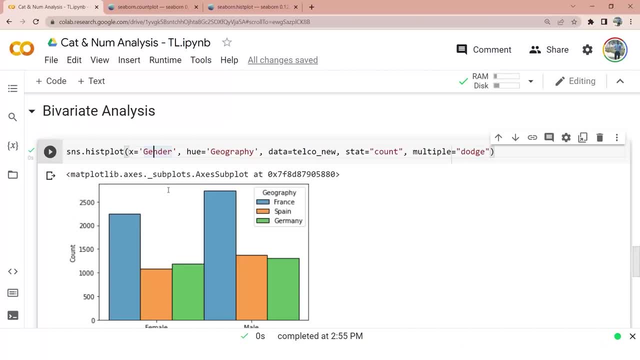 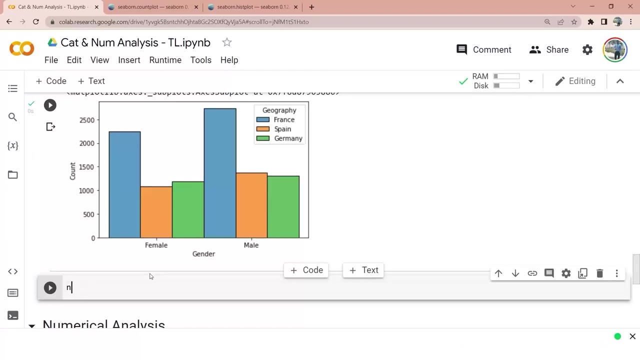 let's say we will create a new data frame only for the churned customers. let's try to do that. so i will create a new df. let's say i will just do telco new of target, which is target one which is telco new dot. lock of telco nu of. 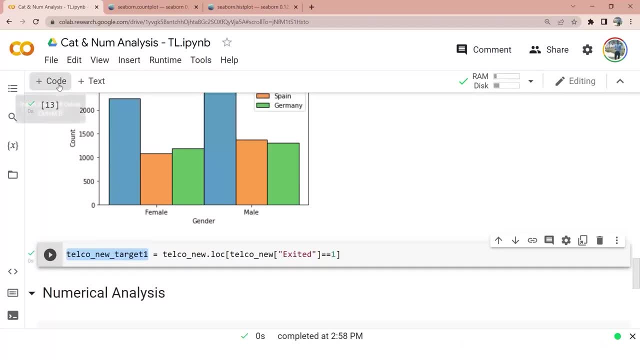 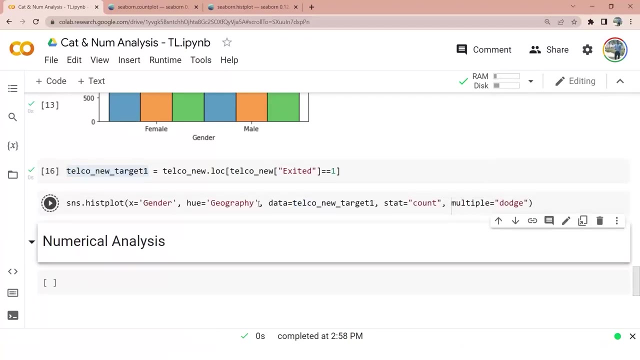 exited equals to equals to zero. equals to equals to one. my bad, so these are all my churned customers, right? so i am only selecting exited equals to one and these are my churned customers here. i will change my data frame. that's it. everything remains the same. now you can see. 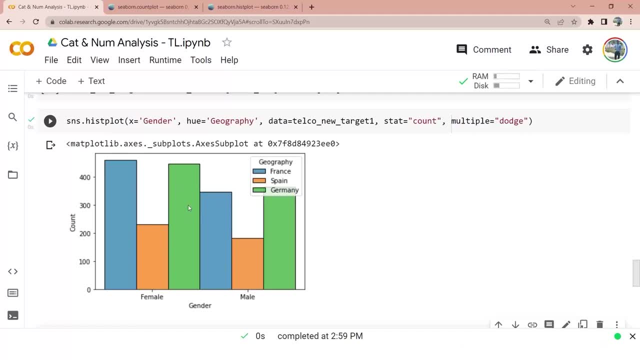 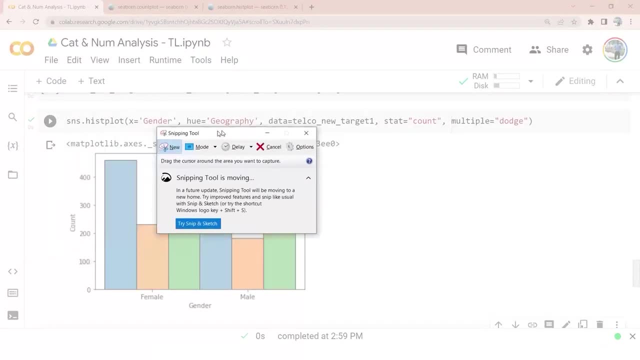 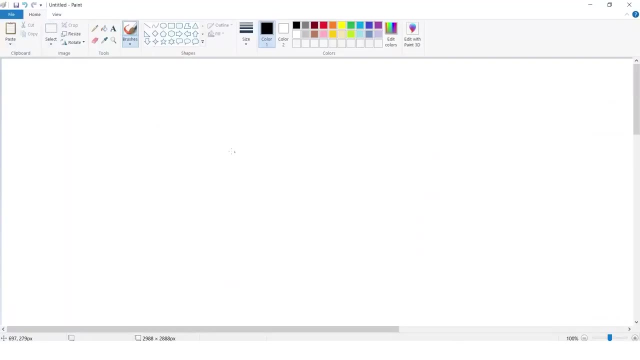 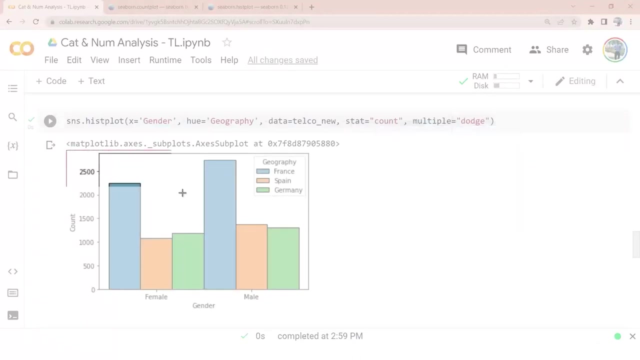 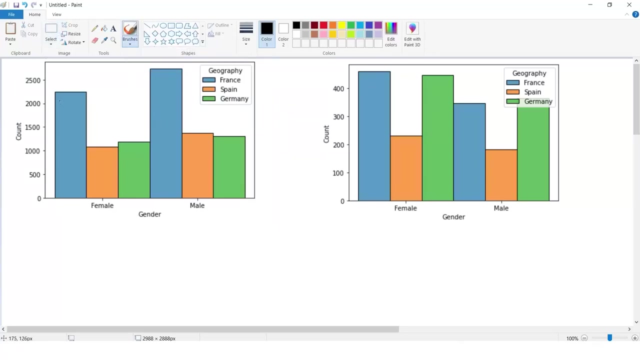 that this is the graph for the churned customers. so let's try to snipe it out and then we will analyze this on paintbrush. so that's my churn customers and that's my original data. that's my original data. now, what do you infer from this? in the original data you can see: 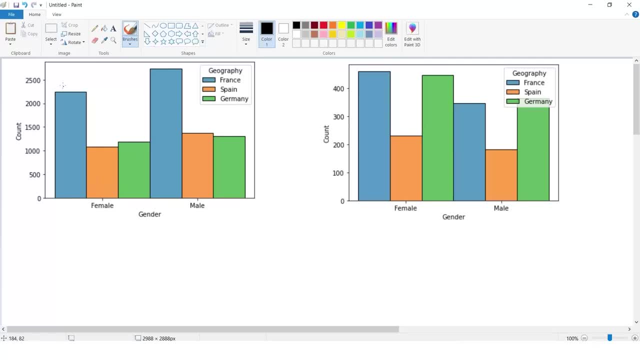 if i just look at the data. i so first of all you have to identify the ratio. let's say, female, there are 2250, france, almost. let's say 100, 1100, uh, spain and around 1200 germany. what is the ratio here? 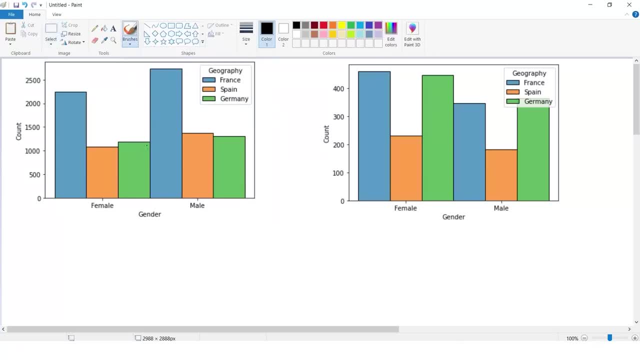 that's my original data. now, what do you infer from this? in the original data you can see, if i just look at the data i. so, first of all, you have to do, is you have to do? is you have? so, first of all, you have to identify the ratio. let's say: 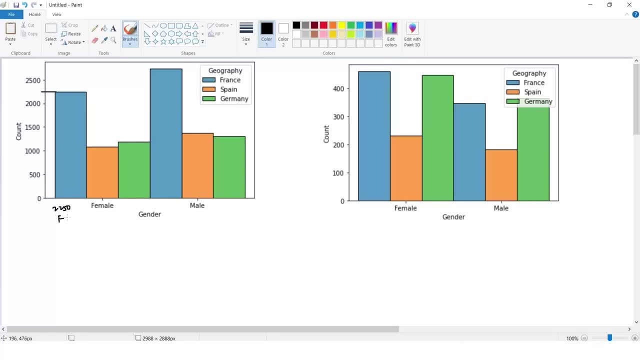 female. there are 2250 france, almost, let's say, 100, 1100 spain and around 1200 germany. what is the ratio here? maybe around 450 in france, around 220 spain and germany is very high- almost 430 Germany. you can see, out of 1200, 430 people who are from Germany. so 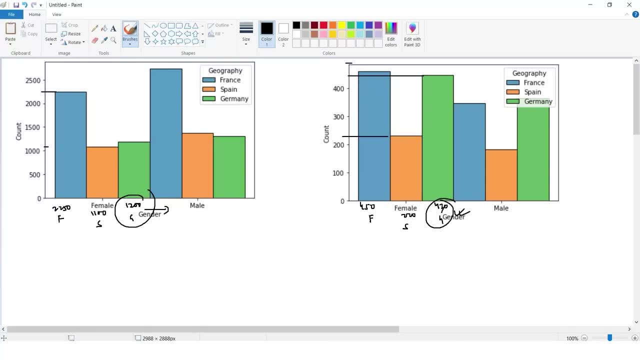 what is the ratio? the ratio is almost almost 430 divided by 1200 in 200, which is almost 36 percent. so female plus Germany, the female customers staying in Germany: 36 percent. what about male in Germany? around 380, and what is here? around 1300. so what is the ratio? 380 around 1300 in 200. so even for the males. 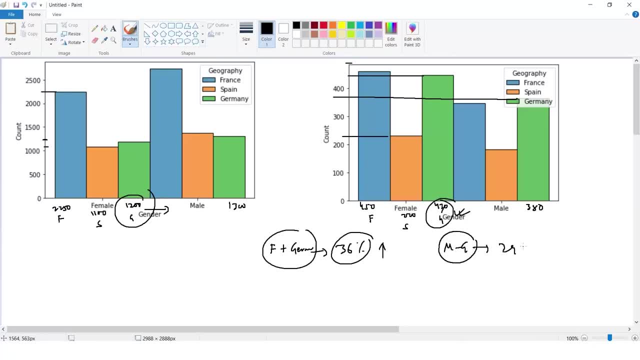 also in Germany the ratio is almost high. the churn rate is high, but this is an insight using univariate analysis. what we got is people staying in Germany are more churners, but now we are getting that female who are staying in Germany are more churners as compared to male. male are also churners, but the female ratio 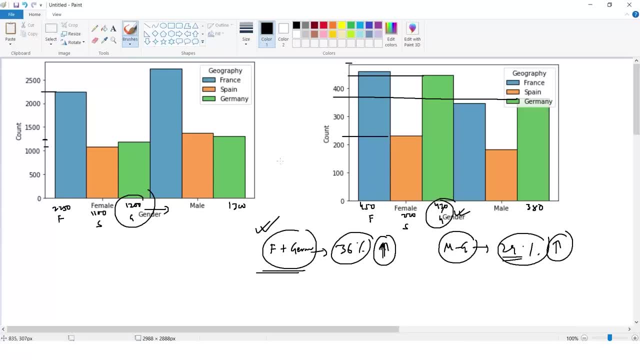 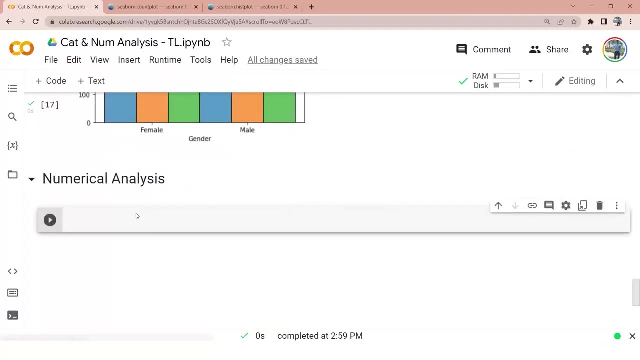 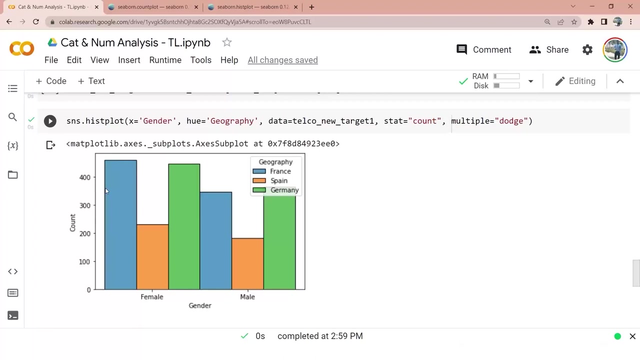 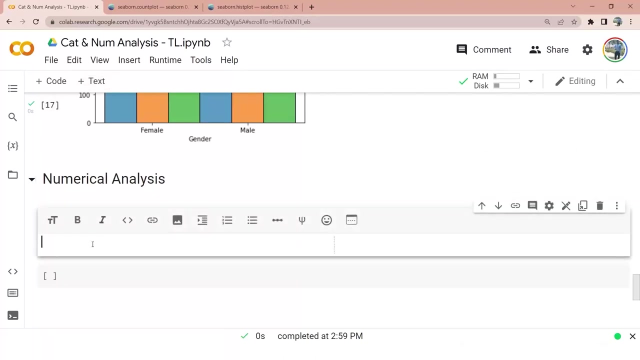 is pretty high. that's one of the insights that we got you right. moving on to other types of analysis, so we will be considering some numerical analysis. in numerical analysis, first of all, you can plot box plots. you can plot any kind of plots. we will get started with the correlation plot. okay, as I told, 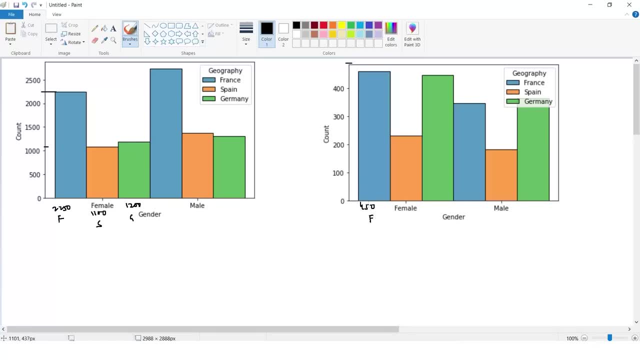 may be around 450. france, around 220. spain. and germany is very high, almost 430 germany, you can see out of 1200, 430 people who are from germany. so what is the ratio? the ratio is almost almost 430 divided by 1200 into 100, which is almost 36 percent. 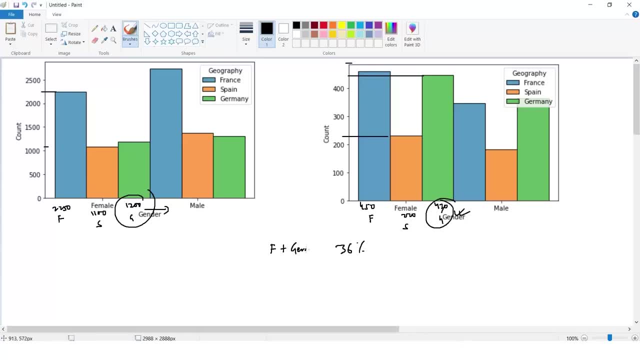 so female plus germany. so female customers staying in germany 36 percent. what about male in germany? around 380 and what is here? around 1300. so what is the ratio? 380 around 1300 into 100. so even for the males also in germany the ratio is: 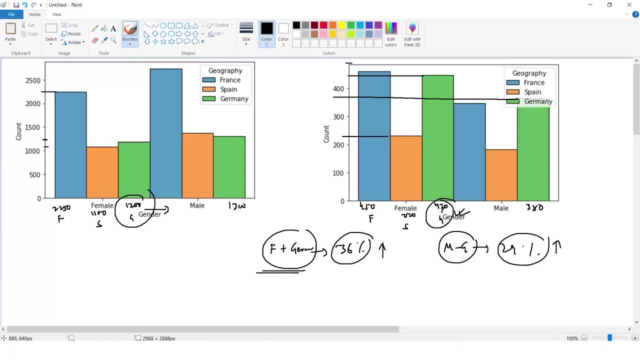 almost high. the churn rate is high, but this is an insight. using univ rate analysis, what we got is people staying in germany are more churners. but now we are getting that female who are staying in germany are more churners as compared to male. male are also churners, but the female ratio is pretty high. 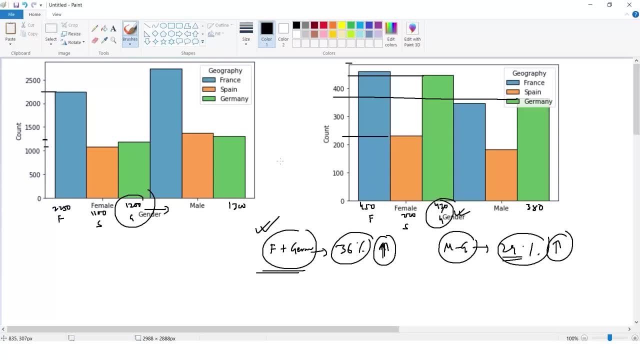 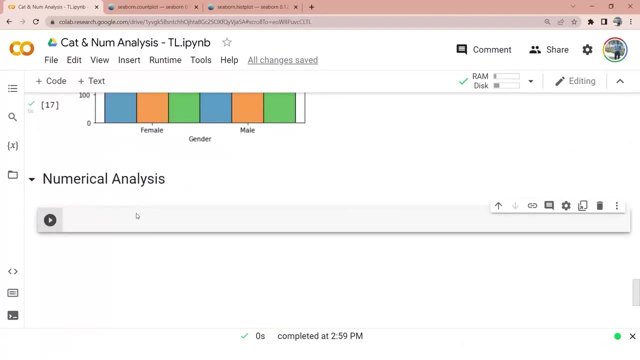 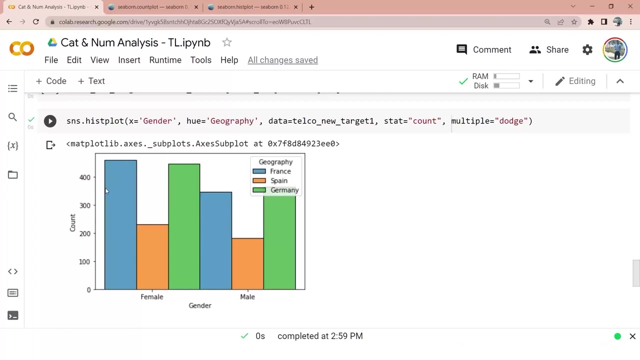 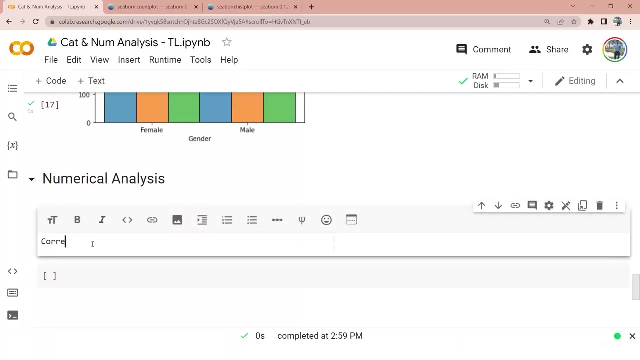 that's one of the insights that we got right. moving on to other types of analysis, so we will be considering some numerical analysis. in numerical analysis, first of all, you can plot box plots. you can plot any kind of plots. we will get started with the correlation plot. okay, as i told you, first thing is correlation. 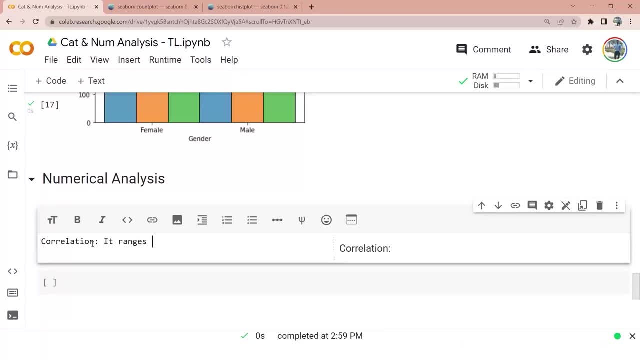 what is correlation? it ranges from minus one to plus one. that we all know right. plus one or near to that positive correlation. minus one to plus one, minus one or near to that is negative correlation and anything near to zero is no correlation. that we already know, right. so 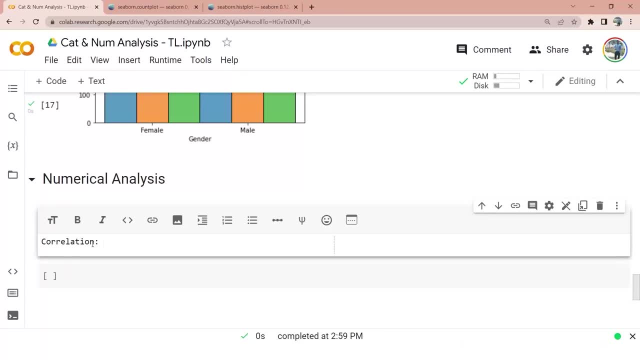 you. first thing is correlation. what is correlation? it ranges from minus 1 to plus 1, that we all know right. plus 1 or near to that- positive correlation. minus 1 or near to that is negative correlation. and anything near to 0 is no correlation. that we already know right. so 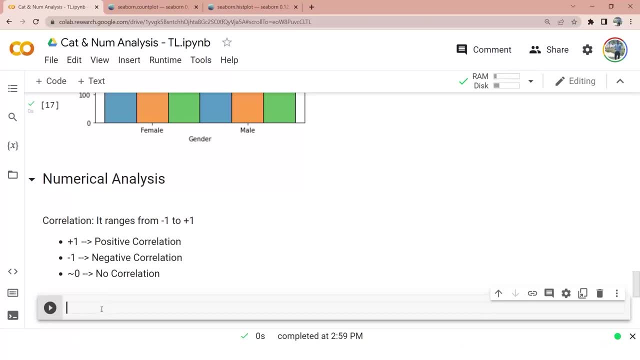 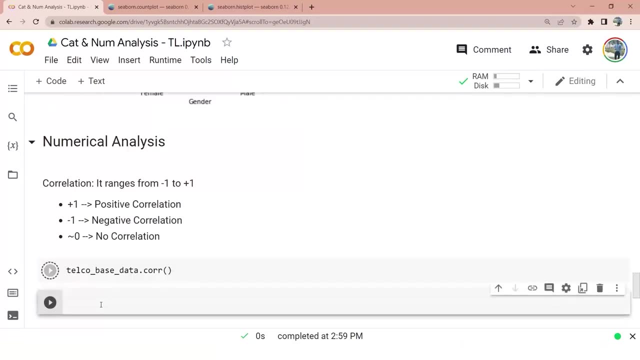 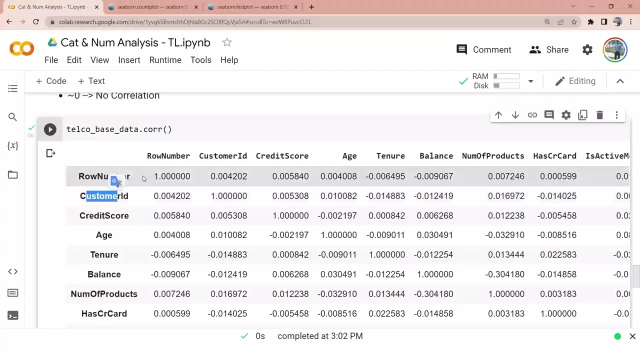 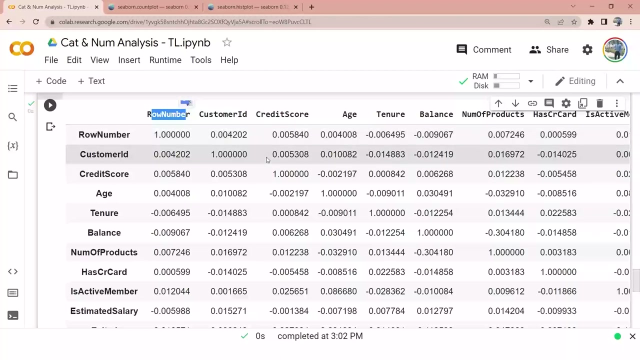 you can calculate, the correlation opens. so what we will do is we will quickly plot the correlation function here. you can see when I'm plotting the correlation. you are able to see a matrix right in your columns and in your rows the names are same. so using this matrix, you can also identify which of them are highly. 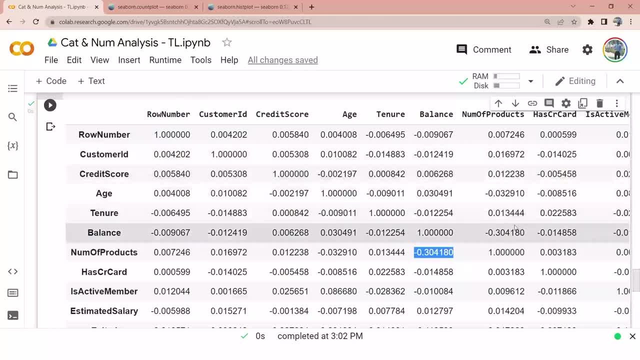 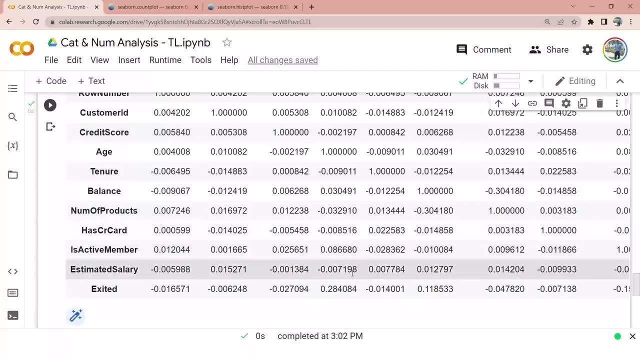 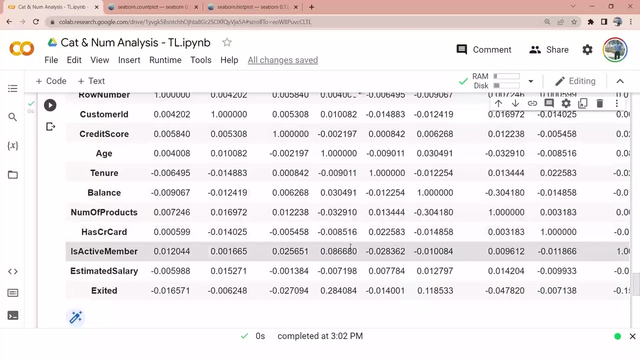 as you can see, this one minus 0.3 or this one same minus 0.3- that means number of products and balance are negatively correlated. do we see a very high positive number? i think the highest positive number that i can see right now is this: exited with respect to age, that 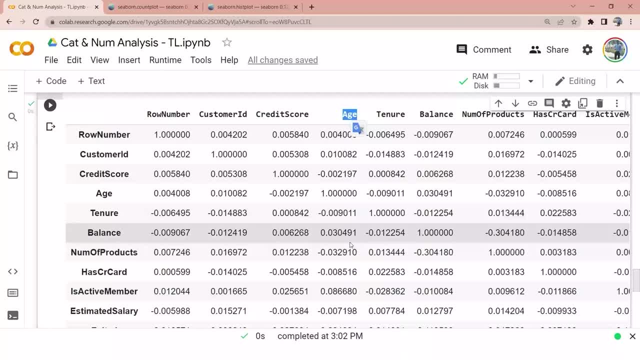 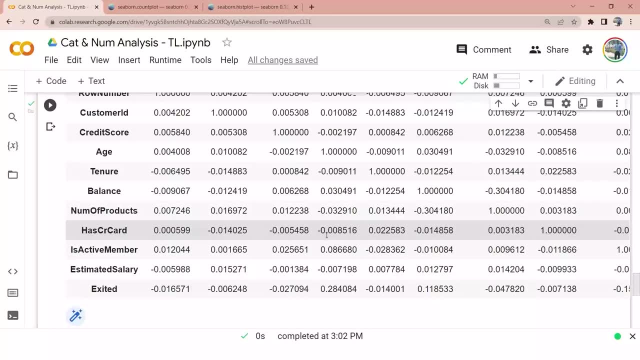 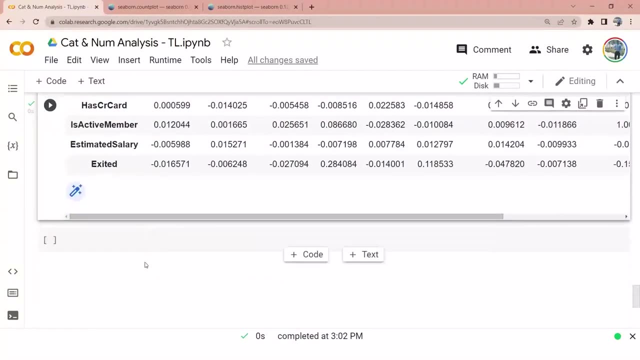 means age and exited are more correlated. that means higher the age possibility of getting more exited. that means people who are into the seniority level are exiting more. now how do we beautify this? using some graphs. so what we will do is plt dot figure. i will just use 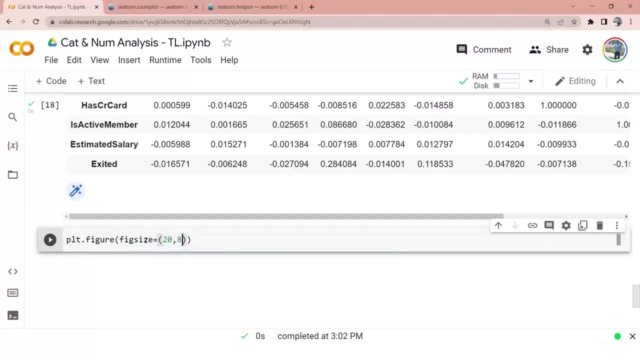 a fixed size, let's say 20 cross 8, and here i will do telco based data dot correlation. i want to have a correlation with respect to to exited, because that is my y variable. our main focus is to understand the correlation of different features with respect to the exited. 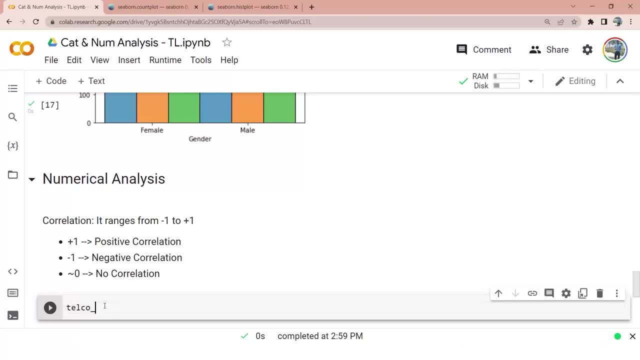 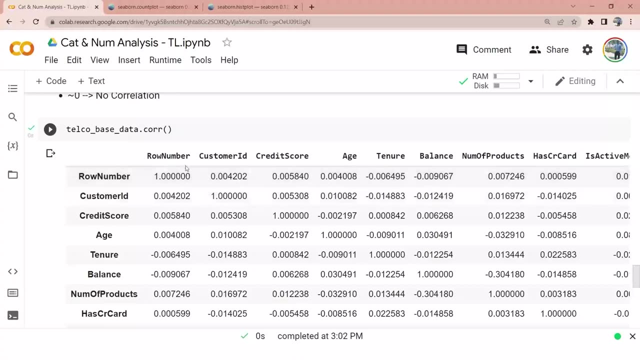 so what we will do is we will quickly plot the correlation function here. you can see when i'm plotting the correlation. you are able to see a matrix right in your columns. this is your subscript and in your rows the names are same. so, using this matrix, you can 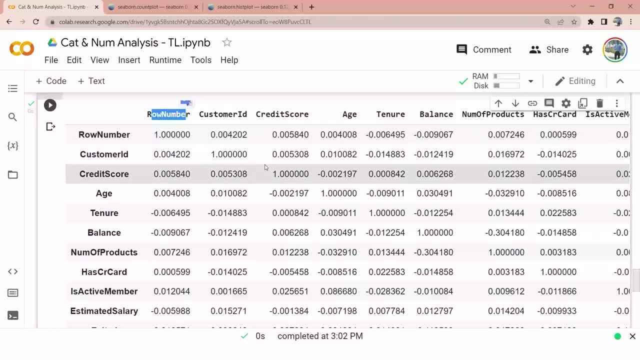 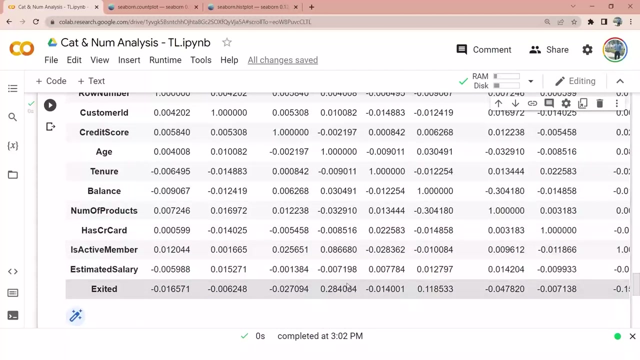 also identify which of them are highly correlated or which of them are negatively correlated. as you can see, this one minus point three or this one same minus point three- that means number of products and balance are negatively correlated. do we see a very high positive number? think the highest positive number that i can see right now is this: exited with respect. 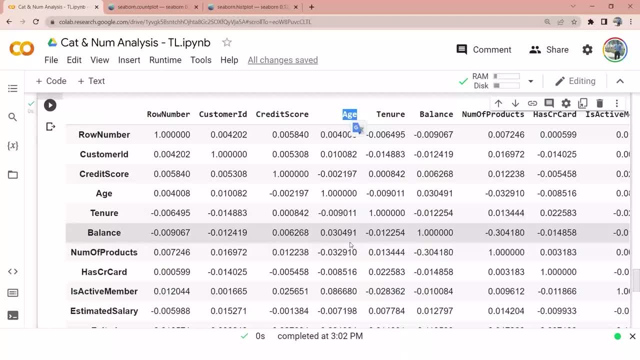 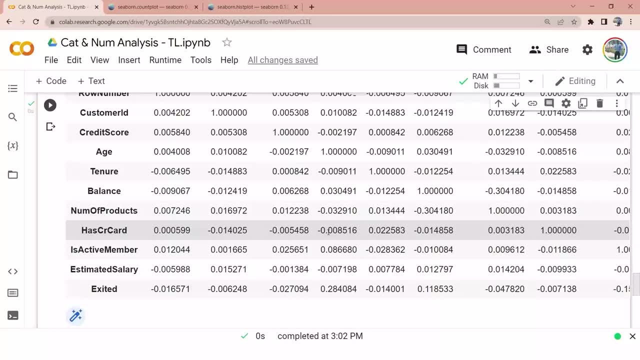 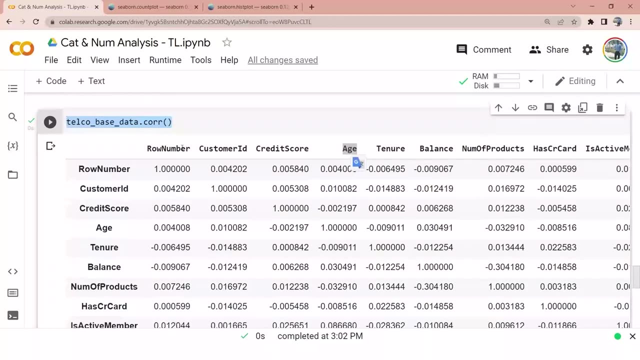 to age. that means age and exited are more correlated. that means higher the age possibility of getting more exited. that means people who are into the seniority level are exiting more. now how do we beautify this? using some graphs. so what we will do is plt dot figure. i will 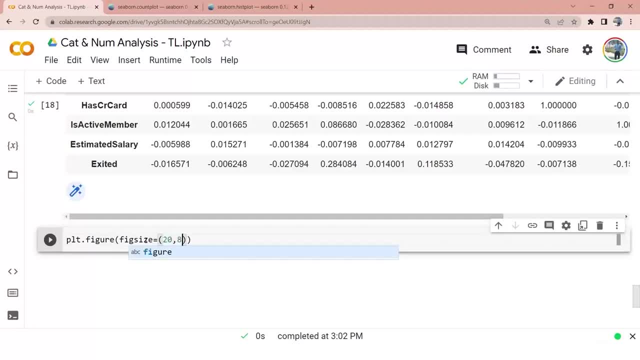 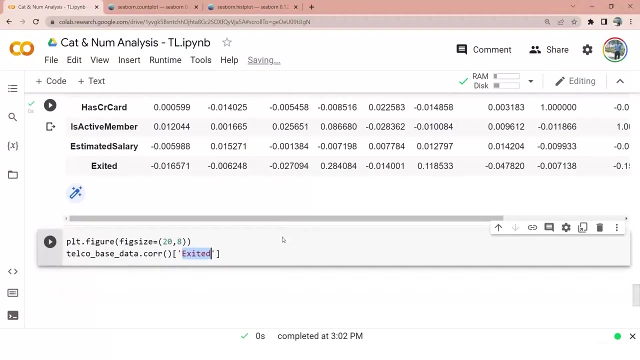 just use a fixed size, let's say 20 cross 8. and here i will do telco base data dot correlation. i want to have a correlation with respect to to exceeded, because that is my y variable. our main focus is to understand the correlation of different features with respect to the 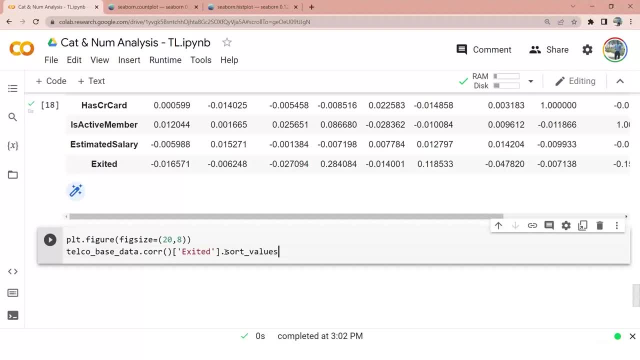 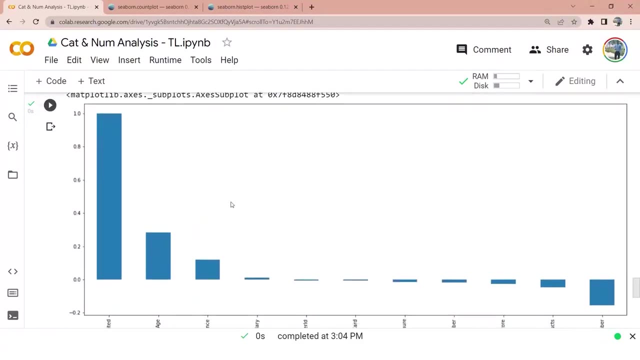 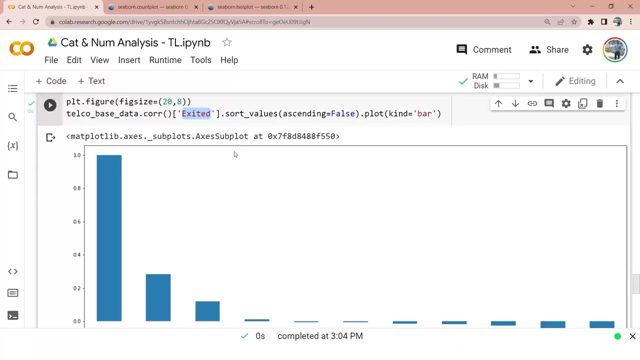 exited column right, and then i will sort the values with respect to ascending equals to false and then plot it using a bar chart. okay, so you can see. this is how my correlation function looks like. correlation output looks like with respect to exited. i'm not doing correlation of each column. 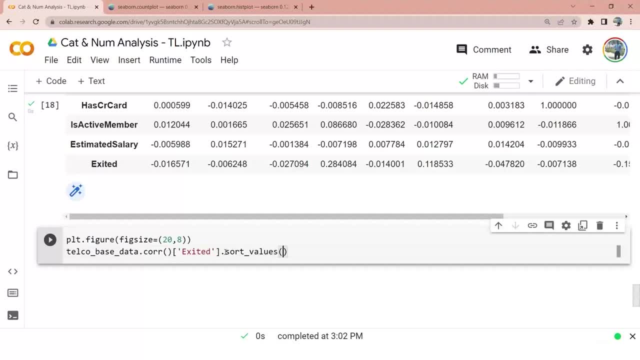 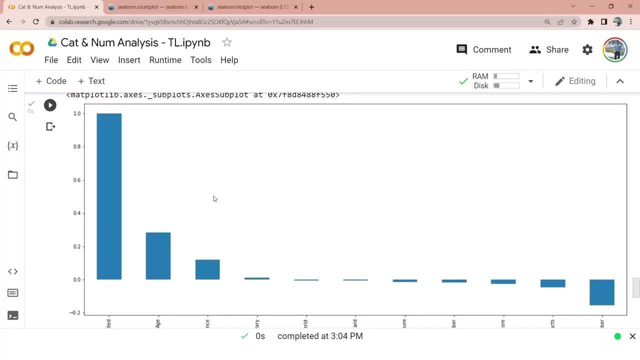 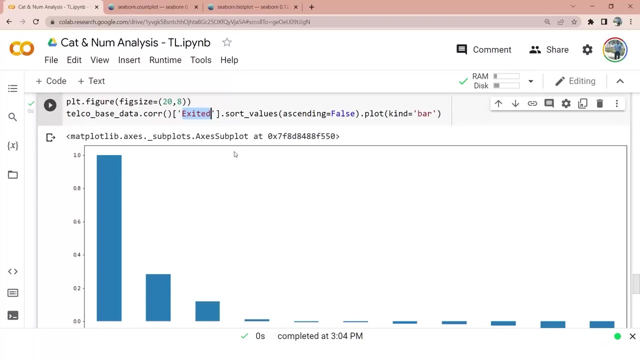 column right and then i will sort the values with respect to ascending equals to false and then plot it using a bar chart. okay, so you can see. this is how my correlation function looks like. correlation output looks like with respect to exited. i'm not doing correlation of each column with respect to each column. this is especially 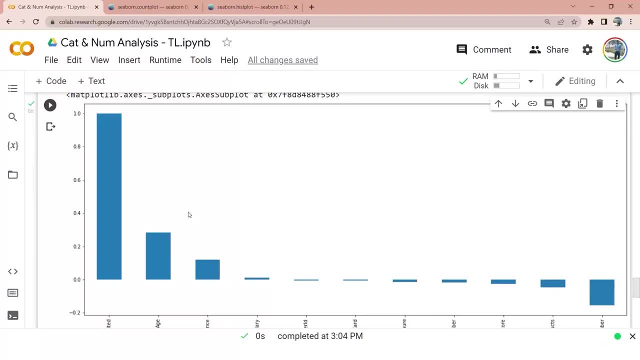 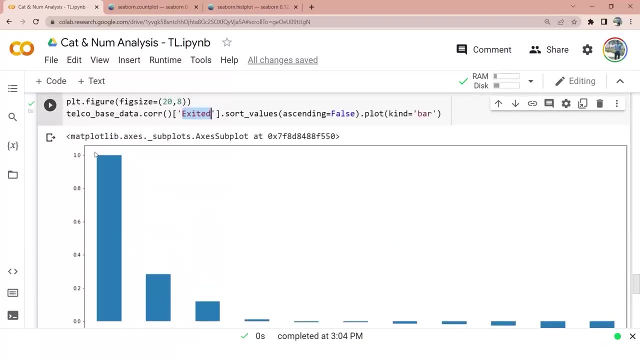 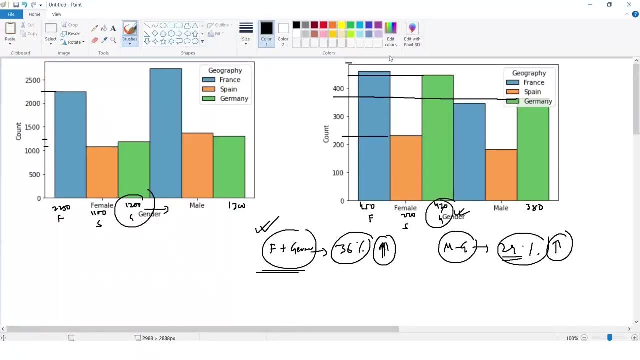 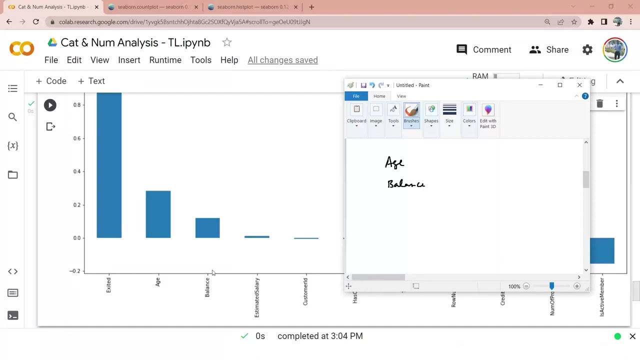 the correlation between multiple columns with respect to exited, and you can see the first one is ignorable because exited with respect to exited, obviously the correlation will be one. so ignore this thing. you can see age is a factor. you can see age is a factor. so we are able to see age is an important factor. balance is also an important factor. they are. 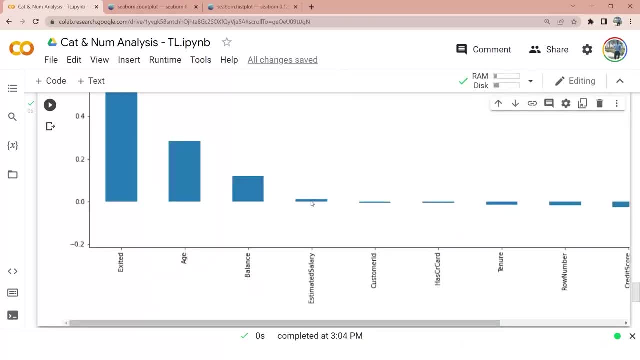 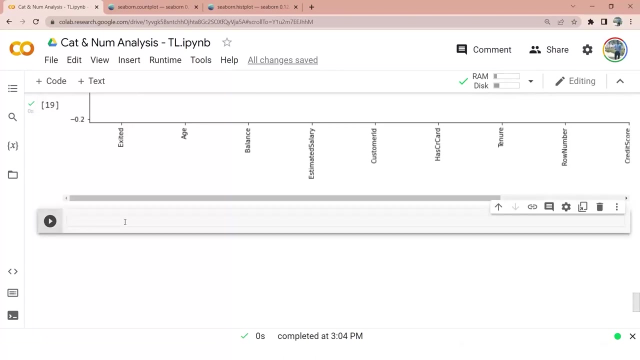 having positive correlation and rest, all of them are very small values, so i will not consider and you can see number of products and is the active member are negatively correlated. so somehow these four features are very important with respect to exited. so this is what my insight we are getting from here. next step is i will simply plot my correlation function, which we 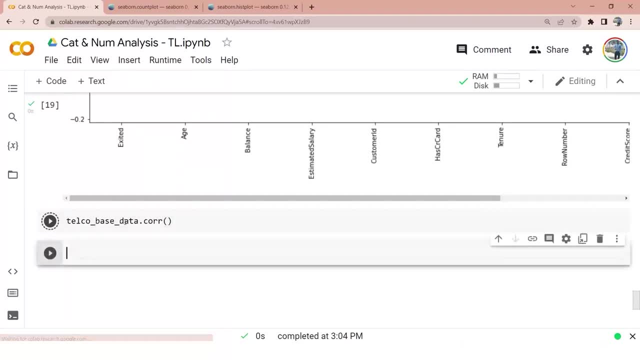 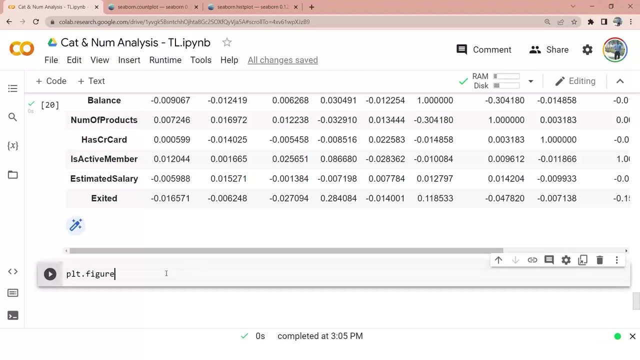 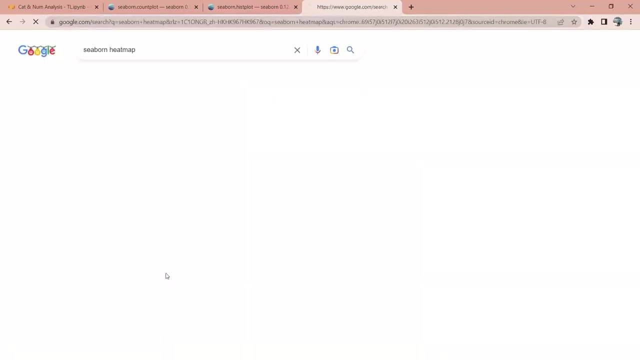 did right now, which was this: we will plot this correlation function using a heat map, so i will use the same concept: plt dot figure fix size equals to 20 cross 20, so 12 cross 12, because it's a square. seaborn dot heat map. you can see seaborn heat map. 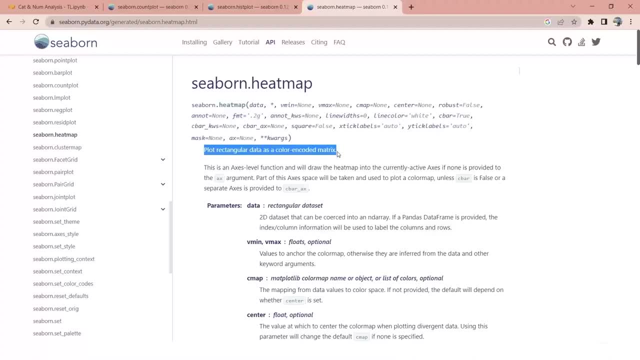 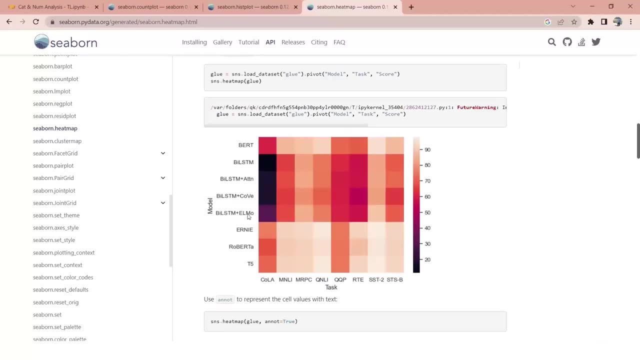 it's a plot, a rectangular data as a color encoded matrix and if you scroll down, you will see some graphs like this. this is a heat map, column with respect to column okay, and you can see on the right hand side you will see a scale that means the lower, the 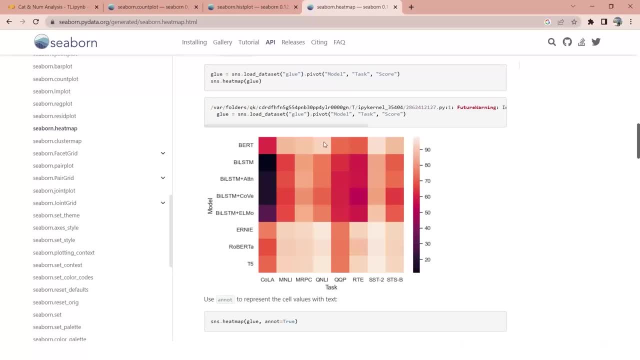 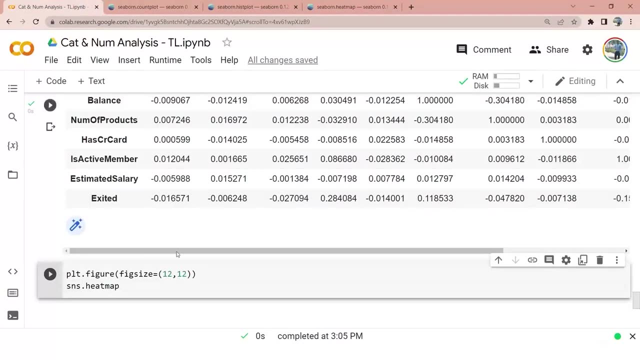 number the darker it is, and the higher the number lighter it is. so you can easily spot where you have lighter values and where you have the darker values right. so we will be using the same concept. heat map of telco base data. dot correlation. there is a. 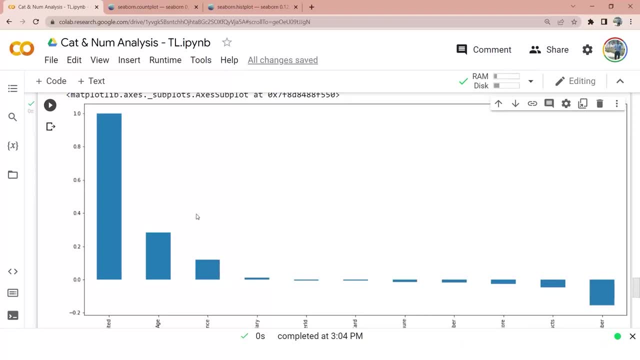 with respect to each column. this is specially the correlation between multiple columns with respect to exited, and you can see the first one is ignorable because exited with respect to exited, obviously the correlation will be one. so ignore this thing. you can see, age is a factor, so we are. 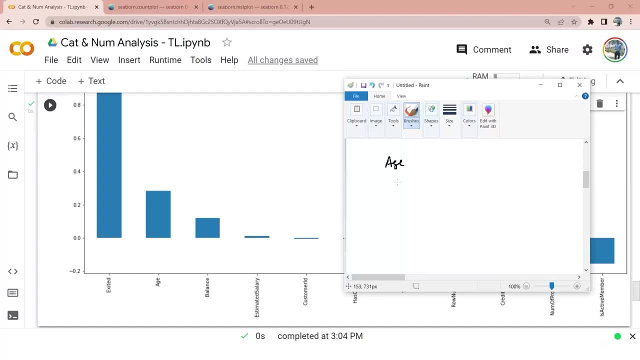 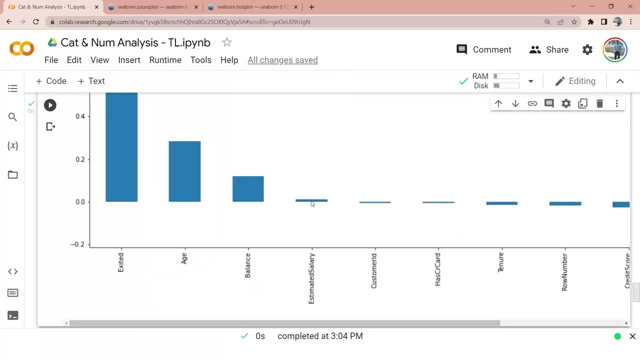 able to see. age is an important factor. balance is also an important factor. they are having positive correlation and rest, all of them are very small values, so i will not consider and you can see number of products and is the active member are negatively correlated. so somehow these four 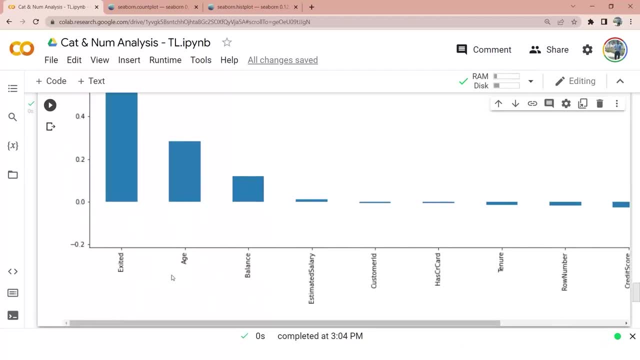 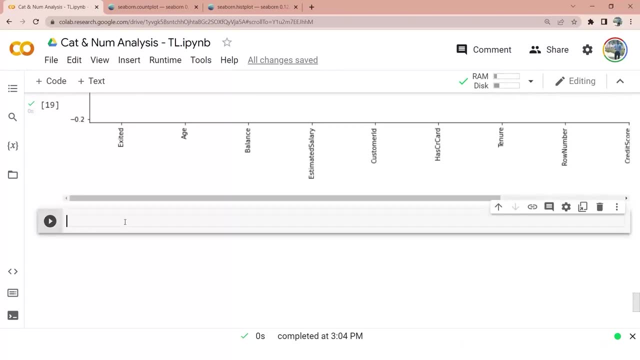 features are very important, so i will not consider and you can see number of products and is the very important with respect to exited. so this is what my insight we are getting from here. next step is: i will simply plot my correlation function, which we did right now, which was this: we will plot this correlation function using a heat map. 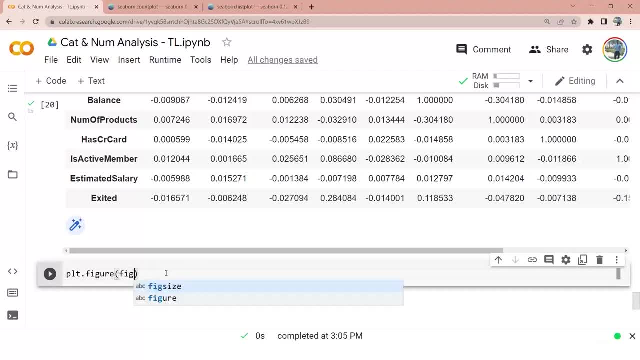 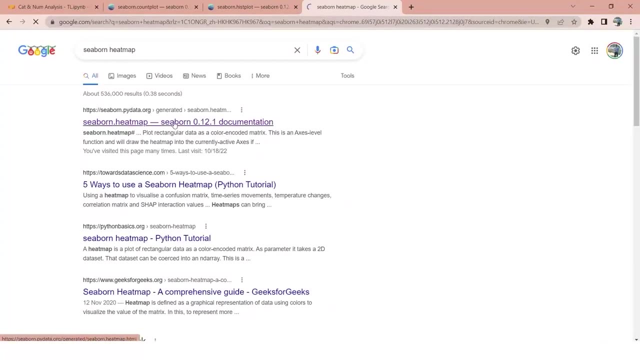 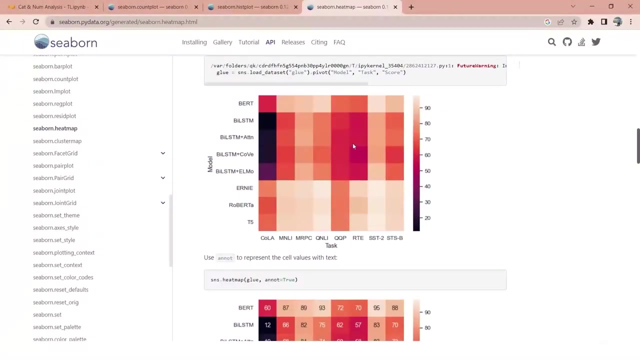 so i will use the same concept. plt dot figure fix size equals to 20 cross 12. cross 12 because it's a square. seaborn dot heat map. you can see seaborn heat map. it's a plot, a rectangular data as a colour encoded matrix, and if you scroll down you will see some graphs like this: this is a heat map. 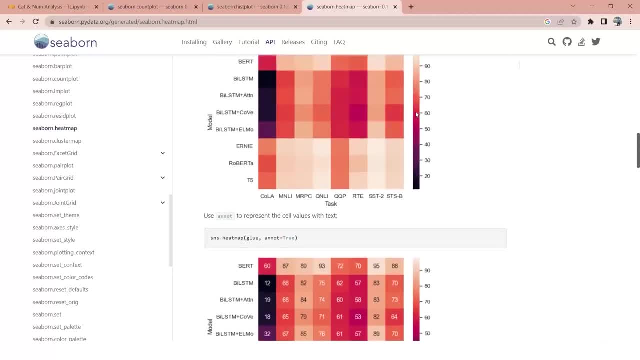 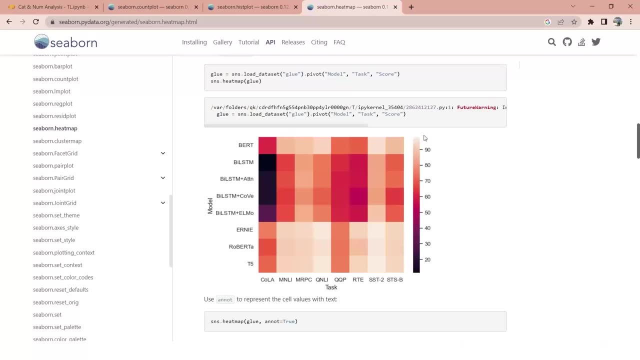 column. with respect to column okay, and you can see, on the right hand side you will see a scale that means the lower the number, the darker it is and the higher the number, lighter it is. so you can easily spot where you have lighter values and where you have the darker. 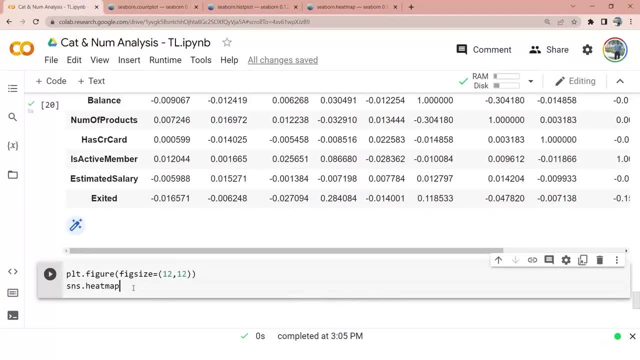 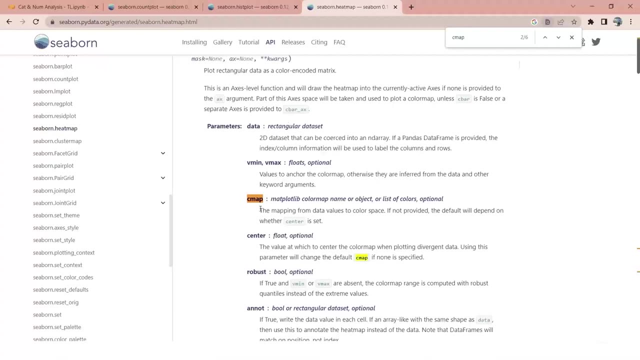 values. right, so we will be using the same concept. heat map of telco based data. dot correlation. there is a. there is a function called a c map. okay, if you go and check c map, there is a function: which type of c map you want to use. crest c map will give something like this: 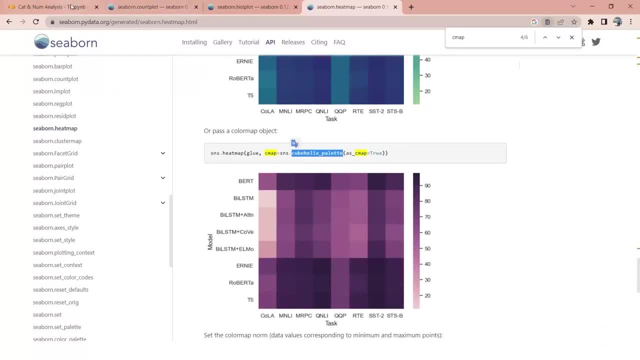 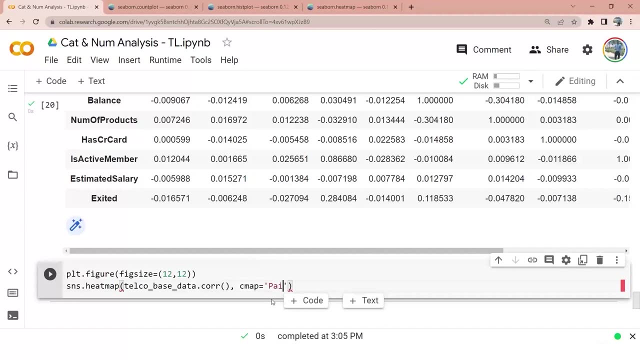 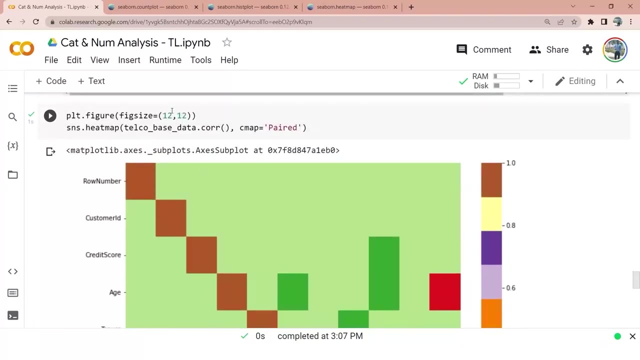 cube helix will give something like this. so you can use cube helix or, you know, crest, whatever you want to. i will simply use a paired one paired. there are multiple options, so i will be using paired and this is how my graph looks like. i will just make it little bit small so that it fits my 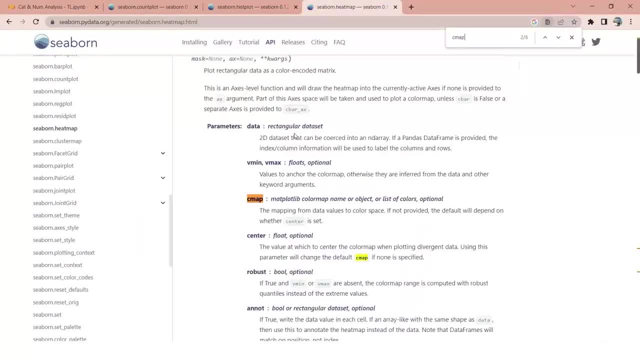 there is a function called a c map. okay, if you go and check c map, there is a function which type of c map you want to use- crest cmap- when you go and check the map done for such like this. so we're using the same concept. that's why i'm leaving it as the model as possible. after we score it, we're. going to be using the Pete there. so what we can do in this region. look at the through the el idol: yes, so according to all the upper and lower expressions, r sausage check, those are the same values. so as we'll be using里 map here for trust, us give us a hitm. prefer you don't click on this map? go ahead and click the Save field, then hit the right number. select the hitting laid inside. 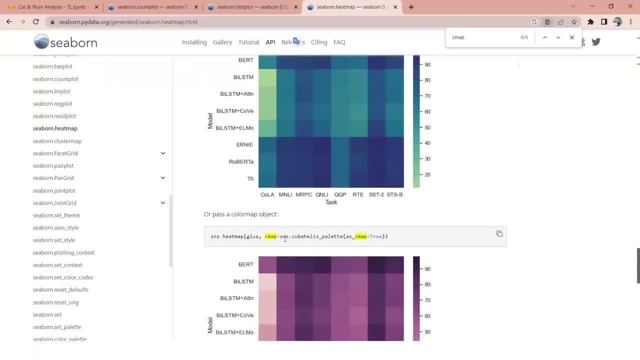 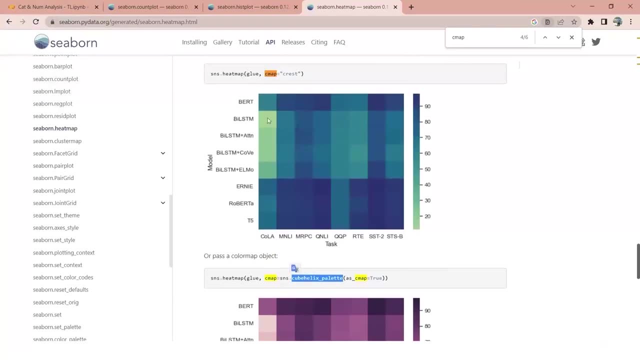 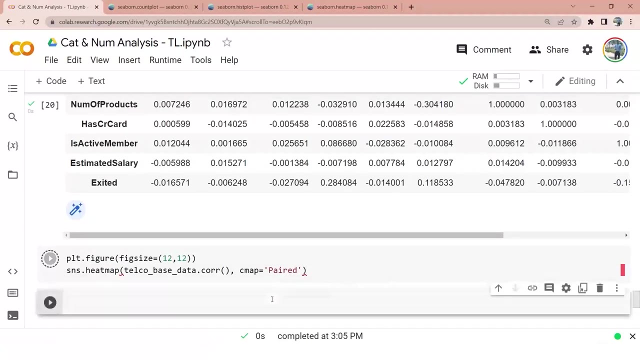 Crest Cmap will give something like this. Cube Helix will give something like this, so you can use Cube Helix or, you know, Crest. whatever you want to. I will simply use a paired, one paired. there are multiple options, so I will be using paired and this is how my graph looks. 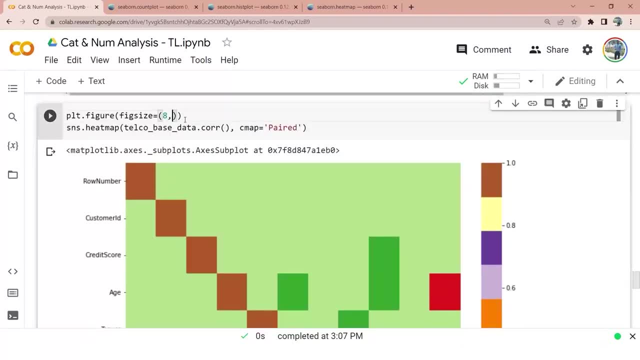 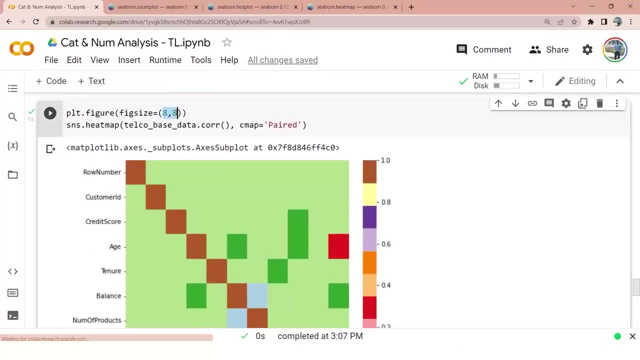 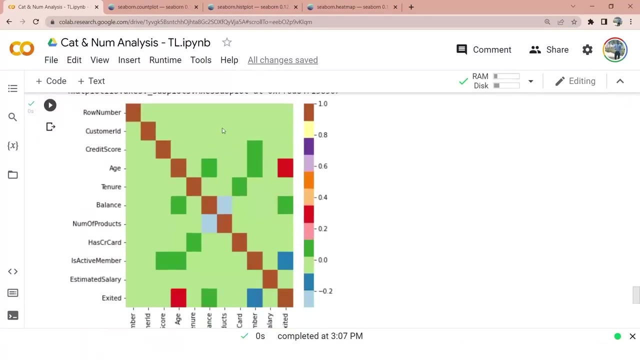 like. I will just make it little bit small so that it fits my screen and you can see again. I will make it even smaller. it is still not visible properly and you can see. this is my graph. how do we interpret this graph? let's say, sky blue is negative correlation. 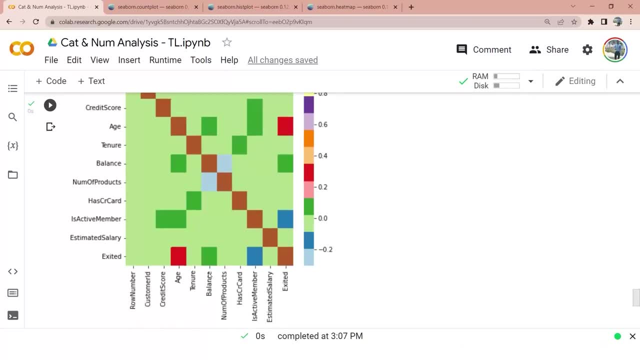 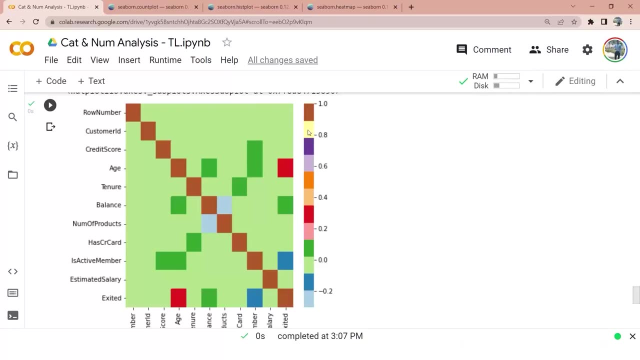 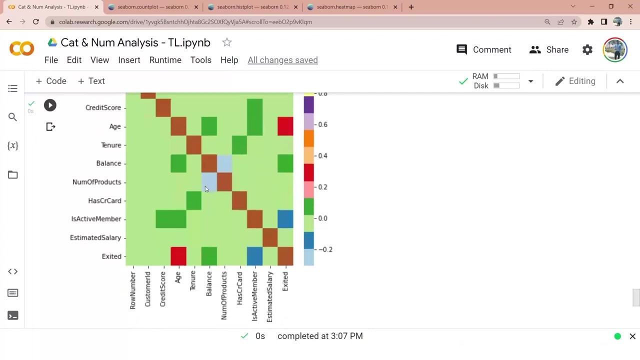 easily identifiable right number of products and balance are negatively correlated. so anything into this box, nothing. anything into yellow, nothing. anything into purple, nothing, nothing orangey, nothing red, yeah, red age with respect to exited high correlation and these one green ones are very low positive correlation, or you can say no correlation, so this is giving. 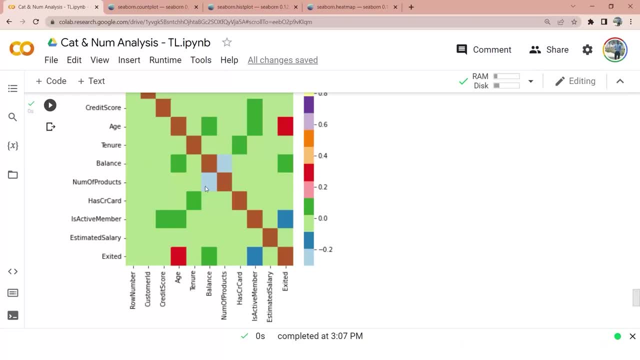 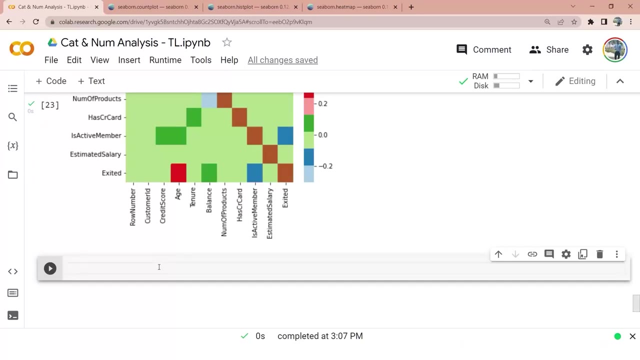 me an insight that age is an important factor, and even number of products with respect to balance right. so that's how you plot your heatmap. we will also try to cover some other plots so that we can also analyze few other numerical attributes. now the simplest thing that we can do is we have this data frame. 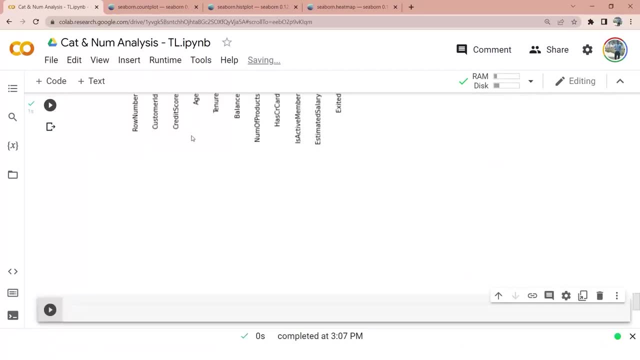 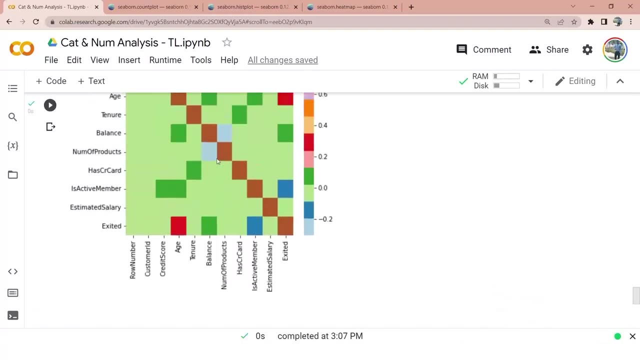 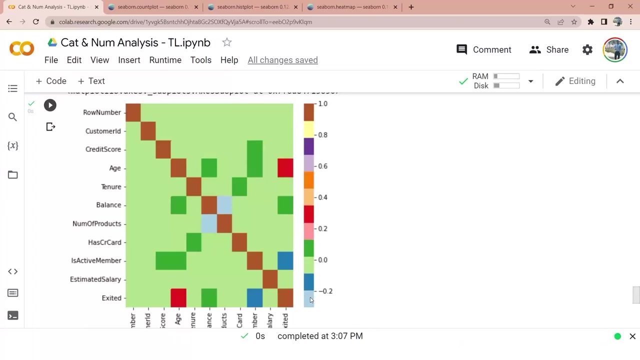 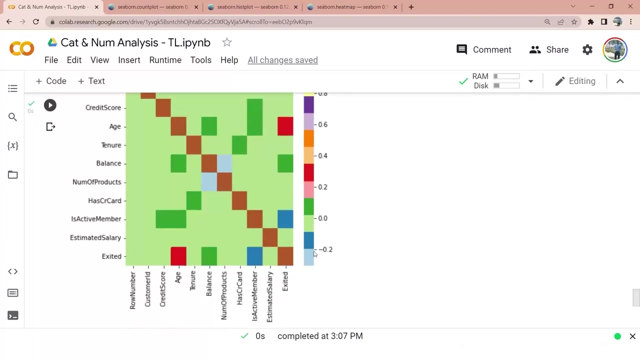 screen and you can see again. i will make it even smaller. it is still not visible properly and you can see. this is my graph. how do we interpret this graph? let's say, sky blue is negative correlation, easily identifiable. right number of products and balance are negatively correlated. anything into this box, nothing, anything. 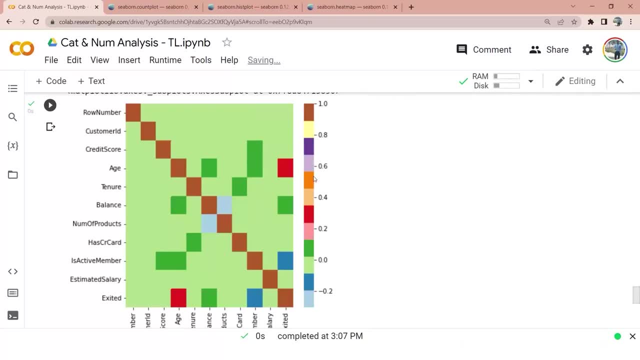 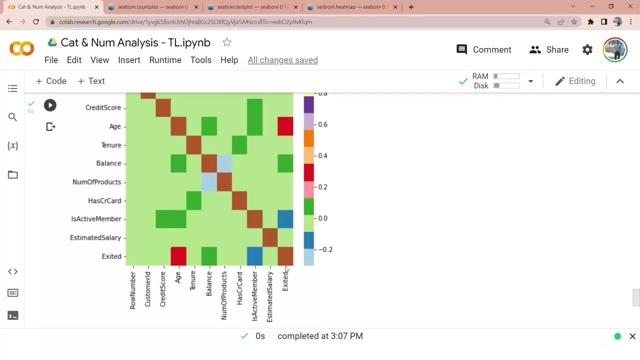 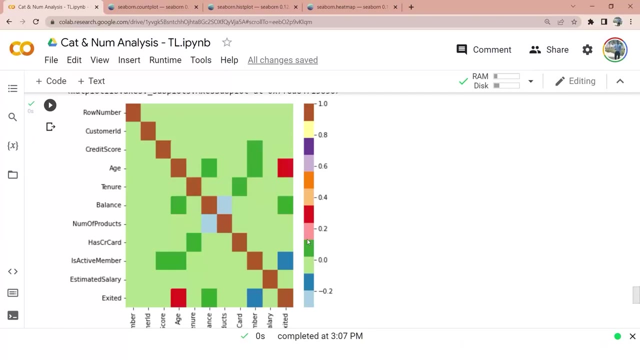 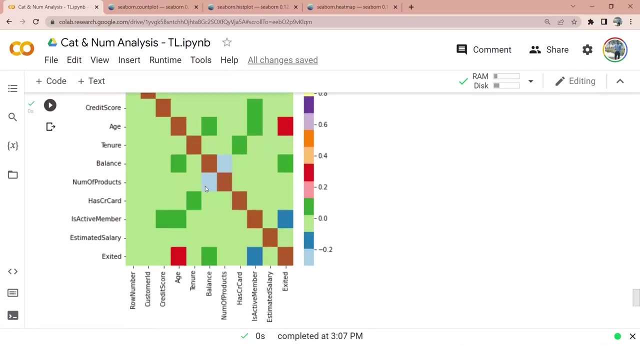 into yellow, nothing, anything into purple, nothing, nothing, orangey, nothing. it's red, yeah, red edge with respect to exited high correlation and these one green ones are very low positive correlation or you can say no correlation. so this is giving me an insight that age is an important factor and even number of products. 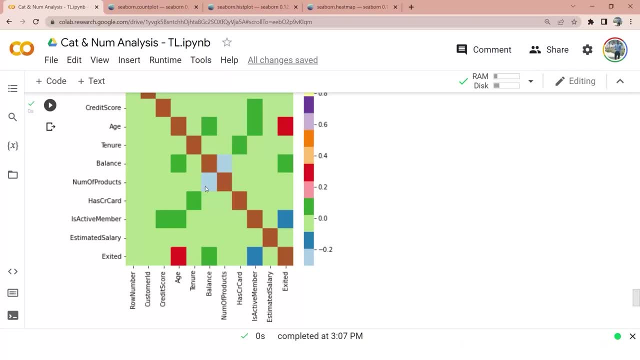 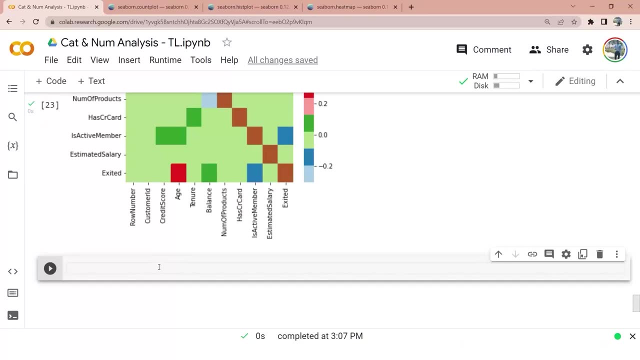 with respect to balance, right. so that's how you plot your heat map. we will also try to cover some other plots so that we can also analyze few other numerical attributes. now the simplest thing that we can do is we have this data frame, base data- no, not base. 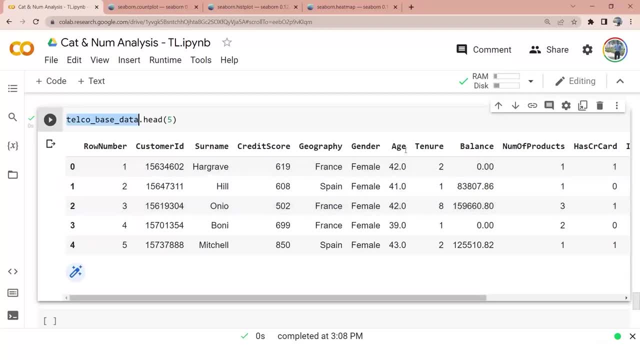 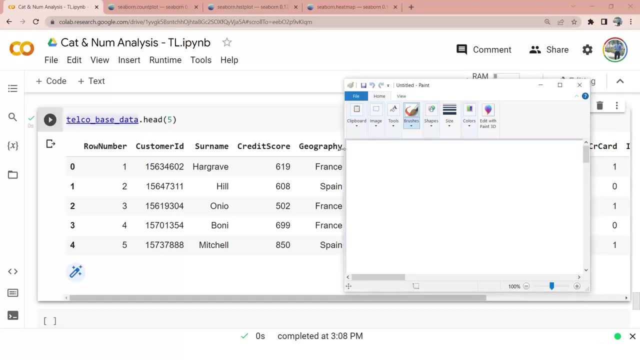 data. yeah, we have base data. so let's say age. let's say I want to analyze age. we all know age is a numerical column, right? it has values ranging from something to something. if you sort it out, you will be able to get it. if you want to plot age, will you be able to plot using a bar chart? a bar chart will. 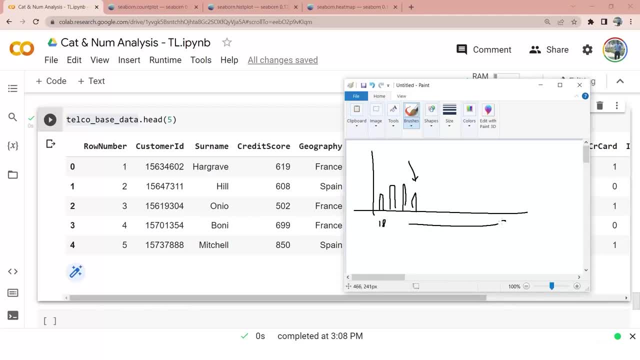 be very clumsy because it could range from 18 till 92 or 95. it could have a lot of bars which will make it look very clumsy. a better way of analyzing it will be using a line chart or, if you convert it into age bins, probably you will be able to visualize. 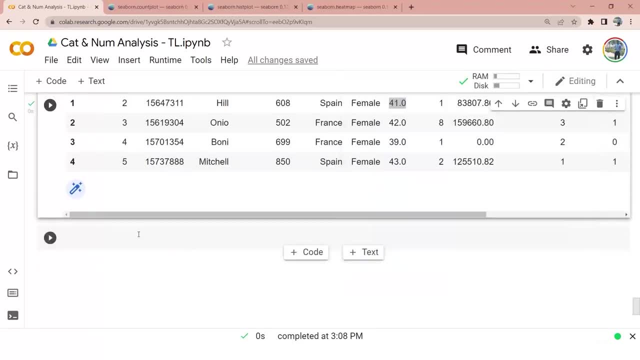 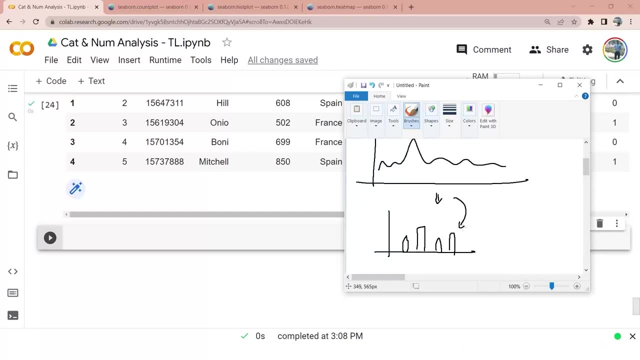 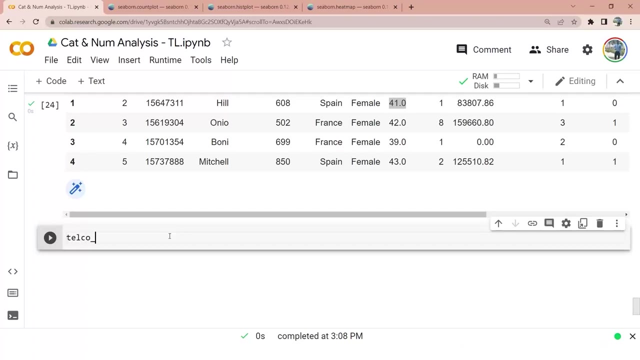 the bins, three to four bins. so converting it into bins will be taught in the next class, where we will teach you the derived matrix. but without converting into bins, let's try to plot it using a line chart. so telco, base data of age, and then I will do value counts. 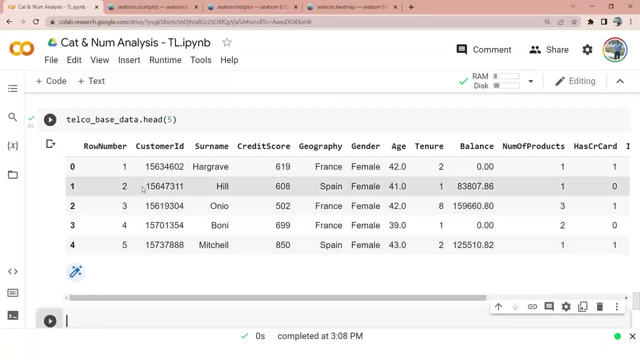 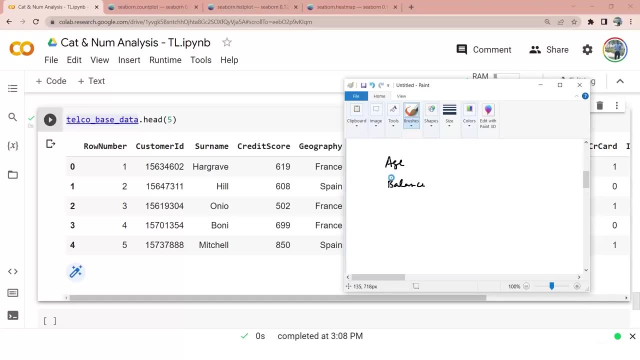 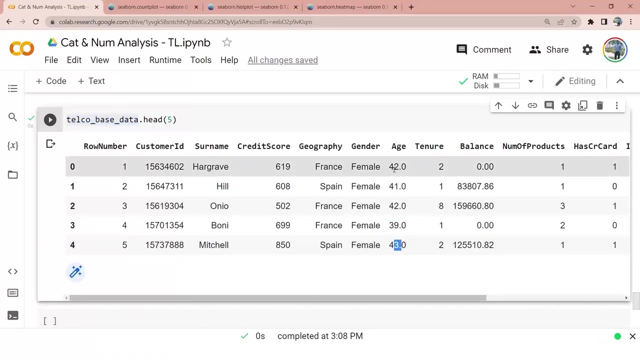 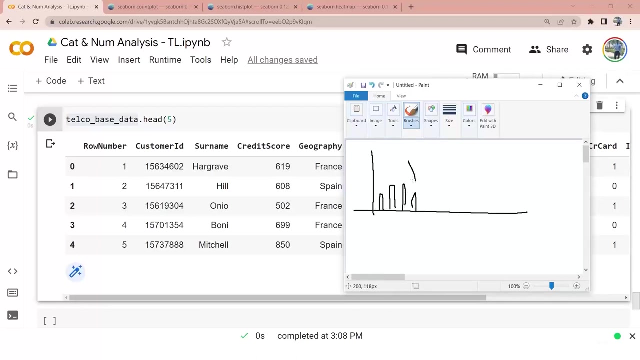 base data? no, not base data. yeah, we have base data. so let's say age. let's say: I want to analyze age. we all know age is a numerical column, right? it has values ranging from something to something. if you sort it out, you will be able to get it. if you want to plot age, will you be able to plot using a bar chart, a bar. 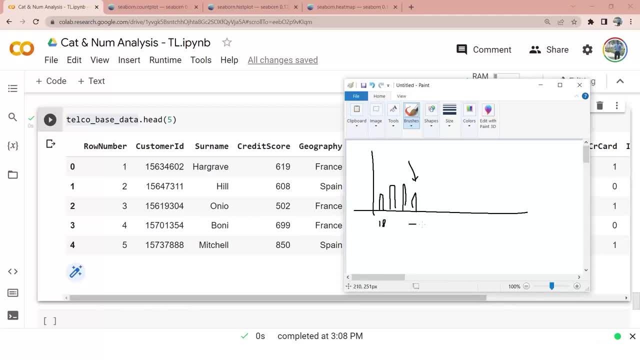 chart will be very clumsy because it could range from 18 till 92 or 95. it could have a lot of bars which will make it look very clumsy. a better way of analyzing it will be using a line chart or if you convert it into age. 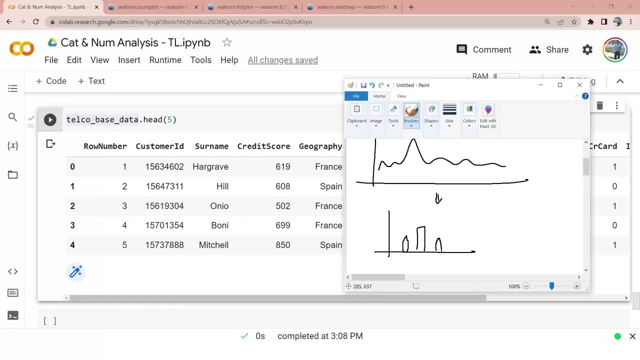 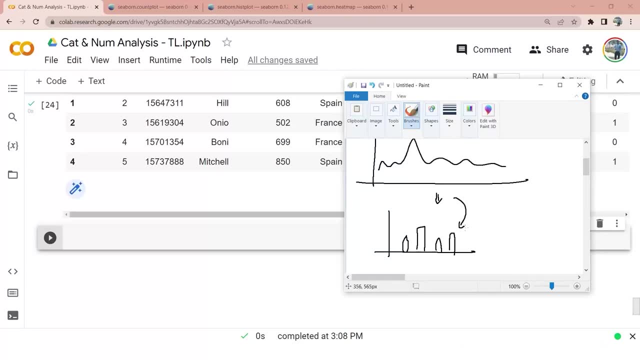 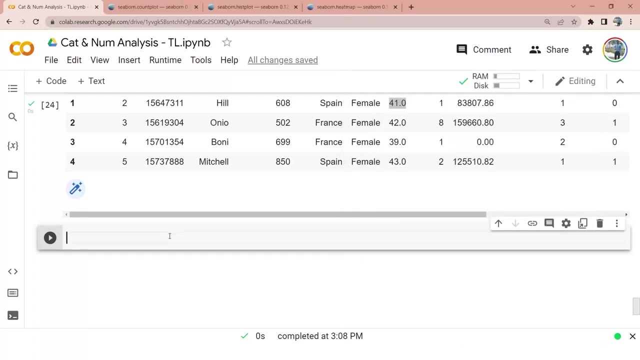 bins. probably you will be able to visualize the bins- three to four bins- so converting it into bins will be taught in the next class where we will teach you the derived matrix. but without converting into bins, let's try to plot it using a line chart. so telco based. 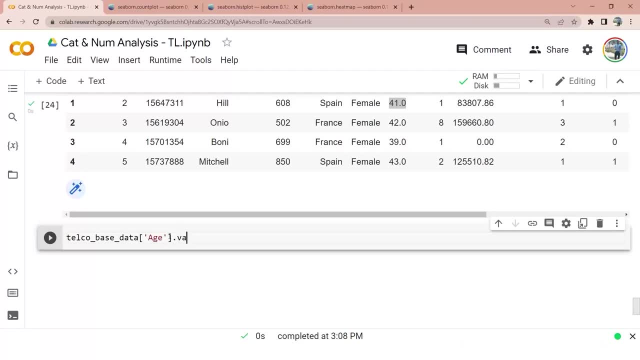 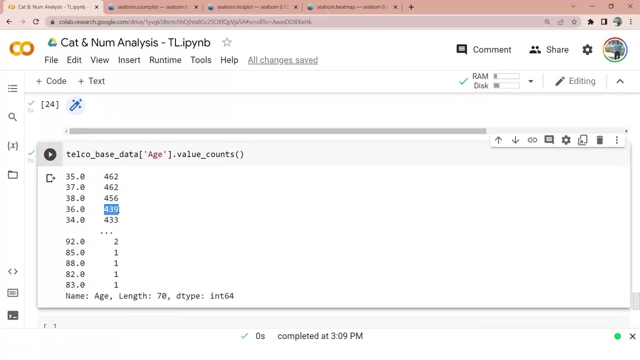 data of age and then I will do value counts and then I will sort the index, because my index here is- let me go line by line- so when I am doing dot value counts you can see for each age I am getting the total number of values. what is my index? my age is my index, so I will sort. 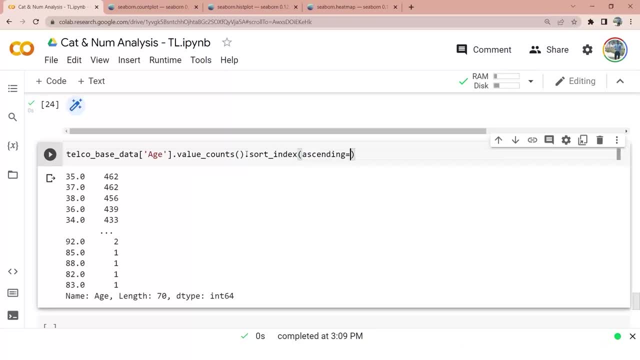 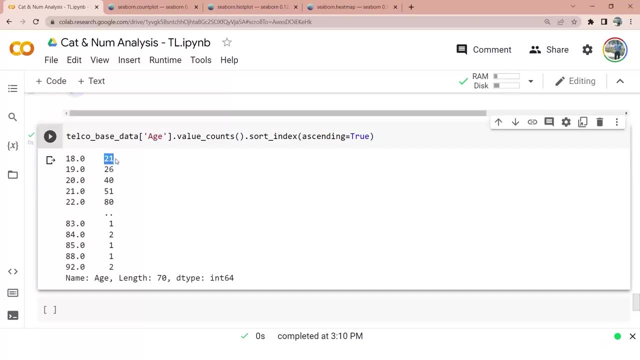 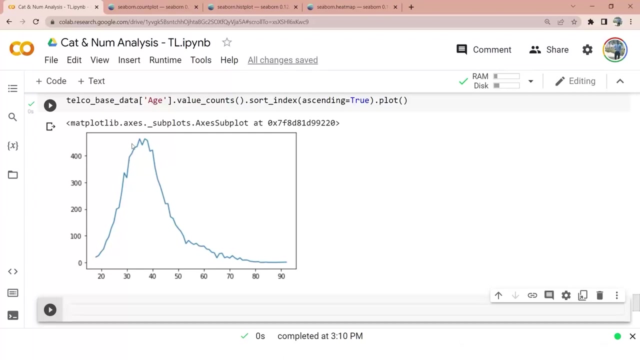 my index, how ascending equals to 2. once that is done, if you plot it, if you just print it, typeあと, the lowest age is at first and the highest age is at end, and then simply do lot. if you plot, by default it will be plotting your line chart, which basically tells you. 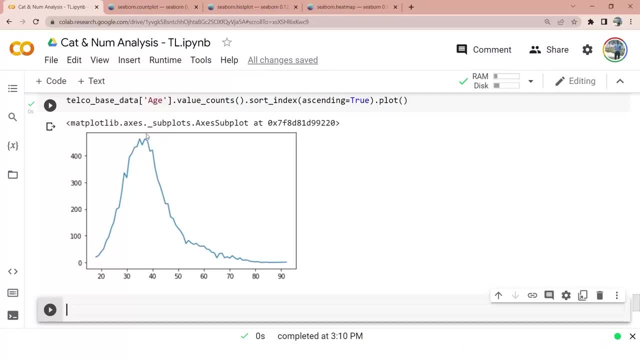 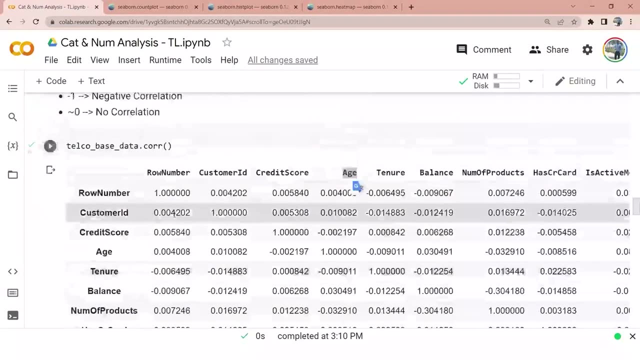 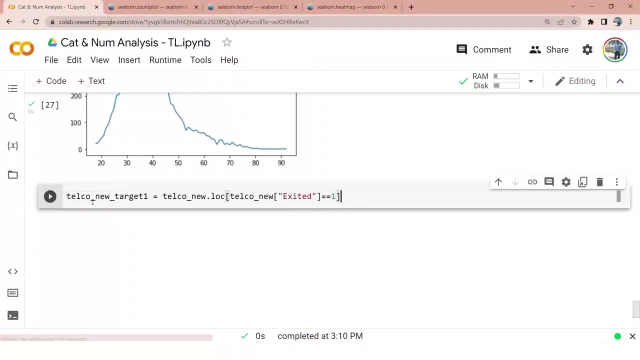 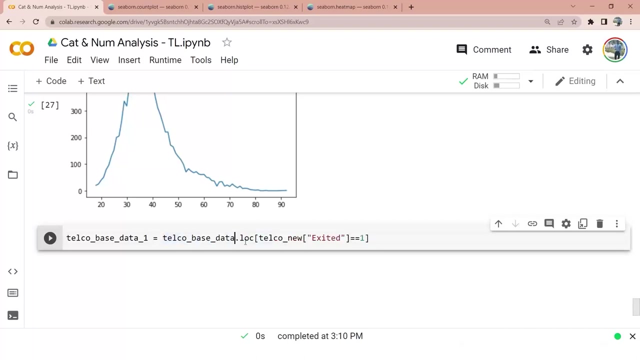 that most of the people- average people- are ranging around this age. let's try to do the same activity for the churn customers. so I will. i will exactly do the same thing what we did earlier. i will create another data frame- telco base data- for one telco base data, telco base data done, and then i will copy paste this code. 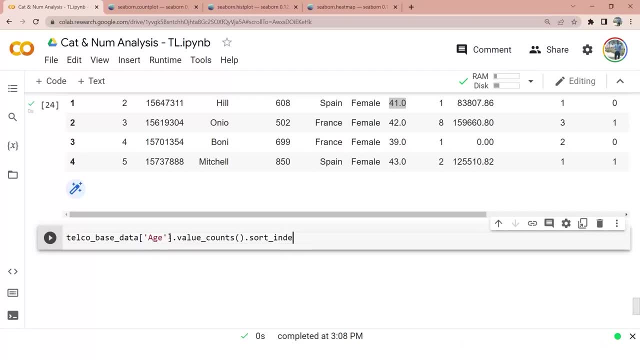 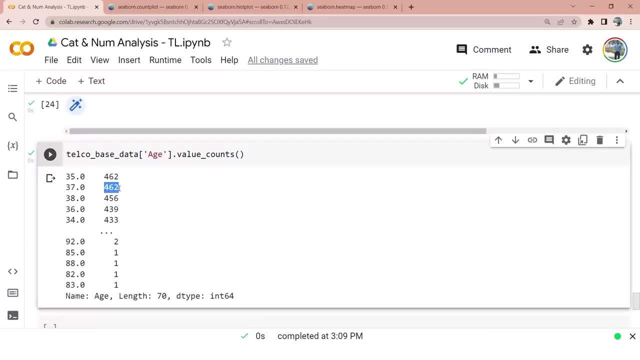 and then I will sort the index, because my index here is, let me go line by line, so when I am doing dot value counts, you can see for each age I am getting the total number of values. what is my index? my age is my index, so I will sort my. 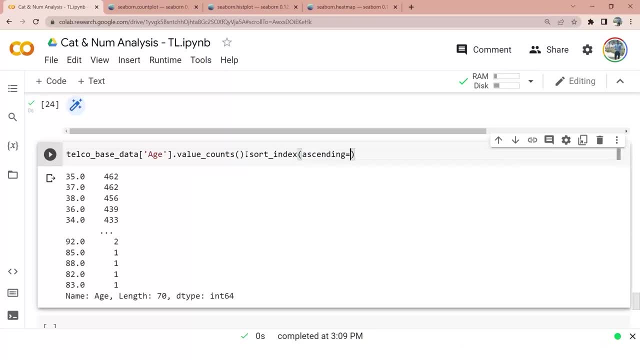 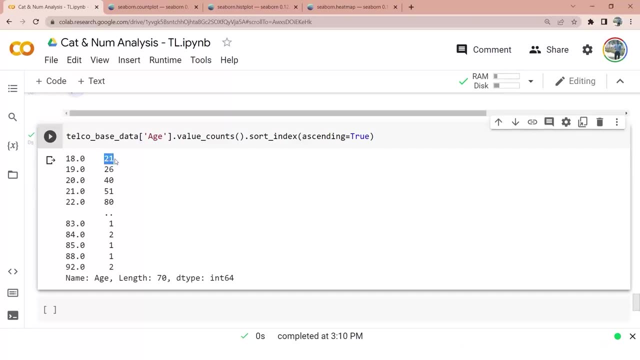 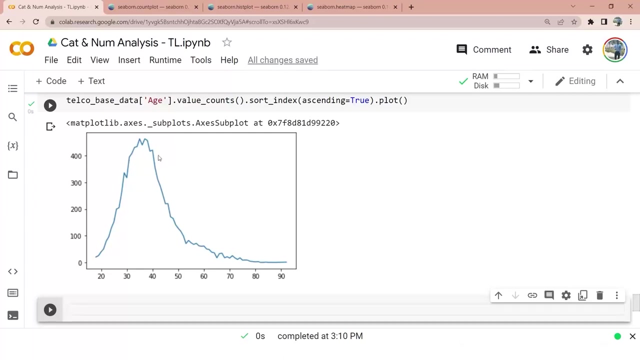 index how ascending equals to two. once that is done, if you plot it, if you just print it, the lowest age is at first and the highest is at end, and then simply do lot. if you plot, by default it will be plotting your line chart, which basically tells you that most of the people, average people- 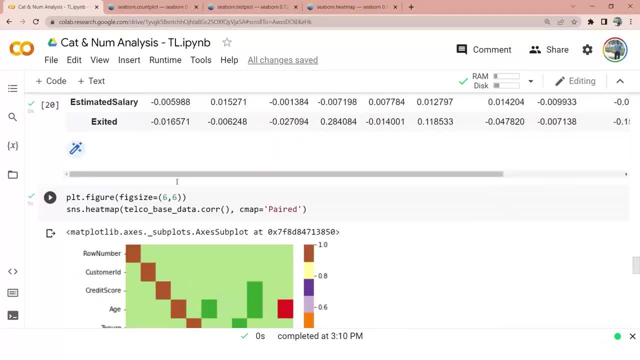 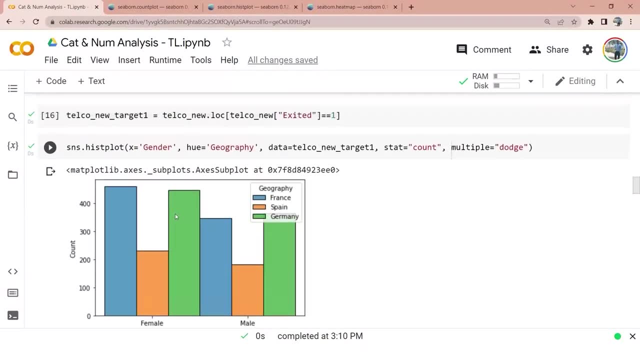 are ranging around this age. let's try to do the same activity for the churn customers, so I will. I will exactly do the same thing what we did earlier. so I will do the same activity for the churn customers, so I will. I will exactly do the same thing what we did earlier. so I will. I will exactly do the same thing what we. 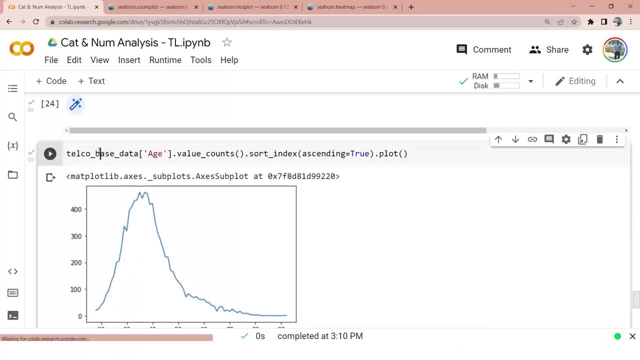 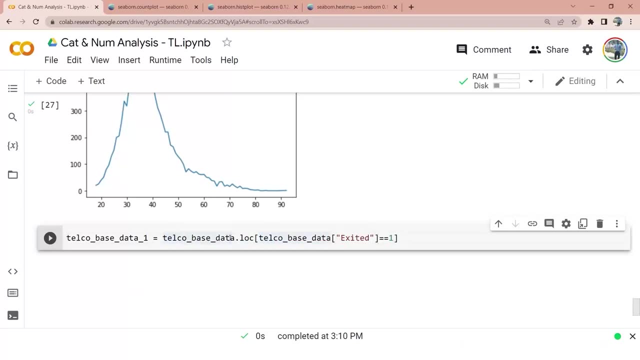 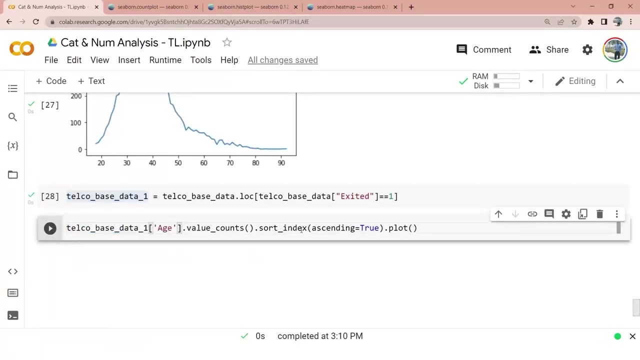 did earlier, I will create another data frame- telco base data- for one telco base data. telco base data done, and then I will copy paste this code and this is for only for the exited customers. I will change it to this, that's it and plot it. 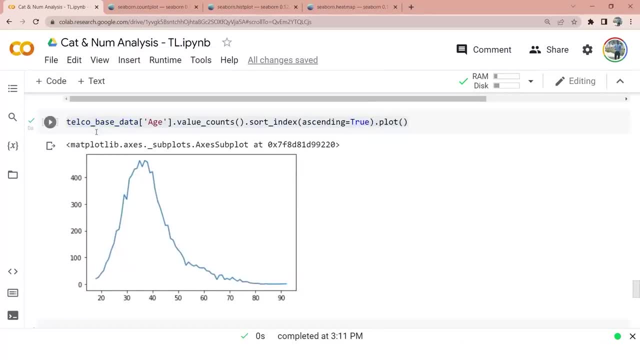 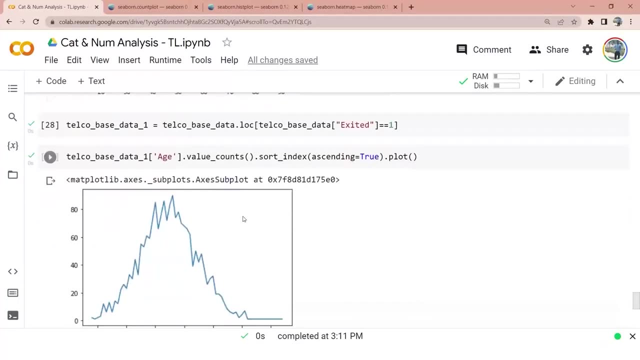 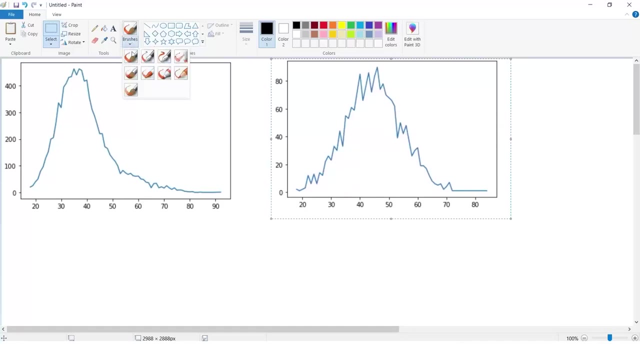 now you can see if I take this graph to this graph and I will just keep this one. but this is my first quiz now. I will put this in my next week. I will post it in the next week, so I will put this in the next week. I will post it in the next week, so I will put this in the next week. 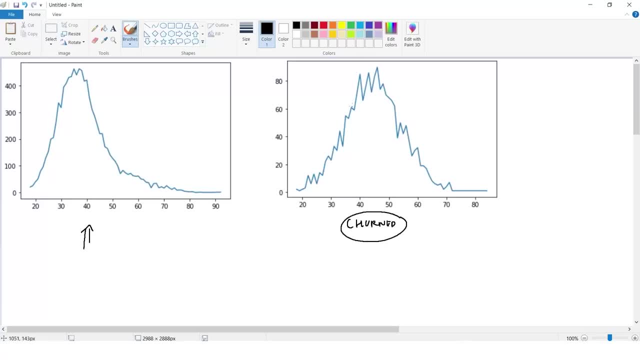 because I want to get all the information from my next week and your audience to know that I have done it first. so I will say, okay, if I just leave this here, I will try to do the same thing that I did earlier. this is my qu ref change. now let's see what happens if I change this to my next week. I will 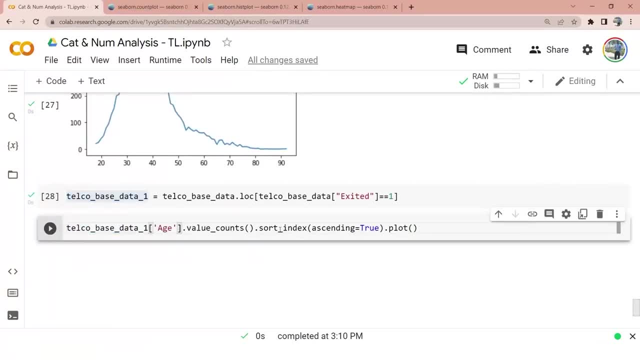 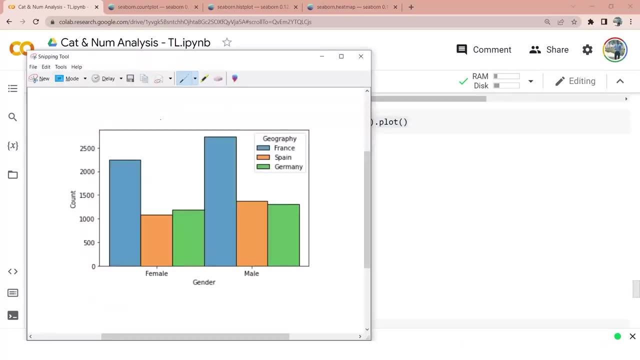 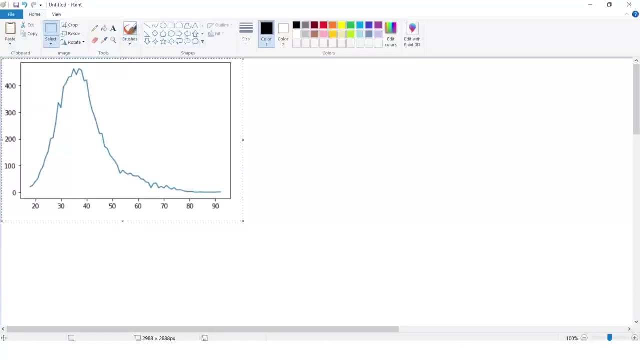 and this is for only for the exited customers. i will change it to this. that's it and plot it now. you can see if i take this graph to the next one, and probably this one. now. this is your original data and this is your churn data. you can see in the churn data. 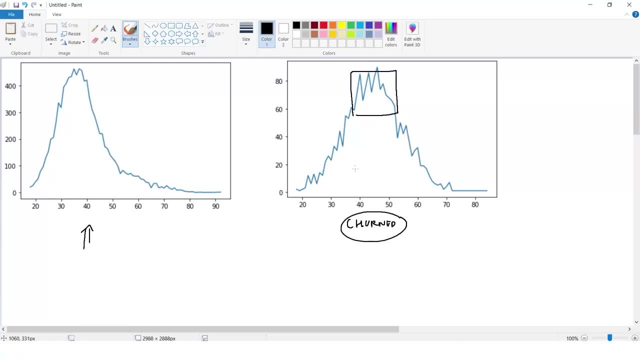 most of the people are around this range, which is around 40 to 55. but in the original data most of the people are in this range around 28 or 27 to 47 or 48. that means people who are churning. age is an important factor: people who are churning. they are more in age, they are some senior people. 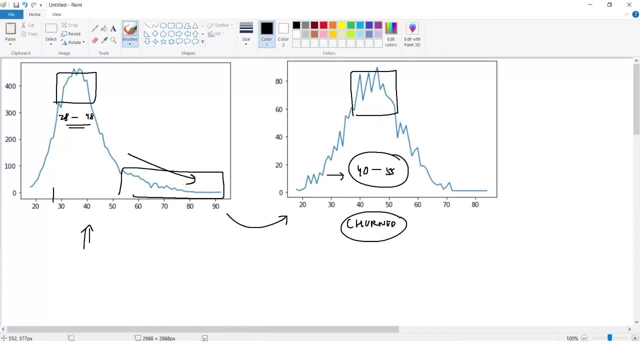 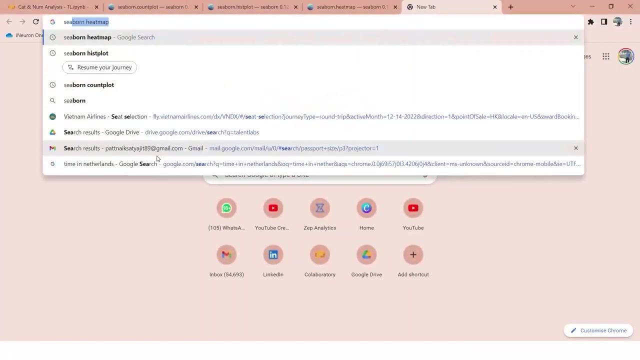 and you can see beyond this line the graph has almost dead. but here during 60 to 70, you can see good amount of spike right. so age is an important factor and we are able to get that from this graph also right. similarly, we will also plot some other graphs. there is seaborn. 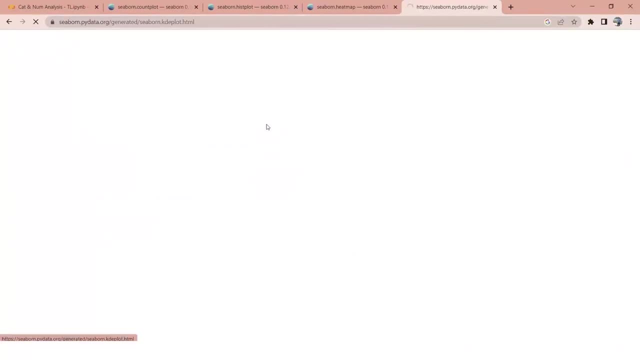 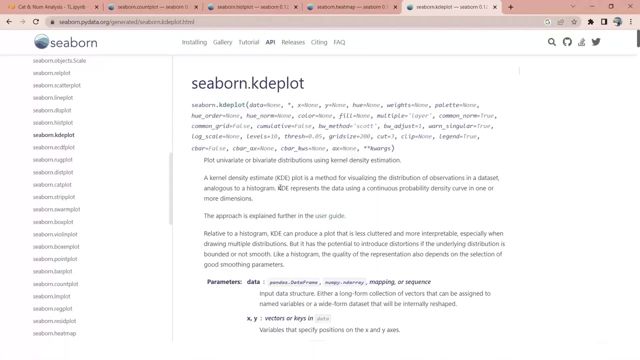 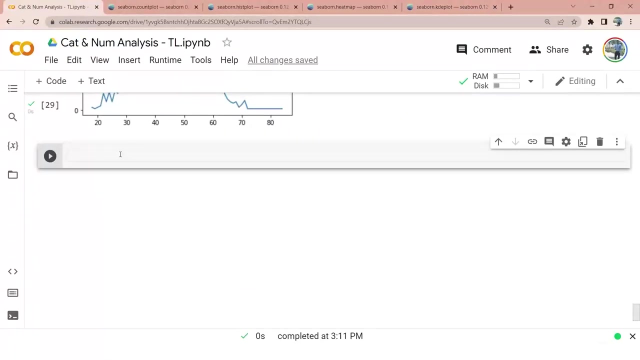 kd plot, which is kernel density estimation plot. it is used to visualize the distribution of observations in a data set analogous to a histogram. kd represents the data using a continuous probability density curve, so we'll try to use this. so let's say i will define kd plot. telco base data. 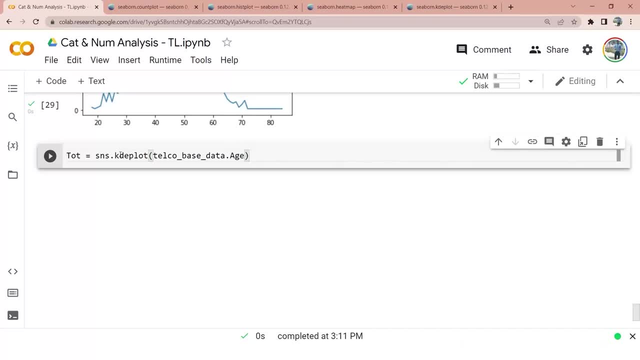 let's say i will analyze my age. okay. age telco base data exhibited equals to equals to zero. let's say i want to have a color as red for my exited people. shade equals to true. okay. and then simply i will copy paste this where exit it equals to one and i will change the color to blue. 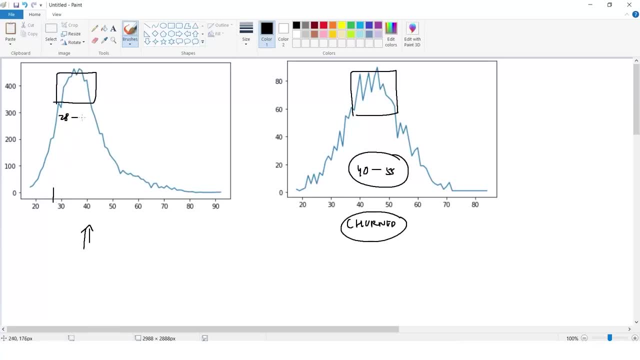 this range around 28 or 27 to 47 or 48. that means people who are churning. age is an important factor. people who are churning, they are more in age, they are some senior people and you can see beyond this line the graph has almost dead. but here during 60 to 70 you can see good amount of spike right. 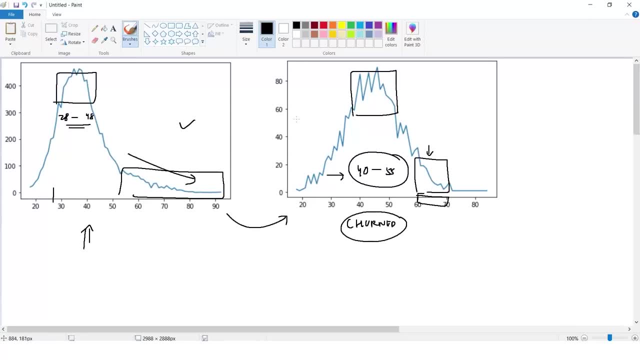 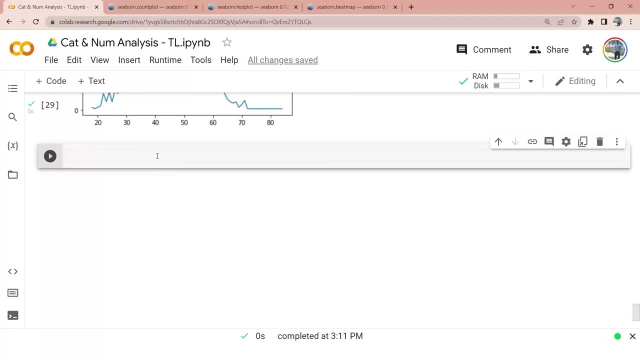 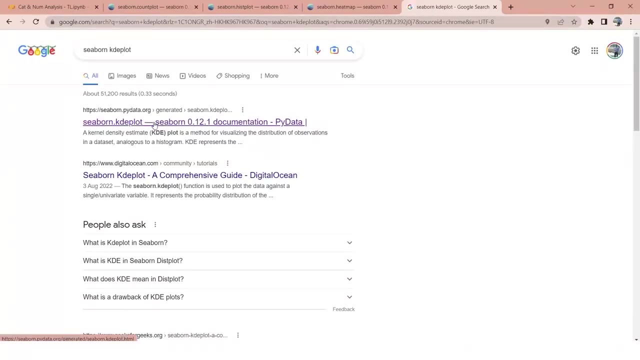 so age is an important factor and we are able to get that from this graph also right. similarly, we will also plot some other graphs. there is seaborn kd plot, which is kernel density estimation plot. it is used to visualize the distribution of the graph. and it is used to visualize the distribution of the graph and it is used to 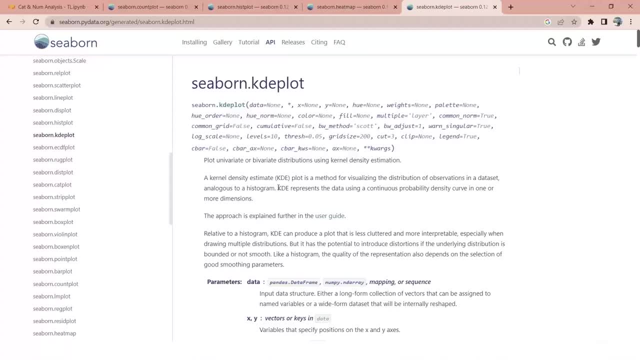 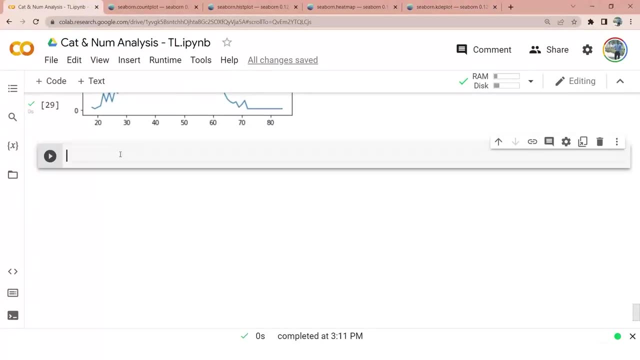 visualize the distribution of the graph, and it is used to visualize the distribution of the graph of observations in a data set analogous to a histogram. kd represents the data using a continuous probability density curve, so we will try to use this. so let's say i will define kd plot. 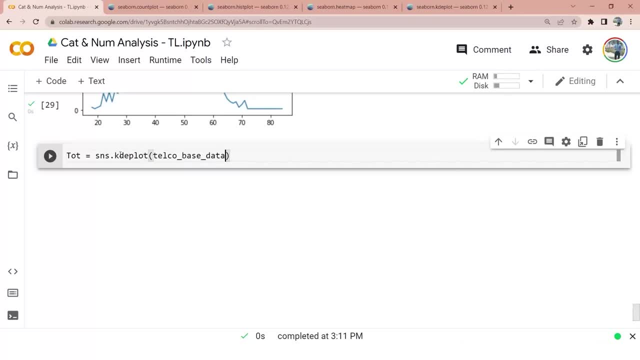 telco based data. let's say, i will analyze my age. okay, age telco based data exists. let's say i want to have a color as red for my exited people shade equals to true. okay, and then simply i will copy paste this where exit it equals to one, and i will change the color to blue. 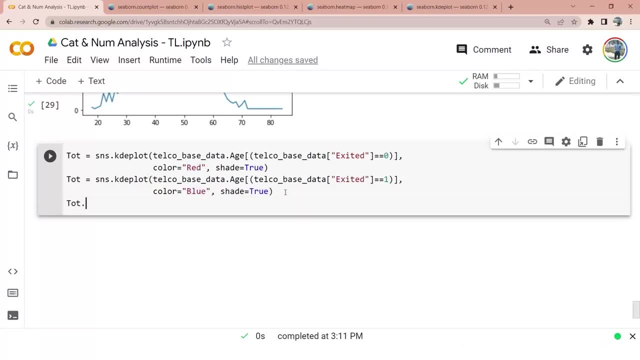 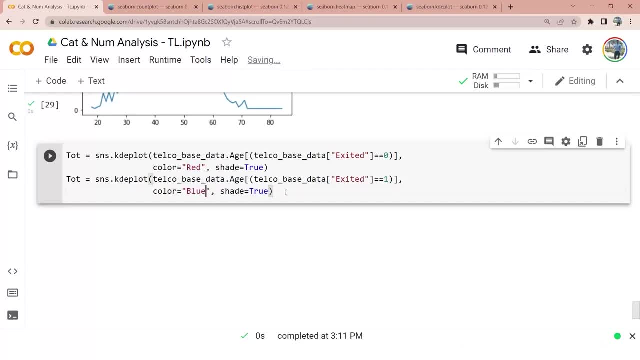 and then i will simply do dot, dot legend. let's say the first one. we need to change the color to red, and then we will simply copy paste it. first legend will be no churn, and the second one will be churned. and then this is the density function, because kernel density, 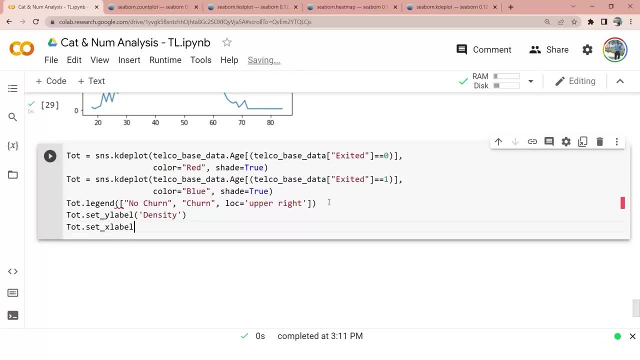 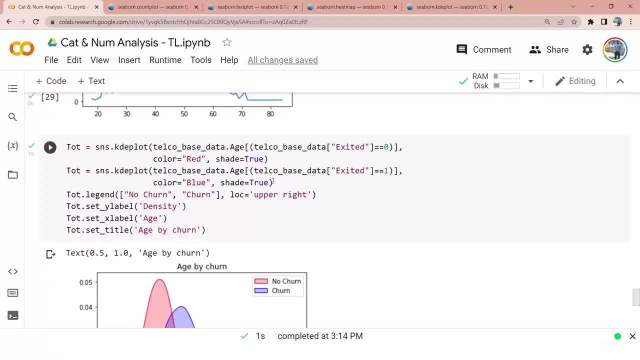 set x label is basically your age, and then i will set a title which is age by churn dot dot legend. yeah, looks fine, this one, this one. so now i'll run this code and you can see a graph will be shown where both churn customers and not churned customers are shown. the active customers are your red customers. 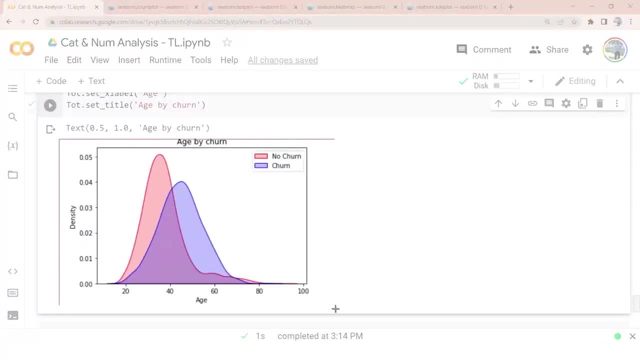 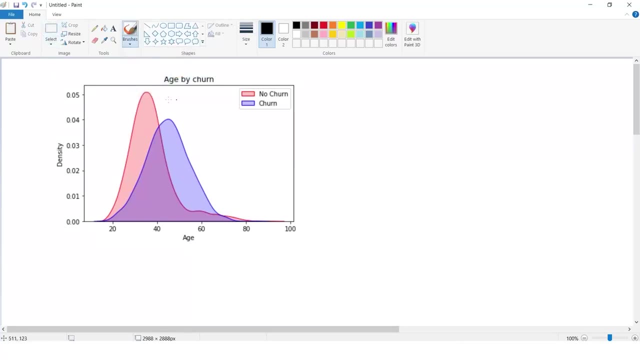 and inactive are your blue ones. so if i take it to my this thing and explain here, it is quite evident that people who are not churning- they are maximum having in this range. the edge is low people who are churning: the highest distribution is around this range, which is: 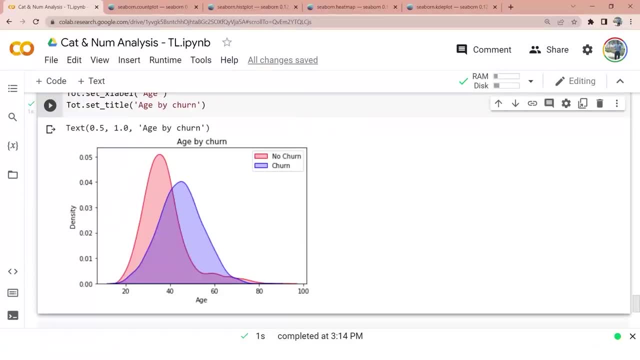 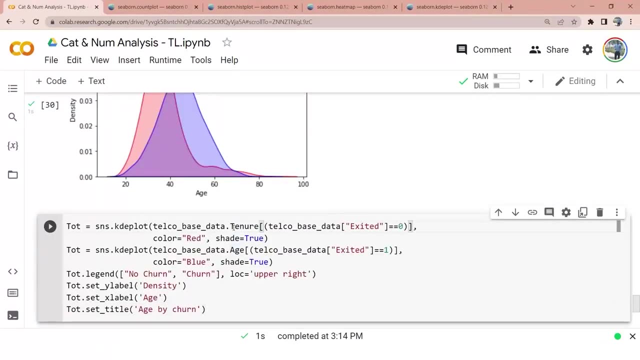 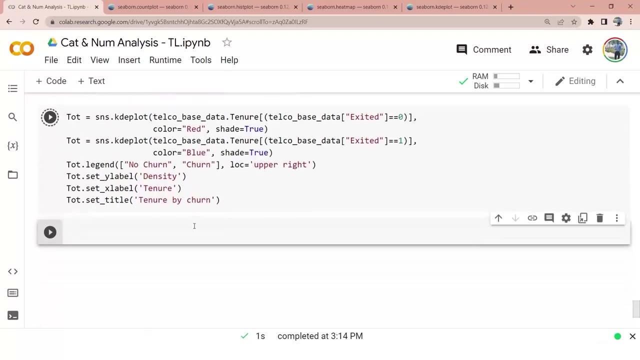 evident that age is an important factor. similarly, you can also use this same piece of code in analyzing other columns. let's say there is a column called as tenure, tenure, tenure and tenure. run this and you can see that this is your tenure graph. i don't see a huge impact with respect to 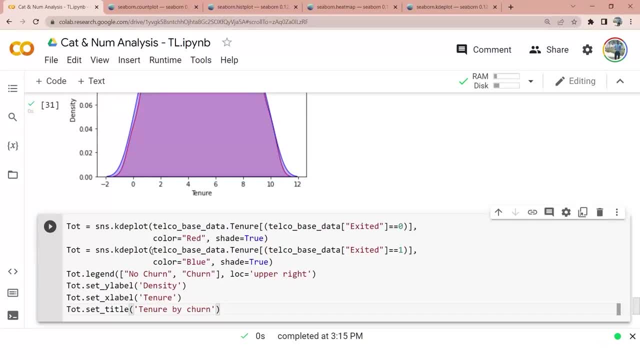 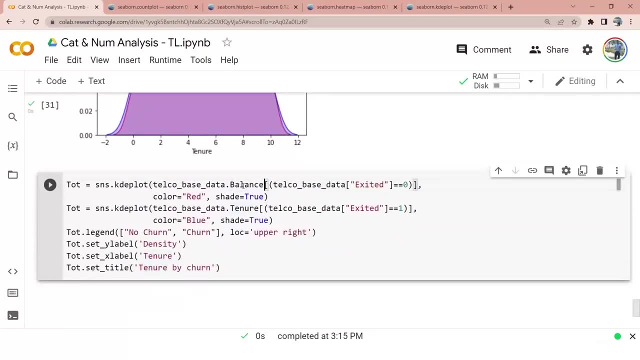 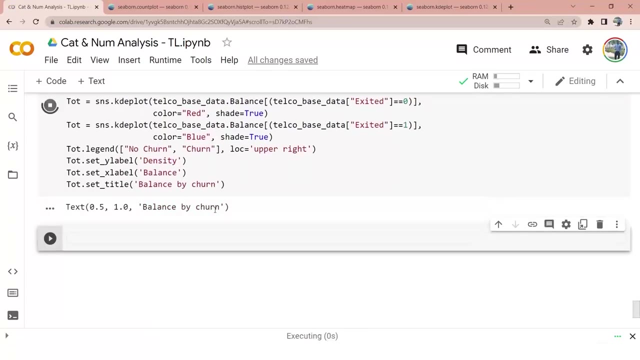 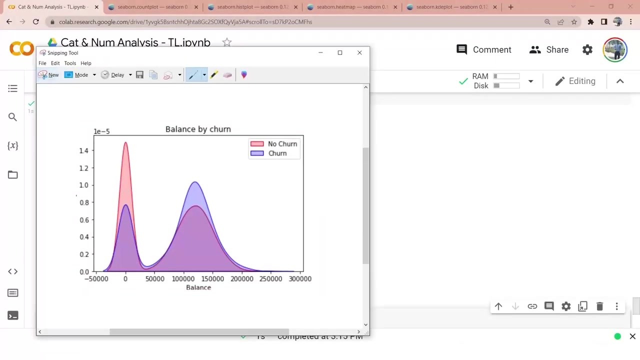 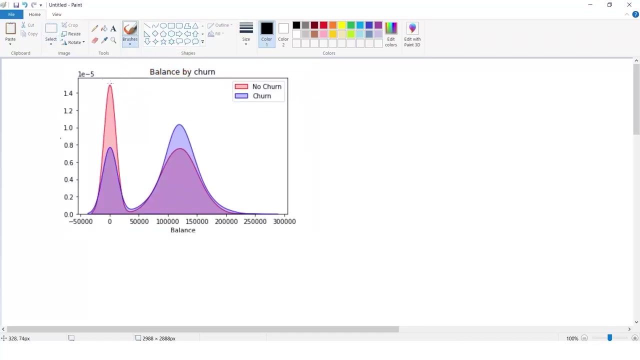 tenure any other numerical columns that we have. let's say, we have a numerical column called as balance, balance, balance, balance, balance. so what does my balance tell if i just use it? so, here, people who have not churned, they are mostly, you know, the density is high here people who have churned. 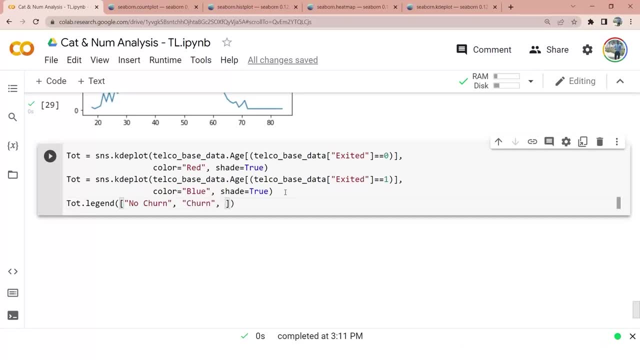 will be John. and then this is the density function, because kernel density, that X level, is basically your age, and then i will set a title which is age by churn dot dot legend: yeah, looks fine this one. yeah, this one. so now i'll run this code and you can see a graph will be shown. 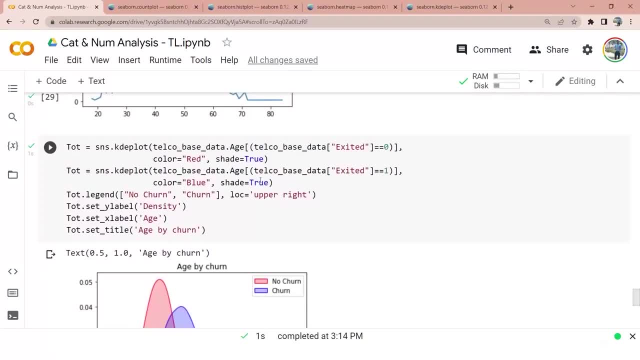 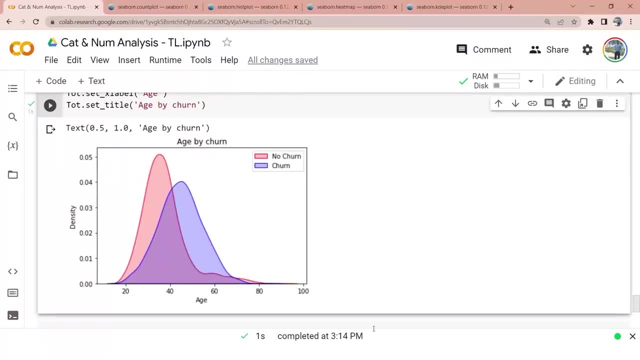 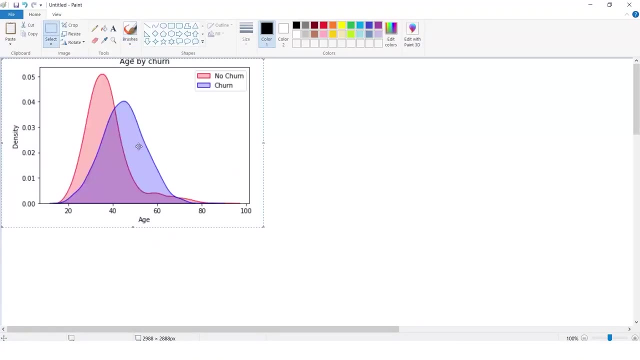 where both churned customers and not churned customers are shown. the active customers are your red customers and inactive are your blue ones. so if i take it to my this thing and explain here, it is quite evident that people who are not churning they are maximum having in this range. the age is low, people who are churning the highest. 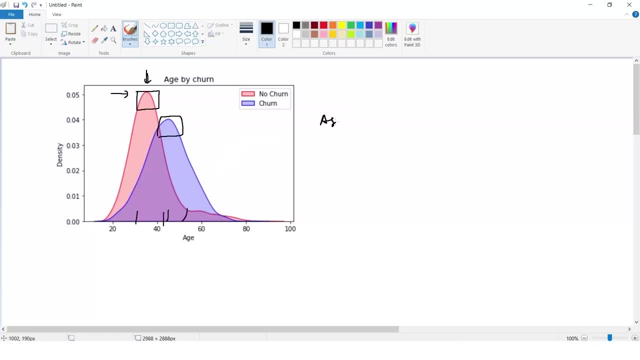 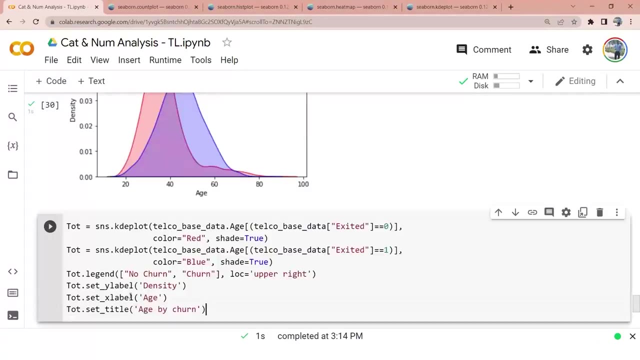 distribution is the age of the person who is churning. the age of the person who is churning is around this range, which is quite evident that age is an important factor. similarly, you can also use this same piece of code in analyzing other columns. let's say: 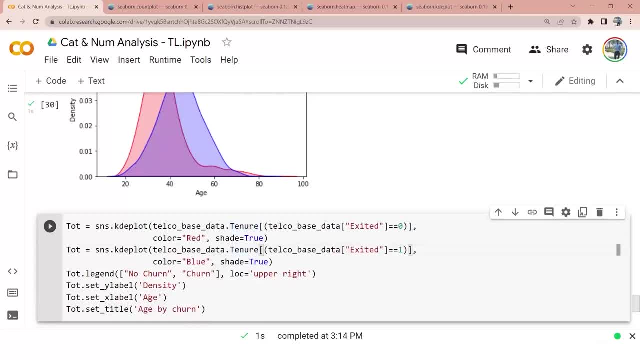 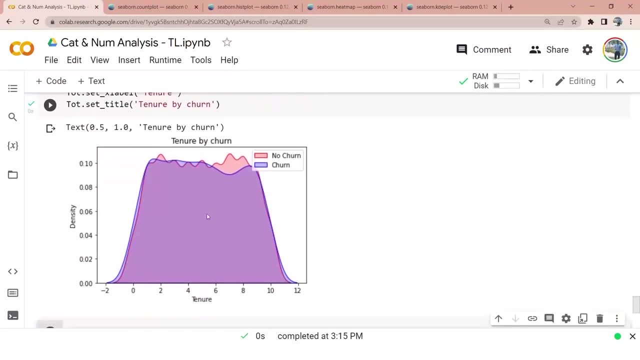 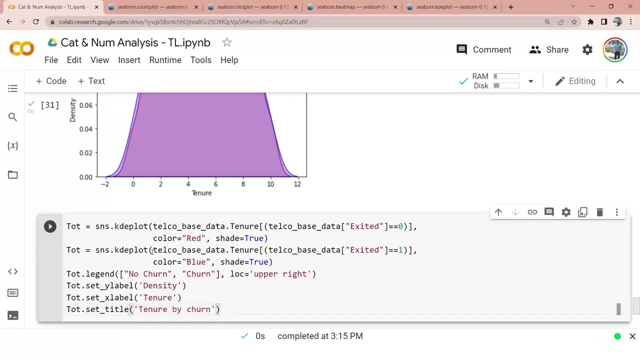 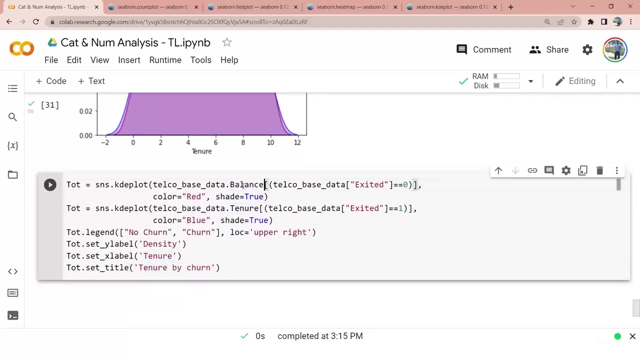 there is a column called as tenure, tenure, tenure and tenure. run this and you can see that this is your tenure graph. i don't see a huge impact with respect to tenure, tenure, any other numerical column that we have. let's say, we have a numerical column called as balance, balance, balance. 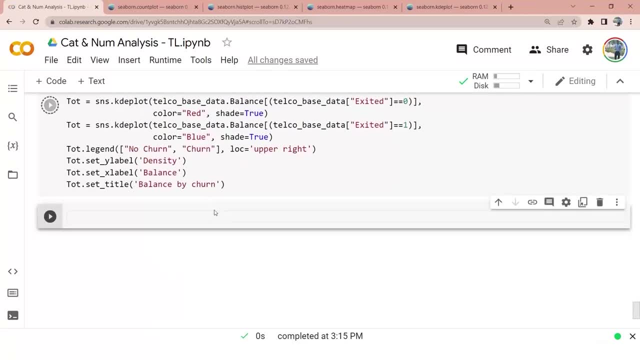 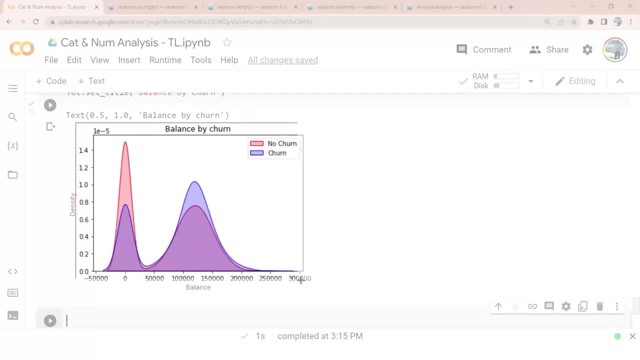 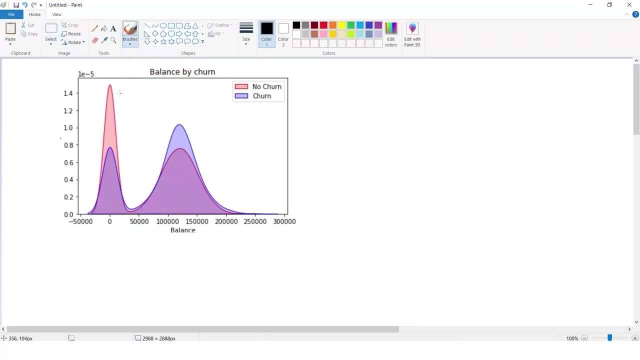 balance, balance. so what does my balance tell if i just use it? so here, people who have not churned, they are mostly, you know, people who have not churned. you know the density is high. here, people who have churned, the density is low. but when it comes to 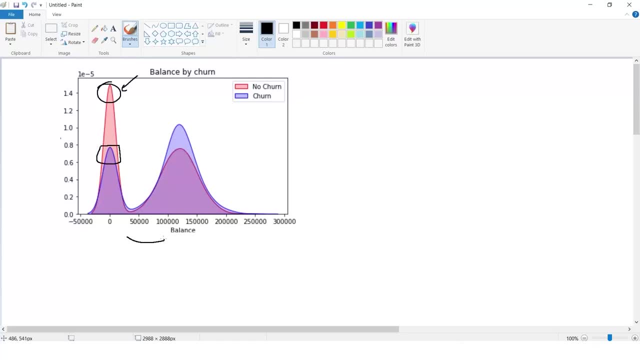 the density is low. but when it comes to larger balance, people who have churned are having larger density, larger balance here and less so. somehow, with less balance, there are less number of people who are churning, who are having less balance. people who are having more balance are more likely to churn because they have balance amount. 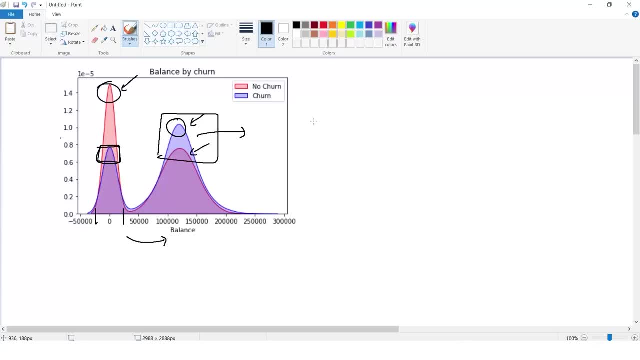 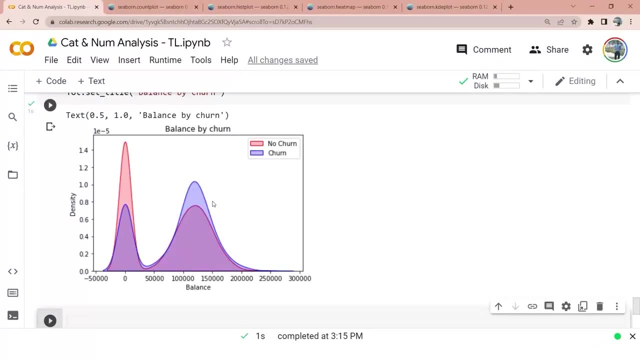 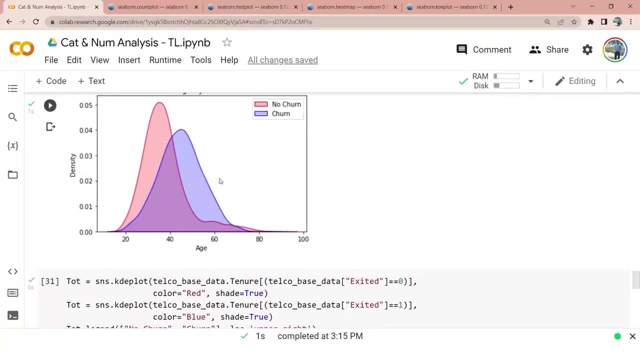 right. that means that amount they have to pay to the company. maybe because of that they are churning, so that they don't have to give that amount could be a reason, but this is, overall, giving you a understanding. so that's all about different types of analysis that we perform. 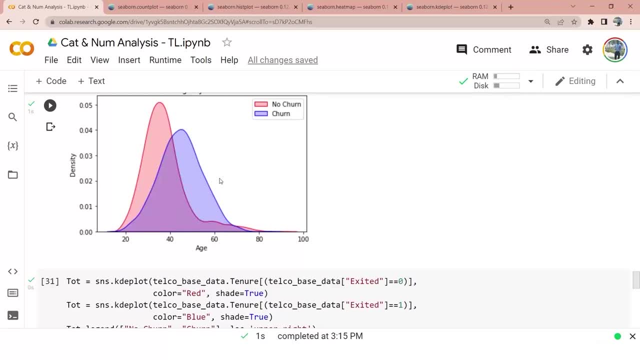 in the next videos we will be talking about derived matrix and then we will be jumping into a case study. in the case study, we will be taking similar churn analysis use case. we will be performing each and everything from scratch, starting from data cleaning, data collection, analysis and finding insights, which will be an end-to-end case study. 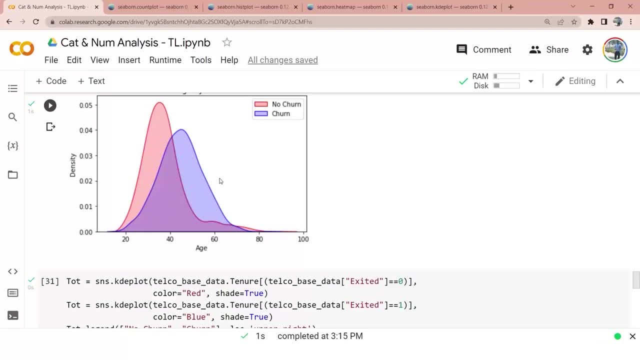 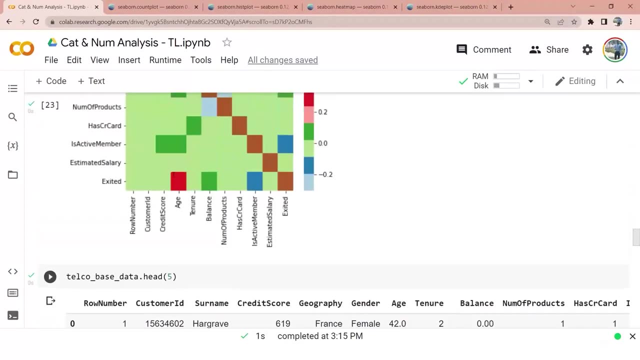 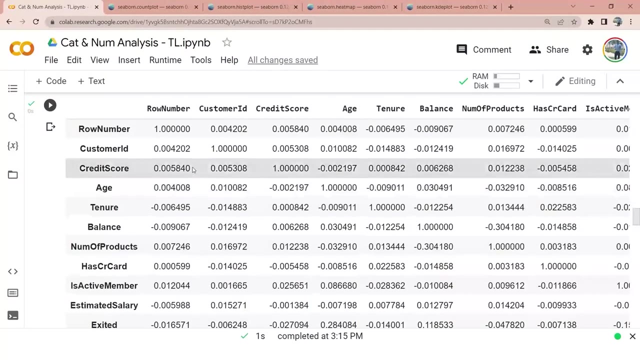 which will give you more ideas on how to approach a problem. but this video was all about, you know, understanding the categorical and numerical analysis using different type of plots. i hope you had good understanding from this particular session. that's all about this particular video. see in the next video. 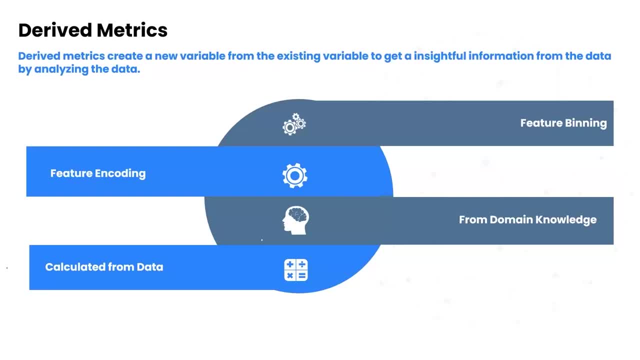 the next topic that we are going to discuss is going to be derived matrix. as the name suggests, derived metrics are those kind of metrics that are derived. derived matrix creates a new variable of value from the existing variable to get an insightful information from the data by analyzing the data. 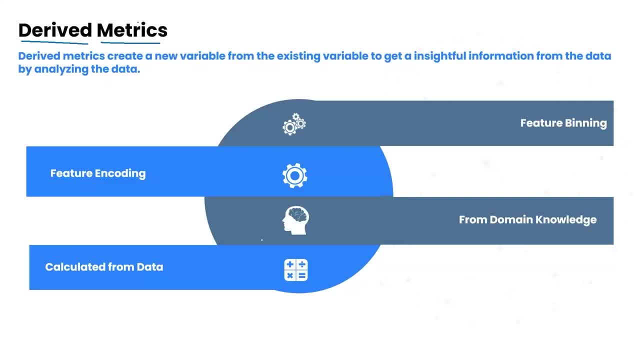 in simple terms, derived metrics are those kind of features or variables that we manually create using certain techniques. imagine you have a data set and there are multiple. obviously there are multiple records and there are multiple features. imagine there is a feature called as age and the age is in this format: 28, 20, 28, 29, blah, blah, blah. what if somebody asks you to? 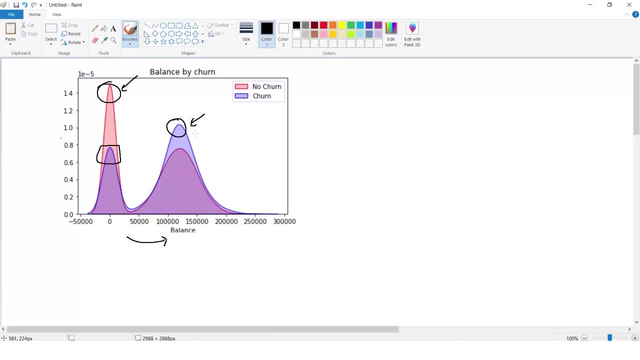 larger balance. people who have churned are having larger density, larger balance here and less so. somehow, with less balance, there are less number of people who are churning, who are having less balance. people who are having more balance are more likely to be churning than people who are. 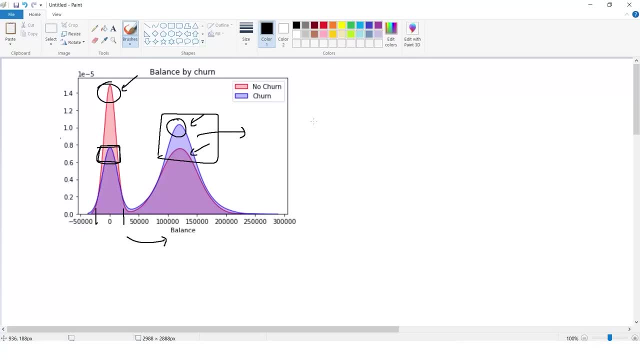 churned and simply compared to them, them more likely to be paid less. more likely to be churning, certainly because they have balance amount right. that means that amount they have to pay to the company. maybe because of that they are churning so that they don't have to give that amount. 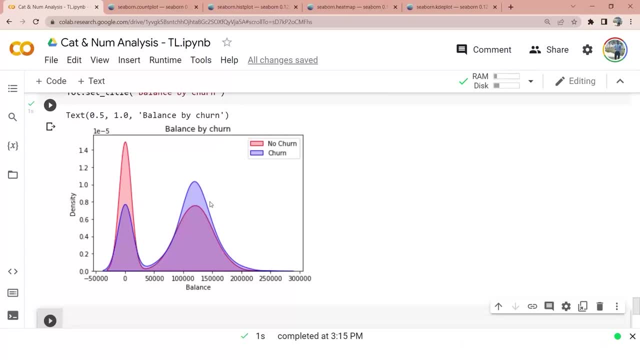 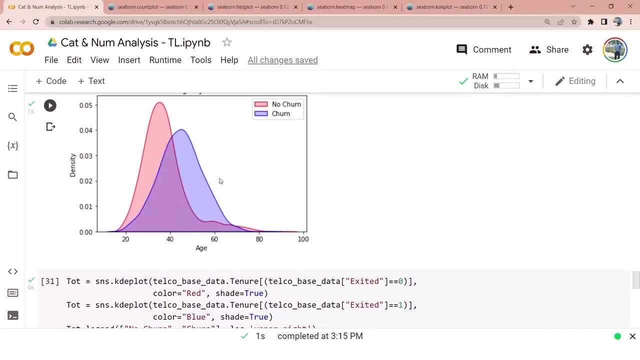 could be a reason, but this is, overall, giving you a understanding. so that's all about different types of analysis that we perform. in the next videos we will be talking about derived metrics and then we will be jumping into a case study. in the case study we will be taking 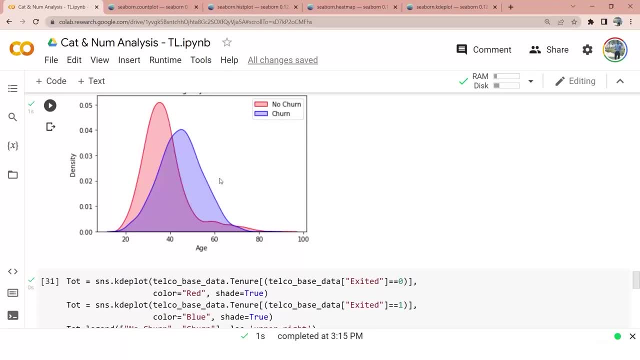 analysis use case. we will be performing each and everything from scratch, starting from data cleaning, data collection, analysis and finding insights, which will be an end-to-end case study which will give you more ideas on how to approach a problem. but this video was all about you know. 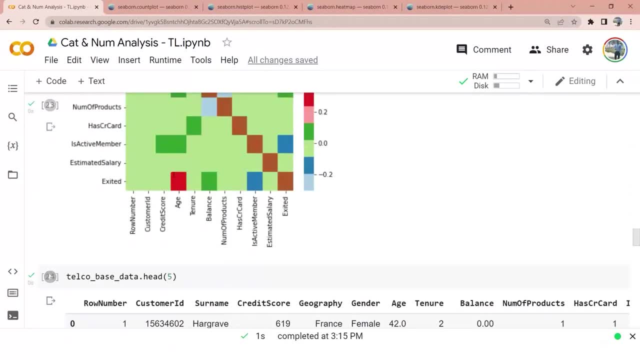 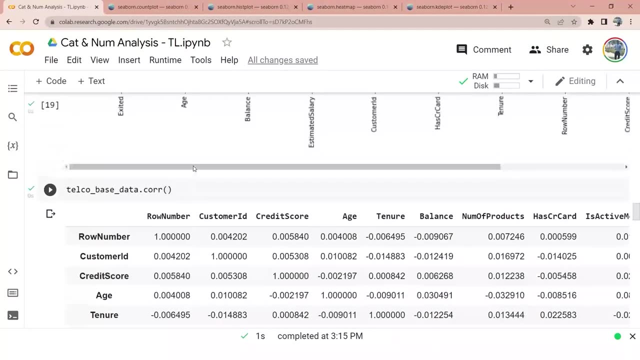 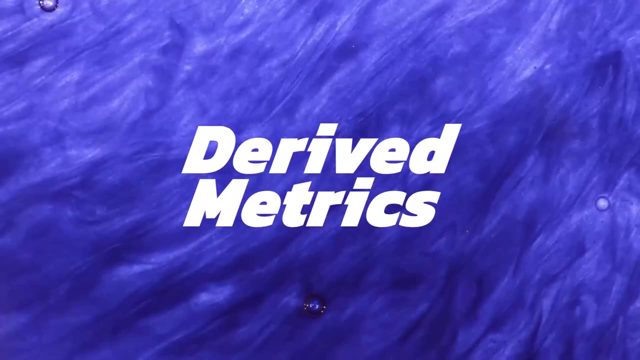 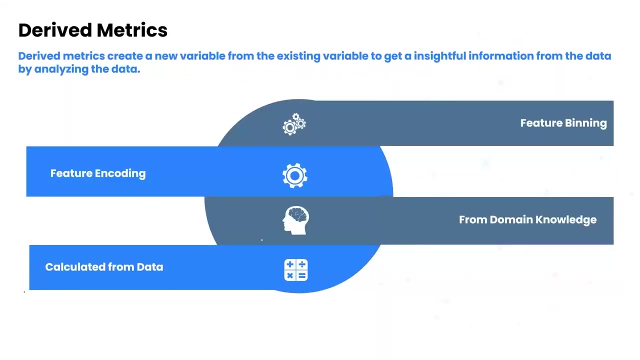 understanding the categorical and numerical analysis using different type of plots. i hope you had good understanding from this particular session. that's all about this particular video. see in the next video. the next topic that we are going to discuss is going to be derived metrics. as the name suggests, derived metrics are those kind of metrics that are derived. 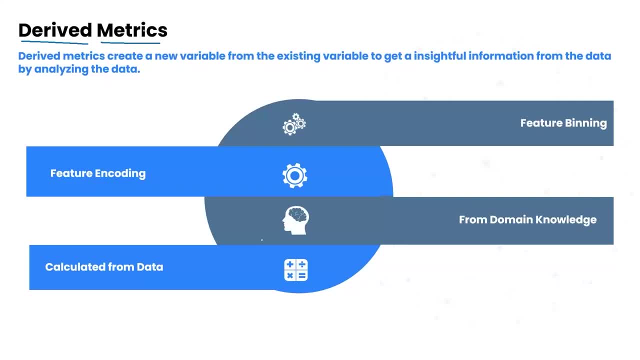 derived metrics creates a new variable from the existing variable to get an insightful information from the data by analyzing the data in simple terms. derived metrics are those kind of features or variables that we manually create using certain techniques. imagine you have a data set and there are multiple. 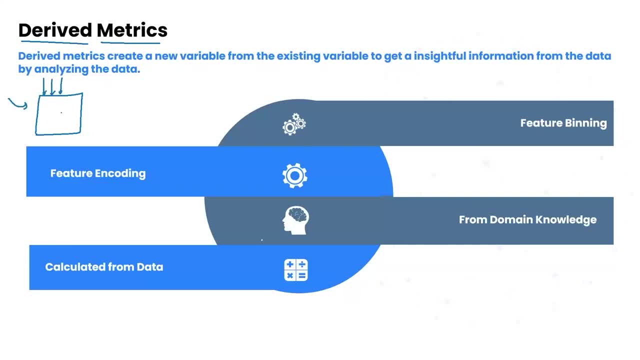 obviously there are multiple records and there are multiple features. imagine there is a feature called as age and the age is in this format: 28, 20, 28, 29, blah, blah, blah. what if somebody asks you to create another feature like age in months? what we do here is we simply multiply the age with 12. that 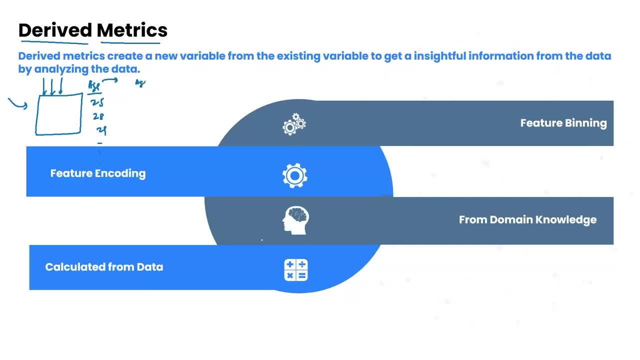 create another feature like age in months. what we do here is we simply multiply the age with 12. that will give me the age in months. right now this feature is not present in your original data, but you have manually created it so it could be a calculated from data feature. some of the features we also 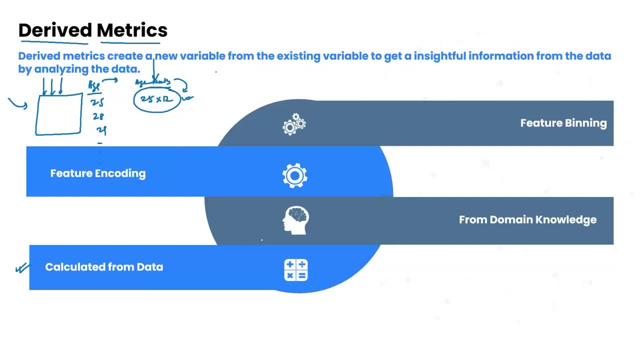 create using domain knowledge. imagine you have a column like x1 and you have a column like x2 and you know that if you combine both of them, probably you will find another column and that could- let let's say it could- be x3. now, that is something from the domain knowledge, for example. 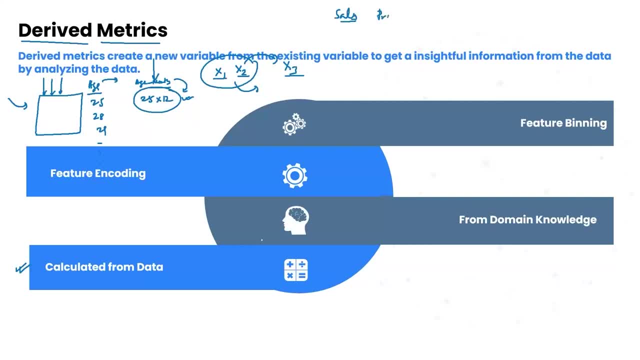 you have a column like, say, sales, and you have a column like profit and you want to find the total expenditure. now, expenditure is not a part of the original data, but you are calculating using some mathematical formulas, using your domain knowledge. now, that is a derived matrix, so we call it as from domain knowledge. 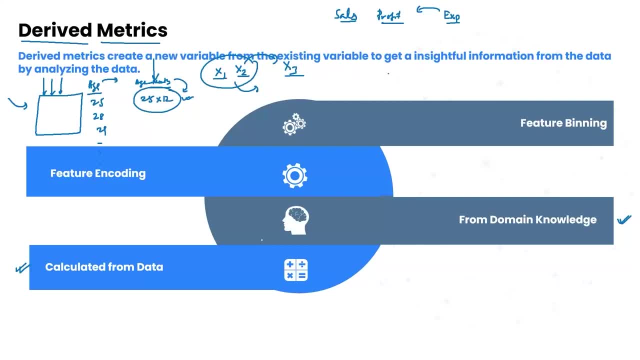 at certain point of time we also do binning. for example, we have a column like age 20, 20 et cetera, so we can understand the variable like four趣 part of it, and then we say, or we may take into account, how many rows you use the table in the form of that. 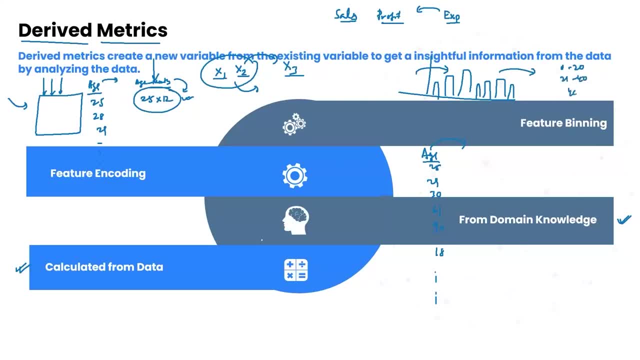 expression with relation to those rows. so literally that is it. this is going to be written as la. that's a just kind of a choice. whatever you like to put in there, to be preventative, anything you would like to put in it, but you will use jeon in at least. it is a good example of the kind well, which is standard things you do when 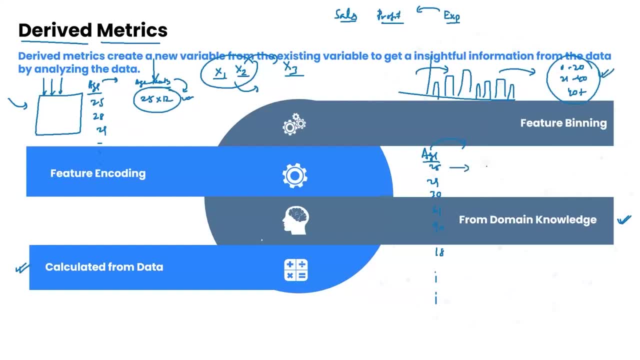 so you created three bins. so this becomes 21 to 40, this becomes 21 to 40, this becomes 21 to 40, this becomes 40 plus, this becomes 40 plus, this becomes 0 to 20, and so on. so this is simply our. 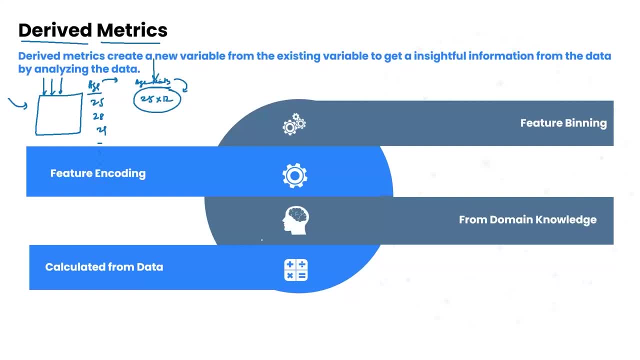 will give me the age in months. right now this feature is not present in your original data but you have manually created it so it could be a calculated from data feature. some of the features we also create using domain knowledge. imagine you have a column like x- 1 and you have a column like x2 and you know that if you combine. 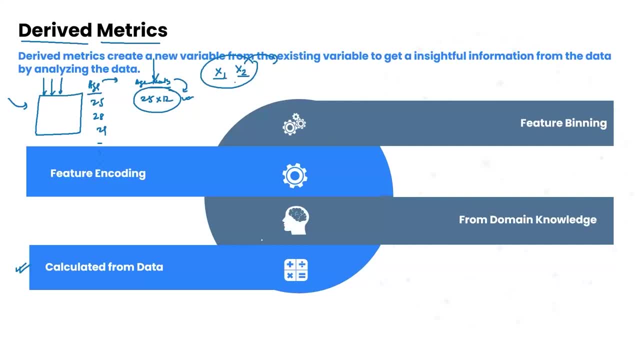 both of them. probably you will find another column and that could- let let's say it could- be x3. now, that is something from the domain knowledge, for example. you have a column like sales it and you want to find the total expenditure. now, expenditure is not a part of the original data. 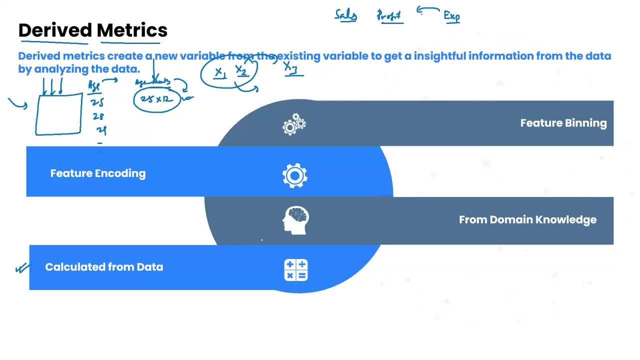 but you are calculating using some mathematical formulas, using your domain knowledge. now, that is a derived matrix, so we call it as from domain knowledge. at certain point of time, we also do bending. for example, we have a column like age 25, 29, 30, 61, 90, 18, dot, dot, dot. what if, when you 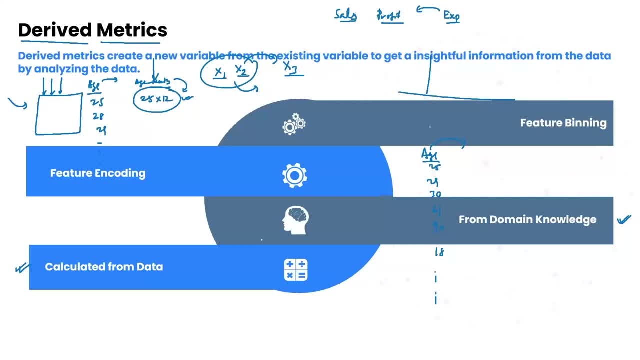 are analyzing the age, you are visualizing age, and it could end up in a multiple bar charts, multiple bars, which is difficult to interpret. in that case, probably what you will do is you will convert it into bins. let's say, 0 to 20, 20 is a bin, 21 to 40 and 40 plus. so you created three bins. so this becomes 21 to 40. this becomes: 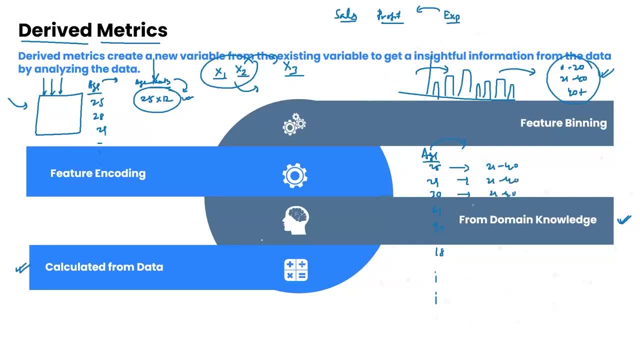 21 to 40, this becomes 21 to 40, this becomes 40 plus, this becomes 40 plus, this becomes 0 to 20, and so on. so this is simply our feature binning. and coming on to feature encoding, there are multiple encoding techniques. 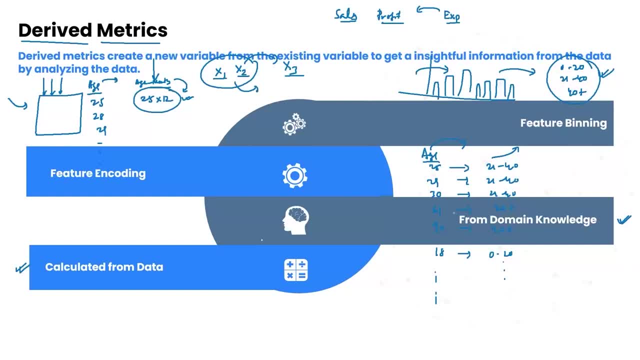 especially in the field of predictive analytics or machine learning, your categorical data can be extremely useful. however, in its original form, it can be unrecognizable to most of the models because, ultimately, we create models and models are run in computers, and computers don't understand categorical features. so in order to solve this problem, we can use different encoding techniques. 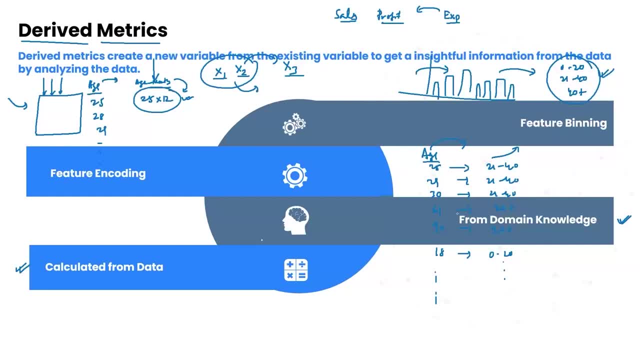 feature binning. and coming on to feature encoding, there are multiple encoding techniques, especially in the field of predictive analytics or machine learning, your categorical data can be extremely useful. however, in its original form it can be unrecognizable to most of the models because ultimately we create models and models are run in computers, and computers don't understand. 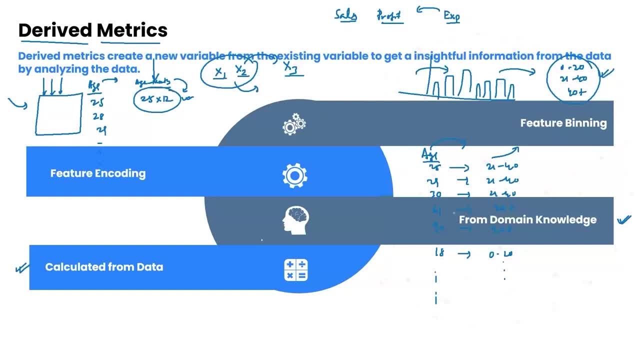 categorical features. so in order to solve this problem, we can use different encoding techniques to make our categorical data legit. so there are multiple encoding techniques that we will understand in the future videos. there are techniques like label encoder, techniques like one hot encoder, dummy encoder, target encoder, hash encoder and so on. so we have a separate session on feature encoding where we will be. 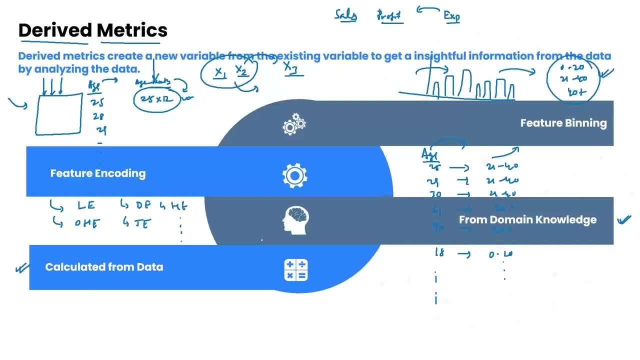 going through each and every encoding techniques, theoretically and practically, but overall that's all about your derived metrics. simply, derived metrics are those kind of columns which are not present in your original data and we have to manually create it based on our domain knowledge or based on our understanding or based on some other features. so that's all about derived metrics. in the next video we shall be jumping into feature binning, feature encoding and various other topics. 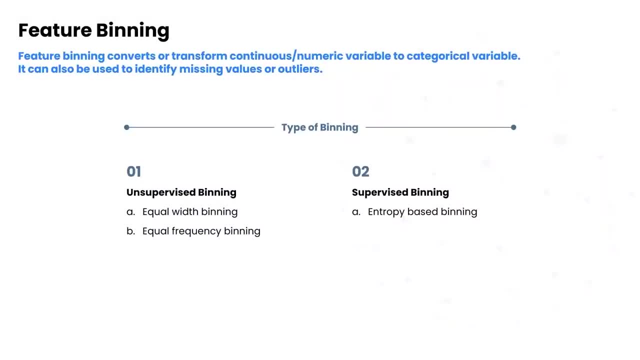 feature binning, as we discussed in a nutshell in the previous video. that feature binning is simply one of those techniques where we create bins out of a feature. feature or variable are nothing but some of the columns from your data set. feature binning simply converts or transforms continuous or numerical variable to categorical variable. it can also be used to identify 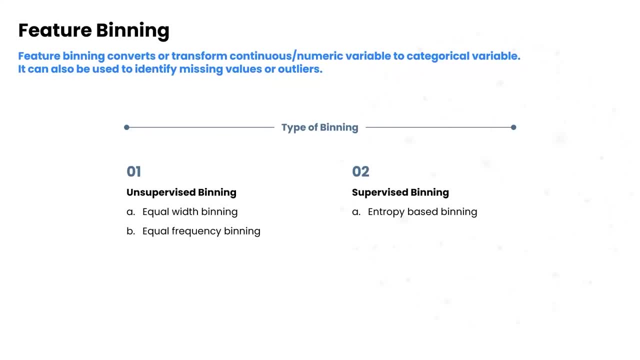 missing values or outliers. there are two types of binning, one of them being unsupervised binning, which is equal width binning: that means you have a column and you divide them with equal width. and one of them is equal frequency binning: that means you divide it with equal frequency. that means each bin will have equal amount of data points. 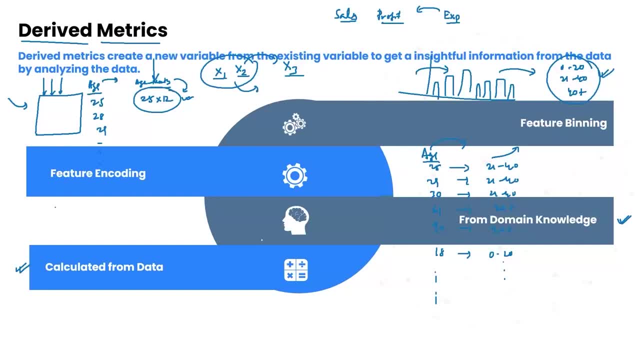 that will be used to make the model data legible. so there are multiple encoding techniques that we will understand in the future videos. there are techniques like label encoder, techniques like one hot encoder, dummy encoder, target encoder, hash encoder and so on. so we have a separate session on feature encoding where we will be going through each and every encoding. 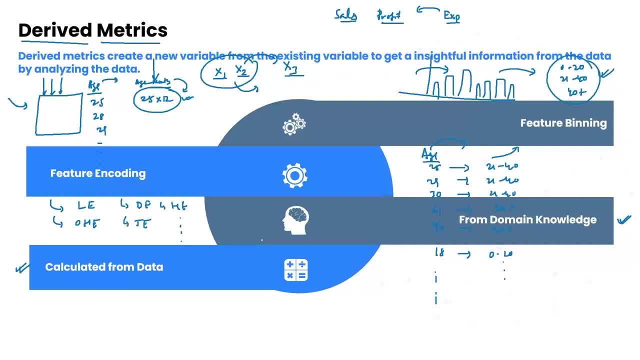 techniques, theoretically and practically. overall, that's all about your derived metrics. simply, derived metrics are those kind of columns which are not present in your original data and we have to manually create it based on our domain knowledge, or based on our understanding or based on some other features. so that's. 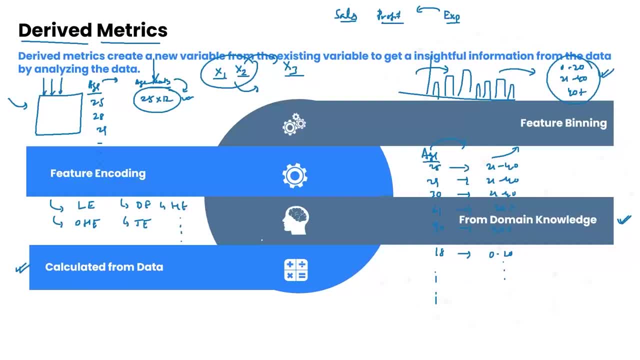 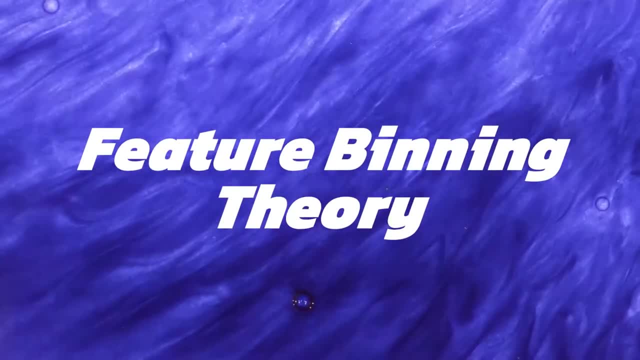 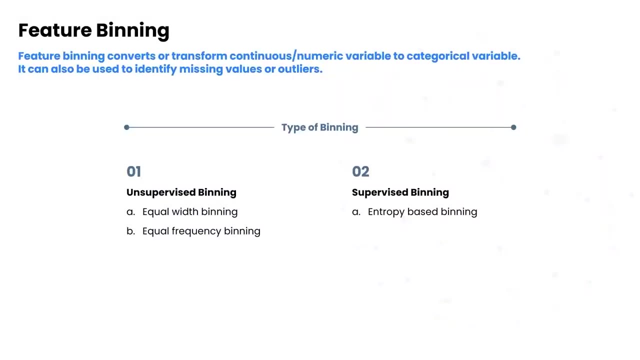 all about derived metrics. in the next video we shall be jumping into feature binning, feature encoding and various other topics. feature binning: as we discussed in a nutshell in the previous video that feature binning is simply one of those techniques where we create bins out of a feature, feature or variable. 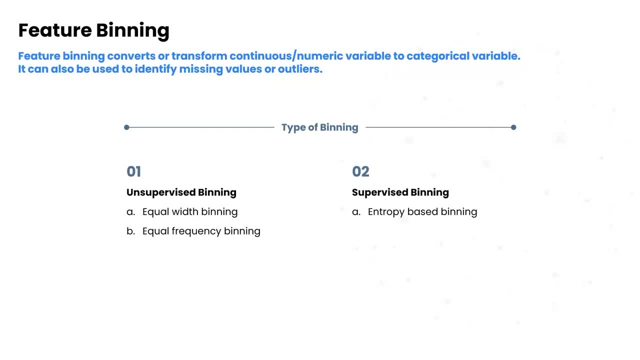 are nothing but some of the columns from your data set. feature binning simply converts or transforms continuous or numerical variable to categorical variable. it can also be used to identify missing values or outliers. there are two types of binning, one of them being unsupervised binning, which is equal width binning. that means you have a column and you 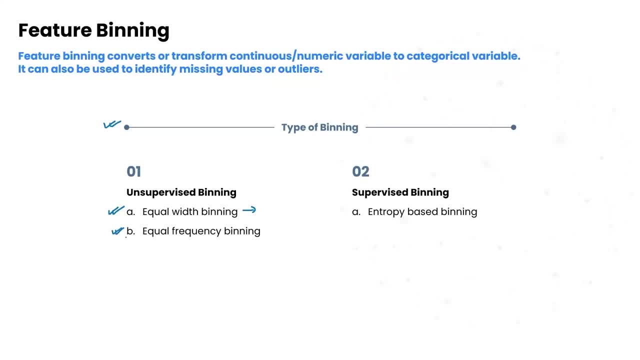 divide them with equal width and one of them is equal frequency. binning that means you divide it with equal frequency. that means each bin will have equal amount of data points and in here each bin will be divided equally. for an example, i have a data set and i have a column called as age. if you 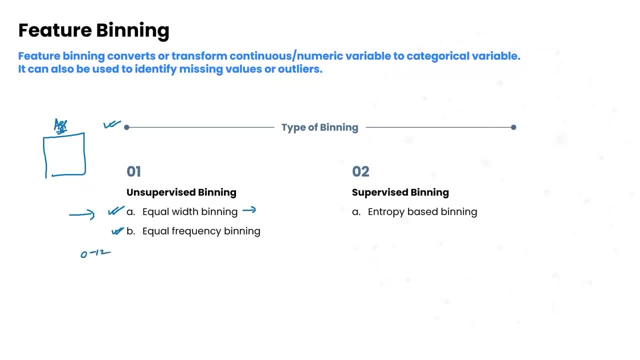 divide it with equal width. that means 0 to 12, 13 to 24, 25 to 36. you can see each bin is having 12 years of data. each bin, but with equal frequency, basically means that each bin that will create it that will have equal. 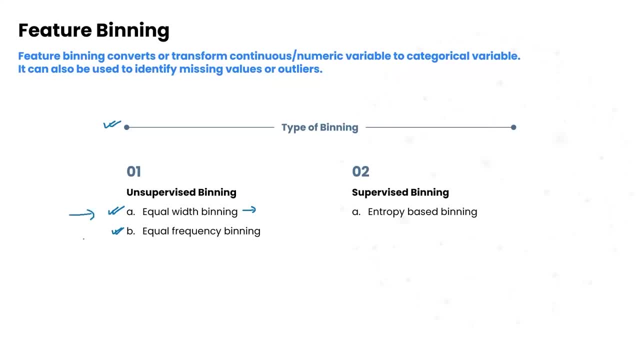 and in here each bin will be divided equally. for an example, I have a data set and I have a column called as age. if you divide it with equal width, that means 0 to 12, 13 to 24, 25 to 36, you can see each bin is. 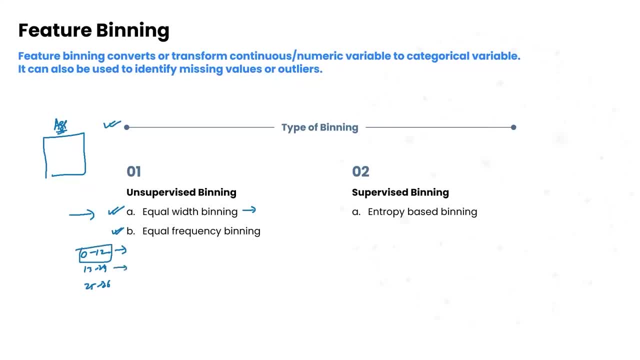 having 12 years of data each bin, but with equal frequency, basically means that each bin that will create it, that will have equal frequency of data points. so let's say the first bin has 100 data points, 100 data points in short, if you have 1000 data points, 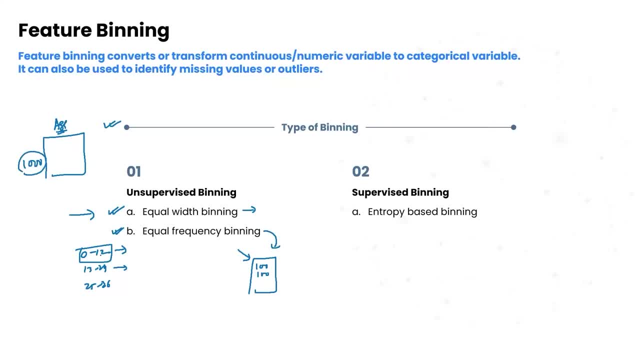 you divide it into 10 bins. so your labels or your bins will be created automatically based on the frequency. which type of winning is preferred? it all depends, as we said, feature winning, feature encoding- all these kind of things we usually use for predictive analytics, which is a hidden trial process. so we have to create bins, perform our analysis, check our models, behavior. 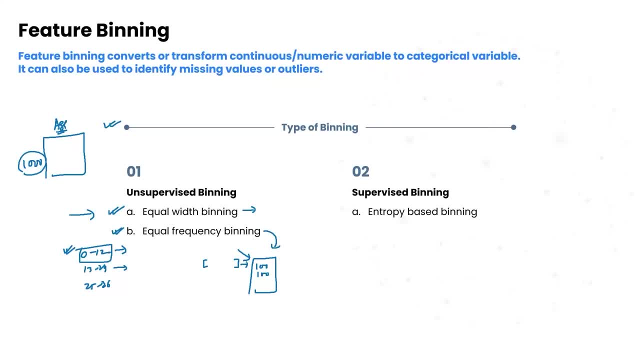 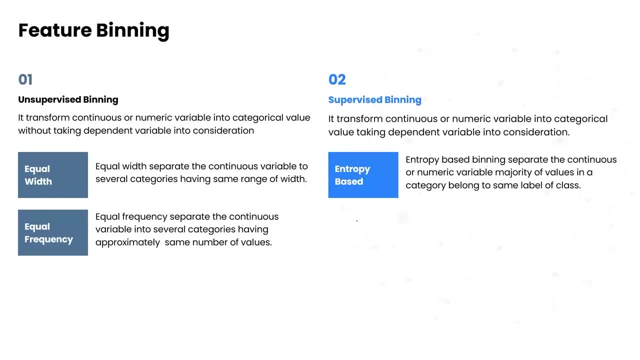 again come back. it's a iterative process. the second type of winning is a supervised winning, which is a entropy based winning. unsupervised winning: it transforms continuous or numerical variable into categorical variable without taking dependent variable into consideration. equal width separation, separate the continuous variable to several categories having same range of width equal. 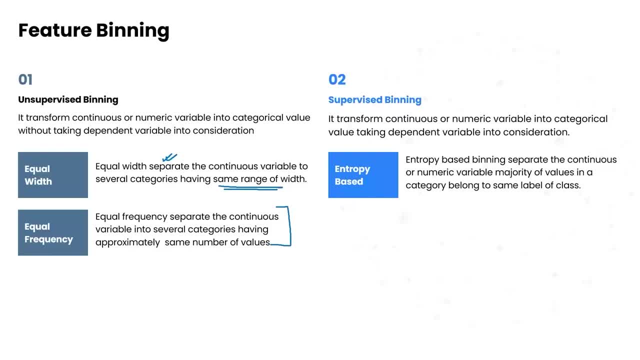 frequency, separate the continuous variables into several categories having approximately same number of values and supervised winning, it transforms continuous or numerical variable into categorical value, taking dependent variable into consideration. now, what do you mean by dependent variable if we are talking about a data set? now, let's say you have a data set of multiple customers. 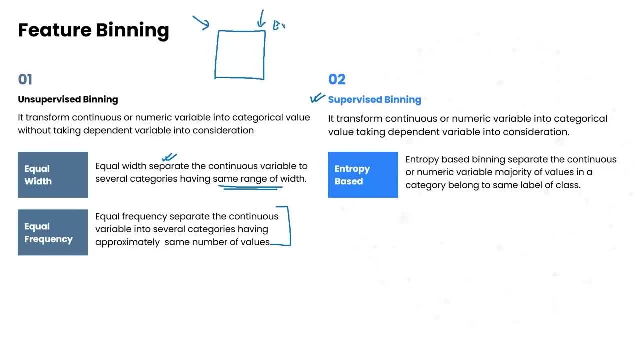 and there is a column called as whether a customer has exited or not, and if your final goal is to create a predictive model that will be able to understand your customers details, understand your customers characteristics and will be able to predict whether a customer will be exited or not, 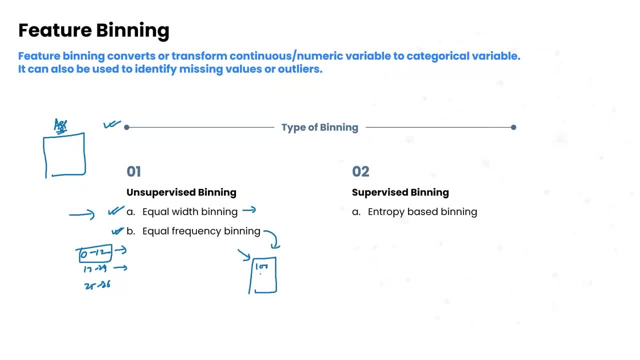 frequency of data points. let's say the first bin has 100 data points. 100 data points in short. if you have 1000 data points, you divide it into 10 bins. so your labels or your bins will be created automatically based on the frequency. which type of binning is preferred? 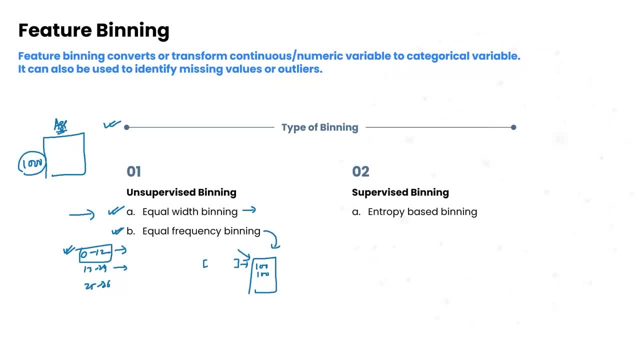 it all depends, as we said, feature binning, feature encoding, all these kind of things we usually use for predictive analytics, which is a hidden, tranquil process. so we have to create bins, perform our analysis, check out, models, behavior. they can come back. it's a iterative process. the second type of building is a supervised. 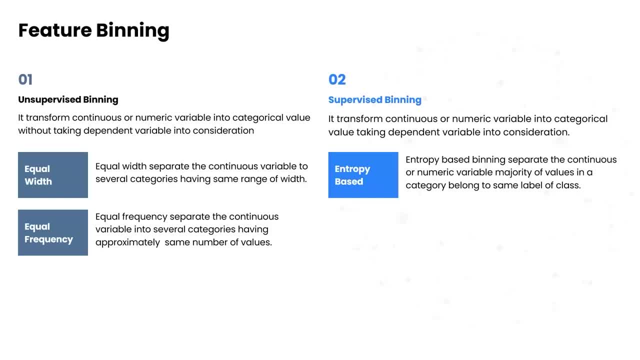 winning, which is a entropy based winning, unsupervised winning. it transforms continuous or numerical variable into categorical variable without taking dependent variable into consideration. equal width: separate the continuous variable to several categories having same range of width. equal frequency: separate the continuous variables into several categories having approximately same. 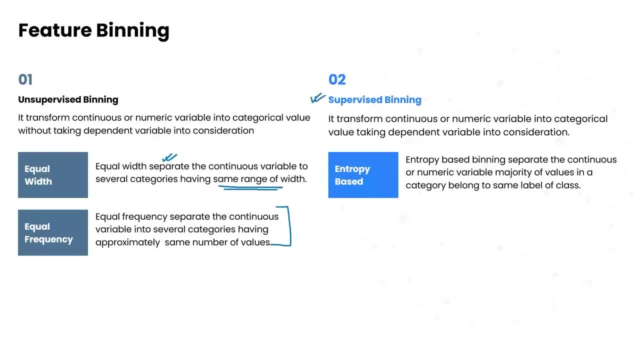 number of values and supervised meaning. it transforms continuous or numerical variable into categorical value, taking dependent variable into consideration. now, what do you mean by dependent variable if we are talking about a data set? now, let's say you have a data set of multiple customers and there is a column called as whether a customer has exited or not. 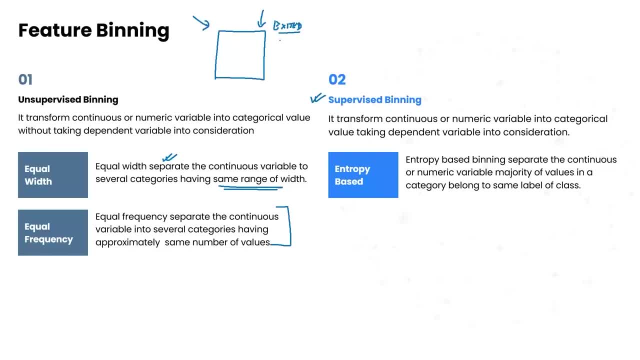 and if your final goal is to create a predictive model that will be able to understand your customer's details, understand your customer's characteristics and will be able to predict whether a customer will be exited or not, in that case you are kind of predicting this exited column. 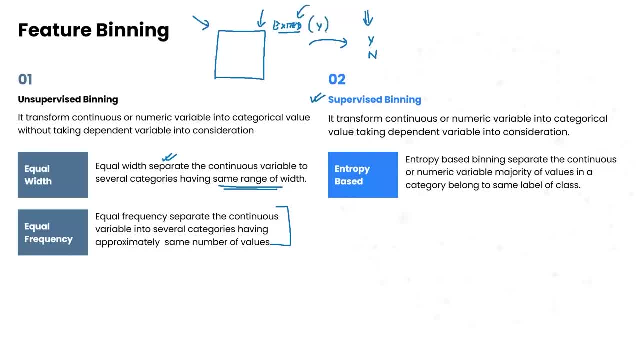 so exited, becomes your Y variable, otherwise called as dependent variable, and all the other columns are called as your X variables, otherwise called as features, otherwise called as independent variables. so supervised winning is when you transform a continuous numerical variable taking dependent variable into consideration. that means, if you are considering age, let's say the people's age are. 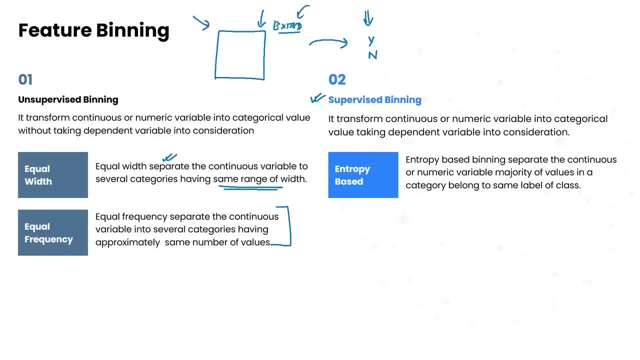 in that case you are kind of predicting this exited column. so exited becomes your y variable, otherwise called as dependent variable, and all the other columns are called as your x variables, otherwise called as features, otherwise called as independent variables. so supervised winning is when you transform a continuous numerical variable taking dependent variable. 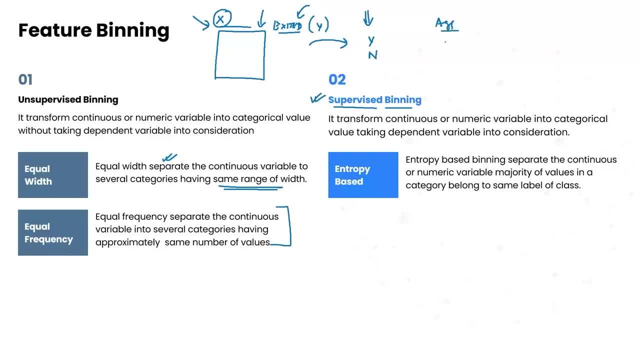 into consideration. that means, if you are considering age- let's say the people's age or something like this- you also consider how the age is impacting the exited column that we are going to predict and based on that you create bins. so this type of binning technology or technique is called as entropy based. entropy based binning. 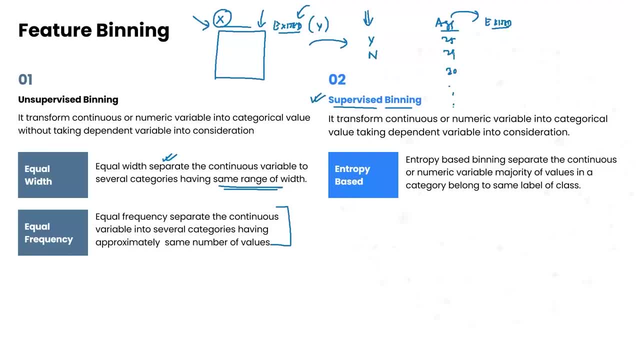 separate the continuous or numerical variable. majority of values in a category belong to same level of class. now supervised binning is not required for a continuous or numerical variable, but it is required if you are just analyzing some data without any y variables. imagine you are working on a eda use case and your data set need not have to be prepared. 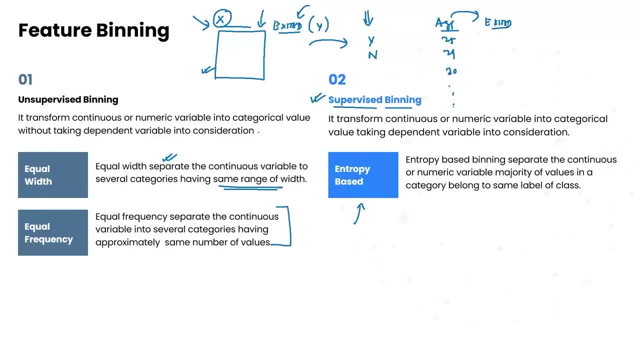 for the predictive analytics part. your only focus is to understand and get insights from the data. eda is your final end goal and your data set does not have a y variable like this. simply, let's say you have customers data, that's it, and you are trying to analyze the customers data. which customers are similar? 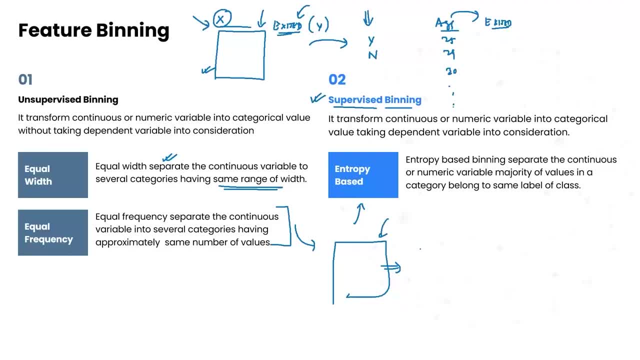 to each other, kind of doing a customer segmentation use case where you are trying to create segments of customers who could be similar to each other. in these kind of use cases where you don't have y variable or dependent variable, in that case you cannot use entropy based. 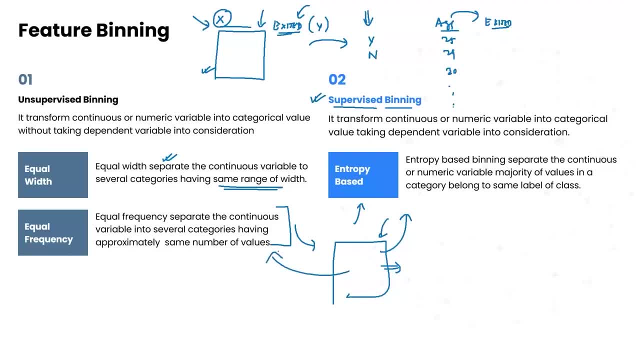 technique, you always have to go for the unsupervised binning technique. so feature binning is very important when you are considering it to be. you are preparing your data for your predictive analytics. if you are only considering eda or exploratory data analysis, feature binning might not be important. only in certain cases it could be. 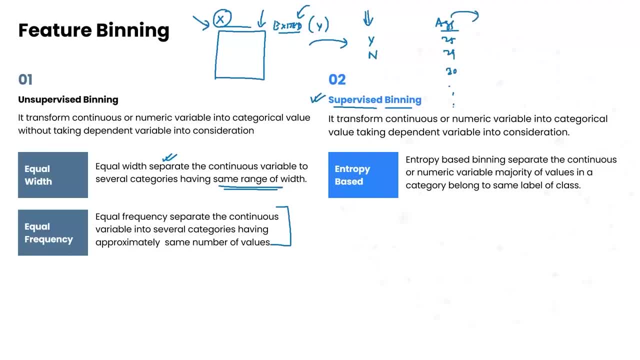 something like this. you also consider how the age is impacting the exited column that we are going to predict and based on that you create bins. so this type of binning technology or technique is called as entropy based. entropy based binning: separate the continuous or numerical variable. majority of. 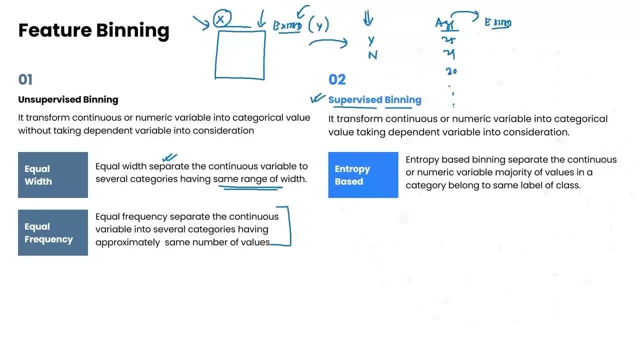 values in a category belong to same level of class. now supervised binning is not required if you are just analyzing some data without any Y variables. imagine you are working on a EDA use case and your data set need not have to be prepared for the predictive analytics part. 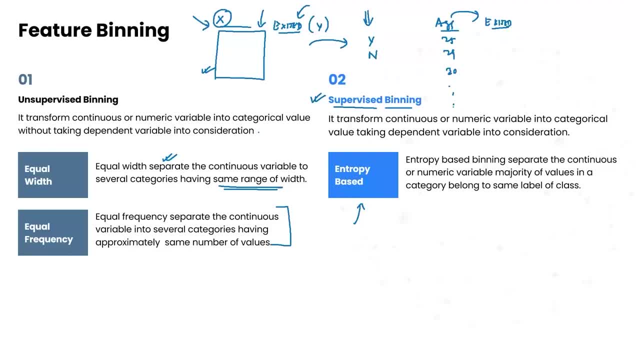 your only focus is to understand and get insights from the data. EDA is your final end goal and your data set does not have a Y variable like this. simply, let's say, you have customers data, that's it, and you are trying to analyze the customers data. which customers are similar to each other, kind of doing a customer segmentation use. 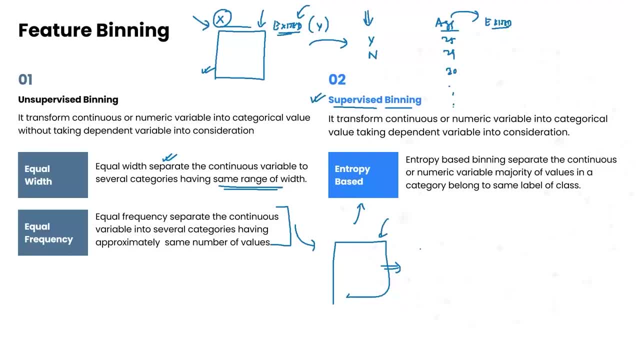 case where you are trying to create segments of customers who could be similar to each other in this kind of use, cases where you don't have Y variable or dependent variable. in that case you cannot use entropy based technique to go for the unsupervised binning technique. 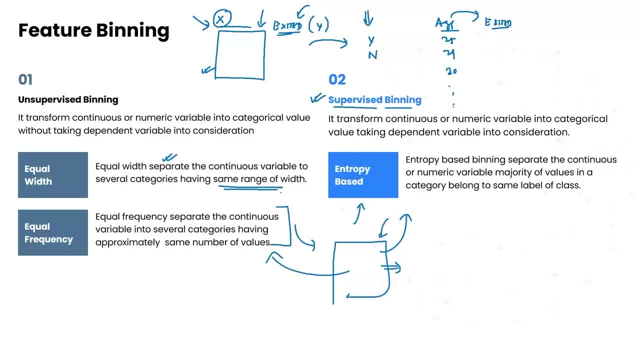 so feature binning is very important when you are considering it to be you are preparing your data for your predictive analytics. if you are only considering EDA or exploratory data analysis, feature binning might not be important. only in certain cases it could be required when, let's say, you have a column like H and when you are 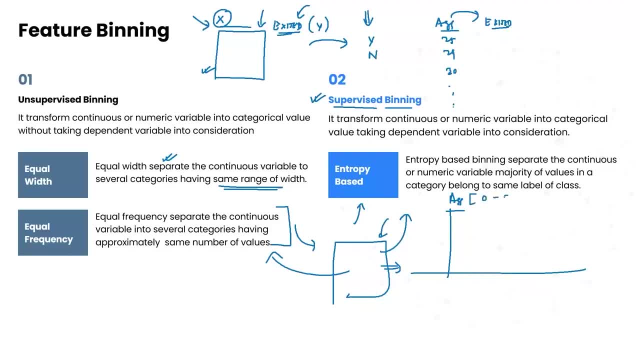 visualising it now, edge could range from 0 to 90 or 100. if you visualize use using a backchat, it could be very clumsy. it could have 100 bugs even when you analyze it using the line Say it, then also you might not be able to. 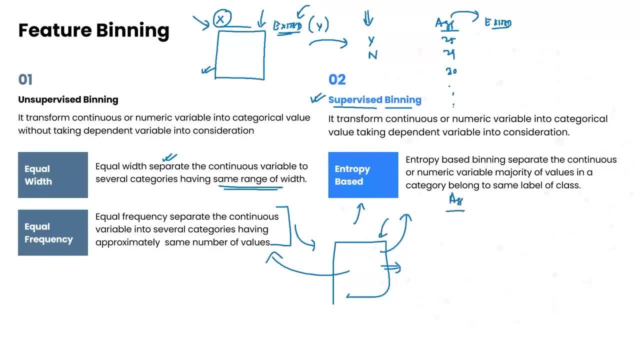 required when, let's say, you have a column like age and when you are kind of visualizing it. now, age could range from 0 to 90. but it is not a problem if you visualize using a bar chart, it could be very clumsy. it could have 100 bars even. 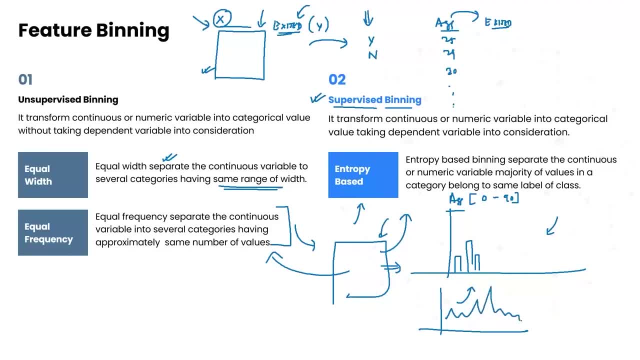 when you analyze it using a line chart, then also you might not be able to get good insights from it. so in this case, what we do is we create bins so that visually, we can have multiple bars and we can understand- oh, most of the people are within the range of 21 to 40. and then 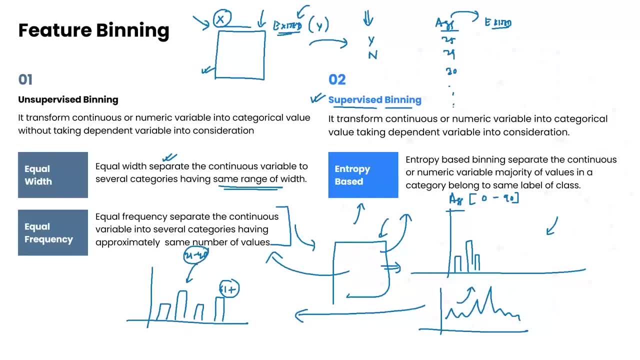 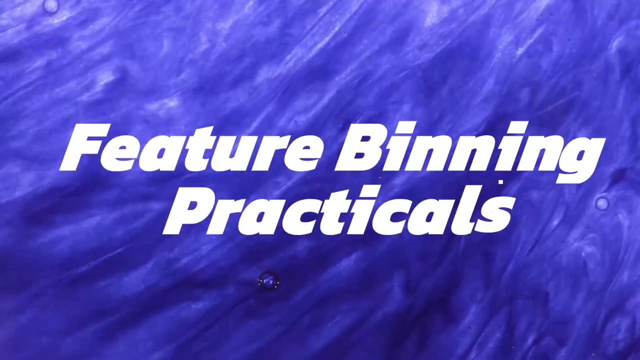 come 61 plus. so it all depends scenario to scenario. if you are required to perform binning, then you can perform binning, else not. that's all about this session on feature binning. in the next session we shall be helping you out in the python part, in the practicals part, how to create bins using a sample data set. 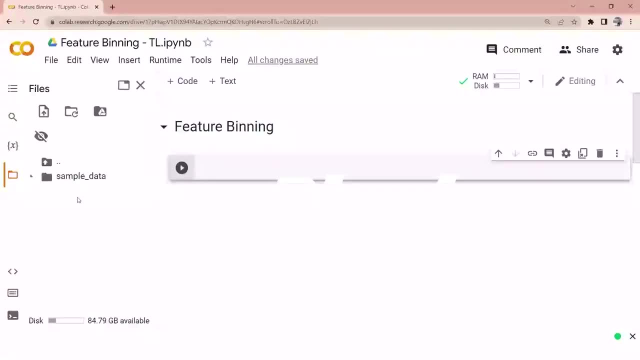 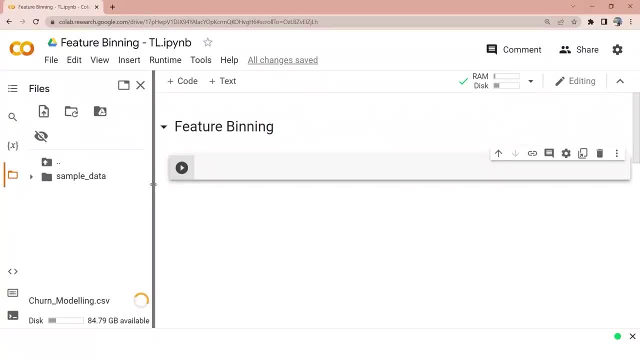 I will upload my csv file here. So my CSV file is uploaded. We will get started with importing the libraries: import pandas as pd, import numpy as np, import matplotlib, pyplot. well, we don't need matplotlib, but just in the case, and we will be using. 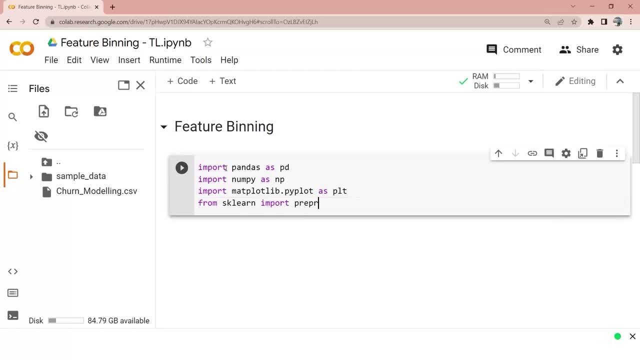 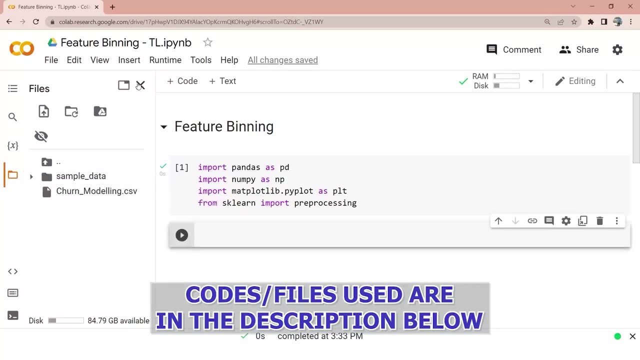 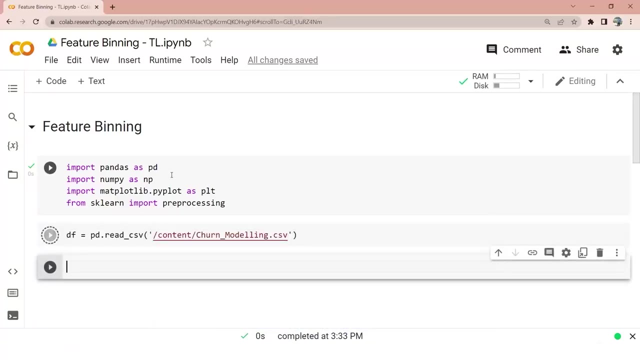 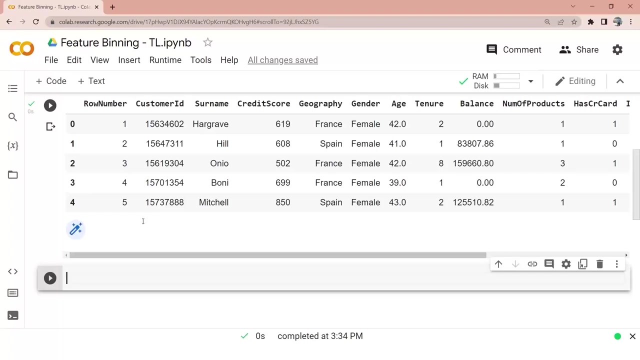 sklearns library library. so i am going to import preprocessing. so once this is done, let me, let me just copy the path of this file, close it. df equals to pd, dot. read csv content, slash, churn modeling and you can see my data is ready. that's my data frame. i have row number, customer id, surname. 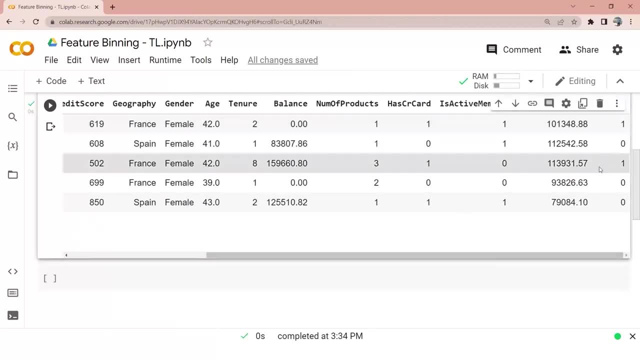 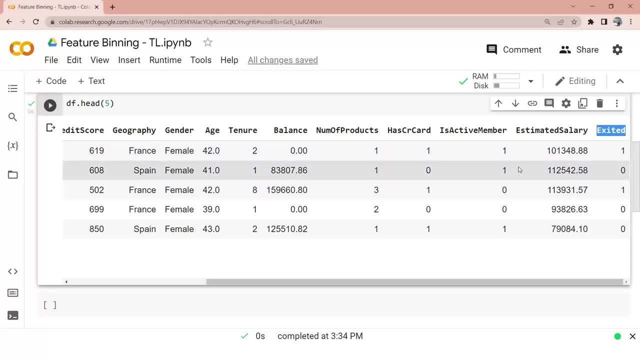 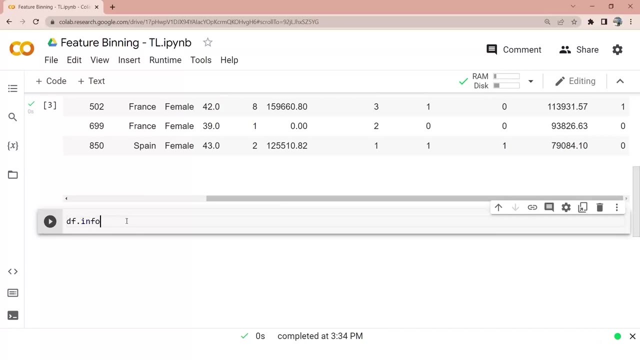 all these features i have and you can see there is a column called as exited. okay, so exited basically means whether a customer is active or exited. one means exited, zero means active. the first thing that we can do is let's say i'll just click on info to check. 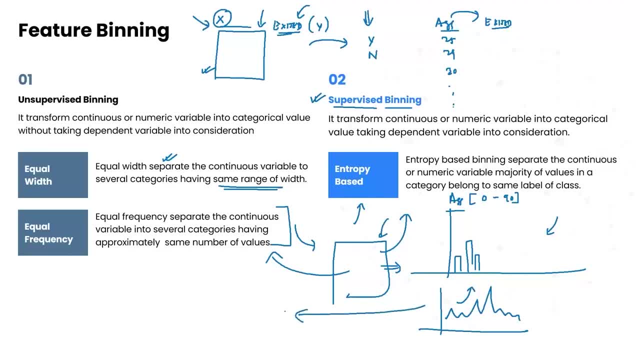 Get good insight from it. it boards but적. So in this case, what we do is we create bins so that we, we we can have multiple buyers and we can understand how most of the people are within the range of כי range of 21 to 40, and then comes 61 plus. so it all depends scenario to scenario, if you are required. 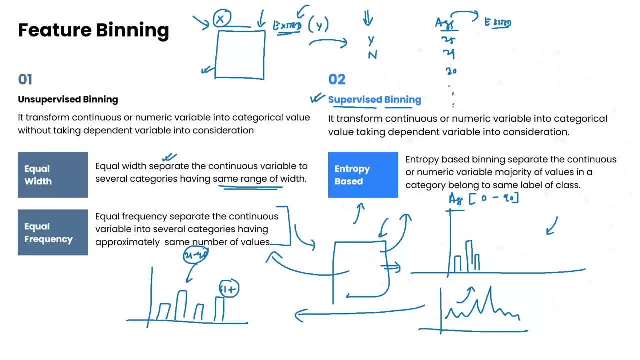 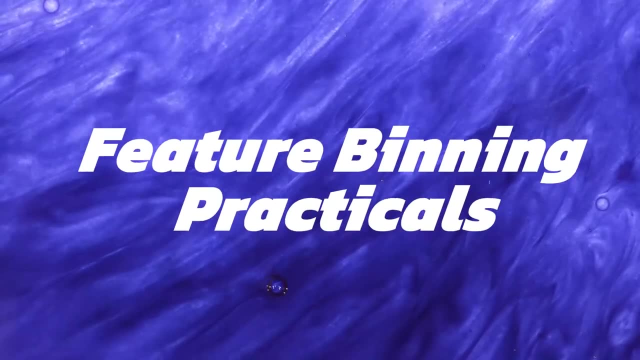 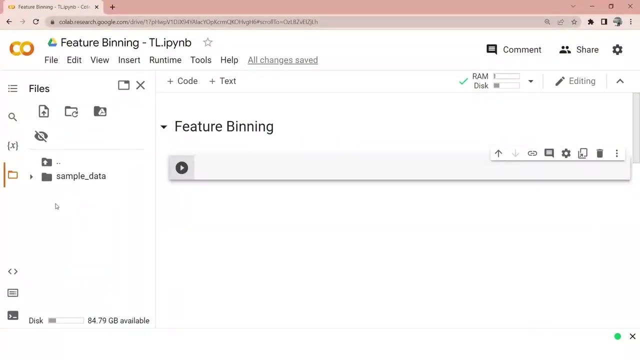 to perform binning, then you can perform binning, else not. that's all about this session on feature binning. in the next session we shall be helping you out in the python part, in the practicals part, how to create bins using the sample data set. so let's get started with the practicals part in order to get started. 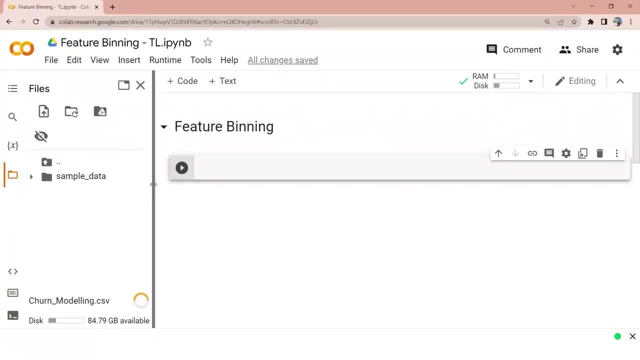 i will upload my csv file here. so my csv file is uploaded. we will get started with importing the libraries. import pandas as pd import numpy as np. import maxpd as pd import numpy as pd import numpy as pd import numpy as pd. matplotlib, dot pyplot- well, we don't need matplotlib, but just in the case and we will be. 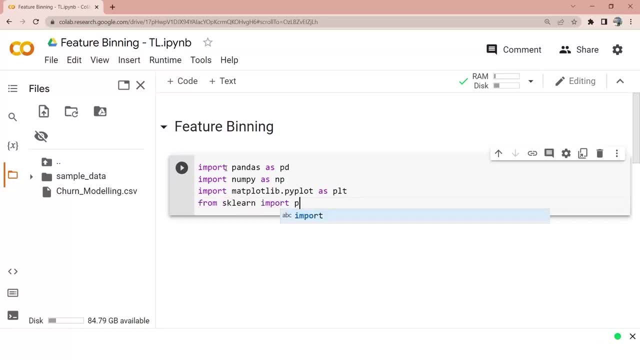 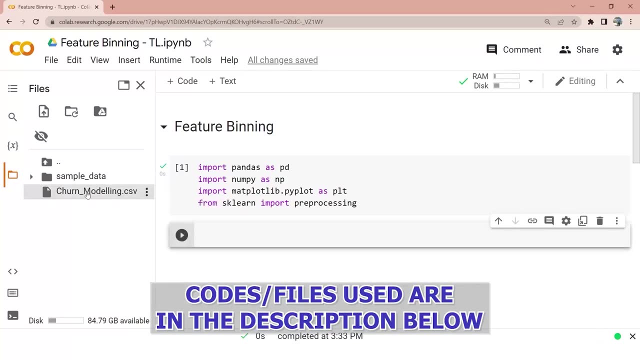 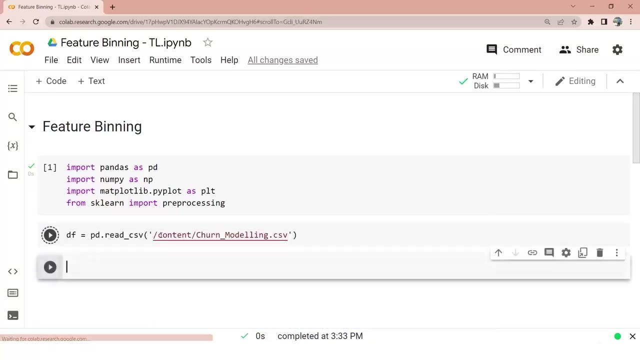 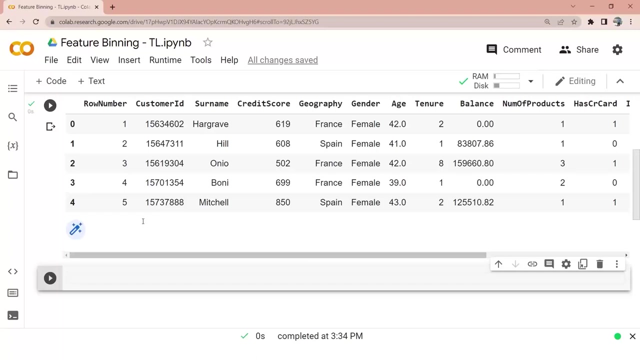 using sk learns library. so i am going to import pre-processing. so once this is done, let me, let me just copy the path of this file, close it. df equals to pd, dot. read csv content, slash, churn modeling and you can see my data is ready. that's my data frame. i have row number, customer id, surname, all these features i have and you can. 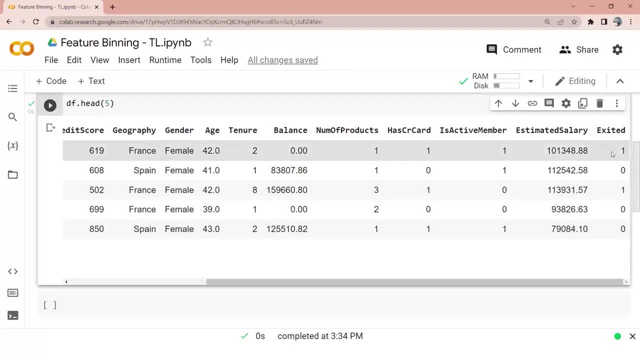 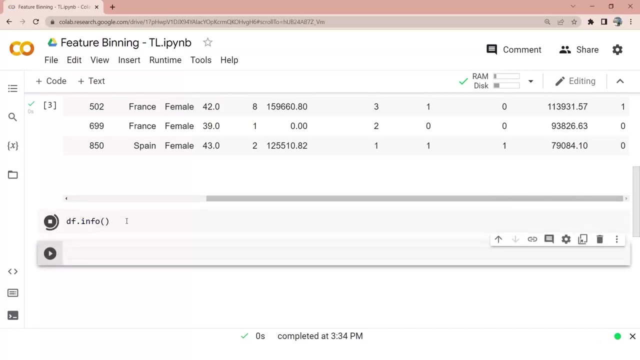 see there is a column called as exited. okay, so exited basically means whether a customer is active or exited. one means exited, zero means active. the first thing that we can do is let's say: i'll just click on info to check whether we have null values or not, and you can see. 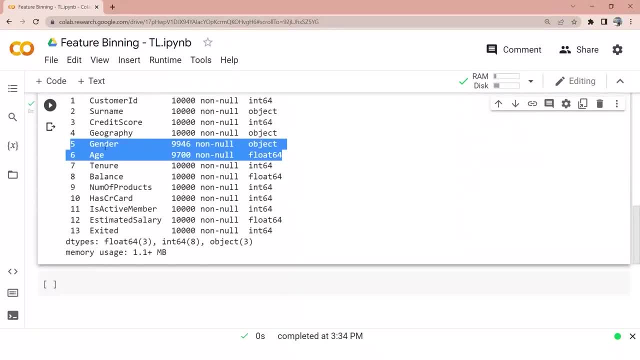 evidently visible that gender has some null values we will be using. we will be using age for performing our task, performing our binning task. age or tenure: we can use any of them, because both of them are your continuous numerical values. so the first thing i'm going to do is i'm going 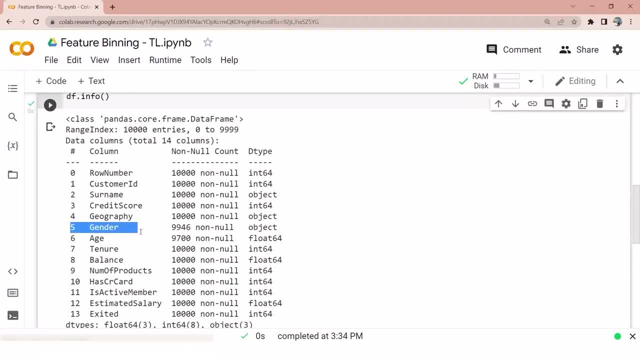 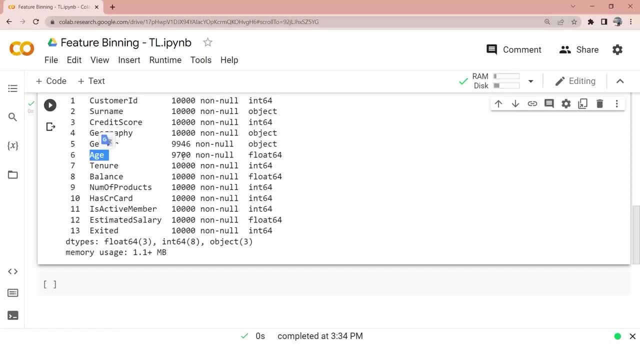 whether we have null values or not and you can see evidently visible that gender has some null values. we will be using uh. we will be using uh. we will be using uh. we will be using age for performing our task, performing our binning task. age or tenure we can use. 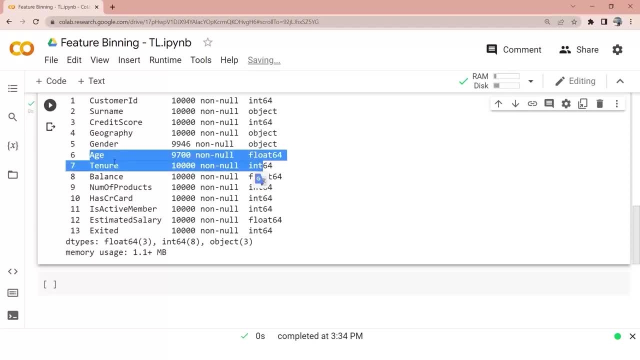 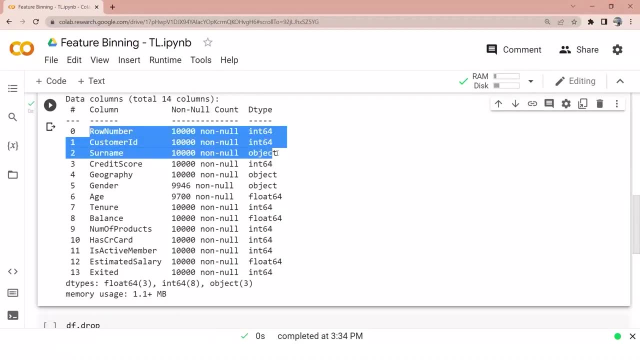 any of them, because both of them are your continuous numerical values. so the first thing i'm going to do is i'm going to drop some of these random columns, which makes no sense in our analysis process. so it's a very good exercise to drop off columns that you don't. 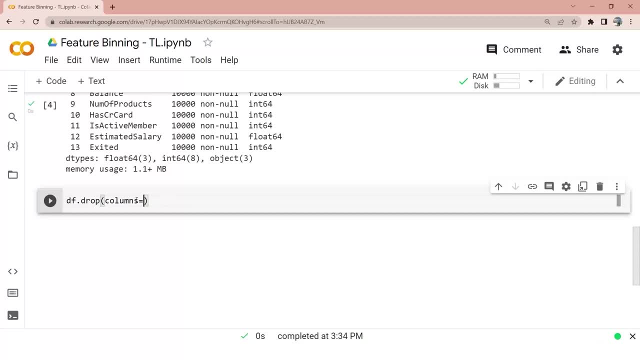 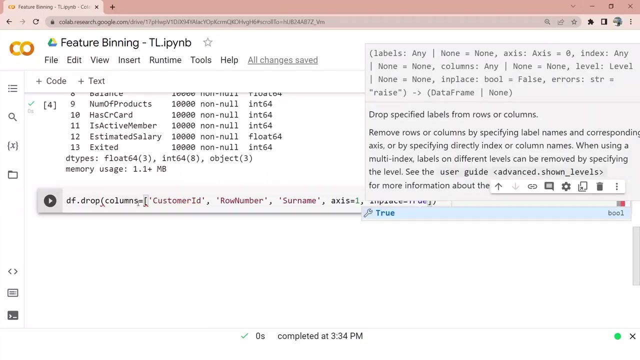 need for your analysis because unnecessarily they will be eating up your data. so let's drop your space and memory. so customer id, row, number and surname- what else we will delete it from axis 1. in place equals to 2. in place equals to 2 basically means when you are performing. 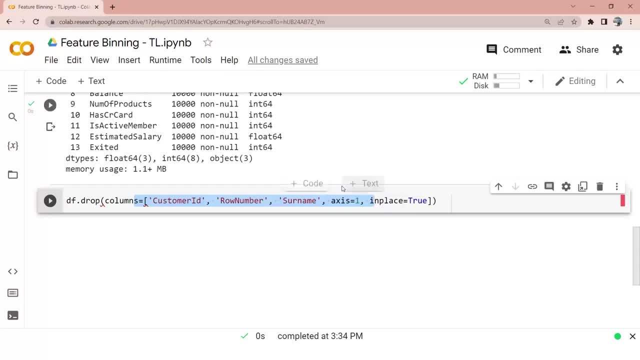 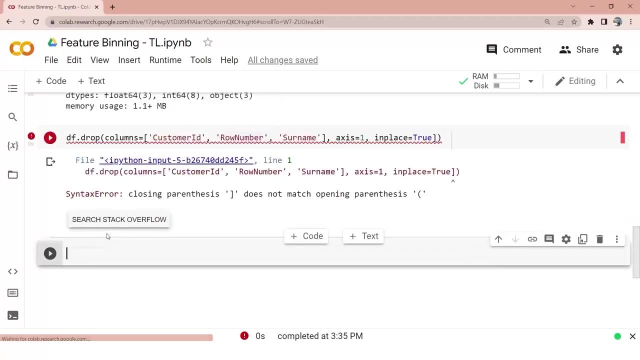 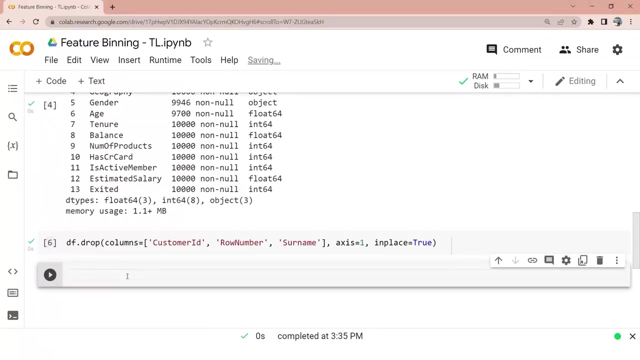 this task you are. you don't need to assign the same thing to your data frame directly. your data frame will be updated df, dot. drop columns equals to this. brackets close access here. done so. okay, so my data frame is dropped. my three columns are dropped, in case you want to check. 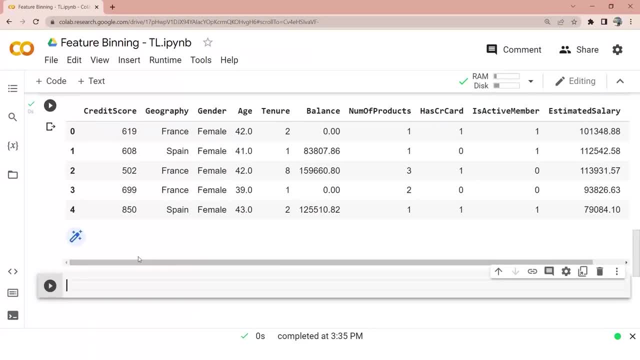 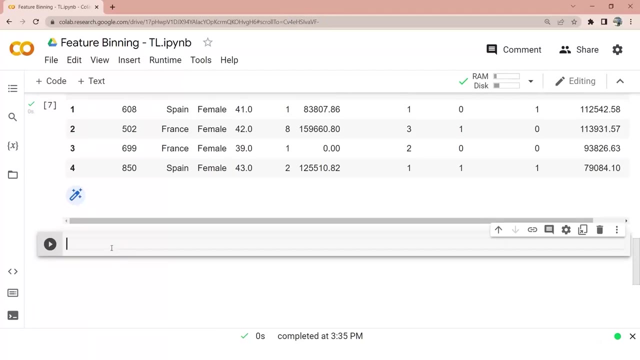 your new data frame. that's how it looks like. my features that are not important. they are gone right, even though it makes no sense for this particular activity, but it's a good practice to do so. we will get started with the binning technique. so let's say i am going to use age. 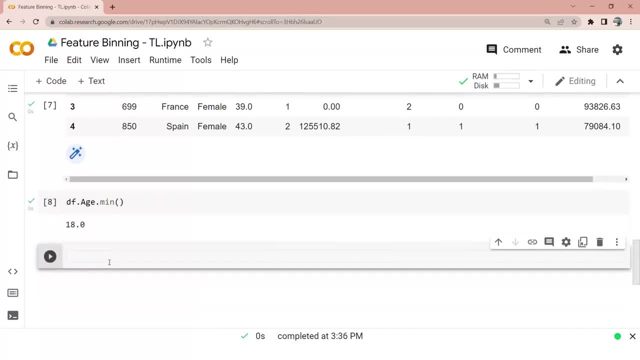 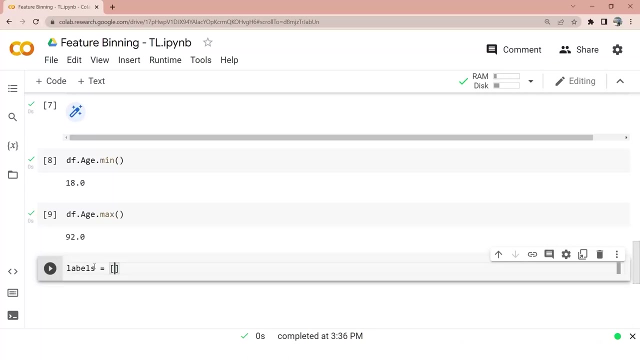 so what's my age? the minimum value is 18 and the maximum value is 92. okay, so 18 till now. let's say i'm going to create some labels, labels 0 to 20, 21 to 40, 41 to to 60 and 60 plus 61 plus or above 61, simply above 61. okay, and then i'm going to create my bins. 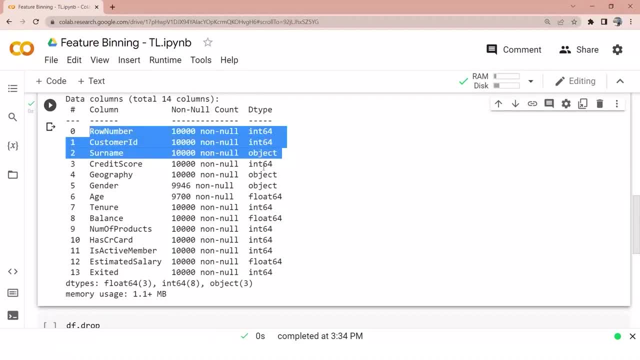 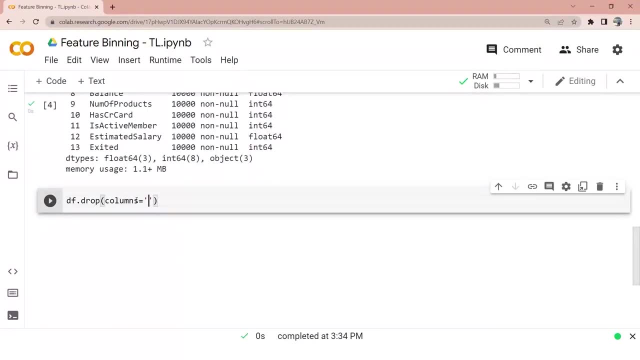 to drop some of these random columns, which makes no sense in our analysis process. so it's a very good exercise to drop off you don't need for your analysis because unnecessarily they will be eating up your space and memory. so customer id, row number and surname- what else we will delete it from access. one in place equals to two in place. 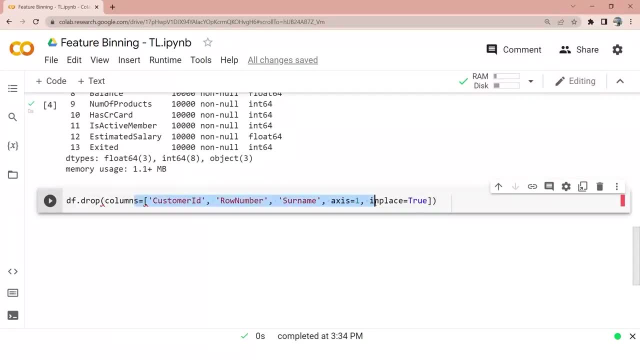 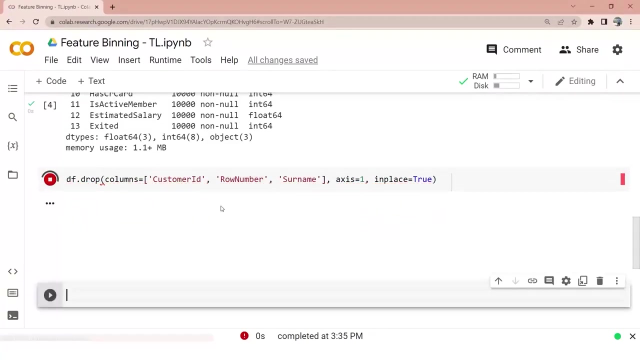 equals to two. basically means, when you are performing this task, you are. you don't need to assign the same thing to your data frame directly. your data frame will be updated. dfdrop columns equals to this. brackets close access here. done so. okay, so my data frame is dropped. my three columns are dropped, in case you want to check your new. 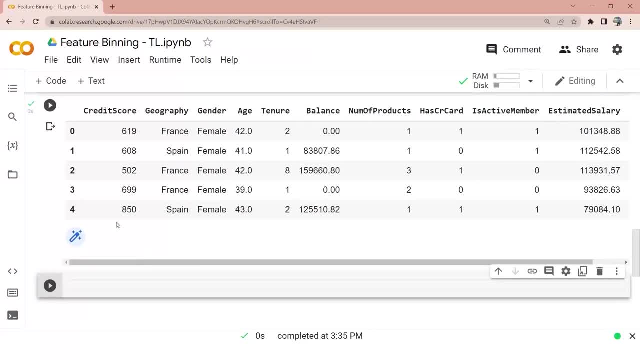 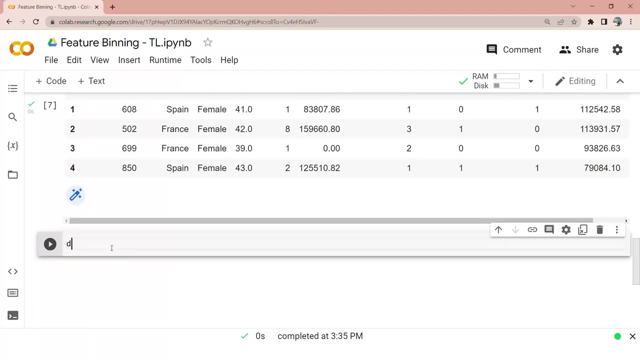 data frame. that's how it looks like. my features that are not important. they are gone right, even though it makes no sense for this particular activity, but it's a good practice to do so. we will get started with the binning technique. so let's say i am going to use age, so what's my age? the minimum value is 18. 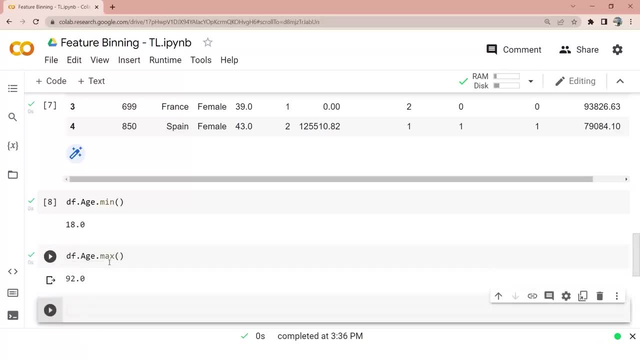 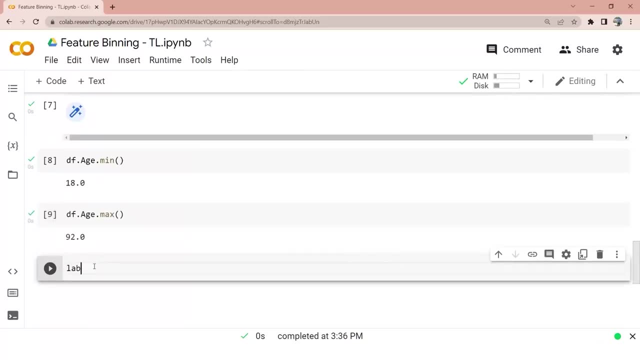 and the maximum value is 92. okay, so 18 till 92.. now let's say i am going to create some labels, labels 0 to 20, 21 to 40, 41 to 60 and 60 plus now, 61 plus or above 61, simply above 60, okay. and then i'm going to create my bins: 0, 21, so 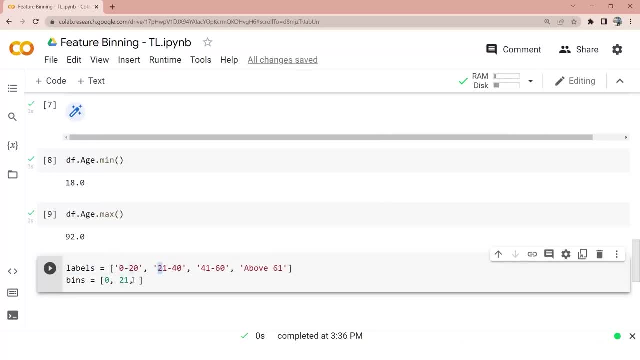 basically, bins has to be the first number from each of your labels, 21.. 41, 61 and let's say, the last number could be 100, which basically means any, any number beyond your maximum value. so let's give 100. so here i'm going to create my age: bins, age. 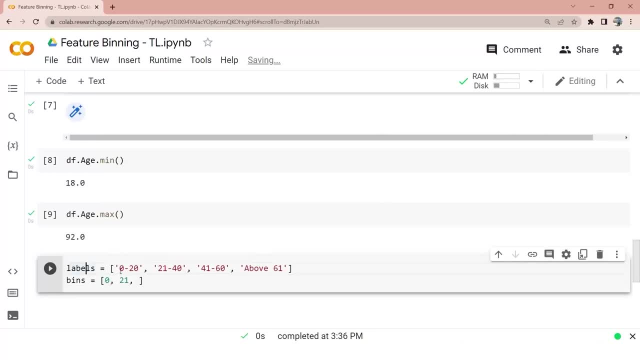 0, 21. so basically, bins has to be the first number from each of your labels: 21, 41, 61 and, let's say, the last number could be 100, which basically means any, any number beyond your maximum value. so let's give 100. so here i'm going to create my age bins. age bins is equals to pdcut. 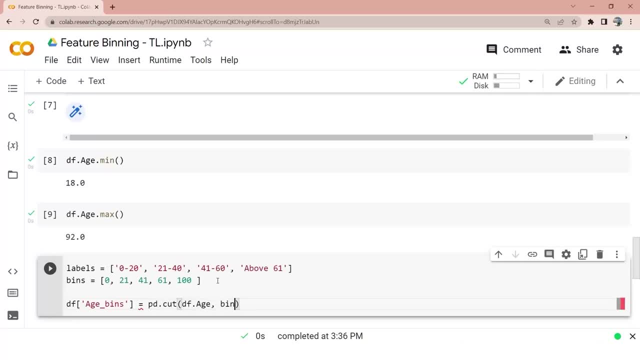 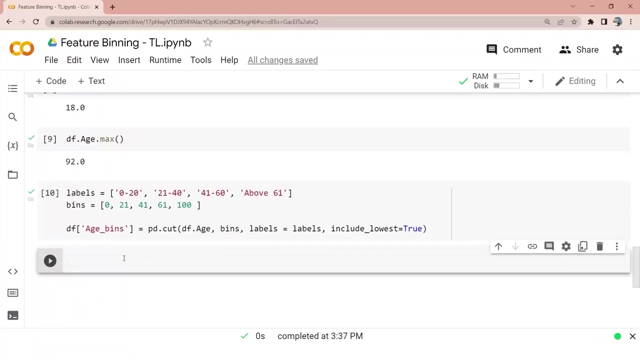 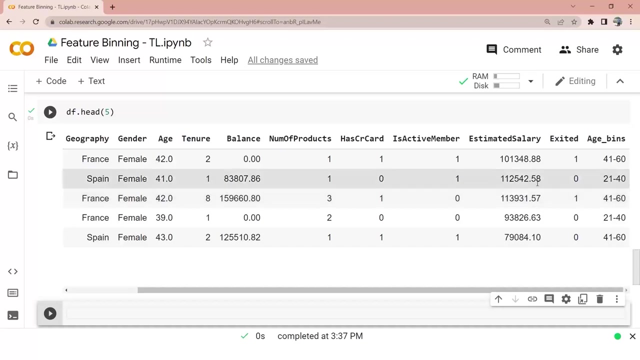 i'm going to pass my age. i'll pass my bins. i'll pass my labels equal to labels in include lowest equals to true. the moment i do this, my bins should be created. df dot head file. you can see that my age bins are created. you can compare 42 falls under this category, which is true. 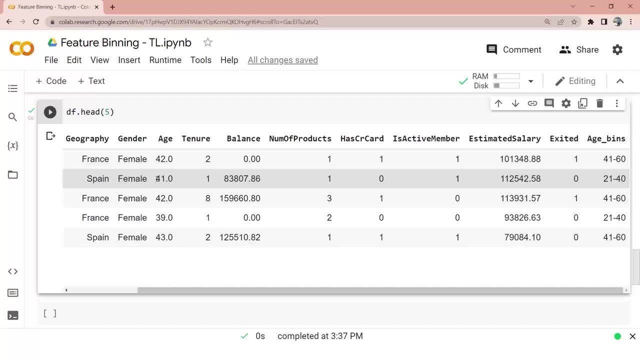 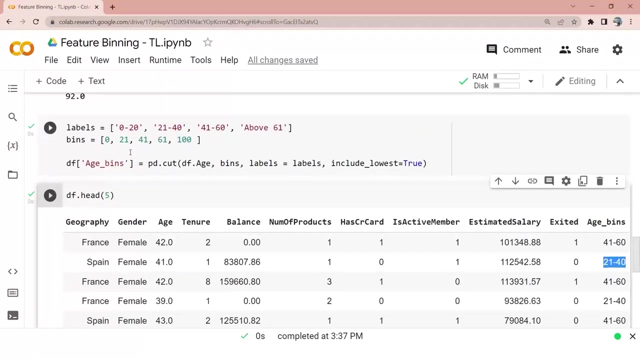 this is some mistake. 41 falls under this category. this falls under this category. why this one has not been into this category? that's going to be a problem. okay, 41 is considered in. uh, it's considered in the second category, so let's just change it to 20: 60. 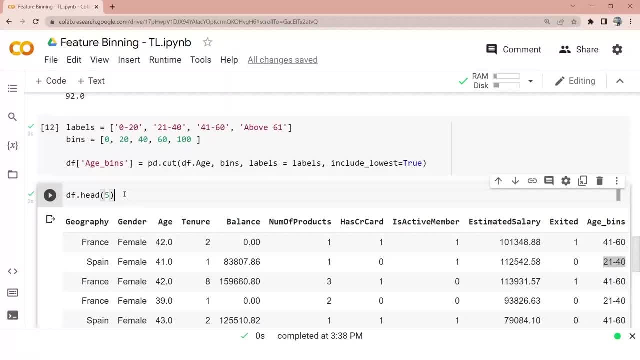 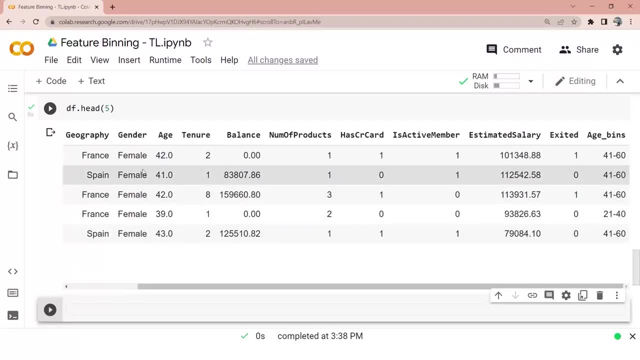 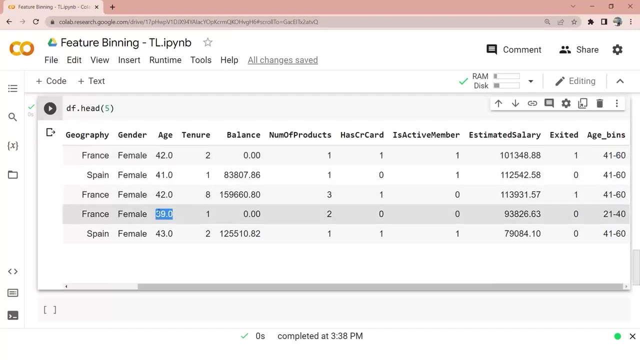 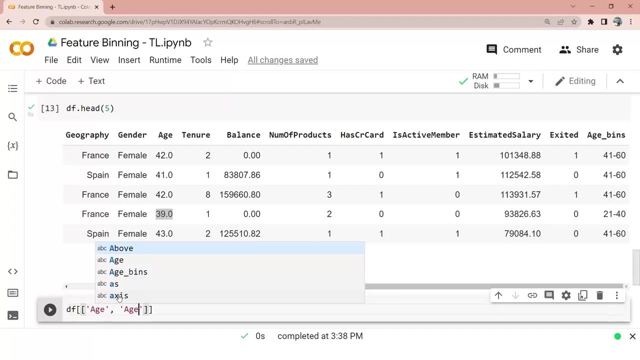 let me run this. yeah, now it works. you can just cross check this thing. for age 42, it falls in this category. 41 to 60, this is 21 to 40 and so on, if you want to just check df of age and age bins. 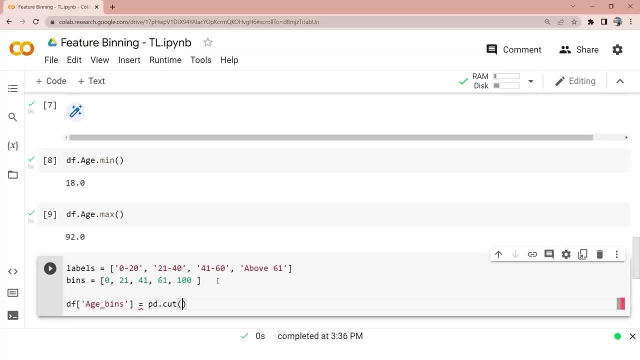 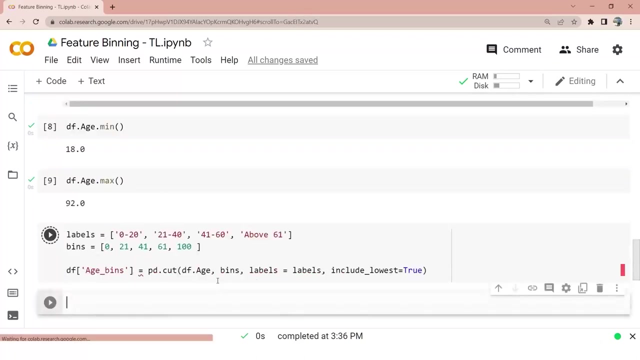 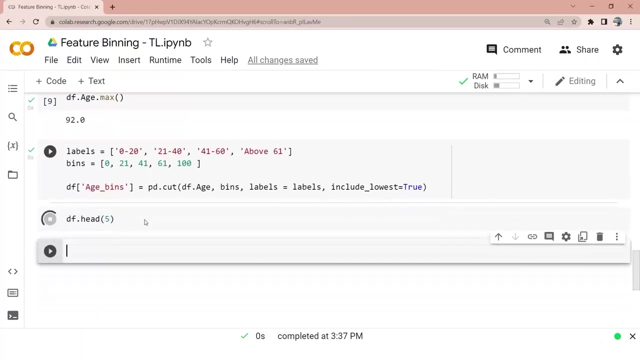 bins is equals to pdcut. i'm going to pass my age. i'll pass my bins. i'll pass my labels. equals to labels include lowest equals to true. the moment i do this, my bins should be created. dfhead file- you can see that my age bins are created. you can compare 42 falls. 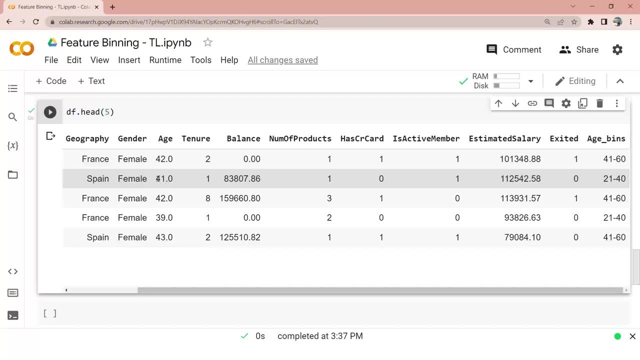 under this category, which is true. this is some mistake. you can see that my age bins are created. you can compare: 42 falls under this category, which is true. 41 falls under this category. this falls under this category. why this one has not been into this category? that's going to be a problem. 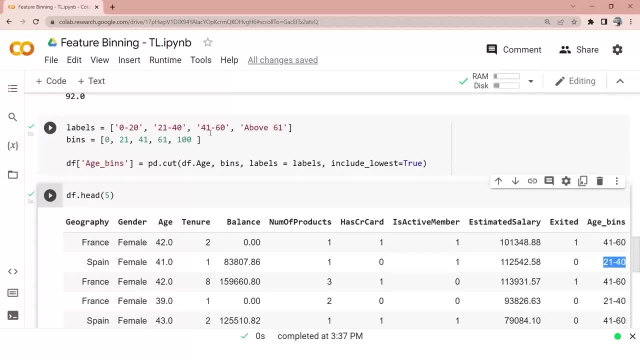 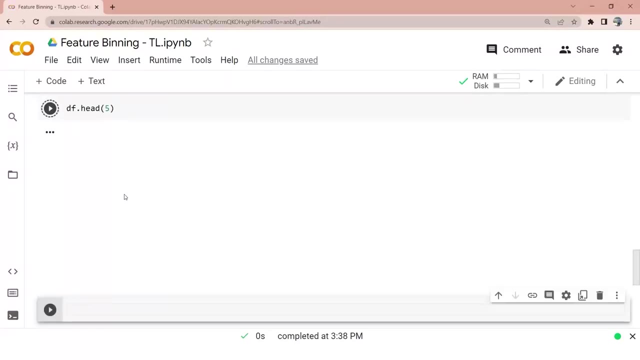 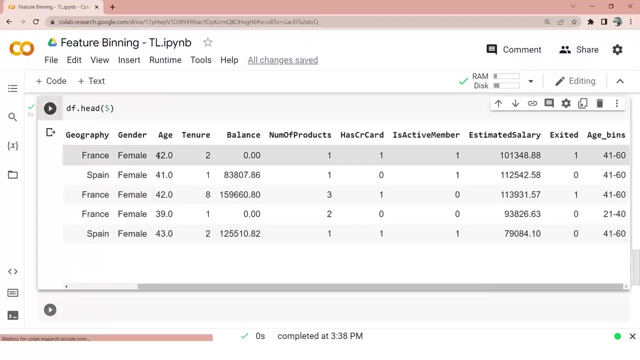 okay, 41 is considered in. uh, it's considered in the second category, so let's just change it to 20- 40.60.100. let me run this. yeah, now it works. you can just cross check this thing. for age 42, it falls in this category. 41 to 60, this is 21 to 40, and so on. if you want to just 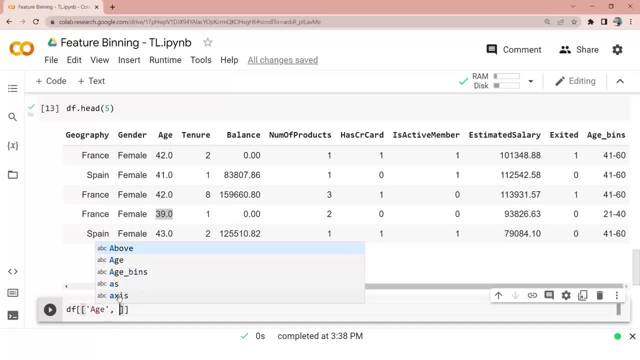 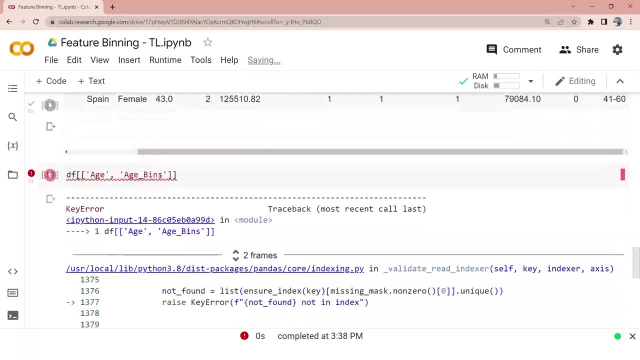 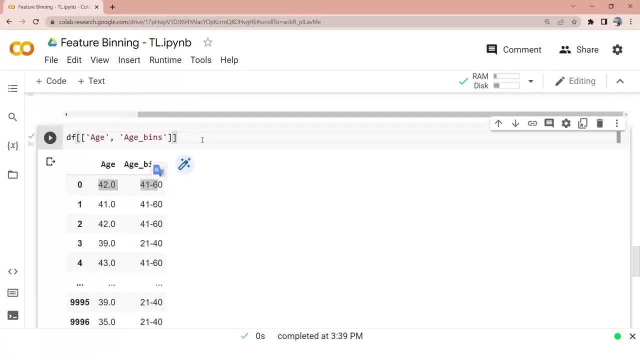 check df of age and age bins. if you want to just check df of age and age bins, so you can. you can just cross check for all the items. in case you want to convert it into a csv file and you want to check it, you can do that to csv and let's say testcsv, the. 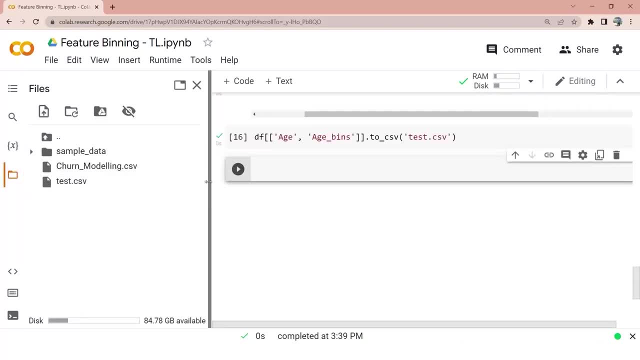 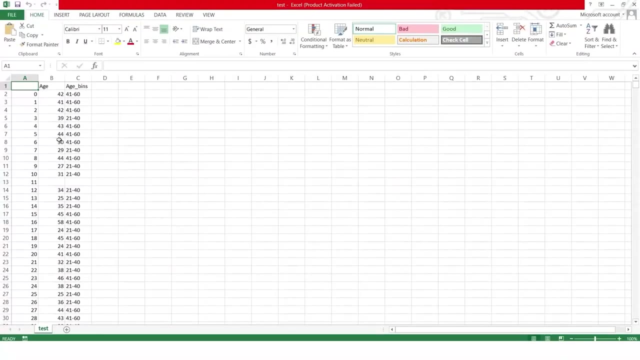 moment you do this, your testcsv is created. download it. as we are using google collab, we have to do this, or else, if you are using jupyter notebook, your file will be created in your local system in the same folder itself. now, in this case, i will just quickly cross. 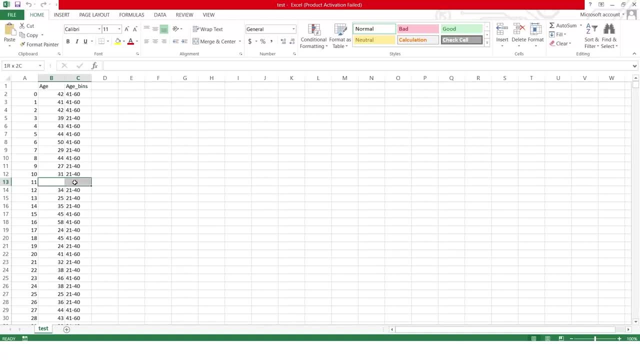 check, there is a null value. for null value it has not imputed anything, so in order to do it for the null values also, if you are going to perform some feature binning activity, make sure you have already treated your null values before doing this step, else there is. 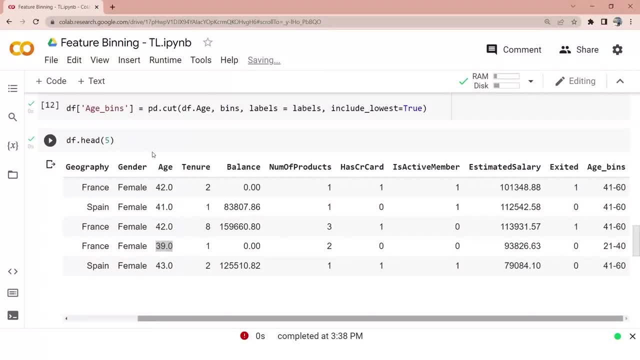 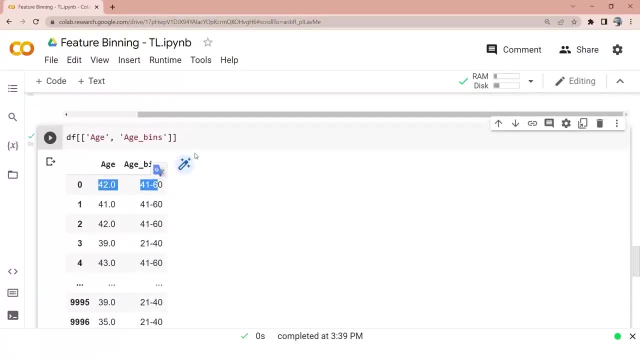 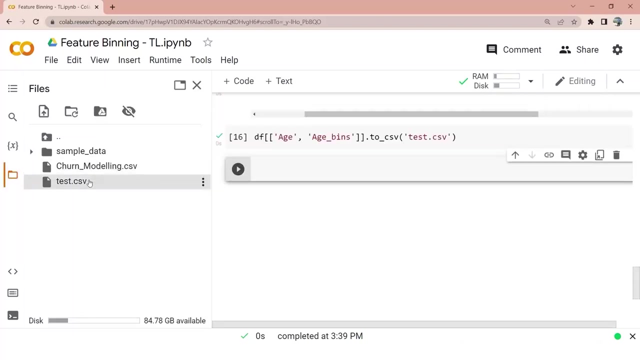 age bins. yeah, age bins, age bins. small bit so you can. you can just cross check for all the items. in case you want to convert it into a csv file and you want to check it, you can do that to csv and let's say testcsv. the moment you do this, your testcsv is created. download it. as we are using google collab, we have to do this, or else, if you are using jupyter notebook, your file will be created in your local system in the same folder itself. 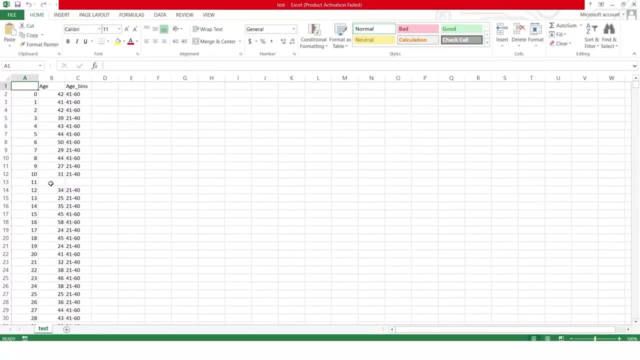 now. in this case, i will just quickly cross check- there is a null value. for null value. it has not imputed anything. so in order to do it for the null values also, if you are going to perform some feature billing activity, make sure you have already treated your null. 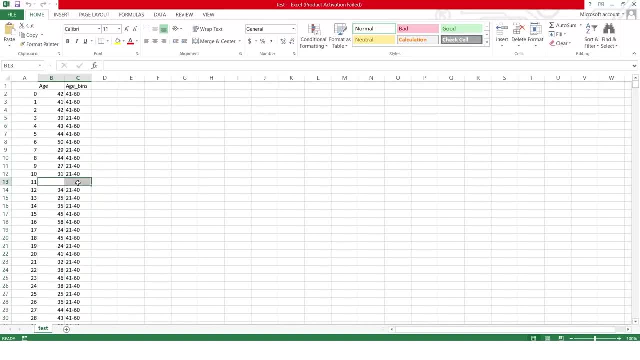 values before doing this step, else you will have to impute your null values twice. so i will cross check some of these entries. this is fine, fine, fine, fine, fine. so almost, it has done a good job. so my bins are ready. so finally, my bins are ready, just in case i want to check. 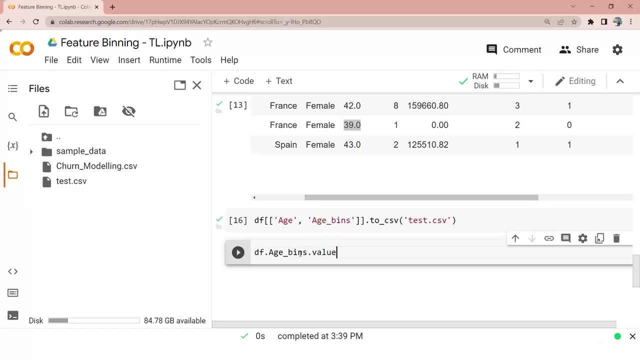 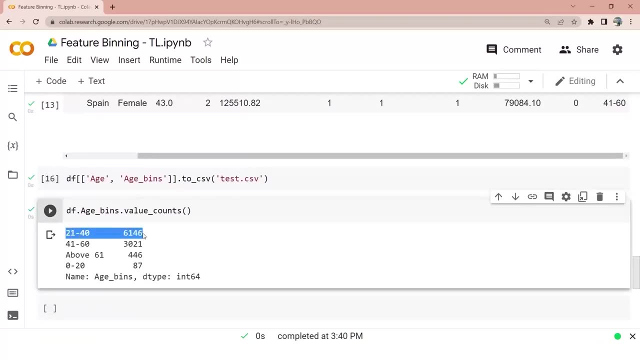 my age bins value counts. that means how many records do we have for each bins? you can see most of the people are in this category, six thousand one hundred and forty six falling under this category. if you feel it's too much of people falling into one single category, you can further divide it into twenty one to thirty and thirty. 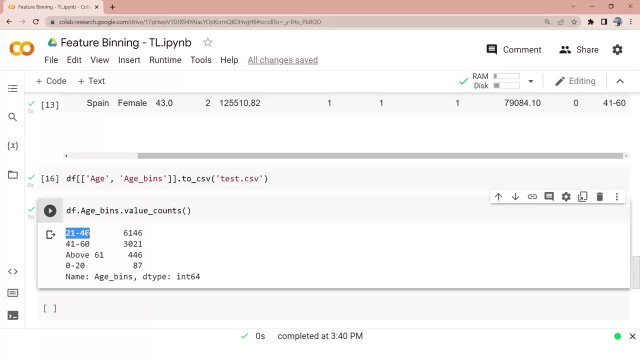 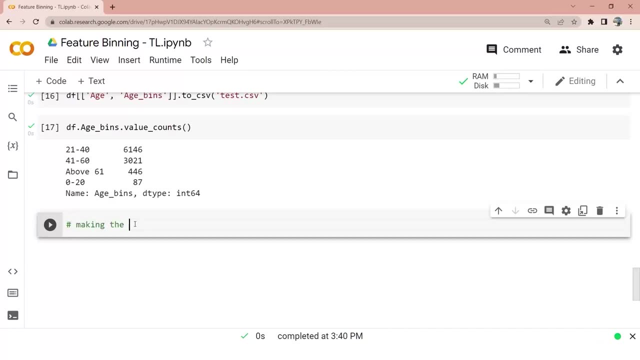 one to forty, so it all depends on your use case. let's say, we want to plot this particular bins, so i will quickly write a small code making the bar chart on the data plt dot bar. i will pass my labels. i will pass my labels and i will pass my labels and we will pass. 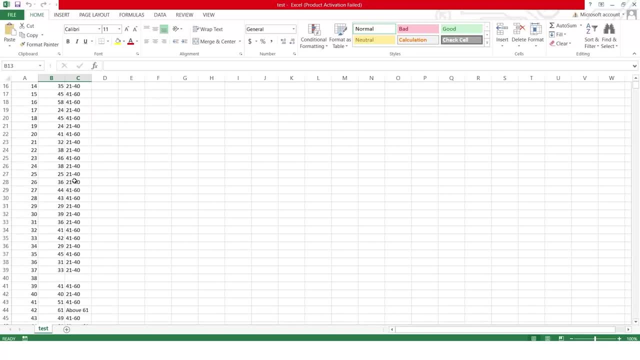 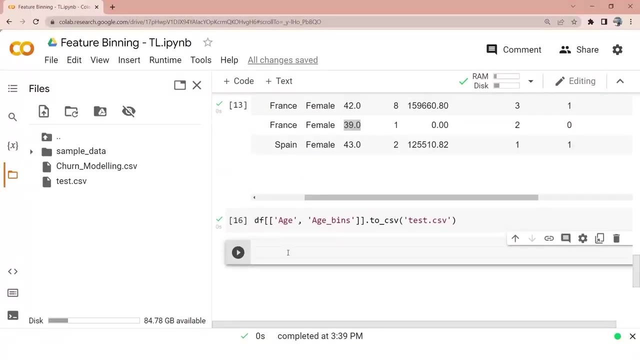 no null value, you will have to impute your null values twice. so i will cross check some of these entries. this is fine, fine, fine, fine, fine. so almost it has done a good job. so my bins are ready. so finally, my bins are ready. just in case i want to check my age: bins value. 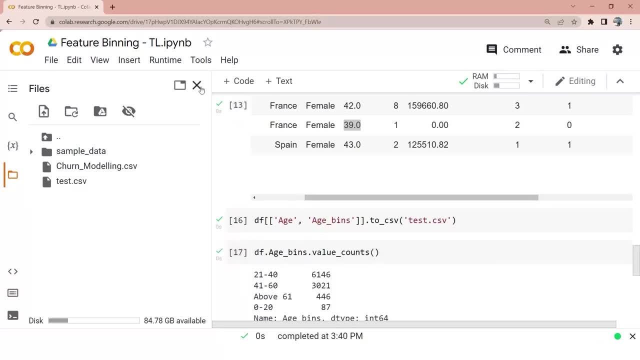 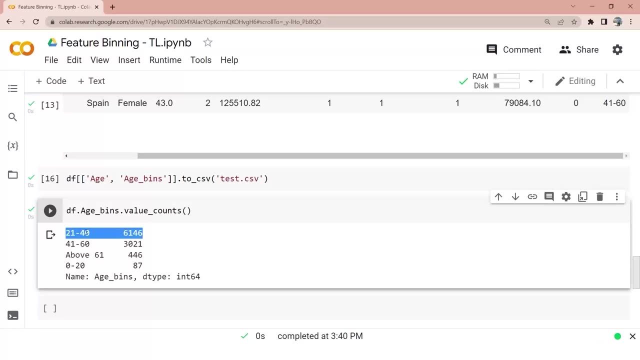 counts. that means how many records do we have for each bins? you can see most of the people are in this category: 6146 falling under this category. if you feel it's too much of people falling into one single category, you can further divide it into 21. 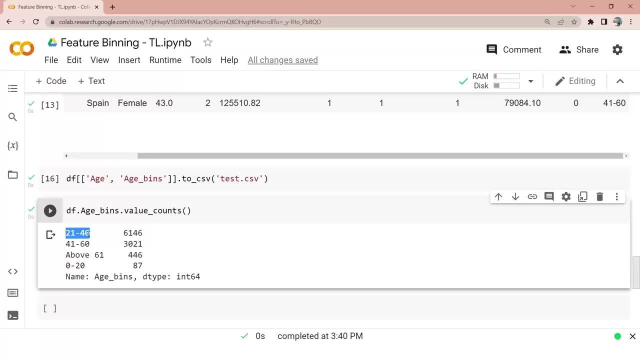 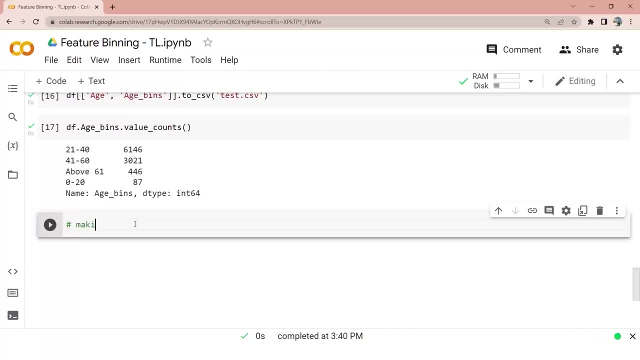 to 30 and 31 to 40, so it all depends on your use case. let's say, we want to plot this particular bins, so i will quickly write a small code making the bar chart on the data, and i'm just going to write this as my label, and then i will go to the next step and i 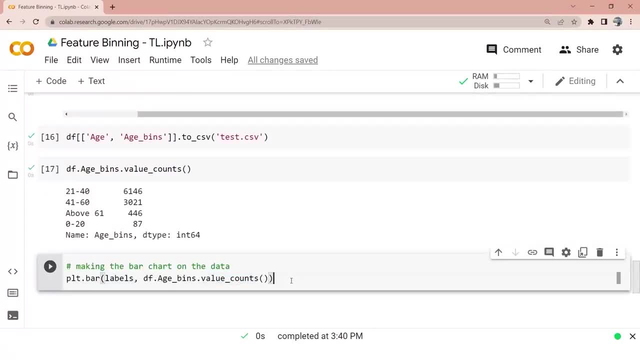 will pass my labels, i will pass my age bins, dot, value counts. so basically, i am asking my bar chart to take the labels as my x-axis and take the value counts as my y-axis and then giving the title: so plt, dot, title, age count, and then, and then i altogether have minus 86 and plus max, just negative 8. and so this is how i have developed a value and i have taken x in that text and i have added a value and i have added a value in here, and so now i have added a value in. this says: what does this mean? the value is just for each. 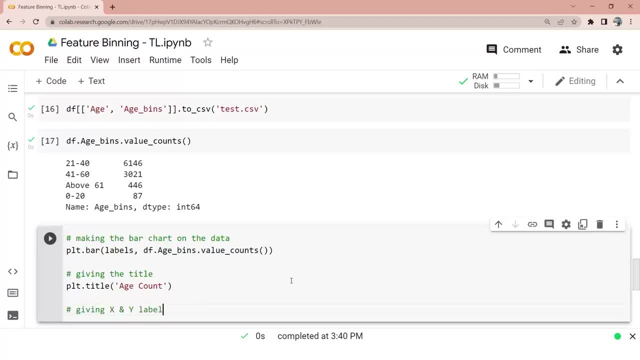 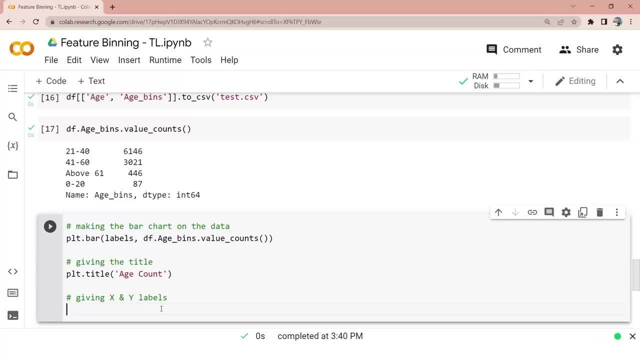 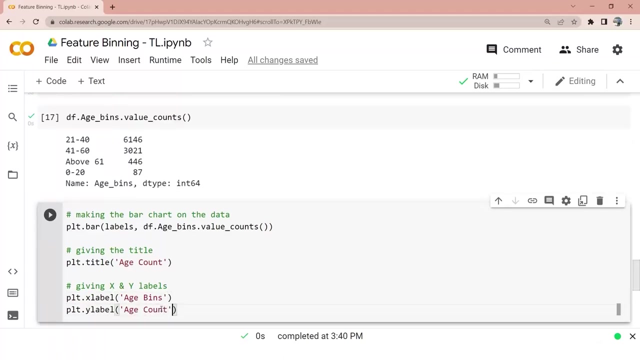 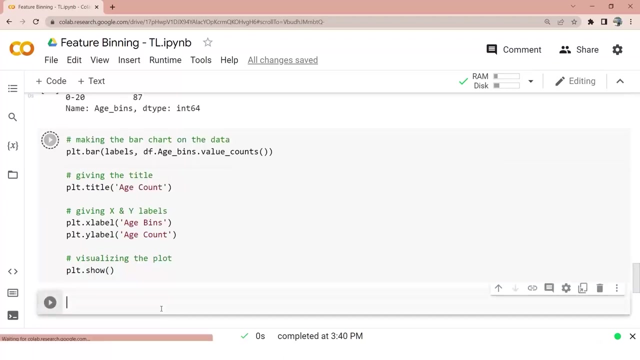 giving x and y labels. that means on your chart, what do you want to write in the x axis and in the y axis? so, plt dot x label. i will give it as age bins and age bins. plt dot y label, age count. and then, finally, visualizing the plot, plt dot show. run this and you can see that that's how. 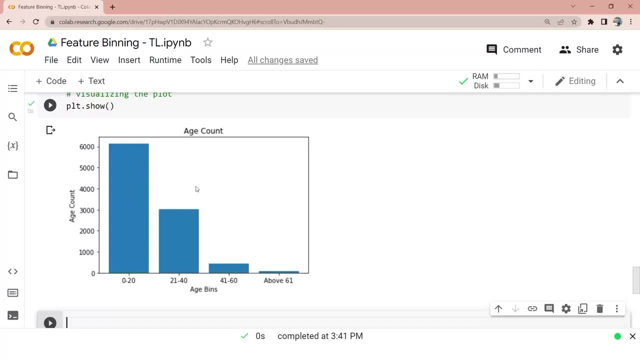 your graph looks like now. this is quite easy to visualize as compared to your numerical attribute. apart from this, if you want to add labels on top of your graphs, that is also possible. however, it's not a part of feature binning, but actually you can do that by adding labels on top of your graph. 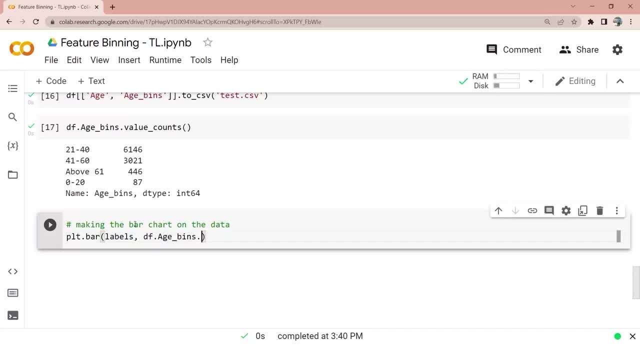 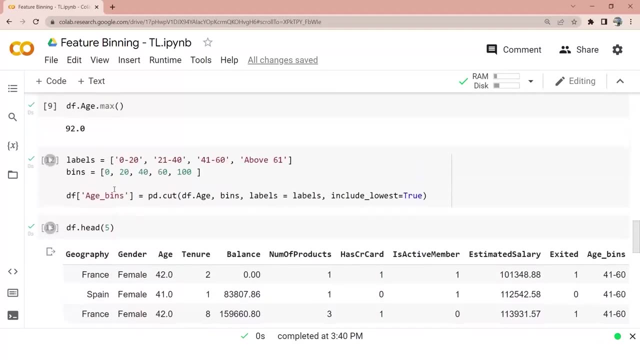 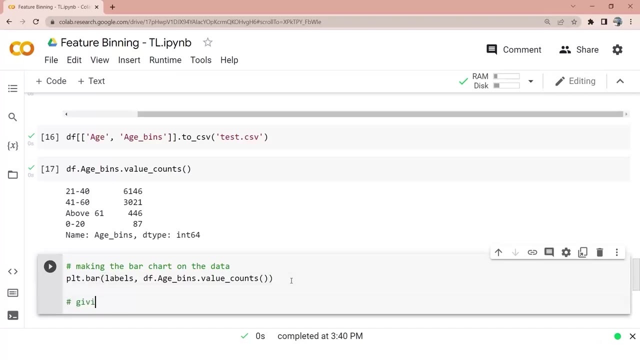 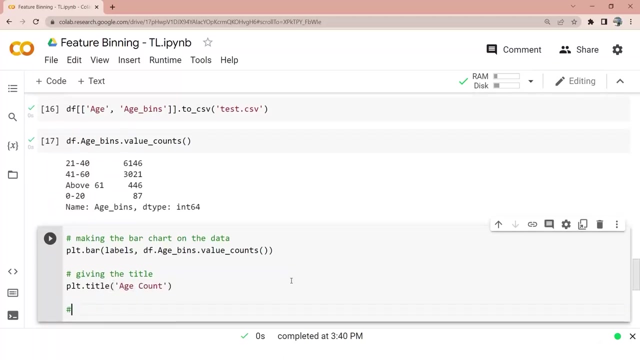 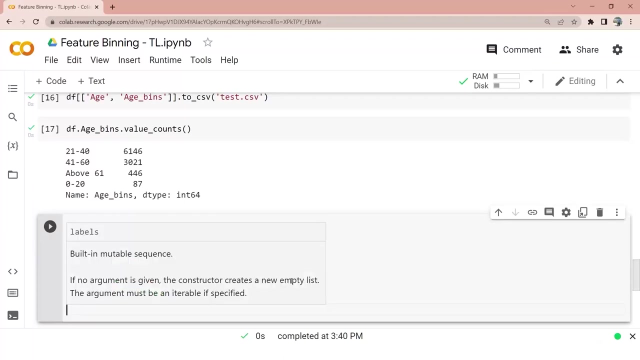 my age bins, dot, value counts. so basically i am asking my bar chart to take the labels as my x axis and take the value counts as my y axis and then giving the title, so plttitle, age count, and then giving x and y labels. that means on your chart. what do you want to write? 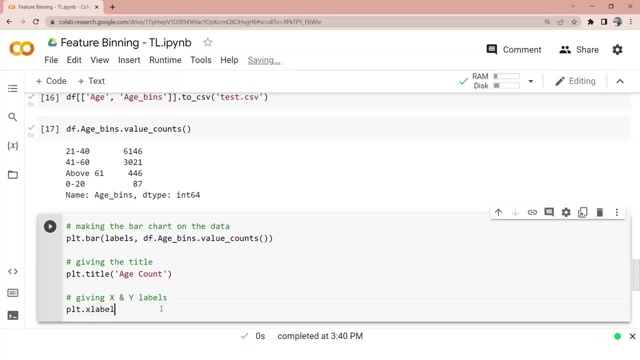 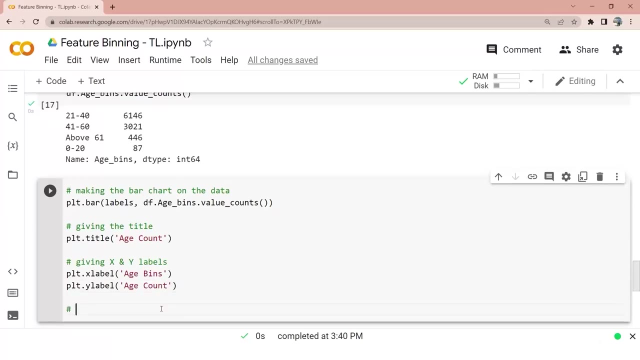 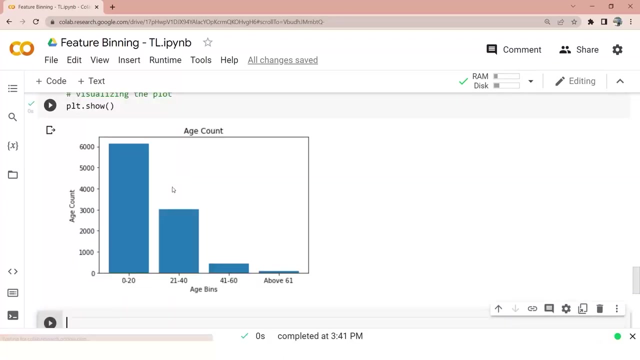 in the x axis and in the y axis. so pltx label- i will give it as age bins and age bins. plty label, age count and then, finally, visualizing the plot, pltshow. run this and you can see that that's how your graph looks like now. this is quite easy to visualize as compared to your numerical attribute. 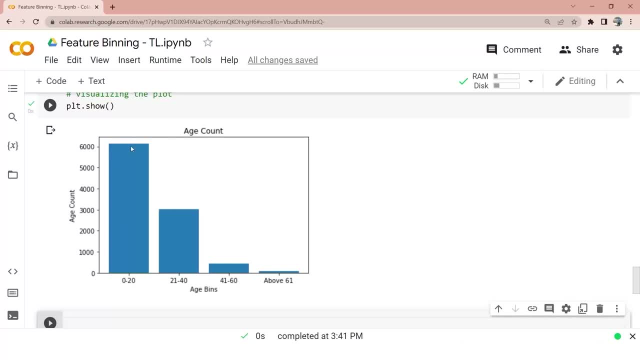 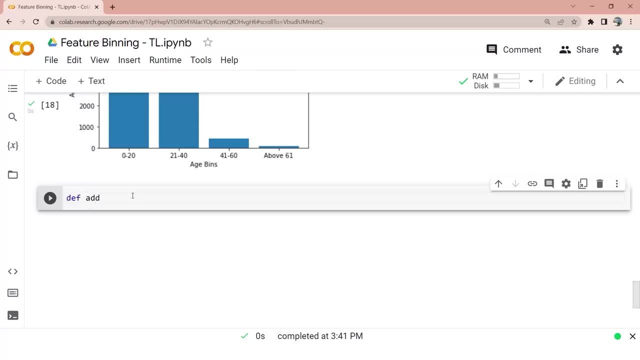 apart from this, if you want to add labels on top of your graphs, that is also possible. however, it's not a part of feature binning, but i'll just quickly show you how it works. let's say, i'll create my one of my functions, add labels and pass x, y and then for there. 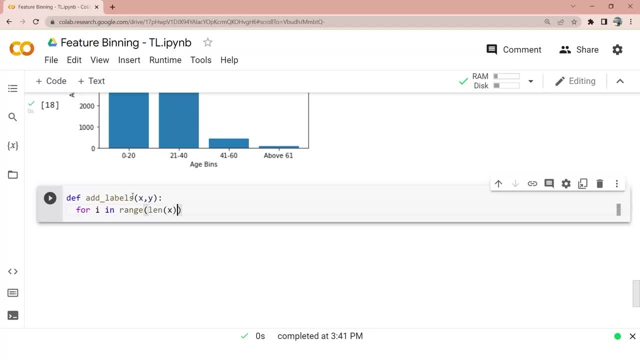 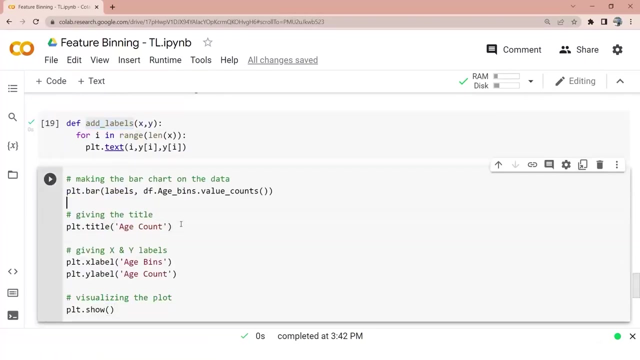 are multiple ways to do this. i'm just choosing one of these ways for i, in the range of length of x: plttext. i'm going to use plttext i, y of i, y of i done, i will copy paste this code and then i will call my add labels. 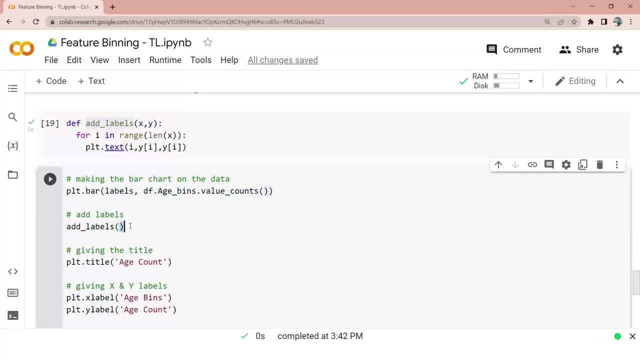 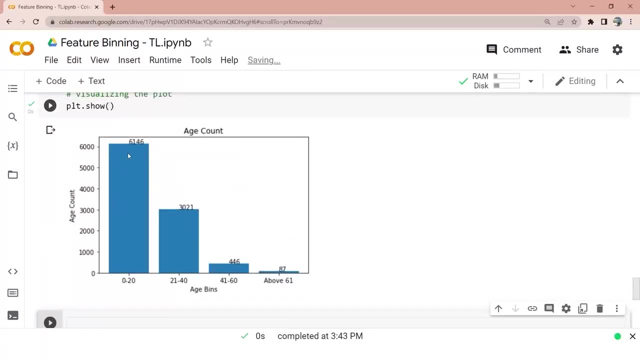 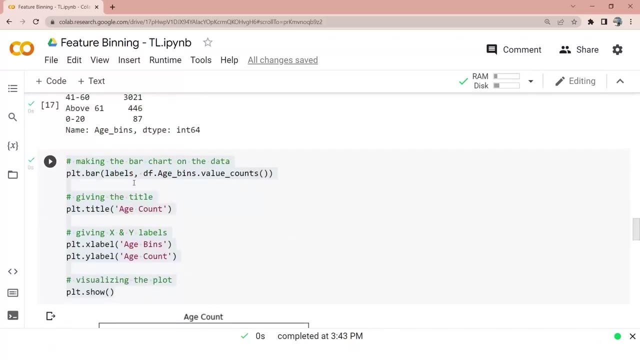 add labels and then i will push this thing, run this and you will be able to see the labels on top of the graph. so that's all about how do we perform feature binning. you can also do some other techniques to create bins. you can also use a simple for loop in that case. 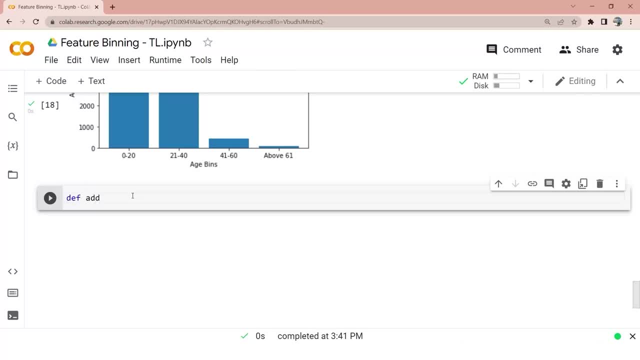 just quickly show you how it works. let's say, i'll create my one of my functions, add labels and pass x, y and then for there are multiple ways to do this. i'm just choosing one of these ways for i, in the range of length of x, plt dot text. i'm going to use plttxt i, y of i. 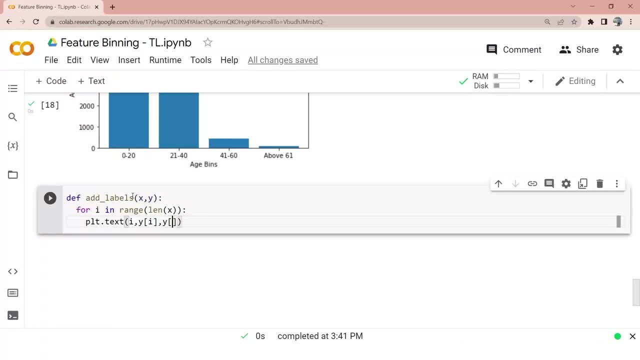 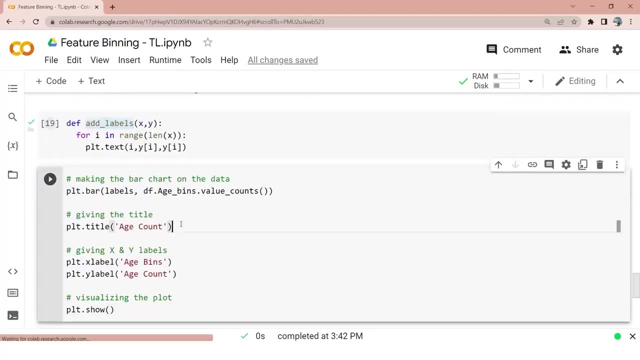 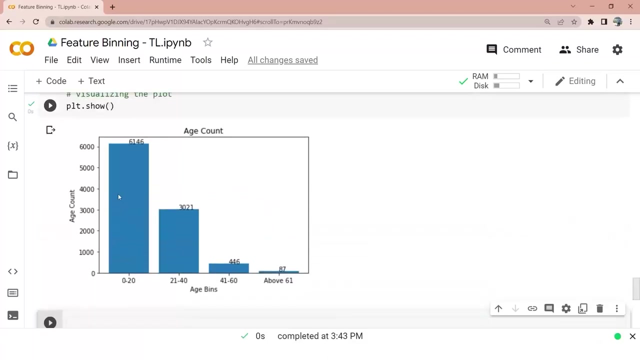 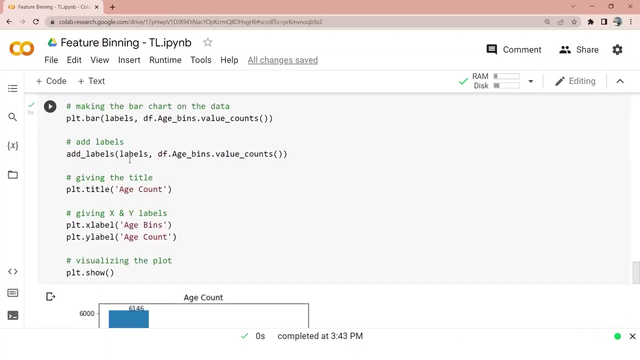 i done. i will copy paste this code and then i will call my add labels- add labels. and then i will run this and you will be able to see the labels on top of the graph. so that's all about how do we perform feature binning. you can also do some other techniques to create bins. you can also use a simple for loop in that. 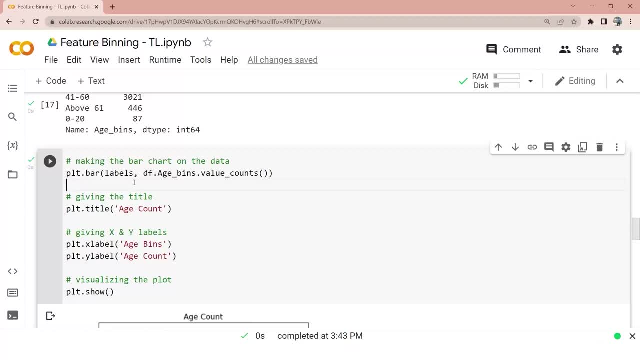 case you have to iterate through your entire data frame dot age column. wherever you see. if age greater than equals to 60, then df of age bins equals to above 60. else, if age greater than equals to 41, then df of age bins equals to 41 to 60. so you can also. 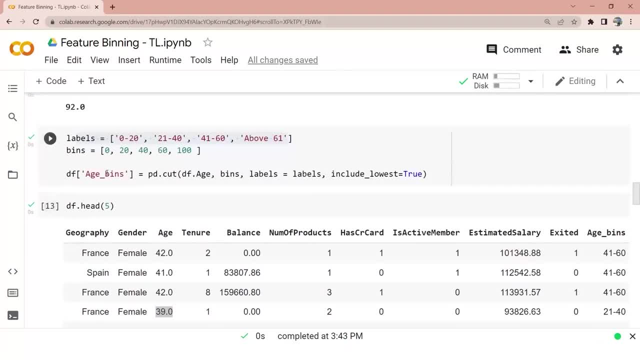 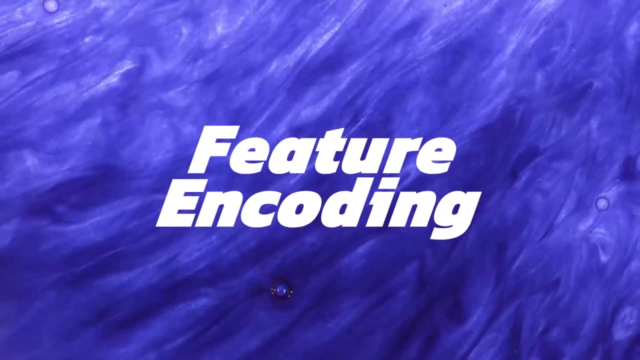 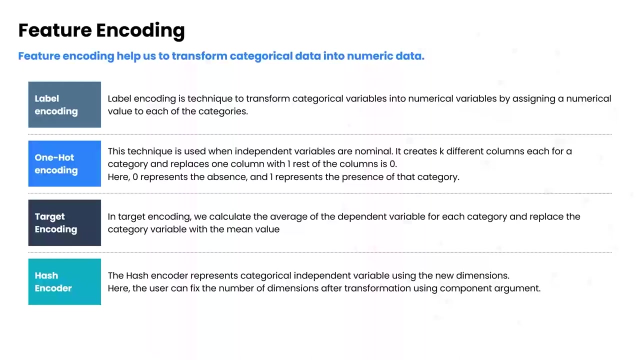 write a for loop in order to accomplish this particular task. so there are multiple ways to do this. but that's all about feature binning. i hope you understood the concepts of feature binning. in the next video we shall be jumping into the feature encoding part hi. in this session we shall be talking about feature encoding. feature encoding is one of the 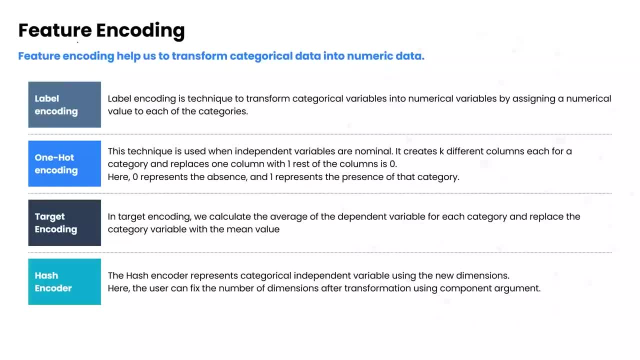 techniques where we try to encode a feature. feature encoding helps us to transform categorical data into numerical data. now, what is the need of feature encoding? let's try to understand that. as we all know, it all starts with business understanding, data understanding, data cleaning, data preparation and then eda. after eda, your next task has to be predictive model building. 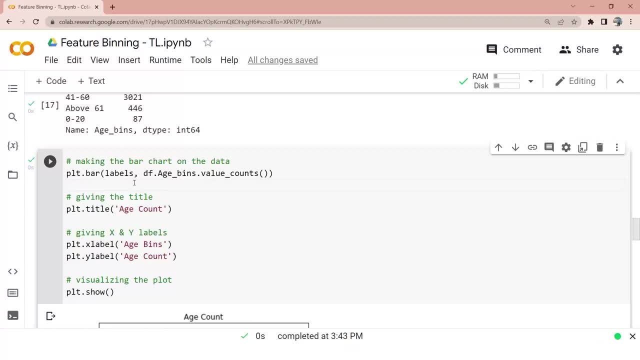 you have to iterate through your entire data frame dot age column, wherever you see. if age greater than equals to 60, then df of age bins equals to above 60. else, if age greater than equals to 41, then df of age bins equals to 41 to 60. so you can also write a for loop in order to 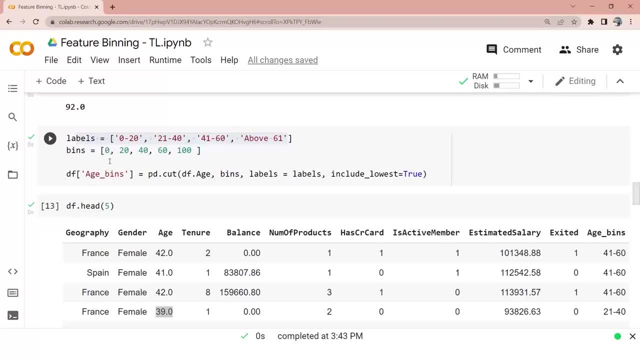 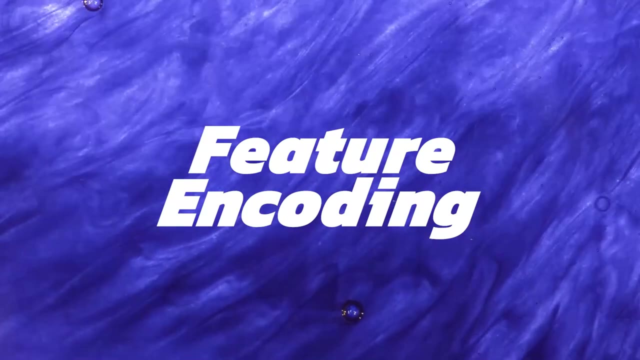 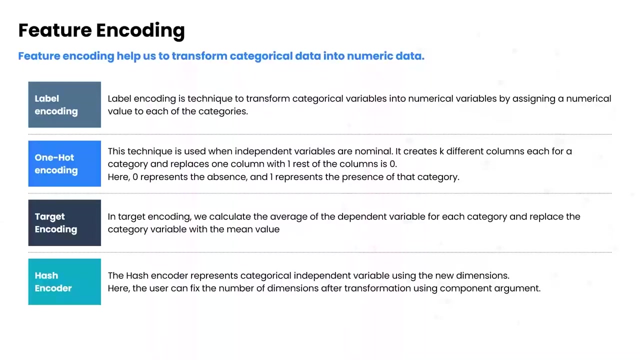 accomplish this particular task. so there are multiple ways to do this. but that's all about feature binning. i hope you understood the concepts of feature binning. in the next video we shall be jumping into the feature encoding part. hi in this session we shall be talking about feature encoding. feature encoding is one of 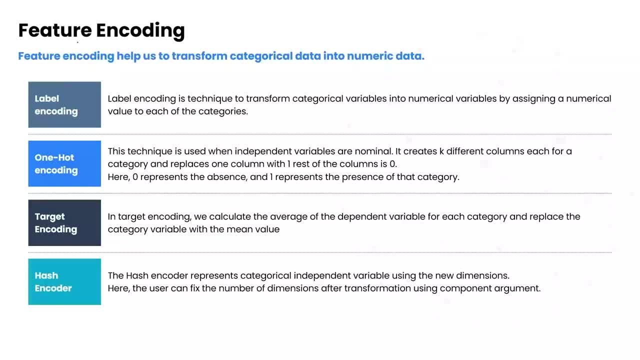 the techniques where we try to encode a feature. feature encoding helps us to transform categorical data into numerical data. now, what is the need of feature encoding? let's try to understand that. as we all know, it all starts with business understanding, data understanding, data cleaning, data preparation and then eda. after eda, your next task has to be predictive model building, or simply, 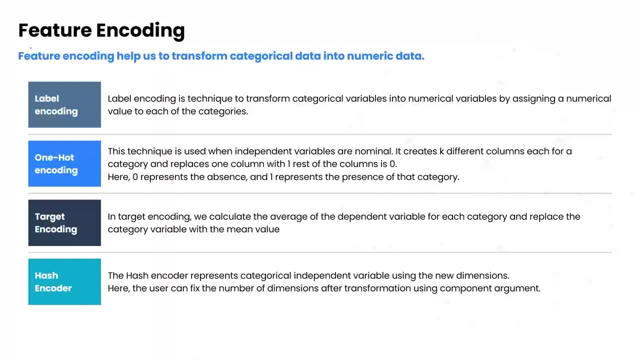 machine learning, model building, predictive analytics or predictive model building is something that we are anyways going to be talking about in this session, so let's get started. so now, what's a creative model building or standard modeling? we shall first seeим. we are going to cover in in the next. 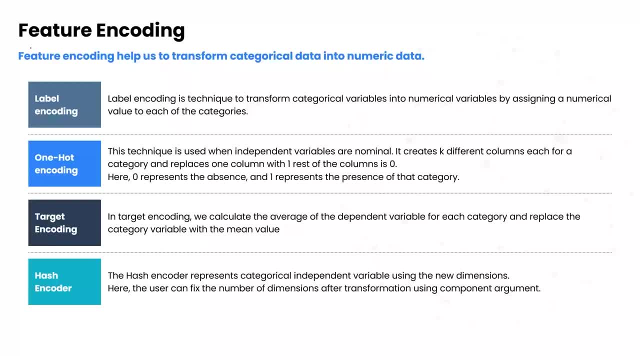 module, but let's try to understand the need of feature encoding. computers don't understand categorical data, even though categorical data could have a lot of lot of information within it. lot of information is there in both categorical and numerical data, but ultimately when you feed your data to a predictive model you heard predicted model might pass categorical. norm and numerical data. but you have to understand it well: if your data comes out, a predictive model from data which is not something illustrative, more than a very amongst, fairly in terms of information, the data right from yourわか, what you can just work with data if you. 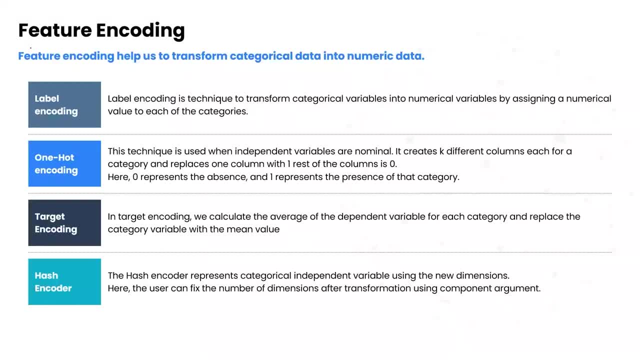 do that make up most decisions. you're good. your predictive model might not work, but the秒 em report is going to give you some information, so now click on the next module. in the next module, not be able to understand categorical data, and hence you have to end up converting a. 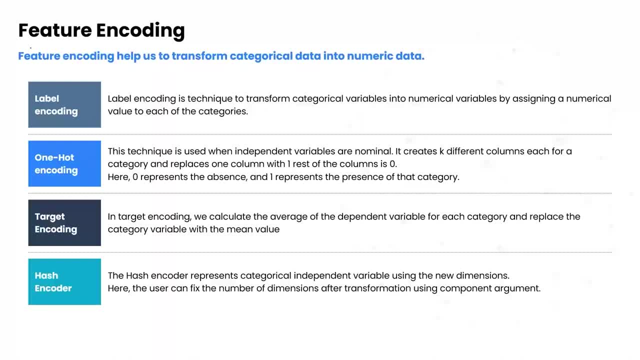 or simply machine learning model building. predictive analytics or predictive model building is something that we are anyways going to cover in in the next module, but let's try to understand the need of feature encoding. computers don't understand categorical data, even though categorical data could have a lot of lot of information within it. lot of information is there. 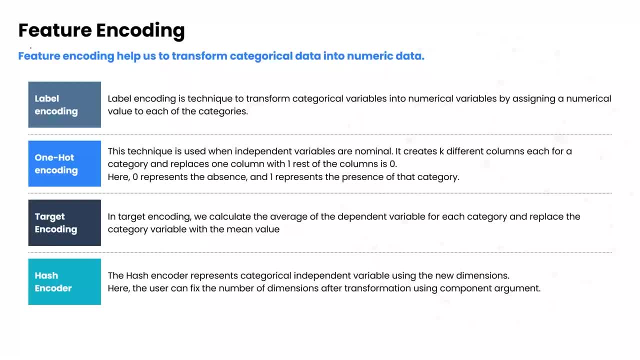 in both categorical and numerical data. so let's try to understand the need of feature encoding data, but ultimately, when you feed your data to a predictive model, your predictive model might not be able to understand categorical data, and hence you have to end up converting a categorical data. 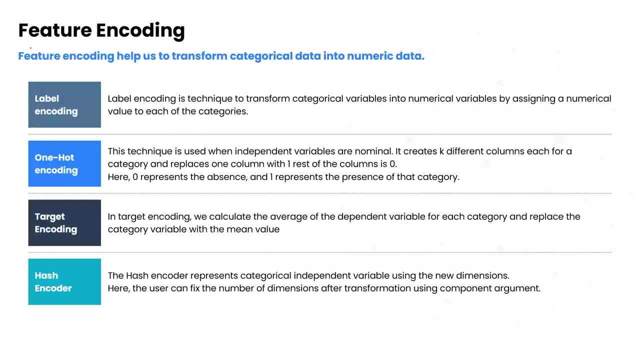 into numerical data. that conversion is basically called as feature encoding, where we convert or transform a categorical data into numerical data. the simplest form of encoding is label encoding. let's say you have a column called as gender, you have f, m, f, f and so on. the most idiotic approach to convert a categorical data to 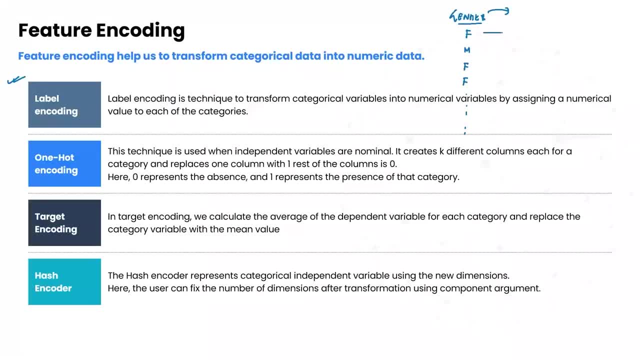 numerical data is to give them some numbers. for example, i give f number one and m number two, so all my f becomes one and all my m becomes two. so this type of function is called gender. type of technique is called as label encoding. label encoding is a technique to transform. 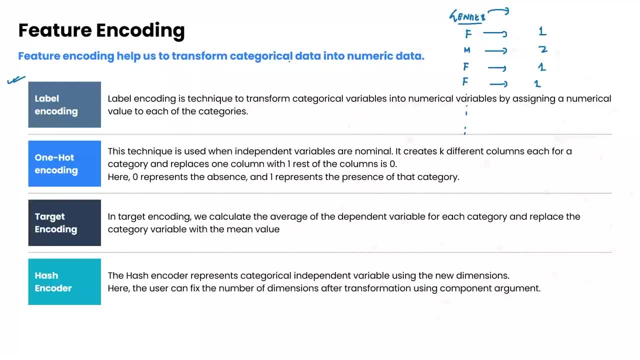 categorical variables into numerical variables by assigning a numerical value to each of the categories. let's say you have a column called as location location. you have hong kong, malaysia, india, korea. you simply give them one, two, three and four. now the drawbacks of this particular encoding technique are many. the first drawback is, if you assign such numbers, 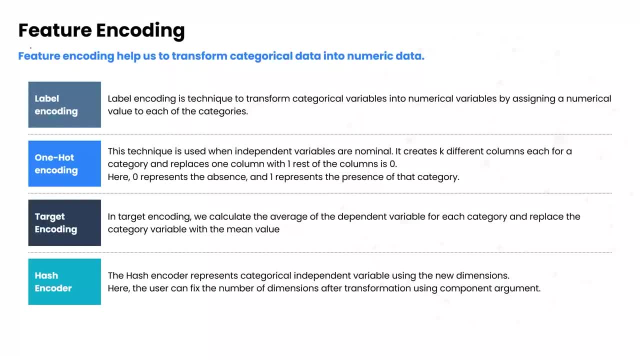 categorical data into numerical data. that conversion is basically called as feature encoding, where we convert or transform a categorical data into numerical data. the simplest form of encoding is label encoding. let's say you have a column called as gender, you have f, m, f, f and so on. the most idiotic approach to convert a categorical data to 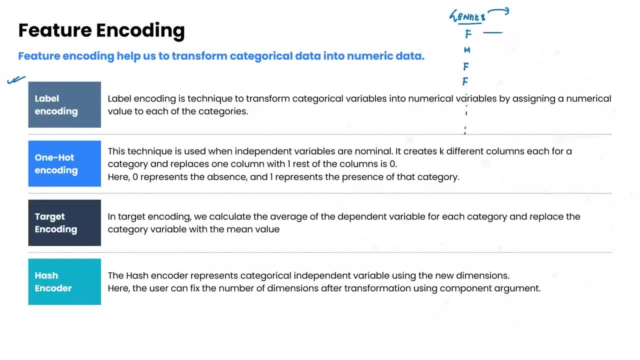 numerical data is to give them some numbers. for example, i give f number one and m number two, so all my f becomes one and all my m becomes two. so this type of technique is called as label encoding. label encoding is a technique to transform categorical variables into numerical variables by assigning a numerical value to. 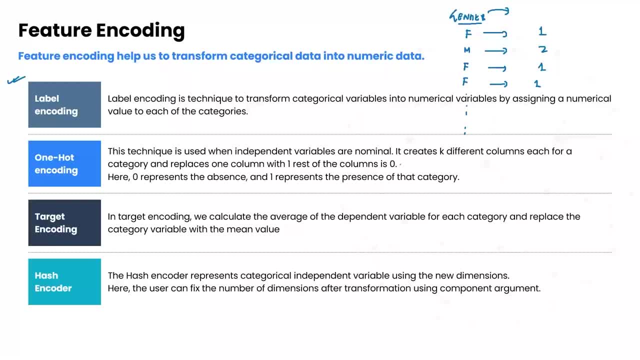 each of the categories. let's say you have a column called as location. location. you have hong kong, malaysia, india, korea. you simply give them one, two, three and four. now the drawbacks of this particular encoding technique are many. the first drawback case: if you were to assign such numbers when you feed this data to computers. 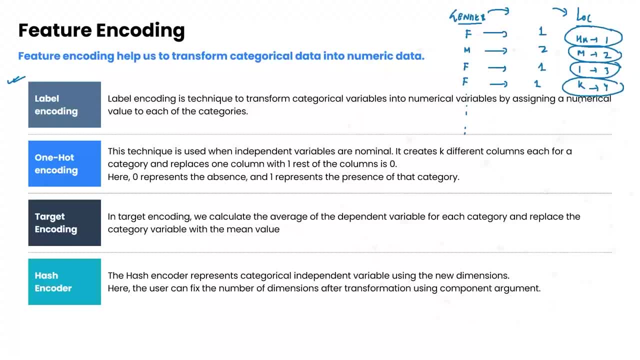 computers only understand numbers. now, in that case, your predictive model could be biased towards this number. they will be treating this number to be more priority than this number. similarly, in the case of gender, there could be a scenario where males would be treated in high priority as compared to females. 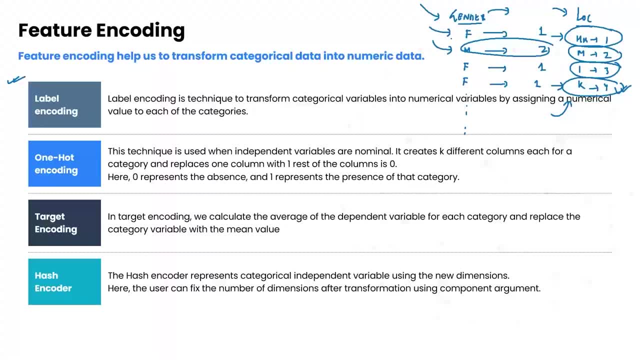 In fast-forward notes in order to have an unbiased priority, so that models won't be biased on these numbers. label encoding should not be used for your x variables or simply your independent variables. so, for example, if you are dealing with a use case, let's say you have data and you are simply doing. 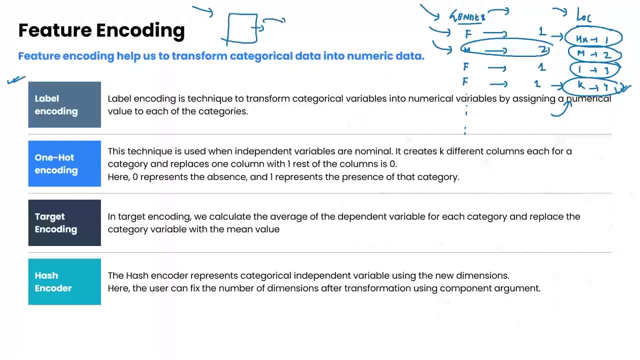 the churn analysis prediction. that means you are going to predict whether a customer is going to churned or not churned. so you have a column like churn and you have other columns as well: age, gender, bandwidth, all those things. so it is not recommended to do label encoding on x variables. 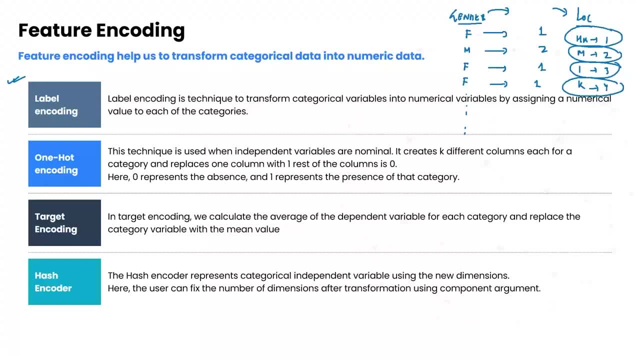 when you feed this data to computers. computers only understand numbers. now, in that case, your predictive model could be biased towards these numbers. they will be treating this number to be more priority than this number. similarly, in the case of gender, there could be a scenario where may else could be treated in high priority as compared to females, in order to have an unbiased priority. 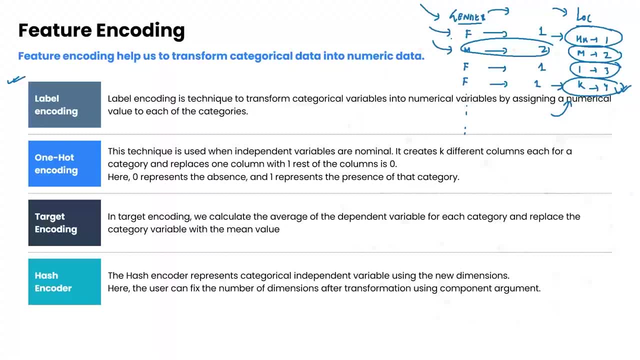 so that models won't be biased on these numbers. label encoding should not be used for your x variables or simply your independent variables. so, for example, if you are dealing with a use case, let's say you have data and you are simply doing the churn analysis: prediction. 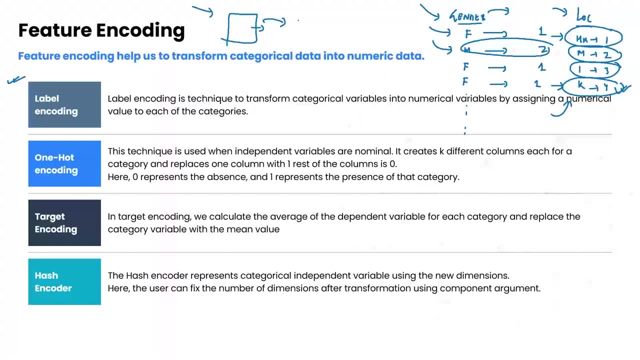 that means you are going to predict whether a customer is going to churned or not churned. so you have a column like churn and you have other columns as well: age, gender, bandwidth, all those things. so it is not recommended to do label encoding. on x variables, label encoding can be. 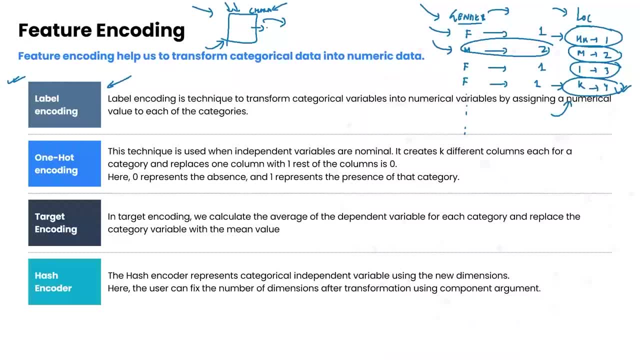 done on y variable, which has- which is a dependent variable- right, but on x variables it is not recommended. we perform label encoding using a simple technique called as label encoder. label encoder- all the encoding techniques are part of sklearn library which we will be using in the practical spot, but label encoder is something that we will be using to perform. 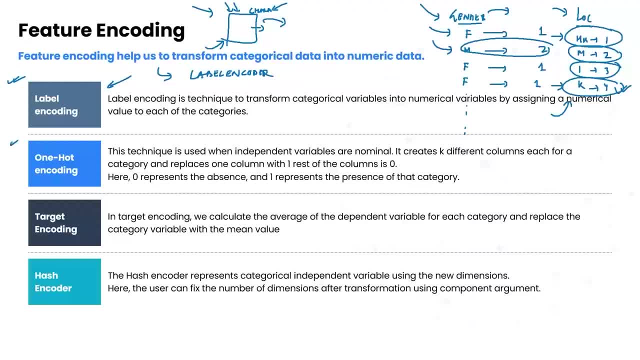 this label encoding. the second technique of feature encoding is one hot encoding. This technique is used when independent variables are nominal. What do you mean by nominal? That means they are not in a specific order. Gender is a nominal data. Location is a nominal data. It creates k different columns, each for a category. 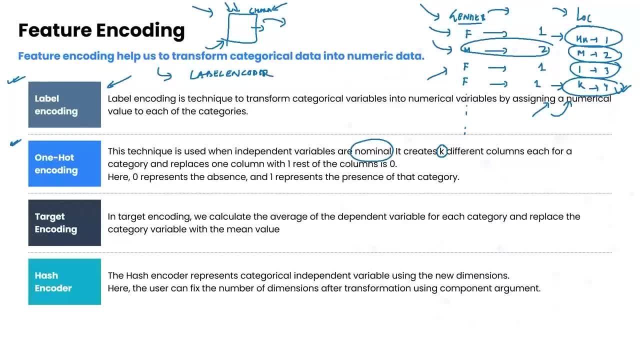 And replaces one column with rest of the columns is 0. Here, 0 represents the absence And 1 represents the presence of that category. So in simple terms, If I talk about a column called as location, Let's say I have 10 customers, Hong Kong, Who stays in Hong Kong? 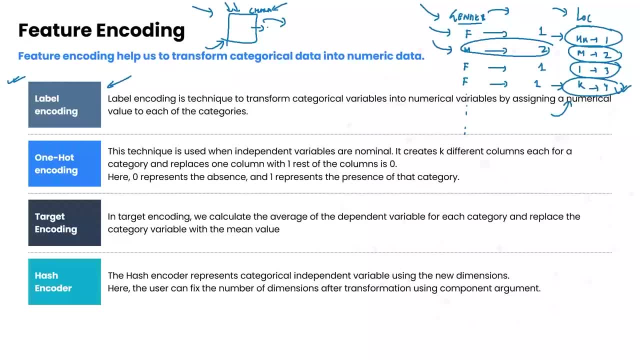 label encoding can be done on y variable, which has, which is a dependent variable, right, but on x variables it is not recommended. we perform label encoding using a simple technique of label encoding. we perform label encoding using a simple technique of label encoding called as label encoder: label encoder. 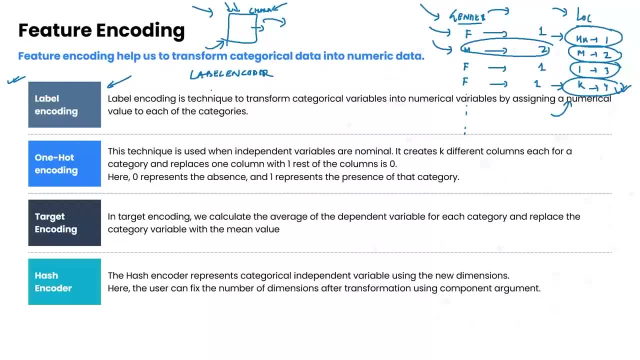 all the encoding techniques are part of sk learn library which we will be using in the practical spot. but label encoder is something that we will be using to perform this label encoding. the second technique of feature encoding is one hot encoding. this technique is used when independent variables are nominal. 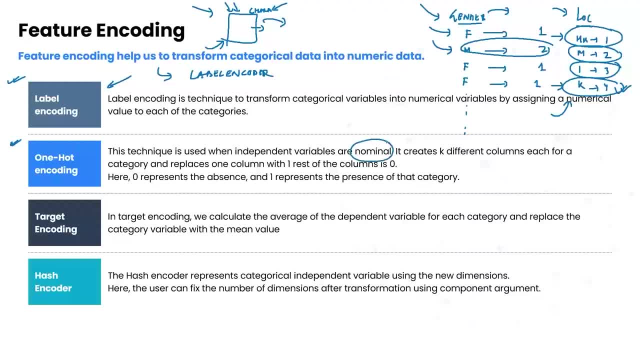 what do you mean by nominal? that means they are not in a specific order. gender is a nominal data. location is a nominal data. it creates k different columns, each for a category, and replaces one column with the rest of the columns. is zero. here, zero represents the absence. 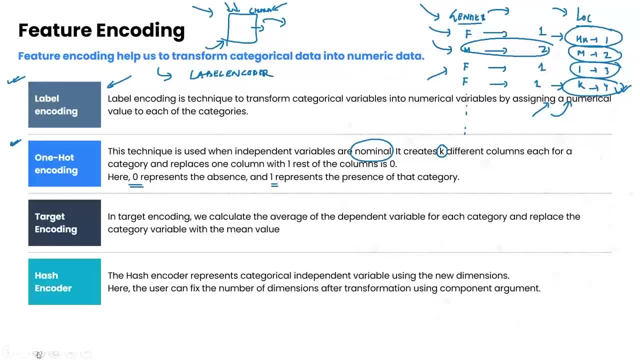 and one represents the presence of that category. so, in simple terms, if i talk about a column called as location, let's say i have 10 customers hong kong who stays in hong kong, one stays in malaysia, one stays in india. this person again stays in hong kong. hong kong, malaysia. 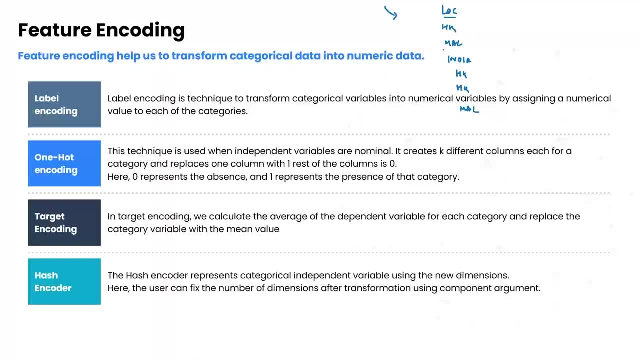 let's say i have six customers- uh, one, two, three, four, five, six- out of which two people stay in malaysia, three people stay in hong kong and one in india. if we have to perform label encoding, this becomes one, two, three, one, one, two, which is not the right step, not the right technique. 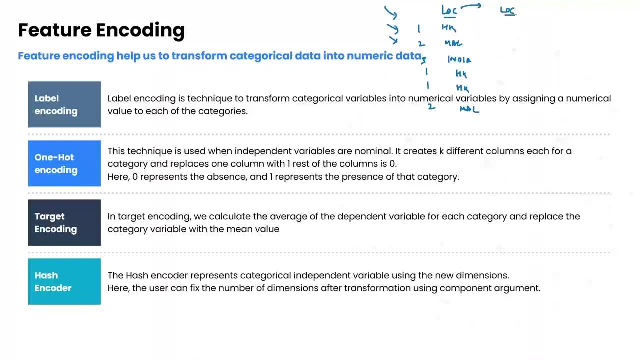 if we perform one hot encoding, what happens is it creates three columns: location underscore hk, location underscore india. location underscore malaysia. so wherever you see hk, this becomes one, others become zero. wherever you see malaysia, others become zero. the malaysia part becomes one becomes one, others are zero, one, zero, zero, one, zero, zero, zero, zero, one. and these are all your. 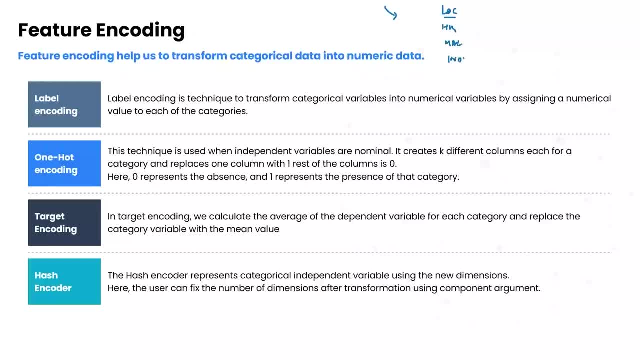 One stays in Malaysia, One stays in India. This person again stays in Hong Kong, Hong Kong, Malaysia. Let's say, I have 6 customers, 1,, 2,, 3,, 4,, 5, 6, Out of which 2 people stay in Malaysia. 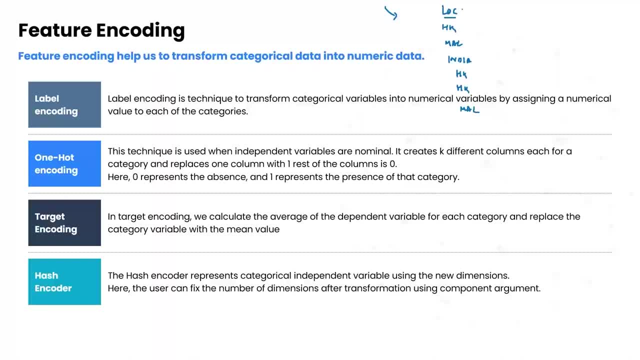 3 people stay in Hong Kong And 1 in India. So, in simple terms, If we have to perform level encoding, This becomes 1, 2, 3, 1, 1, 2, Which is not the right step, Not the right technique. 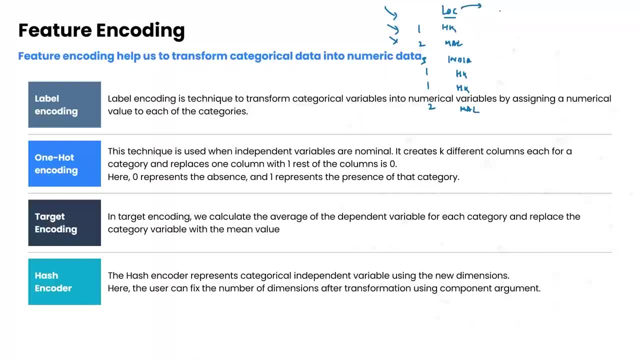 If we perform one hot encoding, What happens is it creates 3 columns: Location underscore HK, Location underscore India, Location underscore Malaysia. So wherever you see HK, This becomes 1, Others become 0. Wherever you see Malaysia, Others become 0. The Malaysia part becomes 1. 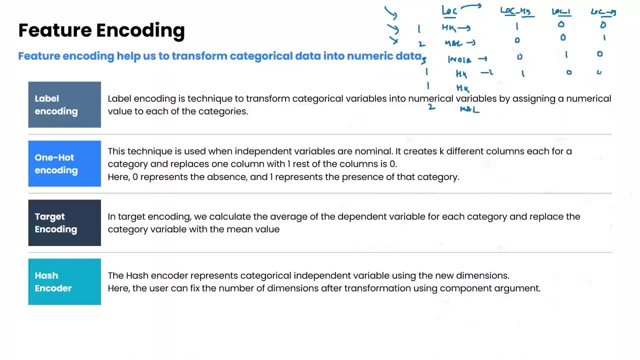 For India, this becomes 1, Others are 0, 1, 0, 0, 1, 0, 0, 0, 0, 0, 1, And these are all your newly created features As part of the one hot encoding technique. 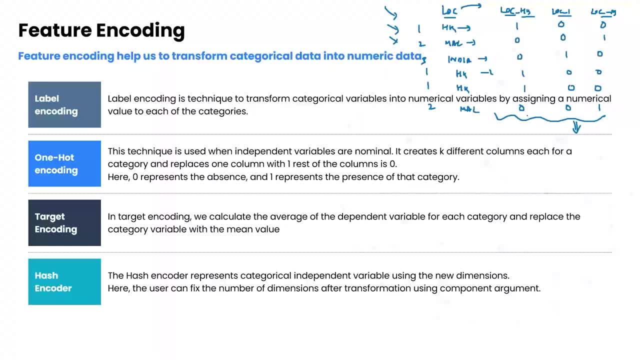 And we all know that binary is the most accepted format For computers. So one hot encoding is one of the most Preferred type of encoding technique. Apart from one hot encoding, There is also another type of encoding, Which is not mentioned here, Which is a very similar technique to one hot encoding. 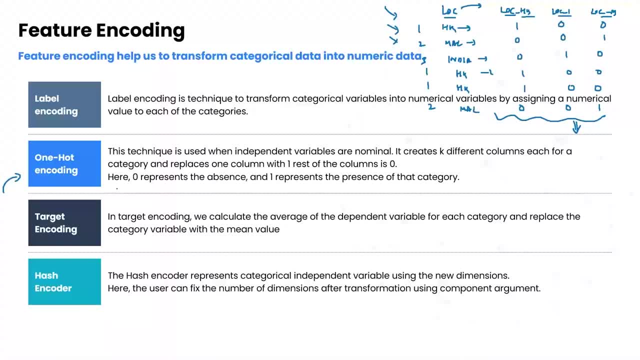 The technique is called as dummy encoding. As part of one hot encoding, The 3 features that we create Are otherwise called as dummy features And in this case we have created 3 dummy features, But you can see that dummy features are not called dummy features. You can see that there is no need of one of them. 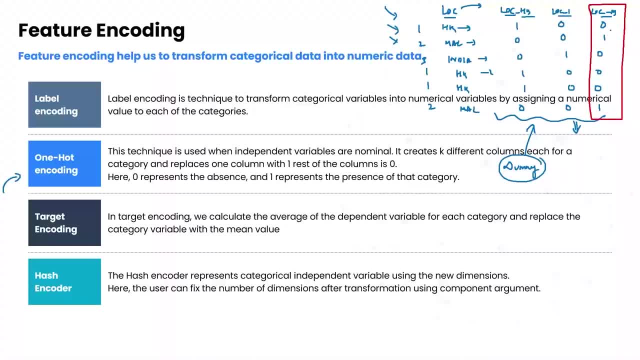 Imagine you don't have this column. Now, this column is a quite obvious column. Why? Because if this is 1, this is 0. Obviously it has to be 0. 0, 0, it has to be 1. 0, 1, it has to be 0. 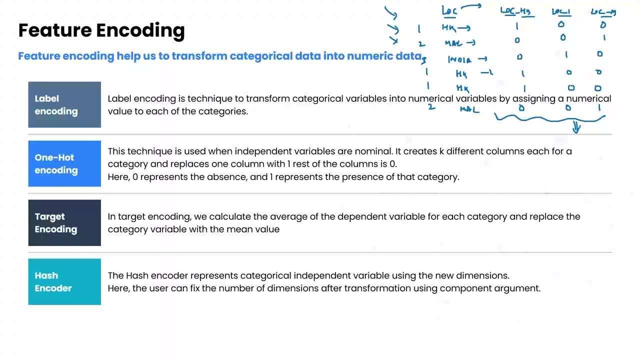 newly created features as part of the one hot encoding technique, and we all know that binary is the most accepted format for computers, right? so one hot encoding is one of the most preferred type of encoding technique. apart from one hot encoding, there is also another type of encoding. 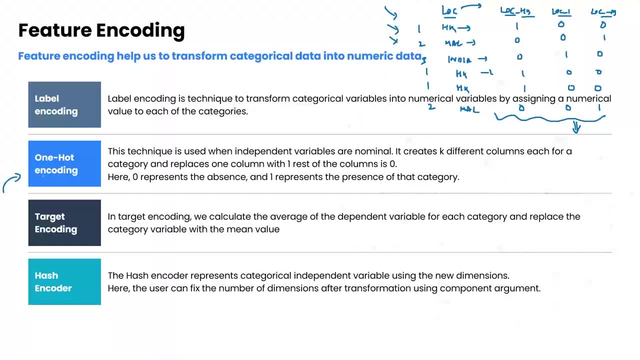 which is not mentioned here, which is a very similar technique to one hot encoding. the technique is called as dummy encoding as part of one hot encoding, the three features that we create are otherwise called as dummy features, and in this case we have created three dummy features, but you can see that 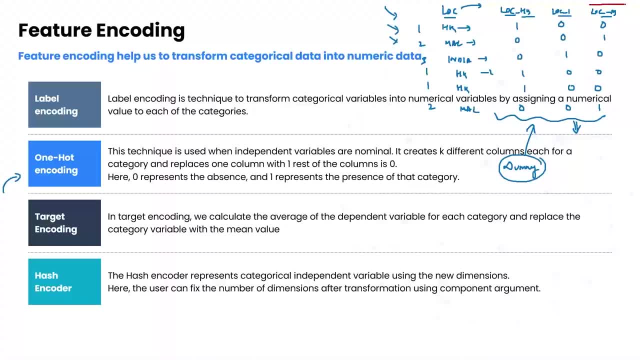 there is no need of one of them. imagine you don't have this column. now, this column is a quite obvious column. why? because if this is one, this is zero. obviously it has to be zero, zero, zero. it has to be one zero one. it has to be zero, zero, one, zero. it has to be. 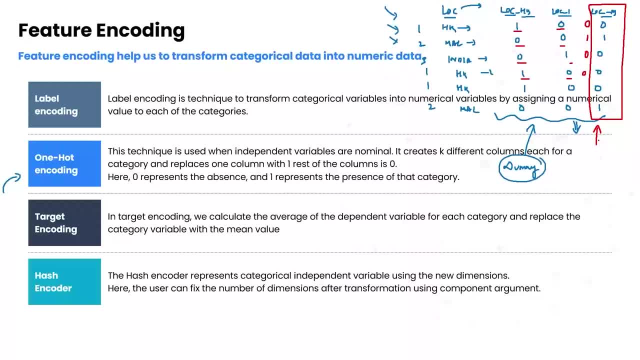 zero. so it's a quite obvious column to have. so in dummy encoding we get rid of one of these columns and we end up having two columns. this is called as dummy encoding. you can remove this column. you can remove this column, you can remove this column. any of these dummy features can be removed, but you just have to remove one of them. 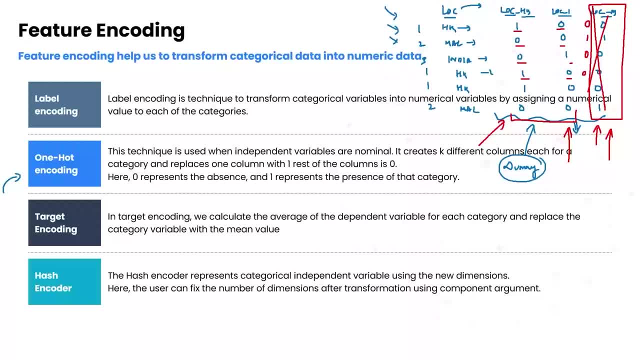 that's dummy encoding. another type of encoding is target encoding. what do you mean by target encoding? in target encoding we calculate the average of the dependent variable- that is, my y variable- for each category and replace the categorical variable with the mean value. it is another type of encoding technique. similarly, we also have hash encoder, which represents 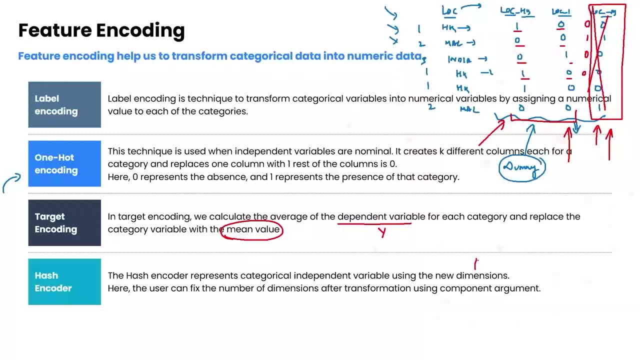 categorical independent variable using the new dimensions. inside hash encoder there is a concept called as n components, which basically means how much newly created columns you want, how many hashed columns you want to create. the user can fix the number of dimensions after transformation using component argument, which is n components if you define it as 8, which is a default. 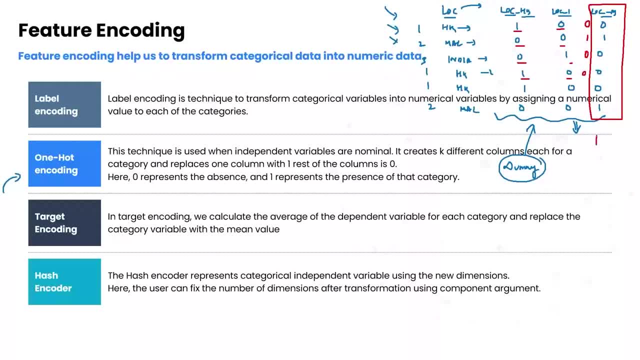 0, 1, 0. it has to be 0, So it's a quite obvious column to have. So in dummy encoding We get rid of one of these columns And we end up having 2 columns. This is called as dummy encoding. You can remove this column. 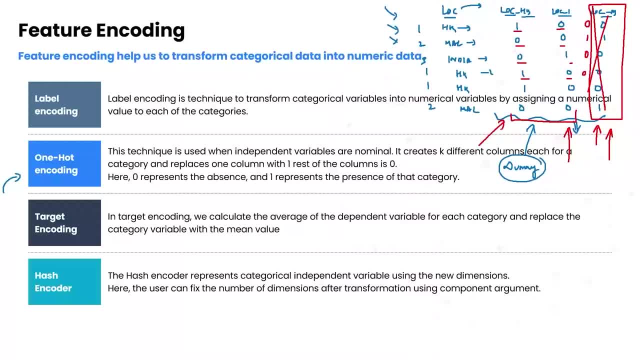 You can remove this column. You can remove this column. Any of these dummy features can be removed, But we just have to remove one of them. That's dummy encoding. Another type of encoding is Target encoding. What do you mean by target encoding? In target encoding, We calculate the average of the dependent variable. 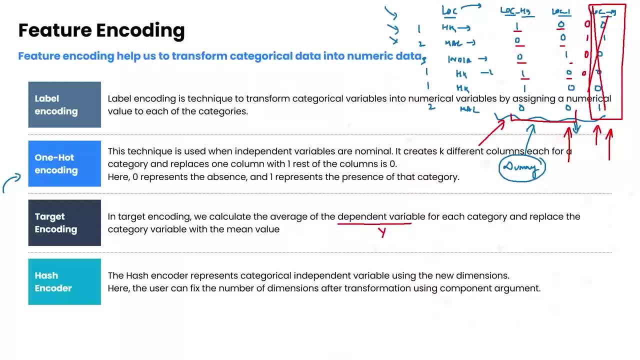 That is my y variable For each category And replace the categorical variable with the mean value. It is another type of encoding technique. Similarly we also have hash encoder, Which represents categorical independent variable Using the new dimensions. Inside hash encoder There is a concept called as n components, Which basically means: 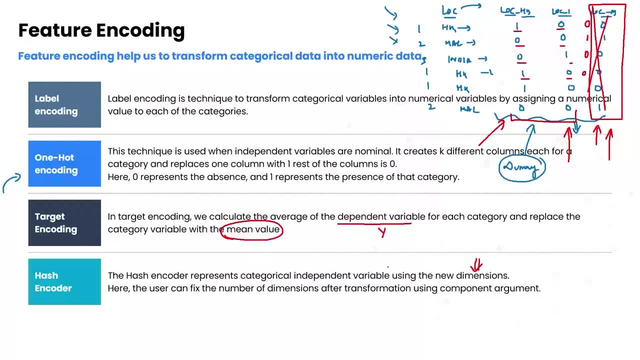 How much newly created columns you want, How many hashed columns you want to create. The user can fix the number of dimensions After transformation using component argument, Which is n components. If you define it as 8, Which is a default value, What happens is Irrespective of whichever column you pass. 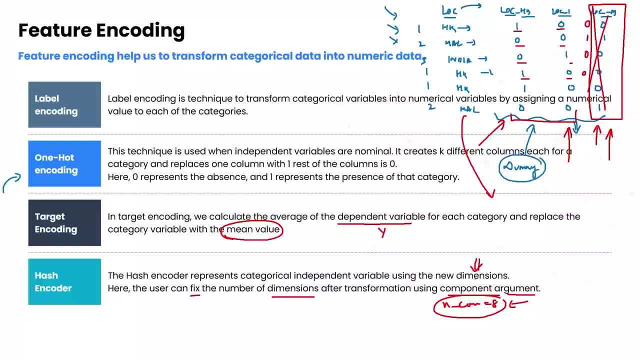 It could be location, It could be gender, It could be anything. Your hash encoder will create 8 new columns. The way it create values Is very difficult to understand Because they are hashed values, But majorly these are the 4 types, Or 5 types of encoding techniques. 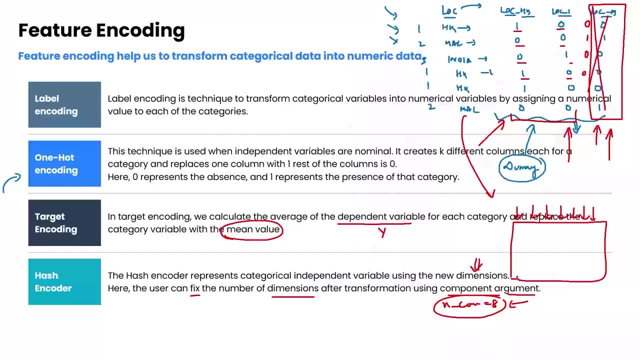 That we discussed. There could be multiple other techniques as well, Which includes binary encoder And various other encoding techniques That we usually don't use. But if you ask me What is the most important one, I would say label encoding, Which is used for your y variables, And one hot encoding. 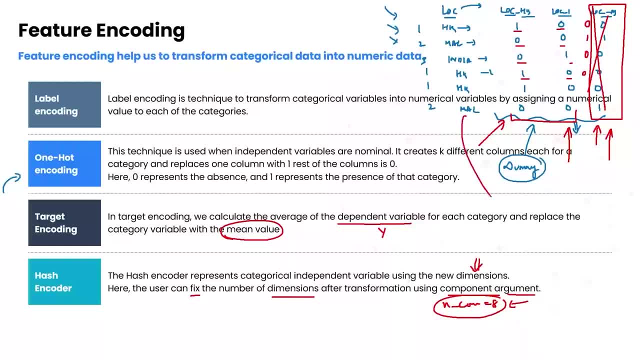 value. what happens is, irrespective of whichever column you pass- it could be location, it could be gender, it could be anything- your hash encoder will create eight new columns. the way it create values is very difficult to understand, because they are hashed values, but majorly, these are the four types. 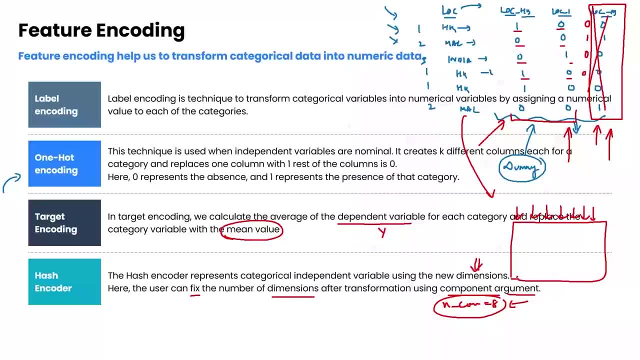 or five types of encoding techniques that we discussed. there could be multiple other techniques as well, which includes binary encoder and various other encoding techniques that we usually don't use, but if you ask me what is the most important one, i would say label encoding, which is used for 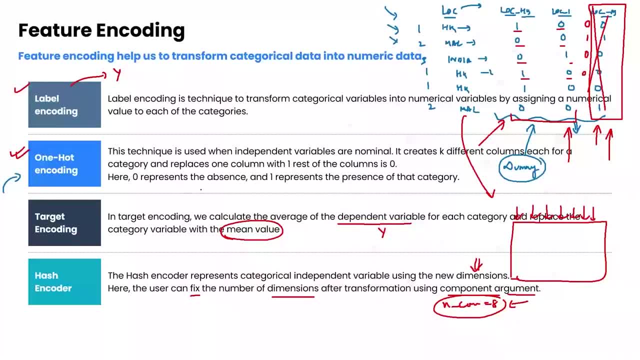 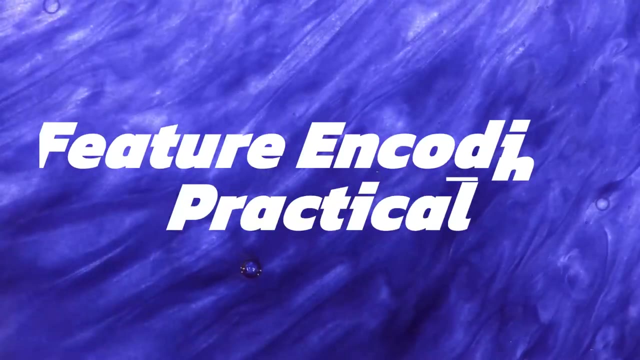 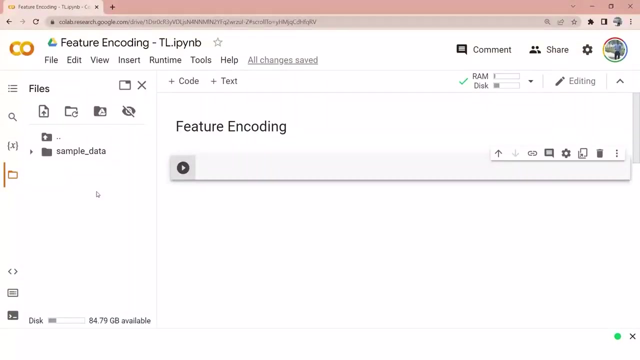 your y variables and one. hot encoding, or dummy encoding, is one of those encoding techniques that we mostly use. so that's all about this particular session on feature encoding. in the next video we shall be talking about the practicals part, on how do we implement these kind of techniques using a sample data set. it's time to jump into the feature. 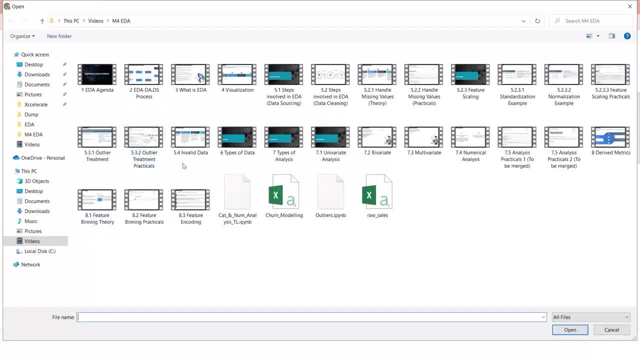 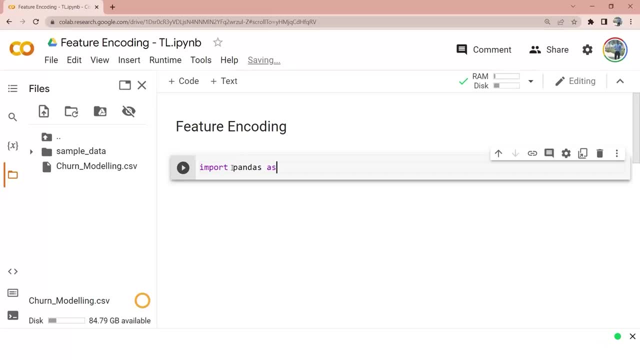 encoding part, the practicals. first of all, i'll upload my data set, which is the same churn modeling data set. in the meanwhile, i'll start writing down my import statements: pandas as pd, import, numpy as num, mp import matplot, libpyplot as plt. and we also need 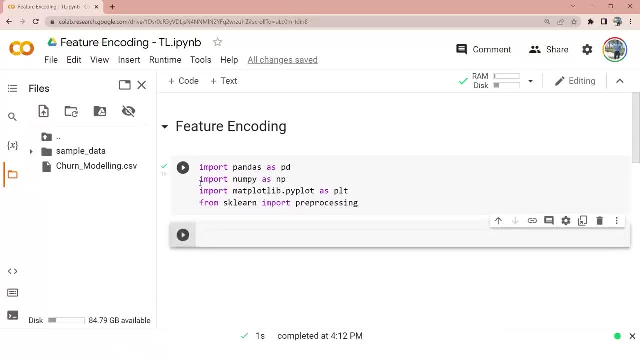 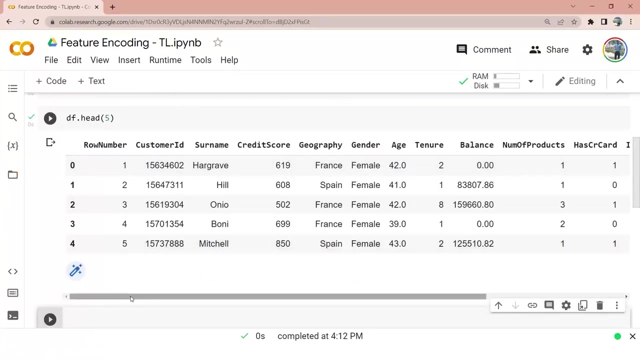 pre-processing from the sklearn. again, we'll read the file using the same technique: pdread, csv, copy path, paste it dfhead. and that's how my data set looks like. let me close it for a better visibility. that's how my data set looks like. i think you all are familiar with the data set, so i'll just quickly do. 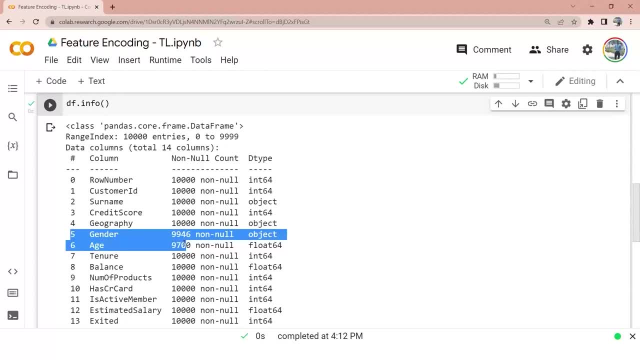 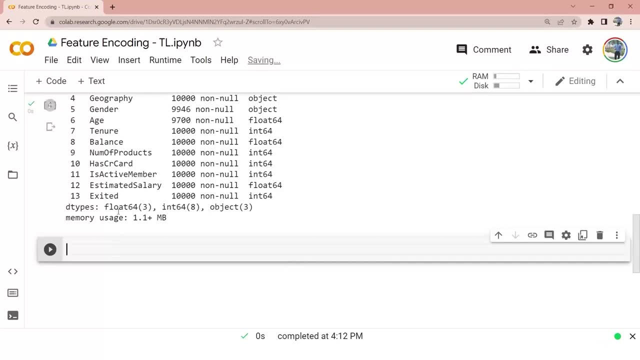 so i don't know what it looks like. this is theanking information. this is the thing that makes a cared not important, because at the end of the data set is related to something big. so it's really like a simple protocol. where i just come, the counter is table name, first row, number iさ, Autumn. i'm not trying to show you how much. 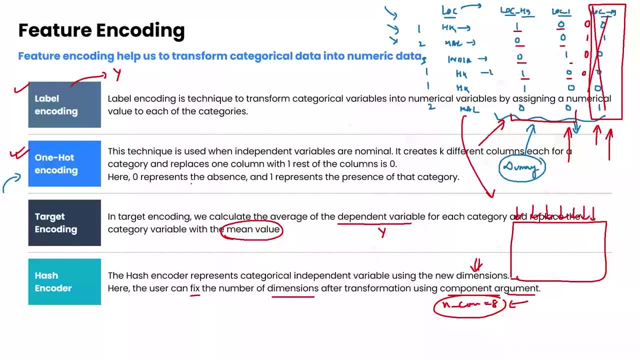 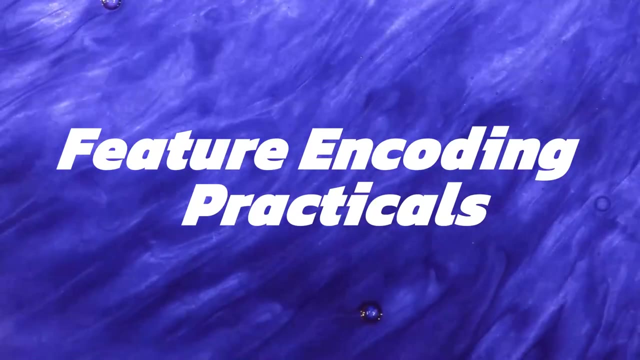 Or dummy encoding, Is one of those encoding techniques That we mostly use. So that's all about this particular session On feature encoding. In the next video We shall be talking about the practicals part, On how do we implement these kind of techniques Using a sample dataset. It's time to jump into the feature encoding part. 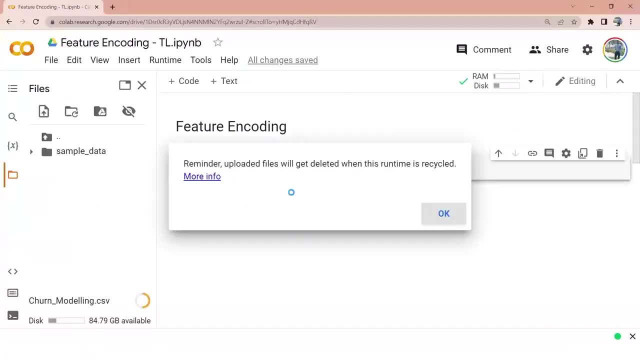 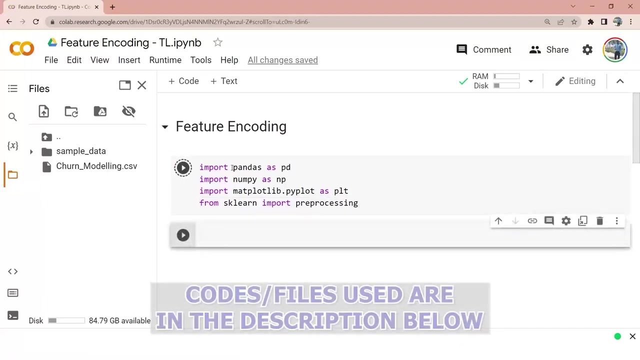 The practicals. First of all, I'll upload my dataset, Which is the same churn modeling dataset. In the meanwhile, I'll start writing down my import statements: Pandas as pd, Import numpy as mp, Import matplot, libpyplot as plt. And we also need Reprocessing from the sklearn. 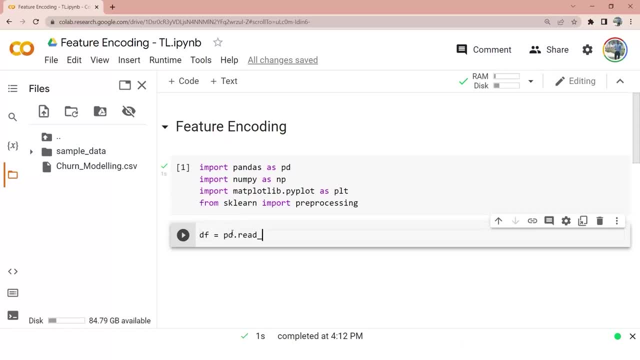 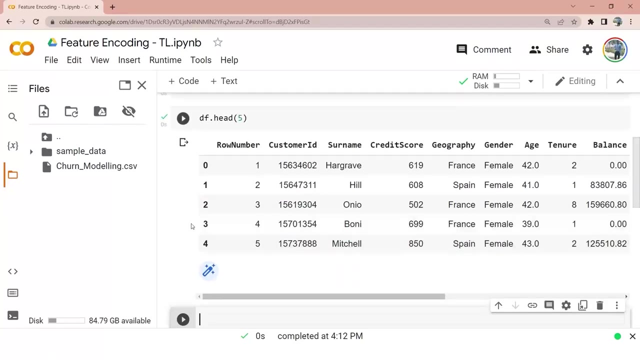 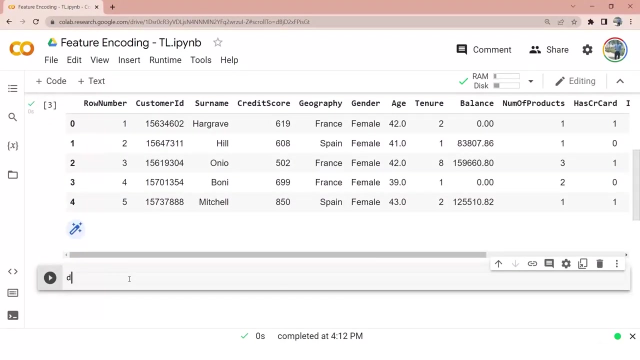 Again. we'll read the file using the same technique: pdreadcsv- Copy path, Paste it dfhead. And that's how my dataset looks like. Let me close it For a better visibility. That's how my dataset looks like. I think you all are familiar with the dataset. 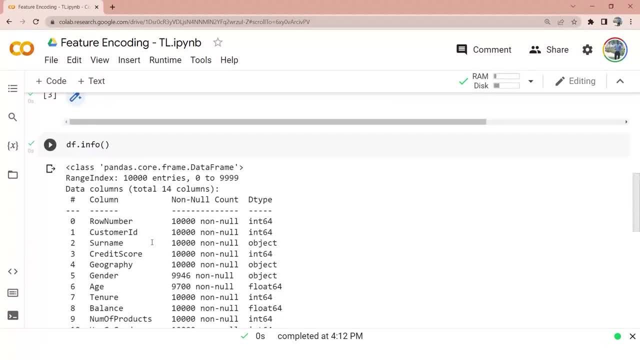 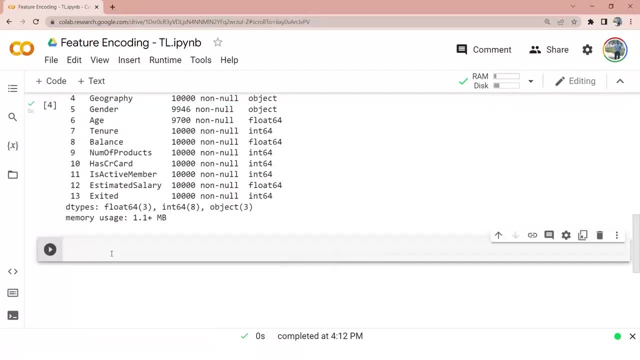 So I'll just quickly do. the information info Is giving me the data set Giving me an information that Gender and age are having null values. So we'll perform the same drop steps Where we will be dropping off the columns that we don't need, Which is row number. 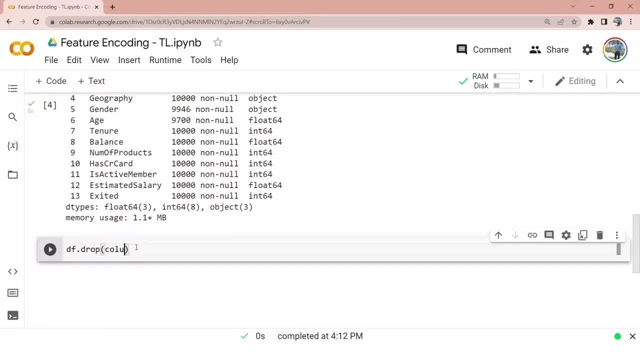 Customer id and surname. So I'll do dfdrop Columns equals to Customer id, Row number, Surname, That's it. And then Axis equals to one And Place equals to true Row number. I believe And is capital And done. And if I have a look at the dataset, 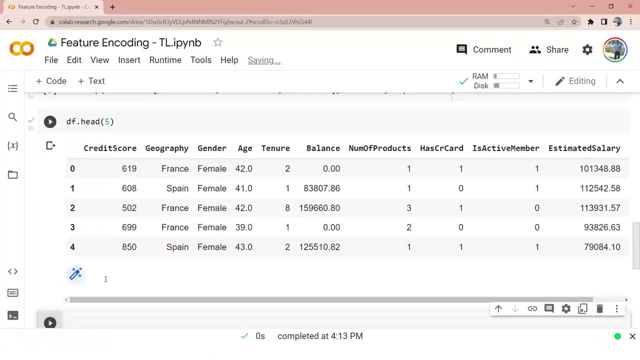 That's how my data looks like, Right? So let's say we will pick one of these columns for performing the encoding steps. Let's say we will be doing, We'll pick any of them: geography or gender. We can pick gender. Now, gender has null values. How many null values does gender have? 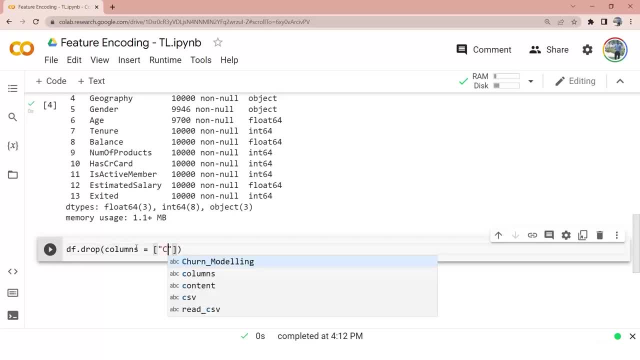 it is worth, but data set uses that for project functions. this includes the attach again. i'll show you in a second, but check it out later. be, there is a disc, them söyles not. and then axis equals to one and in place equals to true row number. i believe and is capital, and 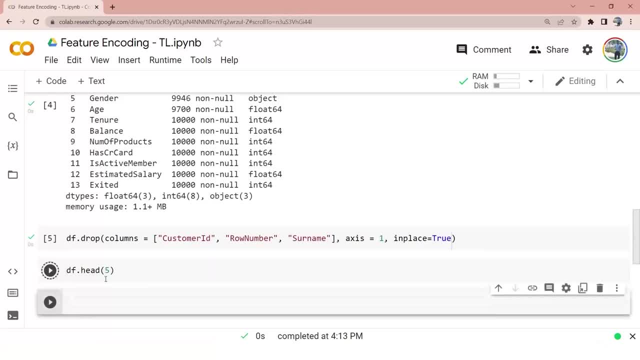 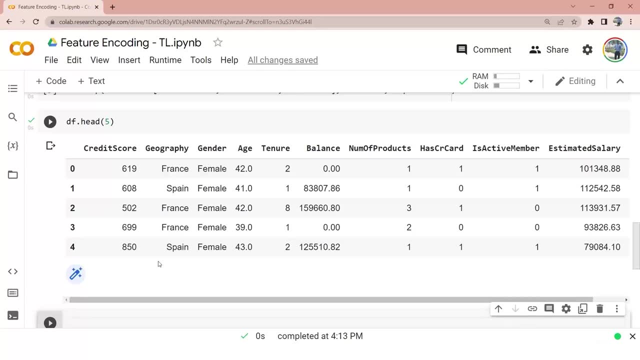 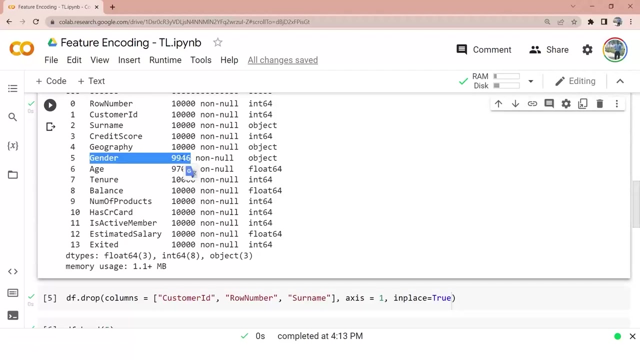 done and if i have a look at the data set, that's how my data looks like, right? so let's say we will pick one of these columns for performing the encoding steps. let's say we will be doing, we'll pick any of them: geography or gender. we can pick gender. now. gender has null values. how many null? 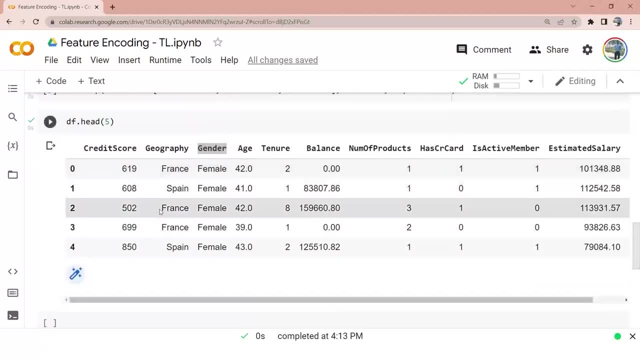 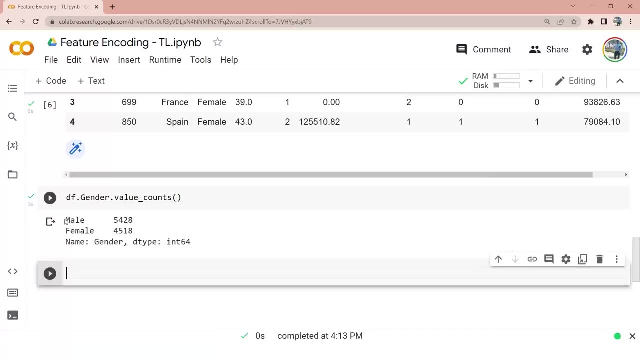 values does gender have 54 null values. so if you simply do df dot gender dot value counts, you will not be able to see the null value because df dot column dot value counts only gives the value counts for the data points that you already have for null values. it will not show you right, but 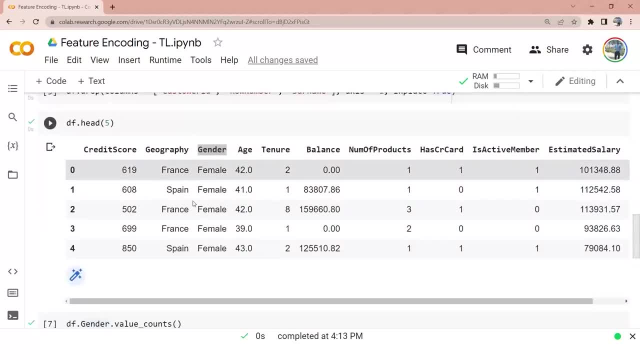 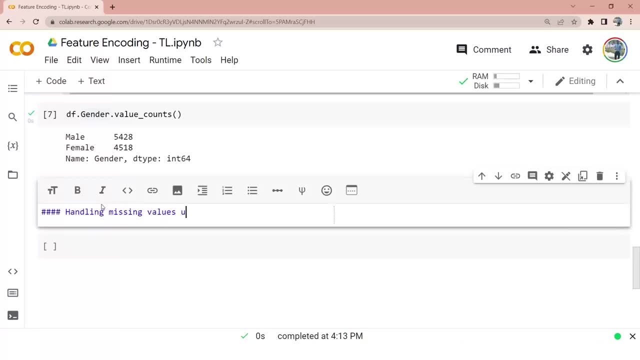 here you can see there are 54 null values. so what we will do is we'll try to handle the null values first, handling missing values in gender. so what we will do is we'll try to find the mode, and we all know the mode is male: df, dot, gender, dot mode. what is the mode? the mode is male, so what i will do is df. 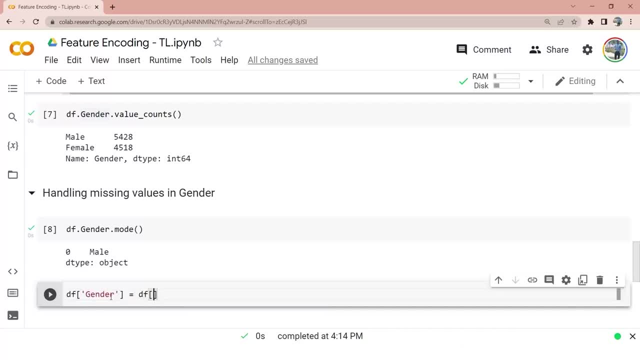 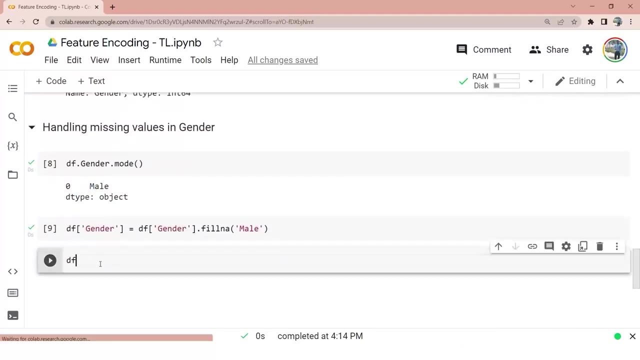 of gender equals to df of gender of gender dot fill na. i'm going to fill the null values with the mode: sorry, male done now. if i do, the value counts. you will see that the male count has to be increased. it has increased by the 54. 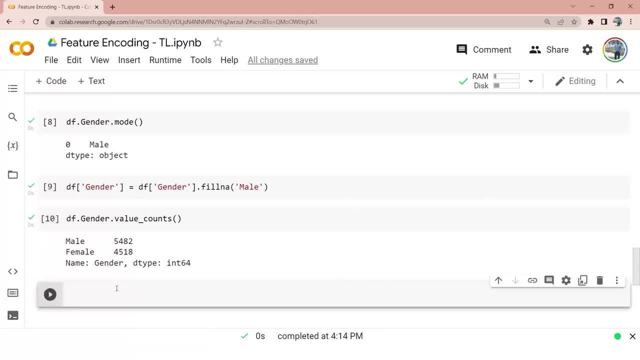 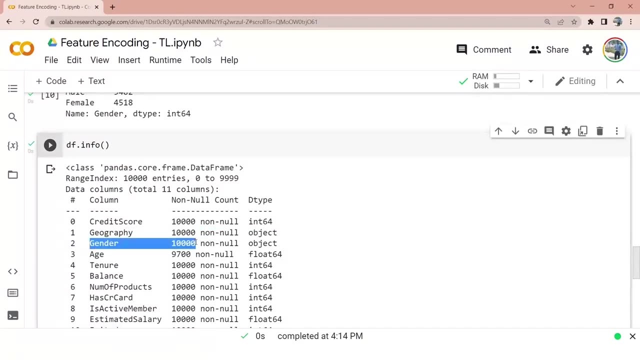 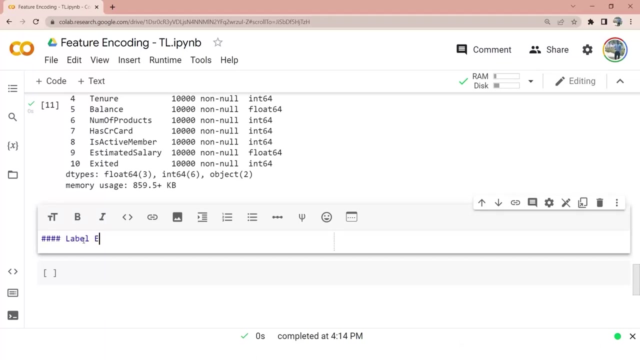 values and we'll give a quick check on the information one. you can see there is no null values for gender. all are not null value. so we'll quickly get started with the encoding techniques. so first one will be label encoding, and we all know label encoding is simply one of those. 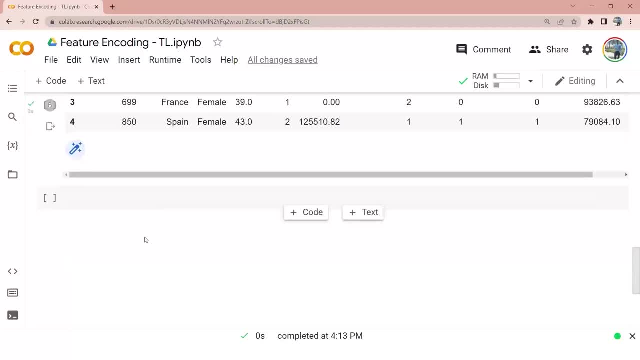 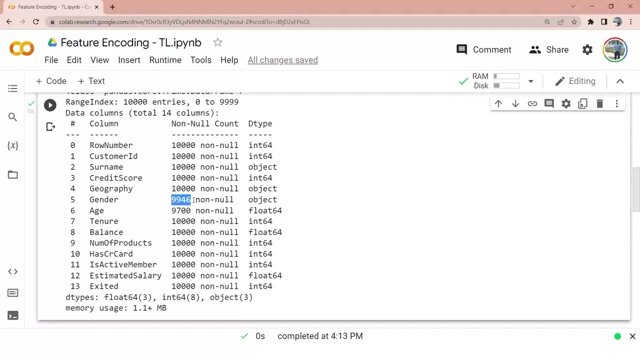 Fifty-four null values. So if you simply do dfgendervalueCounts, You will not be able to see the null values, Because dfcolumnvalueCounts only gives the value counts for the data points that you already have For null values. it will not show you Right, But here you can see there are fifty-four null values. 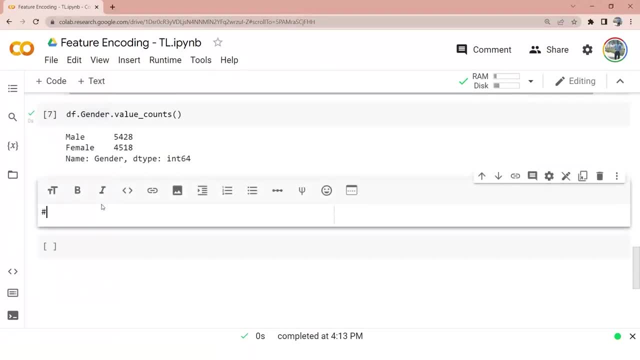 So what we will do is we'll try to handle the null values first, Okay, handling missing values in gender. so what we will do is we'll try to find the mode, and we all know the mode is male: df, dot, gender, dot, mode. what is the mode? the mode is male. so what i will do is: 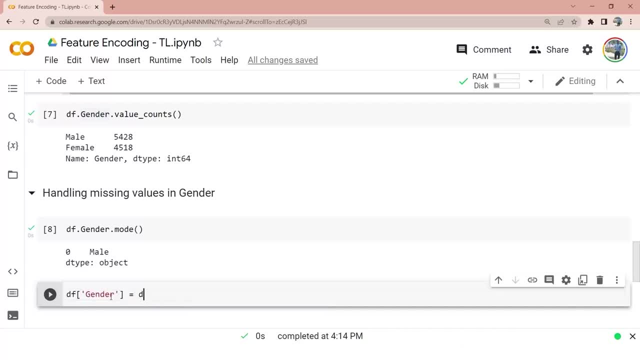 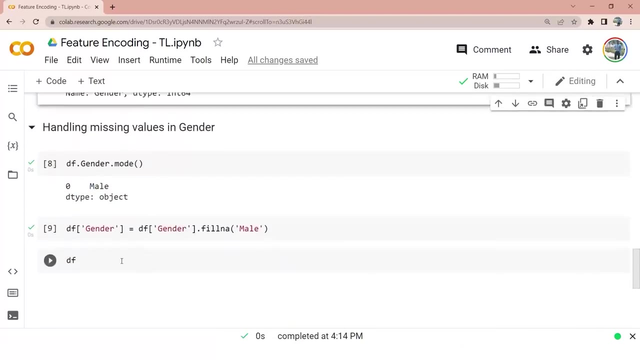 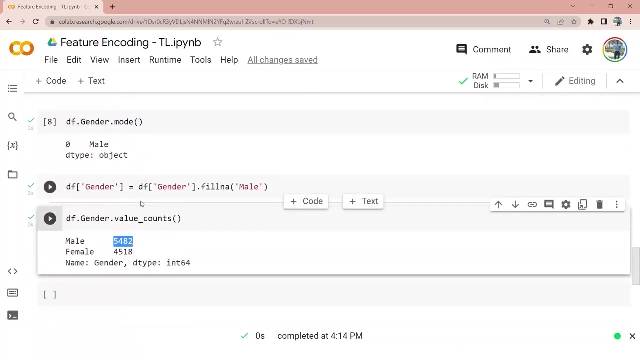 df of gender equals to df of gender dot fill na. i'm going to fill the null values with the mode: sorry, male done now. if i do, the value counts. you will see that the male count has to be increased. it has increased by the 54 values. 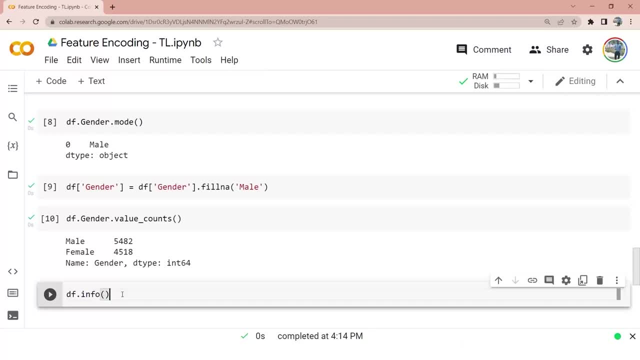 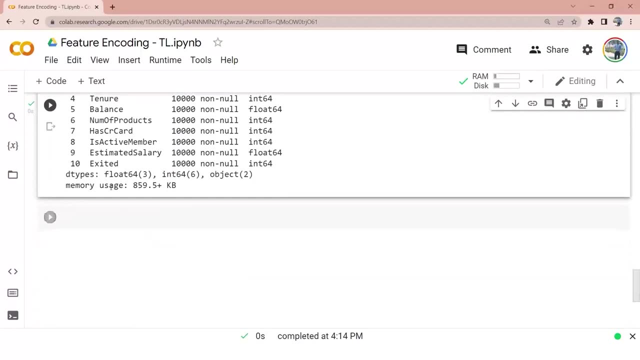 and we'll give a quick check on the information one. you can see there is no null values for gender. all are not null value. so we'll quickly get started with the encoding techniques. so first one will be label encoding, and we all know label encoding is simply one of those. 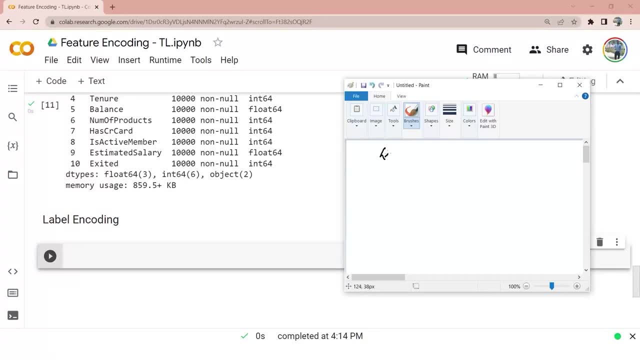 encoding techniques where we, let's say, we have gender- male, female, male, female and so on- it will simply give them some number, give one zero one. so wherever it sees male, it will give zero, female as one, or vice versa. and if you have more values, that's fine, it will give you a number here. so let's see, let's see that in russia, india, korea. 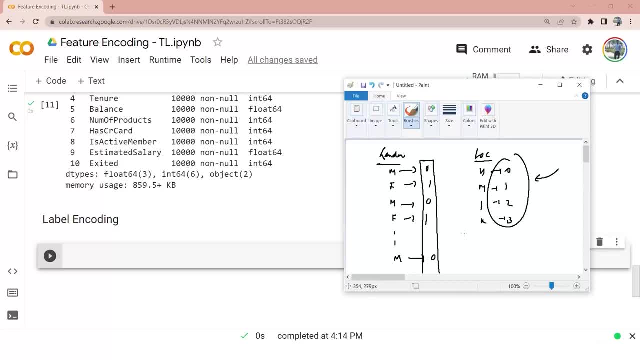 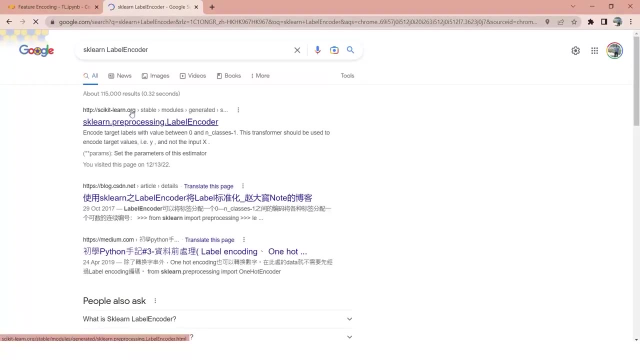 similarly: 0, 1, 2, 3. arbitrarily it will give you some numbers, which is not recommended, but let's see how to be performed. so we'll be using the pre-processing dot label encoder. if you want to have a look at it, simply just search sklearn label encoder and you will be able to get. 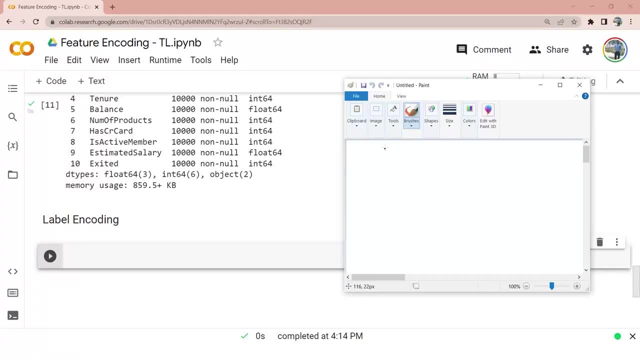 encoding techniques where we, let's say, we have gender- male, female, male, female and so on- it will simply give them some number, give one zero one. so wherever it sees male, it will give zero, female as one, or vice versa. and if you have more values, let's say 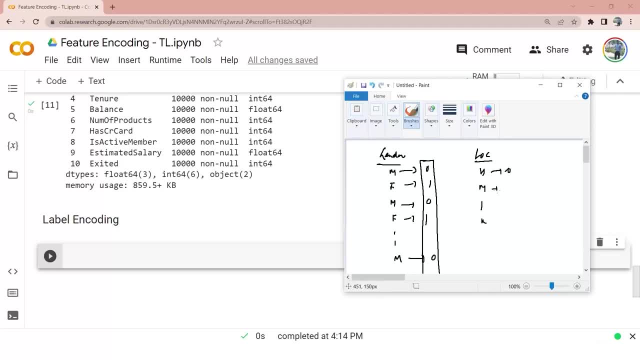 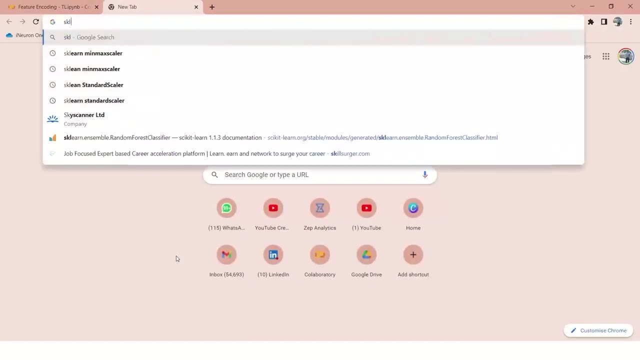 hong kong, malaysia, india, korea. similarly, zero, one, two, three, arbitrarily. it will give you some numbers, which is not recommended, but let's see how to be performed. so we'll be using the pre-processing dot label encoder. if you want to have a look at it, simply just search sk. learn label encoder and. 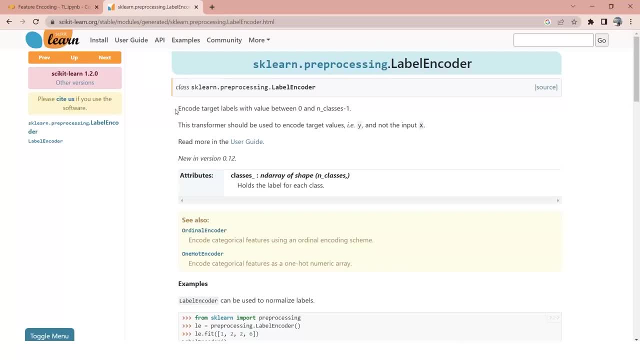 you get sk learn, dot pre-processing, dot label encoder, encode target variables. you can see, this particular technique is only used for target variables, which is your y variable, which is your exited column. but in this case we are taking examples from the x variables and i already explained you that it is not recommended for x variables, just for the sake of showing. 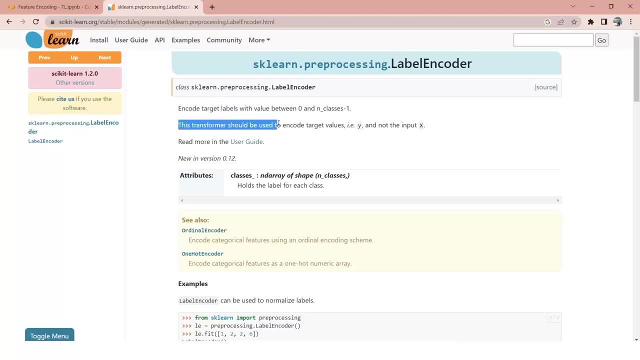 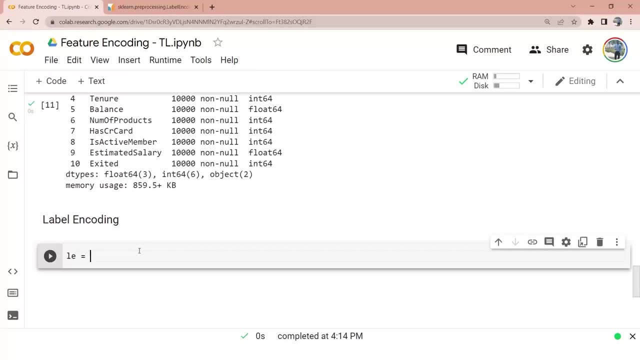 it. i am just showing it. this transformer should be used to encode target variables. that is y and not the input x. so let's try to see. let's say i will define my label encoder as le pre-processing dot label encoder and then i will create gender. let's say i will create a new column: gender. 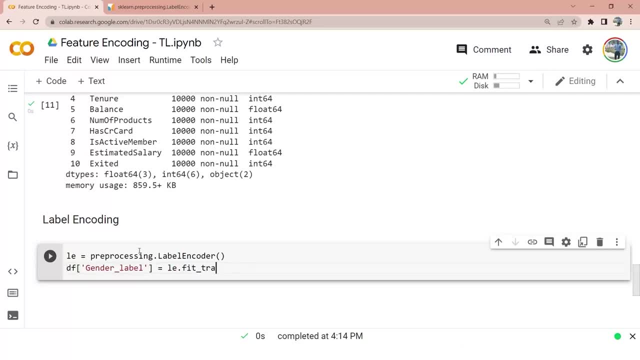 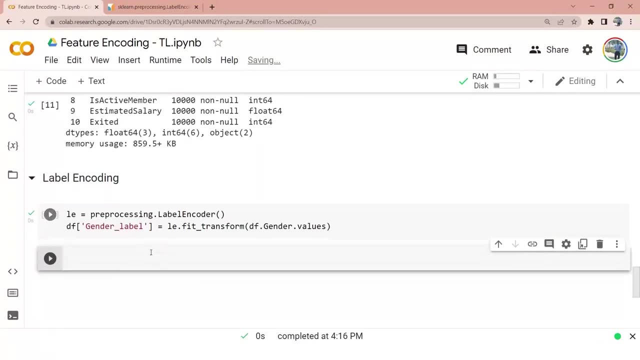 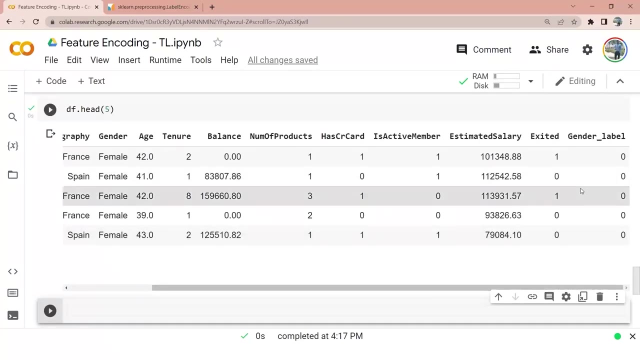 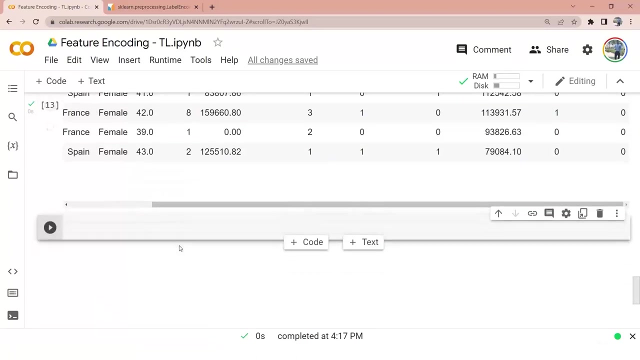 underscore label is equals to le dot fit transform. and here i will pass df dot gender dot values. the moment i run this df dot head, you can see there is a new column that is gender label. so wherever you see female, they have given zero and for male it will be one. if you want to cross check, you can cross check it. 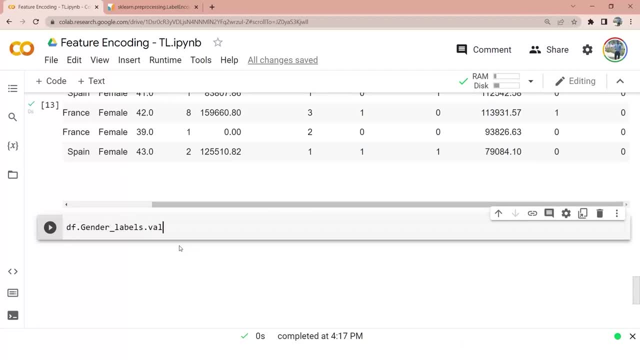 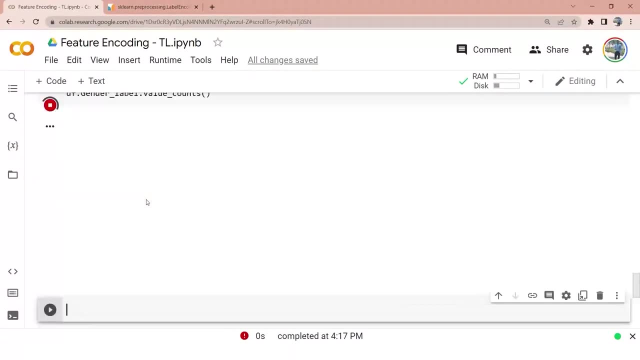 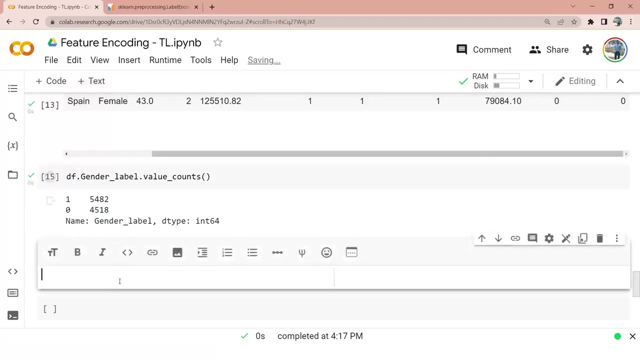 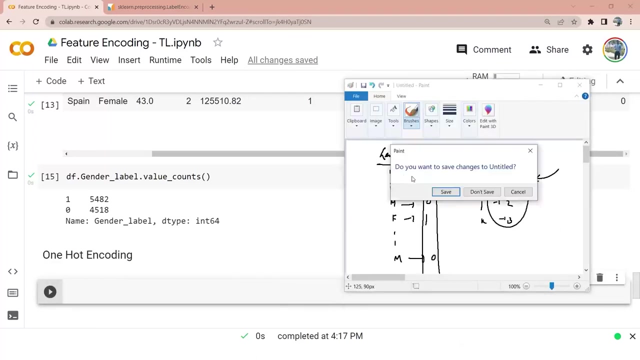 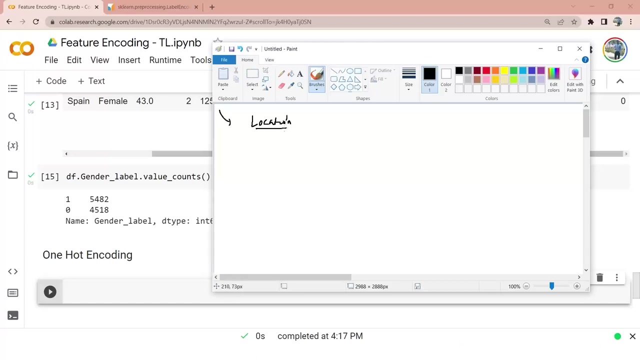 by doing df, dot, gender underscore labels, dot value count labels, label value counts. you can see male and female. so the next technique is going to be one hot encoding technique. how do we perform one hot encoding technique? let's say i have a data set. let's say i am talking about one of these columns called as: 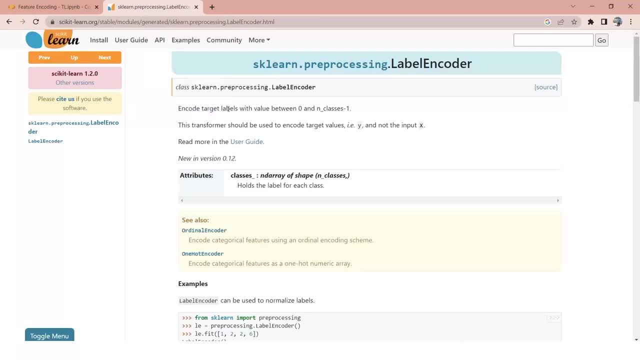 sklearnpreprocessinglevelencoder encode target variables. you can see, this particular technique and it will give us technique is only used for target variables, which is your y variable, which is your exited column, but in this case we are taking examples from the x variables and i already explained you that it. 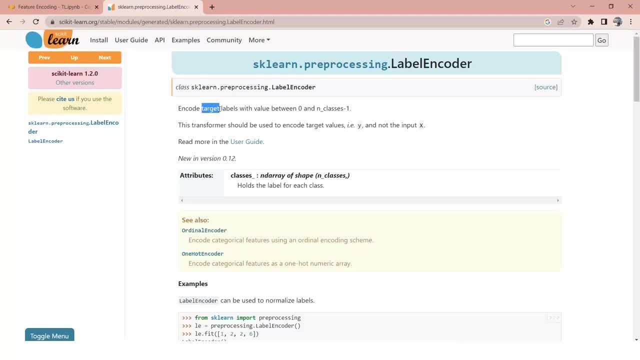 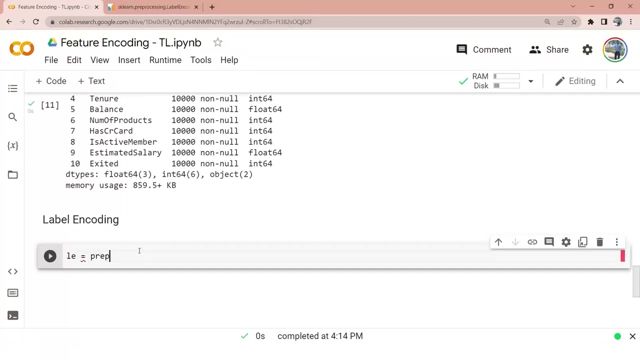 is not recommended for x variables. just for the sake of showing it, i am just showing it. this transformer should be used to encode target variables, that is, y and not the input x. so let's try to see. let's say, i will define my label encoder as le pre-processing dot label encoder. 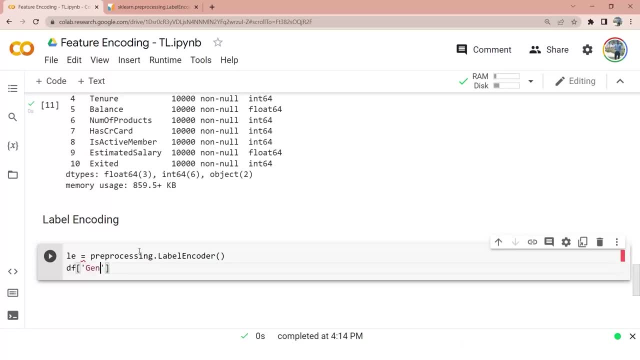 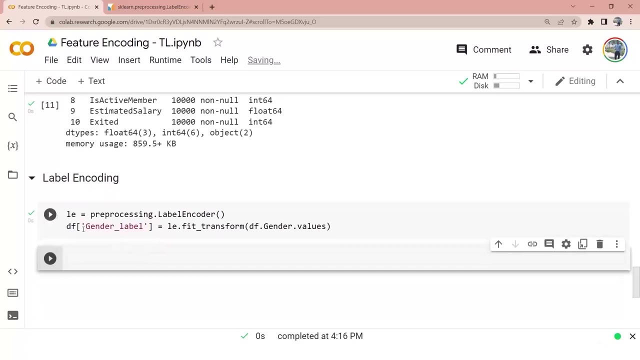 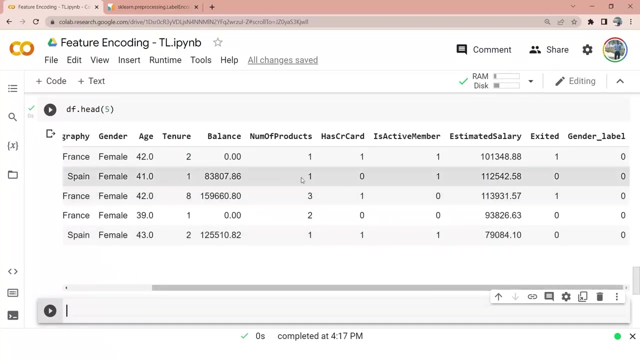 and then i will create gender. let's say i will create a new column. gender underscore label is equals to le dot fit transform and here i will pass df dot- gender dot- values. the moment i run this df dot head you can see there is a new column that is gender label. so wherever you see female, they have given zero and for male it. 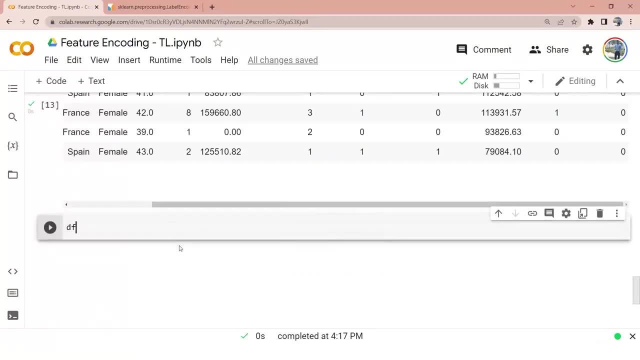 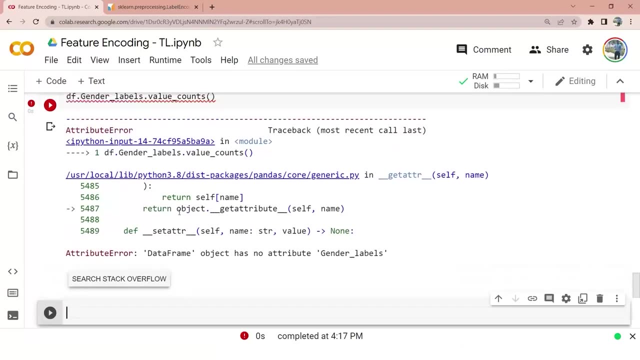 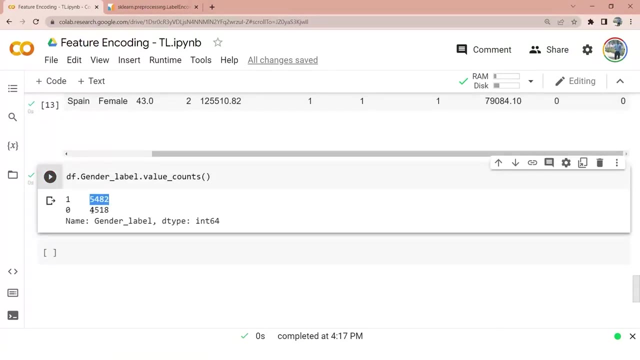 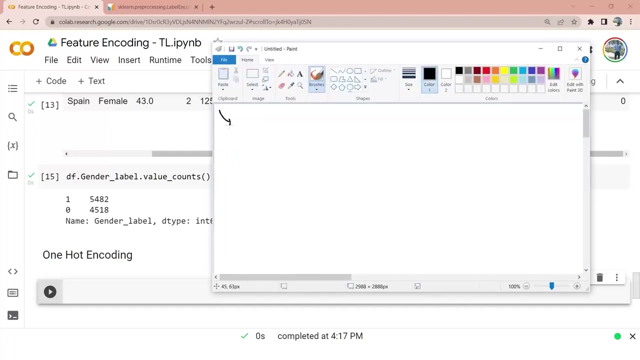 will be one. if you want to cross check, you can cross check it by doing df dot, gender underscore labels. dot value count labels- label value counts. you can see male and female. so the next technique is going to be one: one hot encoding technique. how do we perform one hot encoding technique? let's say i have a data set. 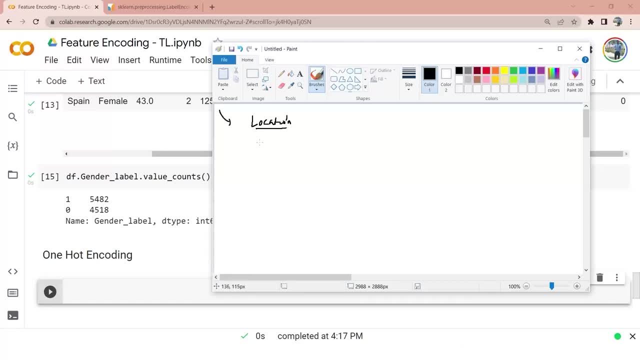 let's say, i am talking about one of these columns called as location, so i have spain. some customers are staying in spain, germany, france, spain, germany, germany, germany, france, something like that. so what happens is you have to create three new columns here, as there are three. 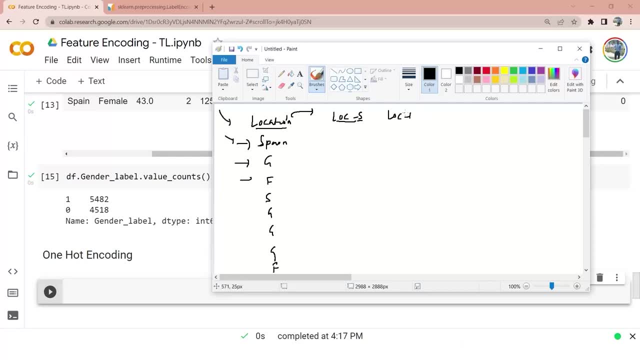 valid value: spain, germany and france. so location underscore spain, location underscore g, location underscore france. so wherever you see, spain, this becomes one. others are zero. germany, this becomes one. this is zero. france, others are zero. this becomes one. one zero, zero, zero. one, zero, zero one. 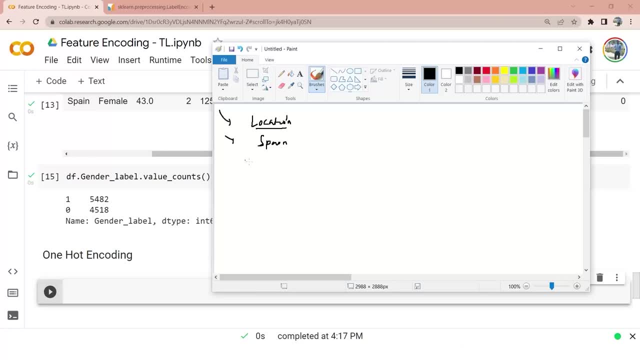 location. so i have spain. some customers are staying in spain, germany, france, spain, germany, germany, germany, france, something like that. so what happens is you have to create three new columns here, as there are three valid values: spain, germany and france. so location underscore spain. location underscore g. location underscore france. 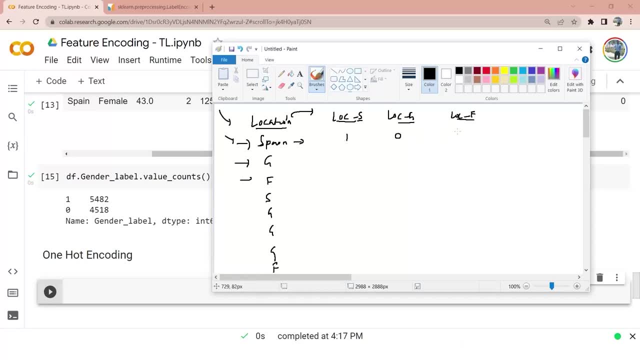 so, wherever you see, spain, this becomes one. others are zero. germany, this becomes one. this is zero. france, others are zero, this becomes one: 1 0 0 0, 1 0 0, 1 0, 0, 1 0 and 0 0, 1, and you can see the. 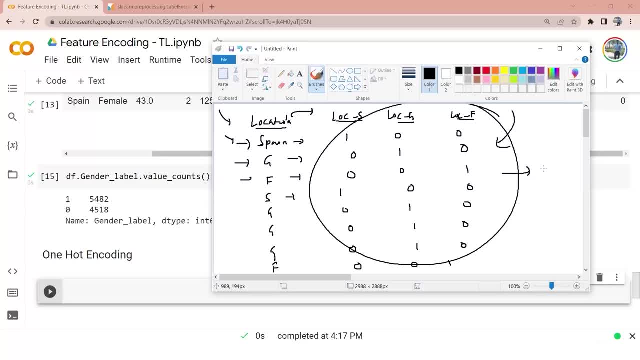 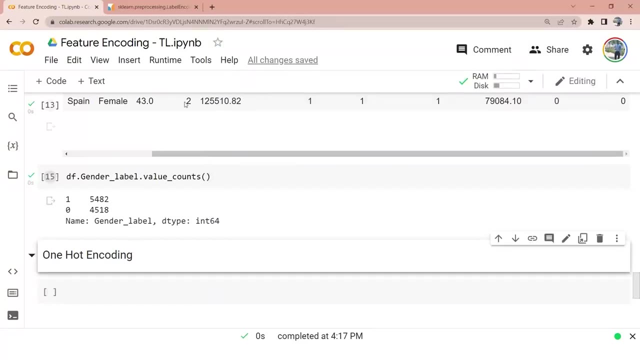 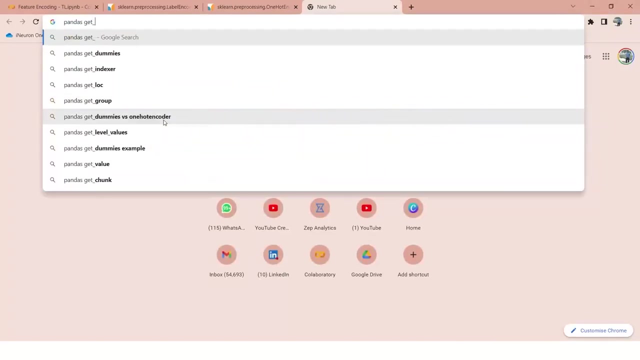 newly created features are in the form of numerical values and are in the most accepted format, which is the byte format. so how do we perform one hot encoding? there are multiple ways to perform one encoding. one of them is to simply use the sklearn. one hot encoder, or else pandas get dummies. this is also a similar. 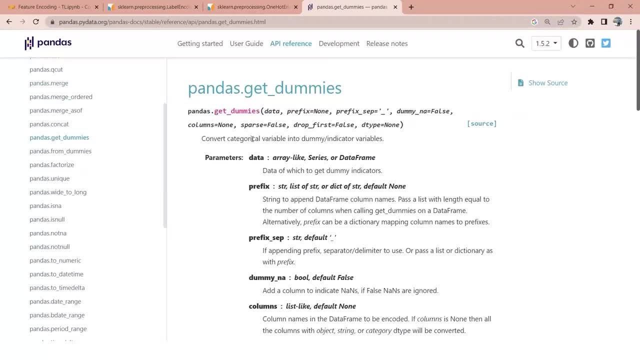 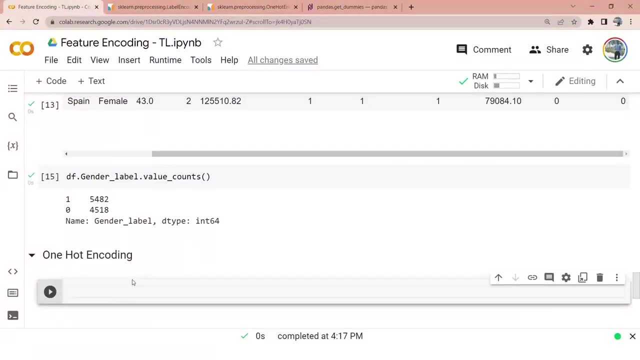 technique- pandas get dummies also is nothing but a technique to convert it into one hot encodings. so we will be using the simplest one, which is get dummies. so i will note it as one hot equals to pd dot get dummies. let's say i will perform it on. 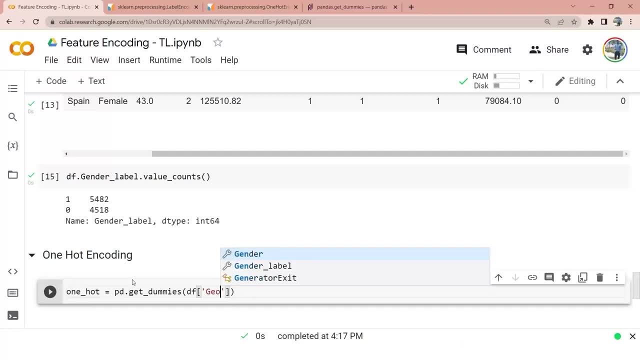 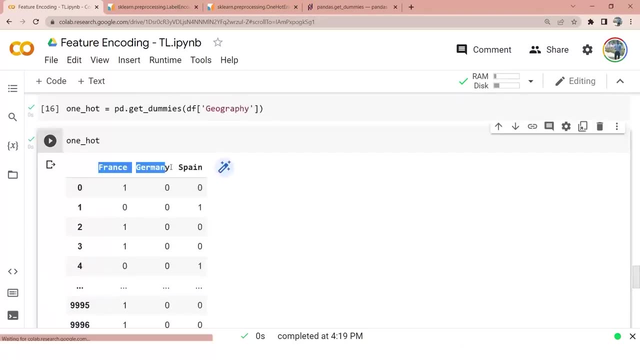 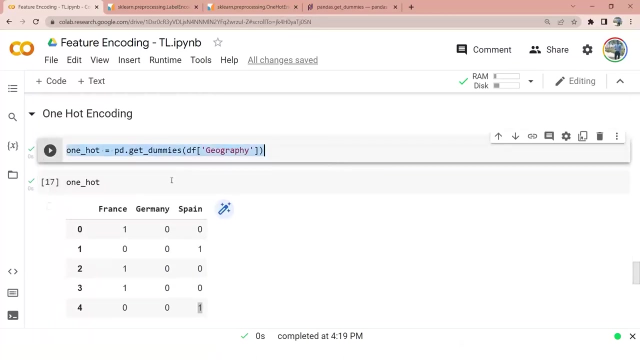 gender, or else let's say, let's do it on geography and you want to visualize or see your one? hot, you can see three new columns has been created. wherever you see france, it is one. wherever you see germany, that will be one. wherever you see spain, that will be one, right in order to perform this task on the entire data set. 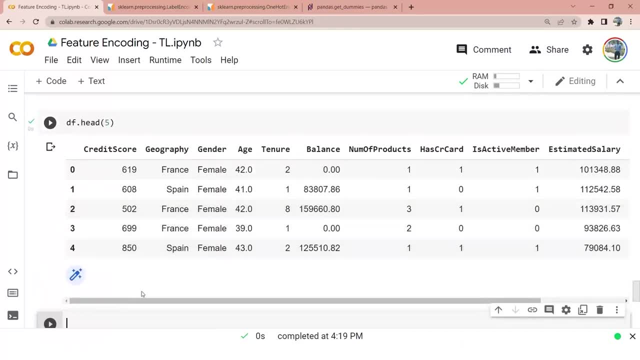 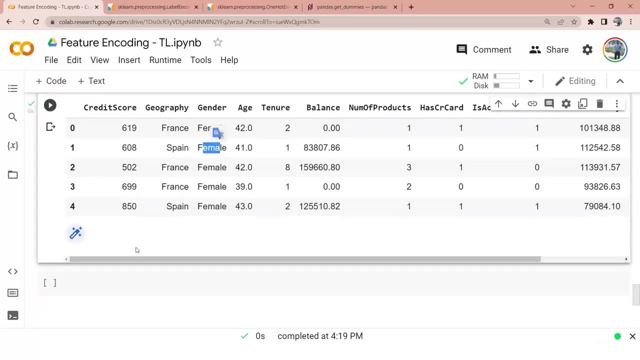 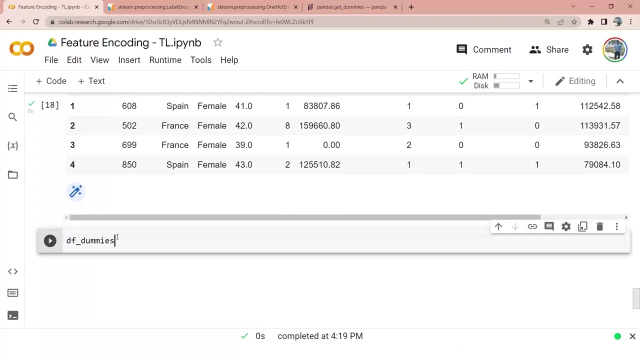 have a look at the data set. your data looks like this. if you look at it closely, only two columns are having categorical values. let's say i want to convert both of them into one hot encodings. so simply, what we can do is df dummies. i will perform. 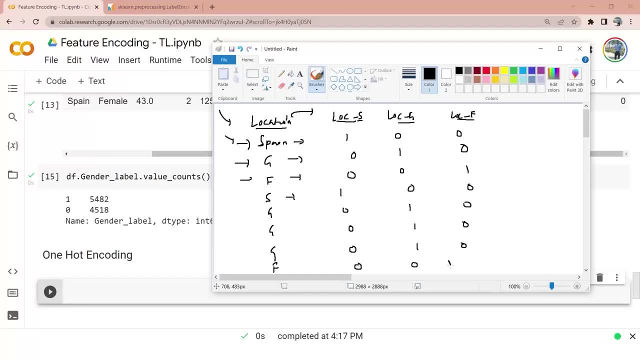 zero, zero one zero and zero zero one, and you can see the newly created features are in the form of numerical values and are in the most accepted format, which is the byte format. so how do we perform one hot encoding? there are multiple ways to perform one hot encoding. 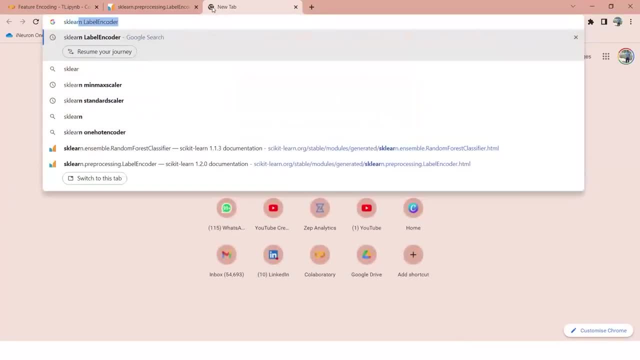 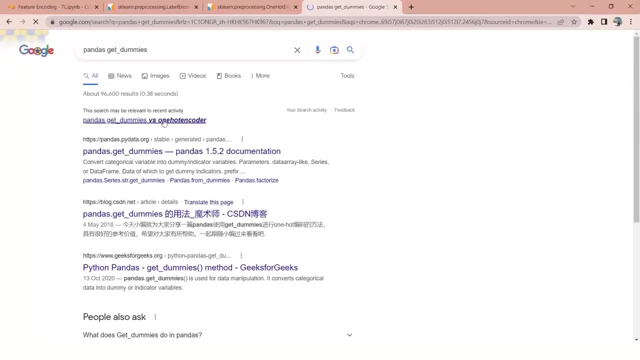 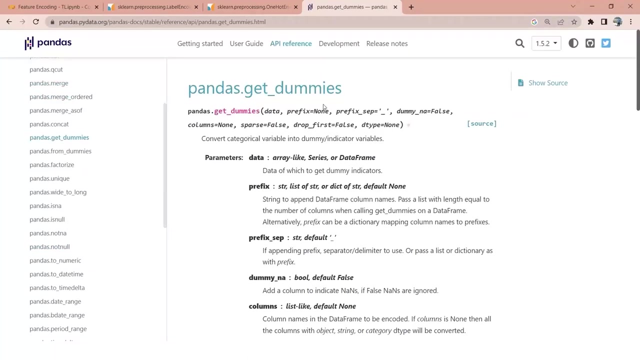 one of them is to simply use the sklearn one hot encoder, or else pandas get dummies. this is also a similar technique. pandas get dummies also is nothing but a technique to convert it into one hot encodings. so we will be using the simplest one, which is: 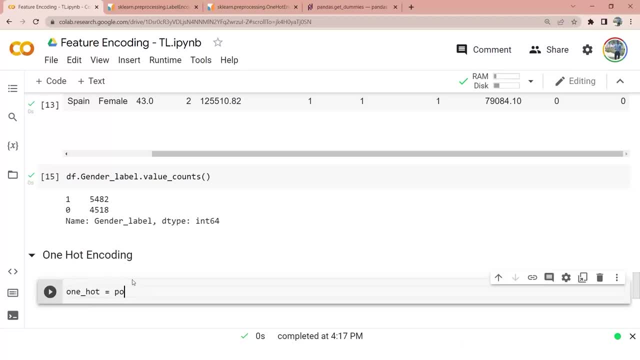 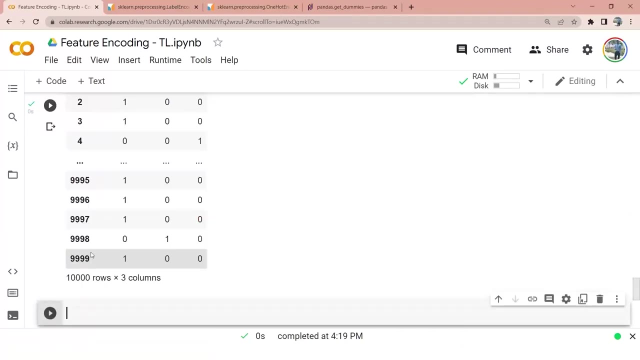 get dummies. so i will note it as one hot equals to pd dot. get dummies. let's say i will perform it on gender. or else let's say let's do it on geography and you want to visualize or see your one onehot, you can see three new columns has been created. wherever you see france, it is one. 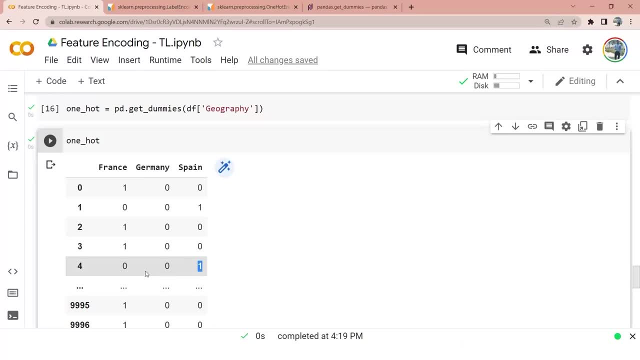 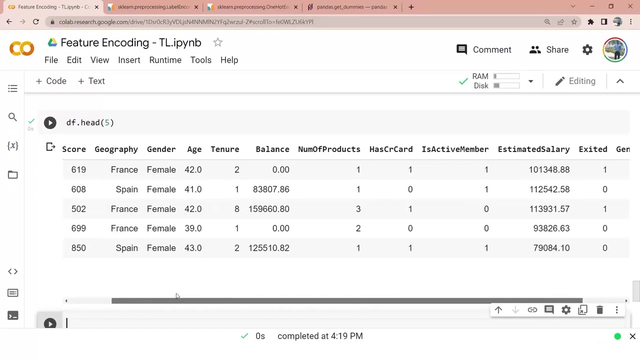 wherever you see germany, that will be one. wherever you see spain, that will be one. right, in order to perform this task on the entire data set, have a look at the data set. your data looks like this: if you look at it closely, only two columns are having categorical values. let's say i want to. 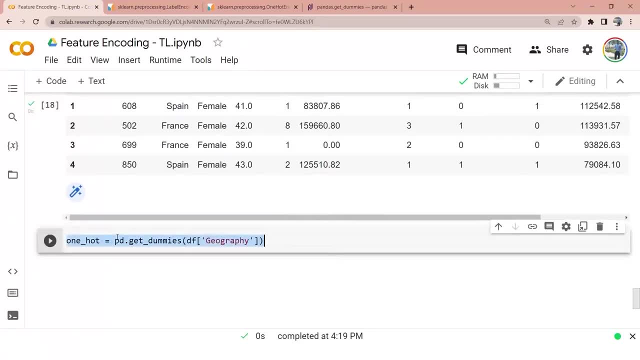 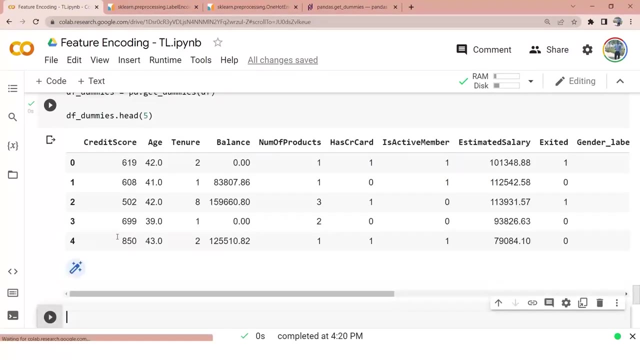 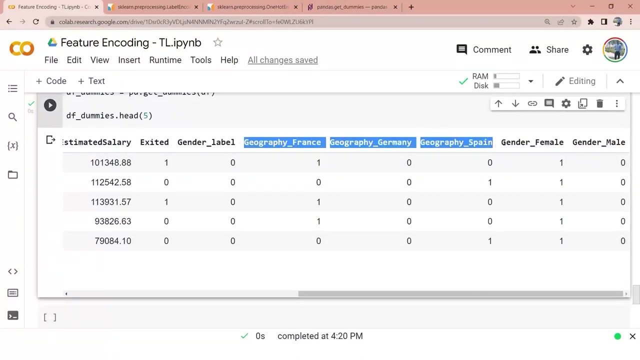 both of them into one hot encodings. so simply, what we can do is df dummies. i will perform it on pd dot. get dummies on df. in the same line, i will do df underscore dummies dot head. now you can see. so dummy variables are created for geography. three variables are created for. 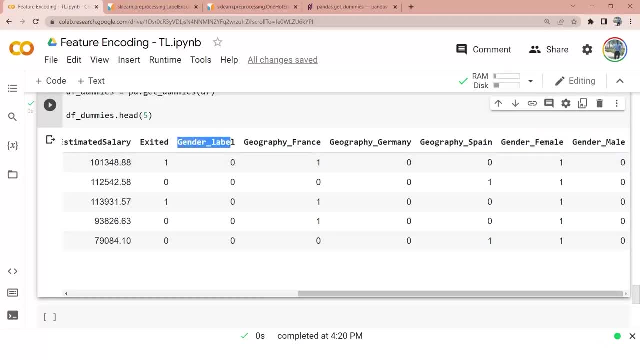 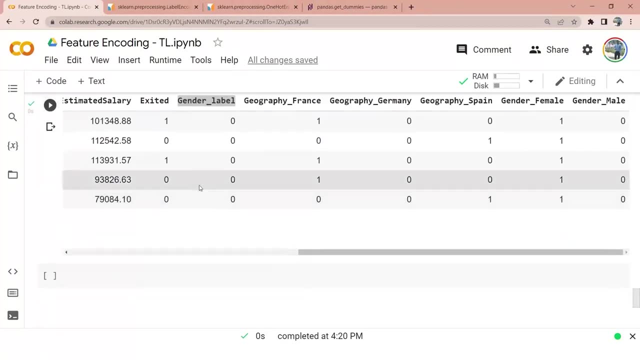 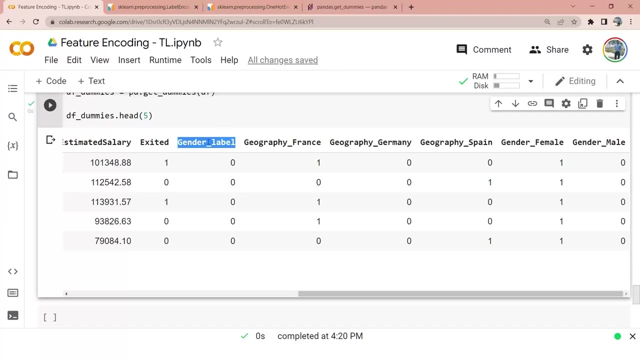 gender, two variables are created. i also see a gender underscore label because, as part of label encoding, we had also created this column, right so? so make sure, when you are actually performing these tasks, make sure you delete this redundant column which makes no sense. so that's how we perform the one hot encoding. dummy encoding, as i explained, is very similar. 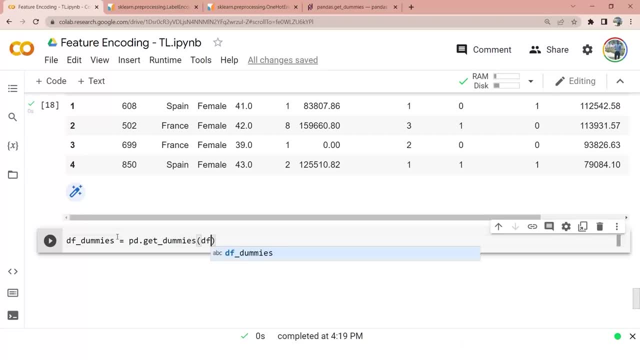 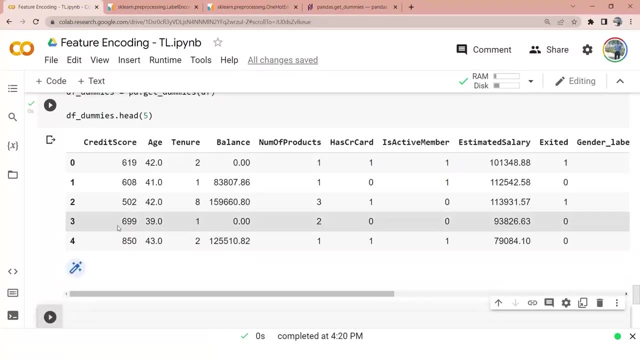 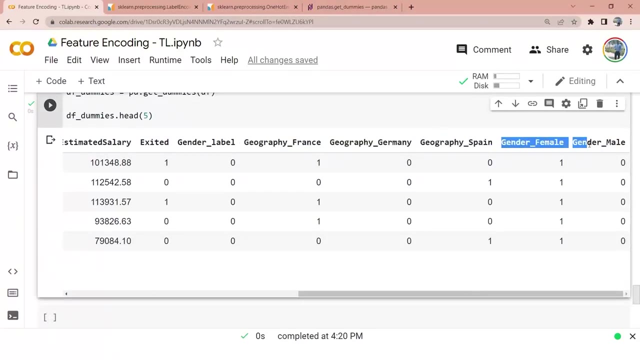 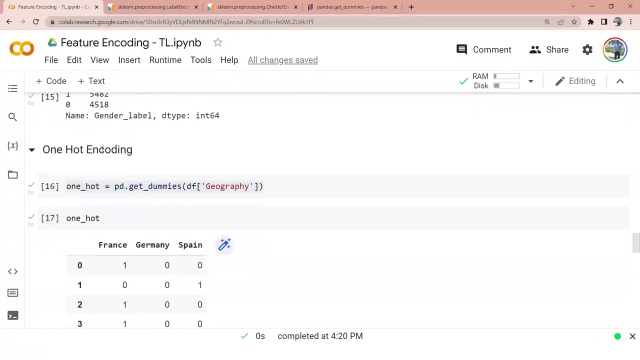 it on pd dot. get dummies on df. in the same line, i will do df underscore dummies dot head. now you can see. so dummy variables are created. for geography, three variables are created. for gender, two variables are created. i also see a gender underscore label because as part of label encoding we had also created this column right. so 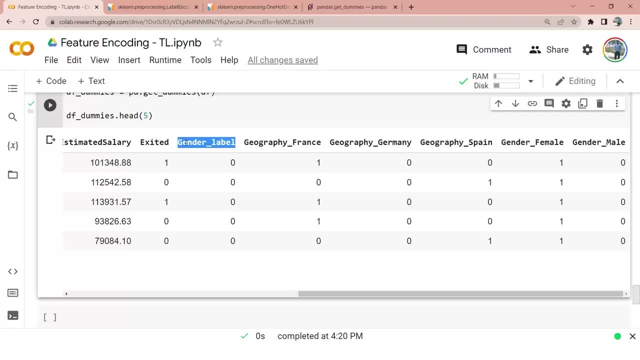 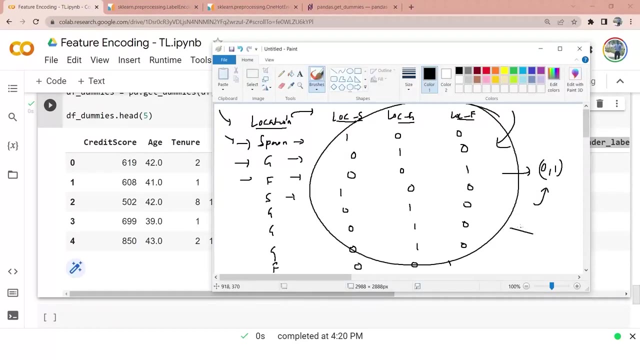 so make sure, when you are actually performing these tasks, make sure you delete these redundant columns, which makes no sense. so that's how we perform the one hot encoding. dummy encoding, as i explained, is very similar to one hot encoding. the three columns that we are getting are called as: 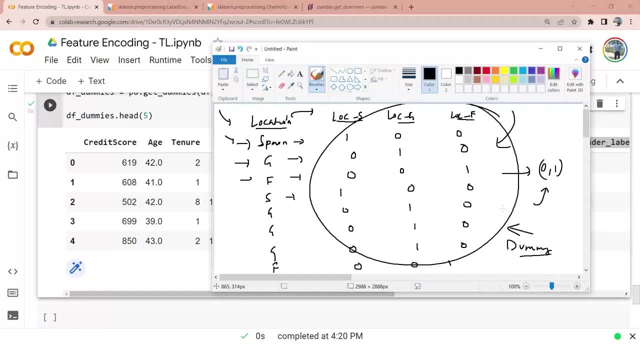 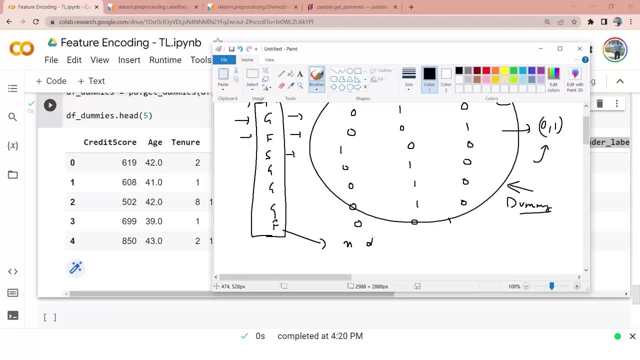 dummy columns, and whenever you create dummy columns based on the column that you are creating, it creates you n dummy columns. so it is always advisable to use n minus one dummy columns, because one of them is just giving you redundant information. so it is fine to delete one of them. 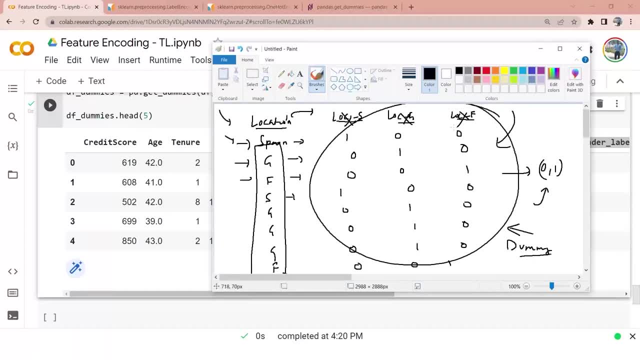 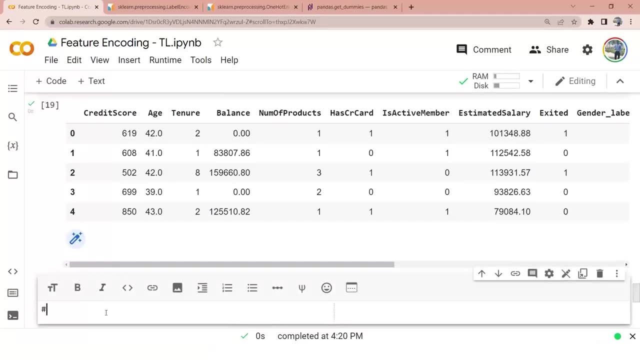 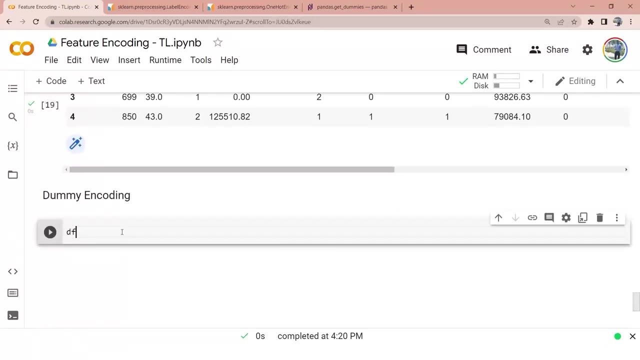 so you can delete this. this or this makes no sense. all of the three techniques are same, so we will be performing one hot encoding- sorry, dummy encoding- which is a similar encoding technique, like like in one hot encoding. so df dummies, let's say i will give it as d pd dot get dummies. i'm doing the same technique. initially i was just doing this. 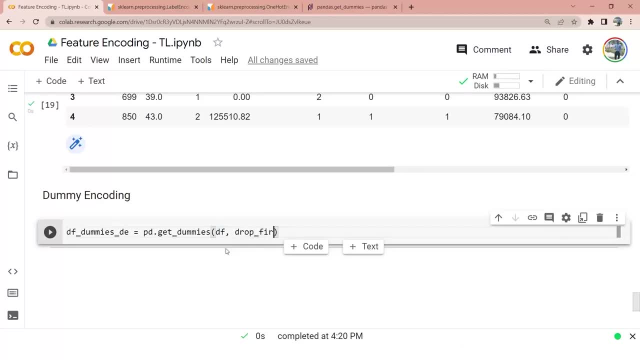 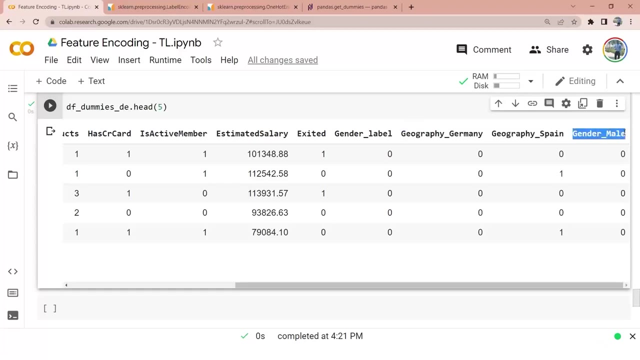 but here i will use the function called as: drop first equals to true, and the moment i do this and then do df underscore dummies. underscore d dot head, you can see that one of the features is gone- france is gone- and gender underscore- male is gone. so that is dummy encoding, one hot encoding. 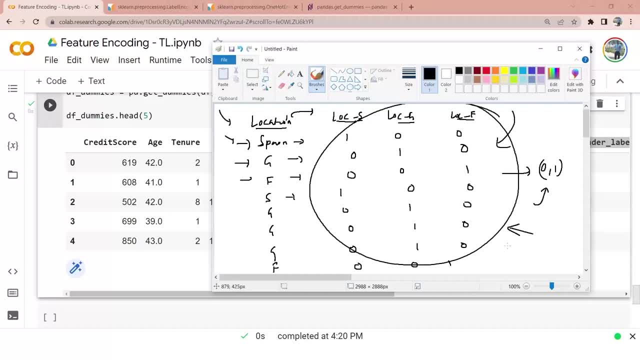 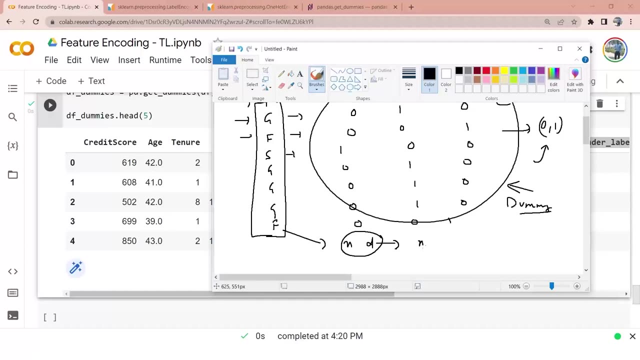 to one hot encoding. the three columns that we are getting are called as dummy columns, and whenever you create dummy columns based on the column that you are creating, it creates, you end dummy columns. so it is always advisable to use n minus 1 dummy columns, because one of them is just giving you redundant information. 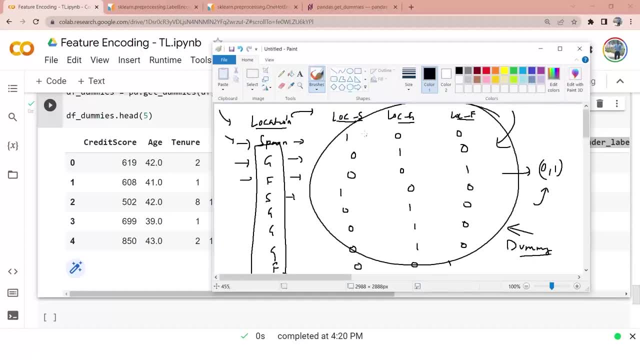 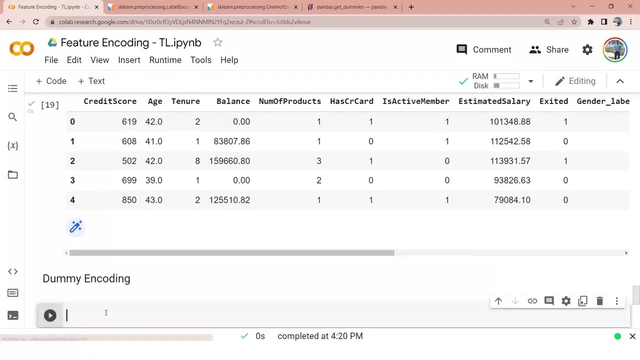 so it is fine to delete one of them, so you can delete this, this or this makes no sense. all of the three techniques are same, so we will be performing one hot encoding- sorry, dummy encoding- which is a similar encoding technique like dump, like in one hot encoding. 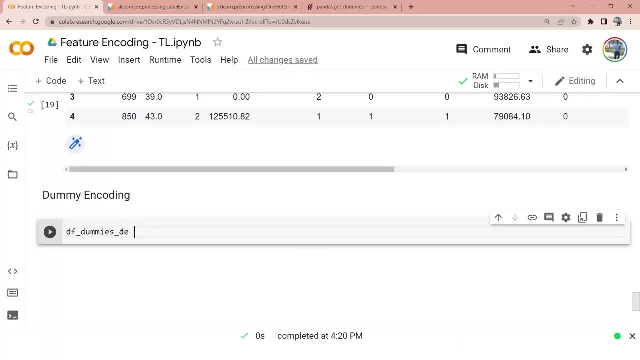 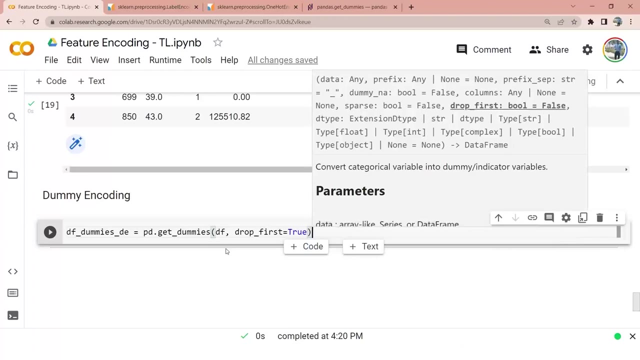 so df dummies. let's say i will give it as d pd dot get dummies. i'm doing the same technique. initially i was just doing this, but here i will use the function called as. drop first equals to true and the moment i do this and then do df underscore dummies, underscore d dot head, you can. 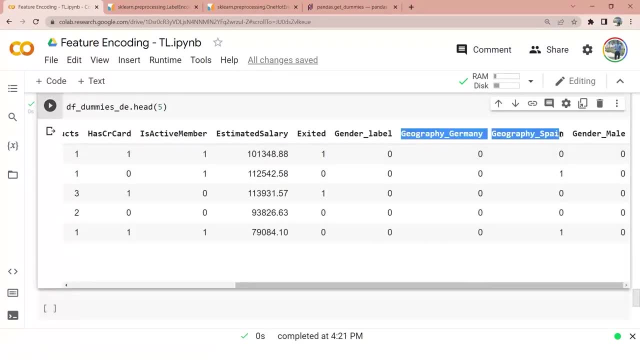 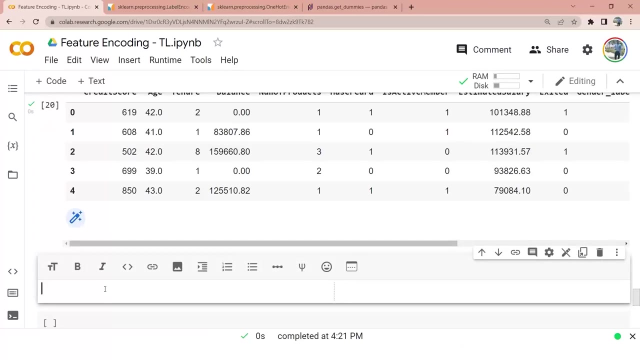 see that one of the features is gone, france is gone and gender underscore mail is gone. so that is dummy encoding. one hot encoding and dummy encoding. both are techniques that we usually go for, and my most preferred technique for x variables are dummy encoding. the next one is target encoding. 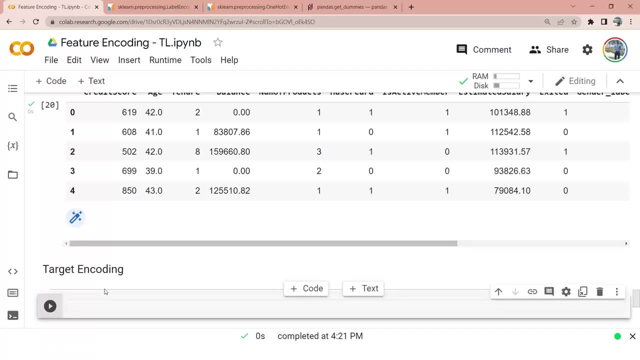 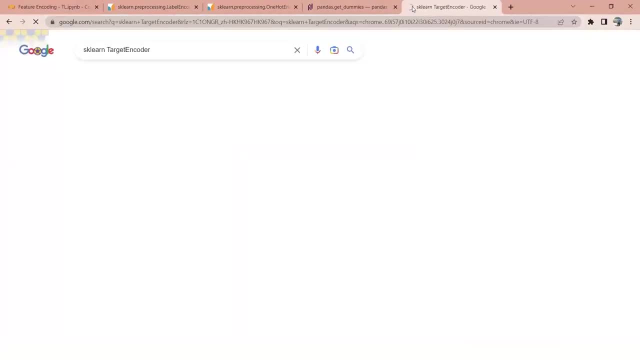 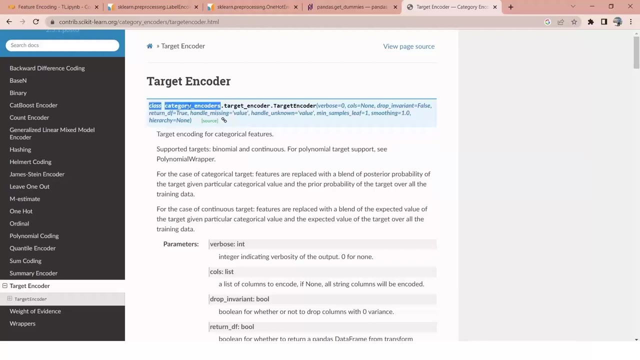 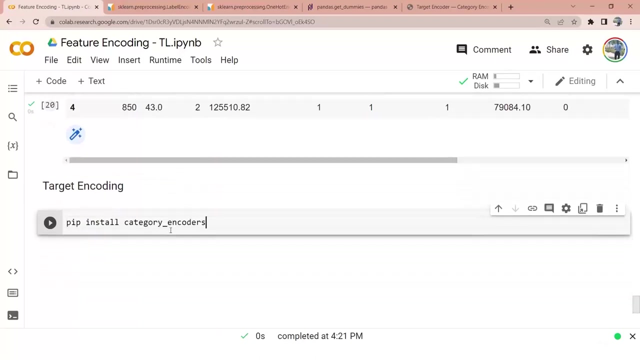 target encoding is another technique. in order to get target encoding, you can simply do sk: learn target encoder. this is basically present inside category encoder, so you have to install this category encoders. so what i will do is i will leave the command for installation, pip. install category encoders. 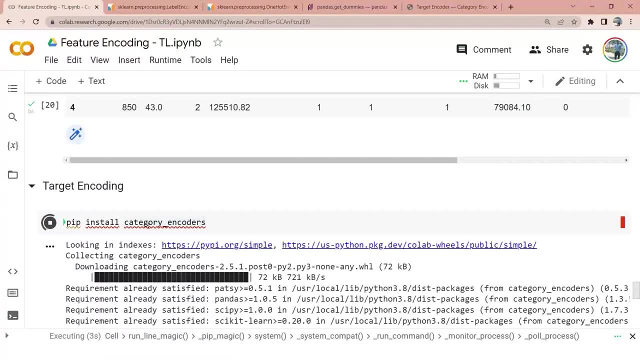 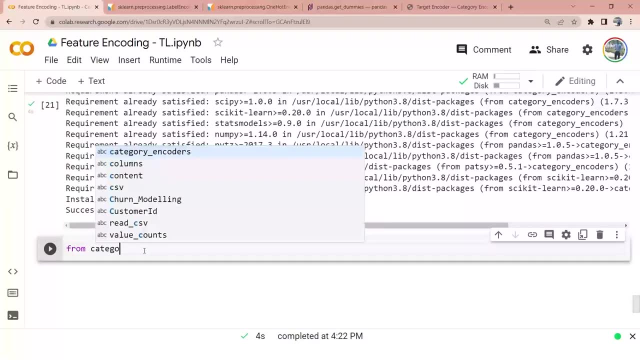 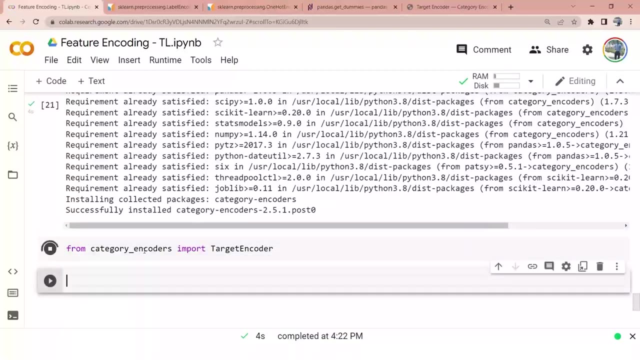 so in my case this is already installed, but in your case it will take some time to install. once that is done, simply import it. import target encoder: run this encoder equals to target encoder. so i'm instantiating my encoder. let's say: i want to create, let's have. i will again read my data frame so that we have a. 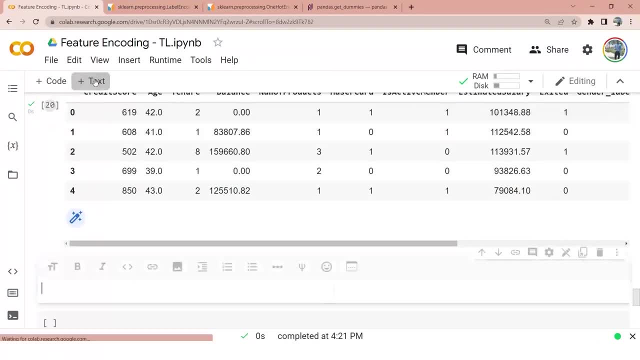 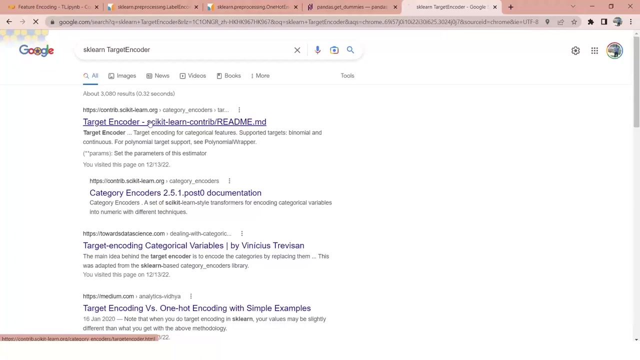 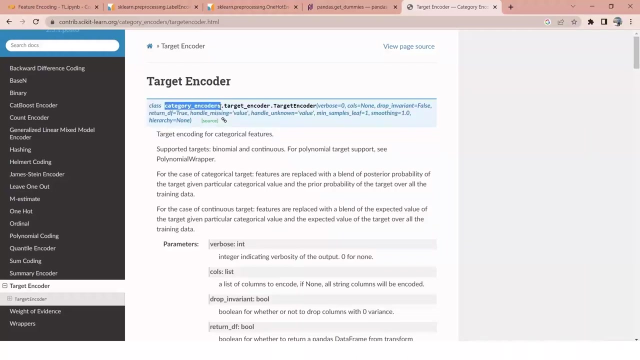 and dummy encoding. both are techniques that we usually go for and my most preferred technique for x variables are dummy encoding. the next one is target encoding. target encoding is another technique. in order to get target encoding, you can simply do sk: learn target encoder. this is basically present inside category encoder, so you have to install this category encoders. 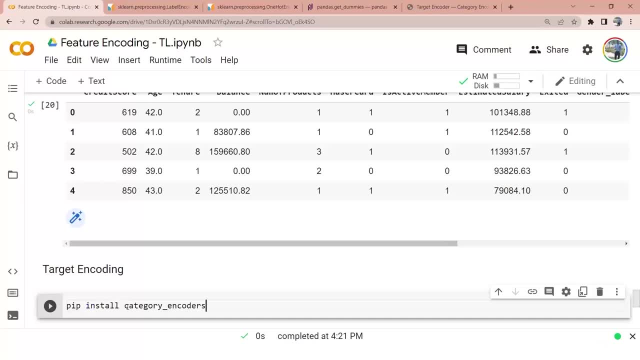 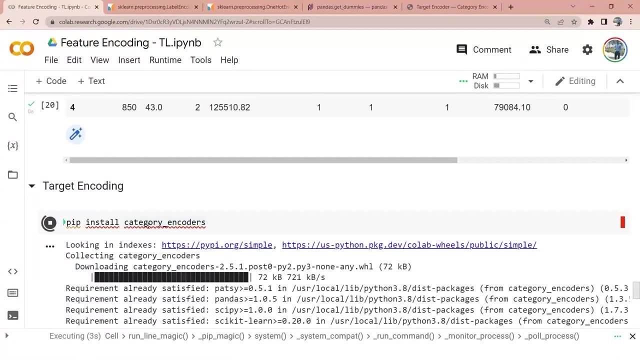 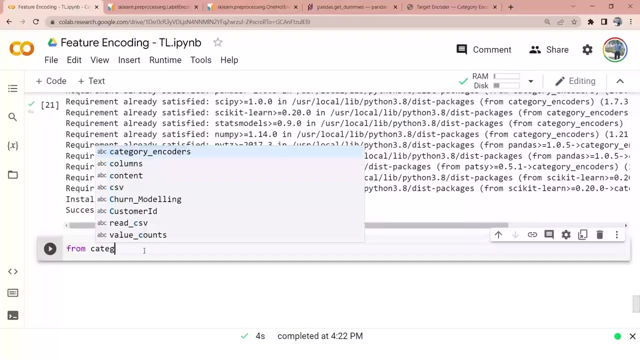 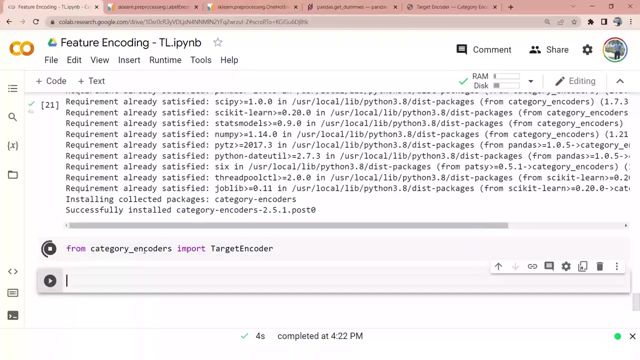 so what i will do is i will leave the command for installation, pip, install category encoders. so in my case this is already installed, but in your case it will take some time to install. once that is done, simply import it. import target encoder- run. this encoder equals to target encoder. 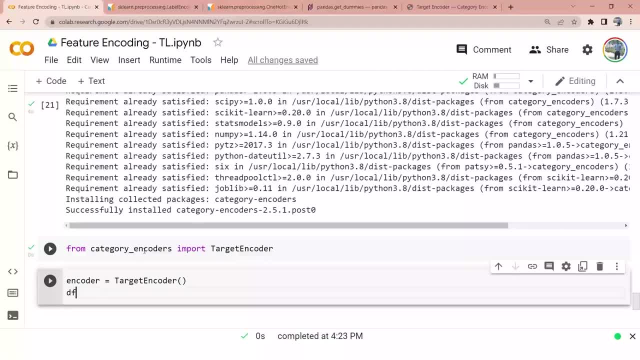 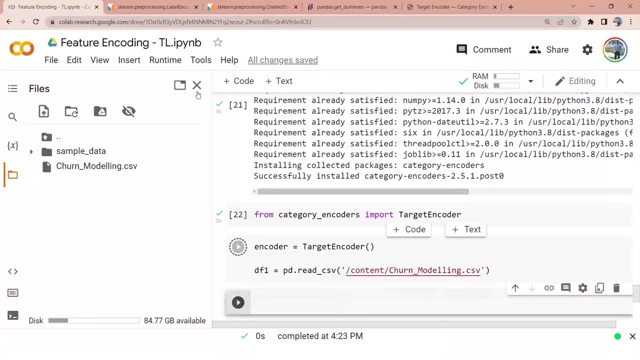 so i'm instantiating my encoder. let's say i want to create. let's say i will again read my data frame so that we have a fresh data, read csv, and then i will take the file path and paste it. so i have my new data frame df1. 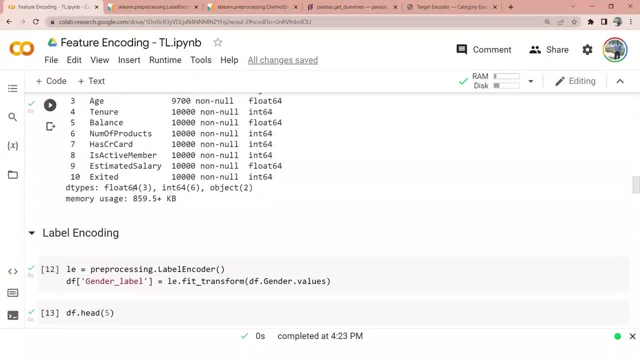 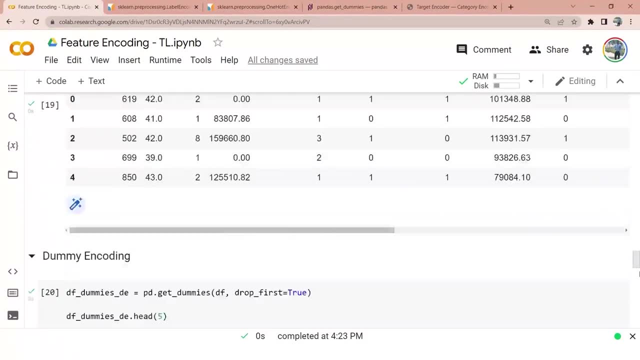 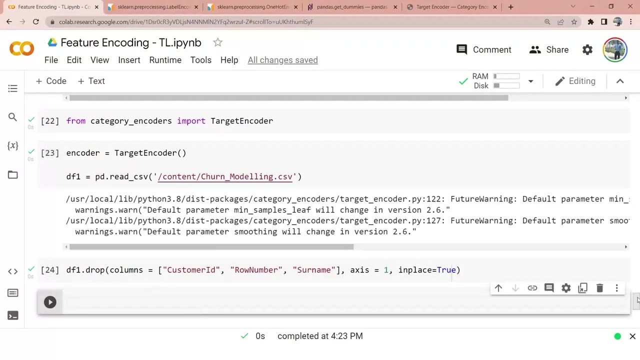 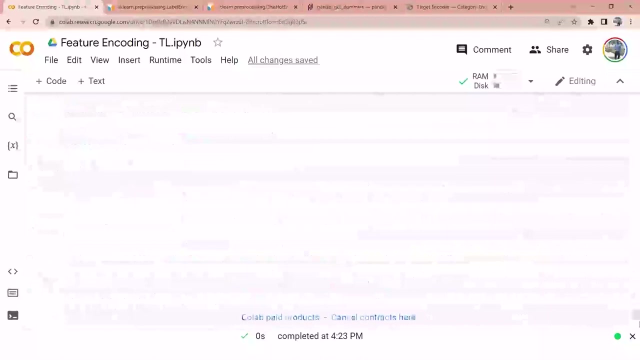 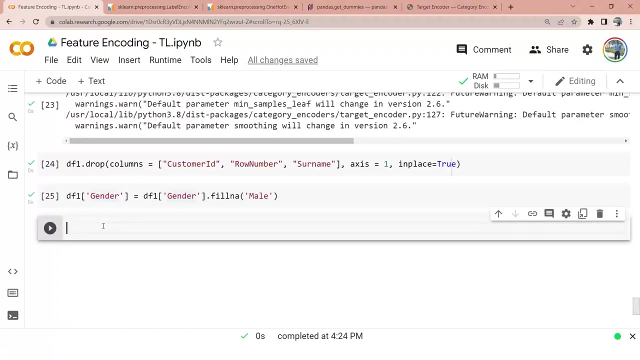 okay, again, i will perform this technique, which is my null values imputation, and this deletion: df1, df1, df1, drop it- and null values imputation. also, i will perform this technique. that's it so: df1 of gender, df1, gender fill and mail done now on top of my new. 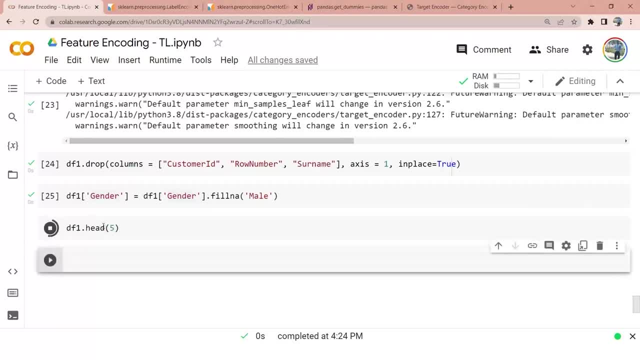 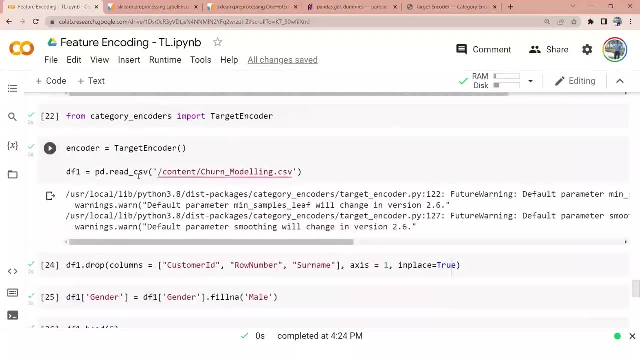 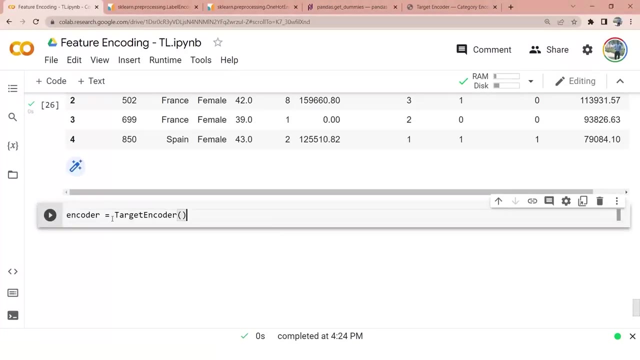 data frame which looks like this: i will be performing the target encoder, so my target encoder is already, which is: encoder equals to target encoder. let me reinitialize it and here i will do: df of gender, encoded equals to encoder. dot fit, transform and then pass df of gender- sorry, df1 of gender encoded df1 of gender and then df1 of exited. 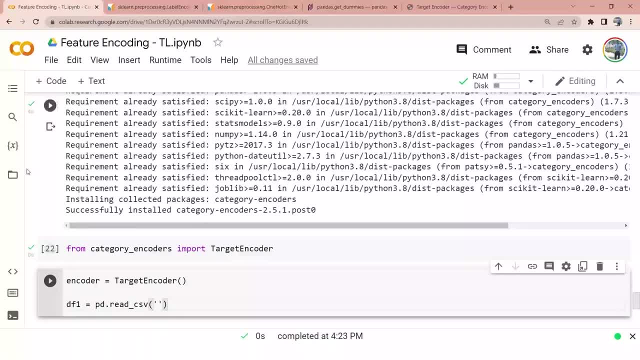 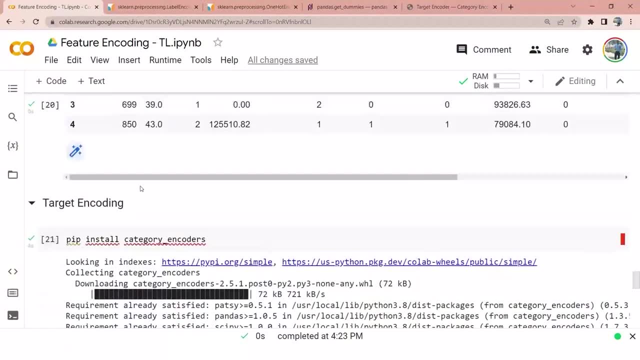 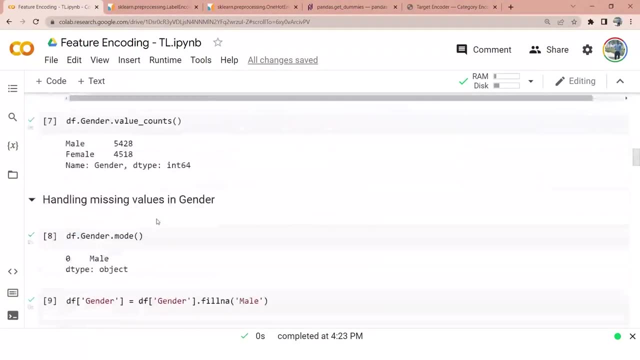 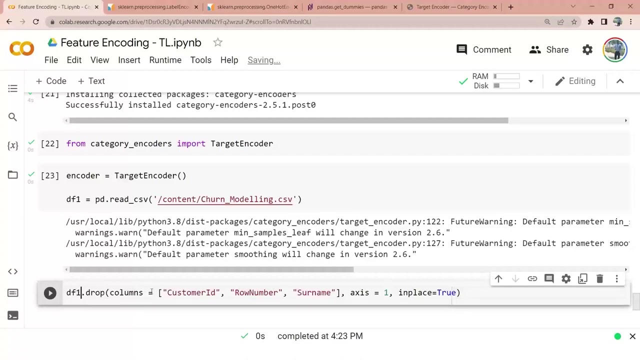 fresh data, read csv, and then i will take the file path and paste it. so i have my new data frame df1. okay, again, i will perform this technique, which is my null values imputation and this deletion df1- drop it- and null values imputation also i will perform. 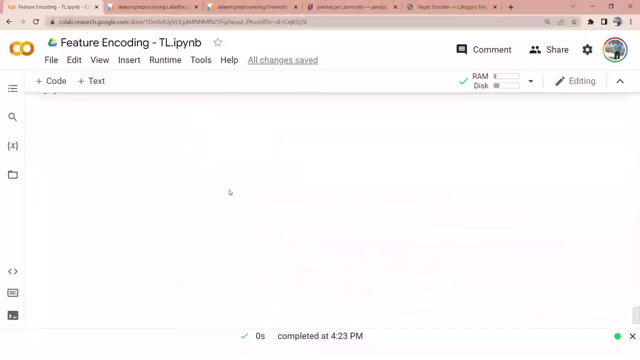 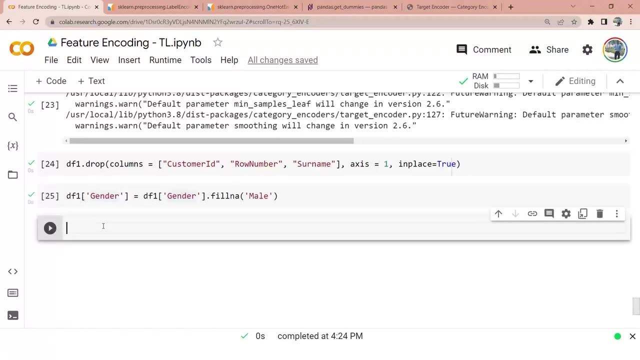 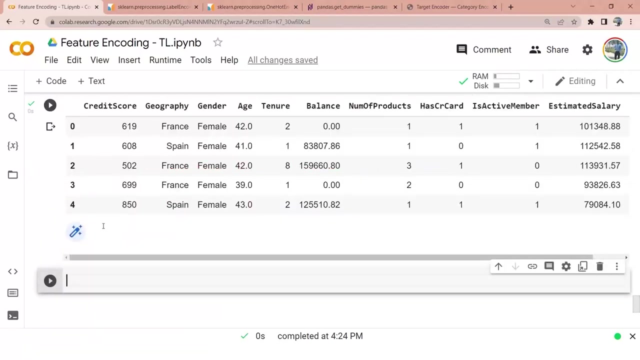 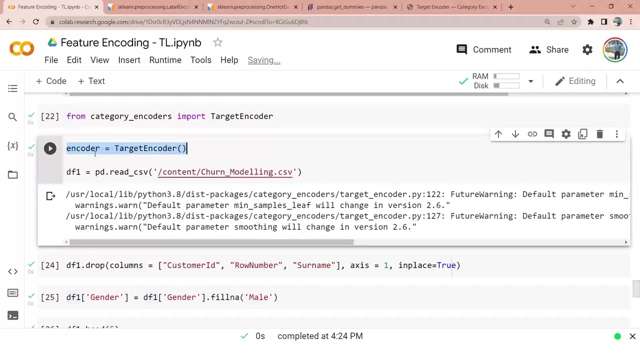 this technique. that's it. so df1 of gender, df1 of gender, fill in a male done now on top of my new data frame, which looks like this: i will be performing the target encoder. so my target encoder is already initialized, which is encoder, equals to target encoder. let me reinitialize it and here i will perform the target encoder. so my target encoder is already initialized, which is encoder, equals to target encoder. let me reinitialize it and here i will perform the target encoder. so my target encoder is already initialized, which is encoder, equals to target encoder. let me reinitialize it and here i will perform the target encoder. so my target encoder is already initialized, which is encoder, equals to target encoder. let me reinitialize it and here i will perform the target encoder. so my target encoder is already initialized, which is encoder, equals to target encoder. let me reinitialize it and here i will perform the target encoder. so my target encoder is already initialized, which 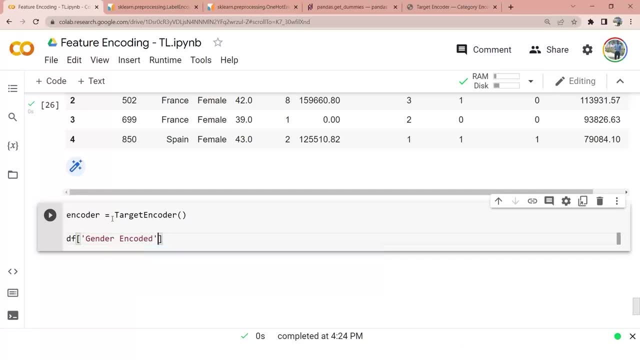 do df of gender encoded equals to encoderfit, transform and then pass df of gender. sorry, df one of gender encoded, df one of gender and then df one of exited right. as we all discussed, target encoding is one of these techniques where we consider the target features. if you don't have, 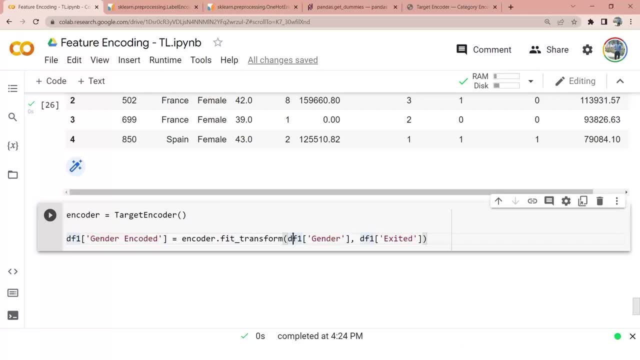 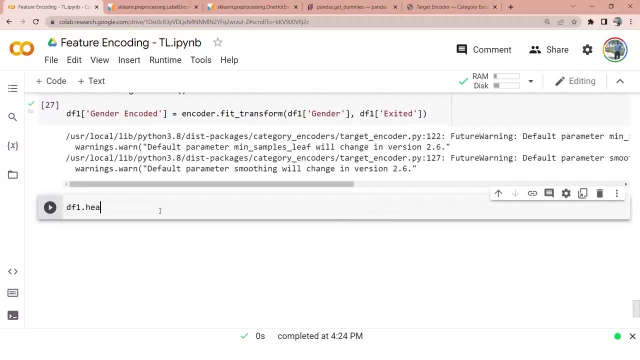 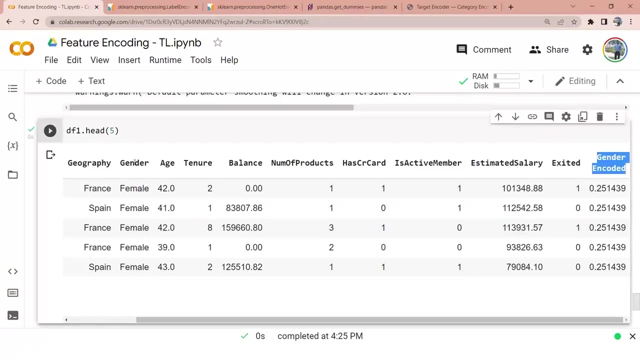 a target feature, then in that case you should not perform target encoder. so once we run this and then i do df1.head, you can see that new feature is created which is gender encoded. so instead of gender you can use this new feature and these values have been created. 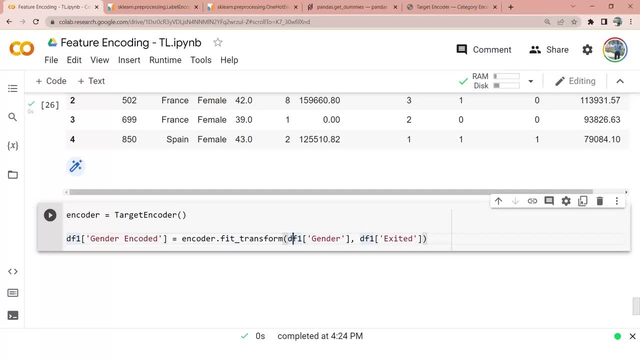 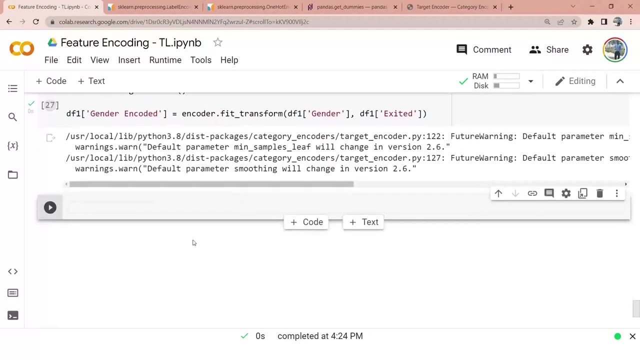 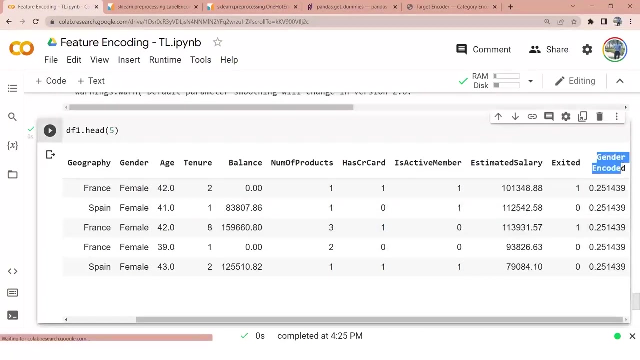 right. as we all discussed, target encoding is one of these techniques where we consider the target features. if you don't have a target feature, then in that case you should not perform target encoder. so once we run this and then i do df1 dot head, you can see that new feature is created, which 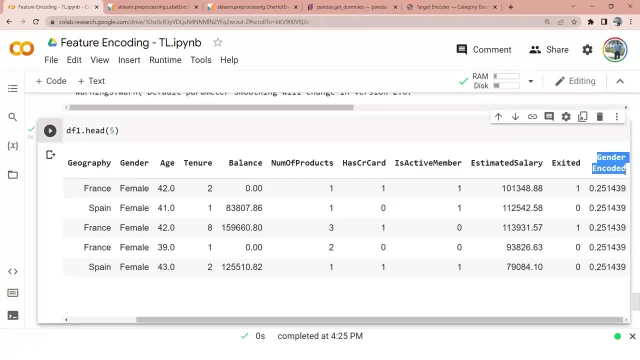 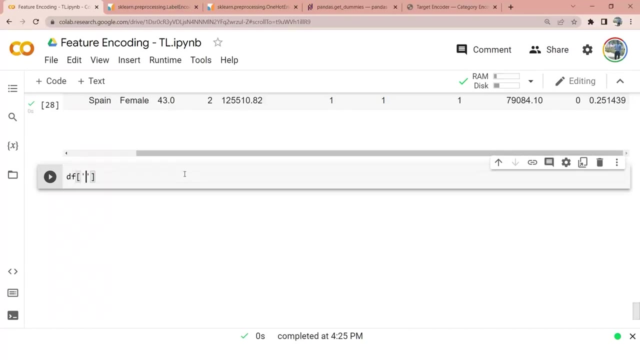 is gender encoded. so instead of gender, you can use this new feature. and these values have been created based on some mathematical calculations between gender and exited right. so if you want to have a look at what are the two values that are created- encoded dot value counts- you can see gender encoded. 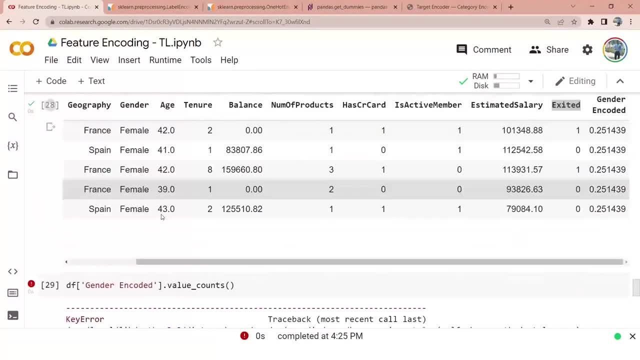 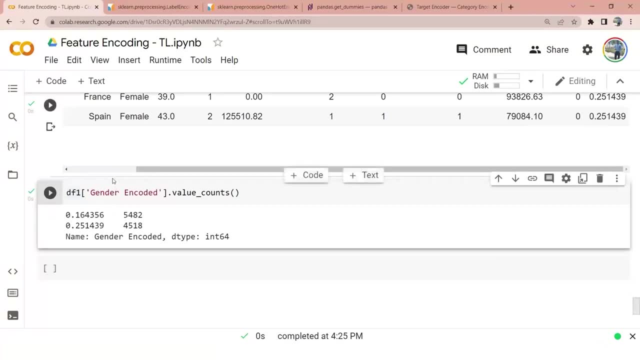 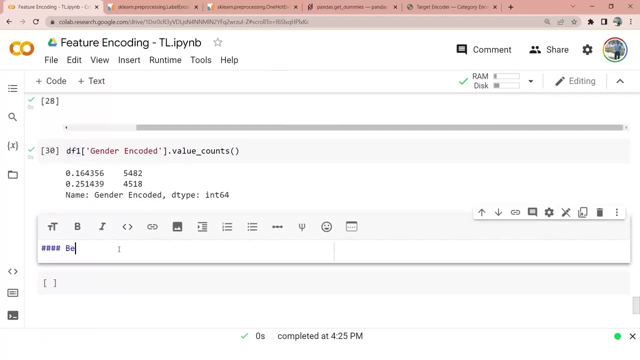 df1. so what are some of the drawbacks and benefits of target encoding? so i will talk about the benefits- benefits of target encoding. target encoding is a simple and quick encoding method. target encoding is a simple and quick encoding method that doesn't add to the dimensionality of thełement. 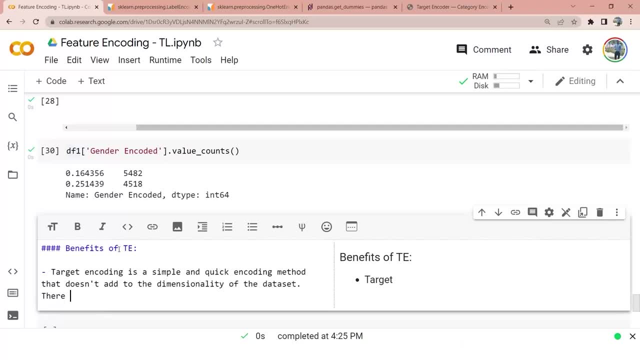 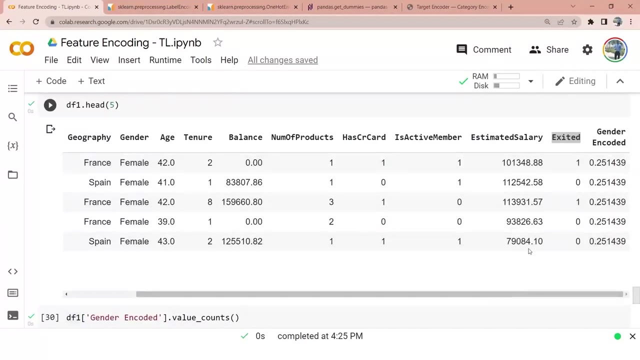 of the data set therefore. therefore, it may be used as a good first try technique. now, what do you mean by dimensionality? you can see here you are creating a new column and obviously, once the new column is created, you will not consider this column. that means originally, if you have x columns, you are adding one column and deleting one column. that 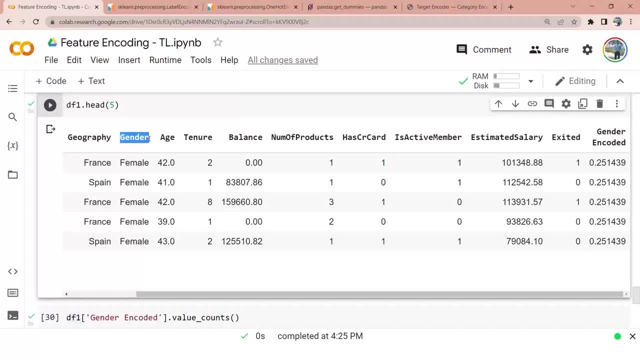 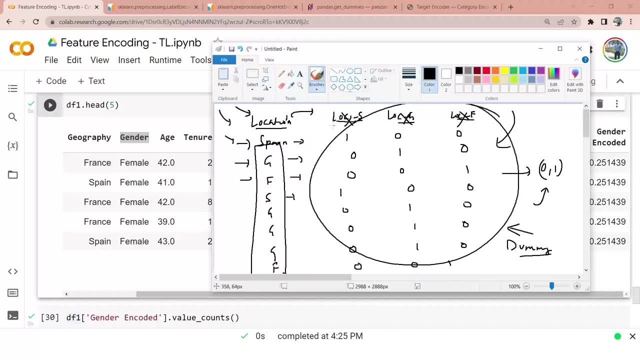 means the dimensions remains the same. however, in one hot encoding you are creating new features. so in this case, instead of location, you are creating three more features. obviously, you will be deleting one, but still you are creating two more features. imagine a column like location, where you have hundreds of locations. you will end up having hundreds of columns. if you consider. 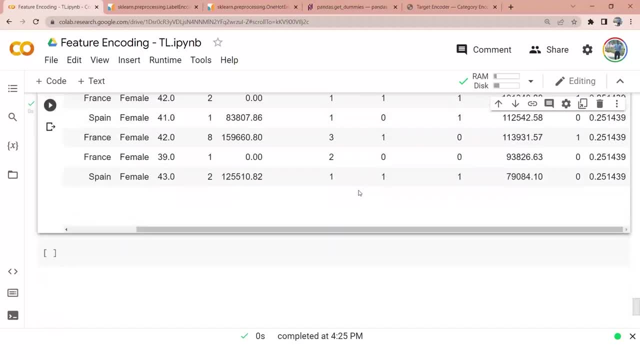 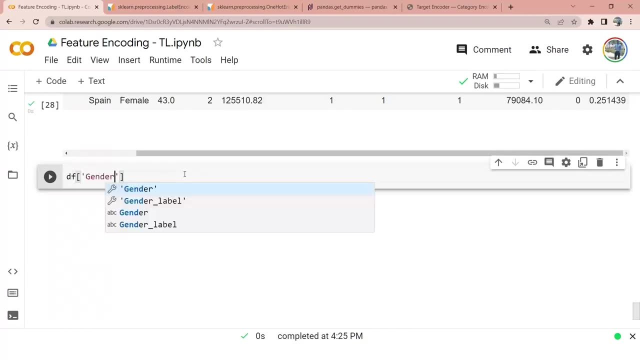 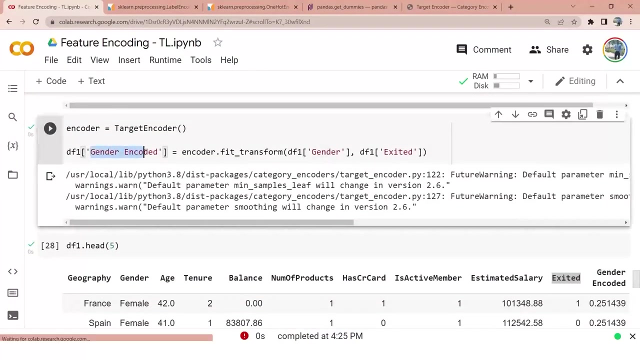 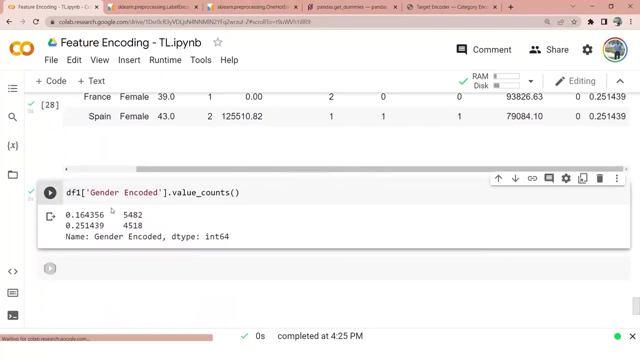 based on some mathematical calculations between gender and exited right. so if you want to have a look at what are the two values that are created, encoded dot value counts. you can see gender encoded: df1- df1. so what are some of the drawbacks and benefits of target encoding? so 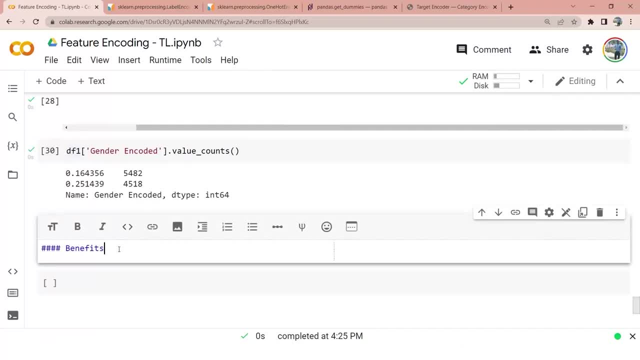 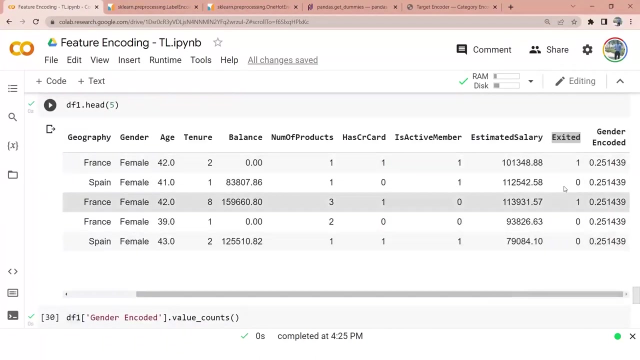 i will talk about the benefits- benefits of target encoding. target encoding is a simple and quick encoding method. target encoding is a simple and quick encoding method that doesn't add to the dimensionality of the data set. therefore, therefore, it may be david. used as a as a good first try. now, what do you mean by dimensionality? you can see here you are creating. 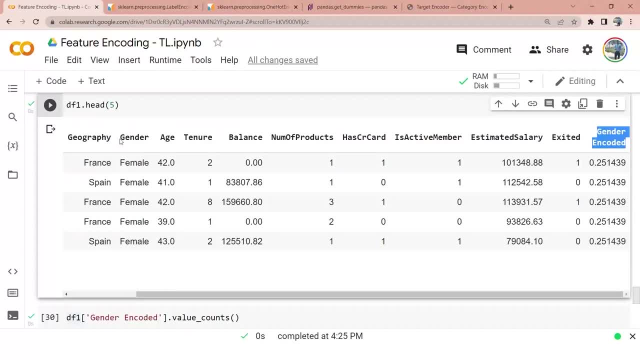 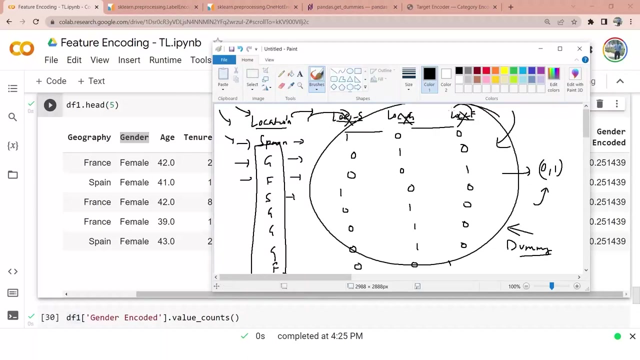 a new column and obviously, once the new column is created, you will not consider this column. that means originally, if you have x columns, you are adding one column and deleting one column. that means the dimensions remains the same. however, in one hot encoding, you are creating new features. so in this case, instead of location, you are creating three more features. obviously. 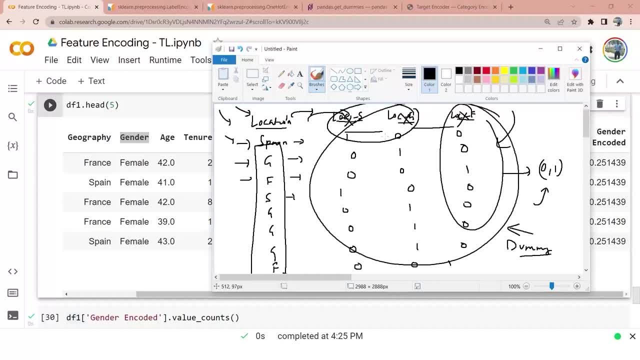 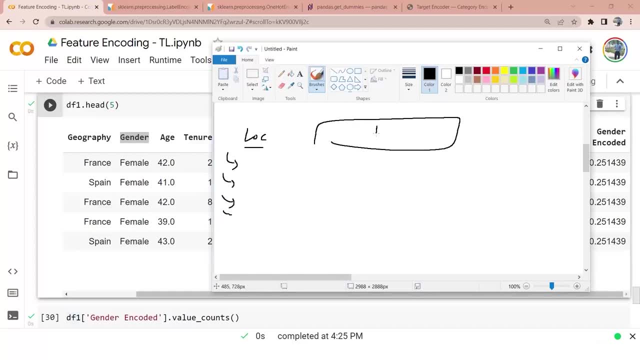 you will be deleting one, but still you are creating two more features. imagine a column like location, where you have hundreds of locations. you will end up having hundreds of columns. if you consider dummy encoding, you will end up having ninety nine columns. that means you are increasing ninety nine more features to the data. so from that point of view, you are 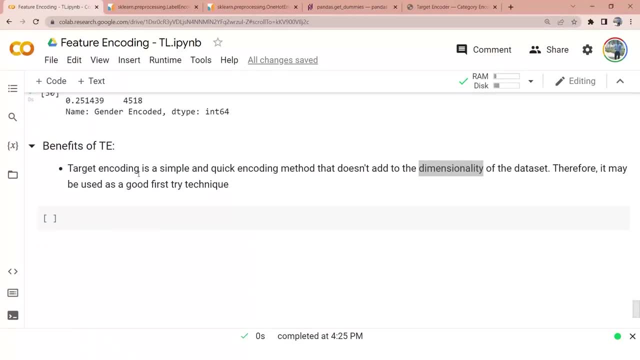 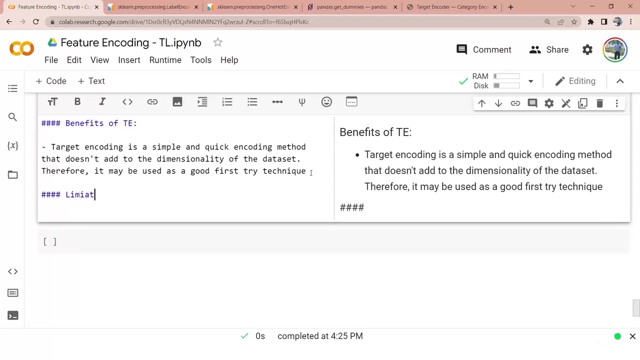 creating a new target encoding. so target encoding is good, but we usually don't go for target encoding. at least i have never used target encoding in my entire data science career. now some of the limitations are: target encoding is dependent on the distribution of the target. let me just write it down: demerits or limitations, limitations: the first limitation is it encodes. 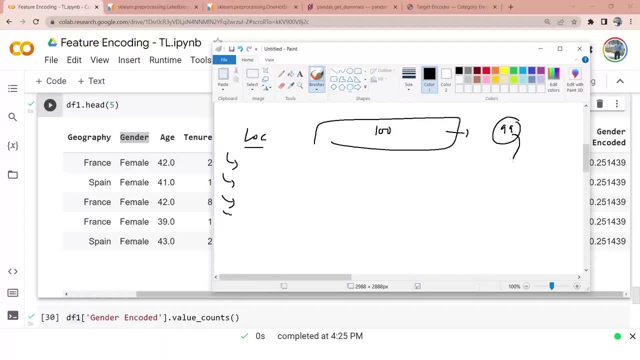 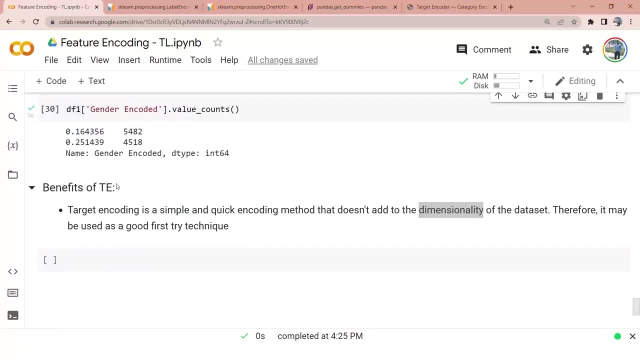 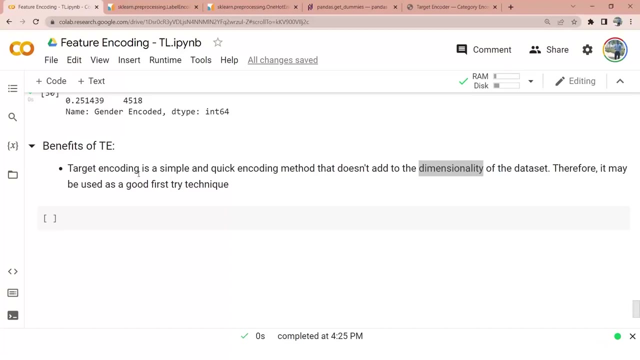 dummy encoding, you will end up having ninety nine columns. that means you are increasing ninety nine more features to the data. so from that point of view, target encoding is good. but we usually don't go for target encoding. at least i have never used target encoding in my entire data science career. now some of the limitations are target. 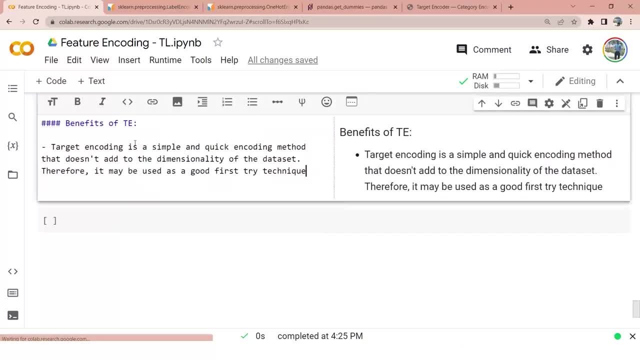 encoding is dependent on the distribution of the target. let me just write it down: demerits or limitations. the first limitation is it is dependent on the target distribution, which means target encoding requires careful validation as it can be prone to overfitting. overfitting is: 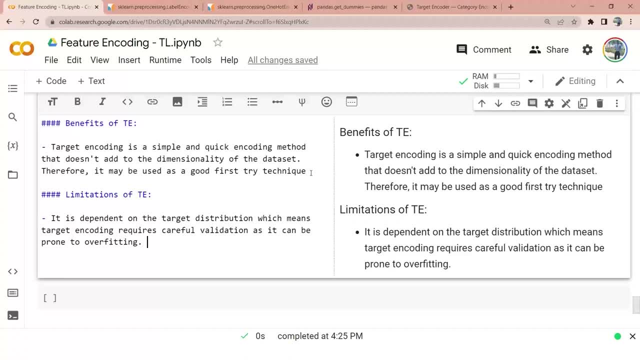 one of the scenarios in predictive analytics which occurs when you are able to achieve good accuracy or a good performance in your training data, but when you are trying to test it on a testing data which is unseen to the model, unseen to your algorithm, your accuracy decreases drastically. that is overfitting, but in details we will be covering that in. 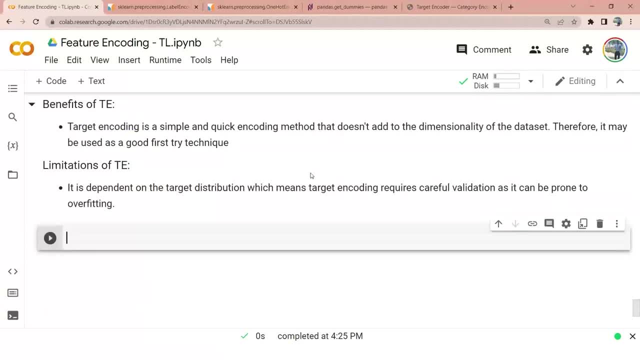 the next session in the next module. so these are some of the benefits and limitations of target encoding. the last feature that we are going to cover in the next session is the target encoding. the last feature that we are going to cover in the next session is the target encoding. 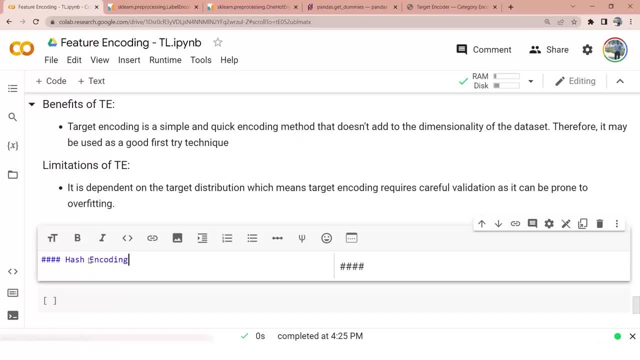 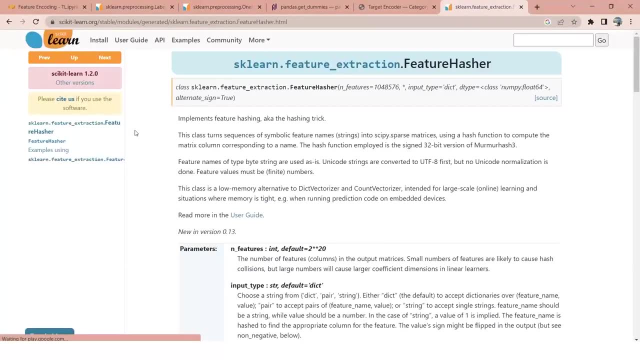 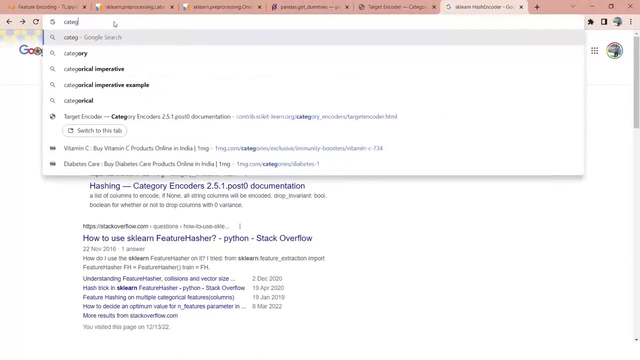 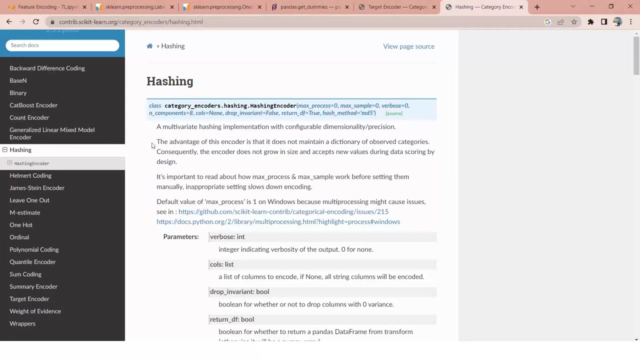 the next feature that we are going to cover in the next session is the target encoding. so target encoding, we are going to consider the apns. so basically, the target encoding is followed by an 672, so this is their title, that we are kind of getting ahead of them. theう in the description. 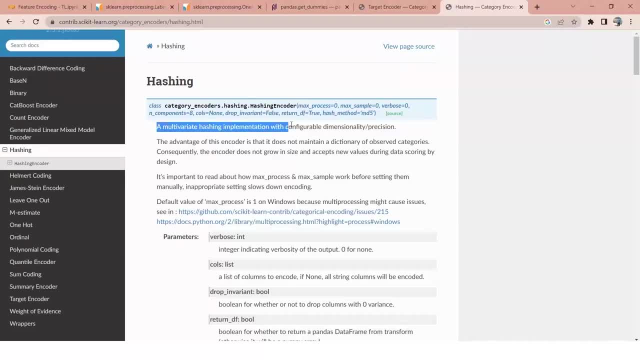 is given, but as a sub establishment for a target encoding me, they will be surfacing as well. so i was telling about the target encoding and target encoding table, how to connect and how to flirt those kinds of target encoding implementation with configurable dimensionality or precision. there is a component called as n. 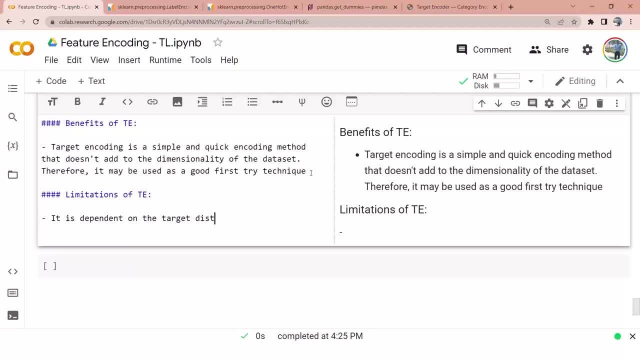 is dependent on the target distribution, which means target encoding requires careful validation as it can be prone to overfitting. overfitting is one of the scenarios in predictive analytics which occurs when you are able to achieve a good accuracy or a good performance in your training data, but when you are trying to test your training data, you will not be able to. 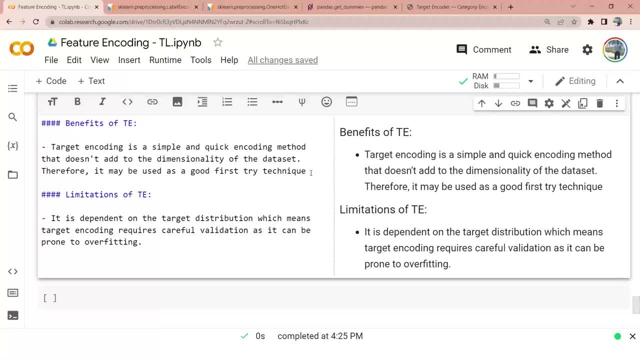 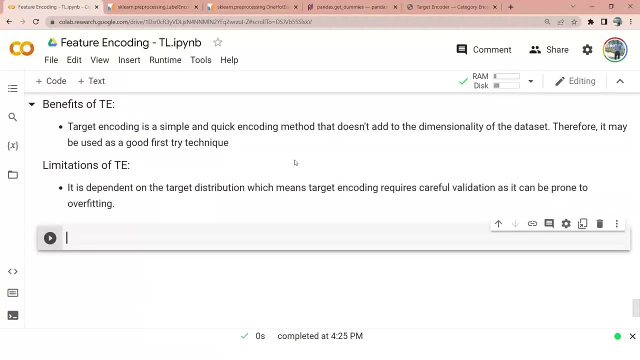 test it on a testing data which is unseen to the model, unseen to your algorithm, your accuracy decreases drastically. that is overfitting. but in details we will be covering that in the next session, in the next module. so these are some of the benefits and limitations of 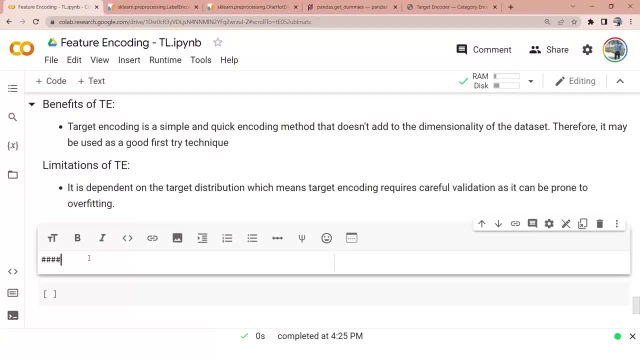 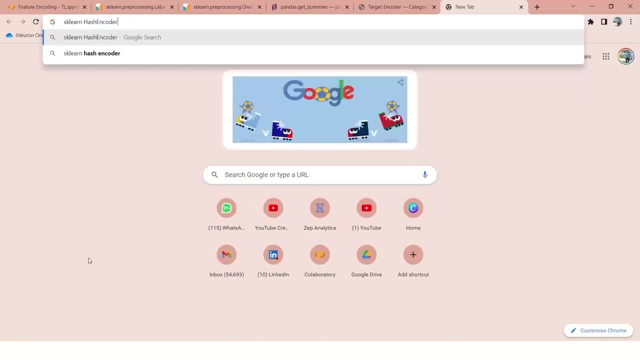 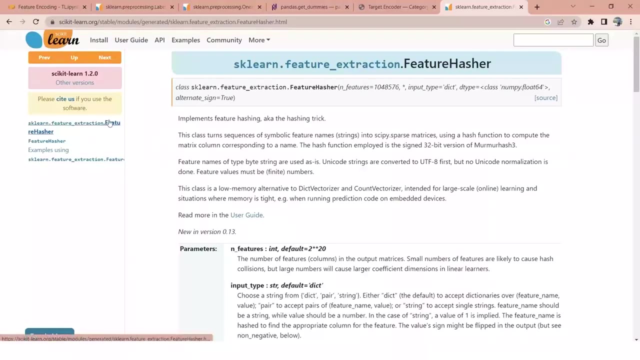 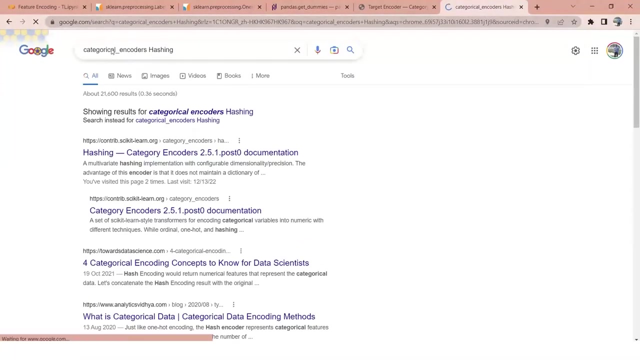 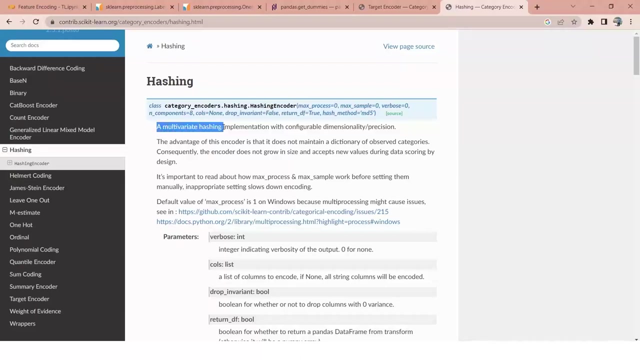 target encoding. the last feature encoding technique i would talk about is hash encoding. so we will learn hash encoder. so i'm not talking about this one. maybe i'll just search categorical encoders, hashing this one. so this is what i'm talking about, which is a hash encoding. it's a multivariate hashing. 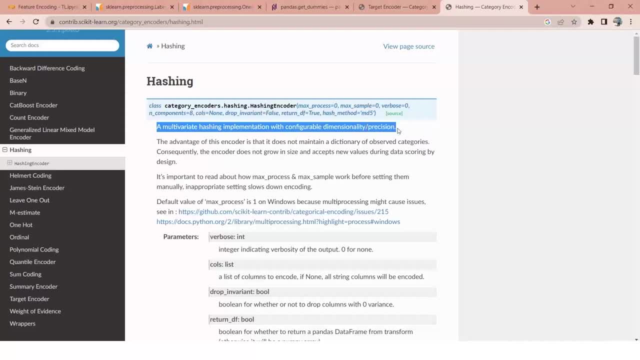 implementation with configurable dimensionality or precision. there is a component called as n components. if you define it as 8, which is the by default number, it will create 8 more columns, 8 more numerical columns. the advantage of this encoder is that it does not maintain a dictionary. 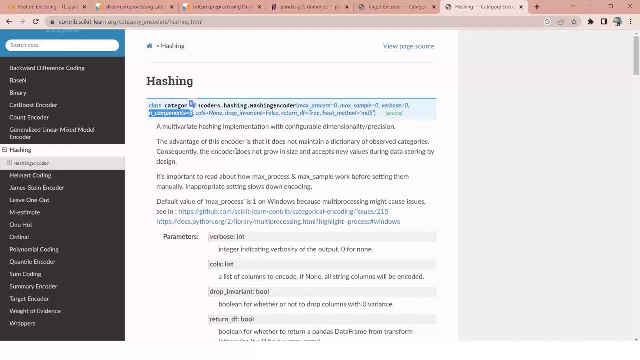 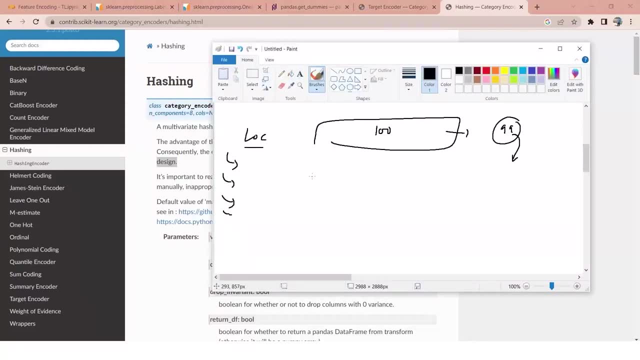 of observed categories. consequently, the encoder does not grow in size and accepts new values during data scoring by design. see if you have a column like gender- you have male or female. then also, if you define n, components are eight, you will get eight new columns. if you have a 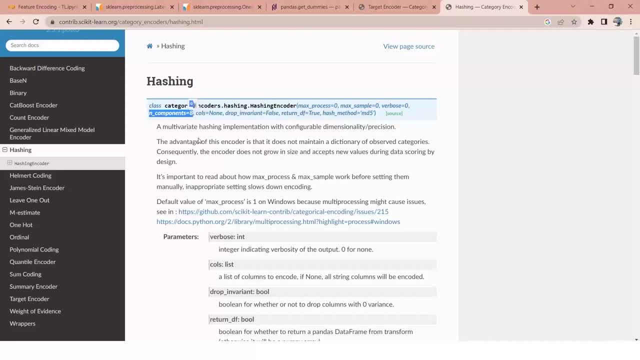 components. if you define it as eight, which is the by default number, it will create eight more columns, eight more numerical columns. the advantage of this encoder is that it does not maintain a dictionary of observed categories. consequently, the encoder does not grow in size and accepts new values during data scoring by design. see if you have a column like gender, you have male or 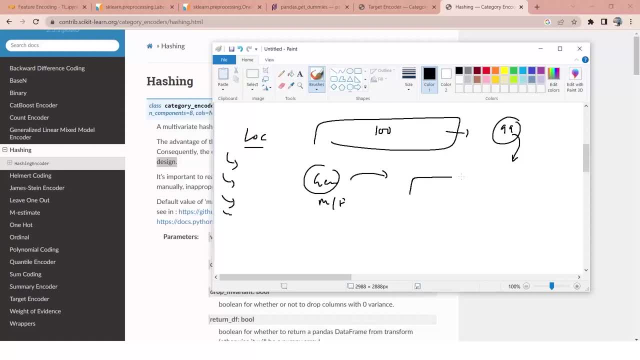 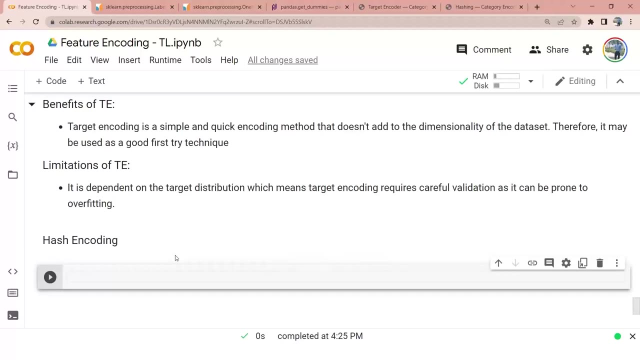 female, then also, if you define n components as eight, you will get eight new columns. if you have a column like location, where you have hundreds of values, then also you can create eight columns. so that's how the hashing is done. so how to create hash encoding simply: 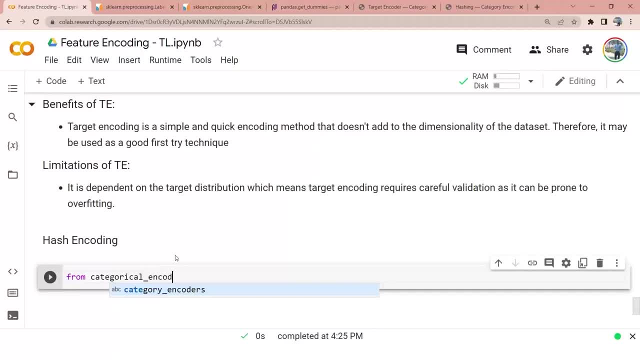 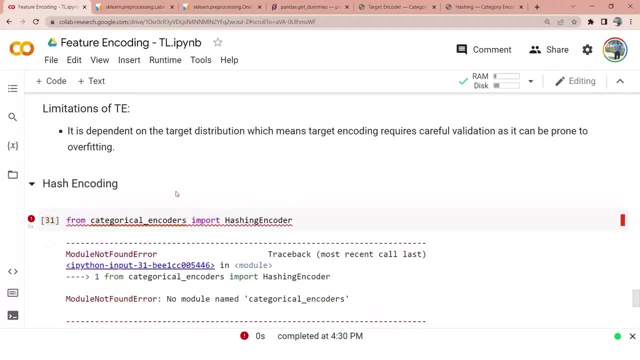 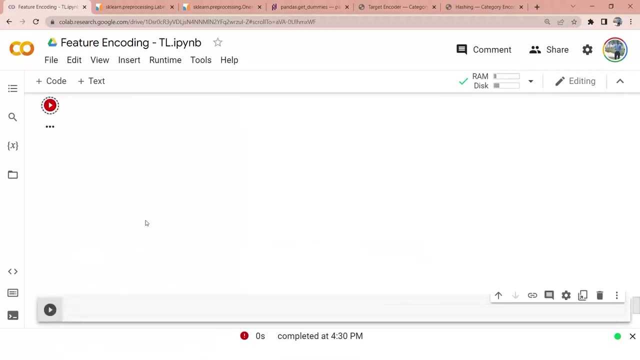 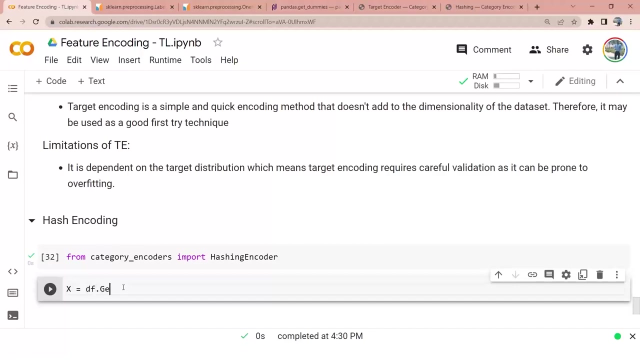 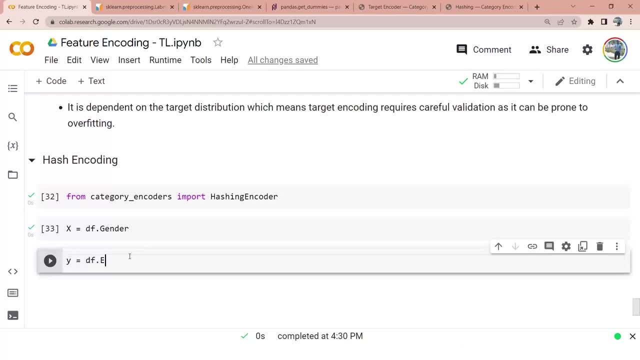 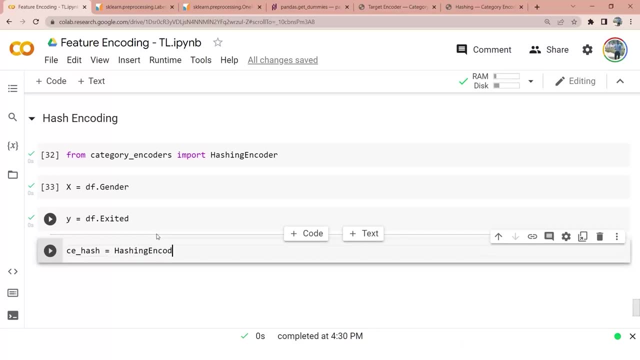 x as my gender and y as my exited column. so let's say i will define my hashing encoding here, which is hashing encoder. let's say i want to do it on gender column and then i will do pe underscore, hash dot fit, transform x and y the moment i do. 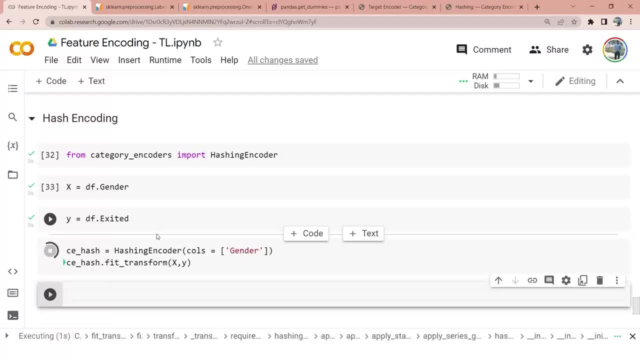 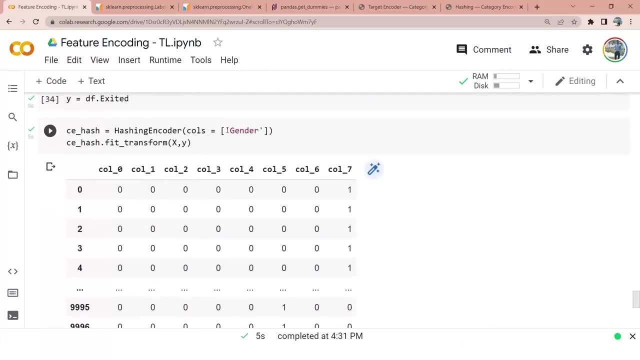 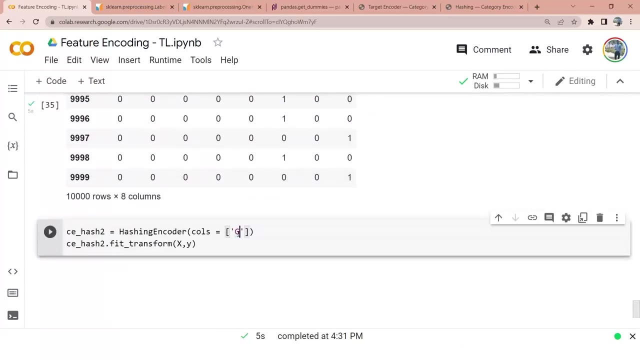 this, you will be able to see six new- sorry, eight new- columns. okay, and those are your hashed numerical columns, which you have achieved from this gender column. similarly, if you want to do it for geography, let's say hash 2, hash 2. so in order to achieve this, you also have to change. 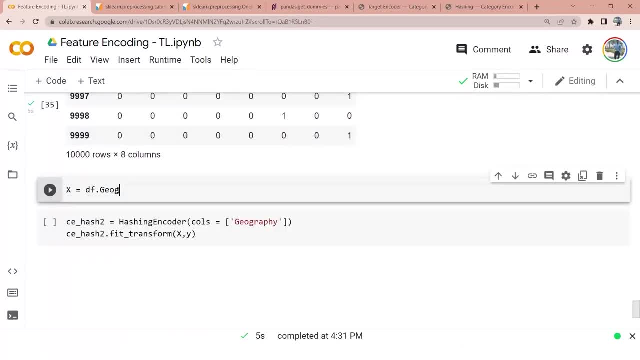 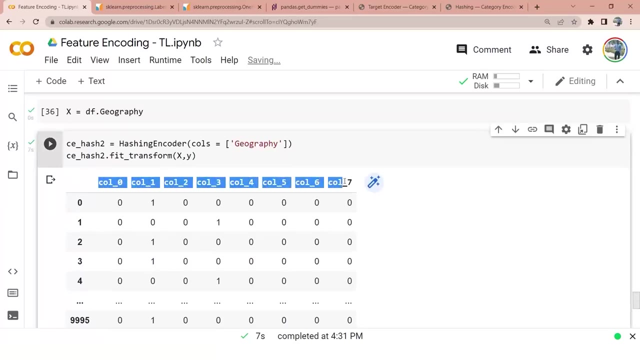 your x variable here. so so, so you can see same eight new columns has been created, and how they have been created is the algorithm that is doing, the hashing algorithm, which is not necessary for us to understand what's happening beneath it, but overall what's happening is, irrespective of the type of values, 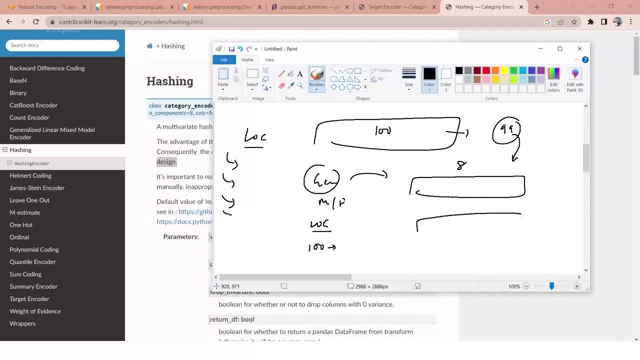 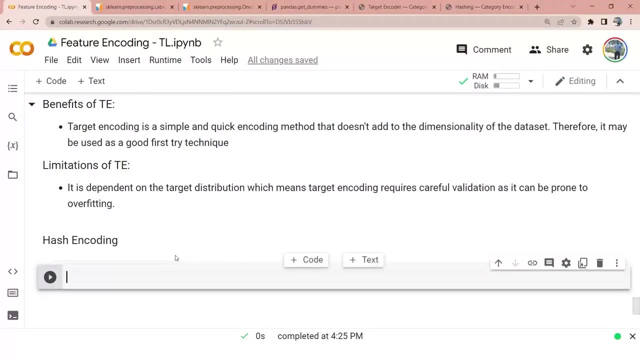 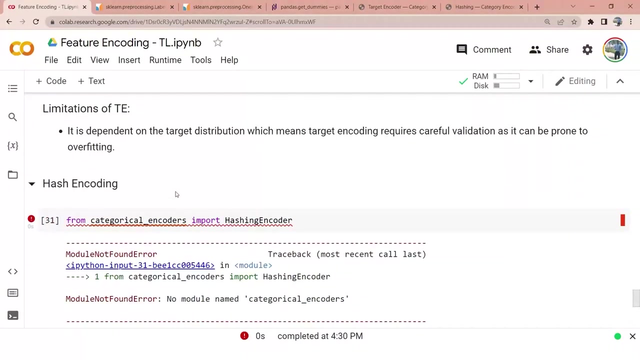 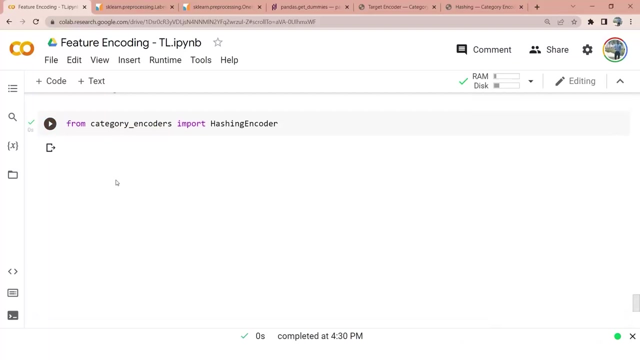 column, like location where you have hundreds of values. then also you can create eight columns. so that's how the hashing is done. so how to create hash encoding simply from categorical encoder: does import hashing encoder? and then let's say: module not found. categorical, no category, category: okay. so let's say- i'm going to take an example- let's say x equals to df dot gender. i'm going 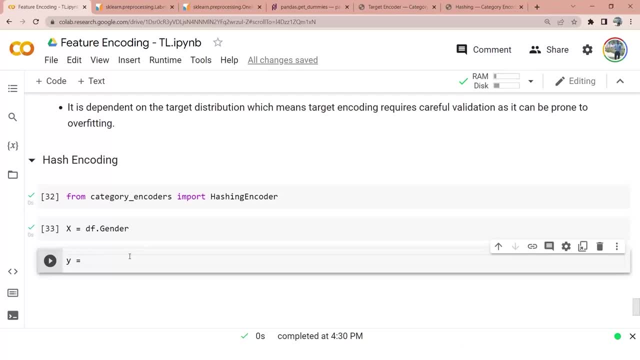 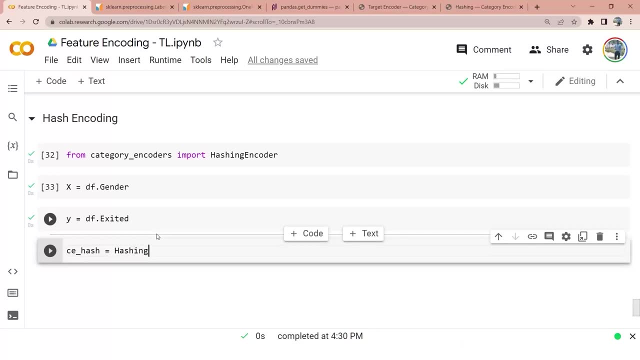 to take x as my gender and y as my exited column. so let's say i will define my hashing encoding here, which is hashing encoder. let's say i want to do it on gender column and then i will do pe underscore, hash dot, fit, transform x and y. the moment i do this, you will. 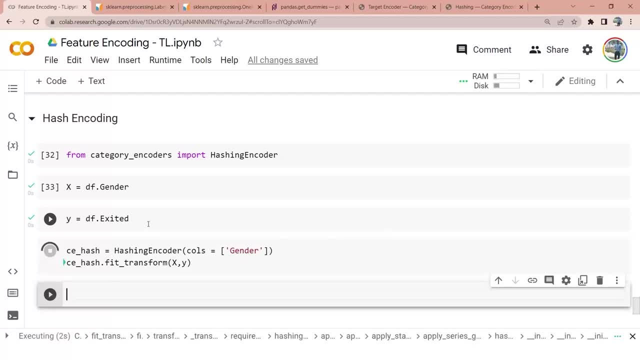 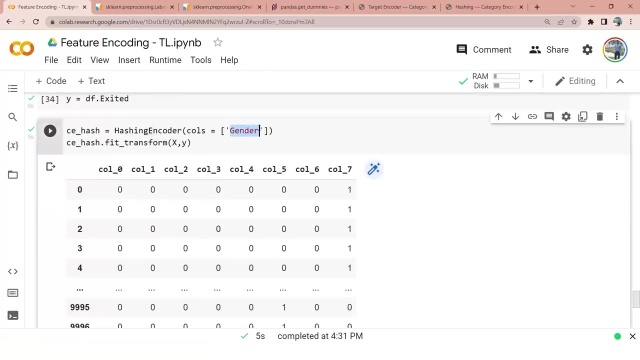 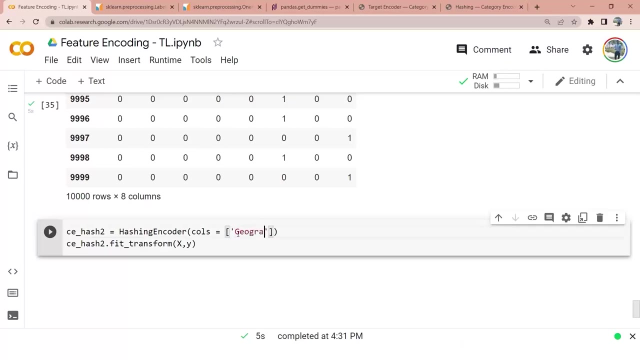 be able to see six new- sorry, eight new- columns. okay, and those are your hashed numerical columns which you have achieved from this gender column. similarly, if you want to do it for geography, let's say hash 2, hash 2. so in order to achieve this, you also have to change your x variable here. 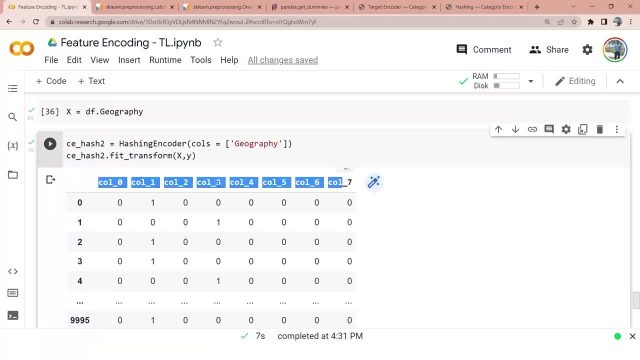 so you can see same. eight new columns has been created, and how they have been created is the algorithm that is doing, the hashing algorithm, which is not necessary for us to understand what's happening beneath it. but overall, what's happening is, irrespective of the type of values you have in your categorical feature. you are ultimately getting eight components. 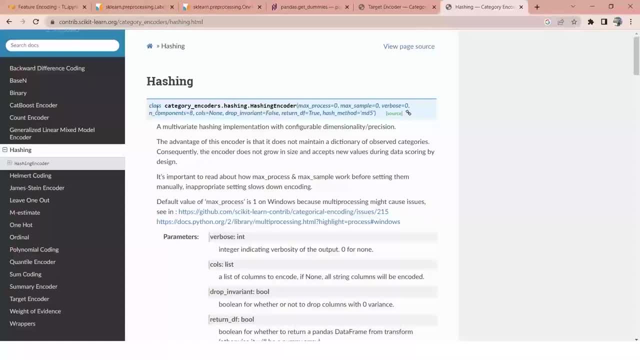 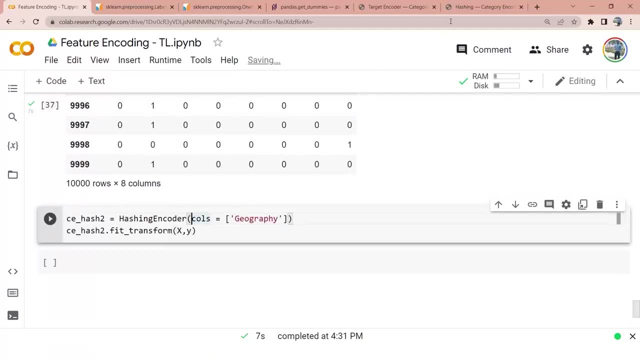 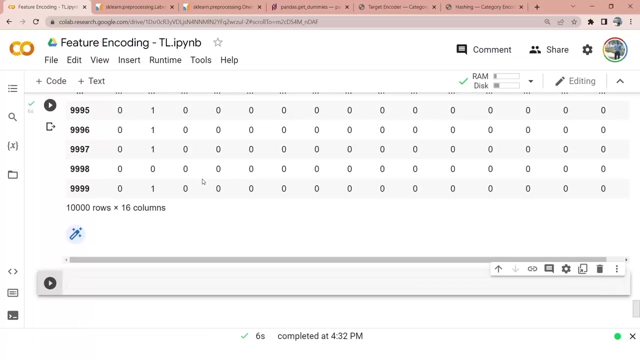 if you want to change it, you have to change your n components. let's say here, instead of the n components 8, i will use n components equals 16. to do this, 16 columns will be created. so that brings us to the end of this entire practical sessions on different feature. 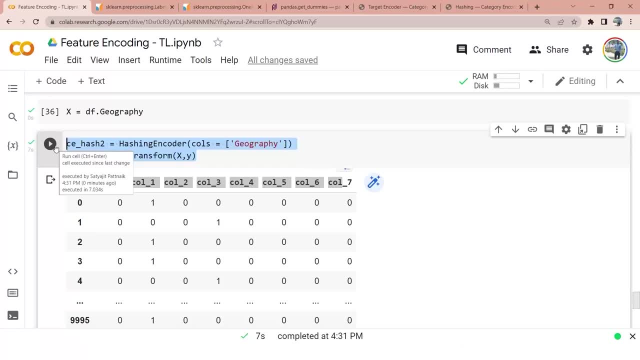 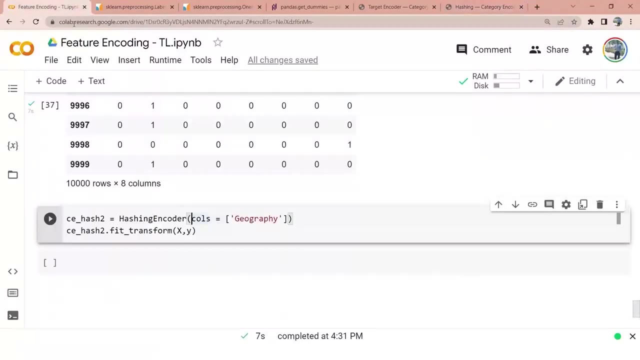 you have in your categorical feature, you are ultimately getting eight components. if you want to change it, you have to change your n components. let's say so here: instead of the n components 8, i will use n components equals 16. to do this, 16 columns will. 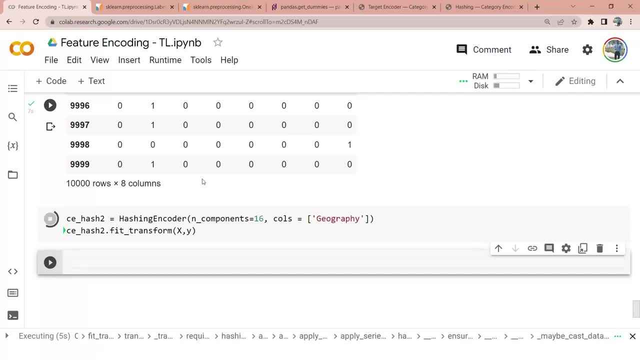 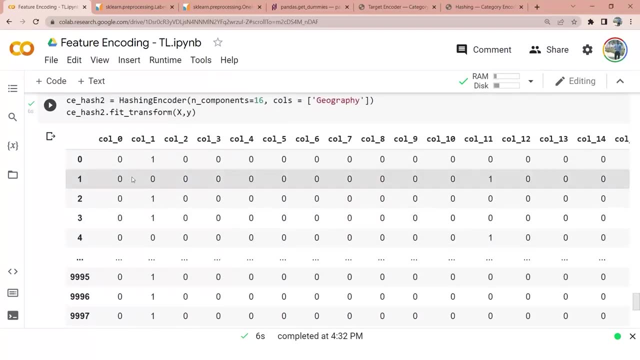 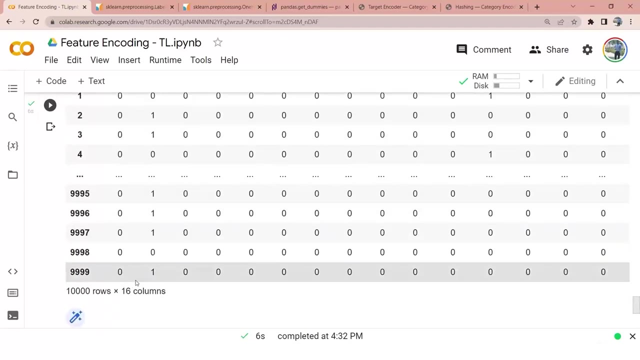 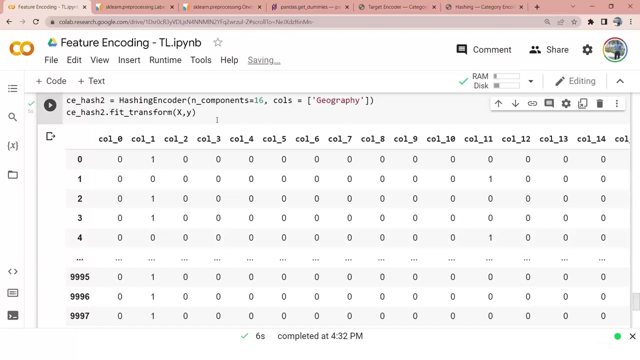 be created. so that brings us to the end of this entire practical sessions on different feature encoding techniques, and this technique is definitely mandatory when it comes to predictive analytics. so you can see on the screen you have 16 columns and these are the columns that are used on all of the Paulson classrooms and these are hashed columns that has been created using some hashing technique. so that's all about. 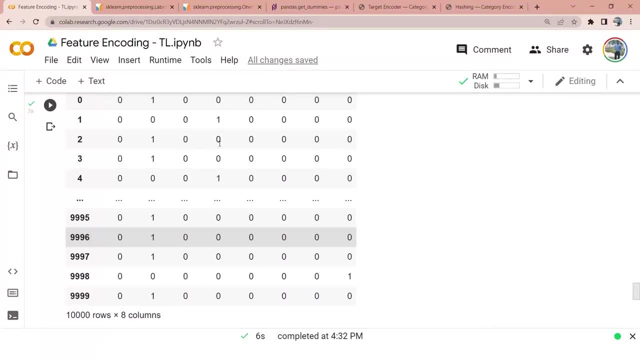 different feature encoding techniques. I hope you understood the concepts behind it. in the next video we shall be jumping into the use case, the case study, where we will be taking example of a live data set or one of the public data sets and we will be performing edas step-by-step and finally analyzing the insights that we will get from the data set. 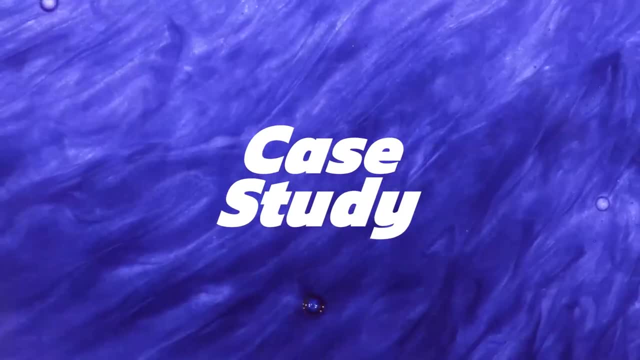 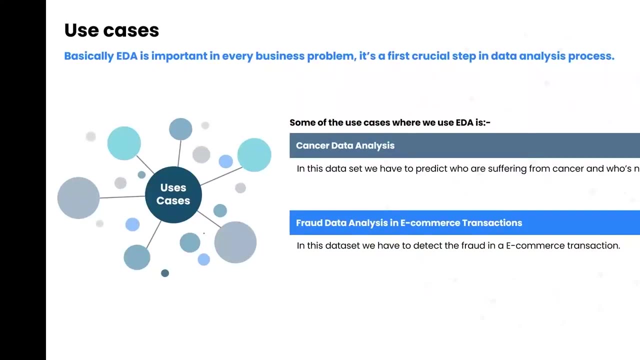 talking about the use cases for eda. basically, eda is important in every business problem. it's a first crucial step in data analysis process. we all know it all starts with business problem statement understanding, then data understanding, data collection, data preparation and then eda. following to eda we have our predictive model building and deployment. 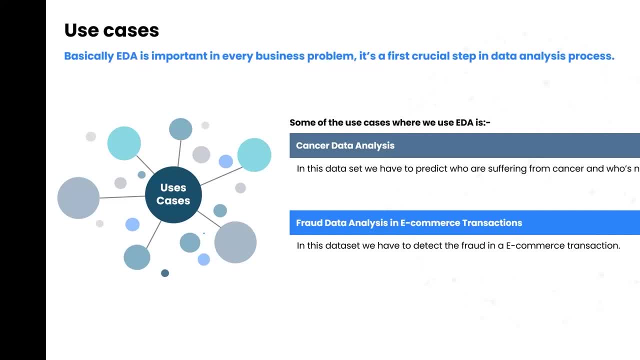 so if your final use case or your end goal is building a predictive model, even if your final goal is not to build a predictive model, in either of these cases, eda is equally vital. eda is one of these areas, one of these topics, one of these concepts. that's going to be very 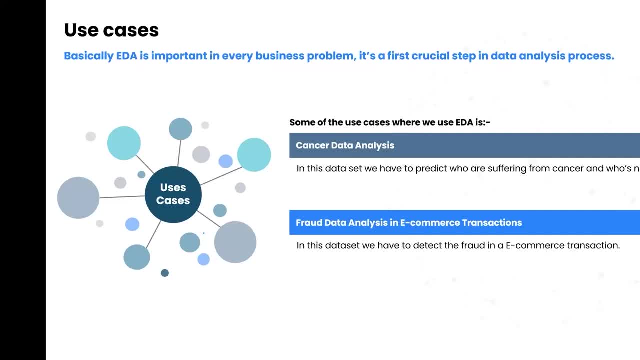 important for you and that's why we are going to talk about eda這些 entities. so eda is going to be very, very important for you and that's why we are going to talk about eda. so mandatory for a data analyst and for a data scientist on which data sets, on which use cases. 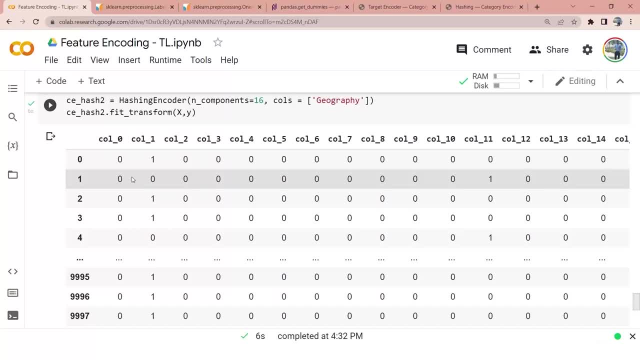 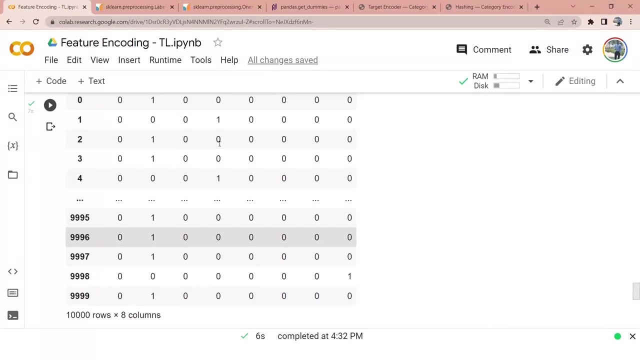 encoding techniques, and this technique is definitely mandatory when it comes to predictive analytics. so you can see on the screen you have 16 columns and these are hashed columns that has been created using some hashing technique. so that's all about different feature encoding techniques. i hope you understood the concepts behind it. in the next video we shall be jumping. 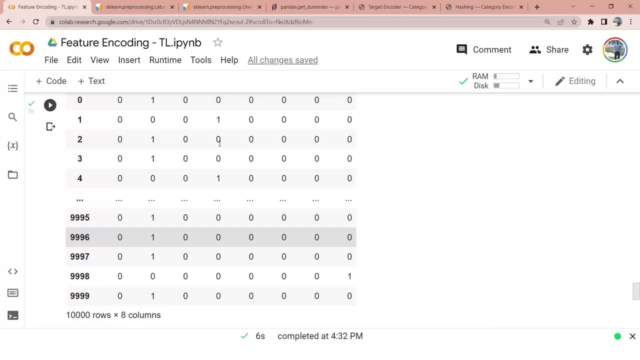 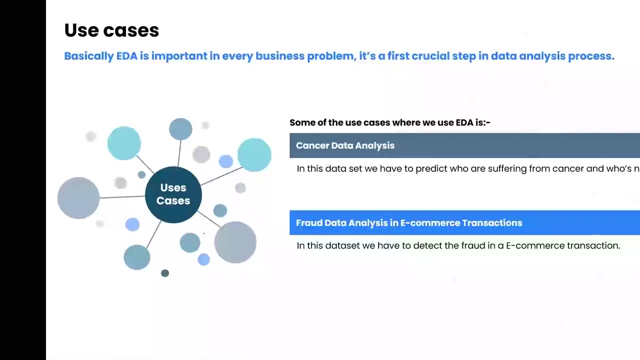 into the use case, the case study, where we will be taking example of a live data set or one of the public data sets and we will be performing eda step by step, you and finally analyzing the insights that we will get from the data set. talking about the use cases for eda: basically, eda is important in every business problem. 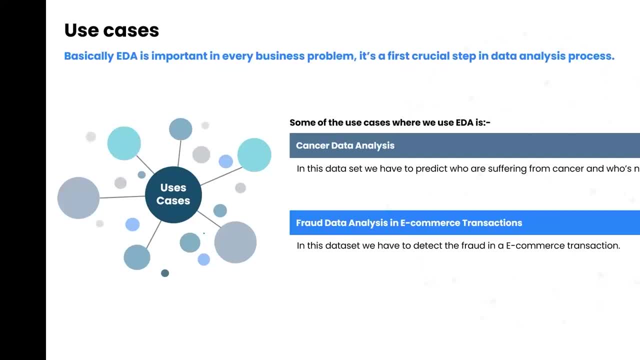 it's a first crucial step in data analysis process. we all know it all starts with business problem statement understanding, then data understanding, data collection, data preparation and then eda. following to eda, we have our predictive model building and deployment. so if your final use case or your end goal is building a predictive model, 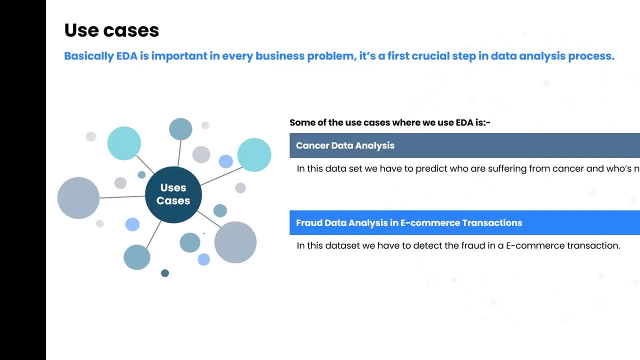 even if your final goal is not to build a predictive model. in either of these cases, eda is equally vital. eda is one of these areas, one of these topics, one of these concepts that's going to be very, very mandatory for a data analyst and for a data scientist on which data sets, on which use. 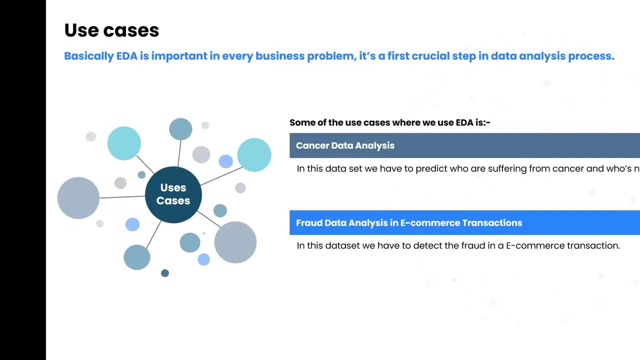 cases, you can perform eda. you can perform eda on each and every data set, on each and every case study, on each and every domain. eda is vast. you pick a domain, you pick a use case. eda is going to be important because eda is simply nothing but exploratory data analysis in. in simple terms, it's 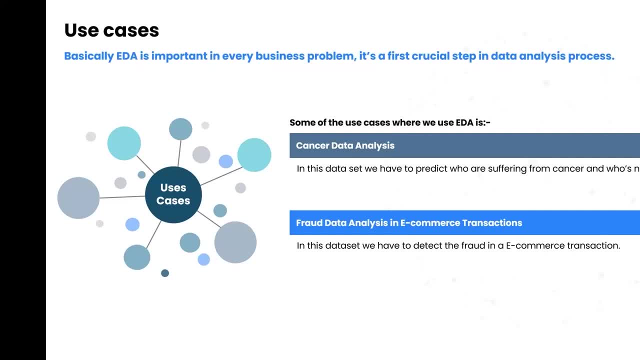 initial data analysis. so some of the use cases where we use eda are cancer data analysis. in this data set we have to predict who are suffering from cancer and who's not. what is the characteristics of people who are suffering from cancer and vice versa. fraud data analysis in e-commerce. 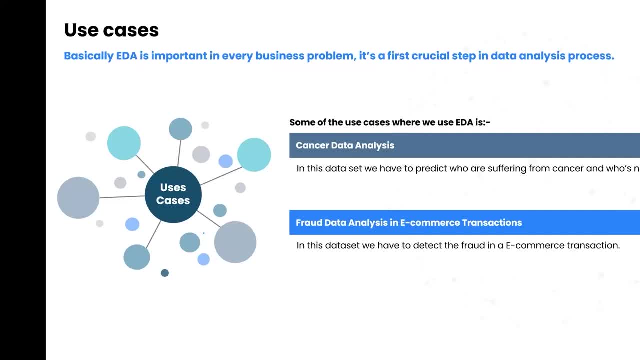 you can perform eda. you can perform eda on each and every data set, on each and every case study, on each and every domain. eda is vast. you pick a domain, you pick a use case. eda is going to be important because eda is simply nothing but exploratory data analysis in. in simple terms, 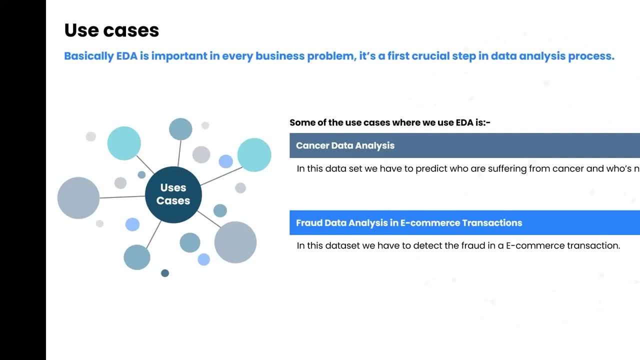 it's initial data analysis. so some of the use cases where we use eda are cancer data analysis. in this data set we have to predict who are suffering from cancer and who's not. what is the characteristics of people who are suffering from cancer and vice versa- fraud data. 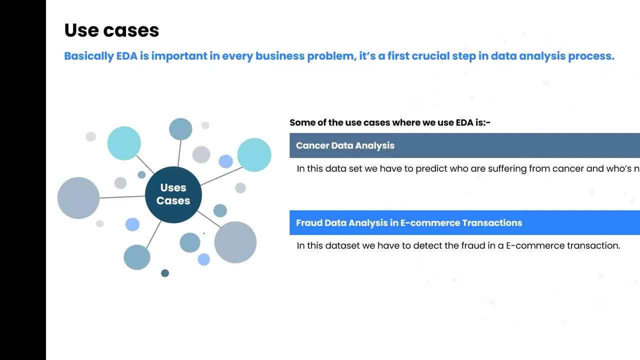 analysis in e-commerce, banking, financial- any areas- fraud data analytics. in these data sets we have to detect the fraud in a e-commerce transaction or in a banking transaction or in a generic cyber security world. any domain related to fraud analytics is going to be important as well. customer churn prediction: customer churn. 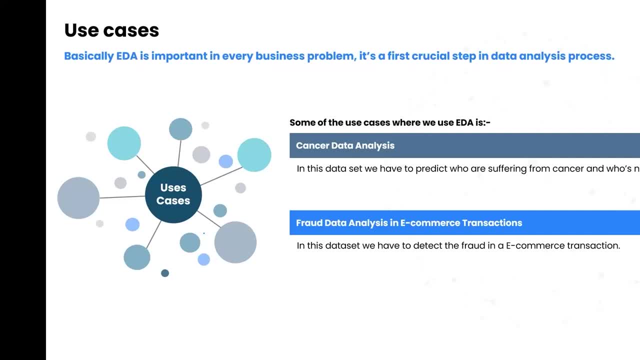 analysis, bank fraud analysis, customer segmentation, market segmentation. so there are so many use cases in this world in which eda is going to be important and we are going to talk about one of these use cases in video. theoretically, we will try to understand the use case. we will try to understand. 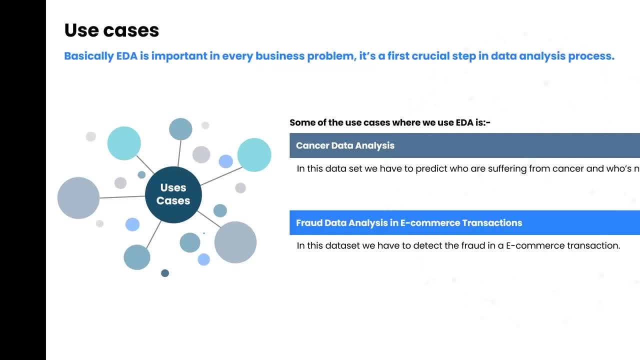 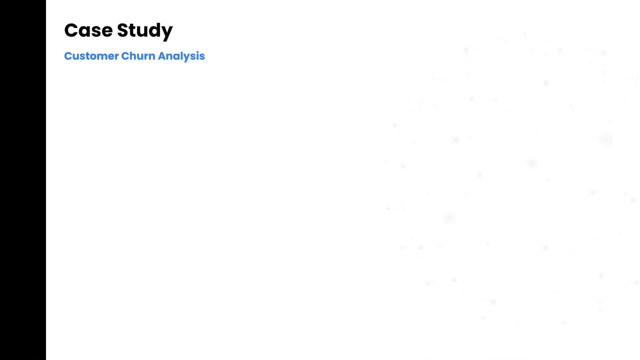 the business problem and then we will jump into the practical spot where we will be using a basic public data set and we will be performing the eda activities and, finally, we will come across with multiple insights from the data. so the use case that we are going to discuss. 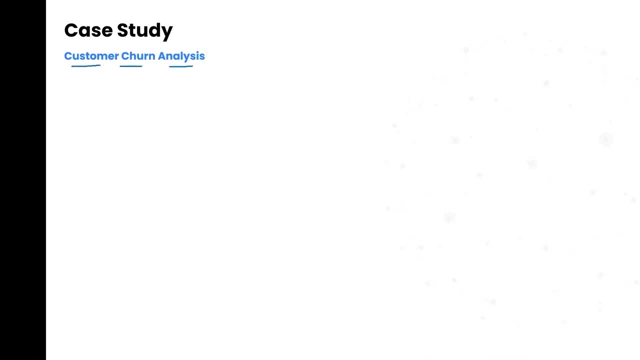 is customer churn analysis. it's one of the use cases that could be applicable in any domain: telecom, banking, financial, hr, gaming, any, any domain. you just pick a domain- customer churn analysis- one of those classic examples that can be related to any domain. let's try to understand. 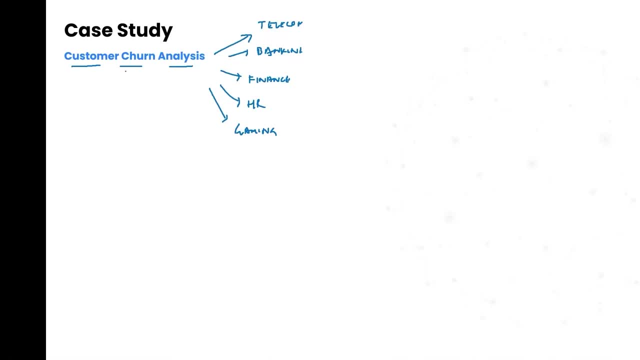 what exactly is customer churn, and then i'll try to give examples on each of these domains so that you can relate with the case study, and once we jump into the practicals part, it will be more clear on how do we perform analysis in python and we come across the insights. churn simply means: 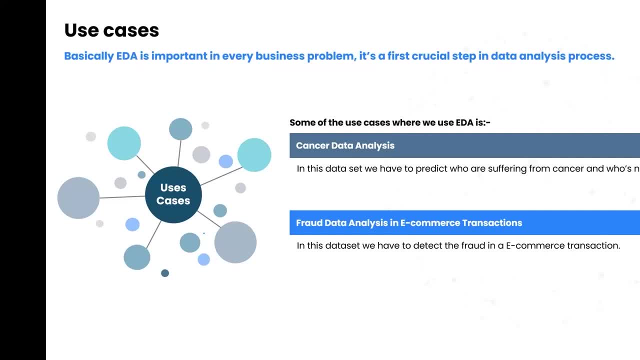 banking, financial- any areas- fraud data analytics. in these data sets we have to detect the fraud in a e-commerce transaction or in a banking transaction or in a generic cyber security world. any domain related to fraud analytics is going to be important as well. customer churn prediction, customer churn analysis, bank fraud analysis, customer segmentation, market segmentation. 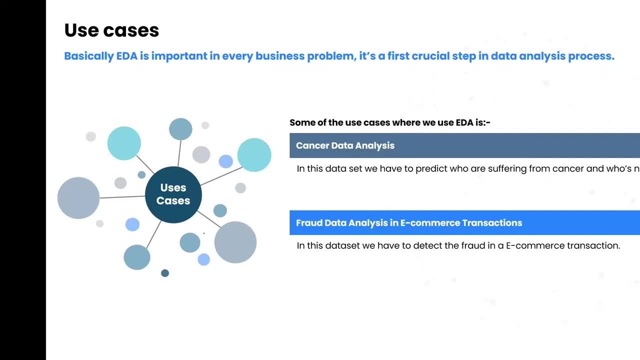 so there are so many use cases in this world in which eda is going to be important and we are going to talk about. one of these use cases is in the following video. theoretically, we will try to understand the use case, we'll try to understand the business problem and then we will jump into the practical spot where we will be. 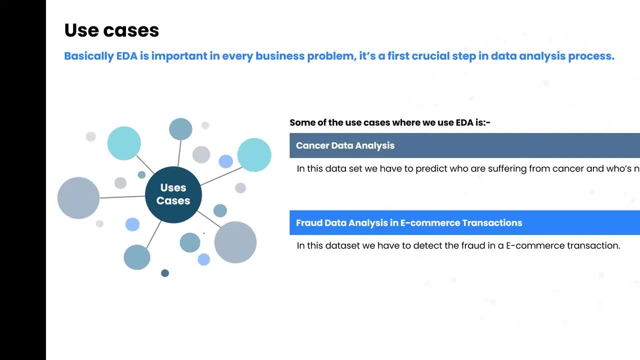 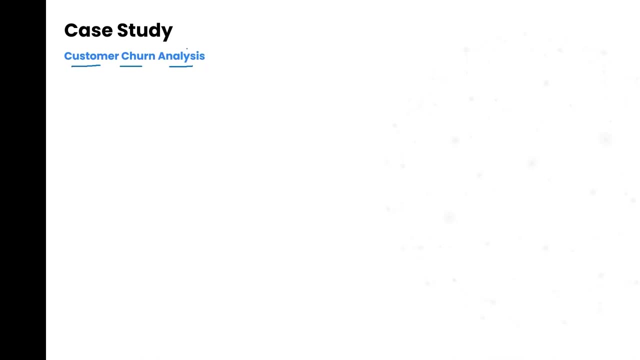 using a basic public data set and we will be performing the eda activities and finally, we'll come across with multiple insights from the data. so the use case that we are going to discuss is customer churn analysis. it's one of the use cases that could be. 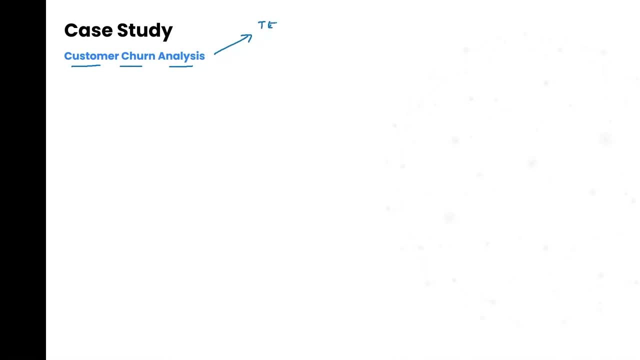 applicable in any domain: telecom, banking, financial hr, gaming, any, any domain. you just pick a domain: customer churn analysis- one of those classic examples that can be related to any domain. let's try to understand what exactly is customer churn and then i'll try to give examples on each of these domains so that you can relate. 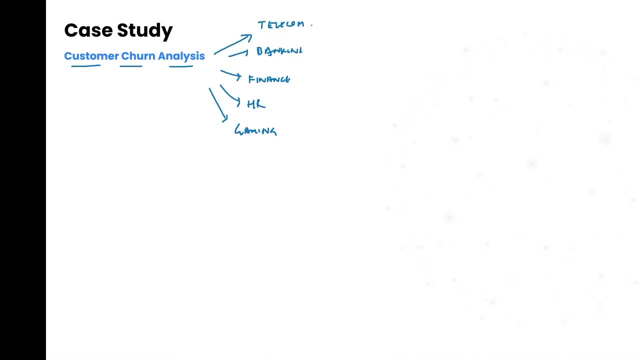 with the case study and once we jump into the practicals part it will be more clear on how do we perform analysis in python and we come across the insights. churn simply means if somebody leaves a company or its organization, so customer churn. so churn basically means simply you have to get rid of that, or probably you just churn out or you just 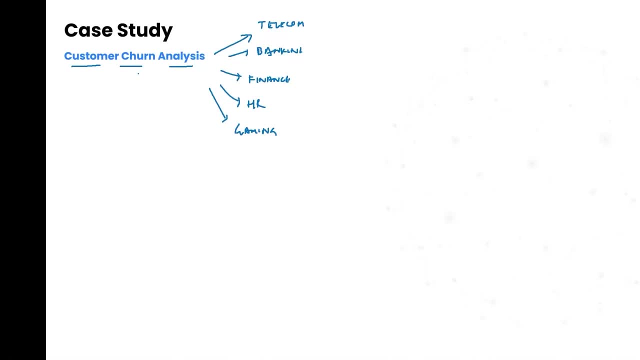 if somebody leaves a company or its organization, so customer churn. so churn basically means you have to get rid of that, or probably you just churn out or you just stop doing business with the company. customer churn analysis simply is that kind of analysis where a customer is getting churned or not churned. now customers leave companies. right with respect to telecom. 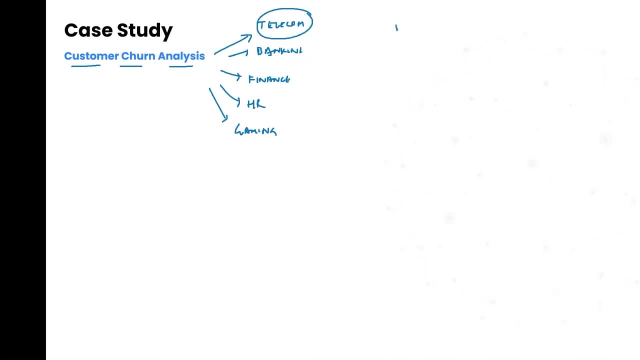 let's say we have a telecom provider called as vodafone and probably- i'm not sure if you are familiar with vodafone, but if you are familiar with vodafone then you might be familiar with vodafone. but if you are familiar with vodafone, then you might be familiar with vodafone and probably similar kind of analysis is done. 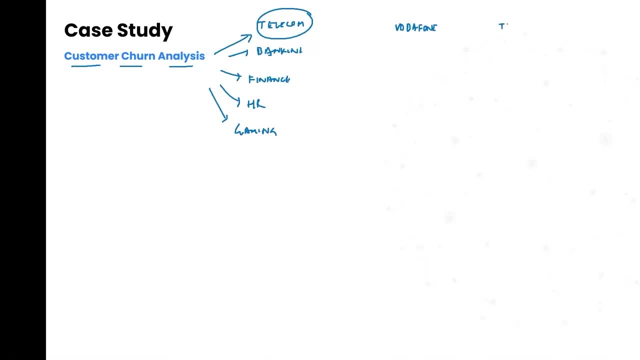 already i can see another telecom provider which is: it could be anything. you can take an example like telecomcell or xcis walk-in system or globe telecom cake. you can take an example like telecom cell, any kind of telecom examples with respect to your country, and you will probably be able. 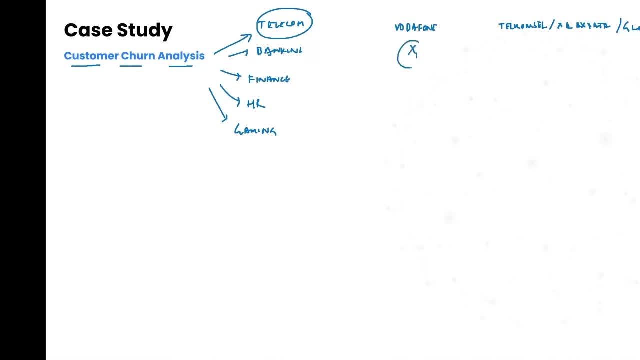 to visualize what i'm talking about. so just imagine we have a company x1 and a company x2. so let's imagine we have a company x1 and a company x2. so let's explain what is this company that is operating on this model. so with a company, the один or human, Angela telecom is actually a single session or personal. 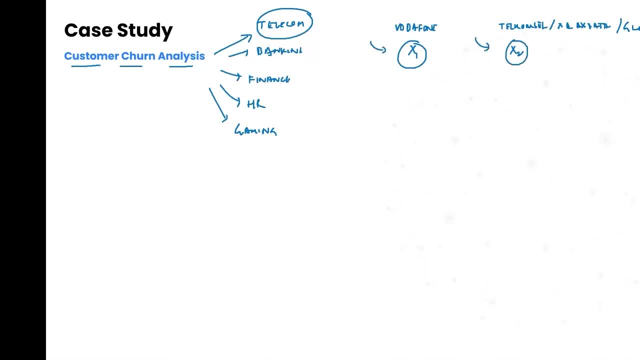 both these companies are telecom providers. they provide you telecom services. they provide you prepaid services and postpaid services. right now, imagine you are a customer of company x1. your monthly usage is you. you probably use 2 to 3 gb of data and you do probably like 50 to 100. calls in a month and for these kind of services, let's say, you pay 10 dollars a month. if another company comes in and they start providing you the same services at five dollars per month, definitely there will be a certain chunk of people who will leave. x1. 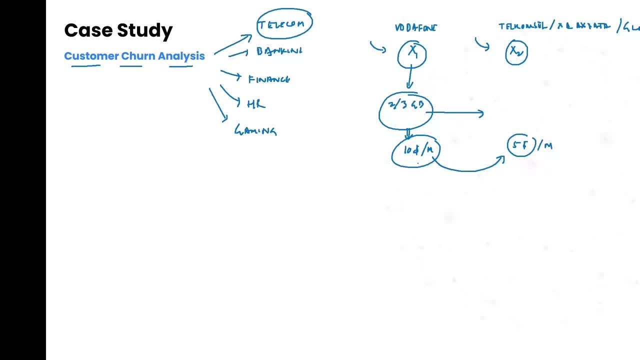 and probably join x2. so if these set of users are leaving x1 and they start providing you the same services, they will probably leave x1 and probably join x2. so if these set of users are leaving x1 and so if these set of users are leaving x1 and 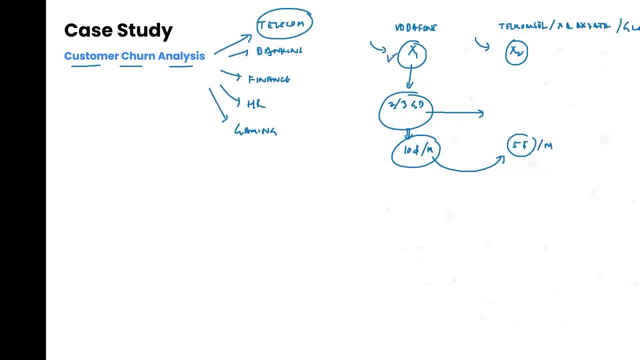 are joining x2, that means it's a loss to this company. so if you are hired as a data analyst or as a data scientist in this company, your main task will be to understand this pattern, to understand what are the characteristics of the people who are leaving the company. are they living? 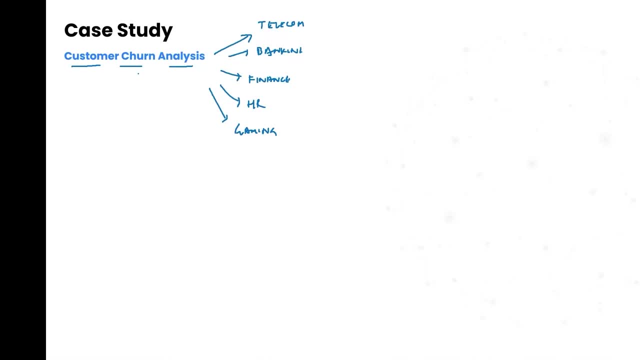 stop doing business with the company. customer churn analysis simply is that kind of analysis where a customer is getting churned or not churned. now customers leave companies right. with respect to telecom, let's say we have a telecom provider called as vodafone and probably another telecom provider which is it could be anything. you can take an example like: 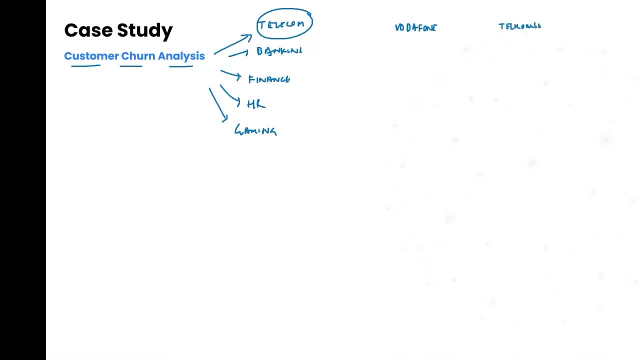 telecom, cell or excel, axiata or globe telecom, any, any kind of telecom examples with respect to your country, and you'll probably be able to visualize what i am talking about. so just imagine we have a company x1 and a company x2, so both these companies are telecom providers. they provide you telecom services. they provide 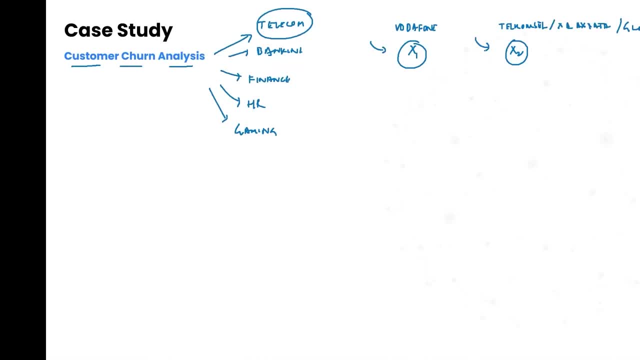 you prepaid services and postpaid services. right now, imagine you are a customer of company x1. your monthly usage is you, you probably use two to three gb of data and you do probably like 50 to 100 calls in a month and for these kind of services. 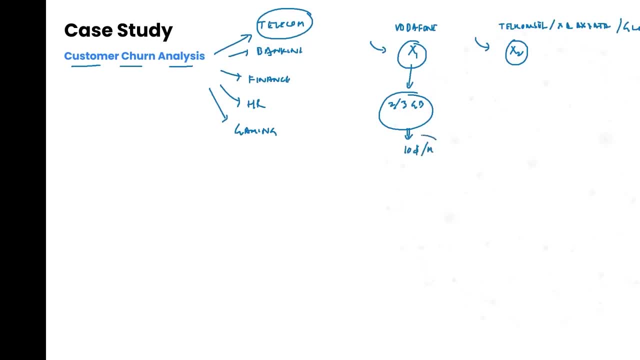 let's say you pay ten dollars a month. if another company comes in and they start providing you the same services at five dollars per month, definitely there will be a certain chunk of people who will leave x1 and probably join x2. so if these set of users are leaving x1 and are joining x2, that means it's a loss to this. 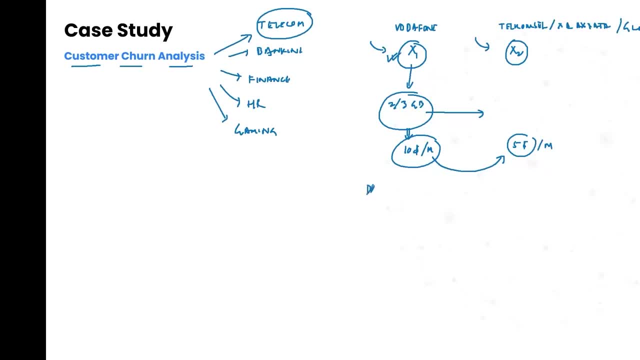 company. so if you are hired as a data analyst or as a data scientist in this company, your main task will be to understand this pattern, to understand what are the characteristics of the people who are leaving the company. are they living because of some offers like this or are they living because? 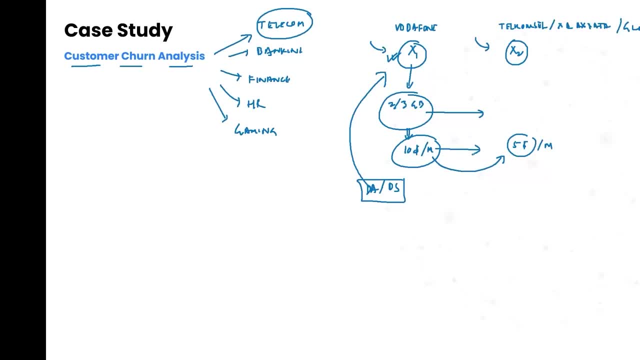 because of some offers like this, or are they leaving because of some service impact, or else right, so there are multiple reasons why a user leave a company and join another company. one reason is this. one reason is probably a customer is genuinely irritated with the service wherever he goes. maybe he's a hiker- he goes for mountain hikings. 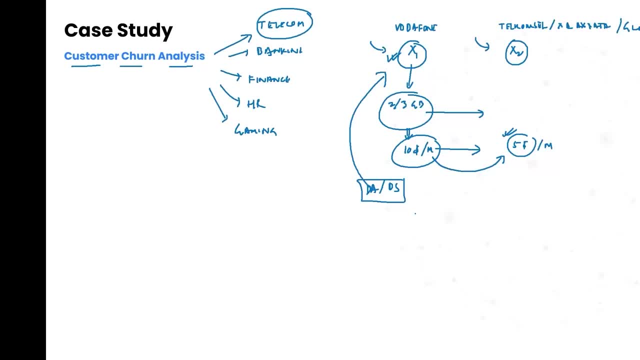 and wherever he goes for hiking he's unable to call anybody because of the bad network. so definitely he will get pissed off and probably churn out and he will probably join x2 or x3 or any any of their competitors. that means that particular customer is churning. 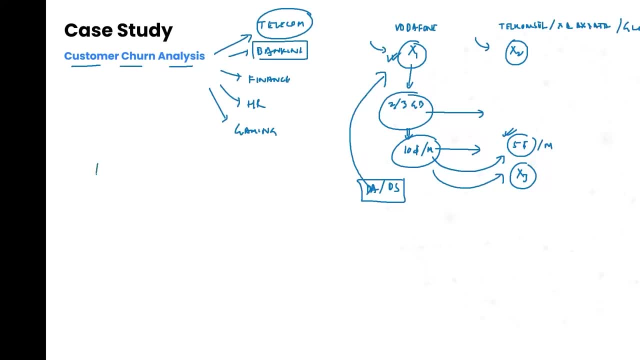 similarly with respect to banking. imagine you are currently an hsbc user. you are using hsbc bank account for all your transactions, for your, you know, for your salary and all those things you are doing, some freelancing work, every kind of transactions you are using hsbc. or simply, let's. 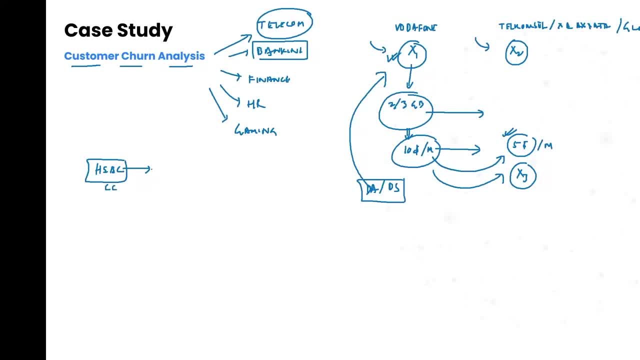 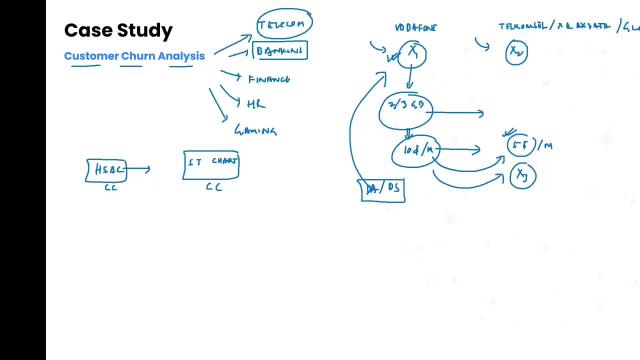 other credit card holders. there will be certain amount of people who will start using standard chatter and with due course of time their usage with hsbc will decline. now that is again a churn scenario. a customer is getting churned from hsbc to standard checker. talking about hr, many people leave companies. today you are working for amazon. after one year. probably you have some fight with your manager or probably you are not getting that much of salary that you are expecting and you got an offer from google at a double play or double pay. you will turn so again. multiple reasons why people churn companies, maybe with because of better pay. 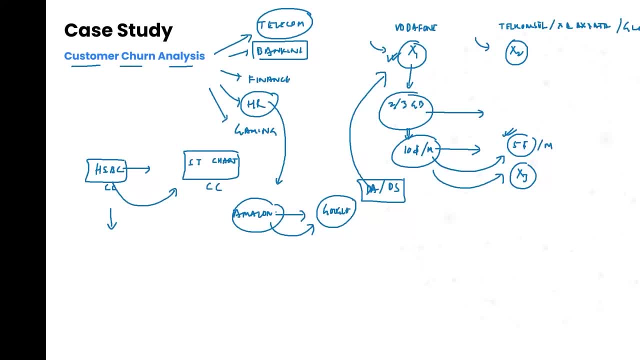 maybe because of location, maybe because of a bad manager, could be anything. talking about gaming industry. imagine you are playing a game. let's say i will name it as game one. you started playing this game. after five to seven days you almost reached 100 levels. you see that the game is still. 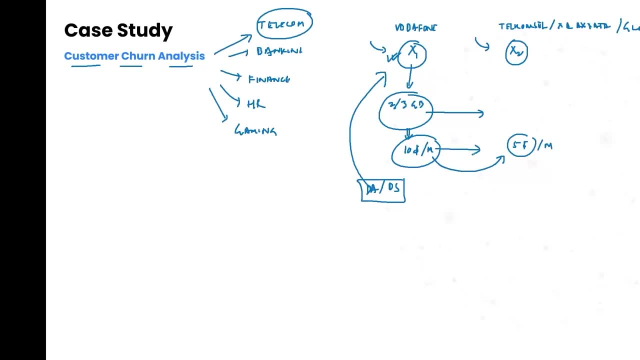 of some service impact or anything else. right, so there are multiple reasons why a user leave a company and join another company. one reason is this. one reason is probably a customer is genuinely irritated with the service wherever he goes. maybe he is a hiker- he goes for mountain hikings. 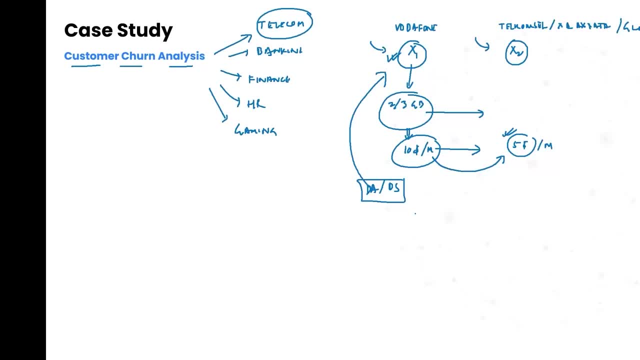 and wherever he goes for hiking, he is unable to call anybody because of the bad network. so definitely he will get pissed off and probably churn out and he will probably join x2 or x3 or any any of their competitors. that means that particular customer is churning. 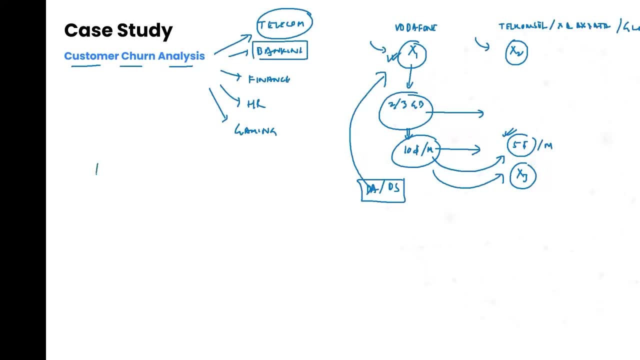 similarly with respect to banking. imagine you are currently an hsbc user. you are using hsbc bank account for all your transactions, for your, you know, for your salary and all those things you are doing, some freelancing work- every kind of transactions. you are using hsbc. 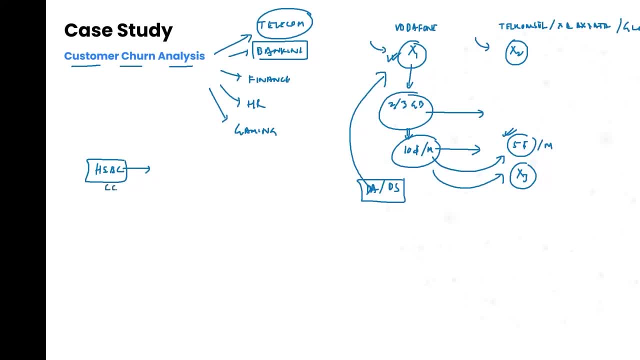 or simply, let's talk about hsbc credit card. you are using hsbc credit card now standard chattered. comes with a plan with a better plan. they come with a credit card better plan that if you start using their credit card, you will get twice or thrice more points, as 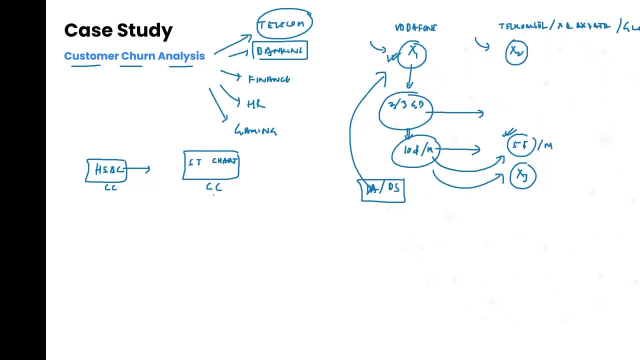 compared to hsbc or any other credit card holders. there will be certain amount of people who will start using standard chatter and with due course of time their usage with hsbc will decline. that is again a churn scenario. a customer is getting churned from hsbc to standard chapter. 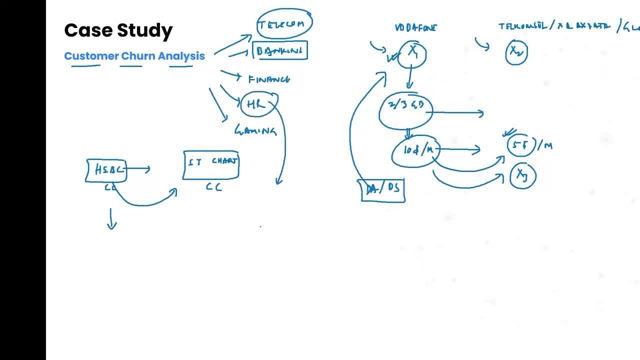 talking about hr. many people leave companies. today you are working for amazon after one year. probably you have some fight with your manager or probably you are not getting that much of salary that you are expecting and you got an offer from google at a double play or double pay. you will churn. 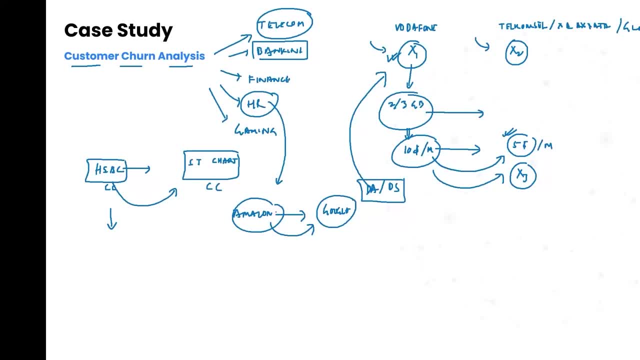 so again, multiple reasons why people churn companies, maybe with because of better pay, maybe because of location, maybe because of a bad manager, could be anything. talking about gaming industry, imagine you are playing a game. let's say i will name it as game one. you started playing this game. after five to seven days you almost reached 100 levels. you see that the game is too. 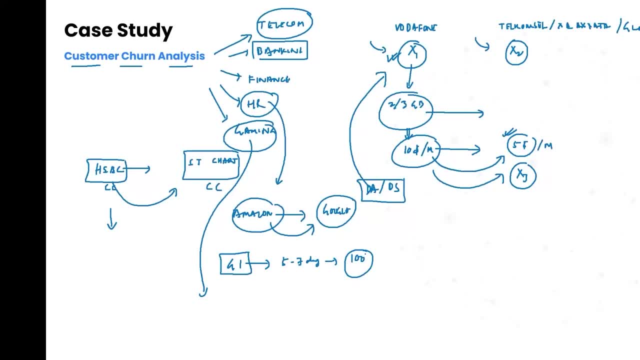 too easy. with just one attempt you are able to clear all the rounds. so at certain point of time you will feel bored and you will churn out and you will start install, installing another game and probably uninstall g1. so g1 will be uninstalled, probably will install g2 or else. 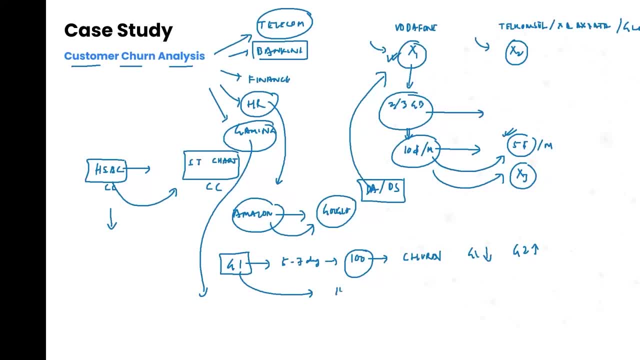 you started playing this game. for five, seven days you are stuck at level 142. you are stuck for the last two days or three days. you get pissed off and you churn because the game is too hard. so any kind of use case, any kind of industry, there will be a certain amount of customers. those will 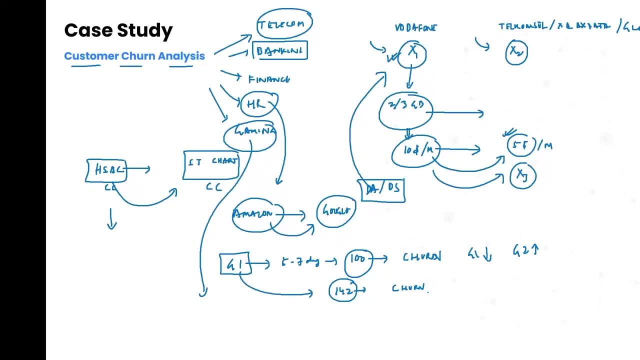 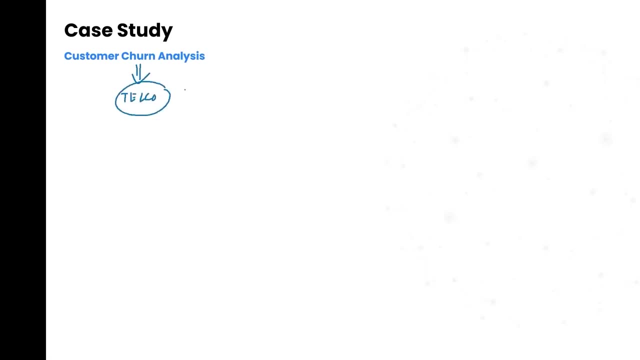 be churning. so churn is one of those common use cases that usually happens in any kind of industry. in this particular video, we will be focusing more on the telecom churn, so we'll talk about telco churn in simple terms. telco is nothing but telecom. right now, theoretically, i will explain you all. 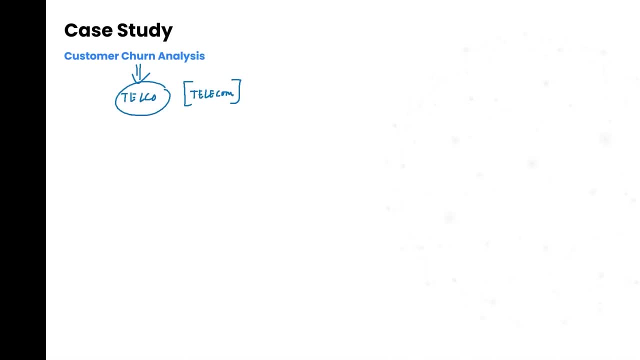 the things and once we jump into the practicals part anyways, we will be having a detailed step by step process. so the use case is very clear. there are. we have a data set- let's say ten thousand, twenty thousand- records certain amount of people that have churned, let's say two thousand. 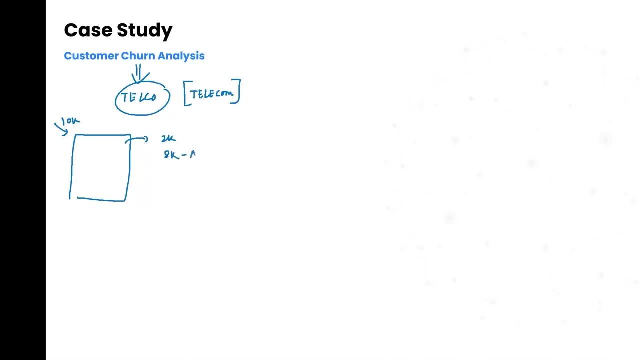 and let's say, eight thousand people are active and of course, there is a column, let's say exited, and this column is telling you about this thing: churned active, churned active, and so on, and there are multiple other columns. what is your? what is your final goal? 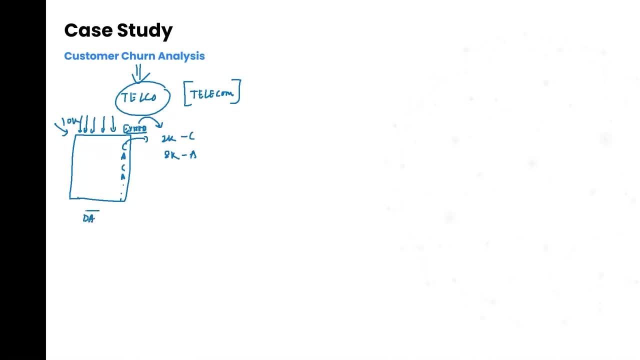 when you receive a data like this, you are working as a data analyst for that company. your task is to perform ada- initial data analysis, or exploratory data analysis- and as part of ada, you should come with insights. that talks more about the churned customers. that means you need to come up with 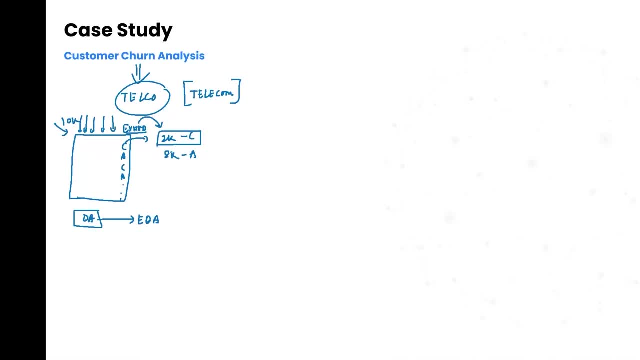 features or you need to come up with some insights: that is triggering or causing the churn and what is the potential characteristics of those people? let's say, out of those 2000 people, you got to know that 1800 of them are females. now, that's an important insight. most of the people who 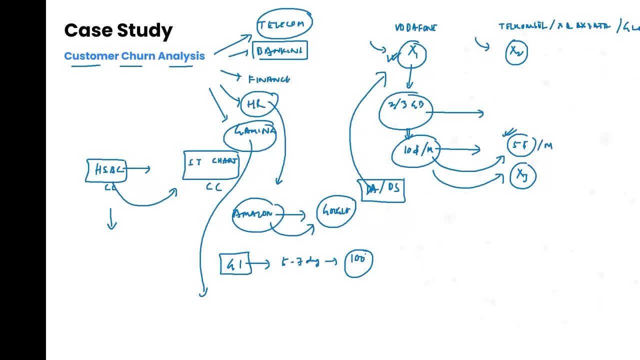 easy. you start playing this game. after five to seven days you almost reached 100 levels. you see that the game is too easy. with just one attempt you are able to clear all the rounds. so at certain point of time you will feel bored and you will churn out and you will start install, installing another game, and probably 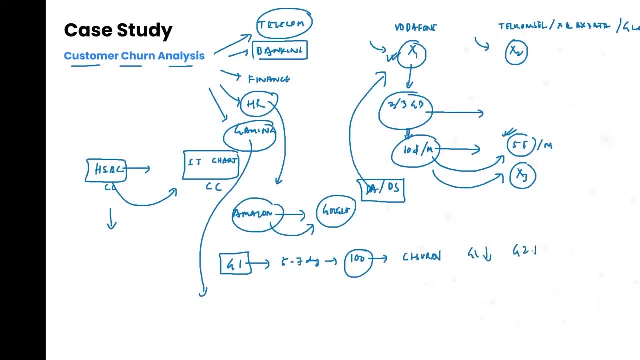 uninstall g1. so g1 will be uninstalled, probably will install g2. or else you started playing this game for five, seven days. you are stuck at level 142. you are stuck for the last two days or three days. you are stuck at level 142 for the last two days or three days. you get pissed off and you churned. 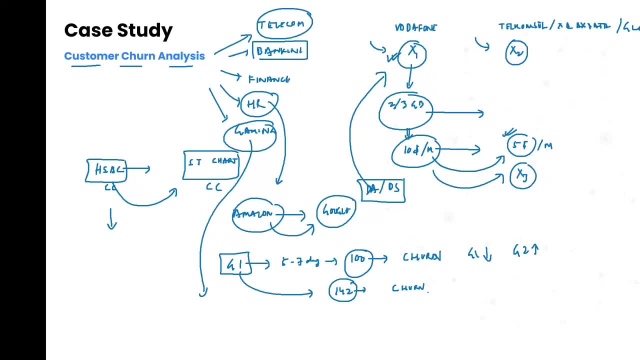 because the game is too hard. so any kind of use case, any kind of industry, there will be a certain amount of customers. those will be churning. so churn is one of those common use cases that usually happens in any kind of industry. in this particular video we will be focusing more. 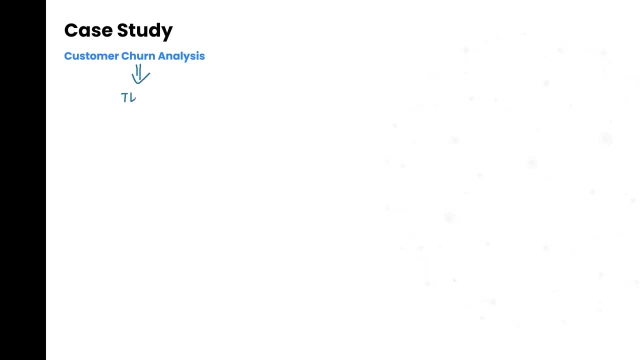 on the telecom churn. so we'll talk about telco churn in simple terms. telco is nothing but telecom. right now, theoretically, i will explain you all the things, and once we jump into the practicals part, anyways, we will be having a detailed step-by-step process. 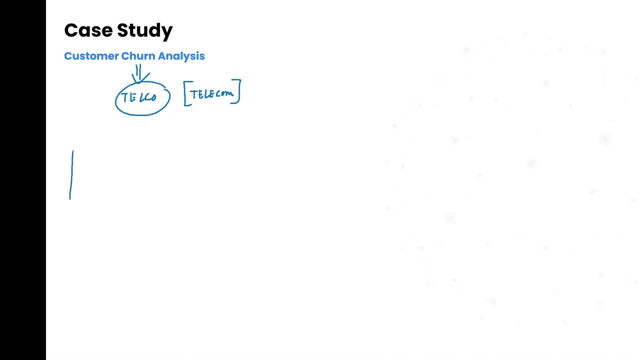 so the use case is very clear. there are, we have a data set- let's say 10, 000, 20 000- records certain amount of people that have churned, let's say 2000 and let's say 8000 people are active. and of course there is a column, let's say exited, and this column is telling you about this thing. 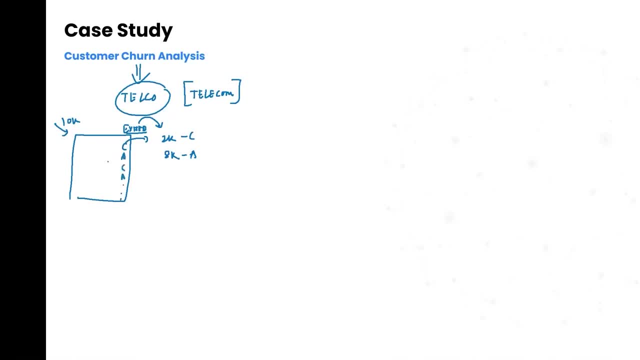 churned active, churned active and so on, and there are multiple other columns. what is your, what is your final goal when you receive a data like this? you are working as a data analyst for that company. your task is to perform ada- initial data analysis, or exploratory data analysis- and as part of ada, you should come with insights. 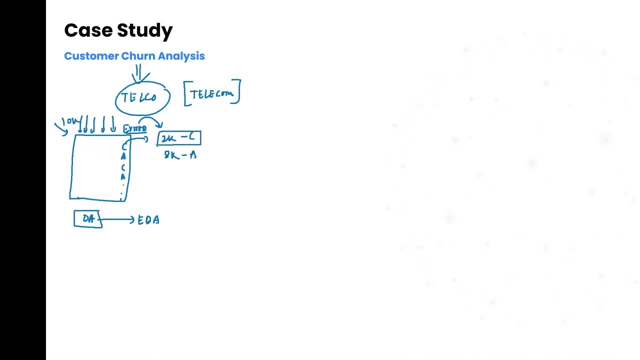 that talks more about the churned customers. that means you need to come up with features or you need to come up with some insights: that is triggering or causing the churn and what is the potential characteristics of those people. let's say, out of those 2000 people, you got to know that 1800 of them are females. now that's. 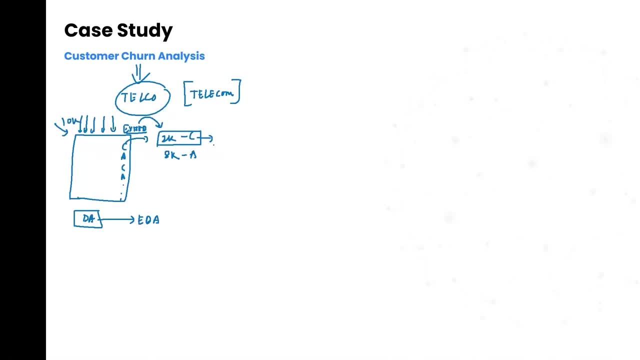 an important insight. most of the people who are females are churning more, or maybe out of those 1800, probably 1600 of them are from a specific location. that means from that specific location. there could be a problem in that location. that's why people are churning right. so you come up with. 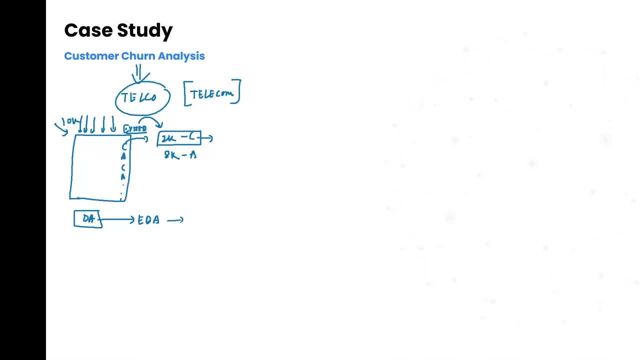 insights and your ultimate goal after eda is to showcase the reports, showcase the insights to your higher management or to your customers and, once they go through them, if that is convincing, your final goal is going to be creating a predictive model which will be able to predict. 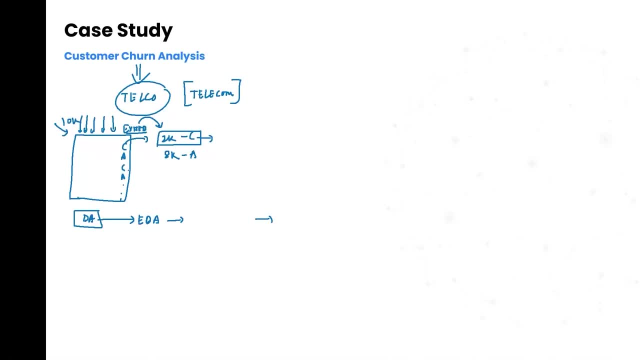 for a new customer, whether that customer will be churned or not churned. that is the entire customer churn analysis and prediction use case. in the practical session we will be using a data set like this. so the steps that we will perform is. the first step we will perform is, of course, we will be checking all the we will be doing data. 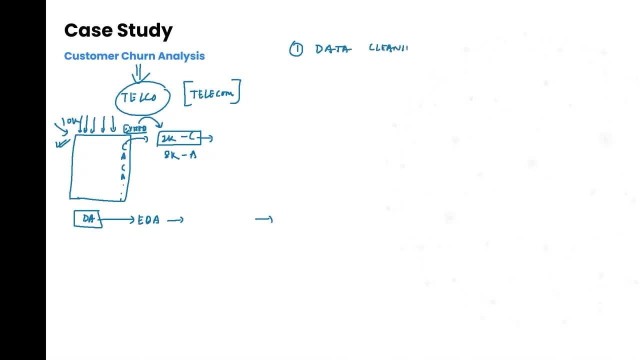 cleaning and data cleaning. definitely it's a one-step process, in eda especially. but when it comes to predictive model part, you could, you know data cleaning could be an iterative process. you could perform some cleaning activity, create your model. if your model performance is good, fine. if it is not good, you can again come back and do another way of data cleaning, right, but especially 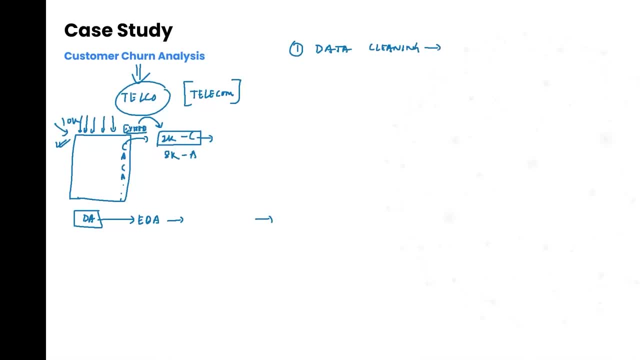 for eda. there is nothing right, nothing wrong. in the data cleaning part. inside data cleaning, we will be handling all the null values. wherever we see null values, we will be handling them. null values occurs because of multiple reasons. right, it could be because of your script, because the null values are actually there in the database, or 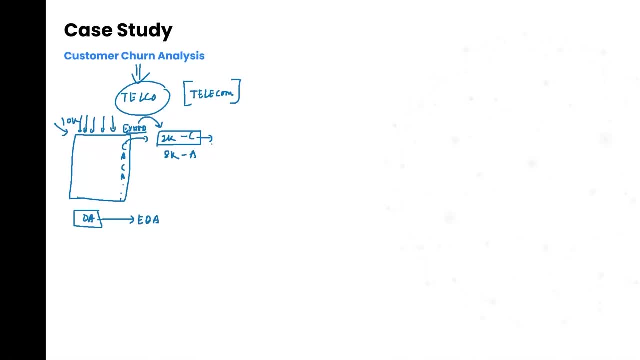 are females are churning more. or maybe out of those 1800, probably 1600 of them are from a specific location. that means from that specific location. there could be a problem in that location. that's why people are churning right. so you come up. 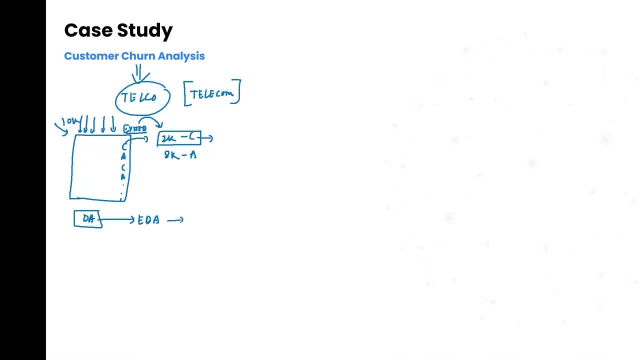 with insights, and your ultimate goal after EDA is to showcase the reports, showcase the insights to your higher management or to your customers and, once they go through them, if that is convincing, your final goal is going to be creating a predictive model which will be able to predict for a new 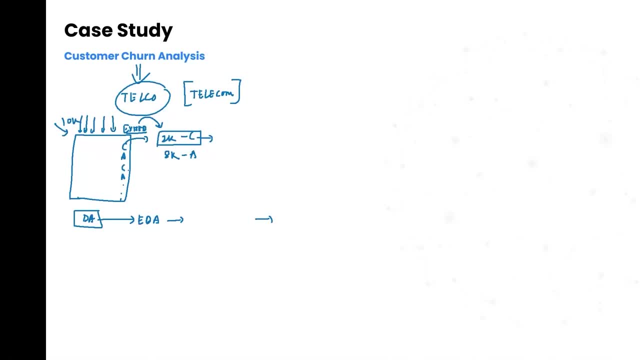 customer, whether that customer will be churned or not churned. that is the entire customer churn analysis and prediction use case. in the practical session we will be using a data set like this. so the steps that we will perform is the first step we will perform is, of course, we will be. 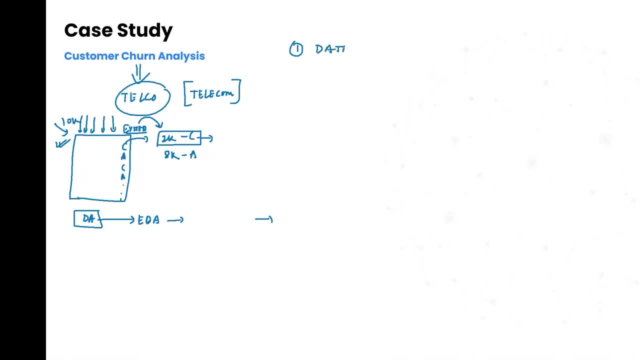 checking all the we will be doing data cleaning and data cleaning. definitely it's a one-step process, in EDA especially, but when it comes to predictive model part, you could. you know data cleaning could be an iterative process. you could perform some cleaning activity, create your model, if your. 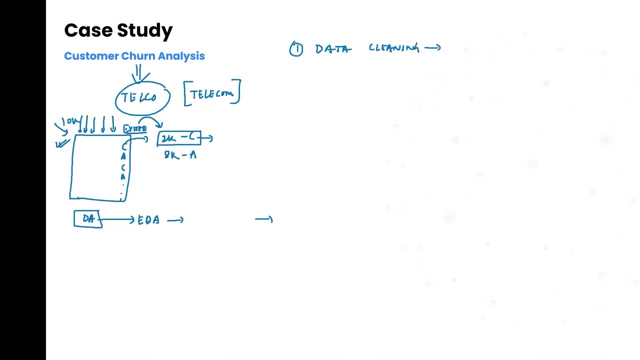 model performance is good, fine. if it is not good, you can again come back and do another way of data cleaning. right, but especially for EDA, there is nothing right, nothing wrong in the data cleaning part. inside data cleaning, we will be handling all the null value. wherever we see null values, we will be handling. 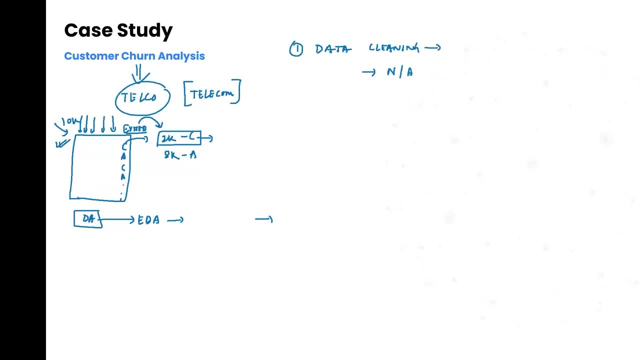 them. null values occurs because of multiple reasons. right, it could be because of your script, because the null values are actually there in the database, or it could be anything, but you have to deal with it. so we all know how to deal with null values. the simplest technique is mm, which is mean median mode. right, for numerical data it could be mean, and. 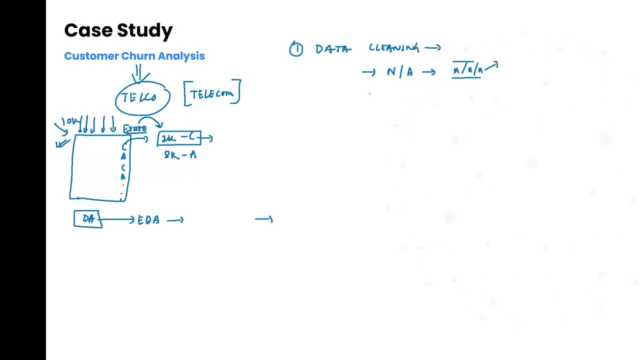 median for categorical data. it will be mode after null value imputation. we also go ahead and do some other checks for invalid data type. we also do some outlier treatment or kind of check outliers, whether our data has outliers or not. once all this cleaning process is done, then we start with our 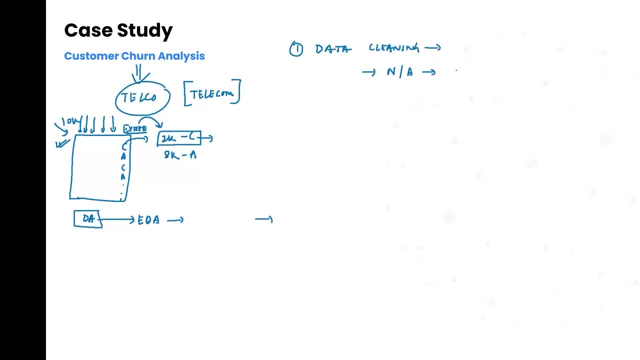 it could be anything, but you have to deal with it. so we all know how to deal with null values. the simplest technique is mm, which is mean median mode. right for numerical data it could be mean and median for categorical data. it will be mode after null value imputation. we also go ahead and do some. 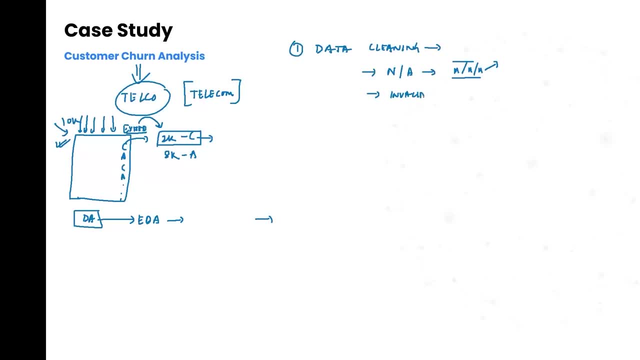 other checks for invalid data type. we also do some outlier treatment or kind of check outliers, whether our data has outliers or not. once all this cleaning process is done, then we start with our analysis. again, analysis is split into multiple things. first we try to do the categorical analysis. 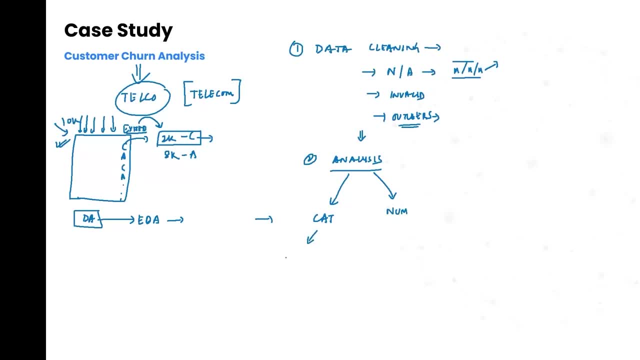 and then we do numerical analysis. in categorical analysis we mostly do the univariate, bivariate. if time permits we also do multivariate, but multivariate could be very much time consuming. so it all depends. if you have time, you can do it. and when it comes to numerical analysis again, 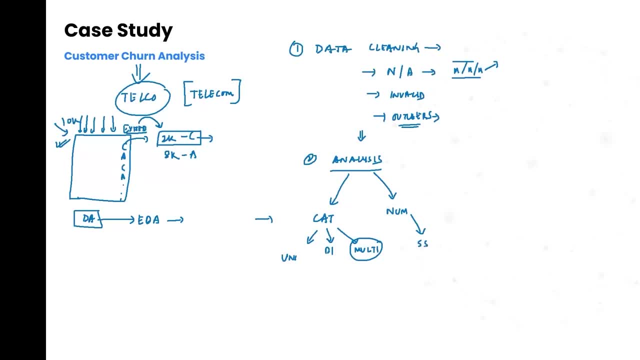 with one numerical attribute we'll probably get some summary statistics, and with multiple numerical attributes we probably go through their correlation and all those kind of things where we check the relationship between various numerical attributes. then we check the relationship between all those kind of things where we check the relationship between various numerical attributes. 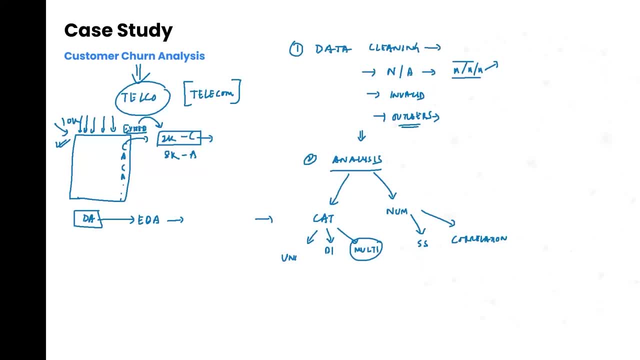 and also relationship between numerical attributes and the y variable, which is exited or not exited, how these numerical attributes are impacting them. right, all these things we do. now we'll quickly try to understand about univariate analysis: univariate. univariate simply means single variable, right? let's say you are talking about gender. you simply go ahead and check what is the 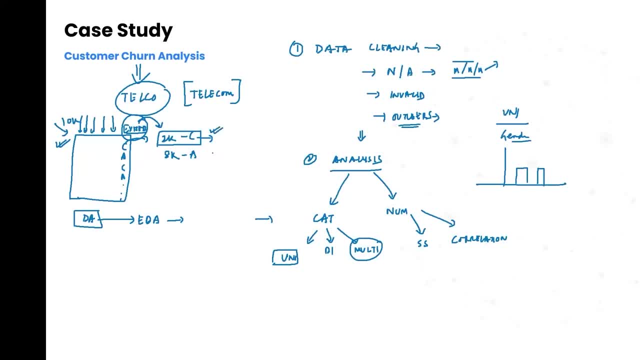 distribution. out of the two thousand, out of the ten thousand customers, let's say the distribution is almost even five thousand fifty and four thousand, uh, nine hundred and fifty, almost one is to one, and again you do the same thing for the churn customers. now let's say again, there is an 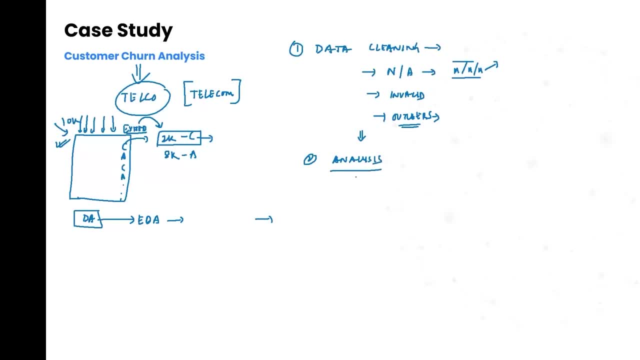 analysis. again, analysis is split into multiple things. first we try to do the categorical analysis and then we do numerical analysis. in categorical analysis we mostly do the univariate, bivariate. if time permits we also do multivariate, but multivariate could be very much time consuming. so it all depends: if you have time you can do it, and when it comes to 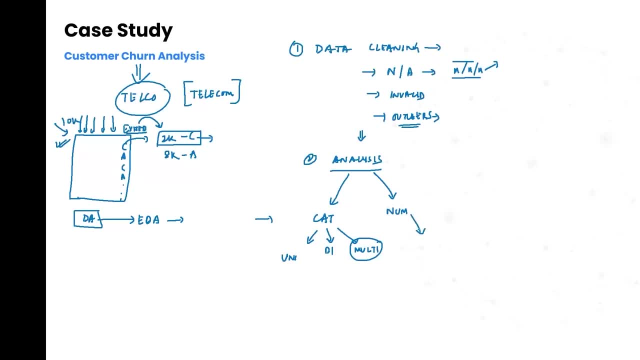 numerical analysis. again, with one numerical attribute we probably get some summary statistics, and with multiple numeric numerical attributes we probably go through their correlation and all those kind of things where we check the relationship between various numerical attributes and also relationship between numerical attributes and the y variable, which is exited or not exited, how these numerical attributes are impacting them. 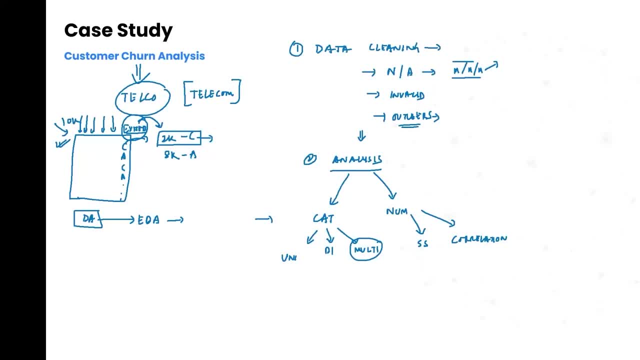 right, all these things we do. now we'll quickly try to understand about univariate analysis. univariate univariate simply means single variable, right? let's say you are talking about gender. you simply go ahead and check what is the distribution out of the two thousand, out of? 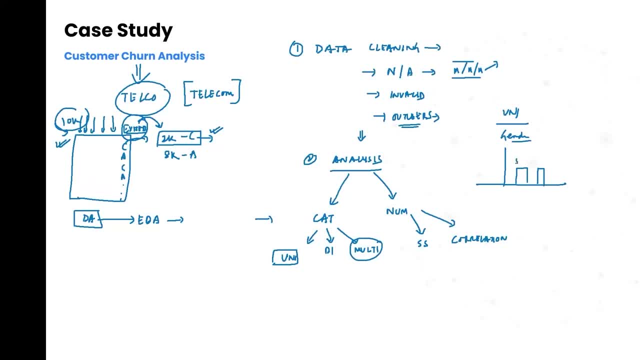 the ten thousand customers. let's say the distribution is almost even. five thousand fifty and four thousand, uh, nine hundred and fifty, almost one is to one. and again you do the same thing for the churn customers. now let's say, again, there is an even numbers or even ratio, almost one is to one. 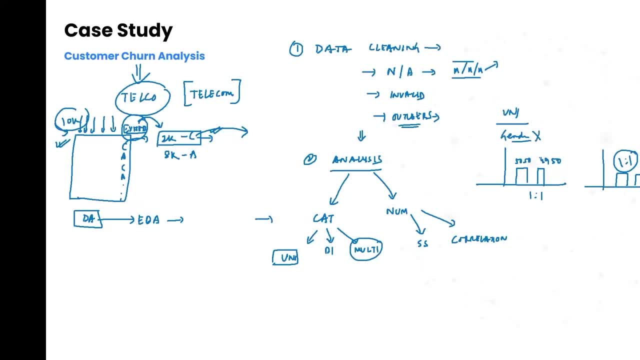 you find that gender is not univariate. you find that gender is not univariate, you find that gender is not that important from the univariate point of view. or else, if you come across a situation like this, probably you can end up telling that more males are likely to churn. 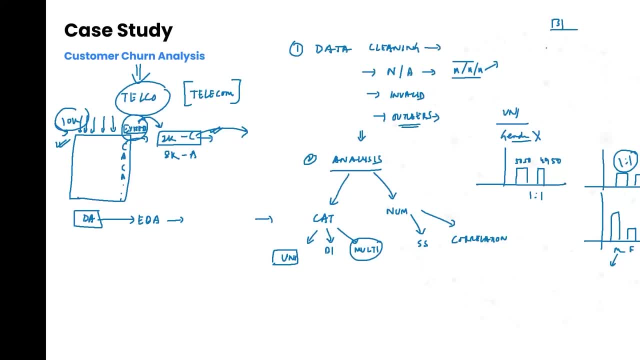 moving on to bivariate analysis, we combine another variable to it, let's say gender plus location. again you do the same thing: male, female. you check with multiple locations what is the ratio? and again you do it for the, only for the churn customers, and then you compare what is the original churn rate? it is 20. 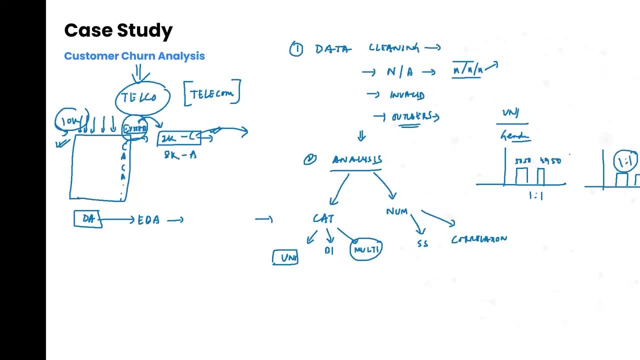 even numbers or even ratio. almost one is to one. you find that gender is not that important from the univariate point of view. you find that gender is not that important from the univariate point of view, or else, if you come across a situation like this, probably you can end up telling that more males 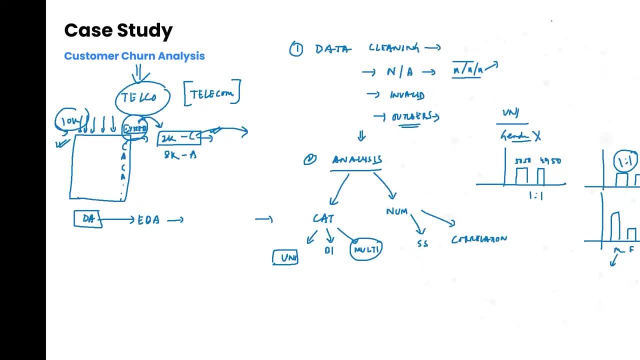 are likely to churn. moving on to bivariate analysis, we combine another variable to it, let's say gender plus location. again you do the same thing, male, female, you check with multiple locations. what is the ratio? and again you do it for the, only for the churn customers, and then you compare. 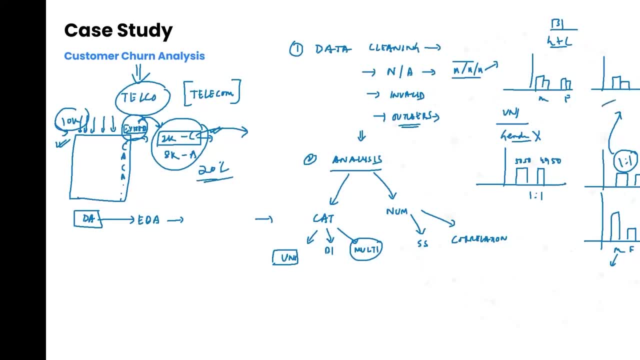 the churn rate. with the original churn rate it is 20 percent. what is the churn rate here? let's say, for male customers staying in france, the churn rate is 40, which means people, especially males, who are staying in france are more likely to churn. similarly, if you want, you can also perform. 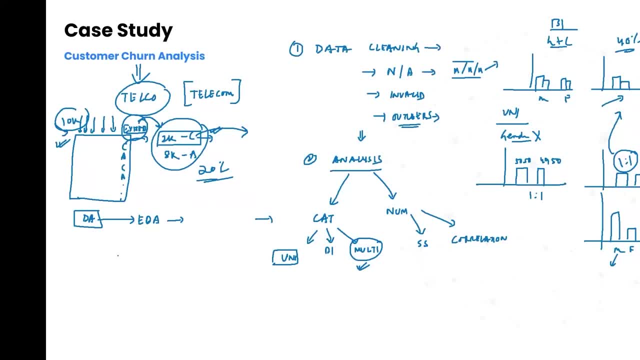 multivariate, which basically means you have to combine three or four variables together and start analyzing it. when we do numerical analysis for single numerical attributes like age tenure and all those things, we try to check their summary statistics. and with multiple numerical attributes we perform firstly, we try to check their, you know, if there are less amount of numerical values or numerical 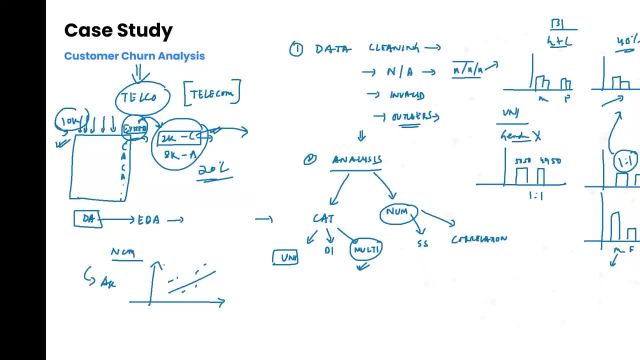 variables, you can simply draw scatter plots between them. if there are huge amount of numerical features, you can go for the correlation matrix- cor matrix- which tells you about each column versus each column's correlation value. right, so these are different analysis that we usually do. at some point of time we can also do: 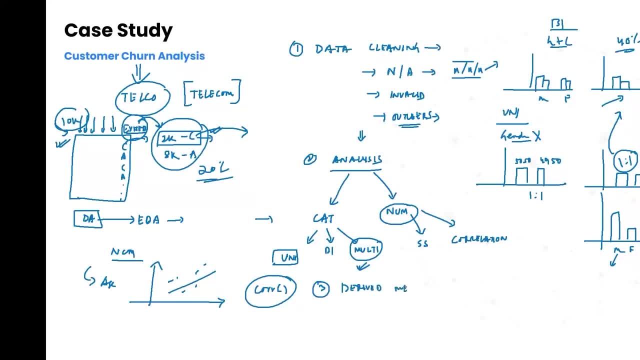 some derived matrix, which basically means some of the columns that are present in your original data set, but sometimes you have to create new columns, for example, simply age. you are not able to understand any pattern because age is a continuous numerical variable, so what you need to do is you need to create some bins out of it so that you can visualize. 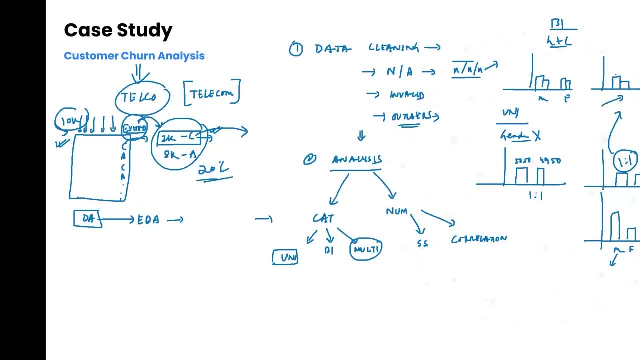 what is the churn rate here? let's say, for male customers staying in france, the churn rate is 40, which means people, especially males, who are staying in france are more likely to churn. similarly, if you want, you can also perform multivariate, which basically means you have to. 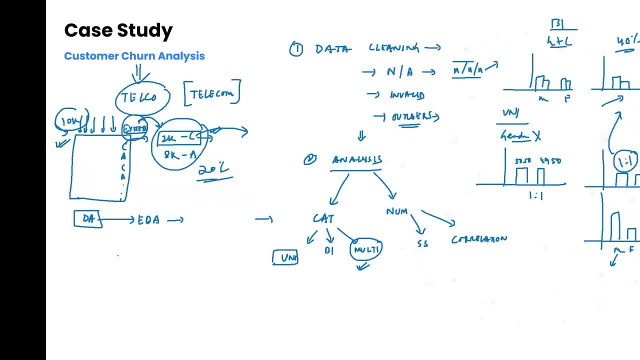 combine three or four variables together and start analyzing it. finally, when we do numerical analysis for single numerical attributes like age tenure and all those things, we try to check their summary statistics. and with multiple numerical attributes, we perform firstly, we try to check their, you know, if there are less amount of numerical values or numerical variables. 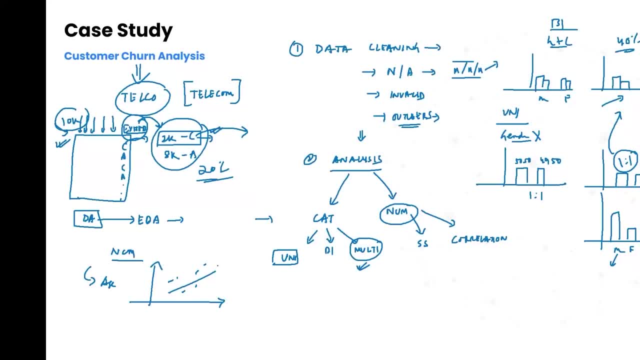 you can simply draw scatter plots between them. if there are huge amount of numerical features, you can go for the correlation matrix, cor of matrix, which tells you about each column versus each columns, correlation value, right? so these are different analysis that we use very do at some point of time. we can also do some derived matrix, which basically means: 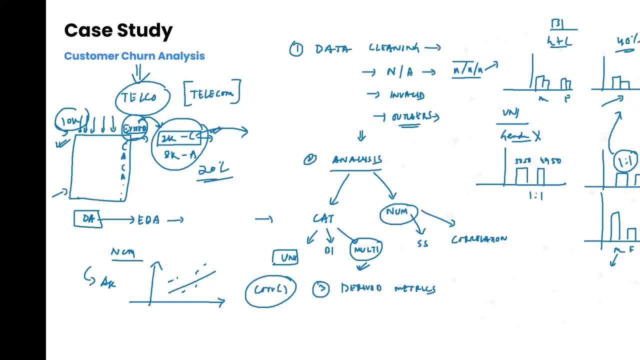 some of the columns that are are present in your original data set, but sometimes you have to create new columns, for example, simply age. you are not able to understand any pattern because age is a continuous numerical variable, so what you need to do is you need to create some bins out of it. 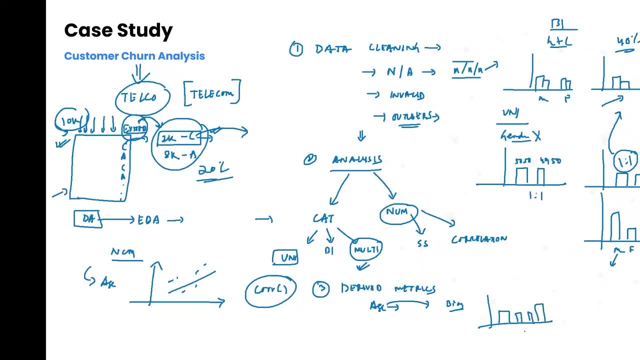 so that you can visualize the bins. so that comes under your derived matrix. so that's overall about the eda process. in the next class, in the next video, we shall be jumping into the practicals part and i will be taking help of a public data set and i will be doing. 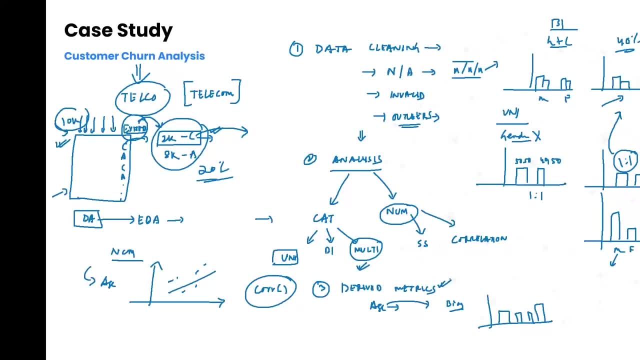 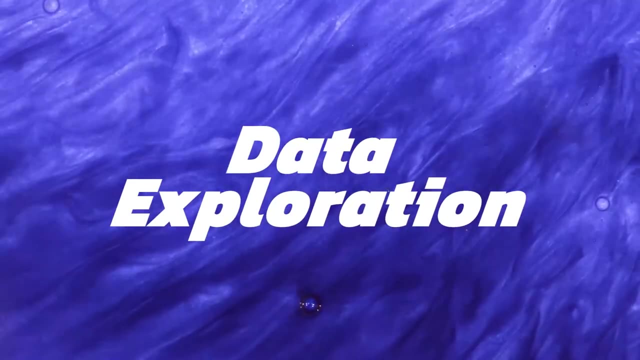 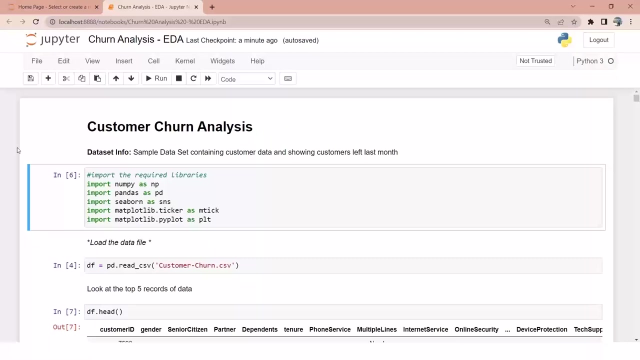 an end-to-end eda case study so so that you can understand everything about what's happening, and exactly similar kind of things. you can also do it for any other public data set as part of your project. let's move into the practicals part, so we will be talking about customer churn analysis. 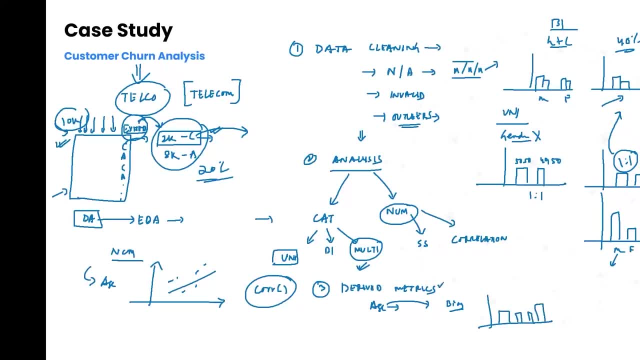 the bins so that comes under your derived matrix. so that's overall about the ada process in the next class. in the next video we shall be jumping into the practicals part and i will be taking help of a public data set and i will be doing an end-to-end eda case study so so that you can understand everything about what's happening. 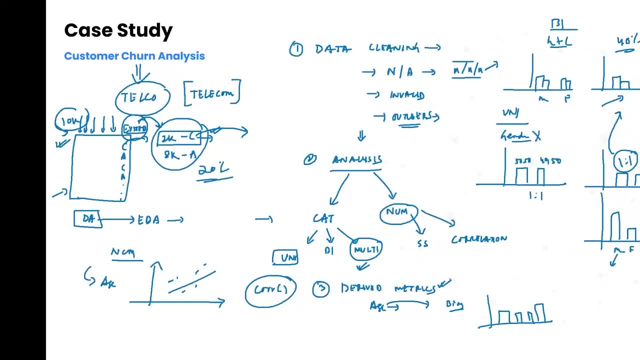 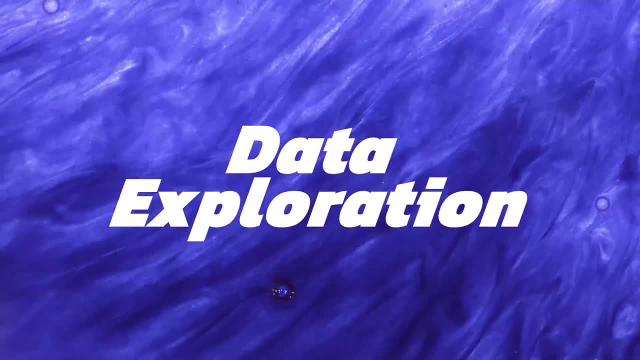 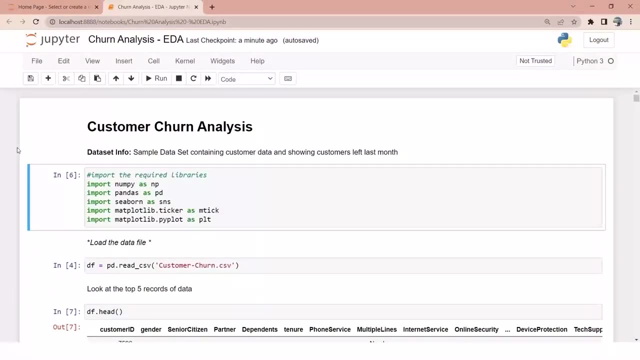 and exactly similar kind of things. you can also do it for any other public data set as part of your project. let's move into the practicals part. so we will be talking about customer churn analysis. we have the data set now. we will also talk about danny's και data set, on which we have class decid departure clause called data state. i will be sure that you have the data set. i will be sure that this will be benefit from scheduling the data t on. it will be centered around data point now it will be connected to the sector data point so you can either tick out private data t. of course, in order to do property, you will need it. so One of the two features is that data set. 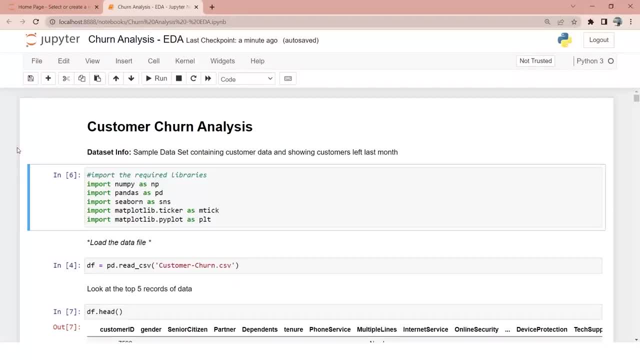 showing you the data set on how it looks like and we'll get started with the entire EDA process. to get started with, the first thing that we need to do is going to be importing the libraries in parallel. I will also be noting down the different steps that we are performing for the 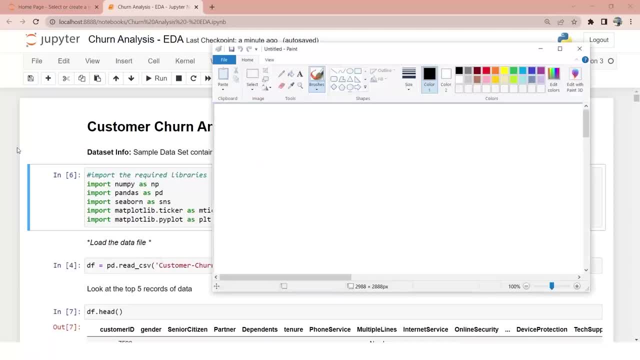 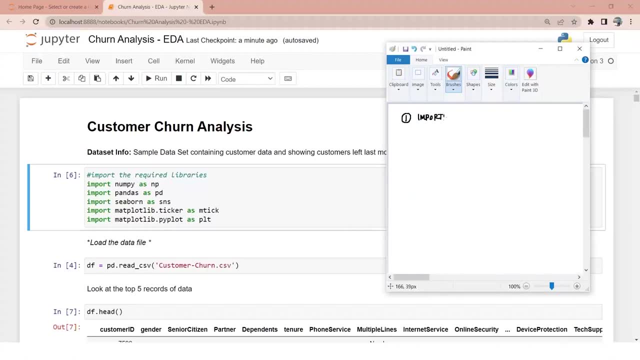 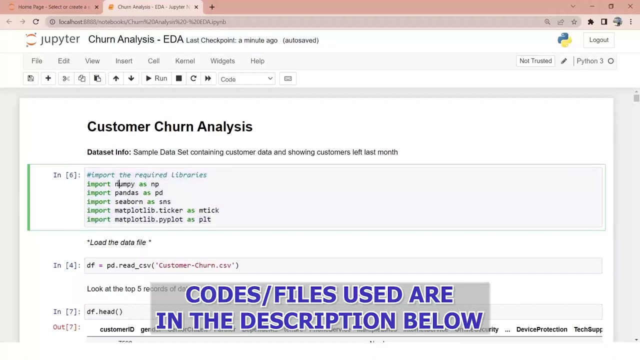 entire EDA process. so I'll quickly open the paintbrush so that we can have the steps written down here. importing the libraries: that's the first step. so in this case we are importing numpy pandas, seaborn, matplotlib and whatever libraries that we have used. we can import it. so I'll quickly. 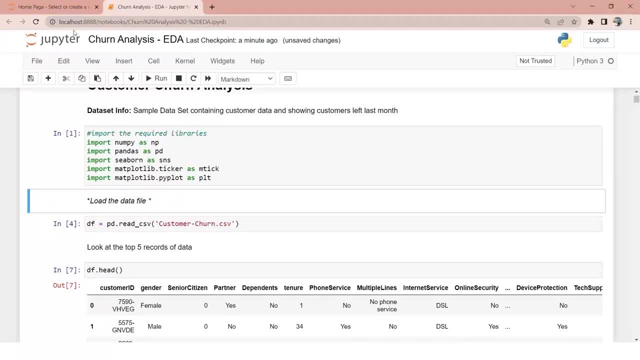 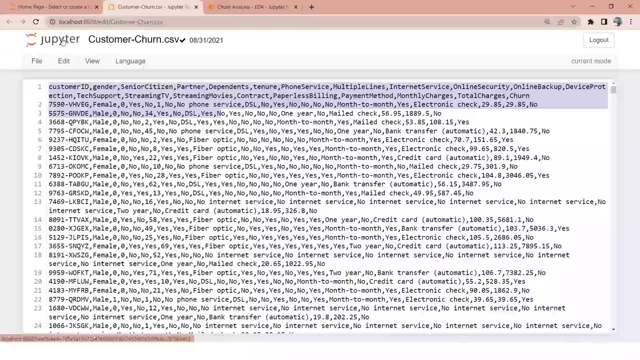 run it. the data set that I'm going to use is customer churncsv. you can see, this is how it looks like, as we have opened it up, so we can see that we have imported the libraries, so we can open it on Jupyter notebook. but yeah, if you download this file and open it on Microsoft. 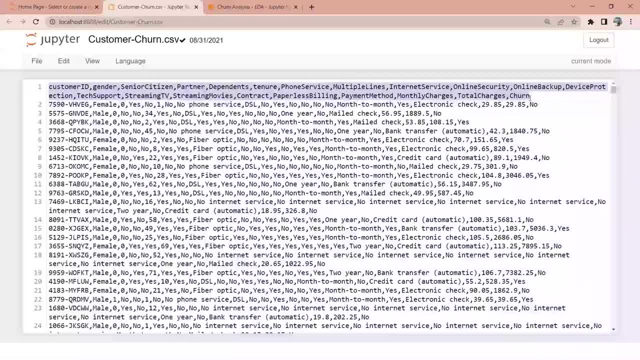 Excel, you will have a better look. it has multiple corner columns, starting from customer ID till the churn. now, just to let you know that this is not the same data set that we have used in the previous videos. it's an updated and upgraded version of it with more features you can see. 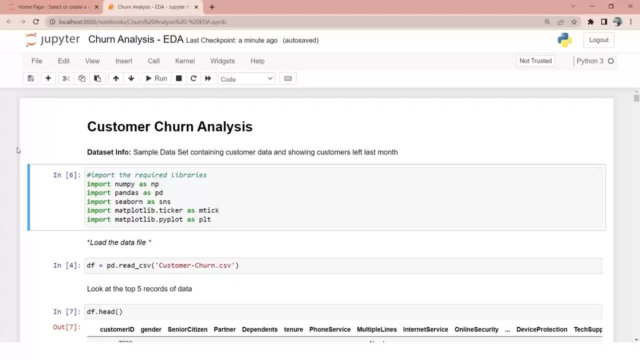 we have the data set. i will be showing you the data set on how it looks like and we'll get started with the entire eda process. to get started with, the first thing that we need to do is going to be importing the libraries in parallel. i will also be noting down the 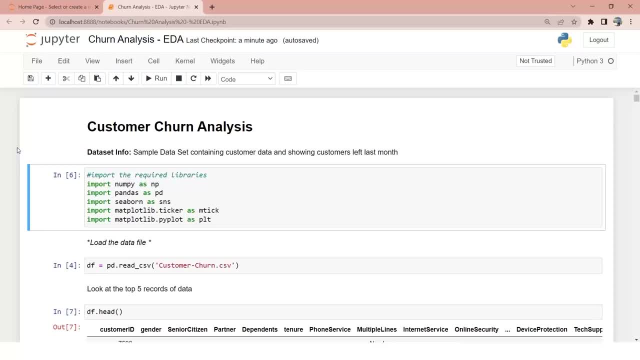 different steps that we are performing for the entire eda process. so let's move into the practicals process. so i'll quickly open the paintbrush so that we can have the steps written down here. importing the libraries: that's the first step. so in this case we are importing numpy, pandas, seaborn, matplotlib and whatever libraries that. 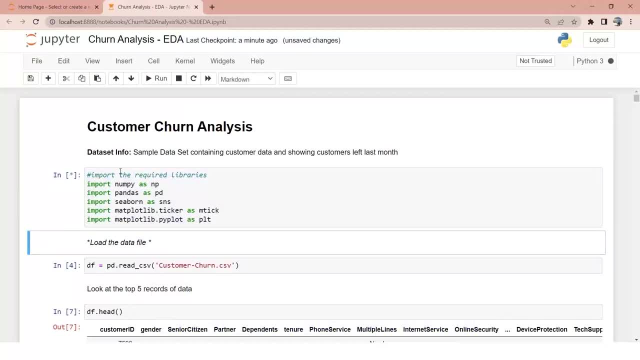 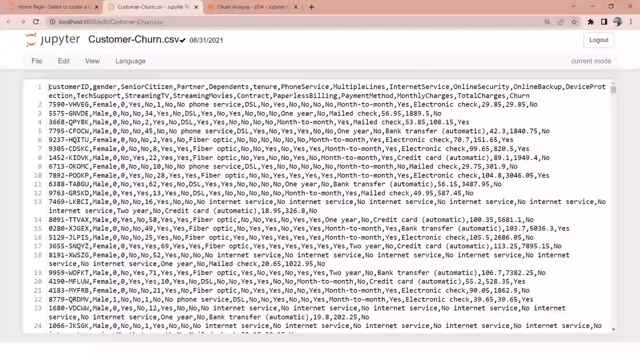 we have used. we can import it, so i'll quickly run it. the data set that i'm going to use is customer churncsv. you can see, this is how it looks like as we have opened it on jupyter notebook. but yeah, if you download this file and open it on microsoft excel, you will have a better look. 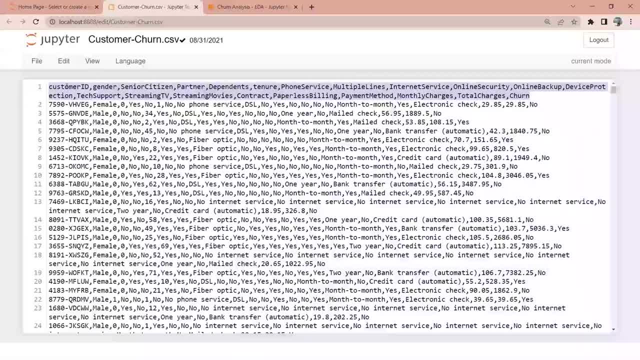 it has multiple corner columns, starting from customer id till the churn. now, just to let you know that this is not the same data set that we have used in the previous videos. it's an updated and upgraded version of it with more features. you can see there are more features here: gender, senior citizen, partner dependents, tenure phone. 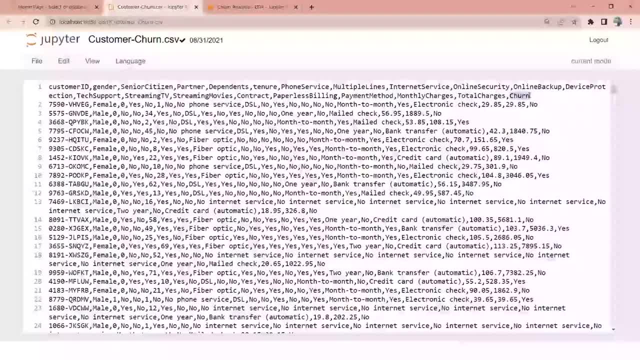 service. so many features are there, and we also have our y variable, which is the churn. our ultimate goal for this use case is to create a model which will be able to predict whether a customer is churning or not, but in our case, for the time being, we are performing the eda, so we will majorly be 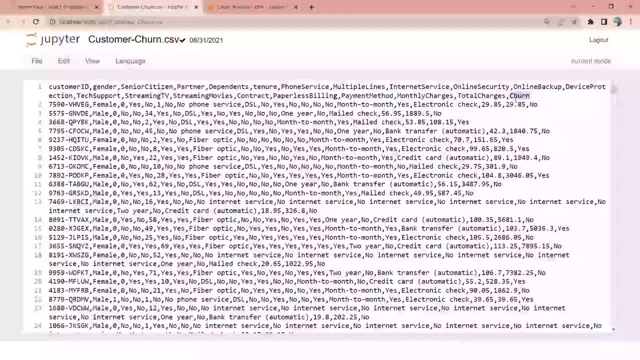 focusing on what are the drivers in this case? we will start with churn, which is the churn bar, and then we can provide you some information on every parameter of the custom data set that we have in this case. factors, or what are the most important factors of people who are churned. what 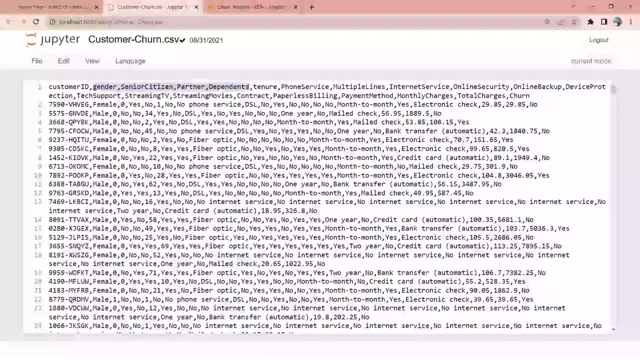 there are more features here: gender- senior citizen partner dependents tenure phone. you can see there are more features here: gender- senior citizen- partner dependents tenure phone service. so many features are there, and we also have our Y variable, which is the churn. our ultimate goal for this use case is to create a model which will be able to predict whether a customer is. 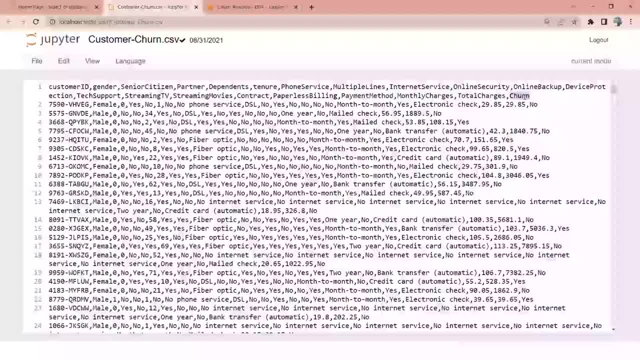 churning or not, but in our case, for the time being, we are performing the ad, so we will majorly be focusing on what are the driving factors, or what are the most important factors of people who are churned. what is the most important factor, or what are the most important factors of people who are? 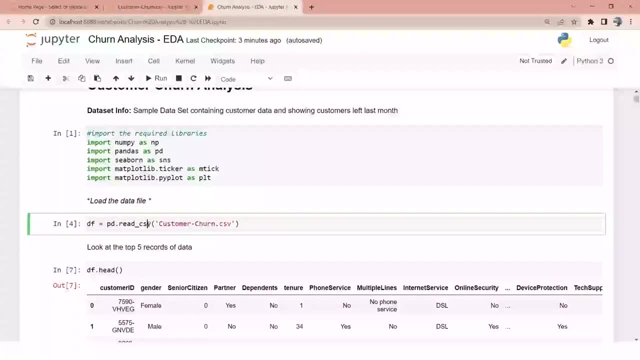 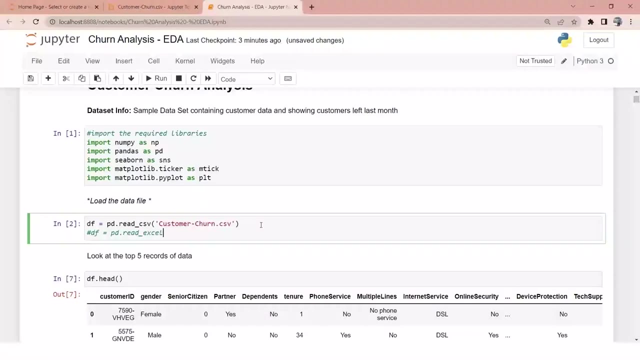 are the insights right? so, jumping back to the code, we will be reading the file using pandas dot read underscore csv. in case you are using an excel sheet, you can simply use read underscore excel and then pass the path. that's it. file name: dot csv or part dot csv. one more thing to understand. 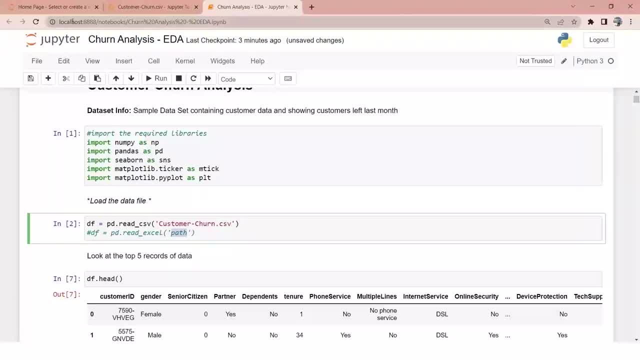 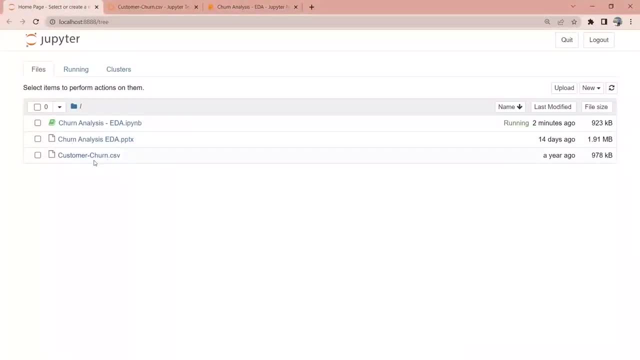 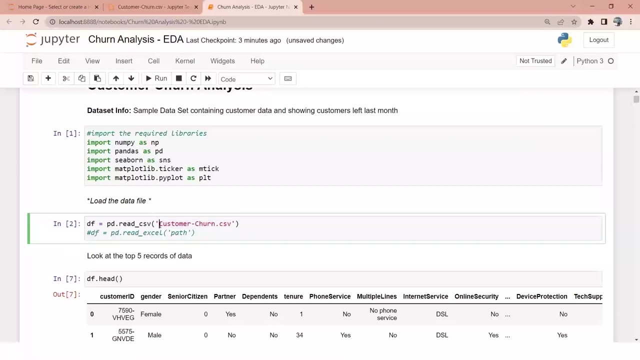 here is, as i am showing, jupyter notebook and it is in my local, local machine. let's say my file is not present in the same folder as my python notebook. imagine my file is present in a completely different directory. in that case you have to pass the entire path, else it will not be able to read. 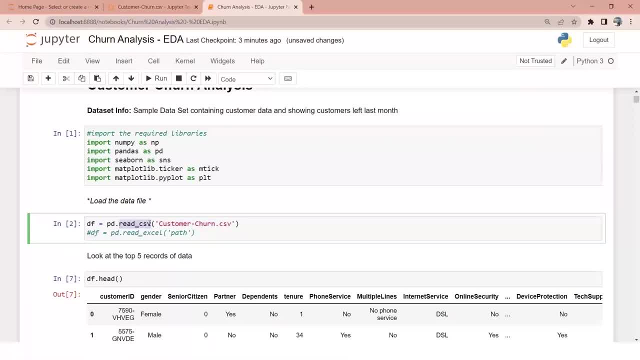 the file. in case you are using google collab, you will have to upload the file, or else you can use it directly from your google drive by creating a connection from from your collab to google drive. that's not a big deal, you can simply google it out whenever you are stuck. 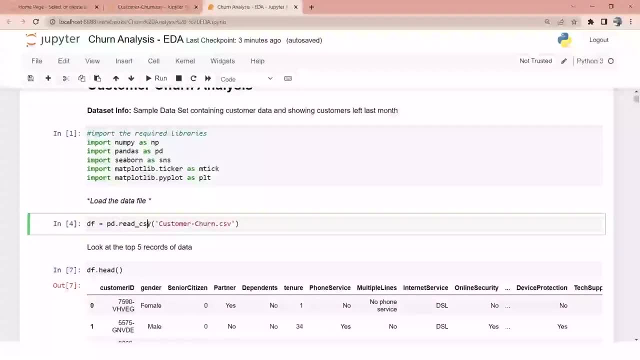 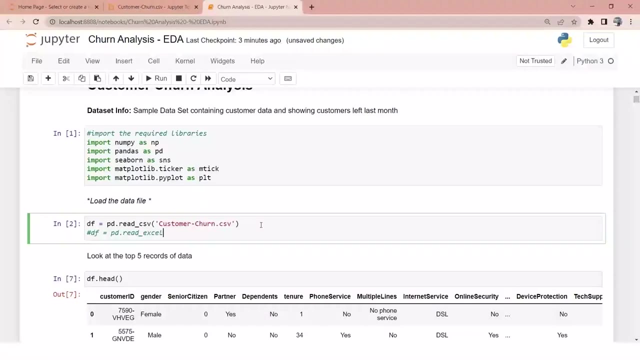 are the insights right? so, jumping back to the code, we will be reading the file using pandas: dot read underscore CSV. in case you are using an excel sheet, you can simply use read underscore Excel and then pass the path. that's it. file name: dot CSV or part dot CSV. one more thing to understand here is, as I am showing: 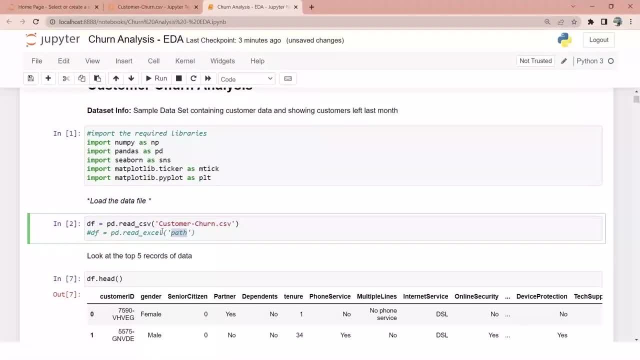 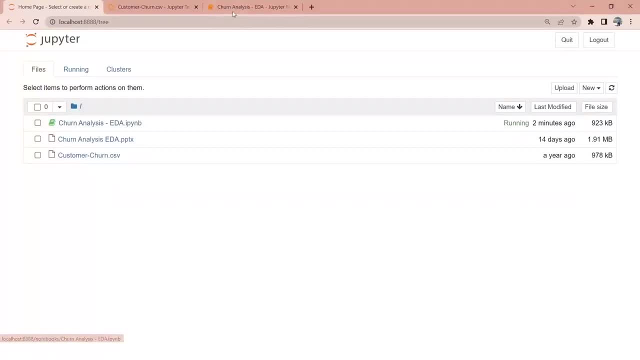 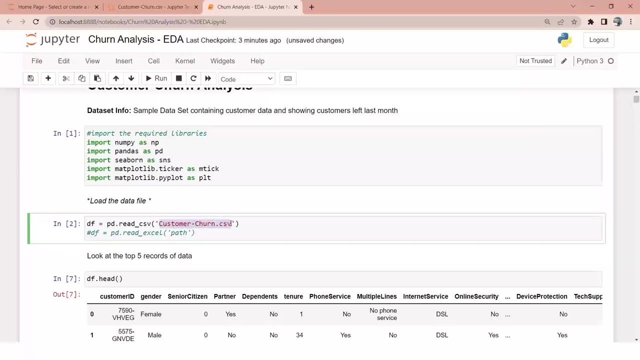 Jupyter notebook and it is in my local local machine. let's say my file is not present in the same folder as my Python notebook. imagine my file is present in a completely different directory. in that case you have to pass the entire path, else it will not be able to read the file. in case you are using 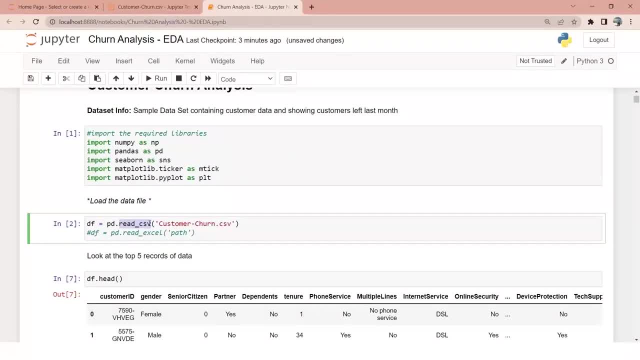 Google collab. you will have to upload the file, or else you can use it directly from your Google Drive by creating a connection from from your collab to Google Drive. that's not a big deal. you can simply google it out whenever you are stuck. you will be able to figure this out. my data is read now. this is the 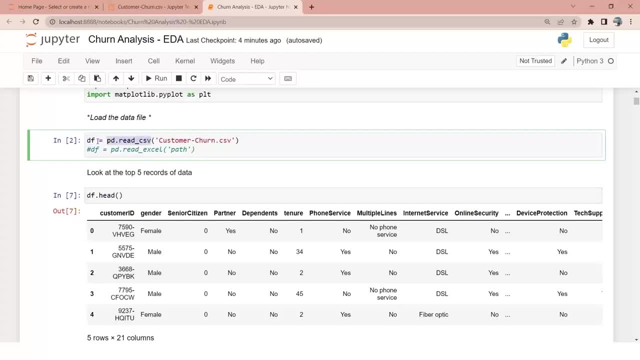 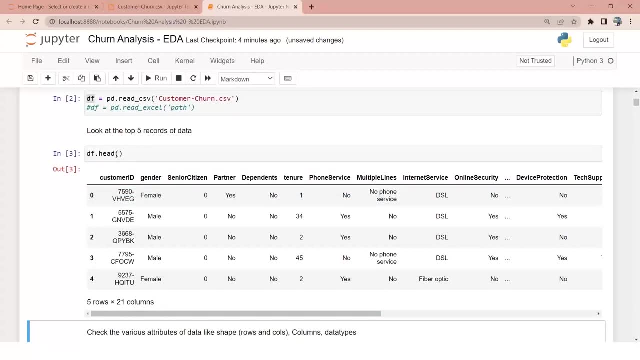 data frame that we are going to use: pandas dot CSV. this is the data frame, so the first thing that I am going to do is look at the top five records of the data. to look at the top five records, you have to use dot head function, which comes. 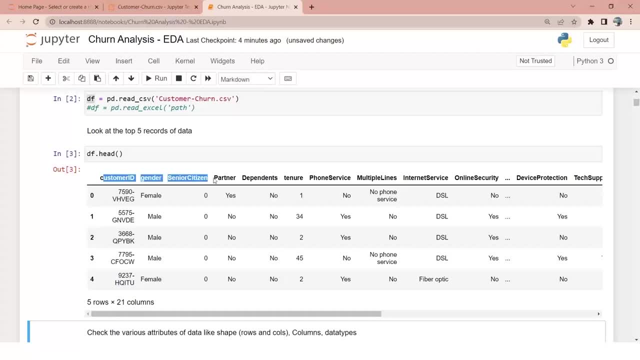 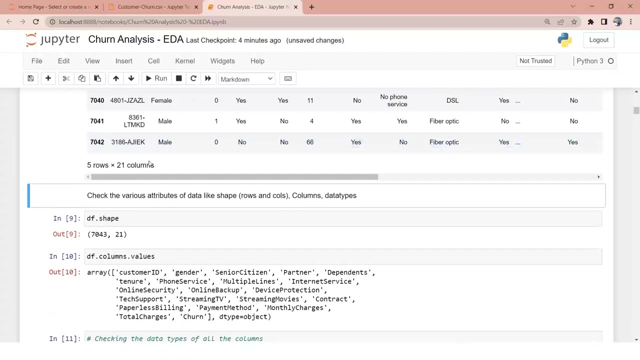 under your pandas library right now. this gives you a quick glance of the data. in case you want to have another glance at the bottom of the data, you can simply do dftel. that's it. dftel check the various attributes of data, like shape, rows and columns. 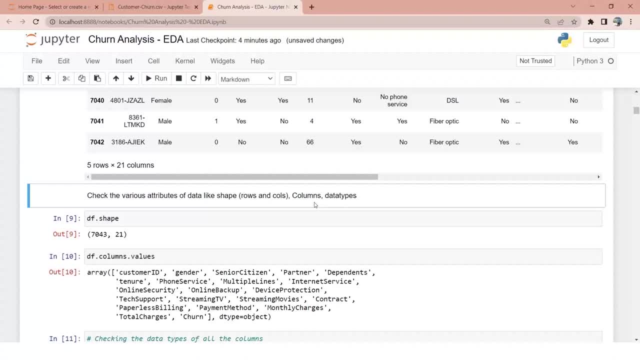 columns, data types. so this is again one of the most important things. before getting into the analysis part, you should be aware how much columns are we dealing with, how many rows do we have, what are the different column names and so on. if you have already seen your file, then completely okay, but if you are, you know. 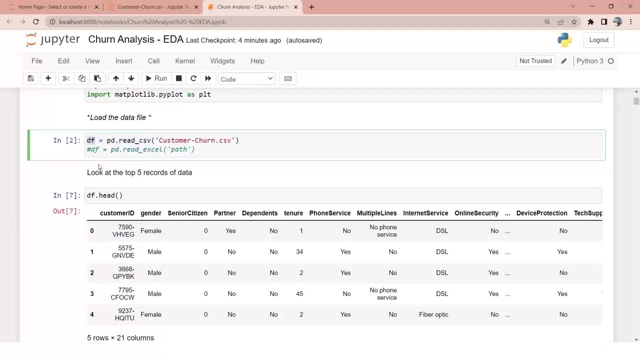 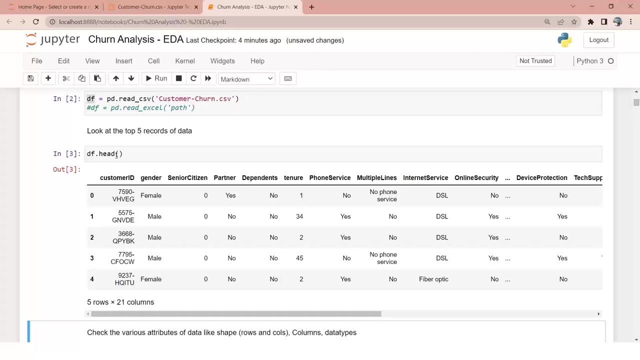 you will be able to figure this out. my data is read now. this is the data frame that we are going to use: pandascsv. this is the data frame, so the first thing that i'm going to do is look at the top five records of the data. to look at the top five records, you have to use dot head function. 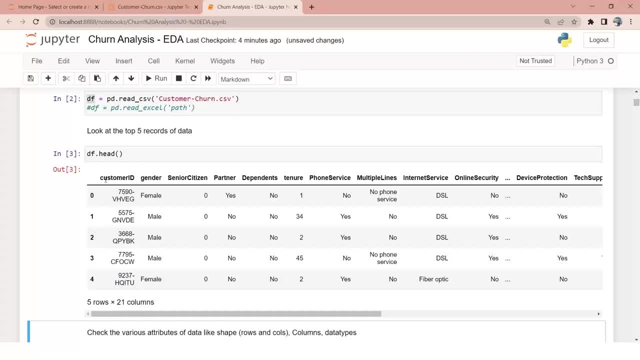 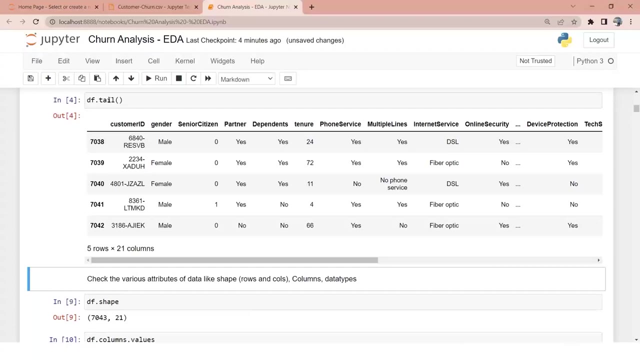 which comes under your pandas library right now. this gives you a quick glance of the data. in case you want to have another glance at the bottom of the data, you can simply do dftel. that's it. dftel check the various attributes of data, like shape, rows and columns. columns- 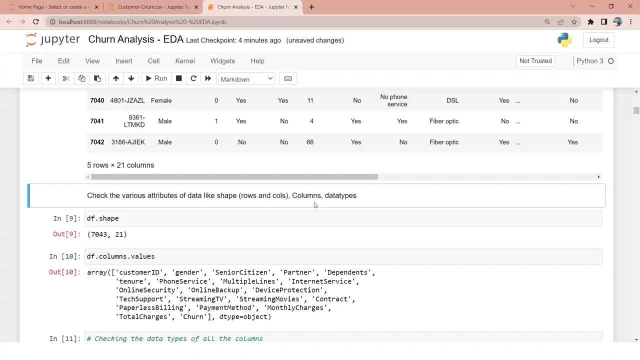 data types. so this is again one of the most important things. before getting into the analysis part, you should be aware how much columns are we dealing with, how many rows do we have, what are the different column names and so on. if you have already seen your file, then completely okay, but 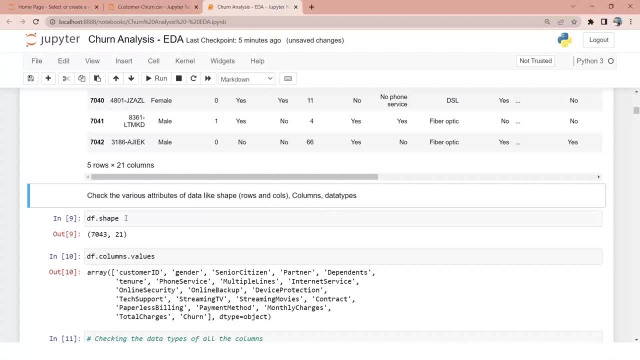 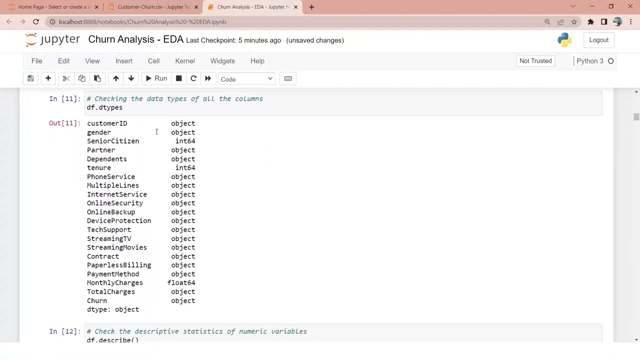 if you are, you know, directly seeing it as part of your pandas data frame, then it is a good practice to perform these activities. so df dot shape gives me an idea that we have 7043 records and 21 columns df dot. column dot values will give me an idea about all the columns that i have. similarly, if 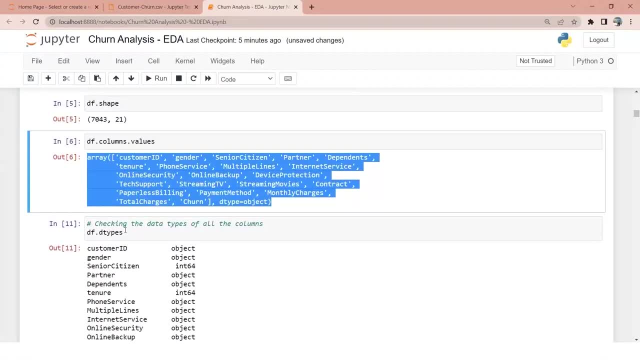 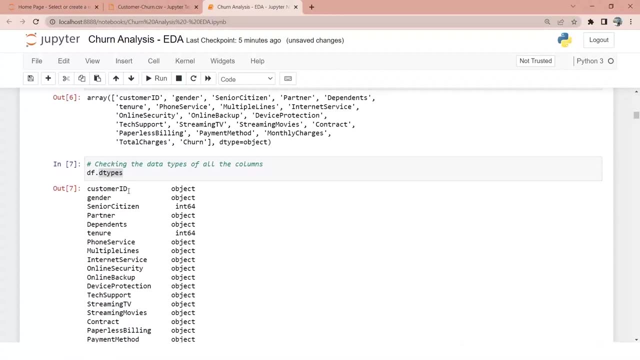 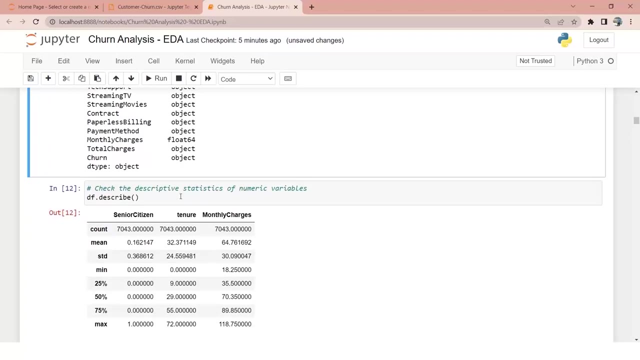 you want to check the data types. anyways, dfinfo will get give you that information, but we have a special method as well, called as d types, which will tell you that which column is of which data type. the next thing is checking the descriptive statistics of numerical variables. now, in this case, 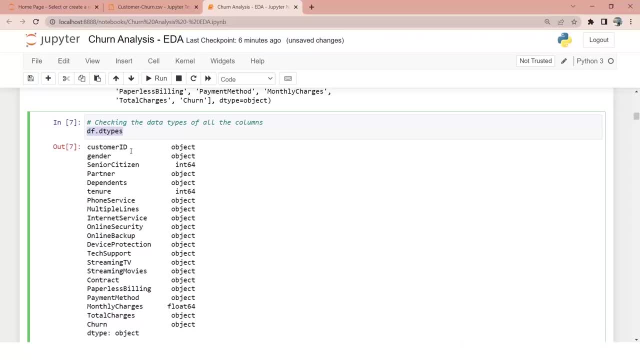 we have written down the digits that we see, so then we will be going to basically calculate the amount of number ofиб te here as well. now, as known in this network. we can have a look at it. how many numerical attributes do we have? we have senior citizen, we have tenure and we have monthly. 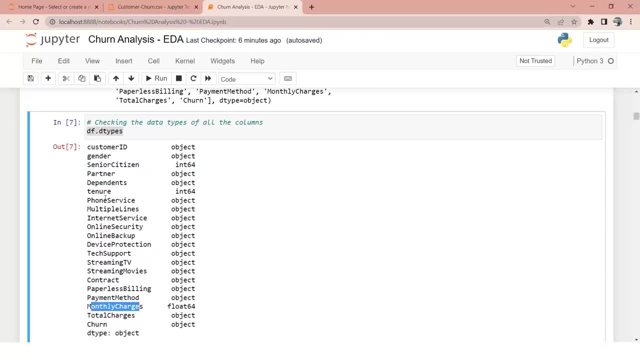 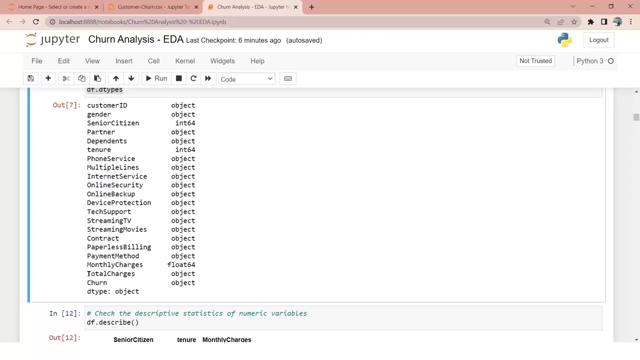 charges, nothing else. everything else is object means string values, only three, which is senior citizen, monthly charges and tenure. from this point of view, i see there is a problem. the problem is here: total charges should have been an integer value, should have been one integer value, should have been onehad吉. 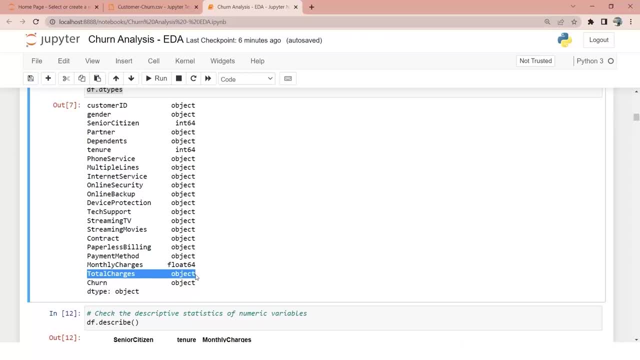 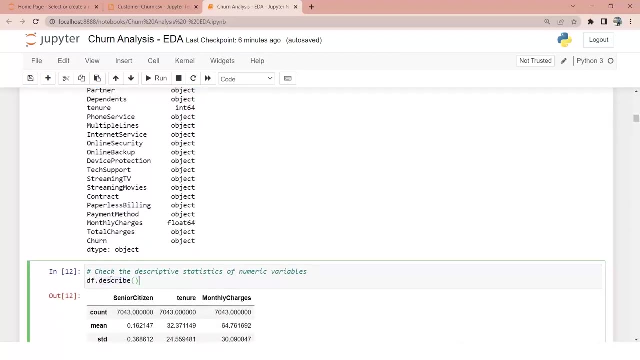 should have been a integer or float value. in fact, should have been a numerical attribute, but it is not, so we will try to keep this in our mind right now. anything else, i don't see any problem anywhere else. dot describe is going through the entire data frame and it is only 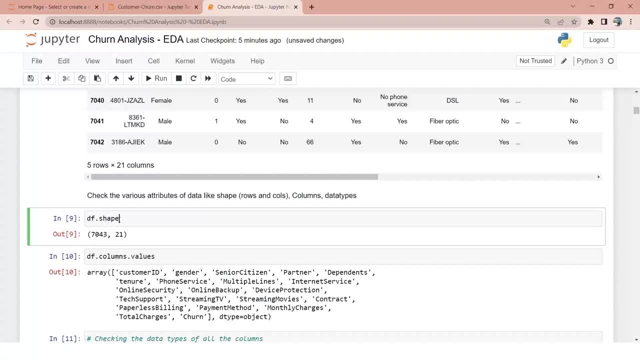 directly seeing it as part of your pandas data frame, then it is a good practice to perform these activities. so df dot shape gives me an idea that we have 1043 records and 21 columns. dfcolumnvalues will give me an idea about all the columns that I have. 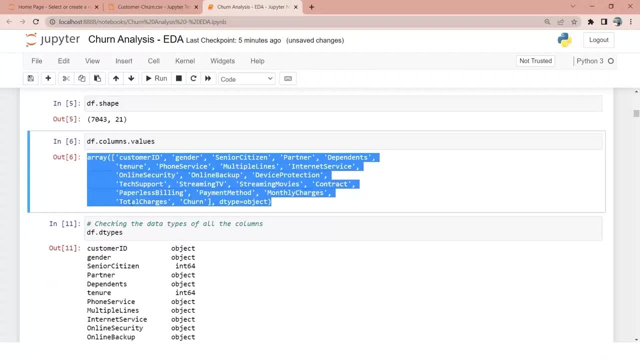 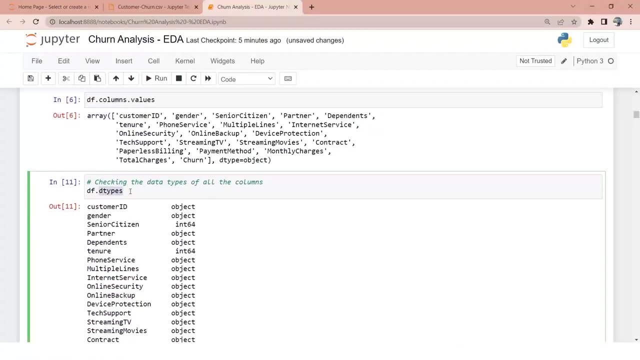 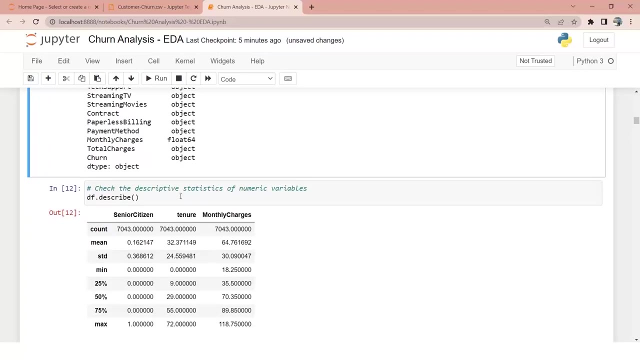 similarly, if you want to check the data types, anyways, dfinfo will get give you that information, but we have a special method as well, called as d types, which will tell you that which column is of which data type. the next thing is which value is there, and that is d calling the function. and if you are 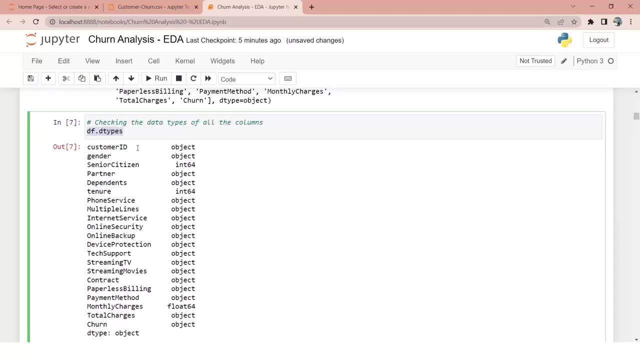 interested in learning more about this. you can go to d types- social security. you can get all the data settings there and you can create a new file and we can go to lp hl and find out what do we have. so many of the other elements are there and, if you want to use it, 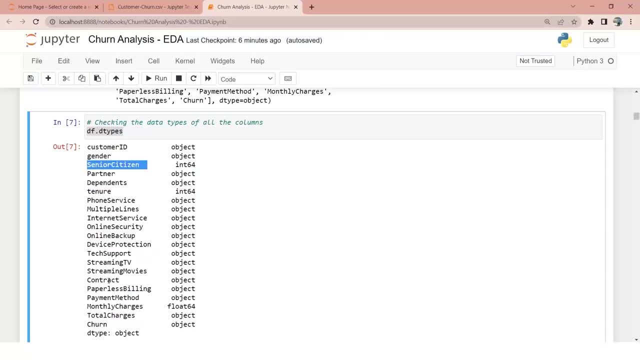 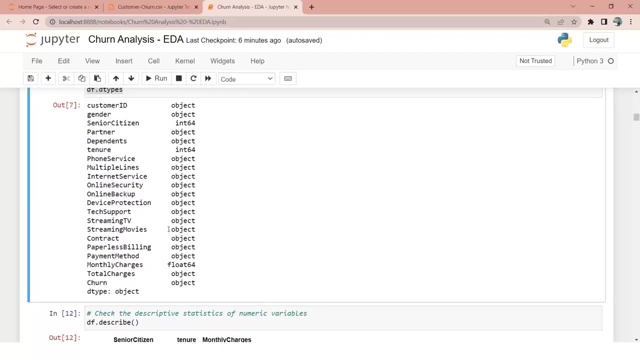 we can call it as a dot and we can use it from here. so what does it look like really? after we have looked at the data here, we can see that we have tenor and we have a monthly charges and from this point of view, I see there is a problem. the problem is here. so, to counter that is where it is and how to do it is there and from this point of view, I see there is a problem. the problem is here. so to counter that is what is it? 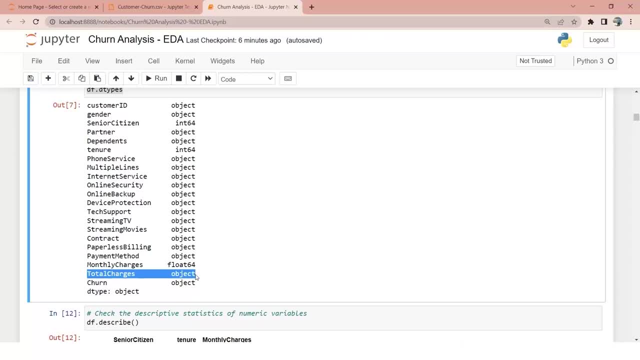 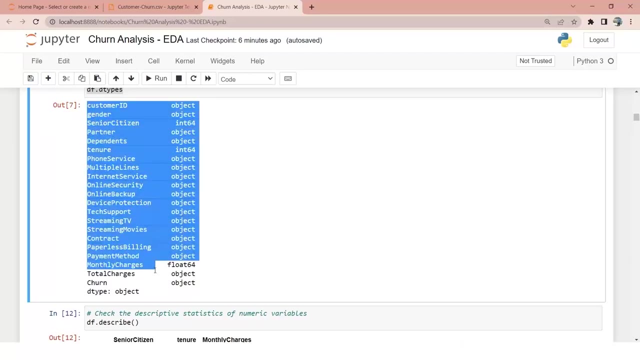 total charges should have been an integer value. should have been a integer or float value. in fact, should have been a numerical attribute, but it is not. so we will try to keep this in our mind right now. anything else, i don't see any problem anywhere else. dot describe is going through the entire data. 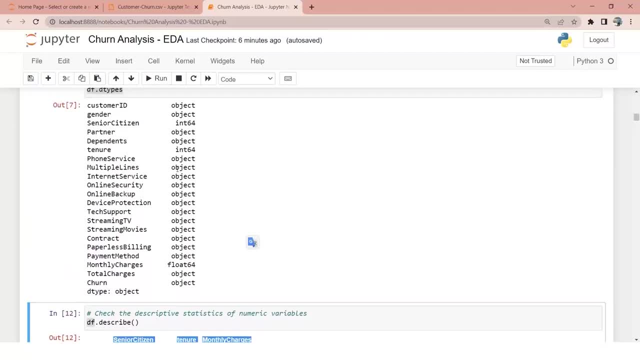 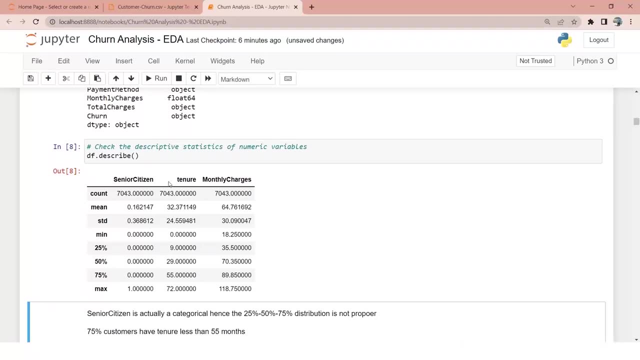 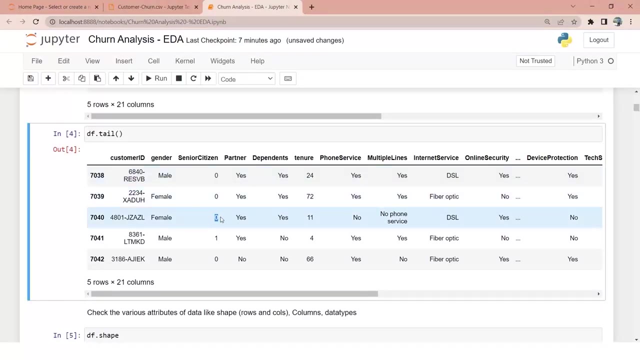 frame and it is only returning you three columns. why? because these are the only three columns that are having int or float type. so you are getting this information, but if you look at the data carefully, senior citizen is having zero or one. basically means zero, means non-senior and one. 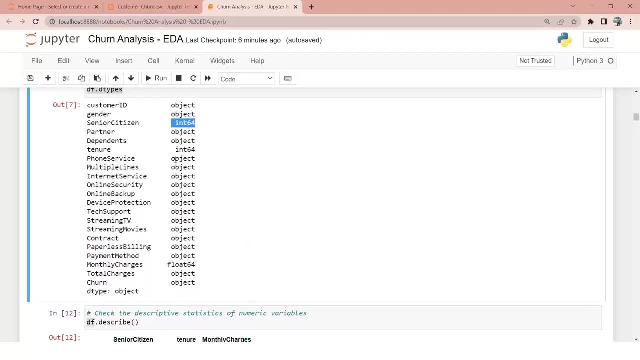 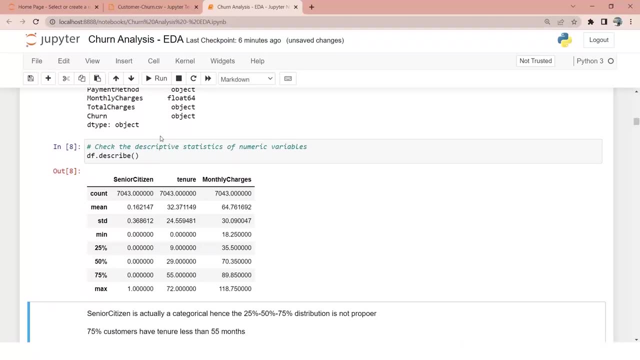 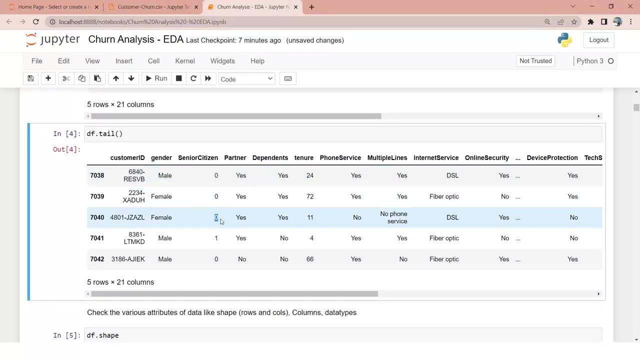 returning you three columns. why? because these are the only three columns that are having int or float type, so you are getting this information, but if you look at the data carefully, senior citizen is having zero or one basically means zero means non-senior and one means senior. 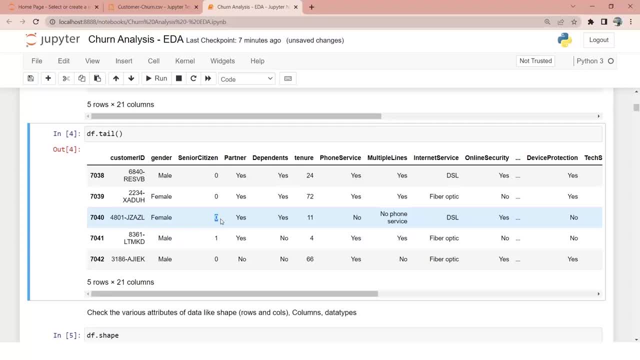 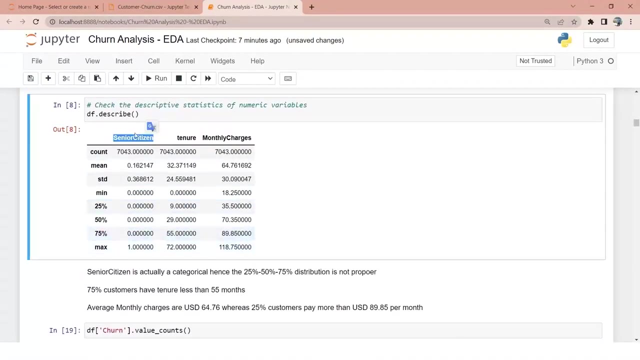 so my intuition is, even though it's a numerical attribute, it should not be treated as a numerical attribute. it is more of a categorical attribute where you can have no and yes right you. that's why i will ignore this box of senior citizen. i will only consider tenure and monthly. 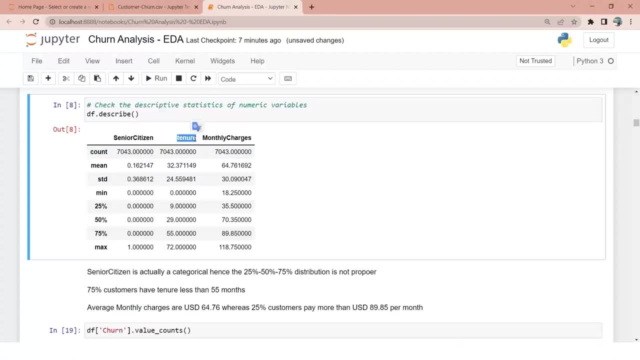 charges. so, from tenure, what do i get? the mean tenure is 32 months. probably it could be months, because 32 years does not sound good, 32 months. 29 is your median value, so i don't see a huge difference between mean and median. so i don't see a huge difference between mean and median. so i don't see a huge difference between. 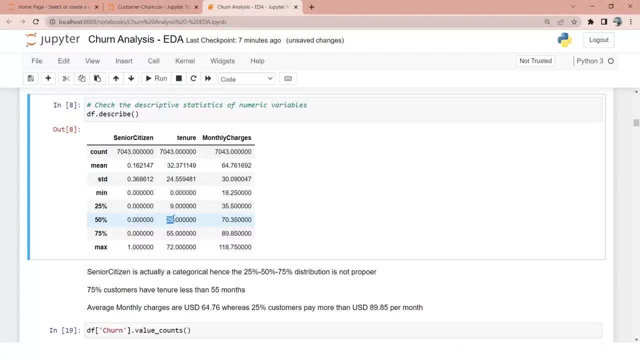 mean and median, so i think there are very less outliers. the maximum value is 72. 75% of the people are less than 55 right? 75% of your customers are having tenure less than 55 months. only one-fourth of the population is having more. 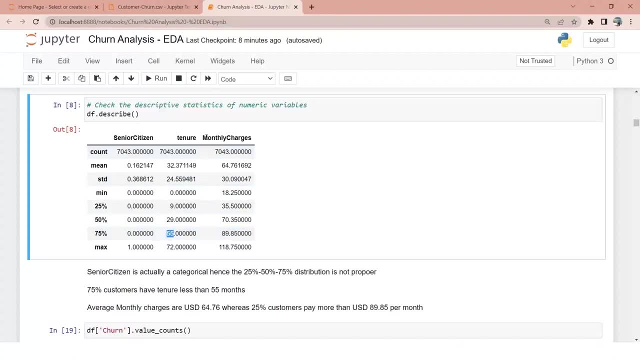 than that. from the monthly charges point of view, there is a very small decline inica from 30 to 52.5% of the population is having more than that. from the monthly charges point of view, there is a very small decline inica from 31 to 32.4% from the annual harvest to 30 to 50.5% from the monthly latest. 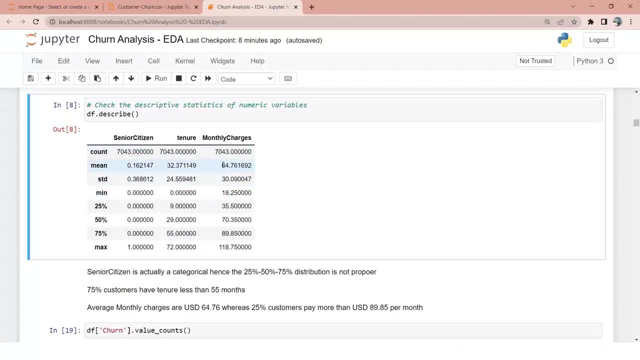 of you mean is 64. median is also 70. almost similar maximum is 118- 89. so average monthly charges is almost 65 usd, but almost 25 percent of the people are paying more than 90 dollars per month. again, not a huge insight, but this is what i'm visualizing the data so you can note down. 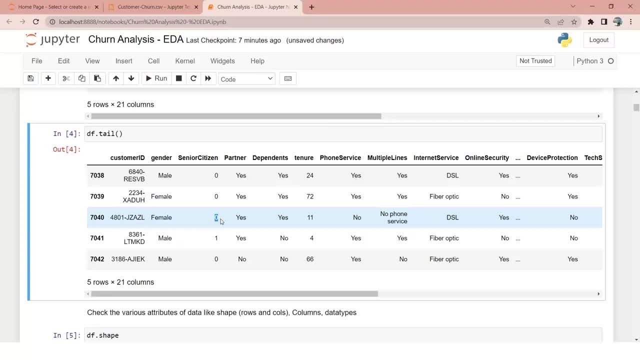 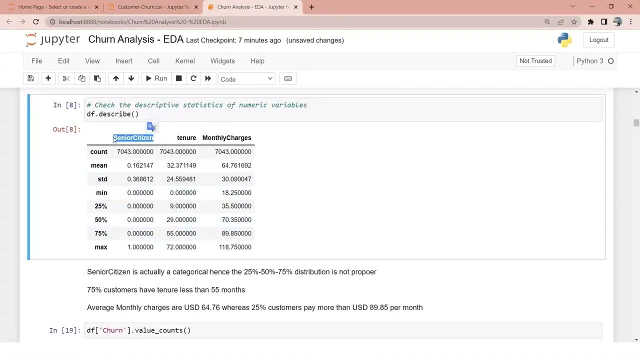 means senior. so my intuition is, even though it's a numerical attribute, it should not be treated as a numerical attribute. it is more of a categorical attribute where you can have no and yes right. that's why i will ignore this box of senior citizen. i will only consider tenure and monthly. 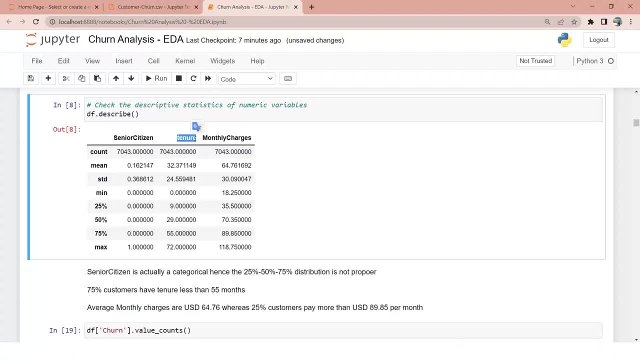 charges. so from tenure, what do i get? the mean tenure is 32 months. probably it could be months, because 32 years does not sound good, 32 months. 29 is your median value, so i don't see a huge difference between mean and median. so i think there are very less outliers. 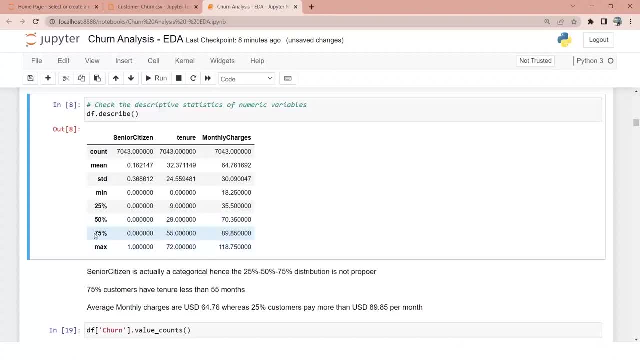 the maximum value is 72. 75 percent of the people are less than 55. right 75 percent of your customers are having tenure less than 55 months. only one fourth of the population is having more than that from the month. �zeń Verantwort mean is 64. median is also 70, almost similar maximum is 118, 89, so average. 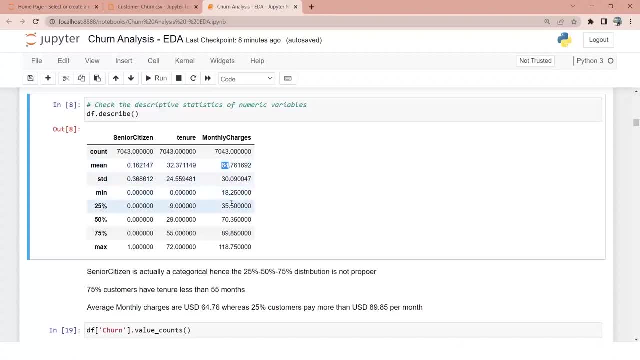 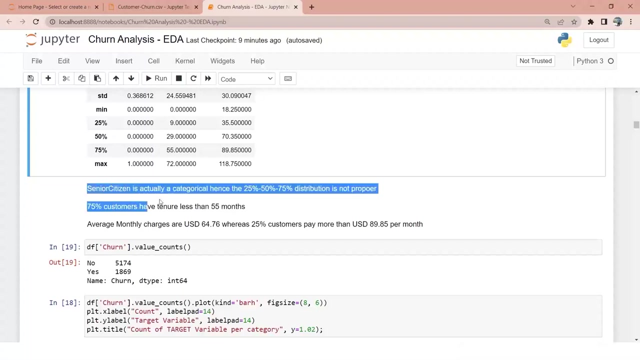 monthly charges is almost 65 usd, but almost 25 percent of the people are paying more than 90 per month. again, not a huge insight, but this is what i'm visualizing: the data, so you can note down what you see. whatever things you see, you can note it down. so i have noted it down here. 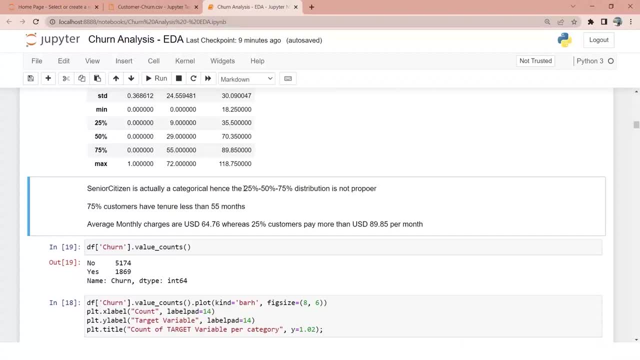 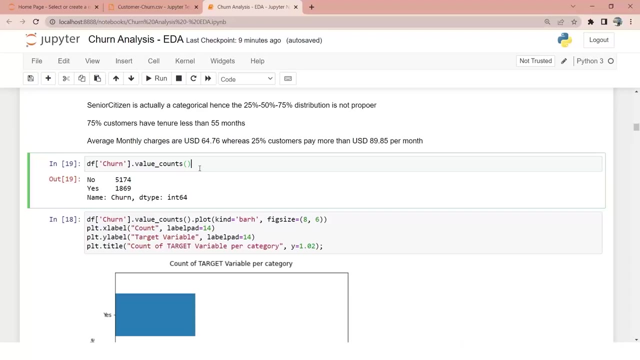 senior citizen is actually a categorical. hence the 25, 50, 75 distribution is not proper. 75 customers have tenure less than 55 months average monthly charges are this? the next thing that i'm doing is, as i know, that this particular data set has a column which talks about whether 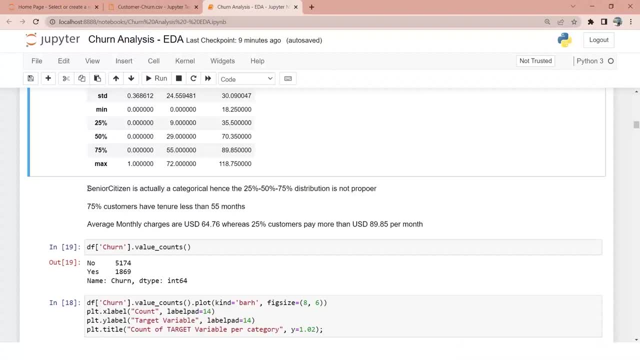 what you see. whatever things you see, you can note it down. so i have noted it down here. senior citizen is actually a categorical, hence the 25, 50, 75 percent distribution is not proper. 75 percent customers have tenure less than 55 months average monthly charges. are this the next thing that i'm 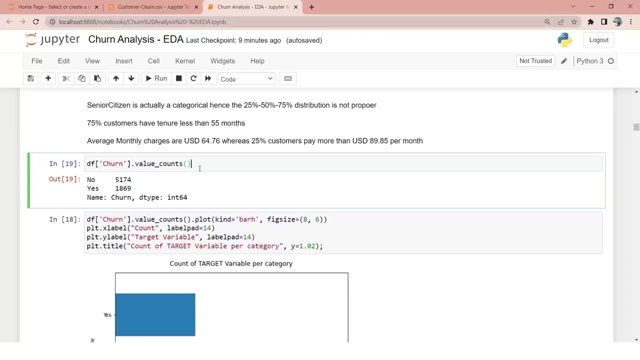 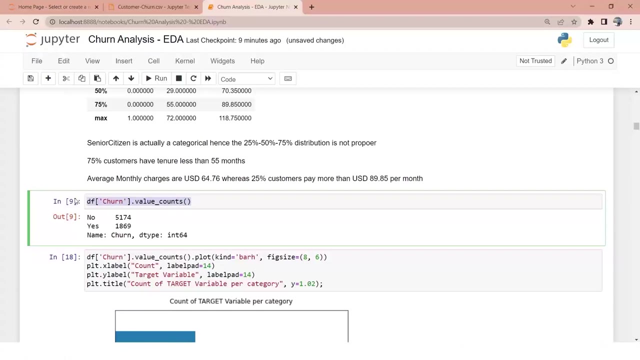 doing is, as i know, that this particular data set has a column which talks about whether the customer has churned or not churned. so i'm quickly doing a value counts on that particular column. so my value counts is returning me this: if you further have to see the distribution with respect to percentage: 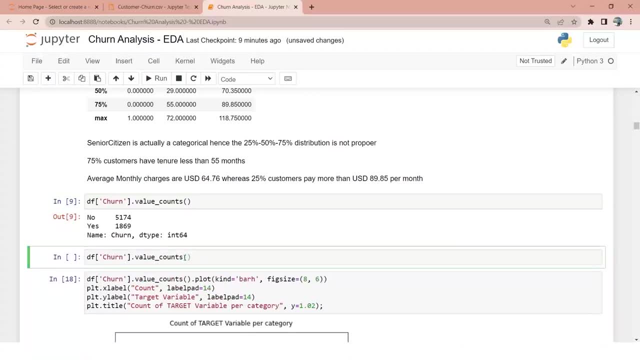 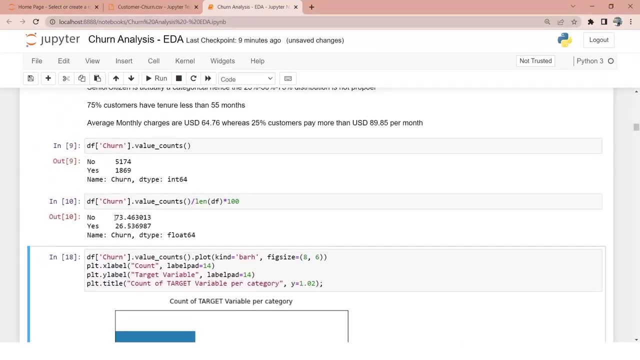 you can simply do this: value counts divided by the total length of the data frame, multiplied with 100, that will give you the value counts of the data frame, which gives you an idea that the distribution is almost. 73.4 is to 26.5, which means the total. 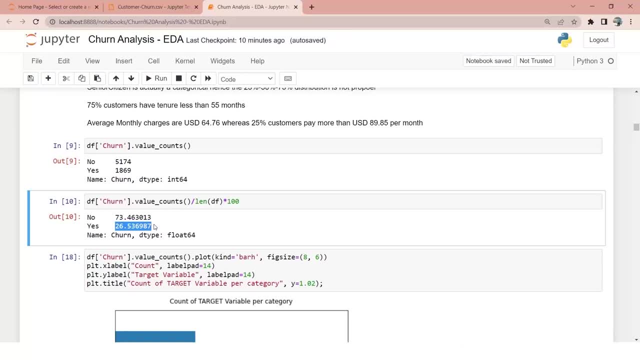 churned rate of the data you have is 26.5. now, that is why, as a data analyst, you should be able to understand the pattern of the people who are churning, and, as a data scientist in the future, your main goal has to be creating a model, so that the model can. 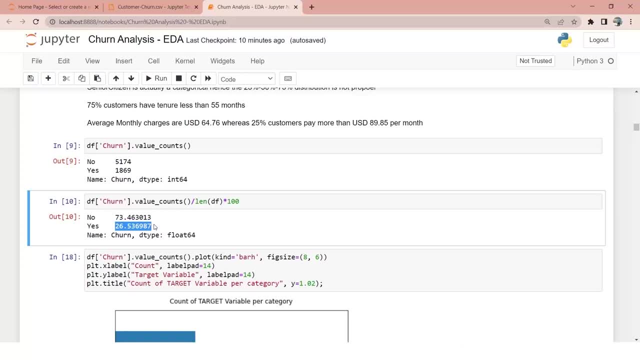 predict any existing customers that are probably likely to churn in the next six months or 12 months, and if you are able to do that by providing them offers, you will be able to retain them. so this percentage goes down, the revenue of the company goes up and you are doing justice for. 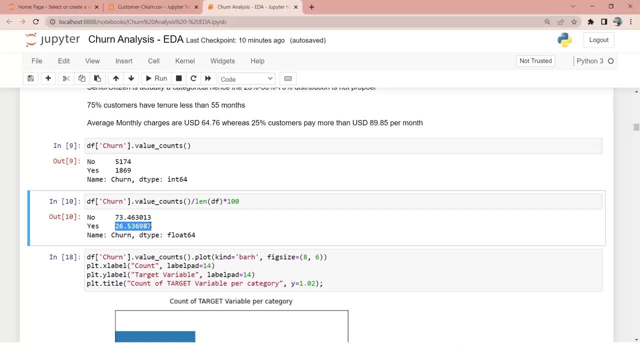 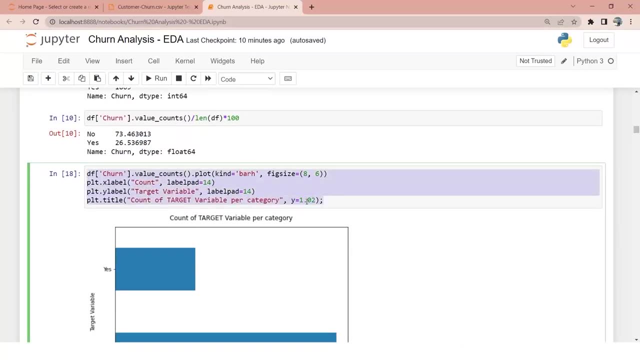 your job. that's how the relationship between analytics and the data science part is right. coming back to the topic, here i am simply building a bar chart using my value counts, so i have my df of churn value counts. i am plotting a bar h bar. h means a horizontal bar. 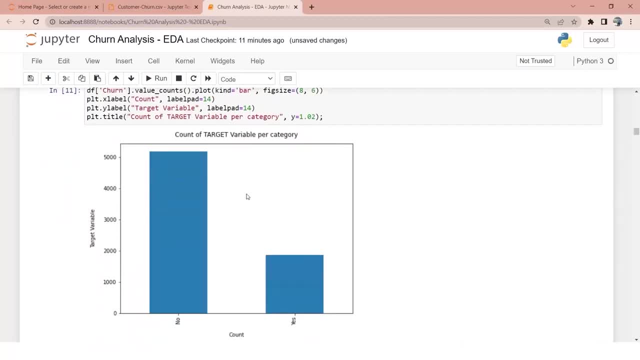 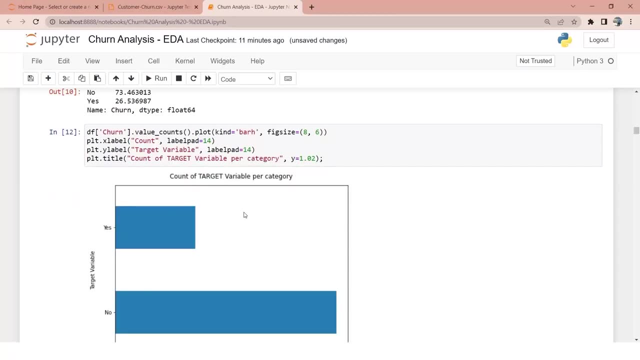 chart. if you do simply bar and you run this, you will get a graph like this. if you run it on a bar h, you will get a horizontal chart. it depends on what you would like to achieve. in my case, i am completely okay with bar or bar h. pick size is basically showing you how big your. 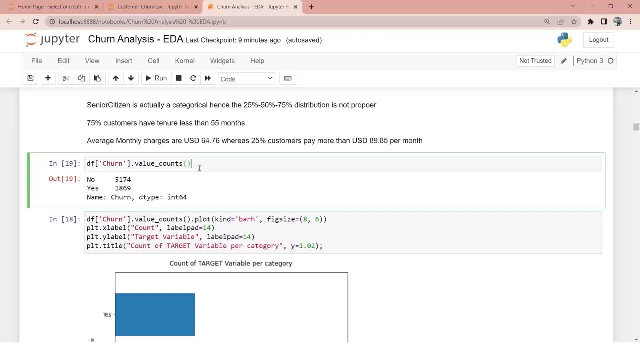 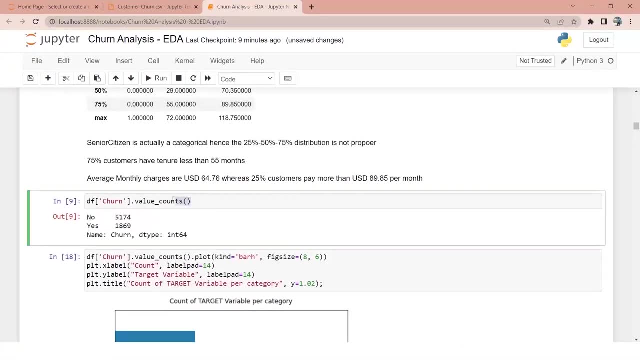 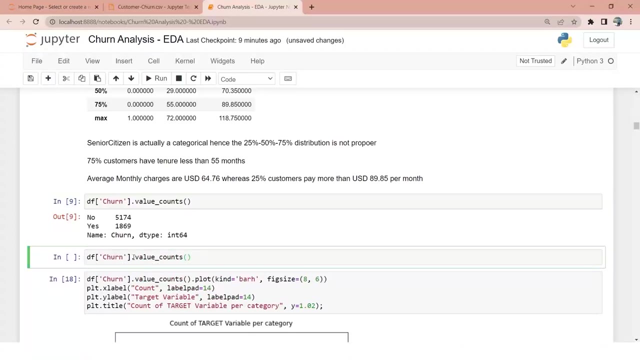 the customer has churned or not churned. so i'm quickly doing a value counts on that particular column. so my value counts is returning me this: if you further have to see the distribution with respect to percentage, you can simply do this: value counts divided by the total length of the data. 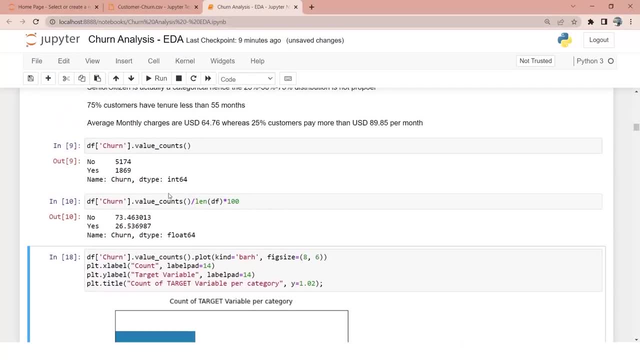 frame. multiplied with 100, that will give you an idea that the distribution is almost. 73.4 is to 26.5, which means the total churn rate of the data you have is 26.5. now, that is why, as a data analyst, you should. 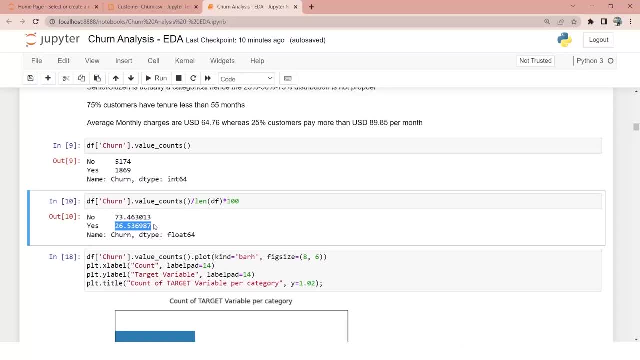 be able to understand the pattern of the people who are churning and, as a data scientist in the future, your main goal has to be creating a model so that the model can predict any existing customers that are probably likely to churn in the next six months or 12 months and if you are, 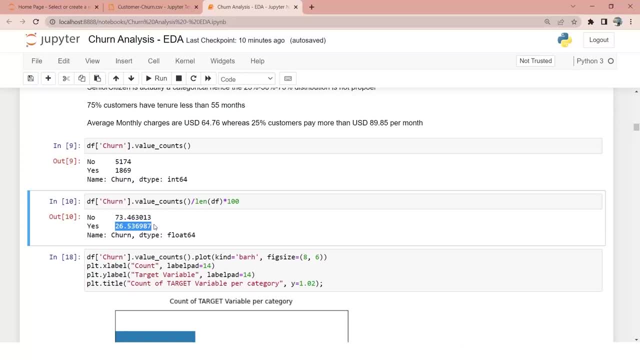 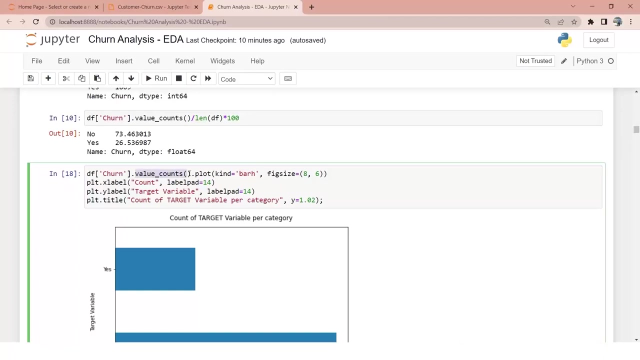 able to do that. by providing them offers, you will be able to retain them. so this percentage goes down, the revenue of the company goes up and you are doing justice for your job. that's how the relationship between analytics and the data science part is right. coming back to the topic here, i am simply building a bar chart using my value counts. 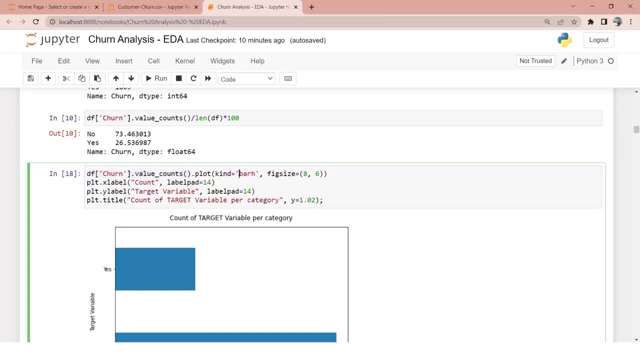 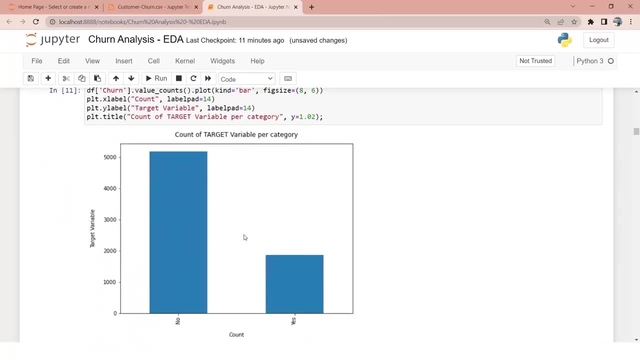 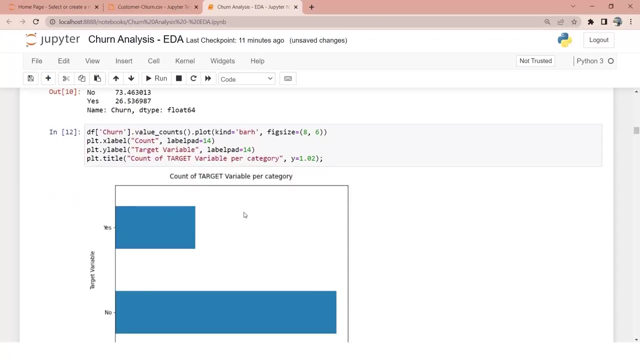 so i have my df of churn value counts. i am plotting a bar h. bar h means a horizontal bar chart. if you do simply bar and you run this, you will get a graph like this. if you run it on a bar h, you will get a horizontal chart. it depends on what you would like to achieve. in my 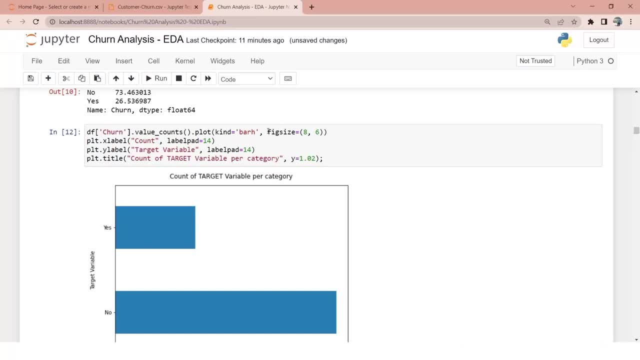 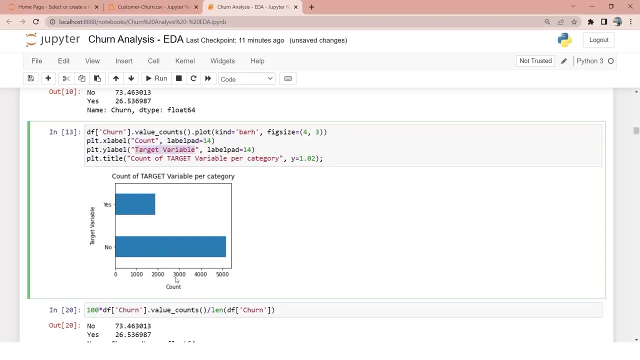 case, i am completely okay with bar or bar edge. pick size is basically showing you how big your figure should be. if it you need to shorten it out, you can shorten it up to you. x label and y label are basically given to provide the labels. you can see your x is count and y is target. 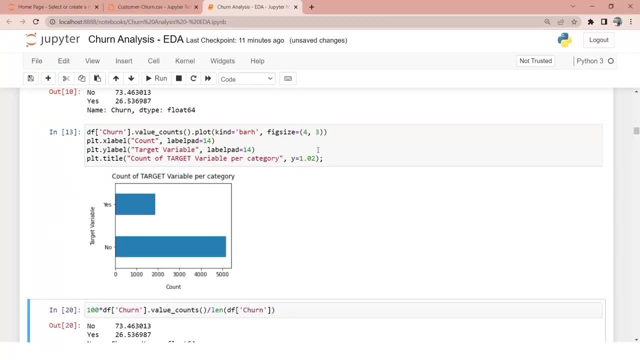 figure should be. if it you need to shorten it out, you can shorten it up to you. x label and y label are basically given to provide the labels. you can see your x is count and y is target variable and title is count of target variable per category. simple if you want to make it very 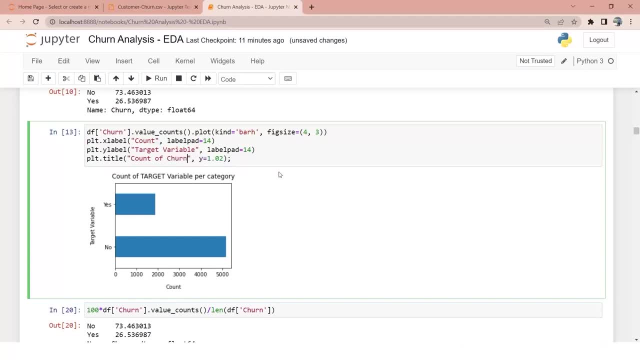 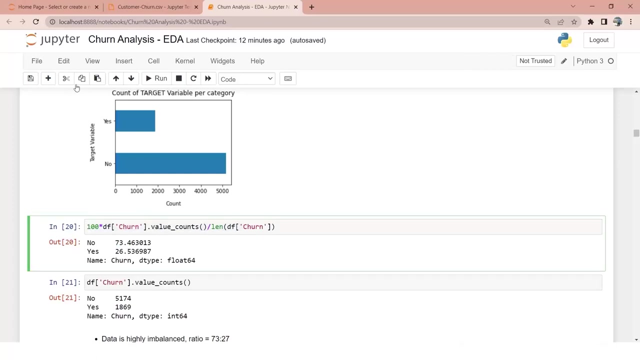 clear count of you, count of customers per turn. category looks, you know. anyways, let's not complicate things. so things are good, right. so you can see this plot. this is the same step that we performed. 73 is to 26, so i'll try to skip this part. 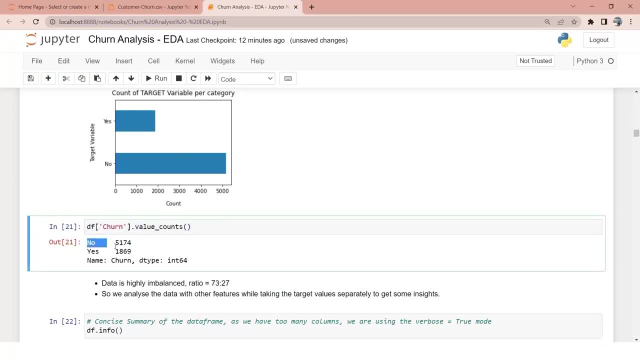 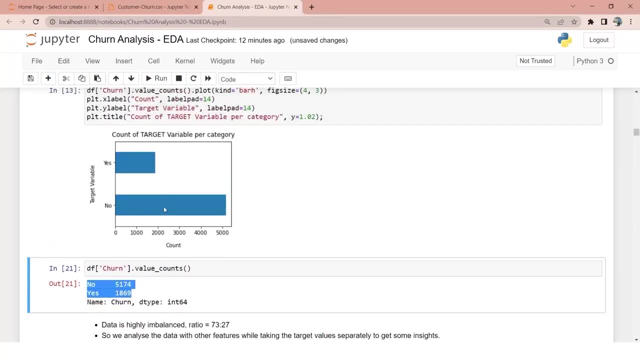 my value counts is also clear. for no, we have 5174 and yes is 1869. now what is the insight here? the insight here is the data is highly imbalanced. it is not in the ratio of one is to one and almost 74 percent of the people are active and rest are getting churned right. 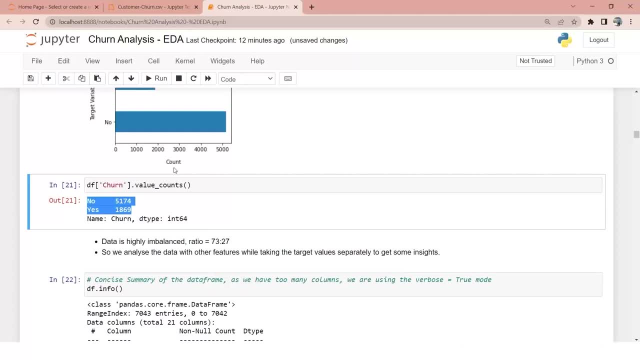 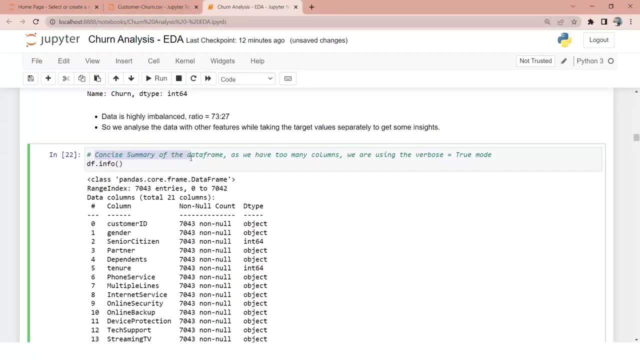 so our further insights analysis has to be done to understand more about the people who are churning. then i am doing a dot info concise summary of the data frame. as we have too many columns, we are using verbose equals to true. verbose equals to true. i'm not using it so i will just 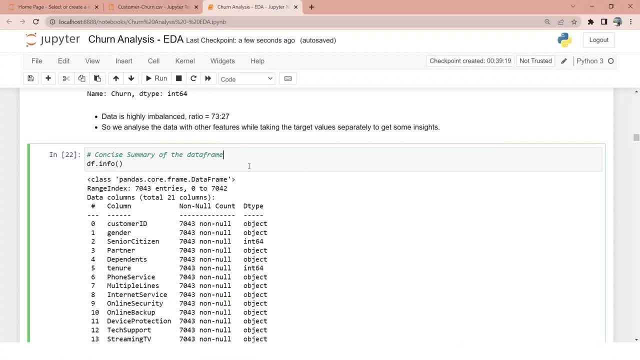 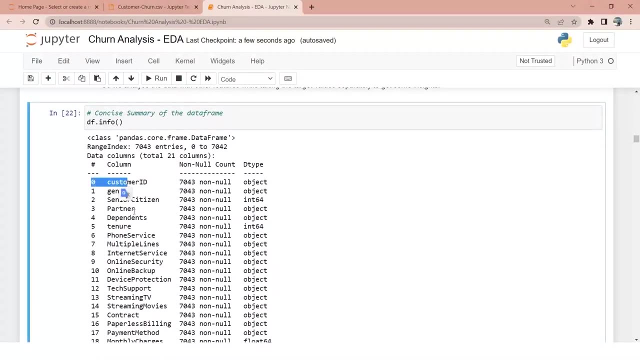 that's it. i'll just remove this part. verbose equals to true is another thing. for example, you are dealing with a data set where you have hundreds and thousands of columns. in that case, what happens is you will not be able to scroll it properly. you will not be able to see all the columns. if you mark verbose equals to true, it will be. 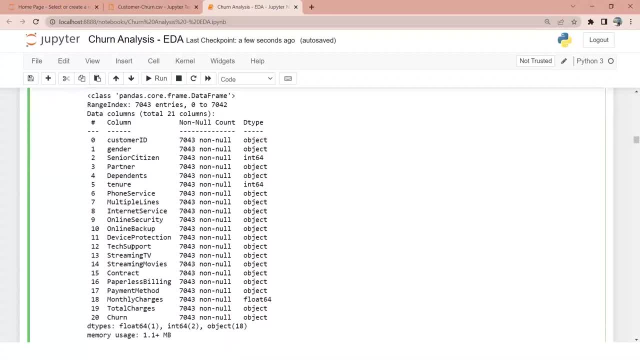 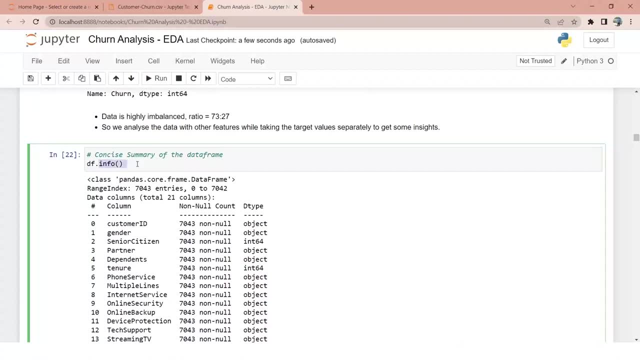 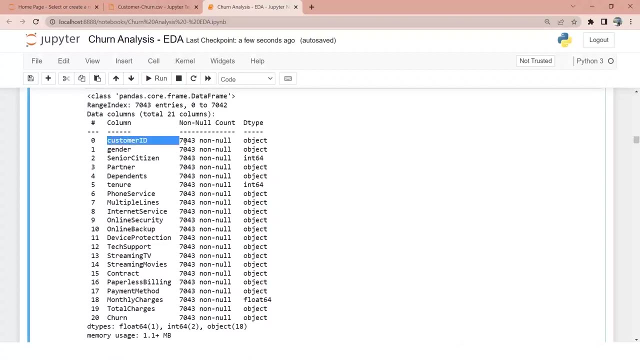 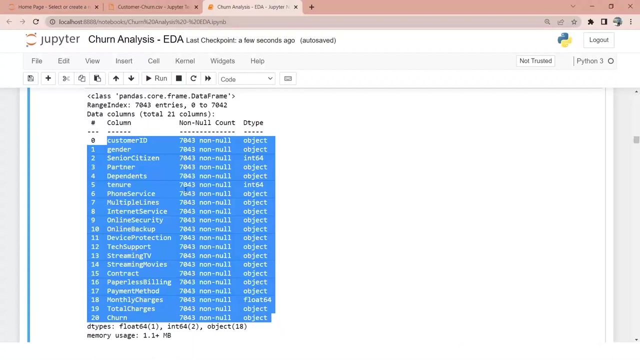 scrollable and you can scroll through all the columns. in this case we are just having 21 columns, so we don't need that option. so i'm just using dot info, which basically gives me an instance like this, and i could see that most of the records here are completely okay. there is no null values. 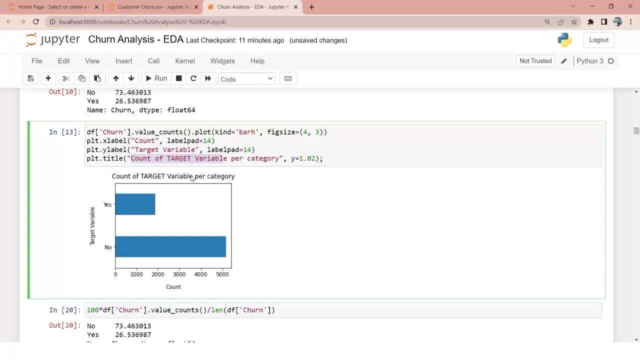 variable and title is count of target variable per category. simple, if you want to make it very clear by running this right so we can say: is this are the counter values? but we will do so for classic, statistical, très small over here. now we have values which are good as minimum. 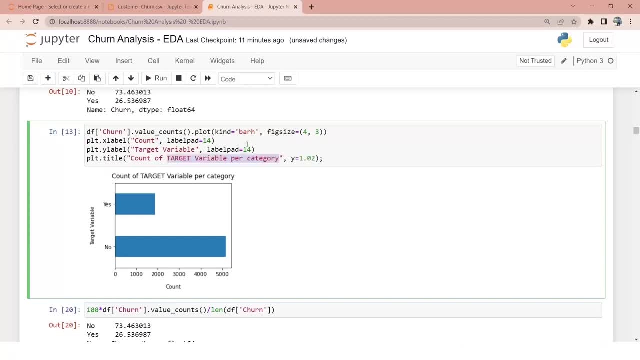 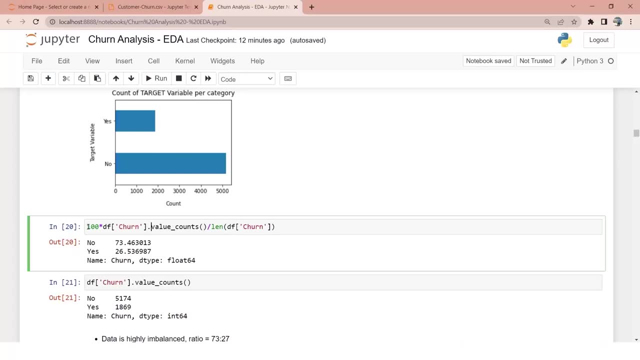 of numbers. this is no і, so that means add negative t2 grade negative 1.3, so that make it also a negative pMS. so our original values would be say5.75 and 1.75, similar values, so above pMS where we have negative values. so n equals zero to n equals zero inside out. 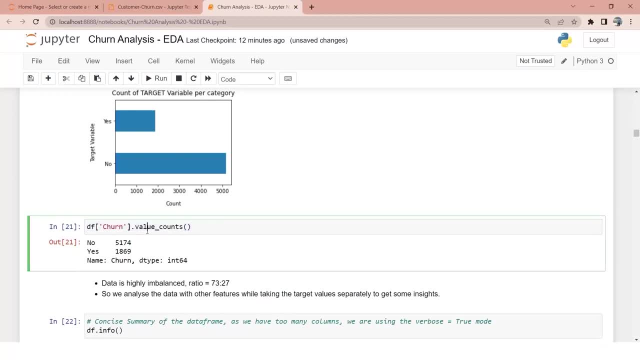 in this case our value counts should be. we make a vectroom vector for background and numbers with variance minus 15. so we make a vectroom vector here, in this case to see if we want to reverse the heart or like to listreet this guys. then we simply write down the entering value. you finally make a. 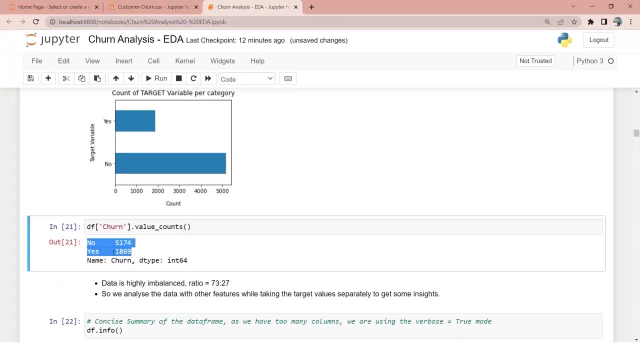 fixed policy here in just only one esse is that we don't have a understand of why the value comes is weird. so for this side you should be keeping a mind, because number degrees own in there, thousand one hundred and seventy four, and yes, is eighteen, sixty nine now. what is the insight here? 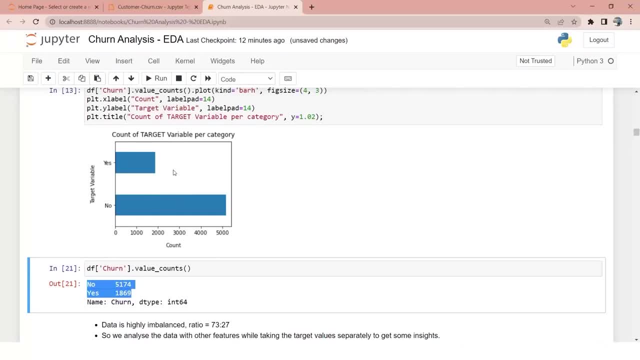 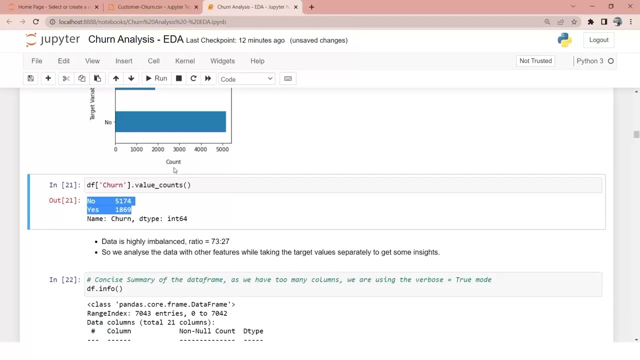 the insight here is: the data is highly imbalanced. it is not in the ratio of one is to one and almost 74 percent of the people are active and rest are getting churned right. so our further insights analysis has to be done to understand more about the people who are churning. 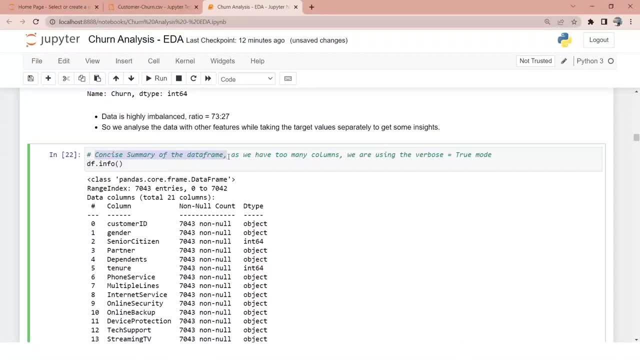 then i am doing a dot info concise summary of the data frame. as we have too many columns, we are using verbose equals to true, verbose equals to true. i'm not using it, so i will just. that's it. i'll just remove this part. verbose equals to true is another thing. for example, 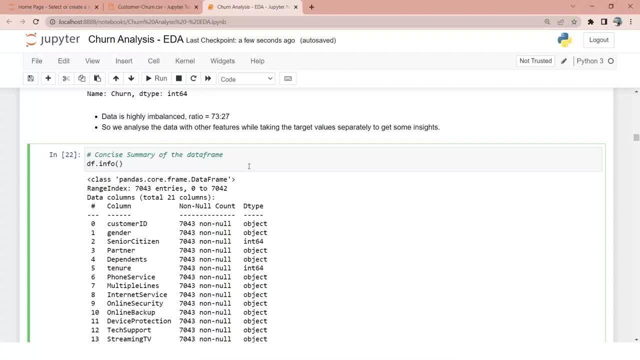 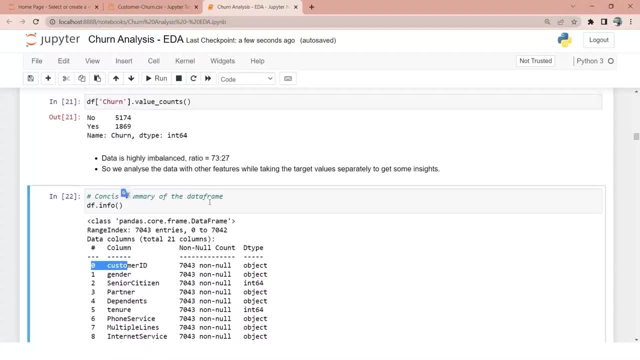 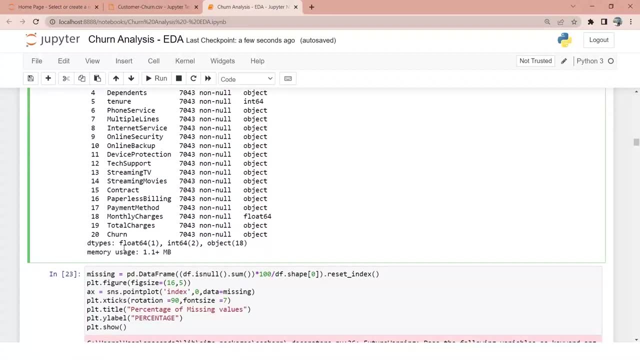 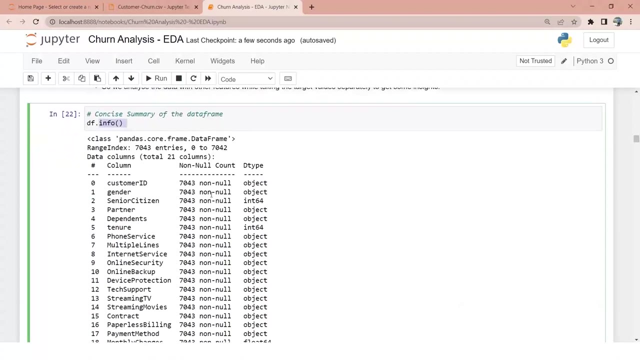 properly, you will not be able to see all the columns. if you mark verbose equals to true, it will be scrollable and you can scroll through all the columns. in this case we are just having 21 columns, so we don't need that option, so i'm just using dot info, which basically gives me an. 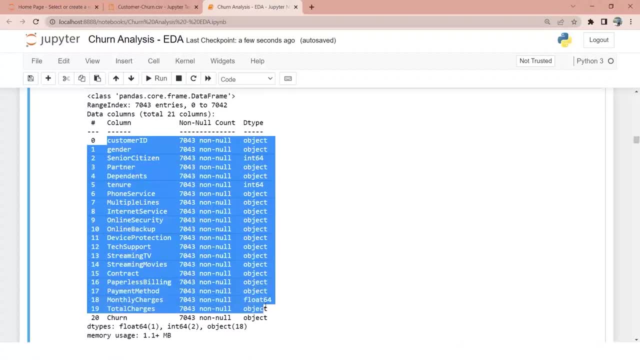 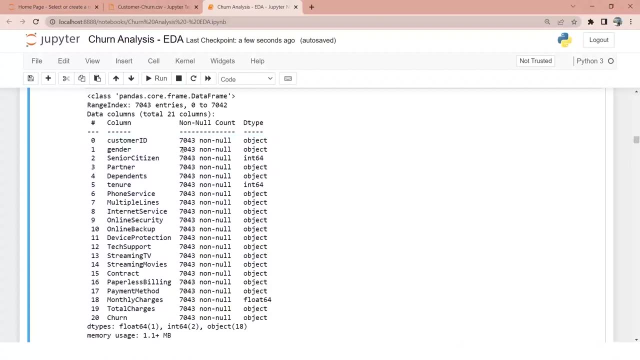 insight like this and i could see that most of the records here are completely open. okay, there is no null values, but one problem is total charges. you can see, total charges is an object type and object basically means a string type. and if total charges would be having null? 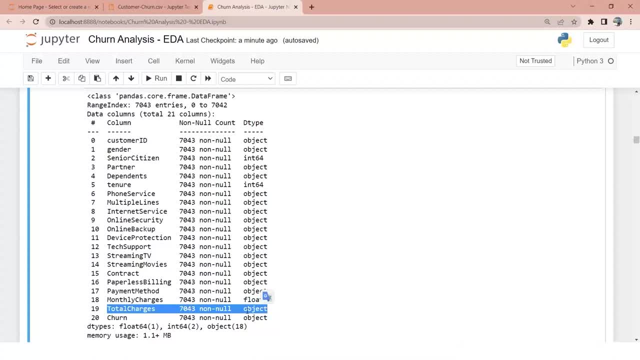 values, then that null values will be treated as not null, because it's an object, because empty value is also a valid object, right, so we need to be careful about total charges. what i need to do is i need to convert this into numerical and then again check the dot info and 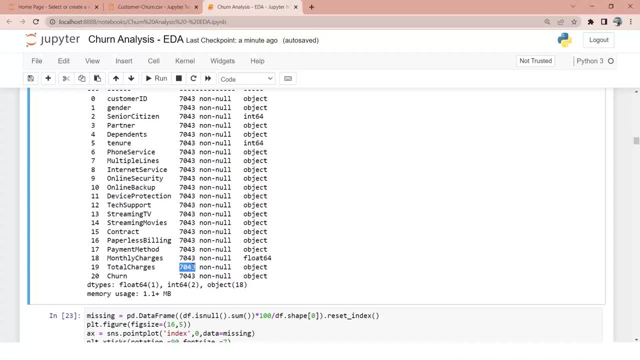 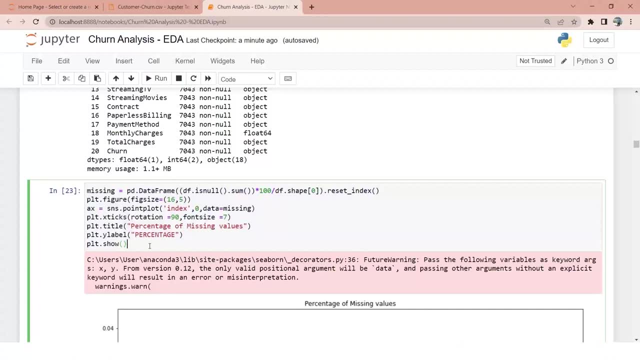 again, if i see 7043, then i will 100, be sure that there are no null values. the next piece of code is a very generic code that you can simply use it in any kind of use cases. this gives you a picture about the entire data set on what are the total percentage of missing values. so you you can simply 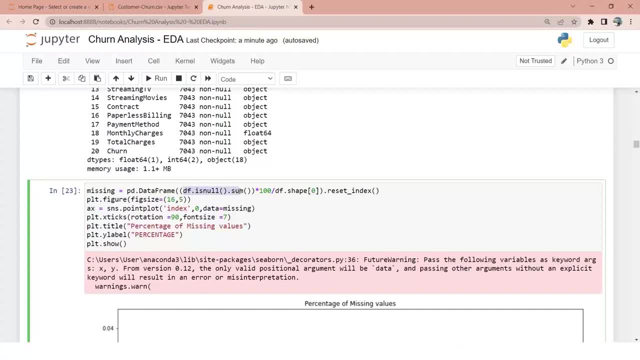 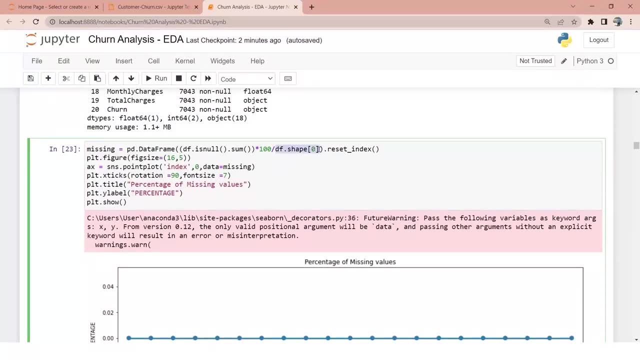 i'm just using that pd dot data frame. df dot is null dot sum. i'll multiply it with hundred so that i can see the percentage of the null values divided by df of shape dot reset index. the code is little bit complicated. if you take some time you will be able to understand it, but you can. 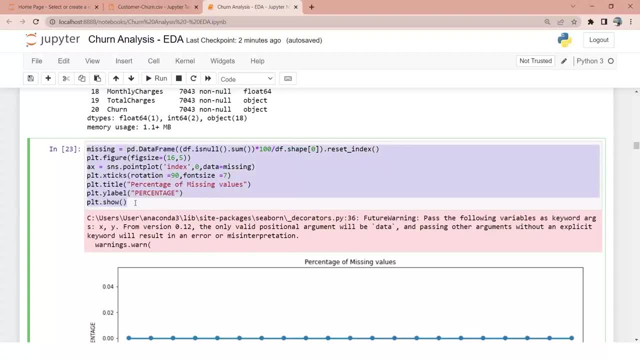 simply copy paste this piece of code in any kind of use cases that you are working with blindly. you just have to deal with all the variables. if all the results are equal, then all the variables you are studying aren't valid completely. there is no sense in that form. it just doesn't. but you 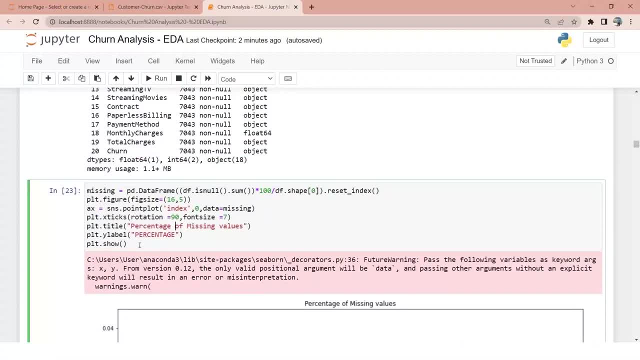 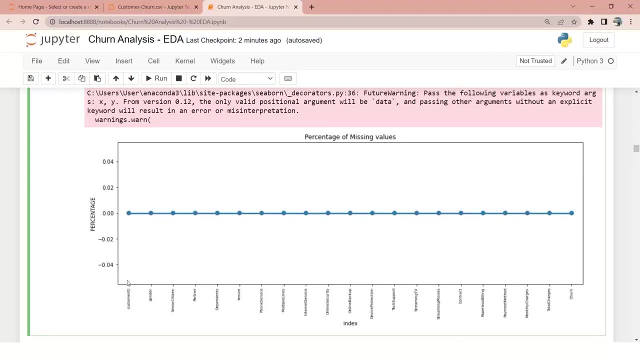 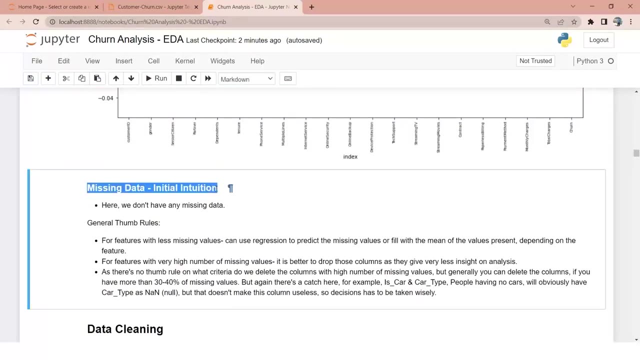 if all the data types are completely fine. just blindly copy paste this code and you will be able to get a graph, something like this, which talks about the percentage of missing values of all the columns in your data set. so the missing data, initial intuition- why are we capturing? 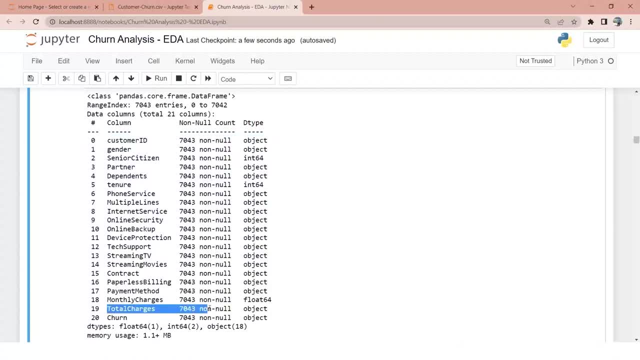 but one problem is total charges. you can see, total charges is an object type and object basically means a string type. and if total charges would be having null values, then that null values will be treated as not null because it's an object, because empty value is also a valid object, right? so we need to be careful about total charges. 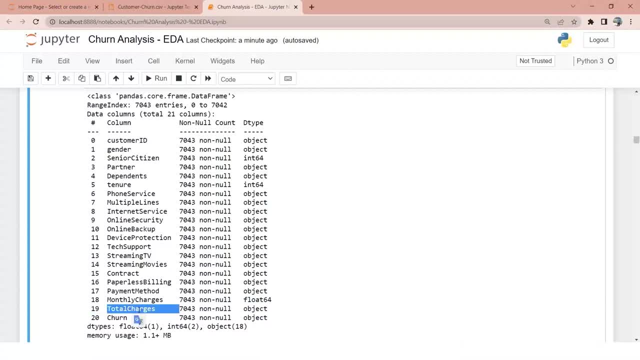 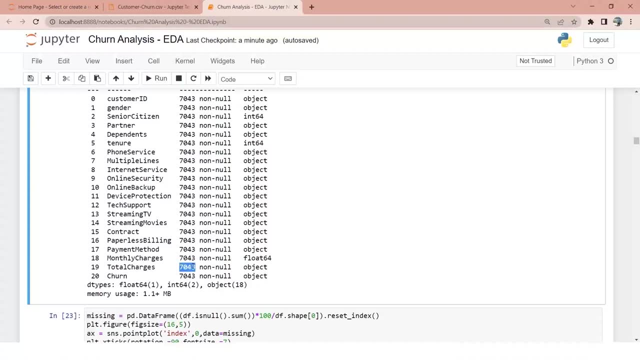 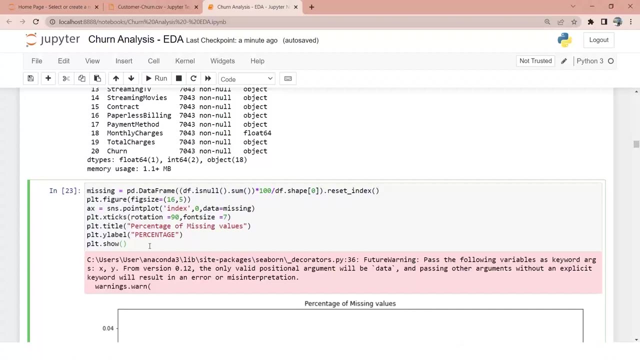 what i need to do is i need to convert this into numerical and then again check the dot info and again, if i see 7043 then i will 100, be sure that there are no null values. the next piece of code is a very generic code that you can simply use it in any kind of use cases. this: 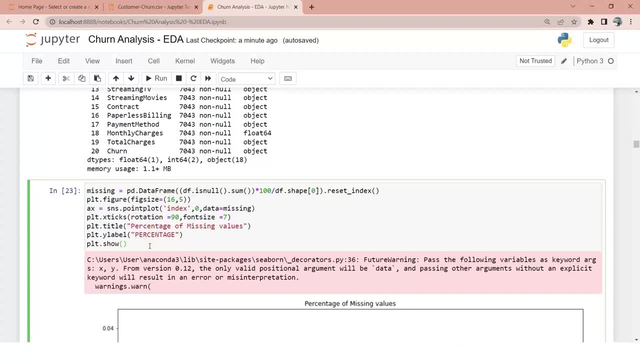 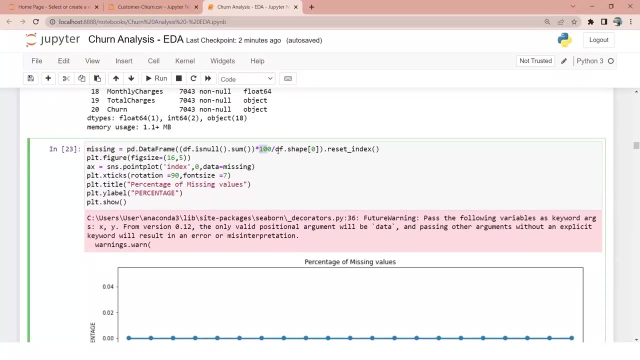 gives you a picture about the entire data set on what are the total percentage of missing values. so you you can simply see. i'm just using the pddata frame df. dot is null, dot sum. i'm multiplying it with 100 so that i can see the percentage of the null values. 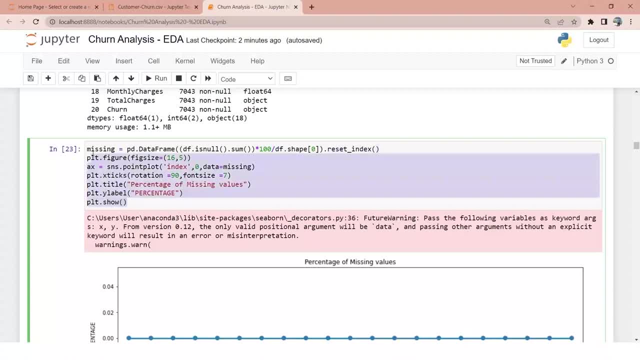 divided by df of shape dot reset index. the code is little bit complicated. if you take some time you will be able to understand it, but you can simply copy paste this piece of code in in the emails that you are using that PDF frame because we have df null value. Need We Understand Something? copied toothpaste to using it so you can get the data frame. once you这 paste view now in the other view that you are using in the other view, you will get the data frame you are put where you are using this instead of the PDF resting. you will get more. then you will get a collection for that data frame and you have to effectively utilize it. 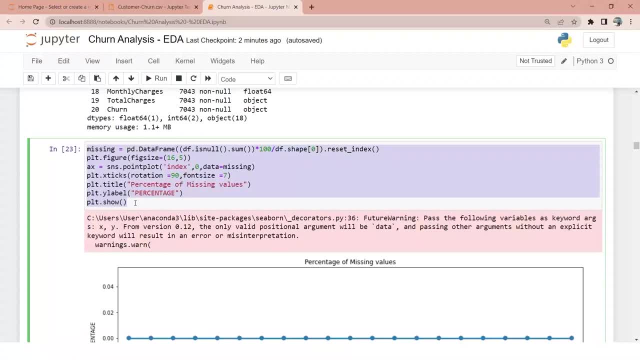 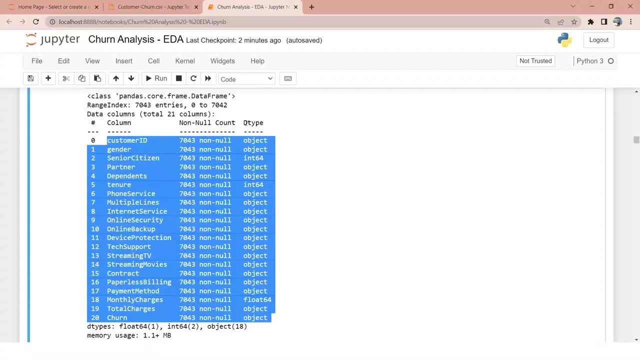 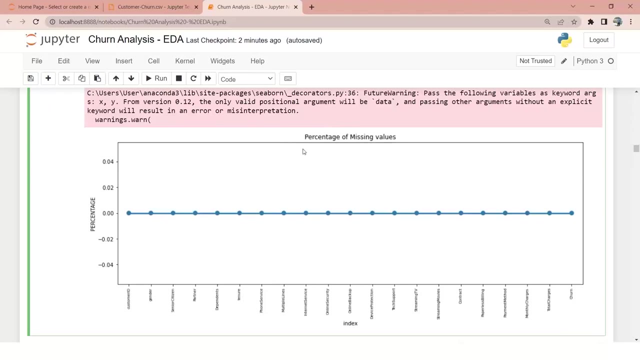 in any kind of use cases that you are working with blindly. you just have to deal with all the variables. if all the data types are completely fine, just blindly copy paste this code and you will be able to get a graph- something like this, which talks about the percentage of missing values. 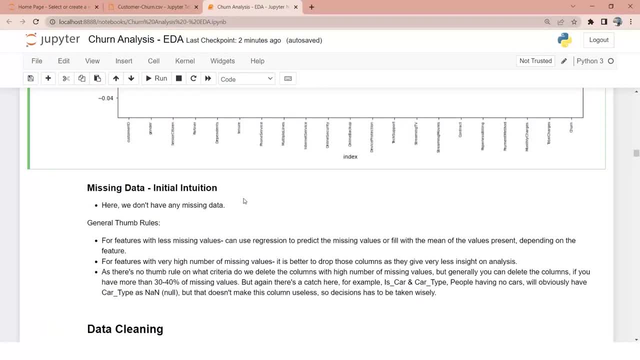 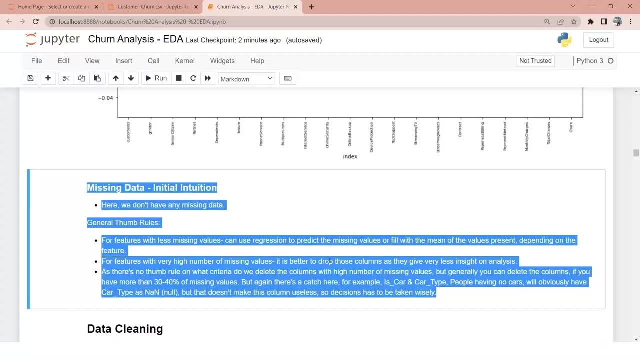 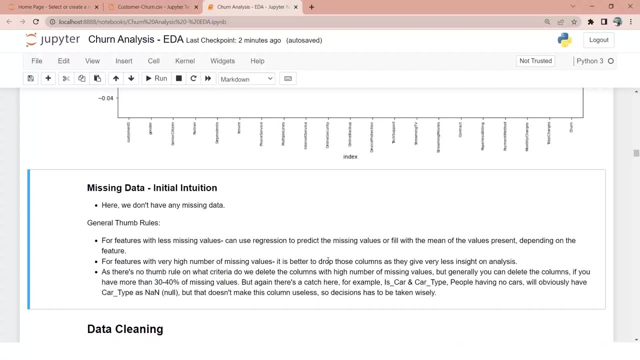 of all the columns in your data set. so the missing data, initial intuition. why are we capturing all these insights after every step? is because your final eda, the output of your edr insights, your output of your eda, has to go to your higher management or to your customer. 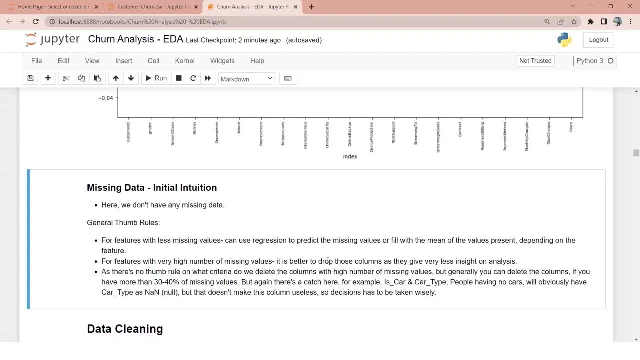 all these insights after every step is because your final eda, the output of your edr insights, your output of your eda, has to go to your higher management or to your customer so that they will be able to understand the summarized data. nobody will be able to see at your code and understand. 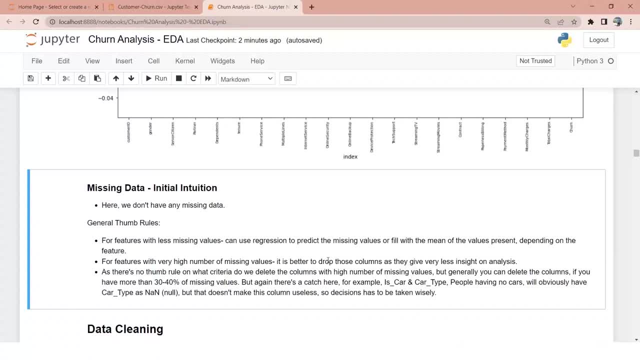 so that they will be able to understand the summarized data. nobody will be able to see at your code and understand. coding is for people who are into analysis, people who are the engineers. right for non-coding people or for higher managements. they understand visuals, they understand. 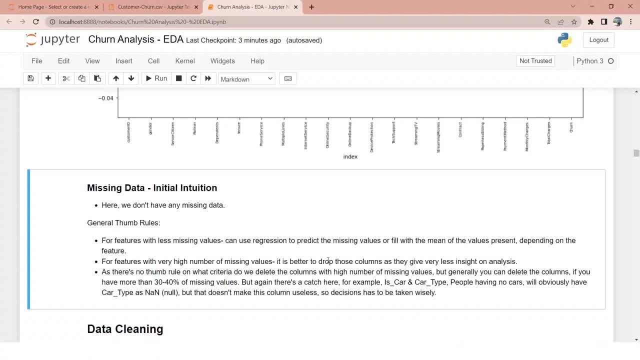 your final insights. so you have to be good enough to whatever you have understood in the ada process. you have to be good enough in the data storytelling part. you have to be good enough in your visual analytics so that you can portray them a proper insights. so the missing. 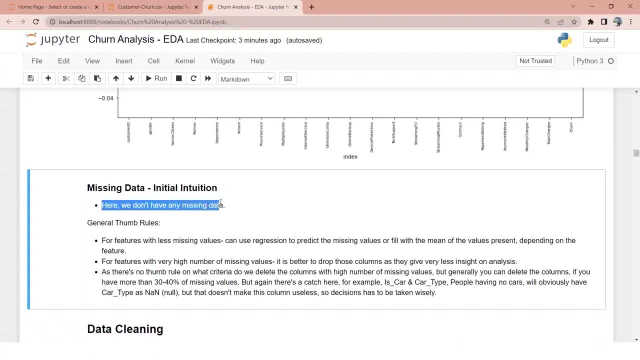 value: missing data. initial intuition is that here we don't have any missing data. general rules: again: here we don't have any missing data. but there is something in my mind that total charges data type is not proper. so in the data cleaning part i will be dealing with that and i will again do the missing value imputation. 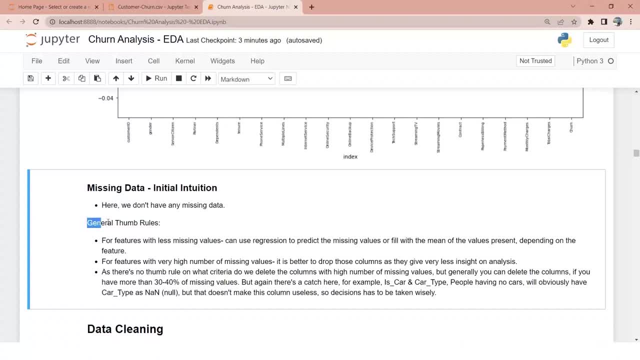 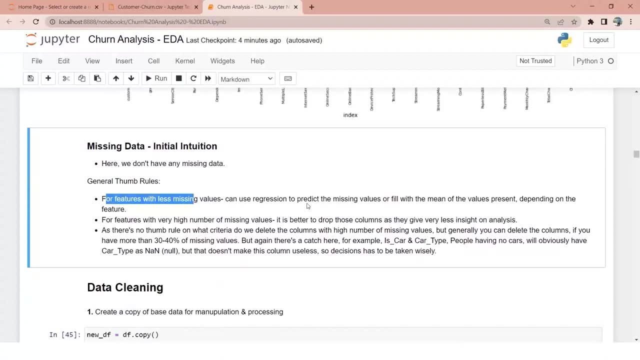 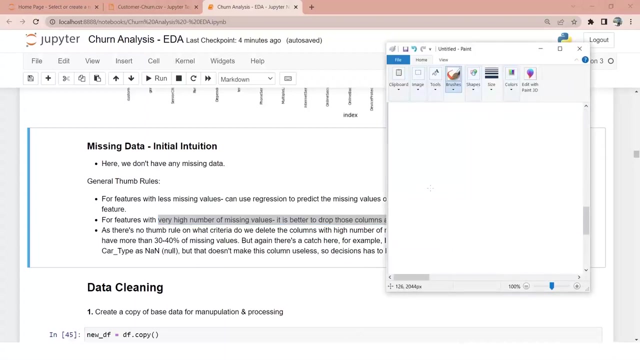 so it has to be a repetitive process. the general thumb rules for missing data is for features with less missing values. we can use regression to predict the missing values or fill with the mean of the values present. for features with high number of missing values it is better to drop. so it simply means that if you have a column, let's say h. 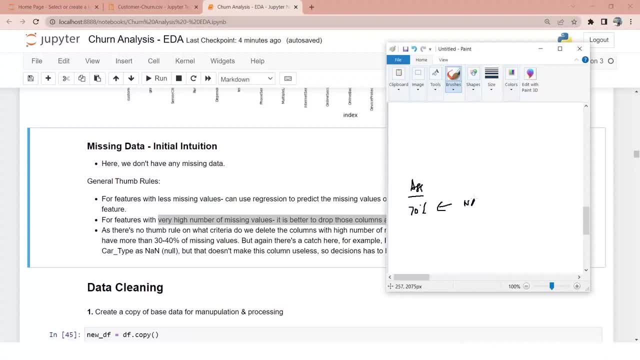 and 70 percent of the column is empty. there is no need of imputing, because if you impute, that means you are manipulating almost 70 percent of the records, which makes no sense. so you can simply get rid of it. but before getting rid of it you should also analyze: is there any column that 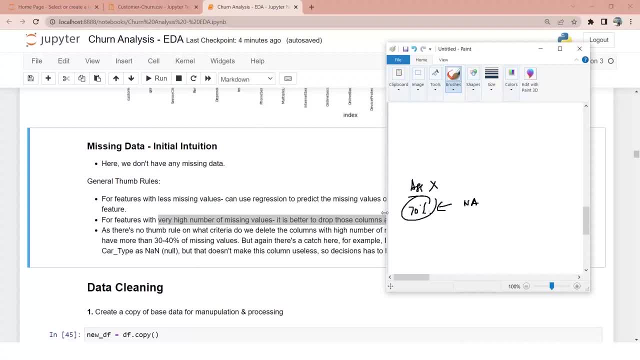 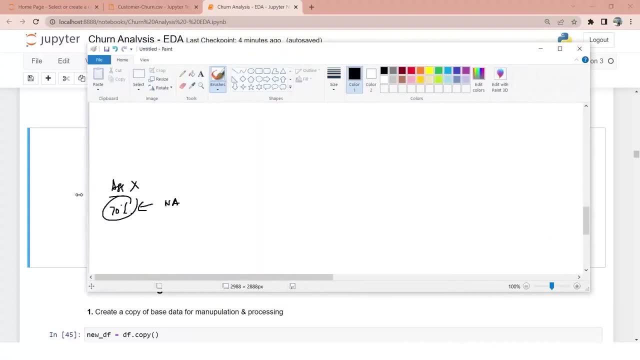 is impacted by this column or is there a column that impact this column? one example will be- let's say i'll talk about a scenario not specific to customer churn- a generic example. let's say there is a column called as car type. you are analyzing some insurance related data and there is a column called as car type- 70 percent of the data points. 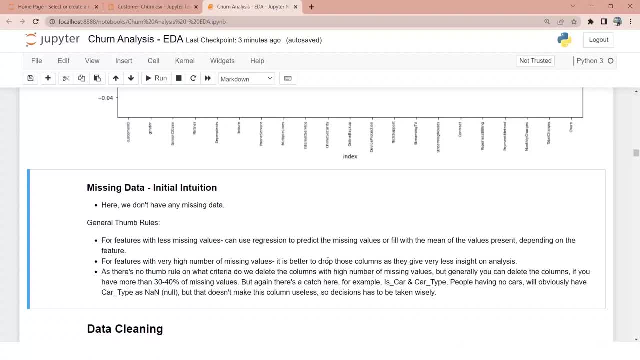 coding is for people who are into analysis, people who are the engineers right for non-coding people or for higher managements. they understand visuals, they understand your final insights. so you have to be good enough to whatever you have understood in the ada process. you have to be good enough in the data storytelling part. you have to be good. 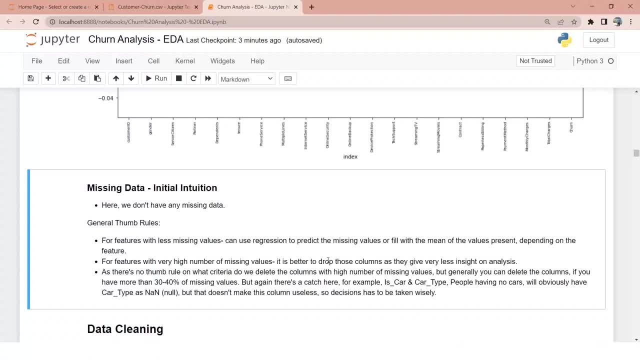 enough in your visual analytics so that you can portray them a proper insights. so the missing value, missing data. initial intuition is that here we don't have any missing data. general thumb rules: again, here we don't have any missing data, but there is something in my mind that total charges. 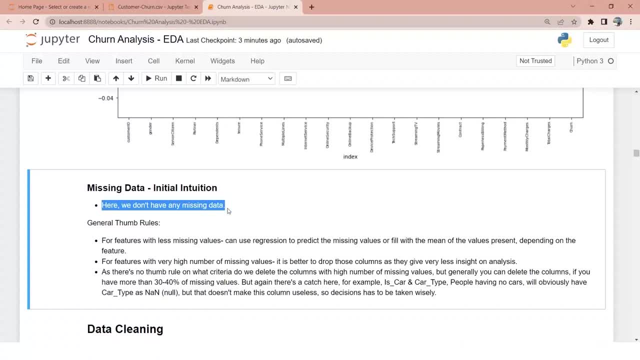 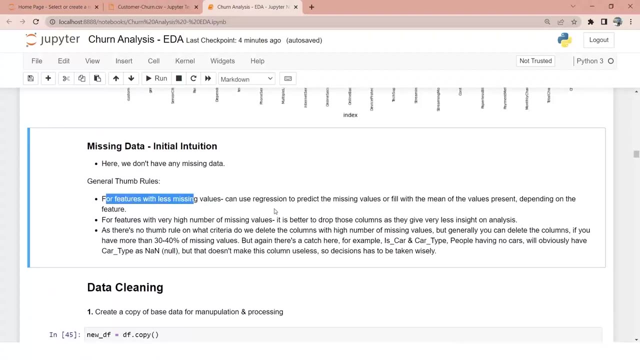 data type is not proper. so in the data cleaning part i will be dealing with that and i will again do the missing value imputation. so it has to be a repetitive process. the general thumb rules for missing data is for features with less missing values. we can use regression to predict the missing values or fill with the mean. 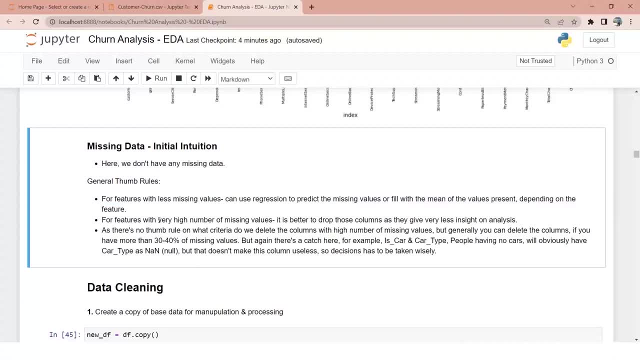 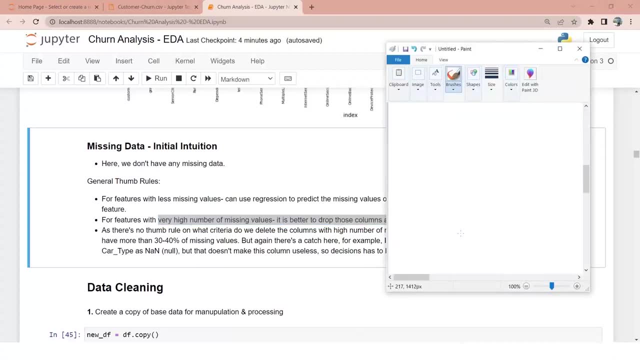 of the values present. for features with high number of missing values it is better to drop. so it simply means that if you have a column, let's say h, and 70 percent of the column is empty, there is no need of imputing, because if you impute that means you are manipulating almost 70 percent of the records. 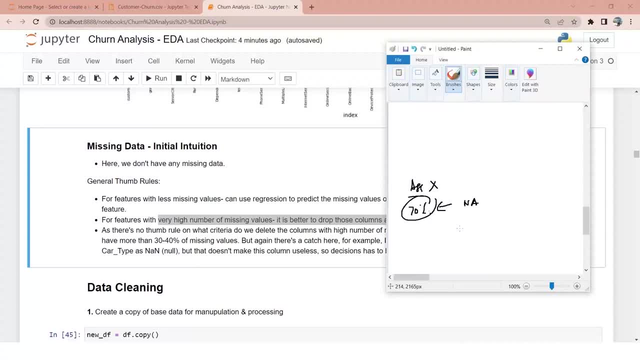 which makes no sense. so you can simply get rid of it. but before getting rid of it, you should also analyze: is there any column that is impacted by this column, or is there a column that impacts this column? one example will be: let's say, i'll talk about a scenario. 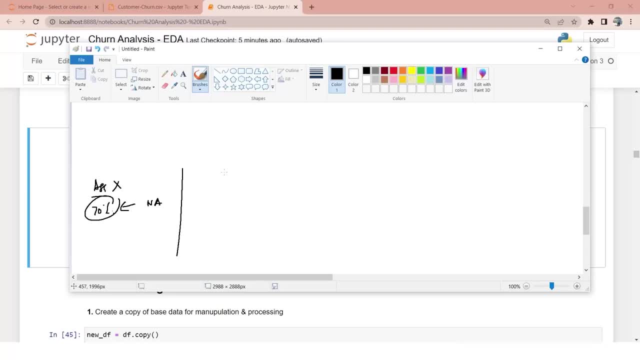 not specific to customer churn. a generic example. let's say there is a column called as car type- you are analyzing some incidence related data- and there is a column called as car type. 70 percent of the data points are null. them is suv- null, null, null, null, xuv, null, null, null, suv, and so on. 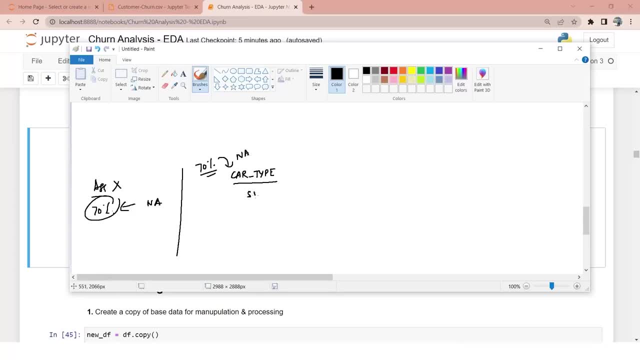 are null. so some of them is suv- null, null, null, null, xuv, null, null, null, suv and so on. will you be able to delete it because it has 70 percent null values? before deleting, you will have all the columns. is there a column that impact this column? let's say there is a column called, as is, car. 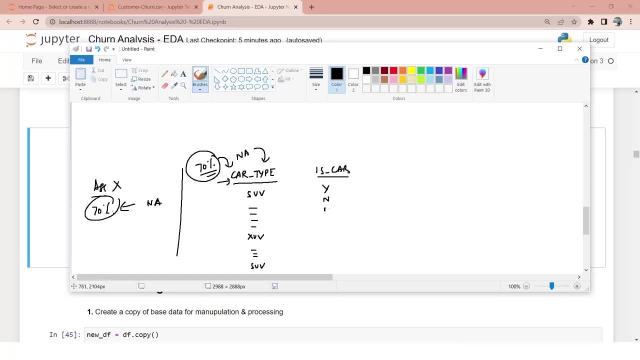 and the records are something like this: n, n, n, n, y, n, n, n and then y, which basically means if somebody has a car or not, somebody is a car. the type is suv. car type is xqb. car type is suv: obviously people who don't have a car, they will have null values right. so in this, 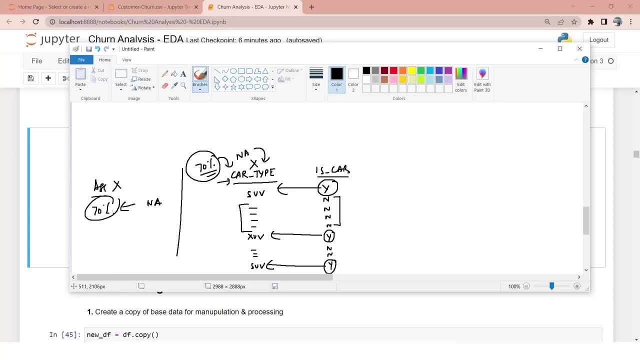 case, instead of dropping this column, i will just simply impute it by no car, no car, right, so this is a better technique to impute data. so before dropping, there is a general thumb rule to drop. if you have more than 50 percent of the null values in the entire column, drop it. 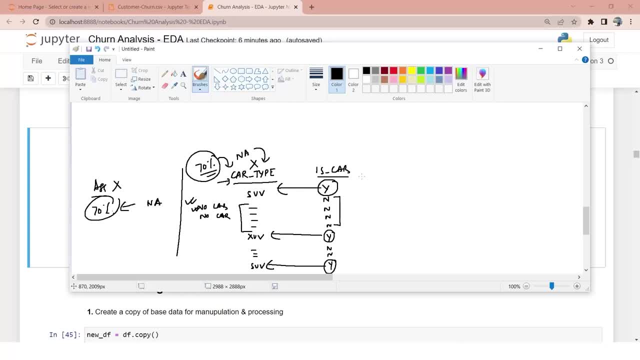 but before dropping, try to use your domain knowledge, analyze it whether that column is impacted by another column or any other column that is getting in. you know any other column that this column is getting impacted from any of these things. then try to analyze them and deal with it. 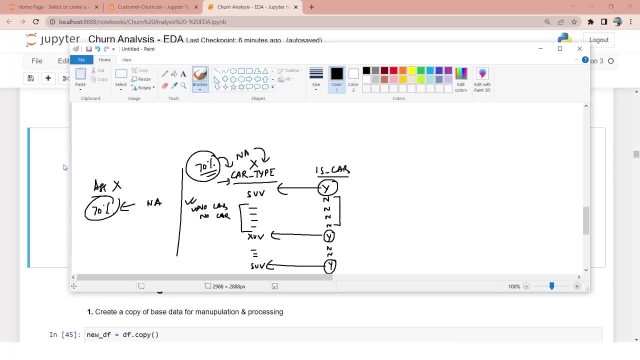 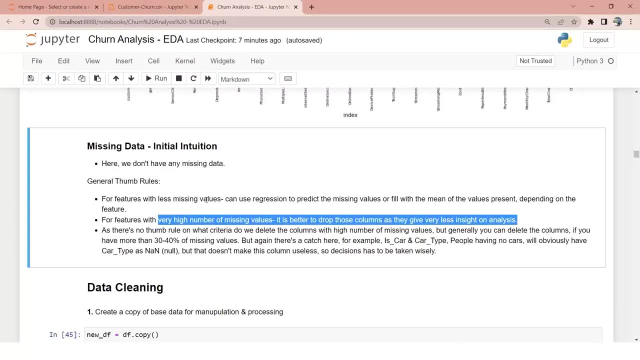 in case you have any doubts, any questions, you can always ask your peers, your superiors, your people who are basically managing you, for any kind of doubts before taking a final call. but again, there is a catch here that this is the same example that i took and 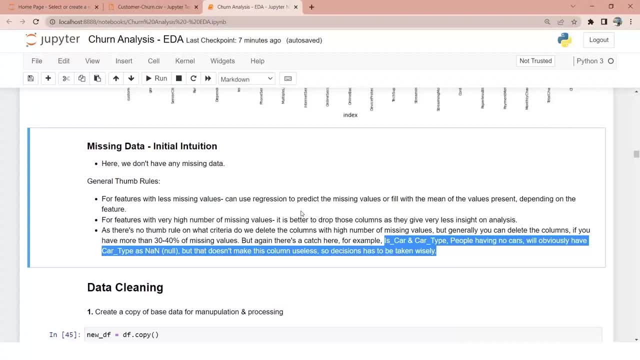 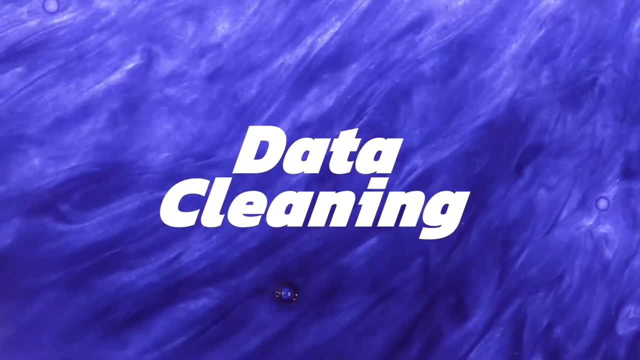 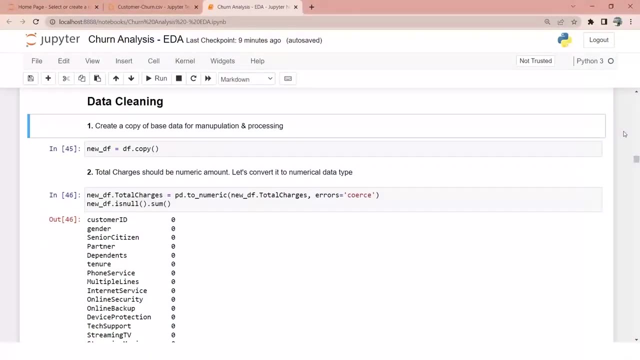 you can take your decisions wisely. that's all about very initial steps. in the next video, we shall be talking about the data cleaning part, jumping into the next part, which is your data cleaning part now. in this part, we will be doing some data cleaning activities, which includes: 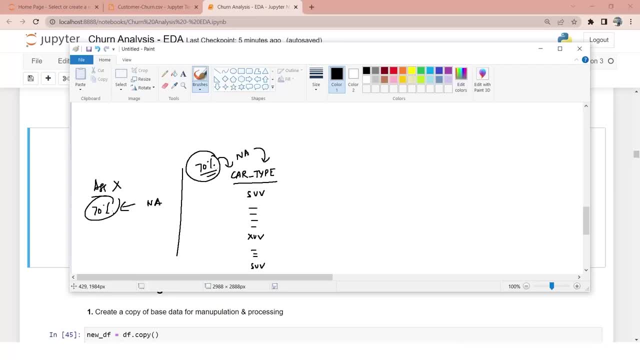 will you be able to delete it because it has 70 percent null values. before deleting, you will have to analyze all the column columns. is there a column that impact this column? let's say there is a column called as is car, and the records are something like this: n, n, n, n, y and n, n and then y, which basically means 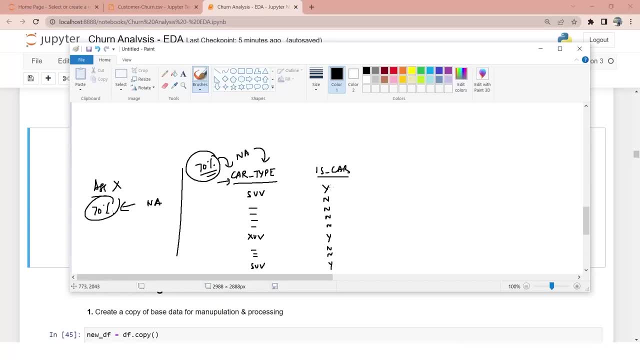 if somebody has a car or not. somebody is a car, the type is suv, car type is xqv. car type is suv- obviously people who don't have a car. they will have null values, right. so in this case, instead of draw, dropping this column, i will just simply imputed by no car, no car, right. so this is a better. 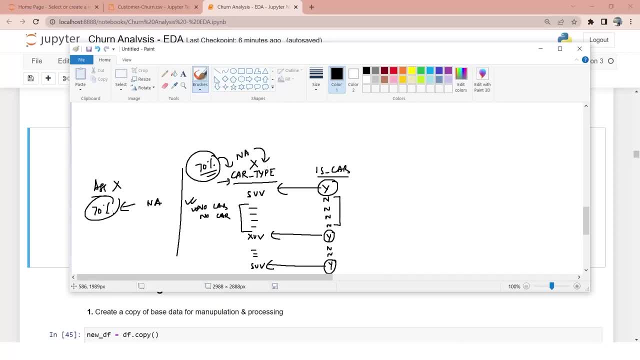 technique to impute data. so before dropping, there is a general thumb rule to drop. if you have more than fifty percent of the null values in the entire column, drop it. but before dropping try to use your domain knowledge, analyze it whether that column is impacted by another. 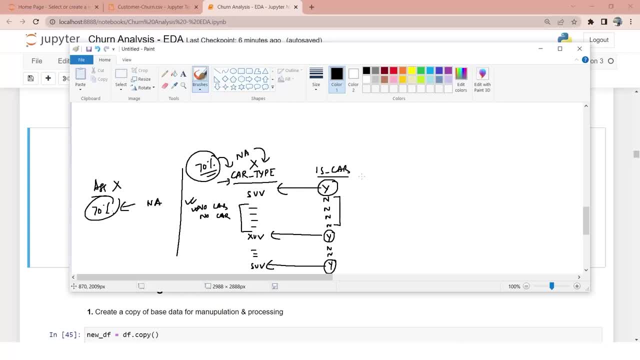 column or any other column that is getting in. you know any other column that this column is getting impacted from any of these things, then try to analyze them and deal with it. in case you have any doubts, any questions, you can always ask your peers, your superiors. 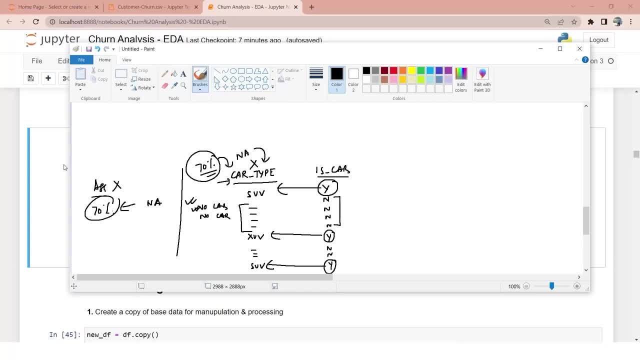 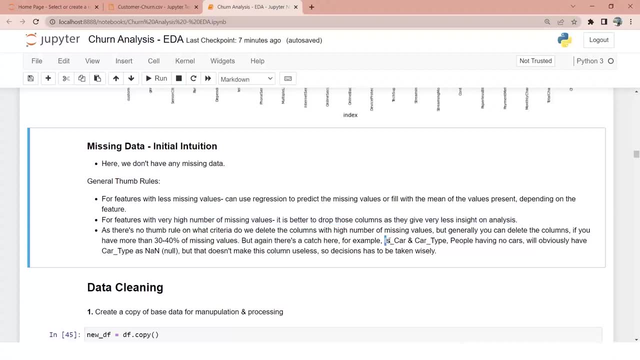 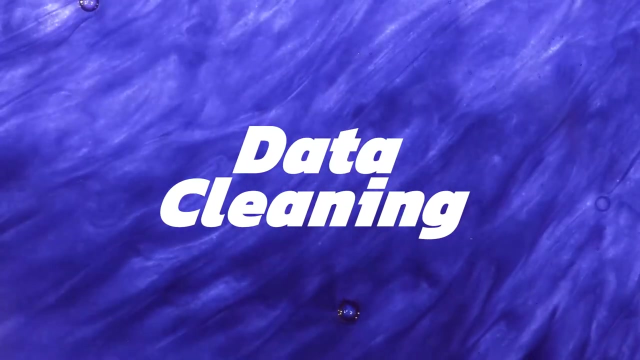 your people who are basically managing you for any kind of doubts before taking a final call. but again, there is a catch here: that this is the same example that i took and you can take your decisions wisely. that's all about very initial steps. in the next video, we shall be talking about the data cleaning part. 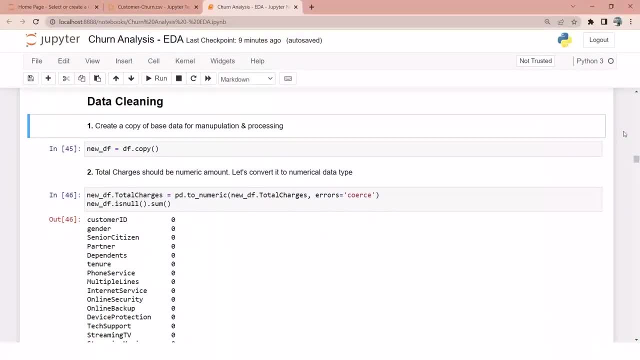 jumping into the next part, which is your data cleaning part. now, in this part, we will be doing some data cleaning activities, which includes conversions of invalid data type to another data type or some large volume of data like values, imputations and so on. let's get started. so we already 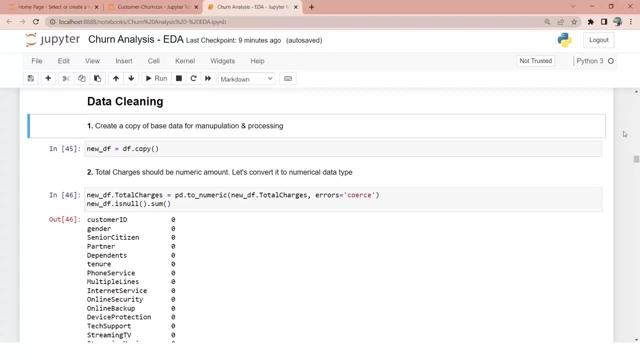 conversions of invalid data type to another data type, or some null values, imputations and so on. let's get started. so we already had this data frame called as df. i don't want to impact anything for this particular data frame, so i'm taking a copy and i'm creating another data frame. 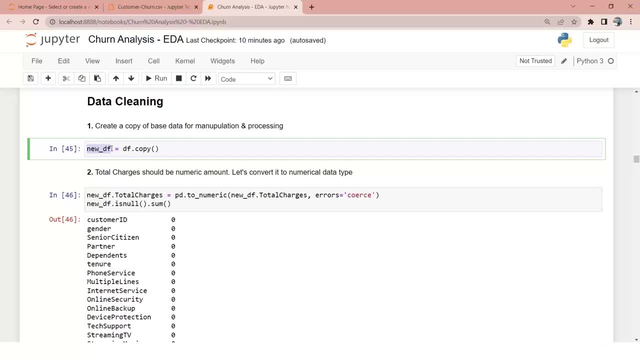 and this is a common practice in eda or whenever we write codes we don't. at some point of time, we feel that we should take backups. and it's a good step as well, right, because you don't impact your variables further. so i'll take a backup of my df. if something goes wrong, i can come back easily and then i will be creating a new. 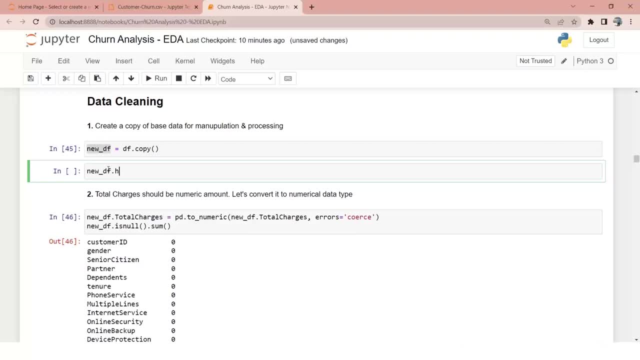 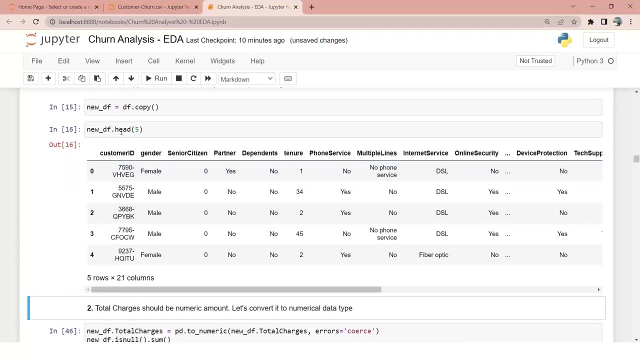 df, which is very similar to what df was. if you want to have a look at it. this is how. this is how your new df looks in- a df which is a 해야 keaye object, and what you will need to do to create a new one is to 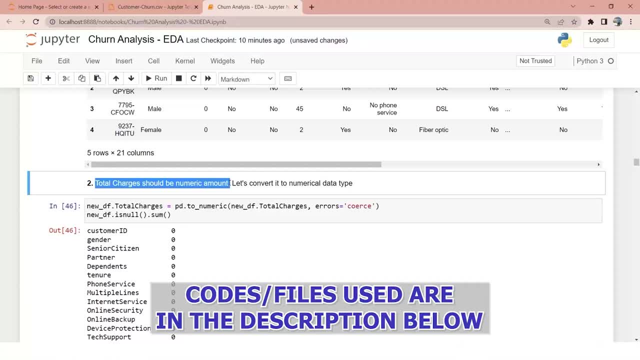 create a new df. in your case, we are going to create a new df and what we did here is to create a new df, and we will be creating a new df in your case and we will be taking an example of the different types of dfs as the standard one. so we will be going over the data frame data in an example of. 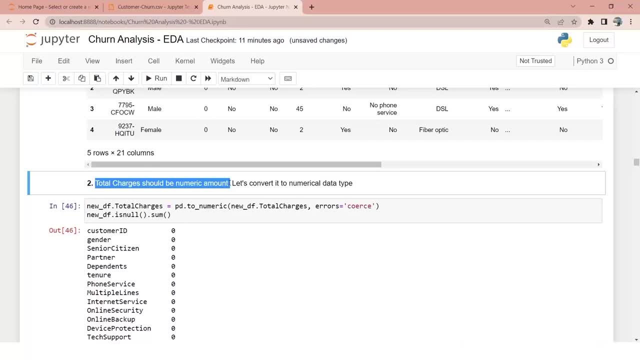 df and we will be taking, perhaps, for example, this one, this one you see here. this is an example of df, which is a public use df. so if you want to simplify the data frame, you can create a new df by using this, an example of the df, and you can take a look at this particular df-adbox. so you will be. 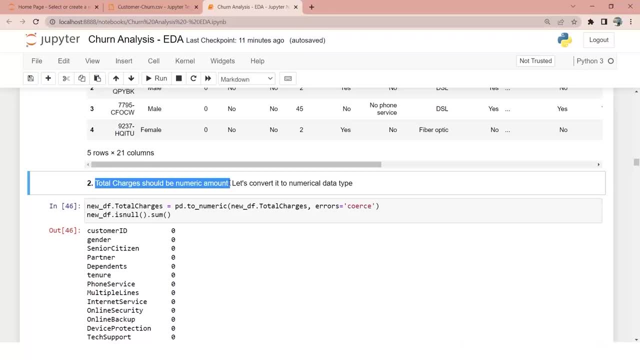 and convert those type of columns to numeric so that you can do the further steps. so total charges should be numeric, so i'm converting them into numerical data. so df new df dot total charges is pd dot to numeric. now pd dot to numeric is used to convert a data frame column to numeric. 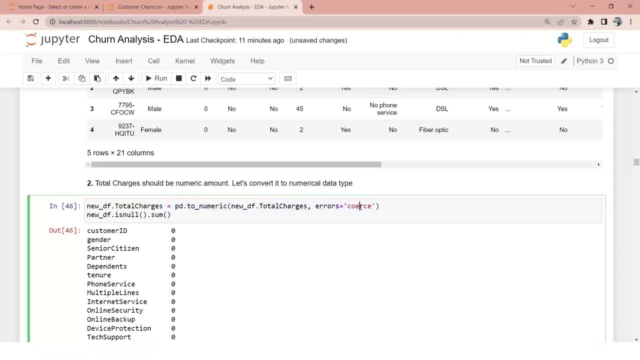 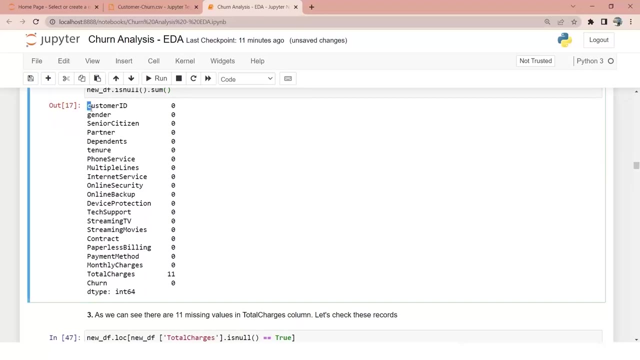 attribute and i'm passing total charges. error equals to coerce. and then i'm doing new df dot is null dot sum. you do this or you do new df dot info. both are same. you can see the output of this is very clear. everybody is every column is having zero, null values. 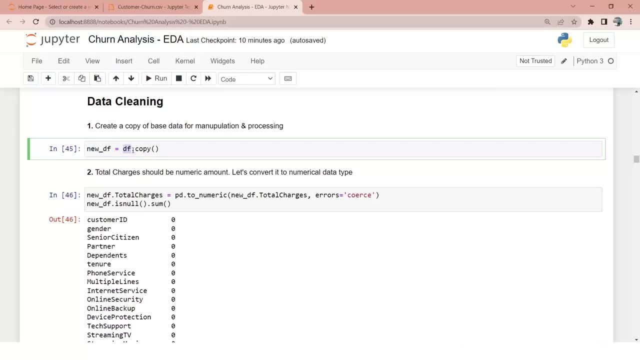 had this data frame called as df. i don't want to impact anything for this particular data frame, so i'm taking a copy and i'm creating another data frame- and this is a common practice in eda or whenever we write codes we don't at some point of time we feel that we should. 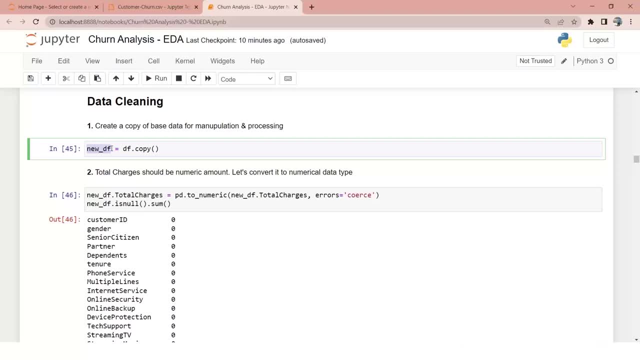 take backups and it's a good step as well, right, because you don't impact the data frame and i'm taking a copy and i'm creating another data frame and at a certain point we feel because you don't impact your variables further, so i'll take a backup of my df if something goes. 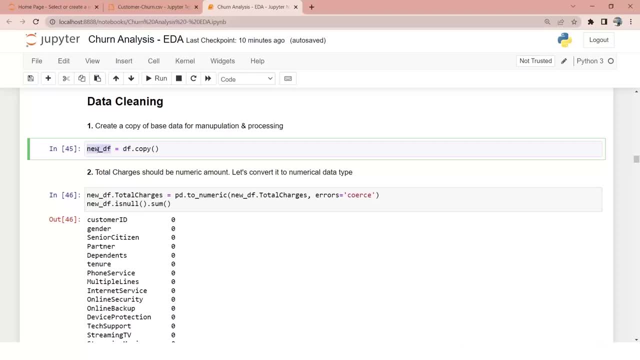 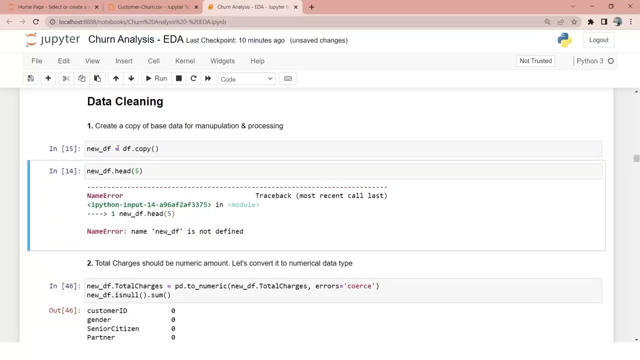 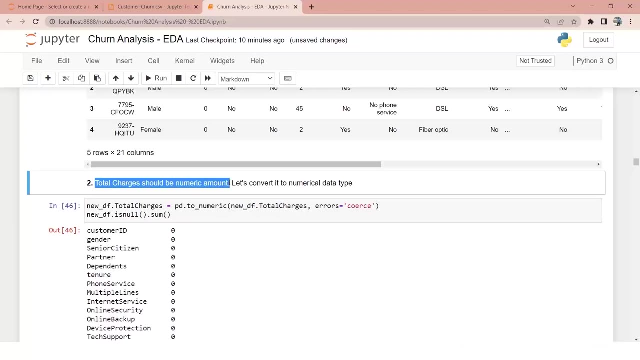 wrong, i can come back easily and then i will be creating a new df which is very similar to what df was. if you want to have a look at it, this is how. this is how your new df looks- a replica of df. total charges should be numeric amount, as i told you that total charges was an object type. 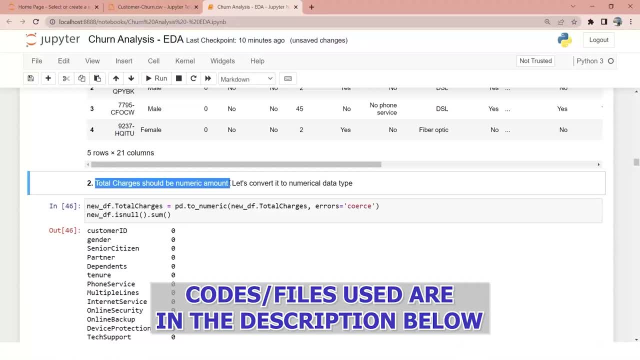 your focus should have been to create it as a numeric. there could be multiple instances where your data is numeric in excel sheets or in your csv files. while reading the data into panda's data frame, it could be treated as an object type. there could be scenarios, so you always have to. 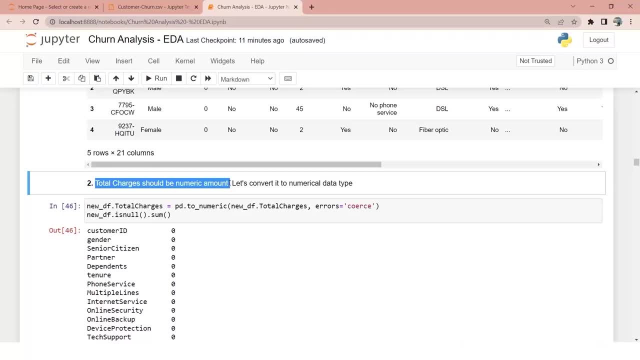 keep an eye and convert those type of columns to numeric so that you can do the further steps. so total charges should be numeric, so i'm converting them into numerical data. so df- new df dot total charges is pd dot 2 numeric. now pd dot 2 numeric is used to convert a data frame column to numeric attribute and i'm 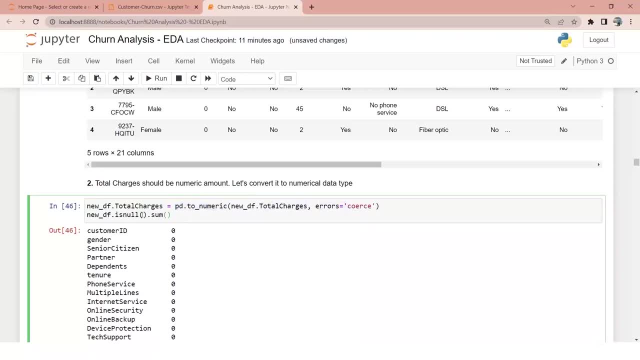 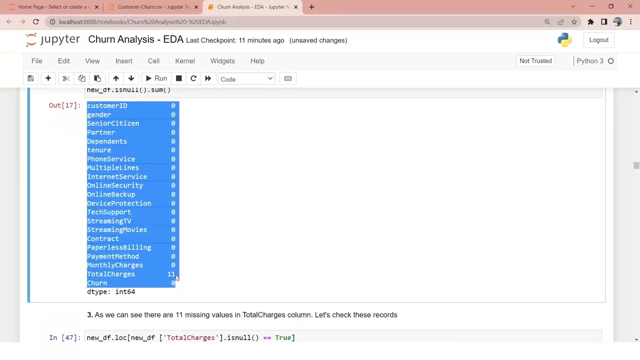 passing total charges. error equals to coerce. and then i'm doing new df dot is null dot sum. you do this or you do new df dot info. both are same. you can see the output of this is very clear. everybody is. every column is having zero, null values, total. 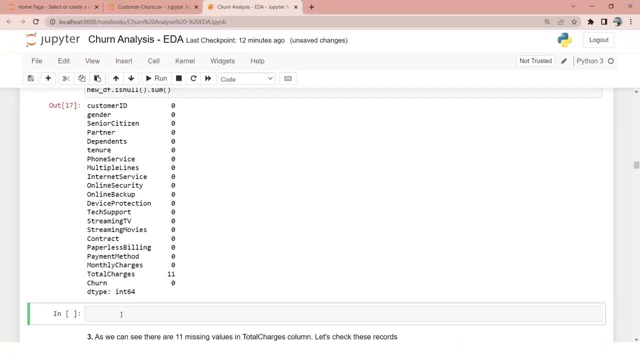 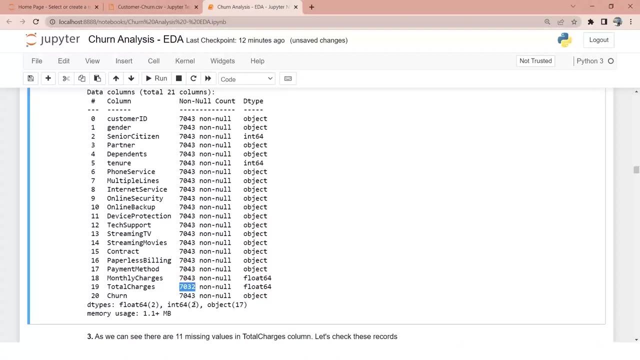 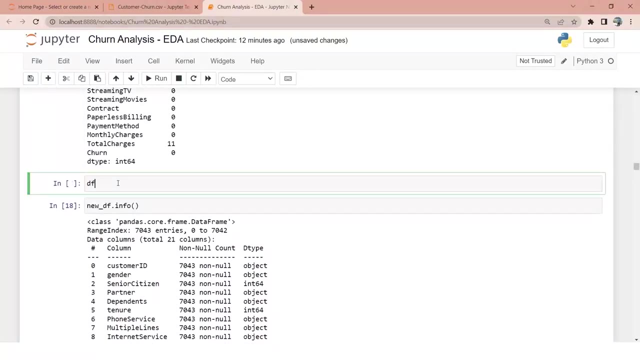 charges is having 11. if you also want to check the traditional approach of info, you can do that. info is telling me that i have 11 null values in total charges. if you remember, in the df, where we have not imputed anything, total charges was showing a seven. 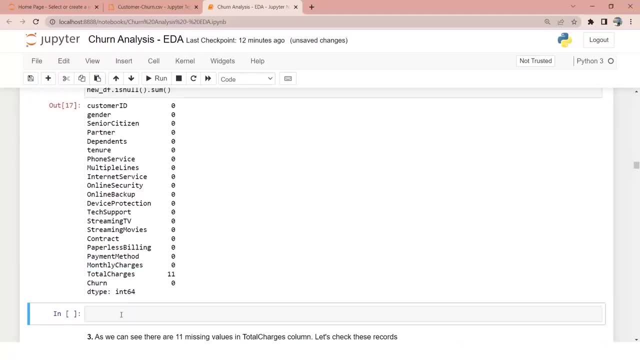 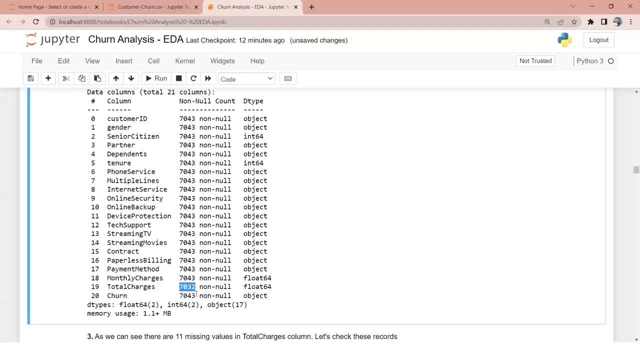 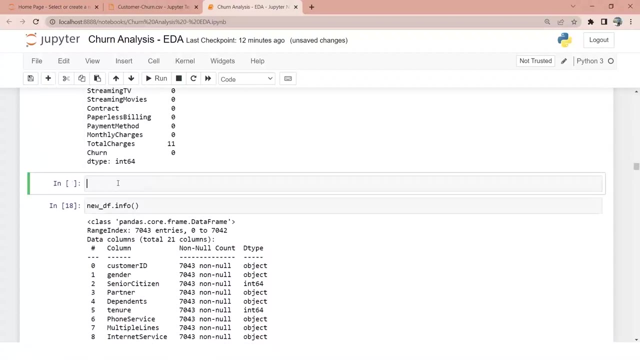 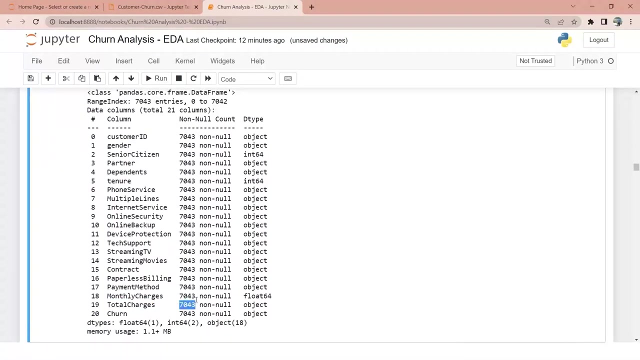 total charges is having 11. if you also want to check the traditional approach of info, you can do that. info is telling me that i have 11 null values in total charges. if you remember, in the df, where we have not imputed anything, total charges were showing a 7043, not null values. that means 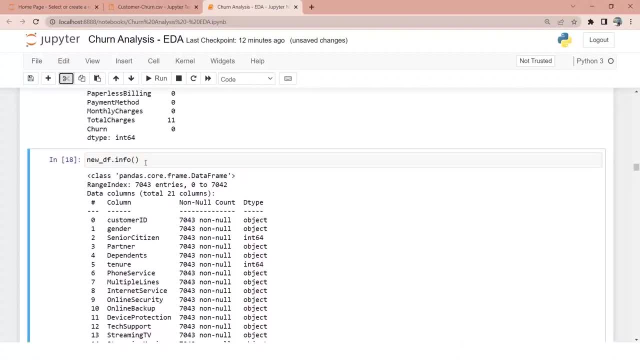 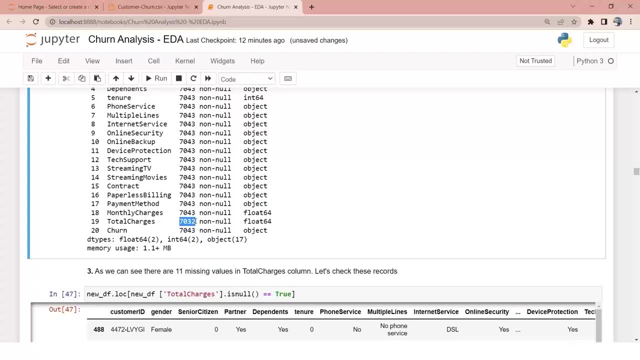 no null values. but that is a wrong assumption because it was an object type. now i can see there are null values. how many null values do we have? just 11 now. sometimes we ignore very small amount of null values if it is just five or six records, just one percent of the data. 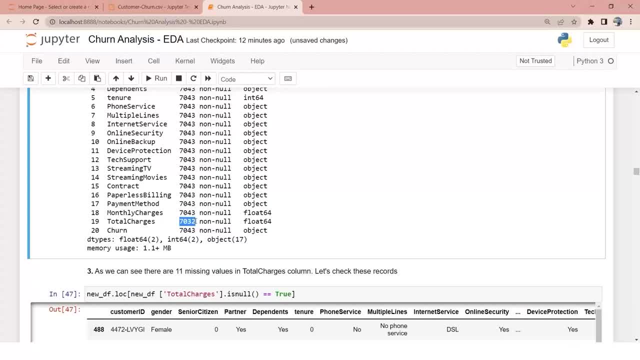 then it is better to ignore what information will be there in just 11 records, right? if i talk about the percentage of data, 11 by 7043 multiplied with 100 is not even one percent. it is less than one percent. 0.15 percentage of missing values. what should we do there? 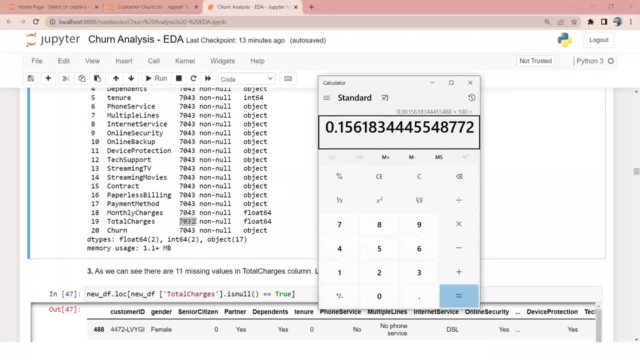 are two techniques. one of them: just impute it and, as total charges is a float object, you can impute it using mean value or median value, but i will delete it because another step is also to delete it, because they are just 11 records, just 0.15 percentage. so even if i delete 11 records, i don't think that i will miss. 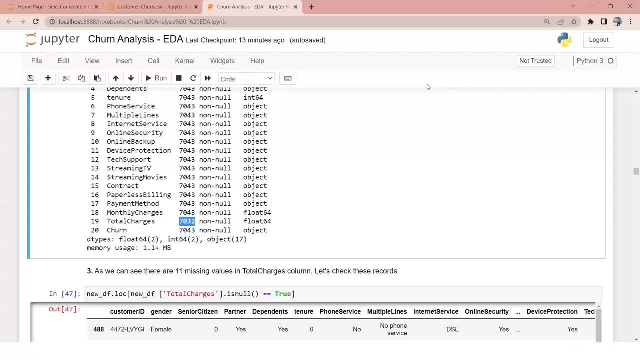 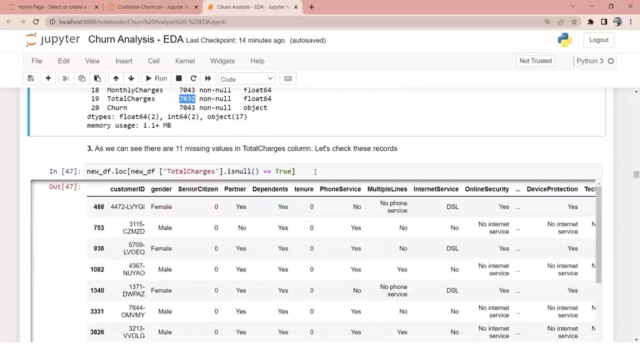 out on a huge amount of records, huge amount of information. if the total percentage would have been two to three percent or five percent or 10 or even till 30, i could have easily imputed it, because you cannot simply delete 30 of the records. it's almost 30, but in my case it is just 0.15, so i will delete it. so these were the null records. 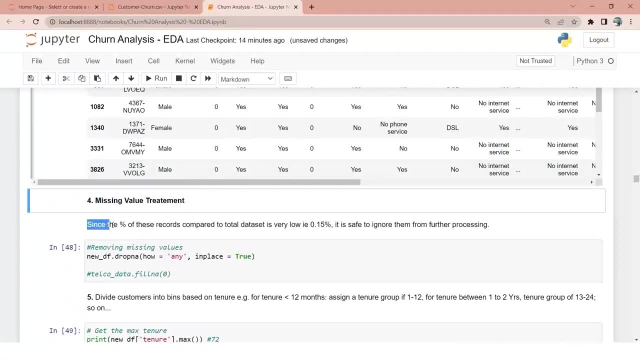 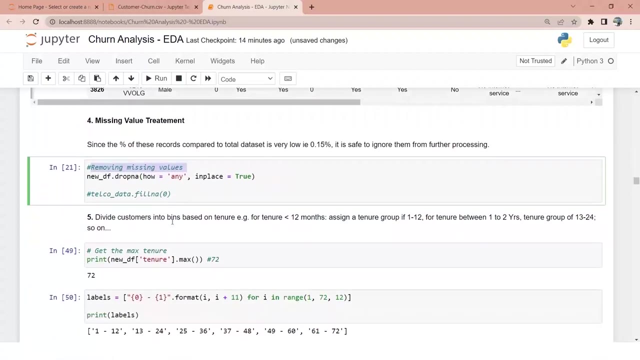 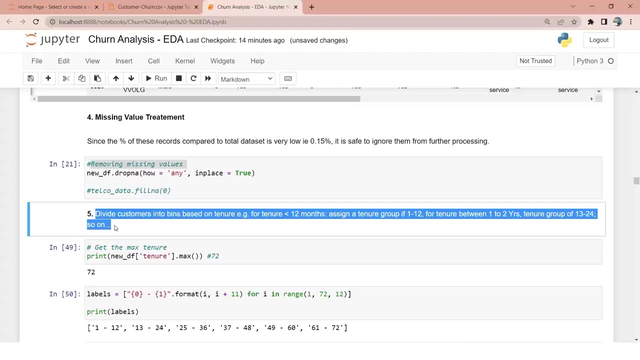 and then i'm doing a missing value treatment here. since percentage of these records are very low, it to ignore them from further processing. so i'm doing drop na how any in place equals to true. okay. so removing all the missing values divide the customers into bin. so my data cleaning is almost done. invalid data type is fixed: null. 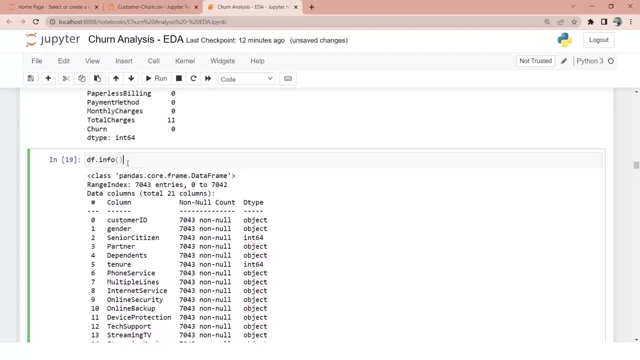 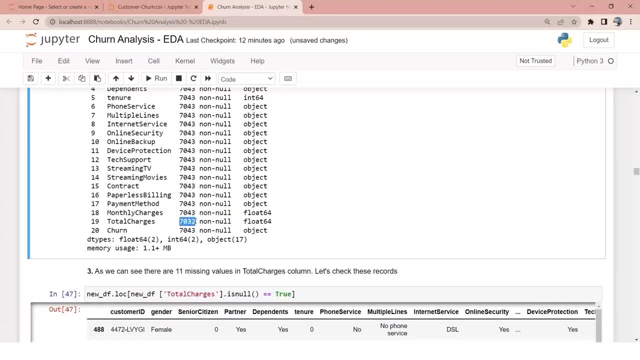 1043, not null values. that means no null values, but that is a wrong assumption because it was an object type. now i can see there are null values. how many null values do we have? just 11.. now, sometimes we ignore very small amount of null values if it is just five or six records just. 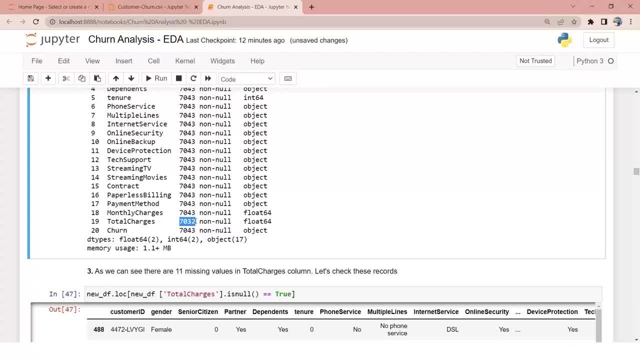 one percent of the data, then it is better to ignore what information will be there in just 11 records, right? if i talk about the percentage of data, 11 by 7043 multiplied with 100 is not even one percent. it is less than one percent. 0.15 percentage of missing values. what should we do? there are two. 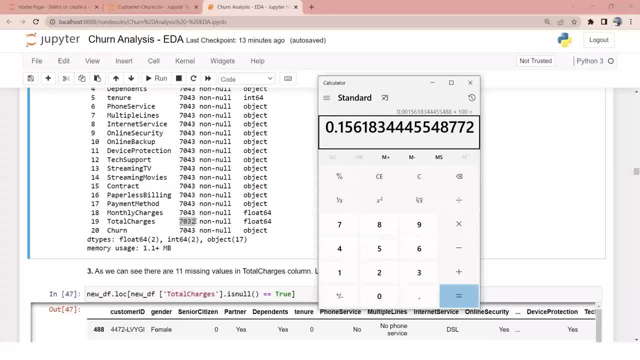 techniques. one of them just imputed and active total charges is a float object. you can impute it using mean value or median value, but I will delete it, because another step is also to delete it, because they are just 11 records, just 0.15 percentage. so even if I delete 11, 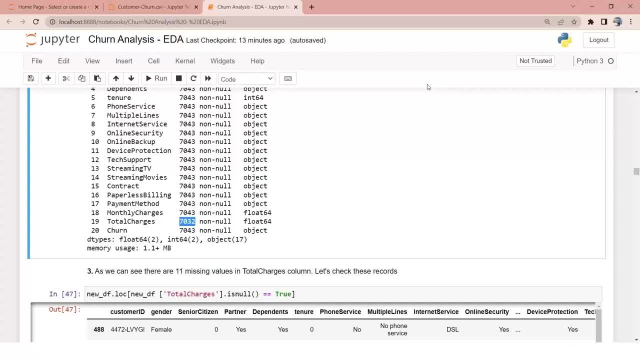 records. I don't think that I will miss out on a huge amount of records, huge amount of information. if the total percentage would have been 2 to 3 percent, or 5 percent or 10 percent or even till 30 percent, I could have easily imputed it, because you cannot simply delete 30 percent of the records. 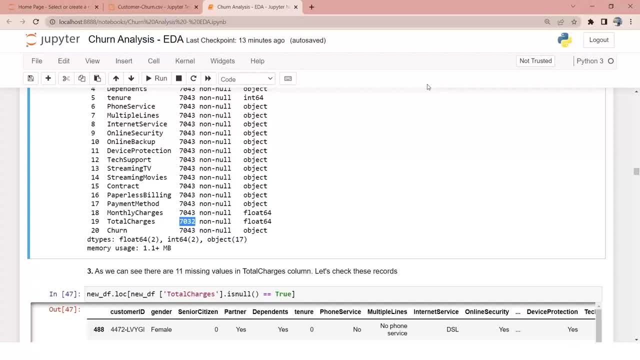 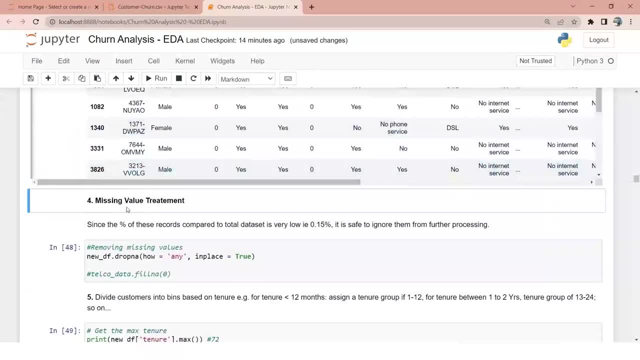 it's almost 30 percent, but in my case it is just 0.15, so I will delete it. so these were the null records, and then I am doing a missing value treatment here. since percentage of these records are very low, it is safe to ignore them from. 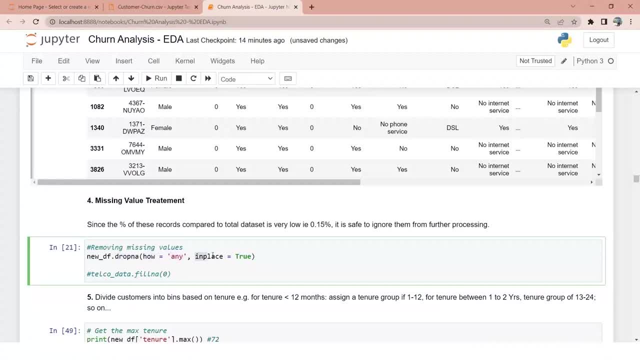 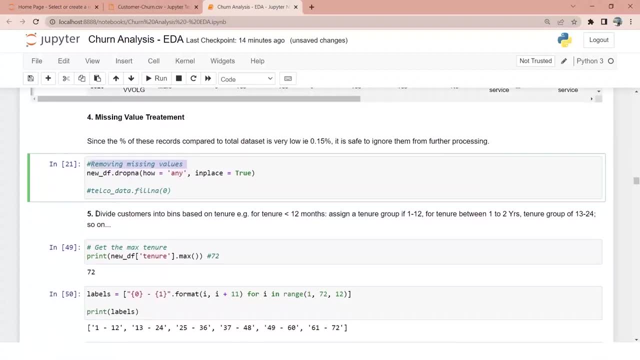 further processing you, so I'm doing drop in a how any in place equals to true. okay, so removing all the missing values divide the customers into bin. so my data cleaning is almost done. invalid data type is fixed. null values are imputed. the next step is I have a. 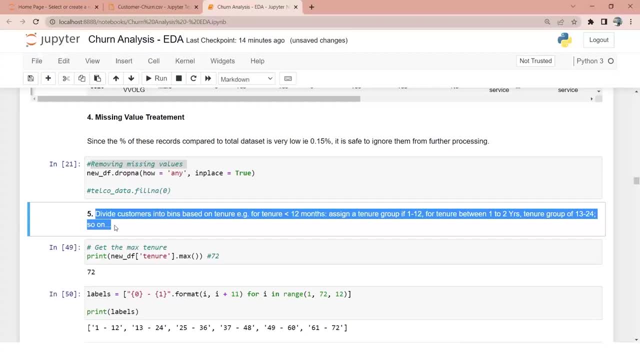 values are imputed. the next step is i have a column called as tenure. now you cannot simply go ahead with this step, so ada is basically an iterative process. now it's very difficult to say why i came up up, came up with this particular step, but the thing is that i initially i didn't 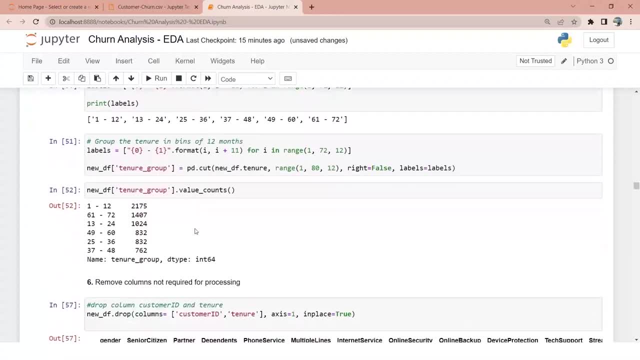 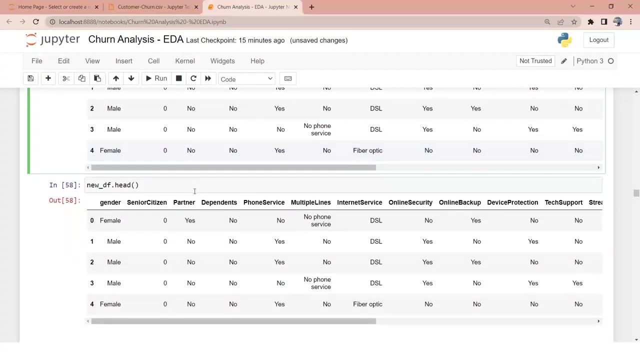 perform this step. initially, after this, i was directly jumping into this particular step where i'm removing some random columns and then my cleaning is done and i'm further. you know, i'm removing some random columns and then my cleaning is done and i'm further, and then my cleaning is done and i'm further. 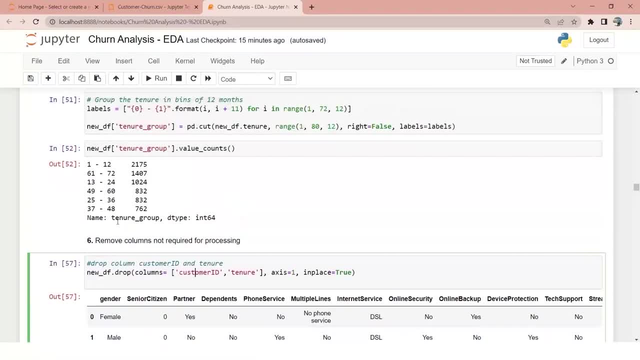 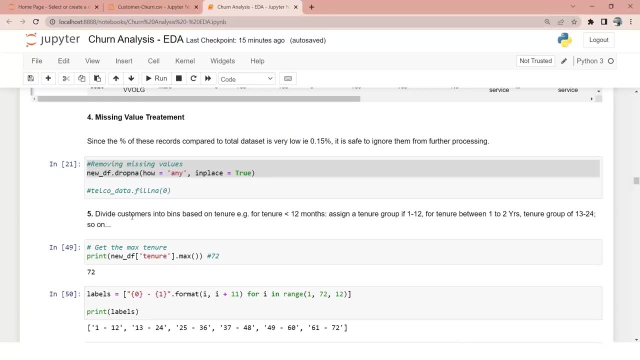 doing my analysis using graphs. and when i was doing analysis using graphs, i came up that i i kind of understood that tenure is a continuous variable and plotting the tenure graph was not giving me any insights. so i had to again come back to this particular step and i performed this step. 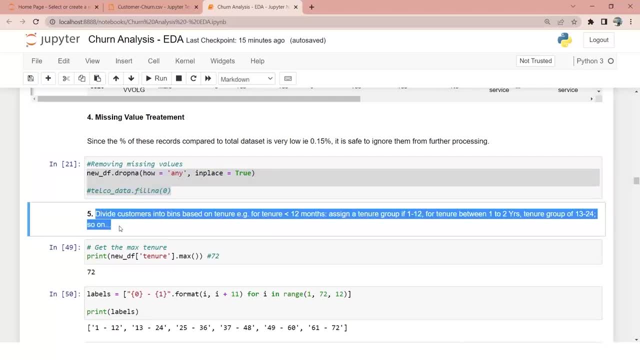 so i kind of helped you to understand why i'm performing this step. but in your case, you can simply check out your data, get an intuition. if there is a continuous numerical column like age tenure, something like that, you can simply convert it into bins or simply do a feature binning. 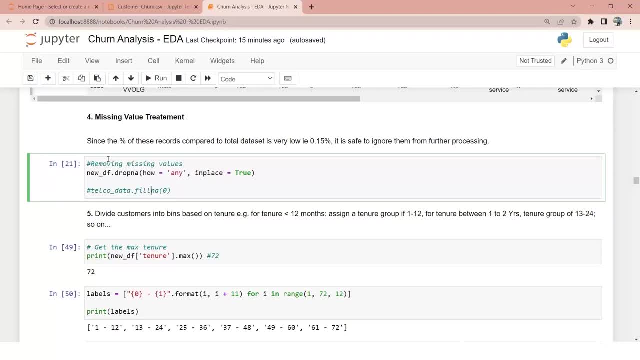 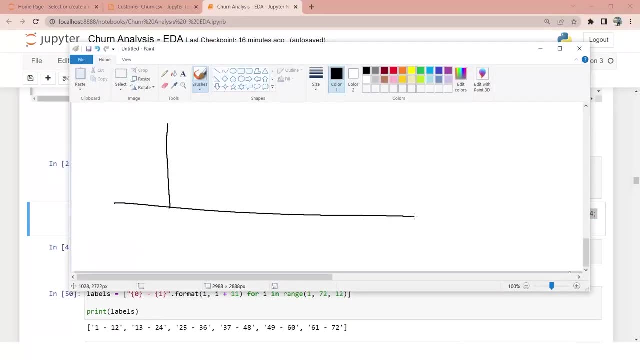 so we are conducting feature binning right now. as we have a column like tenure, it is very difficult to visualize a continuous variable right? you could end up having a lot of bar charts you will not be able to understand and get insights, so you can simply convert it into bins or simply do a feature binning. 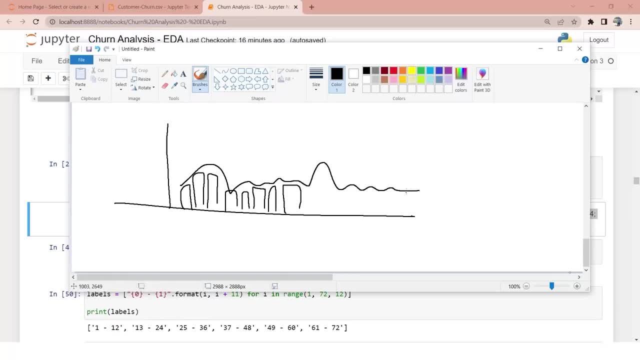 even in line chat also, you will not be able to understand. so better way to understand will be having bins. if you convert it into three or four bins, you will be able to understand that majority of the people are lying here or people who have churned are mostly from this category. 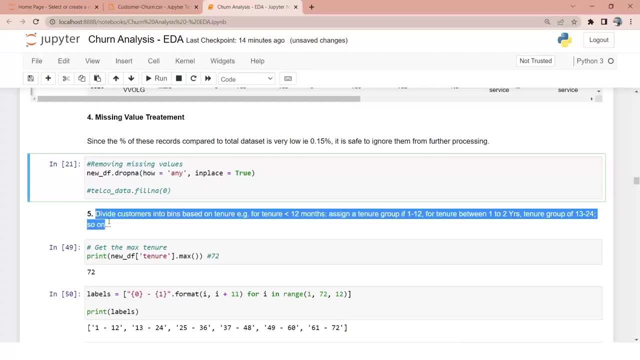 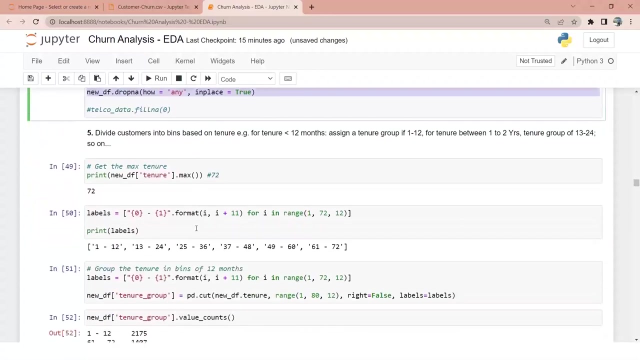 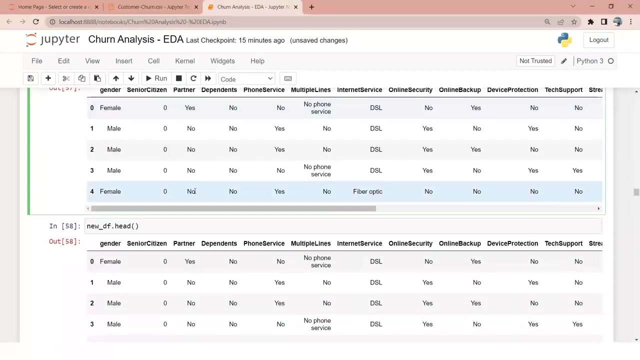 column called as tenure. now you cannot simply go ahead with this step, so ad is sorry Hidden. now I'm doing a missing value treatment at the attached thing in order to remove any missing values here in the column type. in this way I am removing these columns here, so I will go ahead with. 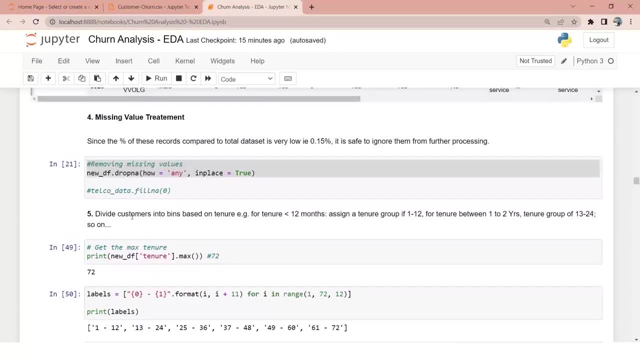 and when i was doing analysis using graphs, i came up that i i kind of understood that tenure is a continuous variable and plotting the tenure graph was not giving me any insights. so i had to again come back to this particular step. and i performed this step. so i kind of 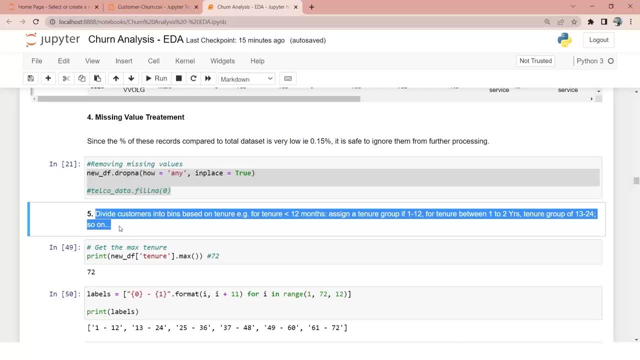 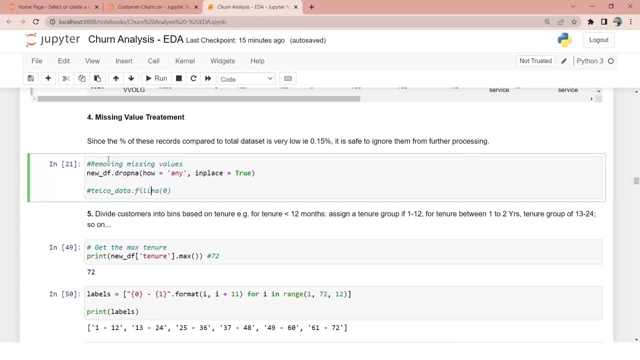 helped you to understand why i am performing this step. but in your case, you can simply check out your data, get an intuition. if there is a continuous numerical column, like age tenure, something like that, you can simply convert it into bins or simply do a feature binning. 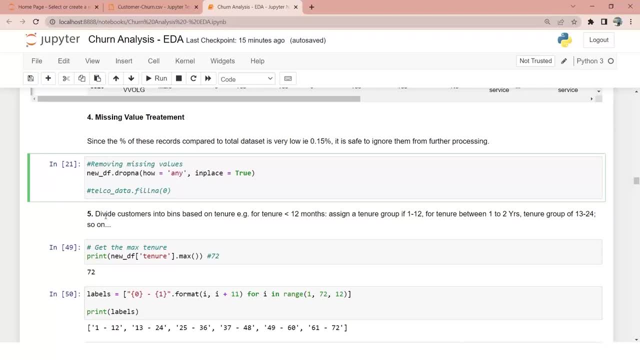 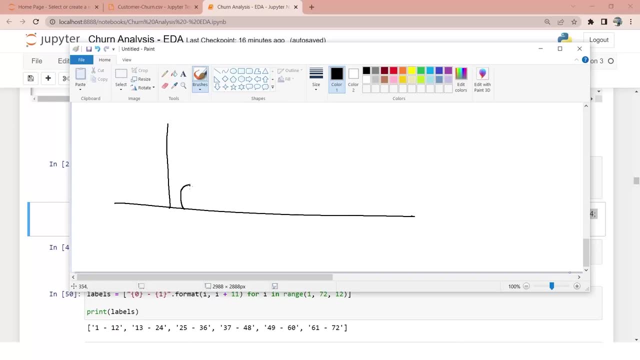 so we are conducting feature binning right now. as we have a column like tenure, it is very difficult to visualize a continuous variable right? you could end up having a lot of bar charts. you will not be able to understand and get insights, even in line chat. also, you will not be able to understand. so better way to understand will be. 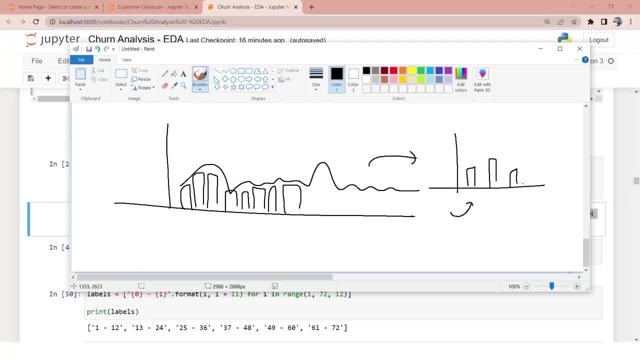 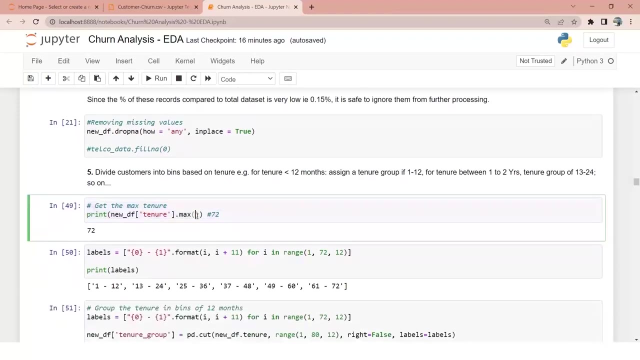 having bins. if you convert it into three or four bins, you will be able to understand that majority of the people are lying here, or people who have churned are mostly from this category, right? so i have divided the data into bins. new df tenure max is 72. so here i'm creating labels. 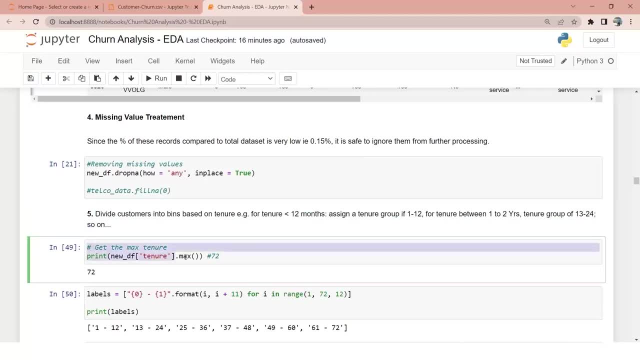 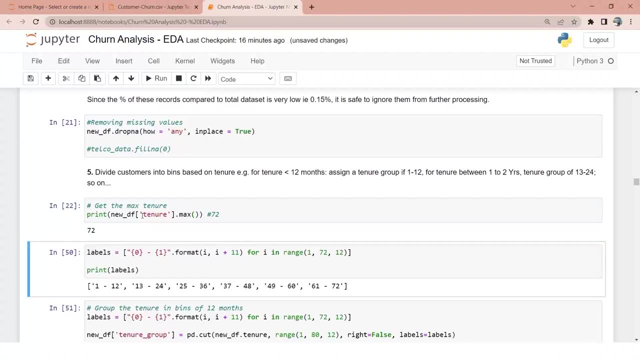 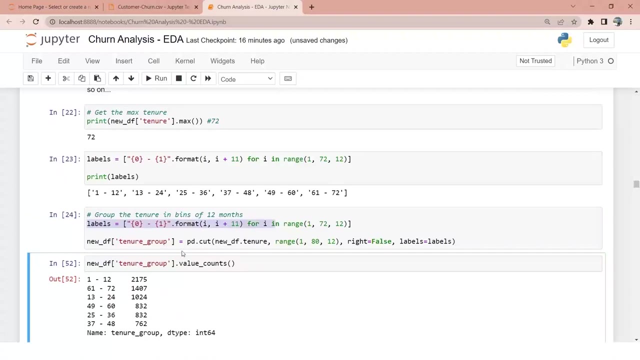 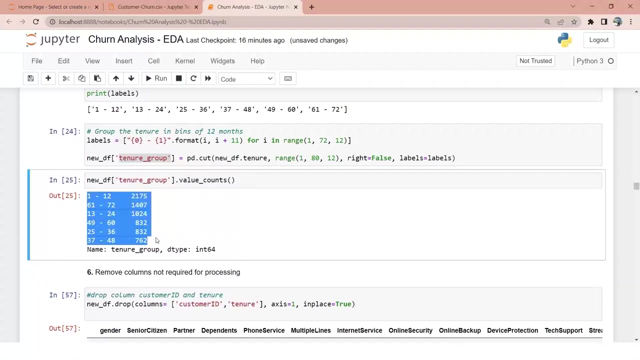 right. so i have divided the data into bins. new df tenure max is 72. so here i'm creating labels. my labels are these: run it. and then i'm creating a tenure group and you can see my tenure group. dot value counts are something like this. so 2175 records for people who are in 1 to 12 category. 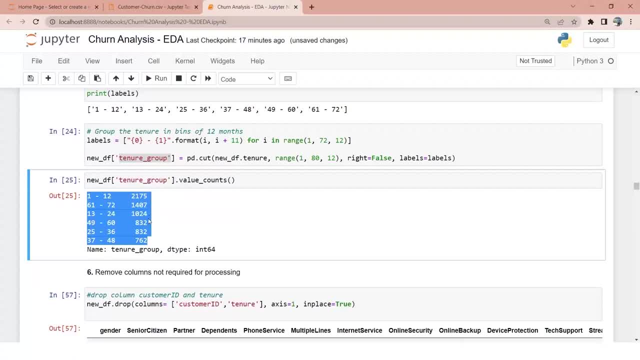 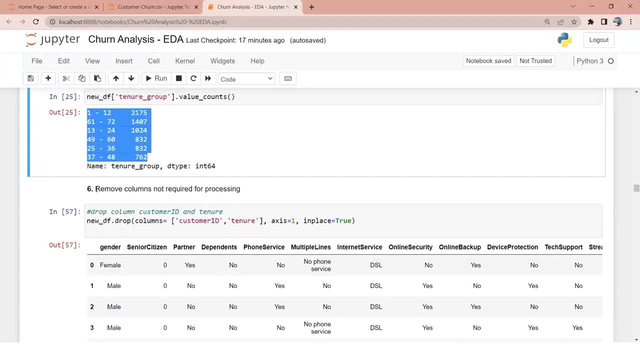 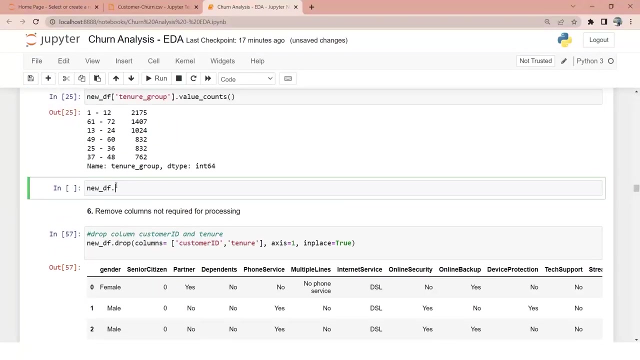 61 to 72, 1400 records, 1024 and so on. after that, as part of the data cleaning process, i'm also removing some of the columns that i know they should not have been a part of this particular data set for analysis. let's say, i will try to see the data frame. customer id is definitely one of. 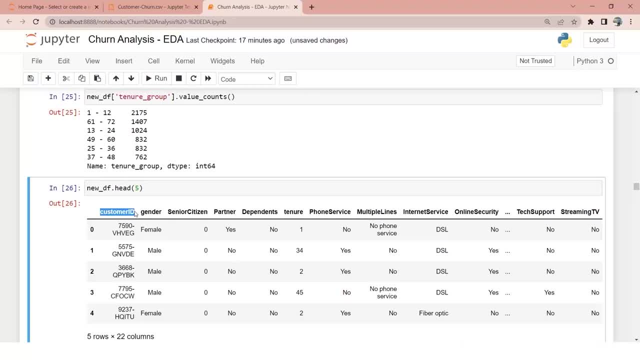 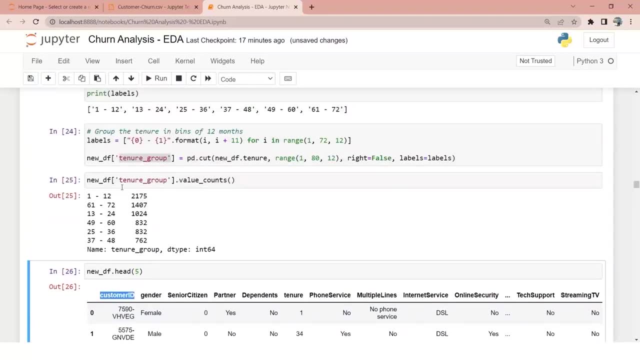 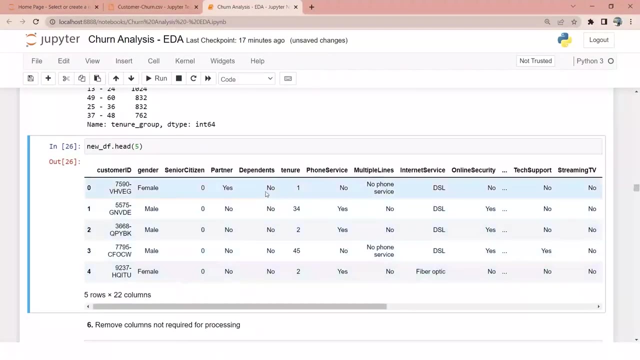 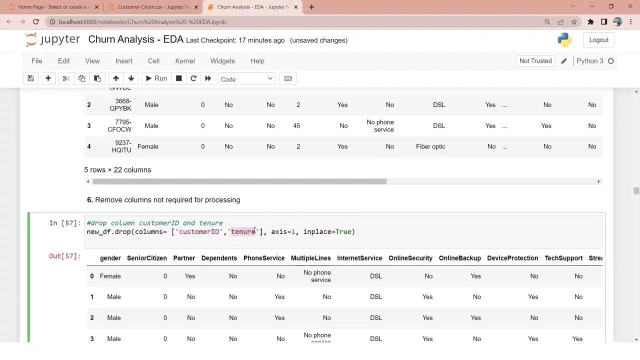 those columns. i don't need customer id because customer id will not give me any information. it's a randomly generated number. apart from that, we also have created tenure group, so i don't even need tenure because my tenure group is already there. so i don't need tenure. so that's why i am removing customer id and tenure from my x-axis. 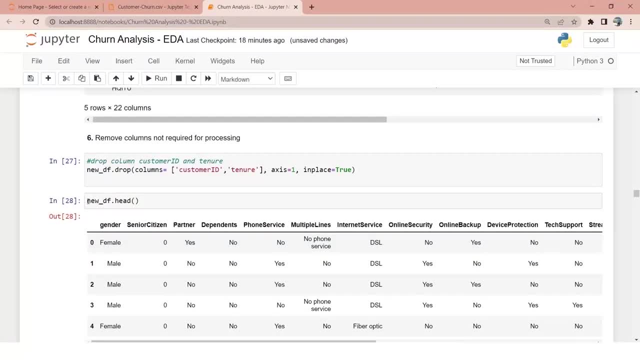 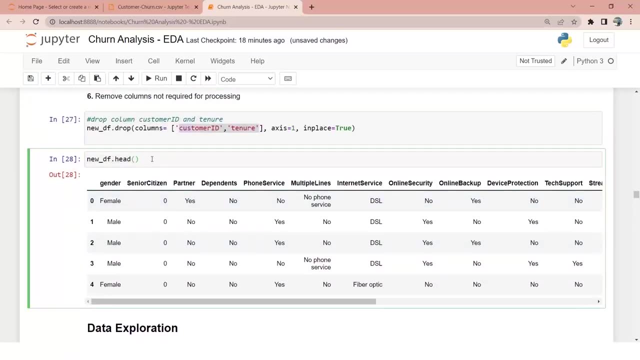 in place. true, if i do this and then i do data frame dot head, you can see those columns are gone. so that potentially brings us to an end to the data cleaning process. i hope you understood each and every step in this particular data set. we didn't had enough null values, but, yeah, in your 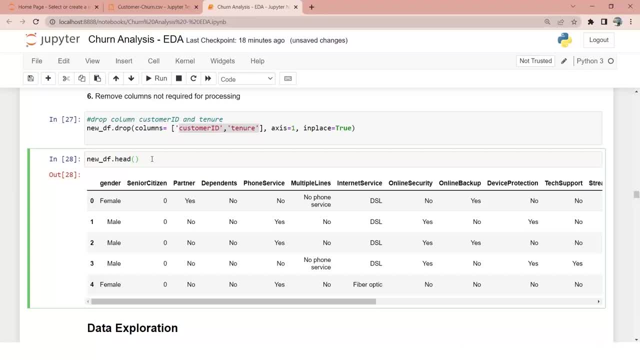 case. there could be different null values. there could be different columns. where you can, you need to combine them to get an aggregated value. there could be scenarios where you have to drop multiple columns and you have to drop multiple columns and you have to drop multiple columns and you have to. 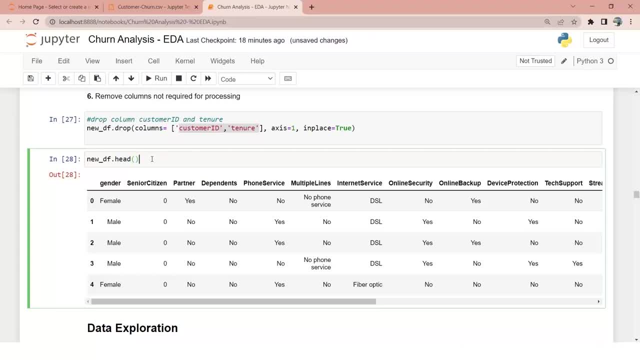 so the number of scenarios are too much. it's very difficult to explain taking just one single example. but i hope you are getting into the process, you are trying to understand what's happening and it's an iterative process. right, you have to work on multiple eda projects to become 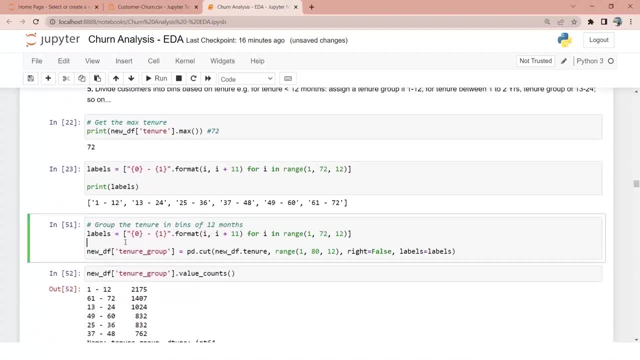 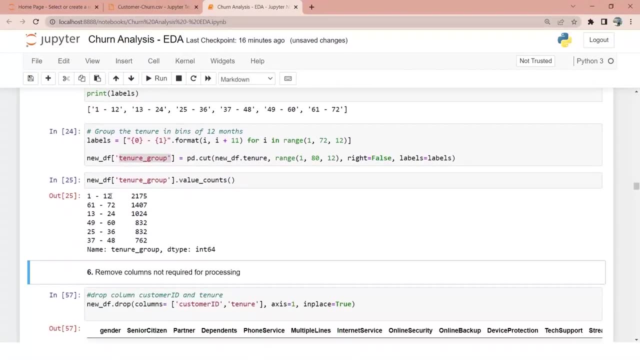 my labels are these: run it. and then i'm creating a tenure group and you can see my tenure group. dot value counts are something like this: so 2175 records for people who are in one to twelve category, 61 to 72, 1400 records, 1024 and so on. after that, as part of the data cleaning process, 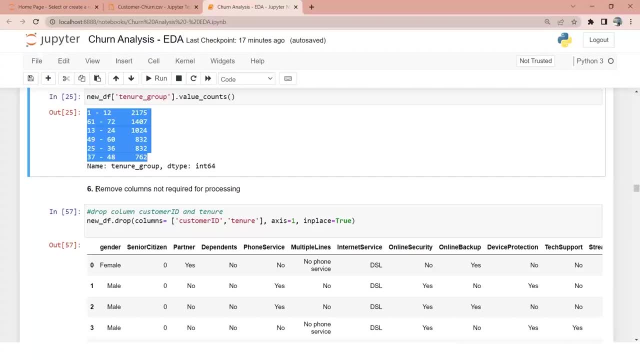 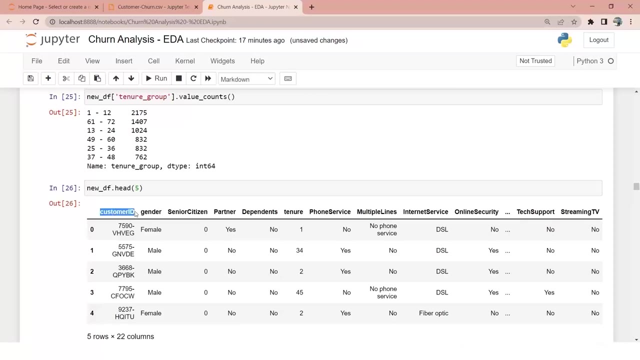 i'm also removing some of the columns that i know they should not have been a part of this particular data set for analysis. let's say, i will try to see the data frame. customer id is definitely one of those columns. i don't need customer id because 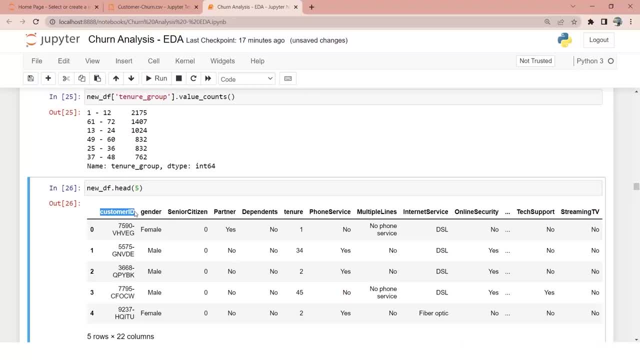 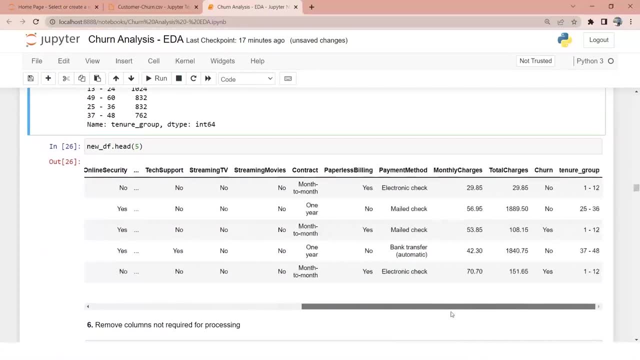 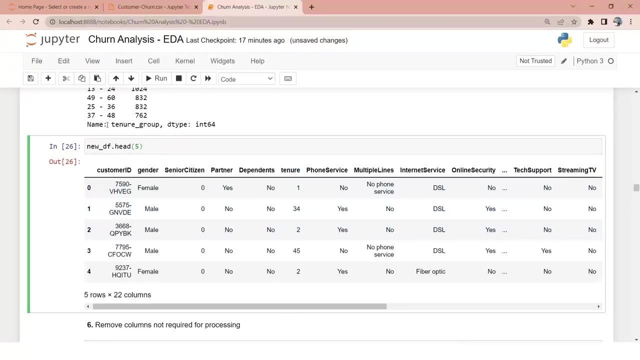 customer id will not give me any information. it's a randomly generated number. apart from that, we also have created tenure group, so i don't even need tenure because my tenure group is already there. so i don't need tenure. so that's why i am removing customer id and tenure from my x-axis. 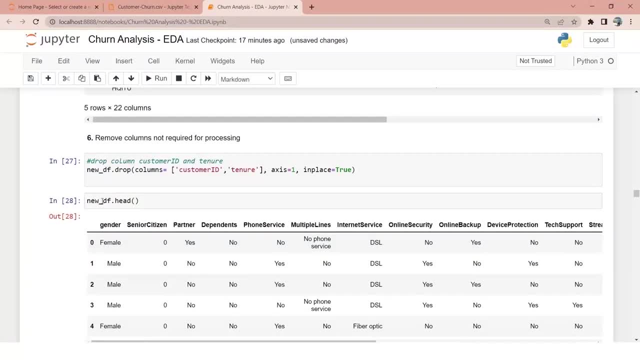 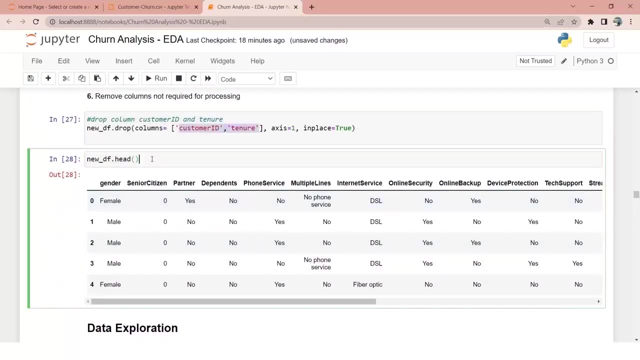 in place. true, if i do this and then i do data frame dot head, you can see those columns are gone. so that potentially brings us to an end to the data clear leaning process. i hope you understood each and every step in this particular data set. we didn't. 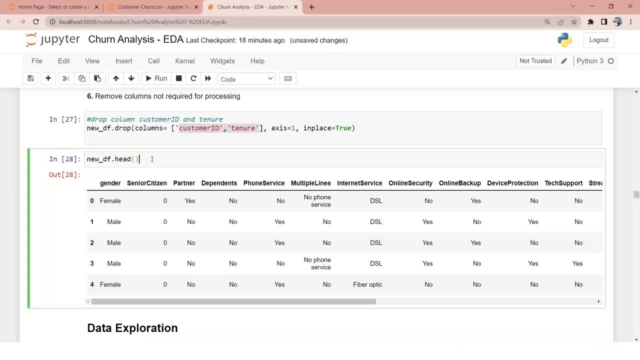 had enough null values. but yeah, in your case there could be different null values. there could be different columns. where you can, you need to combine them to get an aggregated value. there could be scenarios where you have to drop multiple columns. so the number of scenarios are too much. it's very difficult to explain taking just one. 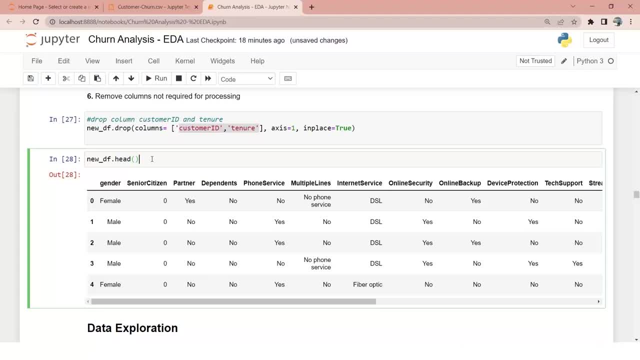 single example, but i hope you are getting into the process. you are trying to understand what's happening and it's an iterative process. right, you have to work on multiple eda projects to become a eda wizard, in order to be a professional or somebody who has good experience or knowledge. 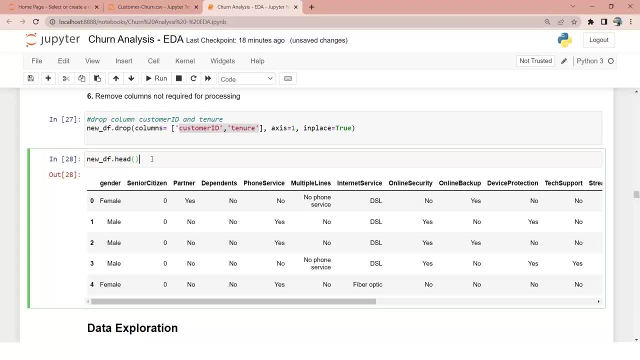 a eda wizard. in order to be a professional or somebody who has good experience or knowledge into eda, you need to work on multiple projects. so that's all about this particular video on the data cleaning part. our next part is going to be our analysis, because the data cleaning part is done. 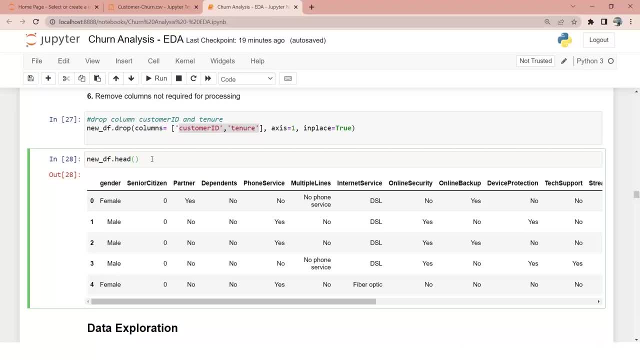 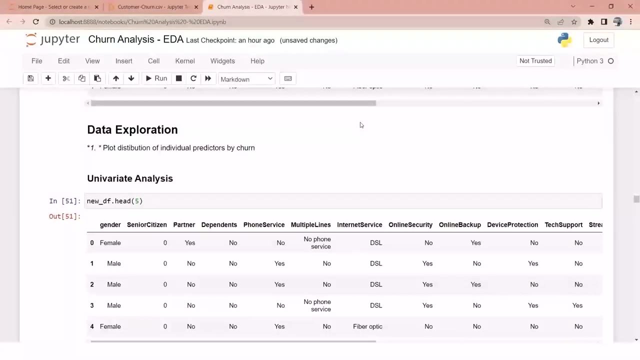 we assume that our data is cleaned- data right now and now we are ready for the analysis part. see you in the next video. so we will get started with the data exploration part. till now, we assume that our data cleaning process is done and the expectation is the data right now is almost cleaned. now our next step is: 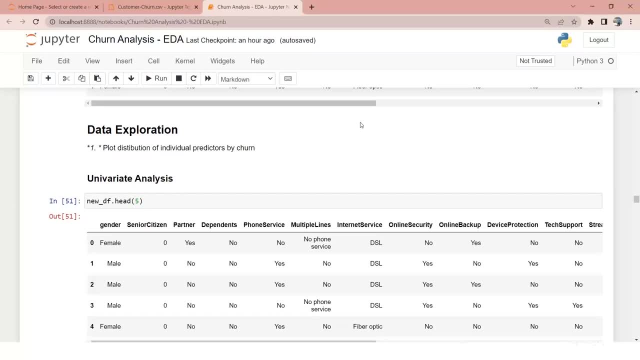 to perform different types of analysis. that includes univariate, bivariate, multivariate, numerical analysis and so on. there could be multiple instances where you could also realize that there could be a problem in the data you are not able to interpret. you again have to go back to the data cleaning process for further cleaning or further changes and then again come. 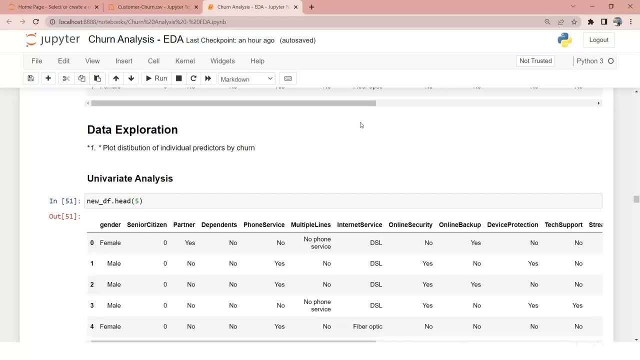 back to the analysis process. it is a possibility, but we assume that in this case, in in the case right now, we are in the state we are in. we assume that our data is already cleaned. let's get started with the different types of analysis. in this video, we shall be focusing more on the univariate analysis part and going forward. we 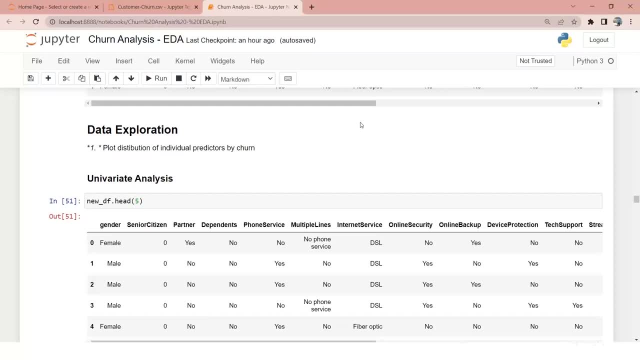 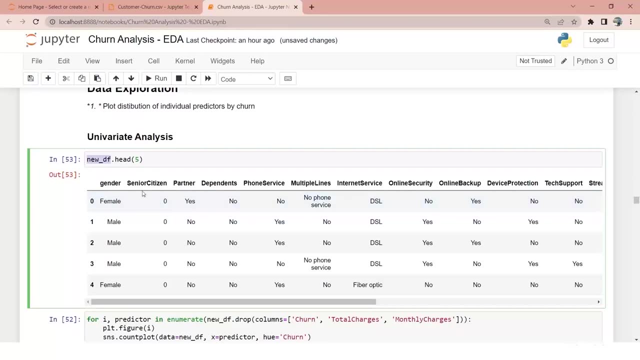 will have numerical analysis, bivariate analysis and so on. so we already have the data set, we already have the data frame, the new df dot head. it has columns like these: gender, senior citizen and so on. so in the next step, what i am doing is ultimate goal is to perform univariate analysis. 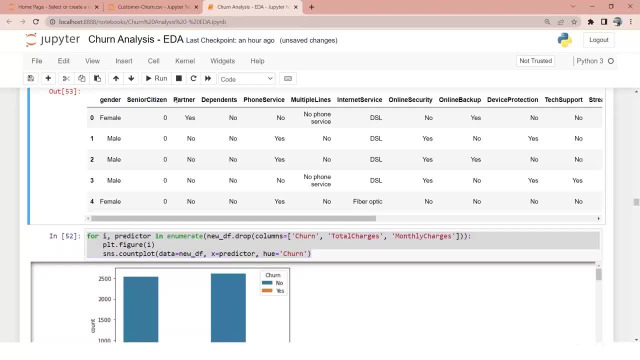 so in the next step, what i am doing is- ultimate goal- is to perform univariate analysis, and so on. so in the next step, what i am doing is- ultimate goal- is to perform univariate analysis, and so on. whatever columns you have- gender, senior citizen, partner- you are free to create multiple charts. 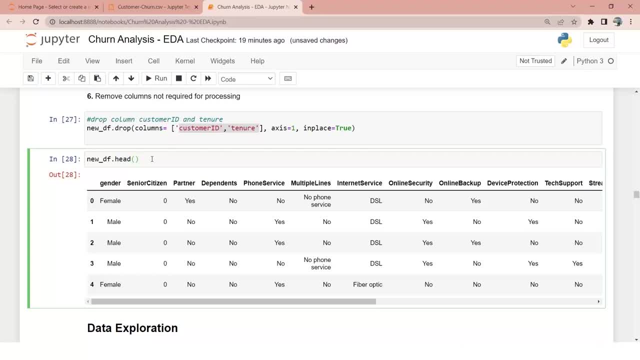 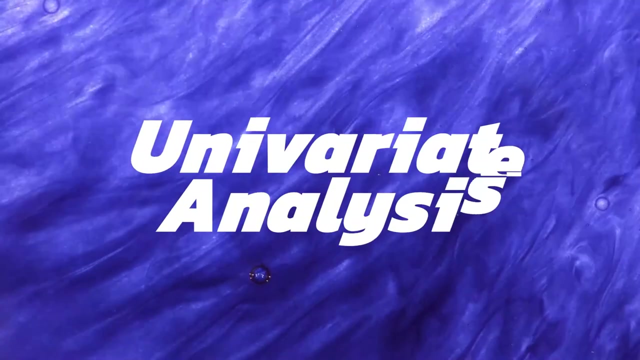 into eda. you need to work on multiple projects, so that's all about this particular video on the data cleaning part. our next video will be on data cleaning, so thank you for watching and i will see you in the next video. next part is going to be our analysis, because the data cleaning part is done. we assume that our data is cleaned data right now, and now we are ready for the analysis part. see you in the next video. 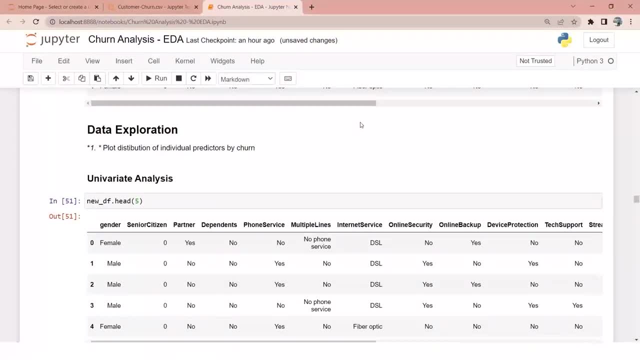 so we will get started with the data exploration. part till now, we assume that our data is cleaned. data cleaning process is done and the expectation is the data right now is almost cleaned. now our next step is to perform different types of analysis. that includes univariate, bivariate. 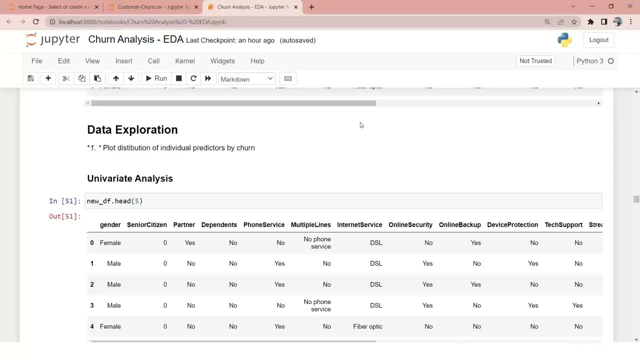 multivariate numerical analysis and so on. there could be multiple instances where you could also realize that there could be a problem in the data you are not able to interpret. you again have to go back to the data cleaning process for further cleaning or further changes and then 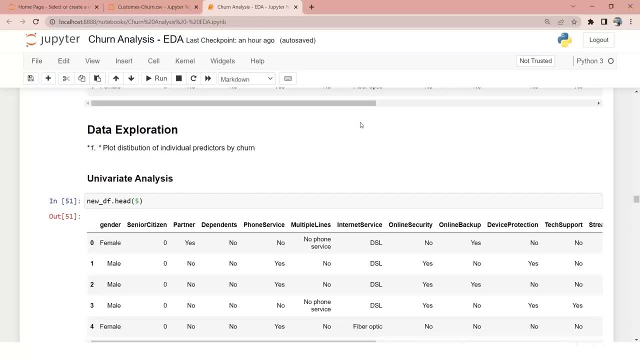 again come back to the analysis process. it is a possibility, but we assume that in this case, in in the case right now, we are in the state we are in. we assume that our data is already cleaned. let's get started with the different types of analysis in this video we shall be 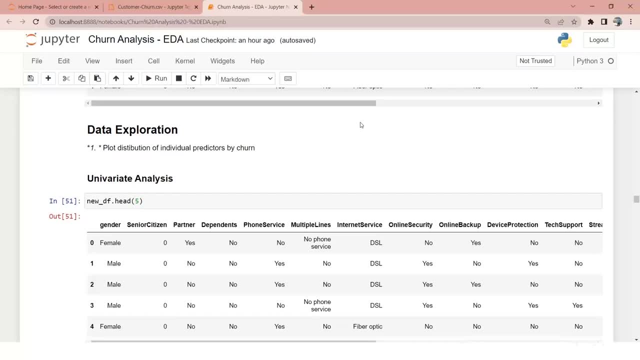 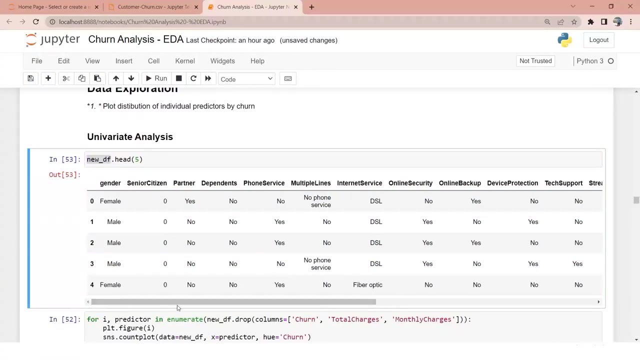 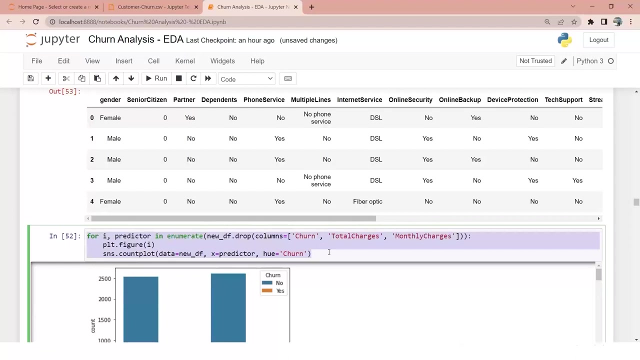 focusing more on the univariate analysis part and going forward we will have numerical analysis, bivariate analysis and so on. so we already have the data set, we already have the data frame, the new dfhead. it has columns like these: gender, senior citizen and so on. so in the next step, what i am doing is ultimate goal is to perform univariate analysis. 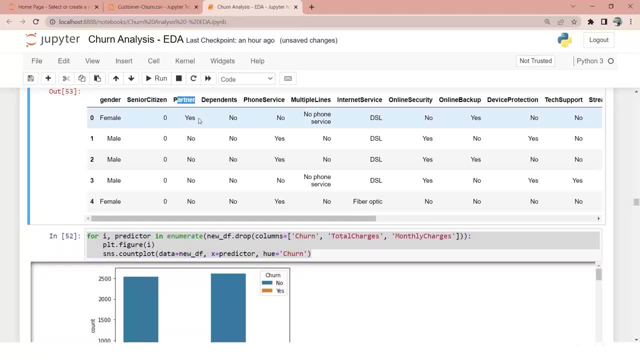 whatever columns you have- gender, senior citizen partner- you are free to create multiple charts. you are free to have one, one line of code for one type of chart. so one by one, by one, is also possible, but i have already automated this process. hence i am running a for loop where i will 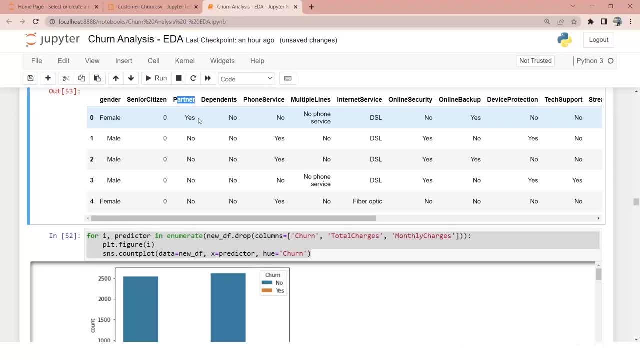 you are free to have one, one line of code for one type of chart, so one by one, by one, is also possible, but i have already automated this process. hence i am running a for loop where i will iterate over the entire data frame and i will be able to plot everything in one single line. 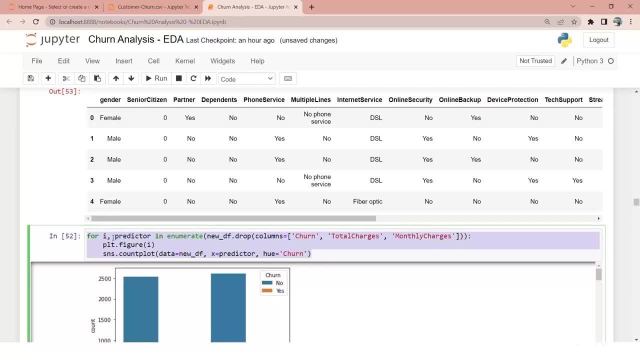 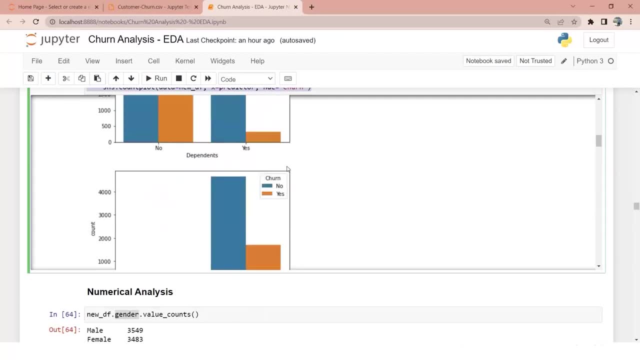 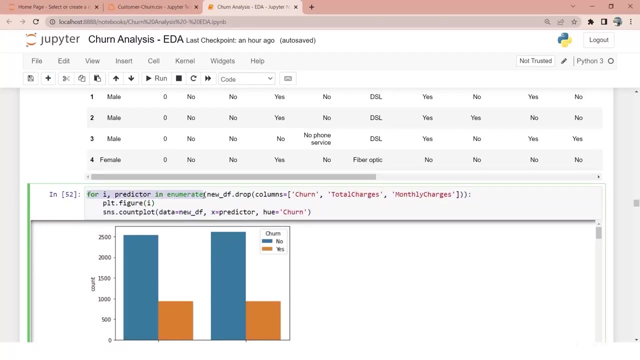 so just three lines of code. i will run, it will iterate through the entire data frame and i will get a whole list of all the graphs, all the univariate graphs, right? so i'll try to explain this piece of code. it's not rocket science here. i am enumerating or basically iterating over the. 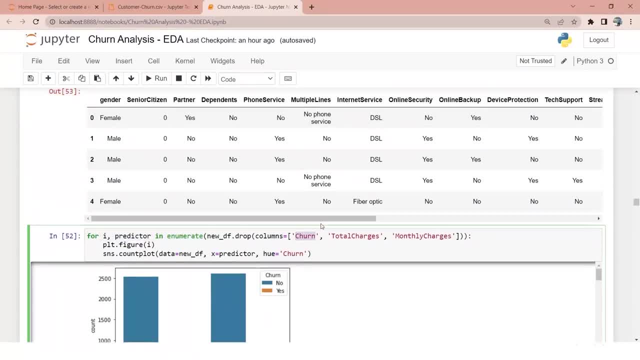 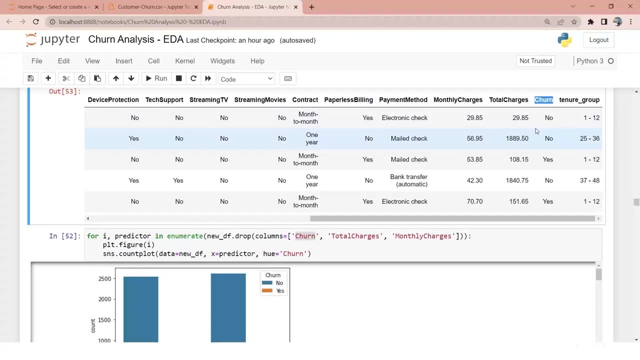 data frame. from the data frame i have deleted all my numerical columns and the churn column. why? because churn is our output, my y? y data, my dependent variable, and total charges and monthly charges are my numerical attributes. so we will be doing numerical analysis for these columns. apart from that, do we have any other? 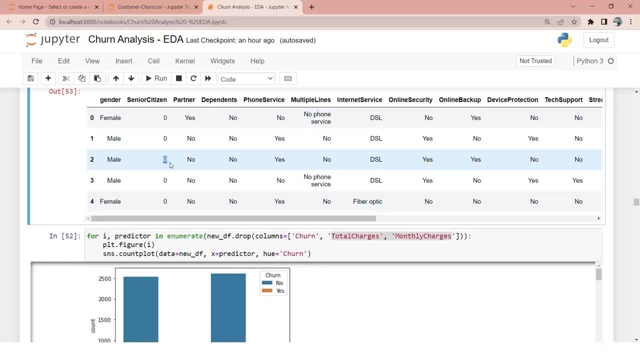 numerical columns. we have senior citizen but, as i told you, it's in the format of 0 and 1 could be considered as a categorical attribute, so i am not dropping them. apart from that, i'm just plt, doing plt dot figure and i'm doing a. 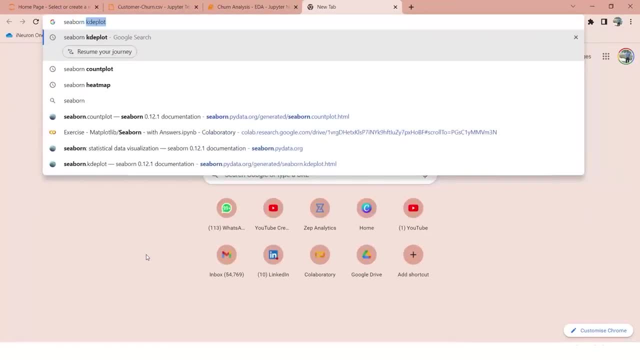 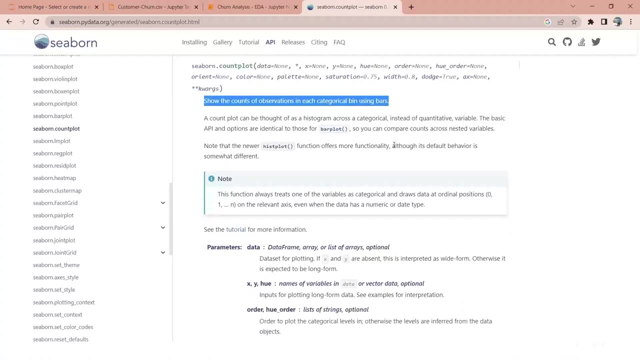 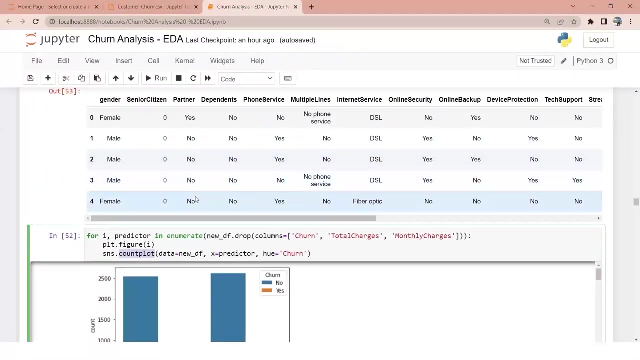 count plot. if you want to have more understanding on count plot, simply go ahead and search c bond dot count plot. you will be able to get the information about it. it is simply a bar chat: counts of observations in each categorical bin. using bar, i'm passing the data frame, my predictor. 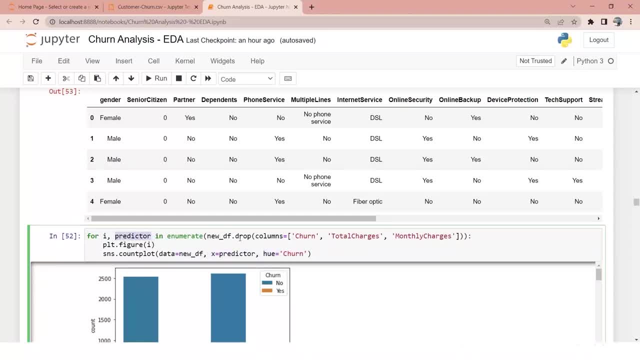 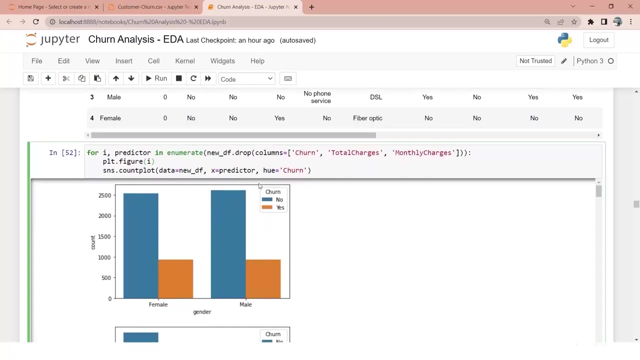 and my hue predictor here is nothing but all my columns. i is nothing but the number of columns. the index values q is churn. so i have already ran this command. so i have the list of visuals in front of me. if you want to add labels, you can add them, but labels are not that important because somehow 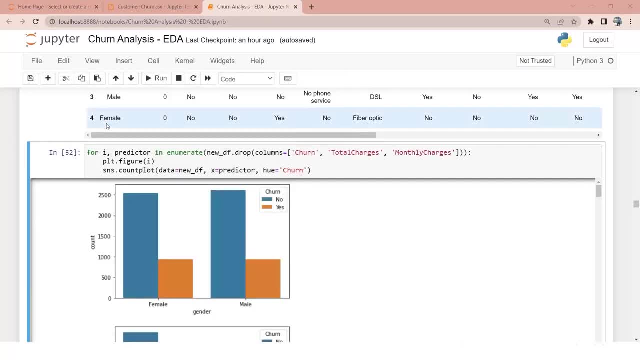 from this graph itself, i am able to interpret some of these numbers. so we'll try to analyze one of these uh graphs, probably couple of them too. i'll put them in the now to do that. one of the other key points is that to interpret the scale of the number of columns is nine number. 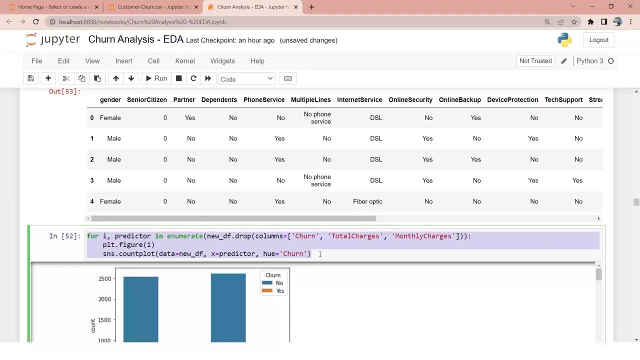 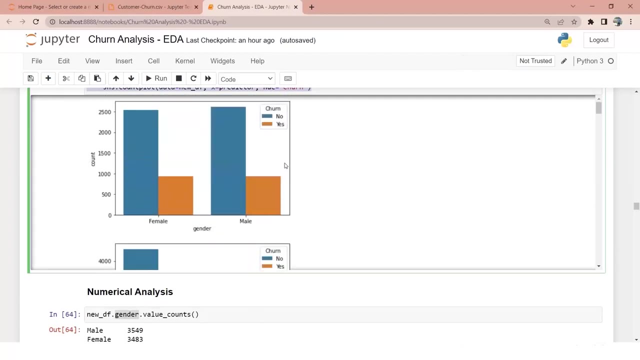 iterate over the entire data frame and i will be able to plot everything in one single line. so just three lines of code. i will run, it will iterate through the entire data frame and i will create a whole list of all the graphs, all the univariate graphs, right? so i'll try to. 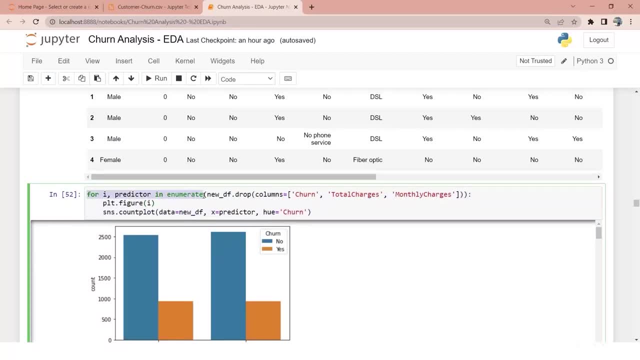 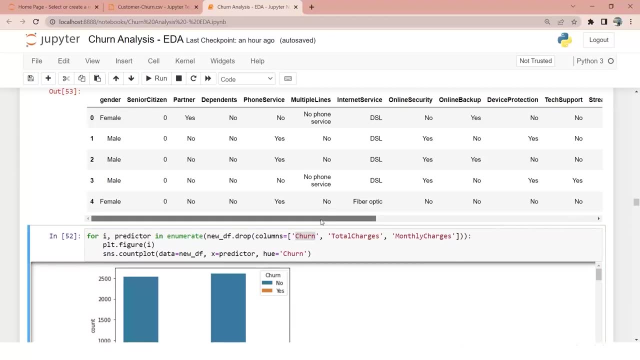 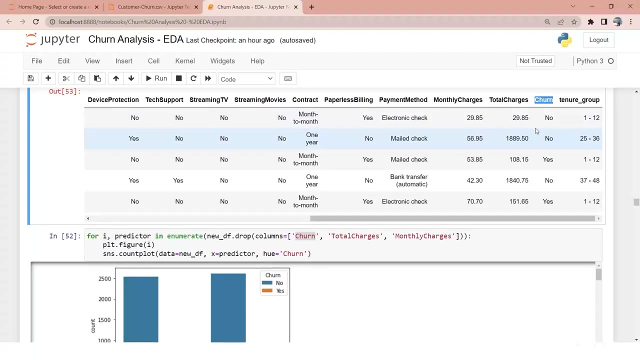 explain this piece of code. it's not rocket science. here i am enumerating or basically iterating over the data frame from the data frame. i have deleted all my numerical columns and the churn column. why? because churn is our output, my y? y data, my dependent variable and total charges and monthly. 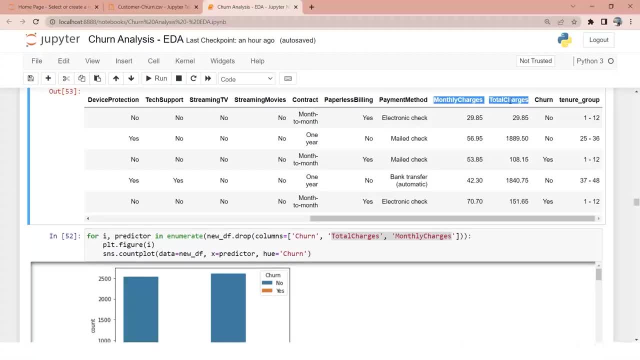 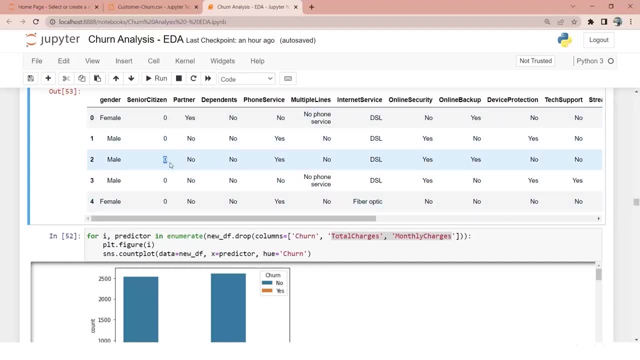 charges are my numerical attributes, so we will be doing numerical analysis for these columns. apart from that, do we have any other numerical columns? we have senior citizen, but as i told you, it's in the format of 0 and 1 could be considered as a categorical attribute, so i am not dropping them. apart from that, i'm just plt. 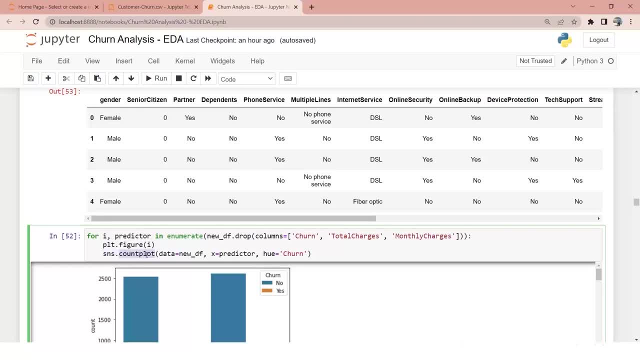 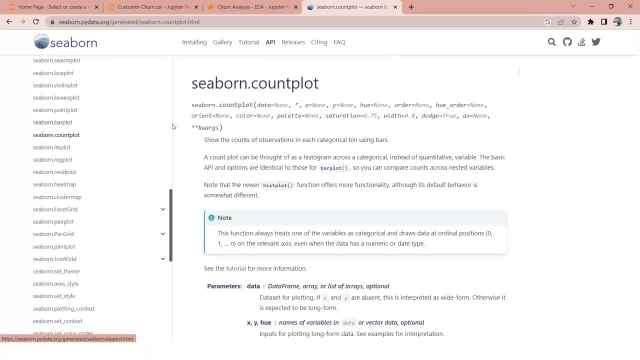 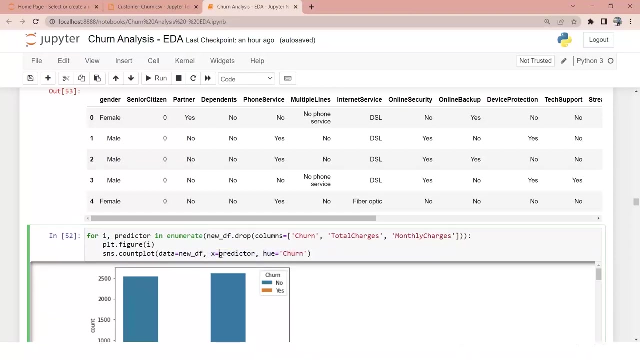 doing pltfigure and i'm doing a count plot. if you want to have more understanding on count plot, simply go ahead and search seaborncom plot. you will be able to get the information about it. it is simply a bar chat counts of observations in each categorical bin. using bar, i'm passing the data frame, my predictor and my hue. 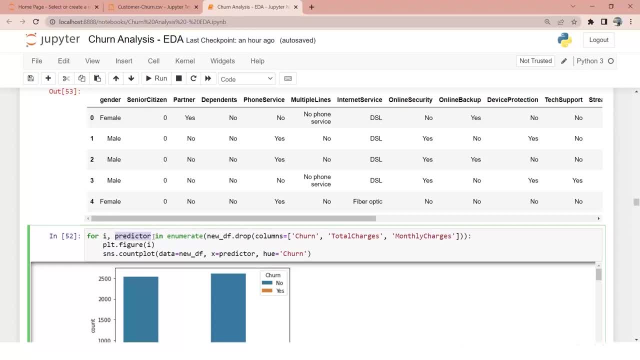 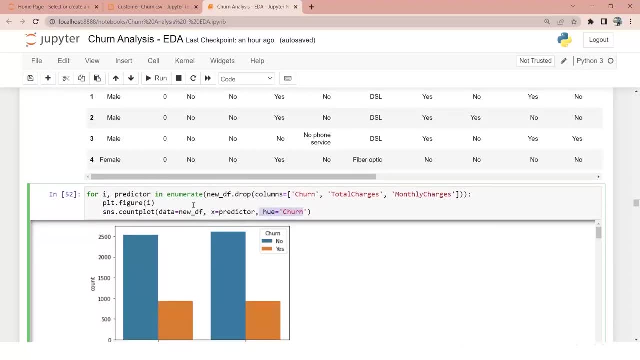 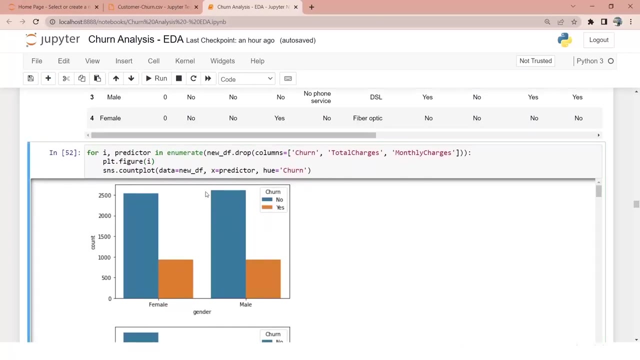 predictor. here is nothing but all my columns. i is nothing but the number of columns, the index values. u is churn, so i have already ran this command. so i have the list of visuals in front of me. if you want to add labels, you can add them, but labels are not that important. 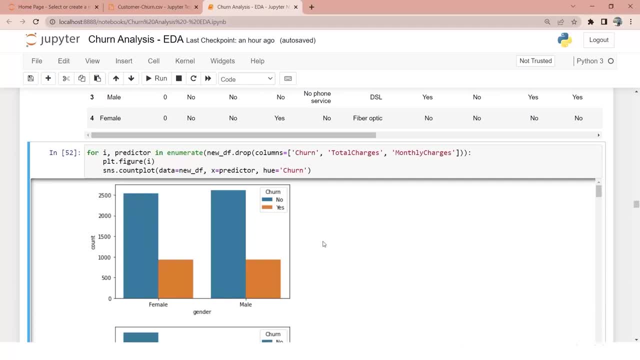 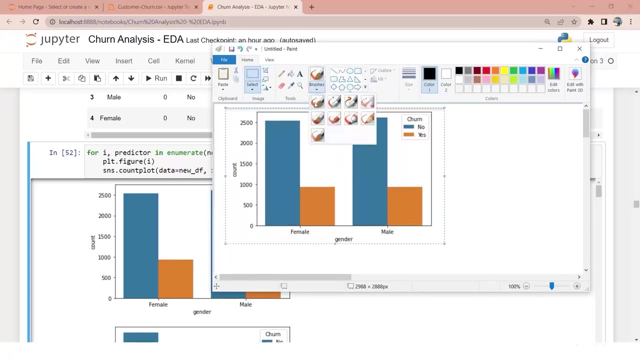 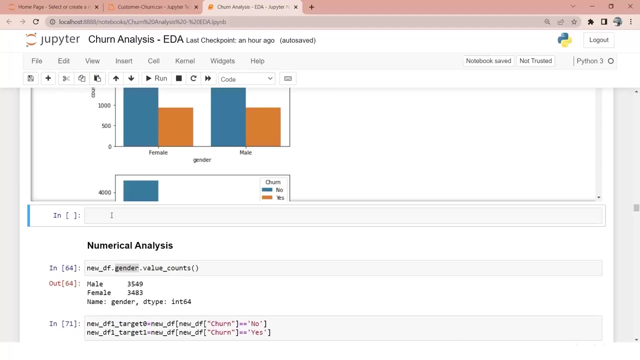 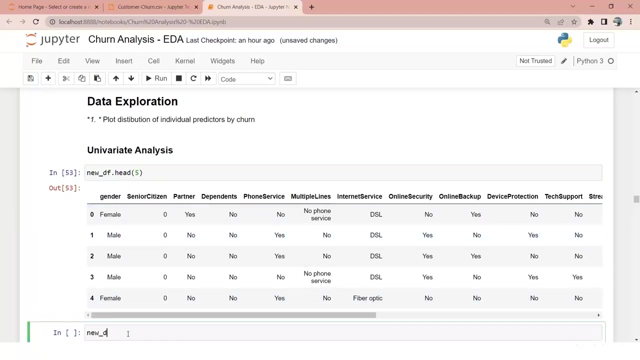 because somehow, from this graph itself, i am able to interpret some of these numbers. so we'll try to analyze one of these uh graphs, probably couple of these graphs, so let's say i'll talk about the first one. that's my gender, what is my origin? data distribution. if you forgot, probably i will create a line of code here: new df dot churn dot. of columns is zero, because the number of columns is three, and so you are able to just make the. so the numbers are the same in terms of color and color, and all of this is completely normal. so that's the last part of this problem. so now let's try to analyze one of these graphs, probably couple of. 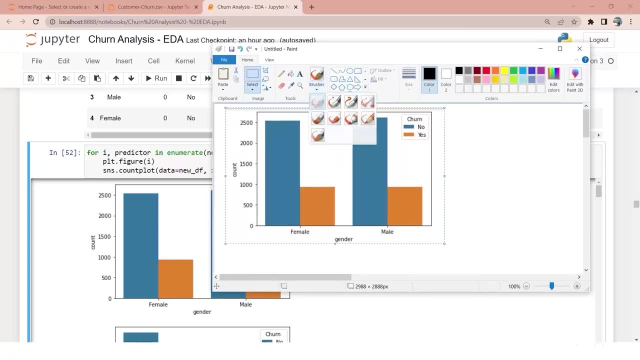 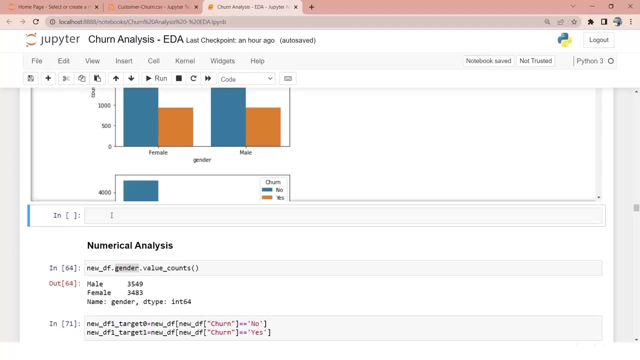 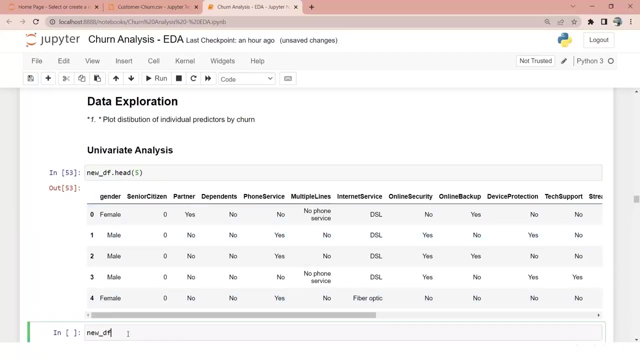 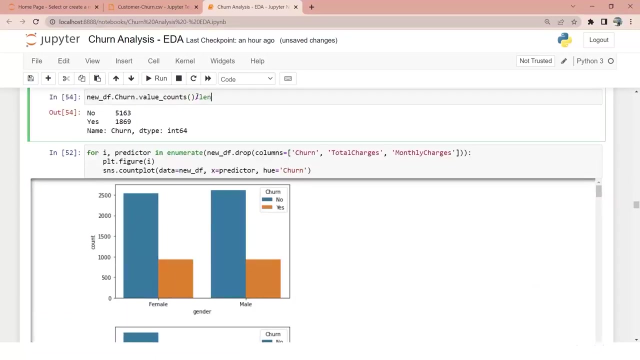 of these graphs. so let's say i'll talk about the first one, that's, my gender. what is my original data distribution? if you forgot, probably i will create a line of code here: new df. dot. turn dot value counts. so my original data i'll just do. length of df. length of new df. 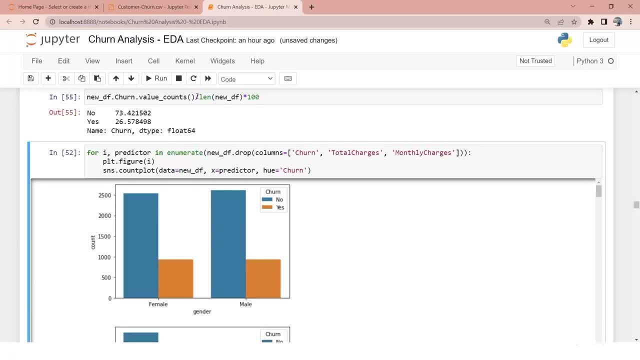 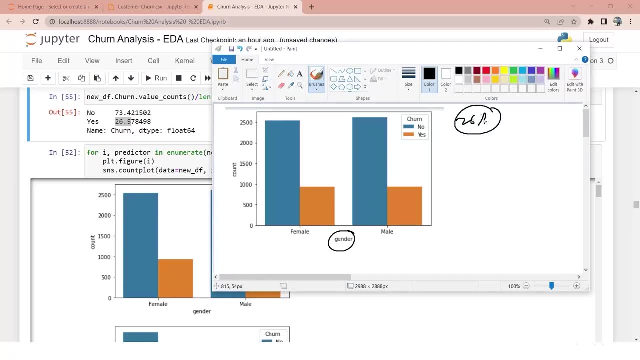 and then into 100, almost 26.57. 26 percent is my churn rate. that is my churn rate right. so i'll try to analyze this graph. first, i have gender. i have my hue as churn, so this is my not churned and this is my churned right. so how many churned customers for female? 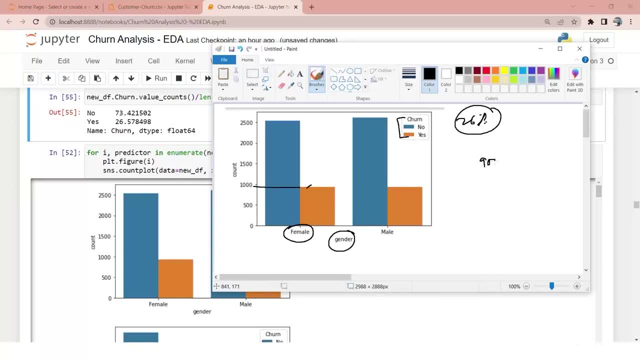 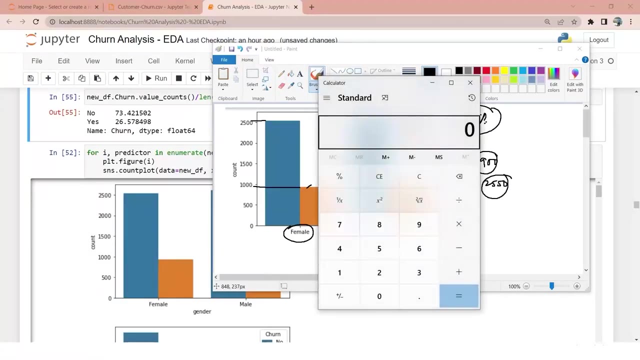 i don't know exactly, but let's assume around 900 and not churned almost around 2500 or 2550, okay, somewhere around that. so what is the churn ratio here? the total is 900 plus 2550, around 3450, so almost 900 churned, 3450 multiplied with 100. 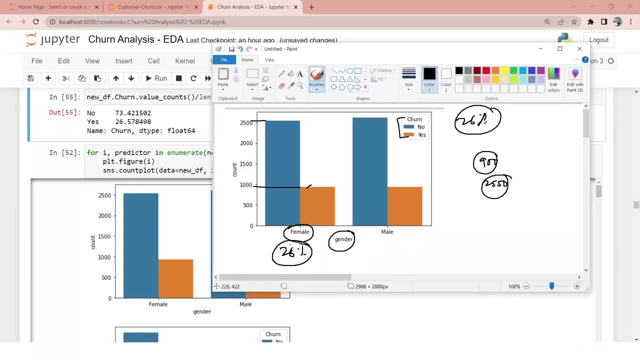 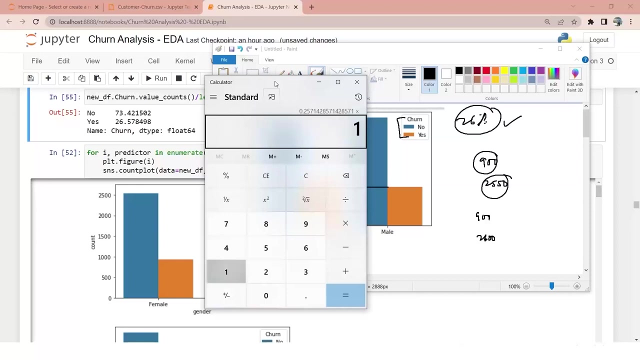 almost 26 percent of the female customers have churned almost. what about male? i see a similar numbers, maybe 900 and maybe a little bit more than 2550 could be 2600. now what is my churn ratio here? 900 divided by 3500, multiplied with 100- almost 25.7. 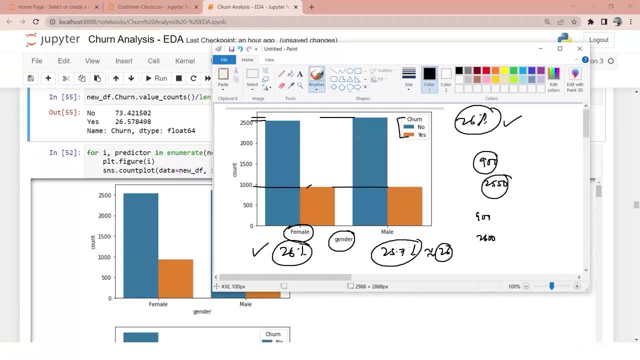 i would assume it's almost 26, right? so what my gender is portraying me? the gender is portraying me nothing. i'm not able to get any insights from only the gender column. does that mean gender is not important? no, gender could be combined with any other feature to become a powerful feature. 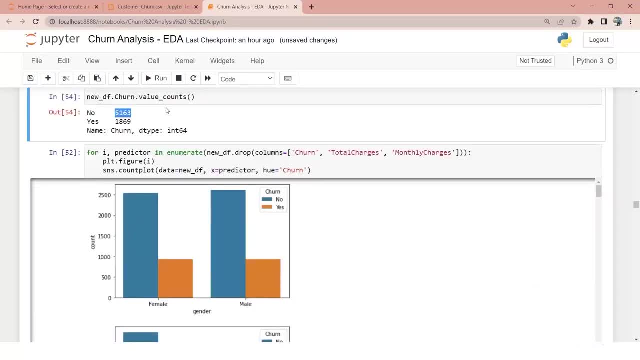 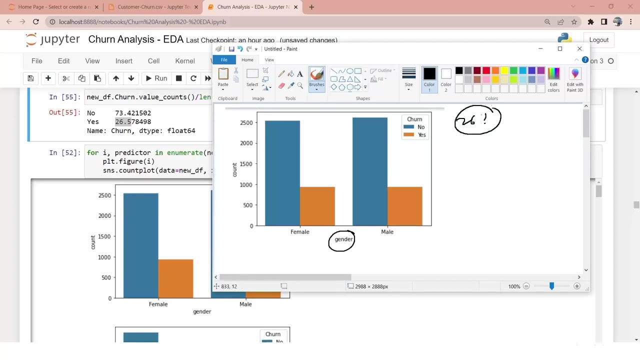 value counts. so my original data, i'll just do length of df, length of new df, and then into 100: almost 26.57, 26 percent is my churn rate. that is my churn rate, right. so i'll try to analyze this graph. first, i have gender. i have my hue as churn, so this is my not churn and this is my churned right. 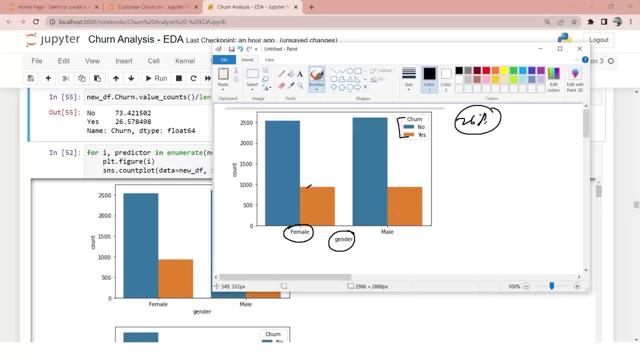 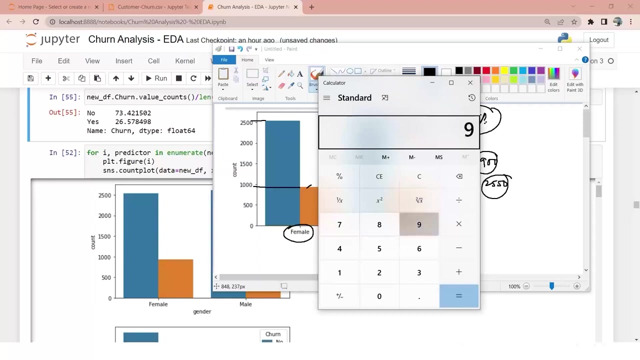 so how many churned customers for female? i don't know exactly, but let's assume around 900 and not churned almost around 2500 or 2500, okay, somewhere around that. so what is the churn ratio here? the total is 900 plus 2550, around 3450, so almost 900 churned, 3450 multiplied with 100. 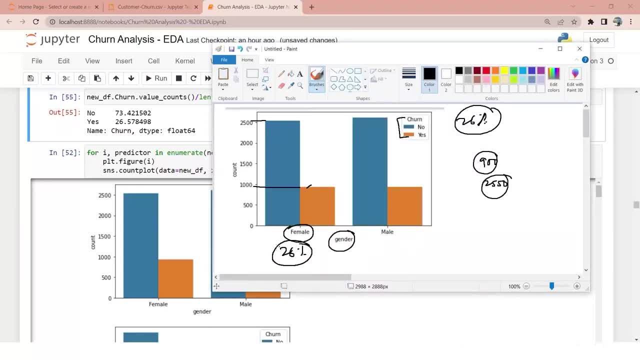 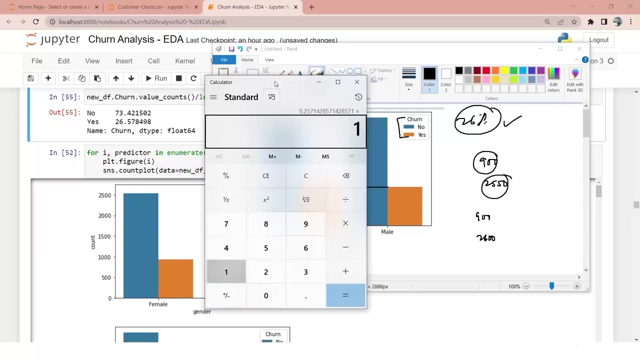 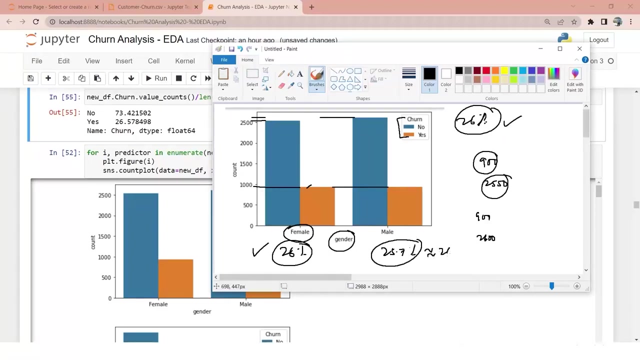 almost 26 percent of the female customers have churned almost. what about male? i see a similar numbers, maybe 900 and maybe a little bit more than 2550 could be 2600. now what is my churn ratio here? 900 divided by 3500, multiplied with 100- almost 25.7 percent, i would assume it's almost 26. 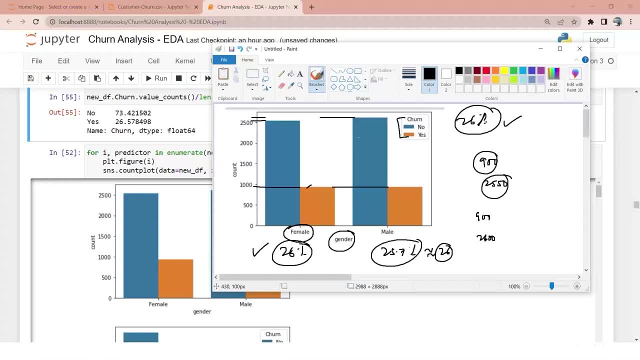 right. so what my gender is portraying me? the gender is portraying me nothing. i'm not able to get any insights from only the gender column. does that mean gender is not important? no gender could be combined with any other feature to become a powerful feature, but alone, standalone, gender is. 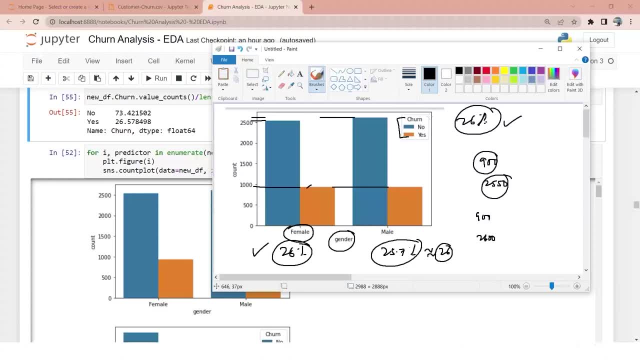 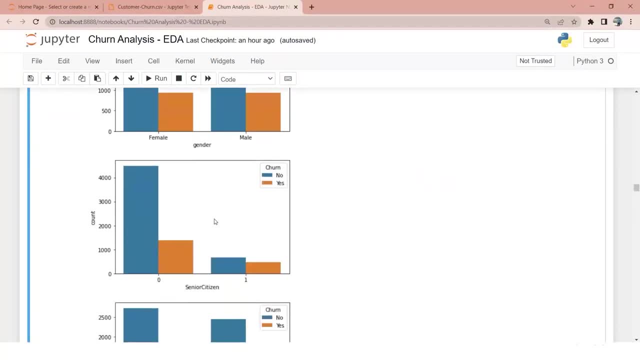 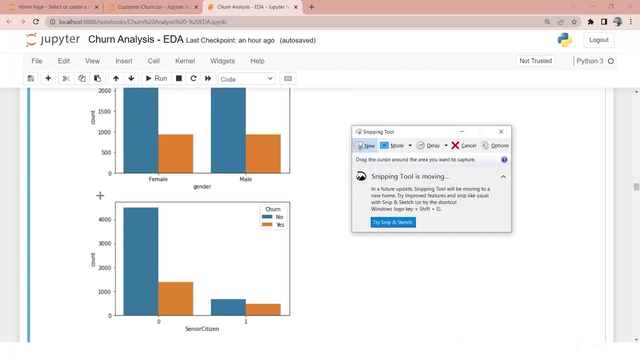 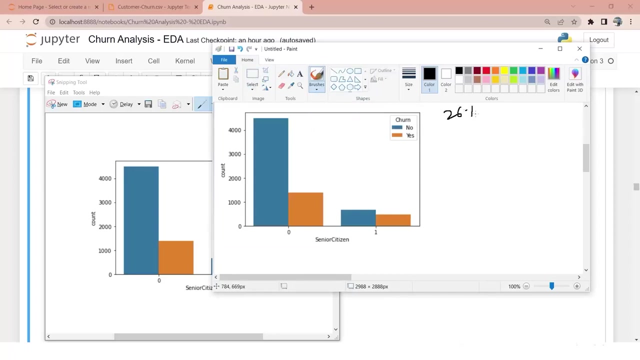 not a triggering point. gender is not impacting the churn. so, coming back to the second graph, let's see, we'll talk about senior citizen. senior citizen. i'll again take this and then paste it now. original data: 26 percent. remember this in your head. how many churned customers again? i probably don't know exactly, but around 1300. 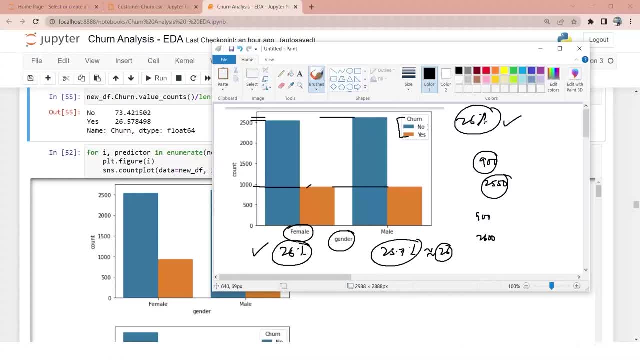 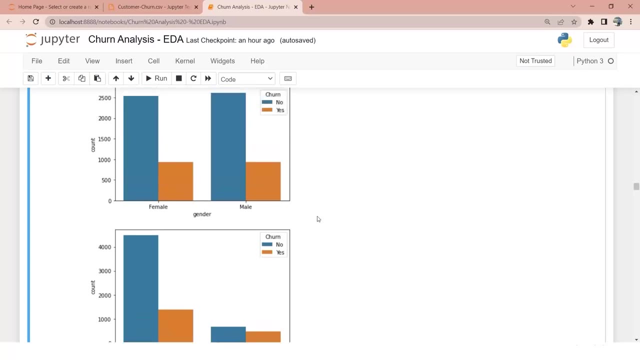 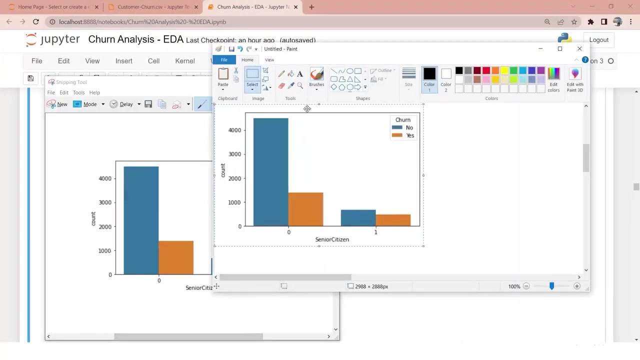 but alone, stand alone. gender is not a triggering point. gender is not impacting the churn. so, coming back to the second graph, let's say we'll talk about senior citizen. senior citizen- i'll again take this and then paste it now. original data 26. remember this in your head? how many churned customers again? i probably don't. 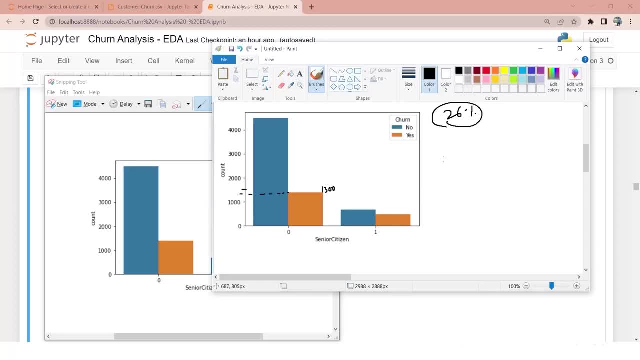 know exactly, but around 1300. okay, you can take help of value counts or take help of any other technique to find these exact numbers, but i am just taking the rough numbers. how many nodes churned? probably around 4500, i would say okay. so what is the ratio? 1300 divided? 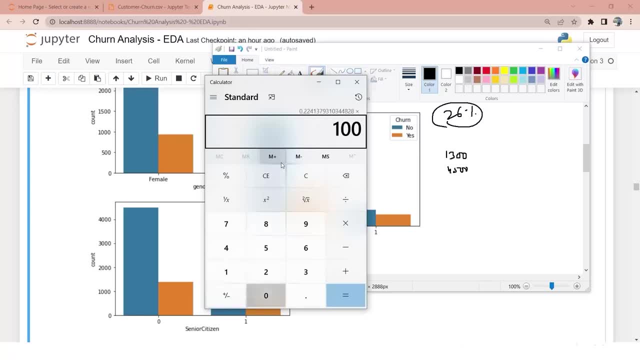 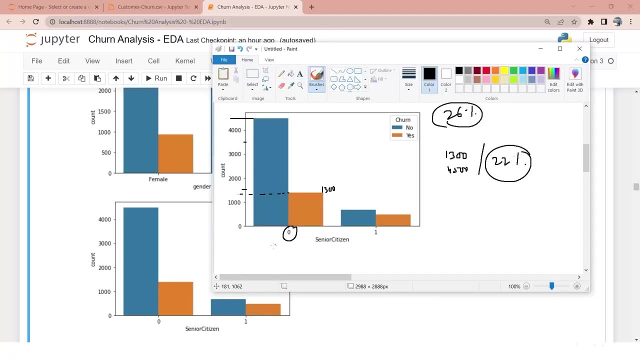 by total, which is five thousand eight hundred, almost twenty two percent. that is размерability glue. Redmi CPU churn value is 65tu to 3200 to understand that number and that's why too much percent- 22 percent- of the people who are not senior citizen are churning. what about senior citizen? 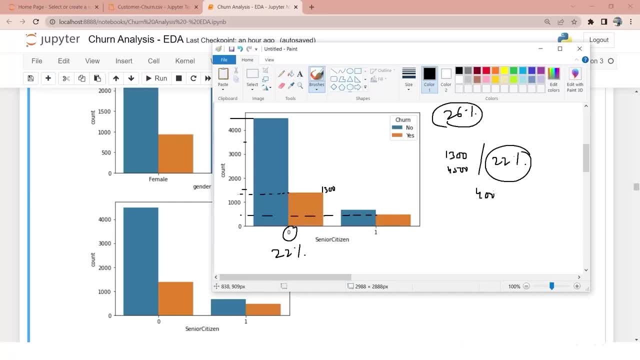 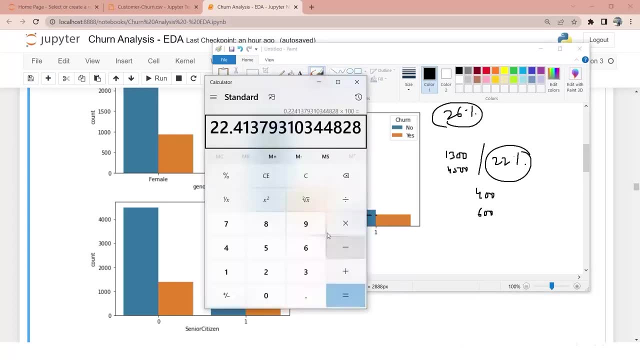 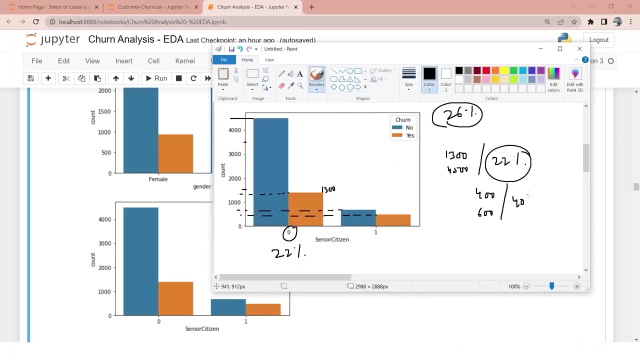 around around 400 or 500 are churned and around 600 or 700 are not churned when senior citizen are becoming same wright for rob like this. so senior citizen, almost st burger 100. so 400 divided by thousand into 100, almost 40 percent. 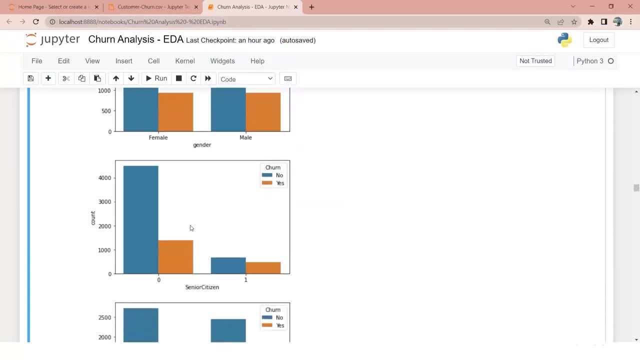 so senior citizen: almost 40 percent. now this is where we got our first insight. what is the inside in every graph? to interpret some analysis, interpret some insights. now i will skip these columns. like partner and you can see in the partner also people who have no partner. they are more likely to churn. 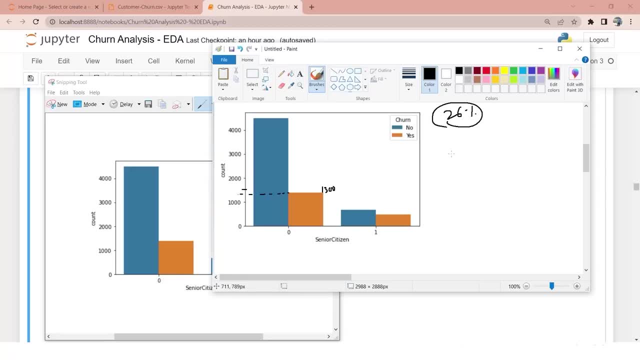 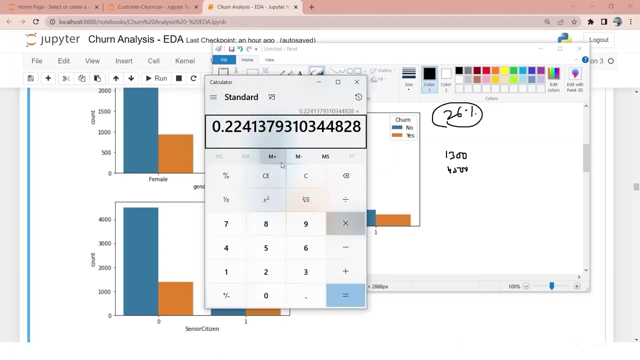 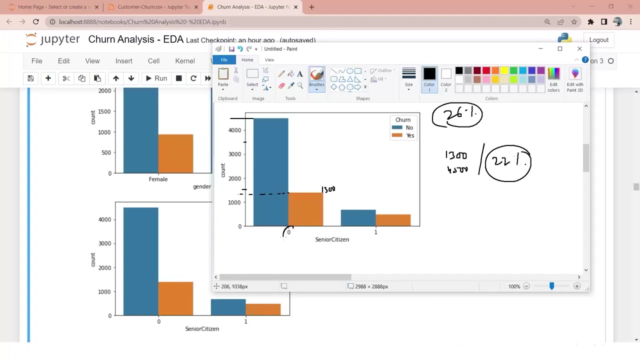 okay, you can take help of value counts or take help of any other technique to find these exact numbers, but i am just taking the rough numbers. how many not churned? probably around 4500, i would say okay, so what is the ratio? 1300 divided by total, which is 5800, almost 22 percent, 22 percent of the people who are not senior citizen. 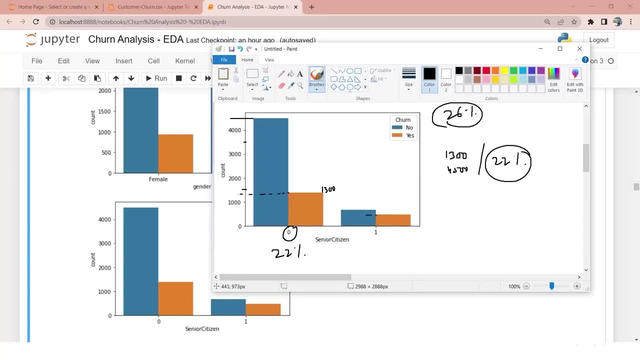 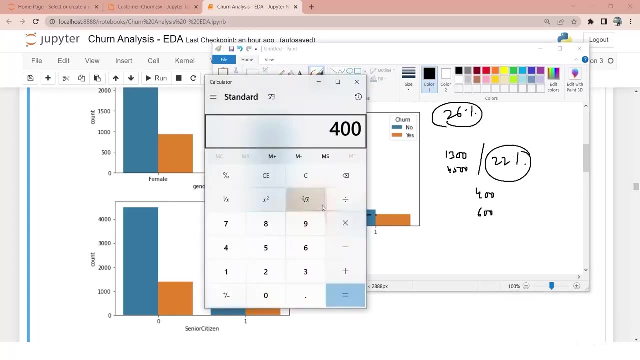 are churning. what about senior citizen? around around 400 or 500 are churned and around 600 or 700 are not churned. so 400 divided by 1000 into 100- almost 40 percent. so senior citizen: almost 40 percent. now, this is where we got our first insight. 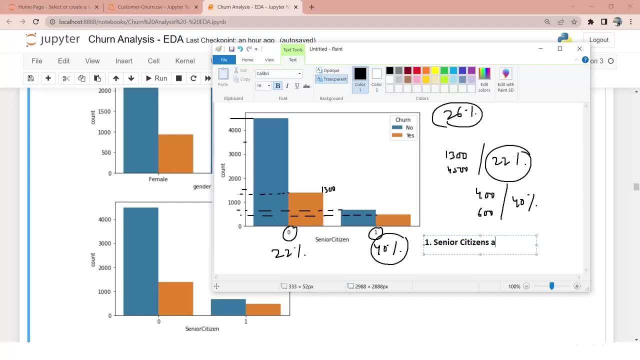 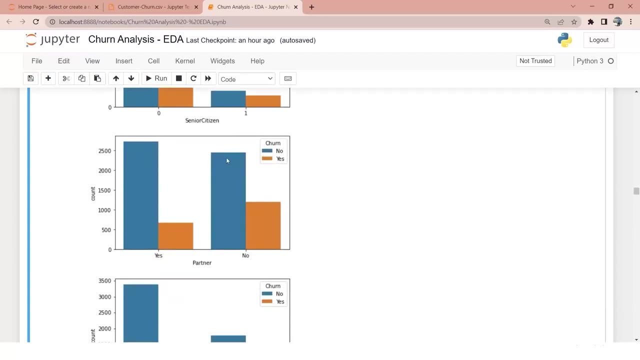 what is the insight? senior citizens are more likely to churn. that is my first insight. similarly, you have to go through each and every graph to interpret some analysis, interpret some insights. now i will skip these columns- like partner, and you can see in the partner also people who have no partner. they are more likely to churn. you can see the. 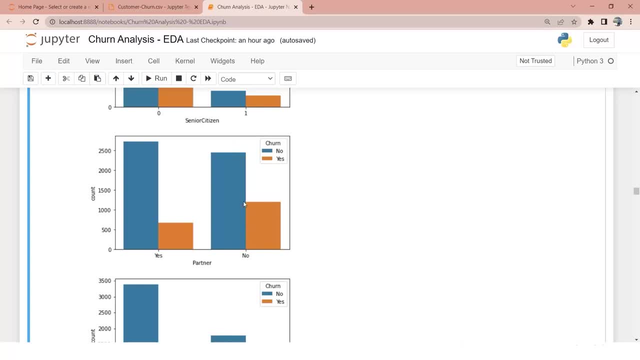 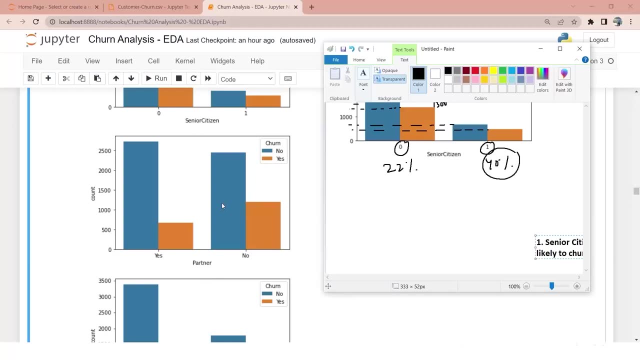 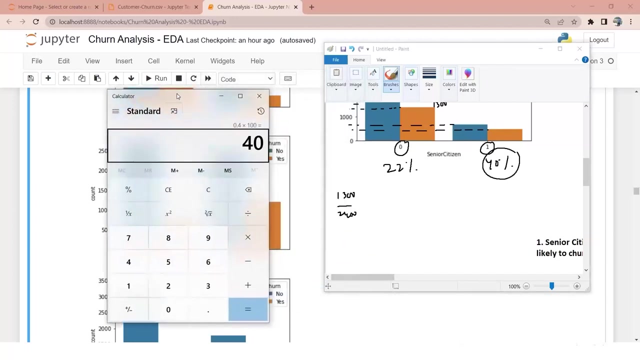 active customer customers are less in case of no, but churn customers are high. if you talk about the ratio, probably I could say let's say, around 1300, around 1300 churned and around 2400 not churned, the total number of around three thousand seven. 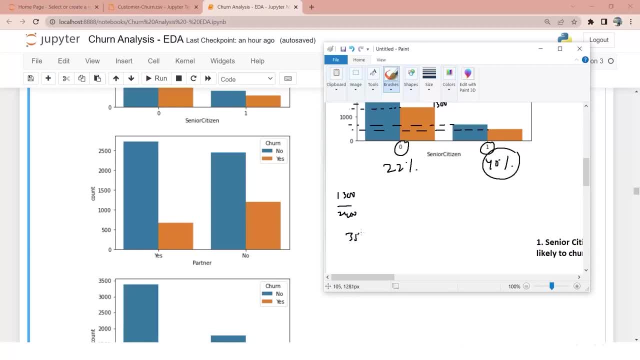 hundred and two hundred around 35 percent- around 35 percent- churn rate for people with no partners. so my second insight could be: people with no partners are more likely to churn. so that's how you build up your insights: you start analyzing data, univariate by variate, combine multiple variables and then come to a conclusion. I'll quickly 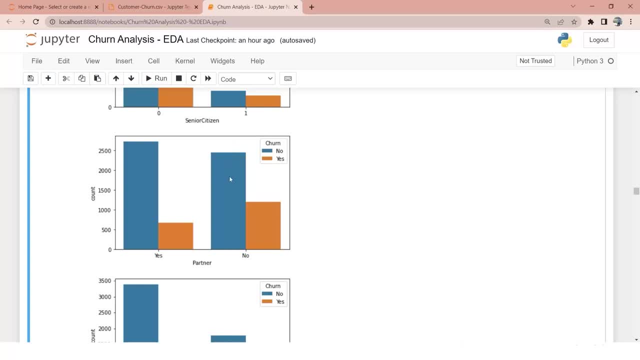 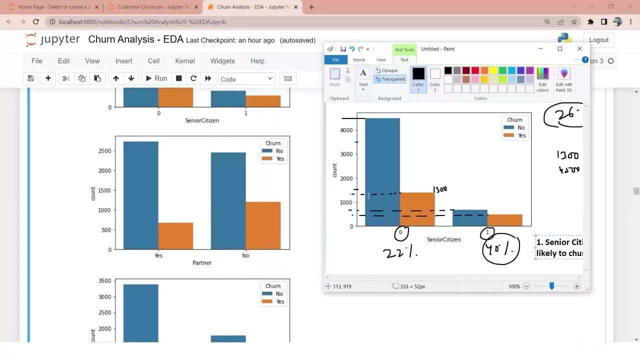 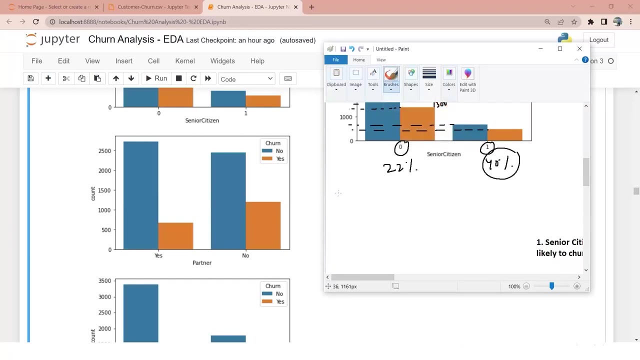 you can see the active customers are less in case of no, but churn customers are high. if you talk about the ratio, probably i could say, let's say, around 1300, around 1300 churned and around 2400 not churned, the total number of around 3700 into 100, around 35 percent. 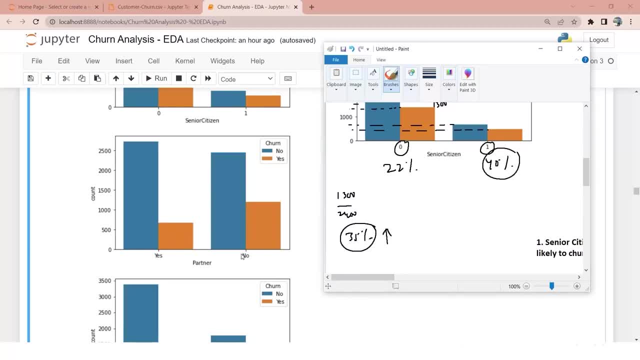 around 35 percent churn rate for people who have no partner- people with no partners. so my second insight could be: people with no partners are more likely to churn. so that's how you build up your insights: you start analyzing data- univariate, bivariate, combine multiple variables and then come to a conclusion. 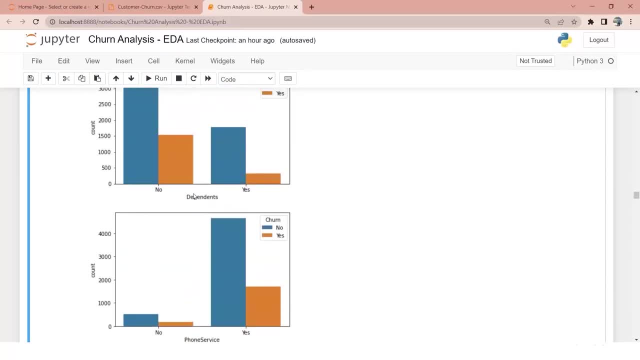 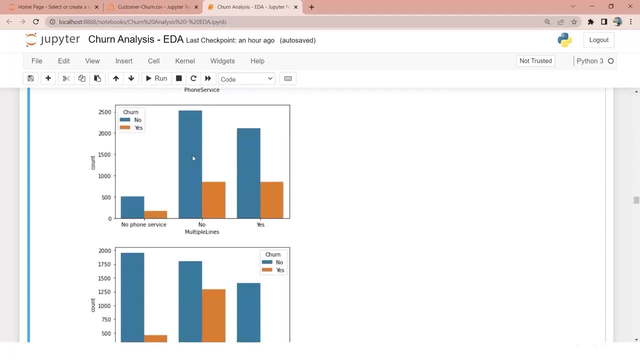 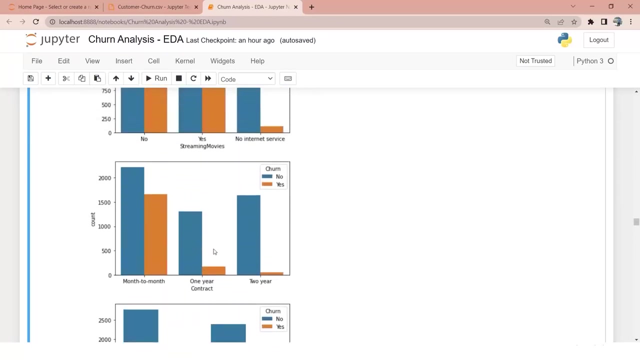 i'll quickly jump into one more important feature, because i have already analyzed this data. you can do the same step for each and every graph, so i'll quickly skip to a feature called as contract. okay, contract is an important feature, so i will take the screenshot using a sniping tool. snipping tool and then. 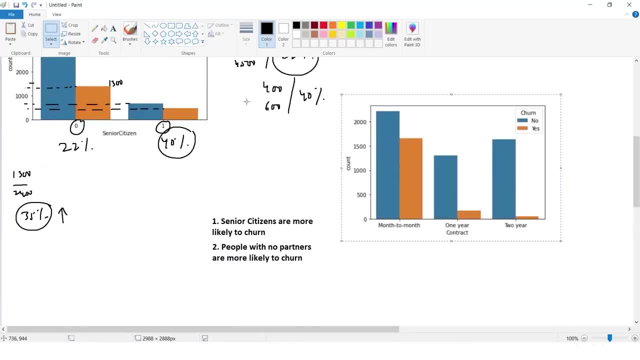 to probably. i will do it here. i will do it here. okay, now, from this particular graph: how many monthly customers who have churned around 1200, how many total not churned around 2400. exact numbers again, i'm not sure: how many one yearly customers around 200 and how many churned. 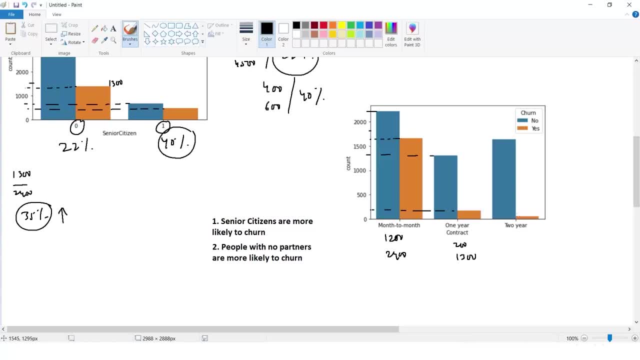 sorry. how many not churned around 1300? how many people churned around 100 or 200? how many not churned again around around 1700 or something? so what is the ratio? let's try to calculate for monthly customers: 1200 divided by 3600 into 100, almost 33 percent of the people are churning. 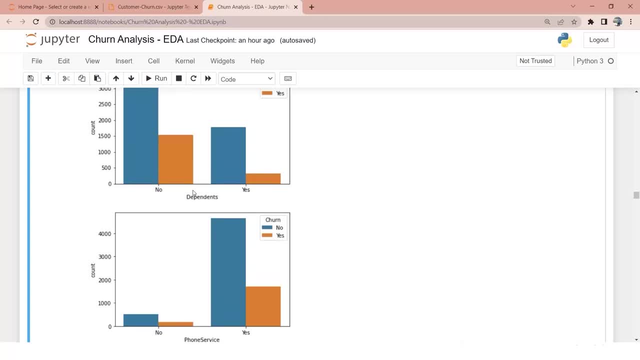 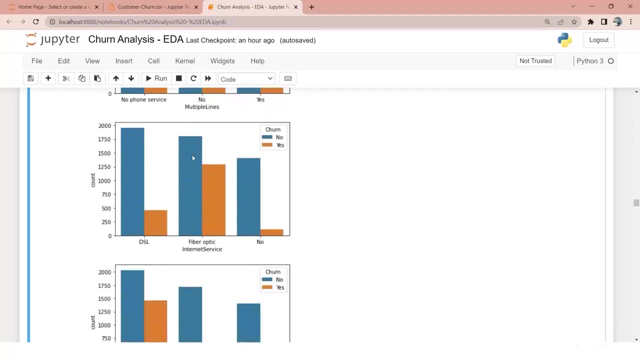 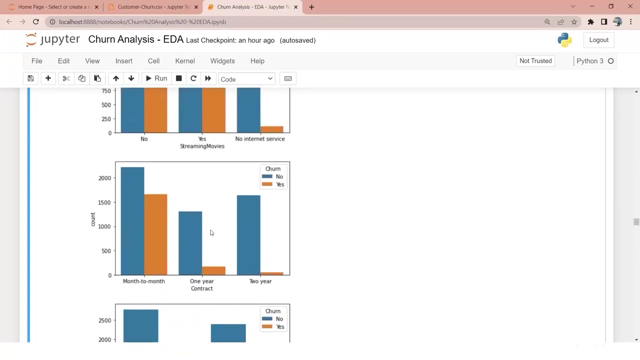 jump into one more important feature, because I have already analyzed this data. you can do the same step for each and every graph. I'll quickly skip to a feature called as contract. okay, contract is an important feature, so I will take the screenshot using the sniping tool. sniping tool. 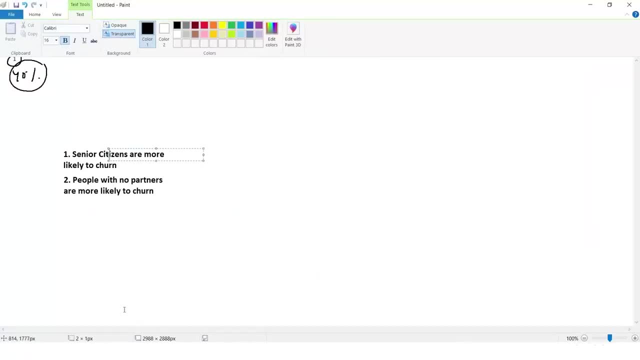 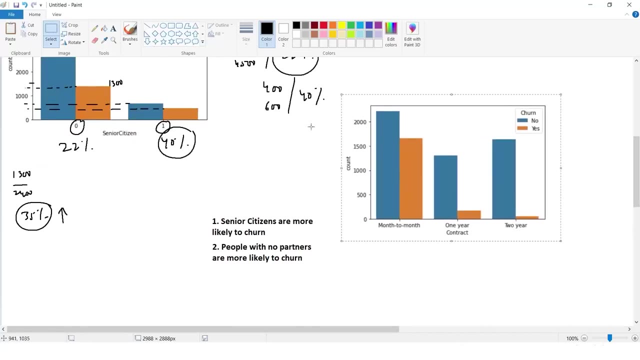 and then probably I will do it here. I will do it here. okay, now, from this particular graph, how many monthly customers will have churned around 12 hundred? how many total not churned around? 2,400, exact numbers again, I'm not sure how many. 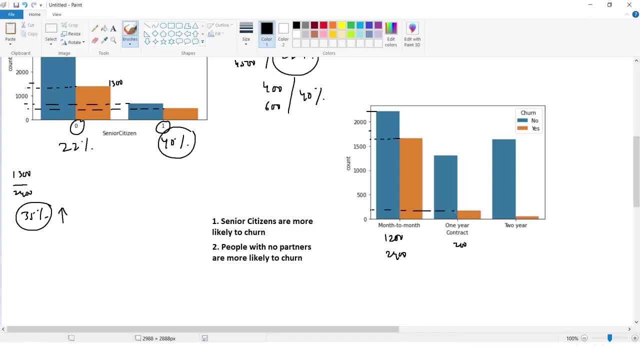 one yearly customers around 200, and how many churned- sorry, how many not churned- around 1300? how many people churned around 100 or 200? how many not churned again around around 1700 or something? so what is the ratio let's try to calculate for monthly customers: 1200. 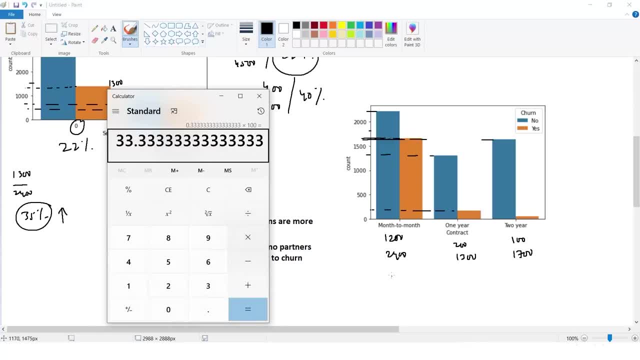 divided by 3600 into 100, almost 33 percent of the people are churning. sorry, not 1200. you can see the orange graph is too high. almost 1700, almost 1700. so there is a mistake here. almost 1700 divided by total would be 4100 in 200. almost. 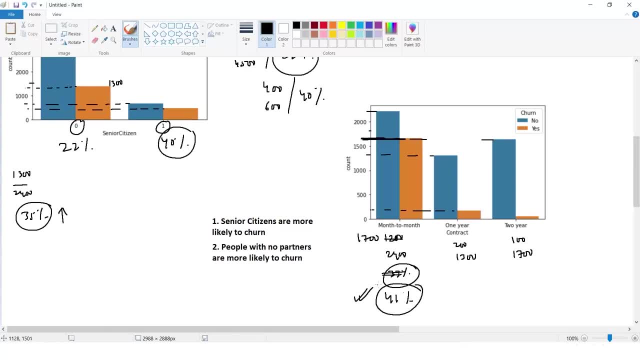 41 percent of the people. people are churning around under…… subtitles for Kannada sub'admin & our politics. the people who are having monthly contracts are churning. what about one yearly? one yearly is around 200 by 1500 and 200 around 13 percent, and two yearly is around five percent. now, this feature. 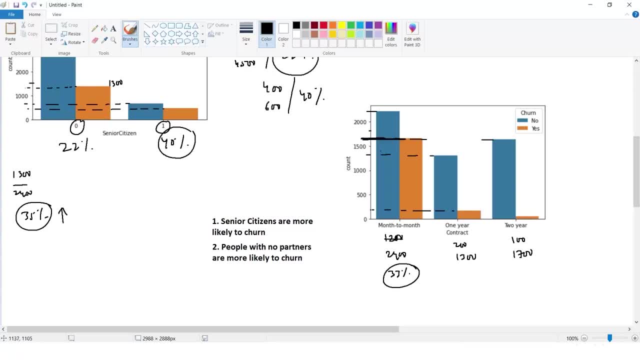 sorry, not 1200. you can see the orange graph is too high. almost 1700, almost 1700, so there is a mistake here. almost 1700 divided by total would be 4100 in 200. almost 41 of the people who are having monthly contracts are churning. what about one yearly? one yearly is around. 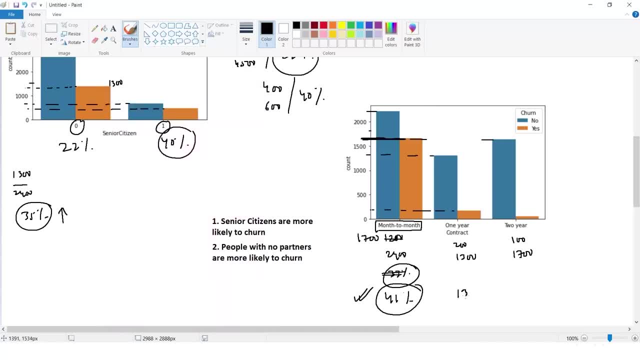 200 by 1500 and 200 around thirteen percent, and two yearly is around five percent. now, this feature. let me explain you about this feature, as you might be having domain knowledge, you can understand the meaning of the feature here. this feature basically means contract. now, how does contract works in telecom? 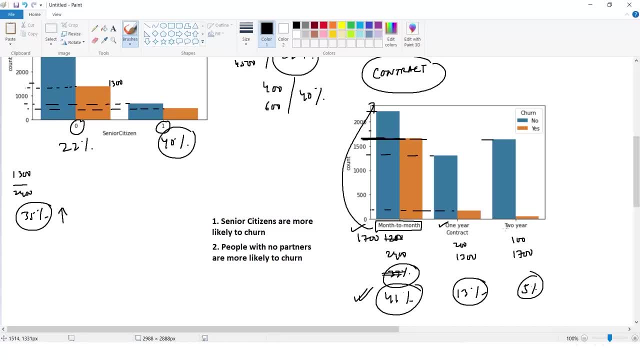 here we have three contracts: monthly contract, one yearly, two yearly. now, if you have a one-year contract, that means even if you don't like the company, even if the company sucks, even if the company has bad offers or bad service- anything- you cannot leave the company without paying the entire fees of one year. 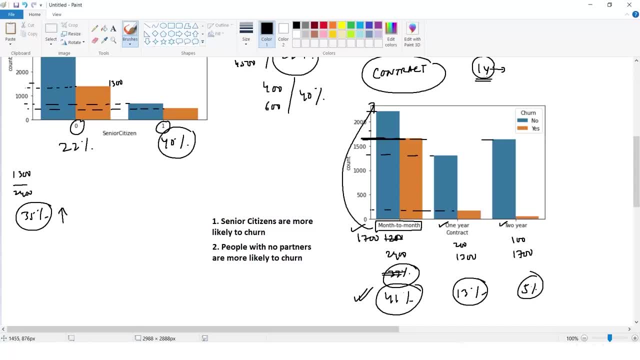 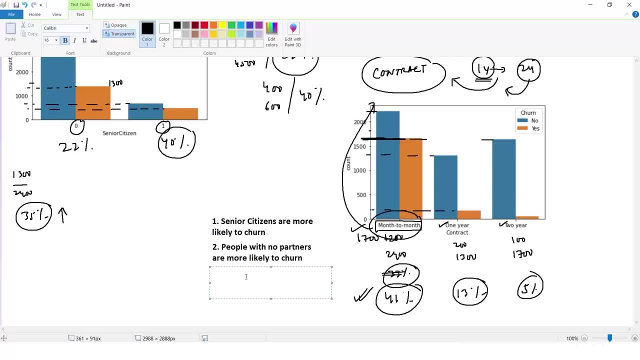 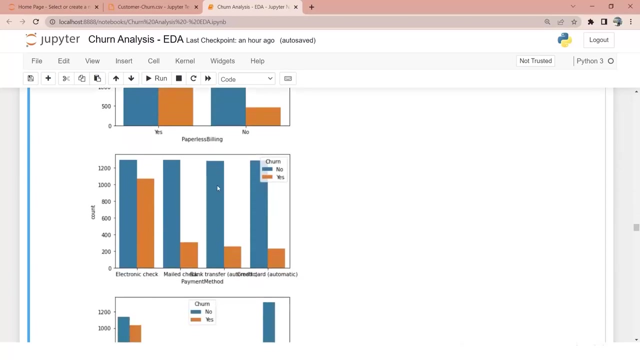 obvious insight. but an insight is an insight, right. so the insight is: monthly contracts are more likely to churn because they're free customers. three customers as in. they don't have any contract. jumping back to the university analysis, similarly you have to do further uni weather analysis. you can see payment method. the first category is electronic check. 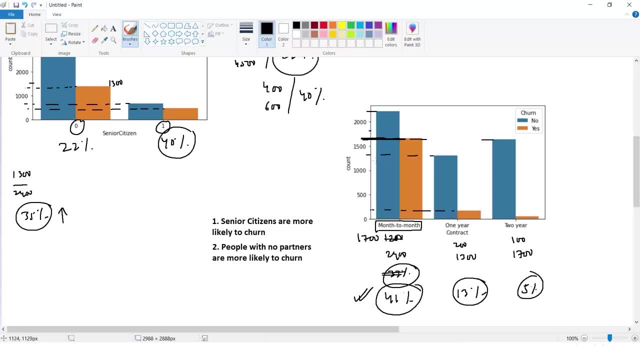 let me explain you about this feature, as you might be having domain knowledge, you can understand the meaning of the feature here. this feature basically means contract. now how does contract works in telecom? here we have three contracts: monthly contract, one yearly, two yearly. now, if you have a one year contract, that means even if you don't like the company, even if the company sucks, even. 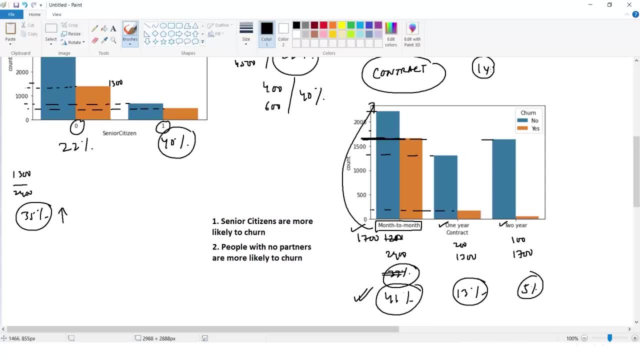 if the company has bad uh offers or bad uh service, anything, you cannot leave the company without paying the entire fees of one year because you are bounded with a contract. so it is quite obvious that less people will churn. same with two yearly. less people will churn, but monthly customers are. 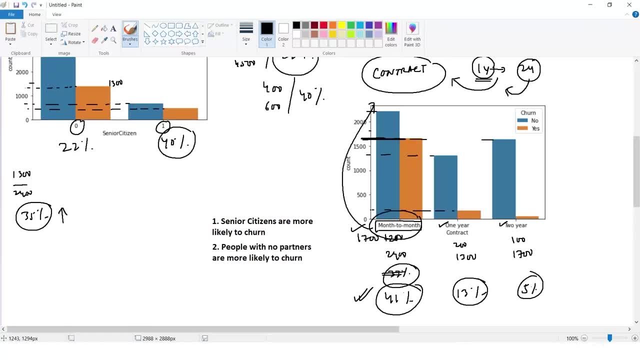 free. if you have a problem, service problem or anything goes wrong, they will quickly churn and jump into another company. so it's a very, quite obvious insight. but an insight is an insight, right? so the insight is: monthly contracts are more likely to churn because they're free customers. 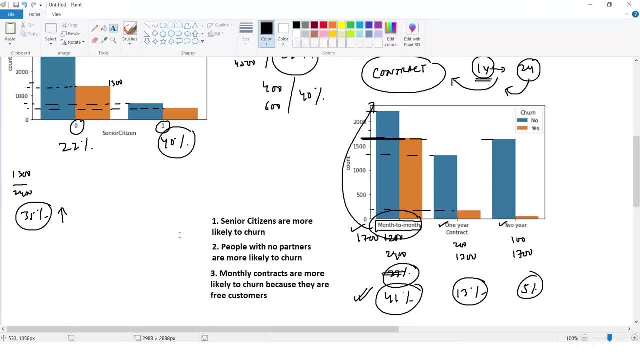 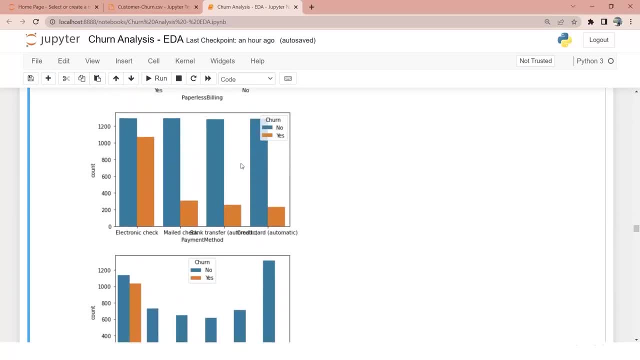 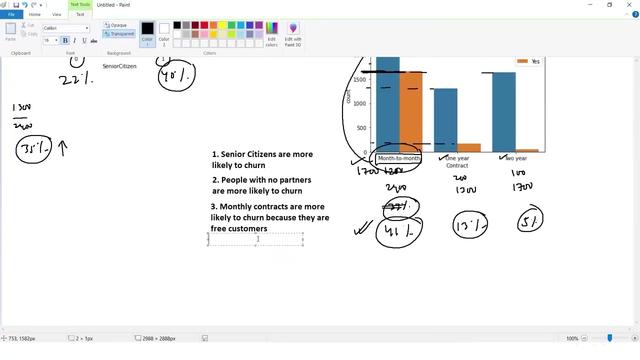 free customers, as in they don't have any contract. jumping back to the univ rate analysis. similarly, you have to do further univ rate analysis. you can see payment method. the first category is electronic check and very high percentage of churn ratio right. so again, another insight would be: 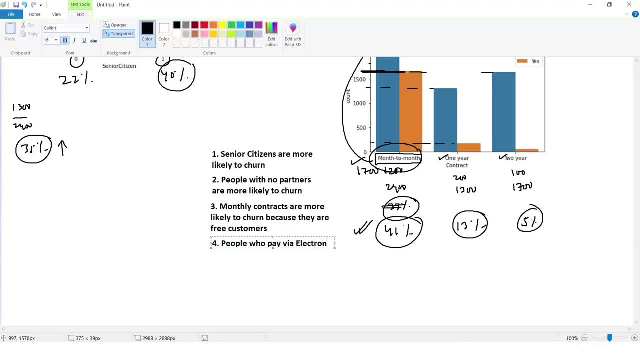 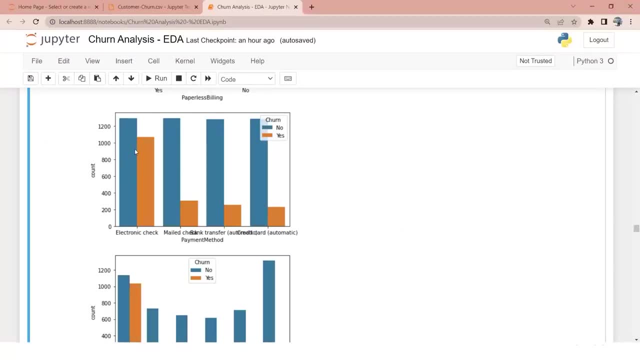 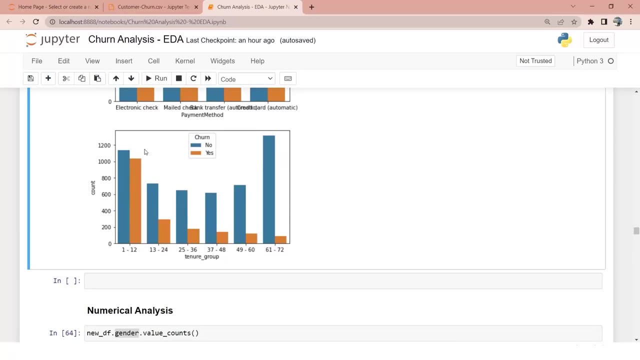 people who pay via electronic check are more likely to churn. electronic check more likely to churn. similarly, you have to go through each and every graph to interpret some analysis. there could be scenarios where you can get insights very easily. there could be scenarios you where you might not get insights. and if you don't get insights then you have to dig into your. 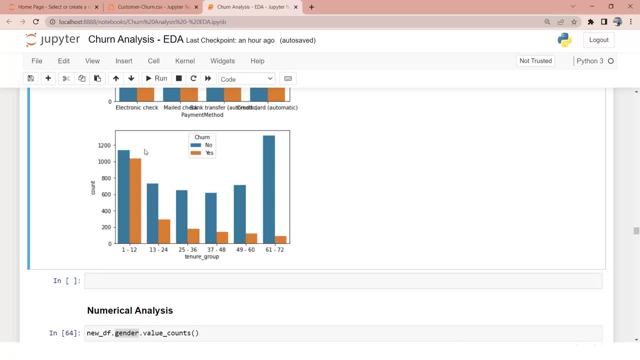 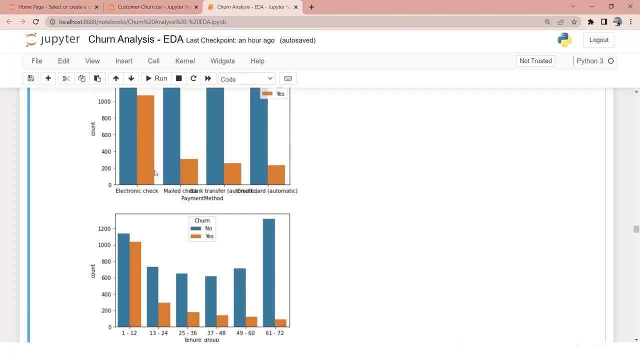 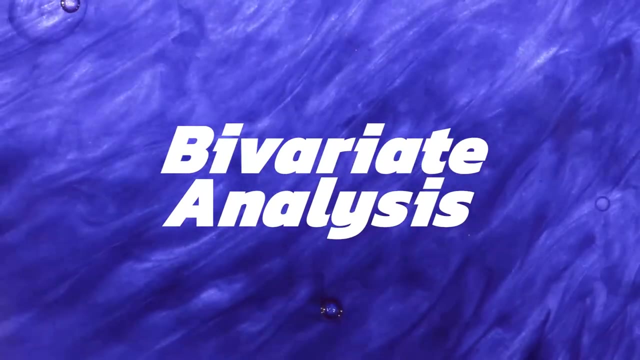 bivariate analysis, multivariate and so on. so overall that's all about univ rate analysis. in the next video we shall be talking about numerical analysis and then in the future we will jump into the bivariate analysis part. here we will be talking about numerical analysis. 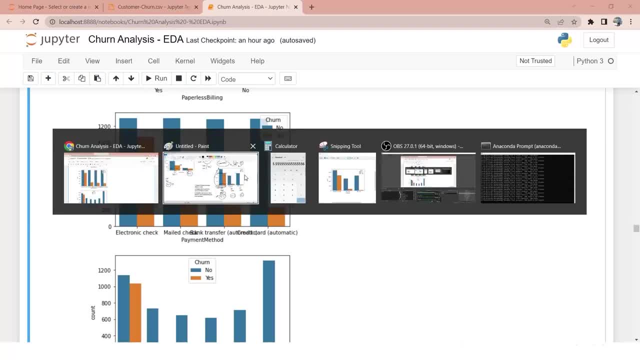 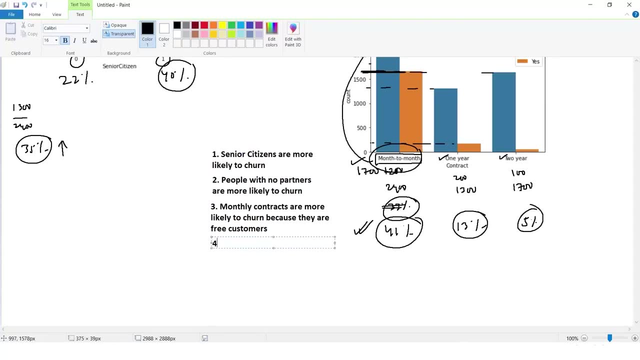 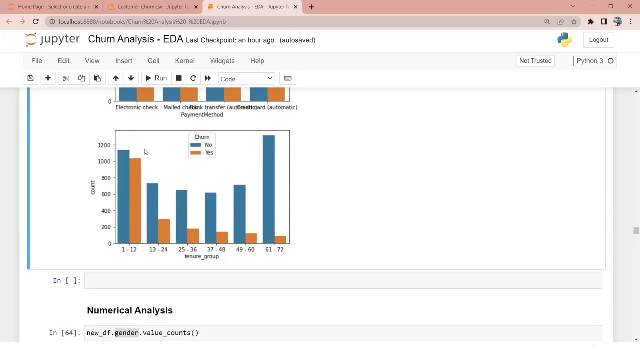 and very high percentage of churn ratio right. so, again, another insight would be: people who pay via electronic check are more likely to jump. electronic check more likely to jump. similarly, you have to go through each and every graph to interpret some analysis. there could be scenarios where you can get insights very easily. there could be scenarios, you where you might not. 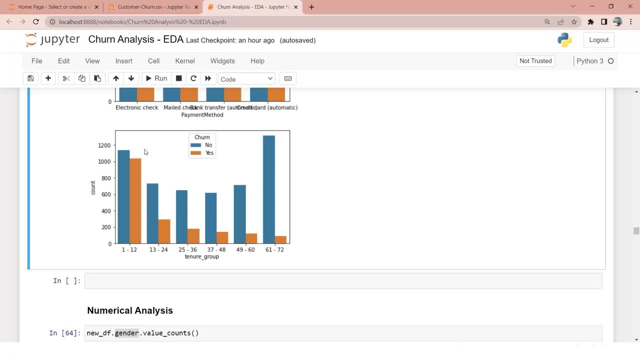 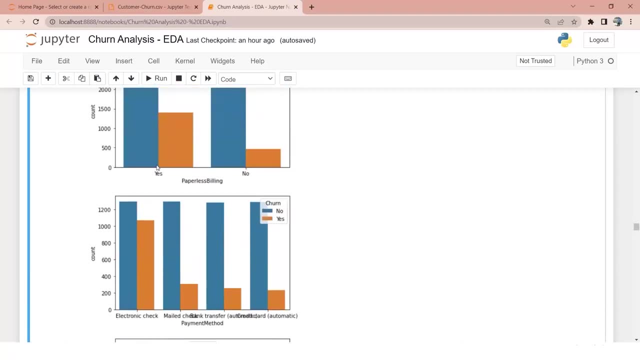 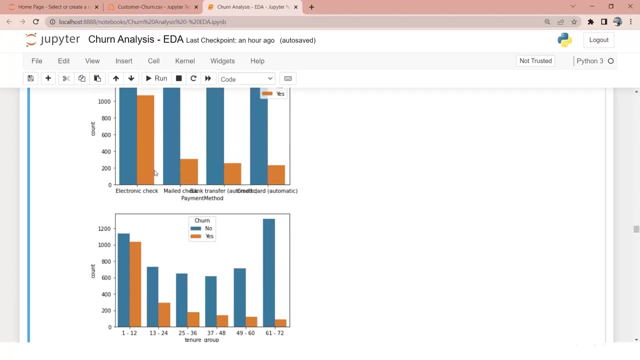 get insights. and if you don't get insights then you have to dig into your bivariate analysis, multivariate and so on. so overall, that's all about univariate analysis. in the next video we shall be talking about numerical analysis and then in the future we will jump into the bivariate. 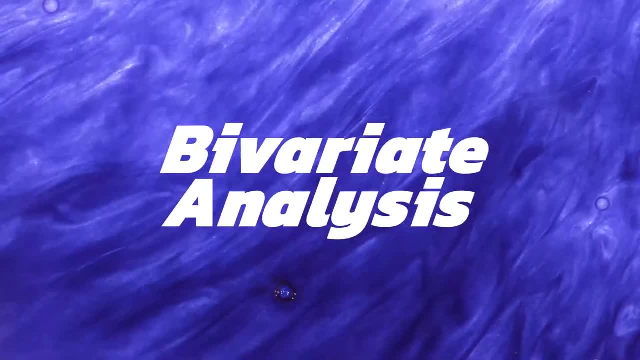 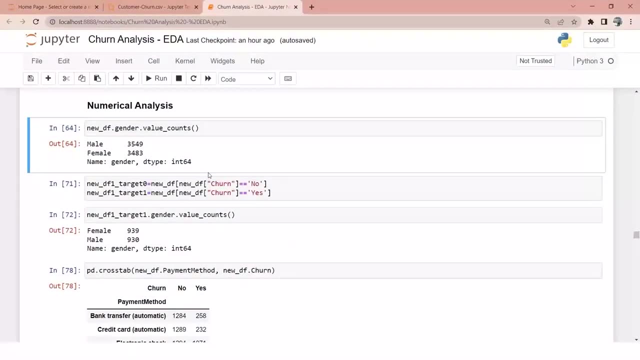 analysis part. jumping into the numerical analysis part. you numerical analysis. we all know that we do this kind of analysis with numerical attributes- single numerical attributes or multiple numerical attributes. we have to perform some analysis. so before getting into the numerical analysis part, i have done some, some quotes probably. i 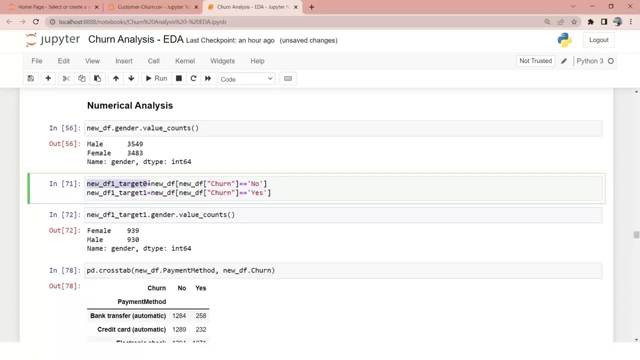 will explain that. so here i am creating a new data frame only for the people who are active, and again another data frame with target one for people who are not active, who have churned. so i am basically dividing the data into churned and active users. talking about the churned users, how does my gender look like? 939. 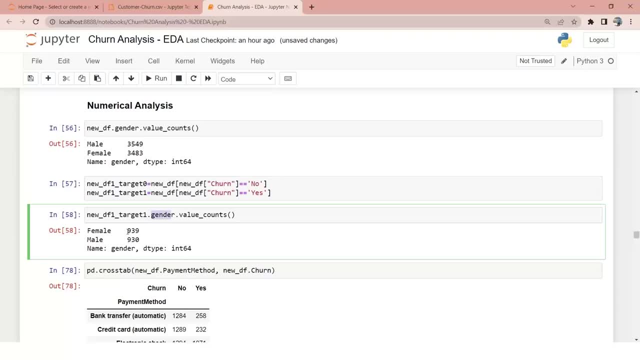 and p-mal and male. similarly, if you talk about the original data, the ratio is almost one. yes to one. here also, it is one to one, and then, if you like, you can also makeraszamSUPS- horrible. sorry, yeah, because this data does not come in one來 for you. ther upstairs again, we will see how. adjust back to our mass. okay, good, so now, as you see, our trends are. you use your data too. you have to check whether you are active or not. cheer, absolutely, that is good over here as well. another example, just to see what the difference between you see, between the bias and без. 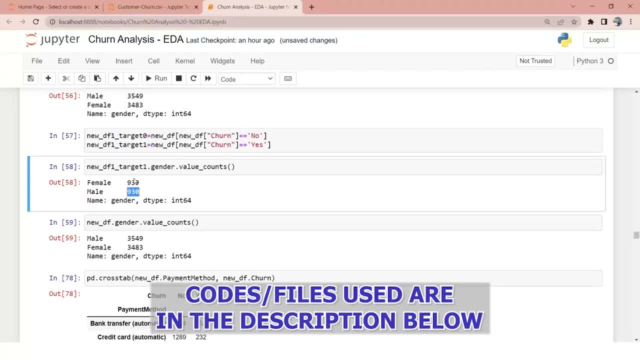 how does my working anything? is it together how you track whether you are active in terms of data use of one over there also, it is one is to one. so if you want to do your univariate analysis using graphical or visual analytics, you can do without visual analytics also. you can do like this. so getting ahead with the 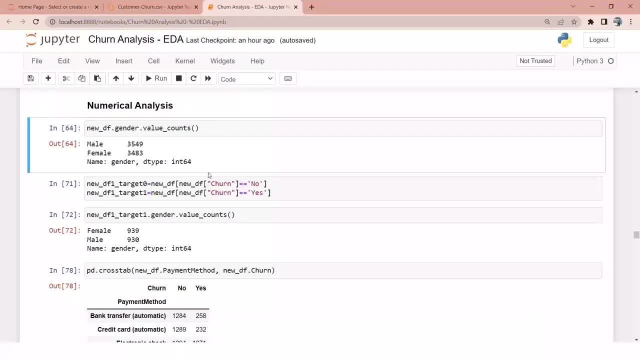 jumping into the numerical analysis spot. numerical analysis: we all know that we do this kind of analysis with numerical attributes- single numerical attributes or multiple numerical attributes- we have to perform some analysis. so before getting into the numerical analysis part, i have done some, some quotes. probably i will explain that. so here i am. 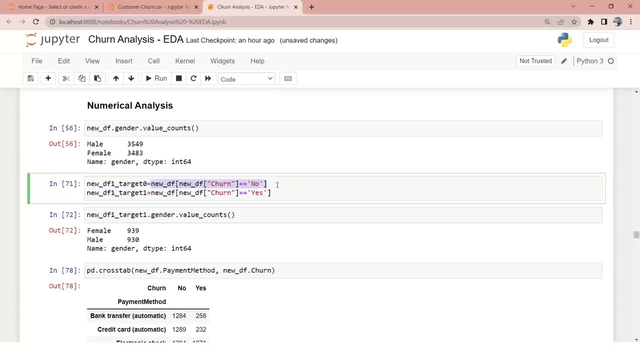 creating a new data frame. i can define the data here. i can define the data frame in the tab. i can frame only for the people who are active and again another data frame with target one for people who are not active, who have churned. so i'm basically dividing the data into churned and active users. 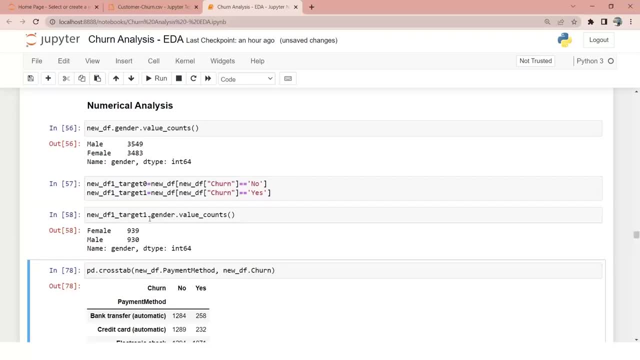 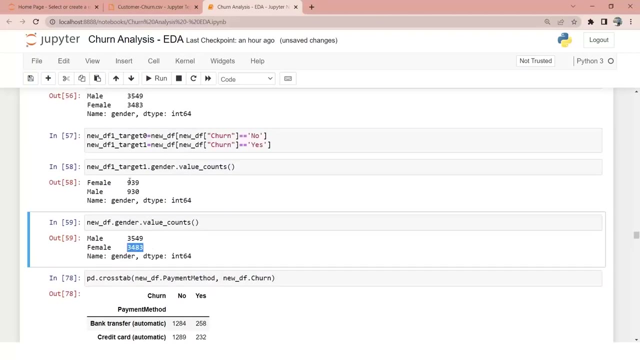 talking about the churned users, how does my gender look like? 939 and 930, female and male. similarly, if you talk about the original data, the ratio is almost one is to one. here also, it is one is to one. so if you want to do your univariate analysis using graphical or visual analytics, you 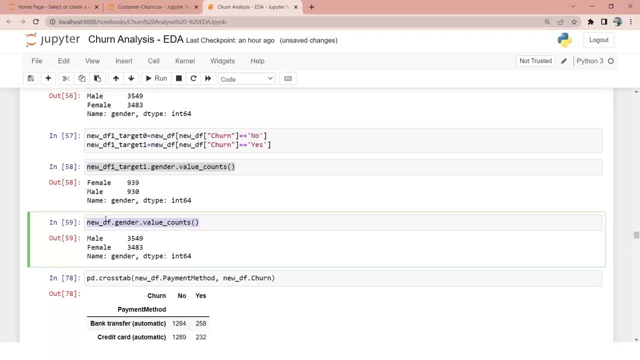 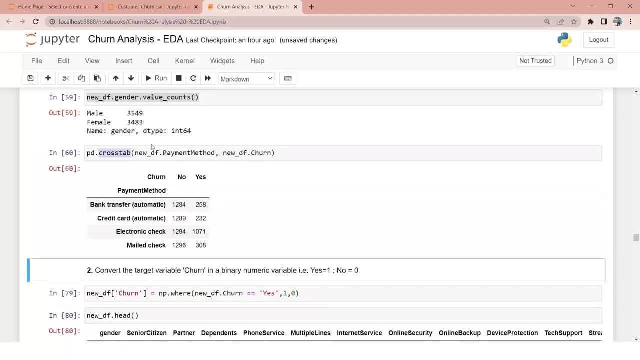 can do without visual analytics also, you can do like this. so, getting ahead with the next things that we have done here, i am creating a cross tab between payment method and churn, which basically tells you that, for bank transfer, people who have churned are 258, not chunder 1284.. 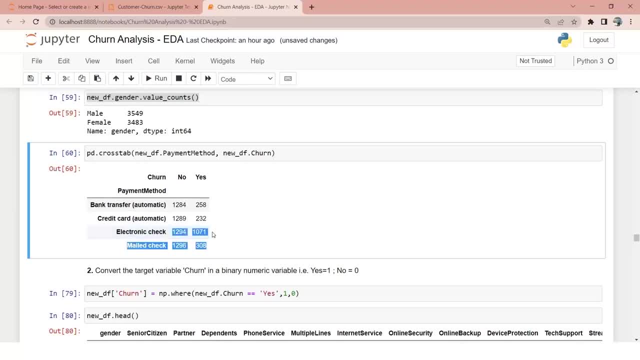 for electronic check. it is a one is to one ratio. you can see one is to one ratio. so if you talk about how many total electronic check do we have 1071, which is 2365, 2365 into 100, almost 45 percent of the people. 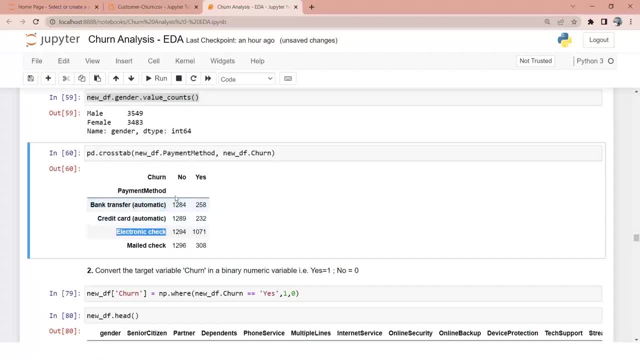 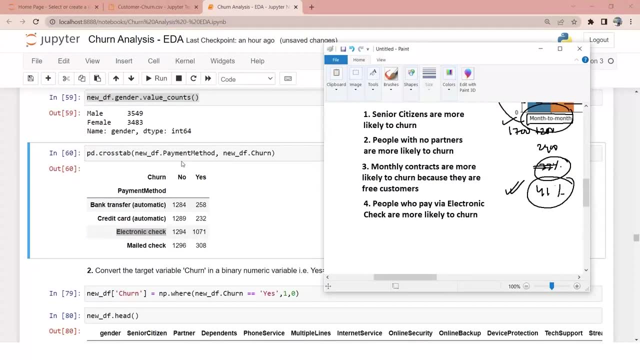 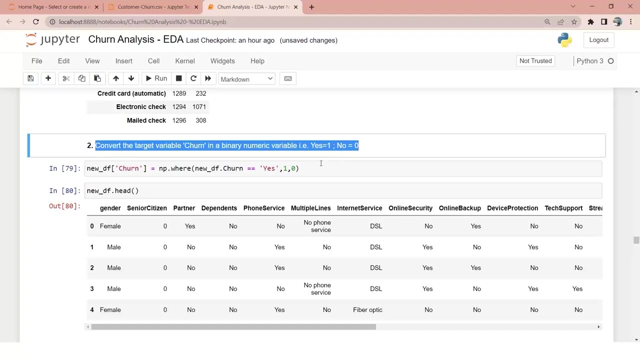 who are using electronic check are churners. right, and this is what we already got from the previous graphs from the univariate analysis part right, so jumping into more into the numerical part. so in order to continue with the numerical analysis, it is better to convert the target variable into numerical attributes as well. so here i am converting my churn into one and zero. 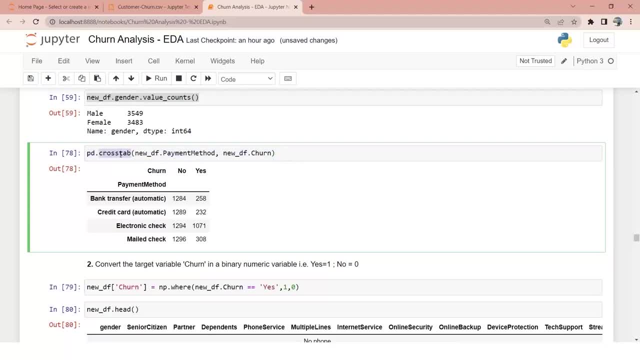 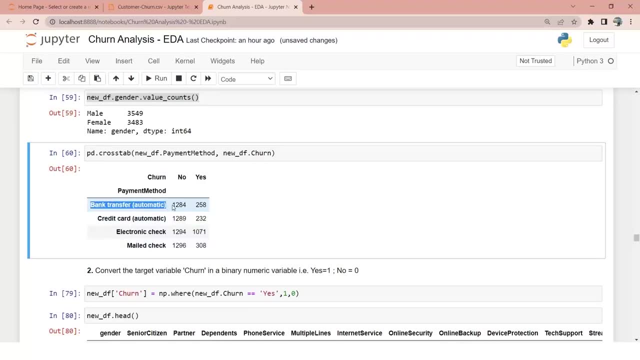 next things that we have done here. i am creating a cross tab between payment method and churn which basically tells you that for bank transfer, people who have churned are 258, not churned are 1284. for electronic check it is a one is to one ratio. you can see one is to one ratio. so if you 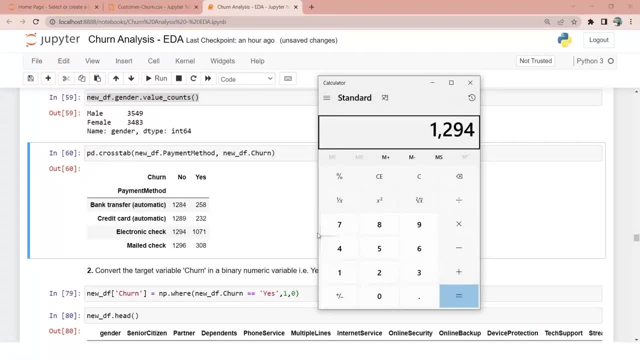 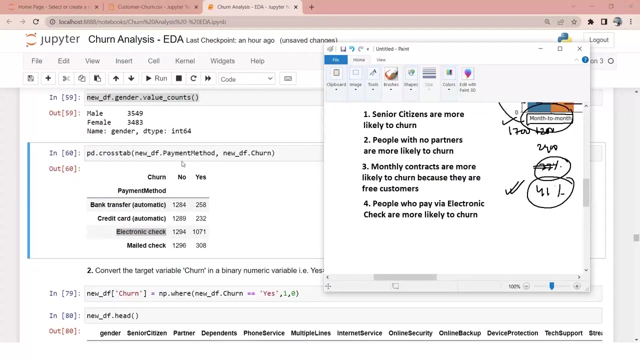 talk about how many total electronic check do. we have 1071, which is 2365, 2365 into 100. almost 45 percent of the people who are using electronic check are churners. right, and this is what we already got from the, the, the previous graphs from the univariate analysis, part right. so jumping into more into the numerical 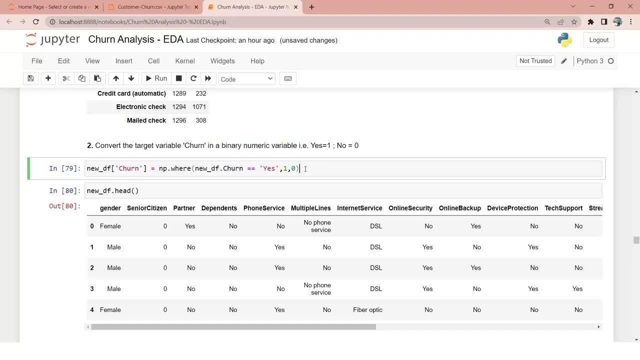 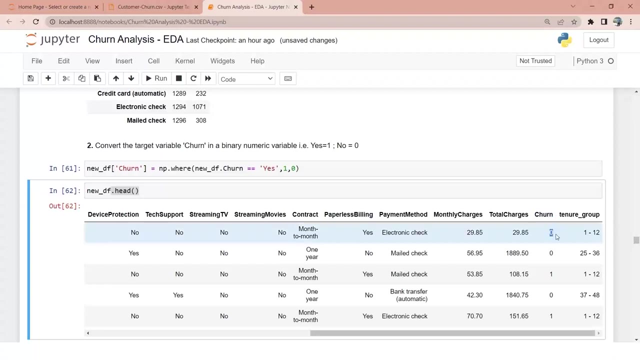 part. so in order to continue with the numerical analysis, it is better to convert the target variable into numerical attributes as well. so here i am converting my churn into one and zero and if you see i am plotting the dot head, you will see the churn has been converted to one and zero. 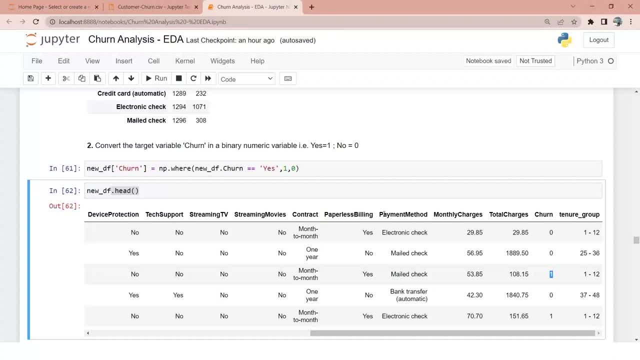 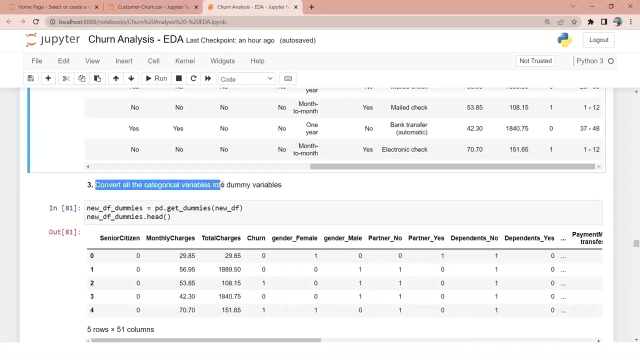 why we have done? because we will be doing some correlation things, we will be calling correlation function, and those statistical and mathematical functions might not work with categorical data. so we are converting into ones and zeros. we are also converting all the categorical variables into dummy variables. now a flashback to 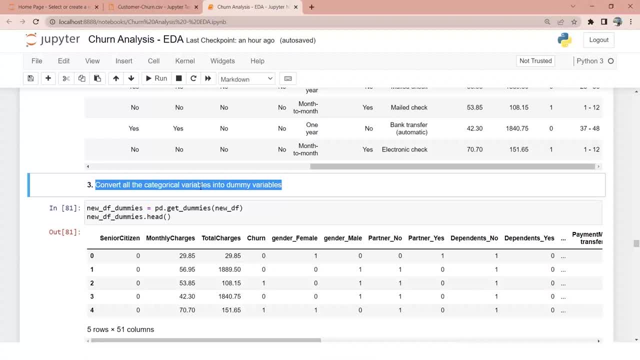 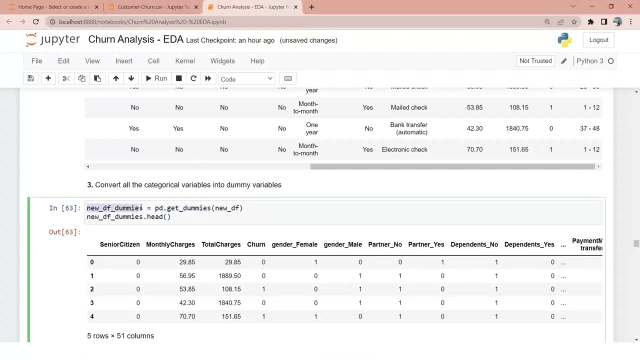 the feature encoding techniques. i told you that there are multiple feature encoding techniques, which includes label encoding, one hot encoding, dummy encoding. here we are performing a dummy encoding, so i'm calling pd dot get dummies and i'm converting my data frame into dummies. so now you can see. initially i had less amount of columns. 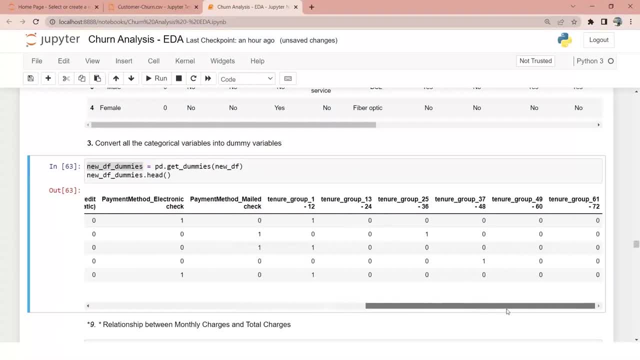 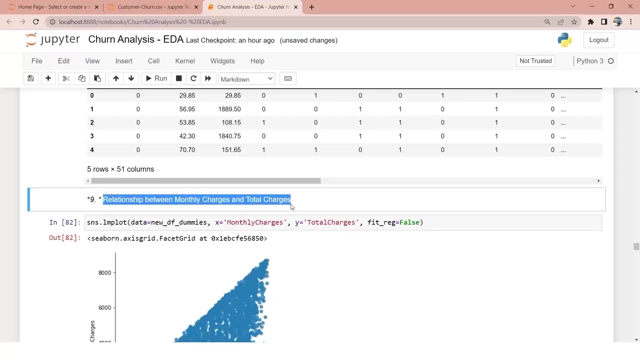 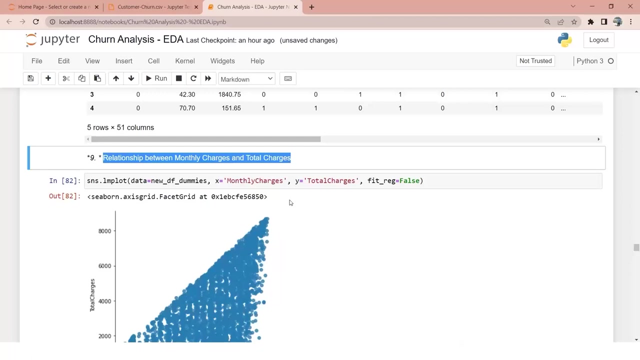 around 2021. now i have 51 columns because dummy variables has been created. okay, for each payment method, multiple dummy variables has been created. we'll first analyze the relationship between monthly charges and total charges. okay, i know. somehow, using my domain knowledge, i already know that monthly charges and total charges are. 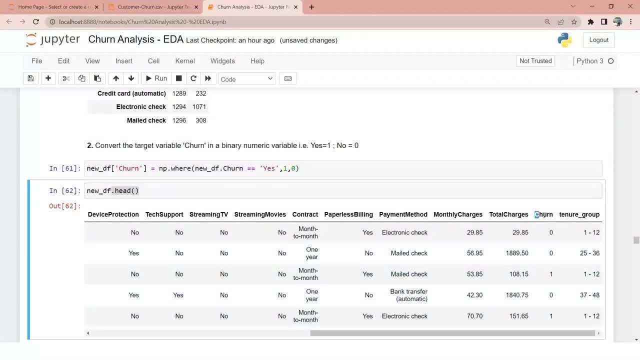 and if you see the dot head you will see the churn has been converted to one and zeros. why we have done? because we will be doing some correlation things we will be calling correlation function, and those statistical and mathematical functions might not work with categorical data. so we are converting. 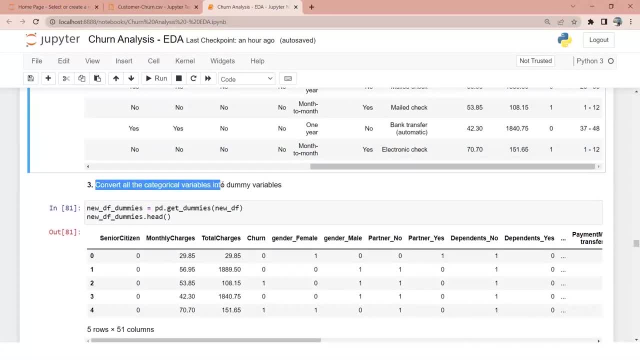 into ones and zeros. we are also converting all the categorical variables into dummy variables. now a flashback to the feature encoding techniques. i told you that there are multiple feature encoding techniques, which includes label encoding, one hot encoding, dummy encoding. here we are performing a dummy encoding, so i'm calling pdget dummies and i'm converting my dataframe into dummies. 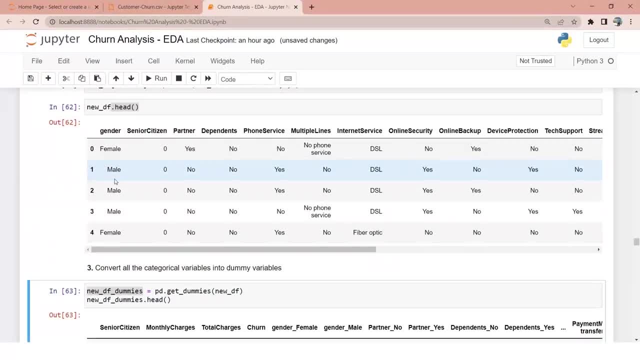 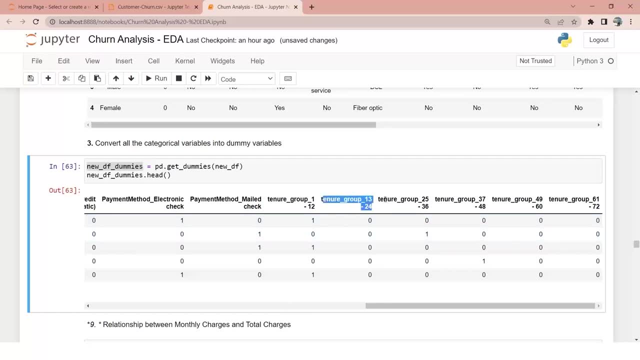 so now you can see: initially i had less amount of columns- around 20- 21. now i have 51 columns because i'm not using more than 50 columns. so that's why i am terming it pd dot get dummies. dummy variables has been created. okay, for each payment method, multiple dummy variables has been. 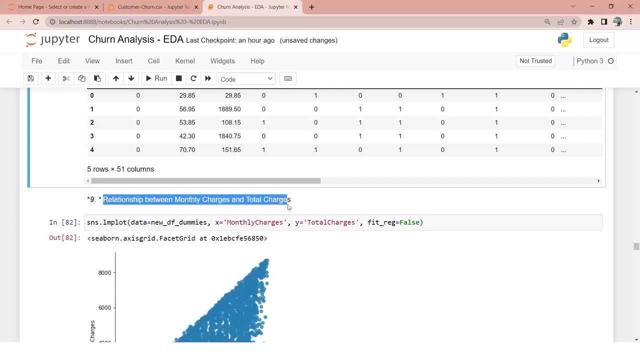 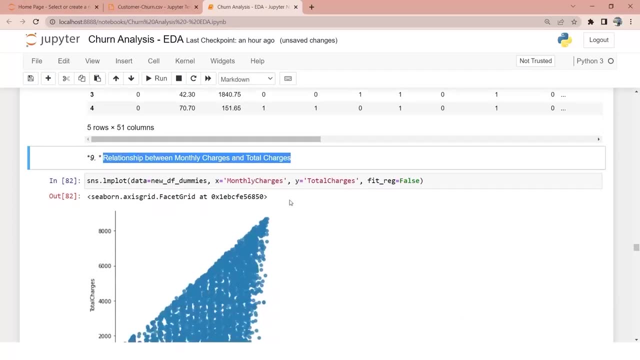 created. so we'll first analyze the relationship between monthly charges and total charges. okay, I know, somehow, using my domain knowledge, I already know that monthly charges and total charges are positively correlated, but I just want to plot it, so I'm using an LM plot and I'm passing. 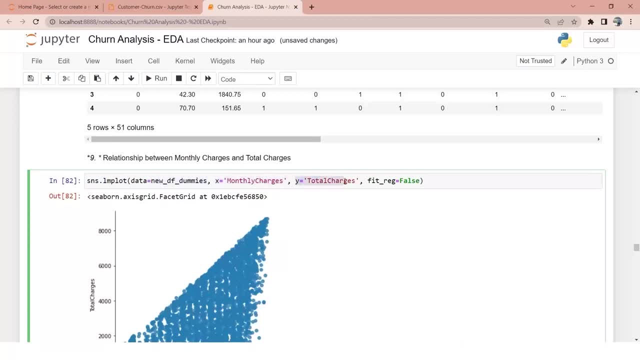 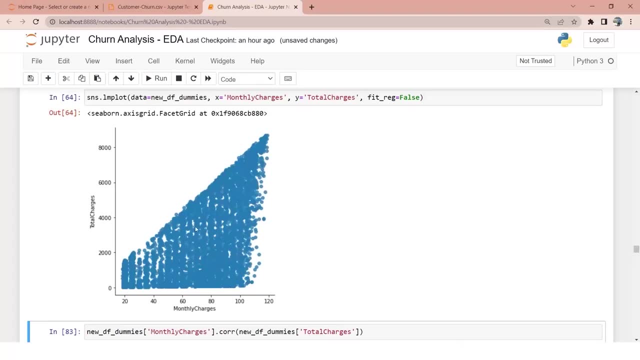 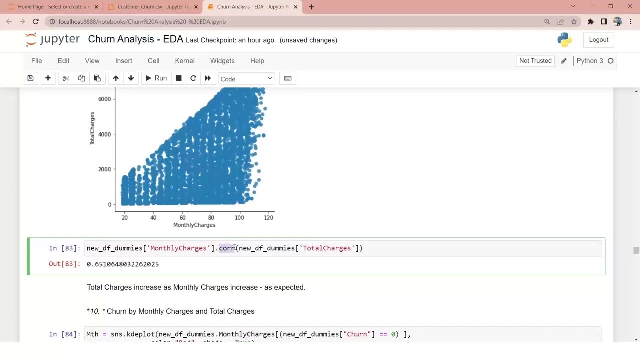 my dummies, data in the x-axis and passing monthly charges, and y-axis and passing the total charges. well, run this and you can see that somehow for some data points it is difficult to interpret, but most of the data points I can see an increasing trend right. if you want to calculate the correlation you can see between monthly charges and the total. 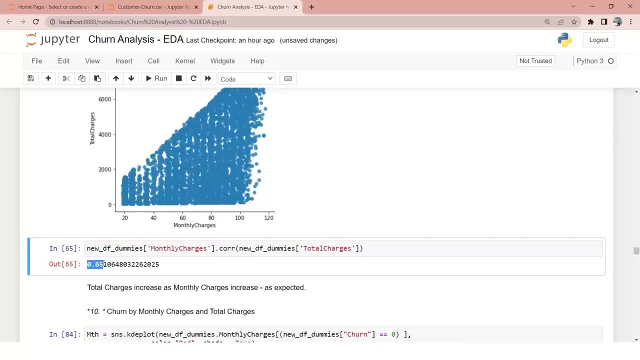 charges. I am calling the correlation function and the correlation is 0.65 and we all know that correlation value ranges from minus 1 to 1, 1 being the highest, minus 1 being the lowest. if the number is very close to 1, that means they are positively correlated- correlated. so, in this case, the variable 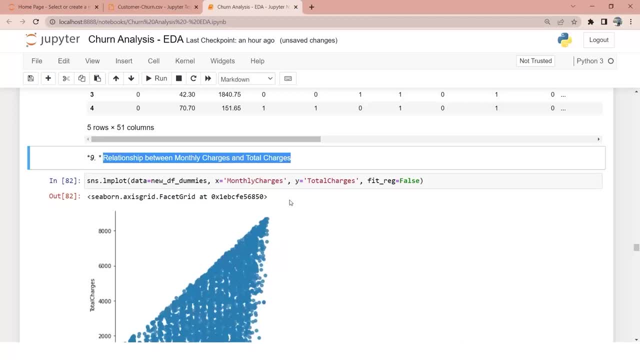 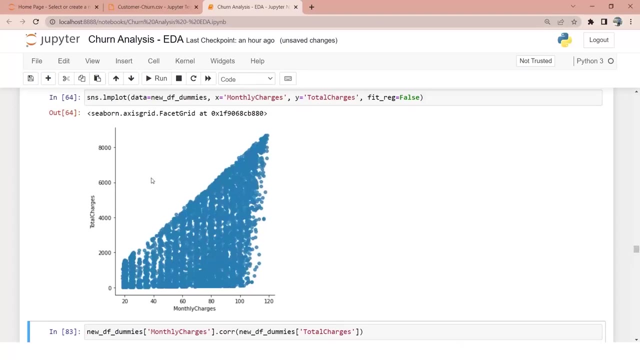 positively correlated. but i just want to plot it. so i'm using an lm plot and i'm passing my dummies data. in the x-axis i am passing monthly charges and y-axis and passing the total charges. i'll run this and you can see that somehow for some data points it is difficult to interpret. 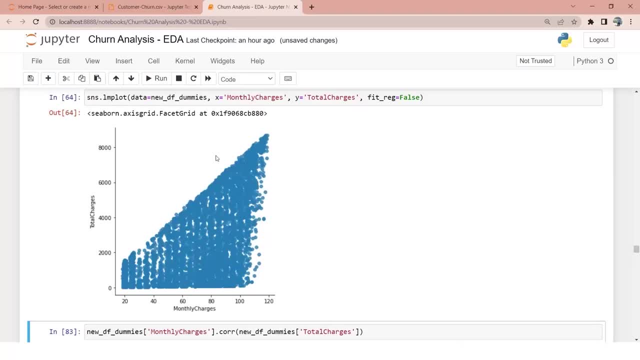 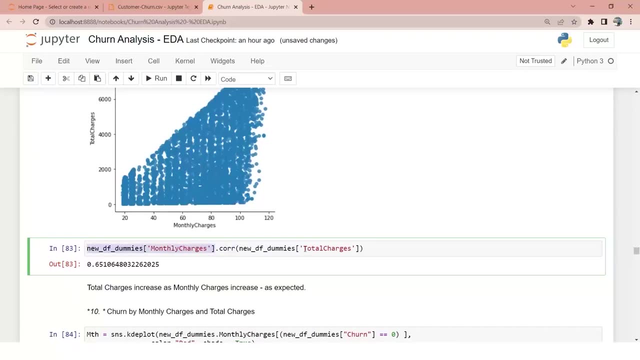 but most of the data points. i can see an increasing trend right. if you want to calculate the correlation you can see between monthly charges and the total charges. i am calling the correlation function and the correlation is 0.65 and we all know that correlation value ranges from minus one to one, one being the highest, minus one being the lowest. if the number 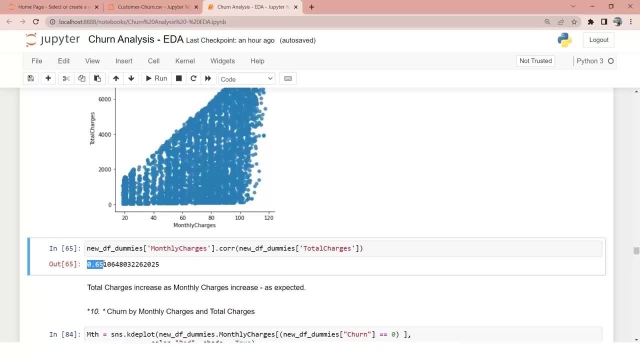 is very close to one, that means they are positively correlated. so in this case the variable is positively correlated. that means monthly charges and total charges are correlated positively, right? so my insight here will be: total charges increase as monthly charges increase and vice versa, as expected. so again, you can go back to your insights. if you want, you can note it down. 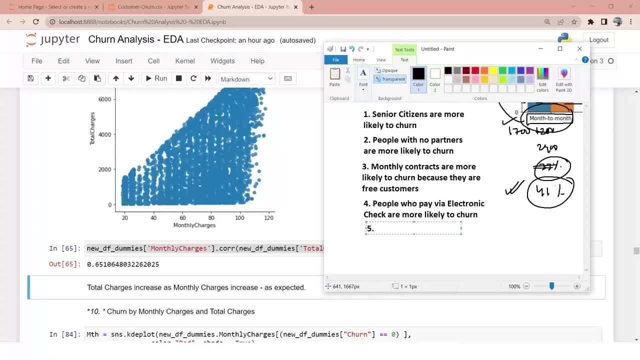 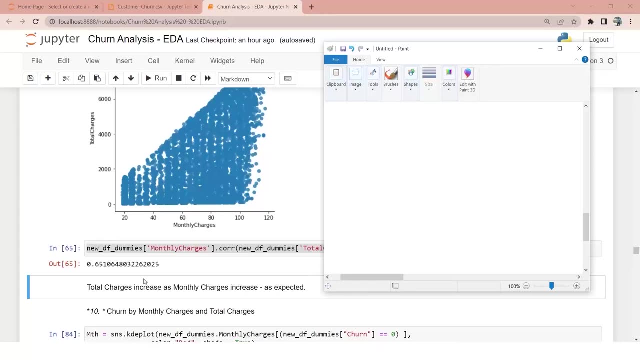 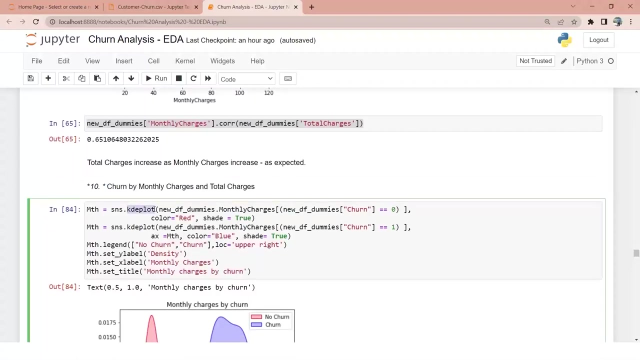 so let's try to note it down: monthly charges and total charges are positively correlated. okay, going back to the code. so here i am performing some activities to plot some kernel density plots churn by monthly charges and total charges. so here i'm calling my monthly charges on my active users and the same thing on my inactive users or exited users or churned users. 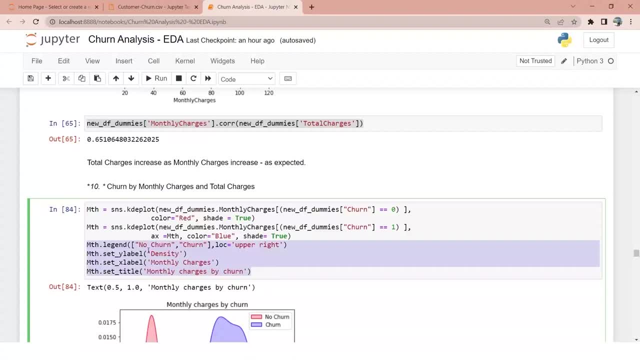 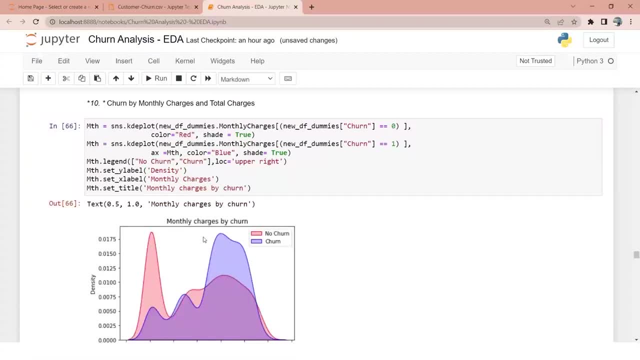 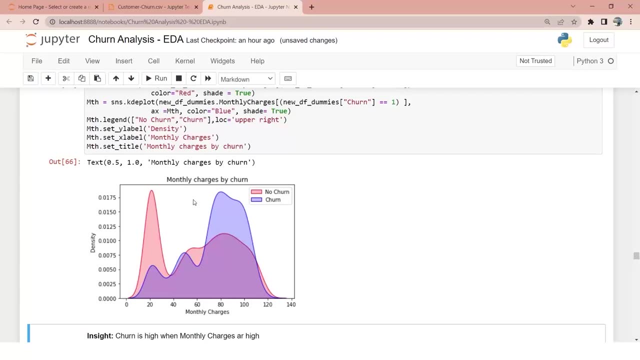 i'm only plotting my monthly charges. if i run this. that's how my graph looks like now. if you look at it closely, you can see the inside that i am getting from. here is the churn, which is the blue graph, is very high when the monthly charges is high and the churn is. 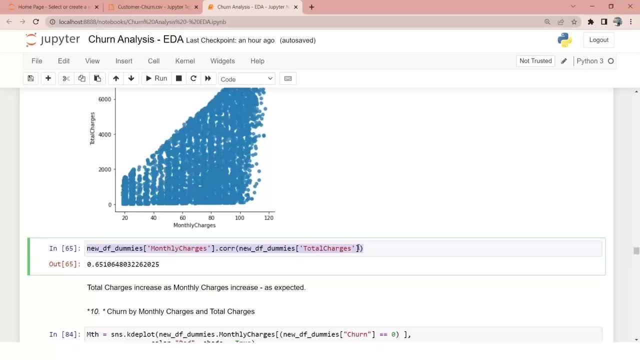 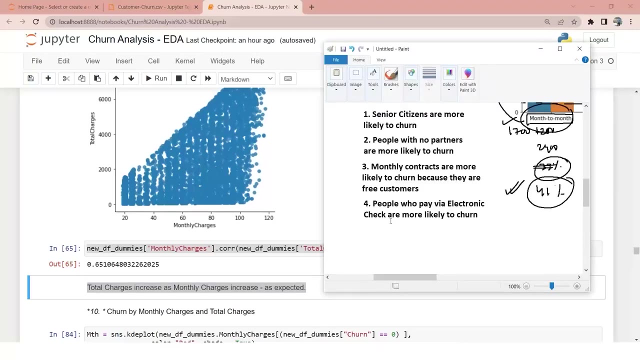 is positive. so in this case the variable is positive. so in this case the variable is positive. so in this case the variable is positively correlated. that means monthly charges and total charges are correlated positively, right? so my insight here will be: total charges increase as monthly charges increase and vice versa, as expected. so again, you can go back to your insights if you. 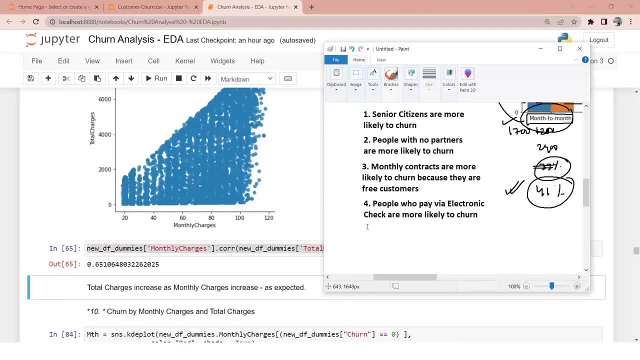 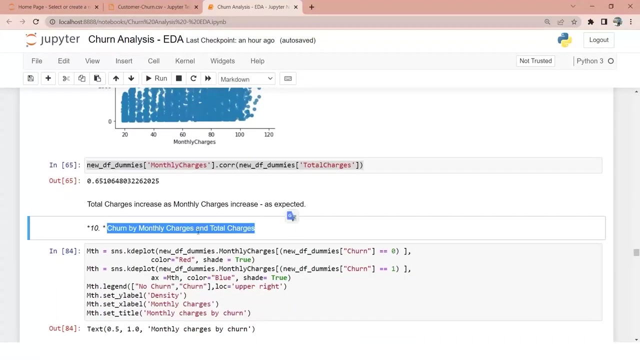 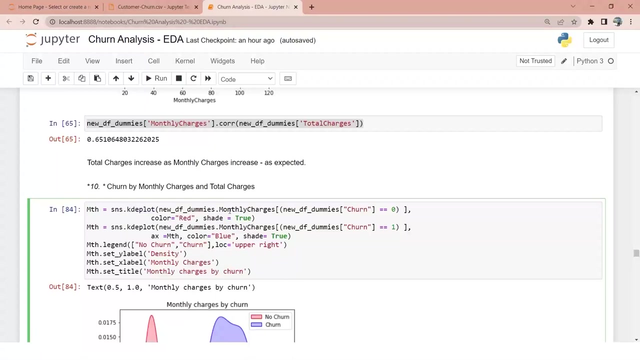 want you can note it down. so let's try to note it down. monthly charges and total charges are positively correlated. okay, going back to the code. so here I am performing some activities to plot some kernel density plots churned by monthly charges and total charges. so here I'm calling. 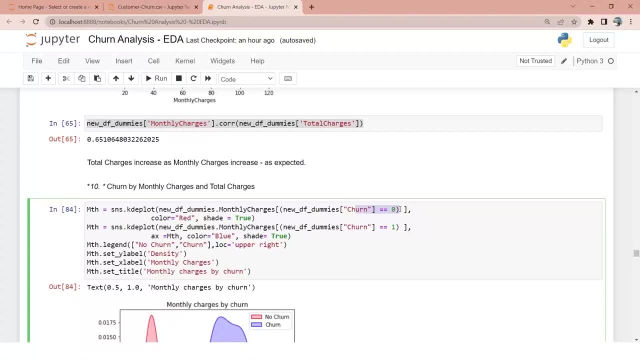 my monthly charges on my active users and the same thing on my inactive users or exited users or churned users. and then I am. all these are very simple. I'm just passing the Legends. Y label, X label and title are very simple. this is the main piece of code. so here I'm calling cbon dot. 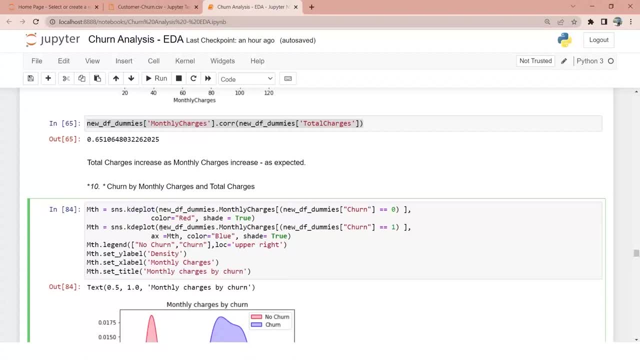 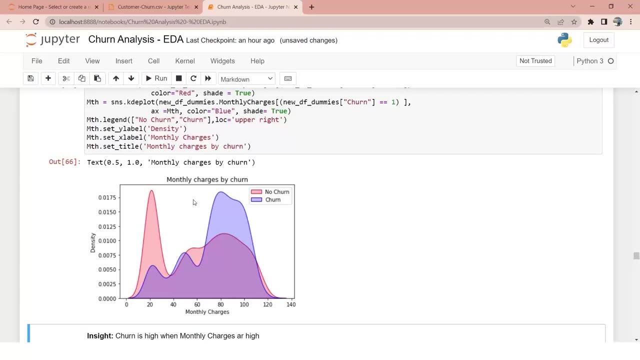 KD plot, which is a kernel density estimation plot, and I am only plotting my monthly charges if I run this. that's how my graph looks like now. if you look at it closely, you can see the inside that I am getting from. here is the churn, which is the blue graph. 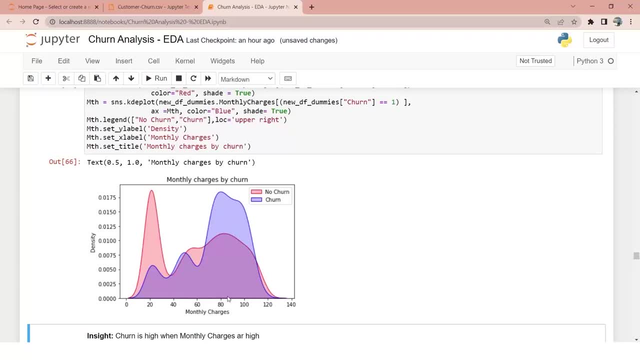 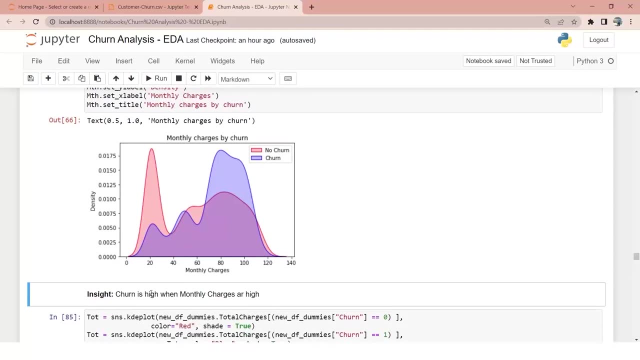 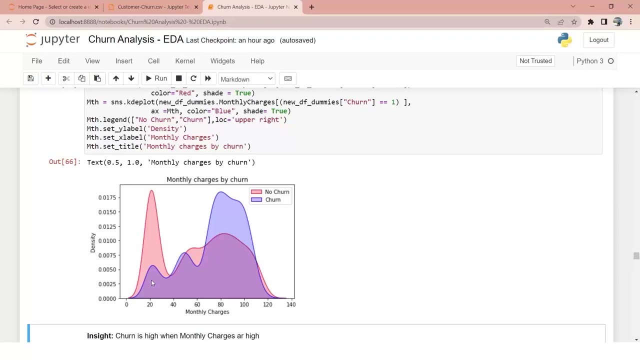 is very high when the monthly charges is high and the churn is very high when the monthly charges are low, which is quite expected, because if the monthly charges are high, maybe because of the monetary aspects, the customers are churning right. so this is an insight. so again, let's go back to our insights part and try to write it down. 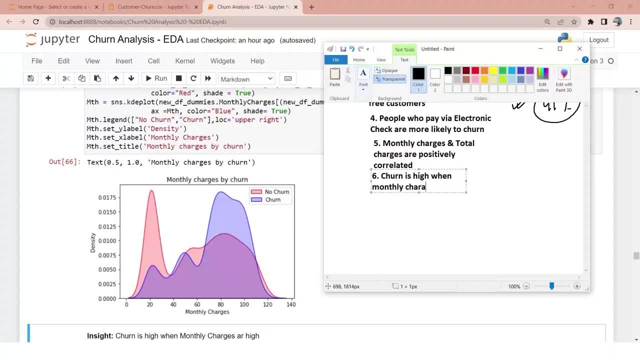 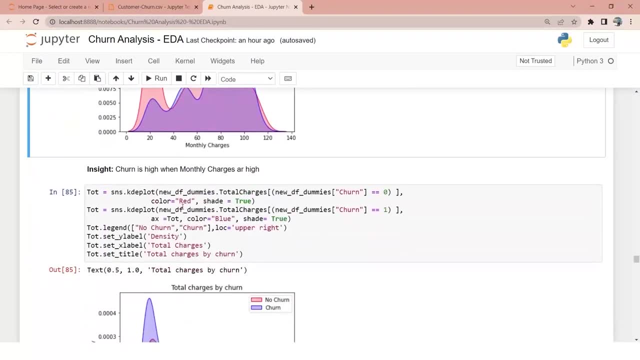 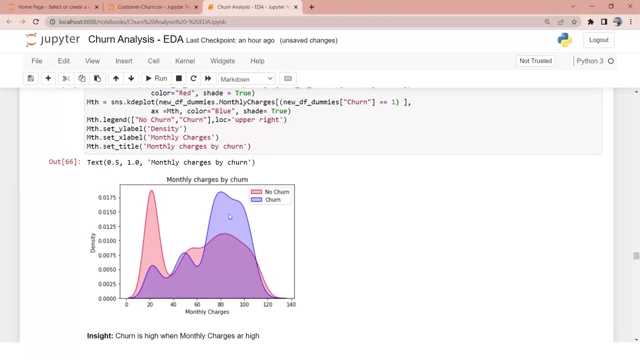 churn is high when monthly charges are high. right. similarly, I will do it for the total charges, so as monthly charges and total charges are positively correlated. I should also be seeing a similar kind of pattern: more total charges, more churn, less total charges, less churn. let's see. 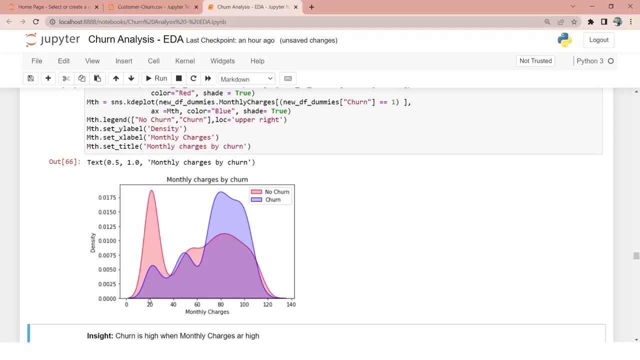 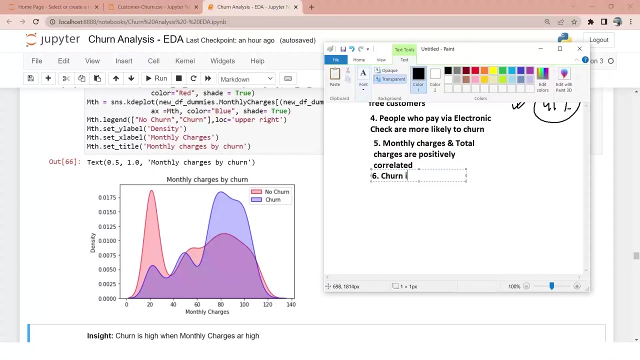 very high when the monthly charges are low, which is quite expected, because if the monthly charges are high, maybe because of the monetary aspects, the customers are churning right. so this is an insight. so again, let's go back to our insights part and try to write it down: churn is high when monthly 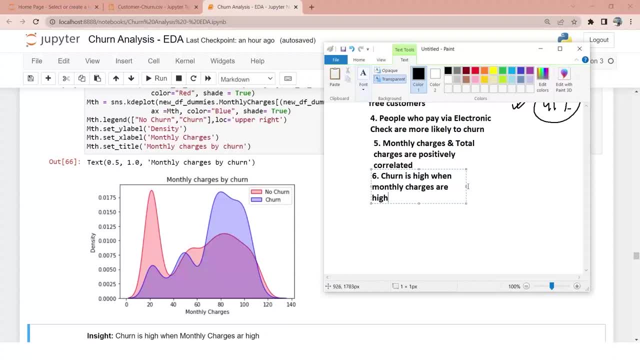 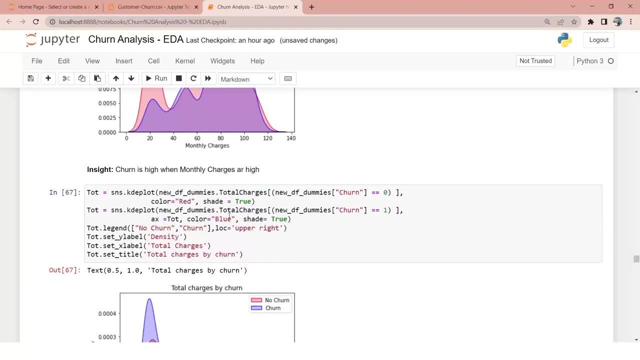 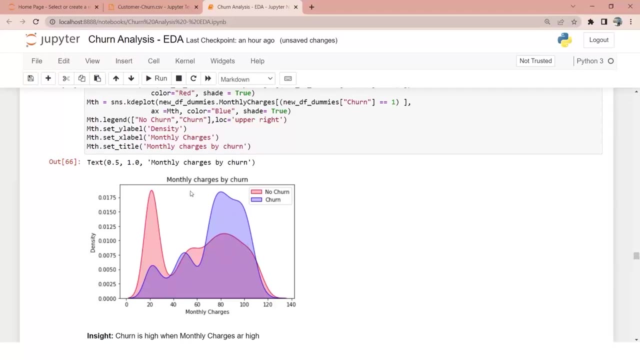 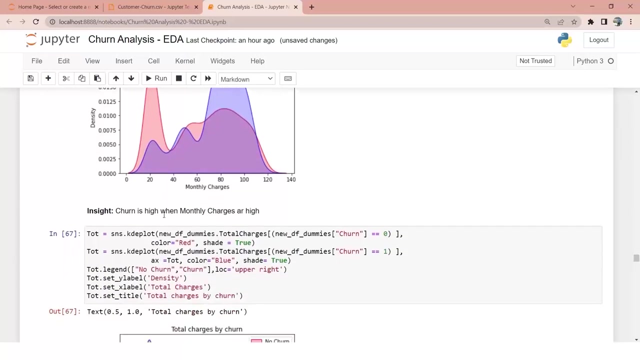 charges are high, right. similarly, i will do it for the total charges, so as monthly charges and total charges are positively correlated. i should also be seeing a similar kind of pattern: more total charges, more churn, less total charges, less churn. let's see. astonishingly, you can see that the churn is high. 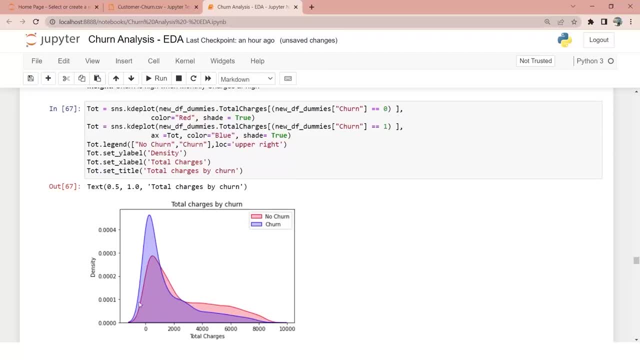 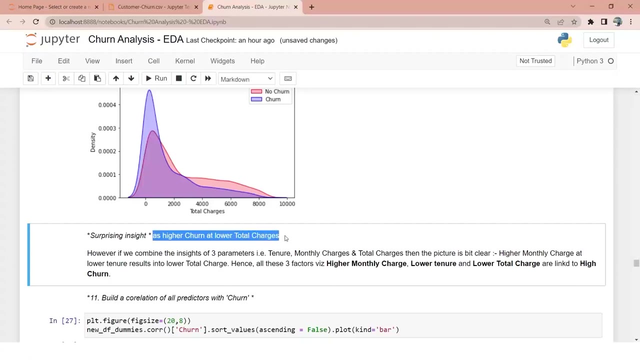 at less total charges. let's see at less total charges, even though total charges and monthly charges are almost highly correlated, but this is a very surprising insight. so the insight here is surprising as higher churner at lower total charges. however, if we combine the insights of three parameters- tenure, monthly charges, 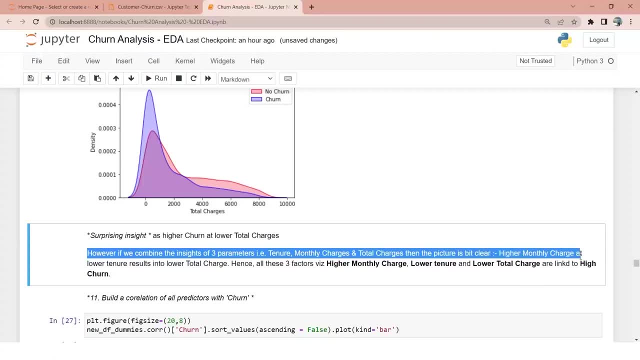 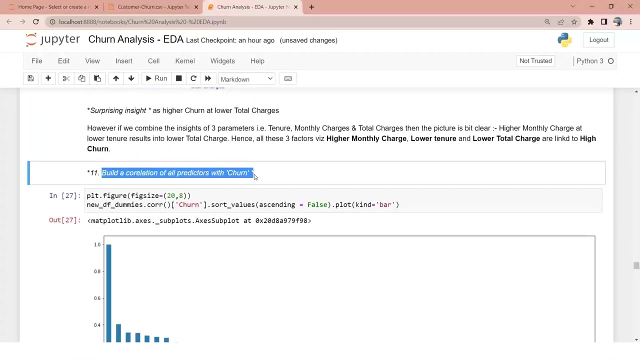 and total charges. then the picture is bit clear: higher monthly charge at lower tenure results into higher monthly charge. hence, all these factors, which is higher monthly charge, lower tenure and lower monthly total charge- are linked to high churn- surprising insight. right, the next step is. the next step is nothing, but i am building a correlation matrix or correlation graph. 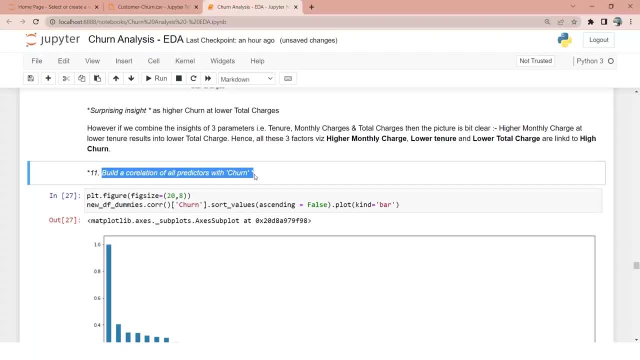 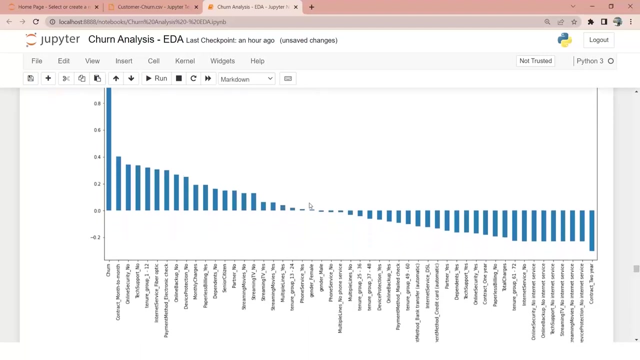 of all the x variables, or all the predictors, with respect to my churn column. calling my data frame dot correlation function with respect to churn, i am sorting the values with ascending equals to false, which means descending is true. dot plot kind equals to bar, so i am plotting a bar chart. if i run this, the graph looks like this. now, what do i infer? 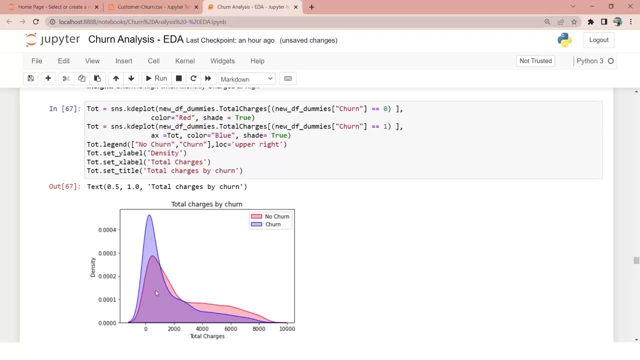 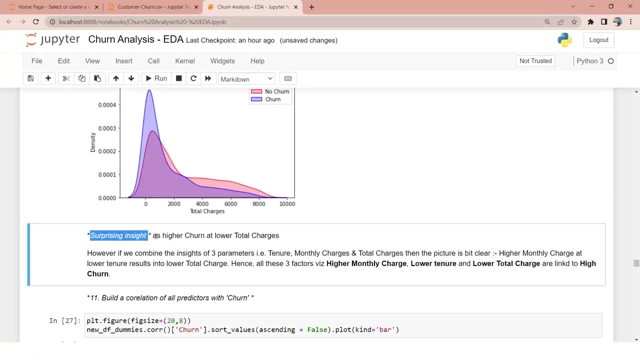 astonishingly, you can see that the churn is high at less total charges, even though total charges and monthly charges are almost highly correlated. but this is a very surprising insight. so the insight here is surprising as higher churner at lower total charges. or if we combine the insights of three parameters- tenure, monthly charges and total charges- then the 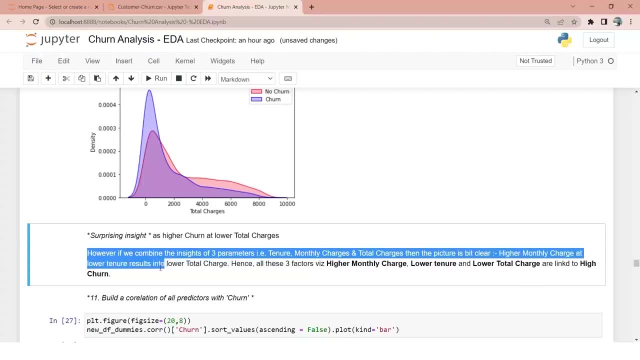 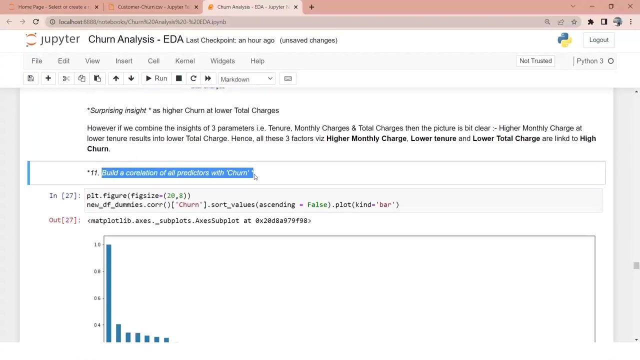 picture is bit clear: higher monthly charge at lower tenure results into lower total charge. hence, all these factors, which is higher monthly charge, lower tenure and lower monthly total charge- are linked to high churn. surprising insight, right, the next step is. the next step is nothing, but I am building a correlation matrix or correlation graph of 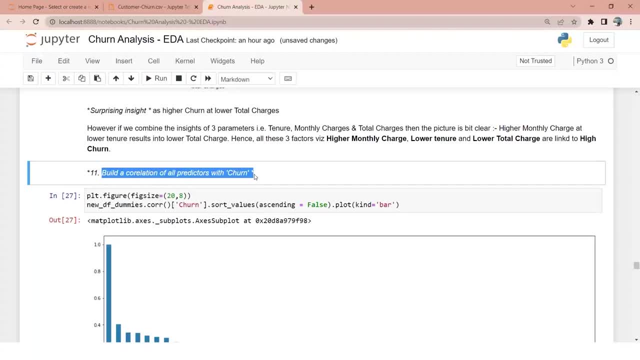 all the x variables or all the predictors with respect to my term column. so I'm calling my data frame dot correlation function. with respect to churn, I am sorting the values with ascending equals to false, which means descending is true. dot plot kind equals to bar, so I'm plotting a bar chat. 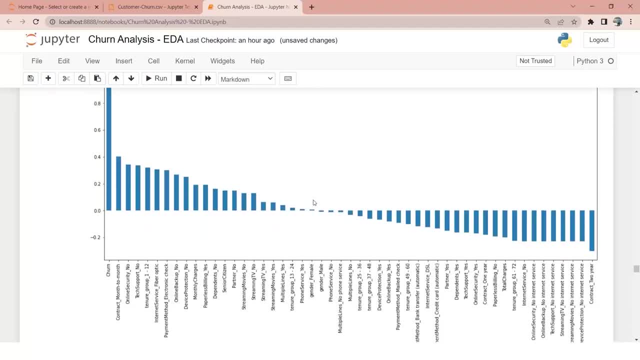 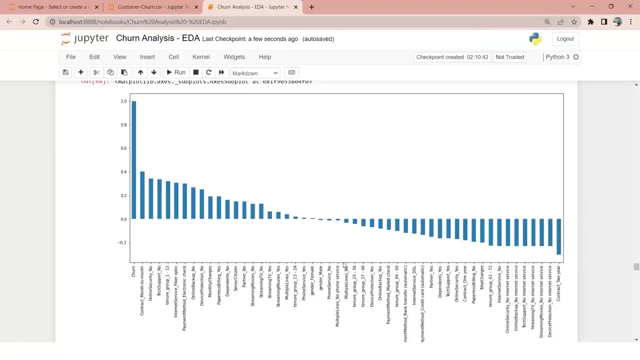 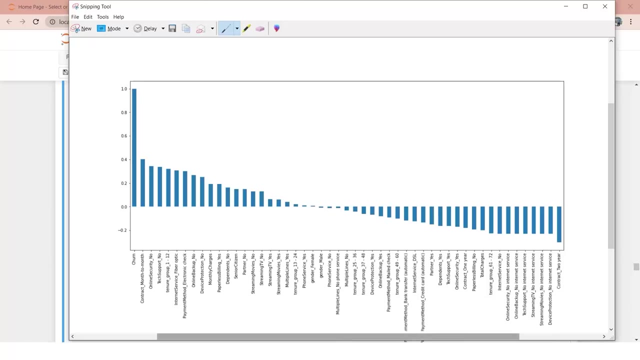 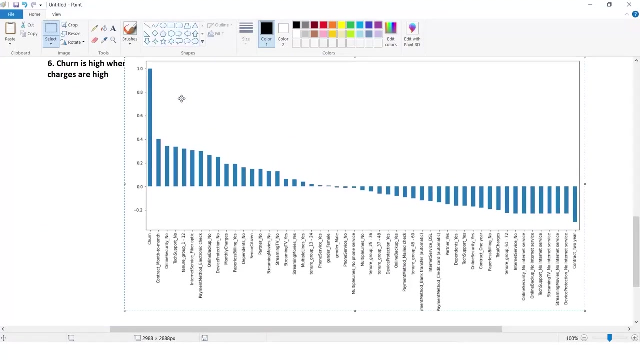 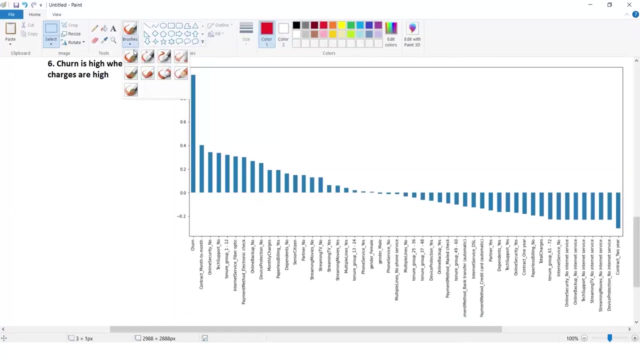 run this. the graph looks like this. now, what do i infer from this graph? so let me just zoom out a little bit so that i can, i can snip out the graph. i'll take it to my paintbrush for a. okay, now you can see the first. the first thing is ignorable. the first bar is ignorable. 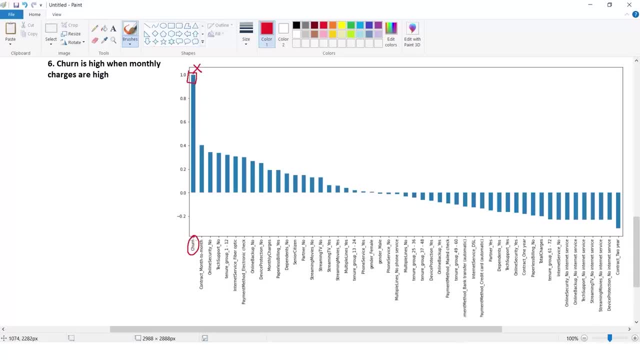 why? because it is churn and we are building this function with respect to churn, so with respect to churn, the correlation will anyways be one right, so ignore this graph. talking about this graph, contract month to month, so this graph basically tells me monthly contractors are more likely to churn. we have already got this insight here. number three: online security. no people. 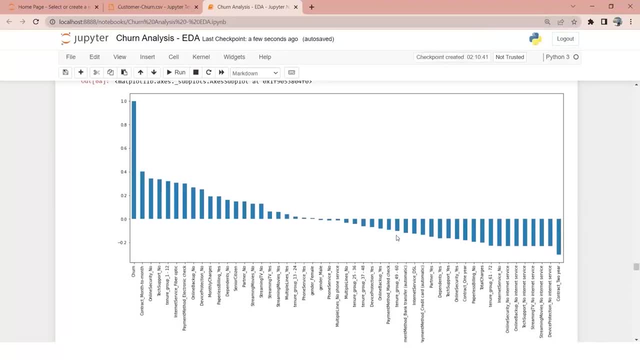 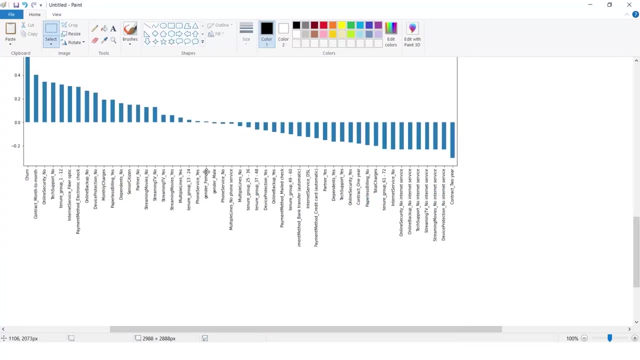 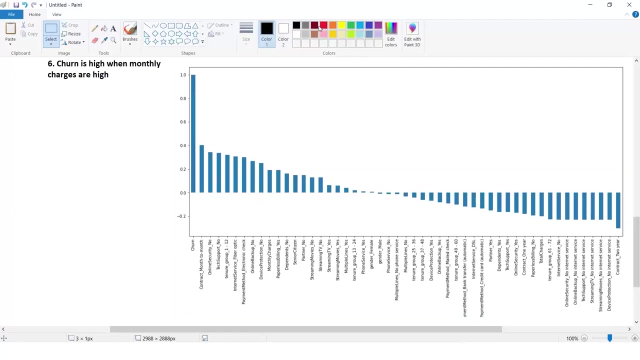 from this graph. so let me just zoom out a little bit so that i can, i can snip out the graph. i will take it to my paintbrush for a. okay, now you can see the first. the first thing is ignorable. the first bar is ignorable. why? 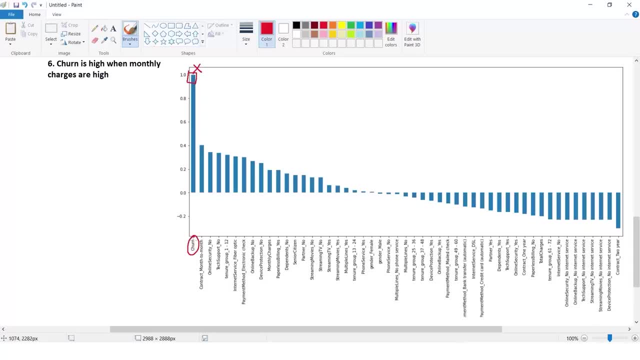 because it is churn and we are building this function with respect to churn, so with respect to churn, the correlation will anyways be one right? so ignore this graph. talking about this graph, contract month to month. so this graph basically tells me monthly contractors are more likely to churn. we have already got this. 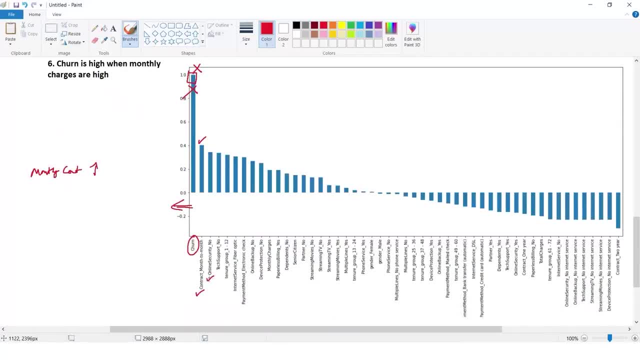 insight here. number three: online security. no, people who don't have online security are high churners. new insight: so you can write down here: tech support- no. tech support- no are high churners. tenure group of 1 to 12, so people who are in the company between 1 to 12 months. that means all the new customers. 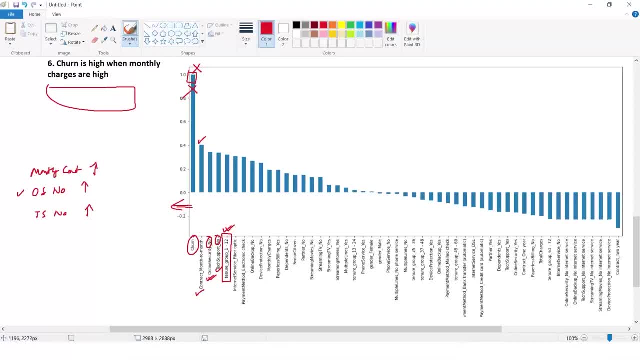 you are more likely to churn, internet service, fiber optics more likely to churn, payment method electronic check more likely to churn, and so on. so we set a threshold by ourselves. let's say I set my threshold as 0.2, so probably anything that goes beyond 0.2, I will choose these as my important predictors. similarly, I 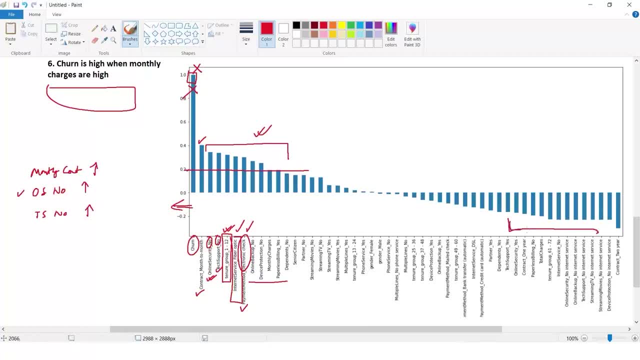 will also choose a set of predictors who are: are also negative correlated. they will also help us in the model right contract, two-year good insight. they are low churners. streaming movies, no internet service- low churners. all these are low churners. you can see tenure group 61 to. 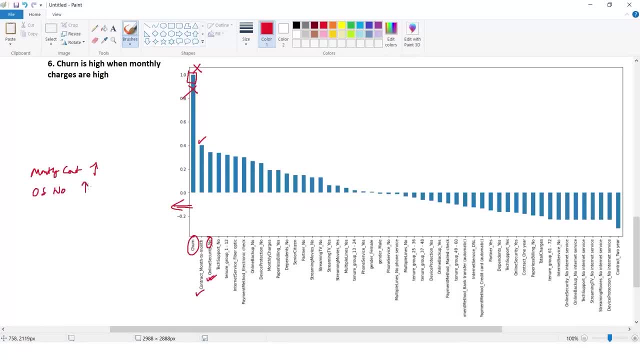 who don't have online security are high churners. new insight: so you can write down here: tech support no. tech support no are high churners. tenure group of one to twelve. so people who are in the company between one to twelve months- that means all the new customers- are more likely to churn internet service. fiber optics. 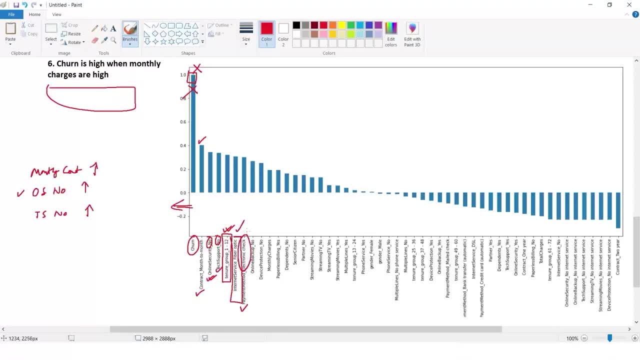 more likely to churn, payment method electronic check more likely to churn, and so on. so we set a threshold by ourselves. let's say i set my threshold by myself. let's say i set my threshold as .2. so probably anything that goes beyond point two, i will choose these. 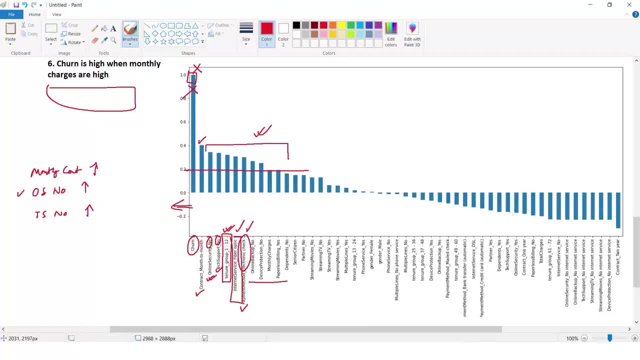 as my important predictors. similarly, i will also choose a set of predictors who are also negative. correlated. they will also help us in the model right contract: two year- good insight. they are low churners. streaming movies, no internet service- low churners. all these are low churners. you can see tenure groups level below ten year and of happiness can. be recognized as a smallobit as well. we set a number by three as fine lines, so that's a good thing. alright, so we set a number by two. now we draw a particular value of chrr. that's also not an issue, but we will take two. so hkm, that's an important factor as well. just once you guys understand. 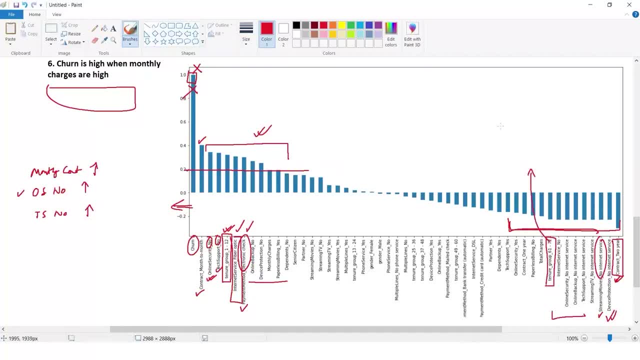 this is point two. we make an argument between the five-year and if there is no contract, excellent, it becomes very clear end so that you are nowhere to fit the job. so if the resources group 61 to 72, which means people who are in the organization for a longer period of time, 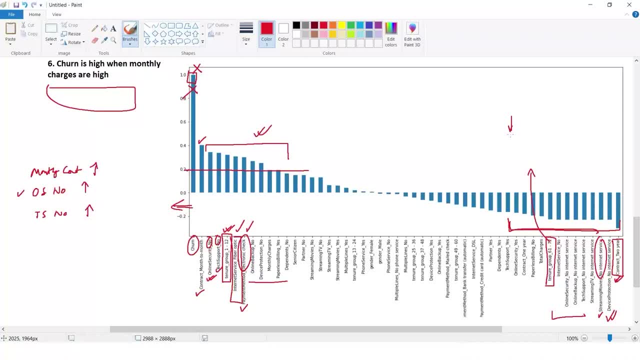 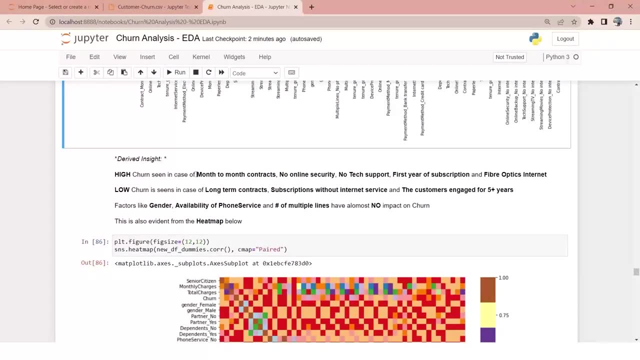 they are low churners. so these are all the insights that i'm getting right. jumping back to the code: high churn seen in the case of month to month contracts. and these are all the derived, derived insights. high churn seen in case of month to month contract, no online security, no tech. 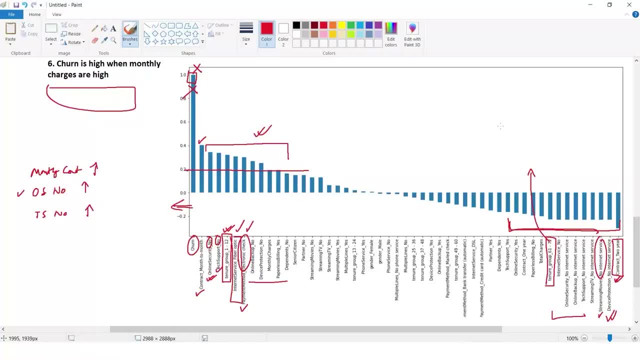 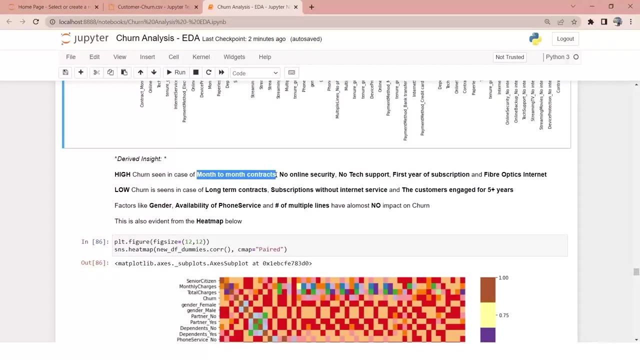 72, which means people who are in the organization for a longer period of time. they are low churners. so these are all the insights that I'm getting right, jumping back to the code: high churn seen in the case of month to month contracts. and these are all the derived, derived insights. high churn seen in case. 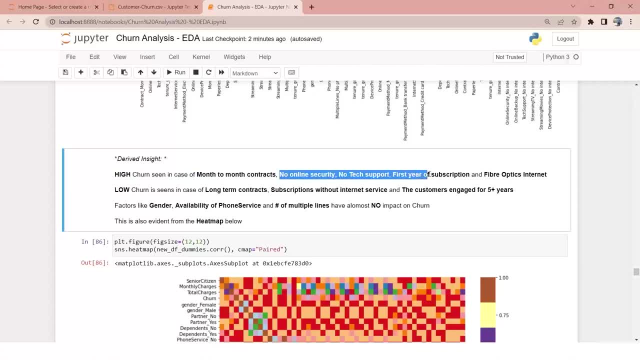 of month to month contract, no online security, no tech support, first year of subscription and fiber optics internet. low churn is seen in case of long-term contracts, subscriptions without internet service and customers engaged for five plus years. factors like gender, availability of this and number of multiple lines have almost 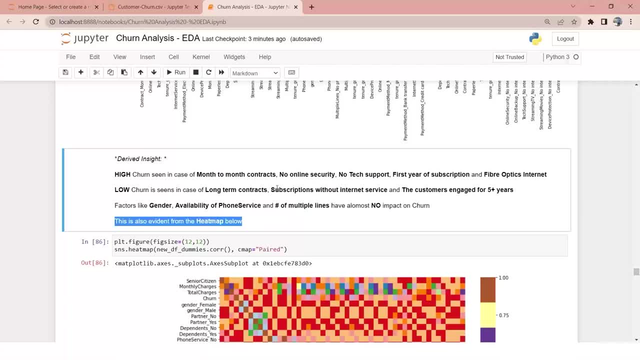 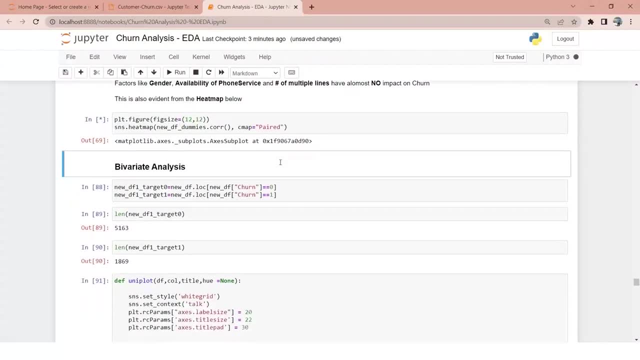 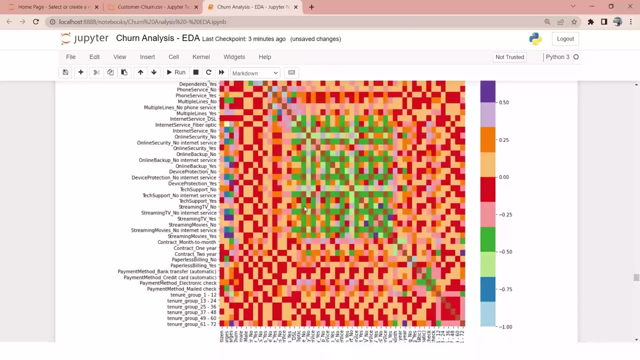 no impact on churn. this is also evident from the heat map below. so I am running the correlation function with respect to the heat map, with respect to the entire data frame. heat map basically tells you the correlation between each and every feature, but the previous graph is telling you the correlation between your target variable. 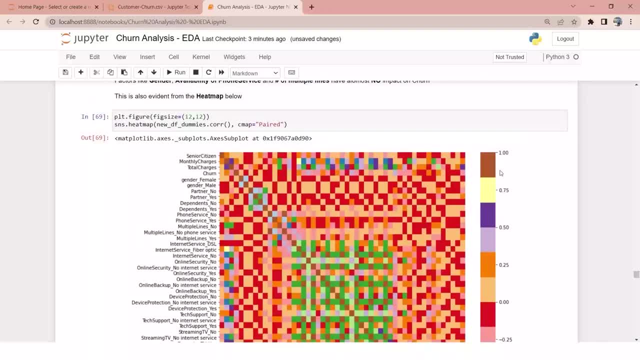 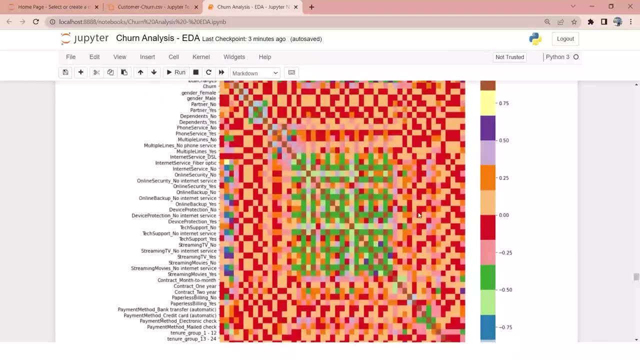 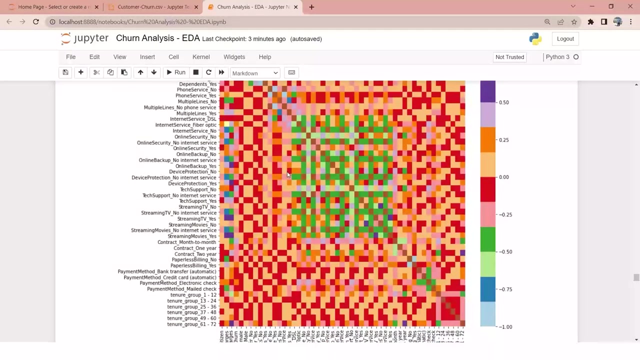 so both are different. now, in this case, we'll try to spot a darker shade of this one. let's say this one: senior citizen and payment method, bank transfer automatic. they are kind of having high positive correlation. so all this kind of graphs will give you an insight about the different types of relationships. right, but more likely we 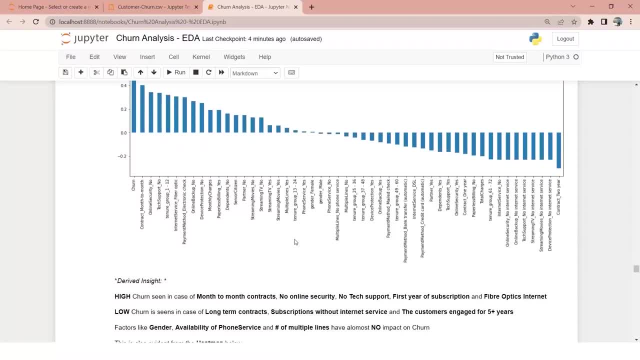 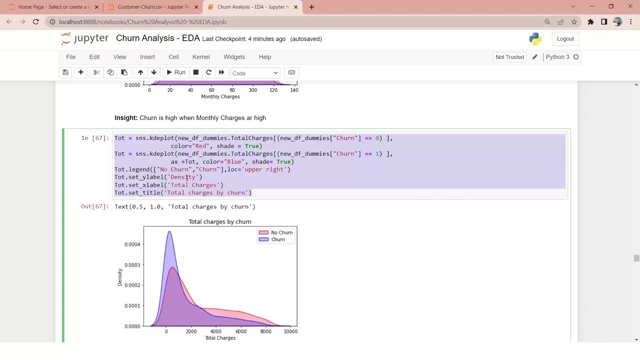 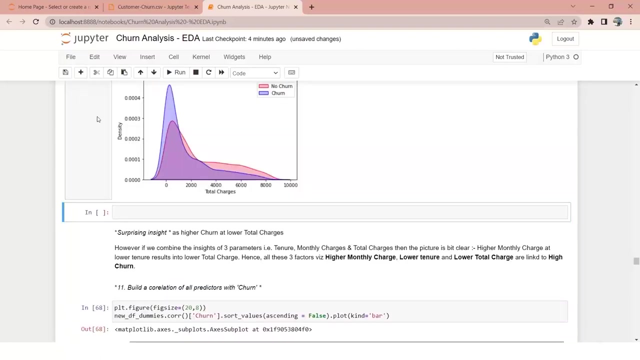 more insights from this particular graph apart from this, the way we did for our total charges and monthly charges, in case in your data set you have more numerical attributes or more numerical columns like salary and other things, you can also do the same technique. let's say: I want to do it for churn. sorry, I want. 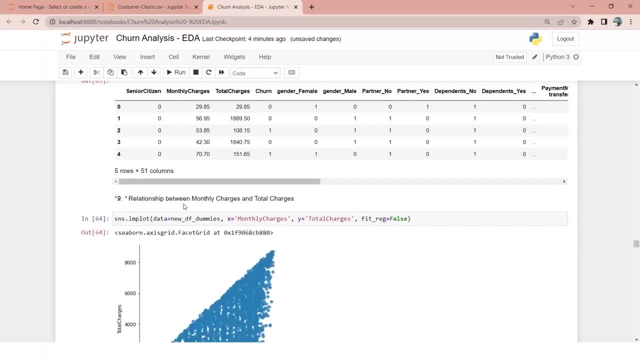 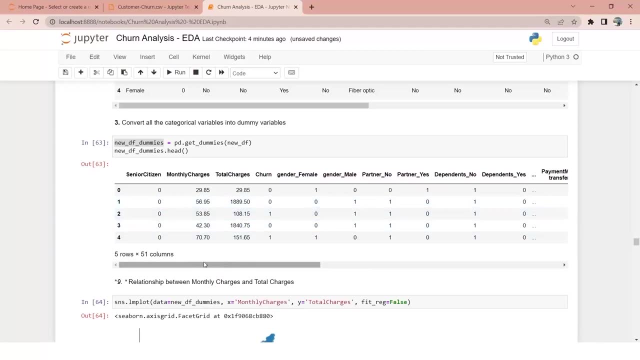 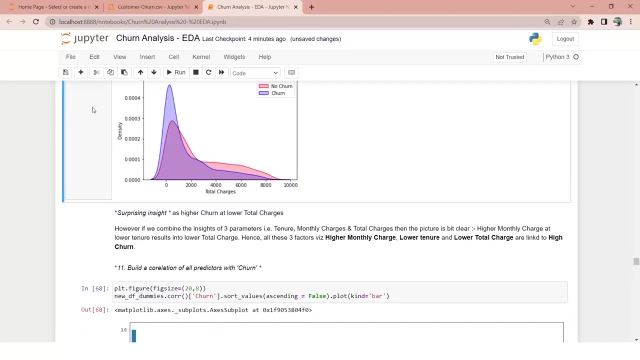 to do it for tenure, but however, I don't have tenure. I have already converted my tenure into tenure groups, so I don't have that column. so I might not be able to do this for tenure, but just in case you want to do it for tenure, I think we 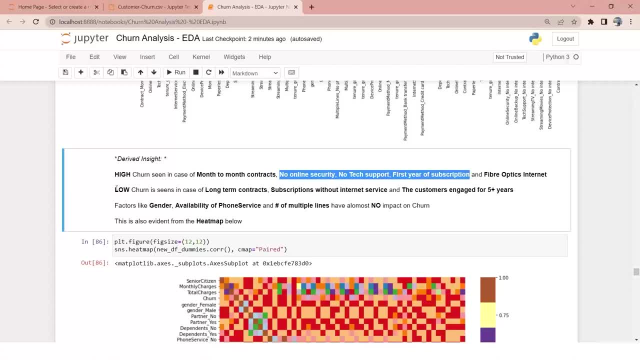 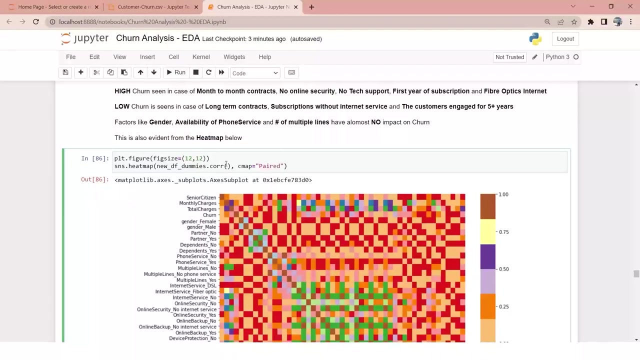 support first year of subscription and fiber optics internet. low churn is seen in case of long-term contracts, subscriptions without internet service and customers engaged for five plus years. factors like gender, availability of this and number of multiple lines have almost no impact on churn. this is also evident from the heat map below, so i am running the correlation function. 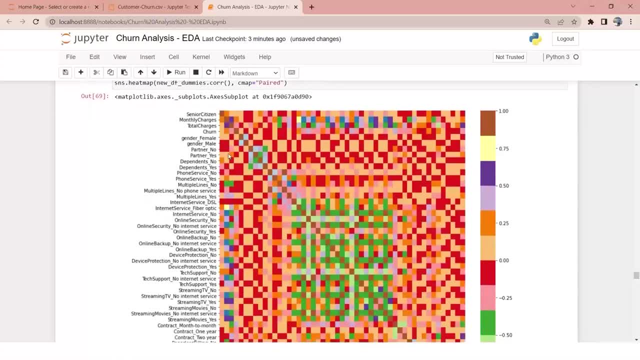 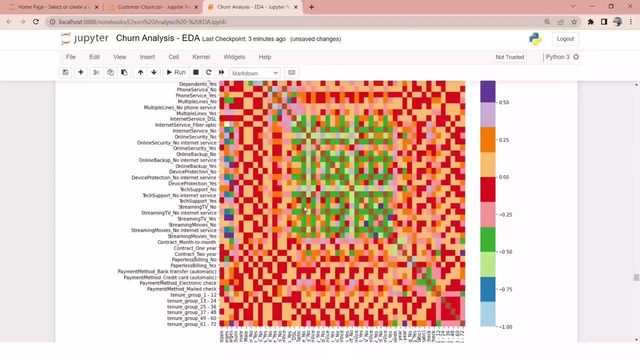 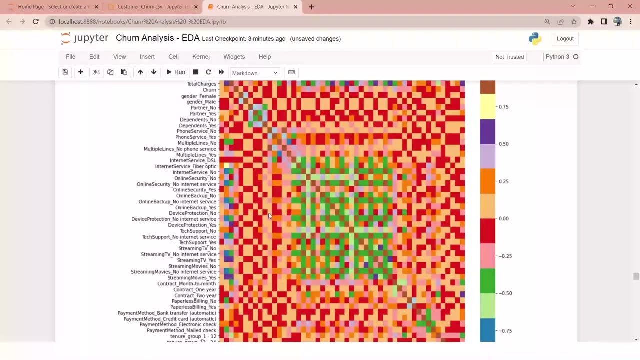 with respect to the heat map, with respect to the entire data frame. heat map basically tells you the correlation between each and every feature, but the previous graph is telling you the correlation between your target variable, so both are different. now, in this case, we'll try to spot a darker shade of this one. 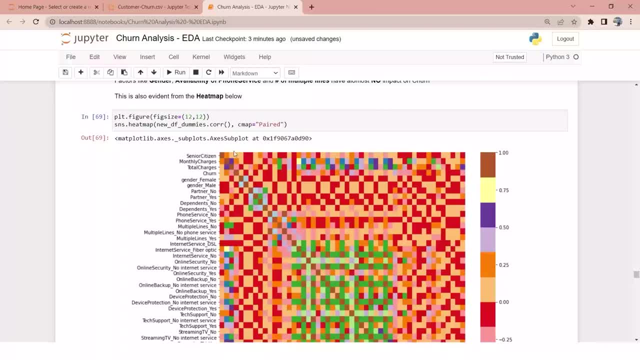 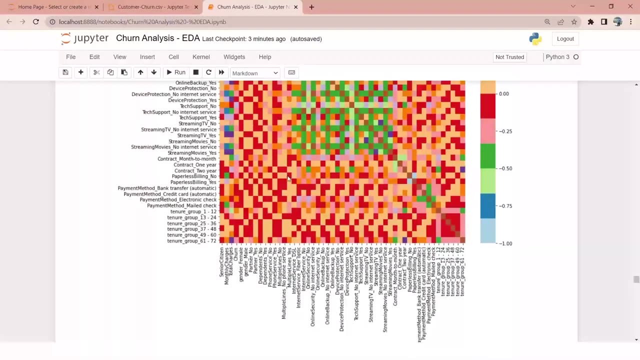 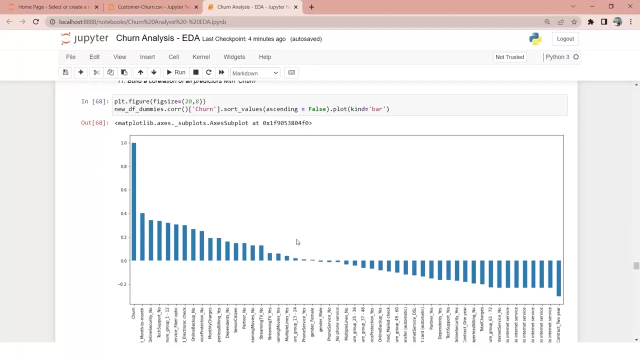 let's say this one, senior citizen- and payment method- bank transfer, automatic. they are kind of having high positive correlation. so all these kind of graphs will give you an insight about the different types of relationships. right, but more likely we got more insights from this particular graph apart from this, the way we did for our total, 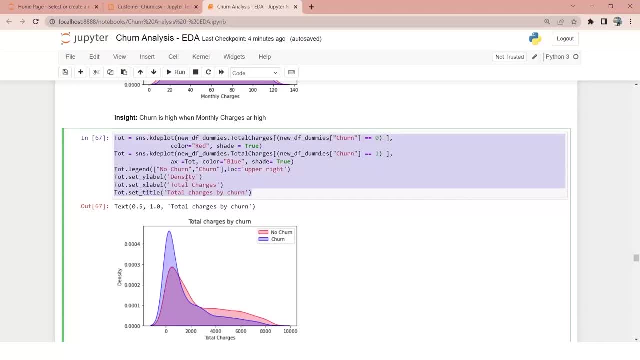 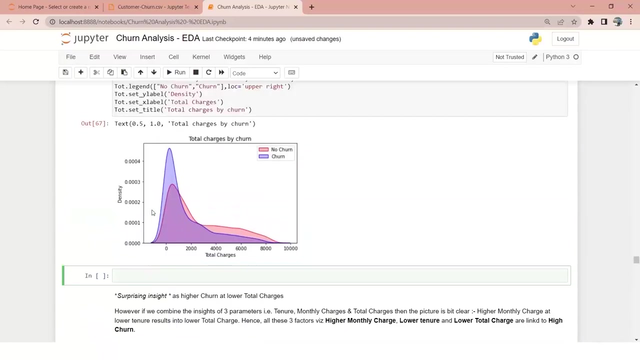 charges and monthly charges. in case in your data set you have more numerical attributes or more numerical columns, like salary and other things, you can also do the same technique. let's say i want to do it for churn. sorry, i want to do it for tenure, but however i don't have tenure, i have already converted my. 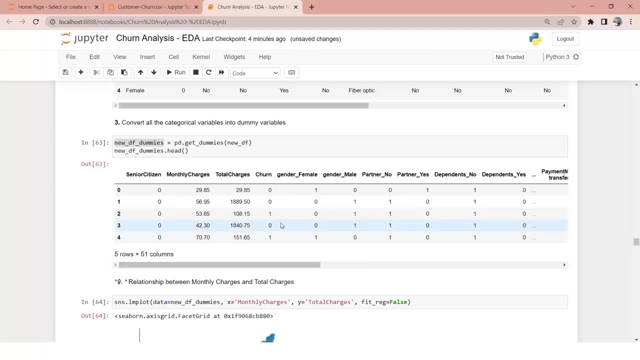 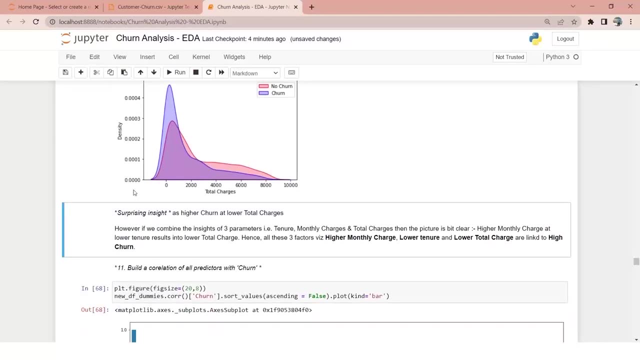 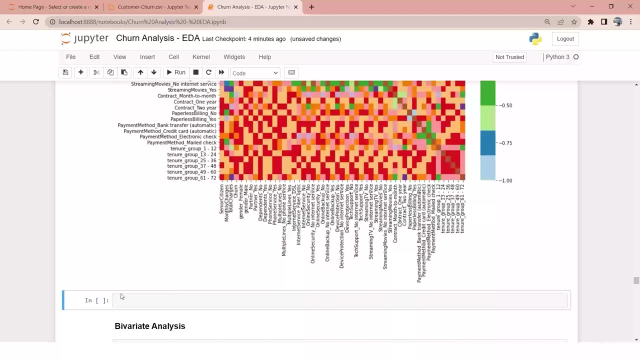 tenure into tenure groups. so i don't have that column, so i might not be able to do this for tenure, but just in case you want to do it for tenure, i think we already have- let me just delete it. we already have a backup data frame, right? 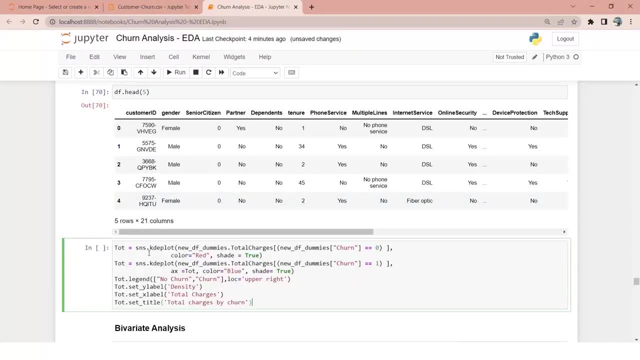 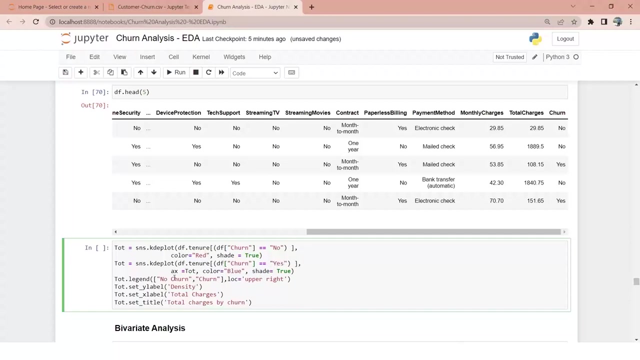 in that we have tenure, so we can just quickly go through that and plot this. let's say df dot, tenure df with respect to churn- here we have no, so i will just change it to no df dot tenure df of churn. yes, and everything remains the same. this is not total charges, is going to be tenure. 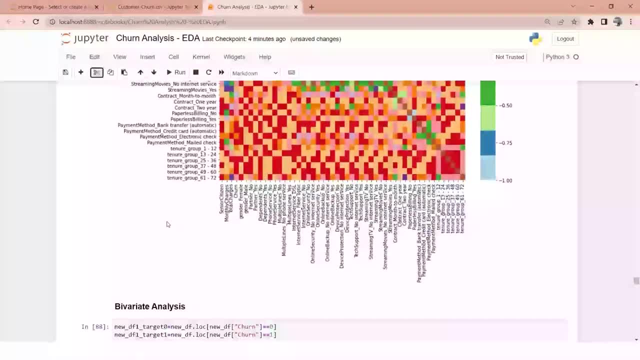 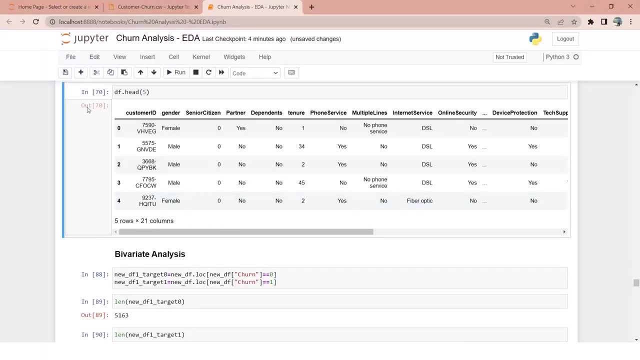 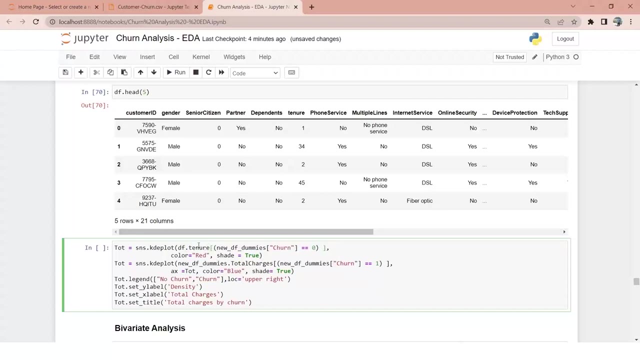 already have. let me just delete it. we already have a backup data frame, right in that we have tenure, so we can just quickly go through the data frame and then we can go through the data frame, and then we can go through that and plot this. let's say df, dot, tenure, df with respect to churn. 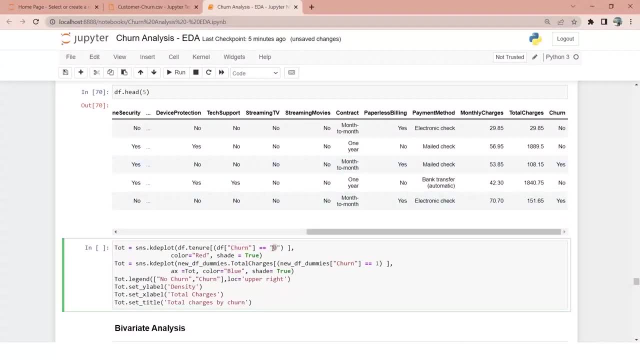 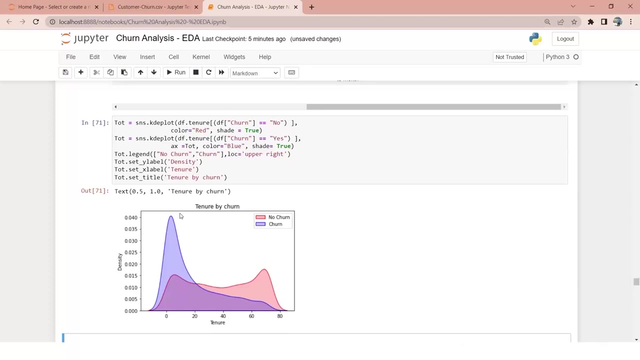 here we have no, so I will just change it to no df dot tenure, df of churn, yes and everything remains the same. this is not total charges is going to be tenure and tenure by churn. let's run this and you can see that less, less tenure. people who are new are high. 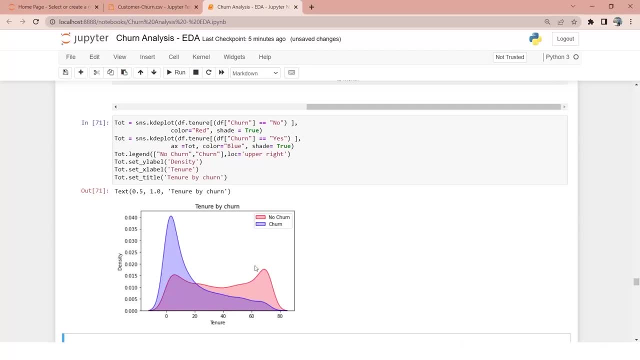 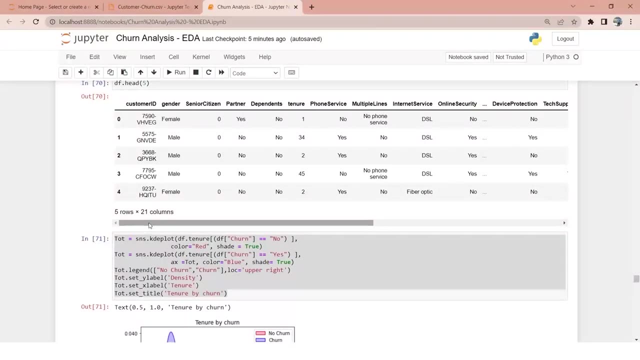 churners and people who are having more tenure are low churners, very good inside right. similarly, if you have any other numerical features, let's say tenure is gone, I think other than that I don't have any other numerical features, but in your case if you have age, salary and other things, you can simply copy paste this code to understand the. 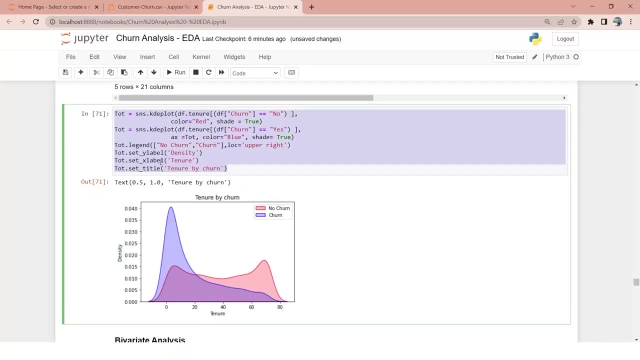 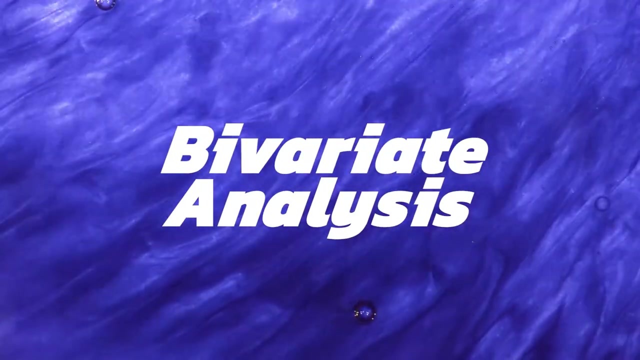 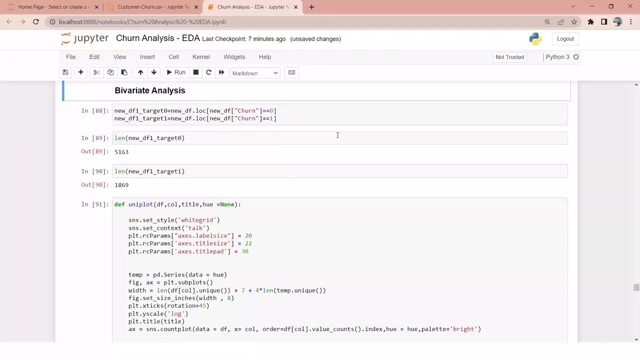 kernel density estimation plot and you will be able to infer something. so that's all about numerical analysis. in the next video we shall be focusing on the bivariate analysis. our next type of analysis is going to be bivariate analysis. however, for this particular use case, with univariate and with the numerical analysis that we have done, almost we have got a lot of. 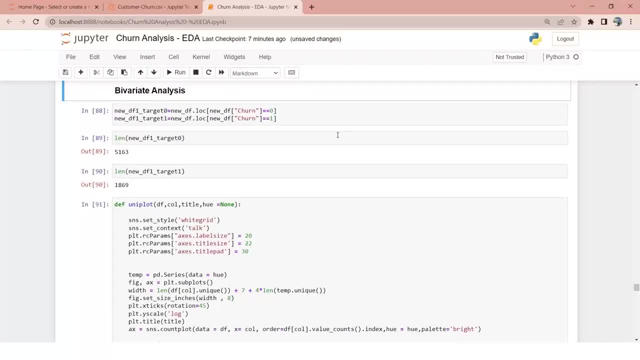 insights. but bivariate is also going to give us more insights. so i have divided the data into target zero and target zero, and i have divided the data into target zero and target zero and get one first data frame is about the non churners and the second one is about the churners. i'll do 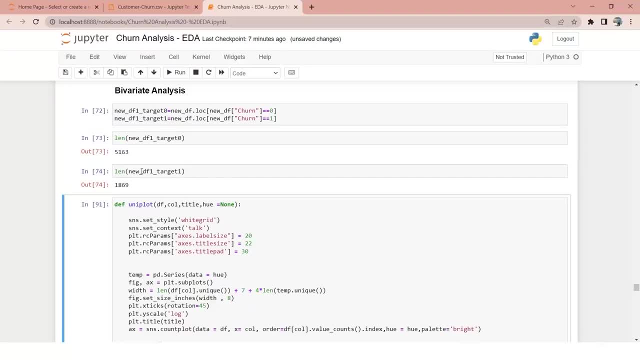 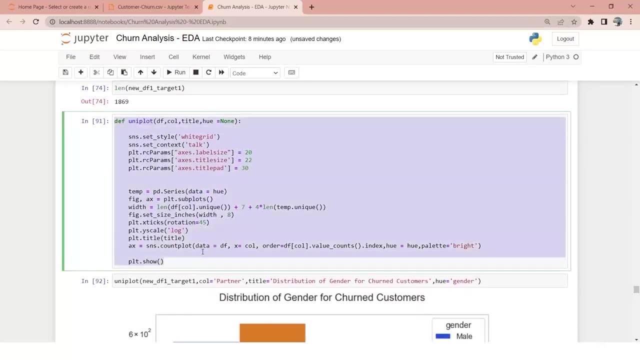 this: the non churners are 5000 and the churners are around 1800- 1869. i have created a function here, uni plot, where i'm taking input some data- column and title and hue, and i'm writing down some pieces of code to plot something. now this again is a reusable code, in case you are doing. 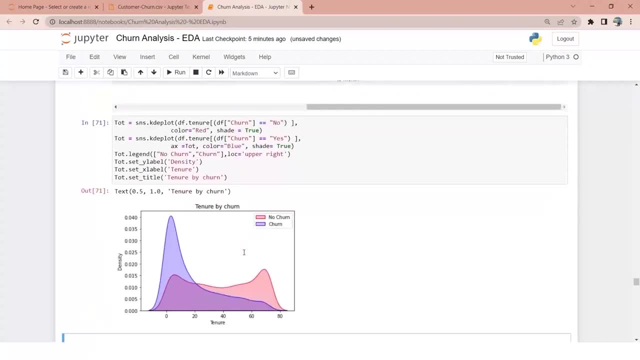 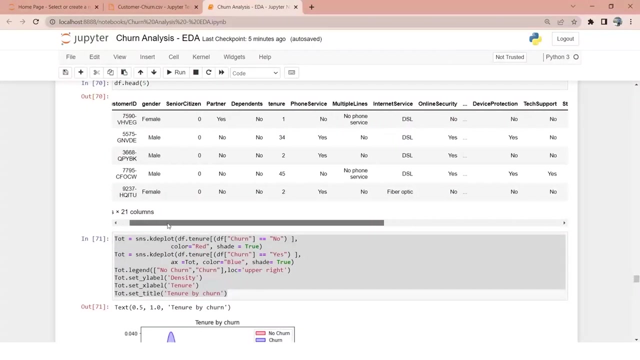 and tenure by churn. let's run this and you can see that less, less tenure, people who are new are high churners and people who are having more tenure are low churners. very good insight, right? similarly, if you have any other features, let's say, tenure is gone. i think, other than that i don't have any other numerical. 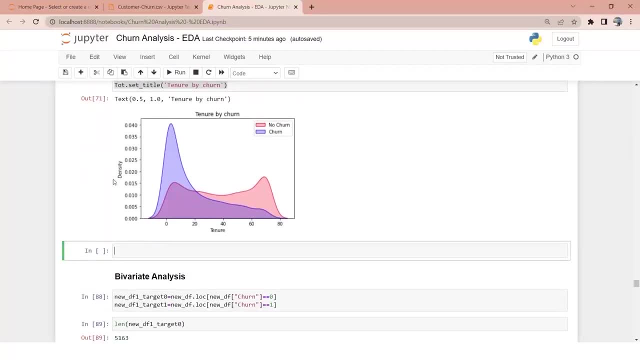 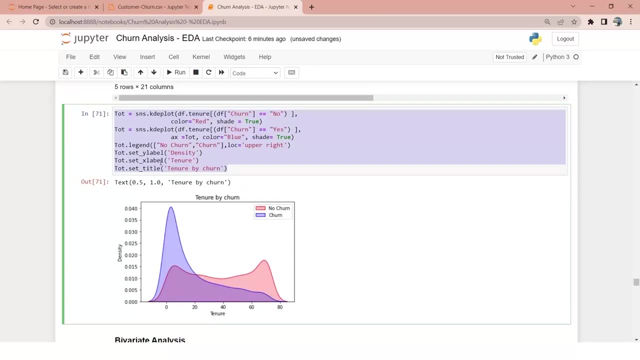 features. but in your case, if you have a salary and other things, you can simply copy paste this code to understand the kernel density estimation plot and you will be able to infer something. so that's all about numerical analysis. in the next video we shall be focusing on the bivariate. 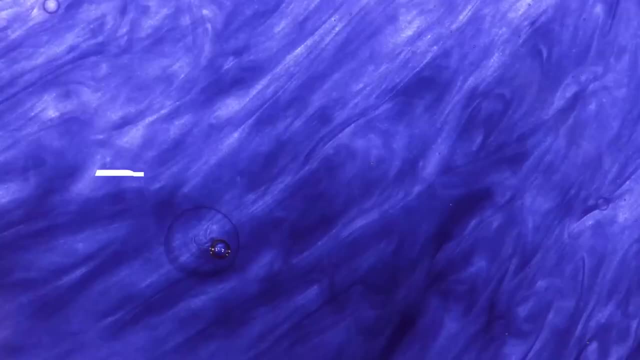 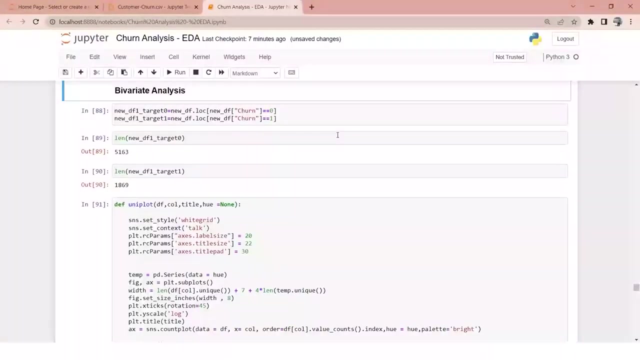 analysis. our next type of analysis is going to be bivariate analysis. however, for this particular use case, with univariate and with the numerical analysis that we have done, almost we have got a lot of insights, but bivariate is also going to give us more insights. so i have divided the data into 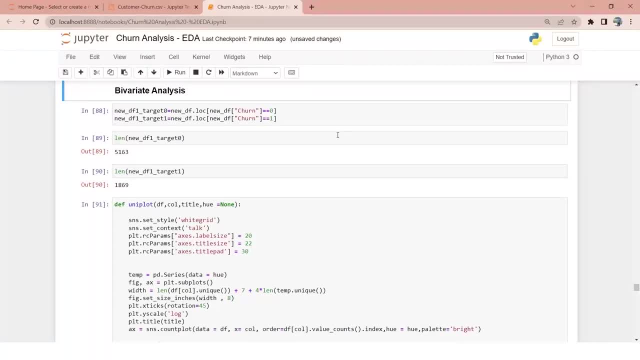 target 0 and target 1. first data frame is about the non-churners and the second one is about the non-churners and the second one is about the non-churners and the third one is about the non-churners and the second one is about the churners. i'll do this. the non-churners are 5000. 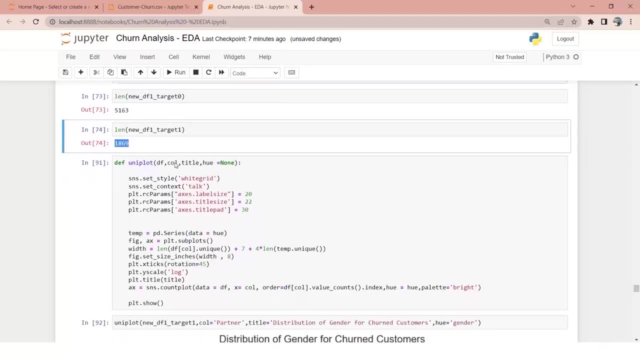 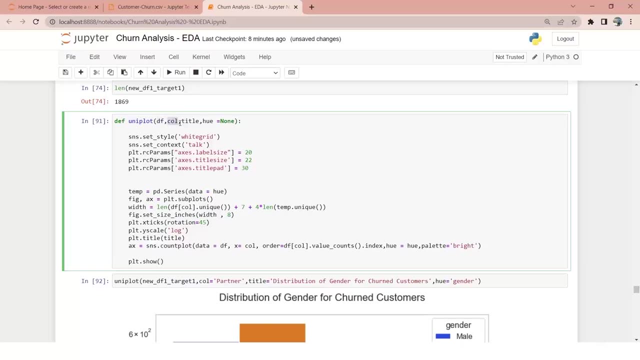 and the churners are around 1800- 1869. i have created a function here, uni plot, where i'm taking input some data, column and title and hue, and i'm writing down some pieces of code to plot something. now this again is a reusable code in case you are doing ada. 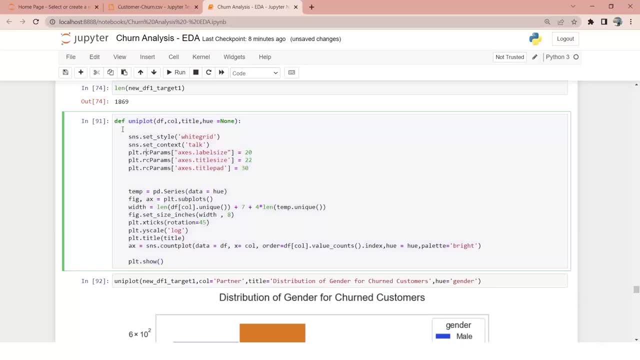 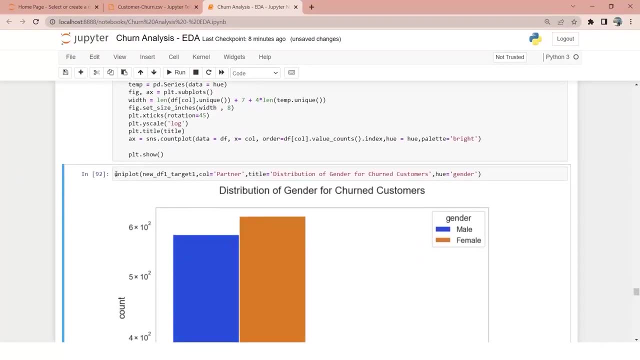 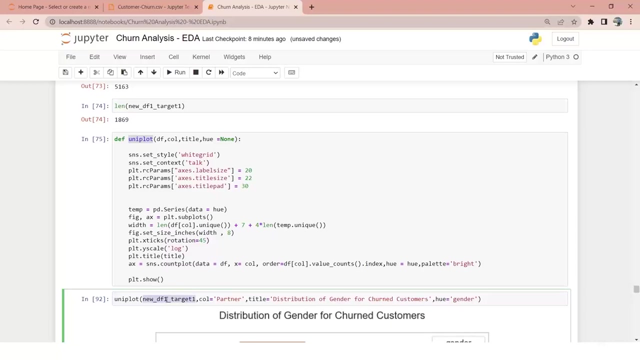 and you are performing some bivariate analysis, you can simply reuse this code. so i will not be explaining you this code. i will jump into the plot part. so here i am just calling my uni plot. i am passing my data frame, which is my target one that means people who have churned. 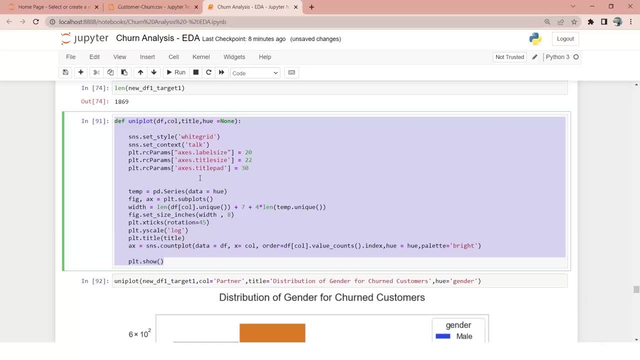 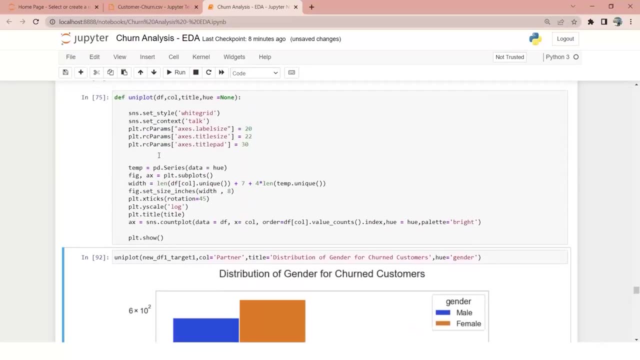 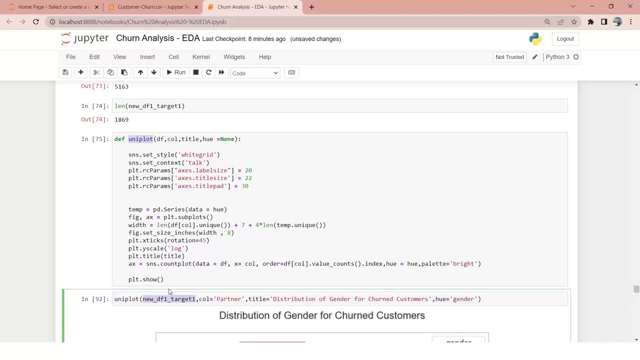 ada and you are performing some bivariate analysis, you can simply reuse this code. so i'll not be explaining you this code. i will jump into the plot part. so here i'm just calling my uni plot. i am passing my data frame, which is my target one that means people who have churned. 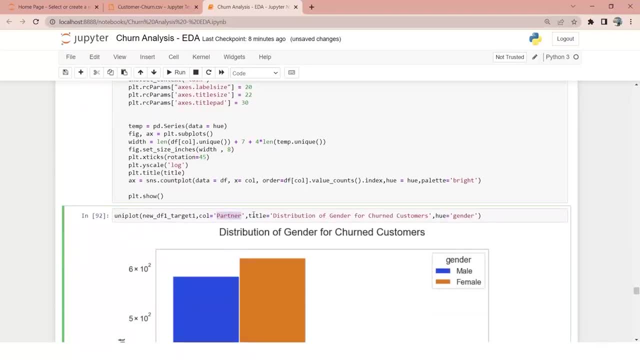 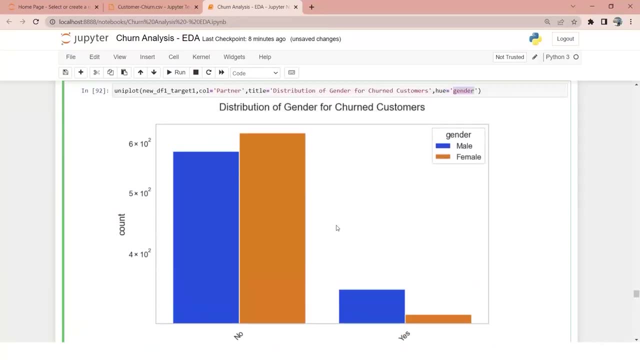 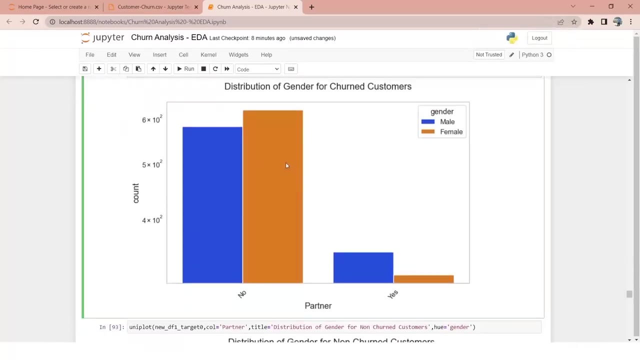 i am passing my column, which is partner. my title is distribution of gender for churned customers. my hue is gender. so this, basically, is partner versus gender graph. okay, partner versus gender. now what do you infer from this? you can see that people who don't have partners female 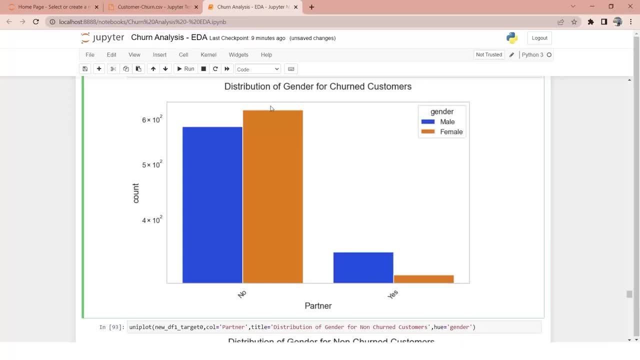 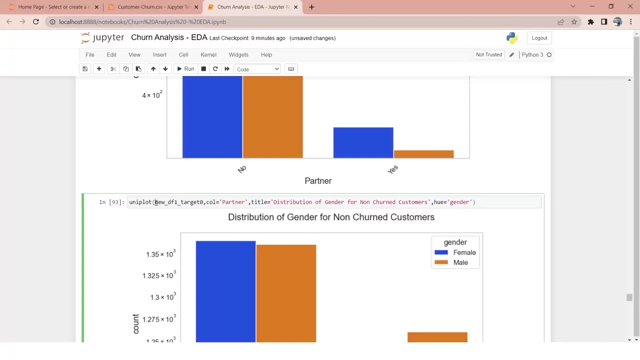 female. female customers who don't have partners are more likely to churn. male male customers who have partners are more likely to churn. so, again, these kind of insights you can infer. similarly, i am plotting the same graph for non-churners, and this is what the graph 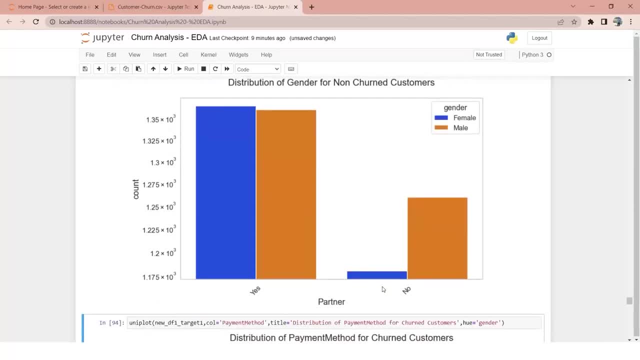 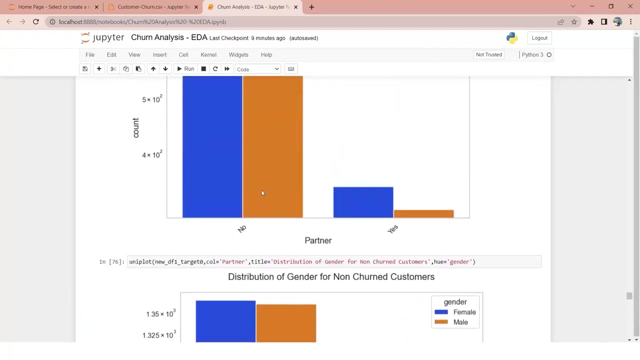 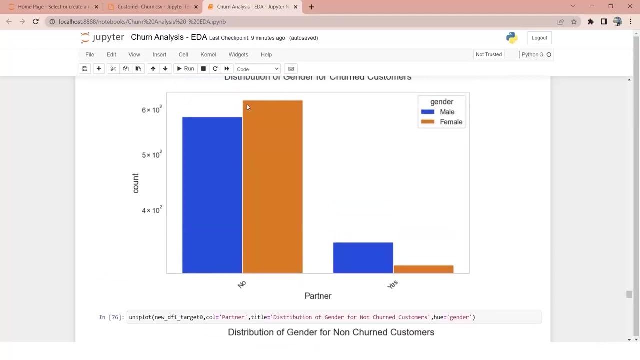 is for non-churners, that people who don't have partners. most of the people, most of the non-churners, are male, right, so churners are female, you can see. so most of the people who are female and having no partners are more churners. now, this is an. 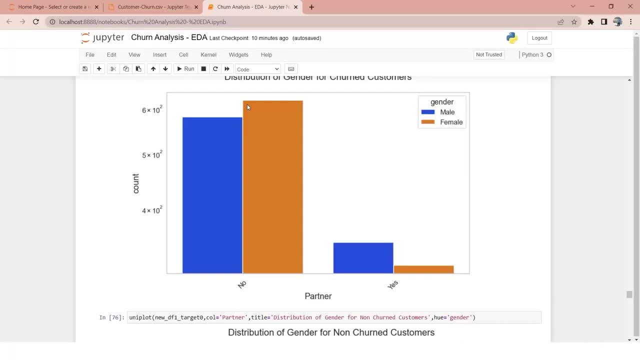 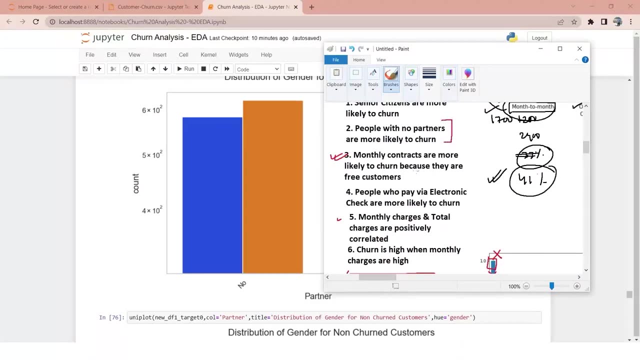 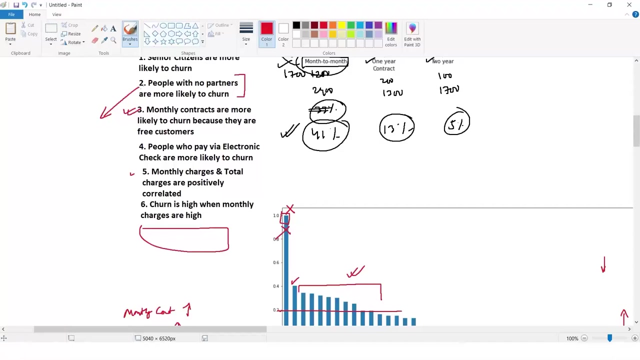 insight that we got from here. so initially we got some insights like this: right people with no partners are more people with no partners are more likely to turn. right people with no partners are more likely to turn. but now i got some further insights, some further insights that i have to be very specific. 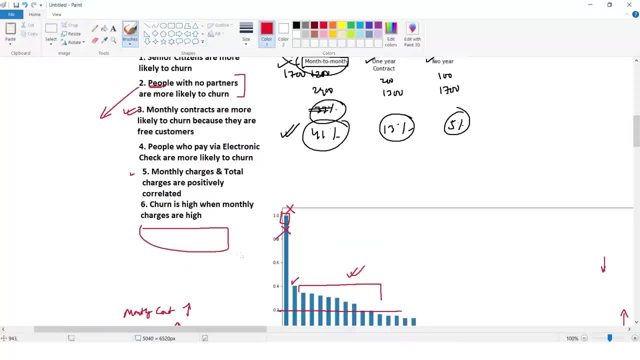 female without any partners. female with no partners are more likely to churn than males. so that is my updated insight. so i'll probably update this insight. i'll not be very specific, i'll not be very generalizing that people with no partners are more likely to churn, but rather i will tell: female with no partners are more likely to churn. 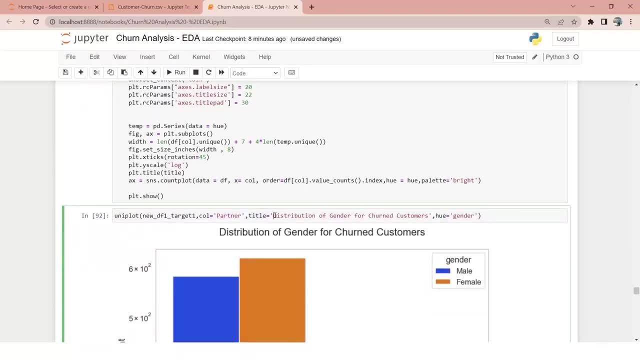 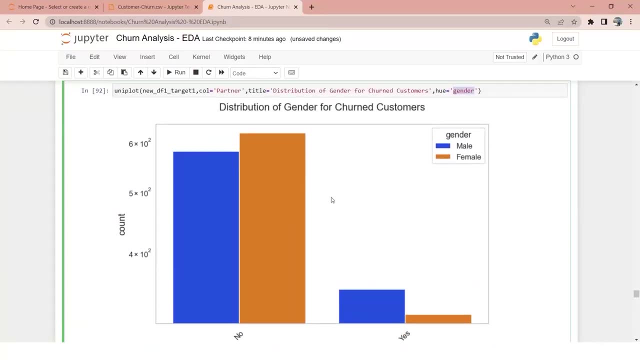 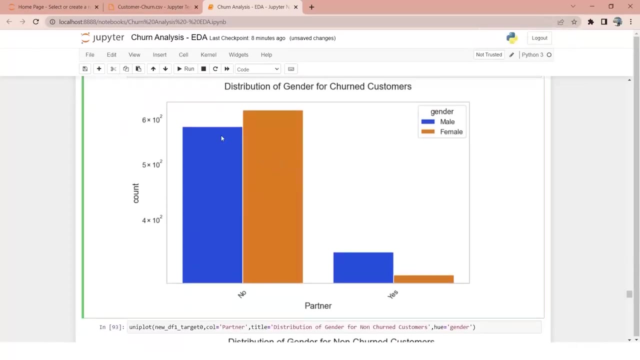 i am passing my column, which is partner. my title is distribution of gender for churned customers. my hue is gender. so this basically is partner versus gender graph. okay, partner versus gender graph. now what do you infer from this? you can see that people who don't have partners female 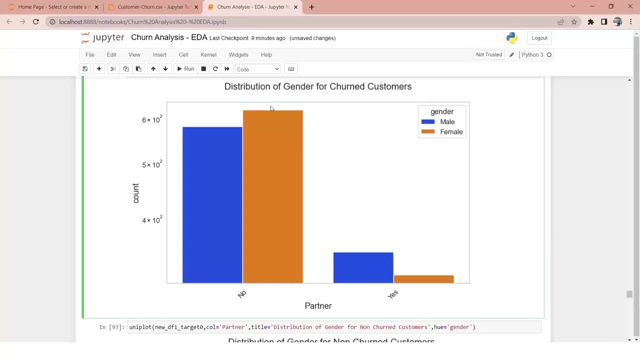 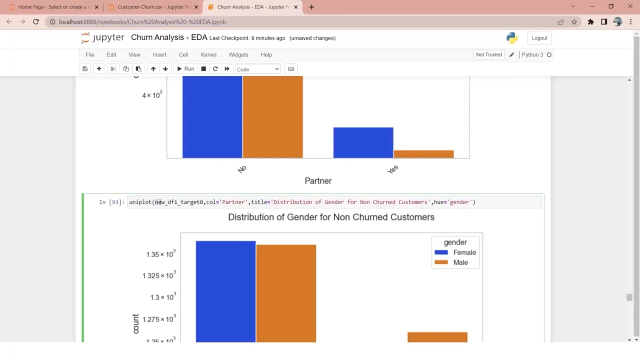 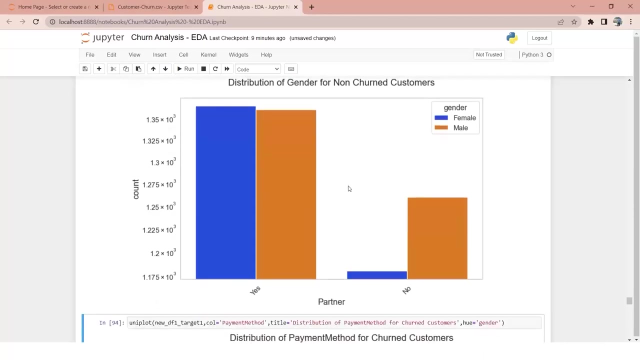 female: female customers who don't have partners are more likely to churn. male part: male customers who have partners are more likely to churn. so again, these kind of insights you can infer. similarly, i am plotting the same graph for non-churners, and this is what the graph is for non-churners: that people who don't have partners 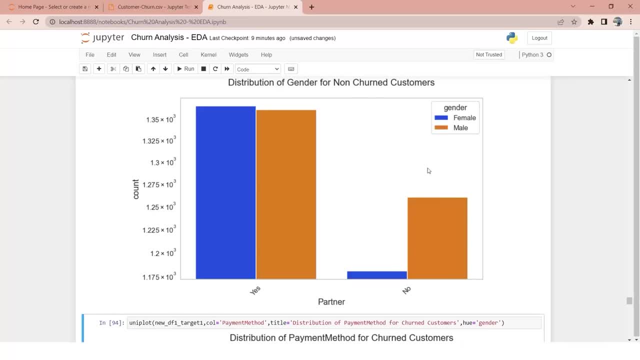 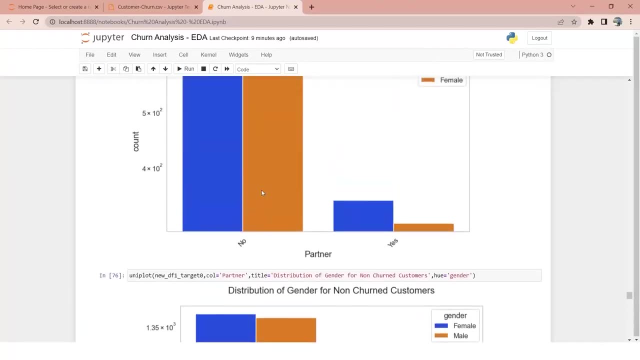 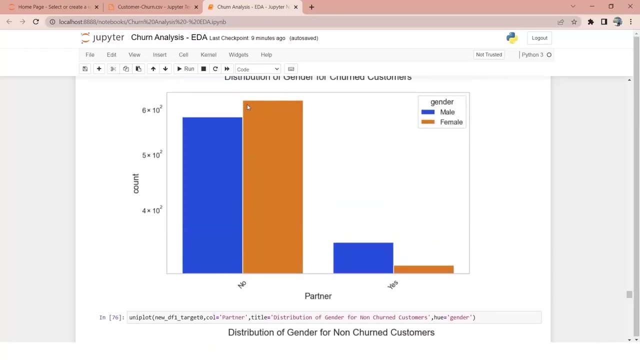 most of the people, most of the non-churners, are male, right, so churners are female, you can see. so most of the people who are female and having no partners are more churners. so this is an insight that we got from here. so initially we got some insights like this right. 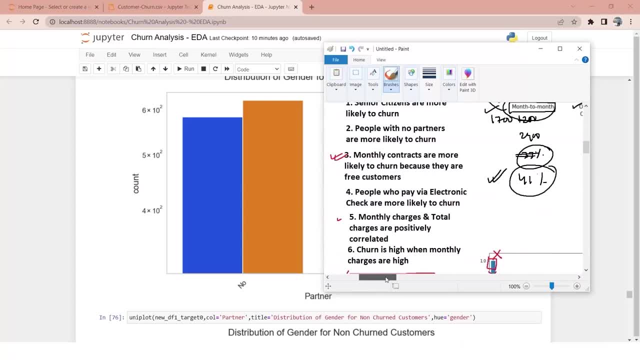 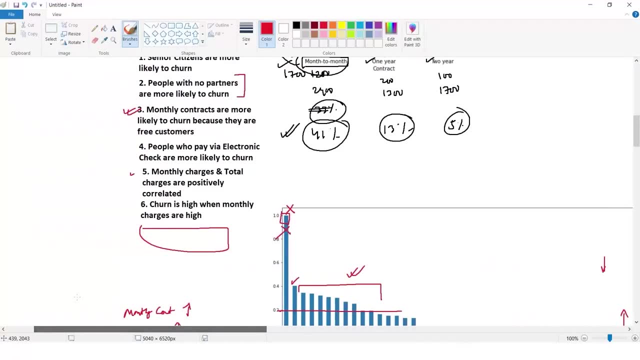 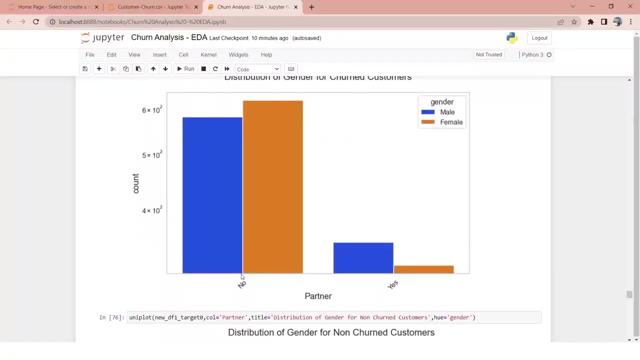 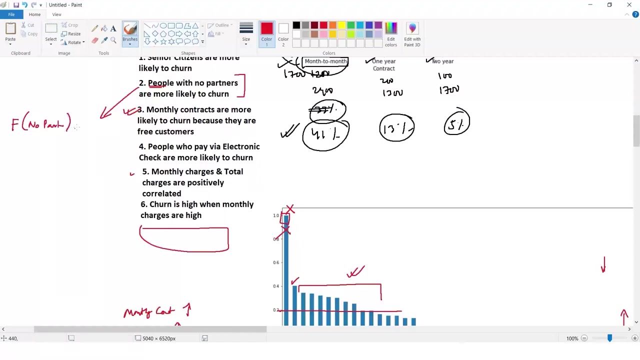 people with no partners are more likely to churn. but now i got some further insights, some further insights that i have to be very specific about, because i have found that most of the people have no partners. specific female without any partners, female with no partners are more likely to turn than males. so 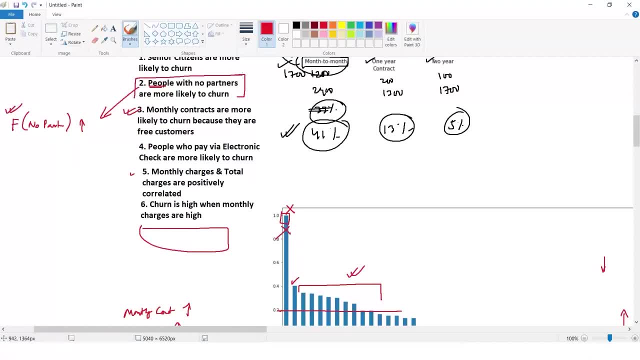 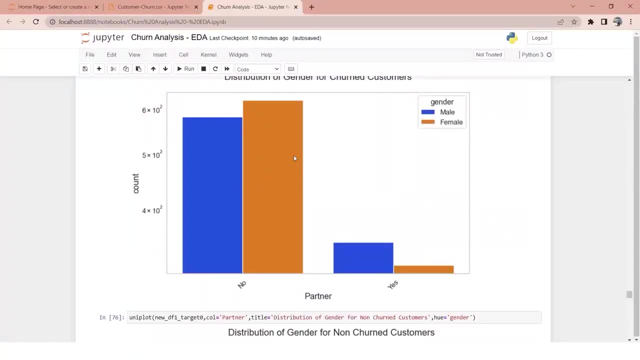 that is my updated inside, so I'll probably update this inside. I'll not be very specific, I'll not be very generalizing that people with no partners are more likely to turn, but rather I will tell female with no partners are more likely to turn, because that is what my graph is telling. 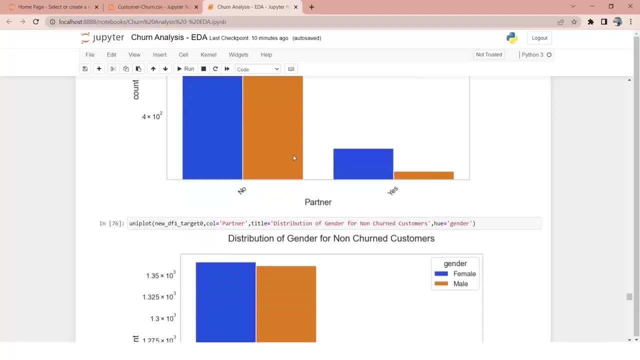 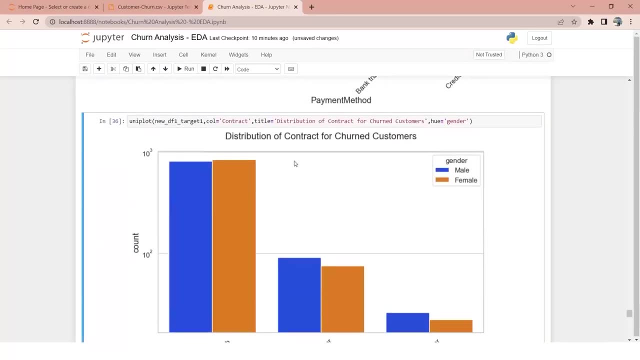 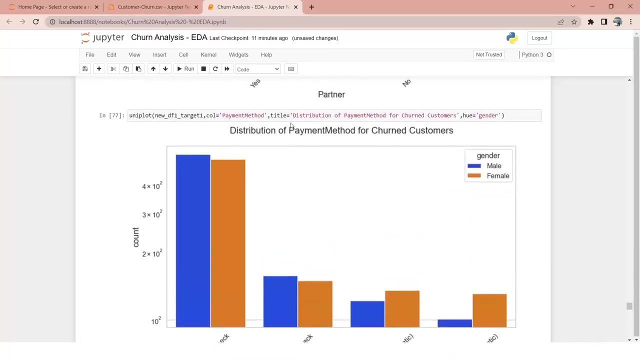 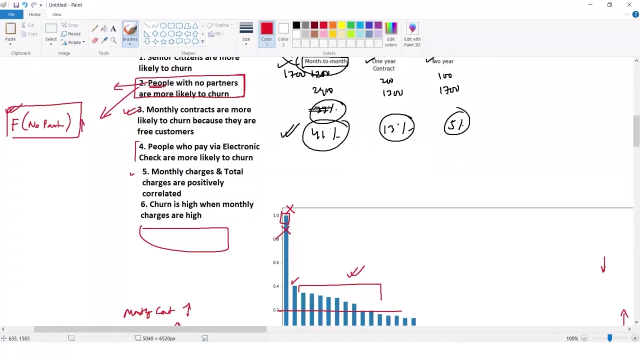 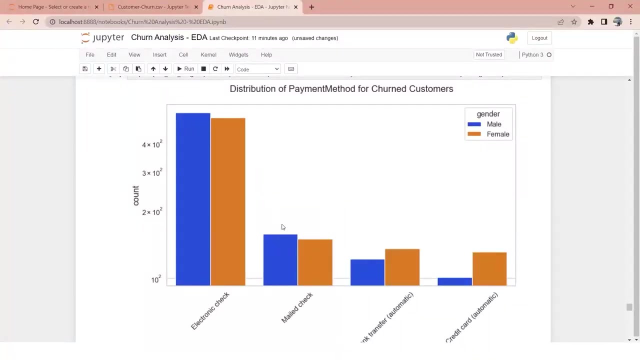 because that is what my graph is telling. similarly, you do it for other things: payment method. so this is a churn graph, distribution for the churn customers. and, sorry, this one payment method distribution for the churn customers. now, we all know that people who are paying via electronic check are more likely to churn. that's already a known insight. here also, it's quite evident that 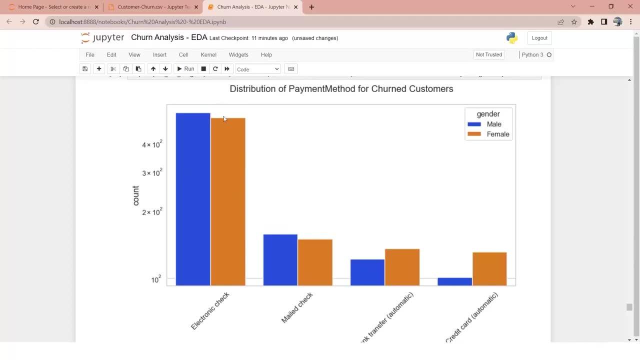 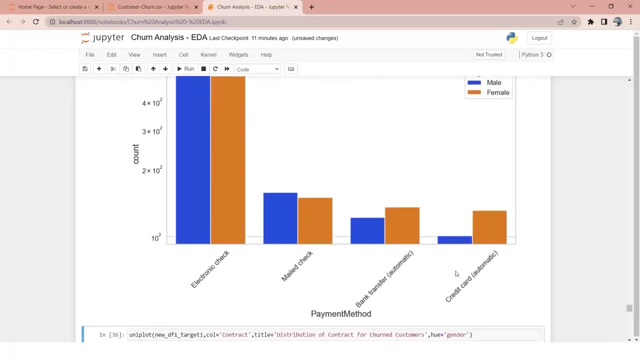 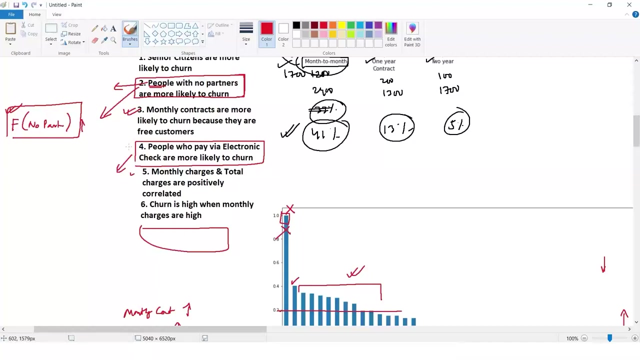 electronic check. the number of churners are high, but one important insight that we are getting here is, even though the credit card transactions are less, but you more female, are into churning. so one more additional insight here will be- i would note it down as an extension of 0.4, maybe 0.4.1- that female who are paying. 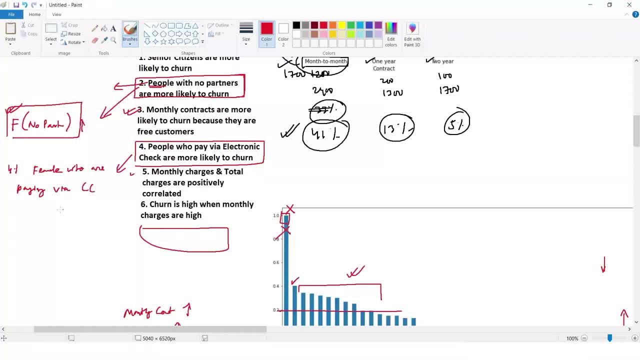 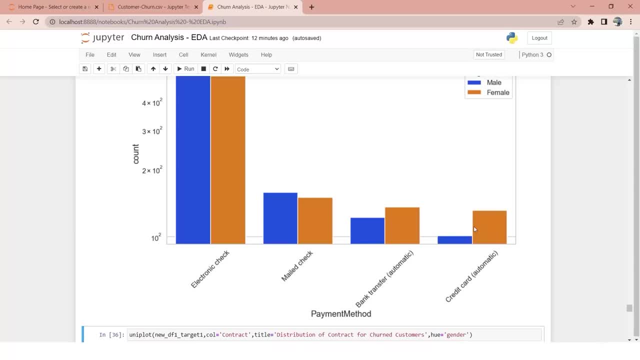 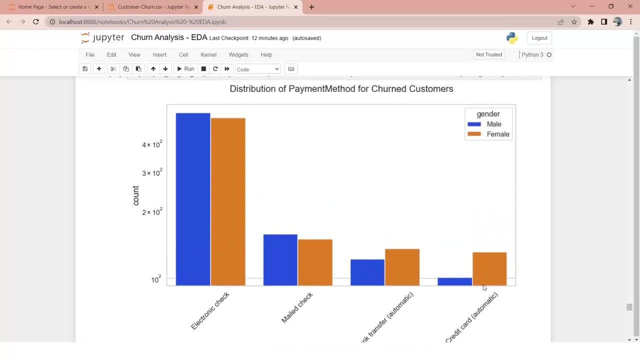 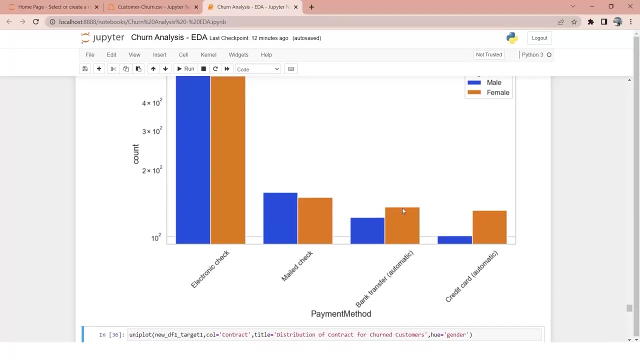 via credit cards are more likely to churn automatic transfers. now i'm not inferring anything, but this is what the data is telling. so female who are paying through credit cards are more likely to churn as compared to males. other than that, even in bank transfer, also, female are little bit more in number as compared to males, but mailed check almost similar, almost. 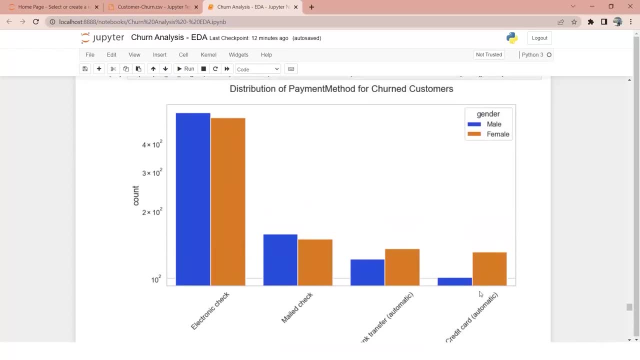 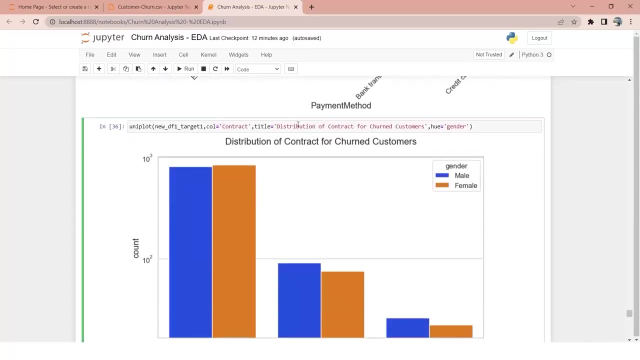 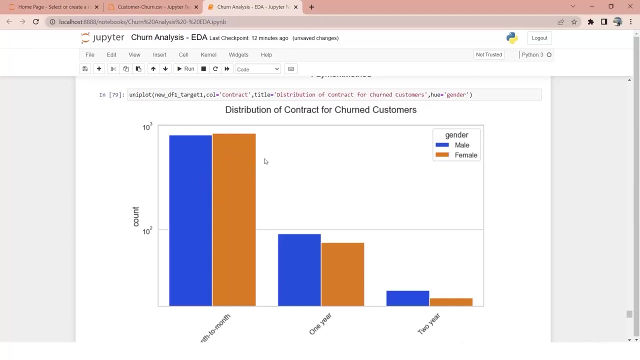 one is to one. here also, almost one is to one. so this is a major insight. this is a medium insight. similarly, i will do it for contract for contract. i don't see huge impact. male and female are equally distributed, okay, but in the two yearly contracts more males are likely to churn. but yeah, this is not. 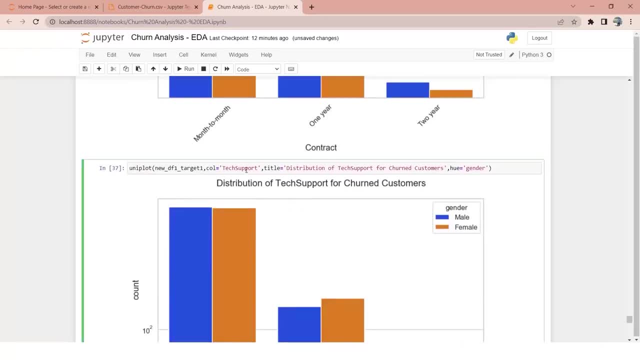 a great insight, so i'll skip it. i'll do it for tech support and similarly, you have to do it for other things. now just imagine how many combinations of graphs there will be in terms of bivariate. if you have 20 columns in univariate, you can simply plot 20 graphs, but you are plotting bivariate analysis, so you can. 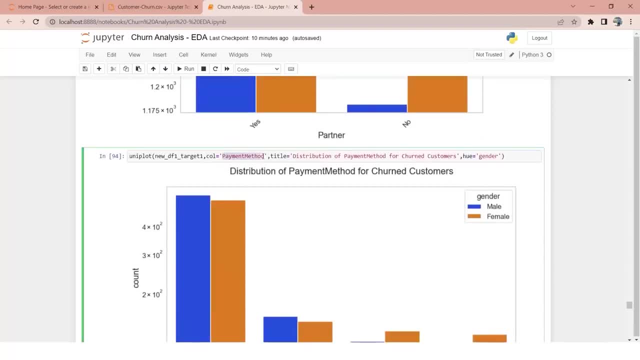 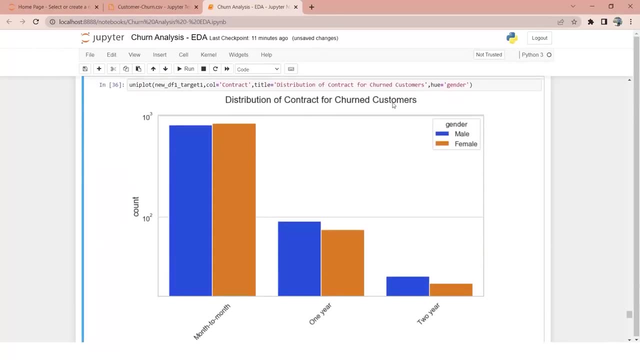 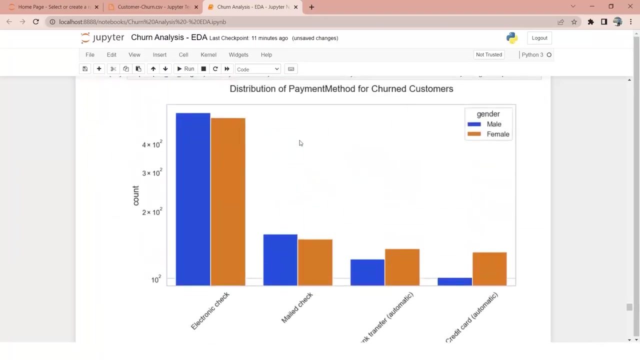 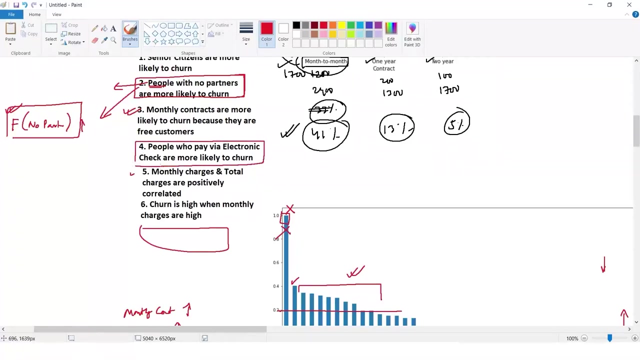 similarly you do it for other things- payment method. so this is a churn graph: distribution for the churn customers. and sorry, this one payment method distribution for the churn customers. now, we all know that people who are paying via electronic check are more likely to turn. that's already a known insight. here also, it's quite evident that 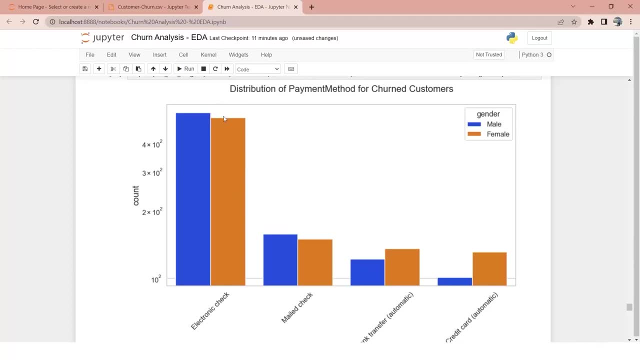 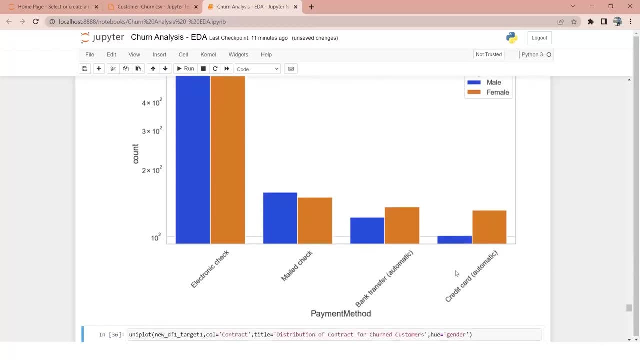 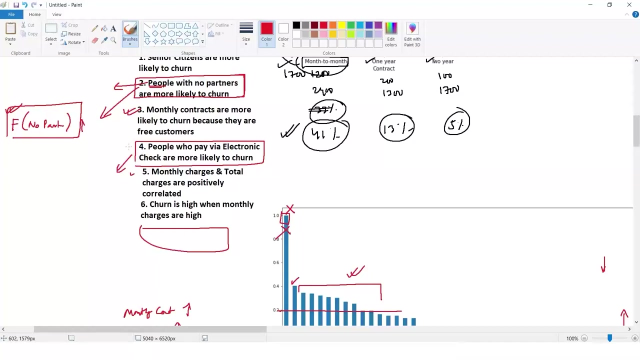 electronic check. the number of churners are high, but one important insight that we are getting here is, even though the credit card transactions are less, but more female are into churning. so one more additional insight here will be- I would note it down as an extension of 0.4, maybe 0.4.1- that female who are paying via credit cards are more likely to. 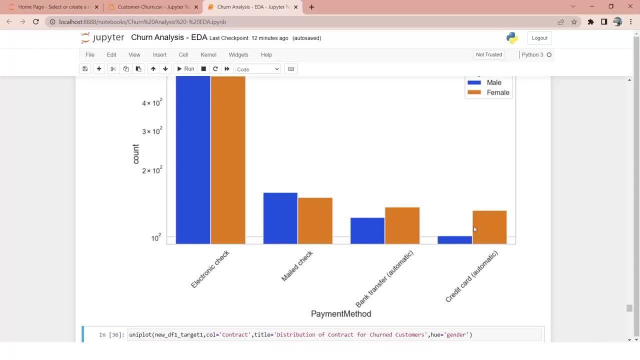 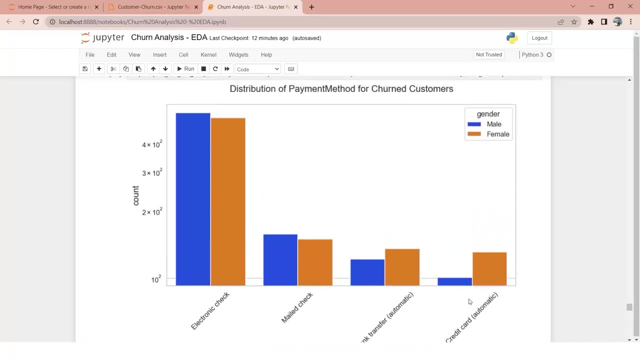 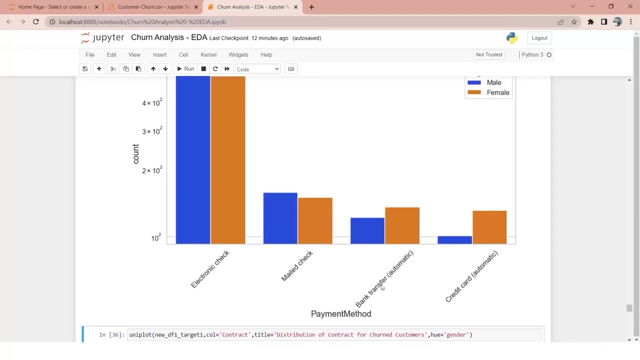 churn automatic transfers. now I'm not inferring anything, but this is what the data is telling. so female who are paying through credit cards are more likely to churn as compared to males. other than that, even in bank transfer also, female are little bit more in number as compared to males. but mailed check- almost similar, almost one is to one here, also almost. 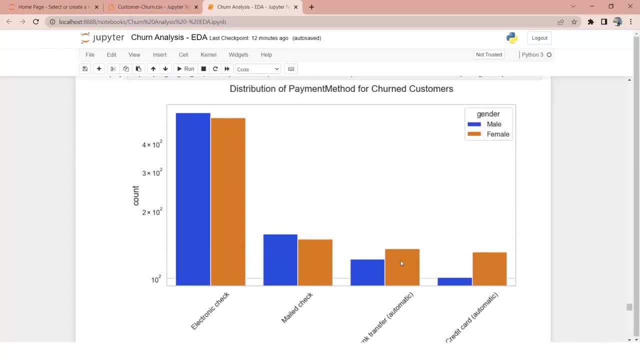 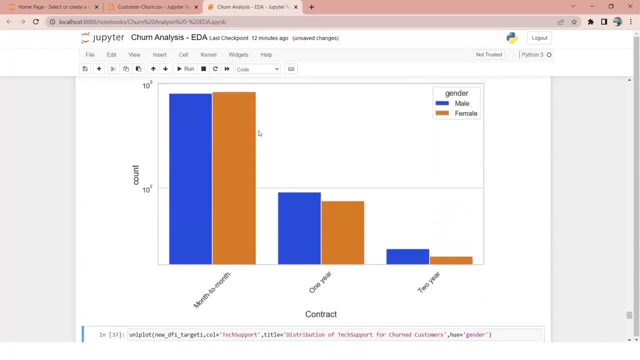 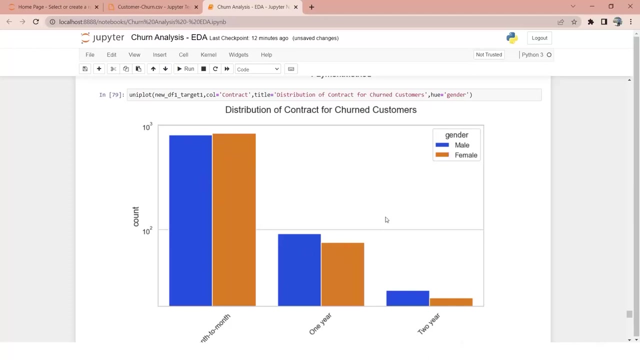 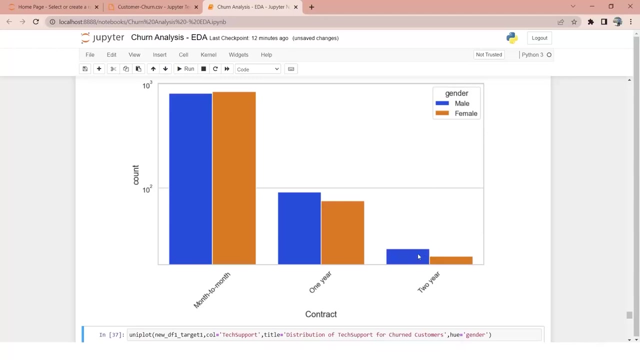 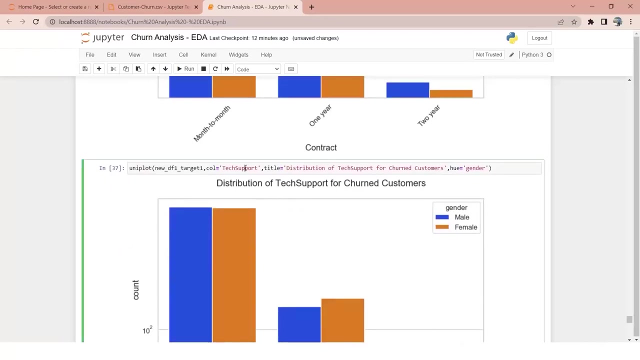 one is to one, so this is a major inside. this is a medium inside. similarly, I will do it for contract for contract. I don't see huge impact. male and female are equally distributed, but in the two yearly contracts, more males are likely to churn. but yeah, this is not a great insight so I'll skip it. I'll do it for tech support and similarly you have to do it for other things. 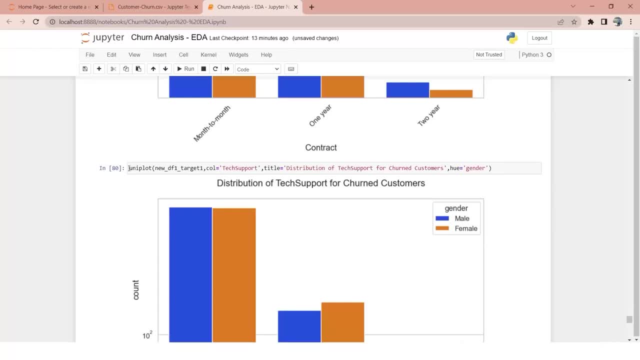 now just imagine how many combinations of graphs there will be in terms of bivariate. if you have 20 columns in, in univariate, you can simply plot 20 graphs, but you are plotting bivariate analysis, so you can imagine how much combinations are possible: one with two, one with three, one with four. dot dot dot. 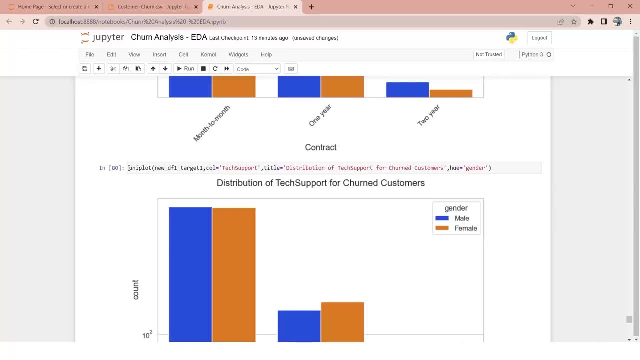 one with ten and same two with one, two with two, two with three, and goes on right. there will be a lot of combinations and, similarly, if you jump into trivariate, four variate or multivariate, you can imagine how many total number of graphs there will be, and that is one of the reasons we 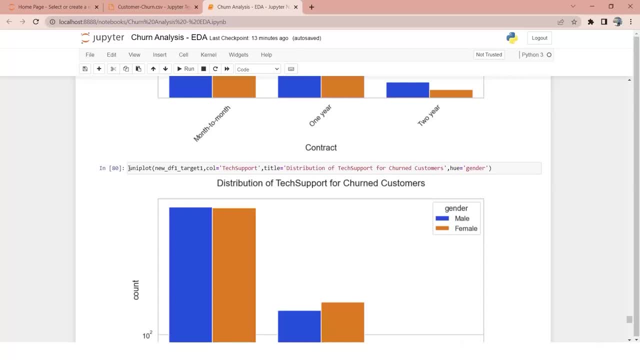 consider eda to be one of the most important steps and one of the most tedious step, because it takes a lot of time and again, it all depends on the client's requirement. if your manager tells you to perform eda in one hour, it is possible. if your manager asks you to perform eda in one day, 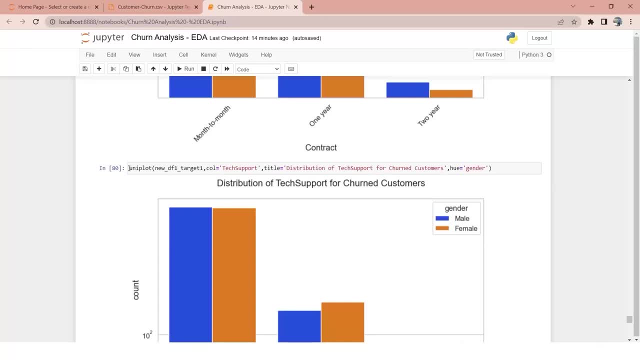 it is possible. if your manager wants you to perform eda for one week or one month, that is also possible. one hour or one day could be less eda. you might not waste a lot of time in cleaning the data probably will jump into some univariate and bivariate if you get more amount of time for eda. 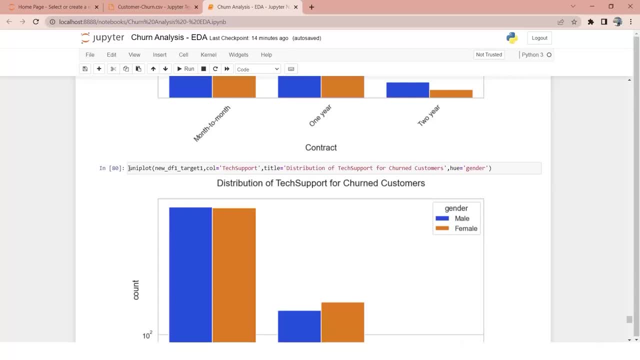 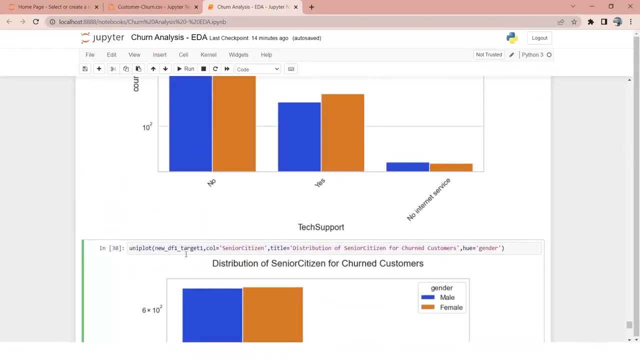 you can probably deep dive, do some mix and match of multiple columns, numerical, with categorical multivariate. a lot of insights can be gathered in that process as well. so overall that's all about bivariate analysis. you can just simply play around with this function: pass multiple columns, multiple hues and just cross. 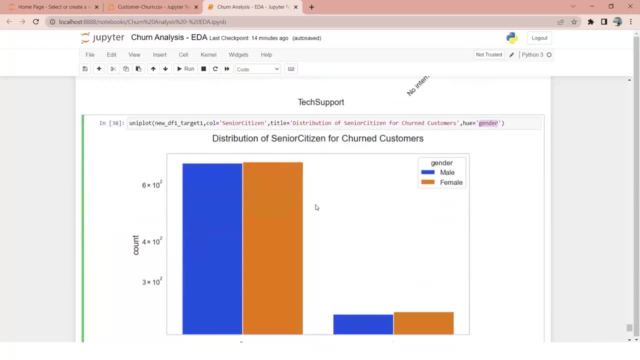 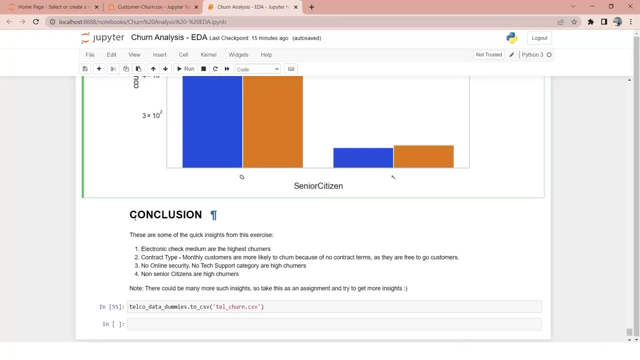 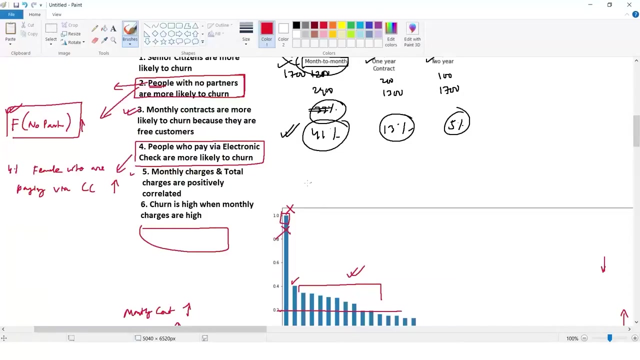 check and gather as much insights as possible. so that brings to an conclusion of this particular exercise on eda. i hope you had a great understanding on this particular use case about churn analysis. the conclusion here are very less. we have drawn more conclusions on this paint brush as compared to what is here. 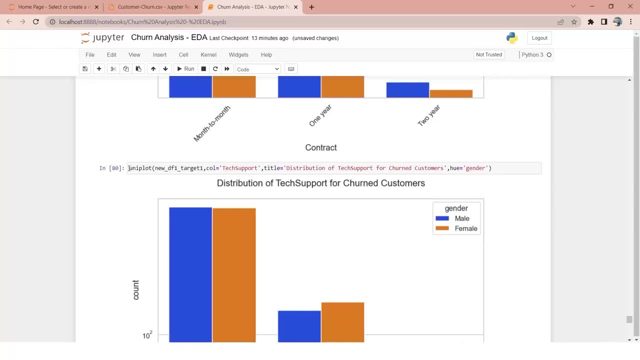 imagine how much combinations are possible: 1 with 2, 1 with 3, 1 with 4, dot dot dot, 1 with 10, and same 2 with 1, 2 with 2, 2 with 3, and goes on right. there will be a lot of combinations. 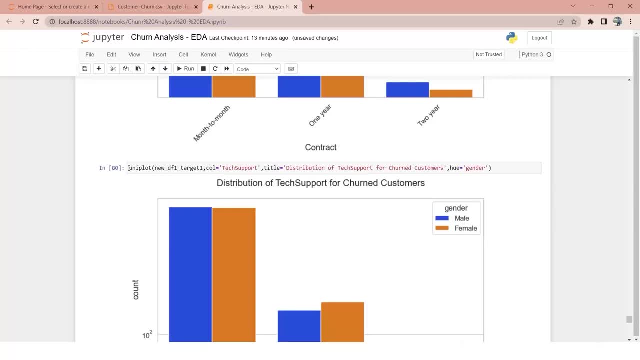 and similarly, if you jump into trivariate, 4 variate or multivariate, you can imagine how many total number of graphs there will be. and that is one of the reasons we consider eda to be one of the most important steps and one of the most tedious step, because it takes a lot of time and again it all. 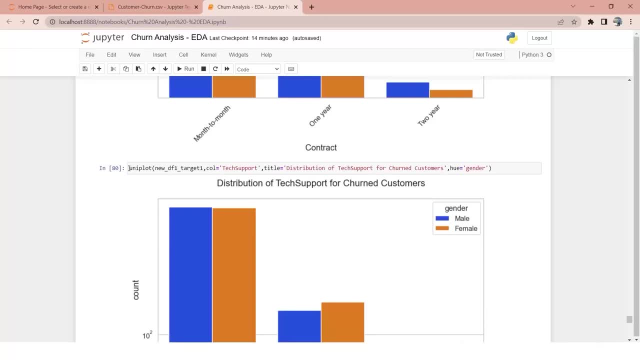 depends on the client's requirement. if your manager tells you to perform eda in one hour, it is possible. if your manager asks you to perform eda in one day, it is possible. if your manager wants you to perform eda for one week or one month, that is also possible. one hour or one day could be less ed. 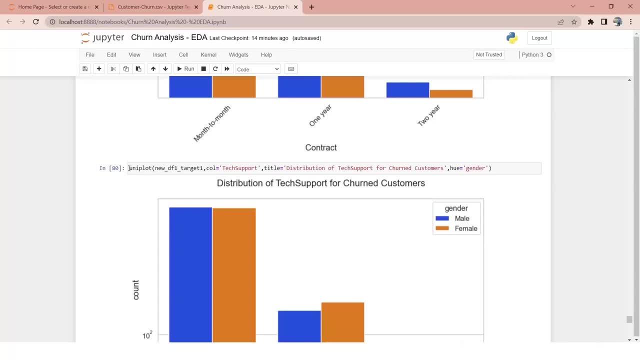 you might not waste a lot of time in cleaning the data probably will jump into some univariate and bivariate. if you get more amount of time for eda you can probably deep dive, do some mix and match of multiple columns, numerical with categorical multivariate. a lot of insights can be. 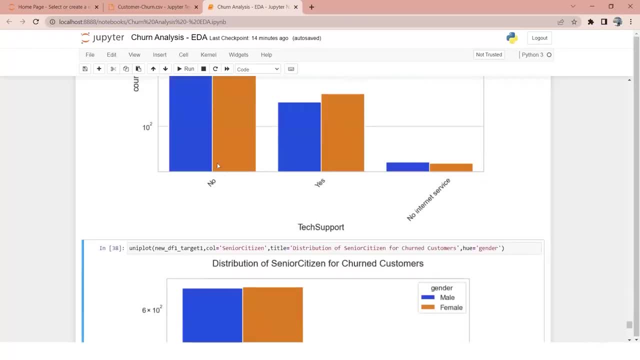 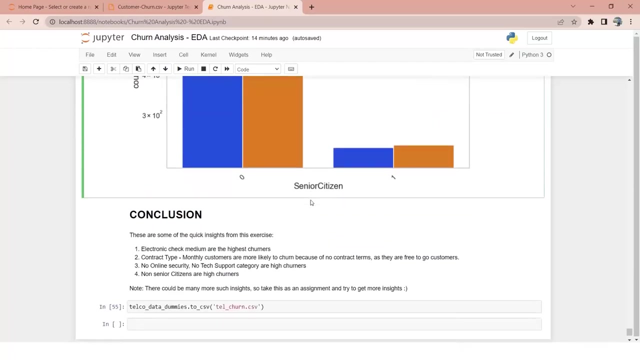 gathered in that process as well. so overall that's all about bivariate analysis. you can just simply play around with this function, pass multiple columns, multiple hues and just cross check and gather as much insights as possible. so that brings to an conclusion of this particular exercise on ada. i hope you had a great understanding on this particular use case. 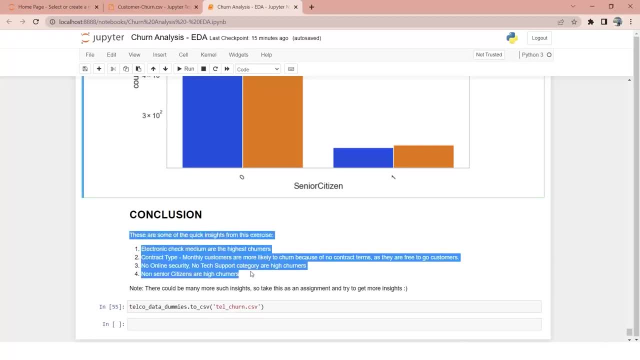 about churn analysis. the conclusion here are very less. we have drawn more conclusions on this paint brush as compared to what is here, but again, i'll keep it as an open assignment to you. probably you can do further analysis and come up with hundreds and hundreds of conclusion. 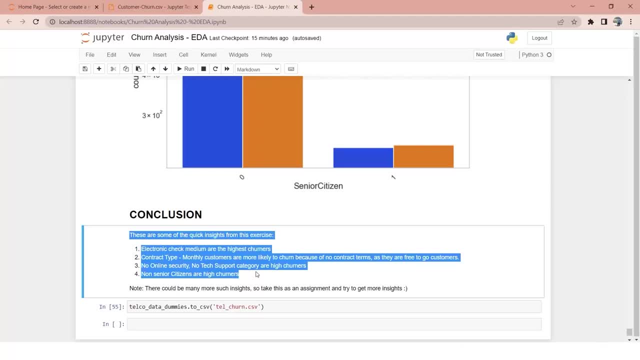 but again, i'll keep it as an open assignment to you. probably you can do further analysis and come up with hundreds and hundreds of conclusion, hundreds and hundreds of insights. apart from that, as part of ed exercise, it is also recommended that you create an end-to-end report, a report that someone 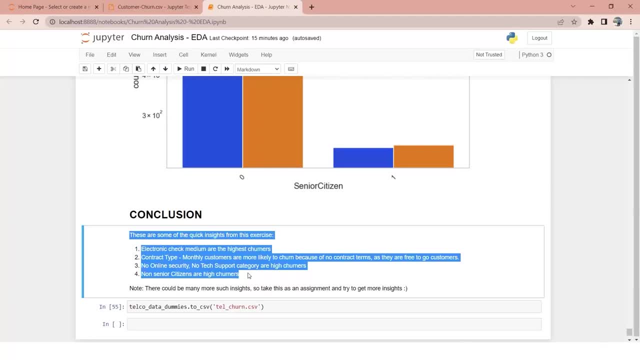 will during the entire session of ed exercise. that will inform you about what is said in the report, a report that you can consume and then cover by providing the results using all the resources available- available in a report as well. it summarizes your ada task because ultimately, you will be showcasing this to your manager or to your customers, who might not understand the 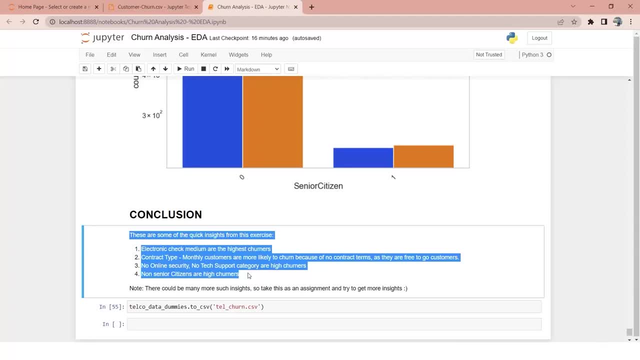 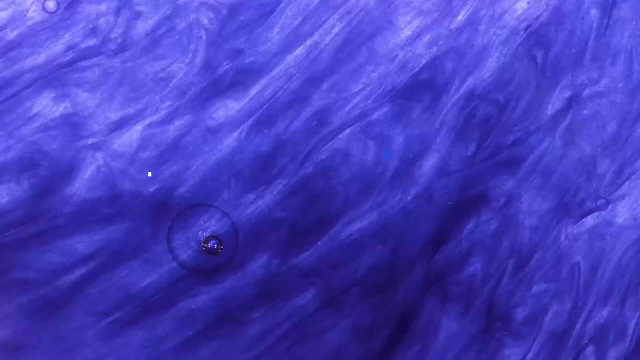 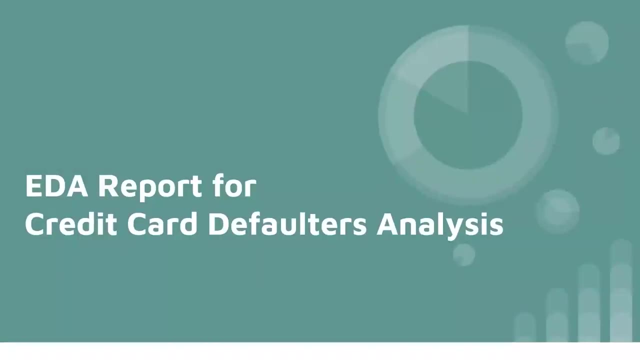 are created, how presentations are created. that will automatically do the data storytelling part of your entire analysis. so we'll go through one of the eda reports for a different eda use case, for a different case study. so the case study was credit card defaulters analysis, where we have to. 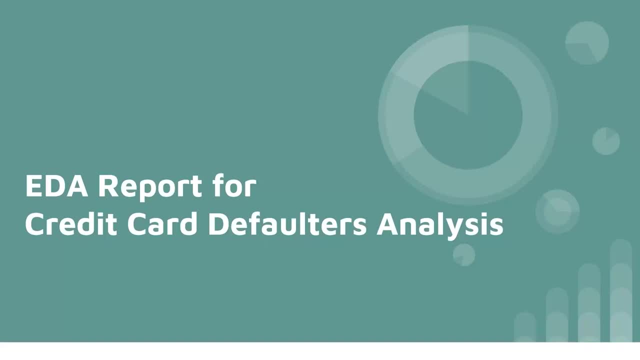 analyze the different credit card defaulters who have been defaulter in the bank. they have not paid or they have missed out their payment and become defaulters, and so on. it's a different use case. the use case that we were going through practically was churn analysis, but this eda report is for. 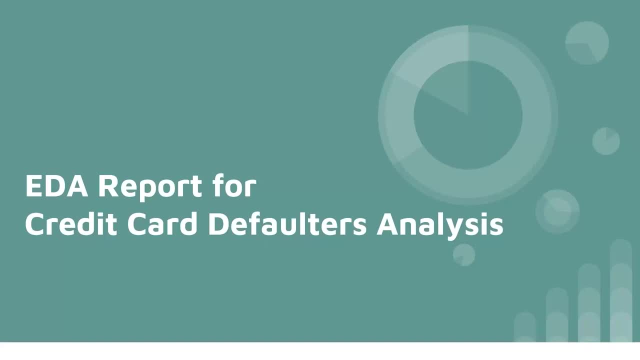 another use case, but, however, this report will give you an idea on how to build an eda report based on the ideas. have to create the eda report, firstly for the churn analysis use case that you have recently studied. apart from that, you will also have to work on multiple other eda use cases and you have to 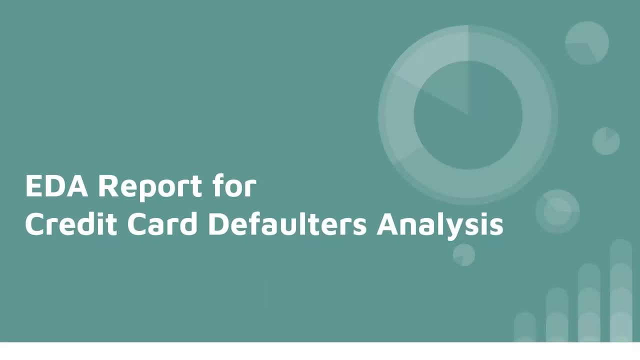 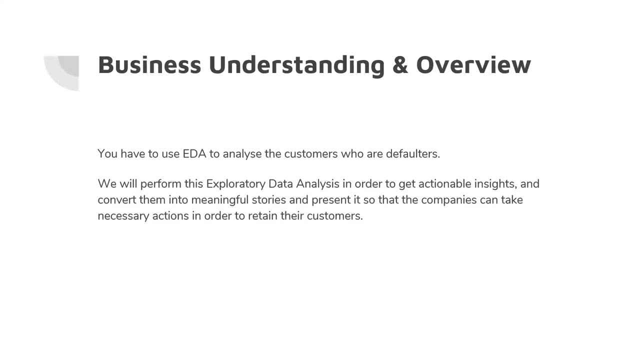 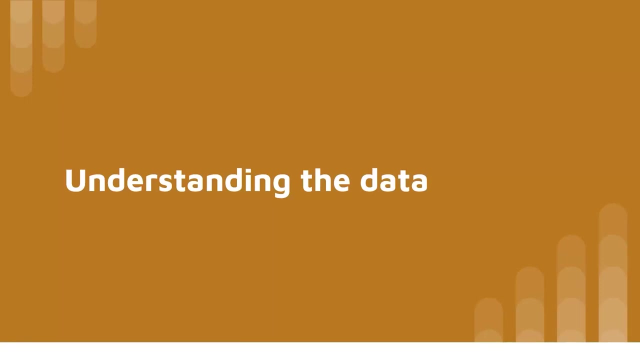 create reports. a report should always start with the business understanding and overview. business understanding is nothing but what the report is all about. what is the use case? then it comes about what is the use case. so, once you know the use case, has pysoalectra. 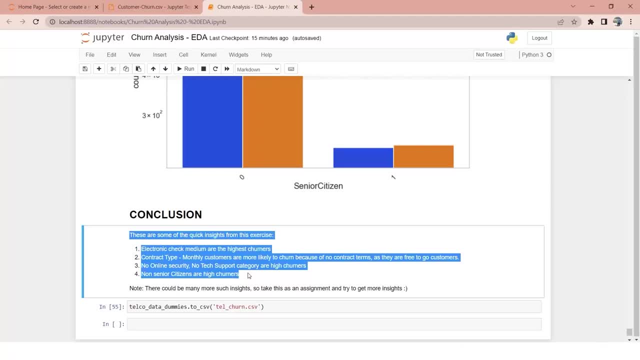 hundreds and hundreds of insights. apart from that, as part of eda exercise, it is also recommended that you create an end-to-end report, a report that summarizes your ada task, because, ultimately, you will be showcasing this to your manager or to your customers, who might not understand the programming. 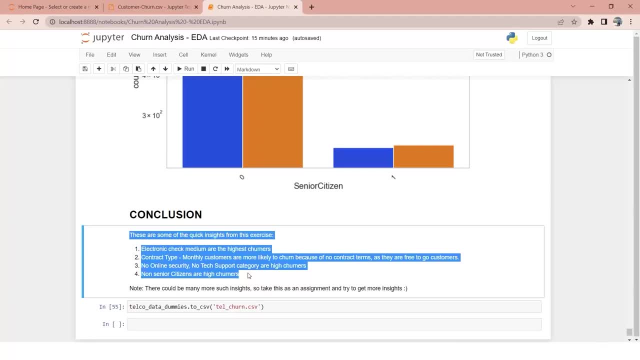 language, so a report is definitely important. i have, however, created a report. probably i will show that report as part of the next video and i will just explain you how i created that report, which will give you an end-to-end idea on how reports are created, how presentations are created. that will automatically do the data storytelling part. 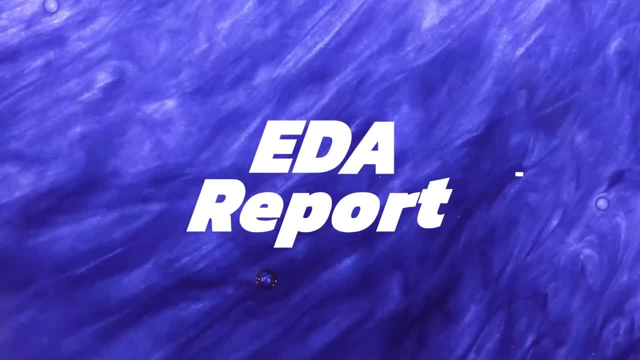 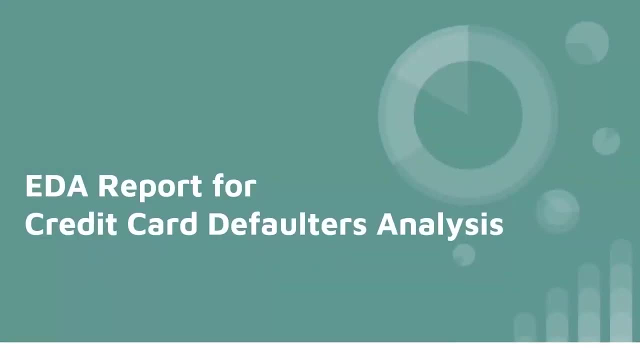 of your entire analysis. so we'll go through one of the eda reports for a different eda use case, for a different case study. so the case study was credit card defaulters analysis, where we have to analyze different credit card defaulters who have been defaulter in the bank. they have not paid or they 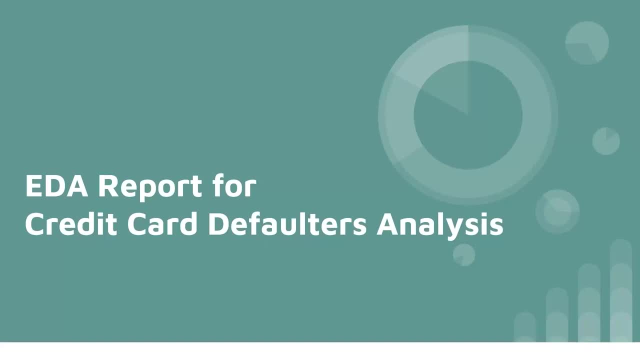 have missed out their payment and become defaulters and so on. it's a different use case. the use case that we were going through practically was churn analysis, but this eda report is for another use case. but, however, this report will give you an idea on how to build an eda report based on the ideas. 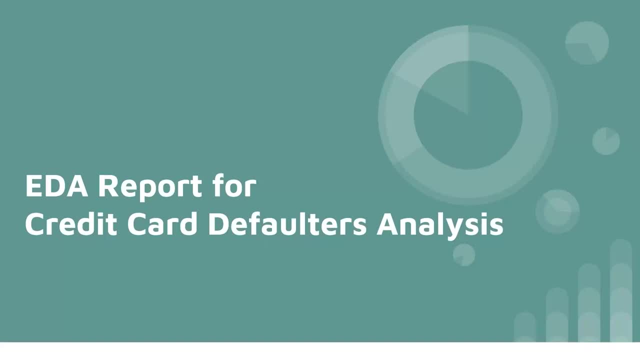 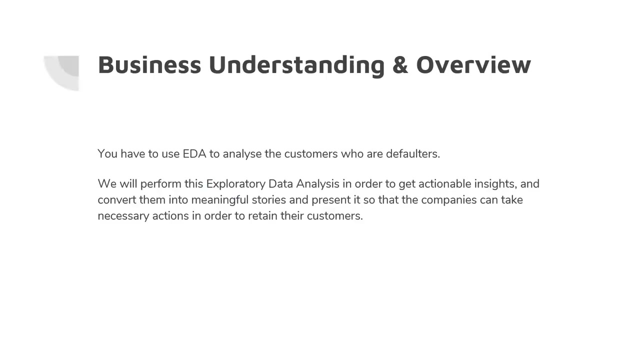 you have to create the eda report, firstly for the churn analysis use case that you have recently studied. apart from that, you will also have to work on multiple other eda use cases and you have to create reports. a report should always start with the business understanding and overview business. 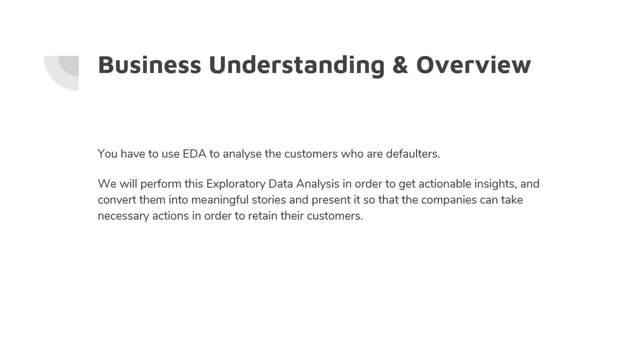 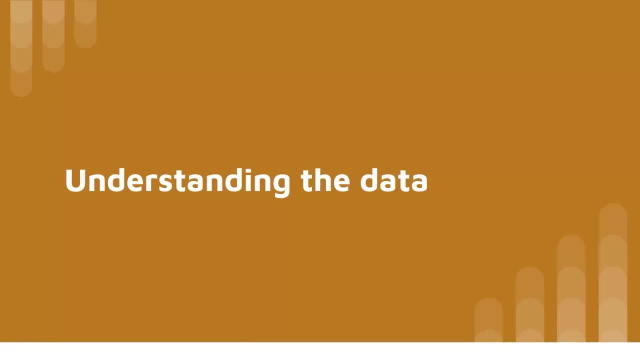 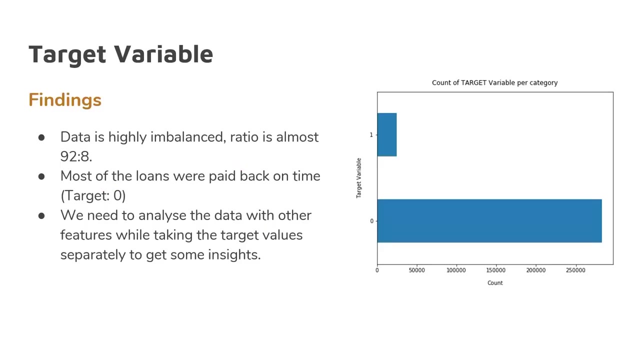 understanding is nothing but what the report is all about. what is the use case? then it comes understanding and overview the data. whatever you have understood from the data, you should start writing it down. first of all, if your use case is having a target variable, which in the case of churn analysis, yes, there was a. 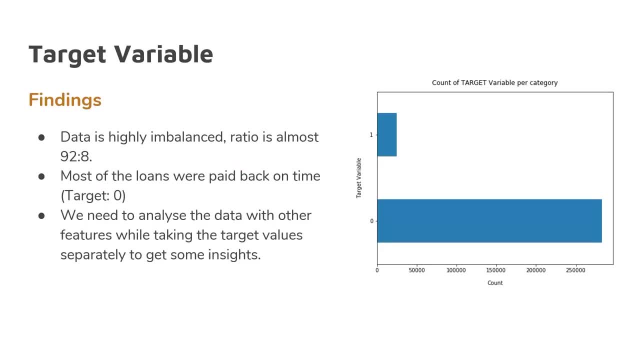 ethnic data. whatever you have understood from the data, you should start writing it down, first of all, if your use case is having a target variable, which, in the case of churn analysis, yes, there was a target variable called as churn column. so you have to write down your insights. 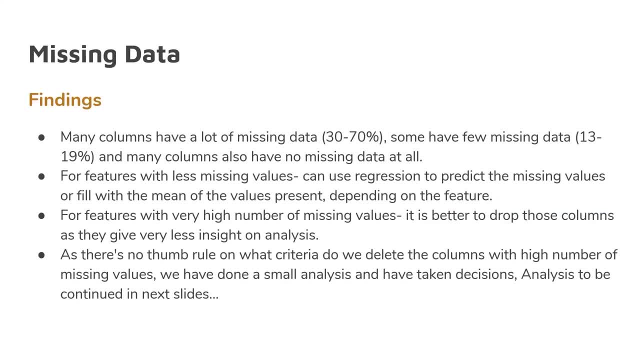 what are the findings? the data is highly balanced or not, and so on. missing data intuition use case. how many missing data did we have? how did you impute the missing data? so in the churn analysis, if you remember, total charges were having 0.15 percentage of missing data and we dropped it. 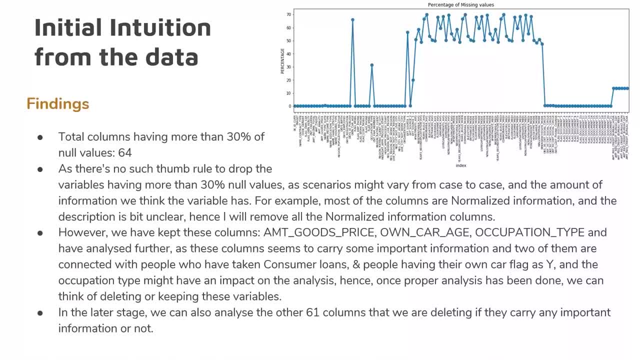 so you have to write down those things here. initial intuition from the data. in our case, again, there were no initial uh, there were no null values, but we understood that total charges was not in the format that we expected. hence we converted into numerical attribute and we got. 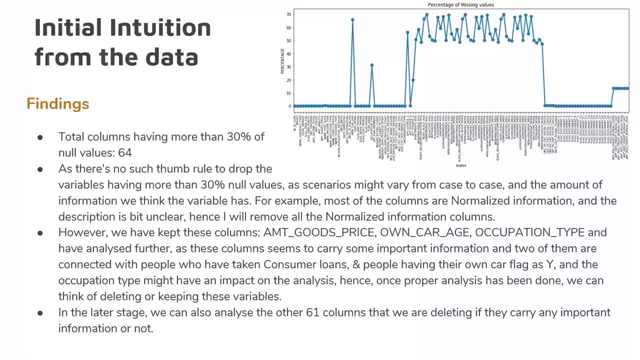 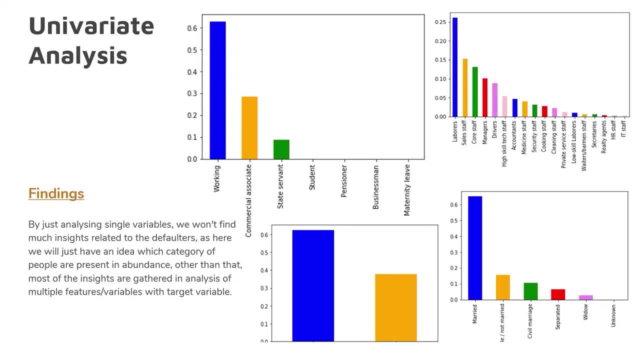 around 0.15 percentage of null values, right, so all those things has to be jotted down, and then comes your analysis part, the categorical analysis, with all the graphs and the findings in the page. whatever findings you have, you can just start mentioning them and it goes on: graphs, findings. 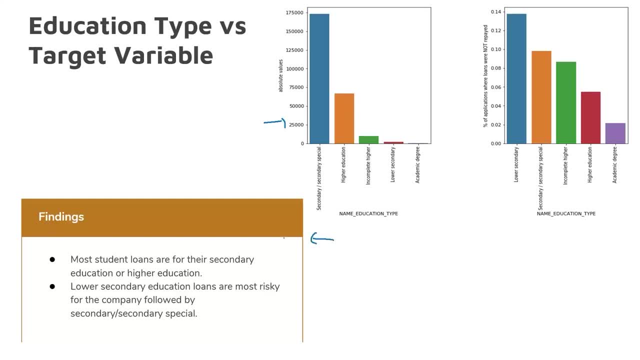 graphs, graphs, findings. so it gives a idea to the person who is actually watching out your report. they will be able to understand, they will be able to relate the graph and what's mentioned here now. for example, in this particular graph we have name education and we have name education type. 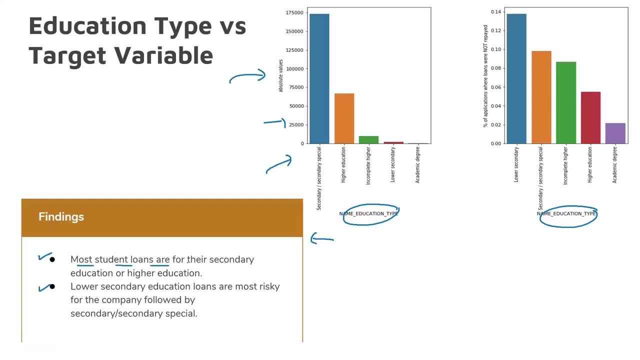 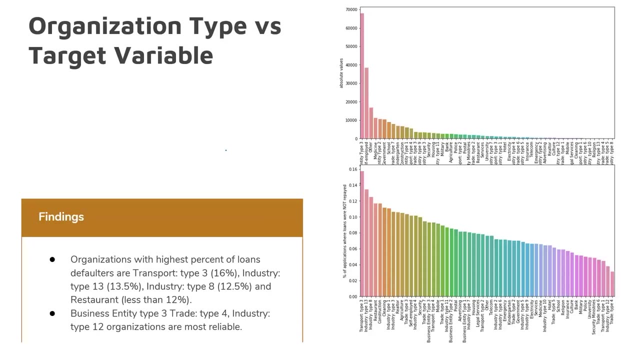 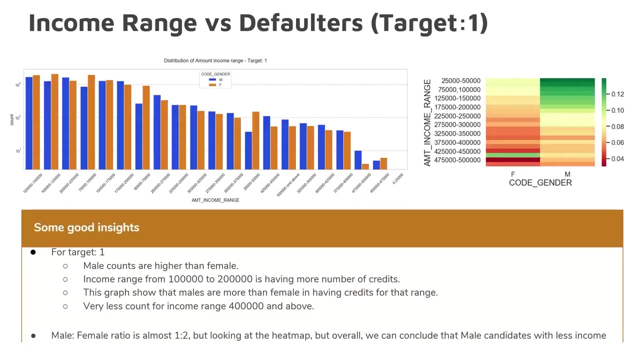 you can see, the findings are more. student loans are for their secondary education or higher education. right, it's quite evident. so you have to write down your findings and plot your graphs side by side. that gives a good understanding about what's happening. and it goes on. so we have done the same thing here: graphs and insights. graphs and insights similarly do it. 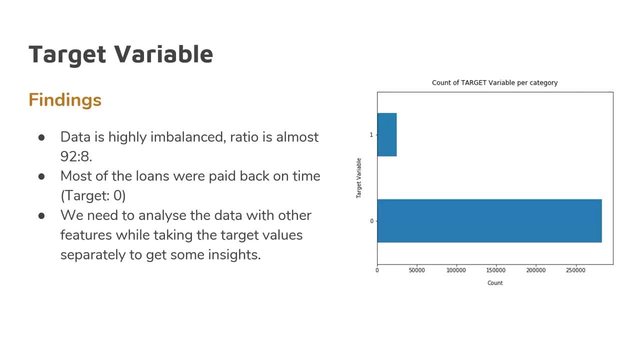 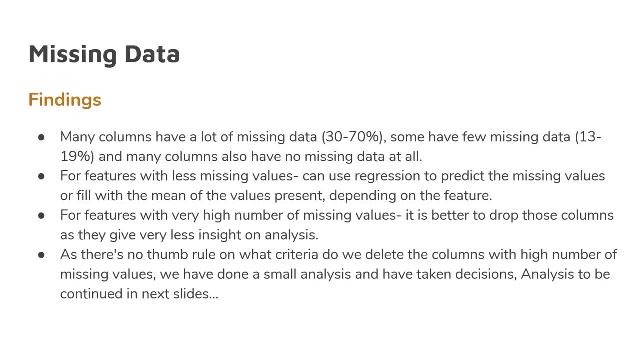 target variable called as churn column. so you have to write down your insights. what are the findings? the data is highly balanced or not, and so on. missing data, intuition: what do we do in missing data in your use case? how many missing data did we have? how did you impute the missing data? so in the churn? 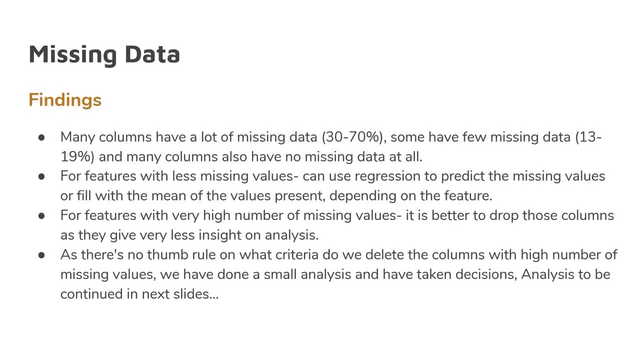 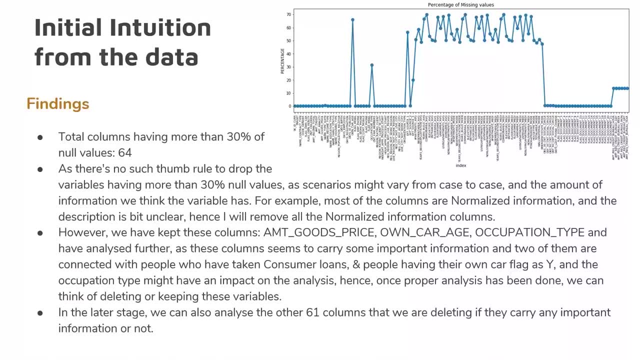 analysis. if you remember, total charges were having 0.15 percentage of missing data and we dropped it. so you have to write down those things here: initial intuition from the data. in our case, again, there were no initial, there were no null values, but we understood that total charges was not in the 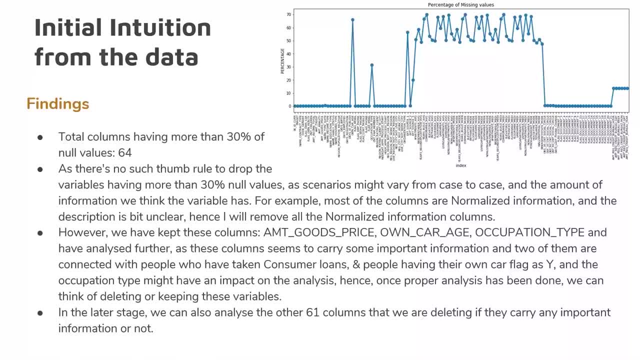 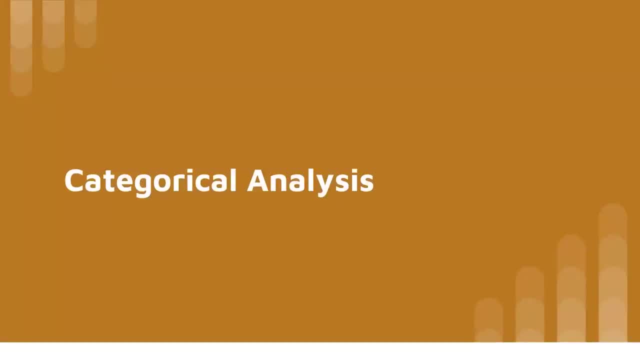 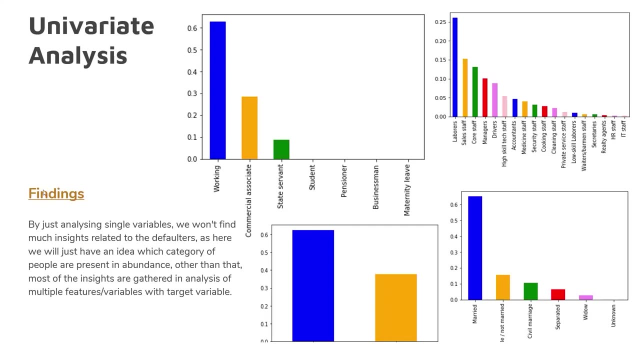 format that we expected. hence we converted into numerical attribute and we got around 0.15 percentage of null values right. so all those things has to be jotted down. then comes your analysis part, the categorical analysis, with all the graphs and the findings in the page. whatever findings you have, 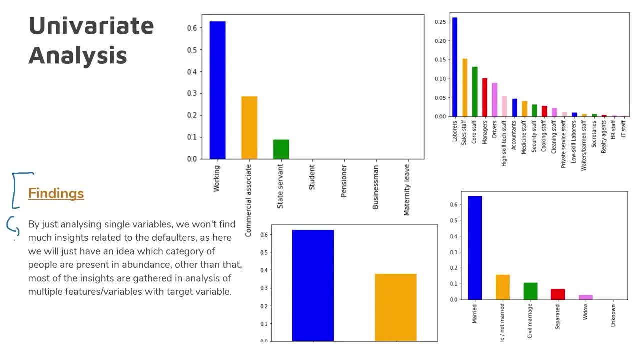 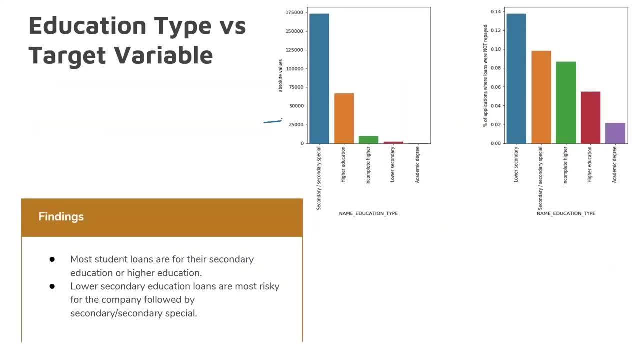 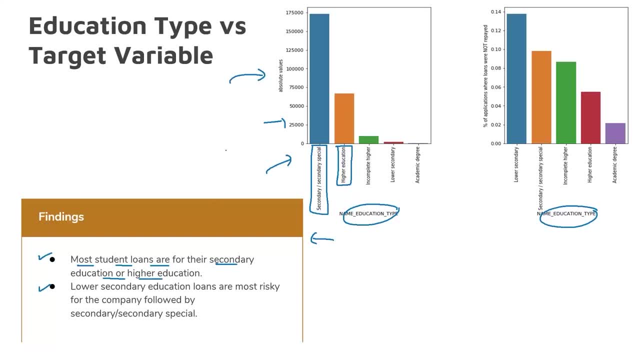 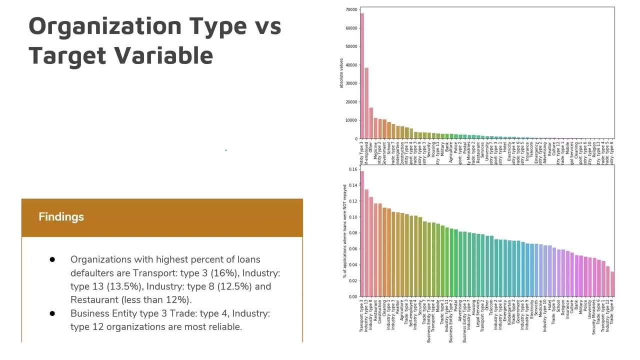 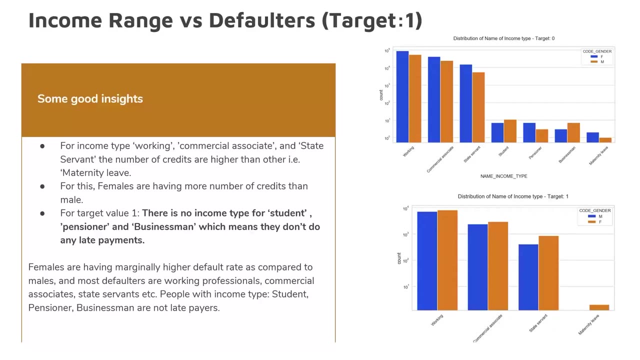 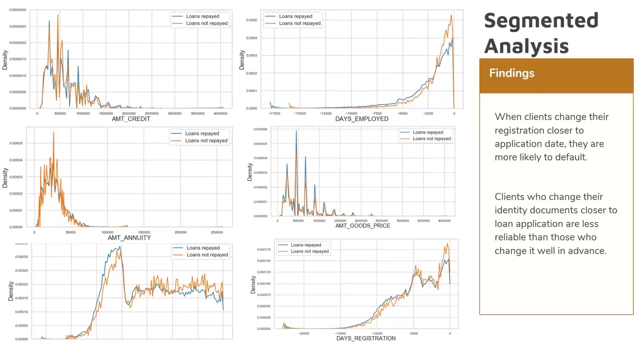 quite evident. so you have to write down your findings and plot your graphs side by side. that gives a good understanding about what's happening, and it goes on. so we have done the same thing here: graphs and insights, graphs and insights. similarly, do it for the numerical analysis: graph findings, graph findings and so on. if you have performed any other activities. 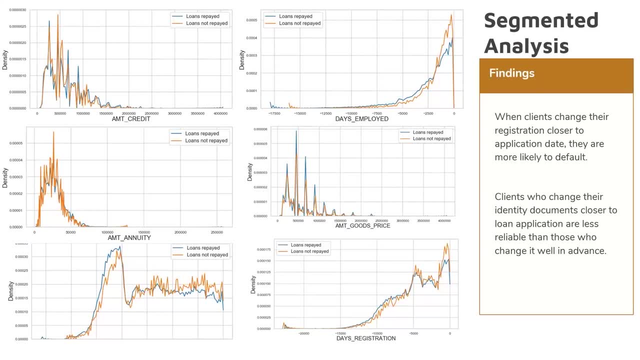 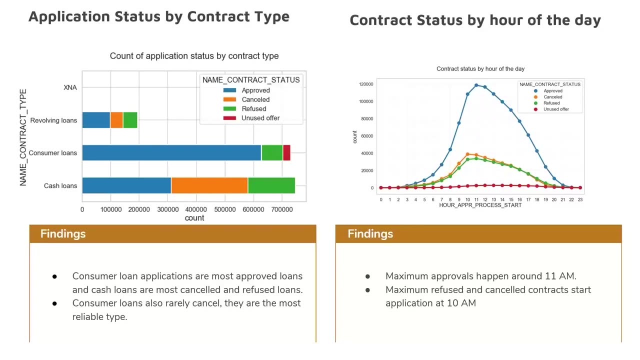 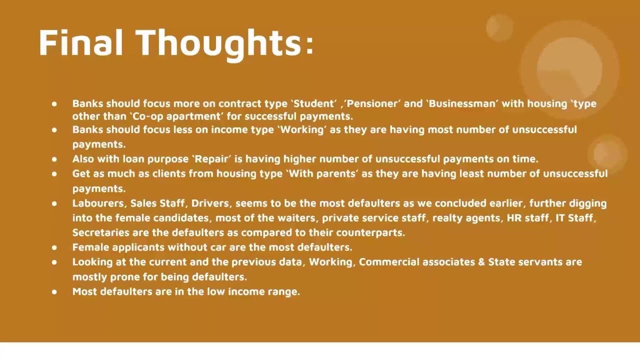 for the numerical analysis, graph findings, graph findings and so on. if you have performed any other activities, like heat maps or correlation maps and all those things, everything has to be a part of this report. and finally, you have to complete or summarize your report, summarize your ada with final thoughts. final thoughts should contain all the insights that you have. 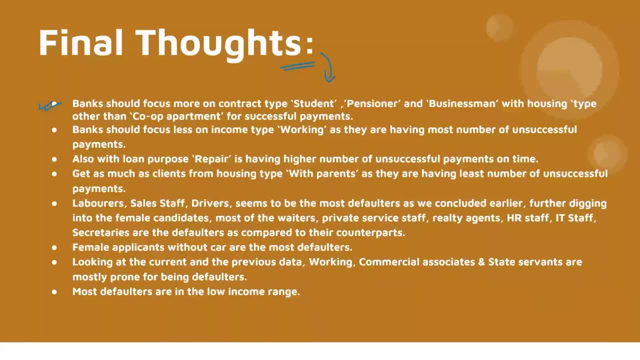 found out now. for example, in your ada case study, one of the insight was: monthly contractors were more likely to churn. female customers with no partners are more likely to churn. people who are paying through payment method, as, uh, which one? there was one of the payment methods: uh, electronic. 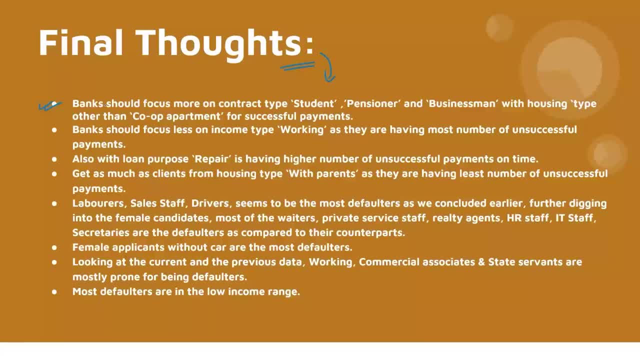 check, they are more likely to churn. female customers who are having credit cards are more likely to chance. so you have to write down all your final thoughts as part of this particular slide, and then you can finish your ppt or your report just by a thank you slide. that's all about. 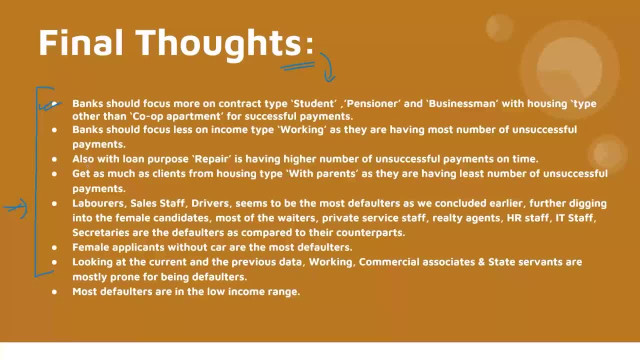 this particular video on how to create reports. i wish you all the luck. please go ahead and prepare an end-to-end report for your churn analysis use case and further. you can take your learnings to the next step by working on multiple eda assignments or working on multiple eda projects. 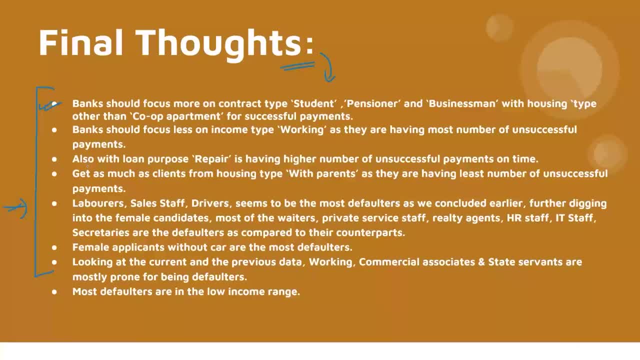 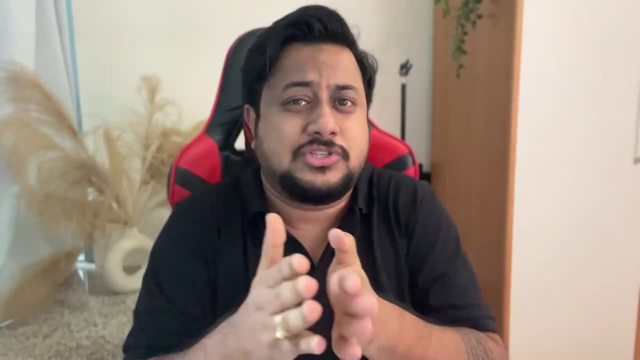 there are multiple eda projects on the web. go ahead, practice, and the more you practice, the easy it will be for you to understand the concept. that's all about this particular video. we are winding up the ada sessions here itself. thank you, that's all about this particular video. it was long, but i'm sure it was informative, in case. 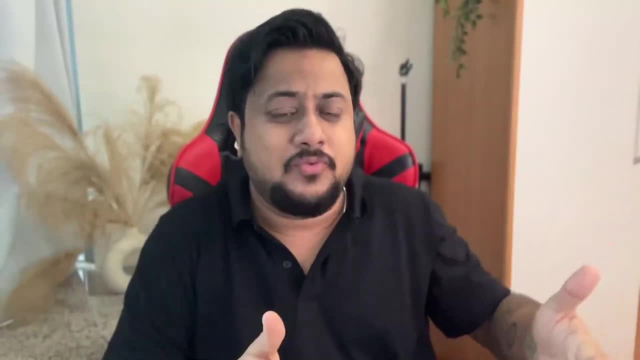 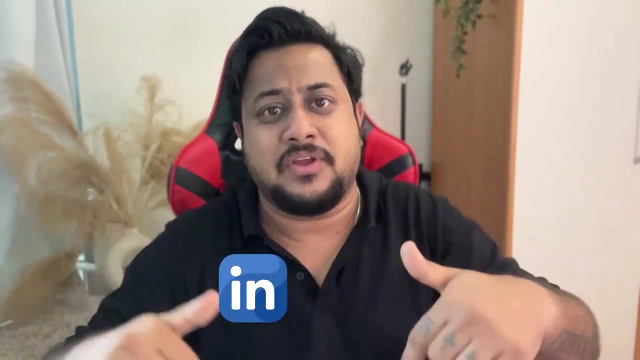 you are confused. what are going to be your next steps? how do we leverage this particular learning and create a portfolio project? reach me out over linkedin or even in the comment section. i go through each and every comments. in case you need any project ideas, i can also. 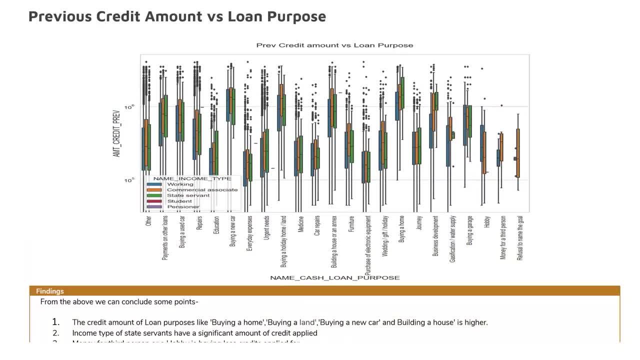 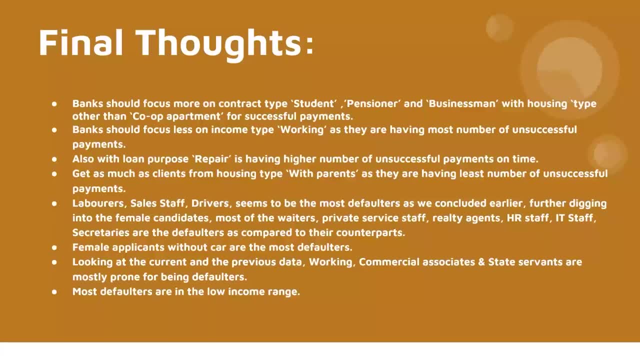 like heat maps or correlation maps and all those things. everything has to be a part of this report. and finally, you have to complete or summarize your report, summarize your ada with final thoughts. final thoughts should contain all the insights that you have found out now, for example in your 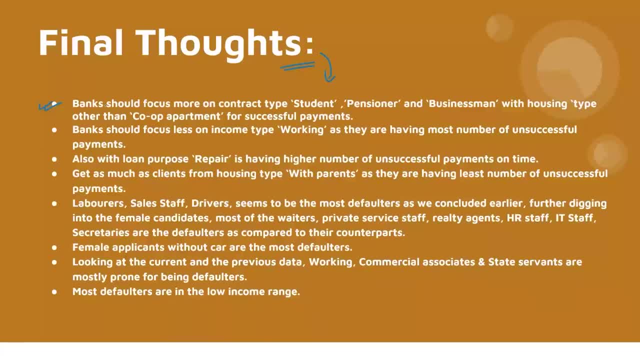 ada case study. one of the insight was monthly contractors were more likely to churn. female customers with no partners are more likely to churn. people who are paying through payment method- as uh which one there was one of the payment methods, uh, electronic check- they are more likely to churn. female customers who are having credit cards are more likely to chance. 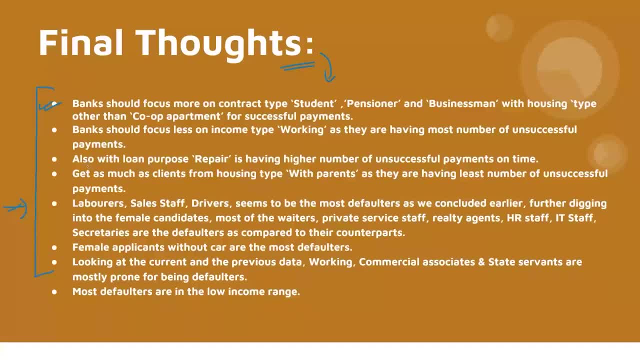 so you have to write down all your final thoughts as part of this particular slide, and then you can finish your ppt or your report just by a thank you slide. that's all about this particular video on how to prepare your end-to-end reports. i wish you all the luck. please go ahead and prepare an end-to-end. 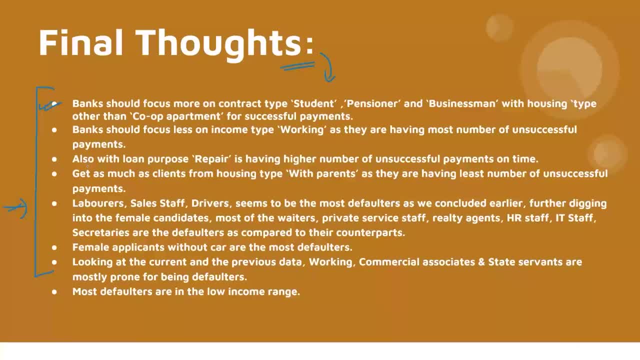 report for your churn analysis use case and further. you can take your learnings to the next step by working on multiple eda assignments or working on multiple eda projects. there are multiple eda projects on the web. go ahead, practice, and the more you practice, the easy it will be for you to. 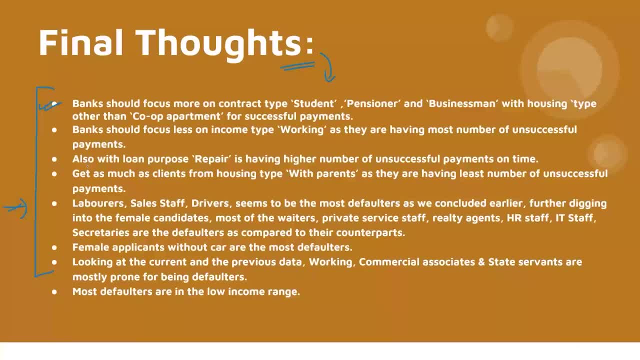 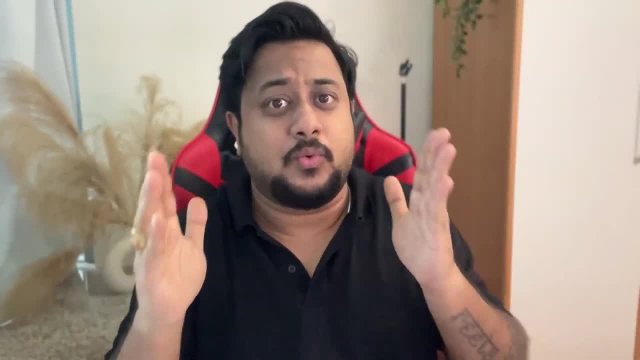 understand the concepts. that's all about this particular video. i hope you have found this video helpful. we are winding up the eda sessions here itself. thank you, that's all about this particular video. it was long, but i'm sure it was informative. in case you are confused, what are going to be your? 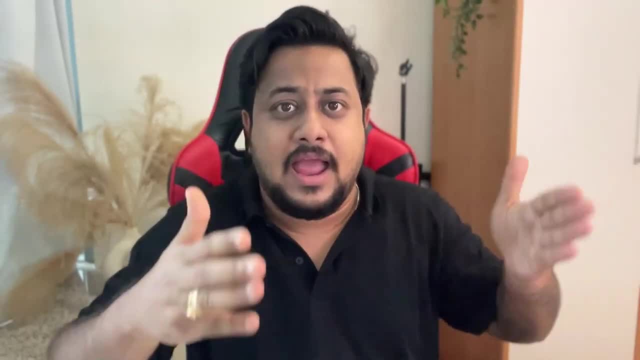 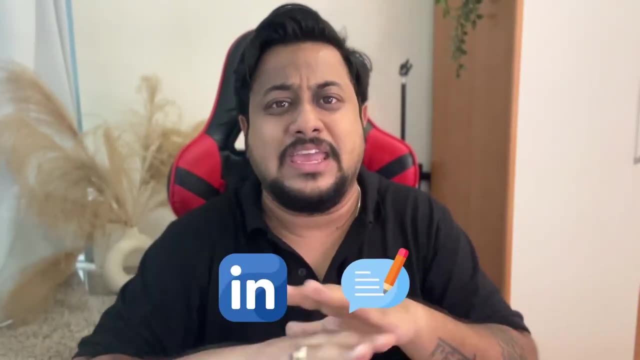 next steps. how do we leverage this particular learning and create a portfolio project? reach me out over linkedin or even in the comment section. i go through each and every comments in case you need any project ideas. i can also help you on that, of course, if you have any questions. 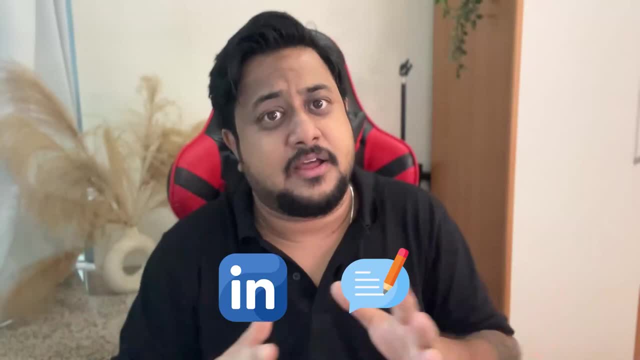 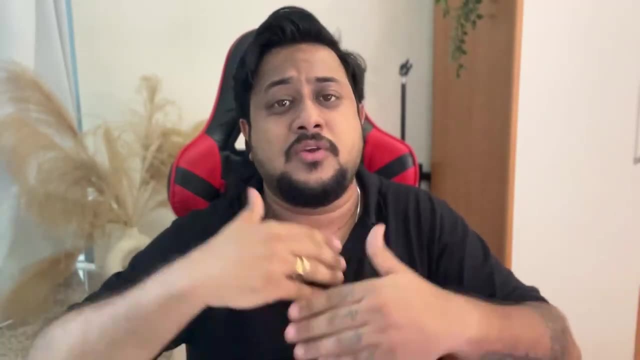 please feel free to ask me in the comment section. i will be happy to answer any questions that you have. in case you need any project ideas, i can also help you and whatever you feel like. if you are going to be a data analyst or a data scientist, or you are.